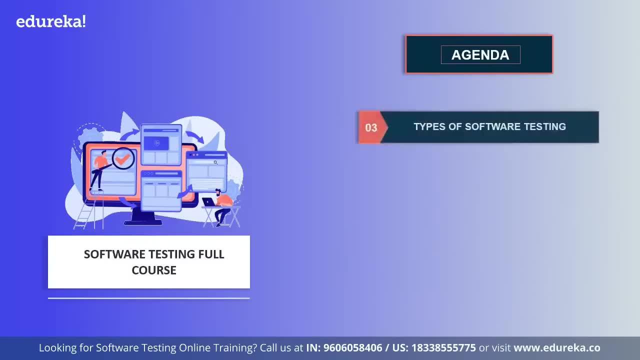 what are they and how to implement them. Moving on, we will understand different types of software testing, where we will discuss what is functional testing, what is non-functional testing and its sub-types. Moving on, we will dig deeper into functional testing and. 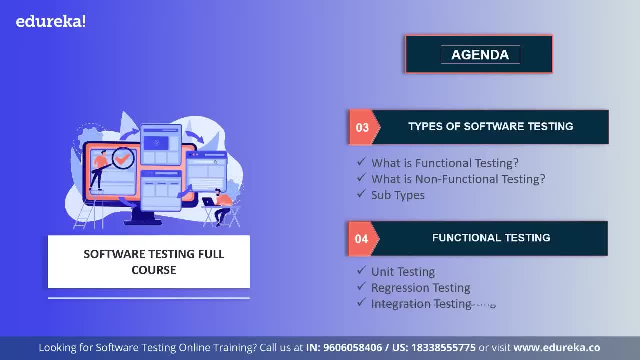 explore unit testing, regression testing, integration testing, sanity and smoke testing, Post that we will move on to non-functional testing and explore performance testing, load testing, stress testing. We will then go on to discuss mobile testing, where we will learn what is mobile testing, how to use Appium for mobile testing, Given that. 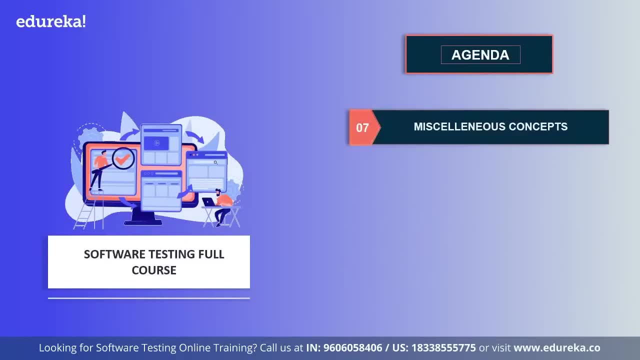 testing is a vast domain. we will also explore some miscellaneous topics like agile testing, python test, automation, cross-browse testing, JMeter and API testing. In the final bit of the session, we will cover the software testing from a carrier perspective, where we will 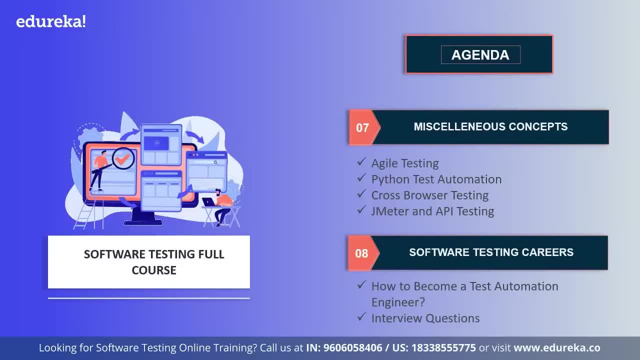 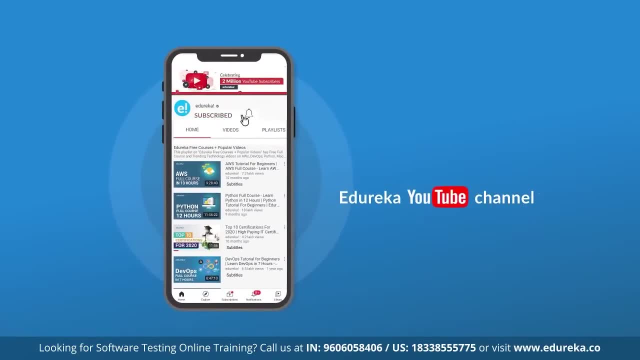 become a test automation engineer and also discuss some important interview questions. With this we come to the end of the agenda for this session. Also, kindly take up some time to go ahead and subscribe to us and do not forget to hit that bell icon to never. 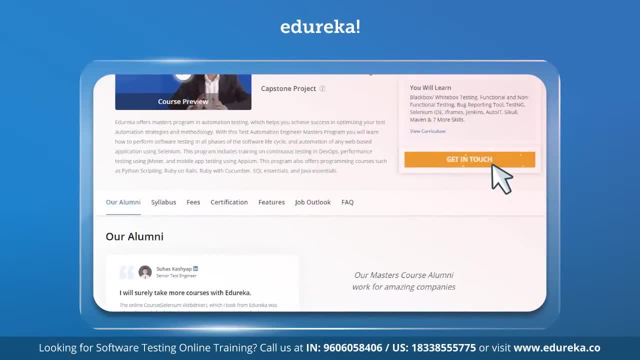 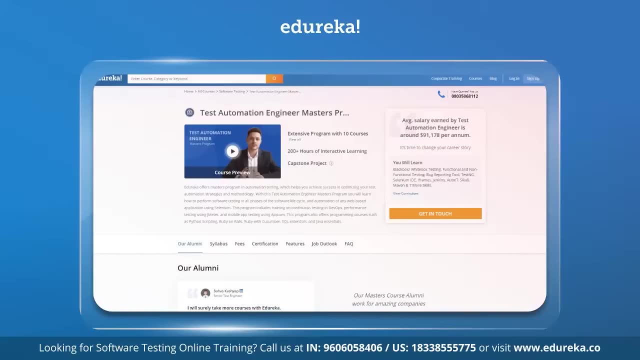 miss an update from the Edureka YouTube channel. Also, to learn more about software testing, do not forget to check out our certification training, the link to which is given in the description box below. So, without much ado, let's get started. 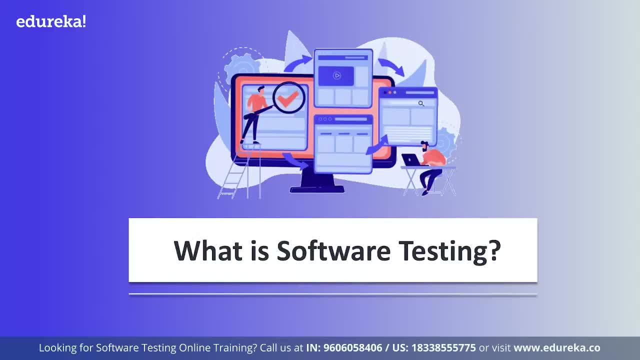 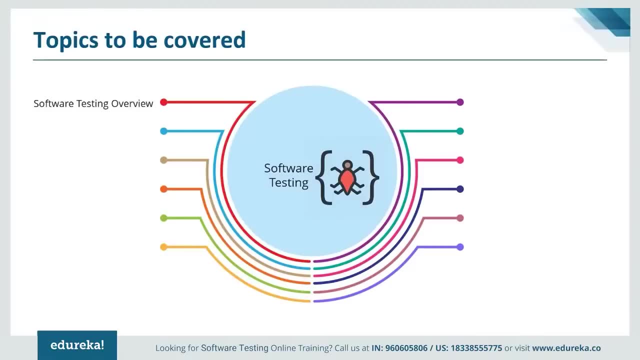 So let me quickly tell you the topics that I will be covering in this session. First, I will tell you what is software testing and what is the need for software testing. Next, I will talk about software development lifecycle and its various models. After that, I will 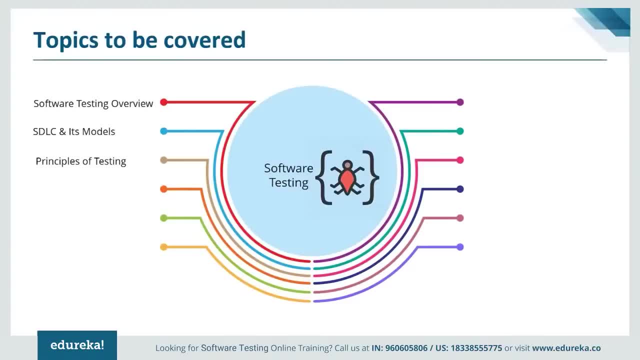 walk you through principles of testing. And once you understand these fundamentals, next let's dive into software testing lifecycle and understand various steps involved in it. And, moving further to the discussion, We'll be seeing methods of testing, its levels and some artifacts of software testing documentation. 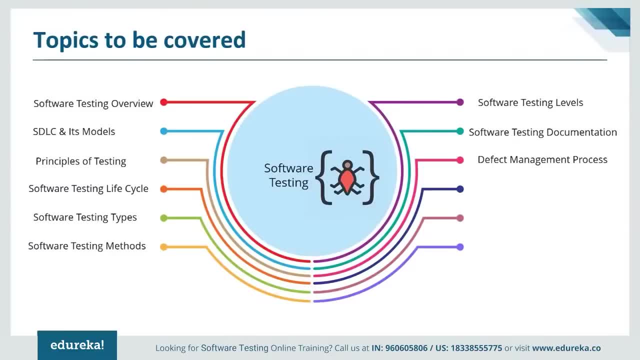 and I will also talk about defect management and bug life cycle. now, moving to automation testing. You will be understanding fundamentals of automation testing and its various tools. You will also be learning by. selenium is most preferable tool for automation testing. And finally, I will wrap up the session by telling you: 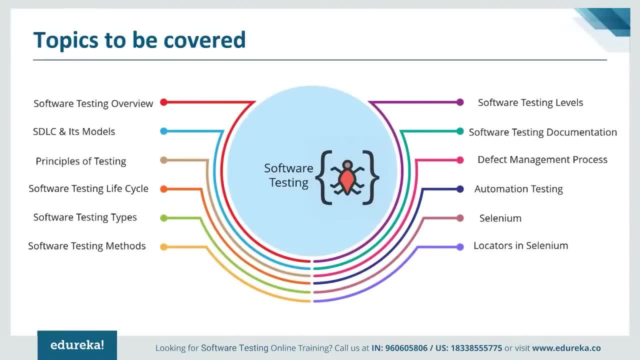 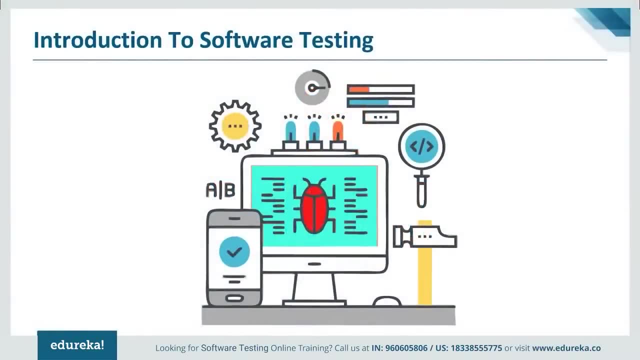 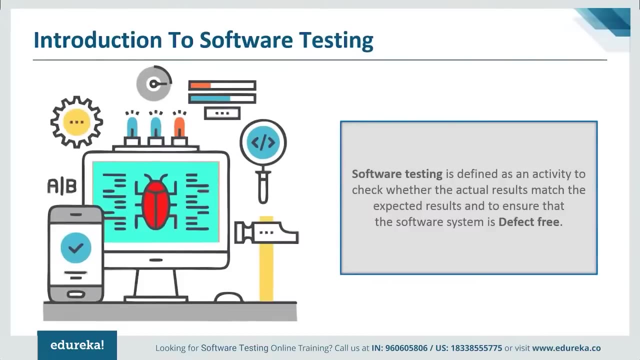 how to locate elements and perform actions on the web page using selenium. without any further, Let's get straight into the module. first, Let's understand what a software testing. software testing can be defined as an activity to check whether the actual results match the expected results. 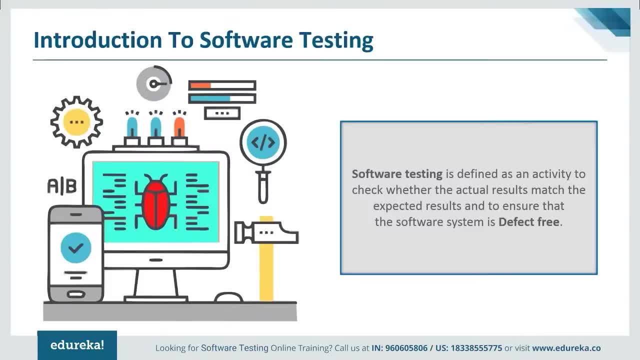 and it also ensures that the product is free from any bug or defect. testing of a software also involves the implementation of products module or system part for evaluating all of some of its properties. through testing, testers can identify errors, gaps in requirement or missing elements in a project. 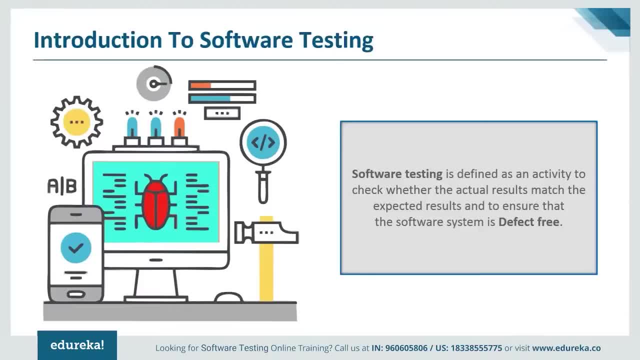 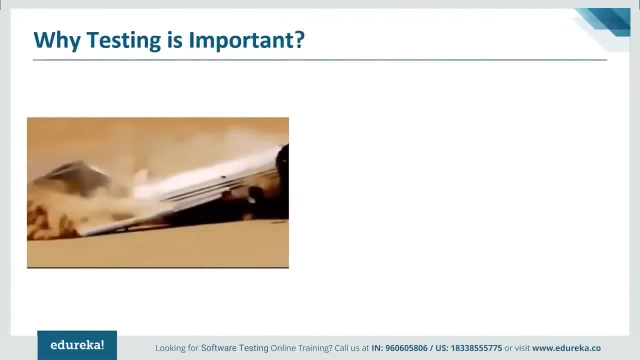 or a system. testing can be done both by manually or with the help of automated tools available in the market. So why testing is important? software testing is where it all boils down to. today's world of Technology is completely dominated by machines and their behavior is controlled by the software powering it. 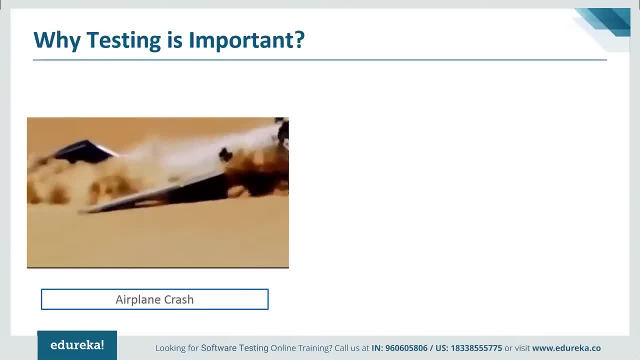 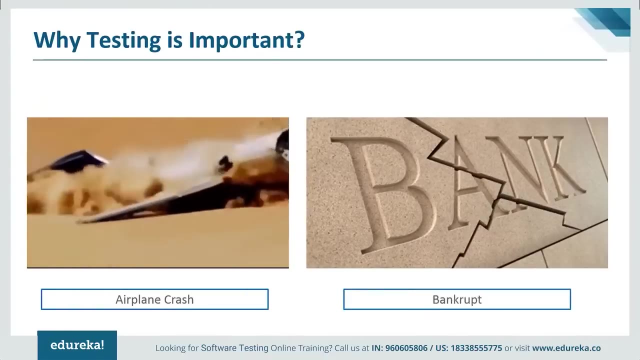 Well, the machines behave exactly as we want them to, every time, everywhere. Yes, the answer. all these questions lie in software testing by the end of the day, at a software application success rate which is going to control your business growth. The same thing can be said even for web applications. 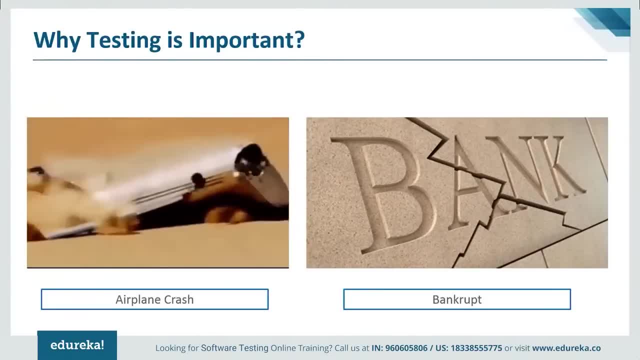 because most businesses today are completely reliant on the internet, For example. you can see here the airplane crash and the bankrupt. why it is happening? just because the system was not tested properly before it was launched, and that's why we say testing. This is important. else. 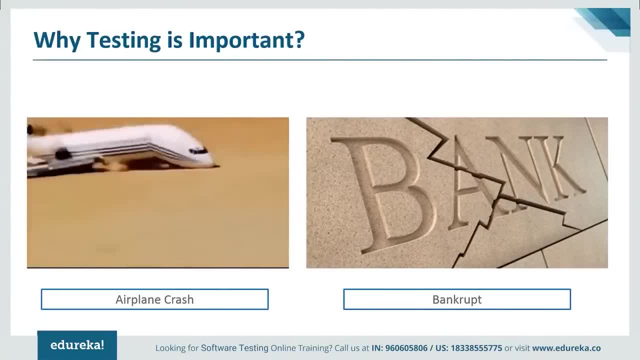 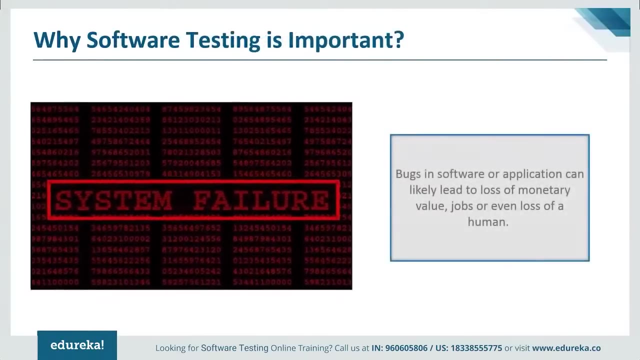 It might lead to a loss of monetary value, jobs or even loss of a human, and these are the examples of untested software that becomes hazardous. So software testing plays a significant role in testing a software or a system. if the bugs or a defect is not properly removed from the system, 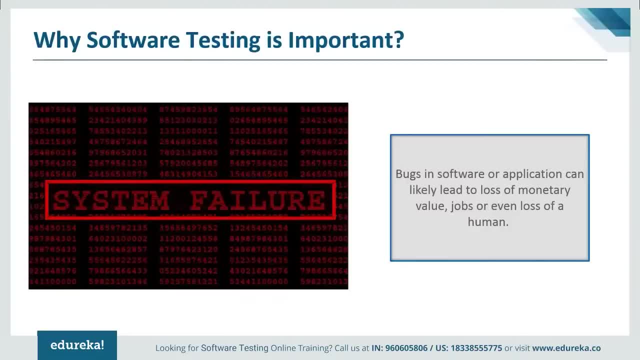 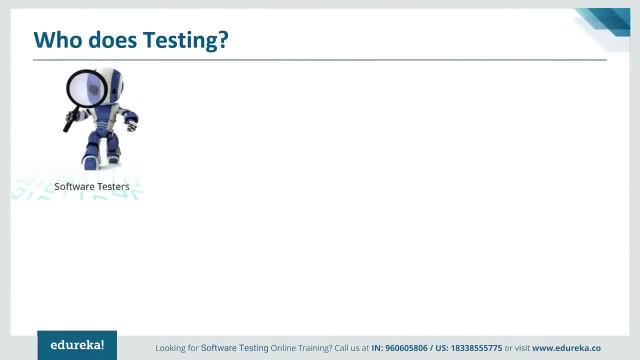 It might lead to system failure, and that's why testing is important. Now let's see who performs software testing. this questions answer is depending on the process and its connected project stakeholders. in the industry of information technology, big companies have team members who bear the responsibility. 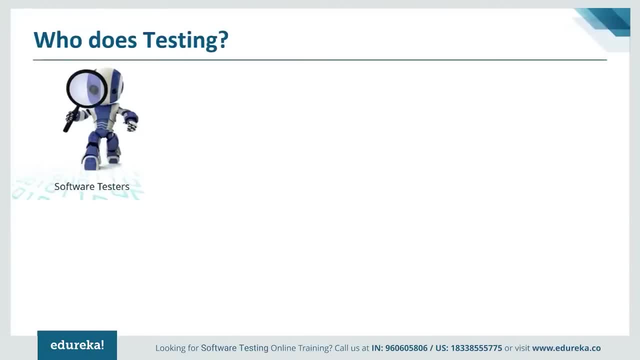 for evaluating the project or software based on the requirements during the test phase. Moreover, some bugs can get detected if proper testing is done in the development of a software or application. So people who can do testing are software testers, project developer, project lead, team manager and end users. 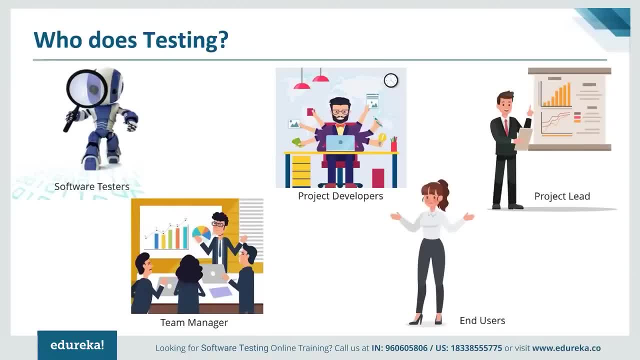 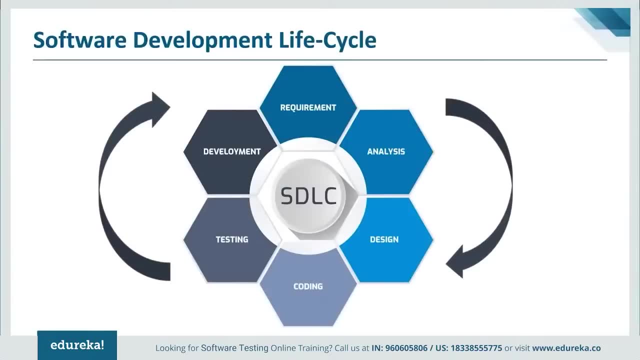 So these are the people who takes care of software testing. having understood this, Let's see. What is software development life cycle? software development life cycle is a process used by the software industry to design, develop and test high quality softwares- STLC that a software development life cycle aims. 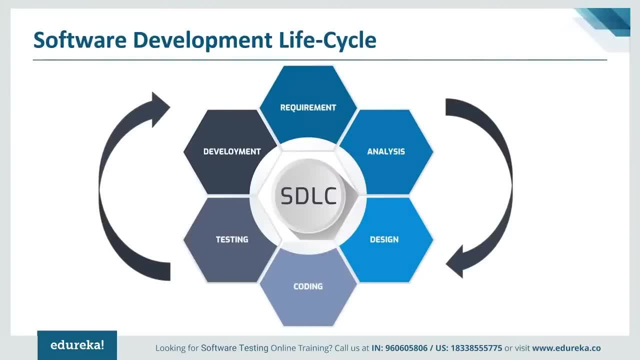 to produce a high quality software that meets or exceeds customer expectations, reaches completion within times and cost estimates. as you can see here, It involves many phases and let me explain you each of these phases. first, requirement phase: requirement gathering and analysis is the most important phase in SDLC. here business analyst collects the requirement. 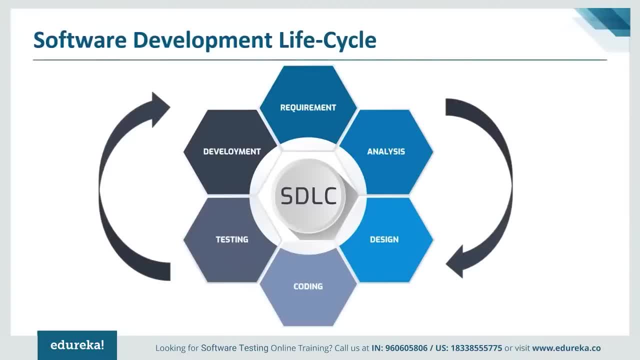 from the customer or client as per the clients business needs and documents the requirements in the business requirement specification. That is the document name and it varies depending upon the organization. Some examples are CRS, that is, customer requirement specification, and some might call it as business specification as well. 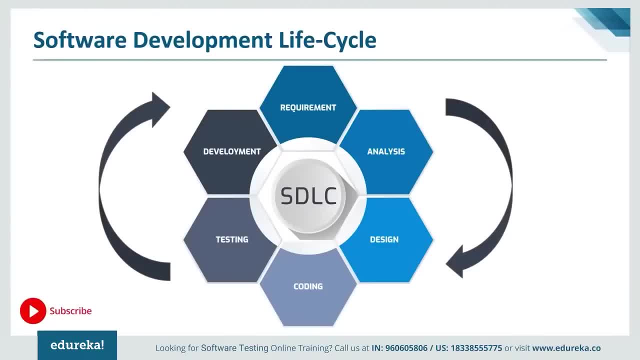 and then they provide the same to the development team. next analysis phase: Once the requirement gathering and analysis is done, The next step is to define and document the product requirements and get them approved by the customer. This is done through SRS, That is, software requirement specification document. 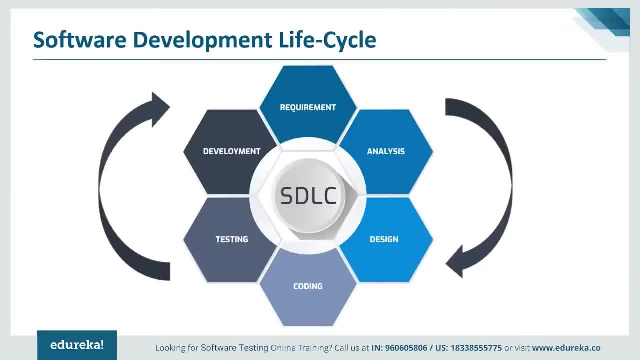 and software requirement specification consists of all the product requirement to be designed and developed during the project life cycle, and key people involved in this phase are project manager, business analyst and senior members of the team, and the outcome of this phase will be software requirement specification. Now moving to design phase. 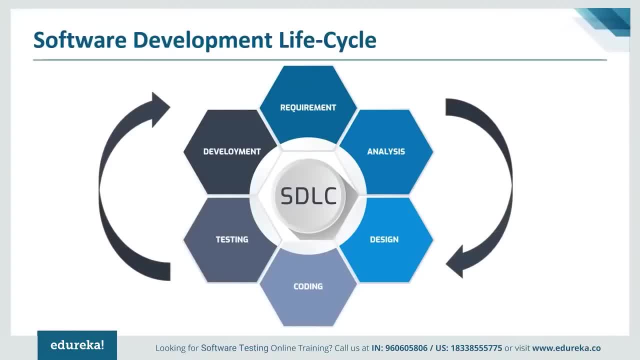 It has two steps: one high-level design and the other one low-level design. So in high-level design it gives the architecture of the software product to be developed and is done by the architects and senior developers. in low-level design It is done by senior developers here describes. 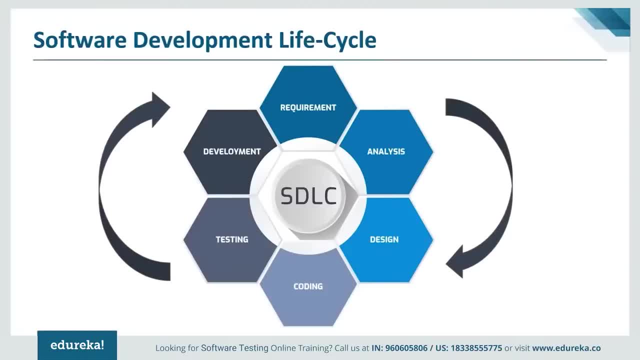 how each and every feature in the product should work and how every component should work. here Only the design will be there and not decode, and the outcome from this phase is the high-level document and low-level document which works as an input to the next phase. 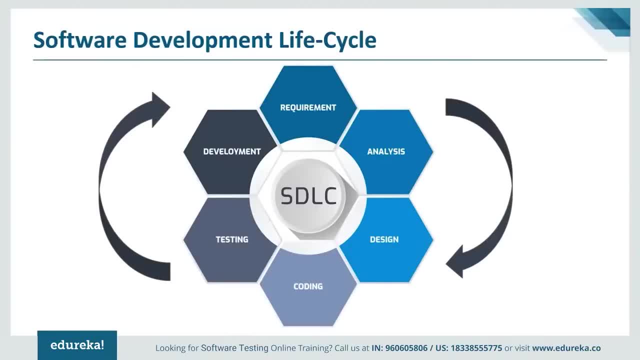 So next is the development or your coding phase. So what happens here? developers of all levels at the seniors, juniors, freshers, all are involved in this phase. This is the phase where we start building the software and start writing the code for the product, the outcome. 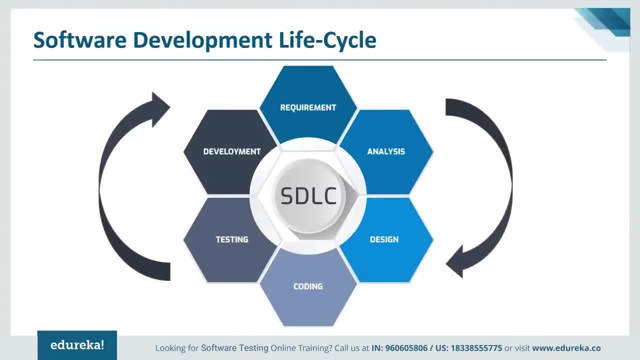 from this phase is the source code document and the developed product. now talking about the testing phase here. when the software is ready, it is sent to the testing document, where test team tests it thoroughly for different defects. They either test the software manually or using the automated tools, depending. 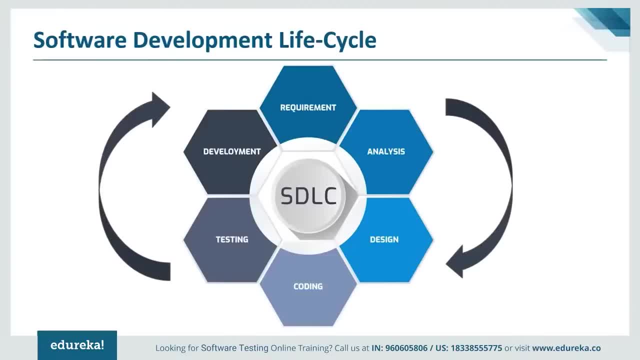 on the process defined in software testing life cycle and also ensures that each and every component of the software works fine. Once the QA, that is, the quality analyst, make sure that the software is error-free, it goes to the next stage, which is implementation and the outcome of this phase. 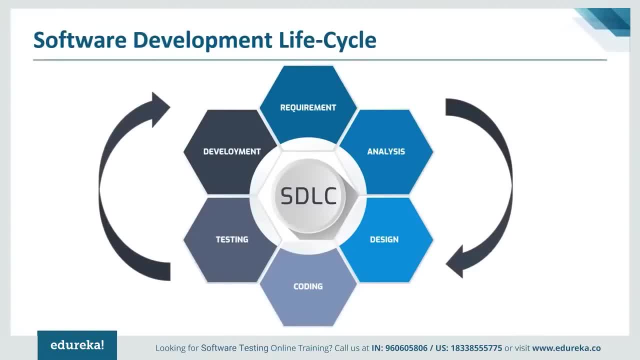 is the quality product and the testing artifacts. I'll talk about the testing artifacts at the later part. So, once all this is done, the next and the last step is deployment and maintenance phase. after successful testing, the product is delivered and deployed to the customer for the use. deployment is done. 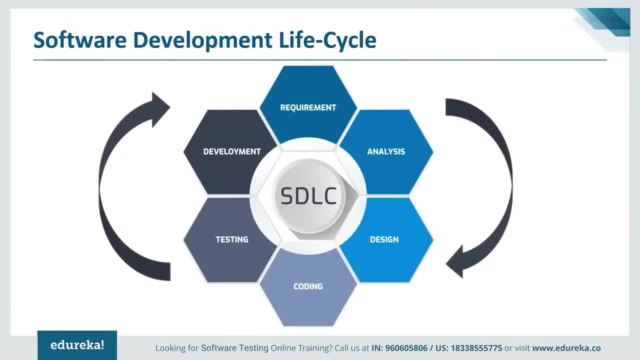 by the deployment engineers or the implementation engineers. Once, when the customers start using the developed system, then the actual problems will come up and needs to be solved from time to time. fixing the issues found by the customer comes in maintenance phase. Hundred-person testing is not possible. 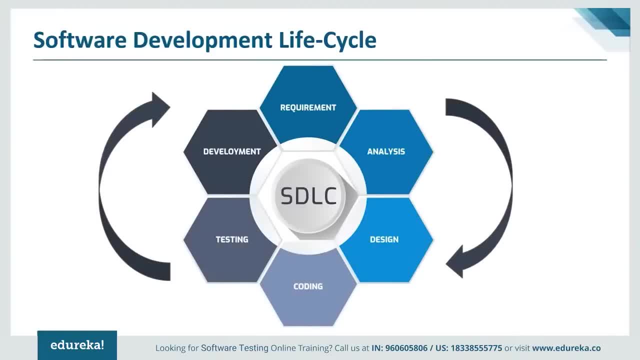 because the way testers test the product is different from the way customer user product maintenance should be done as per SLA, that is, service level agreement. These are the various phases involved in software development life cycle And this is how it works. Now we have different models. 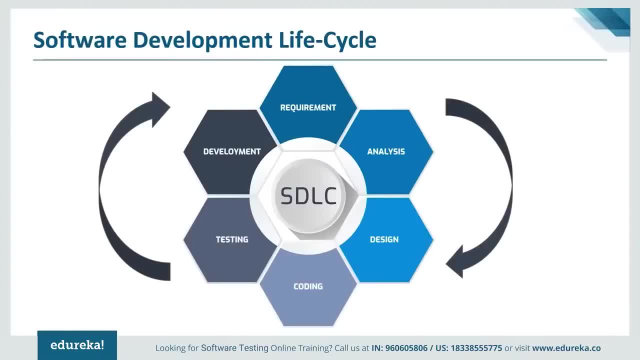 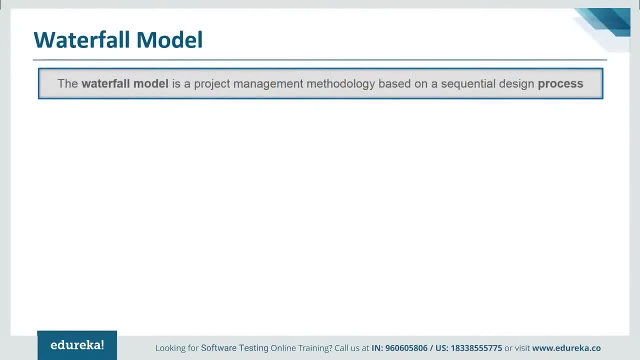 of software development life cycle, like waterfall model, spiral model, agile model, Etc. Now let's talk about waterfall model and understand how it works. Waterfall model is a traditional model. It is a sequential design process that is often used in SDLC, in which the progress is seen as flowing downwards. 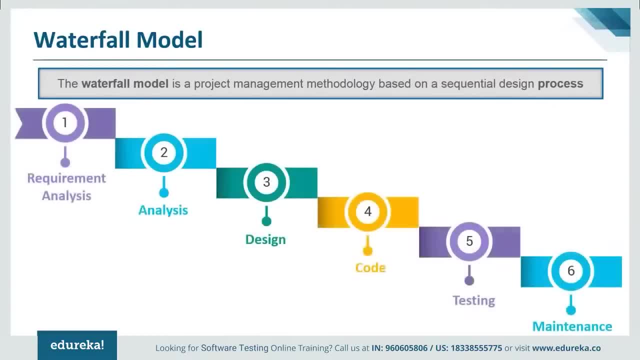 like a waterfall through the different phases, such as requirement gathering, feasibility study, analysis, design, coding, testing, installation and maintenance. Every next phase is big and only once the goal of the previous phase is completed. This methodology is preferred in projects where quality is more important as compared to schedule or cost. 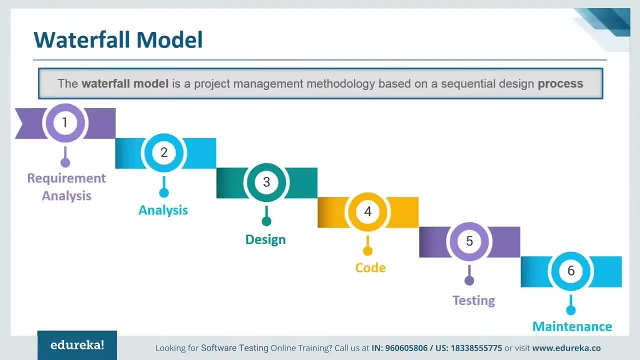 The methodology is best suitable for short-term projects where the requirements will not change, for example, your attendance management or calculator Etc. So benefits of using this model are: requirements do not change, nor does the design and code, so we get a stable product and this model is very simple to implement. requirements. 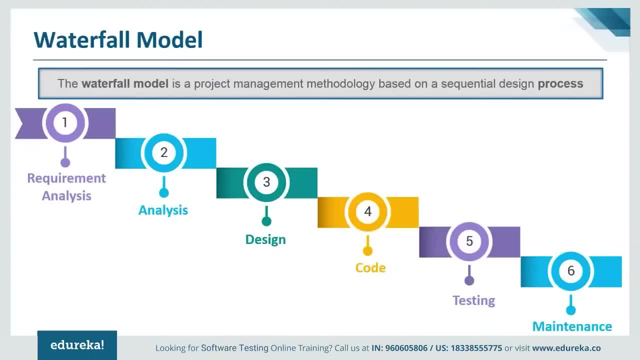 are finalized earlier in the life cycle, So there won't be any chaos in the next phases. and requirement resources to implement this model and minimal compared to other methodologies and every phase has specific deliverables. It gives high visibility to the project manager and clients about the progress of the project. 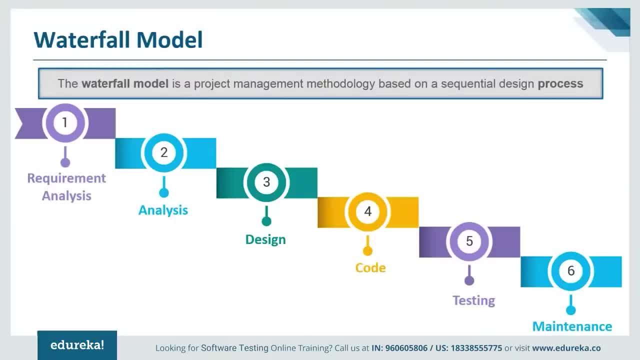 So what are its disadvantages? The main disadvantage is that backtracking is not possible, That is, we cannot go back and change the requirements once the design stage is reached and change in requirements leads to change in design and code, which results defect in the project due to overlapping of phases. 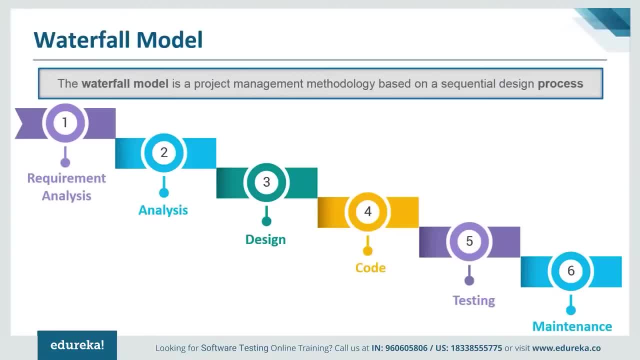 and by this, customer may not be satisfied if the changes that they need are not incorporated in the product, and the end of the waterfall model may not be a flexible product and this model can be used only when the requirements are very well known and fixed, and it is also not suitable for long-term projects. 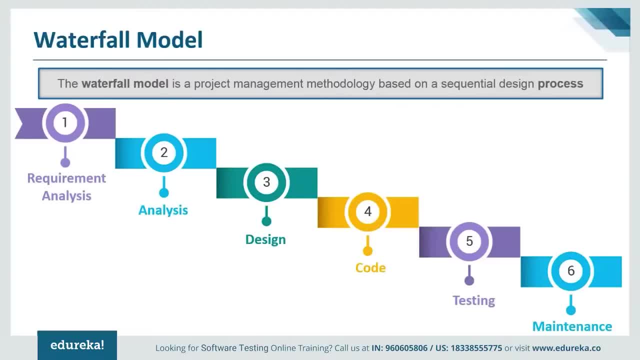 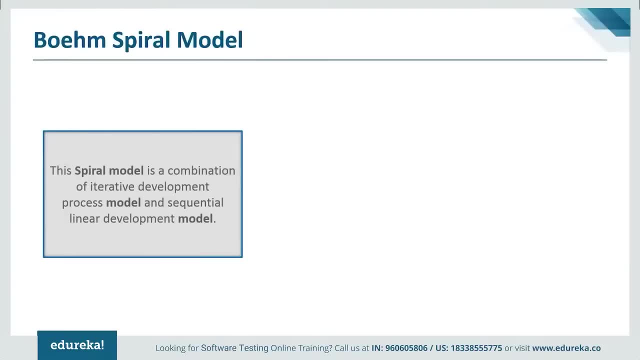 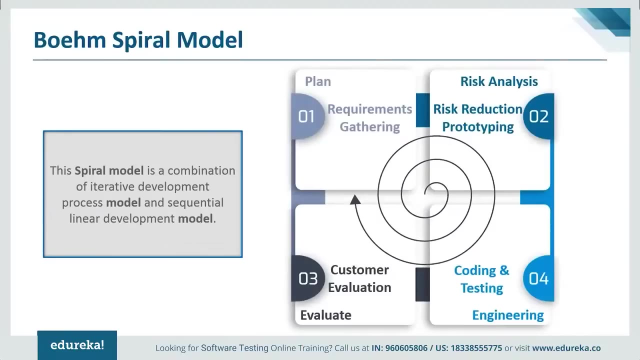 where requirements may change time to time. So this is about waterfall model. Next, Let's take a look at bohem spiral model. spiral model works in an iterative nature. It is a combination of both prototype development process and linear development process. that is your waterfall model. 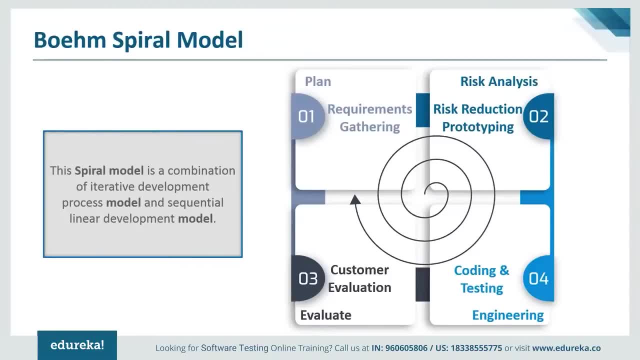 and this model place more emphasis on risk analysis. Mostly, this model adopts to large and complicated projects where risk is very high. Every iteration starts with the planning and ends with the product evaluation by client. So let's take an example of the product development team. like Microsoft, 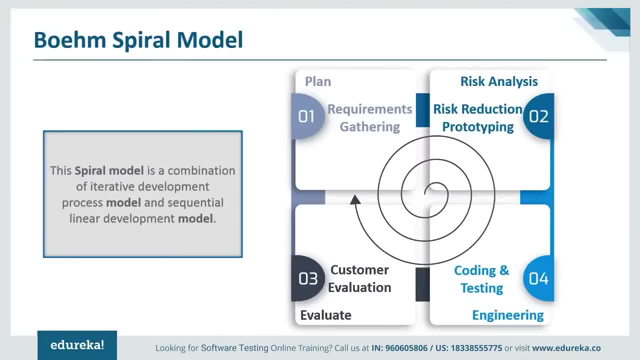 They know that there will be a high risk and they face lots of difficulties in the journey of developing and releasing the project. and also they know that they will release next version of product when the current version is in existence and they prefer spiral model to develop the product. 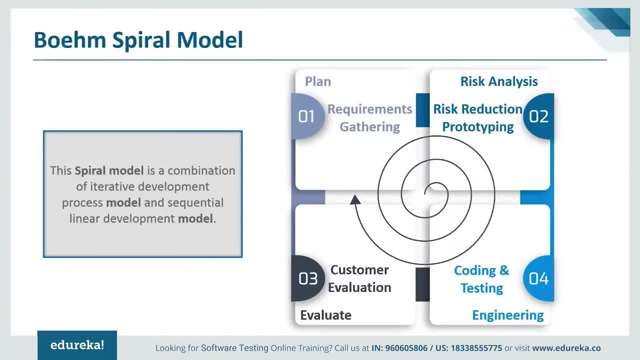 in an iterative nature, So they could release one version of the product to the end user and start developing next version, which includes new enhancements and improvements on the previous version and that is based on the issues faced by the user and the previous version, like Microsoft, release Windows 8. 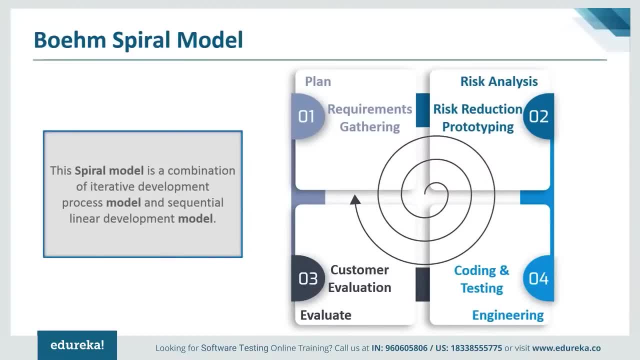 and improved it based on user feedback and release the next version that is 8.1 and it went on. so it mainly undergoes four phases at this planning phase and in this phase, requirement gathering, cost estimation and resource allocation is being done and next phase is risk analysis phase. here strengths 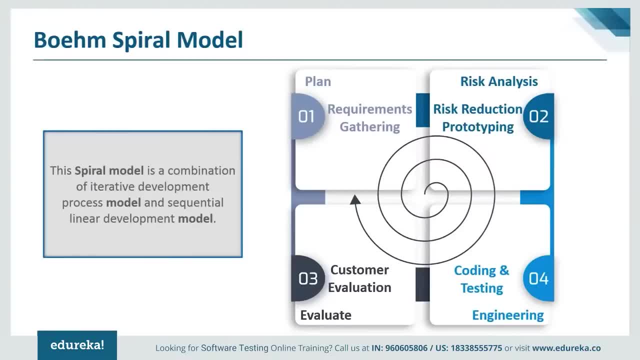 and weaknesses of the project is being known and next comes your design on engineering phase, where coding, internal testing and deployment is being done. and the last is the evaluation phase, like client evaluation, client-side testing to get the feedback, Etc. So benefits of using this model are it allows requirement changes. 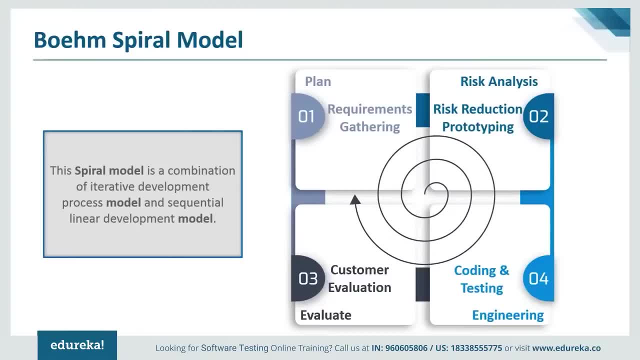 and it is also suitable for large and complicated projects. The main thing is it allows better risk analysis and is cost effective due to good risk management, and disadvantages is that it is not suitable for small projects and the success of a project depends on the risk analysis phase. 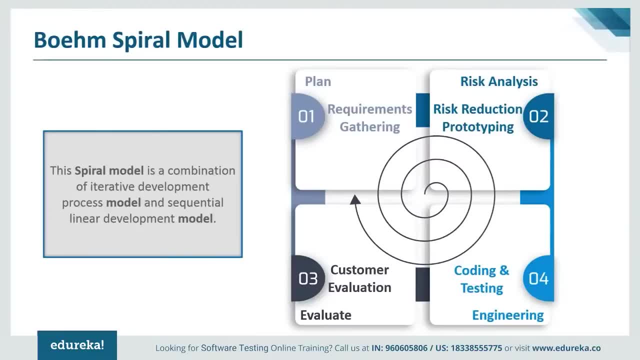 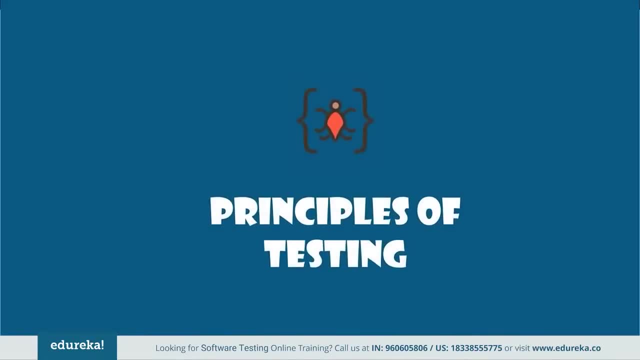 That's all. so this is all about the spiral model and different types of models in SDLC. Now let's move further and understand principles of testing. testing of software. Software is exceptionally imaginative and an intellectual task for testers to perform. testing of software or applications pursue some principles. 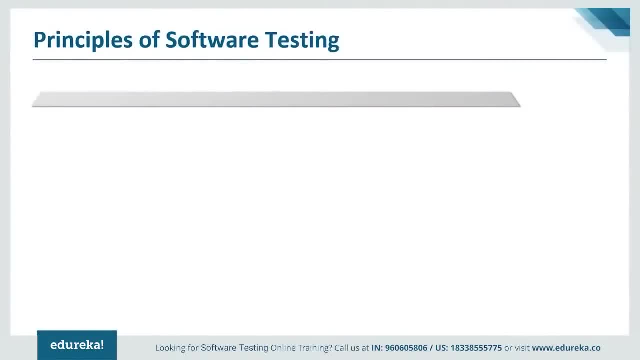 that are mentioned over here. These principles also play a significant role for software tester to test the project, and they are: first one, software testing can help in detecting bugs. testing any software or project can help in revealing few or some defects that may or may not be detected by developers. 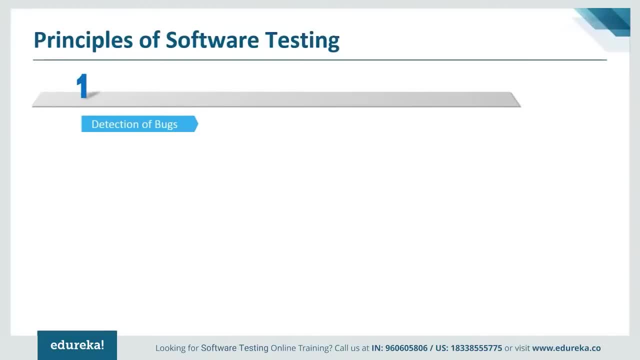 However, testing of software alone cannot confirm that your developed product or software is error-free. Hence it's essential to device test cases and find out as many defects as possible. next, testing with effectiveness is impossible. So what is this? until your project or application. 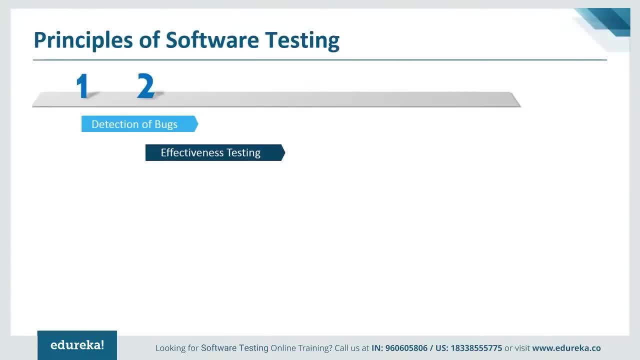 under test has a straightforward structure. having limited input, It won't be likely or achievable to check and test all the feasible sets of data, modules and scenarios. and next, early testing. the earlier you will begin to test your project or software, the better you will find to utilize your existing time. next, defect in clustering: 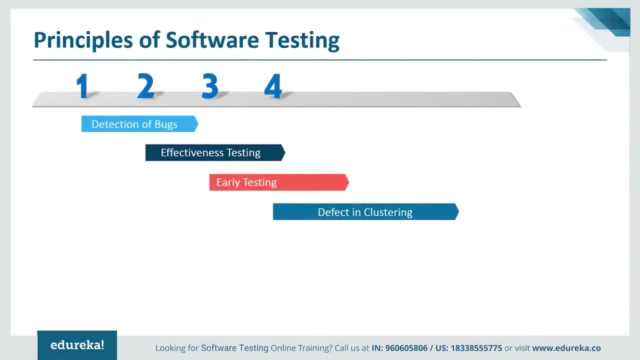 at the time of testing, you can observe that majority of the defects or bugs that are reported are because of a small number of modules inside your software or system. next, software testing is context-dependent, and error-free or bug-free software is a myth, just because when a tester tested an application, 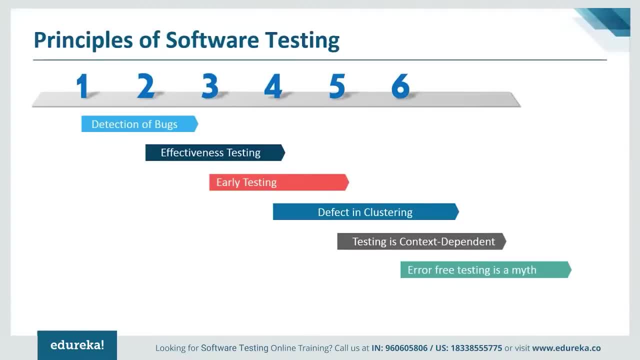 and did not detect any defects in the project doesn't indicate or imply that your software is ready for shipping. So at the time of testing modules or working of software, you as a tester needs to test whether your software is meeting all the requirements of the client or not. 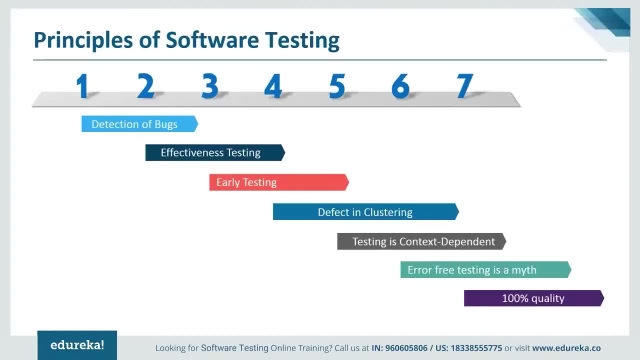 and whether the bugs found during testing has been mended or not. these many factors need to be considered before shipping the software or releasing it to the market. So these are some of the principles of software testing that one should keep in mind while testing a software. 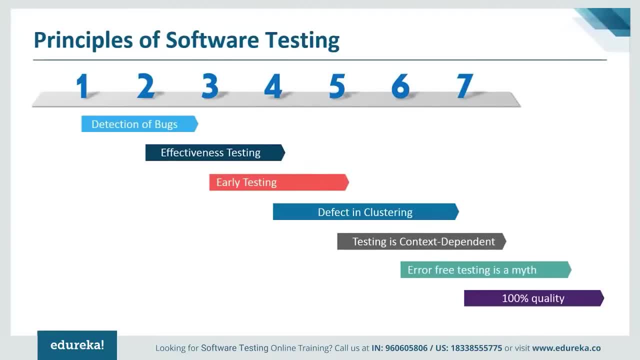 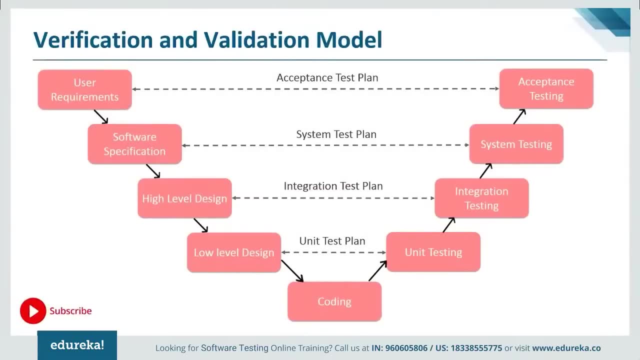 Now let's move further and understand one of the most widely used model, that is, verification and validation model. to understand this model, Let's first understand what is verification and validation and software. first verification: verification as a static analysis technique. in this technique, Testing is done without executing the code. 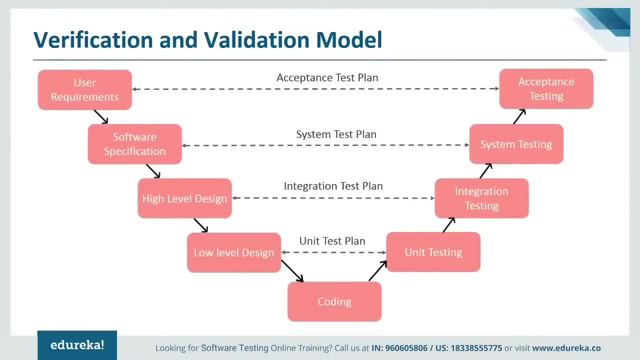 For example, you can say inspection, walkthrough, reviews, Etc. Next, validation. validation is the dynamic analysis technique where testing is done by executing the code, For example, your functional and non-functional testing techniques. in verification and validation model, the development and QA activities are done simultaneously. 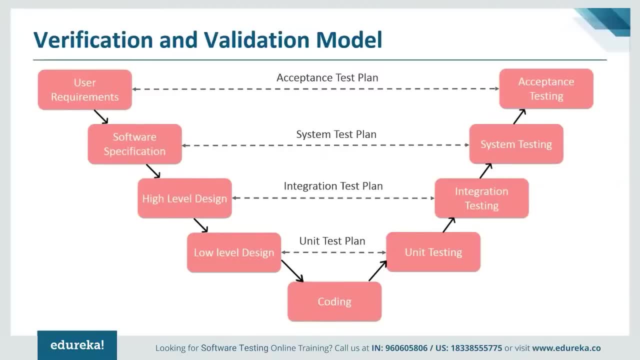 There is no discrete phase called testing. rather, testing starts right from the requirement phase. the verification and validation activities go hand-in-hand. So just have a look at the figure over here and you can see here in a typical development process. The left hand side shows the development activities. 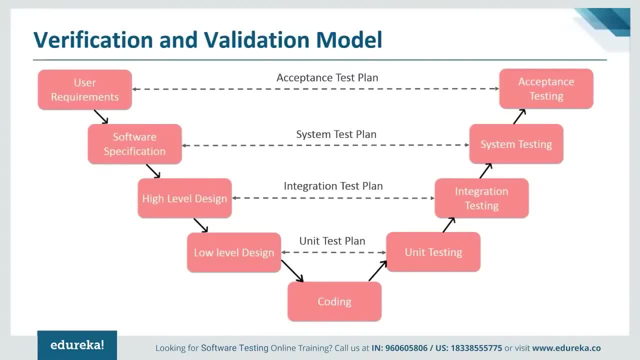 and the right hand side shows the testing activities- I should not be wrong If I say that- and the development phase. both verification and validation are performed, along with the actual development activities. Now let's understand Each of these phases in depth. So first, talking about the left hand side, 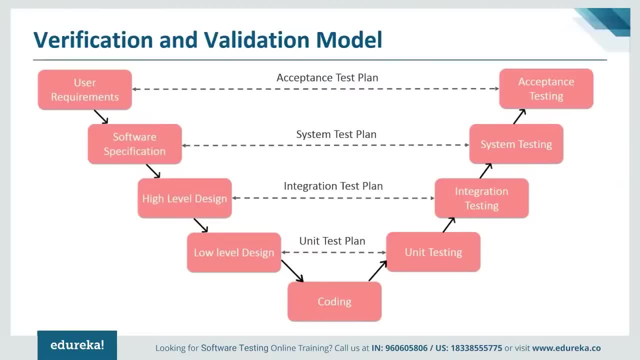 as you all know, left hand side activities are the development activities. Normally we feel: what testing can we do in the development phase? but this is the beauty of the model, which demonstrates that testing can be done in all phases of development activities as well. So here, requirements are collected, analyzed and studied. here, 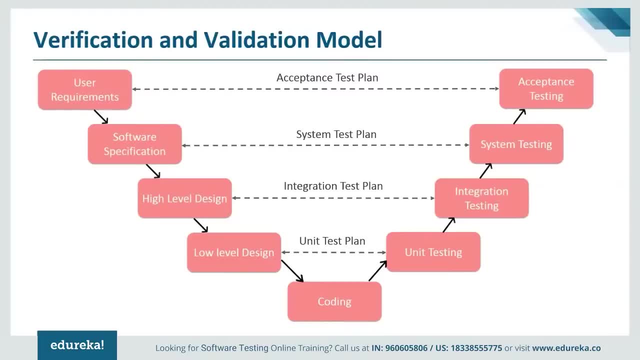 How the system is implemented is not important, But what the system is supposed to do is important, like brainstorming sessions, walkthroughs, interviews are all done here to have the objective set clear. So verification activities like requirements, reviews and validation activities like creation of user acceptance test and its test cases. 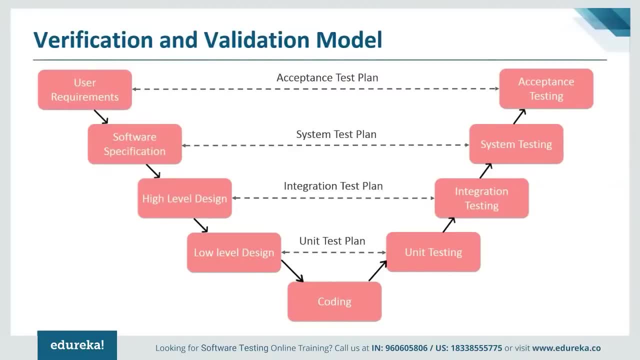 and the artifacts produced here will be requirement understanding document and user acceptance test test cases, that is, UAT test cases. So this is about the requirement analysis phase. now talking about software specification: in this phase a high-level design of the software is built. the team studies. 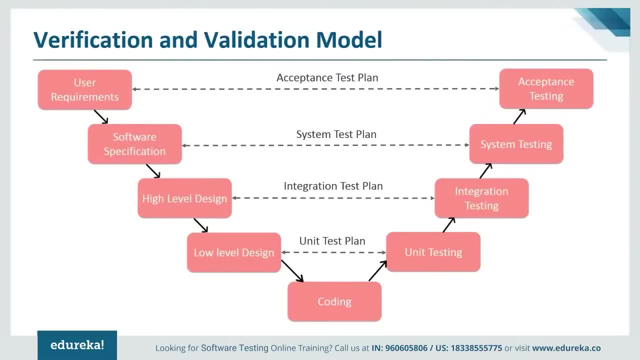 and investigates on how the requirements could be implemented, and the technical feasibility of the requirements is also studied, and here the team also comes up with the modules that would be created based on the software and hardware needs. so verification activities that include here are design reviews and validation activities like creation of system test plan. 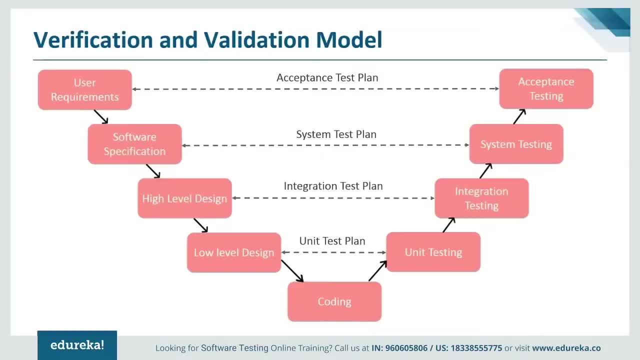 and cases and creation of traceability metrics and the artifacts produced. here are system test cases, feasibility reports, system test plan, hardware, software requirements and modules to be created. So the next phase is the architectural design or your high-level design. in this phase, based on the high-level design, software architecture is created, the modules: 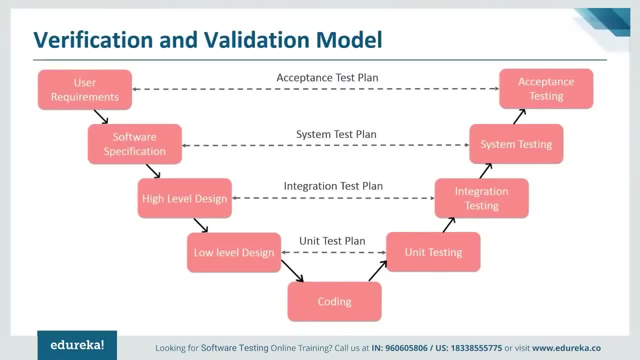 their relationship and dependencies. architectural, Architectural diagrams, database tables, technology details are all finalized in this phase. So again, verification activities like design reviews are included and validation activities like integration test plan and test cases and the artifacts produce our design documents, integration test plan and test cases and database table designs, Etc. 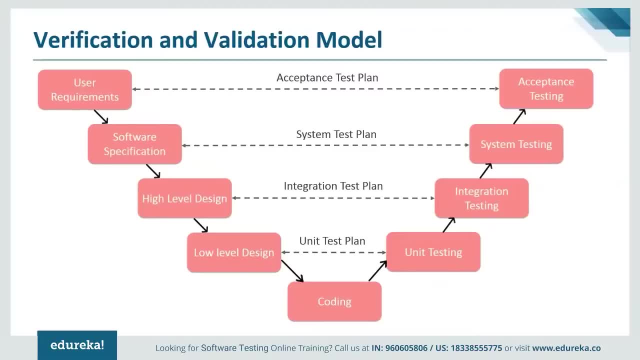 Now coming to module design, also called as low-level design. in this phase, each and every model of the software component are designed Individually. methods, classes, interfaces, data types, Etc. are all finalized in this phase. So again, verification activities, like design reviews, is included. 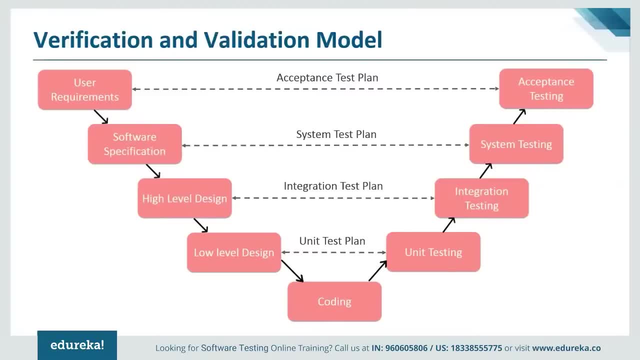 and validation activities like creation and review of unit test cases, and the artifacts that are produced will be unit test cases. So next we have the implementation or code. in this phase actual coding is done. So code review and test cases review are various Modification activities. 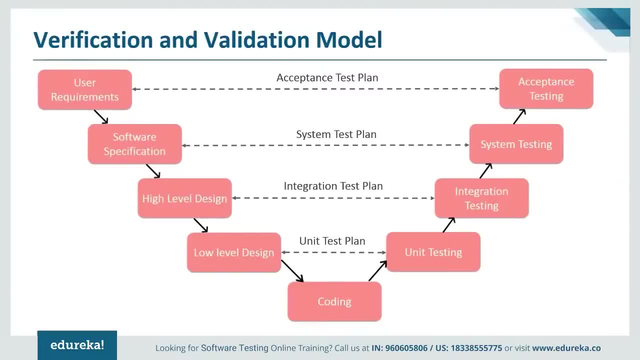 and creation of functional test cases are validation activities, and artifacts produced will be test cases and review checklist. So this is all about left-hand side. that is your development phase. now talking about the right-hand side, this side demonstrate the testing activities or validation space. So we will start from bottom. that is your unit testing. 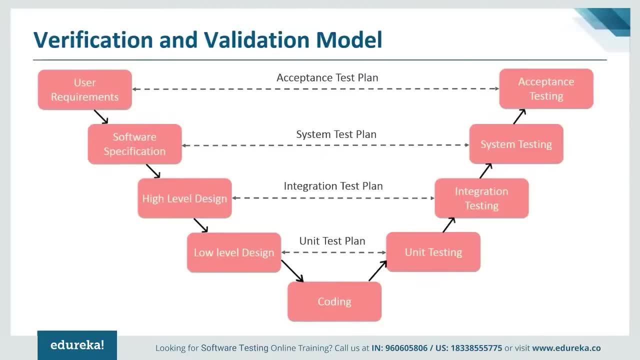 in this phase, all the unit test cases created in the low-level design are executed. So what is unit testing? unit testing is a white box testing technique where a piece of code is written which invokes a method to test whether the code snippet is giving the expected output. 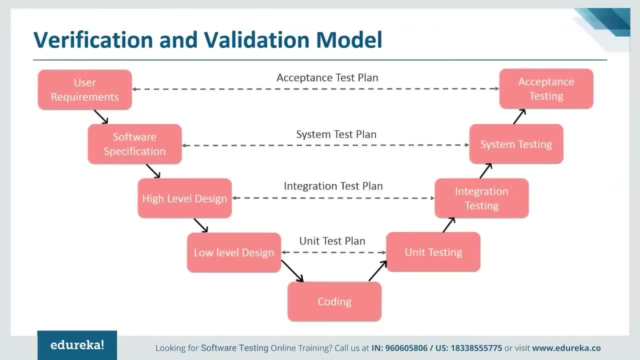 or not. this testing is basically performed by the development team. in case of any anomaly, defects are logged and tracked. So artifacts produced. here are unit test execution results. Next comes integration testing. in this phase The integration Test cases are executed which, where created in the architectural design. 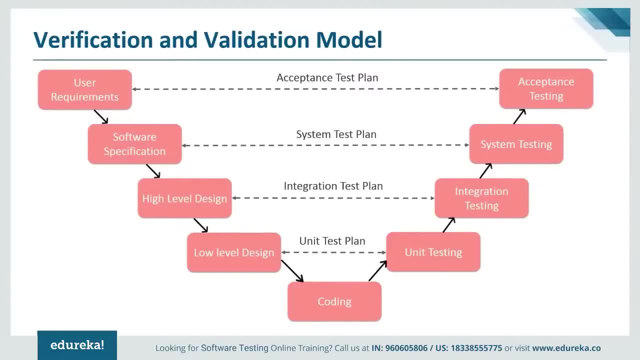 or your high-level design phase. in case of any anomalies, The effects are logged and tracked even here. So now talking about integration testing. in this phase, the integration test cases are executed which were created in the architectural design or your high level design phase, in case of any anomalies. 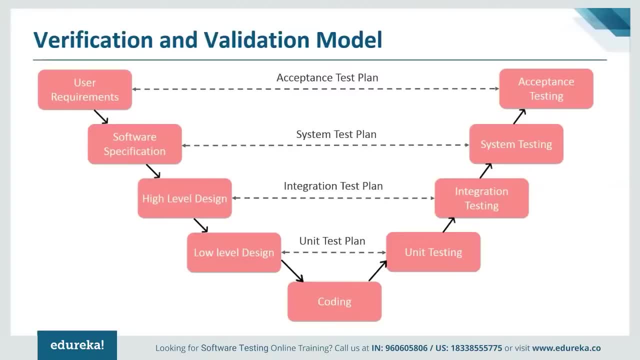 Defects are logged and tracked. So in integration testing it validates whether the components of the application works together as expected, and the artifacts produced here are integration test results. and now coming to system testing. in this phase all the system test cases, functional test cases and non-functional test cases are executed. 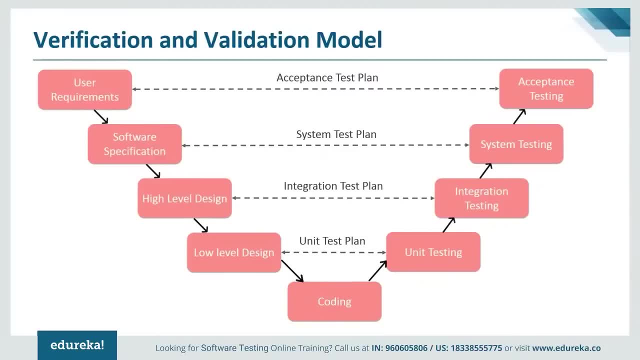 In other words, the actual and full-fledged testing of the application takes place here, So defects are logged and tracked for its closure. Progress reporting is also a major part in this phase. The traceability metrics are updated to check the coverage and risk mitigated. 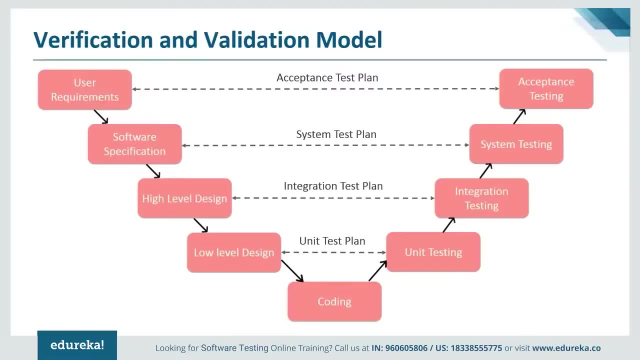 and the artifacts produced are test results, test logs, defect report, test summary report and updated traceability matrices. and now talking about the last phase, that is, user acceptance testing. So acceptance testing is basically related to business requirements testing. here testing is done to validate that the business requirements are met. 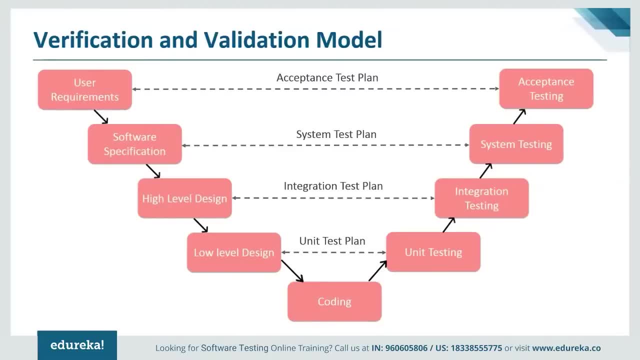 in the user environment and compatibility testing and sometimes non-functional testing are also done in this phase, and the artifacts produced will be user acceptance test results, updated business coverage matrices. So these are the various phases involved in the testing. that is the right hand side of the model. 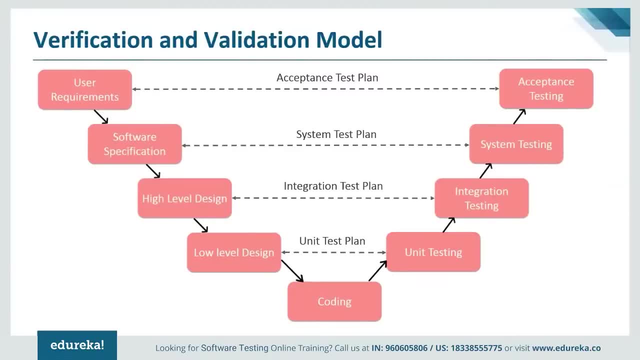 That's why it is called V and V model, where verification is nothing but development phase and validation is testing phase. So when to use V model? V model is to be used when the requirement is well defined and not ambiguous. acceptance criteria are well defined. project is short. 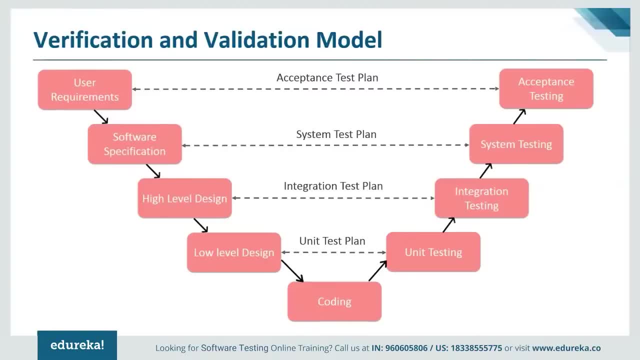 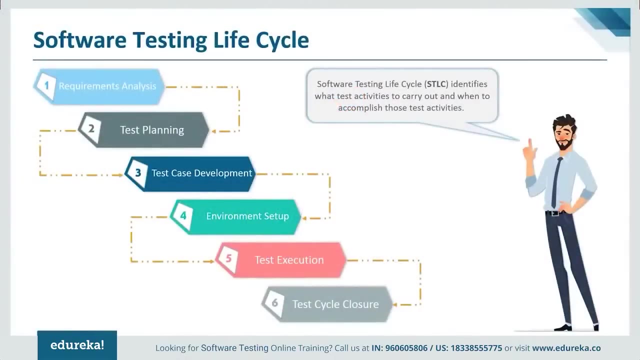 to medium in size and technology and tools used are not dynamic. These are the situations when you should use verification and validation model. Now let's move further and understand software testing life cycle. software testing life cycle is a testing process which is executed in systematic and plan manner. 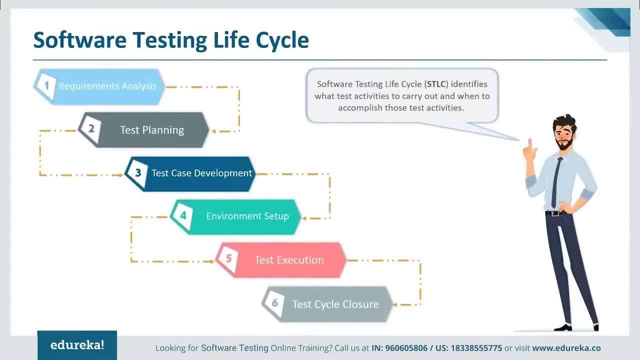 And software testing life cycle process, different activities are carried out to improve the quality of the product. So these are the various stages involved in software testing life cycle. first, requirement analysis. This is the very first step in software testing life cycle. in this step, the quality assurance team 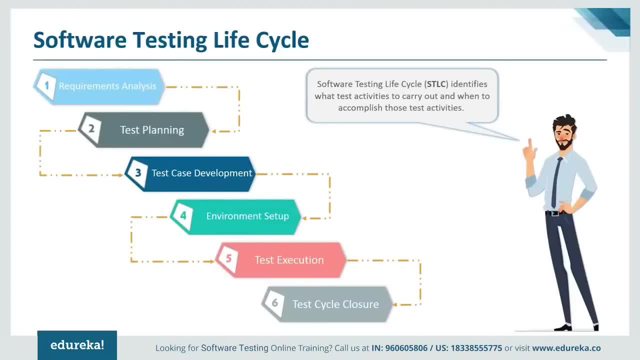 that is, your QA team understands the requirement in terms of what we will be testing and figure out the testable requirements. if any conflict, missing or not understood any requirement, then QA teams follows up with the various stakeholders, like business analyst, system architecture client, technical manager, to better understand the detailed knowledge of requirement. 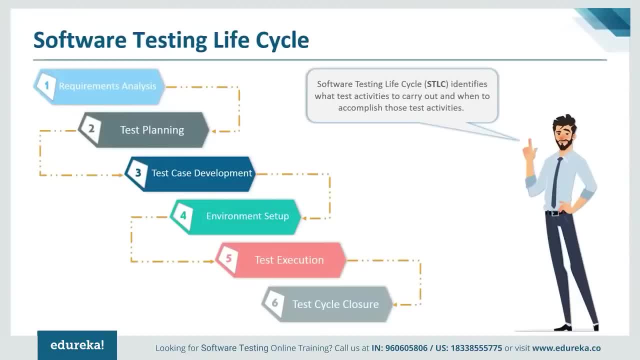 and after that we have test planning. test planning is most important phase of software testing life cycle where all testing strategy is defined. This phase is also called as test strategy phase. in this phase, typically test manager is involved to determine the effort and cost estimates for the entire project. 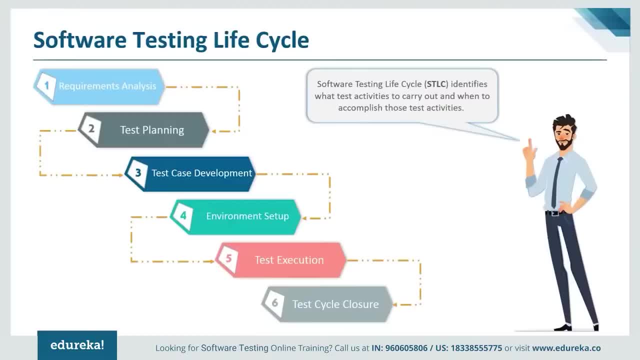 This phase will be kicked off. on the requirement gathering phases completed and based on the requirement analysis, We can start preparing the test plan, and the result of test planning phase will be the test plan or press strategy or testing effort estimation documents Once test planning phase is completed. 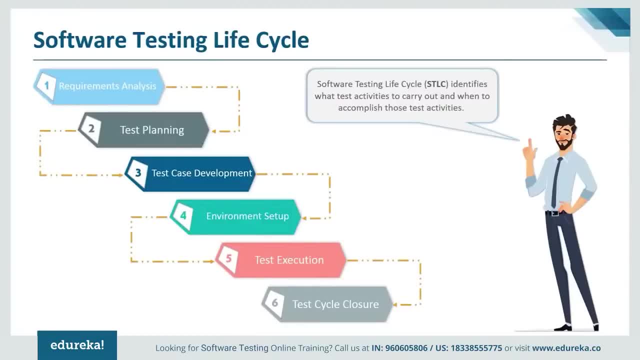 then QA team can start with test cases development activity. So next we have test case development, and this is started once the test planning activity is finished. This is the phase where testing team write down the detailed test cases. along with test cases, testing team also prepares a test data for testing. 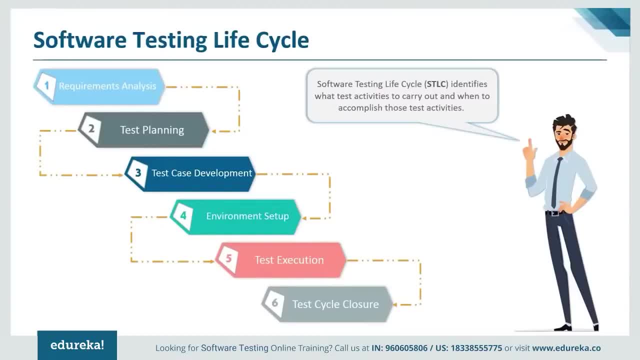 Once the test cases are ready, then these test cases can be reviewed by peer members or QA lead, and also the requirement traceability matrix is prepared. So what is this requirement? traceability matrix is an industry accepted format for tracking requirements where each test case is mapped with the requirement. 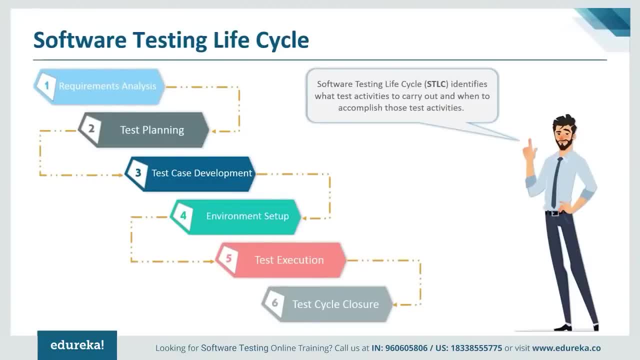 and using this RTM- that is requirement- traceability matrix can track backward and forward traceability. After all this, you have to set up the environment for testing. So this is a vital part of STLC and basically, test environment decides on which condition software is tested. 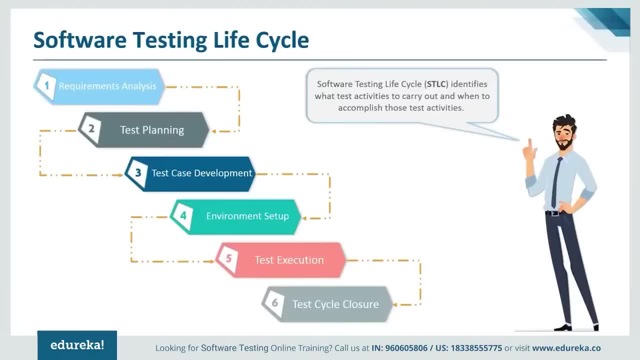 and it is an independent activity and can be started parallel with test case development. Next we have test execution. Once the preparation of test case development and test environment setup is completed, then test execution phase can be kicked off. in this phase, testing team start executing test cases. 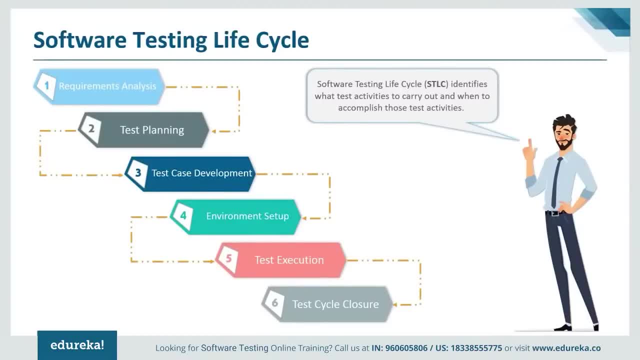 based on prepared test planning and prepare test cases in the prior step. And finally we have the test cycle closure. So in this, once the test case is passed, then same can be marked as passed. if any test cases failed, then corresponding defect can be reported. 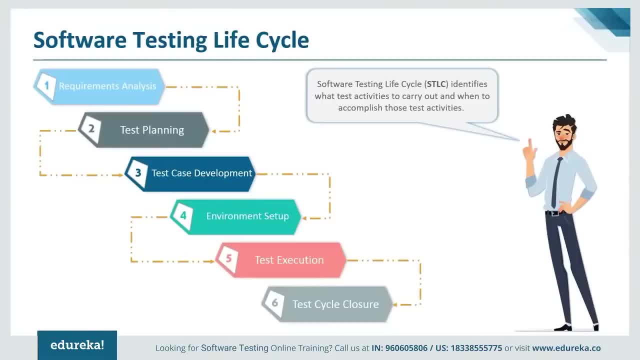 This can be reported to development team by a bug tracking system and bug can be linked for corresponding test cases for further analysis. So these are the various phases involved in software testing life cycle. Before I go further, let me clear out software testing is of two types. 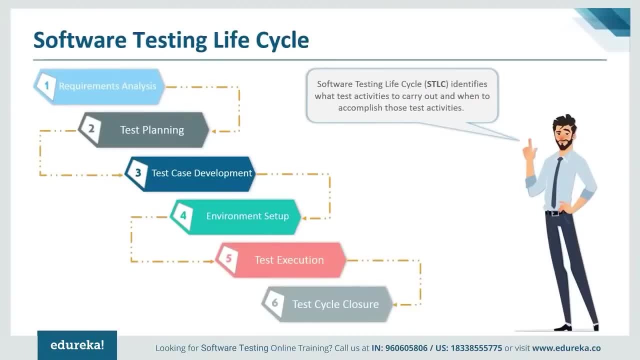 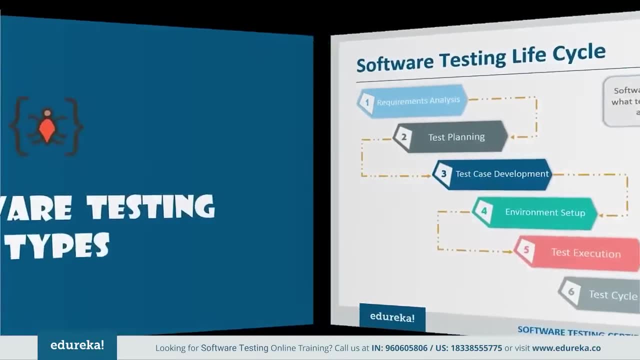 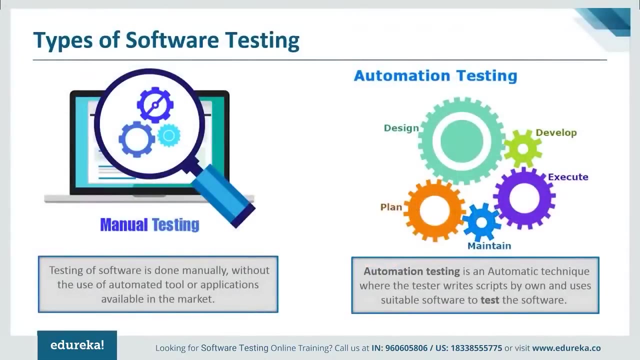 manual testing and automation testing, and selenium was founded as an automation testing tool to overcome the limitations and drawbacks of manual testing. So, till now, whatever you learned was manual testing, that is, the testing of a software is done manually, without the use of automated tool or applications that are available in the market. 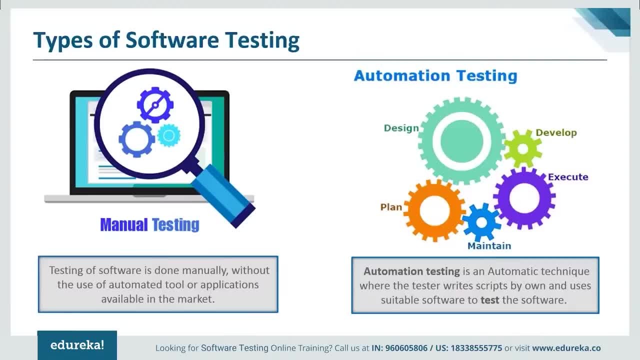 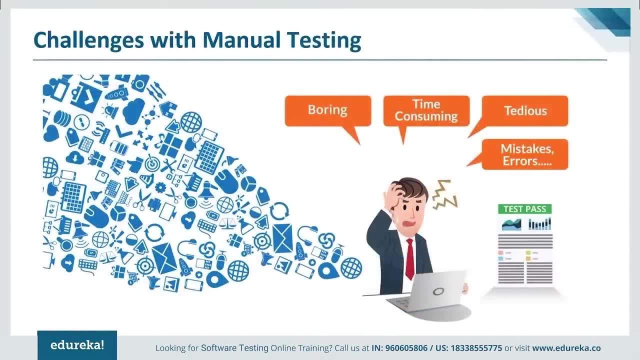 Automation testing is an automated technique where the tester writes scripts by own and use a suitable tool to test the software. It is basically an automation process of a manual process like regression testing. automation testing is also you to test the application from load performance and stress point of view. 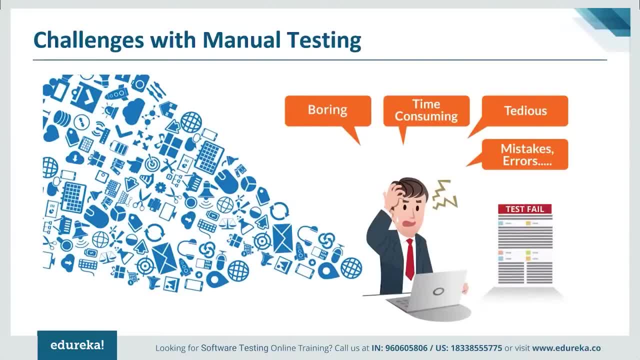 What are the challenges faced by manual testing? manual testing means the application is test manually by QA testers, and test needs to be performed manually in every environment using a different data set, and success failure rate of every transaction should be recorded. So look at the image over here. 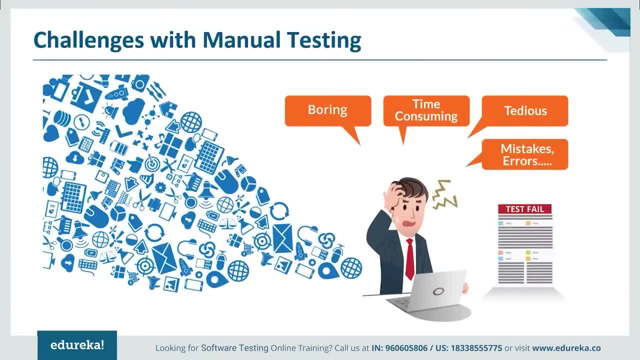 You can see a poor chap over here who manually verifies the transactions recorded. the challenges he is facing cause fatigue, boredom, delay in work, mistake and errors because of manual effort, and this leads to the need for automation testing. and automation testing beats manual testing every time. Why? because it is faster, needs less investment. 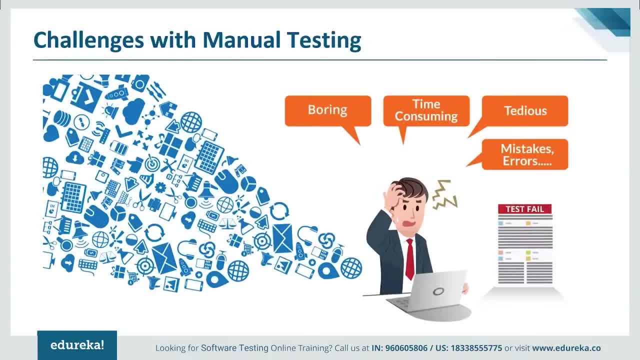 in human resource, It is not prone to errors. frequent execution of test is possible. support lights out execution and also supports regression and functional testing as well. And let's take a similar example. suppose there's a lot of log-in page and we have to verify if all the login attempts are successful. 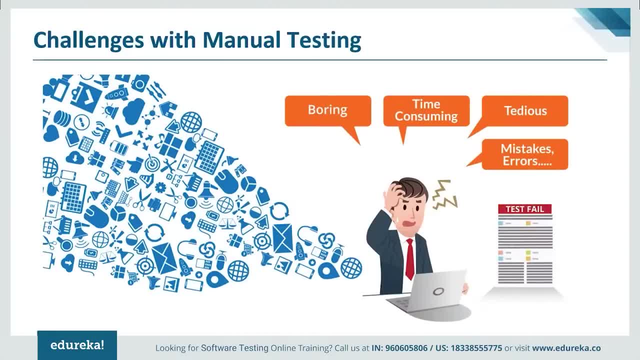 then it will be really very easy to write a piece of code which will validate if all transaction or login attempts are success or not. Moreover, these tests can be configured in such a way that they are tested in different environments and web browsers. What else can be done? 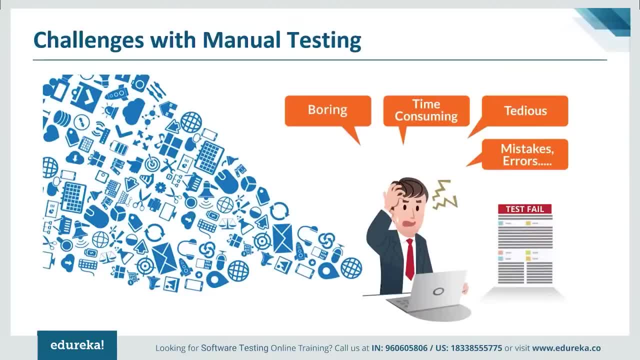 You can automate the generation of result file by scheduling it for a particular time during the day. Then you can also automate the generation of reports based on those results, and the key point is that automation testing makes a tester's job a whole lot simpler. So these are some of the challenges faced. 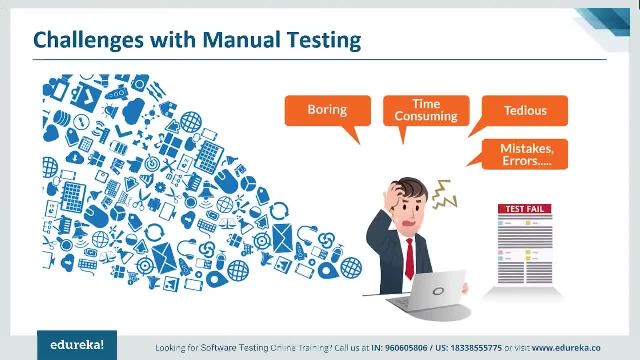 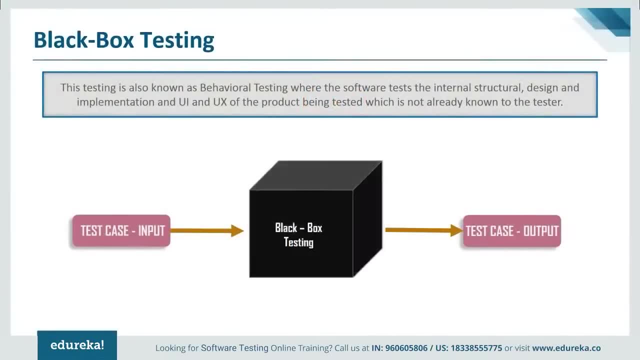 with manual testing and automation testing overcomes it. Now let's see different testing methods of software. First is black box testing. This testing is also called as a behavioral testing, where the software test the internal structure, design and implementation and the user interface of the product. 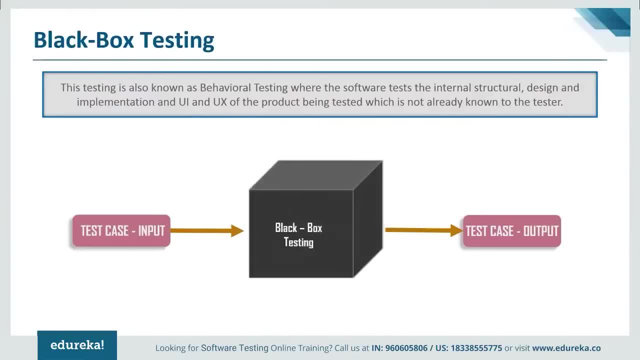 that is being tested is not already known to the tester. So that is the reason it is called as black box, where the input is being passed as a test case to the black box but the internal implementation details are not known to the tester and output is being given next white box testing. 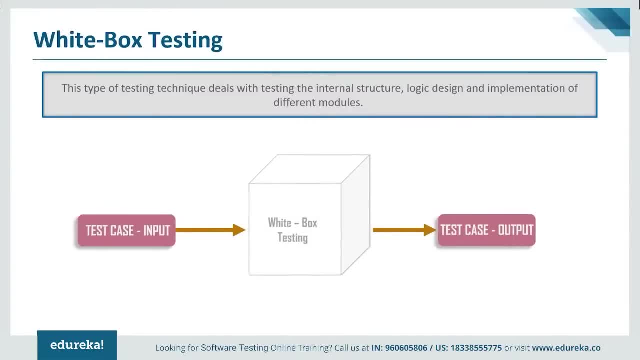 This type of technique deals with testing the internal structure, logic design and implementation of different modules. This is also called as a glass box testing, where the internal implementation details are known to the tester. that is, the code logic, internal logic, design and many more. and next we have gray box testing. in this 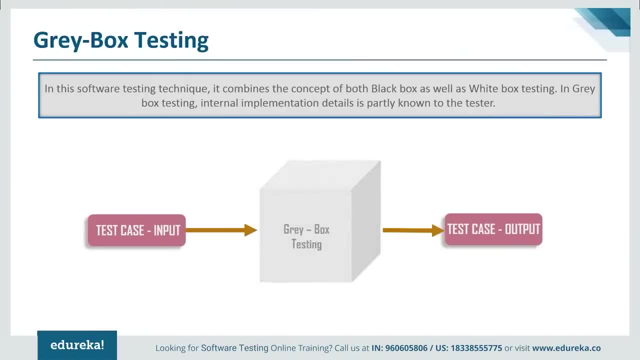 It combines the concept of both black box and white box. that does, internal implementation details are partly known to the tester, while the rest of the internal implementation details are not known to the tester and that's the reason it is called as gray box Testing. so these are the three methods of software testing. 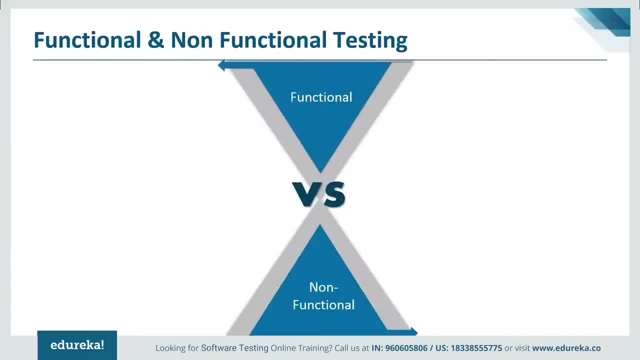 Now let's see the difference between functional and non-functional testing. as already listed, functional testing is performed before non-functional testing and non-functional testing is performed after functional testing, and functional testing is based on customer requirements. On the other hand, non-functional is based on customers expectations. functional testing describes: 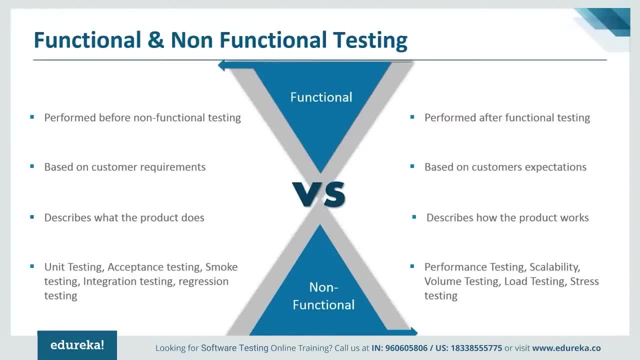 what the product does, and non-functional describes how the product works, and examples of functional testing are unit testing, acceptance, more testing, integration and regression testing. and non-functional testing includes performance testing, volume testing, scalability, load testing, strain and stress testing, Etc. So these are the differences. 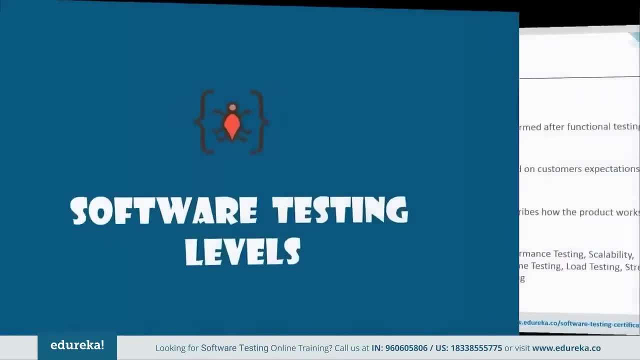 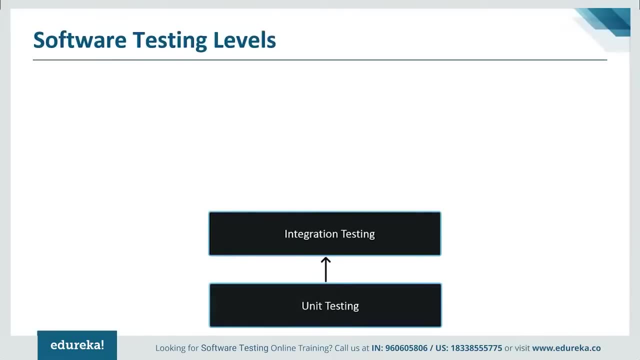 between functional and non-functional testing. Now let's talk about software testing levels. It starts From unit testing, where unit test cases are produced, and then it goes to integration testing, where the software is combined and tested and it produce integration test cases, and then comes system testing. 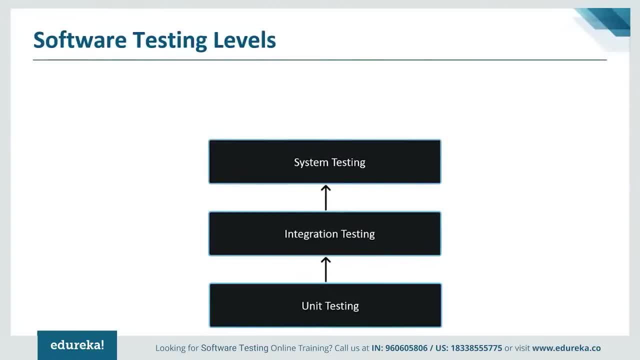 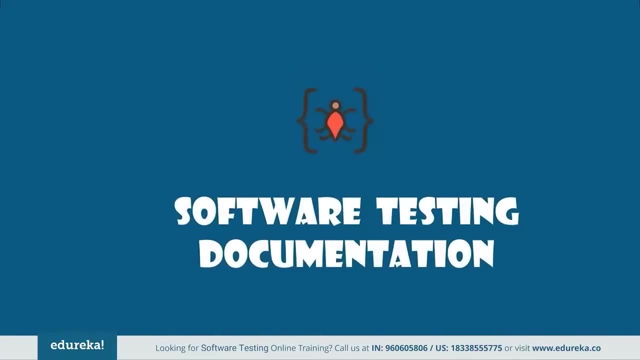 where the integrated software or project is tested, and then comes acceptance testing, where the system needs to be tested for adequacy. So these are the software testing levels. that starts off with unit testing and ends with acceptance testing. now Let's move further and understand software testing: documentation, documenting. 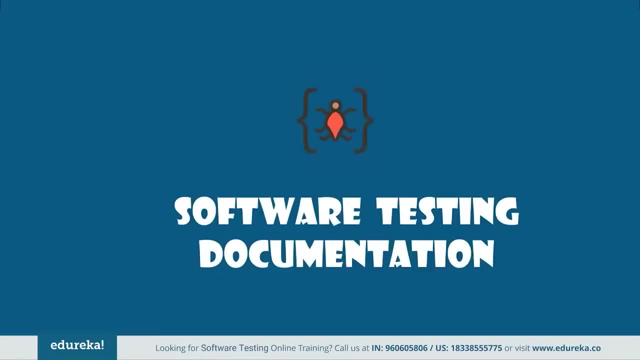 the test case deals with documentation, part of the developed product, which should have to be prepared before or at the time of software testing. documenting the test cases will facilitate you to estimate the testing effort You will need, along with the test coverage and tracking and tracing requirement here. 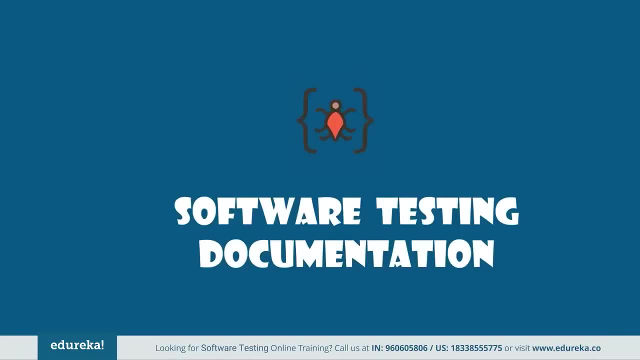 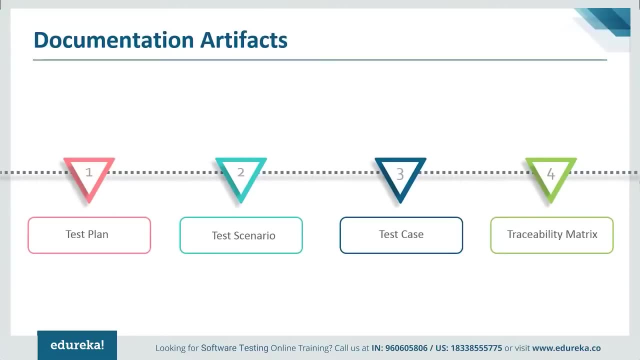 You will learn to dig into how documentation is beneficial by testing, along with some other features of it. So why do you think documentation is necessary? Some commonly applied documentation artifacts associated with software testing are test plan, test scenario, test case and traceability matrix. Let's discuss each of these in brief. 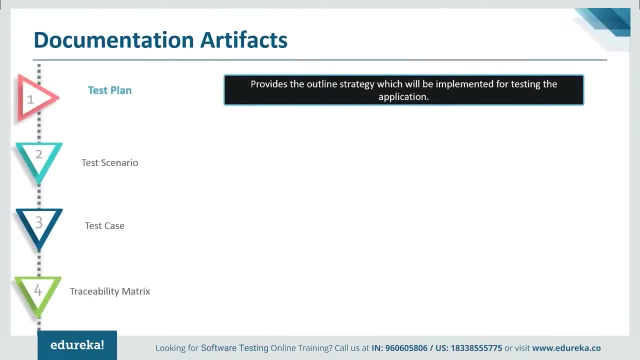 First test plan. test plan provides the outline strategy which will be implemented for testing the application, and the resources which will be needed are also described. It also holds the details about which environment the test will be performed. So let's take an example of how we have to maintain a test plan report. 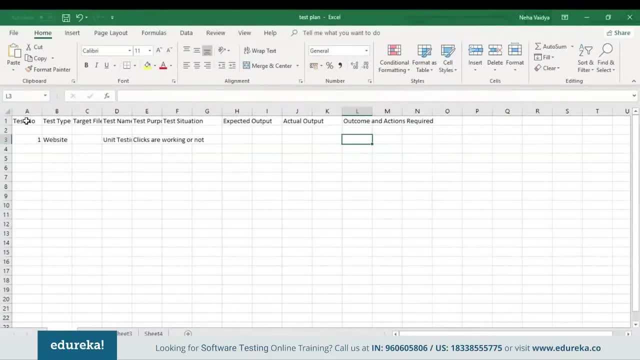 So this is my test plan report where I have columns like test number, the type of the test, target file, test name, purpose of the test, test situation, expected output, actual output and outcomes and actions that are required. For example, say you are testing a website. 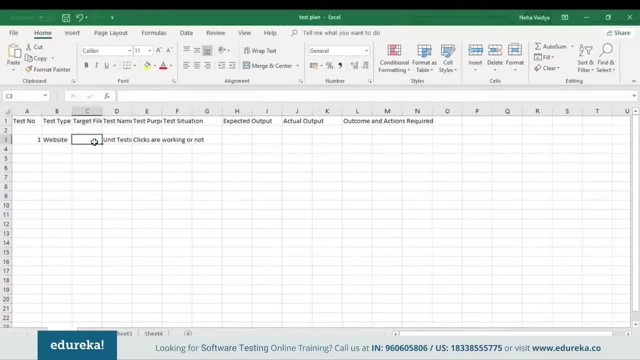 So the test type will be website And you have to give your test number, say or testing on particular login information. You can give the target file as login information and you can give whatever the test that you're performing, Say, for example, unit testing, and you can check the purpose. 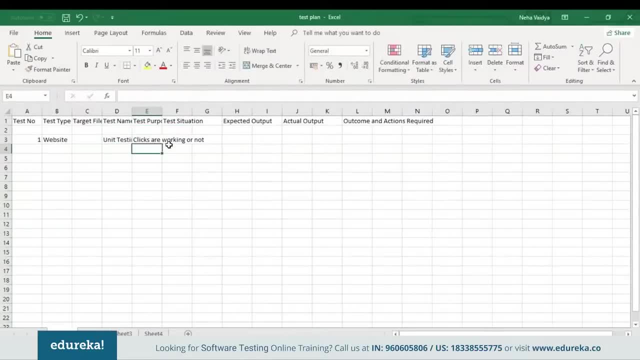 and the situations, whether all the clicks are working or not, or the email address is being entered or not in the login page, and whatever the output that you expect and whatever the actual output that arrives, and what is the outcome of it and the actions that you need to be performed. 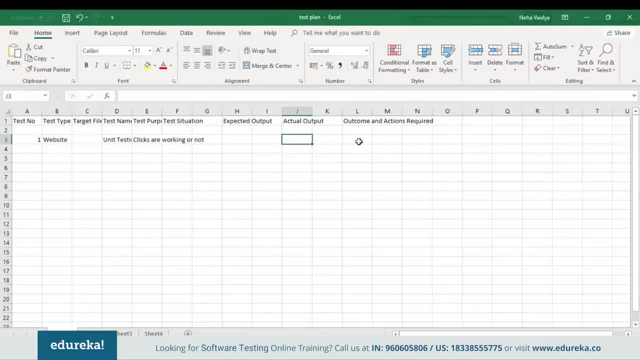 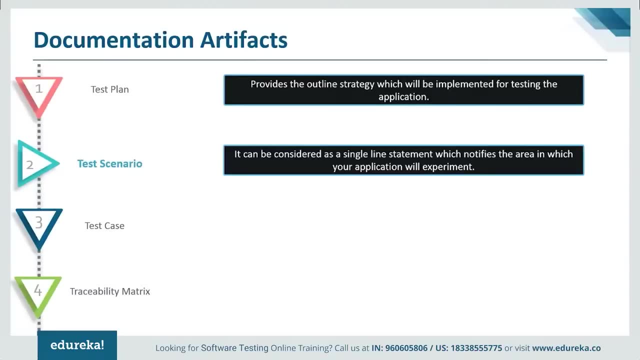 These are all the main considerations of a test plan report. Now let's see what is a test scenario. Test scenario can be considered as a single line statement which notifies the area in which your application will experiment. This artifact is needed for ensuring the overall procedure. 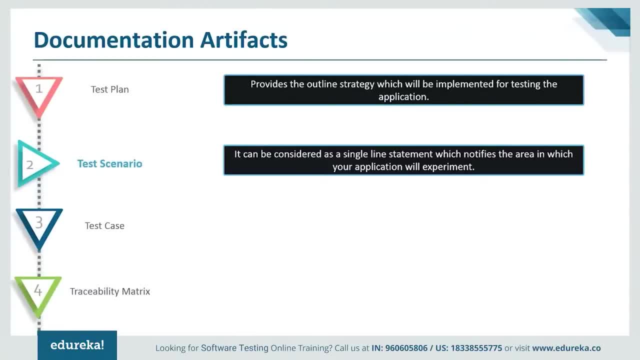 tested from start to finish. So, again, this is your test scenario, where you need to have your use case ID, your requirement ID, the scenario on which you're working on and what is the test scenario and how many test cases. that is the number of test cases that is required. 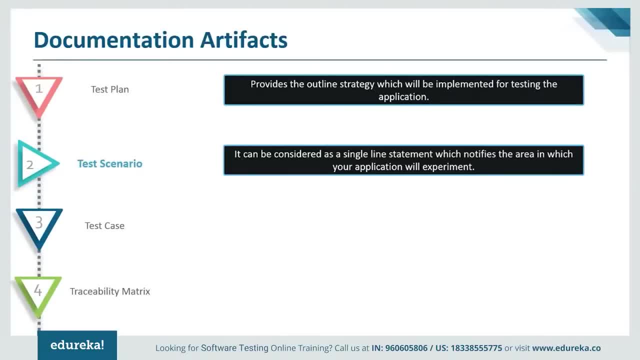 So you can go on documenting all the records over here in the test scenario. Next is test case. test cases engage in collected step and conditions with inputs which can be implemented at the time of testing. This activity focuses on making sure whether a product went through a set of tests. 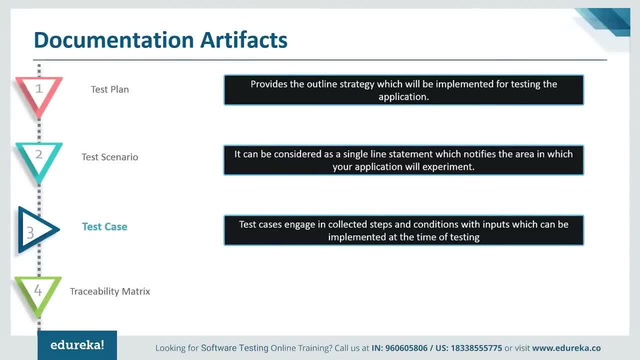 or fails by any means, such as functionality or other aspects. Many types of test cases are being checked during testing, like functional test cases, negative error test cases, logical and physical test cases and user interface test cases as well. So these are the columns which are necessary for a test case. 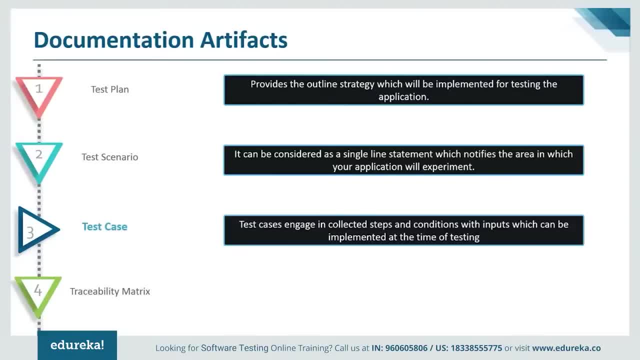 That is your test case ID, your test case, whatever it is, its description, the step that you take for testing a particular software or a particular test case, and this description again, your expected result, actual output, status and comment. Now, the last artifact that we have is traceability matrix. 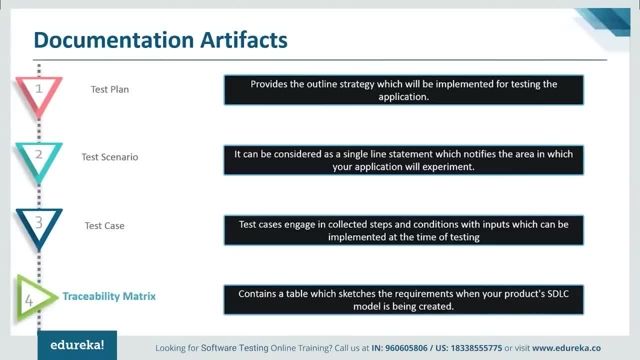 It is also known as requirement traceability matrix, and it contains a table which sketches the requirements when your products software development life cycle is being created. This documenting artifact can be implemented for forward tracing, which is to go from designing, or can be implemented for backward tracing as well. 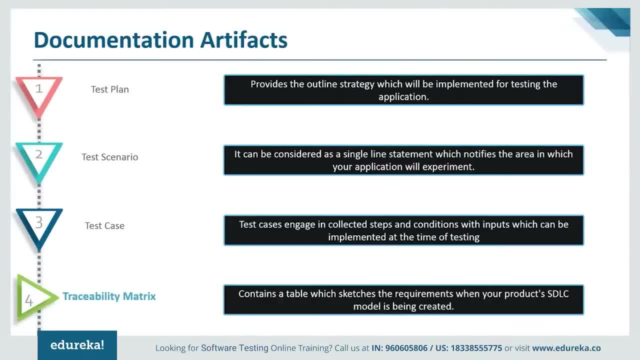 which is the reverse of forward tracing. So this is how you put a traceability matrix. that is, you will be having your requirement traceability where you have n number of test cases, and here you have business requirements. So the matrix will be put if the result will be passed on both the ends. 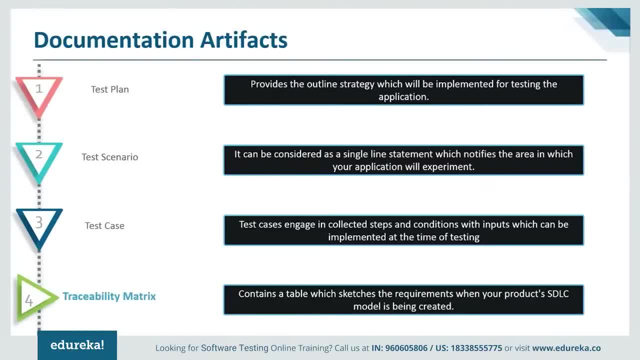 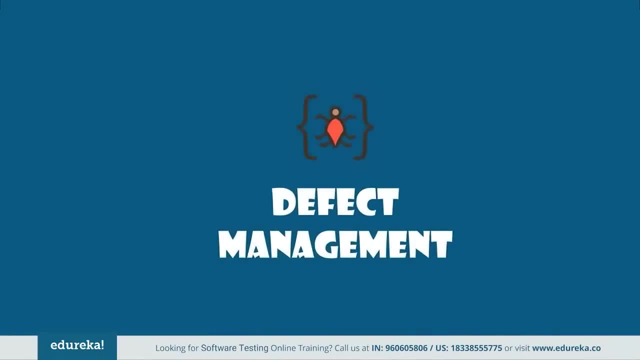 So this is all about the documentation artifacts and the various types of artifacts that are involved in software documentation. Now let's talk about defect management. as we know, defect management is a part of software testing process, But what exactly is defect management in software testing is not being known. 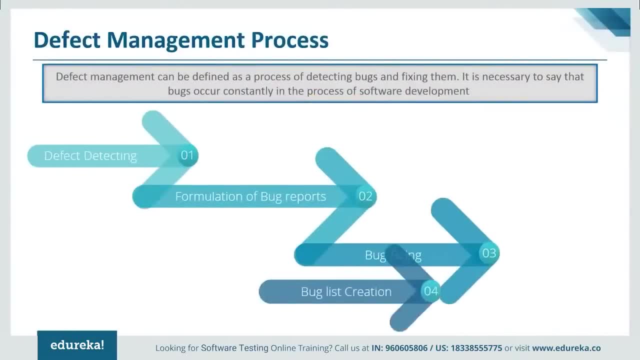 Now I will talk about it and tell you what exactly is defect management process. to realize what defect management process actually is, We should first understand the definition. Generally, defect management can be defined as a process of detecting bugs and fixing them. It is necessary to say that bugs occur constantly. 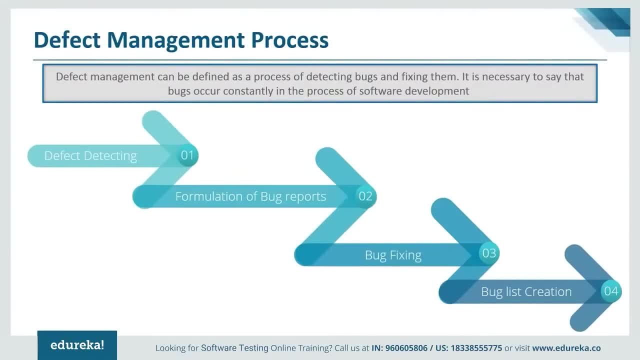 in the process of software development. They are a part of the software industry and that is because of the fact that software development is quite a complex process. The team members are usually placed in strict time frames. They must write large pieces of code every day. 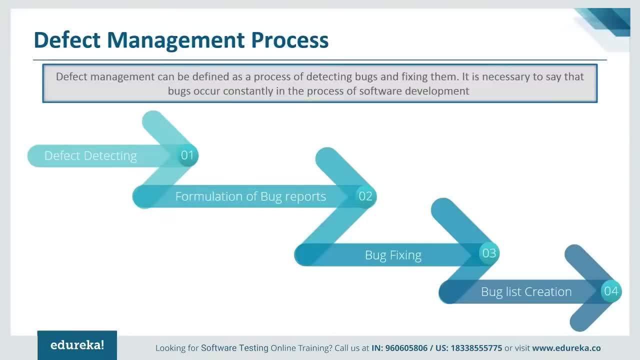 and they usually don't have time to think about how to avoid bugs. Hence, every software development project requires a process that helps to detect defects and fix them. The process of defect management, or bug tracking, is usually conducted at the stage of product testing, Without realizing this. 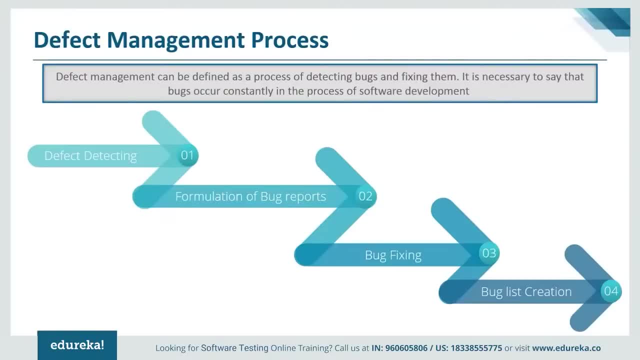 it would be hard to understand the nature of defect management. Software testing can be conducted in two different ways. Usually, the developers test the product themselves. However, there's also a type of testing that is based on user involvement. The final users are often provided. 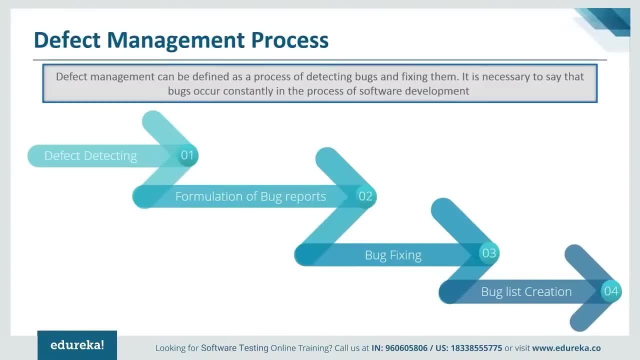 with an ability to report on the bugs they find Nevertheless, but this is not the best way of testing because the users could hardly find all the bugs. and there are four steps involved in defect management process and they are as shown on the screen. The first step is the stage of defect detecting. 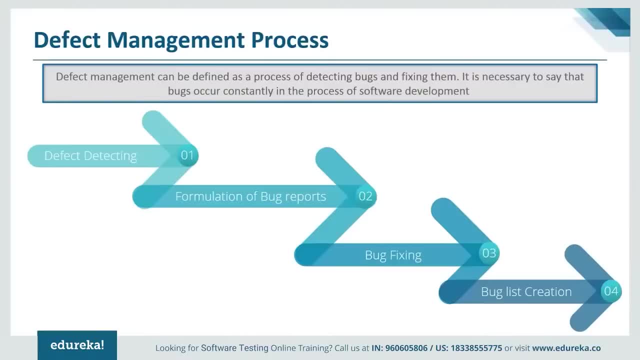 We already mentioned that it can be conducted either by the team of developers or by the users. regardless of the type of the testing, The main goal is to detect all the bugs and the final product, or its part. Next step is formulation of bug reports. 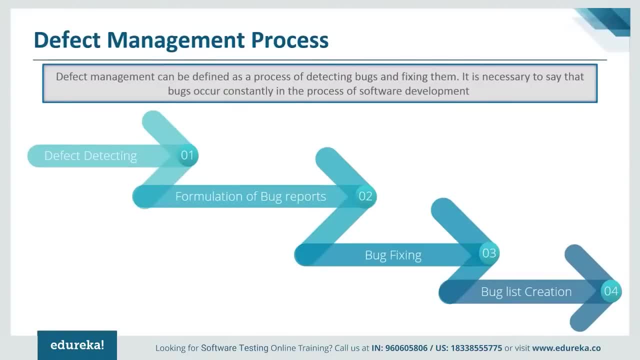 So these are the documents that include all necessary information about certain bugs. Usually they contain data on the type of bug and the possible way of its correction. and next step, that is, the third step, is the stage of bug fixing, After the bugs are fixed. 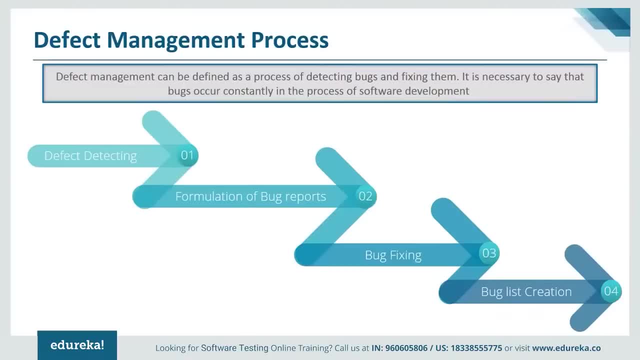 they should be tested once more to make sure that the software works properly, and during the final step, the bug list is created. So this is a document that contains information about all the bugs that occur during the project's performance, and the team often uses the bug list. 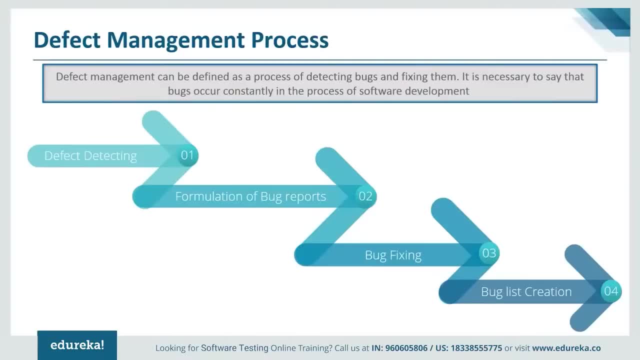 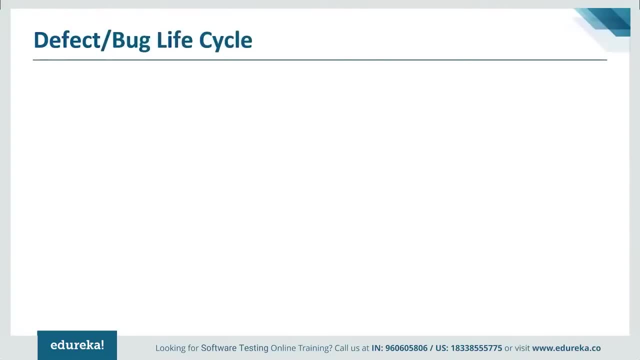 because the similar bugs have occurred. So this is all about the defect management process. Next we'll see what is the defect life cycle or a bug life cycle. Defect life cycle is a cycle which a defect or a bug goes through during its lifetime. 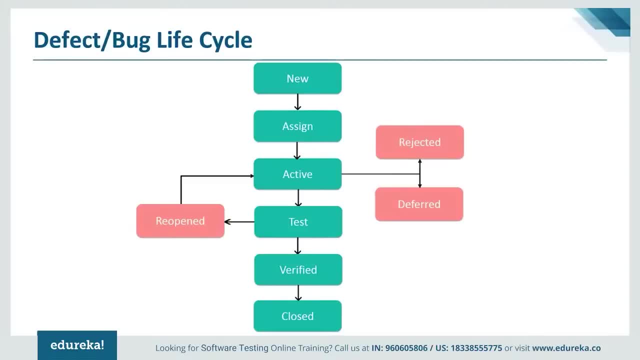 It starts when a defect is found and ends when a defect is closed after ensuring it's not reproduced. Defect life cycle is related to the bug found during testing. This life cycle can vary from organization to organization and also from project to project, based on several factors like organization policy. 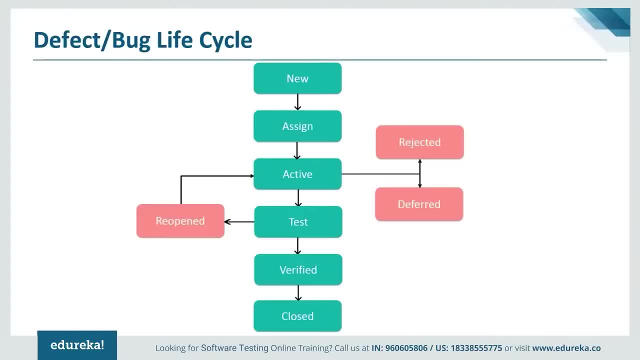 software development model like agile, iterative, project timeline, team structure, etc. Bug or defect life cycle consists of these following stages and that starts from new. This is the stage when a defect is logged and posted for the first time and that defect state is given as new. 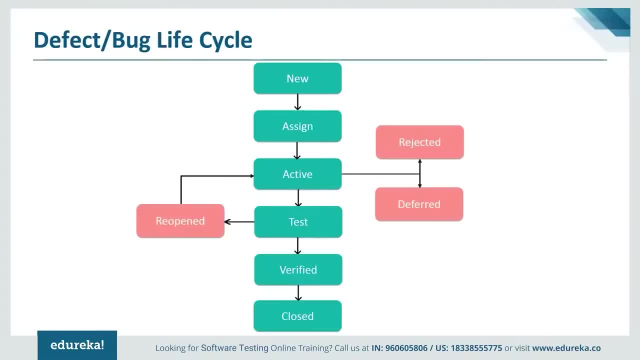 Next assign: After the tester has posted the bug, the lead of the tester approves that the bug is genuine and he assigns the bug to corresponding developer and the developer team and this state is given as assigned. Next active or open At this state. 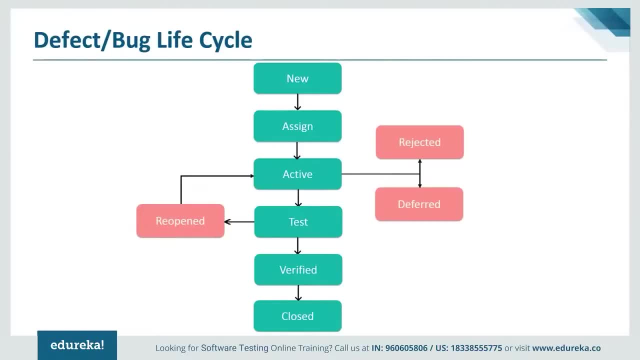 the developer has started analyzing and working on the defect fix and when developer makes necessary code changes and verifies the changes he or she can make the bug status as fixed and the bug is passed to the testing team. So at this stage the tester do the testing of the changed code. 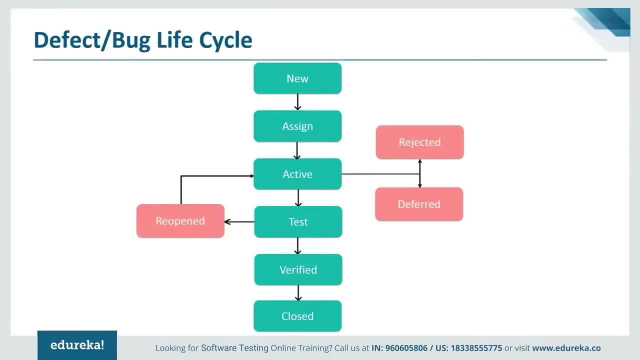 which the developer has given to him to check whether the defect has got fixed or not And, as you can see on the left-hand side, you have a reopen state In this- if the bug still exists even after the bug is fixed by the developer. 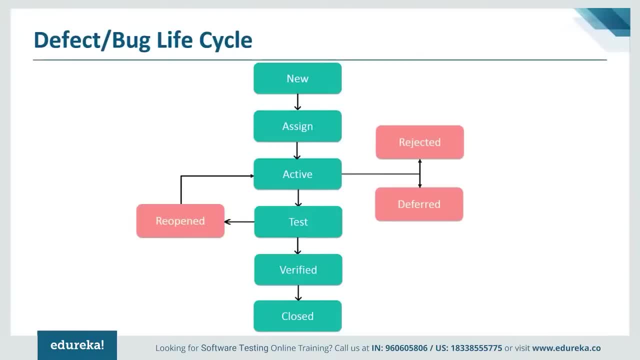 the tester changes the status to reopen Again. the bug goes through the life cycle once again and next again it will go through verified, that is, it should be verified by the tester again and again to check whether the bug is completely removed and the 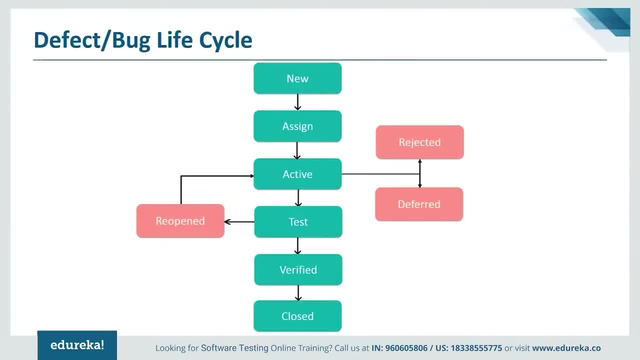 Software or a particular product is error-free and then you have a closed state. That means once the bug is fixed, it is tested by the tester. If the tester feels that the bug no longer exists in the software, he or she changes the status of the bug to closed. 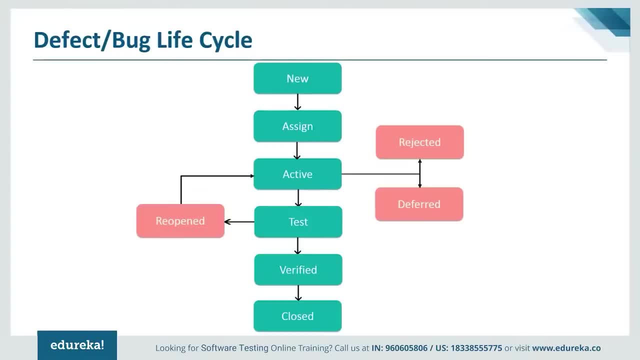 This state means that the bug is fixed, tested and approved and you can see from active state It goes to two more stages, that is, rejected and deferred. Rejected means if the developer feels that the bug is not genuine, he rejects the bug. Then the state of the bug is changed to rejected. 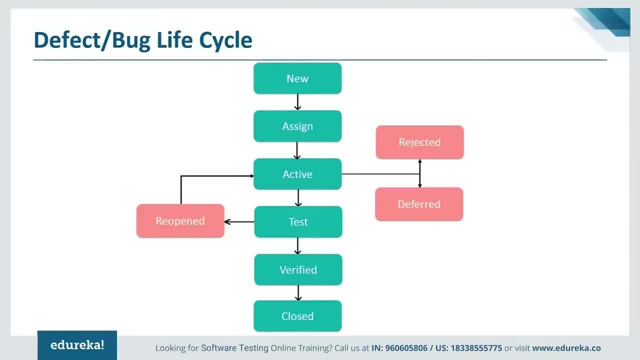 Deferred state indicates the bug is expected to be fixed in next releases. The reasons for changing the bug to this state have many factors. Some of them are: priority of the bug may be low, lack of time for the release or the bug may not have major effect on the software. 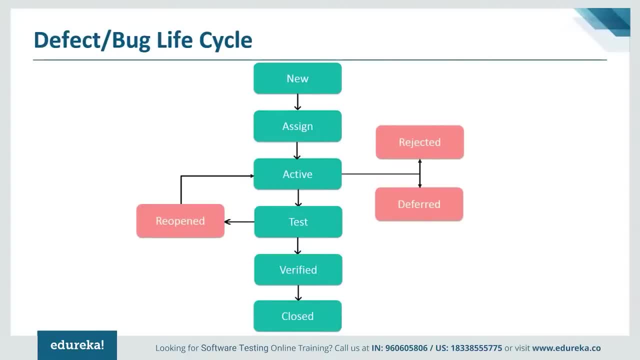 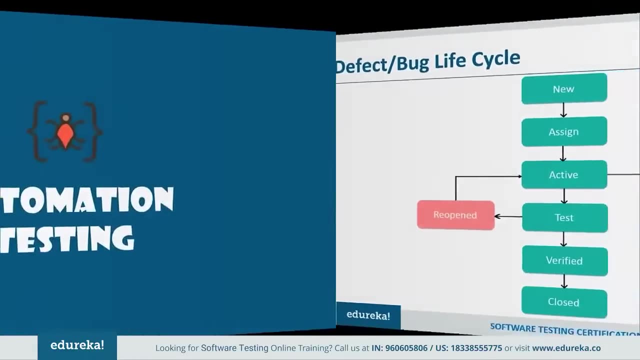 and that's the reason it is said as deferred. So this is all about the bug life cycle and the various stages the bug goes through Once it is new till closed. Now let's move on to the widely used software testing type, that is, automation testing. 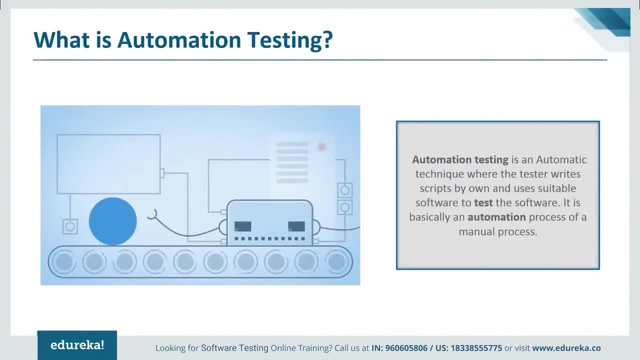 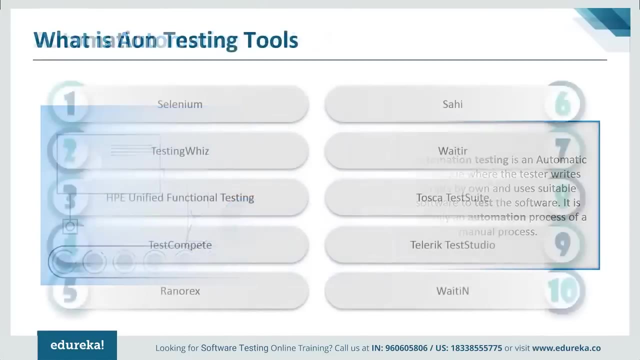 as I have already mentioned, automation testing is an automated technique where the tester writes scripts by own and uses suitable tools to test the software. It is basically an automation process of a manual process. So there are many tools to carry out automation testing, like selenium testing with HPE unified. 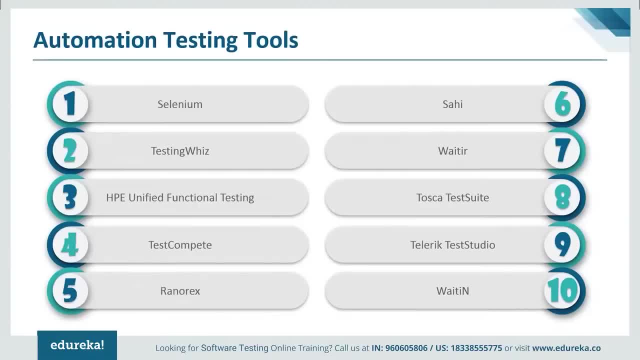 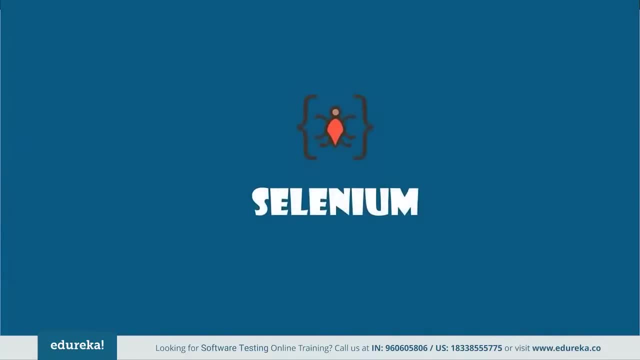 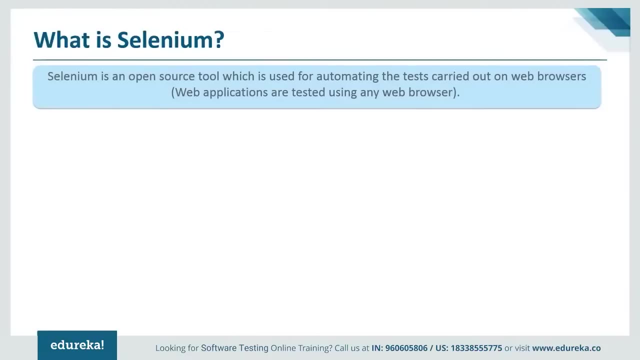 Functional testing test: compete: Rana racks, wait, IR, wait, iron tell Rick test studio toast card test and many more. So what is selenium and why it is a preferable tool? selenium is an open source tool which is used for automating the test carried on the web browser. 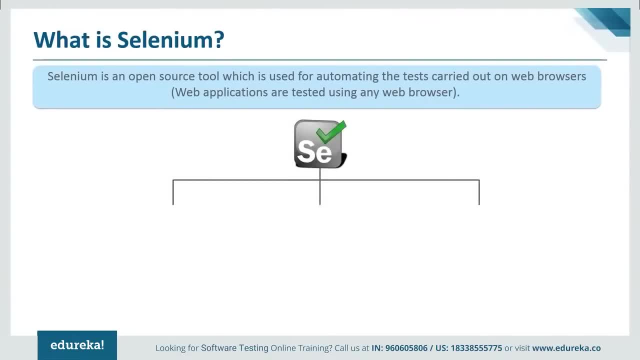 Wait before you get carried away. Let me reiterate it: only testing of web applications is possible with selenium. We can neither test any desktop application Nor test any mobile application using selenium. since selenium is open source, There is no licensing cost involved, which is a major advantage over other testing tools. 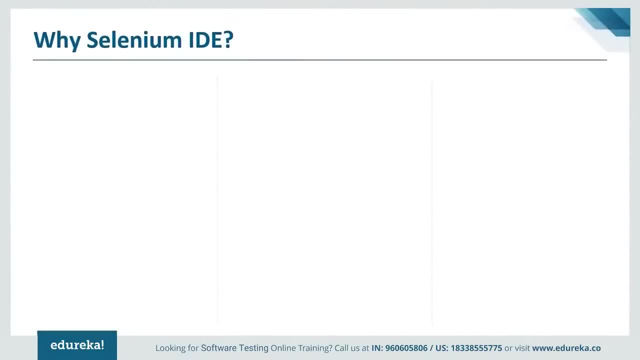 So why do you prefer selenium? The reasons behind ever-growing popularity of selenium are: test scripts can be written in any of these programming languages, like Java, Python, C, sharp, PHP, Ruby, Pearl and dotnet as well, and tests can also be carried out in any of the OS. 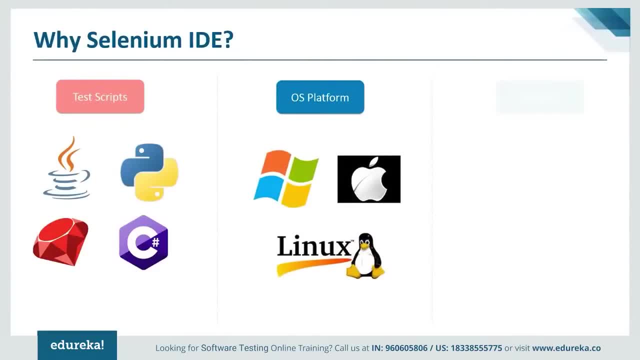 like Windows operating system, Mac or Linux. Not only that, it can be carried out using any browser like Mozilla, Internet Explorer, Google Chrome, Opera, Safari, etc. and tests can be integrated with tools like test NG and J unit for managing test cases and generating the reports. and it can also be integrated. 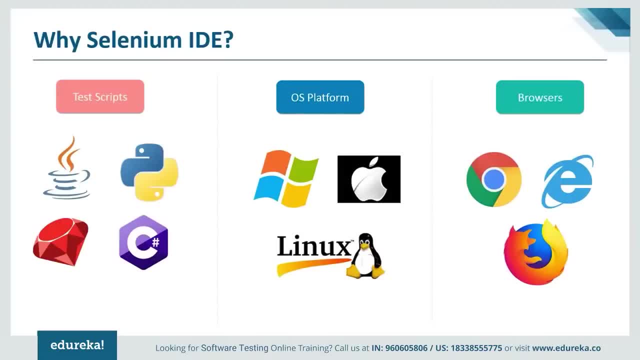 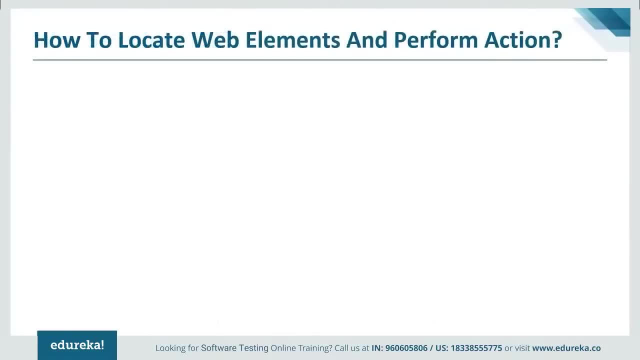 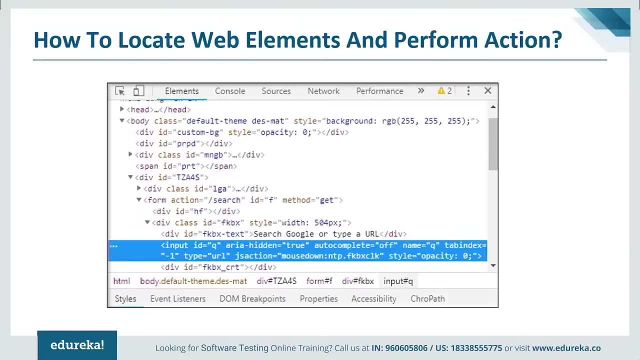 with Maven, Jenkins and Docker to achieve continuous testing, And that is the reason everyone Prefer selenium over other automation testing tools. So how to locate web elements and perform action. So this is nothing but your web page, where you have inspected the element and you're trying to locate a particular element. 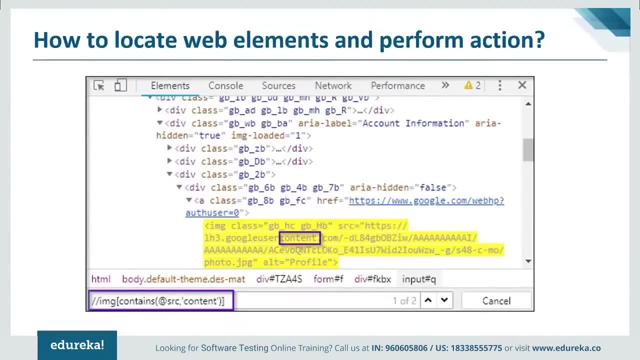 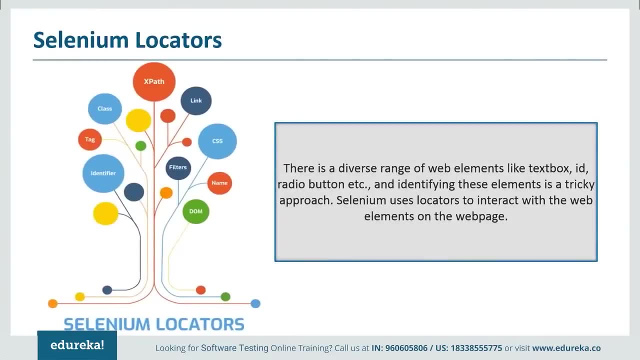 on the web page. So how is that done? I'll tell you how that is with the help of selenium locators. So what is a locator? locator can be termed as an address that identifies a web element uniquely within the web page. They are: 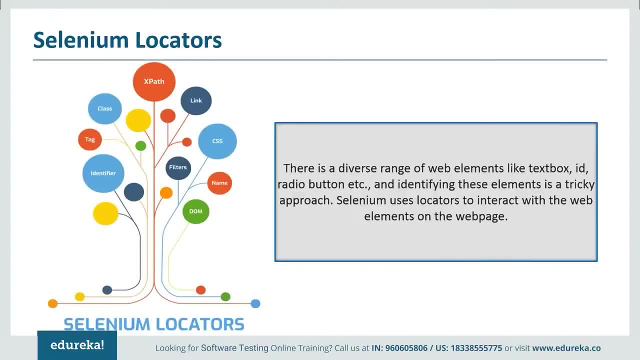 The HTML properties of the web element, which tells the selenium about the web element It needs to perform the action on. selenium uses locators to interact with the web element on the web page. They are considered as the lifeblood of the tests. using the right locator ensures that the tester faster. 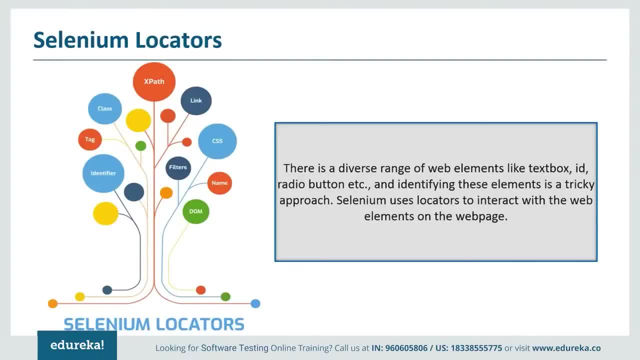 more reliable or has lower maintenance over releases. If you are fortunate enough to be working with unique IDs and classes, then you are usually all set, but there will be Times when choosing a right locator will becomes a nightmare. It can be a real challenge to verify. 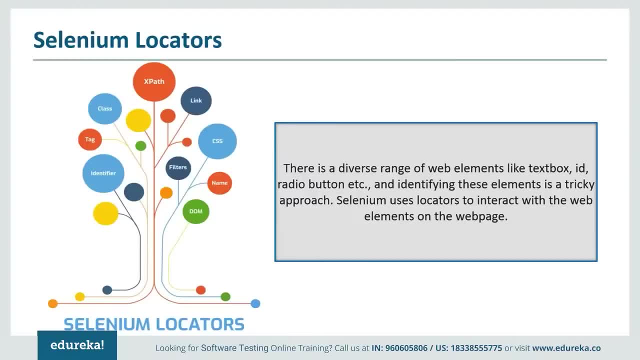 that you have the right locators to accomplish whatever you want. So there are diverse range of web elements like text box, ID, radio button, etc. and identifying these can be a tricky approach. So let's see how and what are the different types of locators. 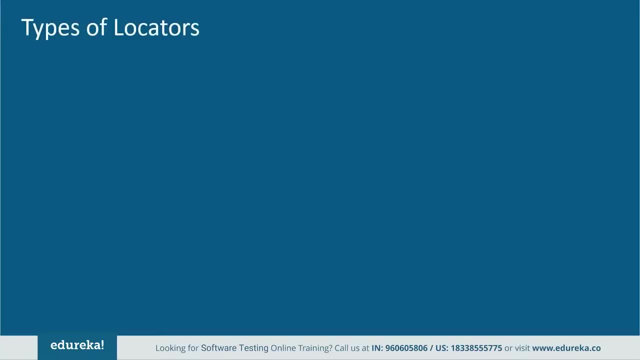 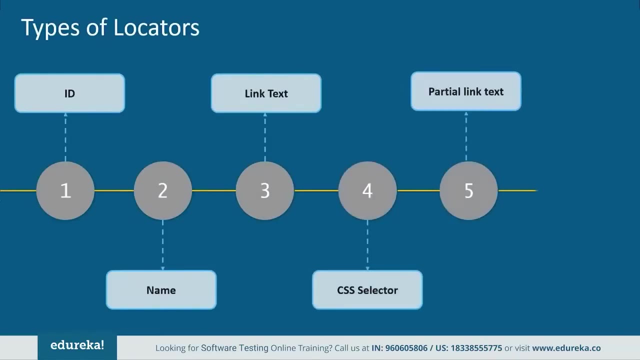 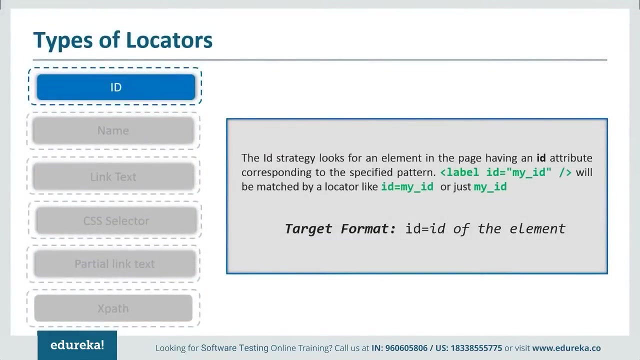 that can be used to locate a particular web element on the web page. So we have ID, name, link text, CSS selector, partial link text and XPath. First coming to ID, the best and most popular method to identify web element is to use ID. 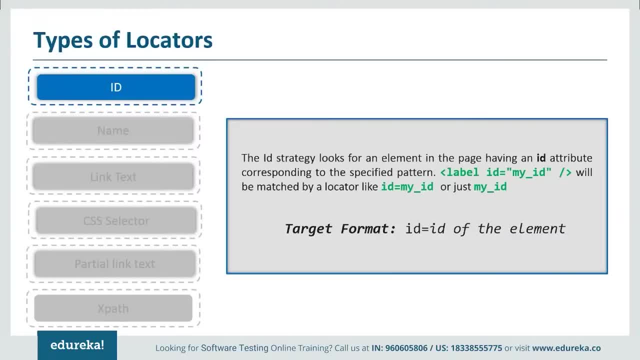 The ID of each element is alleged to be unique. IDs are the safest and fastest locator option and always should be the first choice. Even when there are multiple choices, it's like an employee number or account which will be unique. Let's see an example. 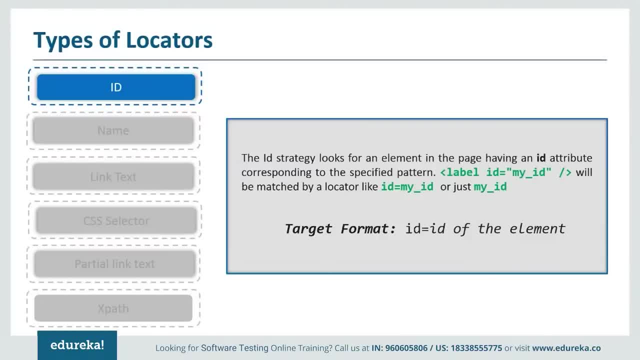 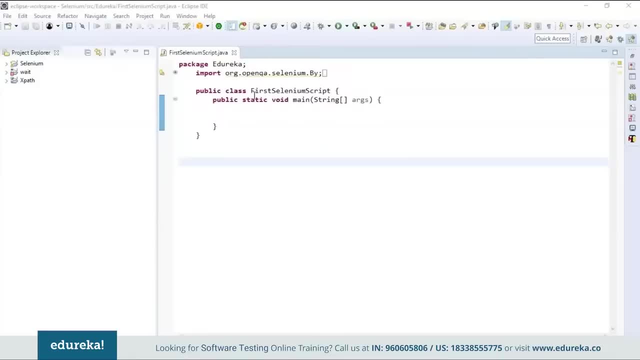 How to locate it and how to write a particular script for Selenium. So the very first step is to open your Eclipse, create a class. I have created a class called first Selenium script, and I have written my main method. Now next what I will do. 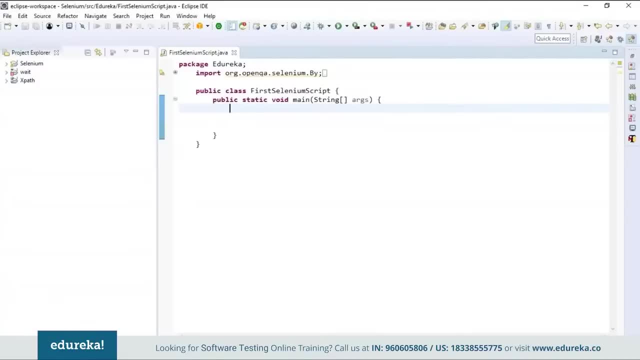 So the first step is to register Chrome driver. Why, When you write a script and run it, the Chrome driver will launch the Google Chrome. If you're using Google Chrome web browser, or if you are using Mozilla Firefox, you can choose Kiko driver. 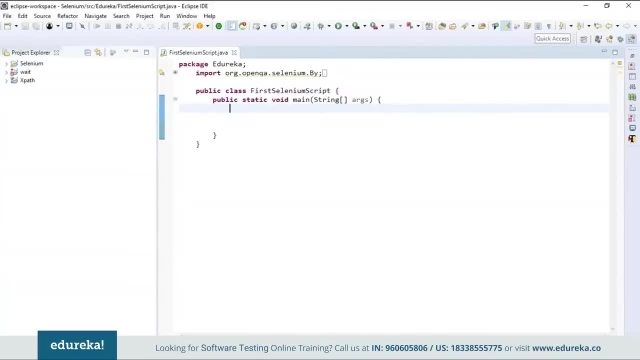 So, as I'm using Chrome driver, I have to set the properties for Chrome driver. I'll set it like this: I'll give system dot set property. Okay, now I have launched my Chrome driver. So what's next? Now I will use driver dot get method. 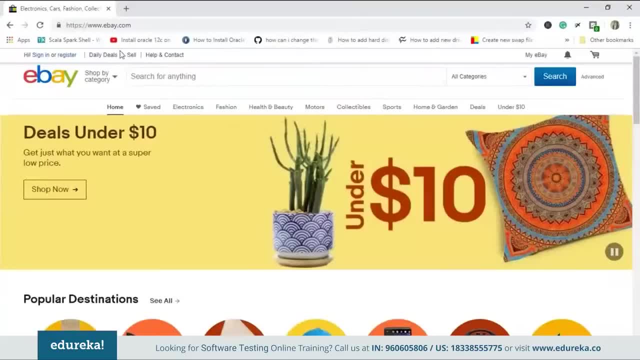 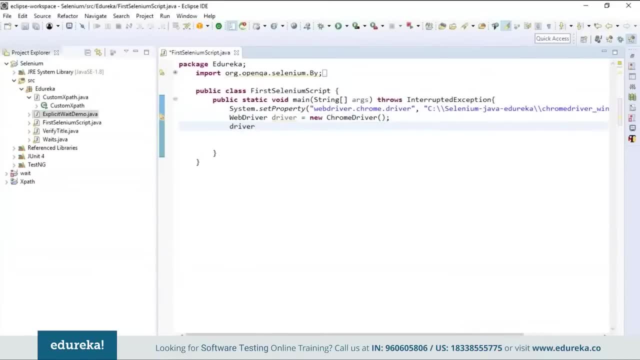 to navigate through ebaycom. Why? Because I'm using ebaycom website to test it, So I'll copy this and here I'll give driver dot get and I will paste the value of eBay within double quotes. Okay, after I do this, 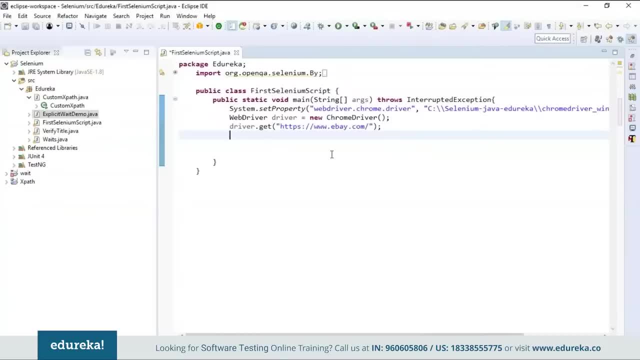 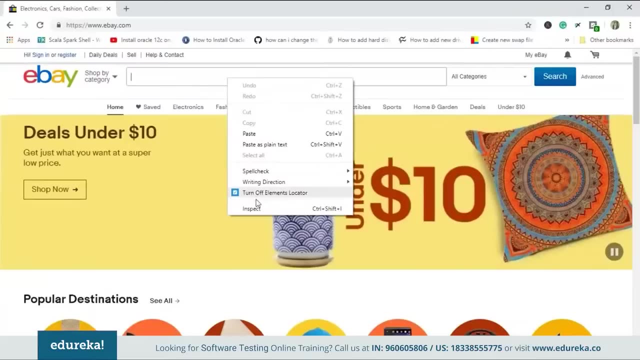 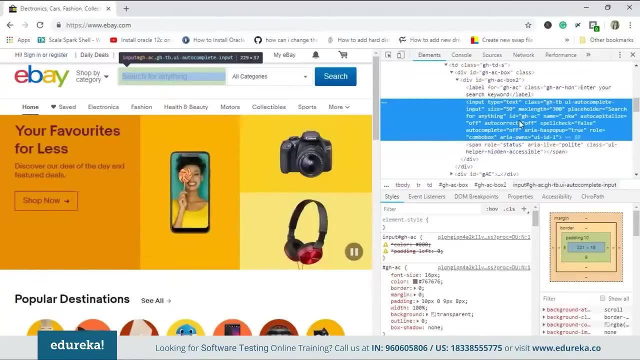 I have to use the ID locator to locate a particular web element. Now suppose, say, I want to locate the search box, What I will do. I'll right click on this: choose inspect. As I click on this thing, you can see the search box is getting highlighted. 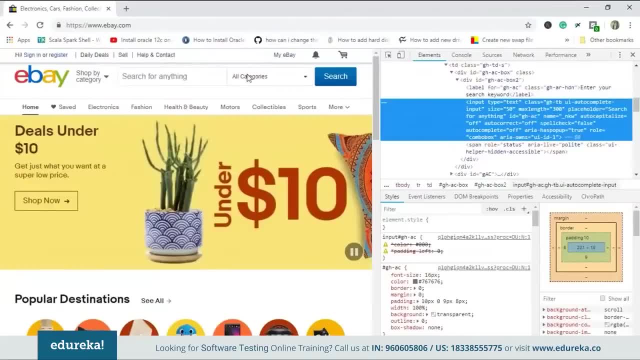 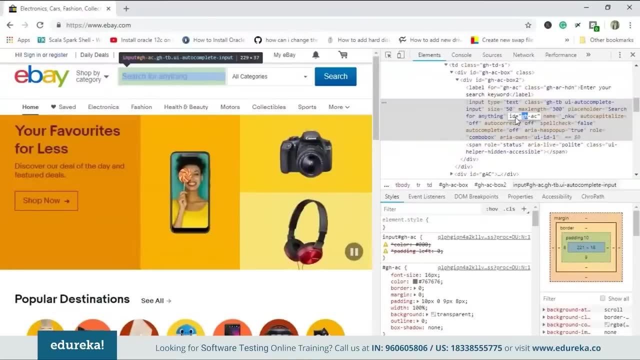 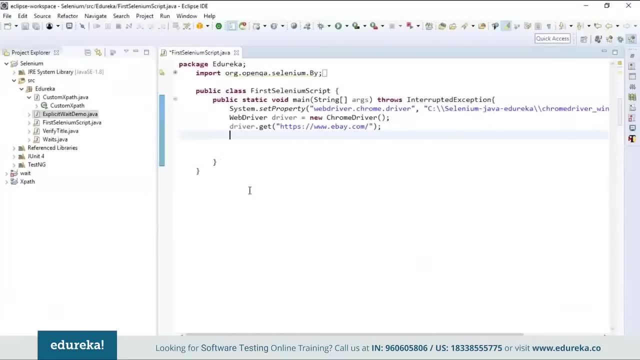 Which implies, as I mouse over on this, you can see this search for anything was getting highlighted. As you can see here, it has a ID attribute whose value is ghac. Okay, so I'll copy this and I'll write one method here. 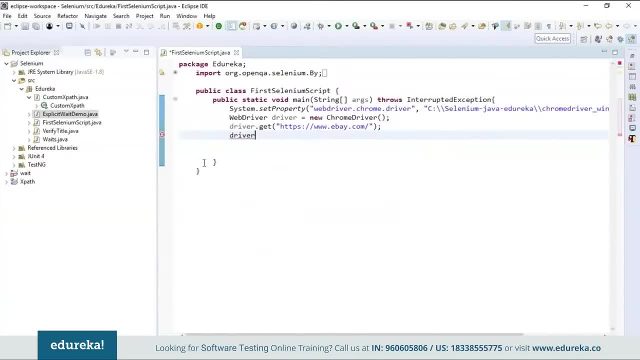 that is driver dot. find element by dot, ID. And what is the value of ID that you copied from ebay? It is ghac, Okay, so when you try to locate this by ID, that particular search box will be highlighted. Okay, now I want to do something like say: 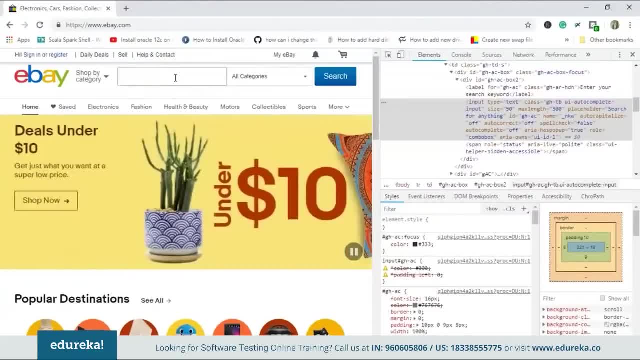 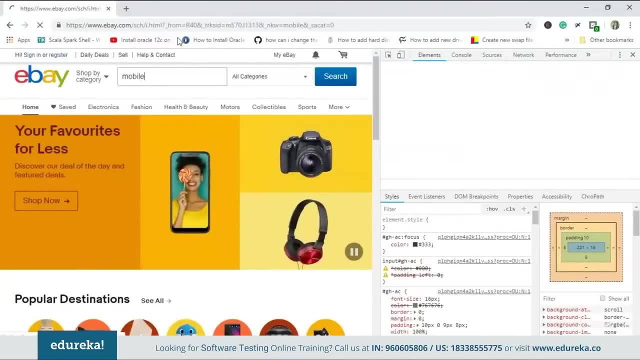 I want to enter some values for this. So how will I do that? I want to give like something called guitar or say mobile, and click on the search. When I search it over here, you can see the search filtered by shop, by brand. 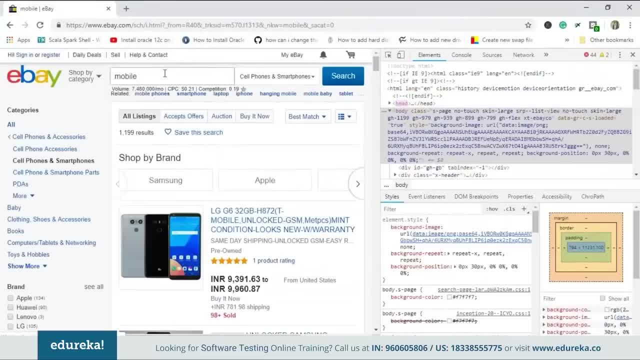 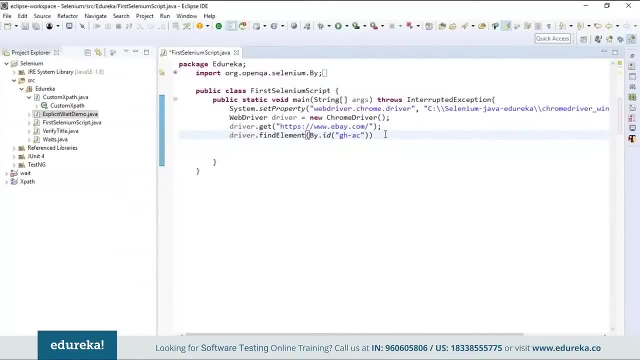 Okay, so what I'm doing here is I'm creating it manually. So if I want to search the same thing by selenium, how will I do that? For that, what I'll use after this, I will use a method called send keys. 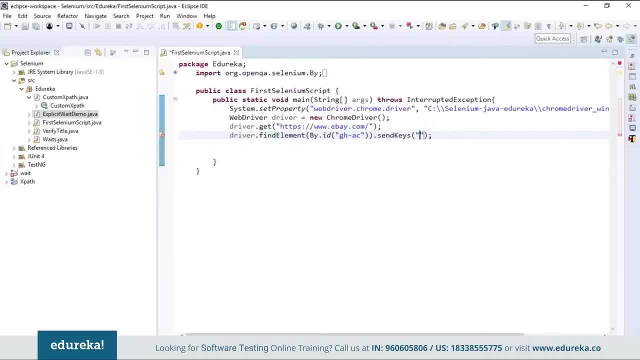 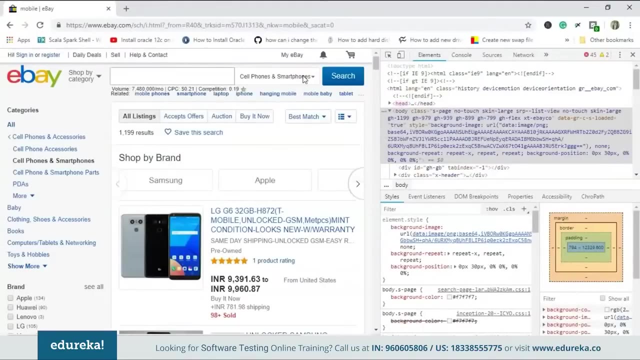 Okay, and I will pass the value of send keys as mobile. So now, next, once you give the send keys as mobiles, it will enter the value over here like mobiles. Okay, but it won't give a search. So, in order to get the search, 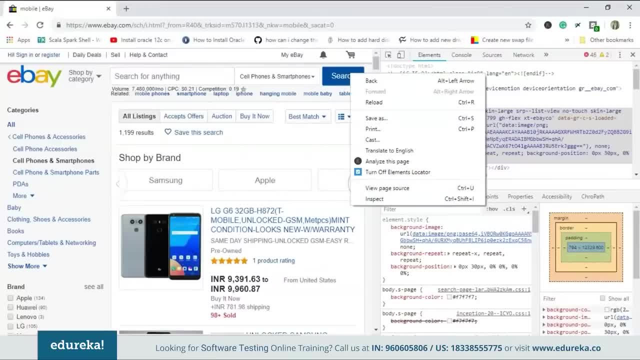 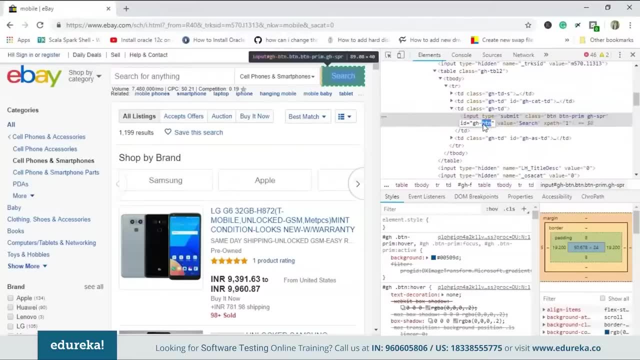 what we should do. you can see there's a search button over here, So inspect that. and again, even that has a ID whose value is gh button. Okay, so what I'll do? I'll just copy this again. I'll try: driver dot find element by ID. 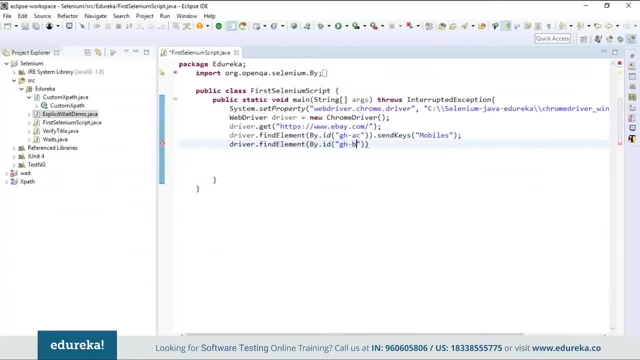 and send it as gh button. as it is a button, I have to use a click method because we are clicking on the button and not sending any values to the button. But if it is a text box, then you can send the keys and send the value. 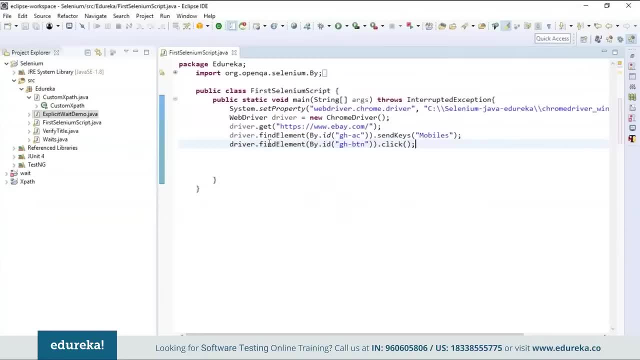 Okay, simple, save it Now. what's the next step? You are giving ID and searching mobiles and clicking on the search box, right, But there is something called implicit weights that is required to wait for a particular amount of time and then proceed further. 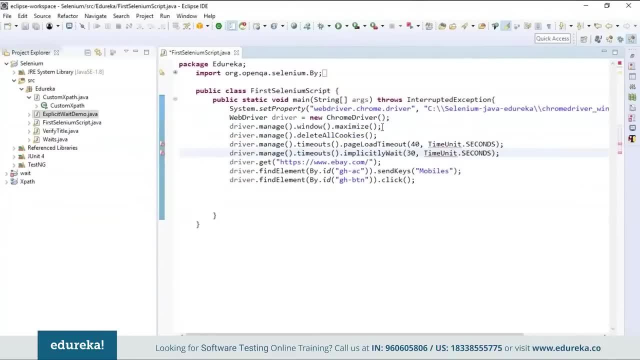 So I will be writing some methods over here, So I will use this method. Why? Because I want to maximize the window of the output and I want to delete all the cookies and I want to set the page timer for 40 seconds. 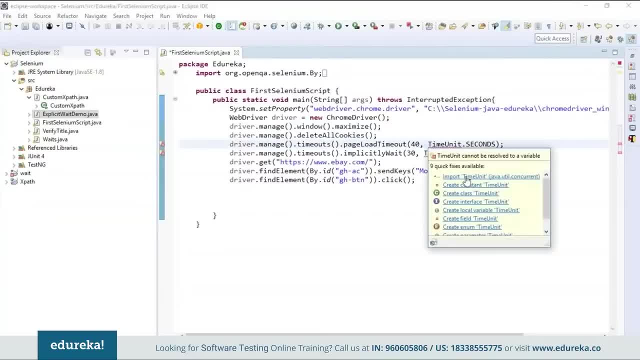 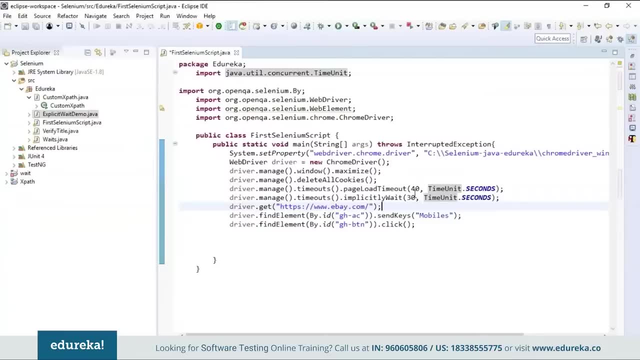 It's throwing an exception because I haven't imported the package. and one more thing I have said: the implicitly wait for 30 seconds, which implies it will wait for 30 seconds and listen until the element is loaded. That is this one. So even after 30 seconds, 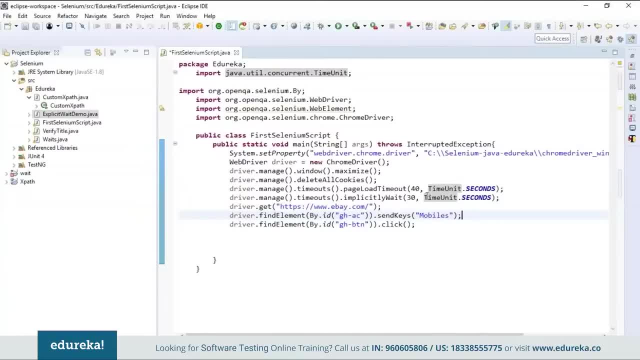 if the element is not loaded, then it will throw an exception saying no such element found. Okay, So that is the reason I'm using implicit weight. But if the element is loaded within first two or five seconds, then the rest of 25 seconds will be ignored. 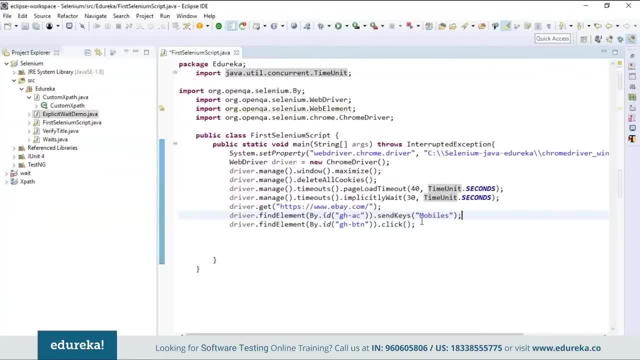 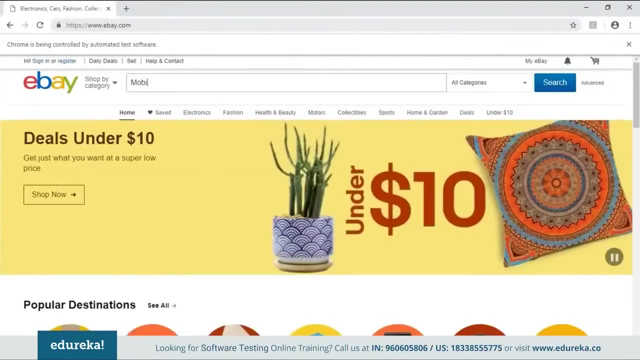 That is the reason. implicit and explicit weights- Both are called as dynamic weights. I'll explain you explicit weight Also. don't worry, for now Let's run the program and check the output. As you can see, Chrome driver launched Google Chrome, maximize the window and opened ebaycom. 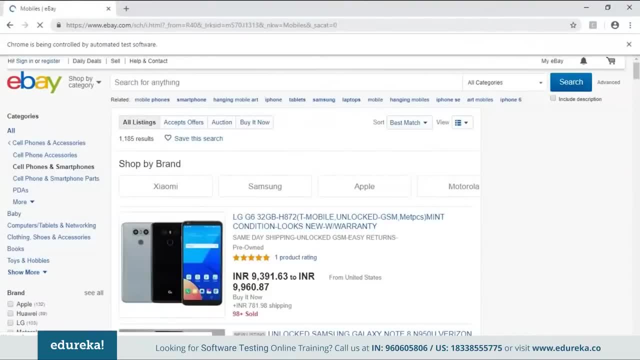 You can see it entered mobiles by itself, Loaded and gave the output as desired. Correct Sounds much interesting, right? Everything is an automated, correct? Yep, that's true. Now Let's learn one more locator, That is, name simple instead of ID. 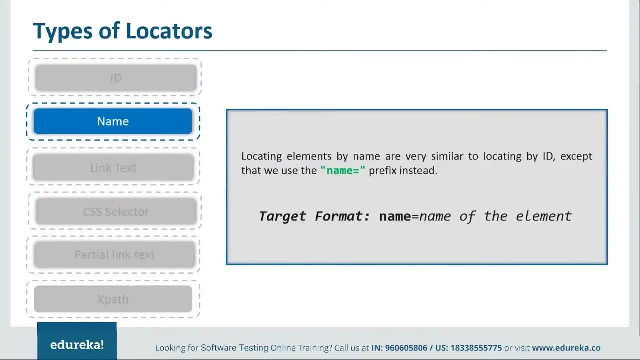 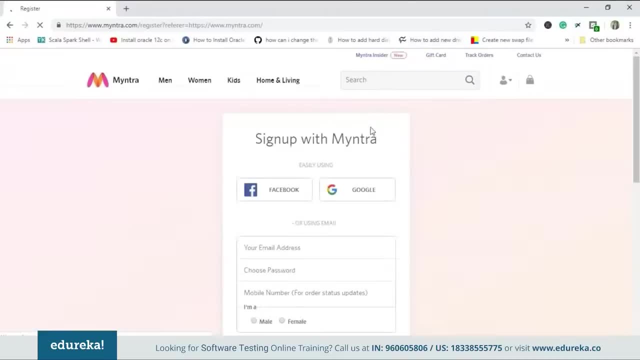 We have to use name, That's all. It's same like ID only, but we have to use name to locate a particular element is in name locator. I'll be using minthacom, say I want to do sign up and you can see here. 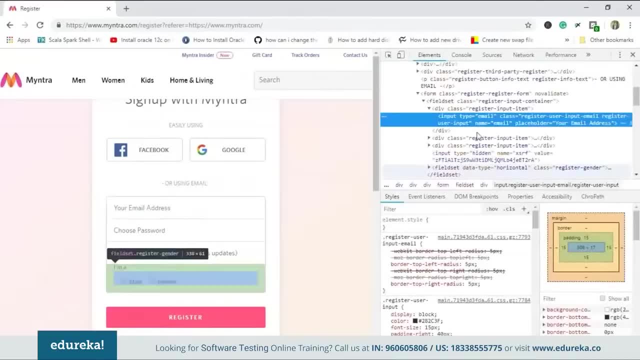 It has an email address tab. I'll just click on inspect and you can see it has element whose value is email. Name is an attribute whose value is email, Correct. So let's see how to do that. I want to sign up. 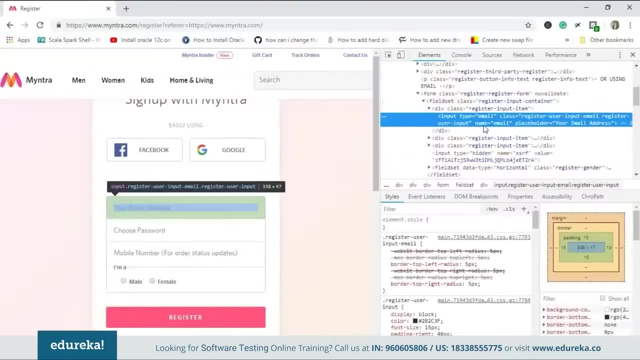 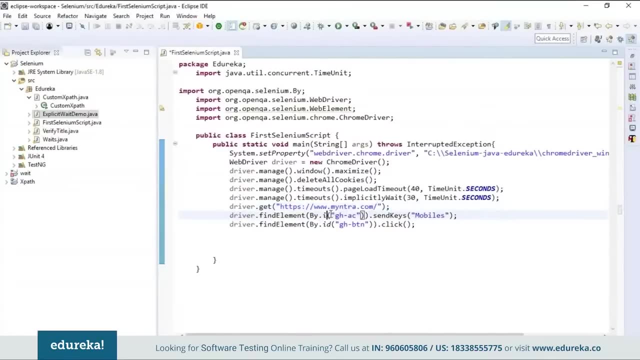 I'll inspect on this. You can see it has a name whose value is email. So I'll copy this and instead of by ID, I will make it as by name. So here by is a class and name will be your locator, or your web element or your locator. 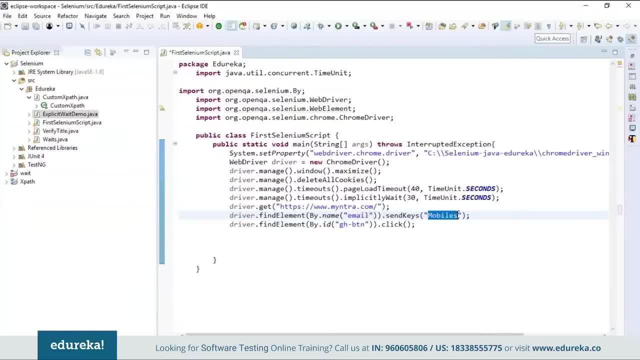 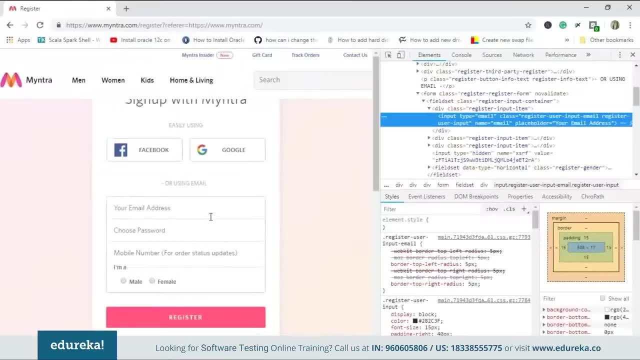 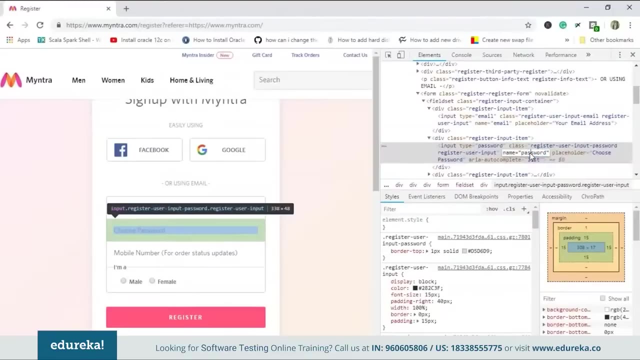 and I will paste the value. that is email, and I want to send email like something at Eureka at the rate gmailcom, my email address, and next I can also write the password as well. Even that has a name attribute whose value is password. So again, by name, I'll give. 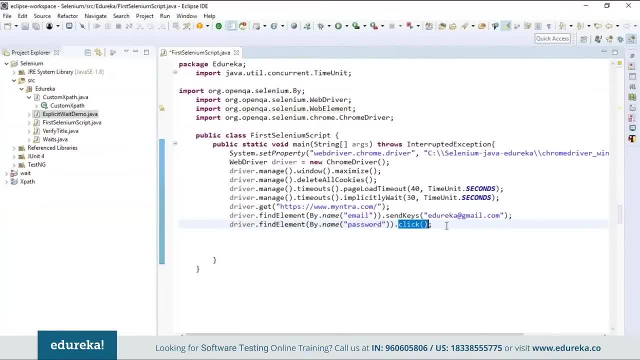 and I'll change this as password And I will send something like, depending on my choice- Sorry, it's capital K- Now, say, once I enter the email, I wanted to wait for two to three seconds and then enter the password. in that case, what I'll do? 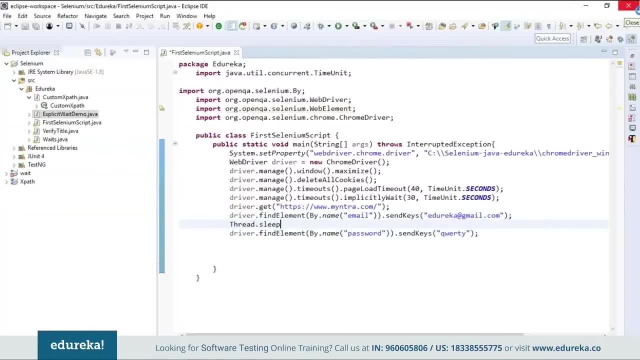 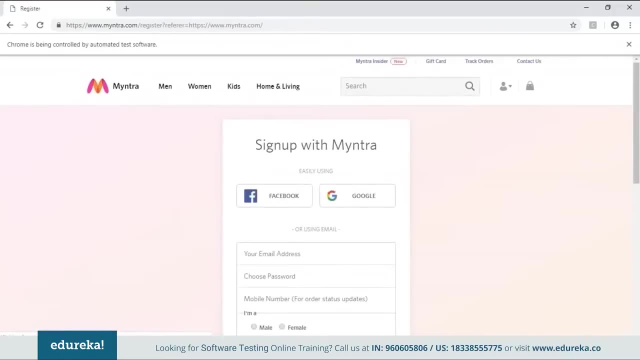 after the statement, I'll give thread dot sleep of 3000, which implies it will take three seconds only. Okay, so save this and run the program. So again, Chrome driver launched. Google Chrome navigated Through Myntracom to this page. 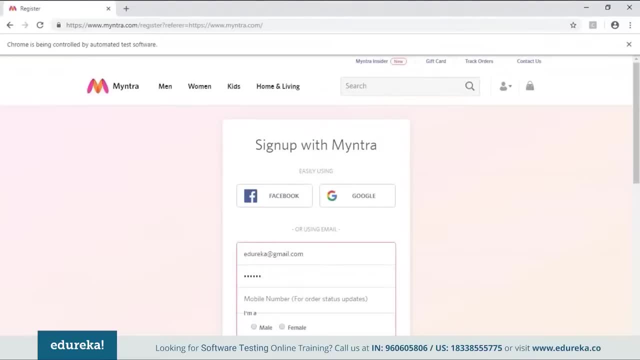 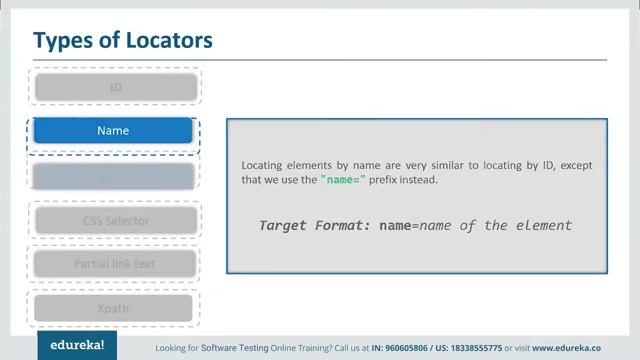 and it entered a direct either gmailcom, waiting for three seconds and then enter the password. Correct. As you can see, it is written as Chrome is being controlled by automated test software, Correct. So this is how you can use threadsleep in between the two elements and go on next. 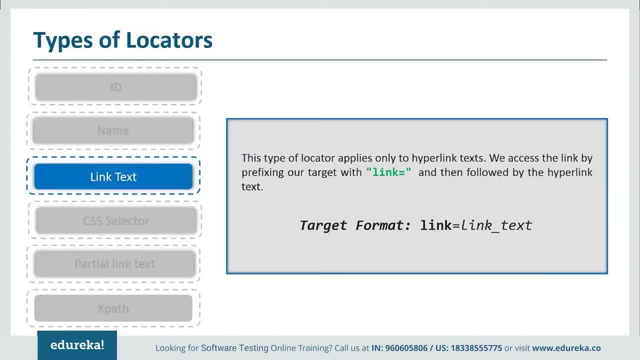 We have link text. that is useful only for links that starts with the anchor tag and H reference, And if something text is present in the link, then you can use this link text locator. and next you have CSS selector. It's very easy. So CSS is mainly used to provide style rules for the web pages. 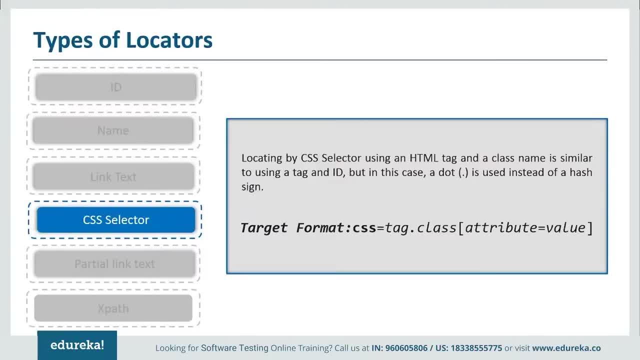 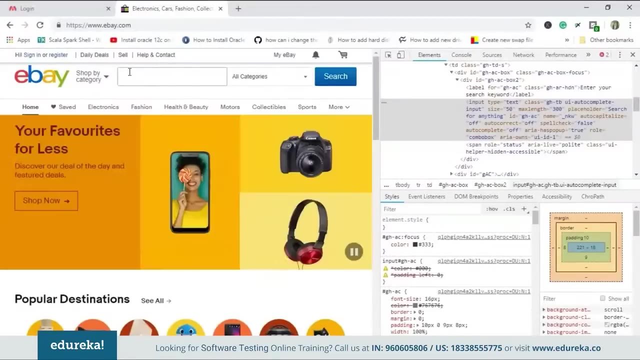 and we can use for identifying one or more elements in the web page using CSS. If you start using CSS selectors to identify elements, you will love the speed, So I'll show you one small example how to use CSS selectors. So to demonstrate CSS selector, say: I want to locate. 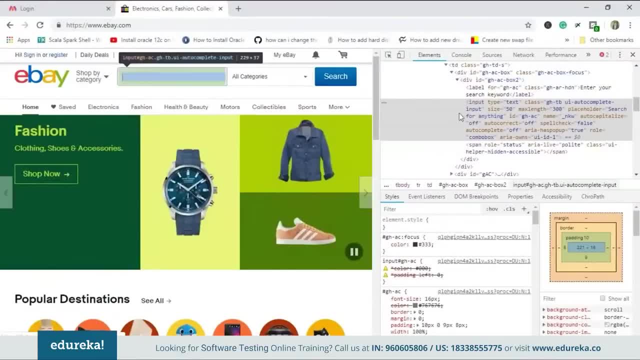 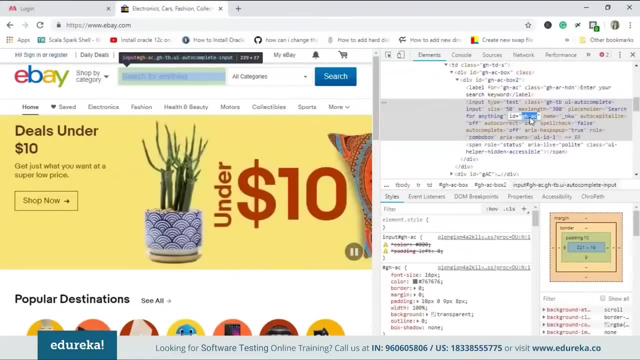 the search box using CSS selector. So I have inspected that and I have mentioned ID as a unique locator. So whenever you write anything, it will be with respect to ID. So I'll show you how to locate the element using CSS. Click on elements and click ctrl F. 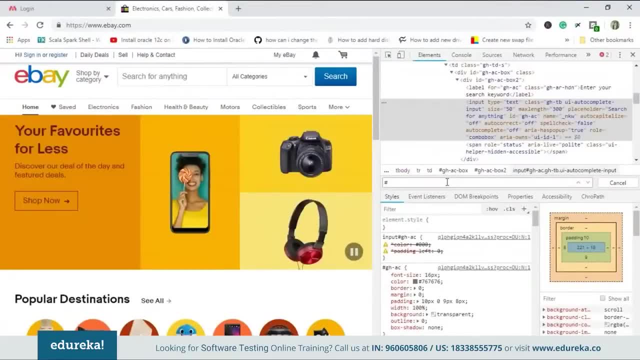 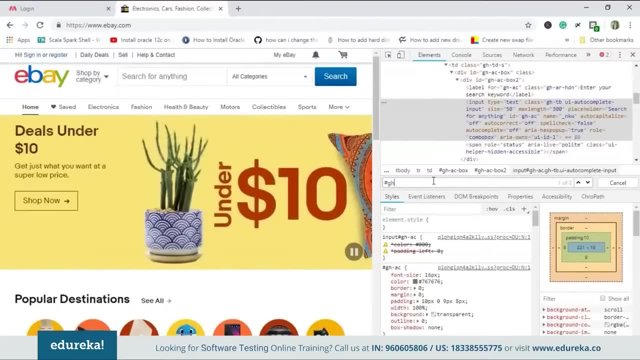 where you can write string selector or X path. and remember CSS selector always starts with hash. And what is the value of ID? It is gh AC, Correct, So I'll just give gh AC On writing that you can see. it highlighted the element. 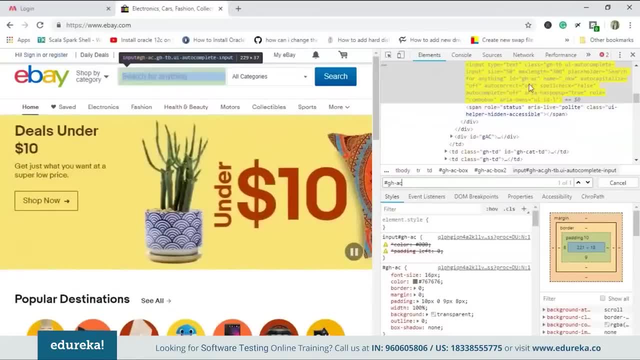 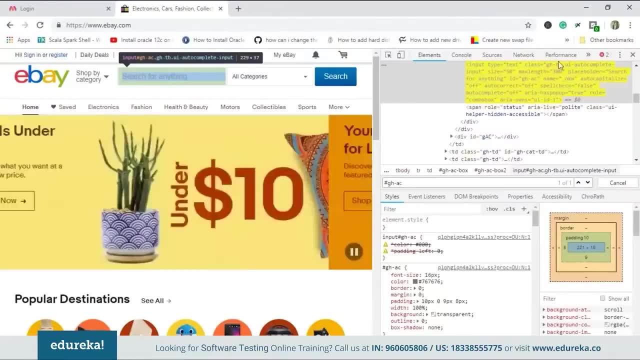 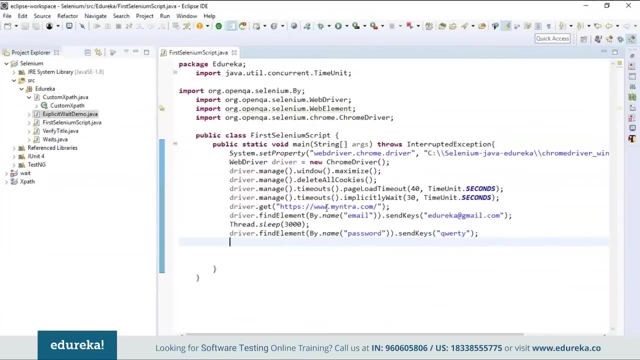 which implies it was able to locate the particular element using CSS selector. sounds much easier, right? instead of finding the name, your link text, everything, just write the ID value and you will be able to locate the particular element. Correct, Same thing. you can copy this and paste it over here. 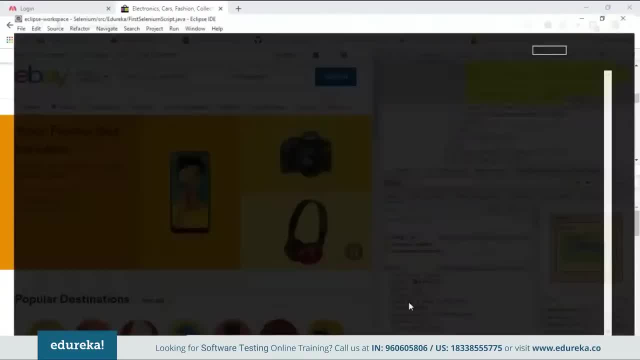 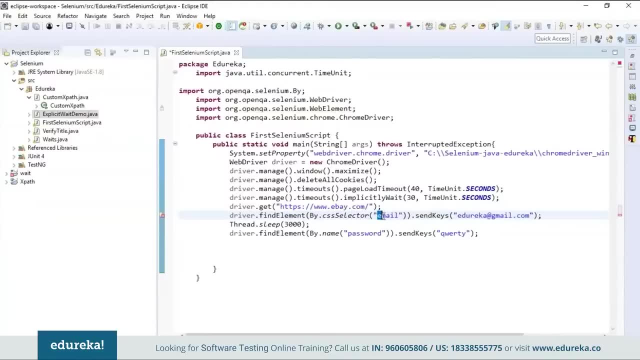 Sorry, I have to again change it to ebaycom first. I'm sorry here. I'll make it as by CSS selector, That's all, and I will pass the value as hash gh AC because that's ID value. Okay, something like no headphones. 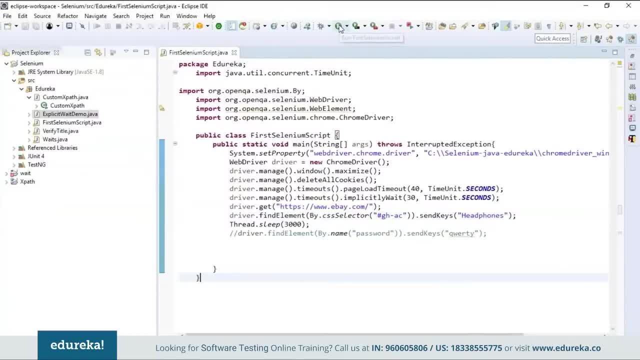 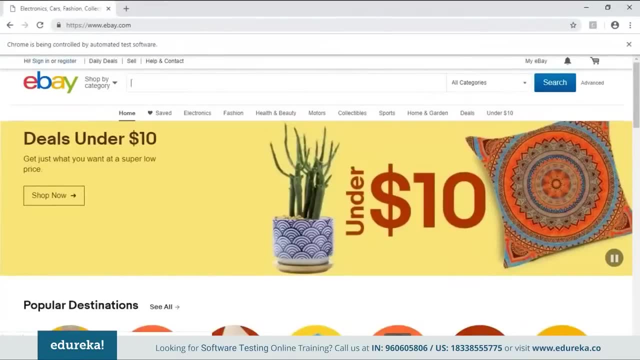 I'll comment this for now. save this and run the program Again. it launched Google Chrome, navigated through ebaycom and enter the value as headphones. as I did not click on the search, It's not taking. if you want again, you can click on the search. 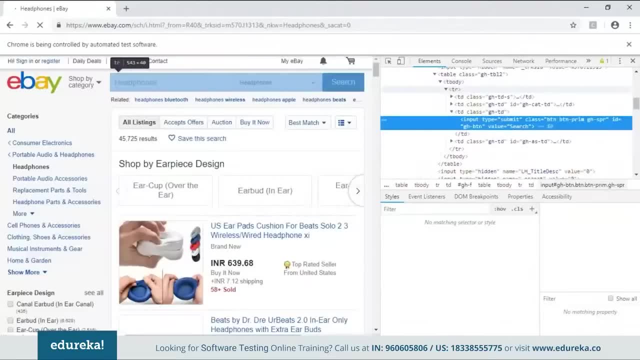 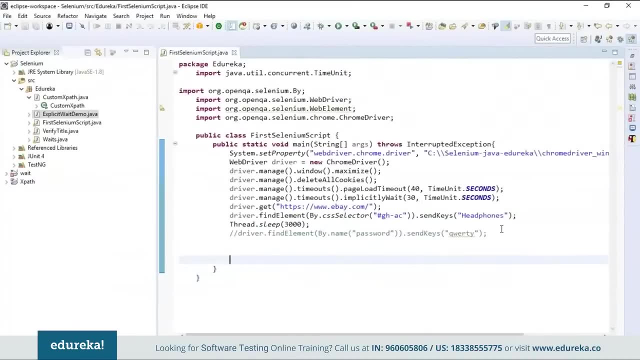 Search, inspect. copy the value, that is, gh button, this one- and you can paste it over here and choose click method, because you're clicking on the search box. So that's how you can use CSS selectors as well. Next will be your partial link text. 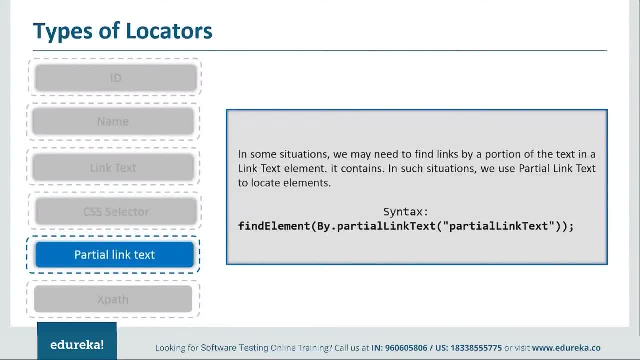 So, if you know, some situations we may have to find the links by a portion of the text and that it contains, because you know proper text will not be there. in such cases We can use partial link text to locate the elements. and now talking about my favorite locator, XPath, 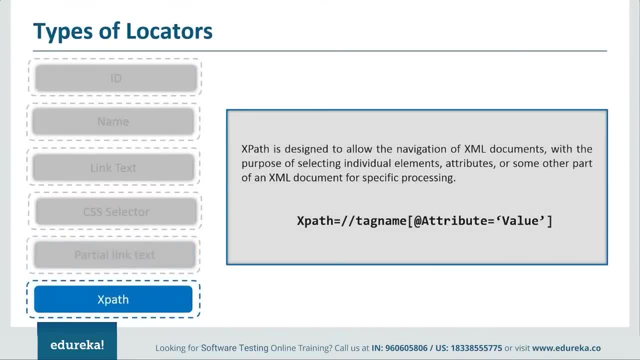 It is designed to allow the navigation of XML elements with the purpose of selecting individual elements, attributes or some part of an XML document for specific processing. So syntax goes like this: It has double forward slash: a tag name at select attribute and attribute name, followed by attribute value. 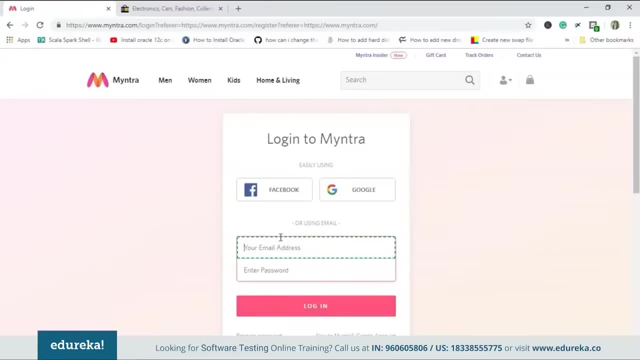 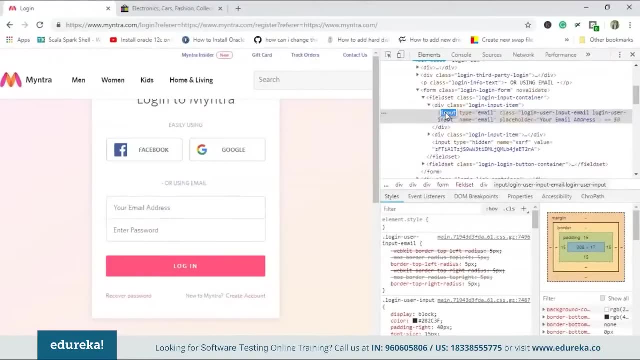 I'll show you a simple example of using XPath. Let's take mantra and try to locate this login information. As you can see here, it has an input tag and it has a placeholder whose value is your email address. So I'll write it over here only. 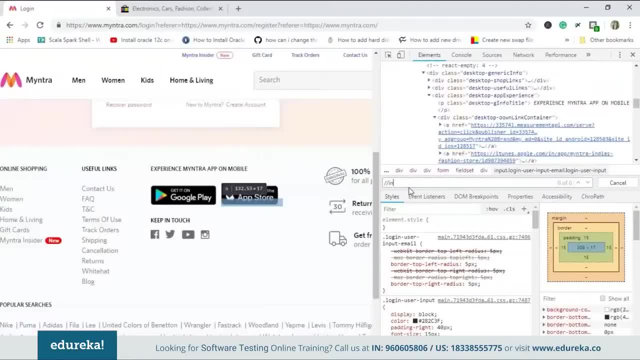 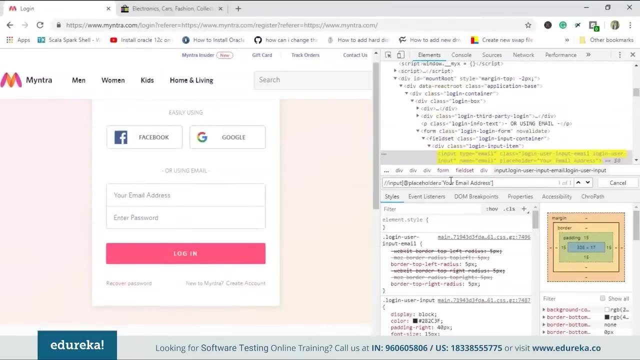 as I have told, it starts with double forward slash. I'll give it. and it has an input tag, Okay, and it also has a placeholder whose value is your email address. So I will place the value and your value should be within single quotes. 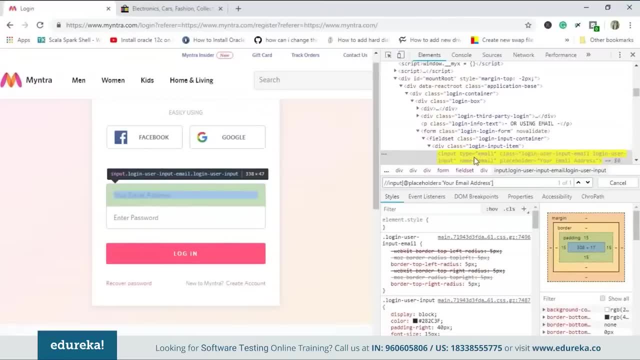 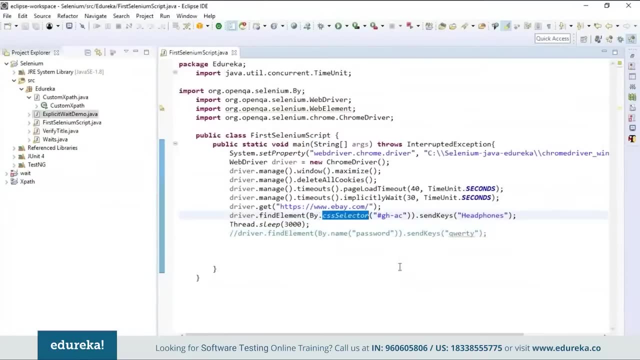 on writing this. You can see it was able to locate the particular element. So now say I want to write it using XPath, I'll copy this XPath and write it over here and I'll send keys like some email address. So just run the program and check the output. 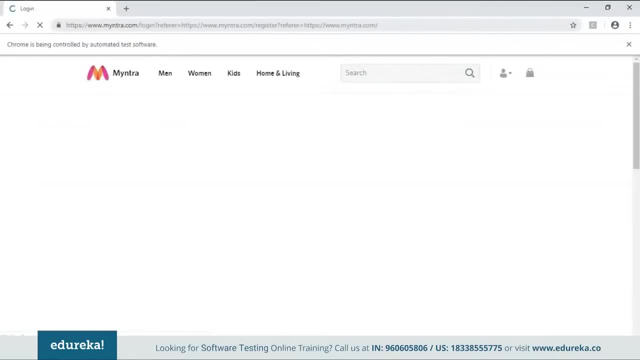 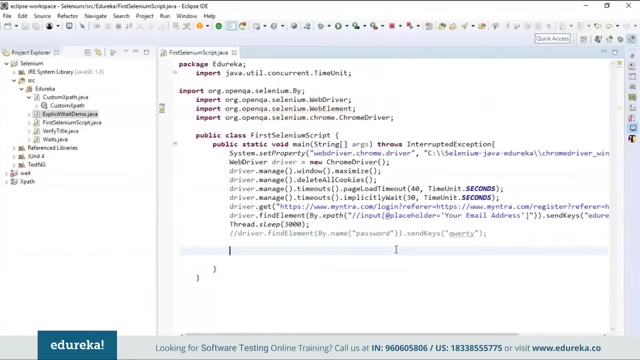 It launched Google Chrome. That is, your Chrome driver launched Google Chrome navigating through mantra, and it will write the prescribed email address. Okay, so this is how you can use XPath to locate a particular element on the web page. Sounds much easier. So this is how, basically, you can use different types. 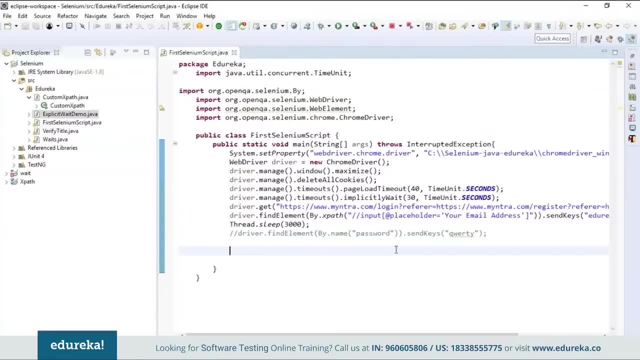 of elements to locate a particular element on the web page, and you can use implicit and explicit weights. Yeah, when I talk about explicit weights, I show you how to use it. Now I want to use yahoocom and I'll explain you explicit weights. 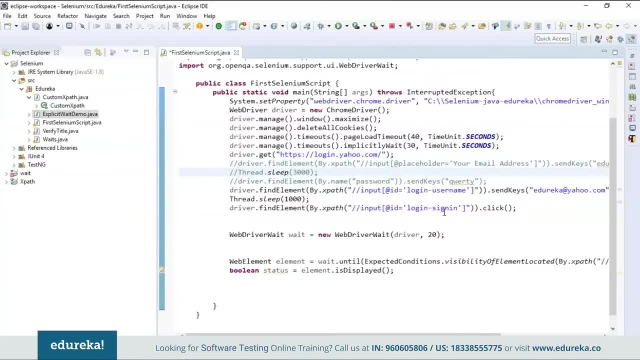 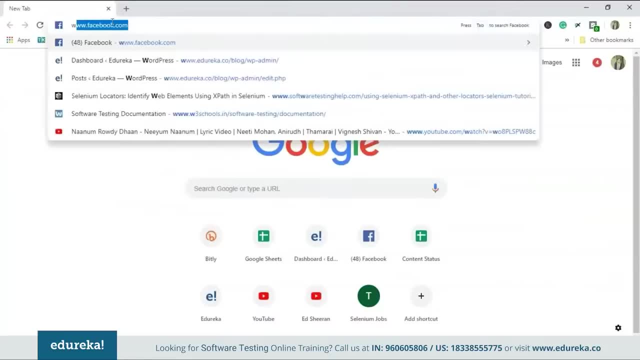 Okay, so I have given the XPath for login username. I'll show you how you can even use for this also, no issues, but. but I want to make you comfortable with different websites, So I'm just showing that. So when you click here, 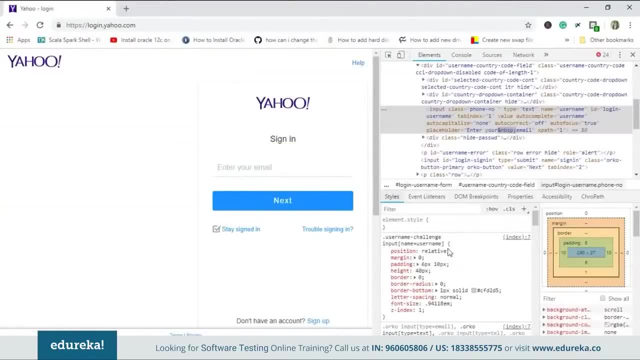 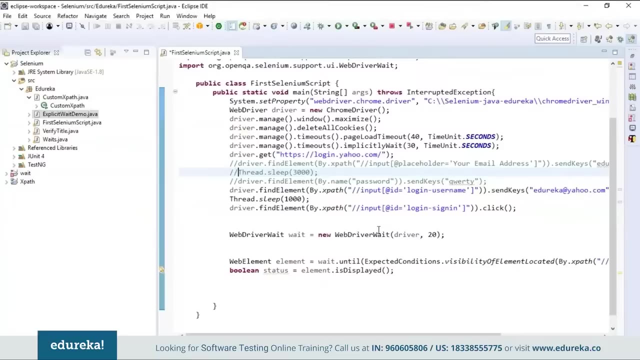 I inspect on this and I will write the XPath. I can give the XPath for this because it contains an ID whose value is login username. So same thing I have given over here. That is ID. That will be your username And send keys as a direct direct yahoocom. 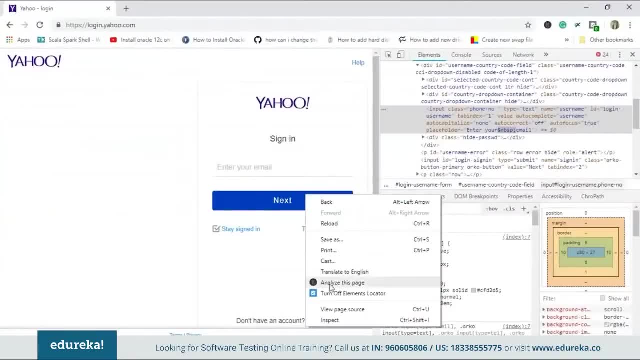 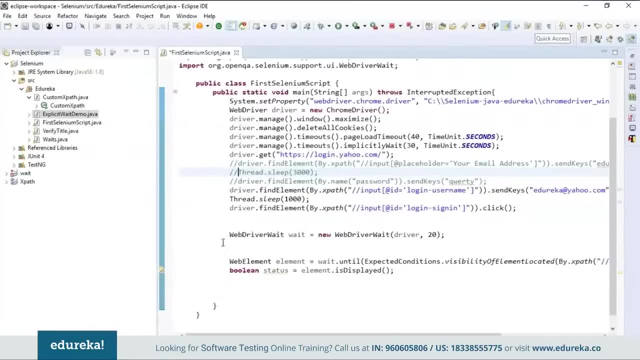 and it has a click button. That is this next button. again, It has an ID attribute whose value is login- sign in. So, based on that, I have written these two statements and I have used a web driver weight. Explicit weight is always achieved using web driver weights. 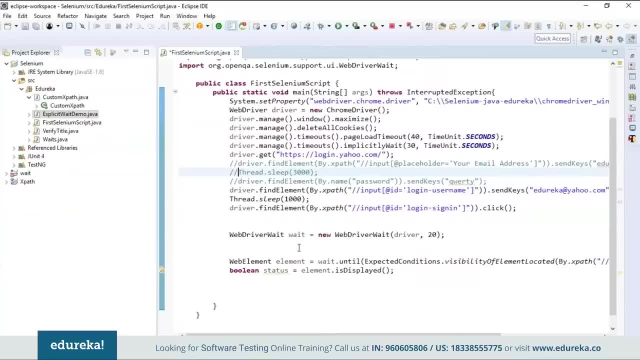 Okay, it's a concept of the dynamic weight which weighs dynamically for specific conditions. It can be implemented by web driver weight class. It doesn't have any keyword like explicit weight, as it has for implicit. We can simply give web driver weight. So here I am creating an object of weight. 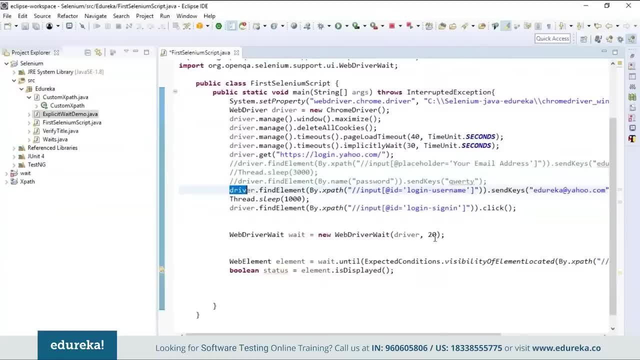 and I'm sending my driver. that will be this and I'm giving explicit weight as 20 seconds, and then I'm creating a web element and asking it to wait until expected conditions is visibility of the element located by XPath. that is login username. That will be your email box. 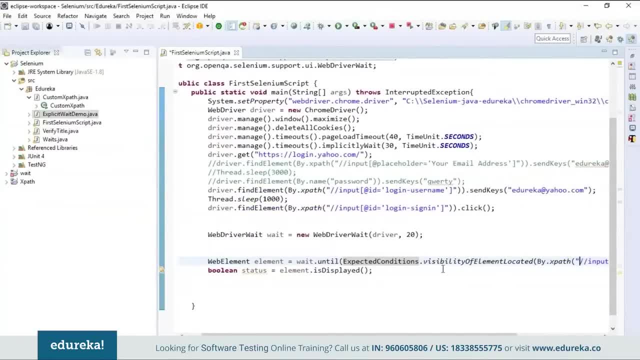 So it will wait until the expected condition says visibility of the element that is located by the sex path. simple, So save this and you can run the program and check the output. So there are many visibility conditions. like you have element to be clickable, element to be visible. 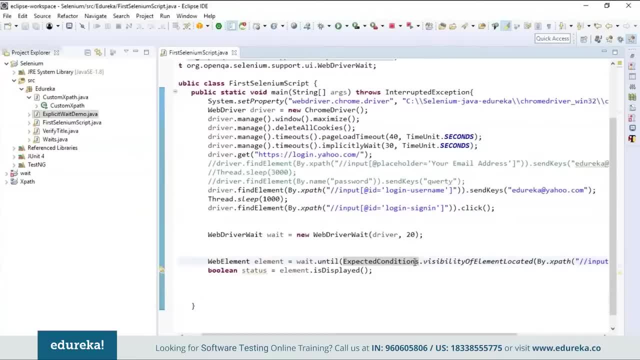 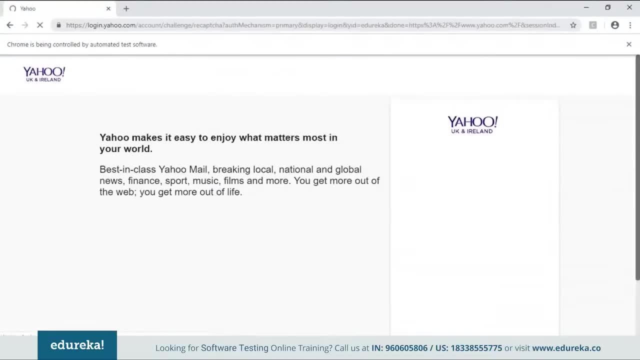 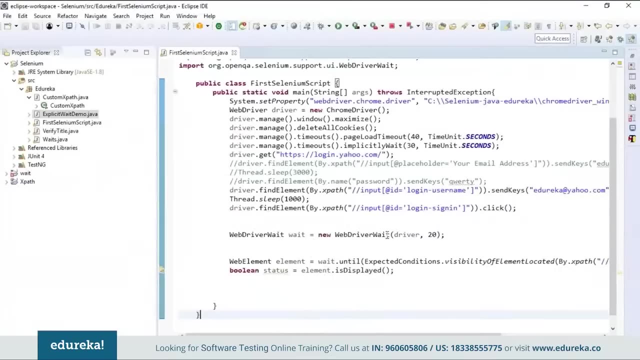 URL to be located and many more. as such, You can simply give control and shift will get to know. Let's see how the output will be. So it entered at you record the rate. yahoocom asking to move to next correct. So as it is explicit weight. 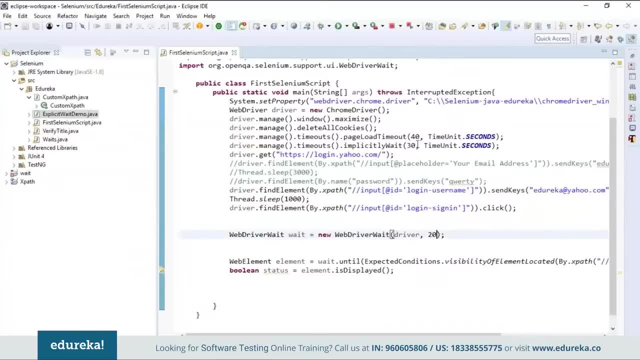 we can change the timings accordingly. but implicit weight- one set cannot be changed as it is a global weight and it can be applicable to the entire program. But for web driver rate, that is your explicit weight. You have to keep on creating a web driver rate. 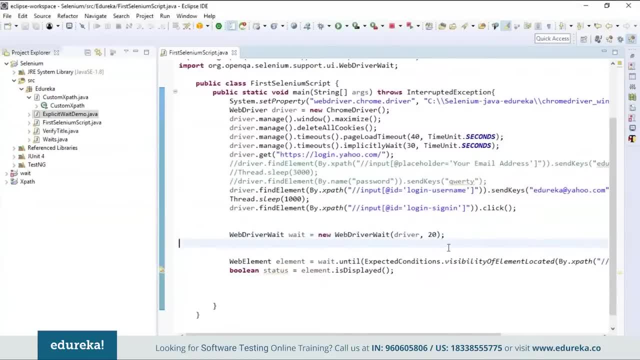 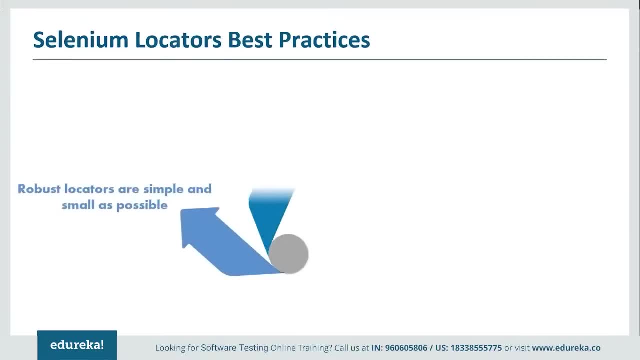 for specific elements. So it goes like that simple. So these are some of the best practices for locators. that is, they are simple and small as possible and they work Even after you change the properties of UI element. and they work even after you change the properties. 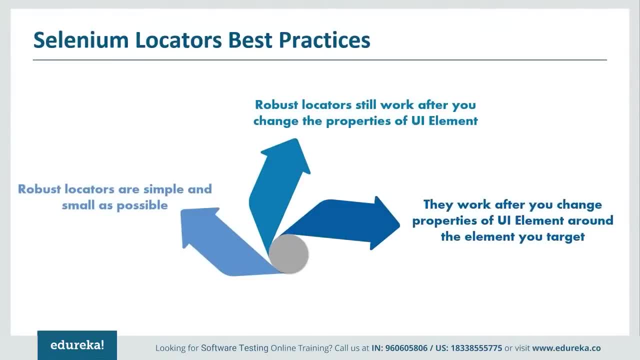 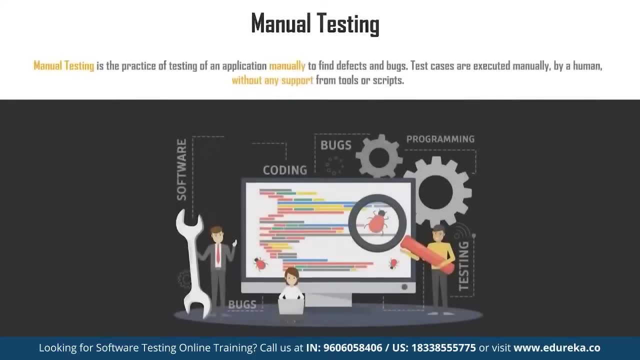 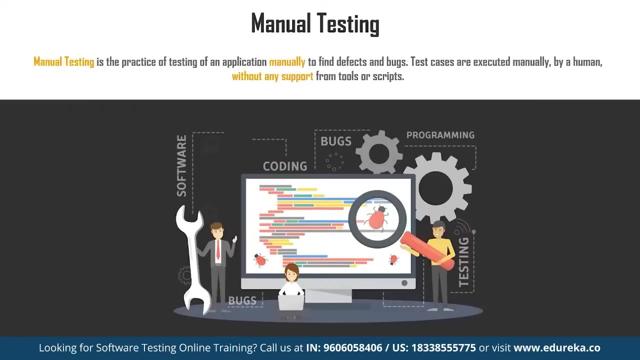 of UI element around the element you target sounds much easier, right? Manual testing means testing of an application manually by a human. a tester performing manual testing ensures that an application is working properly by following conditions written in test cases. This means that someone actually goes on a device. 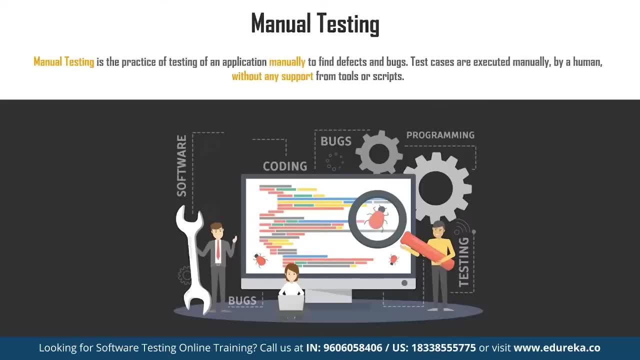 to evaluate numerous components like design, functionality and performance by clicking through multiple elements of the application. Manual testing is really helpful when automation testing is not possible. Let's say, if you want to test a mobile application under unpredictable conditions, you can use manual testing, like when mobile application is running. 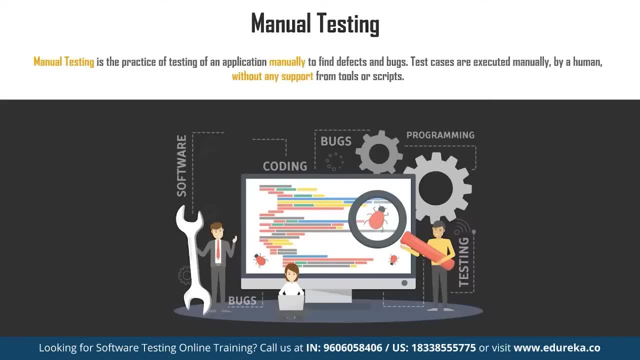 when the phone is in users pocket and there are many unintentional taps. So what will happen when such scenario arouses? the testers simulate condition to check whether this will lead to crashing of the application or not. Well, you can't apply automation there, right? 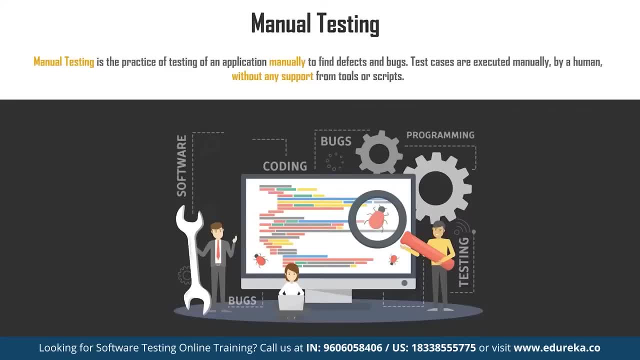 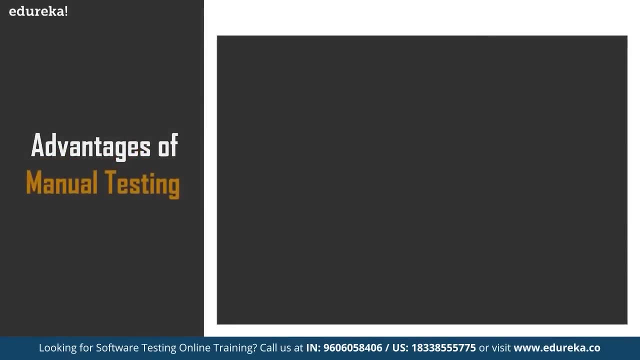 So that's when manual testing becomes handy. So basically, the entire testing process is executed by a human here. This manual testing has a lot of advantages. Let's take a look at few of them. First of all, with the manual testing, testers can test. 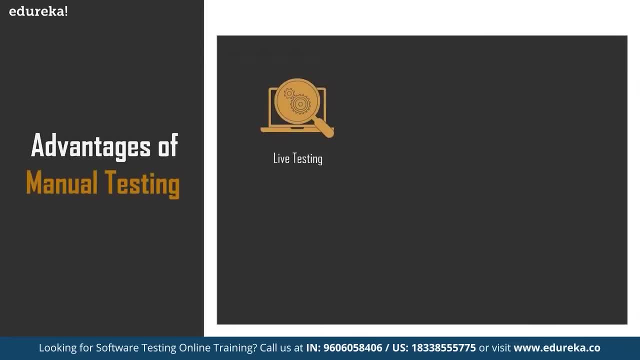 the application under similar conditions when the application goes live. any bugs or glitches or errors which occur when the application is live I can be easily tracked with help of manual testing, so we can call it life testing. and secondly, in manual testing less programming knowledge is required. 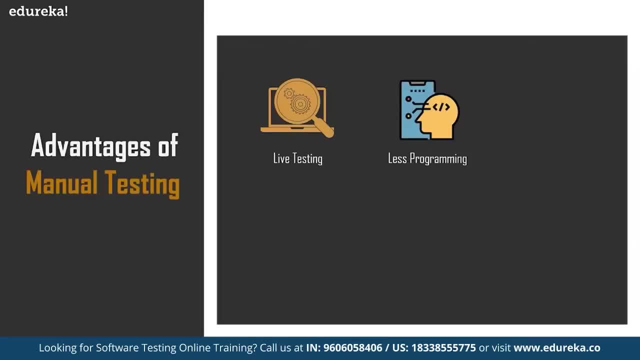 Basically, when you're testing an application manually, the main focus is on understanding the requirements, documenting the test cases and executing test cases as you're performing them as life, So your focus on programming is usually less after that. automated tests are quite literally robotic: They fail to act. 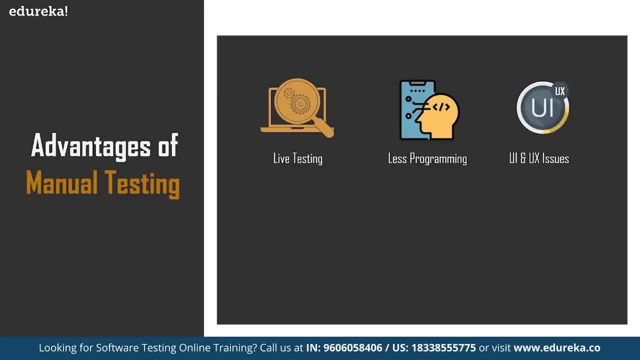 as a real end user world. but manual testing helps tester to identify any issues related to the look and feel of the application. It also helps to find out the usability issues in the application, any bugs and effects that may pop up as soon as user handles the given software. 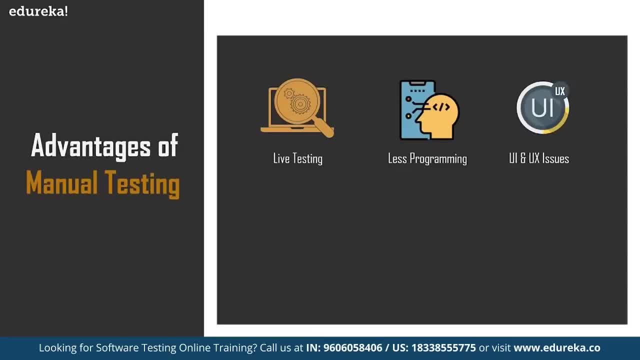 in a certain way, are more likely to be wedged with help of manual testing. So in case of visual testing, manual testing is really helpful. Manual testing requires low investment and it doesn't require any costly Tools or high-level skills to perform. So what I mean to say is: 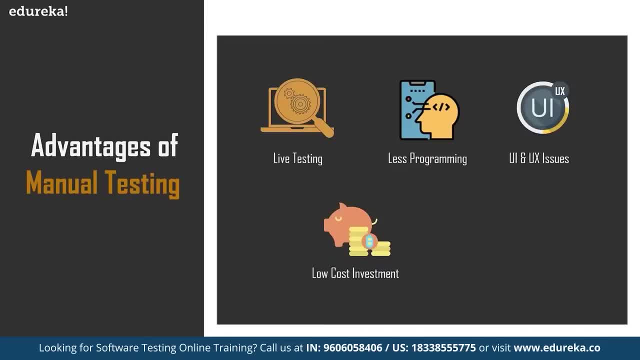 that initial investment in manual testing is very low and manual testing is cost-effective in short-term scenarios. Lastly, in manual testing you can swiftly test and see the outcomes, So it's well suited in case when you're making a lot of unplanned changes to your application or software. 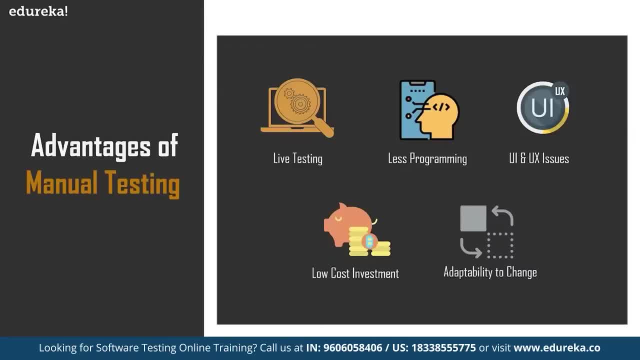 and application needs to be tested immediately after implementing the changes. in such cases, Manual testing is really helpful. So these are few advantages. now that we know what we can benefit from manual testing, Let's go ahead to our next topic. So when you begin testing one of the primary decisions, 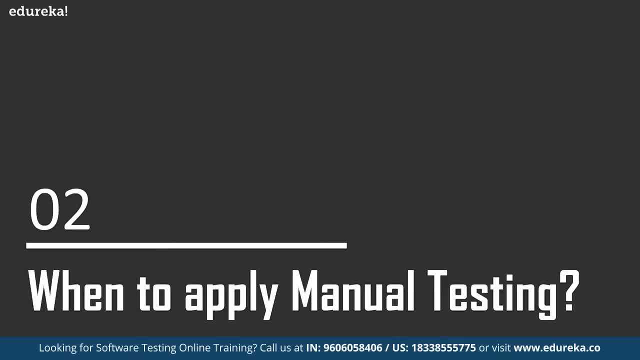 that you'll have to make is when you're going to test manually or if you're going to use automation testing. Well, neither of these options are technically better or worse when compared to other. the features like size, budget, time, allowance of a project will certainly be the factors. 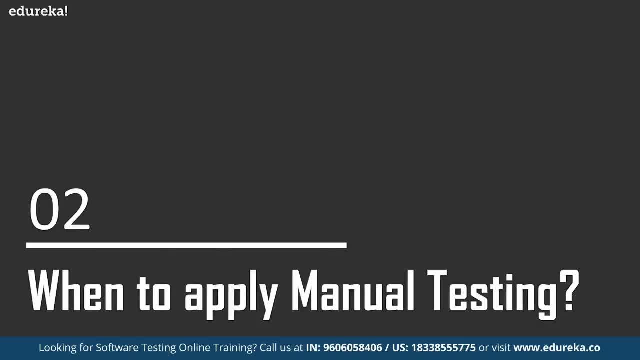 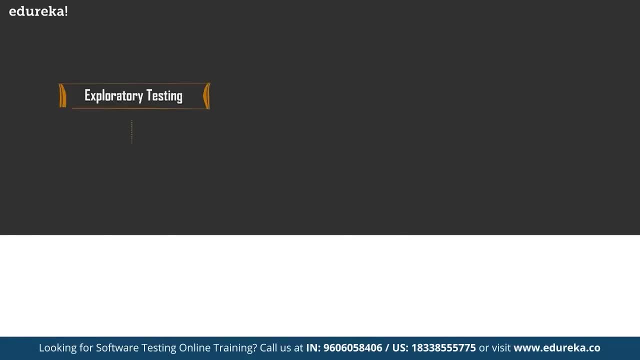 that affect which method you'll choose. So you should know when to choose manual testing right. Let's take a look at few scenarios Where you can apply manual testing. The first such scenario is exploratory testing. Well, exploratory testing is carried out by domain experts. 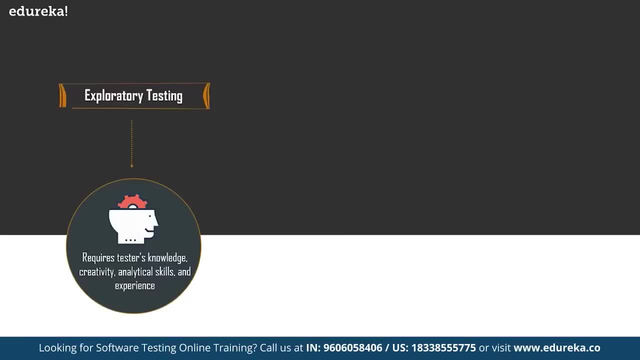 So this type of testing requires testers knowledge, experience, analytical skills, logical skills, creativity and intuition. here, test is characterized by poorly written documentation or a short time of execution. So basically, we need the human skills to execute the testing process in the scenario. So manual testing comes to rescue while working. 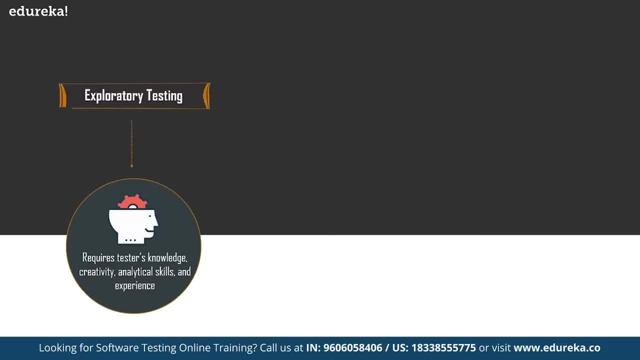 with poorly written documentation And if there's a shortage of time. this approach- basically that's exploratory testing- requires minimal planning and maximum test execution, which is possible if you choose manual testing. So this is one scenario where manual testing is really helpful. after that you have usability testing. usability testing helps. 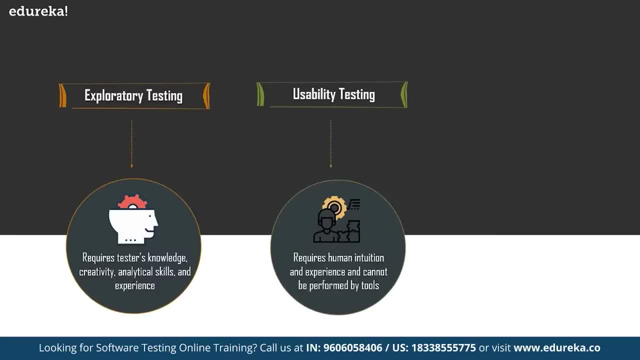 to find out the user friendliness of an application, as the name indicates. So this is an area where you need to measure how user-friendly, efficient or convenient the software or the product is to end users. So, basically, human observation is the most important factor. 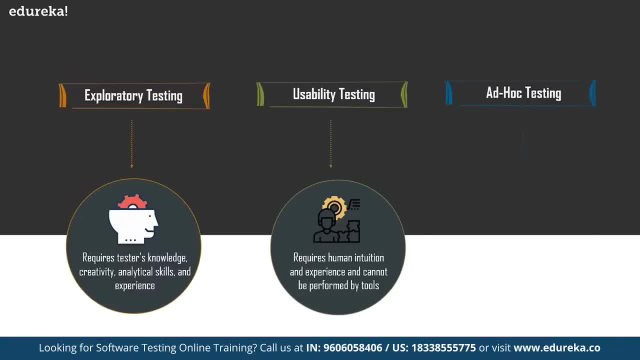 So a manual approach is preferable. Nextly, you have ad hoc testing, So, as the name suggests, this type of testing does not follow any fixed method or approach. you can say: Well, that's why it's called informal type of testing. in ad hoc testing, testers randomly test application. 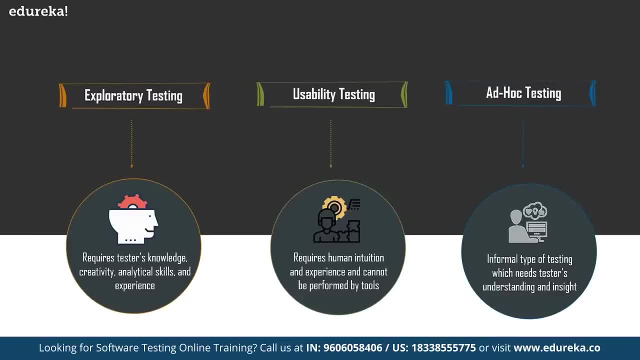 without following any documents and any test design techniques. So understanding and insight of a tester is a very important factor. Naturally, manual testing is preferable here as well. Well, these are three main scenarios where manual testing is preferred over test automation or automation testing. 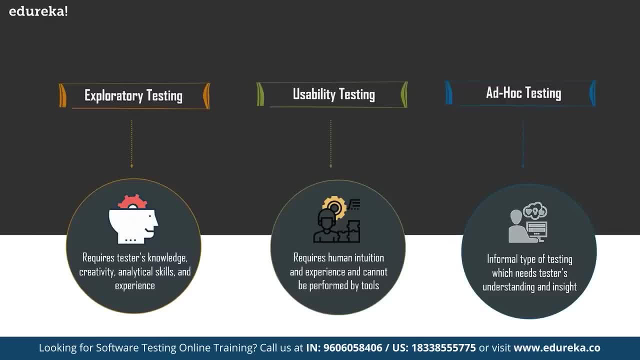 What are those exploratory testing, usability testing and ad hoc testing? apart from these, when should you choose manual testing over automation testing? when the project is usually in the initial development stage? when testing user interface, especially with visual aspects, while if there's a short-term project, mainly? 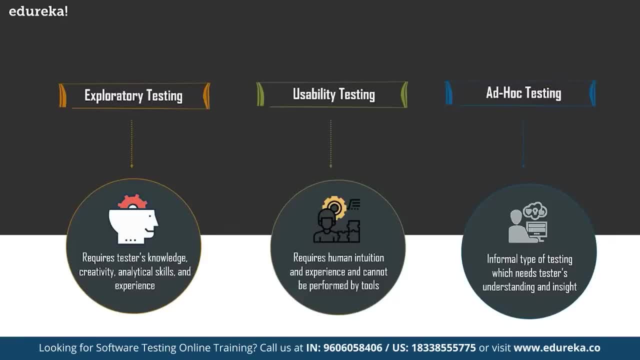 and the writing scripts will be time-consuming. in such cases, you can use manual testing instead of going for automation. Well, after that, the next question that pops out is: is there a specific procedure to perform manual testing? Well, yes, the process is kind of similar to any testing process. 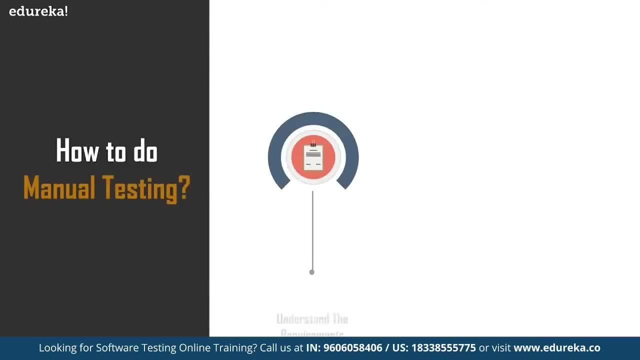 Let's take a look at it. So the first step is understanding the requirements. So in order to successfully conduct manual tests, you first need to understand the requirements of the software. So by understanding the requirements, you will know what needs to be tested. 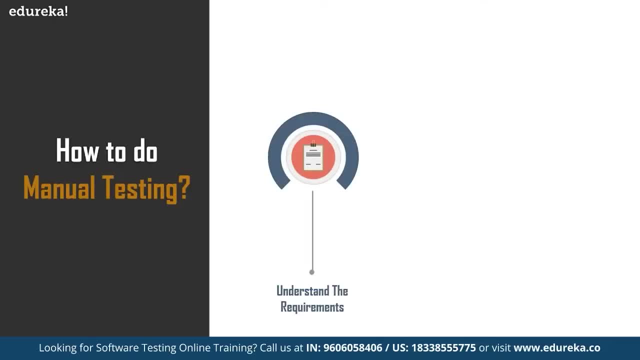 and what classifies as a defect or bug. So that's the crucial part of manual testing. His main goal here is to make sure that your software or application doesn't have any bugs. The next step is writing test cases. So once you understand the requirements, 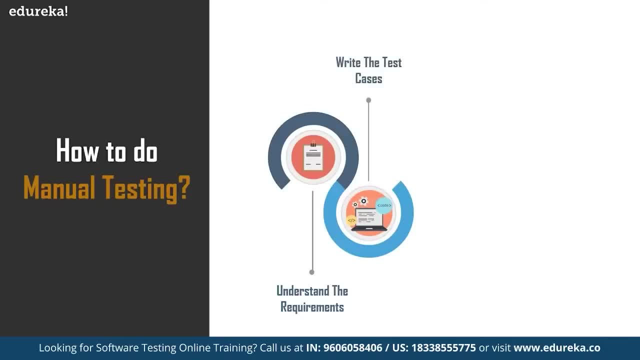 you can write test cases. That's another crucial part of manual testing. These test cases basically guide you through a sequence of tests to test functions and different scenarios written within software application, And remember that writing good test cases is important as they make executing the test go very smoothly. 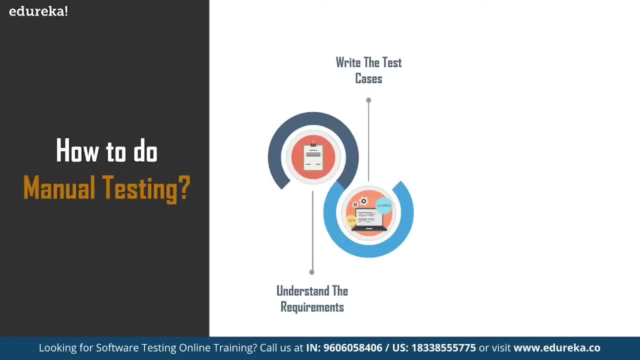 and enjoy good test coverage. So once you're done writing test cases, the next step is conducting the test. So once your test cases are written and test environments is properly prepared, It's time to begin testing. You can follow the test cases and mark each test as passed, failed or skipped. 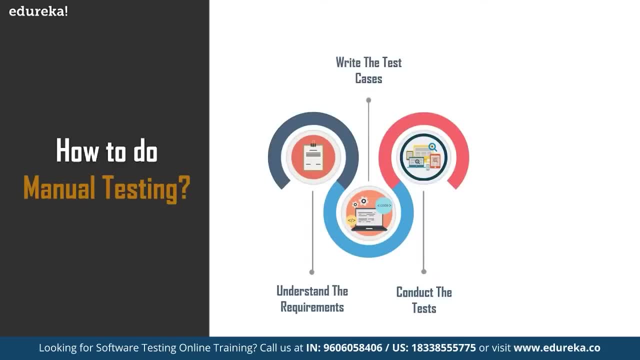 when doing manual testing, It's important to keep notes on what happens when a test fails. That's really important. You can't ignore that fact just because your test failed. The fourth step is to log good bug reports. So, in addition to actual testing as a tester, 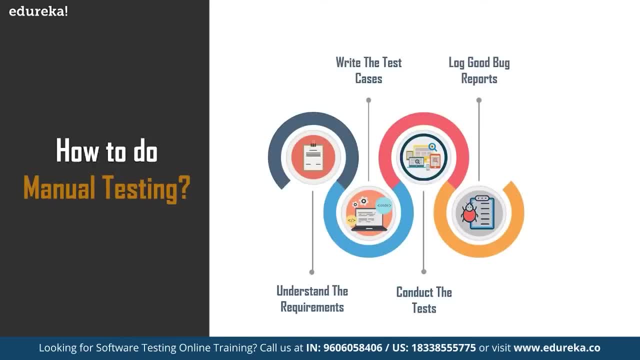 you'll be responsible for logging Bucks as well. So as you encounter Bucks you need to inform log information for the development team about the defect. So writing good bug reports will help you and your team later. You will save yourself time when answering these questions about the Bucks later. 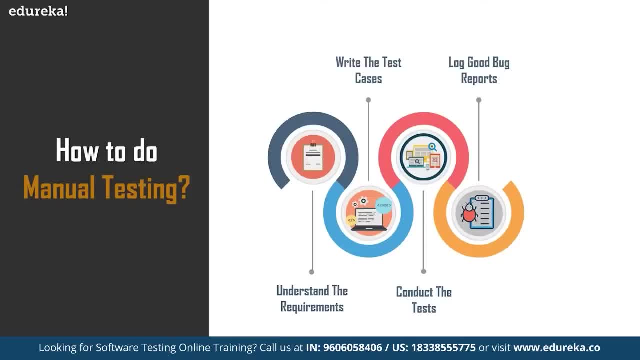 So, basically, you have a document that you can refer to at its code. a good bug report should have a strong title, steps on how to overcome the bug, expected and actual results and any relevant attachments that will help the development team to understand the issue of the bug, like screenshots. 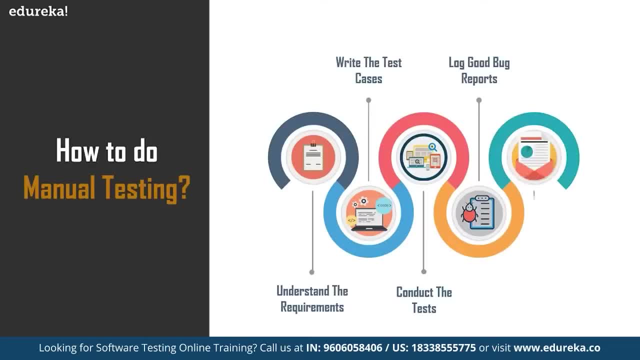 or recordings or export files as such. So, lastly, you need to create a detailed test report. after running test. It's good to know the results of the test at very high level, like how many tests were run, how many tests failed, how many was kept. like that pretty straightforward process. 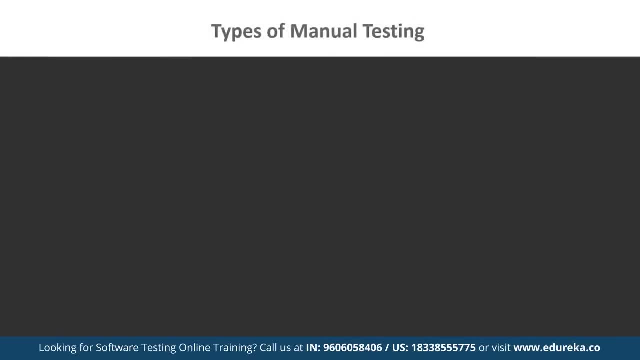 right. Well, with that done, Let's move on to our next topic, Which is different types of manual testing. It's basically divided into six types, But again, these types of testing can be carried out either manually or using a test automation too. 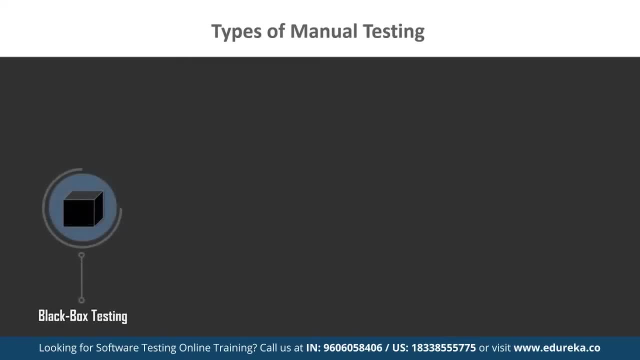 So let's start with the first type of testing, which is black box testing. in this type of testing, The tester does not have any knowledge about the code or the structure of the application or software that is testing. He just interacts with the application and test the functionality. 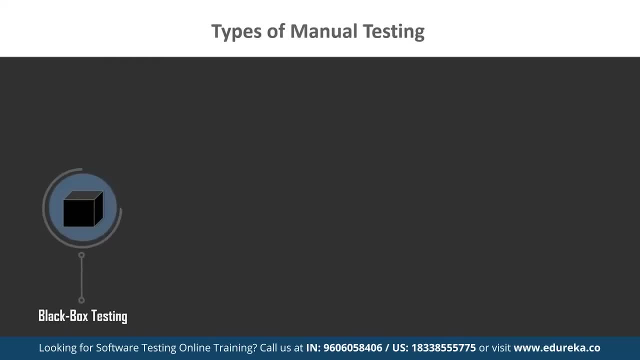 and the non-functional behavior of the application. Well, there are various black box techniques that can be used by the tester to find box and defects. Next is white box testing. So, as the name suggests, in white box testing the tester knows about the code. 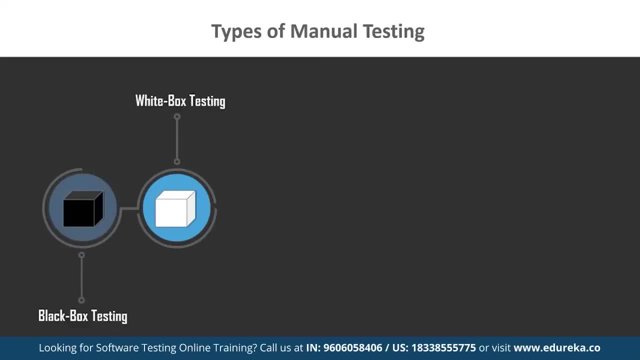 and structure of the application. for that reason It's also known as glass box or transparent box testing. Mostly this type of testing is used by developers to perform unit testing. There are various white box testing that can be used by tester to find box and defects. 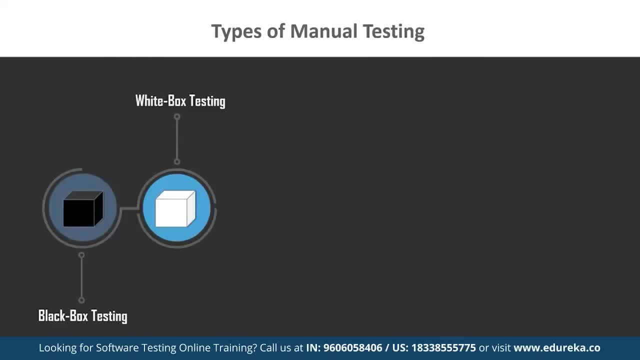 like. you have control flow testing, Data flow testing, then you have branch testing and then statement testing, decision coverage and path testing and many more. apart from black box and white box, You also have something called gray box, which I haven't listed here. It's a part black box and it's part white box. 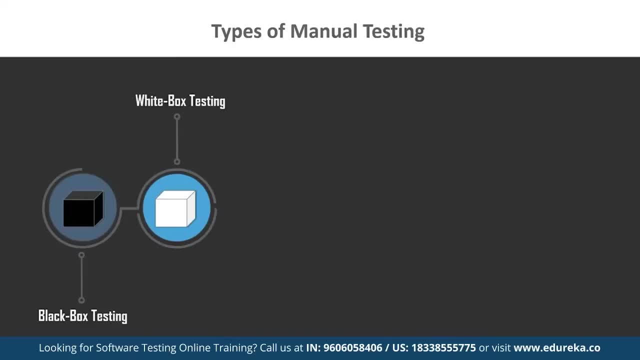 So, basically, you have information about certain factors of an application and you don't have information about certain factors that we call gray box testing. The next type is unit testing. You can call this as first level of testing. It's a way of testing the smallest. 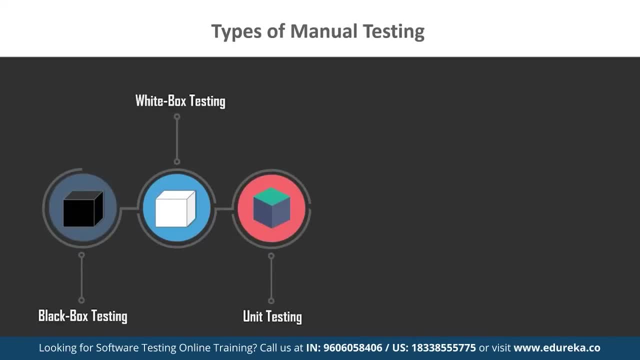 piece of code which is referred to as unit. This unit can be logically isolated in a system. Well, it is logically isolated in a system. It's mainly focused on the functional correctness of the standalone modules. You can say so. unit can be almost anything. 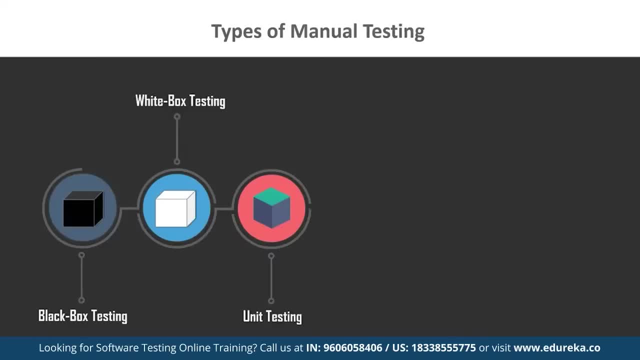 It can be a specific piece of functionality, It can be a part of your code or a program, a particular method within the application. It can be anything, a unit. So this unit testing uses white box testing methods or techniques and usually performed using a preferred 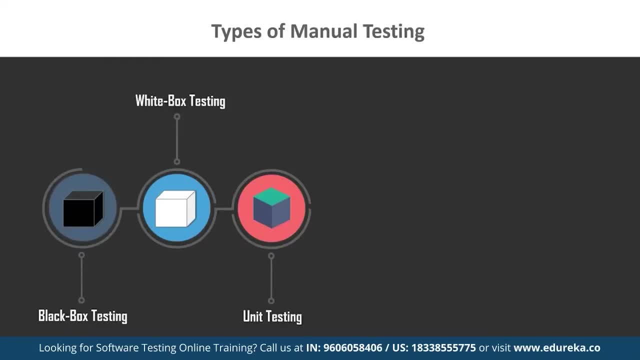 programming language of your choice. It's essential for the developers to unit test the software before handing it over to Q 18, because unit test offers several advantages or benefits. It makes your code reusable as you need to use a modular approach or as you're using modular approach here. 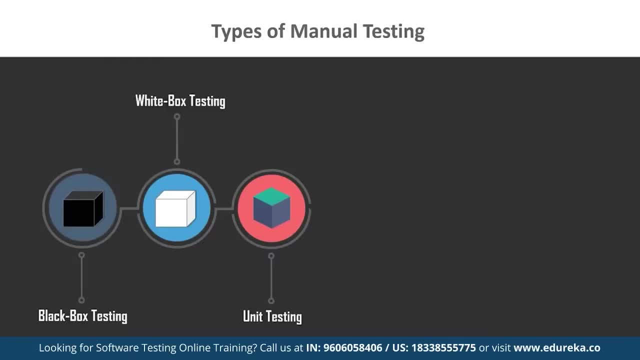 It also makes debugging a lot easier. So, basically, unit testing is performed before moving on to next stage of testing. So what's the next stage of testing? you have integration testing. It is performed after unit testing where different units, modules, components of the software or the application. 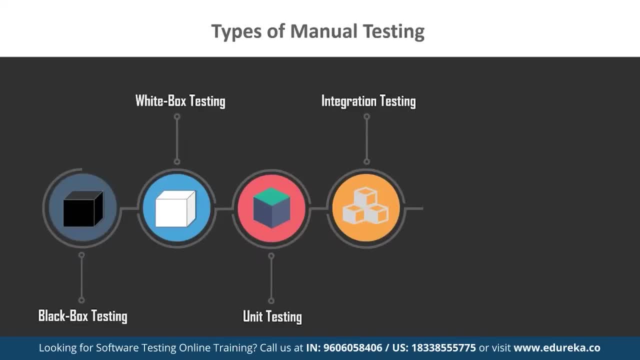 that you're testing on are integrated or combined together. as you can guess from the name itself, The main purpose here is to verify the functionality, stability and the reliability of the modules when they are combined together. The main focus of integration testing is to check the correctness of communication among all these modules or units. 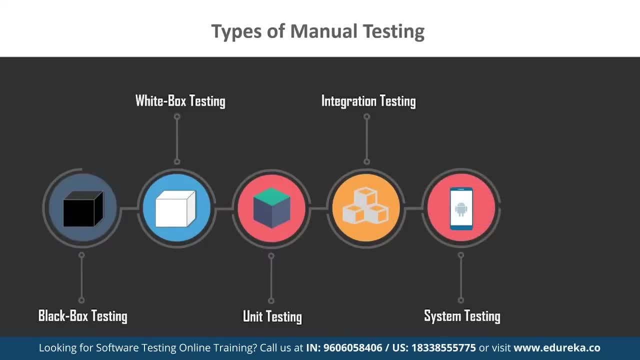 Next up we have system testing. system testing is the next natural step after integration testing. It's carried out on a complete, fully integrated software product to evaluate the behavior of the system in our entire fashion and then to examine how the full working of an integrated software computer system. 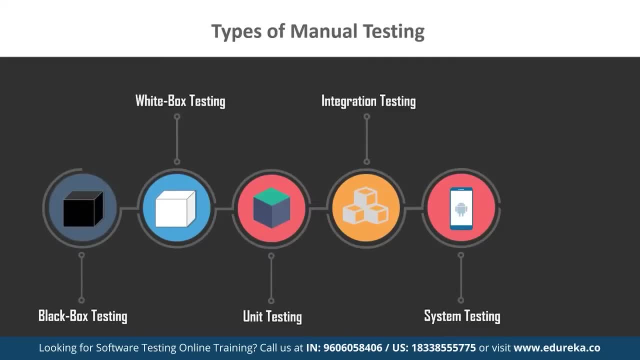 against the given requirements. So basically, you are testing the entire application as a whole here. So there are various system testing techniques here, like you have functionality testing, performance, scalability, stress testing and regression testing. Well, I can't discuss about them here, but we do have other videos in a duty cop playlist. 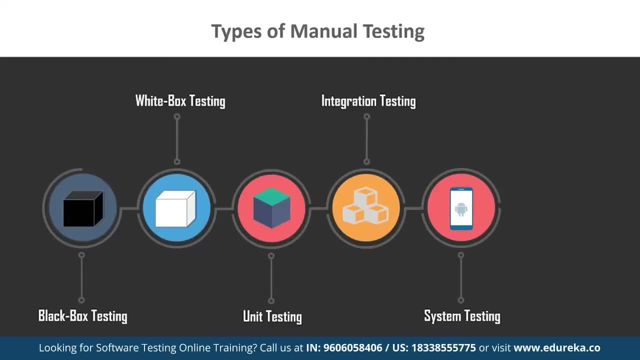 Just to refer to. if you want to know more about this system testing types, so please do that. go ahead and refer to other videos and the software testing at your breakup playlist. Okay, let's move on to next type of testing, which is acceptance testing. user acceptance testing is: 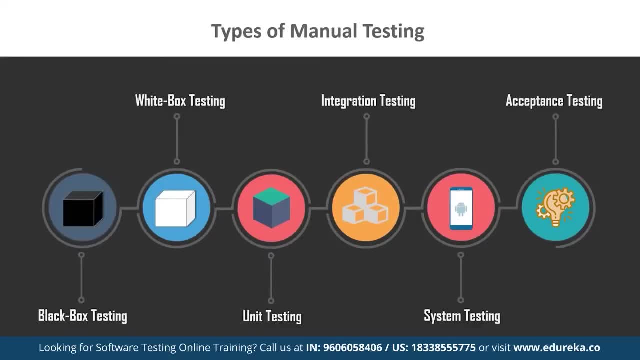 the formal testing that's performed based on user requirements and function processing. Well, this type of testing covers end-user real-world scenarios. It's the last step of testing. It needs to be done very correctly, because it will provide you with the results on basis of which your software product 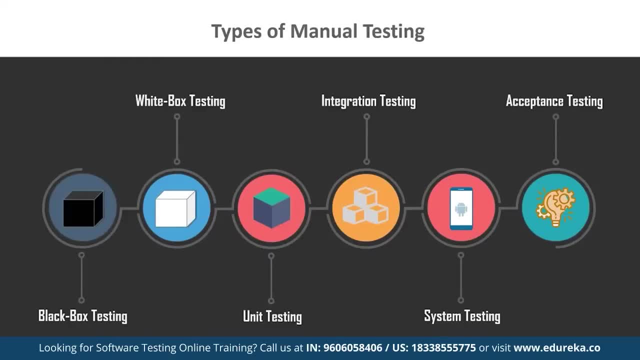 will either be approved or rejected by the senior management, So it's a very important and final step. So, guys, these are different types of manual testing, but please do remember that these type of testing can be carried out either manually or using a test automation tool. 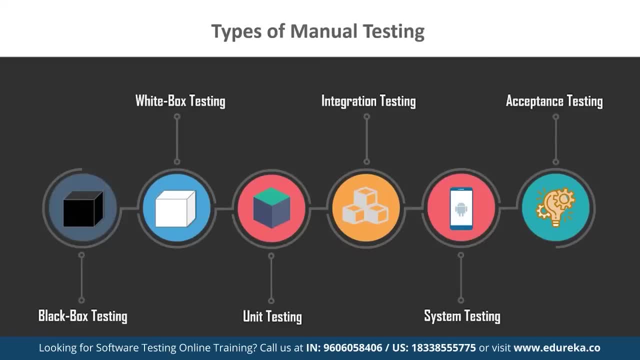 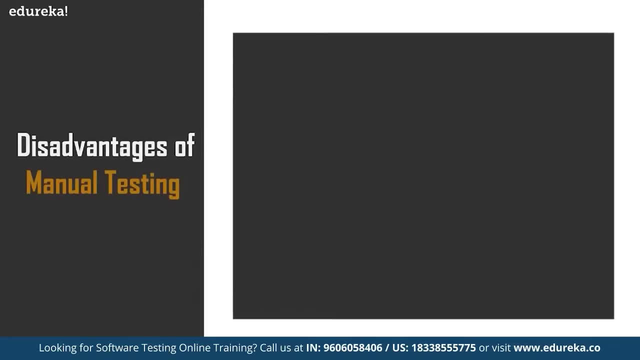 Like I said earlier, so they particularly do not belong to manual testing. So, guys, earlier I did tell that, just like automation testing, manual testing to has its pros and cons. We did discuss certain advantages. now let's go ahead and discuss disadvantages of manual testing. 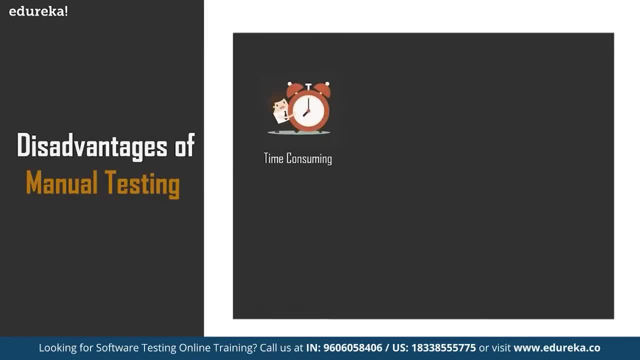 First of all, it's really time-consuming. manual test can be used, which means every time there's a change in application, The tester needs to run all the test cases again from the beginning. Hence, the tester need to test the application even in case of minor changes. 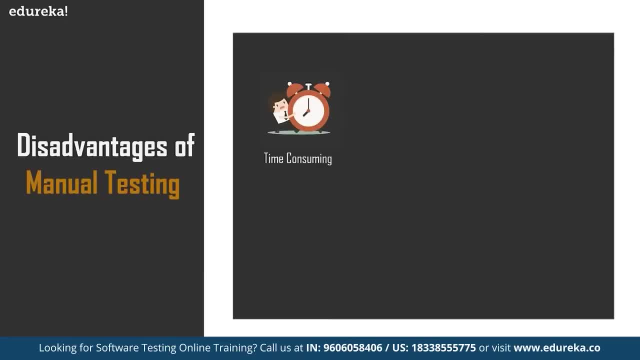 Imagine that it's really very time-consuming process, right? As you can see, the important resources here are nothing but humans, because basically the entire manual testing is performed by humans. So to repeat the same task again and again is really time-consuming and there's high possibility of errors in manual testing. 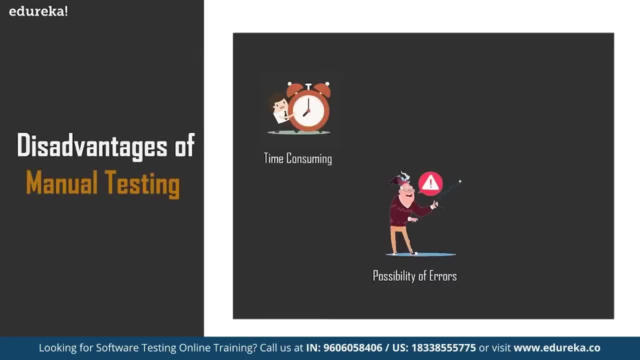 That's because manual testing is dependent on humans and there's a high possibility of errors. because of that, The testing results will be as good as tester performing the test. So if the person who is performing the test is really good at what is doing, then you can expect no errors. 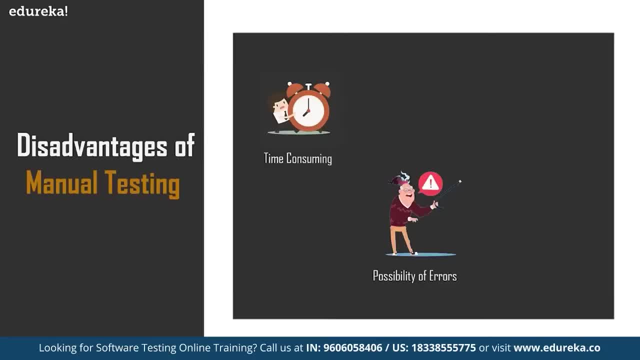 Otherwise you might find certain errors and box. with manual testing, There are chances that test time and miss out on some bucks or some repeated bugs which are resting within the application. So what I'm trying to say here is that, since manual testing performed by humans, 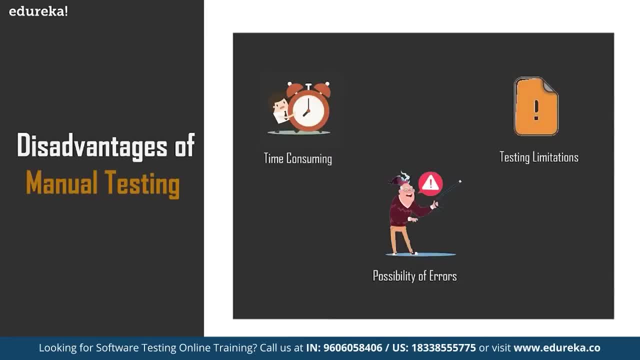 it's more prone to errors. and then you have testing limitations. manual testing is not good for load and performance testing. to check the performance of an application- manual testing- There's a requirement of large number of users and gadgets. The moment the term gadgets comes in, it is no more a manual testing. 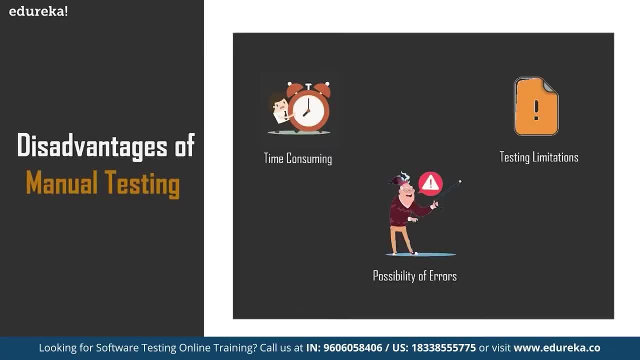 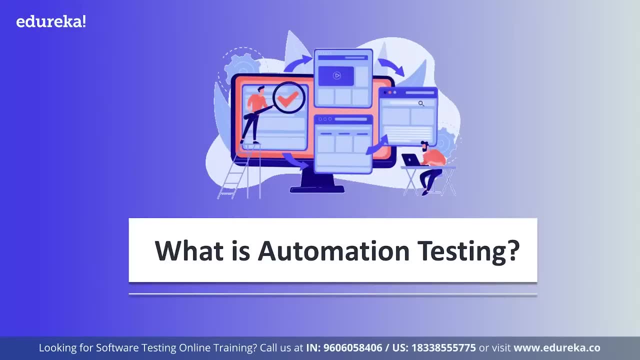 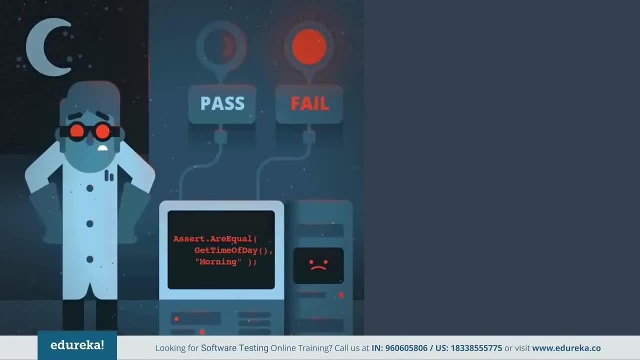 It belongs to automation testing. So you have certain limitations in manual testing. Testing is broadly classified as manual testing and automated testing. So manual testing. it's pretty self-explanatory. right testing of a web application is done manually by human action. That's what we call manual testing. 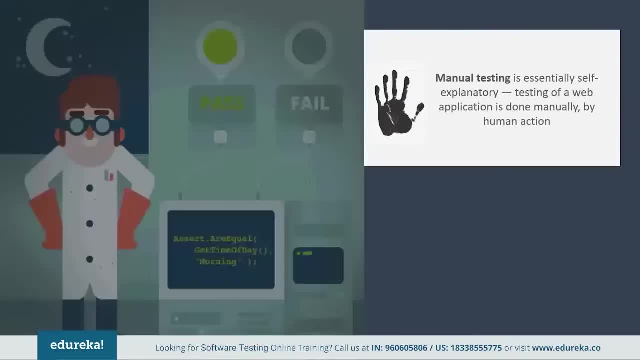 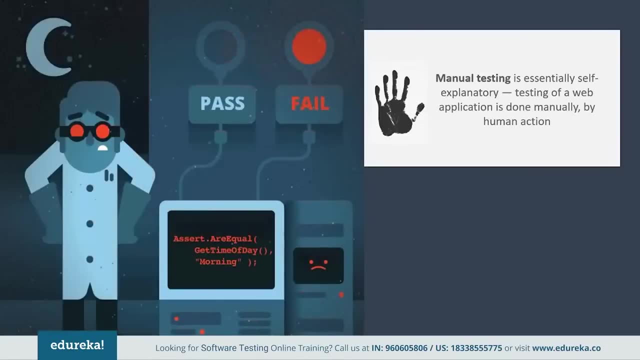 This means that someone actually goes on a device to evaluate numerous components, including design, functionality and performance of software, So they click through multiple elements or units of web application without any support from tool or script. thorough testing is crucial to the success of a software product. 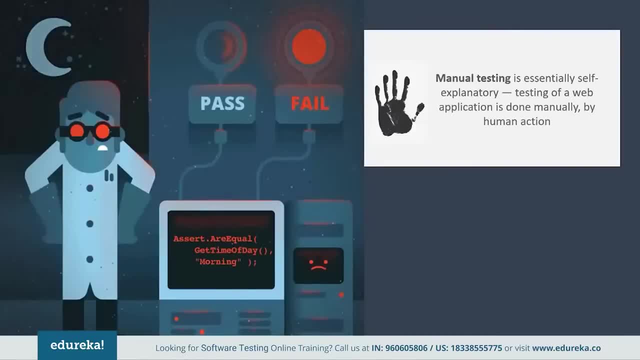 If your software doesn't work properly, chances are strong that most people won't buy it or even use it, at least not for long, even if they buy it. but testing to find defects or some sort of box is very time-consuming, expensive, often repetitive and subjective to human error. if you are using manual testing, 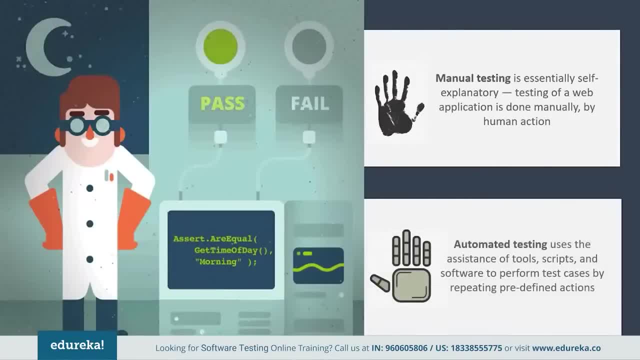 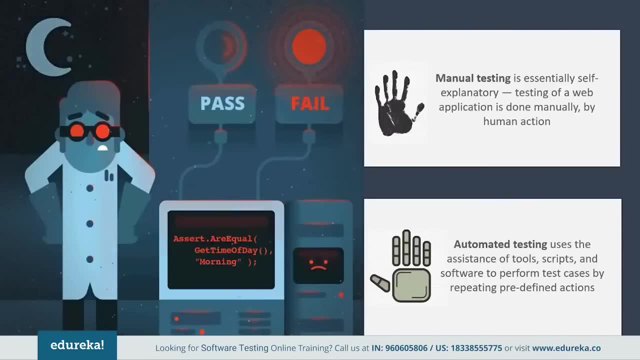 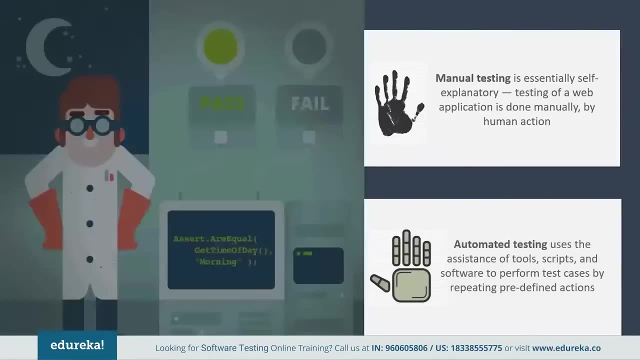 So this is where automation testing comes into picture. automation testing? Well, it's automated. the buzzword automation focuses on replacing manual human activity with systems or devices that enhance efficiency of software. test automation, or usually referred as automation testing, uses different kind of tools, scripts and software to perform test cases. 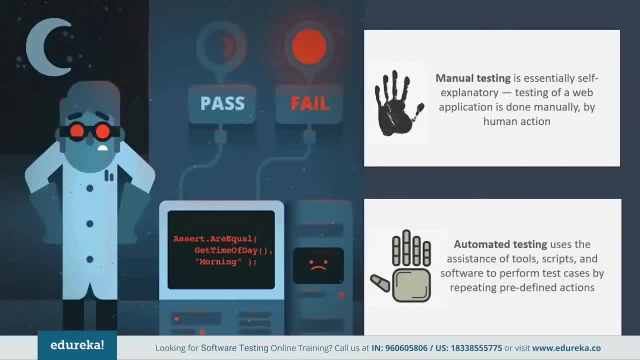 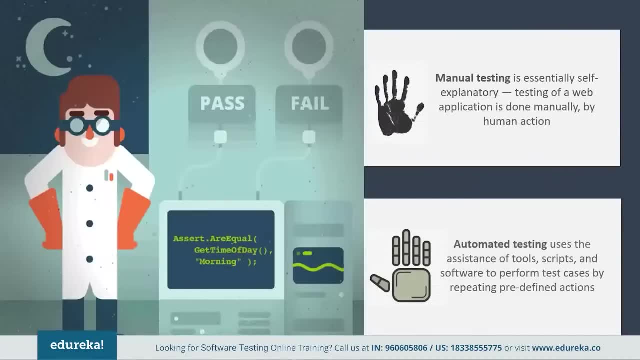 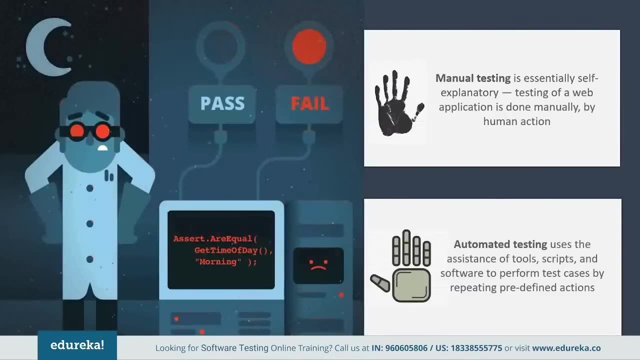 by repeating predefined actions. So by automating your software testing activities, you will definitely get a comparative Edge in the market. So let me give you some examples. Amazon is testing Delivery drones that pick up warehouse orders sorted by robots. Google is testing self-driving cars. 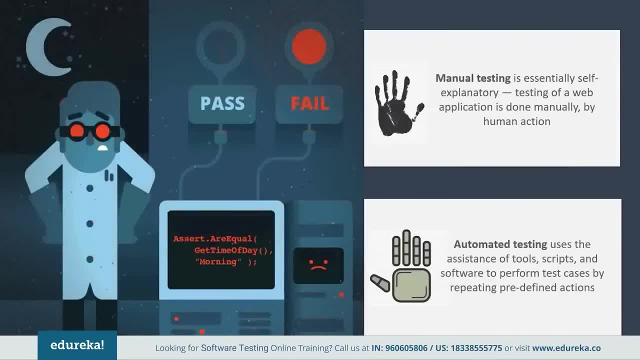 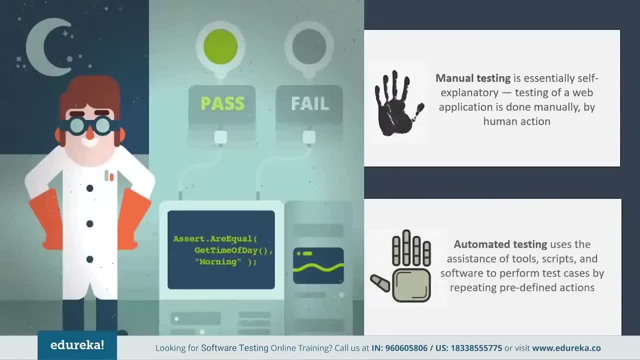 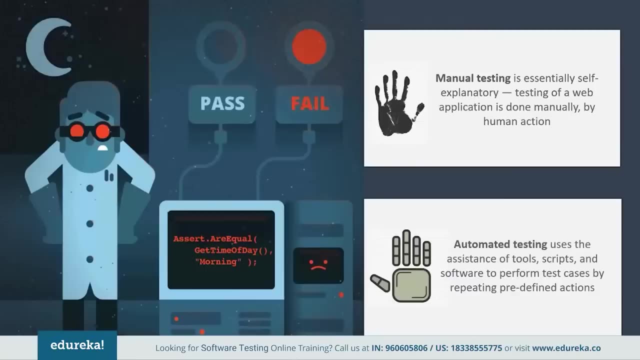 Starbucks is testing cash-free stores dedicated to mobile ordering and payment. Facebook is testing a brain computer interface that may one day translate thoughts into digital text. Fascinating right, There are mundane versions of automation technology behind all this testing. software automation testing Companies use automation technology to create the software. 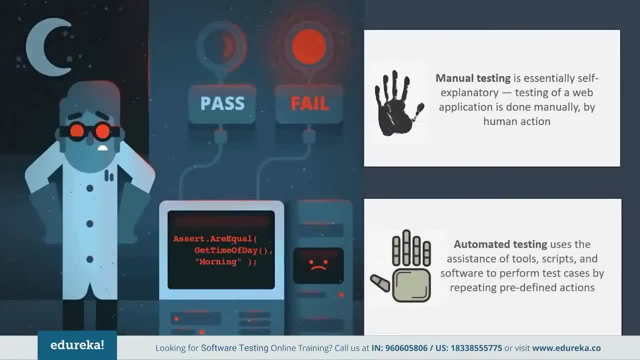 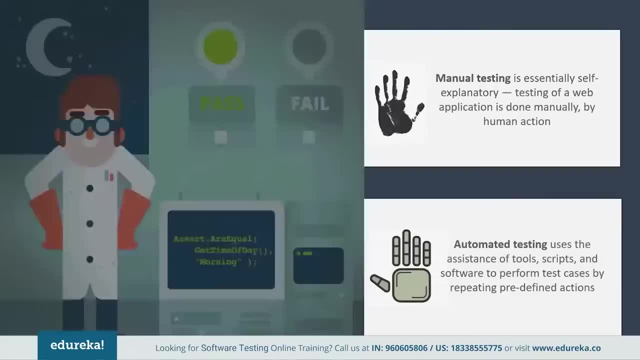 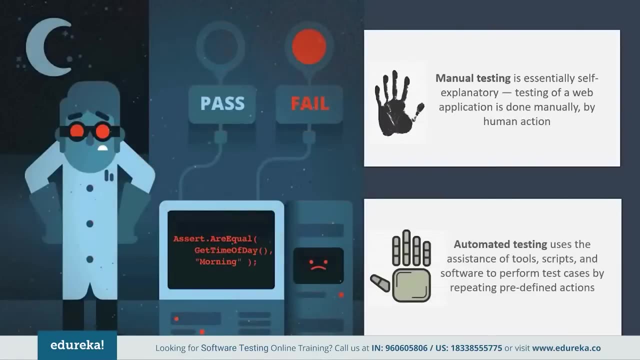 responsible for the products and services causing all this hype about automation testing. when you actually begin testing, One of the primary decisions that you'll have to make is if to choose manual testing or automated testing. Well, neither of these options are technically better or worse when compared to each other. factors like size, budget time, allowance. 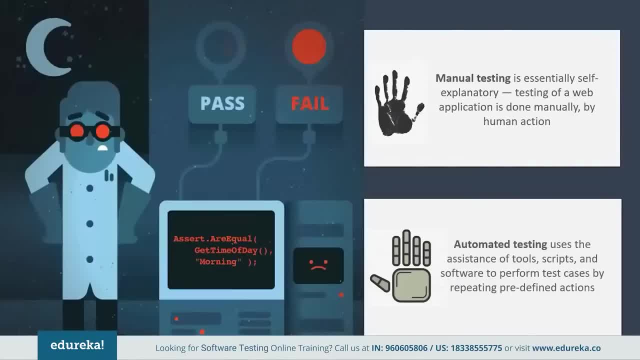 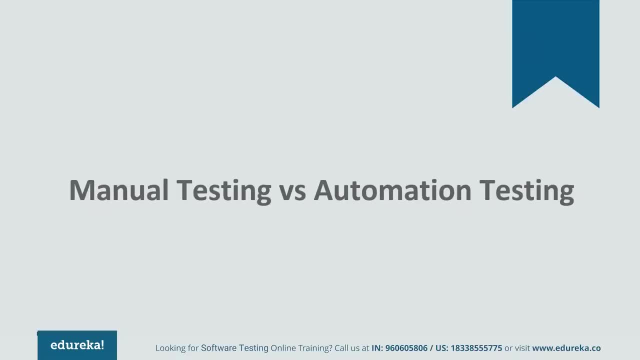 of the project will certainly be factors that effect which method will work best in the situation. So you should be aware of distinct differences between manual testing and automated testing. So here we go. The first difference, obviously, the definition which we discussed earlier in manual testing test cases. 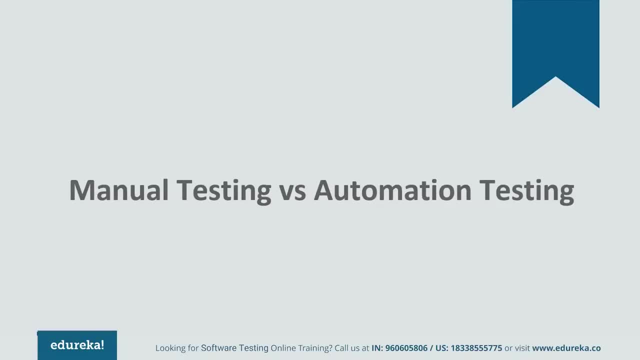 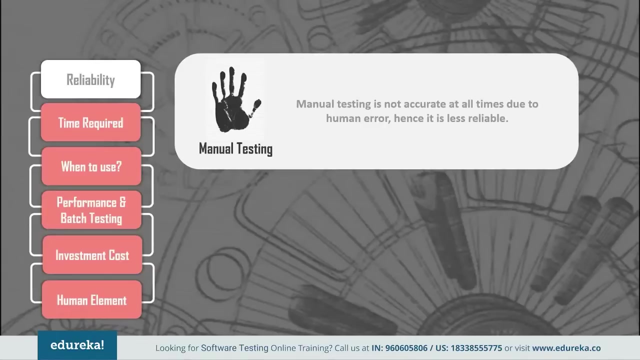 are executed by human tester and software, Whereas automation testing uses different kind of automation tools and scripts to execute test cases. So let's get started with other factors. The first is reliability. for a testing phase where duration is very long, There are high chances of an undetected error. 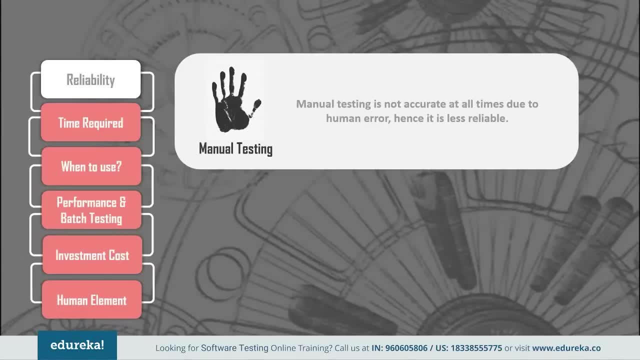 when testing is performed manually. every time a small defect is fixed, The entire application needs to be tested to ensure that any other breakage is not occurring. Well, the process is tiring and boring, So testers often miss out critical defects while performing repeated testing. 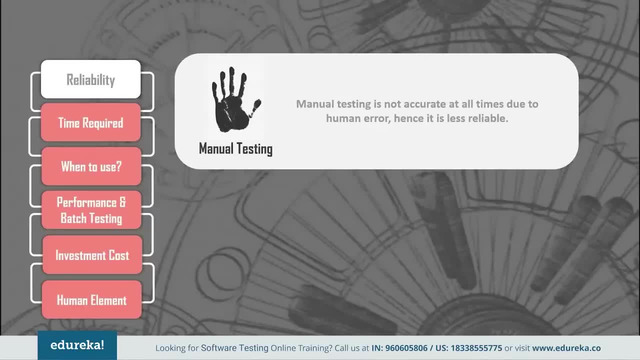 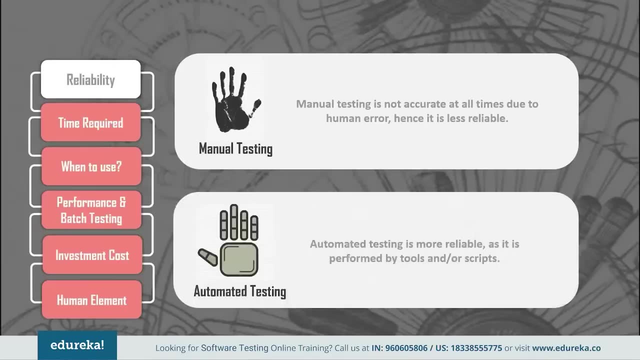 It's a common human behavior right. Therefore, the accuracy and reliability of manual testing is very low. automated testing, On other hand, is more reliable tools, or the scripts that you use from the automated test. If the script is properly written, there is no chance of missing a defect. 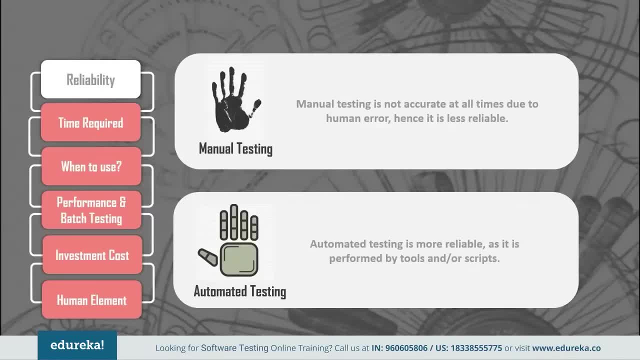 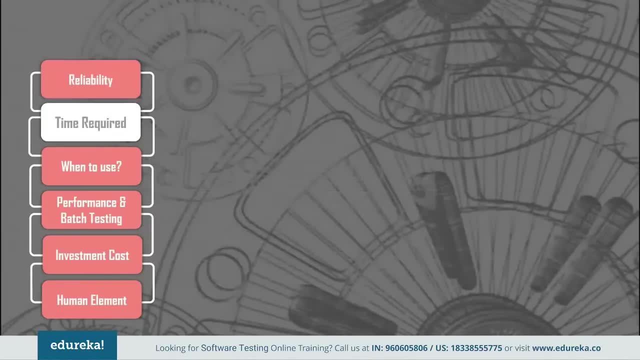 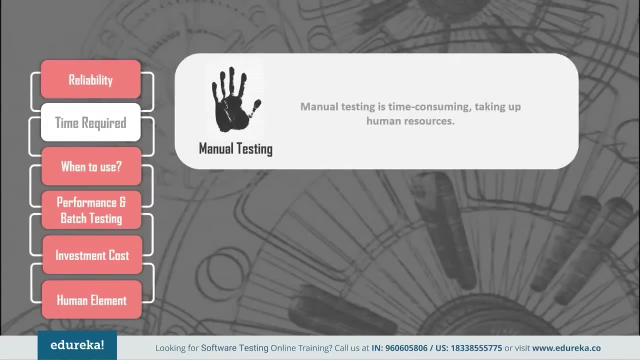 when the test is executed over and over again, and obviously it's not boring as well for the machine, right? When it comes to reliability, automated testing is highly reliable. then comes the time required to perform the testing. Manual testing is obviously time-consuming. It takes up human resources. 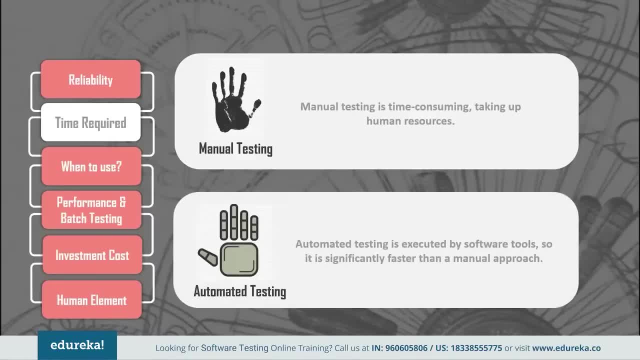 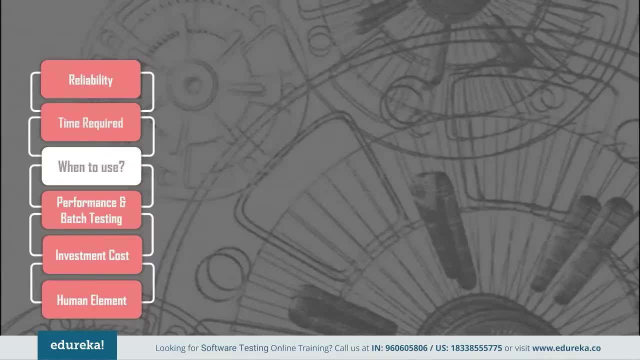 but when it comes to automated testing, it's executed by software tools and different kind of scripts, So it is significantly faster when compared to manual testing. Next, we have when to use which kind of testing. Manual testing is suitable when the test cases are run once or twice. 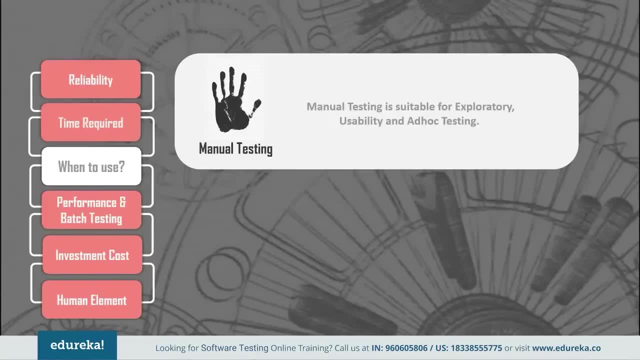 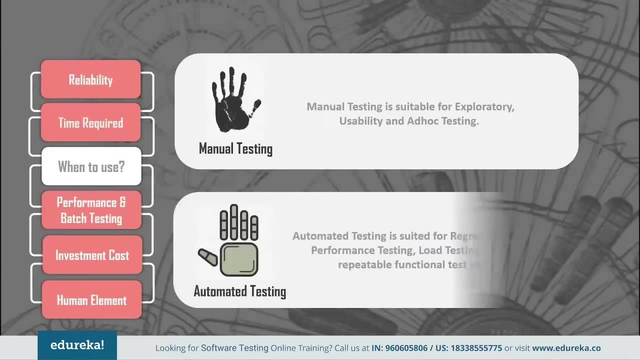 Therefore there's no frequent repetition of test cases in manual testing. So to name: manual testing is suitable for exploratory or usability and ad-hoc testing. Automated testing is suitable when the test cases need to be run repeatedly for a long duration of time. 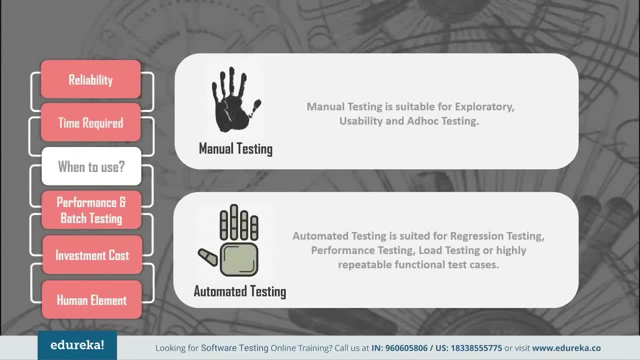 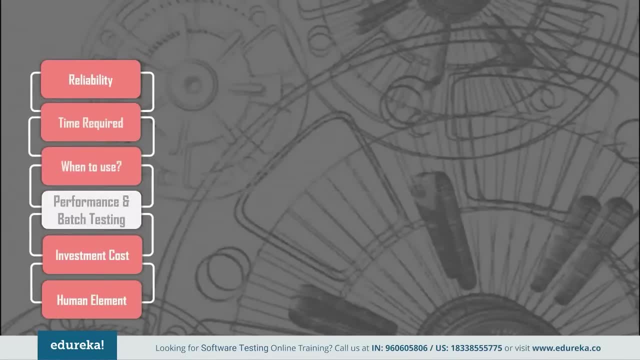 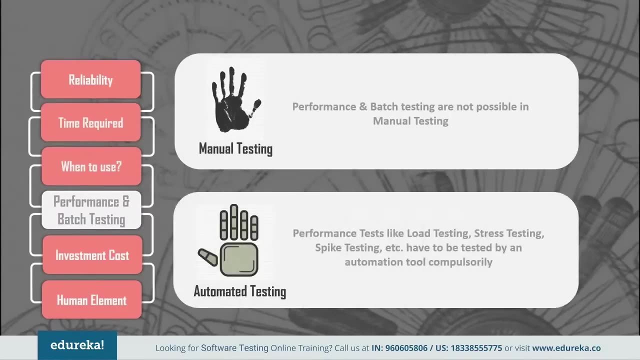 Automation testing is suited for regression testing, performance testing, load testing or highly It will functional test cases. and next we have performance and batch testing, which is not possible in manual testing. You can batch multiple test scripts in automated testing: performance test, like load testing, stress testing, spike texting. 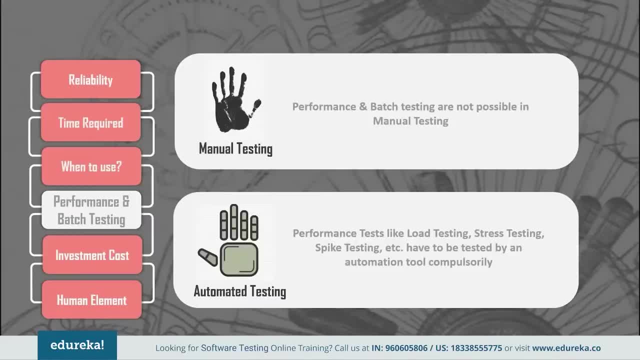 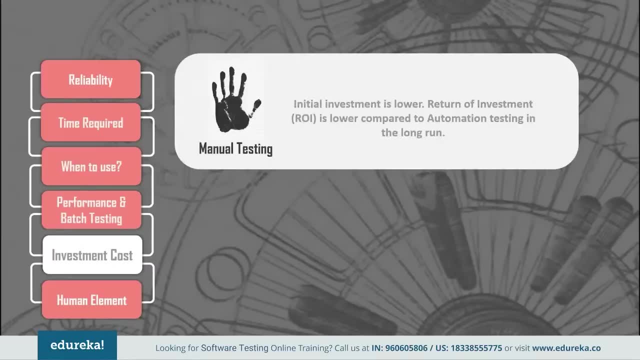 etc. have to be tested by an automation tool compulsorily, and software testing process. Then we have investment costs. The cost of manual testing is usually dependent upon the human resources deployed in the testing during the initial stages of testing. the initial investment in manual testing is comparatively lower. 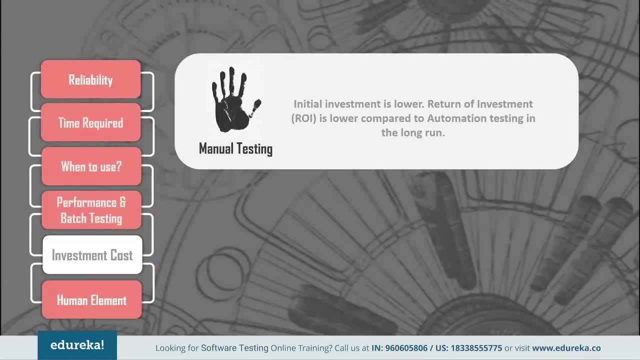 but the written of investment is very low when compared to automation testing. when I say written of investment, I mean the money that you earn as a revenue at the end of the software testing or after selling the product is actually low when compared to automation testing in long run that is. 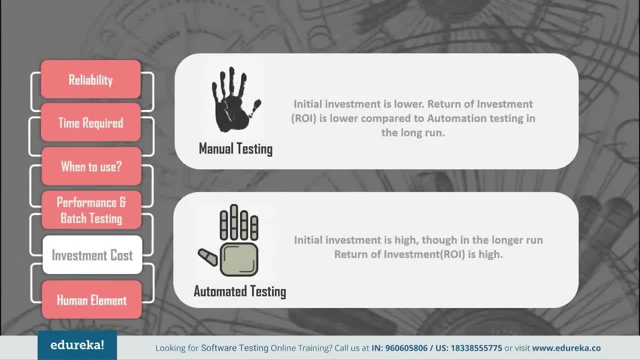 but the cost of automated testing is dependent upon testing tools deployed for performing the test. but the initial investment in automation testing is usually higher, though The return of investment is better in long run. So when it comes to investment cause initial investment, manual testing is much preferable. 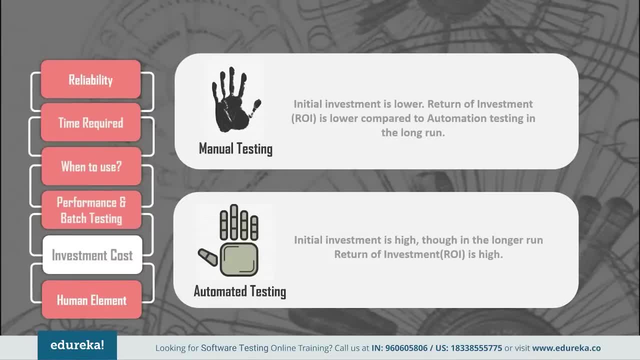 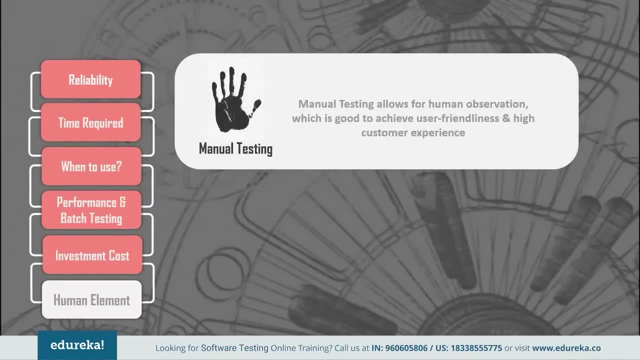 But if you want to perform testing for longer run, then automation testing is much preferable. as the last criteria we have human element. manual testing allows human observation right, So you're getting exact kind of feedback a person would give you, and that can be invaluable- being able to predict. 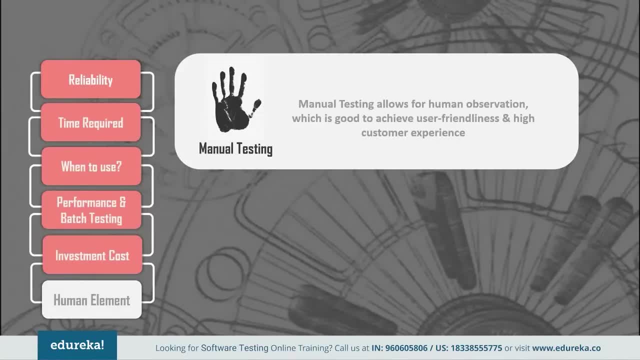 what your users will or won't like. things that a computer can't give feedback on ahead of time, can influence your design and make it much better from the bottom up. It improves the customers experience, But when it comes to automated testing, as there is no human observation involved, 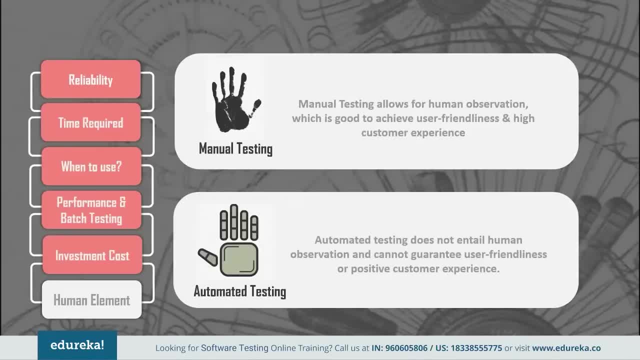 there is no guarantee of positive customer experience. So, when it comes to human element, manual testing is much better, because you get to have a nice experience, since the humans are the ones who are checking the software. So, guys, these are some differences that you should be aware. 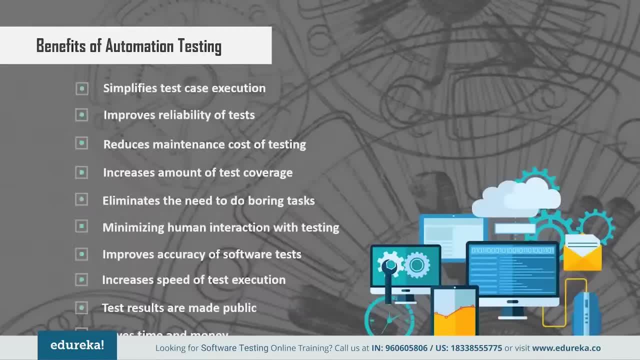 of between manual testing and automation testing. So to summarize what you've learned till now, automation testing is a lot of advantages over manual testing. First of all, it saves a lot of time and money. It improves test accuracy. It increases the test coverage. 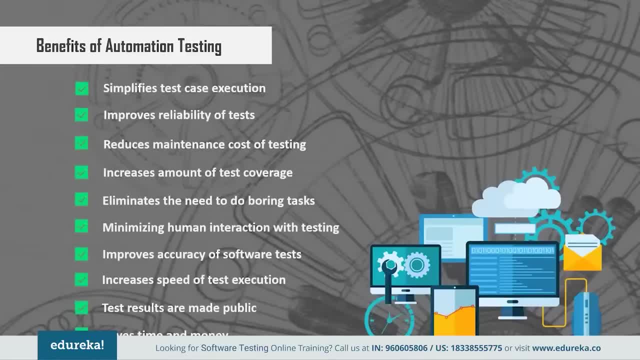 as in. you can perform tests repetitively on different kind of devices. complex test and boring tasks are made very easy and comfortable. It increases efficiency and team morale. You no longer have to do the boring and repetitive task. There'll be no human errors. 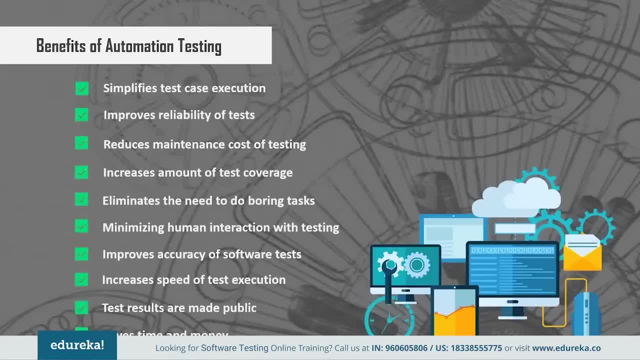 Obviously, it reduces maintenance cost of testing, It increases speed of executing tests and many more advantages. So, in short, while manual testing is effective and projects with multiple operating environments and hardware configurations, automation testing is absolutely essential today to successfully deliver large-scale products that need execution of repetitive and complex test cases. 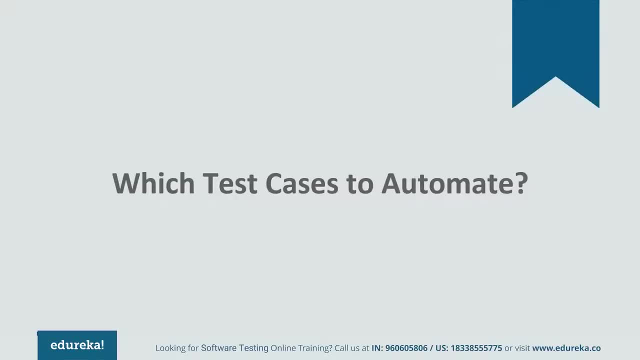 but it's impossible to automate all testing, So it is important to determine what test cases should be automated first. So, guys, let's go ahead and take a look at use cases where automation testing have to be applied, because, like I said, you can't apply automation everywhere. 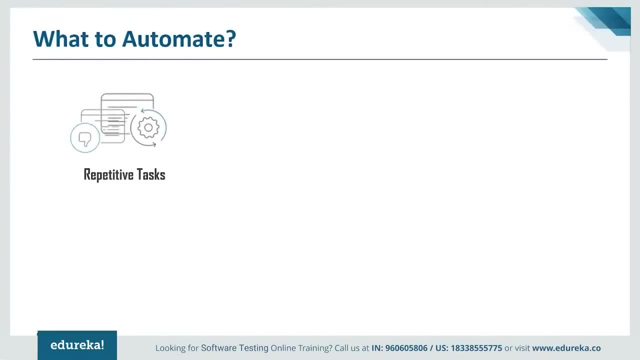 First of all, as you guys know, repetitive tasks are primary candidates for automation. Take an e-commerce site, for an example. It may be testing entering in user credentials multiple times. consider the task that you hate doing. not only are the stars boring to you. 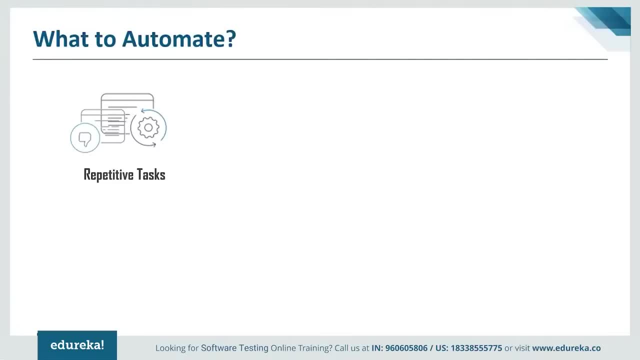 but they're often the ones where mistakes are made, Very commonly, so automate them and do something more fun. Next, capturing and sharing results is obviously a critical part of successful test strategy. rather than manually exporting your data, crunching the numbers and making petty graphs, invest in a tool. 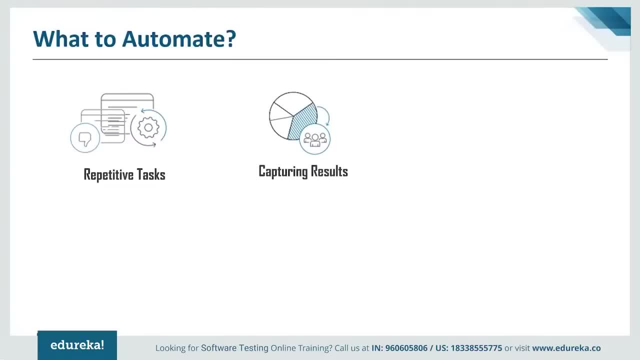 or automation strategy that will do this for you. Thereby you can save time and lot of effort on your part and, obviously, test that require multiple data sets rather than manually typing in information into forms or fields. Automate this process to read an information from a data source. 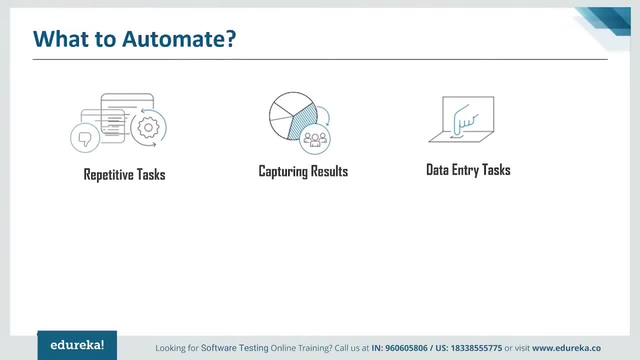 and automatically type into the respective forms. This way you will have better handle on your data variability and it also decreases the chances of making mistakes repetitively again. And suppose if you're waiting for an on-screen response it can be automated So you do not have to waste time staring at a screen. 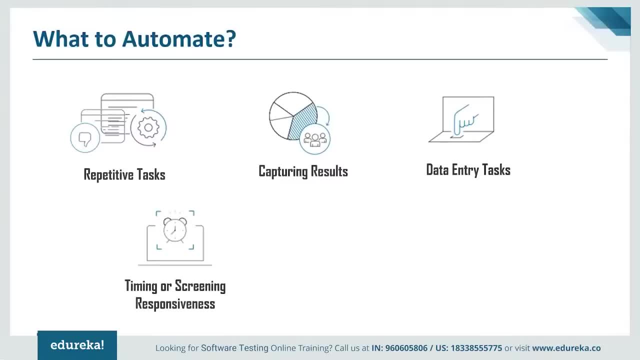 and watching for a response. right, You have other better things to do. put that time to better use and use automated controls like wait until in your program code. Then you have Non-functional testing. a good example of automating non-functional testing types is automating load testing. 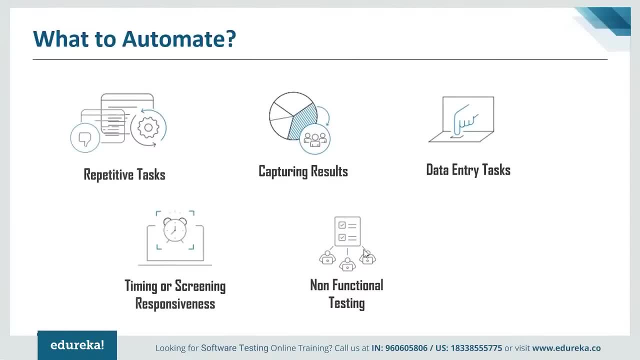 Think about having to see if your application can handle a load of 10,000 users. automate this testing So you do not have to worry about manually spinning up 10,000 users hitting your application all at once. test the Tron on several different hardware. 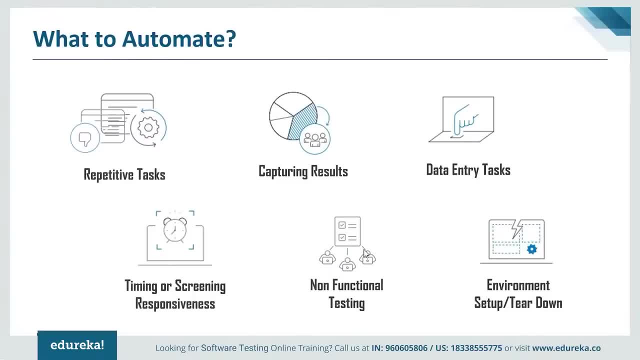 or software platforms and configurations. So as the number of device users in track with increases, automating your setup or tearing down your setup environment will continue to be critical. Additionally, these are scripts that you will use over and over again and multiple testing frameworks right. 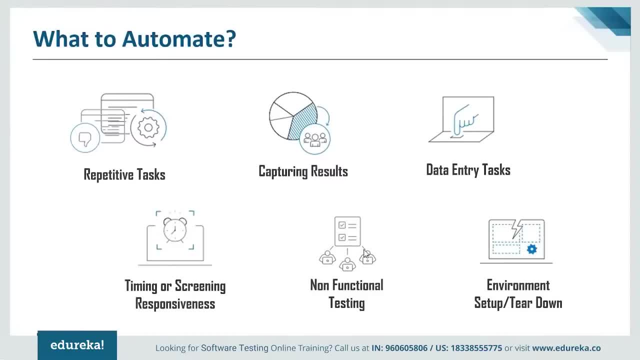 It's better to automate than to do them manually. So, basically, the cases where you have to automate is when you have repetitive and boring tasks, or if you have to capture some results and share the results, or if you have to repetitively enter the data task. 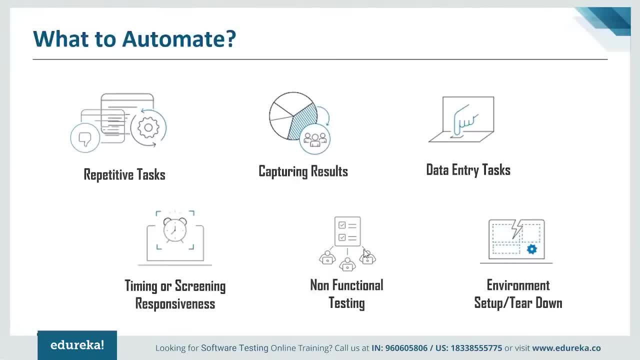 as in data entry task or some sort of timing or screening, responsiveness and especially in load testing, and suppose if you want to set up or tear down your environment, set up, then you can use automation. So, guys, it's always better to know when to use or when to apply automation and software testing. 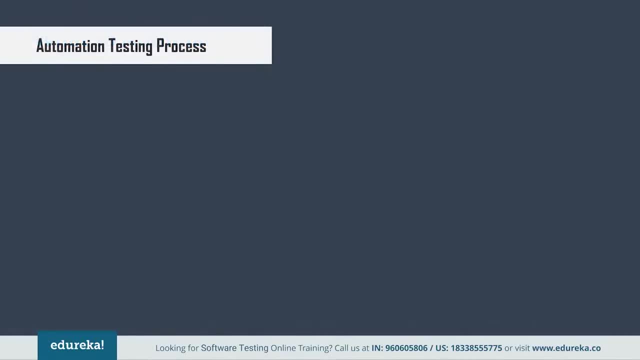 So, guys, success and test automation process requires careful planning and design work. start out by creating an automated plan. This allows you to identify the initial set of tests which to automate and serve as a guide for future test as well. There are a lot of helpful tools to write automation scripts. 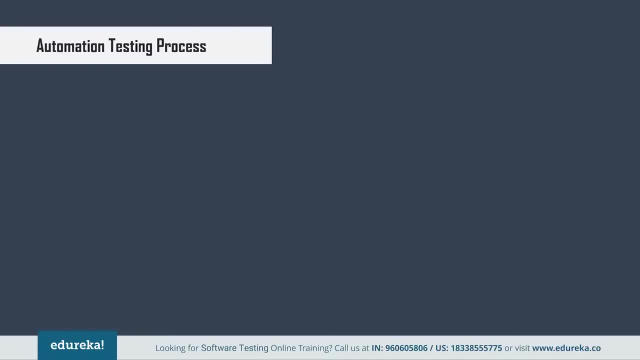 before using those tools, It's better to identify the process that can be used to automate the testing or the procedure that you have to follow to start automation. So, as next part of session will discuss the steps that you need to follow when you're performing automation testing, 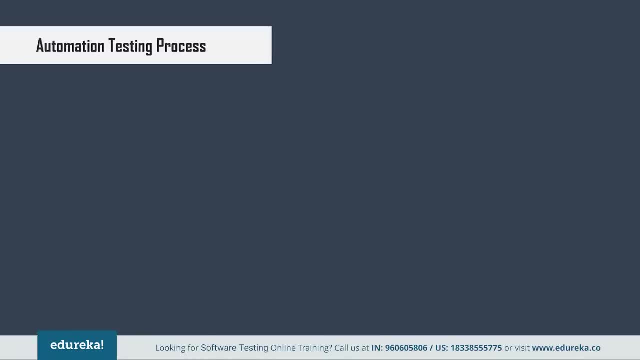 So, like I said earlier, success in test automation requires care for planning and design work. So start out by creating an automation plan. First of all, you should define your goal for automated testing and determine which type of test to automate Once you're sure of what kind of test are you performing. 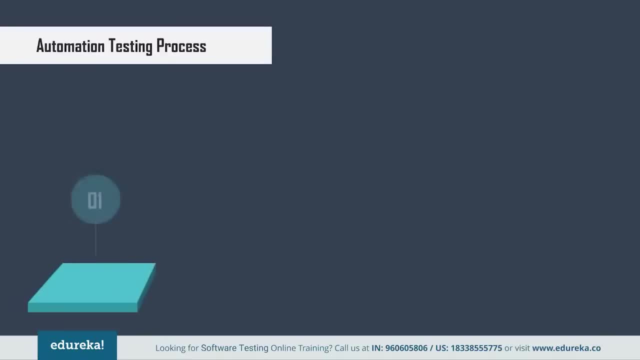 You need to select the tool. So the first step here is test tool selection. There are several kinds of testing tools available. However, choosing the right tool, keeping in mind the nature of test involved, is very important for your automation to be successful. So, whether it's a code driven testing process, 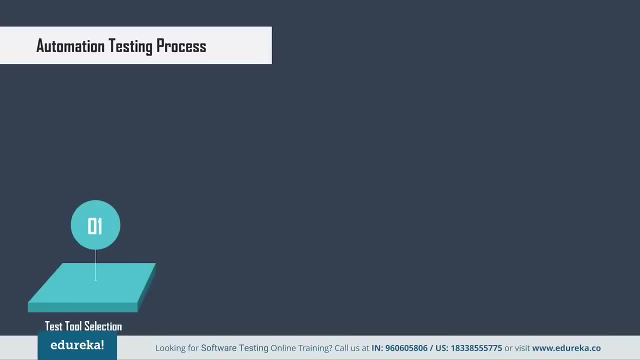 or graphical user interface based testing. you must sell the appropriate tool to automate the testing. So the first step is selecting the proper tool required for automation of your application or testing. Next comes defining scope of automation, As in you need to select which test cases to automate. 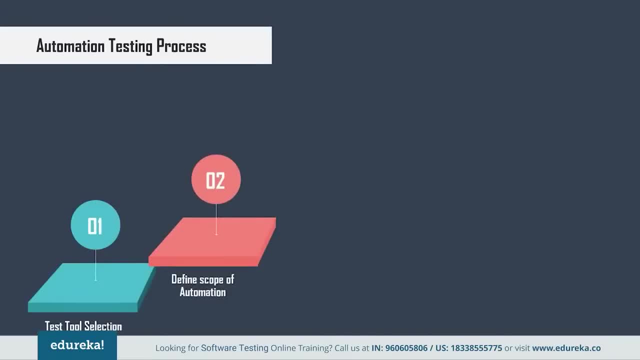 Here you can follow certain pointers, like the features that are important for business scenarios which have large amount of data or those which has common functionalities across different platforms and applications, technical feasibility, the extent to which business components are reused, the complexity of test cases, etc. So, by keeping these pointers in mind, 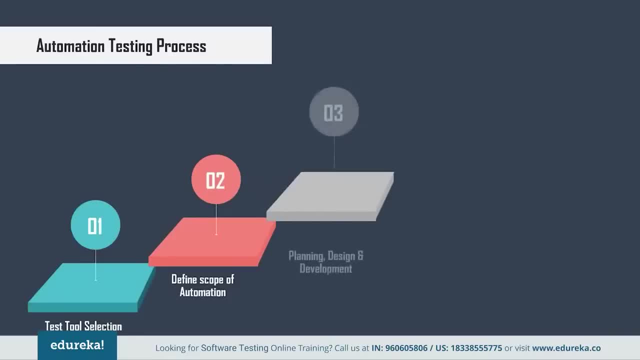 you can define the scope of automation. and the third step is planning, design and development. after determining your goal and which type of test to automate, you should decide what actions you automated test will perform. planning design and development, develop test cases, Don't just create test steps. 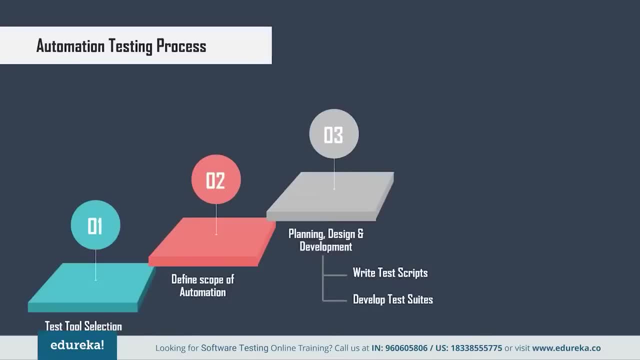 that test various aspects of applications behavior at one time, It becomes overwhelming. large, complex automated tests are difficult to edit and debug as well, So it will be a problem for you later on. So it is best to divide your test into several logical smaller tests. 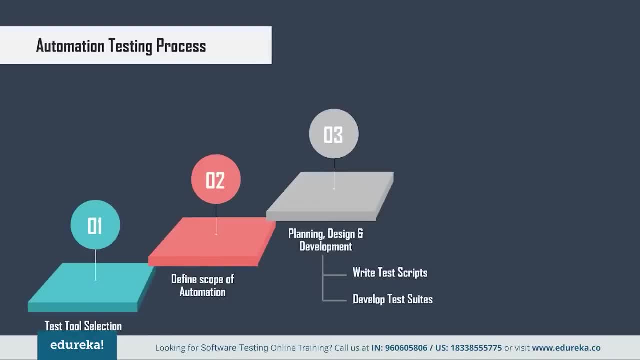 So once you've developed your test cases or you have written your test scripts, next step is to develop test suits. test suits are developed to ensure that the automated test which you have written run one after the other without any manual intervention. This is done by creating a test suit that has multiple test cases. 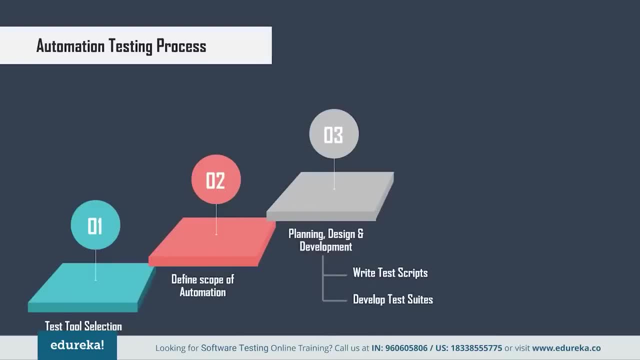 a library and command line tool that runs the best suit. So, guys, the next step is test execution. Once you're done with writing your scripts and placing them in suitable test suits, the next step is to start executing them. automation scripts are executed during this test execution phase. 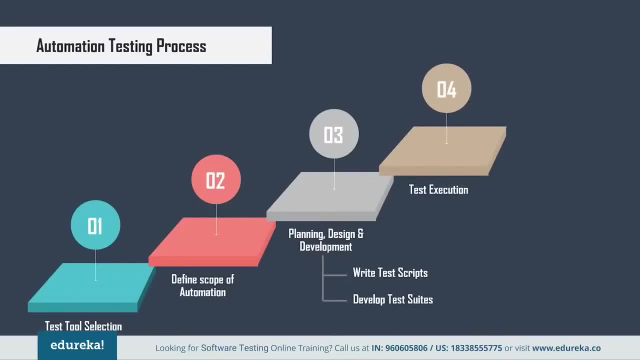 So execution can be performed using automation tool directly or through the test management tool, which will invoke the automation tool which you have chosen to get the most out of your automated testing. testing should be started as early as possible and as often as needed as well. the earlier testers get involved. 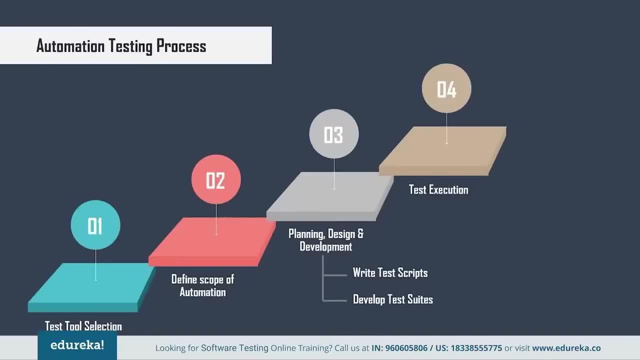 in the life cycle of the project. the better and more you test, the more box you can find right. so yeah, your scripts are executed in this phase. once executed, The next step obviously is to create report format so that individual test logs with details of action performed. 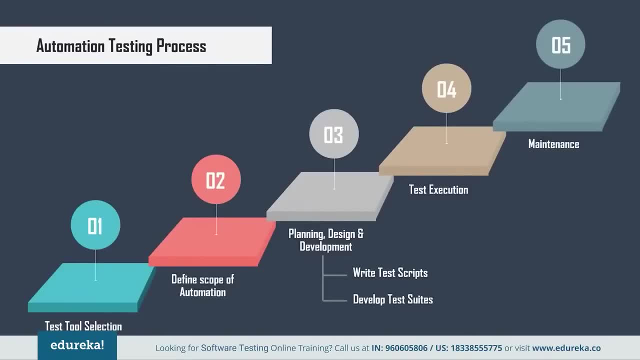 during tests are recorded properly for references. So you define the type of test report format to be created: screenshots, messages, Etc. So all such things you include in your report. as new functionalities are added to system under test with successive cycles, automation scripts need to be added. 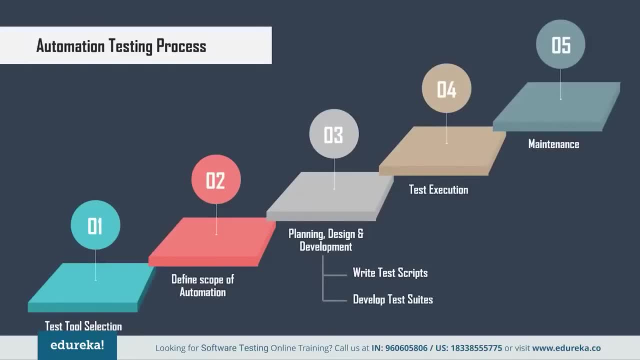 reviewed and maintained for each release cycle, right? so maintenance becomes necessary to improve the effectiveness of automation scripts. So what I mean here is that you do not entirely finish your product and start testing. suppose if you have found some bug, you add additional features and again start your testing from the beginning. 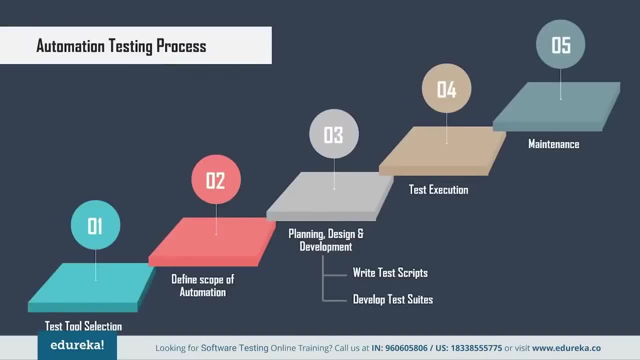 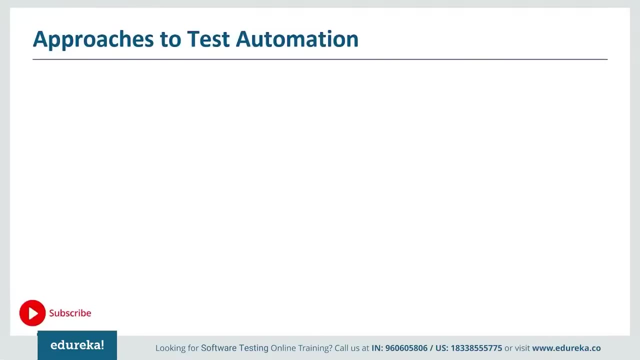 So maintenance plays a very important role and it becomes necessary step to improve the effectiveness of your automation scripts. So you need to follow these steps when performing automation testing to get the best results and efficient results. next comes to automation tools. There are several innovative automation testing tools. 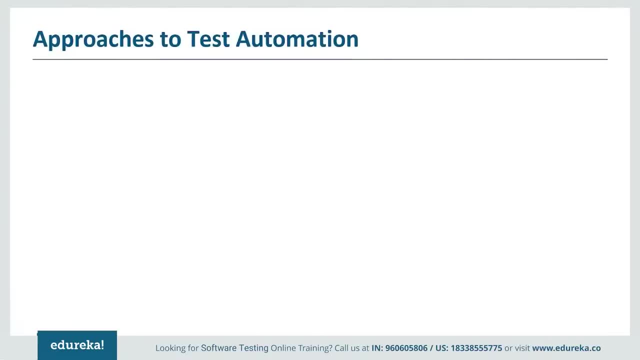 But before we discuss that, we need to understand there are different kind of approaches to automation. The first one is we have code-driven approach. This approach uses testing frameworks like x unit framework, Etc. The focus here is mainly on test case execution to find out if various sections of code are performing. 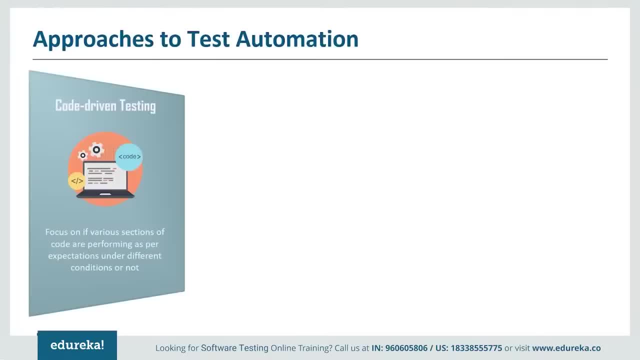 as per our expectations, under different conditions or not. So code-driven testing approach is a popular method used in agile software development. Then we have graphical user interface. applications that have g-wise or graphical user interface may be tested using this approach. It allows the testers to record user actions. 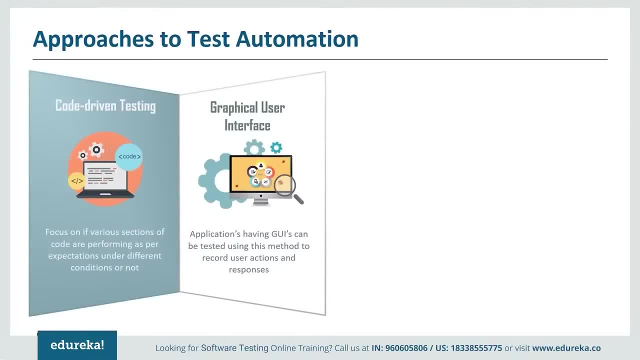 and analyze them any number of times. So this is one way of going at automation. For example, if you want to test a website, you can use automated testing tools like selenium that provides a record and playback tool for authoring tests without any knowledge. 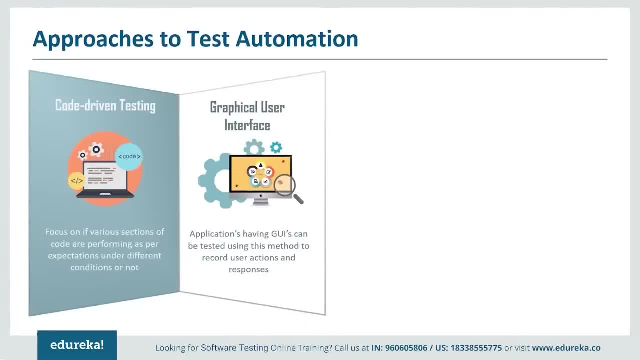 on test scripting language, So you do not basically have to know the scripting language here. You do have record and playback tool using which you can start executing your test. Test cases can be written in any number of programming languages, like C, sharp. You have Java, Pearl, Python, Ruby and many other options. 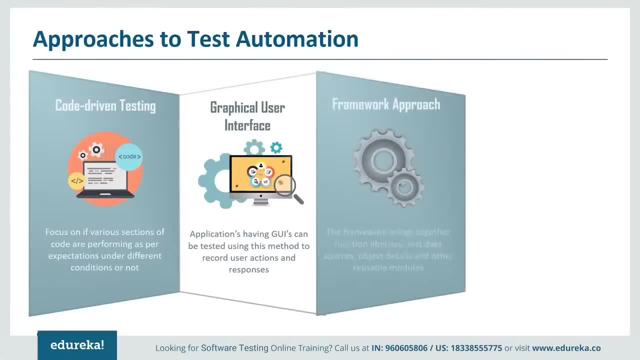 So the next approach is using automation framework. So basically, a test automation framework is set of guidelines which are used to produce beneficial results of automation testing activity. This framework brings together function libraries, test data sources, object details and other reusable modules. It lays down the general rules of automation. 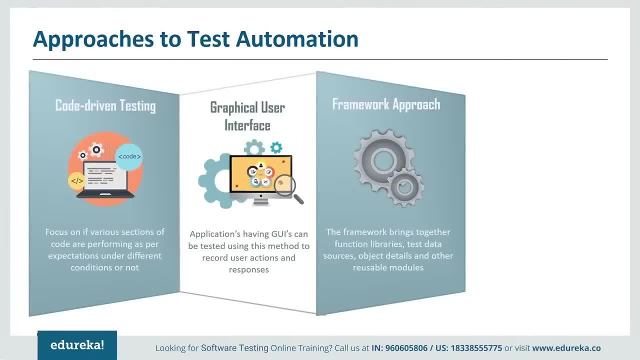 and it simplifies the effort required to bring the efficient results and lower your maintenance cost as well. So, basically, you can say you're setting down a set of rules that you need to follow while performing your automation testing. Let's consider, example Suppose, if there is any change in a test case. 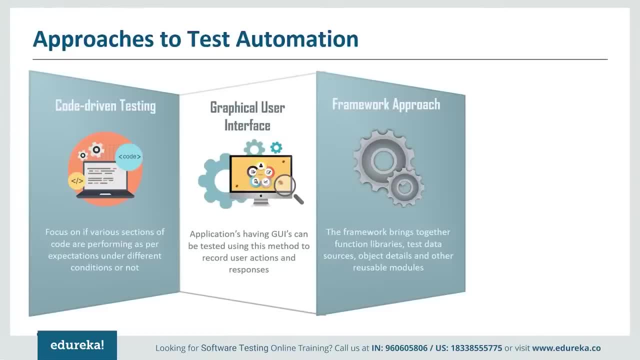 then only that particular test case file needs to be updated without having to make any change to the driver or the startup script. So you have multiple approaches when it comes to frameworks. frameworks could be linear scripting, framework recording and replaying test scripts in sequential, or you can say a linear fashion. 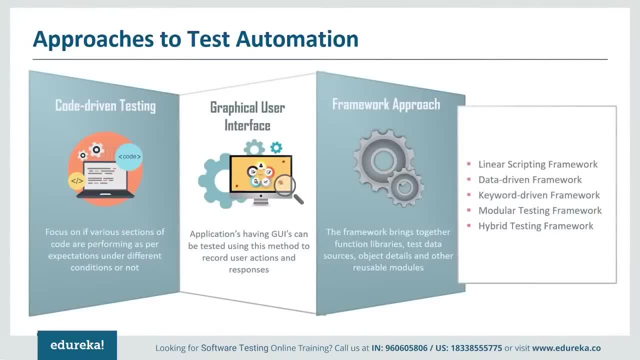 You have data driven framework. a constant source of test criteria specifies the test scripts which you have to run here. Then you have keyword driven framework. here The tables on a spreadsheet actually specify the action of a test scripts that need to be formed, based on the library of functions for an assigned keyword. 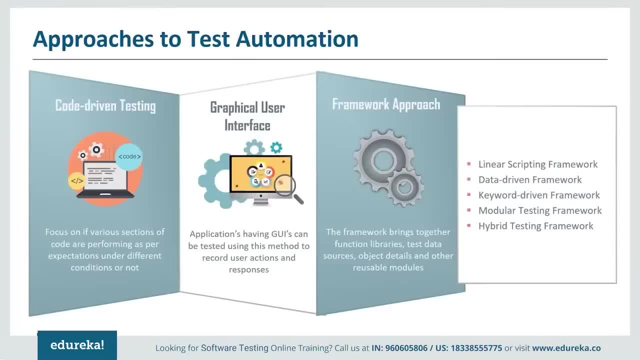 Then you have modular testing framework. modules of an application under test are divided and then tested with individual test scripts, and then they can be combined for larger test scripts. Then you have I breed testing framework. Obviously, it's a combination of frameworks to leverage the strengths of each of the ones. 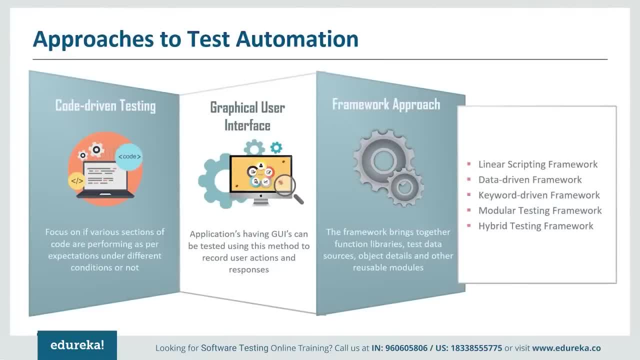 which we discussed earlier. when you've decided to perform automation testing, you can opt for any of these approaches. You can go for code driven testing. You can also go for graphical user interface. If you're testing graphical user interface, then you can go for framework approach. 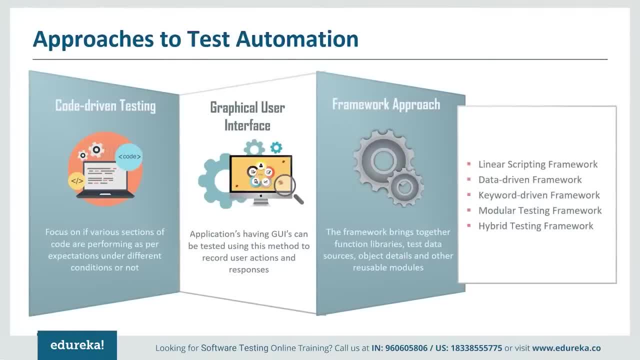 and you have multiple framework options here as well, like linear, which performs testing in a linear fashion. Then you have data driven, keyword driven, modular testing and hybrid testing, which is a combination of all the other framework types. So yeah, guys, basically there are ways you can implement automation. 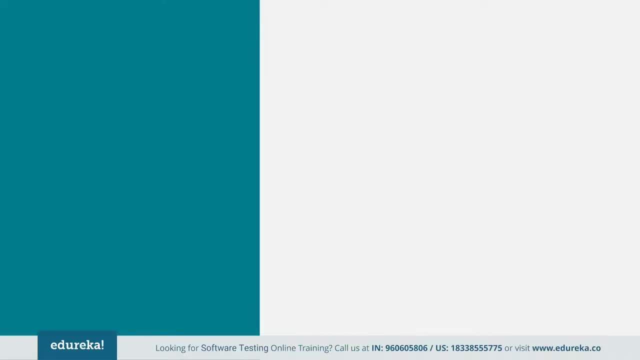 while software testing. So now, moving on to test automation tools. selecting an automated testing tool is essential for test automation. Well, there are a lot of automated testing tools in market, and it is important to choose the automated testing tool that best suits your requirement. 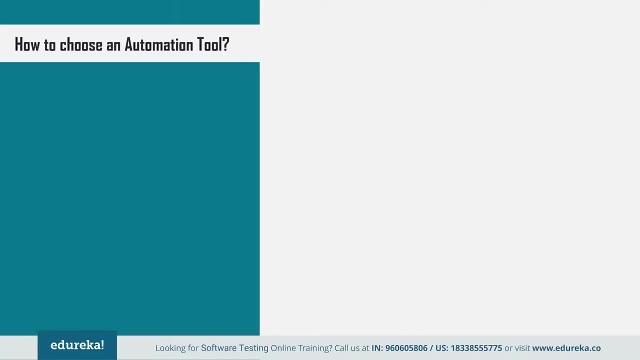 So, basically, when you're trying to test or select an automation tool, please do follow the key points which I'll mention now. first of all, check if the tool is compatible with platforms and the different kind of technology that you're using. ask yourself: Do you need support for mobile automation testing? 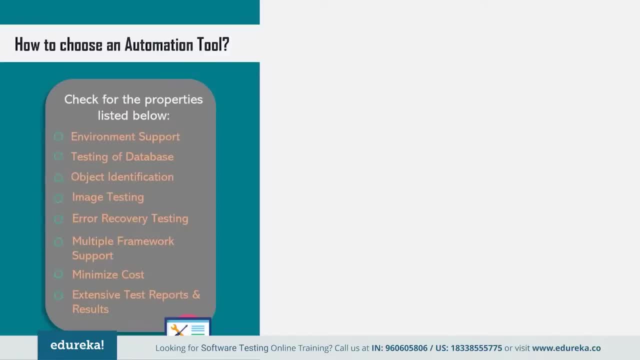 or different other kinds of testing? Are you testingnet C, sharp or other applications? if yes, and then on what operating systems? so next, flexibility of the testers also plays a very important role. that is, what kind of skills your tester have also plays a very important role. 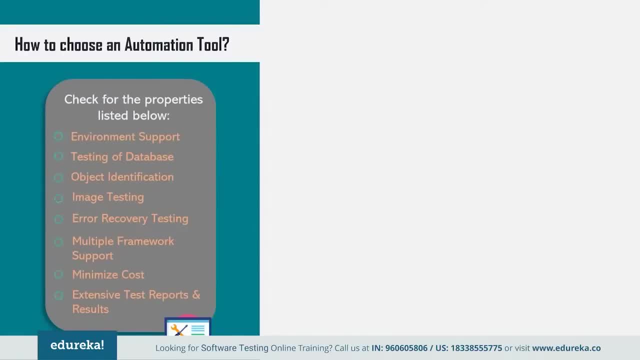 For example, can your QA department write automated test scripts or is there a need for keyword testing? thirdly, does the automated testing tool support record and playback test creation, as well as manual creation of automated tests? So, basically, you need to consider these sort of questions. 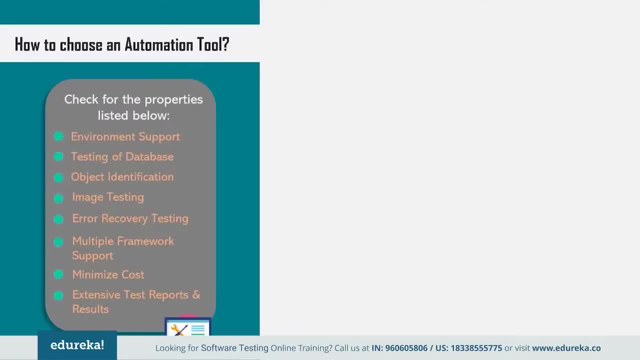 or situations. before you go ahead and select a tool, You can also look if the tool includes features for implementing checkpoints to verify values, data Basis or key functionality of your application. You need to create automated tests that are reusable, maintainable, resistant to changes in the application UI. 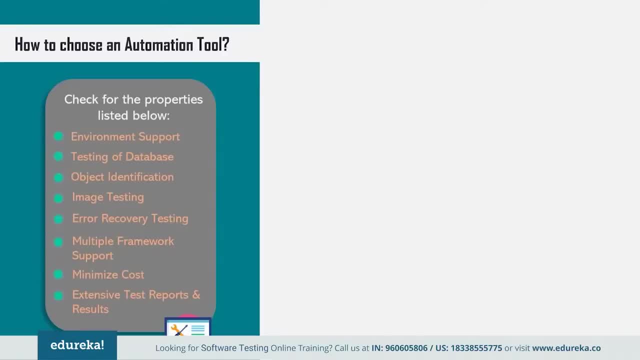 right. So ask yourself: will my automated test break if my UI changes? So, based on that, choose a tool. make sure that the application is stable enough to automate the early development cycle. unless or otherwise, it is agile environment, It not be a good idea. 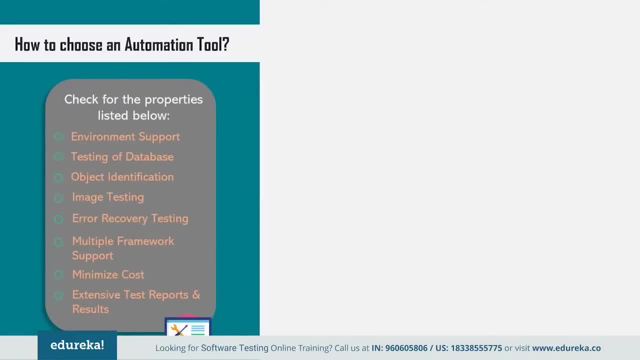 And finally, the cost and the effort that you need to put in is also a very valuable concept That you should consider when you're choosing an automation tool for your testing. Well, these are certain categories or scenarios or key points that you should take care. 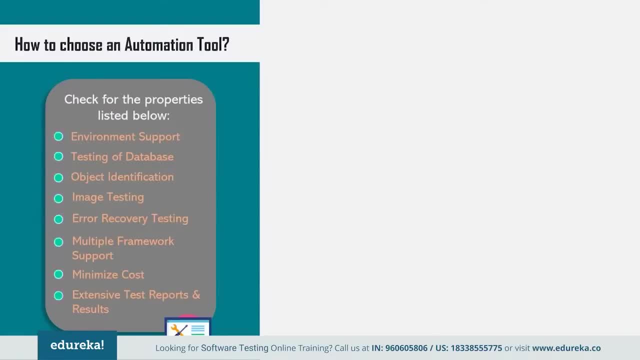 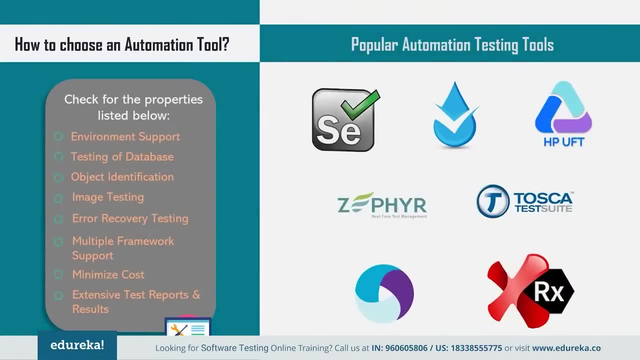 of when you're actually choosing an automation tool. Now, to name few popular automation testing tools, We have selenium. selenium is a popular testing framework to perform web application testing across multiple browsers and platforms like Windows, Mac, Linux. Then we have water w-a-t-i-r. basically it's pronounced. 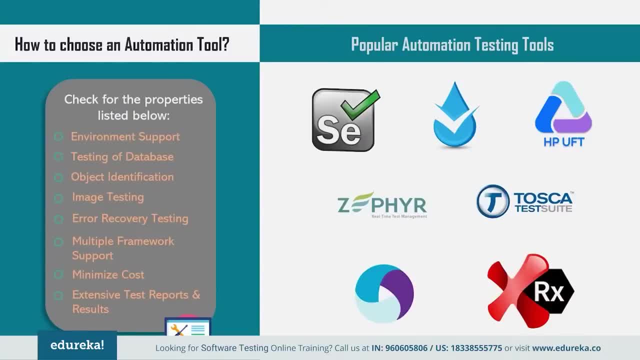 as water is an open source testing tool made up of Ruby libraries to automate web application testing. Then you have something called ranorex. It is inflexible all-in-one GUI testing tool, So using an analytics you can execute automated test flawlessly. 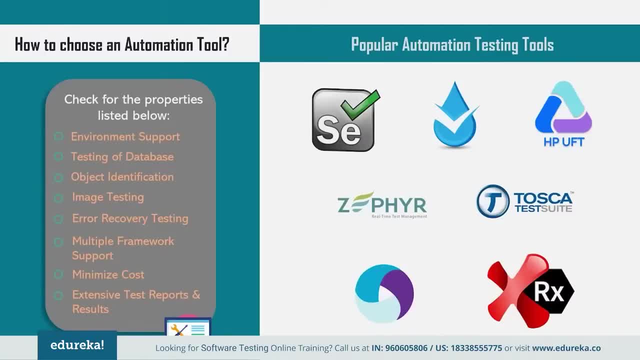 throughout all environments and browsers and devices. Then you have APM: It's a mobile testing tool. It is an open source mobile test automation software. Obviously, it's free and supported by a high active community of developers and experts. So, apart from these, you also have Zypher Tosca. 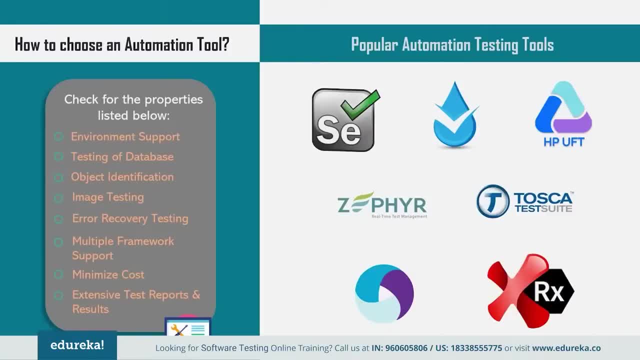 for end-to-end testing, Then HPE, or unified functional testing, which was formerly known as HP, quick test, professional or QTP, and I can just keep going. There are plenty of automation testing tools, So tool selection is one of the biggest challenges that need to be tackled before you actually start. 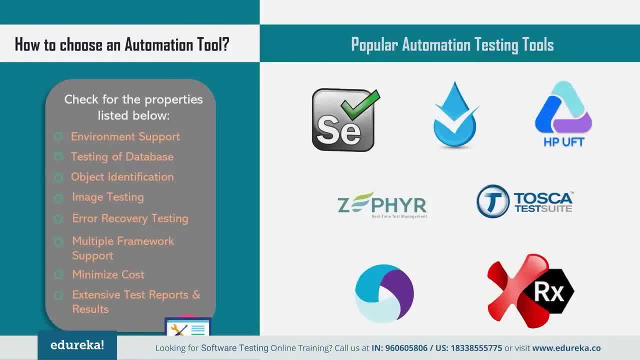 with your automation. So first identify the requirements, explore various tools, get to know them and their capabilities, set the expectations from the tool and go for a proof of concept. So that's how you choose a tool of your choice. So, guys, in some situations, automation testing is very important. 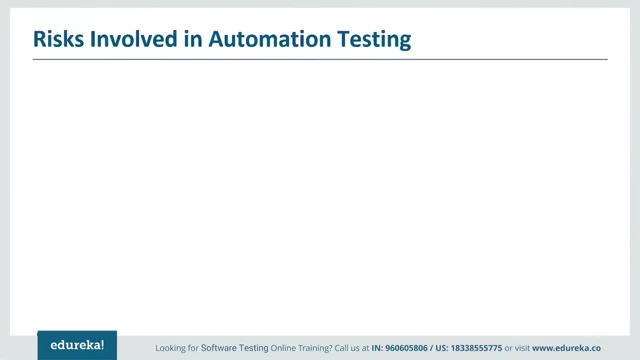 but as much it is comfortable, that much it is risky too. So if you decide to do automation testing, then think of following scenarios. first, starting cost for an automation is very high. automation tool purchasing cost, training and maintenance of test script- All these costs are very high because of this reason. 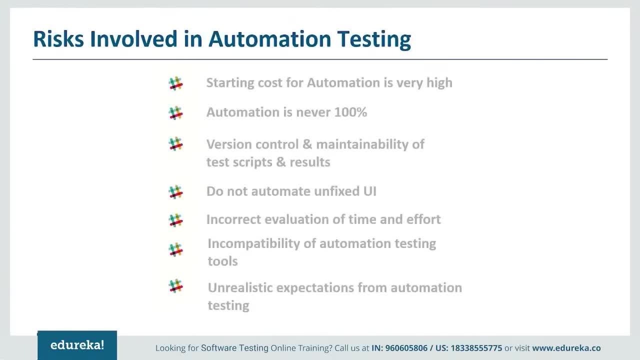 Some companies are worried to take decision to automate their work. Secondly, automation is not hundred percent automation. testing Cannot be hundred percent, and don't think of that. There are areas like user interface, documentation, installation, compatibility and recovery where testing should be done manually. You can't do all this using tools. 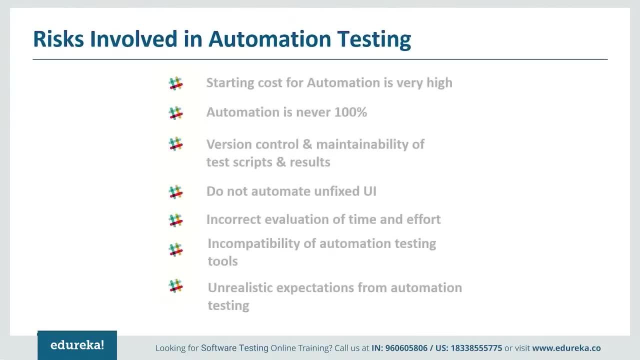 You need to have a person involved in this, and another risk that you might encounter is when you have unrealistic expectations from the automation testing tool. So, like I said earlier, know the requirement, study different kind of tools, get to know their capabilities and choose the tool. and then comes the incompatibility. 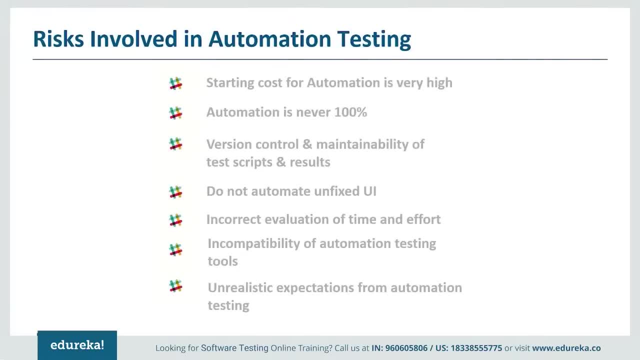 of automation testing tools with the test environment and other software testing tools in test environment. Then you have vendor issues like inability to provide technical support, inability to update the automation testing tools with changes in software testing platform. and all that and one more point: do not automate unfixed user interface. 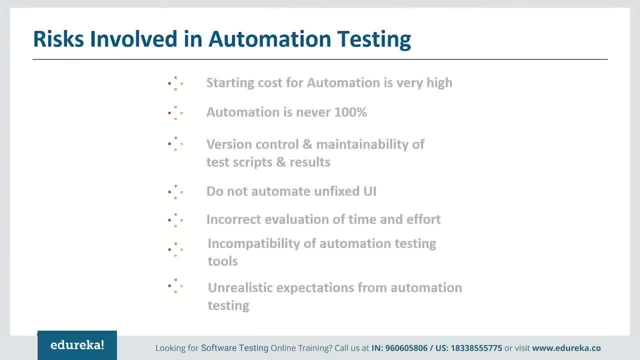 Be careful before automating user interface. if user interface is changing always, cost associated with script maintenance will be very high. So basic user interface automation is enough in such cases. by mentioning all this points, What I wanted to tell you is automation is not possible every time, and these are some cases. 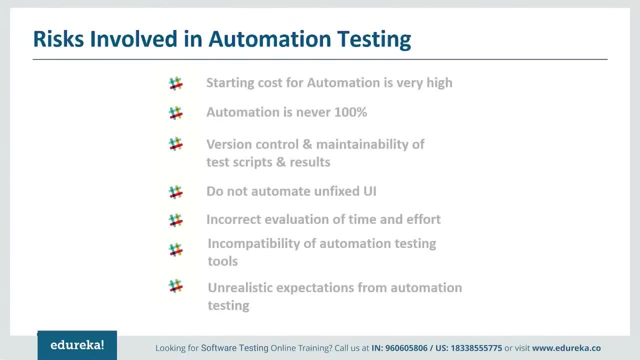 where you might have to start looking twice before you actually implement automation. you so, guys, there's no silver bullet for testing during the development process. despite the wide variety of techniques and tools, We cannot rely on a single approach: automated and manual testing each have this strength and weaknesses. 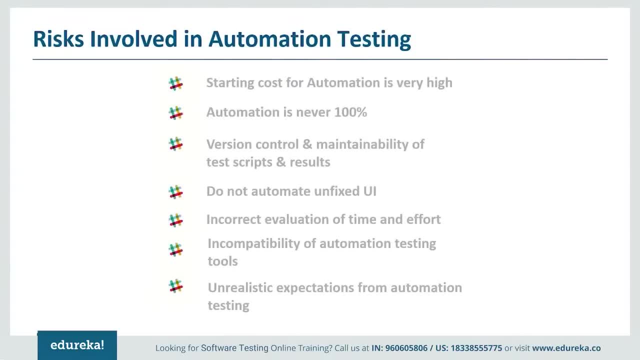 What we want to stress here is that, no matter how great automated tests are, you cannot automate everything. manual test play important role in software development as well, and they come handy when you cannot automate the process. So, guys, we have reached the end of the session and by now I'm sure you know what automation testing is. 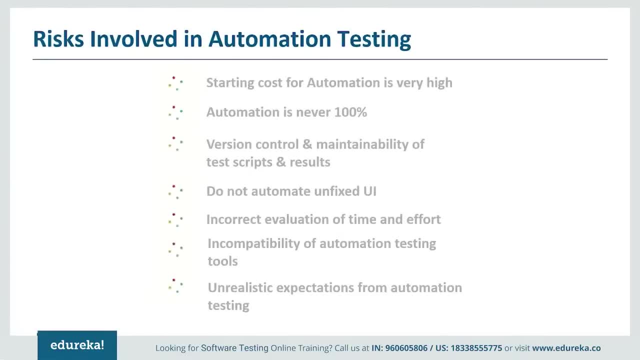 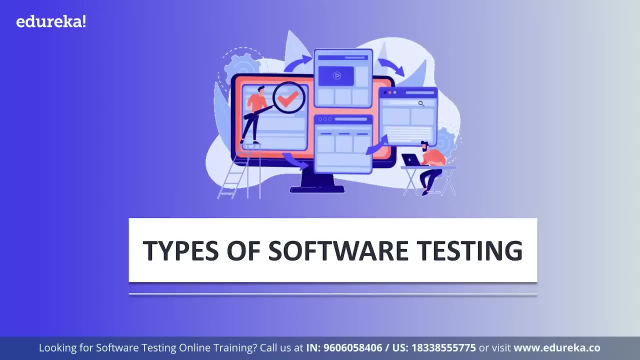 and benefits of using automation testing, when to use this and which test cases need to be automated, and how different it is from manual testing. So make sure to consider all these points when you go ahead with automation next time. So now let's see the different types of testing. 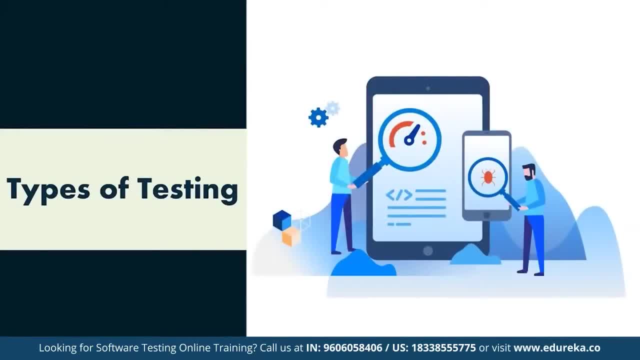 So quality assurance, or software testing, is crucial because it identifies errors, bugs from a system at the beginning by considering the problems in the base, helps return improvement in the quality of product and brings confidence in it. Now, by beginning, means where it comes, feasible and able to resolve the existing bugs now functional. 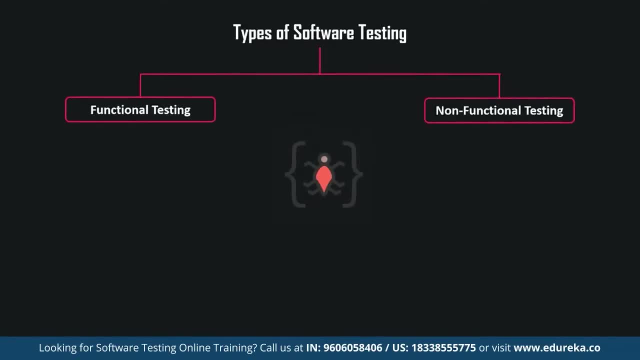 testing and non-functional testing are the two kinds of testing that are performed by the QA or the software tester. So the types of software testing are basically the key role where the tester determines the right testing for the apps. So here we have two main types of software testing. 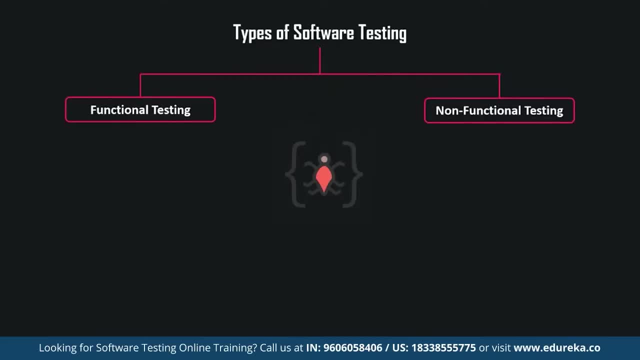 such as the functional testing and non-functional testing. Now, under functional testing, We have unit testing, integration testing, system interface regression and user acceptance testing, And under non-functional testing We have documentation, installation performance, reliability and security testing. also, performance testing can be divided into load, stress endurance and spike testing. 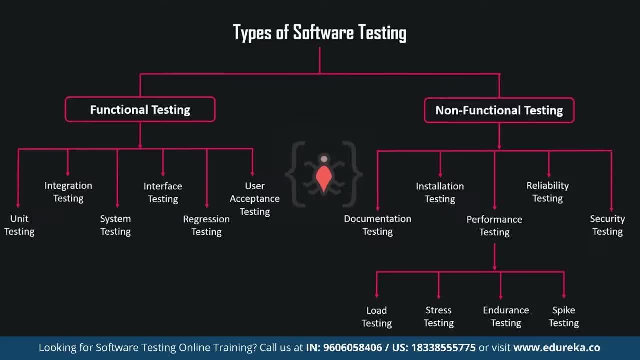 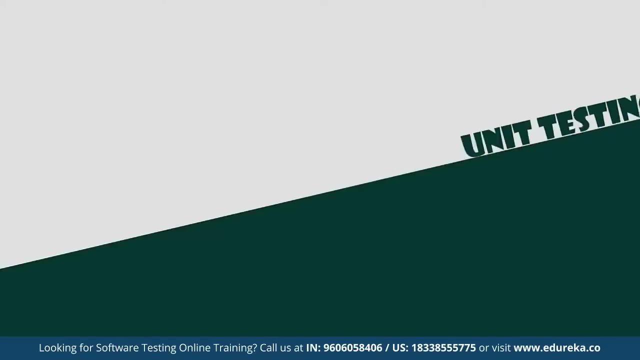 So now let's move ahead and have a look at all of these types of testing in details. So the functional testing focuses on manual as well as automation testing. a functional testing is a bunch of various types to execute the perfect product. Now, the first one is the unit testing under functional testing. 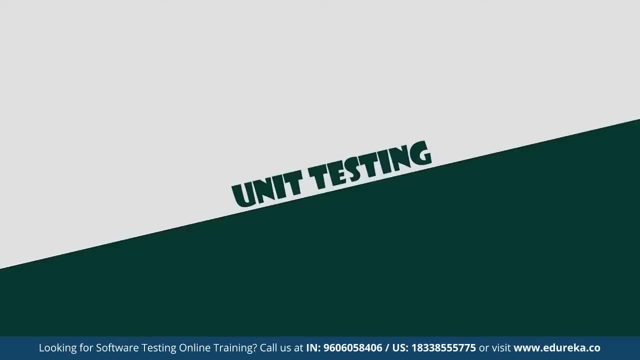 So unit testing is basically a level of software testing where individual units or components of a software are tested. Now the purpose is to validate each unit of the software performs as designed Now. a unit is the smallest testable part of any software. It usually has one or a few inputs. 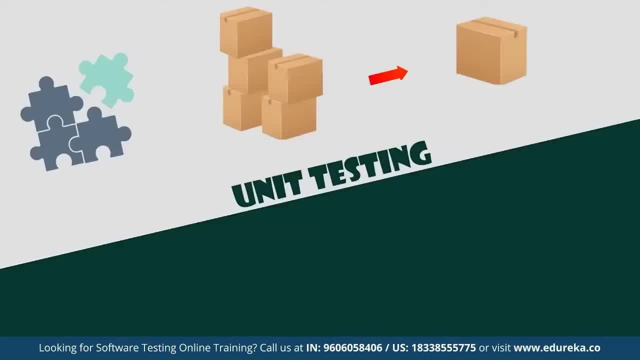 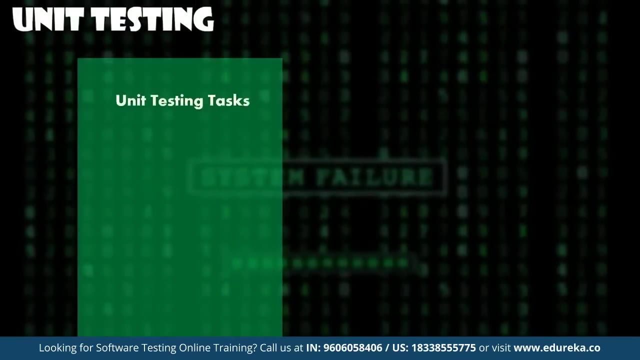 and usually just a single output. Now, who performs this unit testing? It is normally performed by the software developers themselves or their peers. Now, in rare cases, it may also be performed by independent software testers. Now let's have a look at the unit testing task. 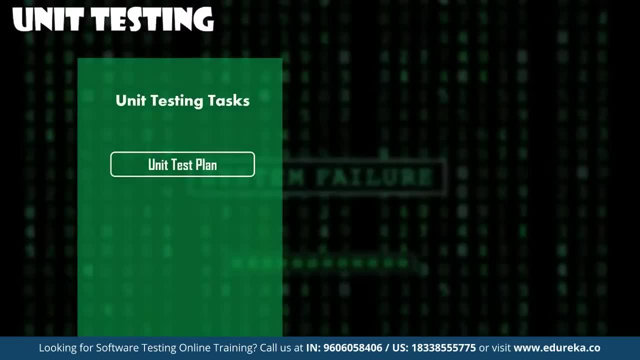 So first we have the unit test plan, under which we prepare, review, rework and form the baseline. Next up we have the unit test cases or scripts, where again we prepare, review, rework and check the baseline of the scripts. And finally We have the unit test step, where we perform our final task. 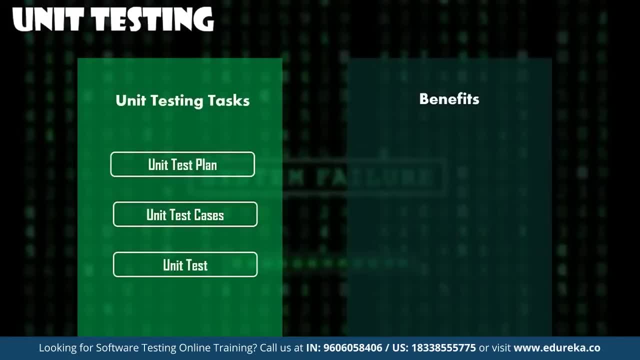 Now let's have a look at some of the benefits of unit testing. Now, unit testing increases confidence in changing or maintaining code. So if good unit tests are written and if they are run every time any code is changed, we will be able to promptly catch any defects introduced. 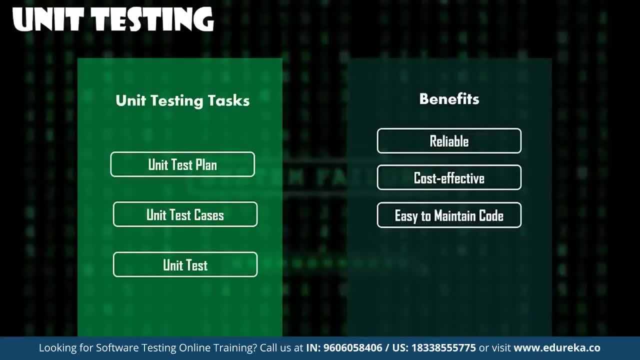 due to the change Next up, codes are more reusable. in order to make unit testing possible, Codes need to be modular Now. this means that codes are easier to reuse. Also, the development is faster Now if you do not have unit testing in place. 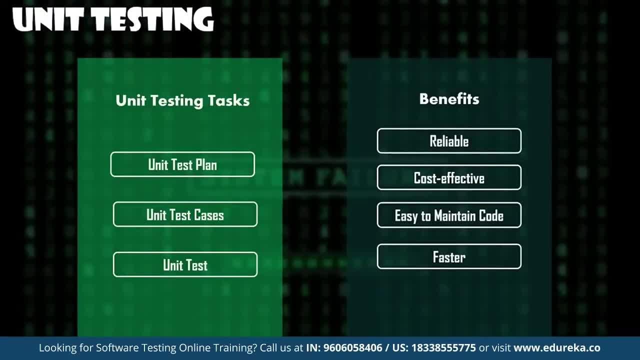 you write your code and perform that fuzzy developer test. But if you have unit testing in place, you write the test, write the code and run the test. Now, writing tests takes time, but the time is compensated by the less amount of time it takes to run the tests. 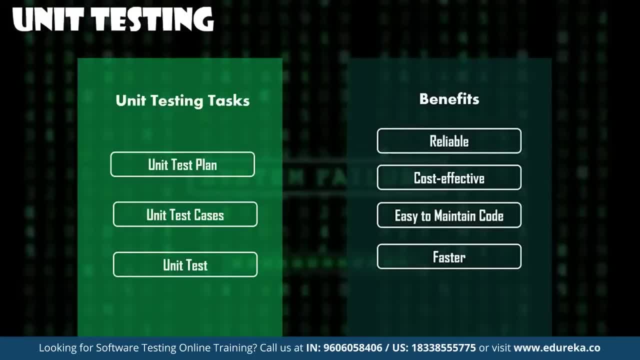 You need not fire up the GUI and provide all those inputs Now. the cost of fixing a defect detected during unit testing is lesser in comparison to that of defects detected at higher levels. So compare the cost of a defect detected during acceptance testing or when the software is live. 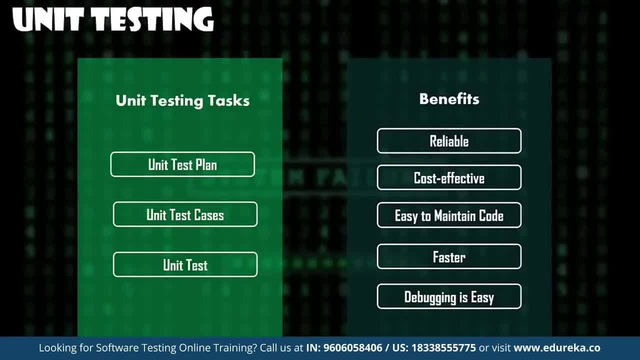 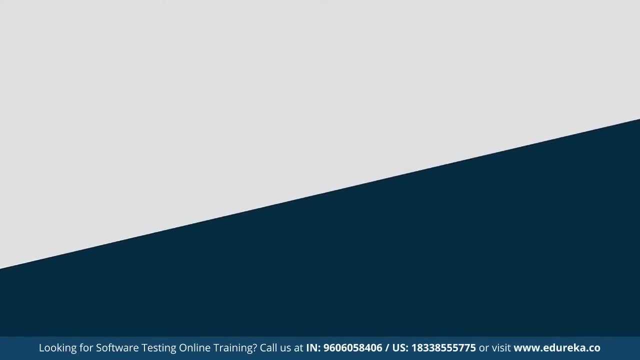 Next up, debugging is very easy. So when a test fails, only the latest changes need to be debugged. So with testing at higher levels, changes made over the span of several days or weeks or months need to be scanned. Also Are more reliable here. now moving on the next type. 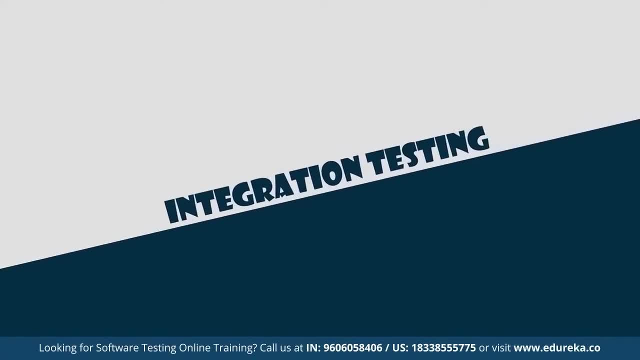 is the integration testing. So integration testing is a level of software testing where individual units are combined and tested as a group. So the purpose of this level of testing is to expose faults in the interaction between integrated units. test drivers and test stubs are used to assist in integration testing. 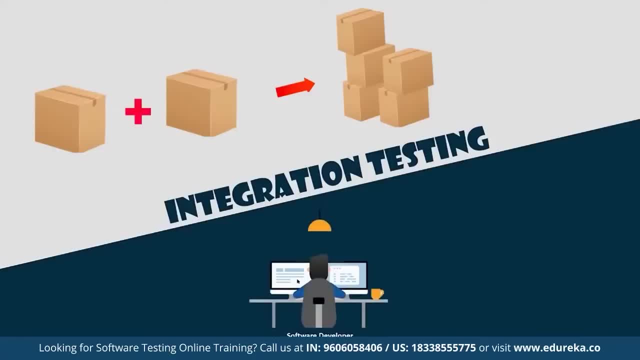 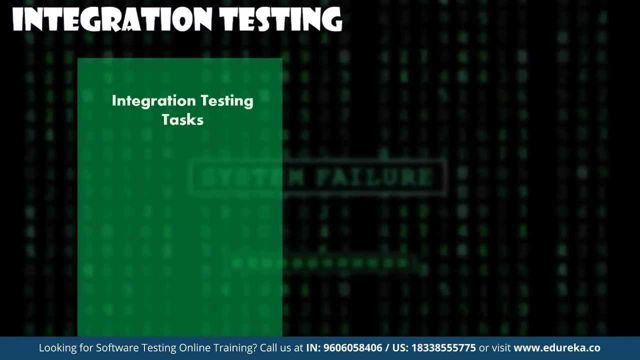 So who performs integration testing for this? the developers themselves or some independent Testers perform this sort of testing. integration testing also involves a task plan, such as the integration test plan, where we prepare, review, rework and form the baseline. Also, we have integration tests cases. 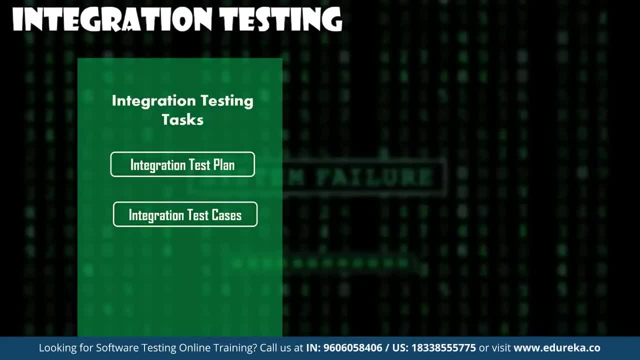 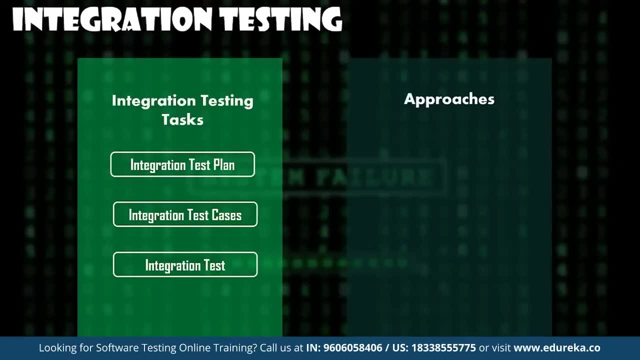 or scripts under which we prepare, review, rework and form the baseline And finally, again, we perform the integration test. Now let's have a look at some of the approaches of integration testing. The first one is the Big Bang. now, Big Bang is an approach. 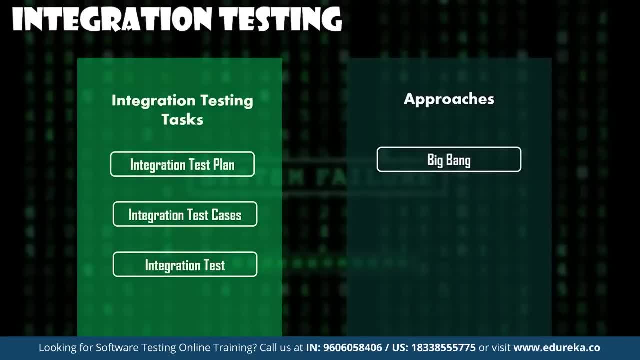 to integration testing, Where all or most of the units are combined together and tested at one go. Now this approach is taken when the testing team receives the entire software in a bundle. So what is the difference between Big Bang, integration testing and system testing? 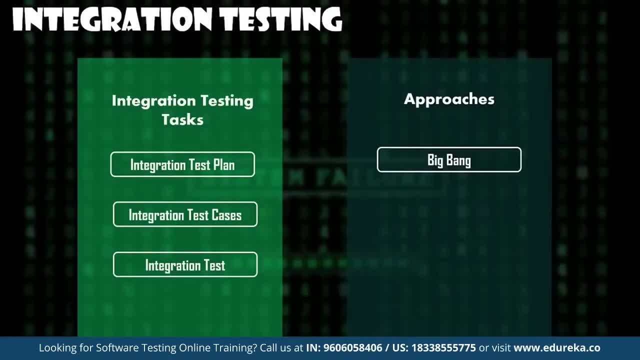 Well, the former tests only the interactions between the units, while the later test the entire system. Next up, we have the top down. Now this is an approach to integration testing, where top level units are tested first and lower level units are tested step by step after that. 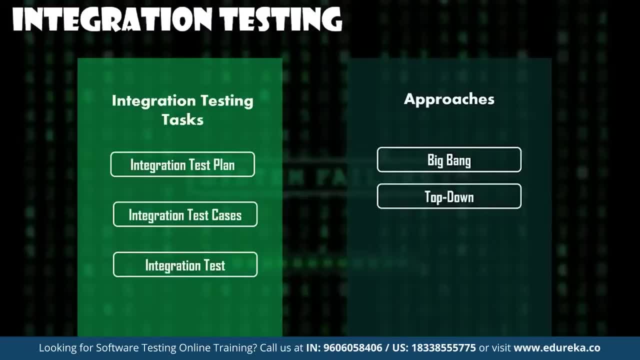 This approach is taken. when top-down development approach is followed, The test hubs are needed to simulate lower level units which may not be available during the initial phases. Next up, we have the bottom up. Now. this is an approach to integration testing, where bottom level units are tested first. 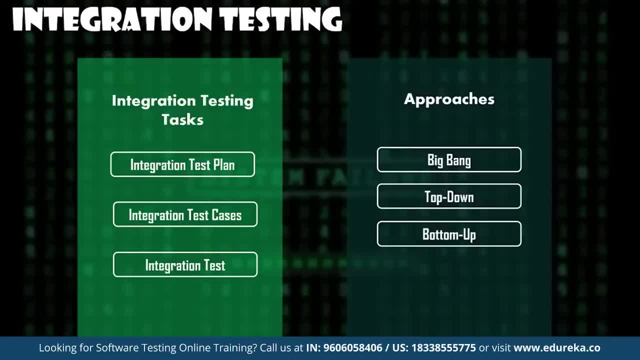 and upper level units step by step. after that, Now this approach is taken when bottom up development approach is followed. The final one is the sandwich or the hybrid. Now, this is an approach to integration testing, which is a combination of top-down and bottom-up approaches. 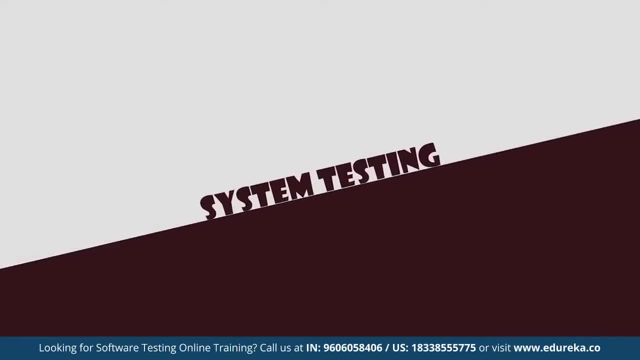 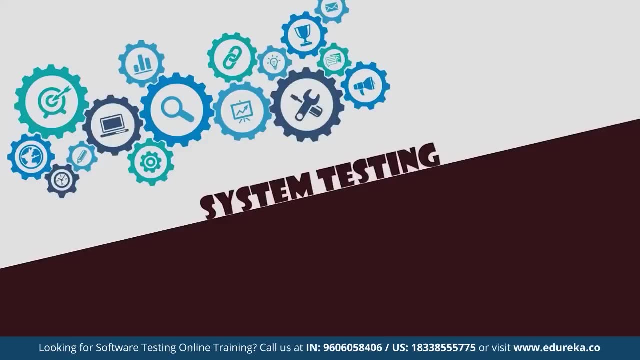 Next up, we have the system testing. System testing is a level of software testing where a complete and integrated software is tested. Now, the purpose of this test is to evaluate the system's compliance with the specified requirements. System testing is the third level of software testing. 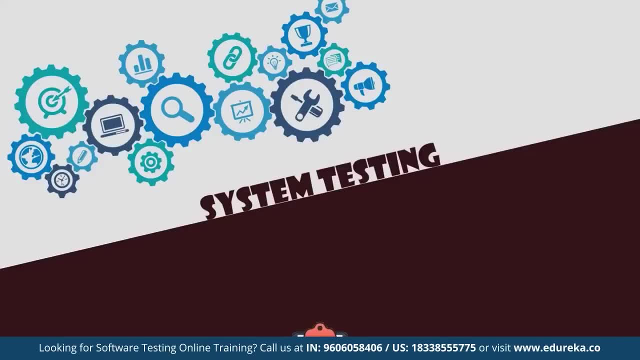 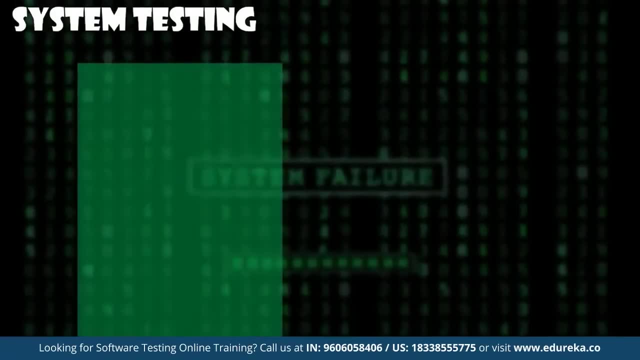 performed after integration testing and before the acceptance testing. So basically, the independent testers perform the system testing. Now again, the system testing also has certain tasks, such as the system test plan, where we prepare, review, rework and form the baseline, And next up we have the system test cases. 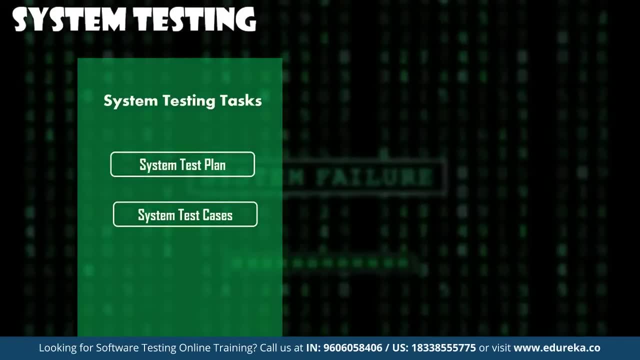 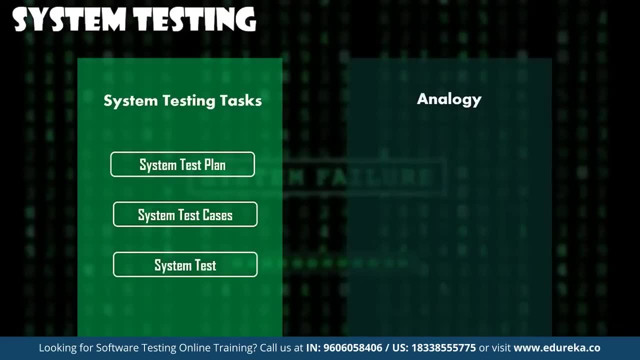 where we prepare, review, rework and form the baseline as well, and then finally perform the system test. Now let's have a look at an analogy of system testing Now, during the process of manufacturing a ballpoint pen: the cap, the body. 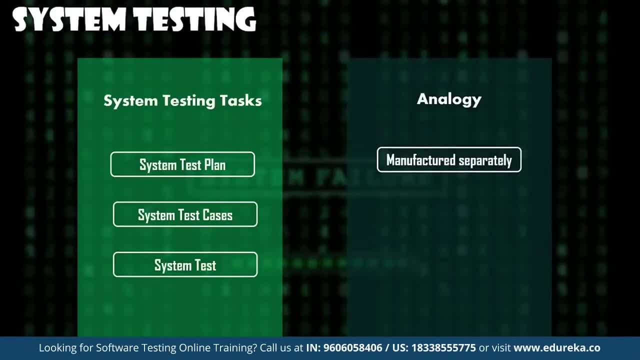 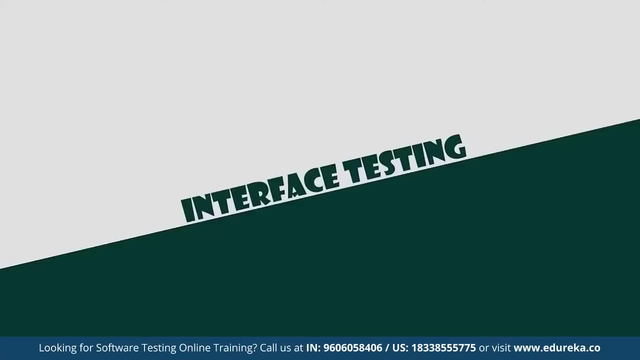 the tail, the ink cartridge and the ballpoint are produced separately and unit tested separately. so when two or more units are ready, they are assembled and integration testing is performed. now, when the complete pen is integrated, the system testing is performed. so this is all about the system testing. now let's move on and have a look at the interface testing. now it basically verifies: 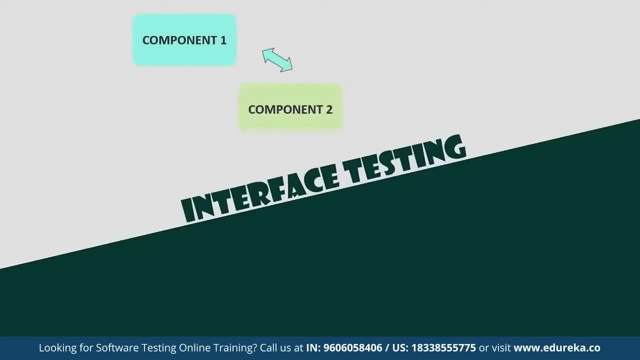 that communication between the systems are done correctly. if all supported hardware or software has been tested. now, when an application or a software or a website is developed, then there are several components of it. those components can be server, database, etc. now the connection which integrates and facilitates the communication between these components is termed as an interface. 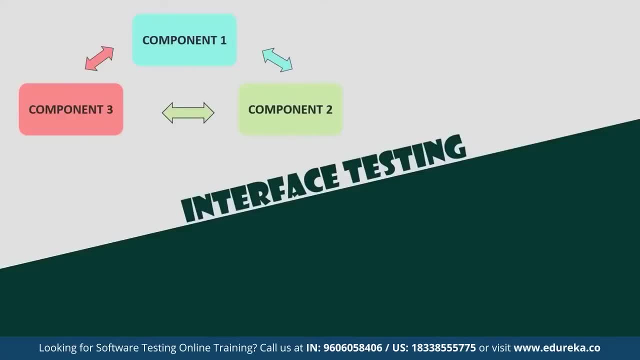 so there are three phases of interface testing in an interface life cycle. first, you're going to develop the interface. from the interface to the software, go through the First, we have the configuration and development. So when the interface is configured and once the development starts, the configurations. 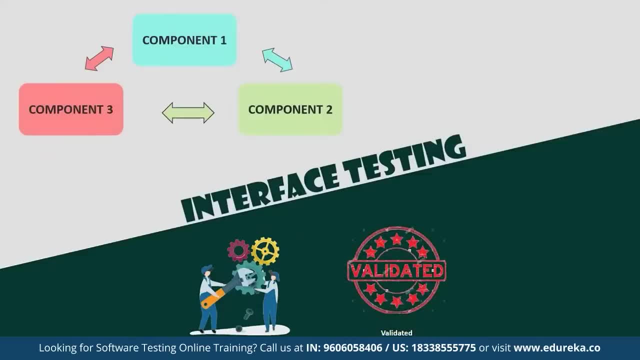 need to be verified as per the requirement. Next up is the validation. So when the development is completed, the interface needs to be validated and verified Now. this can be done as a part of unit testing also. Finally, we have the maintenance. now. 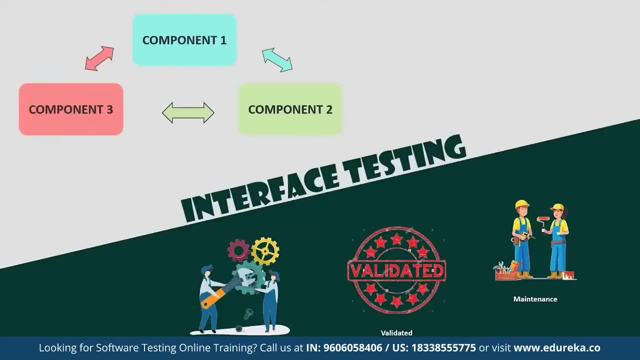 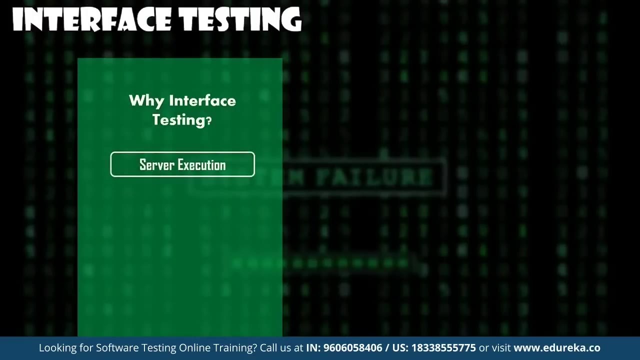 once the whole software is ready, deployed and working, then the interface needs to be monitored for its performance and any new issues introduced due to the changes made or deteriorating performance. Now let's see. Why do we have to perform interface testing? So it is required to check if the server execution is proper. 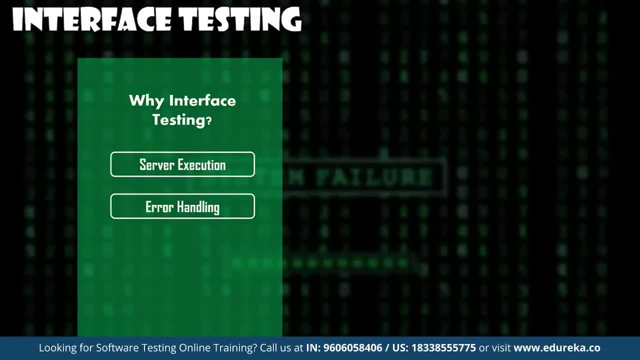 Now error handling is done properly and appropriate error messages are shown for queries made by the application or software. It is also used to check the result when a connection to the server is reset and also to check the security aspect when the components communicate within themselves: interface testing. 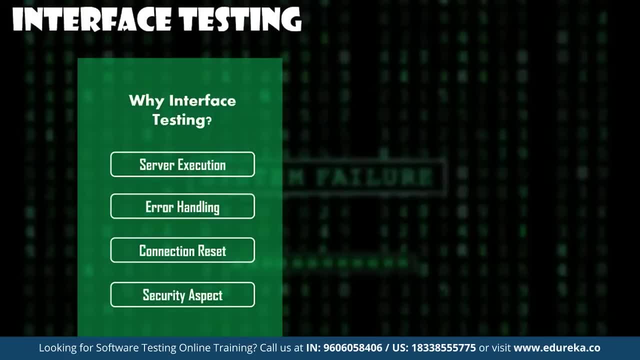 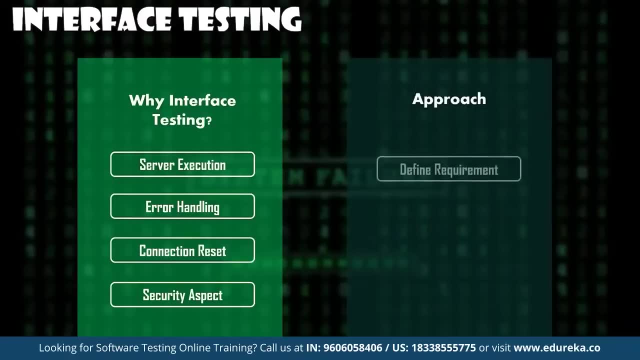 is also done to check the impact of Network failure on the communication between the components. Now let's have a look at few steps that ensure interface testing is successful. First one is define your requirement now, before creating the interface tests, It is essential to understand the application. 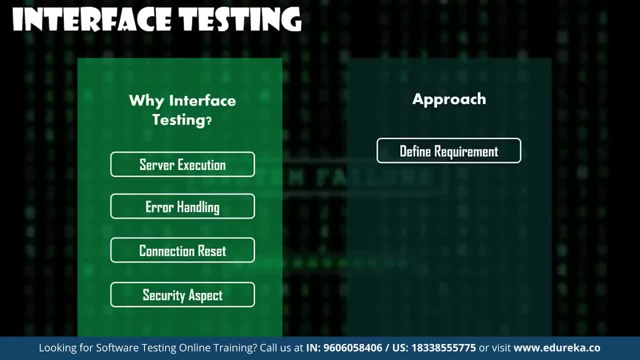 hence try to find answers to questions like: what is the purpose of the interface or what is the workflow of the system or application? now, defining all such answers will help you to understand the requirement. Next up is the expected output. Now we know and understand the requirement very well. 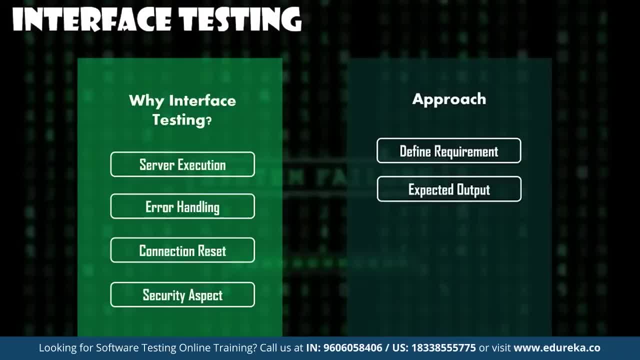 It is the time to finalize the output that we will be expecting from the tests, not just a pass or fail. It can be some data call to another API Etc. Third one is start small. So with interface testing we can't directly move on with creating big test cases. 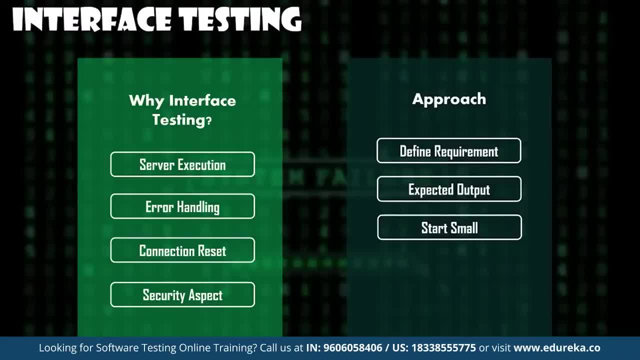 creating small test cases or calls is relatively simple, at least in small functions. Create small test code and verify if the output is as expected or not. next, try automating now. writing codes for testing and interface can be boring. You will not only be spending time in writing the code. 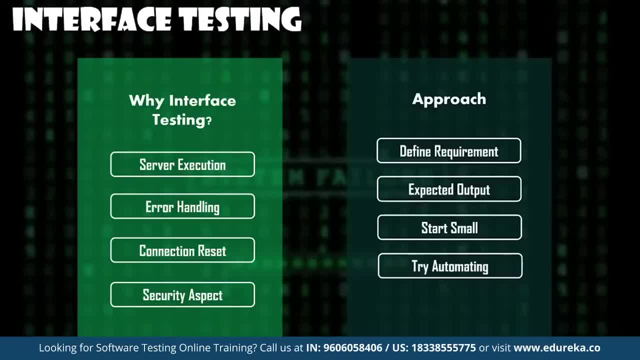 but along with this, you will also have to spend time to understand the format, style, the coding language used for development. and then, as an icing on the cake, you will have to make sure that your code isn't creating a problem to the app or system code. 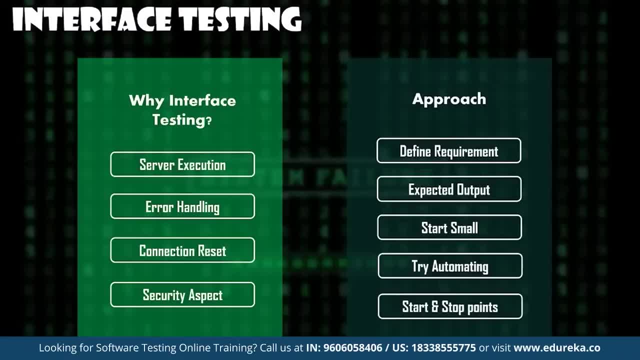 Finally, define the start and stop points. now, before starting the execution of a test, We always decide the start and the stop point of the test, as well as decide how the entire testing process will start and end. next up, We have the regression testing. now, regression testing. 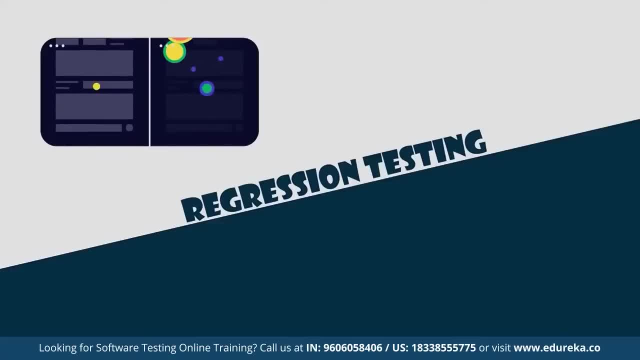 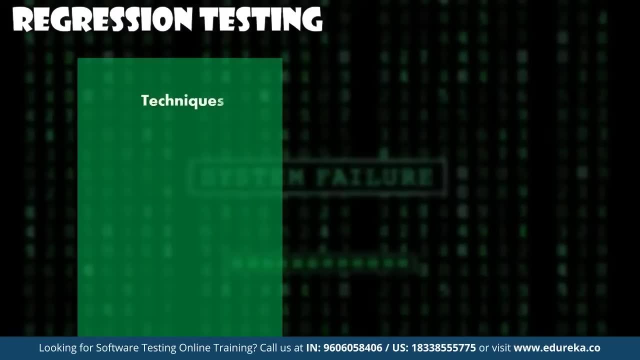 is a crucial stage for the product and very useful for the developers to identify the stability of the product with the changing requirements. Now let's have a look at some of the techniques of regression testing. First one is retest- all now as the name itself. 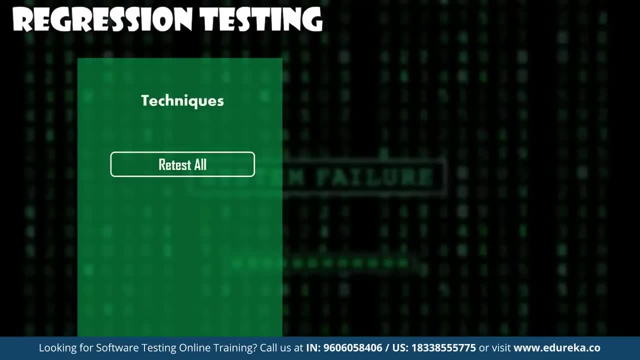 suggests the entire test cases in the test suit are re-executed to ensure that there are no bugs that have occurred because of a change in the code. next up, We have the regression test selection. now, in this method, test cases are selected from the test suit to be re-executed. 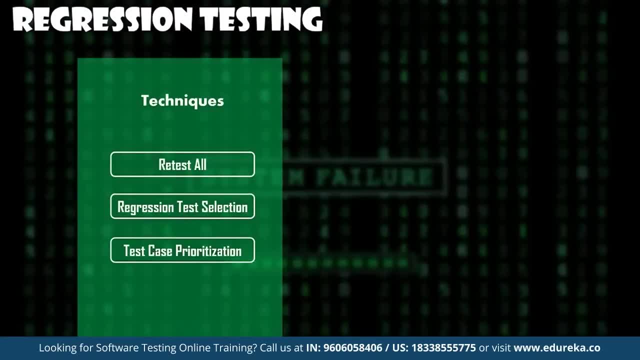 Not the entire suit is re-executed here. Next up, We have the test case prioritization. test cases with high priority are executed first, then the ones with medium and low priority. Finally, we have the hybrid technique. Now, this is a combination of regression test selection. 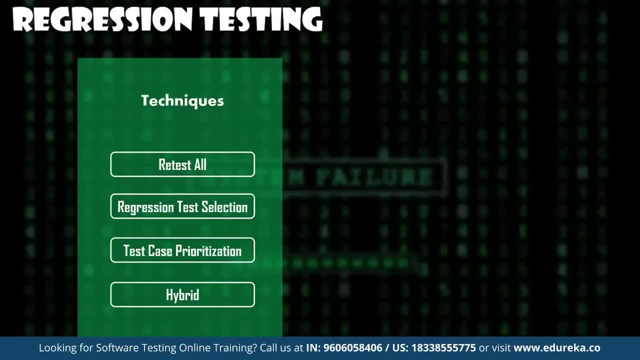 and test case prioritization. Now how do we select the regression test suit for? most of the bugs found in the production environment occur because of the changes did or bugs fixed at the 11th hour, that is, the changes done at a later stage. 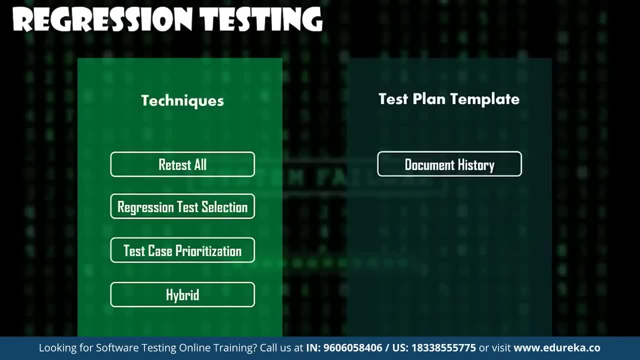 So let's have a look at the test plan template. first We have the document history. now it consists of a record of the first draft and all the updated ones. next, We have the references column. that keeps a track of all the reference documents used or required for the project while creating a test plan. next up, 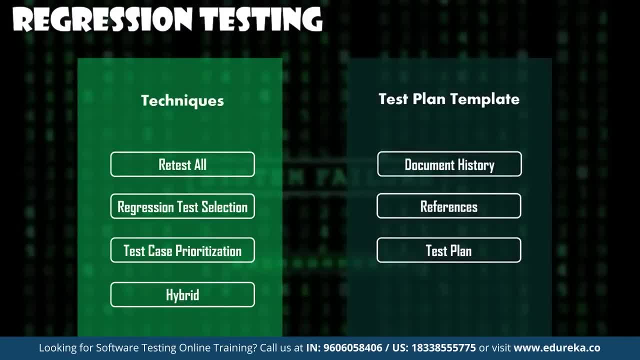 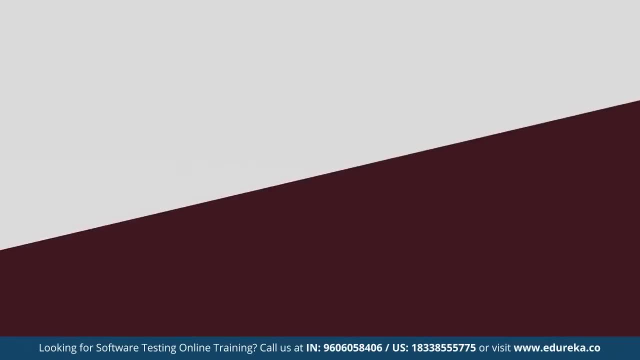 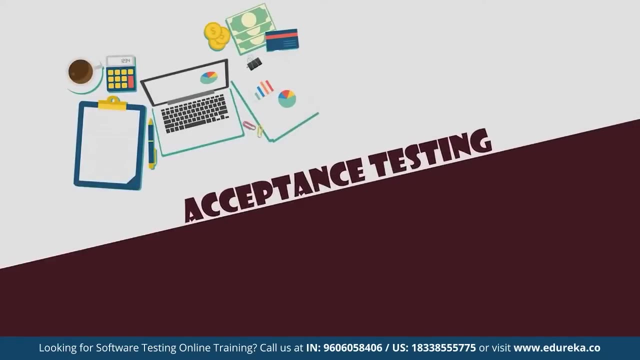 We have the regression test plan. that consists of all the introduction and details that are involved in the testing. Now the final one in functional testing is the acceptance testing. now, acceptance testing is a level of software testing where a system is tested for acceptability. The purpose of this test is to evaluate the system's compliance. 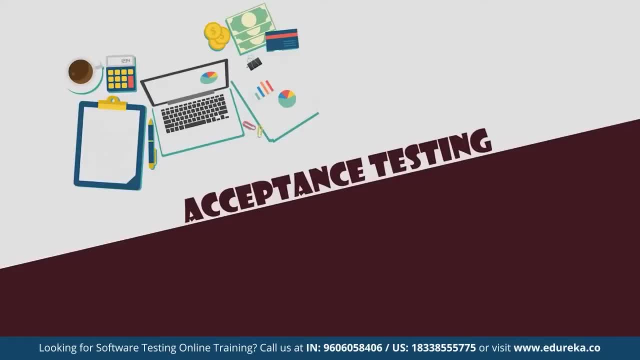 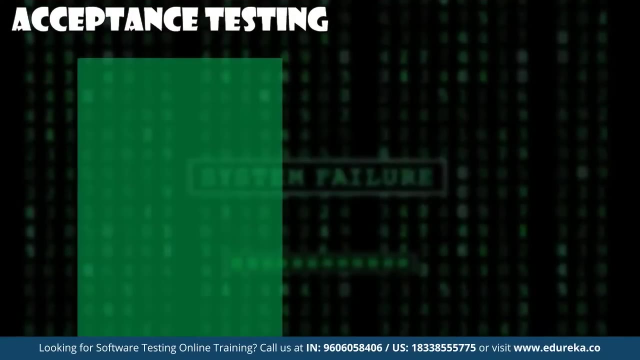 with the business requirements and assess whether it is acceptable For delivery. So basically the management, sales or the customer support performs these kind of testing also. the customers and the end users of the software can do the following: acceptance testing also has a task plan, such as the acceptance test plan. 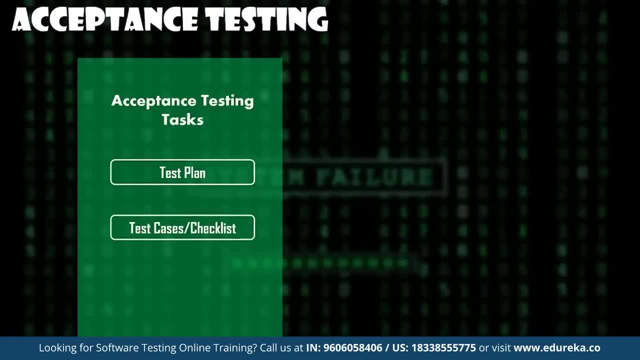 where we prepare, review, rework and form the baseline. and then we have the acceptance test cases or checklist, where we again prepare, review, rework and form the baseline and finally perform the acceptance testing. Now let's have a look at some of the types of acceptance testing. 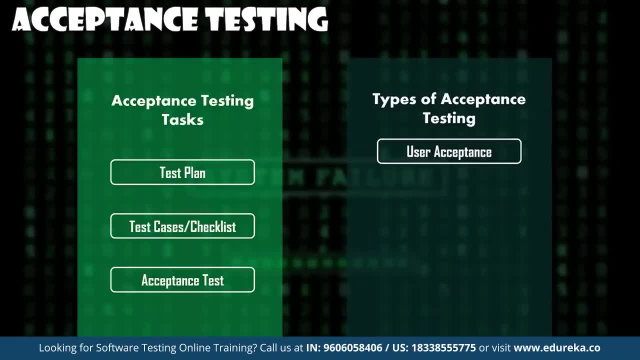 First one is the user acceptance testing. Now this is used to assess whether the product is working for the user correctly for the usage. next up, We have the business acceptance testing. Now this is required to assess whether the product meets the business goals and purposes. 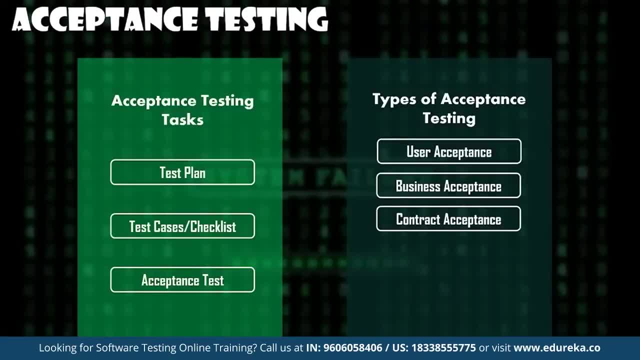 or not. next we have the contract acceptance testing. Now, this is a contract which specifies that once the product goes live within a predetermined period, the acceptance test must be performed, and it should pass all the acceptance use cases. Then we have the operational acceptance testing. 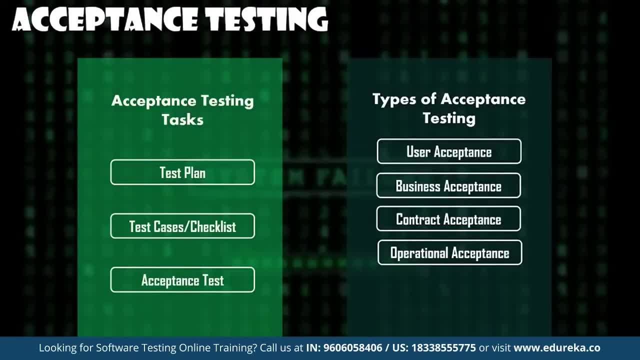 Now this is to assess the operational readiness of the product and is a non-functional testing. It mainly includes testing of recovery, compatibility, maintainability, technical support, availability, reliability, failover, localization, Etc. Then we have the alpha testing. Now this is to assess the product in the development. 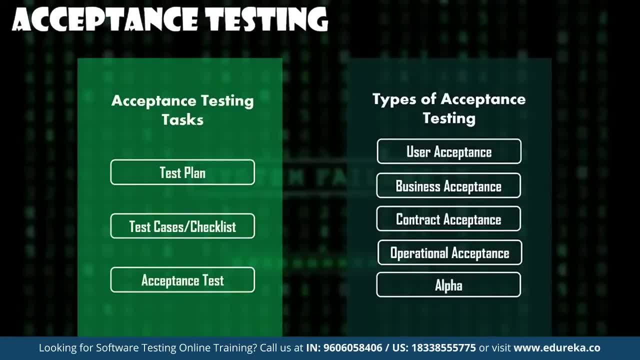 or testing environment by a specialized testers team, usually called the alpha testers. And finally, we have the beta testing. now this is to assess the product by exposing it to the real end users, usually called the beta testers, or beta users in their environment. Now, these were some of the functional testing now. 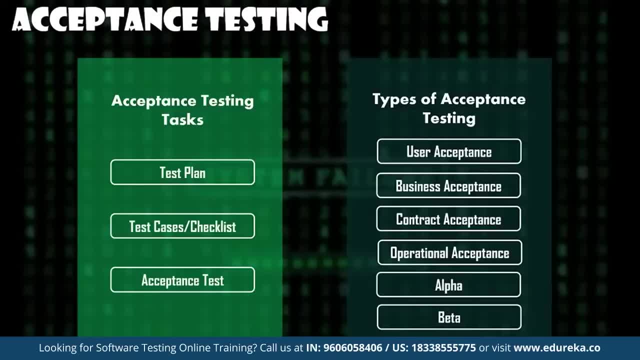 let's move on and have a look at some of the non-functional testing types. Now there are a bunch of software testing types which differentiate the job: work for the QA while testing the apps. it is a testing to determine the performance of the system, to measure the measure. 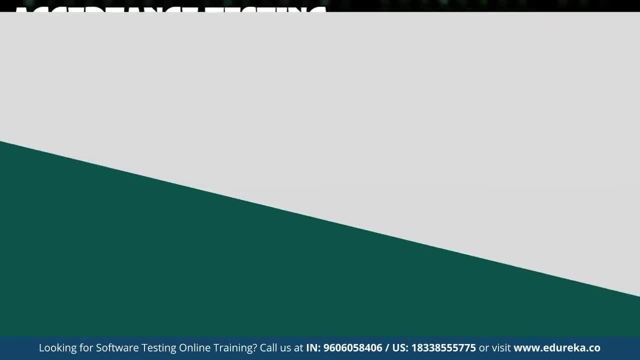 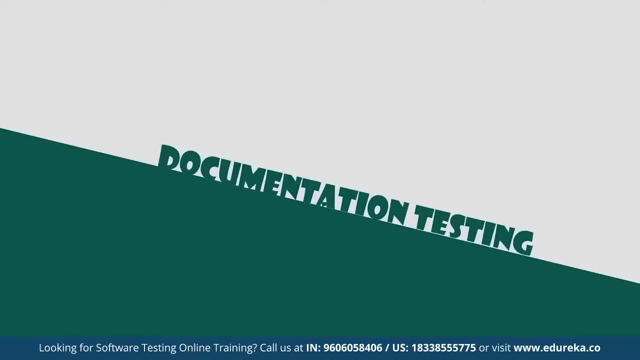 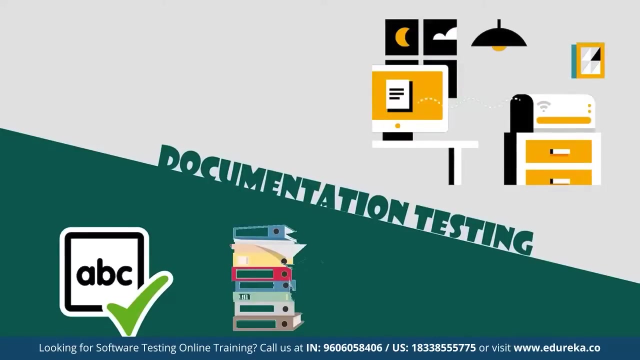 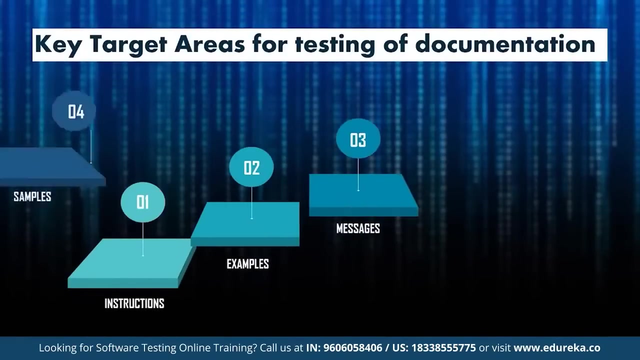 Validate or verify quality attribute of the system. The first one is the documentation testing. now documentation testing helps to estimate testing efforts required and test coverage. now software documentation includes test plan, test cases and requirements section. So there are four main focus areas when testing documentation, that is, instructions, examples, messages and samples. 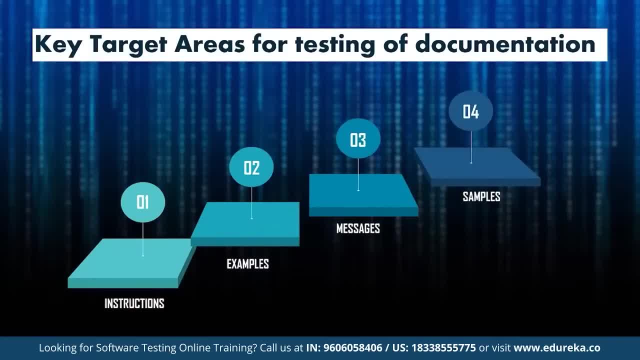 So specific instructions are provided for certain activities. It's likely we will have test scenarios defined for those same activities. Similarly, step-by-step examples may be provided to explain GUI screen inputs, clarify syntax for commands or other interfaces, show expected outputs or illustrate other important points. 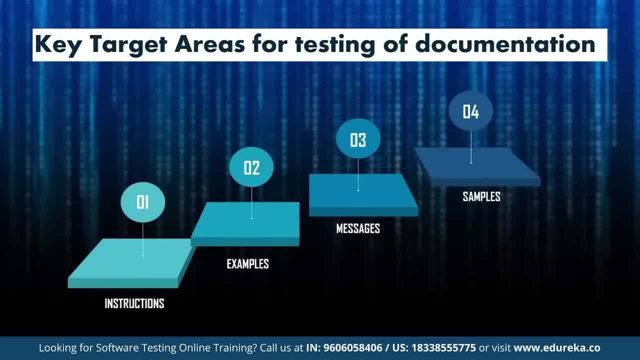 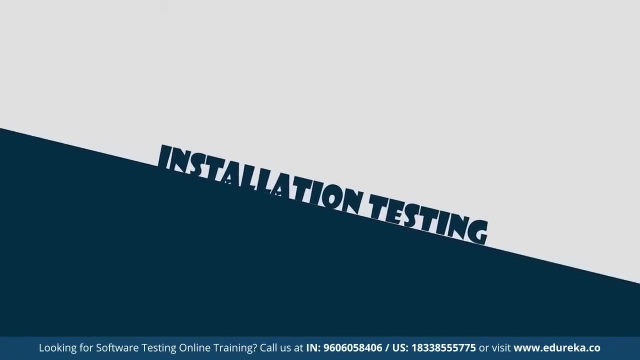 Now, when we hit a problem, for example an error message, we should verify that the documentation for the message is correct. Now, finally, samples are sometimes documented for such things as initialization Or tuning parameter input files. Now, next up, we have the installation testing. 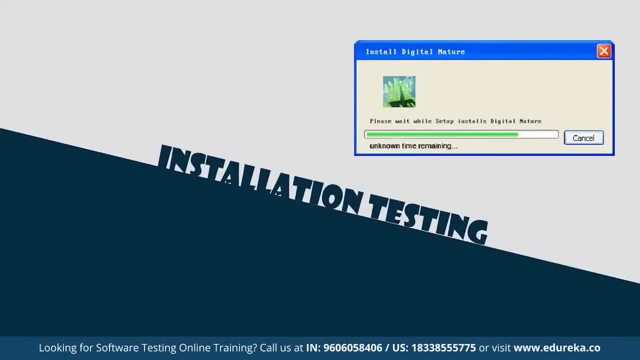 So installation testing is a type of quality assurance work in the software industry that converges on what customers will need to do to install and set up the new software successfully. Now the testing process may involve full, partial or upgrades, install or uninstall processes. Now let's have a look at some of the installation testing tips. 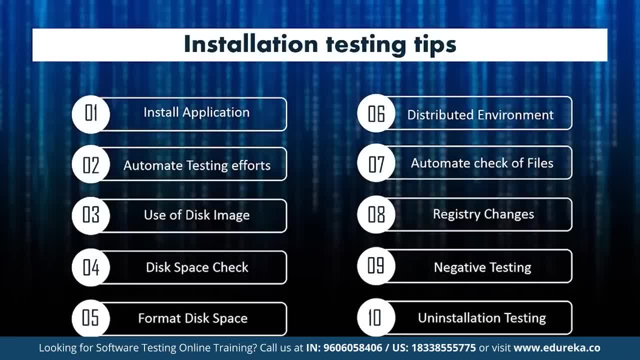 First, We need to install the full version Of application now. in case, if you are upgrading the application or previously installed a basic version, now installing the full version on same path, then system should allow you to install full version application without any error. Next we have the automate testing efforts. 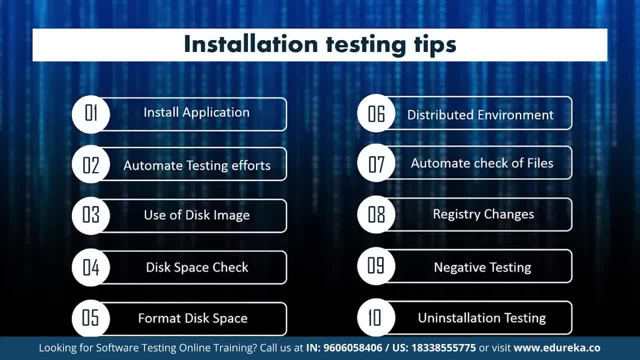 and the flow chart will help you to create the automated scripts. using the flow chart, You can easily make out the automated script for installation testing now, after execution, every test case use of the disk image to be installing on dedicated machine, Which will save some time next up. 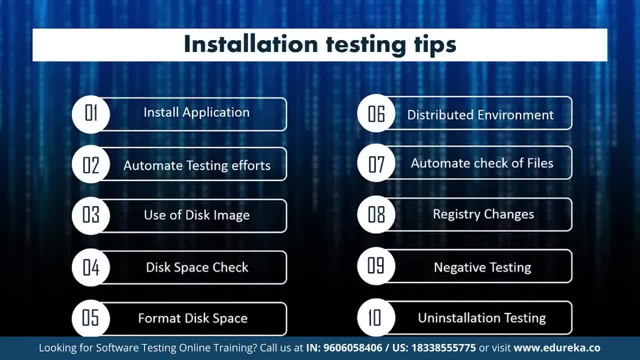 We have the required disk space check in installation. Now. this is the most critical scenario in the installation testing. Now the disk space checking is done using automated and manual testing method So you can verify calculated disk space by installer is correct or not by using manually or automated tools. now. 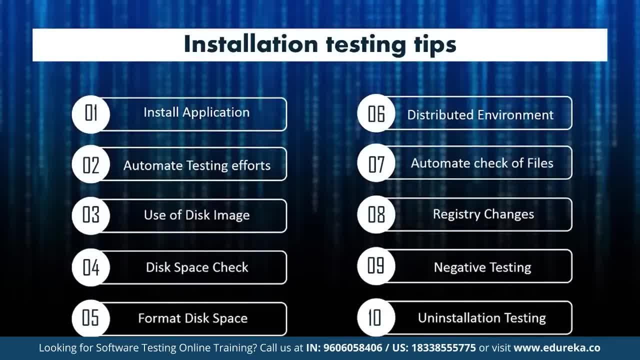 on different file system format. the disk space may vary, like on NTFS F80, 32 and F80 16, Etc. Next we have the use of distributor testing environment. now to executing test cases effectively. you can use distributor testing environment, which will save your cost and time. next we have the automate. 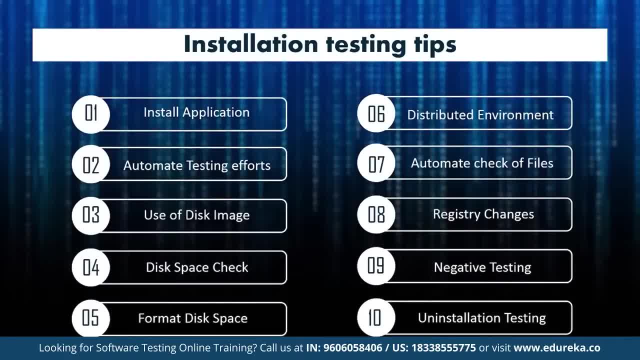 the check of files installed after installation. So you can use the automated script to check that all the required files are installed successfully or not. then we have the confirm for registry changes after installation. So here you have to check for registry changes after the installation of your software. 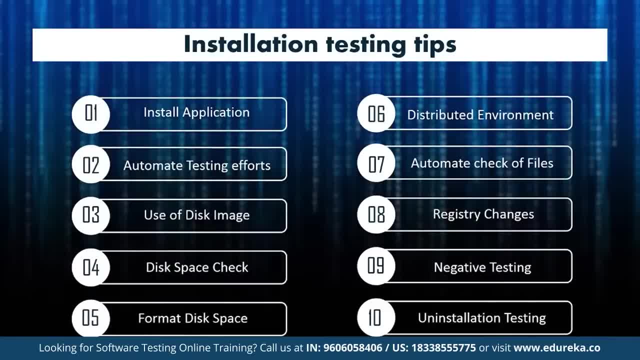 Then we have the negative testing and installation testing. now this intensely tried to break the installation process to check the behavior of application under such conditions. Finally, we have the uninstallation testing. Now you should also check for the uninstall testing, to check whether the user is able. 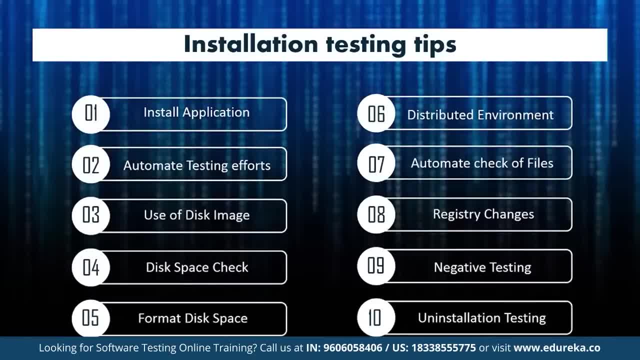 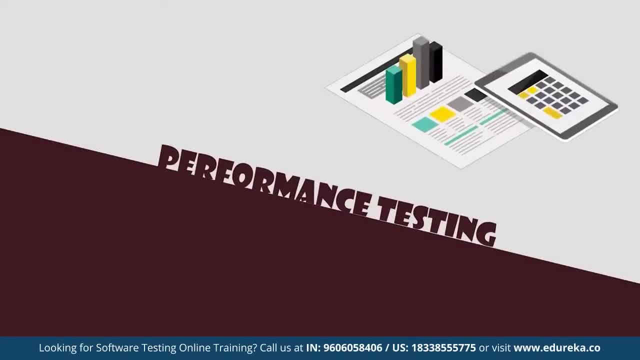 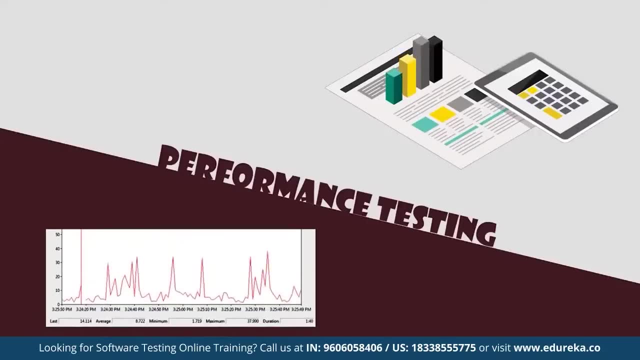 to uninstall the application without any error and removing all folders and files related to installation. Next up, We have the performance testing. now the performance testing includes load testing, Stress endurance and spike testing. now, here the software tester team provides performance testing on amazing projects. 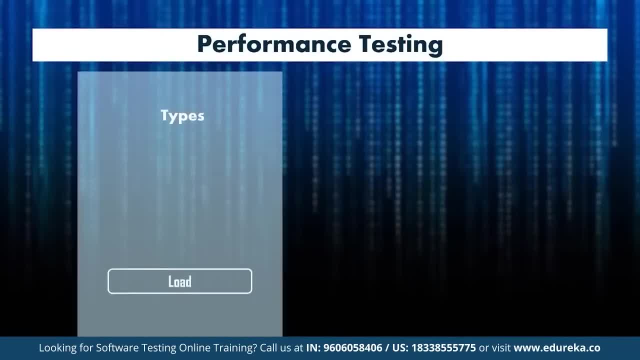 Now let's have a look at the types of performance testing. So we have load testing, which is a type of performance testing conducted to evaluate the behavior of a system at increasing workload. Then we have the stress testing, which is a type of performance testing conducted to evaluate. 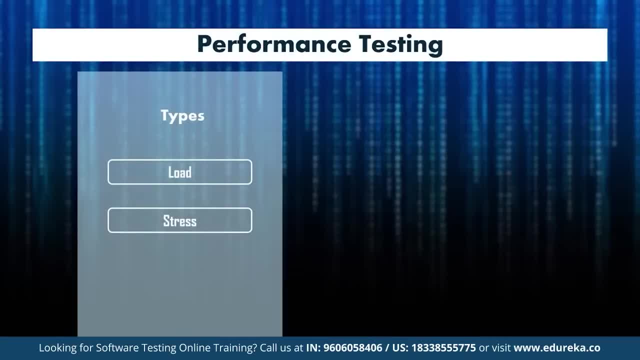 the behavior of a system at or beyond the limits of its anticipated workload, that we have the endurance testing, which is a type of performance testing conducted to evaluate the behavior of a system when a significant workload is given continuously. Finally, we have the spike testing, which is a type of performance testing conducted to evaluate 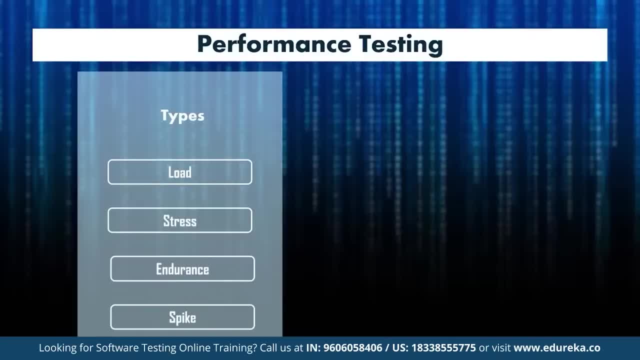 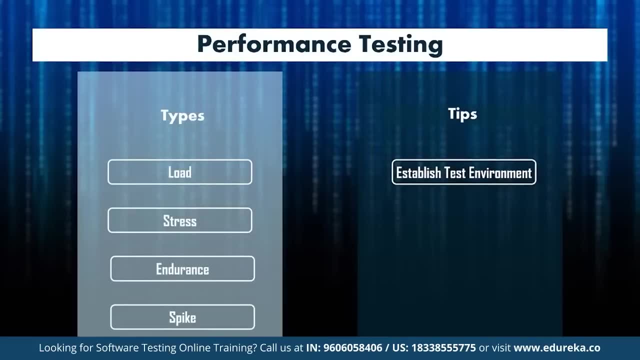 the behavior of a system when the load is suddenly and substantially increased. now let's have a look at some of the tips for performance testing. So first we have to establish a test environment as close to the production environment as possible. Then we have to isolate the test environment even from the QA. 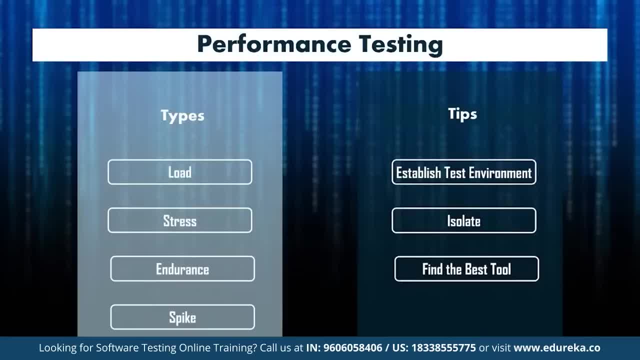 or U80 environment. though There is no perfect tool for performance testing, research and decide on the tool that best fits your purpose. Also, do not rely on the results of just one test. You should conduct multiple tests to arrive at an average number. be wary of any changes to the test environment from one test. 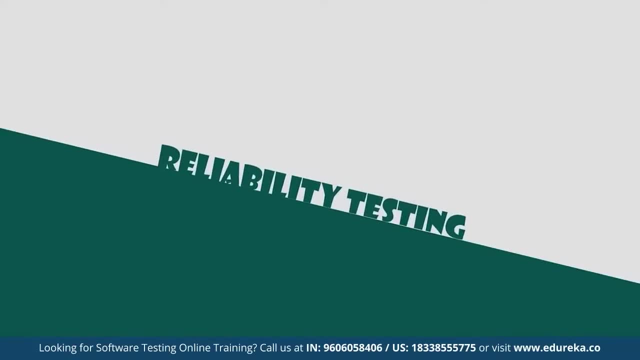 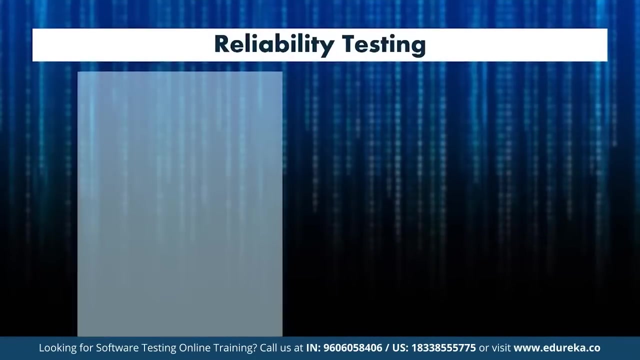 to the other. next up, We have the reliability testing. Now, reliability testing assures that the product is fault-free and is reliable for its intended purpose. It is about exercising an application so that failures are discovered before the system deployed. Now let's have a look at some of the types of reliability testing. 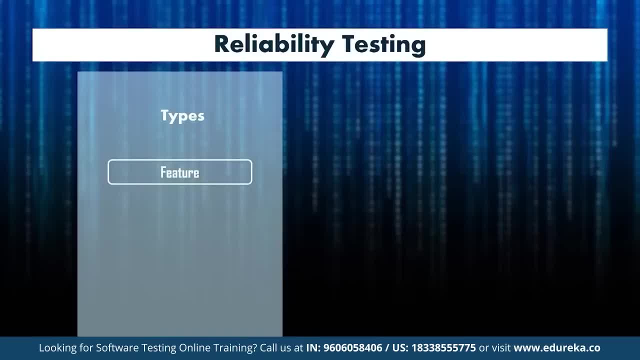 First We have the feature test. now in this, each function in the software should be executed at least once, and the interaction between two or more functions should be reduced. Also, each function should undergo proper execution or functional test. Next we have the regression test. 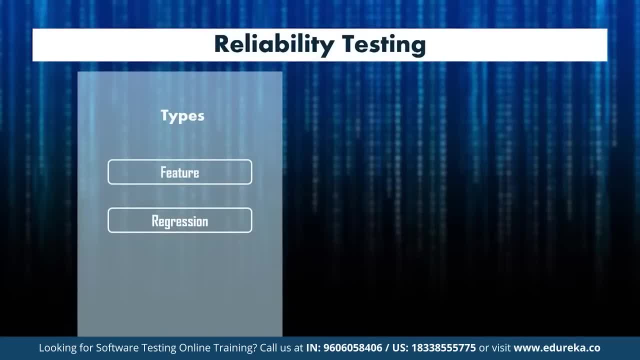 So whenever any new functionality is added or old functionalities are removed in an application, it undergoes a regression test to make sure with introduction of Q functionality, No new bugs are introduced. then we have the load test. Now load test is done to test whether the application is supporting the required load. 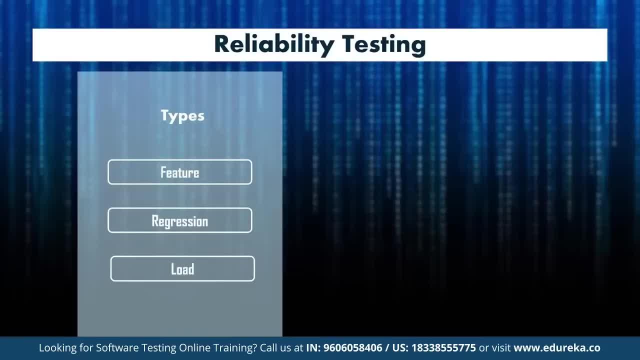 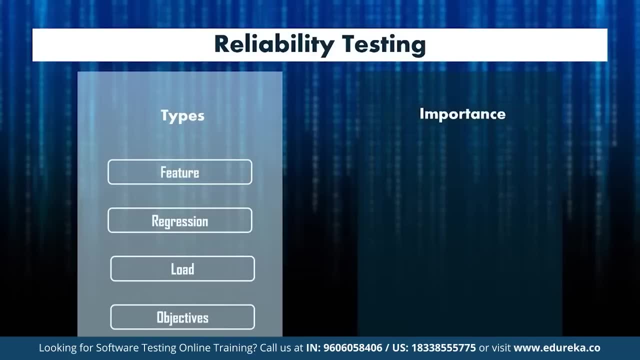 without getting break down now. in order to find the breakpoint of an application, The load is gradually increased until the application gets hung. Now let's have a look at some of the importance of reliability testing. as we know, software applications are in use in almost every sector of manufacturing: healthcare, defense government. 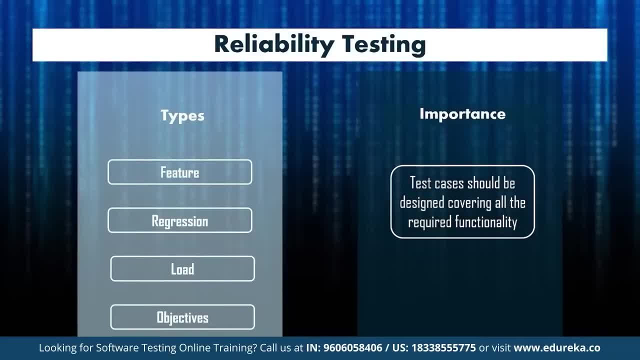 telecommunication, Etc. Therefore, the question is that how reliable the software application is. this question is very important because the reliable software is of great use and the organization working on it can feel the confidence in their business systems. Now the test cases should be designed covering all the required functionality. 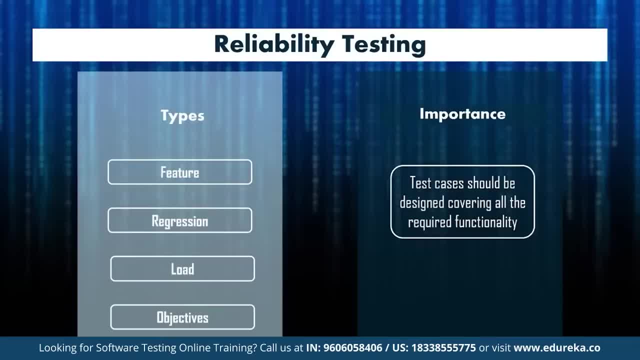 of the software application, And these test cases should be executed for sufficient amount of time to get a rough estimate of how long the software can execute fine without failure. Now the test case execution sequence to run the overall functionality of the software application should match these real production operational plan. 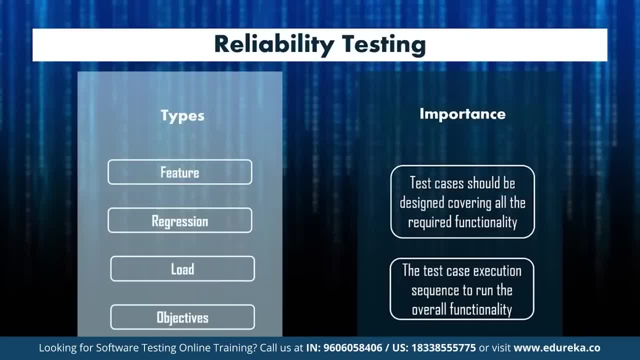 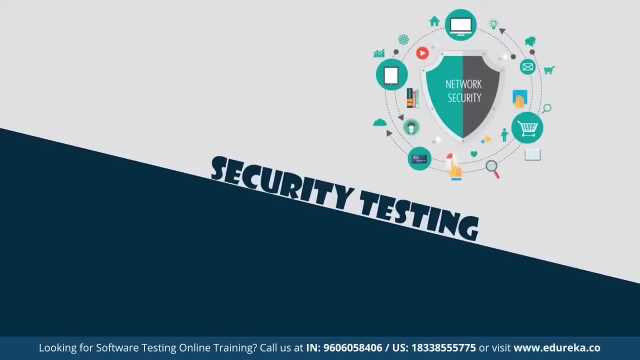 of the application. now, moving on, Let's have a look at the final type of non-functional testing. The next type is the security testing. now, the security word itself defines that something has to run, Relate with technique to strengthen the security. It's not about securing data and information. 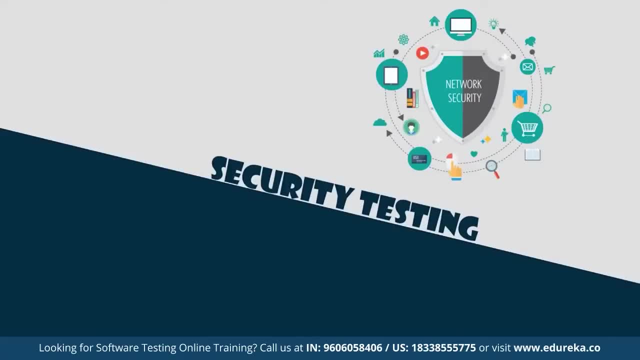 It can affect the whole functionality of the system. So there are basically four main focus areas that are to be considered in security testing. That is the network security, which involves looking for vulnerabilities in the network infrastructure. Then we have client security, which ensures that the client cannot be manipulated. 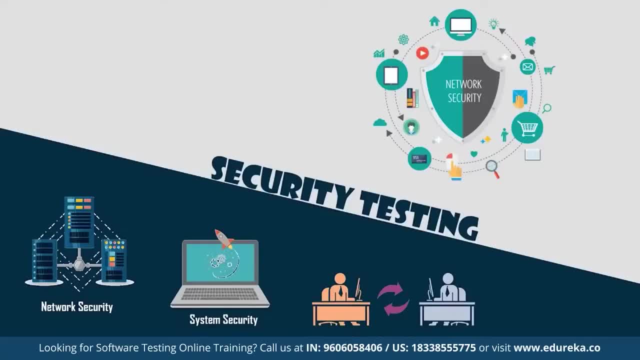 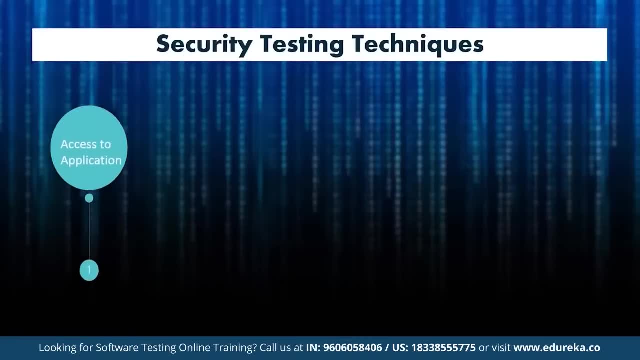 and the server code and its Technologies are robust enough to fend off any intrusion. Now let's have a look at some of the security testing techniques. First one is access to application. So, whether it is a desktop application or a website access, security is implemented by roles and rights management. 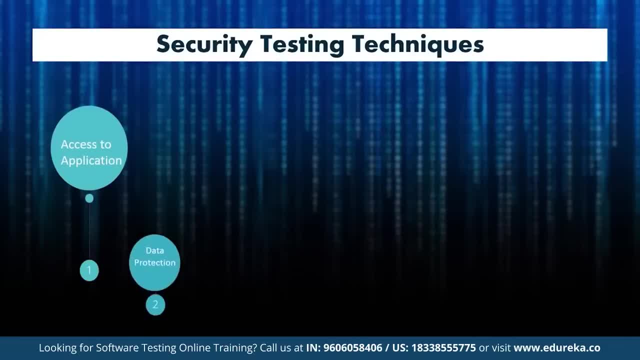 It is often done implicitly, while covering functionality, then we have the data protection. Now there are three aspects of data security. First one is that a user can view or utilize only the data which he is supposed to use. The second aspect of data protection is related to how 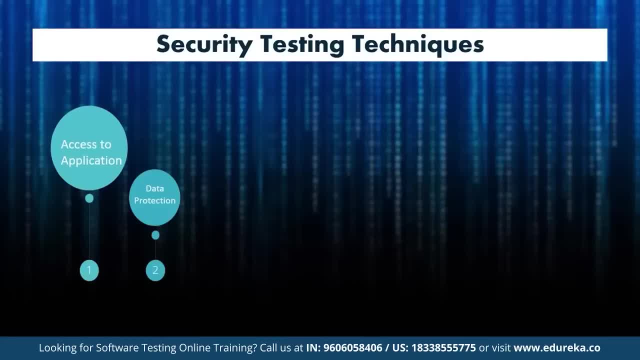 that data is stored in the database. and the last one is an extension of the second aspect. proper security measures must be adopted when the flow of sensitive or business critical data occurs. Next up, we have the brute force attack. Now, the brute force attack is mostly done by some software tools. 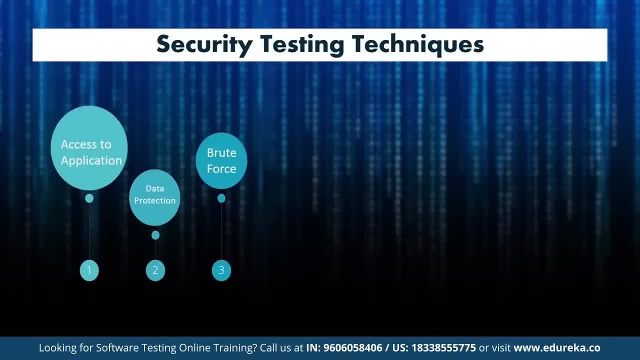 The concept is that by using a valid user ID, the software attempts to guess the associated password by trying to log in again and again. then we have the SQL injection and XSS. So conceptually speaking, the theme of both days hacking attempts is similar. 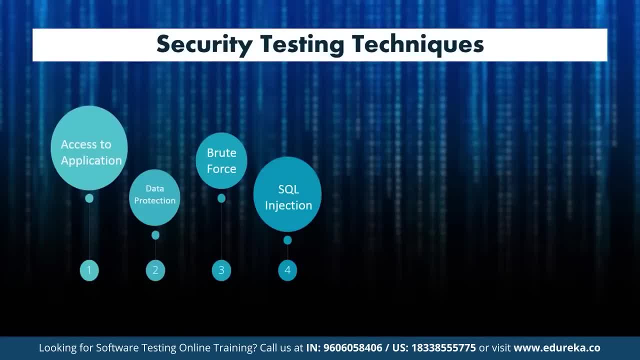 So for all input fields of the website, field length should be defined small enough to restrict input of any script. Then we have the service access points. So when there is a large number of the target audience, the access points should be open enough to facilitate all users. 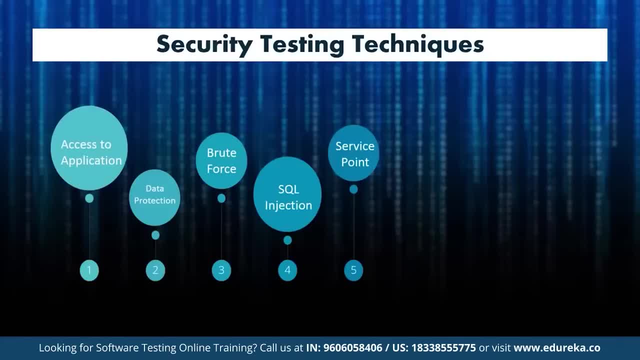 accommodating enough to fulfill all users requests and secure enough to cope with any security trial. Next up we have the session management So you can test for session expiry after particular idle time. session termination after maximum lifetime. session termination after logout. check for session cookies: scope. 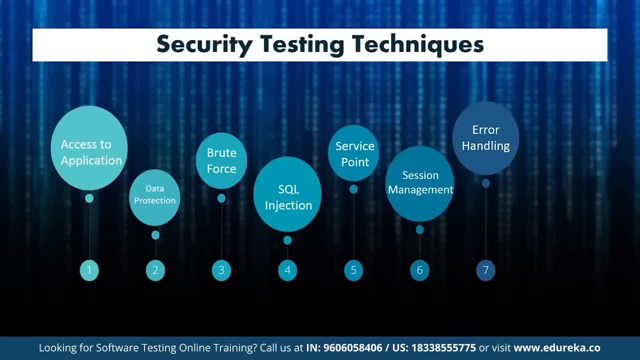 etc. Then we have the error handling, So the error codes are returned with a detailed message. These messages should not contain any critical information that can be used for hacking purpose. Finally, we have the specific risky functionalities. Now, mainly the two risky functionalities are payments. 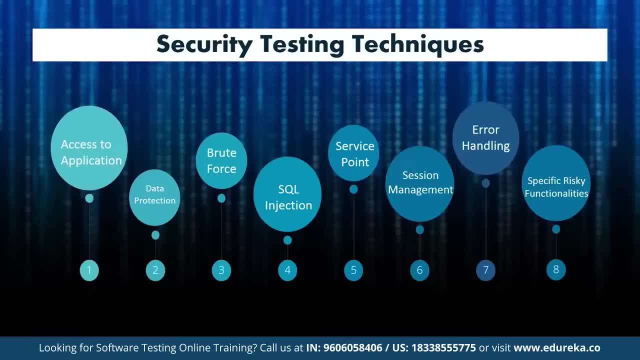 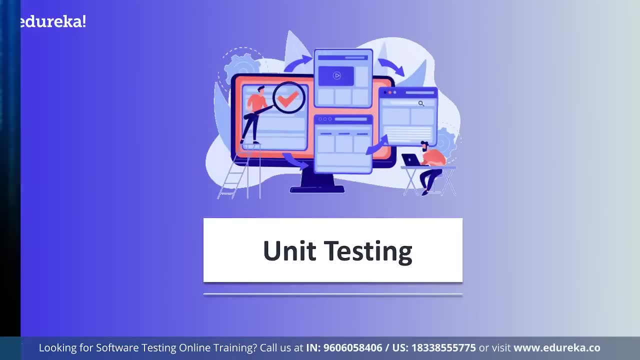 and file uploads. These functionalities should be tested very well. So these were the different types of software testing that are involved in our everyday life. So the most basic type of testing is unit or component tested. The goal of unit testing is basically to segregate each 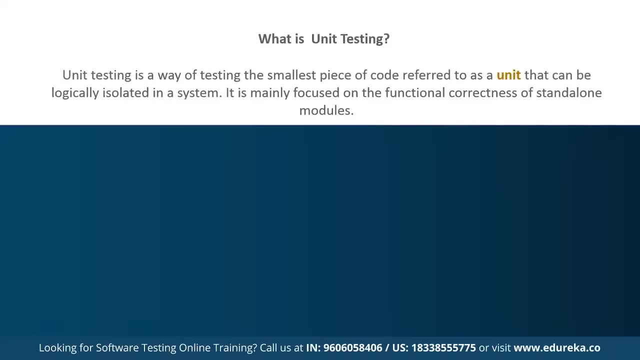 part of the program and test those part individually to check if they're working properly or not. So it isolates the smallest piece of testable software from the remainder of the code And determines if it behaves exactly as you expected and according to your requirements or not. 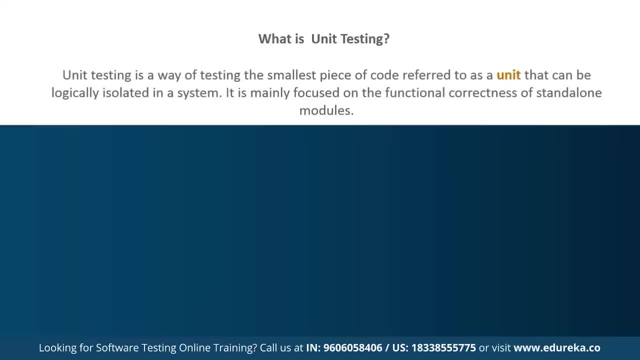 Generally, those small pieces of software that have been telling before are usually referred to as unit. So this unit can be almost anything you want it to be. It can be a line of code, It can be a method or a class or some sort of program or a. 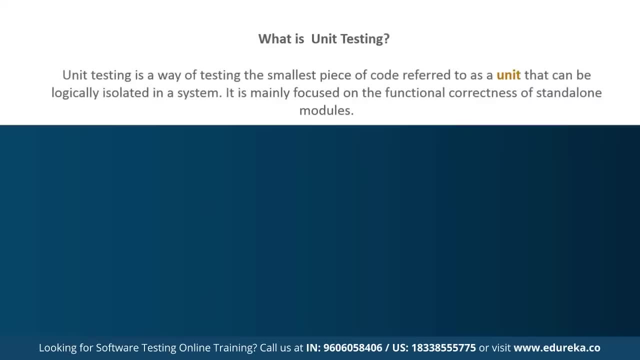 part of application program anything but smaller, the unit test. It's always better smaller test give you much more granular view of how your code is performing At basic level. There is also the practical aspect that when you test very small units, you test can run very fast like a thousand test. 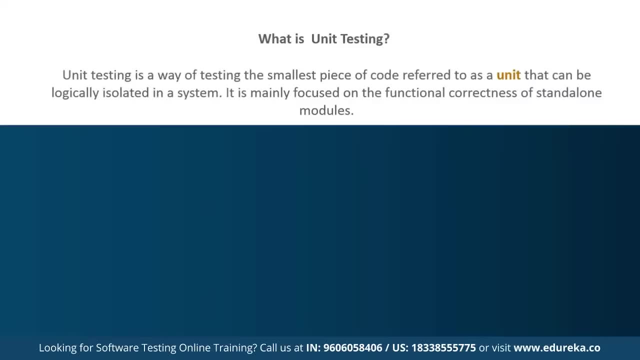 and second, fast that fast. Well, here's a simple example to help you understand what a unit can be or how unit testing is. So consider the simple code. Well, I have a simple function or method here, the function as you can see, the main function. 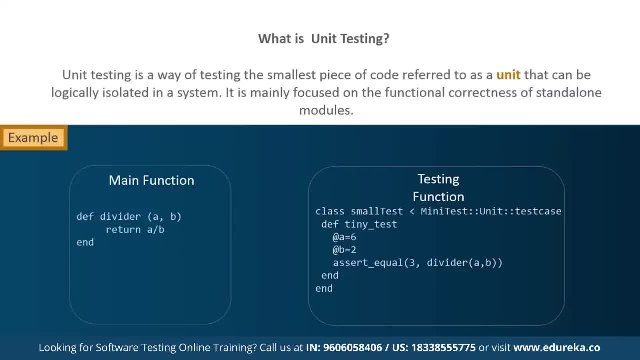 It's performing division operation. It's accepting two parameters, a and B, and it's returning the value that you get after dividing a by 2.. A by B, and next comes the testing function. as you can see, the testing function is written in Ruby. 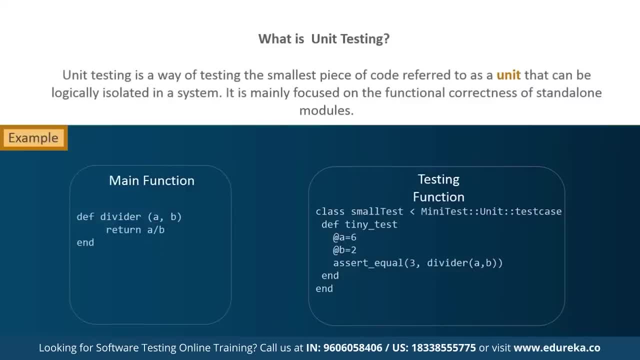 Well, the language doesn't matter. the language whichever you're comfortable with, you can use that. Anyway, as you can see, I have two variables, a and B, and I'm assigning values 6 and 2 and in the assert equal function. 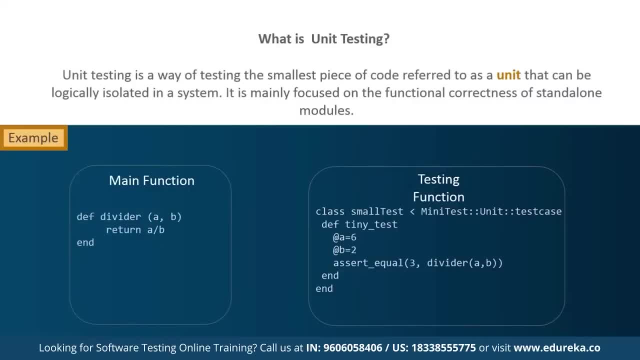 I'm calling the divider function and I also have the first parameter, which is the value which I'm expecting that the division function should give it to me. So the value which I'm expecting is 3 and I'm passing the function and parameters to that function. 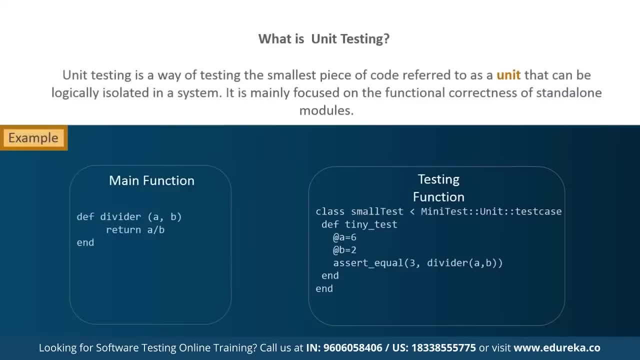 So after dividing a by B, which is 6 by 2, I get the answer 3 and assert equal functions tells me that 3 and 3, the expected answer and the actual answer I got, are the same. So my function is working properly. 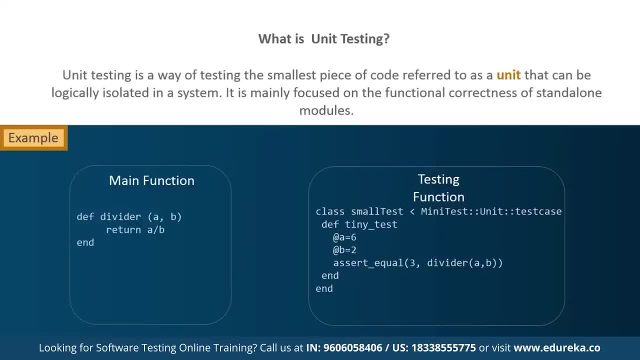 Well, this is a positive case. You can also do that with the negative case, as in. you can just change the 3 expected value to 4 and see if the assert equal function returns to the actual answer. It says that your test phase. it means that the expected answer. 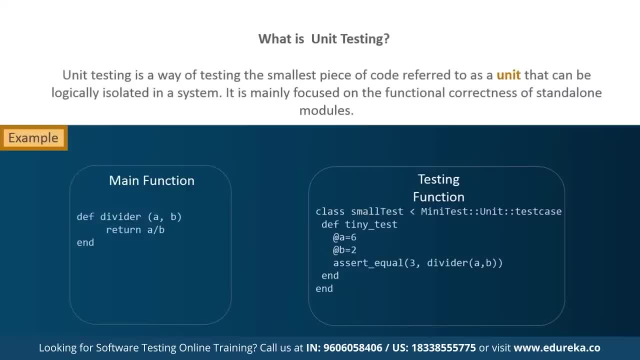 and the obtain answer not the same. So that's how you perform a testing on small unit which is a part of your entire program. So here the small unit is division function. So, like I said, a unit can be almost anything you want to be. 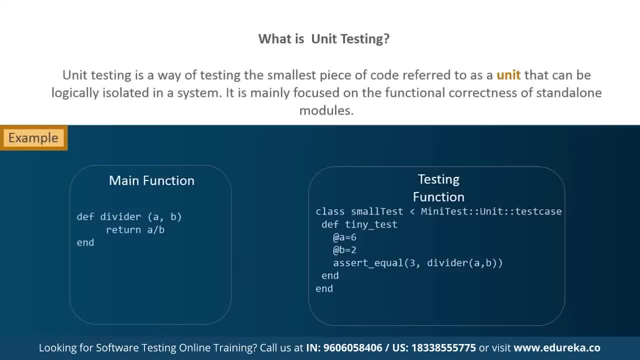 it can be a line of code, or it can be a method, or it can be a class. So this is very basic example, but I'm sure it gives you an idea of unit testing, right? So, guys, unit testing is usually performed at the earliest stages of development process. 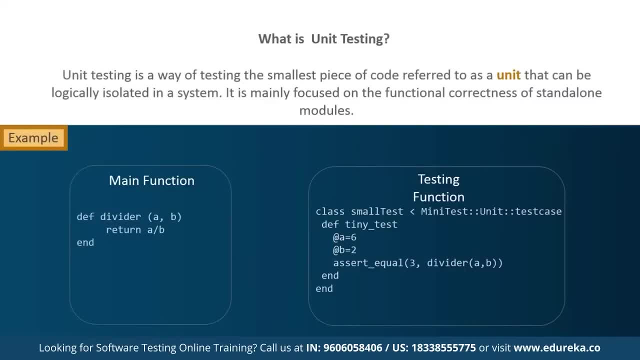 Like I said earlier, and many cases, it is executed by the developers themselves before handing the software over to testing team. One of the biggest benefits of this testing is that it can run every time a piece of code is changed, So that way you can resolve. 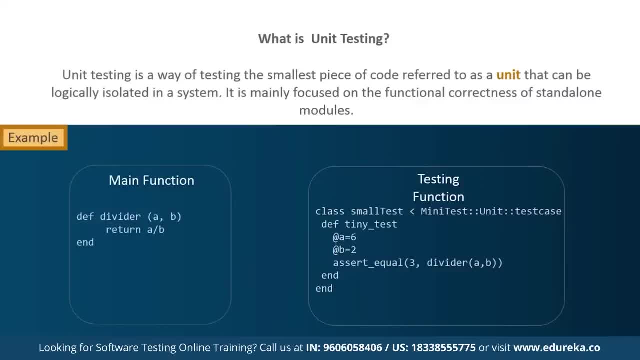 if there are any errors very quickly, and since you're dividing your code into modules here, you can reuse your code and testing becomes much easier and efficient and your product is well worst in the market. Now to understand unit testing better, Let's go ahead and see a simple algorithm. 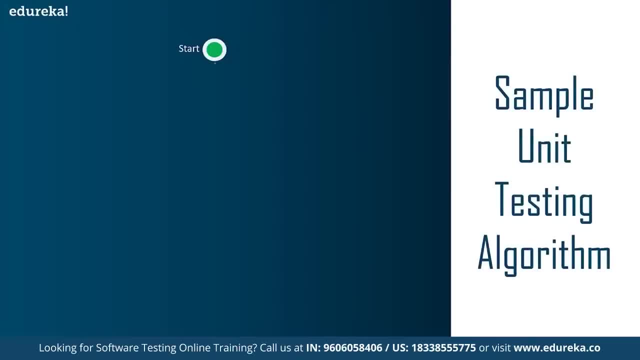 So you start writing your test, So you add your test to the test suit, then you run the unit test. if the test passes, then you add one more test or add it to the next level of testing. in case your test fails. What you do, you make the necessary changes. 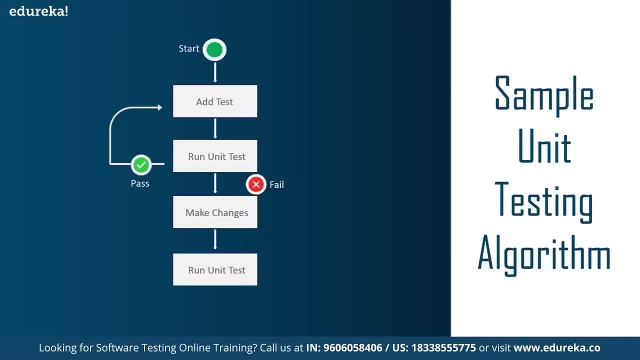 and you run unit test again and after you run your test again, if it fails, then you make changes again and you repeat the cycle until the code which you have written is perfectly working and it's returning the value that you're expecting or the results. that meets your requirement. 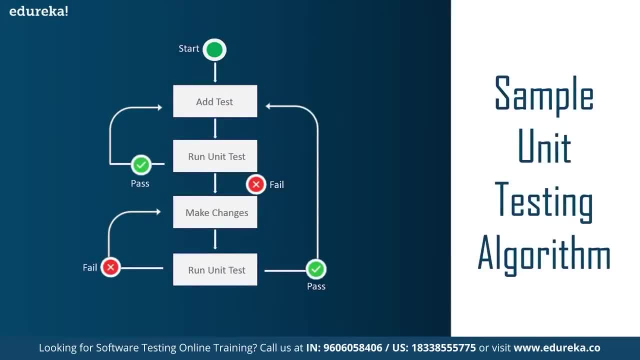 and suppose, after making changes, if your test passes, then you can add it to the test. Let's switch and move it on to the next level of testing. So once you are sure that all your tests are working properly, it means their test suit is perfect. 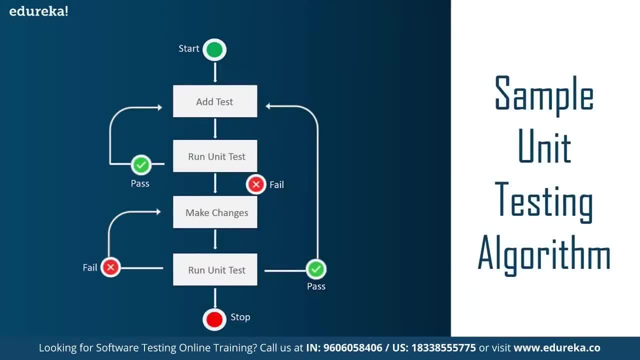 and your product is working properly, You can stop unit testing and perform next level of testing. very simple, right. This type of basic testing offers a lot of advantages, guys. unit testing provides numerous benefits, including finding software bugs, facilitating change, simplifying integration, providing a source of documentation. 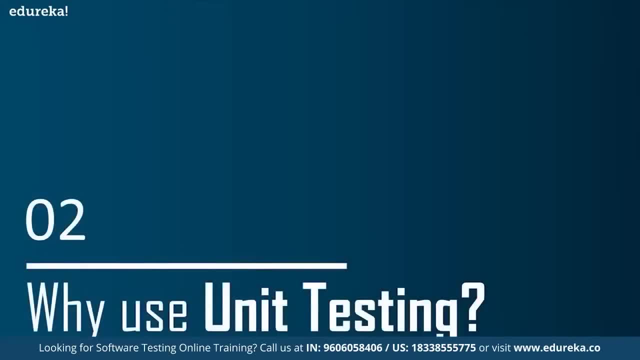 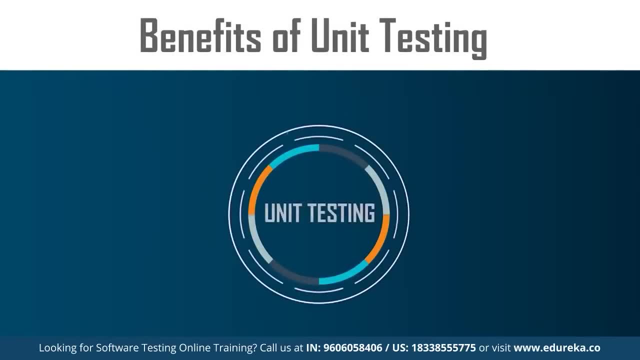 and many others, So let's take a look at them right now in more detail. So here are the benefits of using unit testing in software development cycle. So, first of all, it makes coding process more Agile when you add more and more features to software. 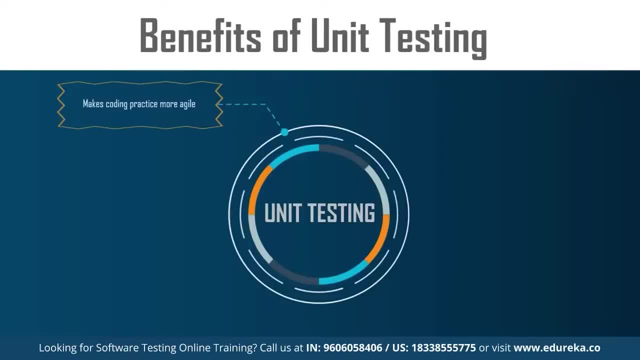 You sometimes need to change old design and code. I'm sure you agree with that. However, changing already tested code is both risky and extremely costly. if we have unit test in place, then we can proceed for refracting very confidently because we know that each part of a code is working properly. 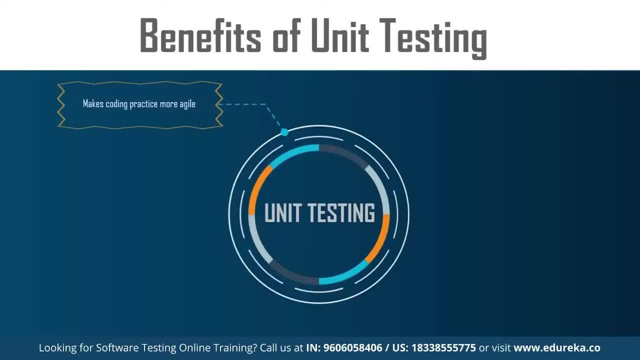 So code complete nets is very important in software testing, especially a gel process. So running unit test can demonstrate code complete nets. So unit testing makes code practice more Agile and very simple. Secondly, unit testing improves the quality of your code. It identifies every defect that may have come up. 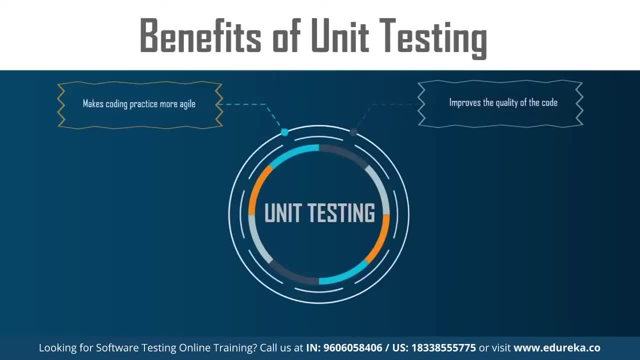 before the code is sent further for further testing. So writing test before actually coding makes you think harder about the problem. It exposes the edge case And makes you write better code. Also, the code that you've written is since divided into modules. that becomes reusable. 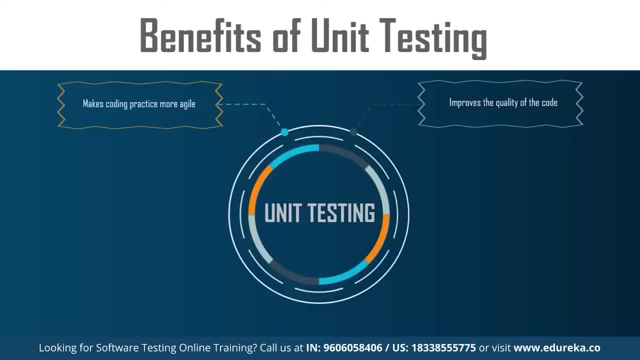 This means that codes are easier to reuse when you perform unit testing. unit testing also helps find software bugs early. since unit testing is usually carried out by developers who test individual code before integration, issues can be found very early and can be resolved easily without impacting other pieces. 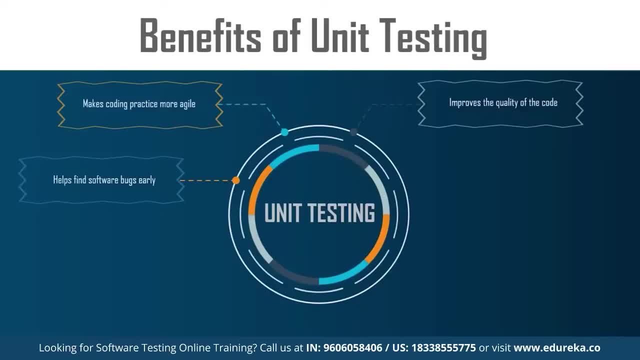 of code. so that advantage of detecting any errors in software early in the day is that by doing so, the team minimizes software risk and avoid spending too much money in time. unit testing also facilitates changes and it simplifies integration. it allows programmers to refactor code and upgrade system libraries at later date. 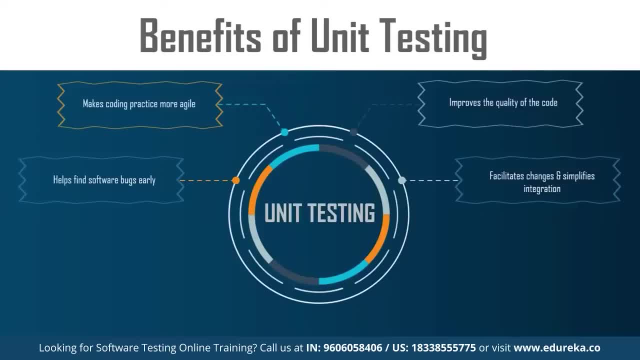 and make sure that the module still is working properly. unit testing helps with maintaining and changing the code. it reduces the defects in your newly development or the newly developed module of your code. It reduces parks when changing the existing code Functionality as well. unit testing actually verifies: 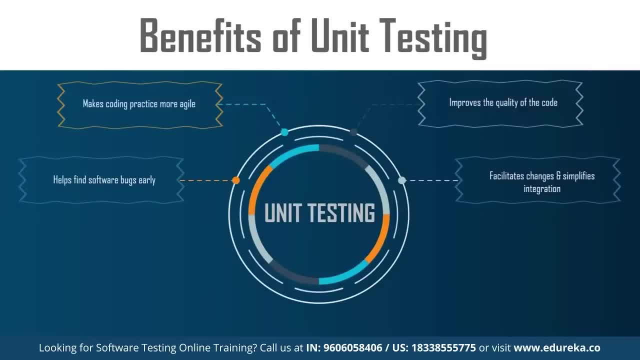 the accuracy of each unit after what the units are integrated into an application by testing parts of the application via unit testing. So basically it makes integration much more better. It provides documentation to developers, So code documentation is basically drag and it shows mostly how little code documentation gets written. 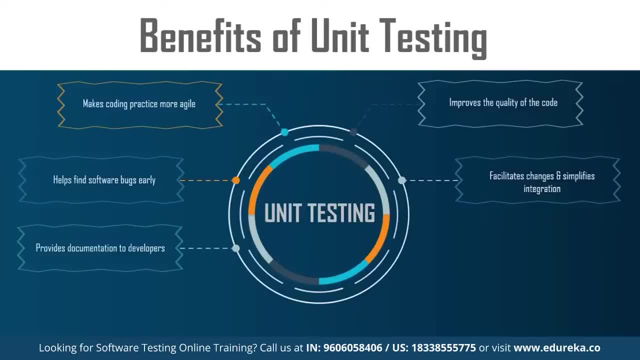 unit testing can make the documentation burden a little easier by encouraging better coding practices and also leaving behind the piece of code that describe what your program is actually going to achieve. unit testing also makes debugging easier and quicker. it helps simplify the debugging process. If a test fails, then only the latest changes made. 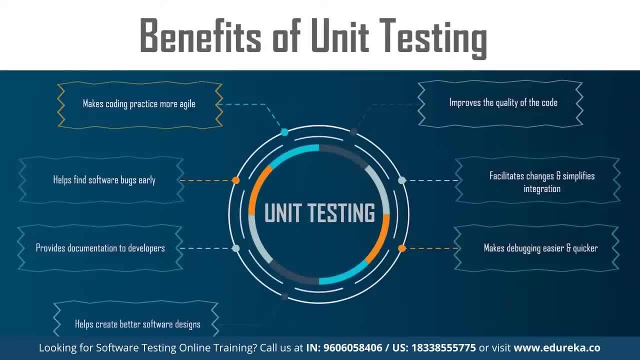 in the code need to be debugged. It's easy, right? It helps create better software designs. writing the test first forces you to think through your design and what it must accomplish before you actually write the code. This not only keeps you focused. 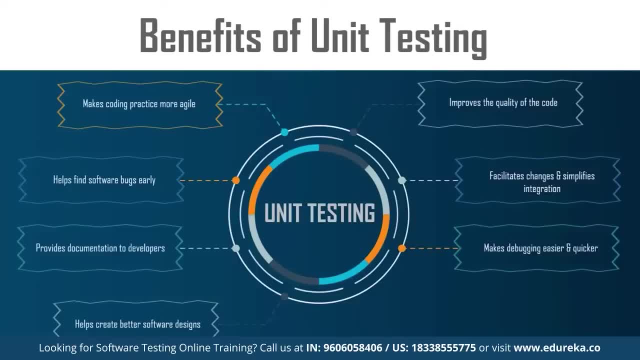 It also makes you create better designs, So that way you're sure that the code you write will perform The right thing at the right time. And lastly, it reduces testing costs, since the bucks are found early. unit testing helps reduce the cost of buck fixes. 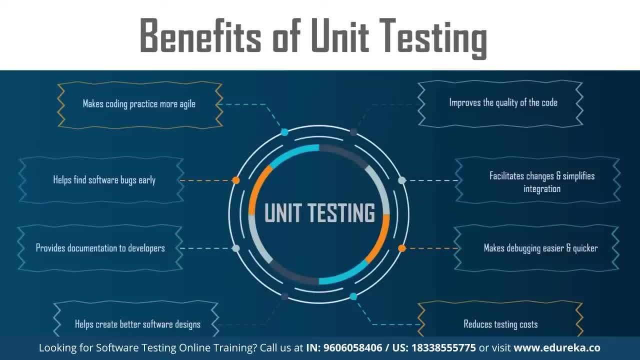 So just imagine the cost of buck found during the latest stages of development. You will have to modify the entire code of your project. that sounds really tiring and waste of money. So performing unit test saves you a lot of money and effort on your part. 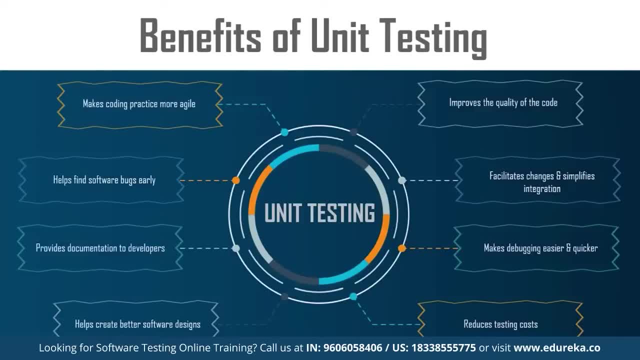 So, guys, these are a few benefits of regression testing. I'm sure there are others as well. Make sure you research on it and learn more about them. So there we go, guys. I hope you're convinced as to why you should use unit testing. 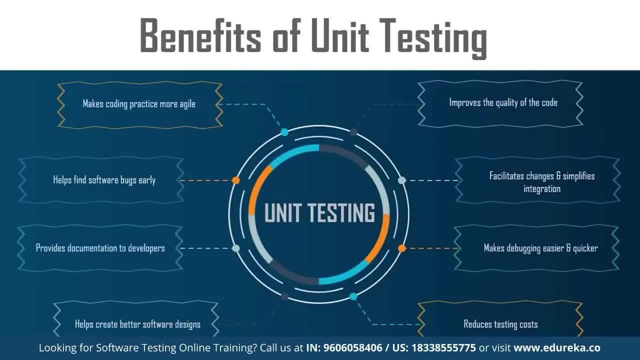 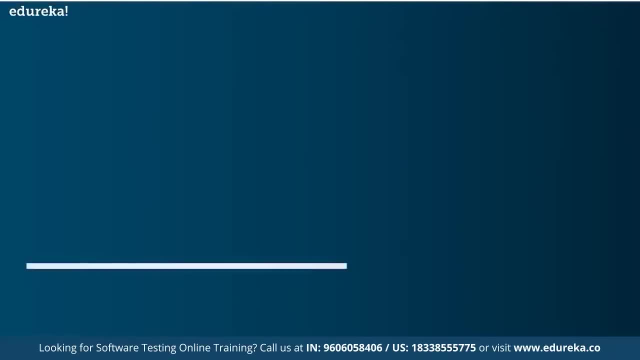 So we have covered the basics of unit testing. If you have any queries regarding what we have discussed and now, please to post them in the comment session and we'll get back to you as soon as possible. So, moving on, let's do a simple demo on how to write unit test. 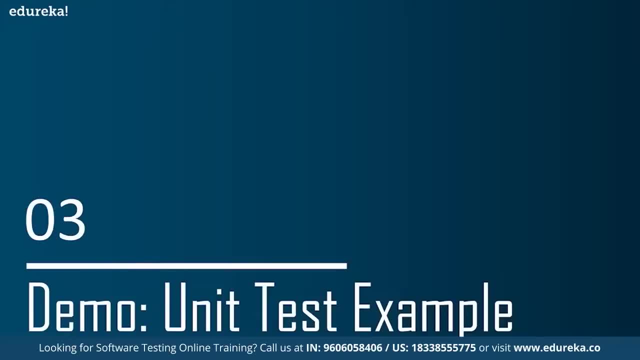 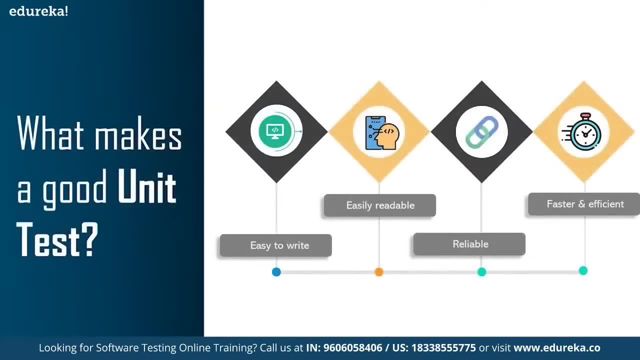 But before diving into the main part of this tutorial and writing unit test, let's quickly discuss the properties of a good unit test. unit testing principles demand a good test is easy to write, It's easily reliable, It's readable, and faster and efficient. 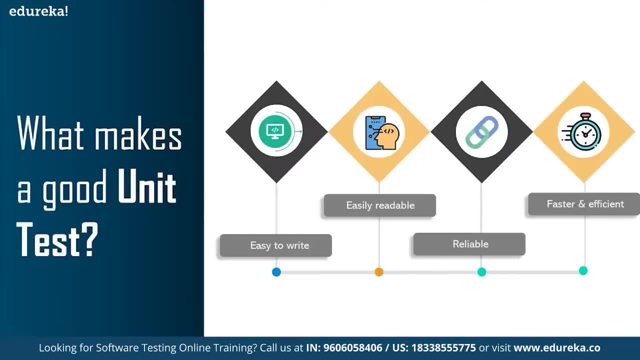 So easy to write. developers typically write lot of unit test to cover different cases and aspects of application behavior, So it should be easy to code all those test routines without much effort. It should be readable. the intent of unit test should be clear. a good unit test tells a story. 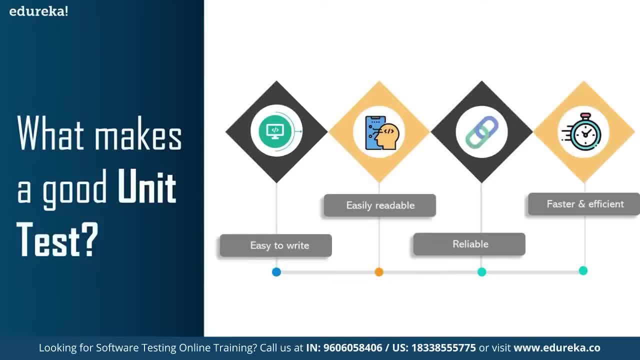 about some behavioral aspect of your application. So it should be easy to understand which scenario is being tested and if the test fails, it should be easy to detect the bug without actually going through the entire program. That's how easily readable your unit test should be. 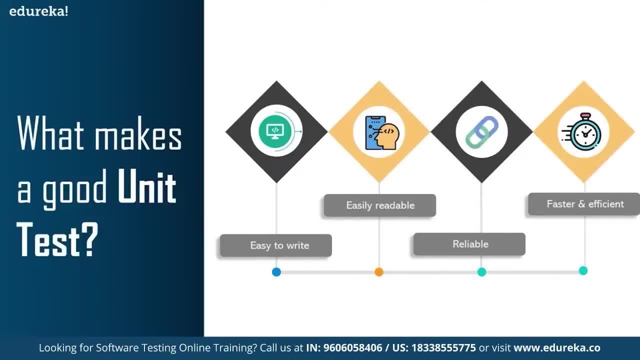 So with a good unit test we can fix a bug without actually debugging the code, then it should be reliable. unit test should fail only if there's a bug in the system under the test. Well, the thing is, programmers often run into an issue when the test fail, even when no books are introduced. 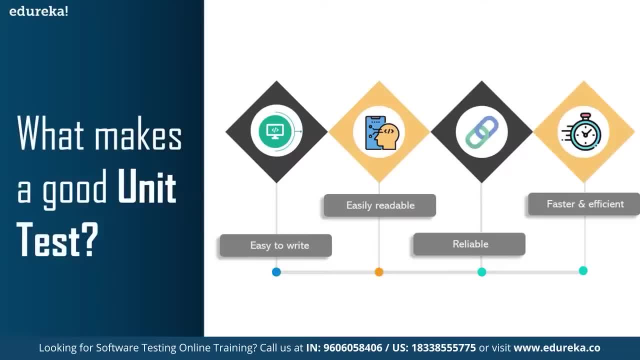 So good. unit test should be reproducible and independent from external factors. Lastly, you write your unit test so that you can repeatedly run them and check that no books have been introduced. If your unit test is slow, it will affect the final product. one slow test. 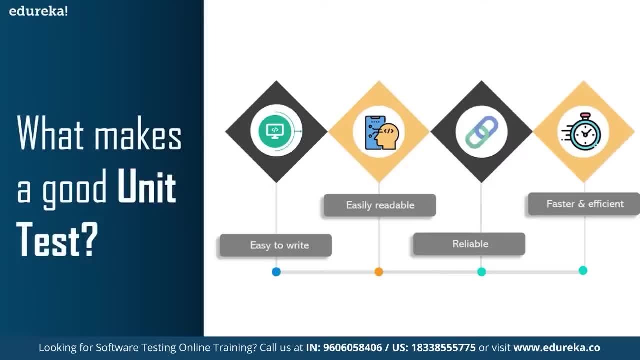 won't make a significant difference, but add 1000 more and we're surely stuck waiting for a while. slow unit test may also indicate that either the system under the test or the test itself interacts with external system, making it environment dependent, which is not a good thing. and unit testing 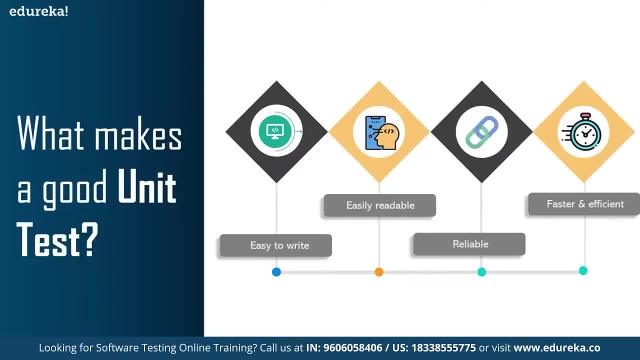 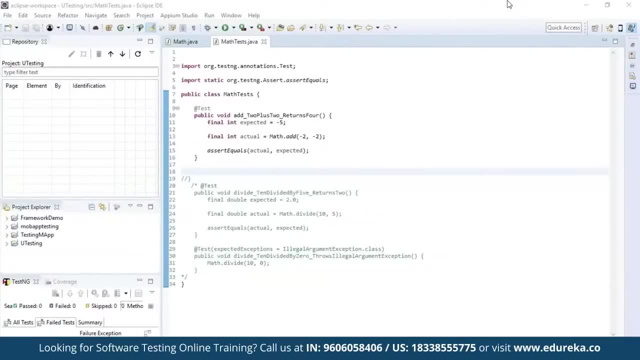 So that's it, guys. There are no secrets to writing unit tests, So let's go ahead and write one. So, guys, before we actually start with the simple demo, that certain things which you should know. first of all, to perform this demo, you need ID. 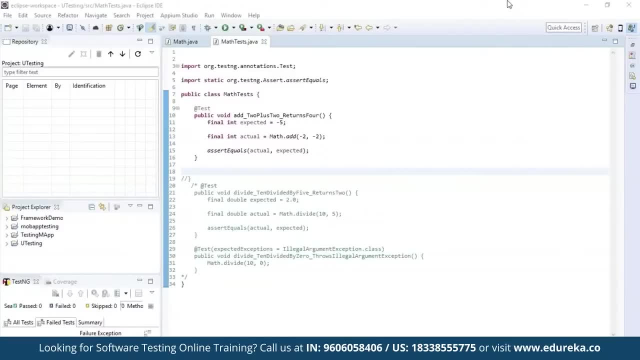 It could be your Eclipse or IntelliJ, anything that you're comfortable with, and you need a unit testing platform, or you can say framework in here. in this demo I'm using a framework, a popular framework for Java, called test NG. There's another one called J unit. 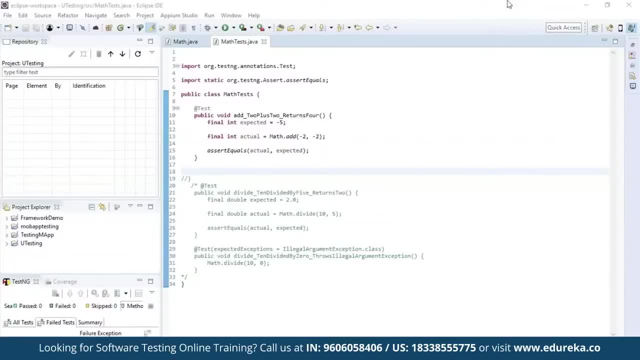 You also have different frameworks for different languages that you can use. will discuss about the unit testing frameworks later, But as for in this demo, as you should know, I'm using Eclipse ID and I'm using test NG for my unit testing framework. So that's all you should know. 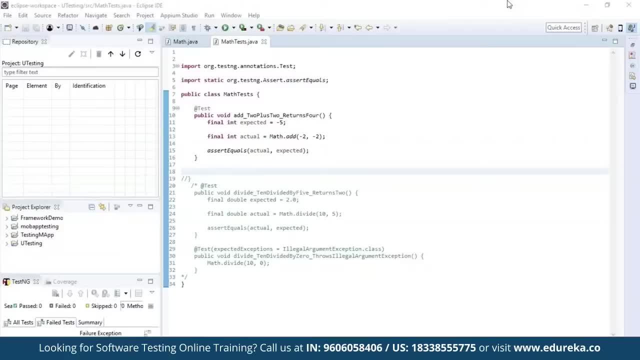 and regarding how you should install test NG. There are different ways. you can install it using Maven. The easiest way in Eclipse is you can actually install it using Eclipse Marketplace. Well, you have help command here. You can see the menu. you can go for Eclipse Marketplace here. 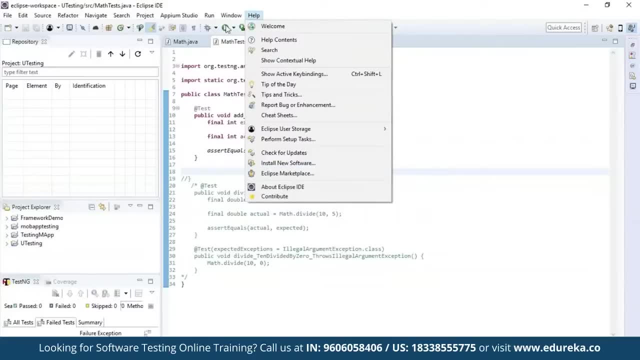 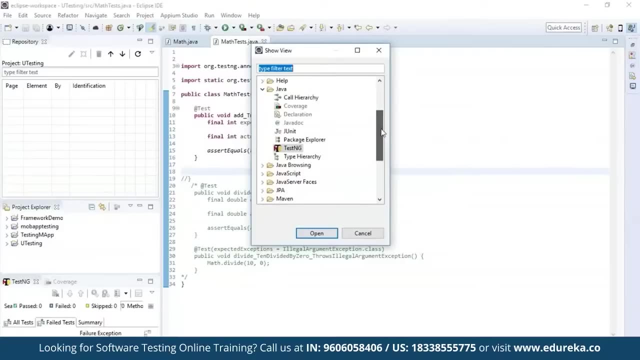 and click for test NG and just click on install. after you've done that, to make sure it's installed properly, All you have to do is go for show you here and click on other and, under Java, make sure that you have test NG installed here. 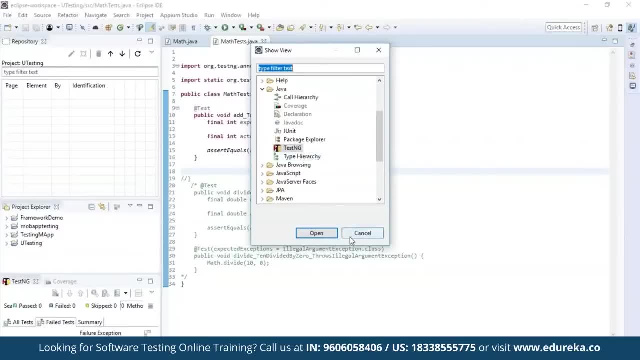 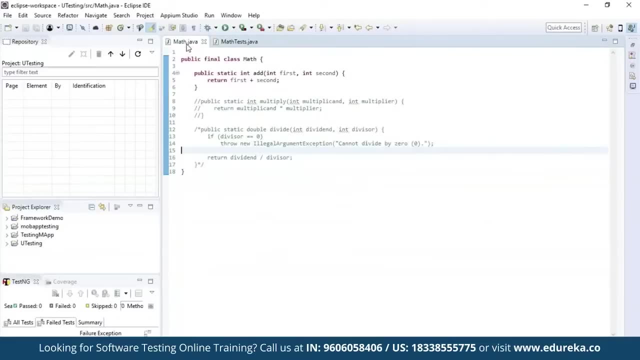 If it's showing test NG here, it means that installation has been done properly. So that's all, guys. I've already written program. Well, it's a very easy program. as you can see, I have a math function. first of all. 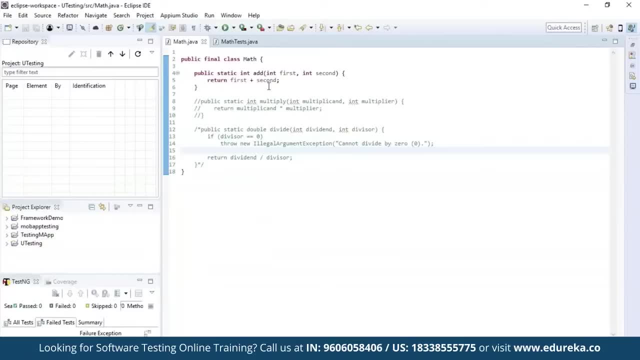 and it has one method which adds two numbers. So it's returning into value and I have first parameter in the second parameter and I'm adding and I'm returning the value to my testing function. So this is my basic function and I have a test function. 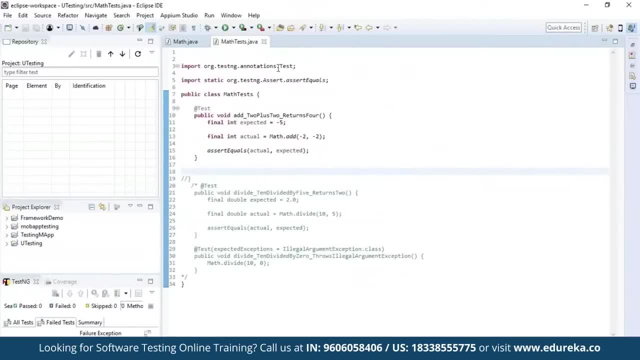 which is conducting the test here. So, as you can see, I'm using annotations here and importing this because to perform test, since I'm using test NG, I need to import these details, So I'm using annotations. which is at test. This is called what we call annotations. 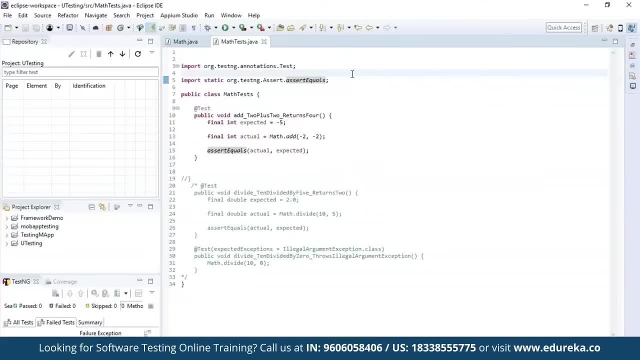 and I'm using a method called assert equals, So I'm importing that as well. So again, this class contains a single method which is adding two numbers. I have two variables here. one is expected, and actually expected is the one which you want the method to return to. 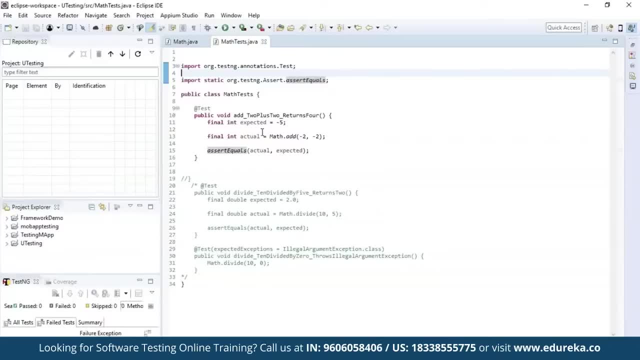 and the actual is the one which actually the method returns to you. So, as you can see, the expected value I'm giving it as, let's say, four, and as for the actual value, I'm using a math add function which have created here, as you can see. 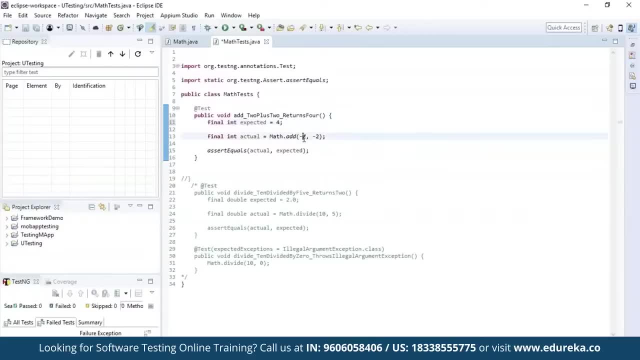 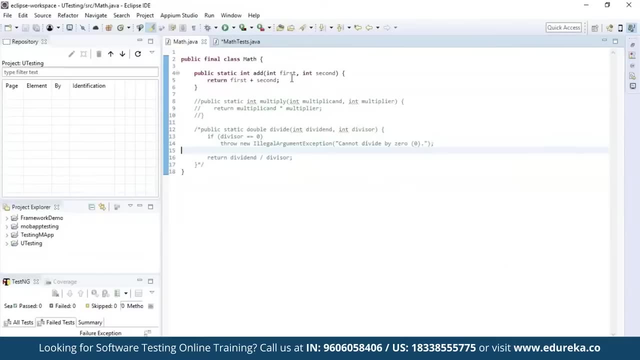 I have add function here and I'm sending two parameters, which is 2 and 2.. So if I go back to function, since I'm calling this function, the parameters here will be: first is also 2, second is also 2, so if 2 plus 2, it should written for. 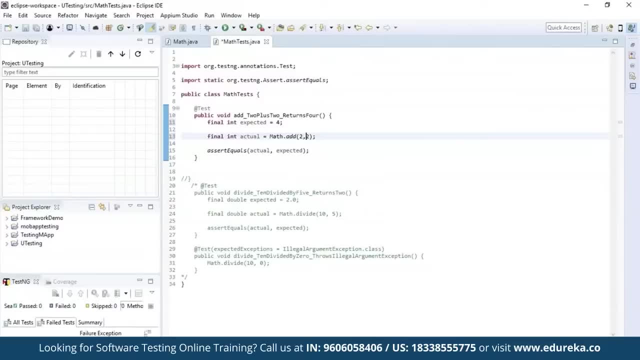 and here I have a method: assert equals. this is the actual value which I'm getting from the math function and is the expected value which I've given it for, and since both are for, the test should result success. Let's go ahead and check it. 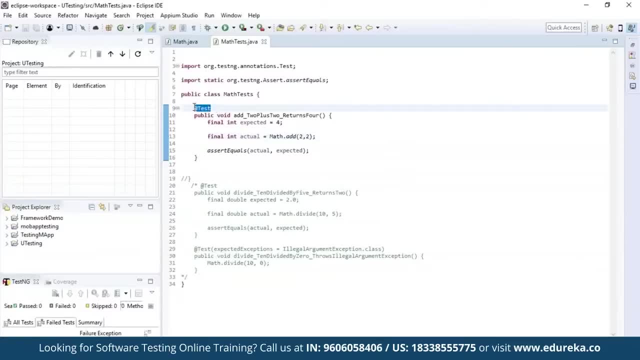 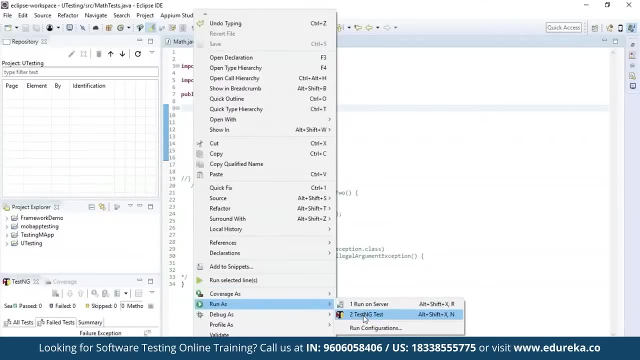 It's as easy as that, guys. So this is one unit of your entire program. You can keep adding units in this way. So first we're checking if this unit is working properly. for that, Let me run the test. As you can see, it says this test has passed. 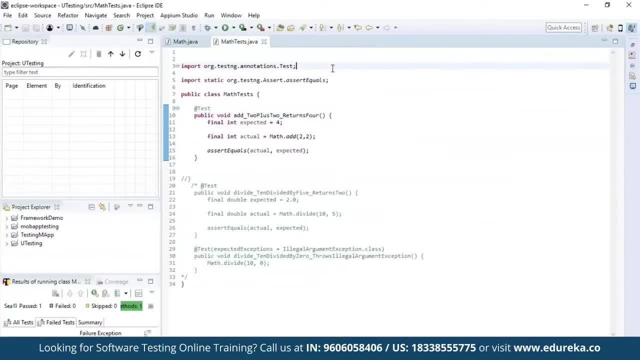 and the test run. one failure: 0, skip 0. it works right, Let's go ahead and check another further. What are the values? Let's say: let me give it as minus 4 and minus 2, plus 2, that should be. let me just give it as minus 3.. 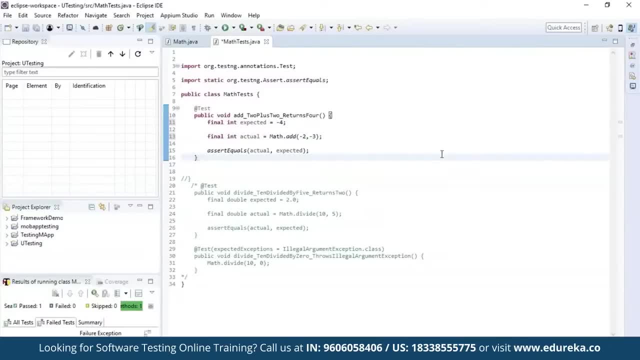 So minus 2 plus minus 3 should be minus 5.. Now, if I call asset equals function, the expected value is minus 4 and the actual value is minus 5.. So the test should written failure. Let's go ahead and check it. 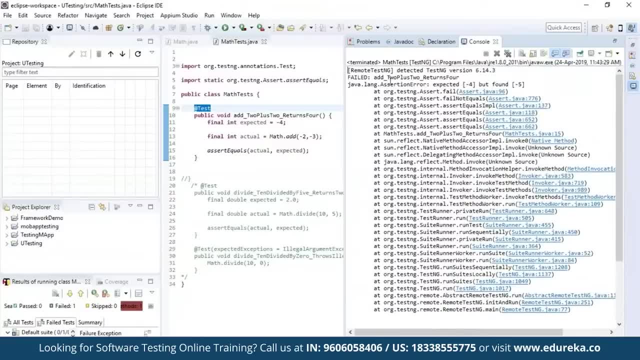 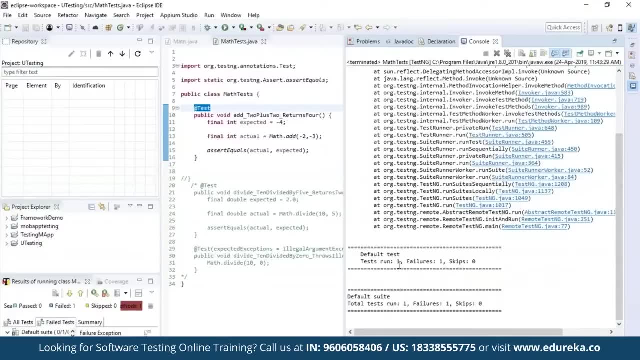 So here, as you can see, it's giving a long message. It says: this test is failed because expected value is minus 4, but the actual value is found to be minus 5 and, as you can see in the default test, one test was run. 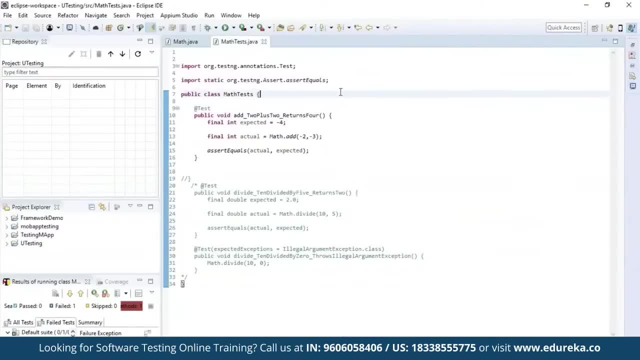 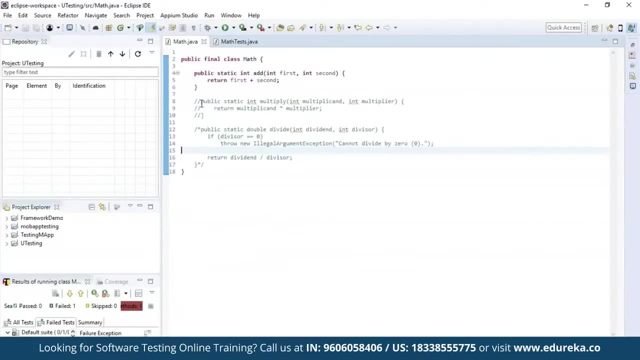 You have one failure and zero skips. That's it, guys. And now let's make it a little more bigger, as in: let's add one more function in the math function. I have a multiply function here, So let me go ahead and add it. 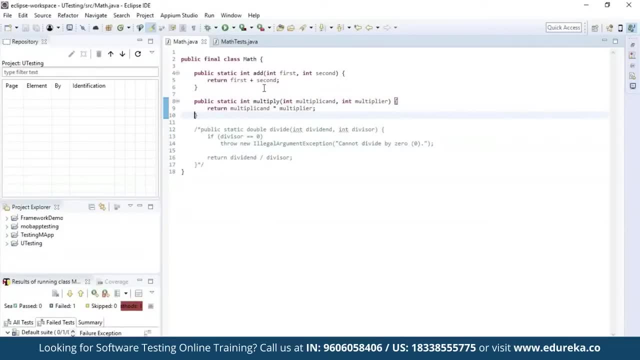 So I'm not negating or I'm not commenting that function. Let it be there. It's going to give us result for both the functions here. So this multiplier function: again it's taking two parameters, one is multiplicand, one is multiplier. 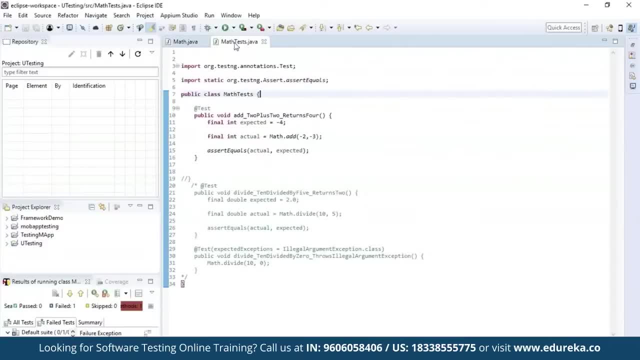 It's multiplying them and returning the answer to us. Let's go to math Java test here. I don't have a test annotation for that right, So let's go ahead and write one. So public void: Multiply two numbers. Return some any name of your function. 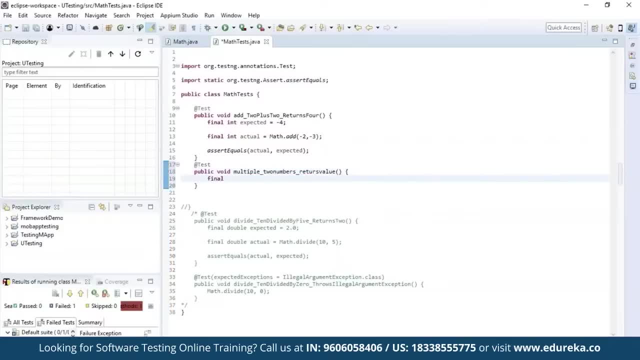 could be according to your wish. and here I go. So, finalint expected, Let's give it for. let's keep it simple for a while and then we'll make it complicated, final and actual. So, multiplicand, let's give it as two and the multiplier also, let's give it as two. 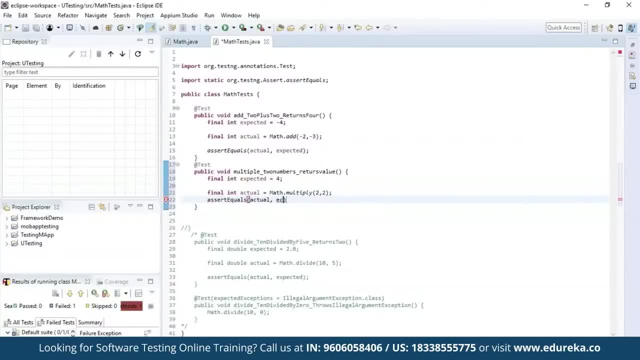 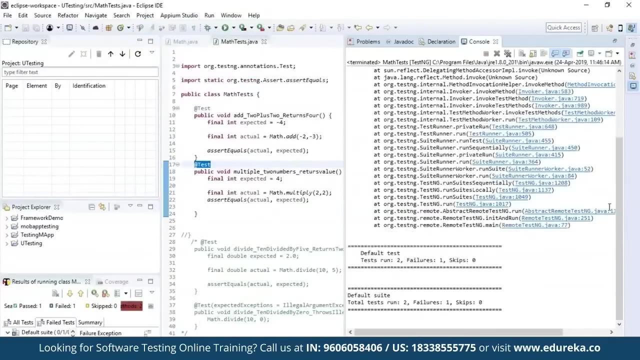 Assert equals actual and expected. Okay, let me save it. So obviously the add function, it should result of failure and multiply it should later the correct value. So let's go ahead and test it. So, as you can see, to test a performed one failure. 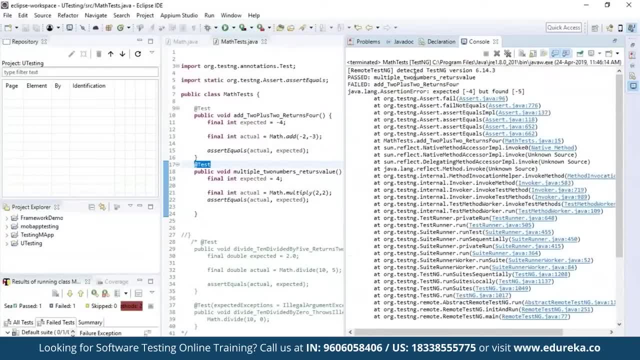 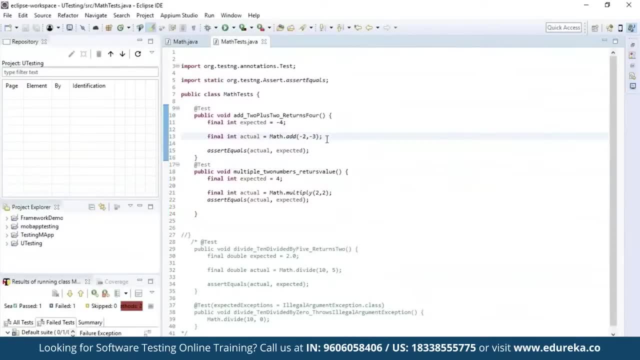 So let's go ahead and see. it is multiply. two numbers has successfully passed, but add has failed because expected values minus 4, but it was found to be minus 5.. So that's how you write unit test. Let's make it minus 4. 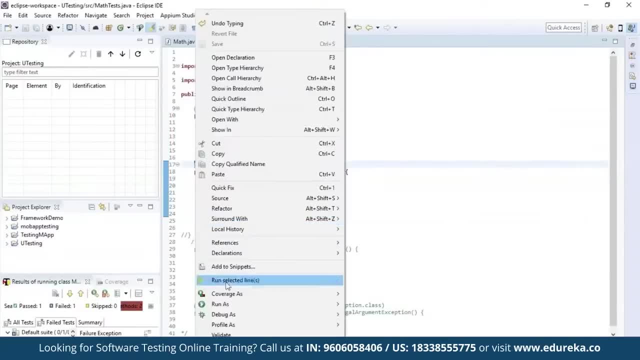 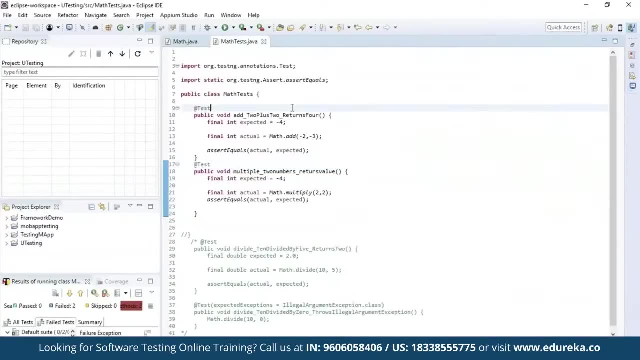 and check if it's working for the negative numbers as well, As you can see it showing two failures here, both of multiply function and add functions have failed. So, guys, it's as easy as that. first, I wrote a unit test for add function. 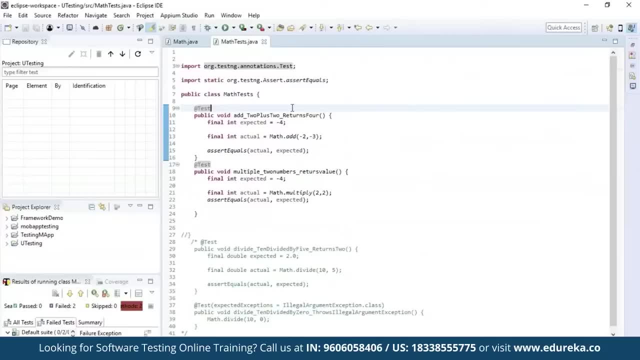 So that's add function is a unit. You can call it a unit, a part of your program, and I've checked them, tested. since the method is working properly, I'm going one step ahead and added one more unit, which is a multiply function. Even it's working properly. then you go ahead. 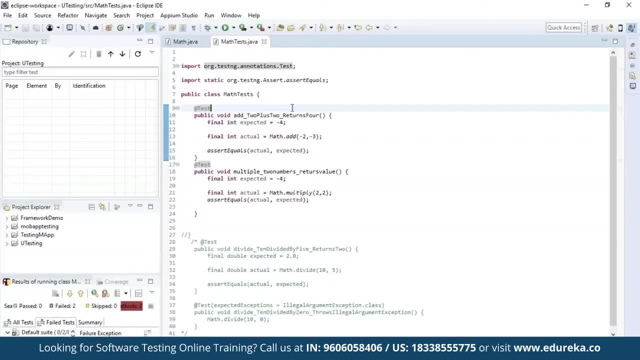 and add one more part of our more unit to your function or the program of your application. So, guys, that's how you write simple unit test. as you can see, the tests were very simple and these are very basic Level test. you can go ahead. 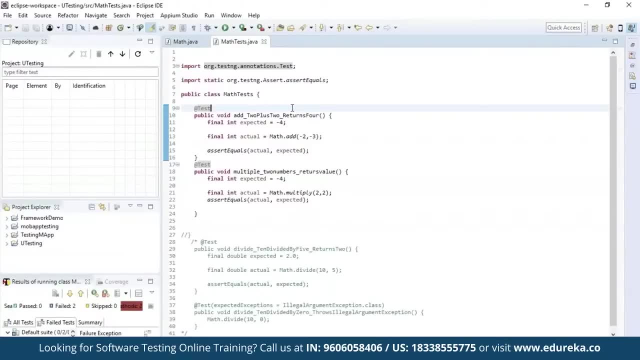 and make, explore and make them complicated. So I'm not going to do the divide function. the purpose of this demo was for you to understand how simple it can be and how your unit test should be not very complicated. There should be very easy to understand. one look at it. 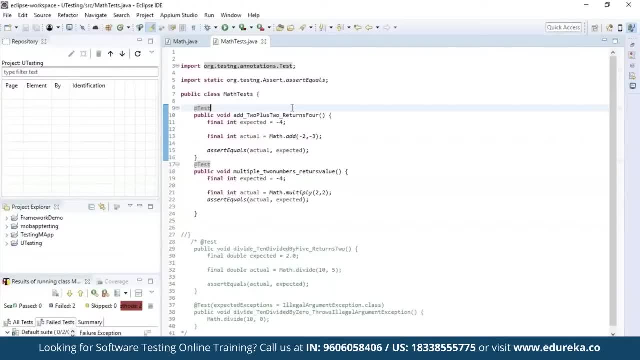 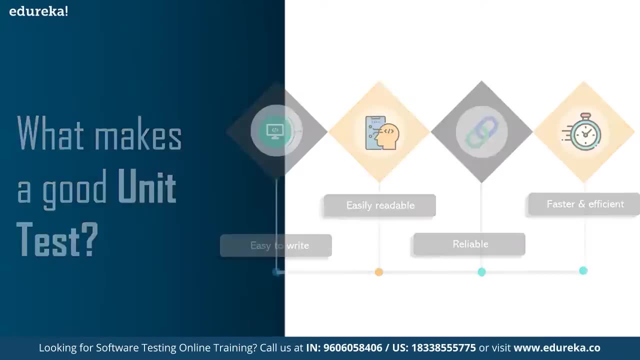 The person who is looking at your coach understand what your code is actually performing. So there you go, guys. That's how you write your unit test. Let's get back to the theory part. So I hope you understood what we did in the demo. 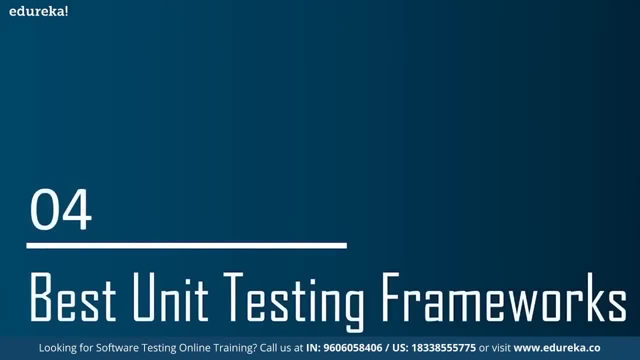 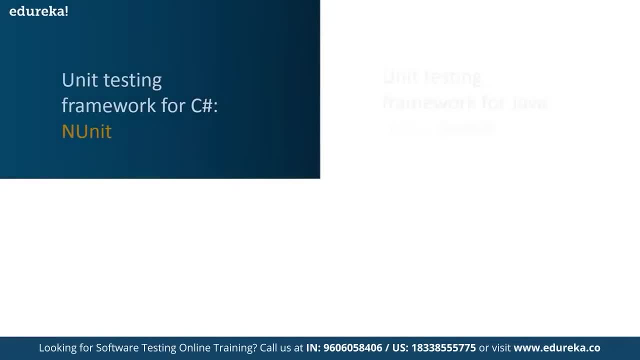 Let's move forward and check out the most popular or the best unit testing frameworks to automate unit tests. So the unit testing framework for C sharp is an unit and unit is a unit testing framework that belongs to X unit family and it's written entirely in C sharp. 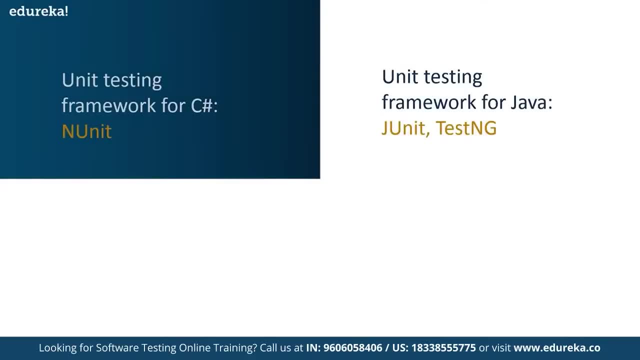 Now, as for Java, you have many. the most popular ones are J unit and test and G. J unit is basically an open-source unit testing framework for a test driven development environment. We call it TDD. It's opposed the core concept of first testing, then coding. 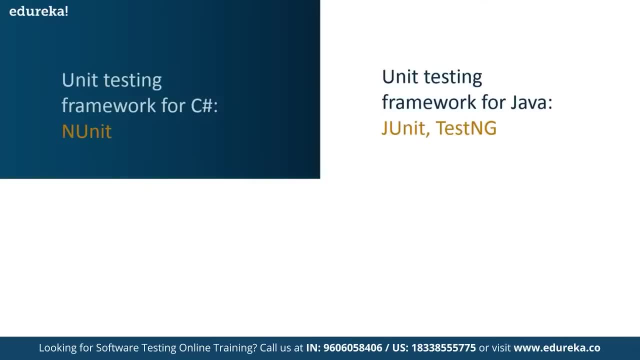 this framework is specifically designed for Java programming language. Then this data is first tested and then it is inserted in the piece of code, So it provides the simplest approach for writing code very swiftly and easily. It also offers annotation for test method identification, as we did in the demo part. 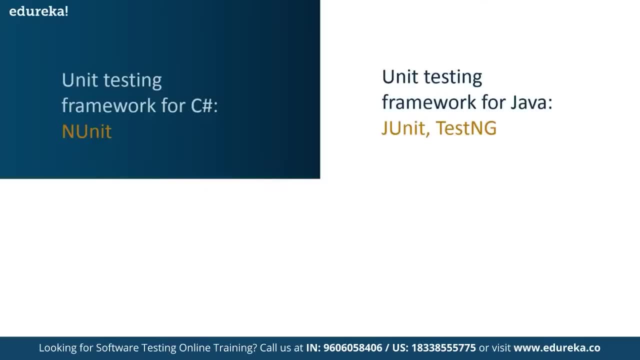 We use test injury and I've showed you how to use annotations and an asset equal function. moving on, a unit testing framework for C and C plus plus is M unit. It's an open-source unit testing framework which is designed for software application which is written in C. 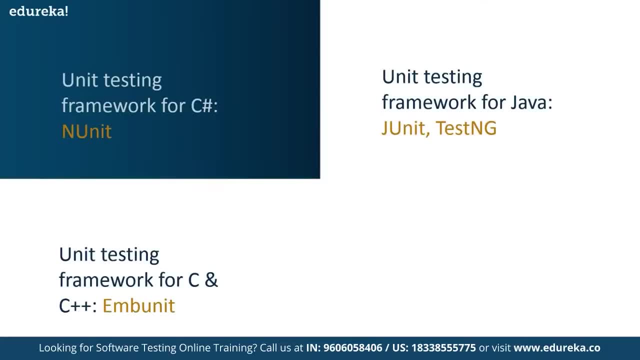 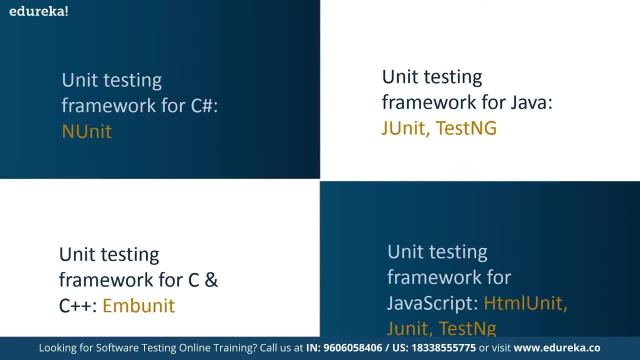 or C plus plus. well, it's used by both developers and testers for software applications which are written again in C and C plus plus. So next we have unit testing frameworks for JavaScript. As you guys know, JavaScript is the language of web, which is the reason there are large number. 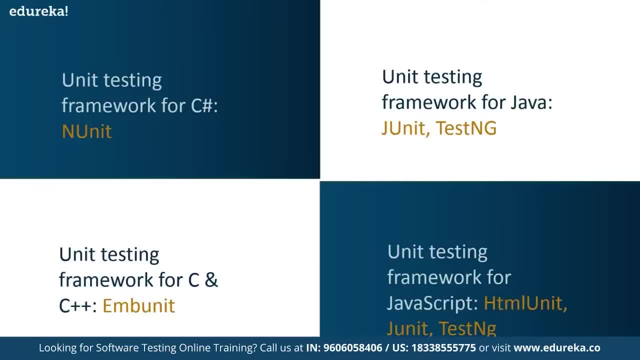 of test automation frameworks that support Java JavaScript. So here's one of the most popular unit testing framework for JavaScript. It's called HTML units. It is an open-source unit testing framework that supports JavaScript and it provides graphical user interface features like forms, links, tables. 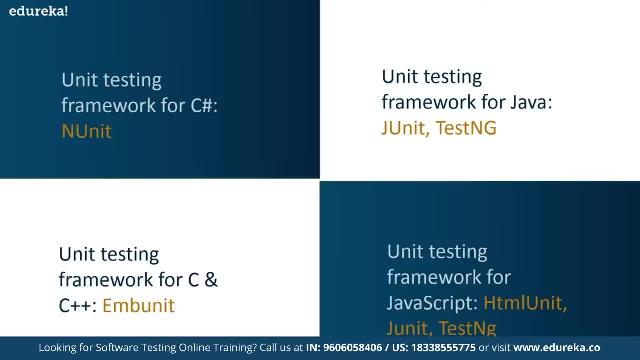 etc. It offers an open-source Java library which contains graphical user interface- less browser for Java programs. It also supports cookies, submit methods like get post and proxy server. It is used for testing applications that are used within frameworks like J unit and test injury. 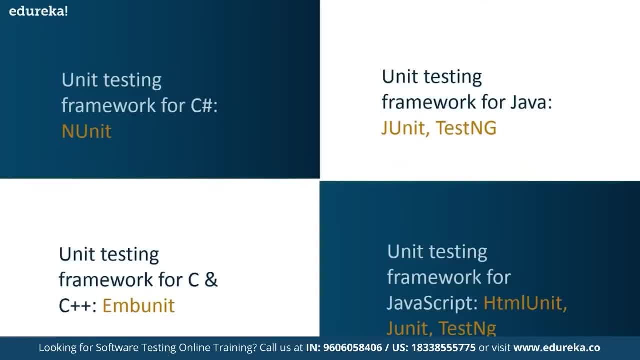 So right, these are not the only ones which are there in the market that have any other popular frameworks, but these are the top unit testing frameworks which support different languages. as we discussed for C sharp, It's an unit. for Java, You have J unit. 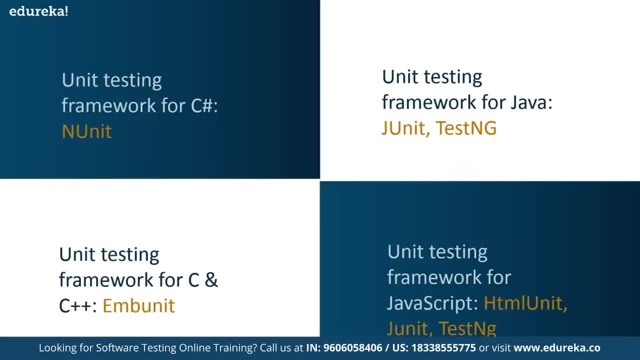 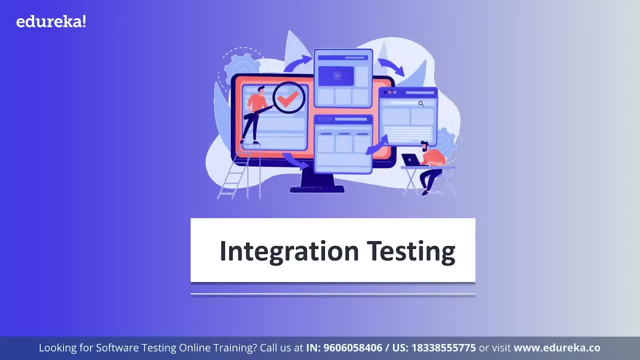 and test injury for CNC. plus plus you have MB unit for JavaScript. You have HTML unit J in a test engine, many others. Integration testing is done to test the modules of components when integrated, to verify that the work as you expected. that is, to test the modules. 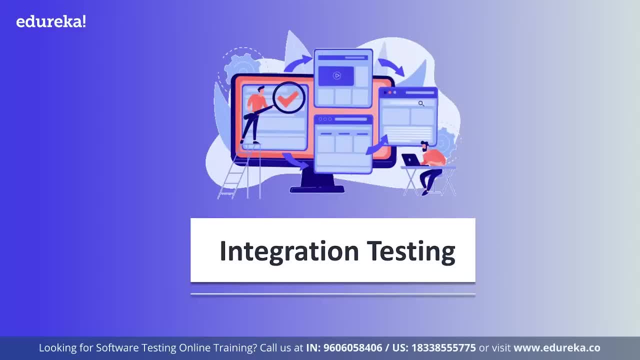 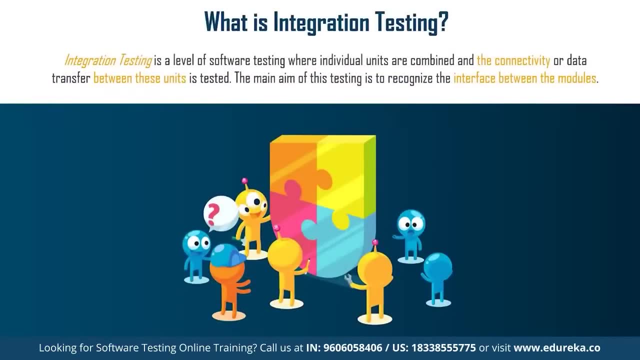 which are working fine individually, does not have any shoes when integrated. So the meaning of integration testing is quite straightforward: integrate or combine the unit tested module one by one and then test the behavior as a combined unit. That's what integration test means. So we normally do integration testing after unit testing. 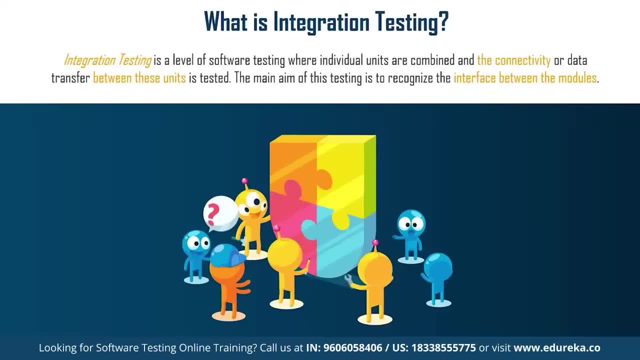 as you guys already know it, once all the individual units are created and tested, we start combining those unit tested modules and start doing the integration testing. So, once again, the main function of goal of integration testing is to test the interfaces between these modules, not the modules. 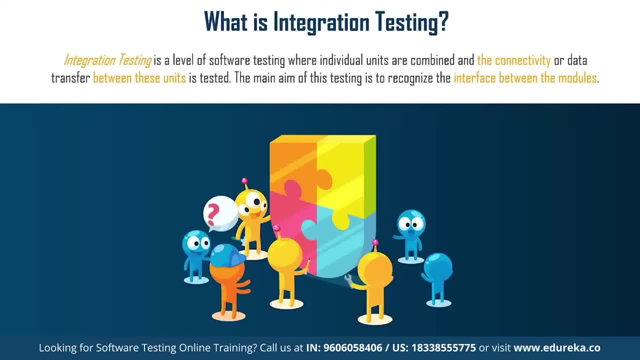 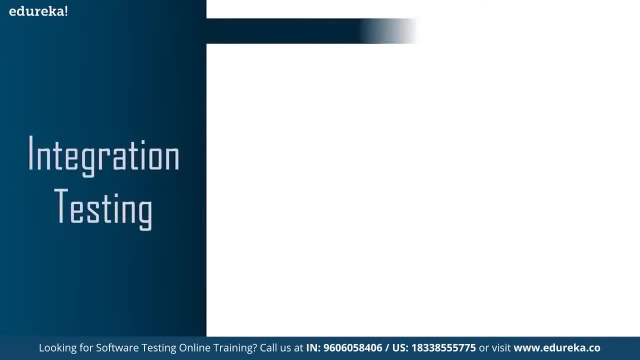 but the connection or the communication or the interface between these modules. That's the aim of integration testing. Let's learn more about integration testing. integration testing basically make sure that integrated modules and competence work properly. integration testing can be started once the modules to be tested are ready. 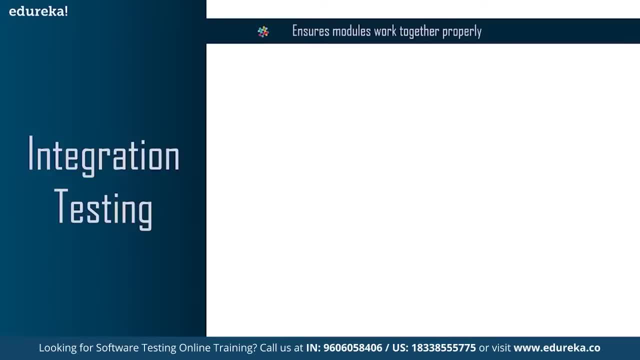 Well, it does not require the other modules to be completed for testing to be done. And how is it possible? will check that out later. and integration testing also helps detect the errors which are related to interface between the modules. like I said earlier, it is also helpful. 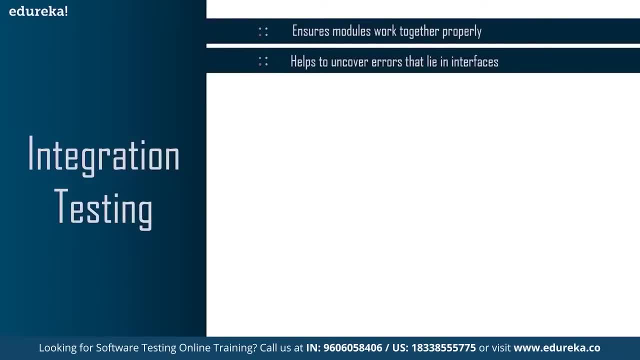 when there are frequent requirement changes. It's very common for a developer to deploy changes without unit testing sometimes, so integration testing can help. when the modules need to interact with api's or some sort of third-party tools. You can test the modules to find out if the third-party tool 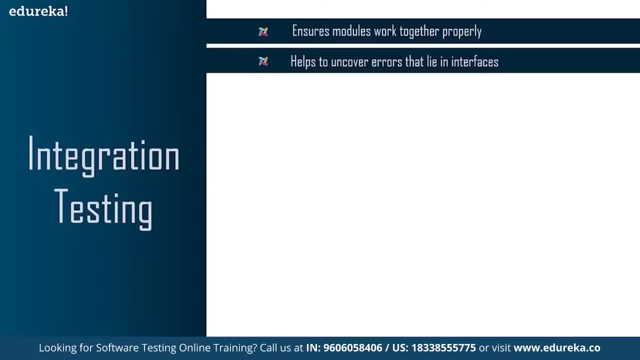 accepts the modules, data or not. integration testing typically covers large volume of your system than a single test, So it's more efficient and, lastly, writing both unit and integration test increases the test coverage at faster speed and it improves the reliability of your software. Well, these are the advantages of using integration testing here. 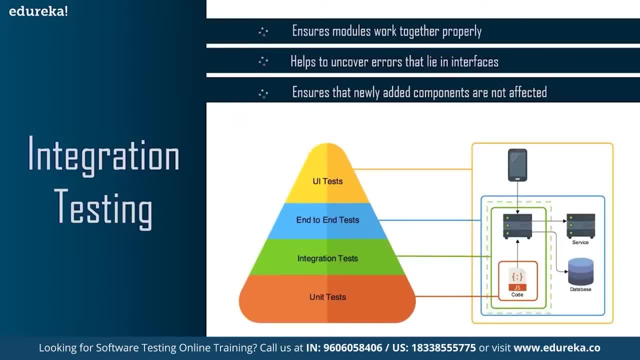 I have a simple diagram for you to understand what integration testing is. as you can see, I have four levels of testing. we begin from down. We have unit test. integration test- end-to-end- is nothing but system testing. then you, I test. that's nothing but acceptance testing, as you can see in the diagram. 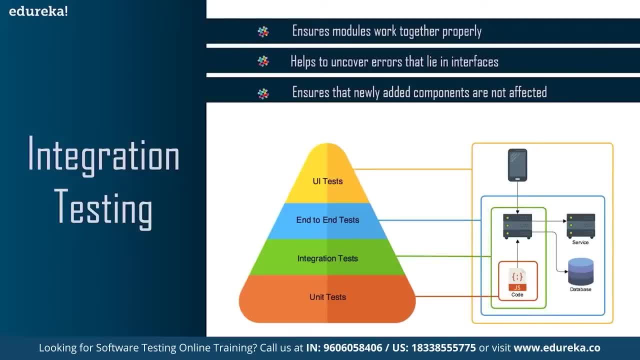 We have the red coded part, which is a small unit or a module. it's tested, Then it's combined with other unit and these both encoded, as you can see in the green part. So that's integration testing. you're combining two modules and you're checking out the interface. 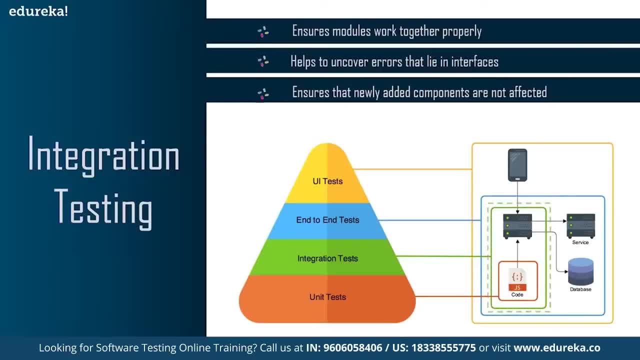 or the communication or the interaction between these modules. that's integration testing. as next level, Obviously, you have system tests that you combine multiple modules and check them as a whole and, lastly, you have acceptance test before the product or application is released to market. So it's as simple as that. 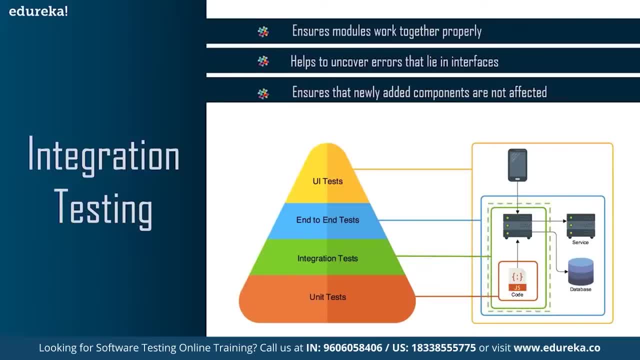 So, before we proceed any further, here's one more question: who performs integration testing? Well, software engineers or developers usually perform integration testing. However, there are instances when the company employs independent testers to do it for them. So, guys, there are different approaches to perform integration testing. 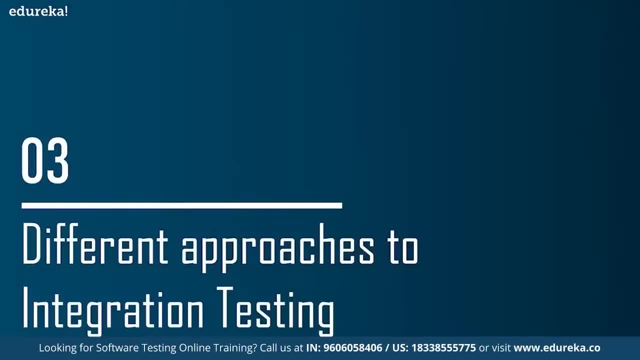 But before that, you should know that integration testing does not happen at the end of the cycle. rather it's conducted simultaneously with the development. So in most of the times all the modules are not actually available to test. So the challenging thing here is: how do you test something? 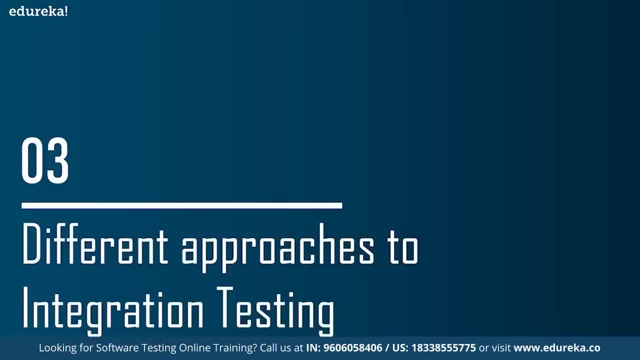 which does not exist. For that we have concept called stops and drivers. So sometimes we might face a situation where some of the functionalities are still under development. So the functionalities which are under development will be replaced with some dummy programs. These dummy programs are named as stops and drivers. 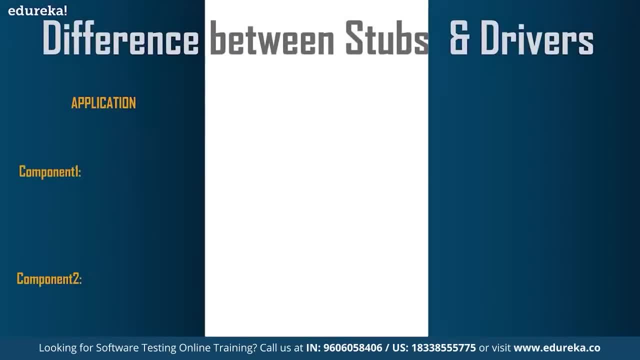 Let's check what they are. So here I'm considering a single application, and this application is two components: component one, which is login page, Let's say module A, and we have module B, which is admin page. as you can see, Login page is dependent on admin page. 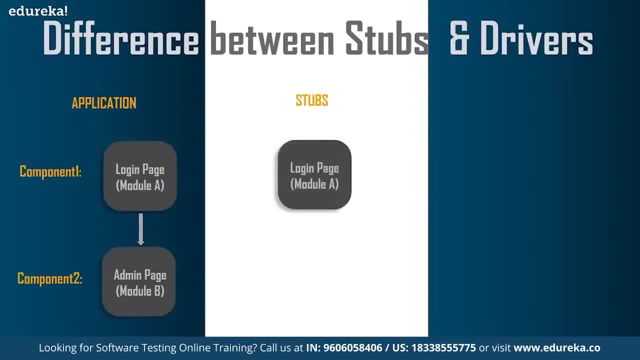 Now suppose if you have to test login page, developers have developed the login page and they have sent it to the testing team to test. The problem here is that admin page is not yet developed. So what do you do? instead of actual admin page, You create an dummy admin page. 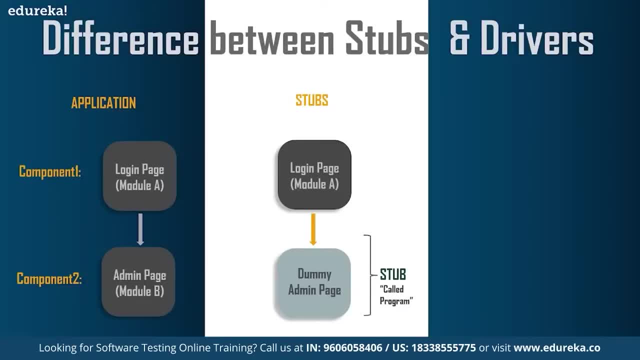 which has same functionality of the original one, but not all the core functionalities. and then, since login page is dependent on dummy page, you check the functionality of the login page in linking with admin page. So, without waiting for another module to be developed, you finish the test it here. 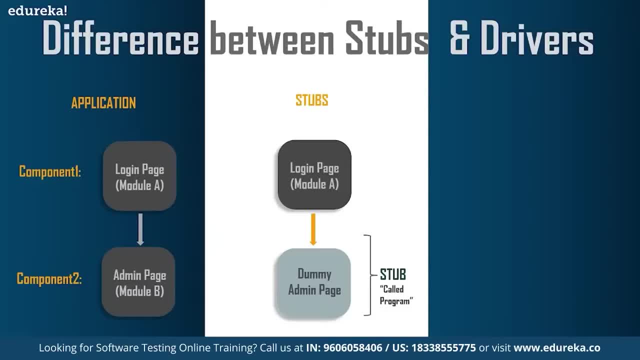 The dummy admin page is what we call stop or a called program. next coming to drivers, It's just reverse of stops. Let's say you have to test the admin page. It's ready, It's developed, It's been sent to testing team for testing. 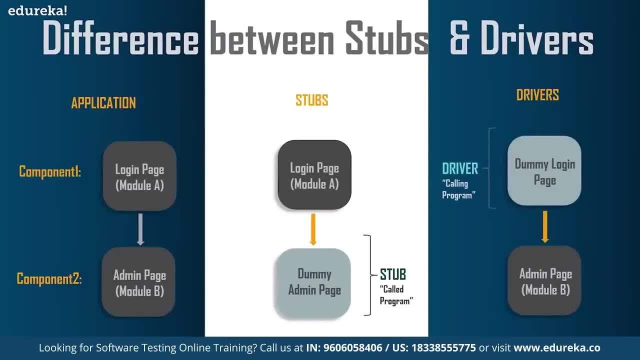 But the problem is login page is not yet developed. what you do- just like you created dummy admin page, here You create a dummy login page which is dependent on admin page. So this dummy login page is what we call a driver. It's called a calling program. 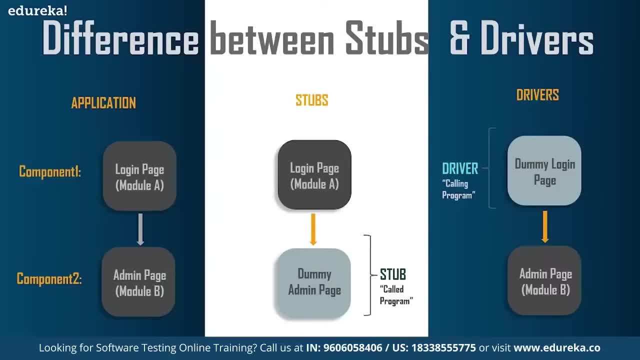 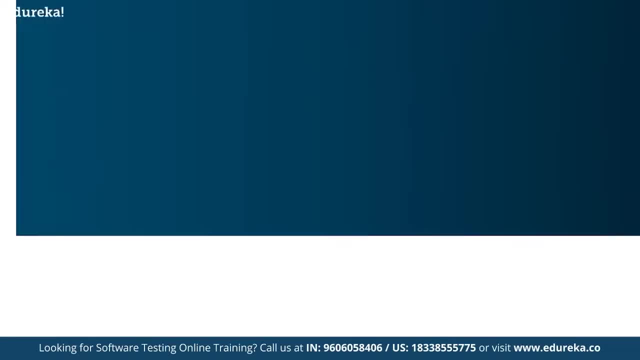 So now you know the difference between stops and drivers. right stops is a call program and drivers is a calling program. So now that you're aware of these concepts- which is stops and drivers- Let's get started with different approaches to integration testing. 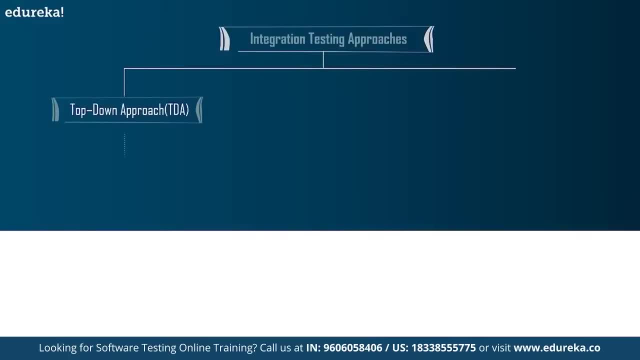 So basically, there are three types. to begin with, we have top-down approach. the top-down approach starts by testing the topmost modules and gradually moving down to the lowest set of modules, one by one. and then we have bottom-up approach, Which is exactly opposite of that of top-down. 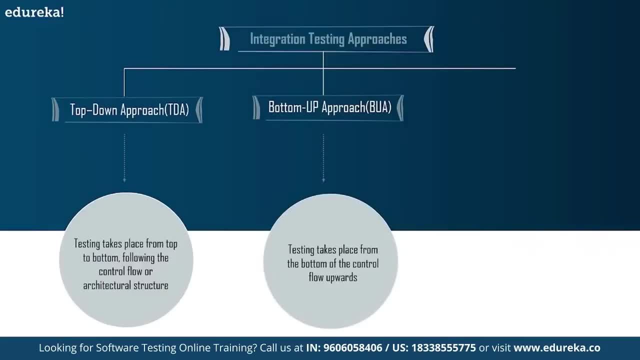 So, in bottom-up approach, starts with testing the lowest units of application and gradually moving up one by one, and then we have something called Big Bang testing. This Big Bang testing involves testing the entire set of integrated modules, of components together simultaneously, since everything is integrated together and being tested at once. 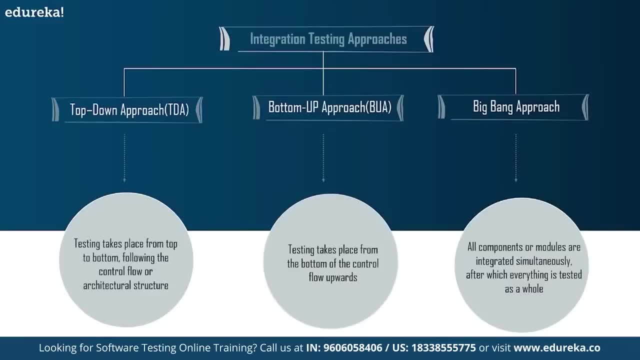 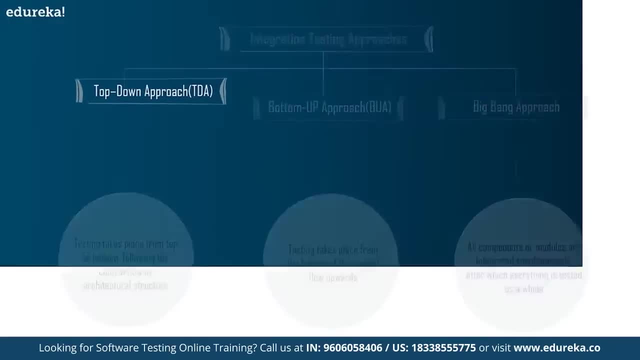 this approach makes it difficult to identify the root cause of problems. We will discuss more about advantages and disadvantages later on. Let's explore each of these techniques in detail. So let's begin with top-down approach first. So, like I said earlier, top-down approach testing takes place. 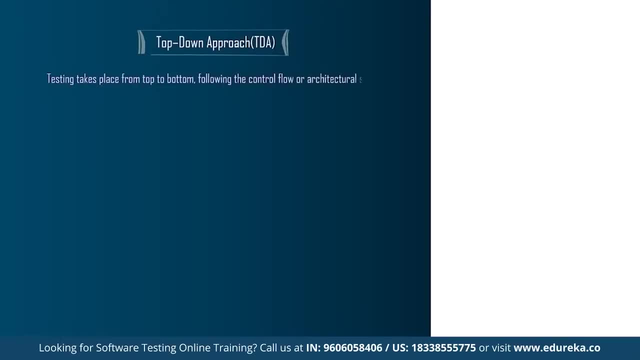 from top to down following the control flow of software system or architecture. So high-level modules are tested first, and then low-level modules, and finally integrating the low-level modules to a high level to ensure the system is working as it's intended to, but it's quite 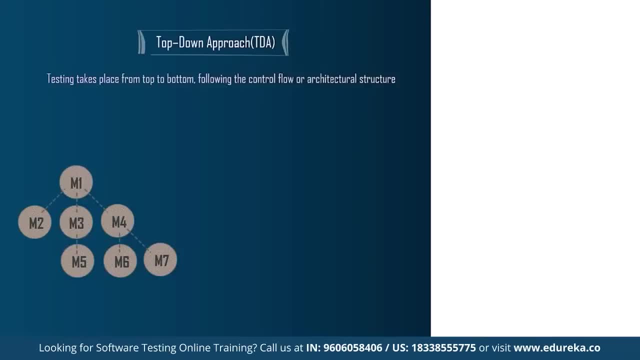 possible that, like we discussed earlier, when we are testing the high-level modules, Lower level modules might have not been developed yet. So what do you do in such cases? you deploy stubs. like we discussed, stubs are dummy modules that simulate the functionality of a module. 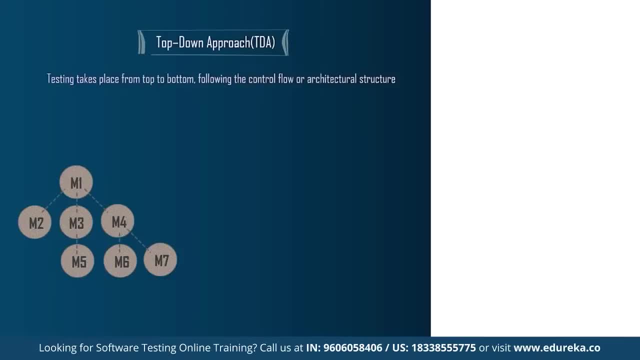 by accepting the parameters received by the module and giving an acceptable results Basically acts as a dummy. missing module generally stops. have hard-coded input and output. that helps in testing the other modules integrated with it. So for you guys to understand top-down approach in a better 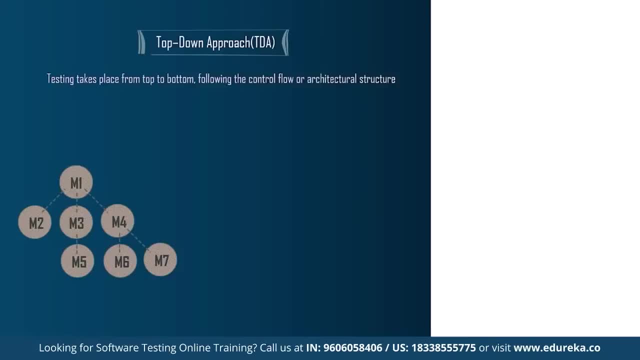 way. I have an example here. I have seven modules. module M1 is dependent on M2, M3 and M4. similarly, M3 depends on M5 and M4 depends on M6 and M7. now will performing top-down approach. we begin with a granular module. 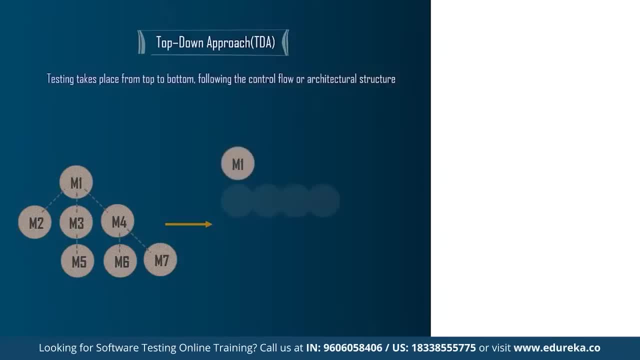 the first one, which is module M. So you want to test module M as you perform unit testing. It's working well and fine before you even start with integration testing. all this modules undergo unit testing, So they're well and fine now that you start integration testing. 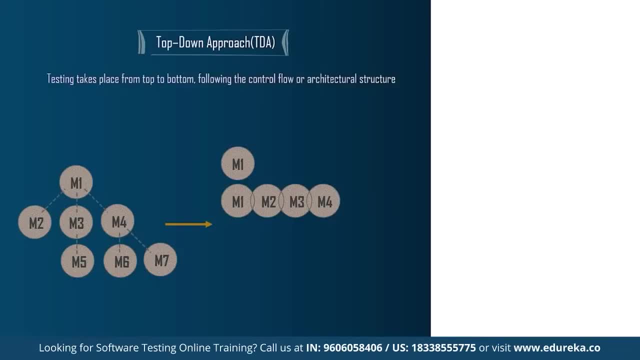 their module M1 depends on M2, M3 and M4.. We want to check module M1, but M2, M3 and M4 are not yet ready. what you do, you employ or deploy stops instead of these original modules, since they're not developed yet. these stops simulate the activity of M2, M3. 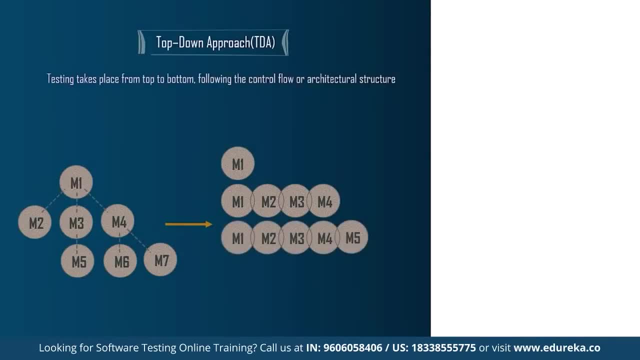 and M4. similarly, when you're testing M3, it depends on M5, and if M5 is not ready yet, you again use a stub here. same goes for the next level of testing, which is M4, which depends on M6 and M7. easy to understand. 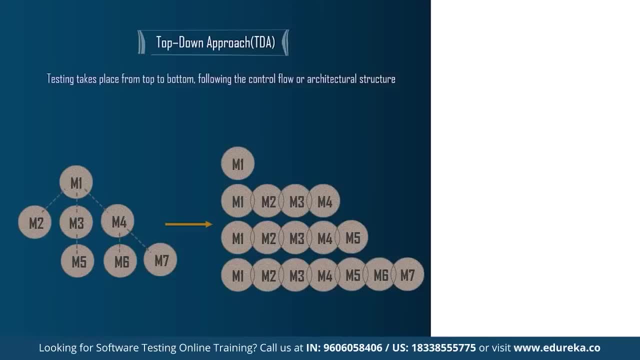 right with the help of an example, So that what stops are. these are called programs. and one more thing: simple applications may require stops which would simply written the control to their superior modules or high-level modules. more complex situation demands that sub stimulate a full range of responses like parameter passing and many of 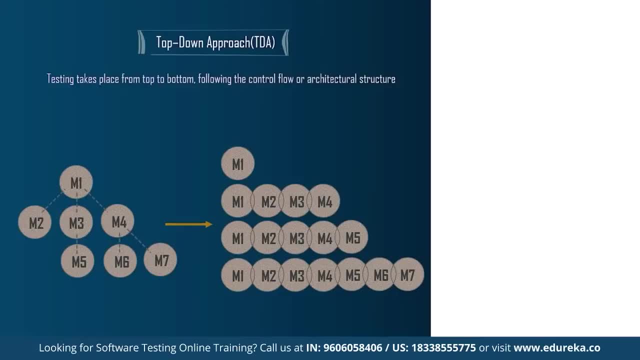 the features. these stops may be individually created by tester or they can be provided by software testing harness, which is a sort of software specifically designed to provide a testing environment. So in top-down approach, if the dependent modules are not ready yet, we use a concept called stubs. 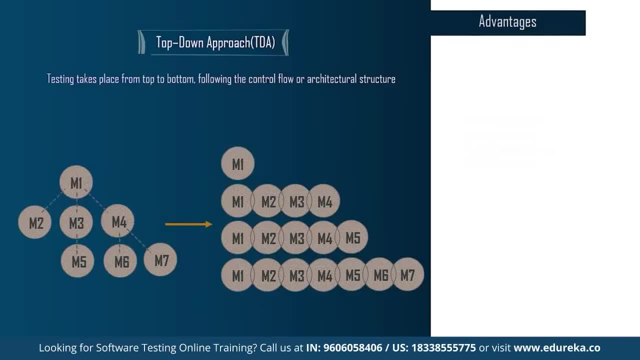 Well, just like any approach, this approach has advantages and disadvantages as well. The tested product here is extremely consistent because integration testing is performed in an environment which is mostly similar to real-world environment. Secondly, the stops and top-down approach can be written in lesser. 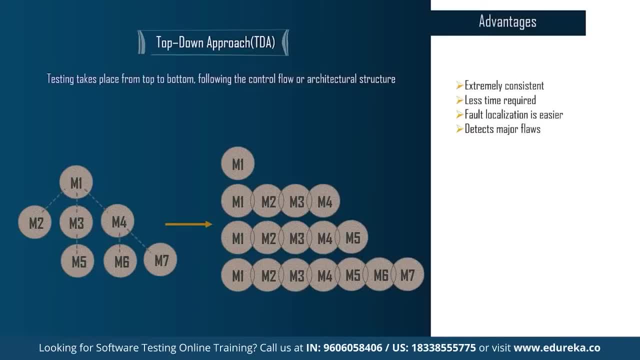 time compared to drivers because these stops are simpler to author. here for localization is also very much easy. in top-down approach The critical modules are tested in priority, which further helps tester in finding major design flaws early in the stage of testing. detecting major flaws is done very early in the process. 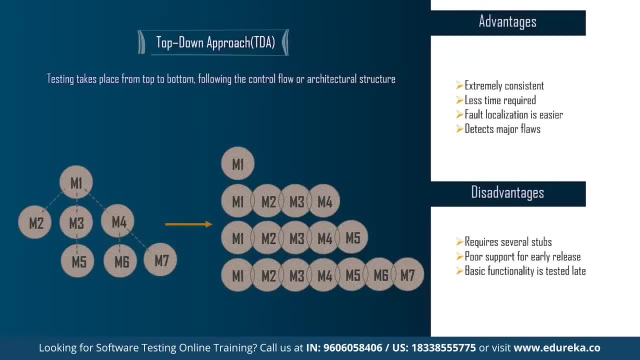 coming to disadvantages. as you can see, if the modules are not developed or ready yet, that requires several stops. modules at lower level of software are tested inadequately when compared to other modules. in the most popular disadvantage that you have to remember is that the basic functionality of the 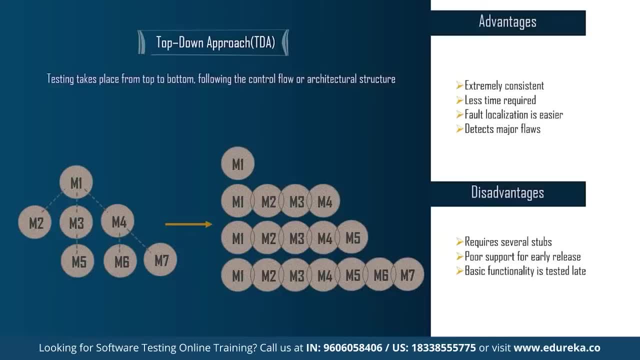 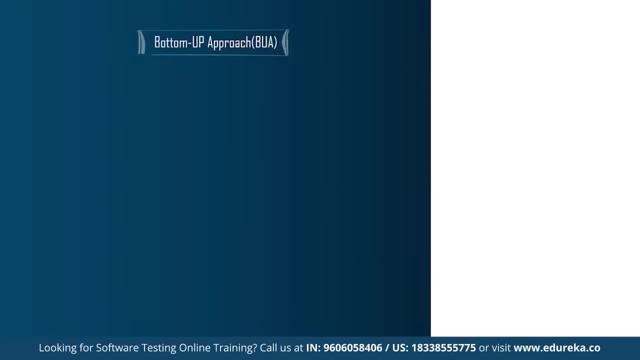 software and top-down approach Is tested at the end of the cycle. that can be a problem sometimes. that's all with top-down approach. Let's go with next approach, which is bottom-up approach. Well, it's complete opposite of top-down here. 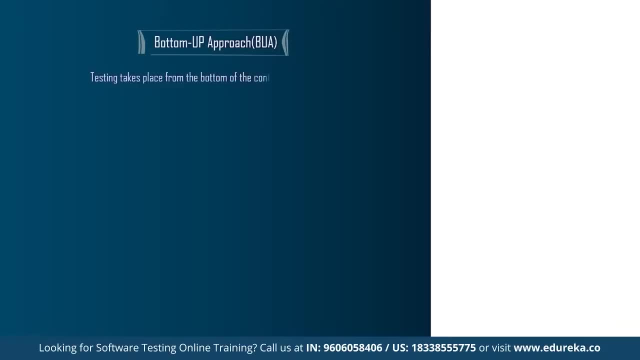 The bottom level units are tested first, and upper level units are tested then, step by step after that. So here testing takes place from the bottom of the control flow to approach. again, It's possible that the higher level modules might not have been developed by the time lower level modules are tested. just 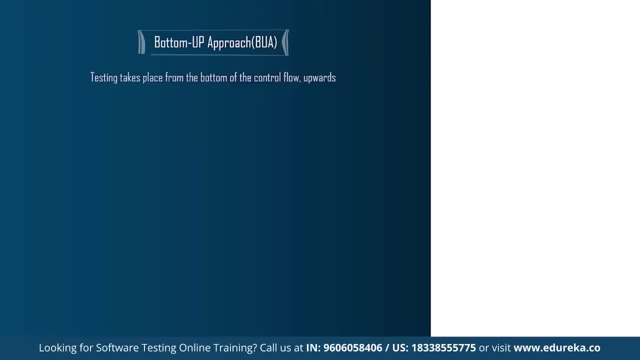 like we use tops In top-down approach, We use something called drivers here. These drivers are calling programs to simulate the functionality of higher level modules in order to test lower level modules. Let's consider the similar example which we did earlier. as you can see, I have seven modules: M1, M2. 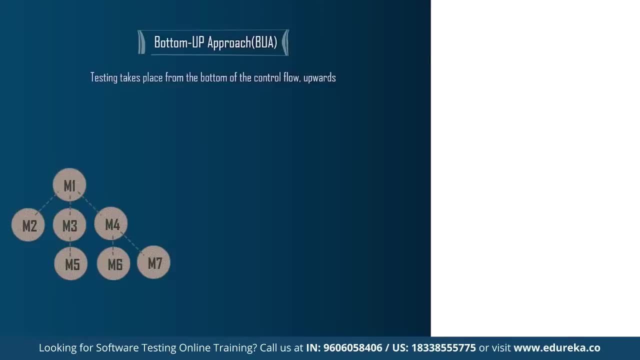 M3, M4, M5 and M6 and M7, M1 dependent on M2, M3 and M4 and M3 on M5, M4 and M6 and M7. now, each of these modules are unit tested, So that's well and fine. 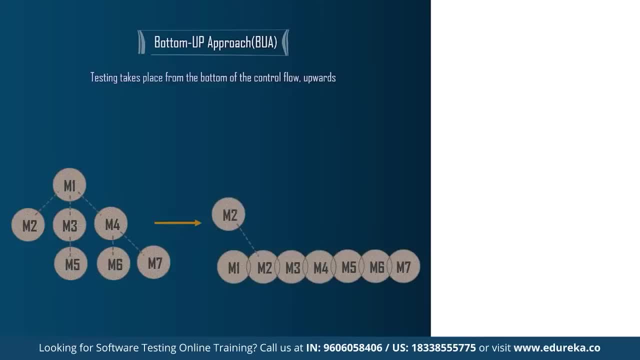 So we begin here from the lower level. So we start with M5, M6 and M7, but, as you can see, M3 and M4 are not developed yet. So what you do? you replace this M3 and M4 by drivers and then you test M5, M6 and M7. same goes for M3 and M4. 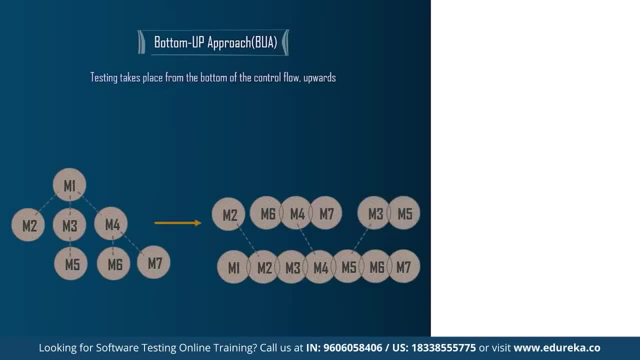 if M1 is not ready yet, and same goes for M2, because M1 is dependent on M2. and if M1 is not ready, we create a driver which simulates the functionality of module M1. here, just like stops, the driver can have different functionalities. the driver- 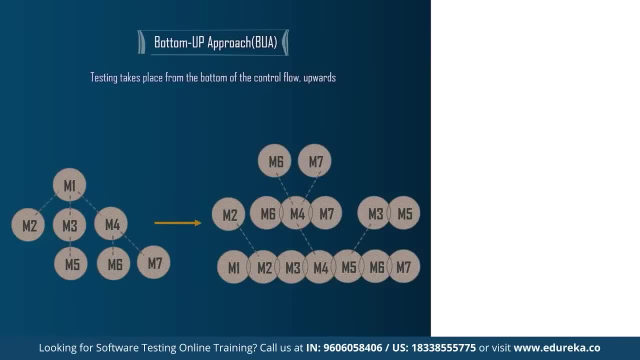 would be responsible for invoking the module under test. It could be responsible for passing the test data or it might be responsible for receiving the output data. and similarly, just like stops, the driving function here can be provided through a testing harness or may be created by tester as a program. 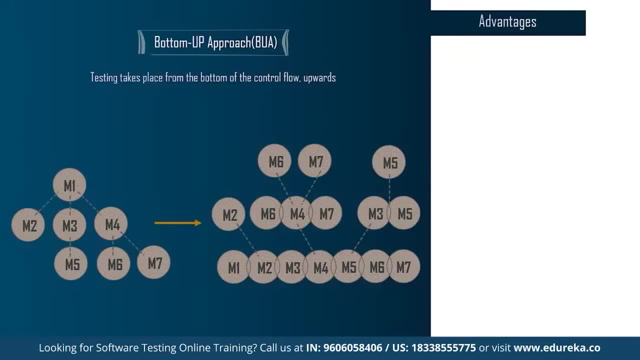 So that's the choice that the tester have to make, you coming to advantages in this approach. development and testing can be done together, So the product of the application here will be efficient and it will be according to customer specifications. the time requirement here is relatively less and tester conditions are much easier. 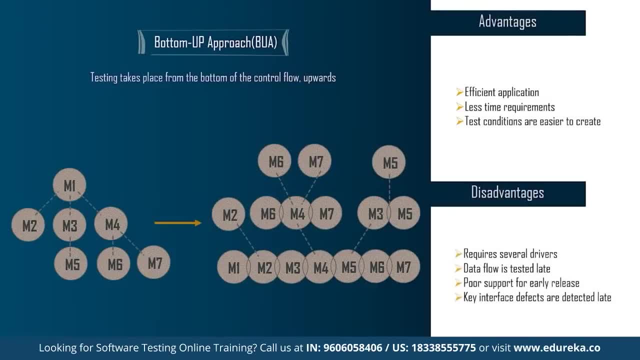 to create your coming to disadvantages. just like top-down approach, the bottom-up approach also provides poor support for early release of limited functionality and the need for drivers, because we use drivers right. if the modules are not developed, it complicates the test management, sometimes high-level logic. 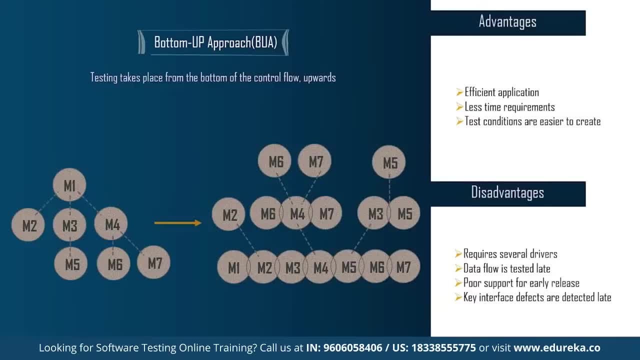 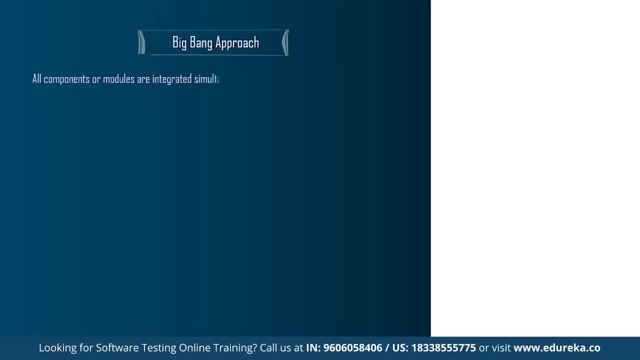 and data flow are tested late during the test process, and even the key interface defects are found later on than earlier stage. So these are the disadvantages, And then after that we have another approach, called Big Bang approach, once all the modules are ready after testing individually. 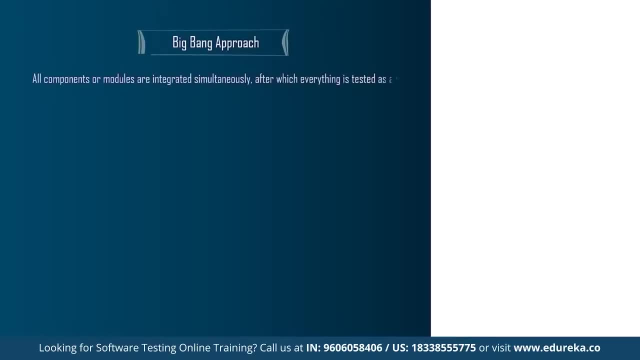 this approach of integration testing combines them at once and perform testing. That's what Big Bang testing is. So instead of just starting from top or down, it just combines all the units or modules once they are ready and performs testing at once. though Big Bang approach seems. 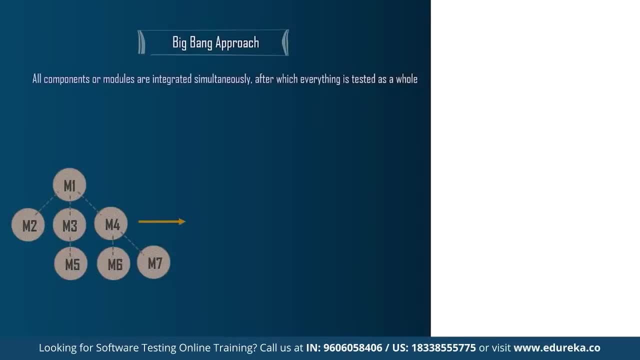 to be advantages when we construct independent modules concurrently. this approach is quite challenging and risky because when you combine all the modules and test them at once, and if there are any errors, it's difficult to find out what is the reason for error, since all the modules are combined. 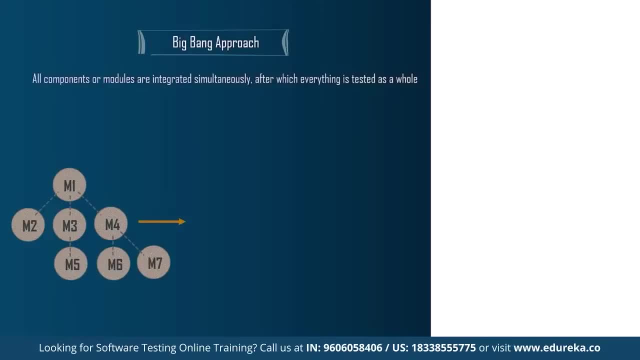 and tested at once. I'm going to take similar example here. There's nothing to explain, It's pretty straightforward. all the modules are unit tested. Then you wait until all the modules are developed. You don't use any stops or drivers here. Once all the modules are developed, you combine them. 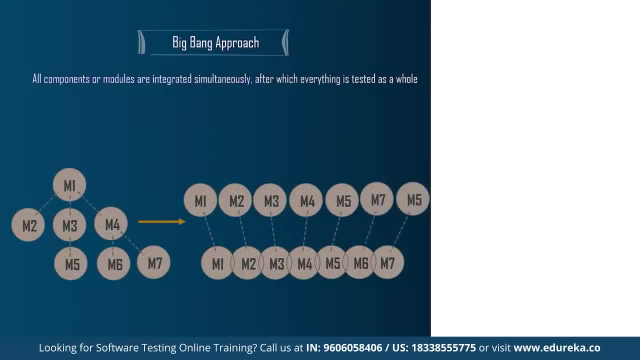 and test them as a unit, as a combined unit, as a whole. So that's what Big Bang testing is, and we have advantages and disadvantages. talking about advantages, As you can see, all the components are tested at once, So it saves a lot of time. 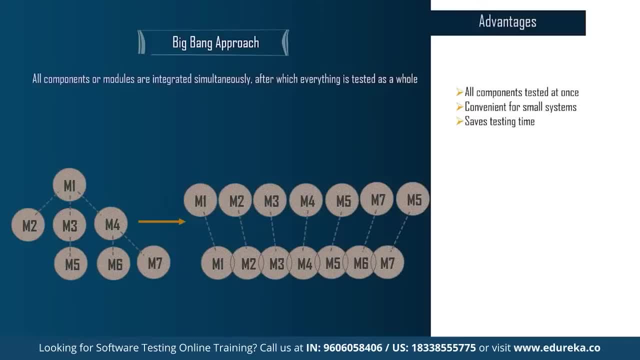 because we don't use any stops and drivers and also it saves a lot of time. and this process is convenient for smaller systems because there will be less number of modules to combine or act on, coming to disadvantages. You'll have to wait for each of this module to be developed. 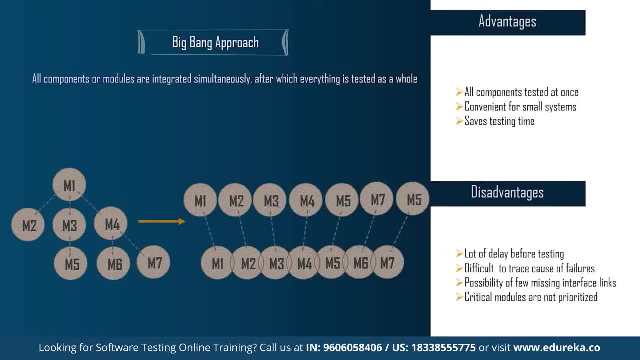 right before you start testing, So lot of time is wasted or delay. There's a lot of delay before you actually start Big Bang approach and since there are a lot of modules which are combined and tested at once, It's difficult to trace the cause of failures. 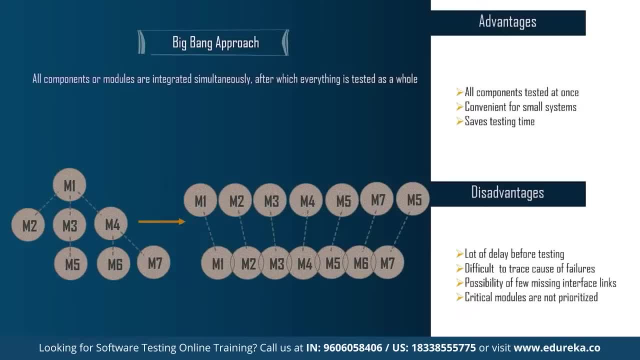 if there are any, and sometimes it's quite possible that when there are so many modules, few interface links between some modules might be missing and you will not even notice that and, as you can see, no module is prioritized, which sometimes might be problematic. critical modules need to be prioritized sometimes. 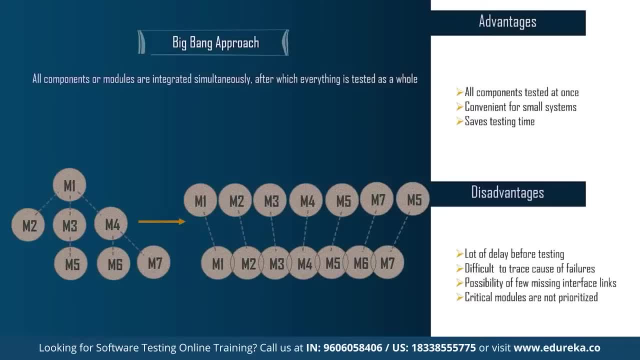 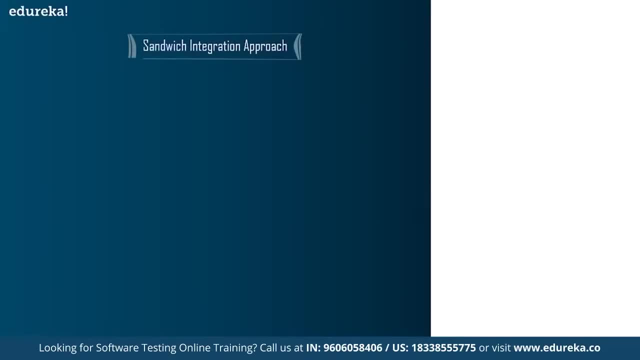 So these are the disadvantages. so, to overcome the limitations and exploit the advantages of each of these top-down, bottom-up and Big Bang approach, We have something called sandwich integration approach, or it's also known as hybrid testing approach. Well, as the name suggests, it is a mixture of two approaches. 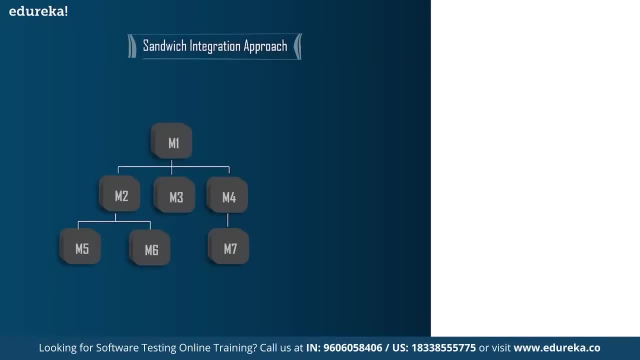 like top-down approach as well as bottom-up approach. in this approach, The system is viewed as three layers consisting of the main target layer in the middle, another layer above the target layer and the last layer below the target layer. So three layers, as you can see. m2, m3, m4 are the middle layer. 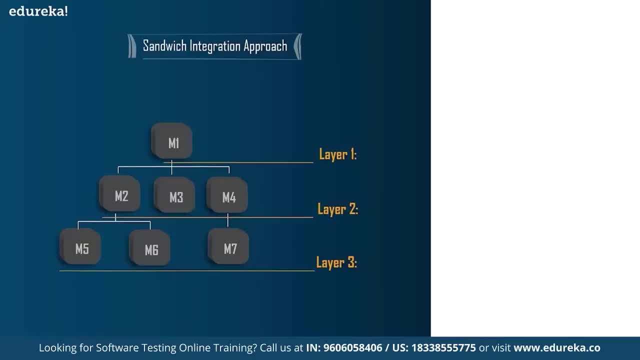 the target layer. m5, m6, m7 are the layer below that and m1 a layer above target layer. So the top-down approach is used in the top most layer, that's layer 1, and bottom-up approach is used in the lower most layer, which is layer 3. it might sound a little complicated. 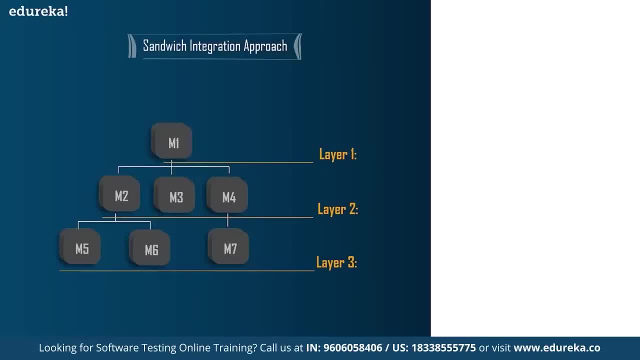 but sandwich approach is very useful for large enterprises and huge projects that further have several sub projects, and sometimes, when development teams follow a spiral model, the module itself is as large a system. then you can use sandwich testing. the resources that are required here are immense and big team perform both top-down as well as bottom-up method. 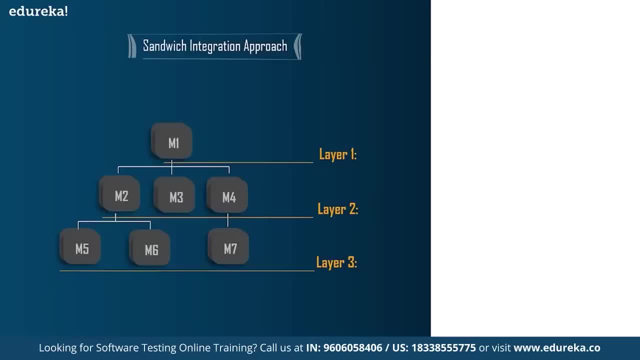 at once, Sometimes one after the other. so basically, here you use the advantages of both top-down as well as bottom-up. Well, obviously this process, as it looks complicated, It has a lot of disadvantages, since both top-down and bottom-up are executed at the same time, or one after the other. the cost: 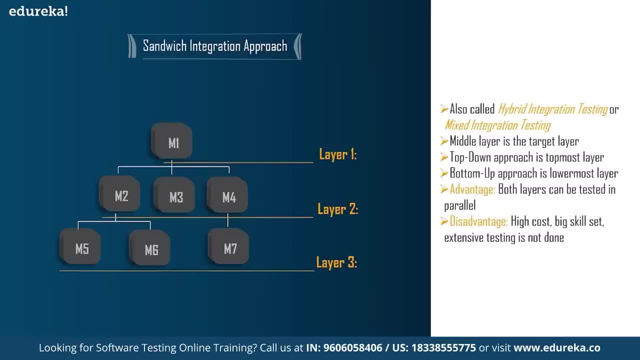 of testing is literally high. it cannot be used for smaller systems because the interdependency between the modules is quite complicated. It also makes sense that when individual system is as good as complicated system, then sandwich integration is best, and obviously you're using different approaches here. 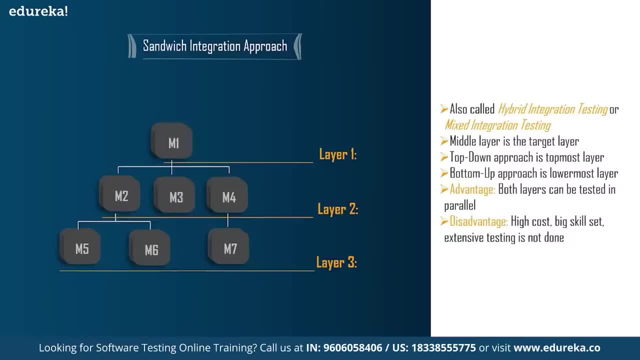 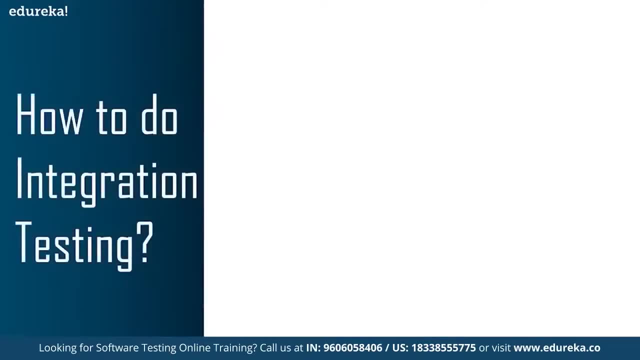 So the development team or the testing team should have different skills to ensure that the testing is done in a proper way. So these are the disadvantages. moving on to next topic, Let's see how you actually perform integration testing. Well, it's highly similar to any of the testing process, just 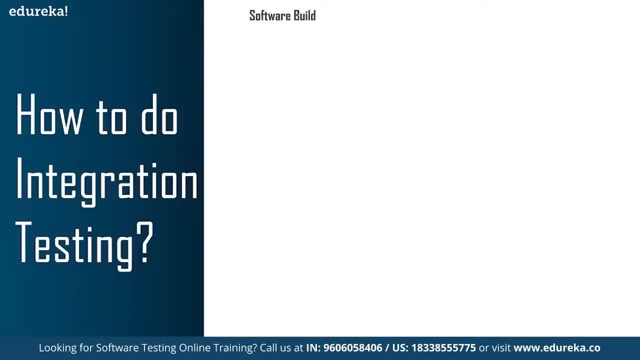 like unit testing or any other testing. So the first thing you do is choose the module or the component which you have to test, and you also select the strategy that you want to employ out of the strategies which we just discussed. and before you actually proceed, you have to make sure. 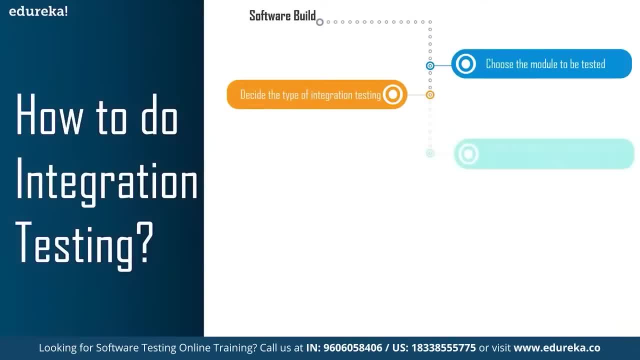 that each of these module which have selected is unit tested already. then you deploy the chosen modules or the components together and you make the initial fixes that are required to get started with integration testing. then you perform functional testing and test all use cases for the components chosen similarly. 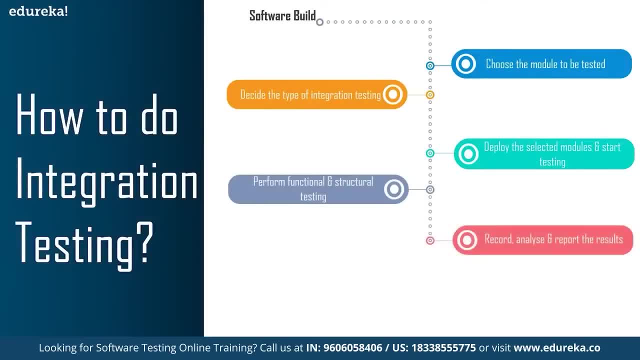 you perform structural testing and test the component chosen. after you've done all the testing, you record the results of the above testing activities. you repeat the above step until the complete system is fully tested. as in, you combine the new module, test them and again, everything is proper. 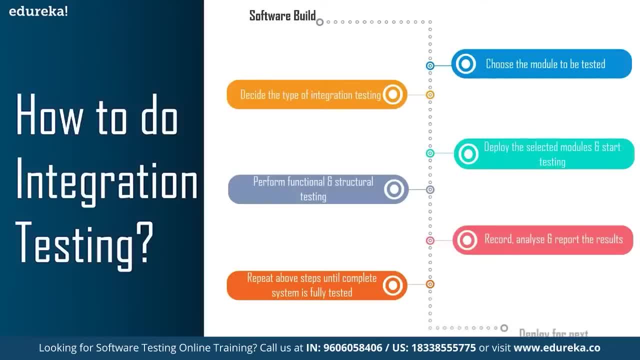 you combine with the third module and do the same thing again and again. So to summarize very simple: first you should prepare a test plan, then your design test cases, test scenarios, test scripts according to your plan. execute the test cases, followed by reporting of defects. now track. 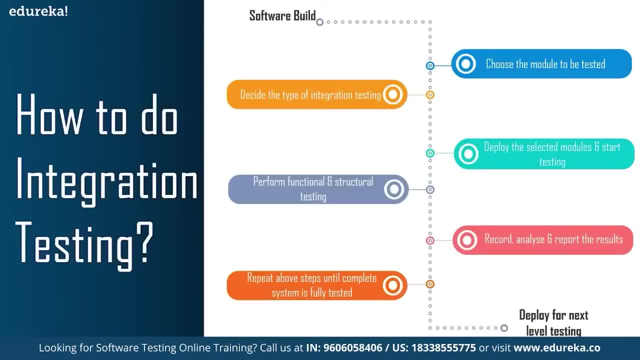 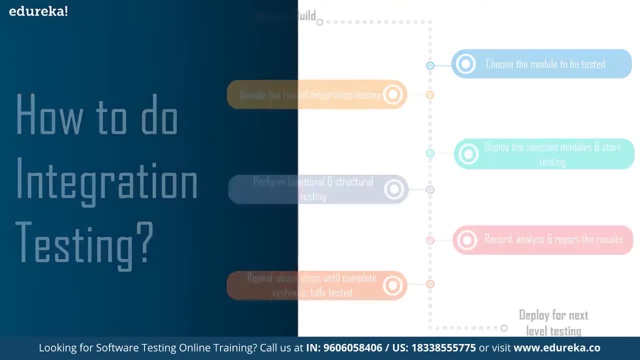 and retest effects as soon as they arise, and then you follow the entire process again and again until your entire system is tested. So that's how you perform integration testing. simple, right. Moving on to the next part of the session, I'm sure you guys have understood what integration testing. 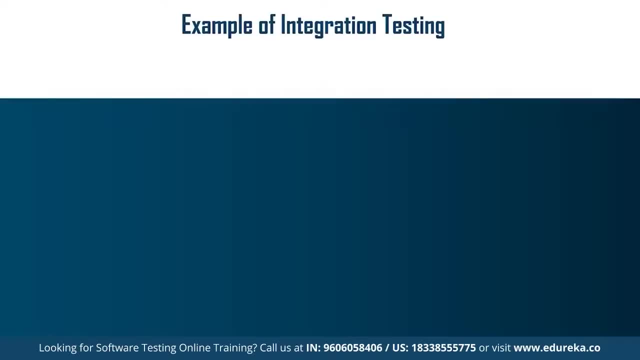 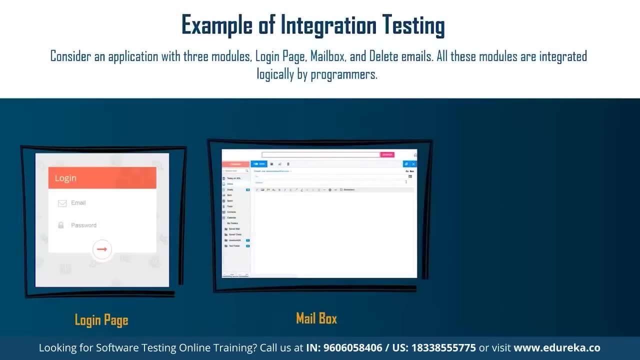 is by now, But anyway, let's go ahead and try to understand it in much better way with help of an example. So, as you can see, I have three modules here: a login page, a mailbox and a delete email page. So, like I said earlier, integration testing majorly focuses. 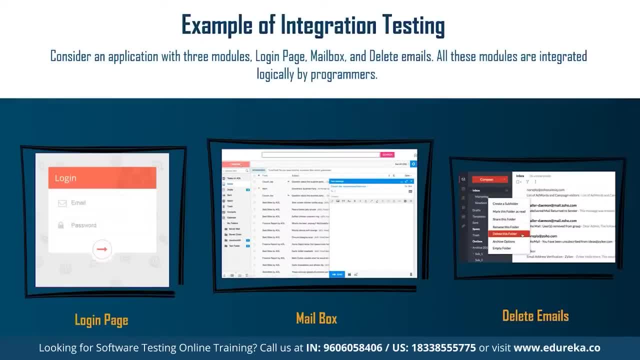 on interfaces and the flow of information between these software modules. So priority here is given to the integrated links instead of the unit functions that are tested in advance. So you do not have to focus on testing the login page, as it's done already in the unit testing. 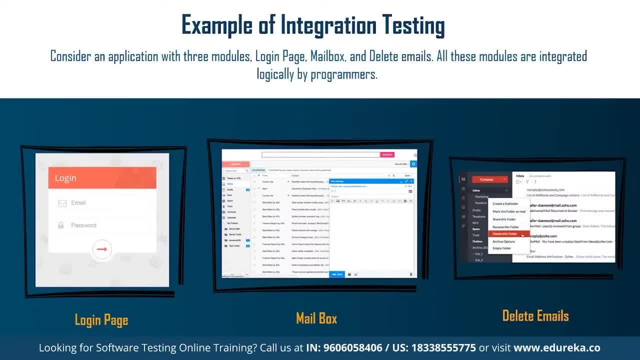 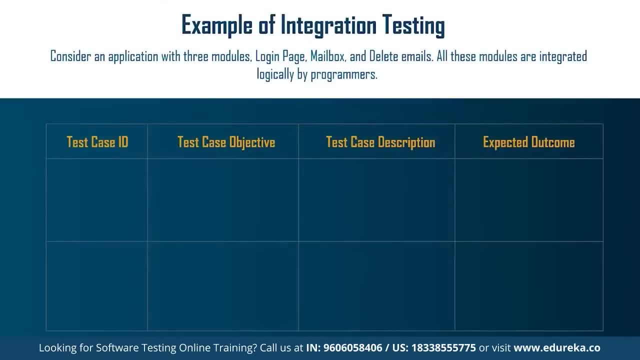 You should focus on its interface link with the mailbox page. Similarly, check the interface link of mailbox with the deletes email module. So let's go ahead and take a look at the test cases. So the first test case objective here is to test the interface. 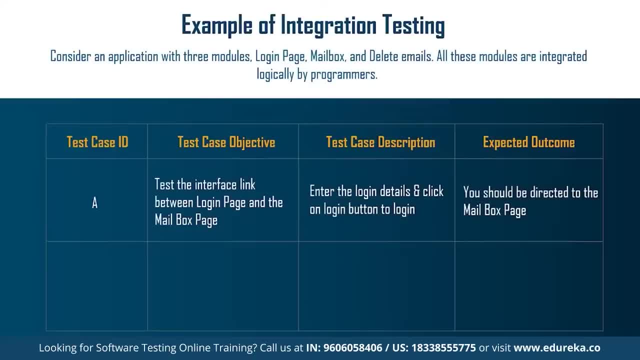 link between the login page module and the mailbox page module. So the description: you enter the login details and you click on the login button. As soon as you do that, you should be taken to the mail page. If that's happened, it means that the interface link between your login page as 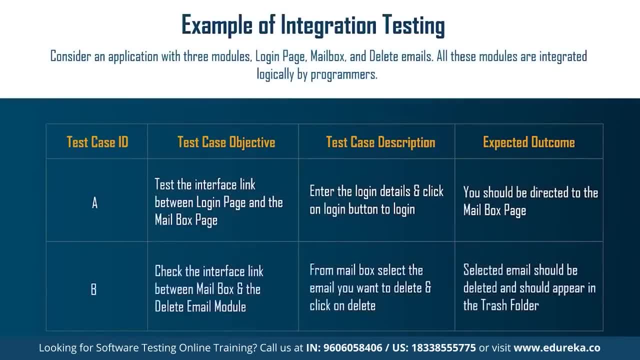 well, as mail page is working properly. Similarly, we have second test case to check the interface link between mailbox and delete email module. So what do you do? you go to mailbox, check the email that you want to delete and click on delete option. As soon as you do that. 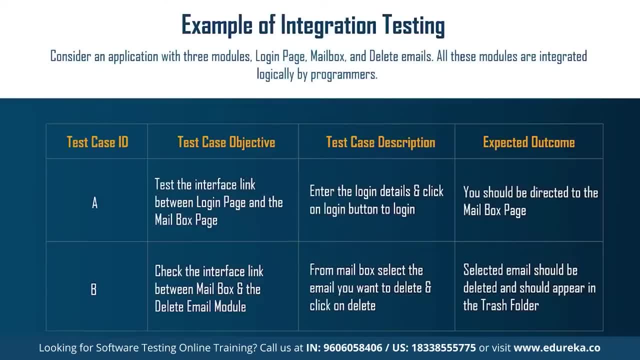 it's quite straightforward that email should be deleted. That's not what we're checking. What we're checking here is that the deleted email should have to appear in the trash folder. So that's the interface between the mailbox and the delete interface page. 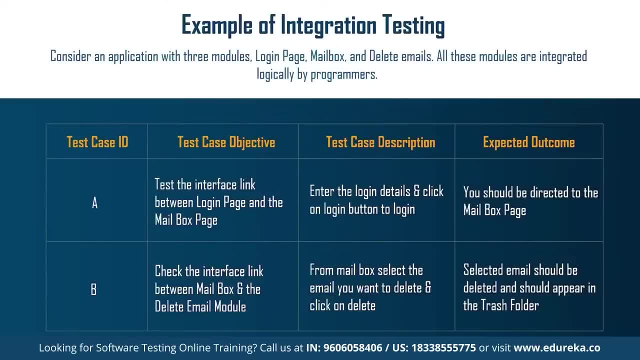 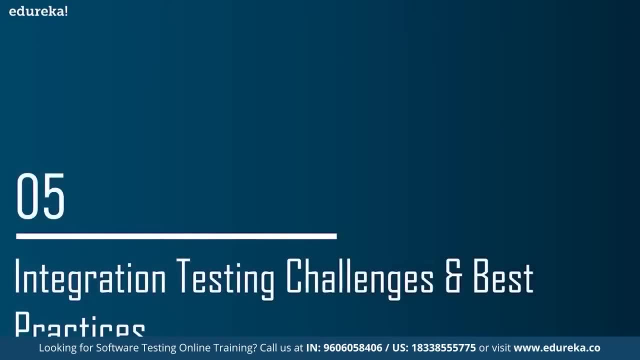 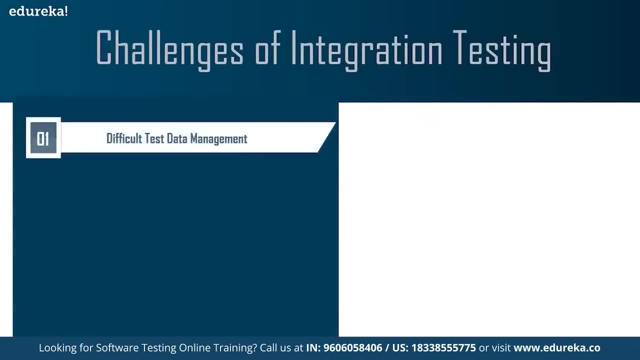 So integration testing, like I said earlier, is all about the interfaces between modules, not about the functionality of individual module. So, guys, like any other testing, integration testing also has challenges that you might come across. For example, integration testing means two or more systems are integrated to ensure that system is working properly. 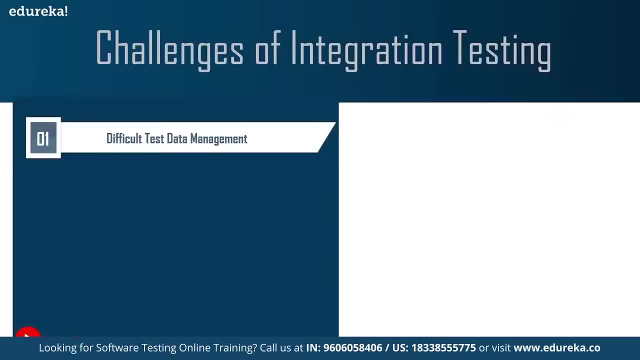 So not only the integration links are to be tested, but exhaustive testing related to environment And should also be performed. it ensures that all the integrated system components are working properly. There are different parts and permutations to apply for testing the integrated systems, So basically, test data management becomes difficult because 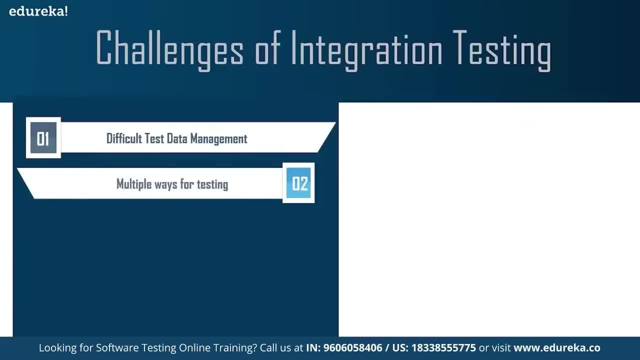 you have multiple test cases and different parts and permutations that you have to follow to perform integration testing. It's tough managing integration testing sometimes because you have various factors that you should consider, like database platforms, environments, etc. Similarly, whenever a new system System is integrated with the legacy system, 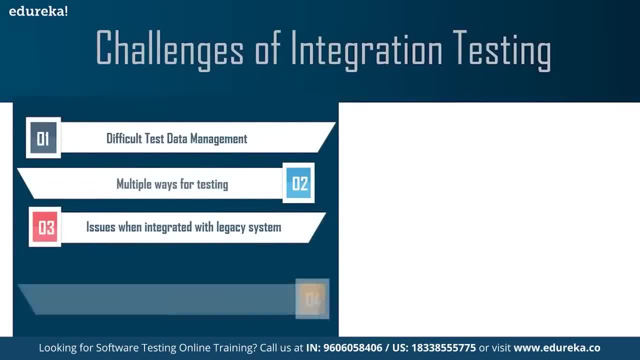 It needs a lot of testing efforts and changes. same goes when you are combining one legacy system with other legacy systems. in such cases you have to develop test cases which test the entire unit functionality or combined unit functionality. So developing test conditions and test cases also becomes. 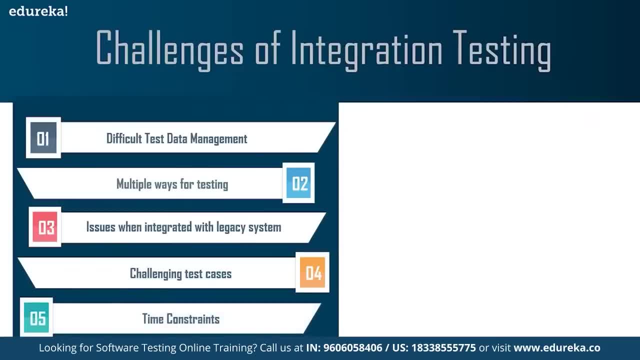 quite challenging. and lastly, when you're integrating two systems developed by two different companies, It's a big challenge for programmers. No one is sure how one system will affect the working of another system. So to minimize this impact, several considerations should be kept in mind to make integration more successful. 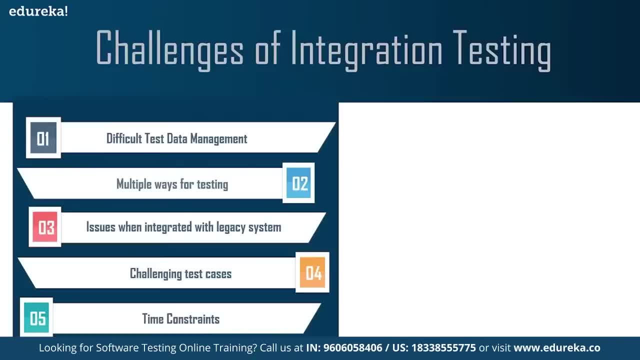 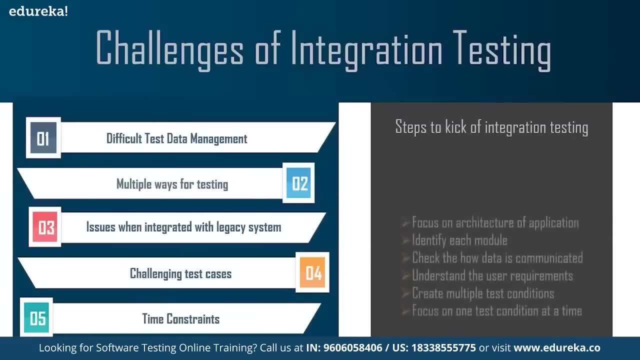 Well, they cannot avoid all this, but you can follow certain practices to at least make the effect of these challenges a little lesser on your testing. First of all, you need to check if the testing strategy that you have applied is suitable one for your requirement, that is, for your application. 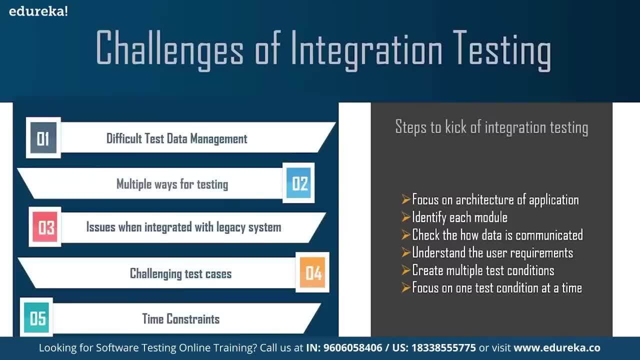 requirement or software requirement or not, and based on the test strategy that you have chosen, and if you're sure it's right, you prepare the test data and test plan accordingly. after that, you need to focus on the architecture design of an application and identify the critical modules. these critical modules should: 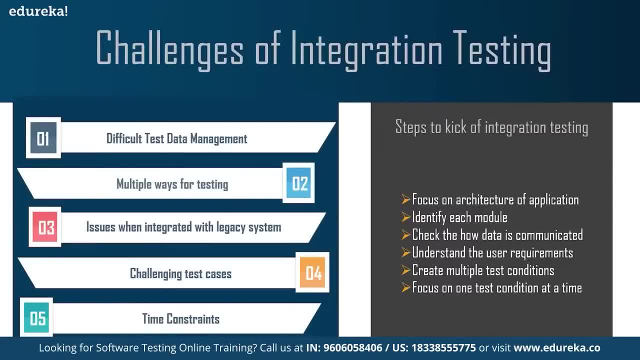 be tested on priority. and then you get the interface designed for the application from the architecture team and generate test plans to verify interfaces in detail. So the main concept of goal of integration testing is to check the interface link between modules right. So you need to have the basic understanding of the interface. 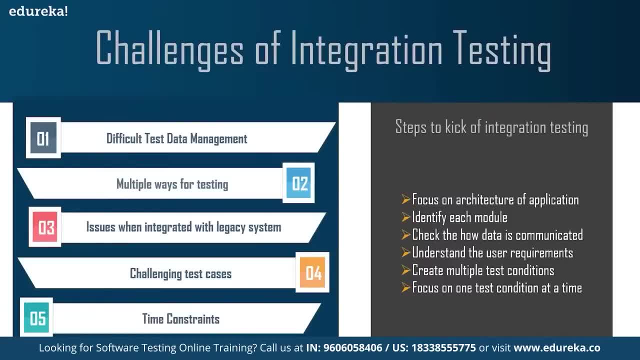 architecture. each of these interfaces, like database, external hardware or any other software application, should be tested and should be understood in detail. test data plays a critical role in any integration testing, So you have to take into consideration that as well. So keep mock data handy before the execution of test cases. 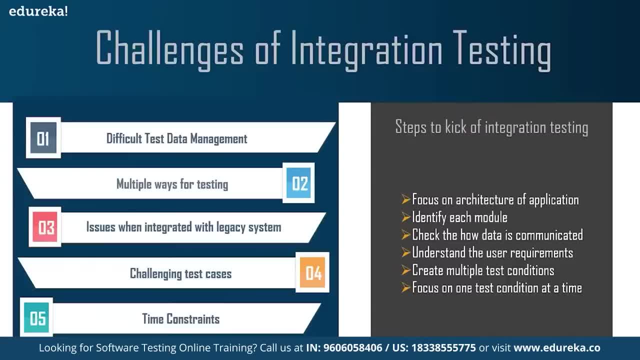 So do not decide on the test data while executing test cases itself, because, as you know, that user requirements keep changing and, according to that, you might have to change the data that you want to test on. apart from these, I have few things which have put up on the screen, as you can see. you need to identify. 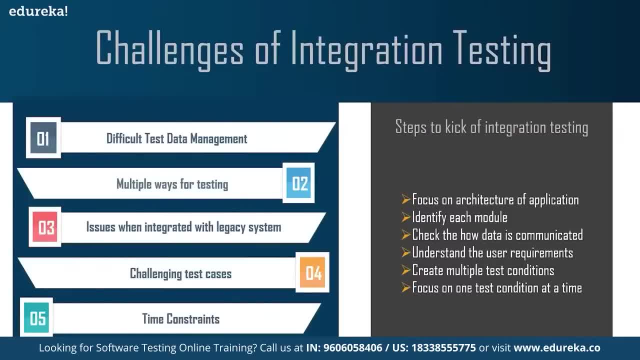 each module, check how data is communicated, understand the user requirements, create multiple test conditions according to those requirements and focus of one condition at a time. So these are certain things that you can follow to make integration testing much more simpler and less complex. So, guys, that's all about it, integration testing. 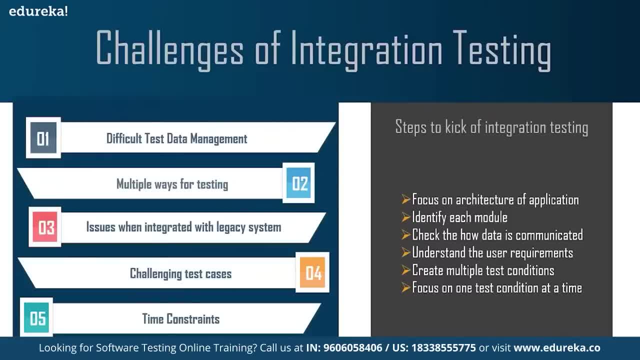 It's types, example, strategies, practices, challenges. We have discussed everything, have tried to explain what integration testing is with an example for better understanding of the concept. So integration testing is an important part of testing cycle that makes it easy to find defects when two or more units are. 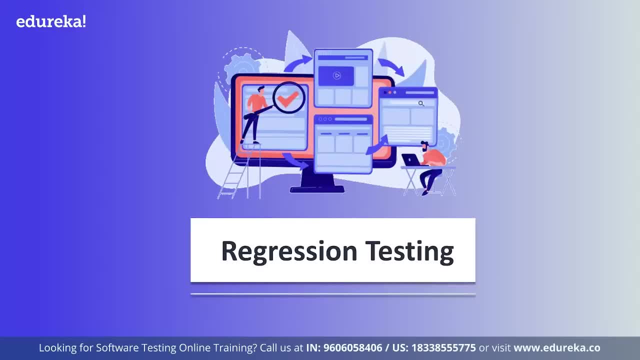 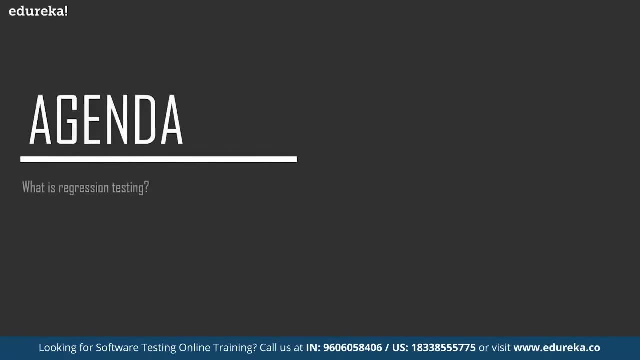 integrated Regression testing. so we will begin this session by discussing what is regression testing and benefits of using regression testing. moving on, We'll see when to apply regression testing. then we will check out types of regression testing, how to do regression testing and techniques of regression testing. and then comes 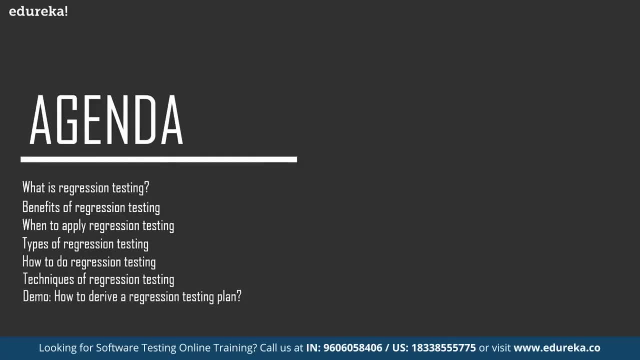 the interesting part will be doing a demo in which we will see how to derive a regression testing plan And finally, we will end this session by talking about regression testing challenges and best practices that you should follow while performing regression testing. So I hope agenda was clear to you guys. 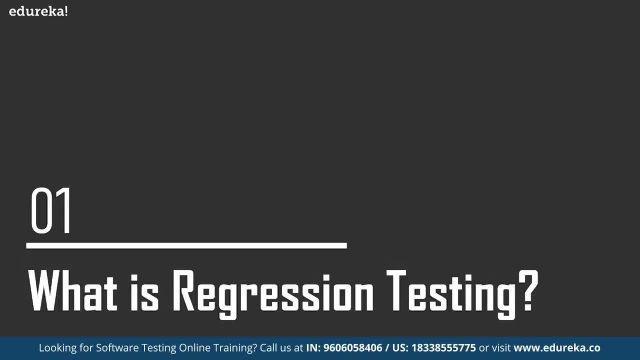 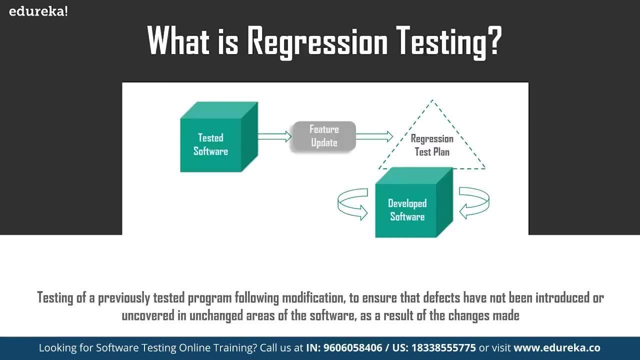 Let's get started there. So what is regression testing? a regression test is a system-wide test that's intended to ensure that a small change in one part of the system does not break existing functionality elsewhere in the system. It's important because without regression testing it's quite. 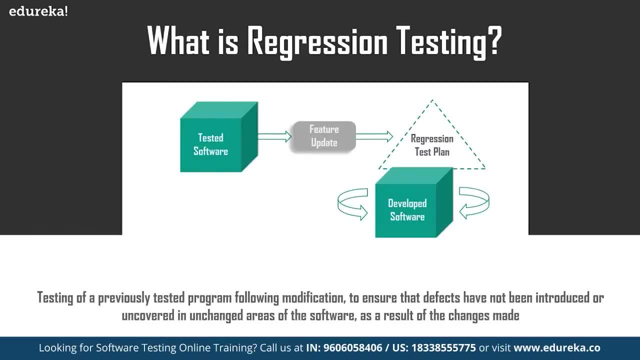 possible to introduce Intended fixes into a system that could create more problems than the souls. So let me give you a simple real-world example. You take your car to a mechanic to get the air conditioning fixed and when you get it back, the air conditioning is working. 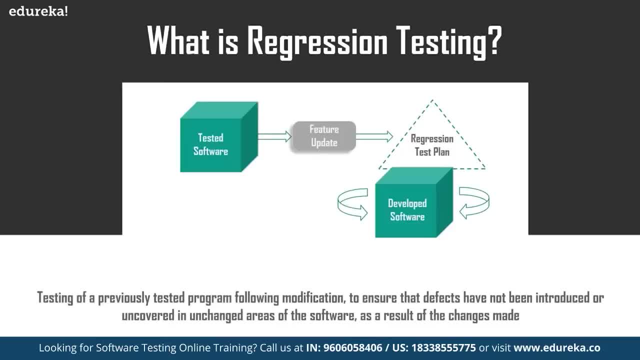 properly, but the gas tank sensor is no longer working. If regression test is an unintended change, then regression testing is the process of hunting for those changes. put simply, regression testing is all about making sure old bugs Don't come back to haunt you. Let's take a look at technical example that illustrates what 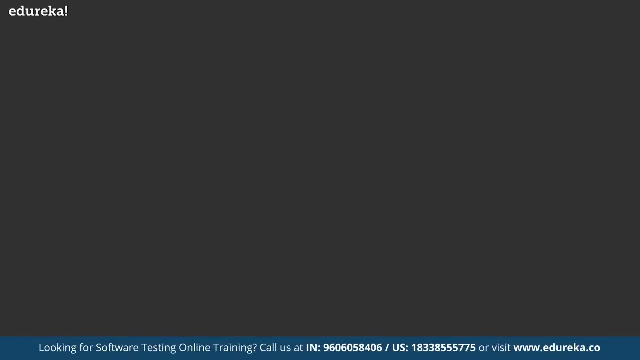 can happen when regression testing is not used. So one day the manager of accounts receivable Department at Wayne Industries uncovered a bug in company's financial system. It turns out that the module responsible for reporting overdue invoices was not listing all the overdue invoices. The bug was assigned to a developer to make the fix. the developer 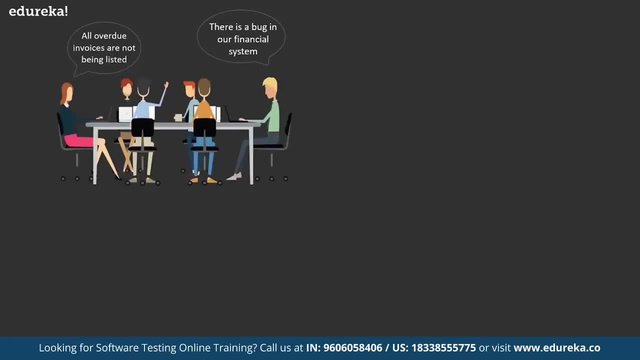 followed company policy and unit Tested the new code. the unit test proof beyond a shadow of doubt that fix worked as intended. developer did a good job. The fix was released into production. so far, So good. a week passes. then a strange behavior occurs when the 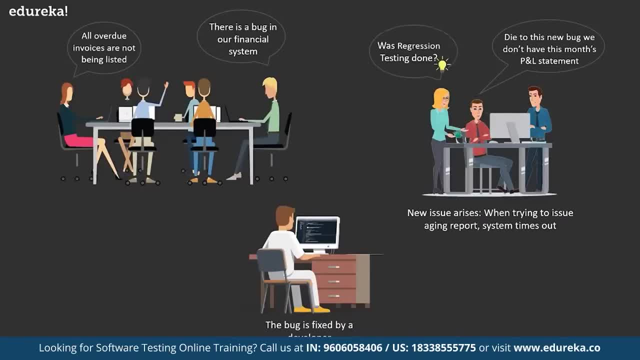 accounting department tries to run the company's month and profit and loss statement. whenever the system tries to issue an aging report, the system times out. So what is aging report now? a aging report separates and sums invoice amounts according to age, Like 30 days past you, 60 days past you, 90 days past you, Etc. 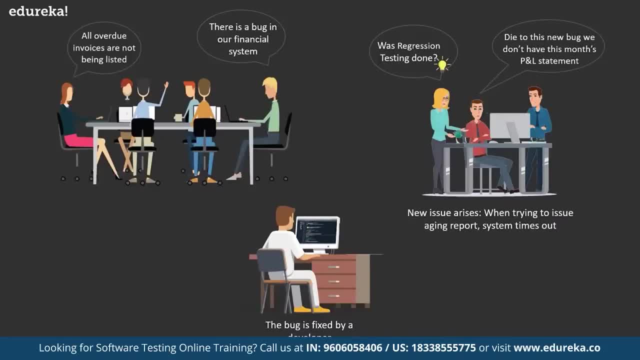 So what happened was when they were trying to issue an aging report, the system timed out without its month and profit and late statement. the company doesn't know if it's making money or losing money. The accounting department is really upset about it. The accounting manager contacts the software development. 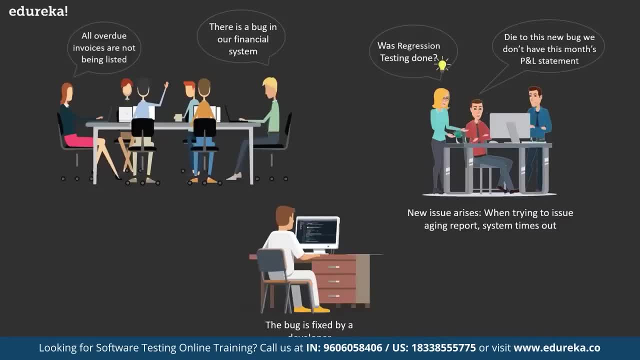 manager to report the issue and seek remedy as soon as possible. So tech leads and quality analyst manager brought in to find out the issue. Turns out that the new code which was encapsulated in the function was only tested for small database when the same was applied for production data. 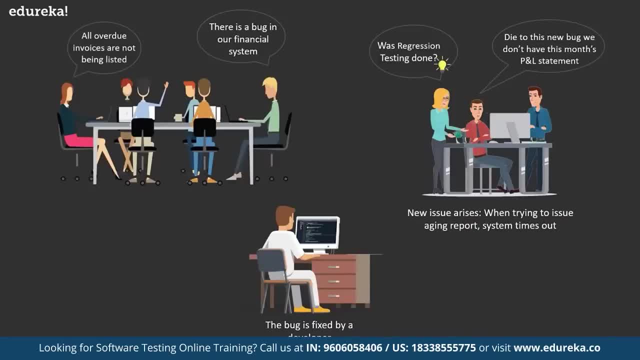 which is usually very large. the code didn't work as expected. So what you have to notice here is that if the fix had been incorporated into system-wide regression test that used a copy of data running in production, the chances are very good that issued have been resolved before the release to. 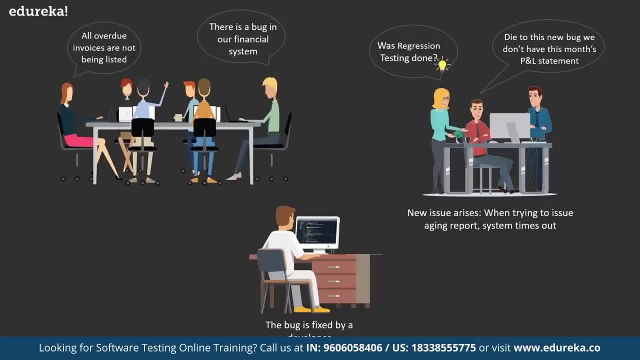 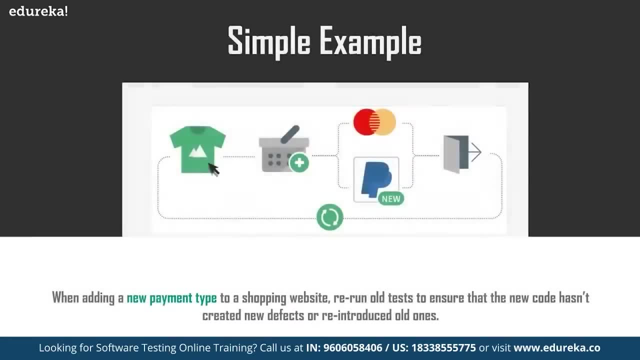 production or discovered. actually, that's how important regression testing is. Well, that was a little technical right. Here's a simple one. This is just the testing of a simple e-commerce website, and here we're checking the functionality of payment options. So first of all, there was only one payment option. 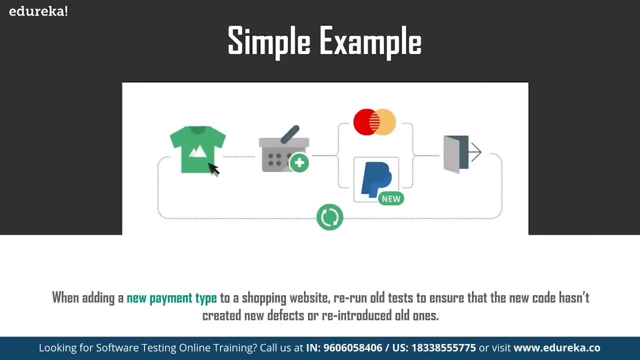 Let's say credit card. So item has been added into card. You use the one payment option which is available, then make the payment and everything is working properly when tested. now the company wants to add one more payment option, Let's say PayPal. So now the company checks if the option of using the credit card 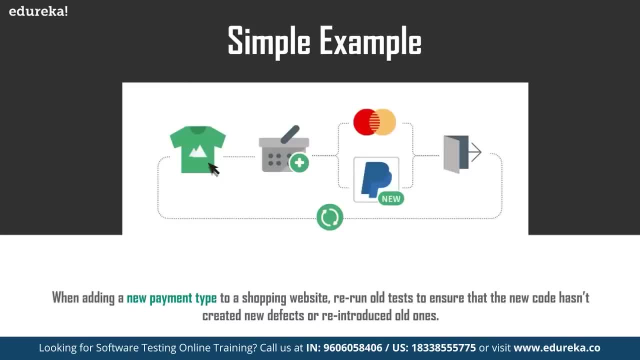 option of using PayPal is working properly or not. So again, the item is added to card, the payment is made through the new option which is added, and everything is working again. Now what company does is it goes ahead and test for the previous payment option again. then they find out that the previous 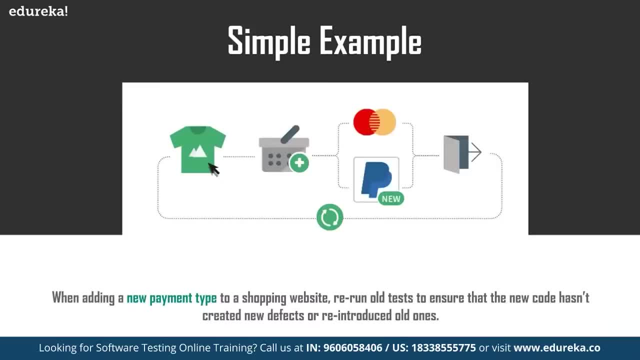 payment option is not working properly. So what happened here? the new payment option, which is PayPal, has affected the old one, which is credit card. So what they do, the perform regression testing. So what they have done here is They're checking if the new payment option has affected. 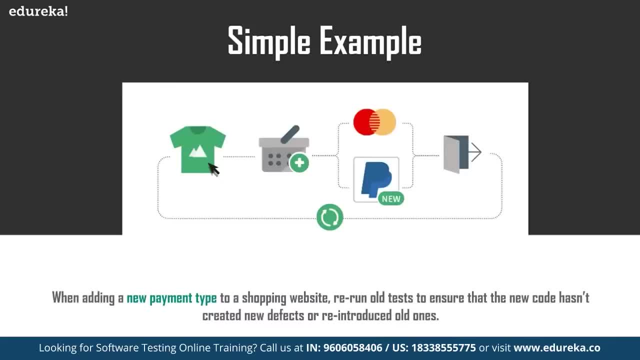 the old one in any way. If so, the box are identified and resolved. That's what regression testing is all about. So, basically, this regression testing is not just done at the beginning, It's done throughout the testing phase, and that we call regression testing cycle. 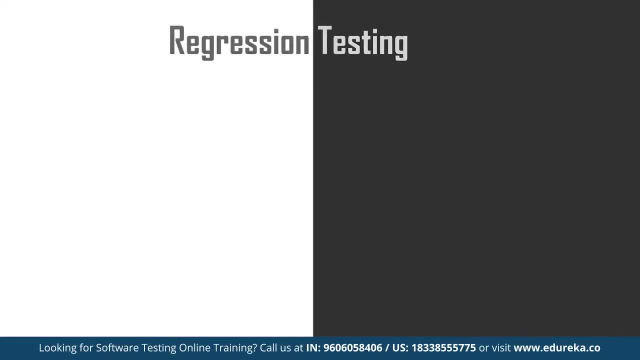 Let me show it to you guys here. it is So, as you can see, the one on the left side is the regression cycle. So you incorporate your cold into the bill and schedule the tests to find a bug, resolve it and write your regression test again based on those bugs and the fixed issues. 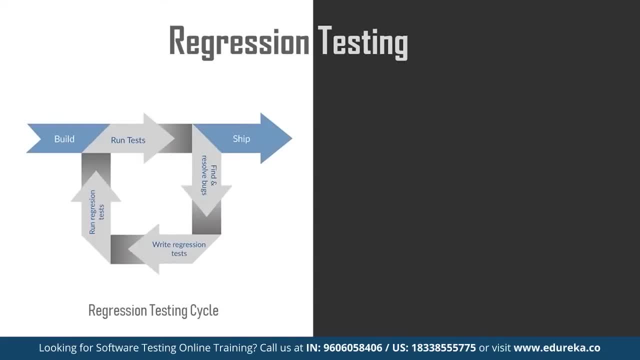 and run those regression test and the cycle goes on until you get a perfect product and then you release your product into the market. So that's what we call a regression cycle, and on the right side you have a graph which represents what regression testing is basically. 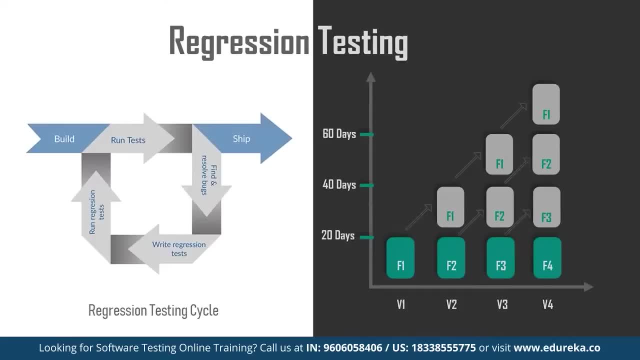 Let's say you have version one of your any software product and this is the feature one which you have enabled during the version one and that was released After 20 days of its development. and then you have version two or released to you have added new feature F2. it's working properly. 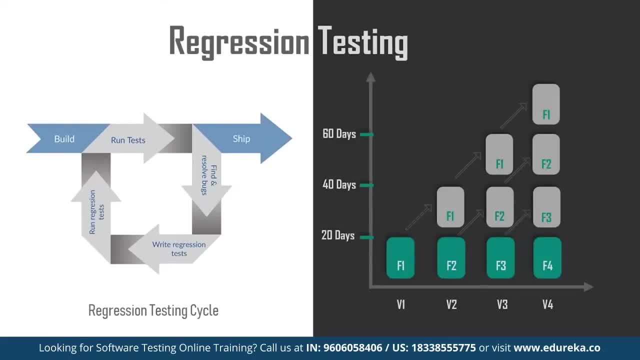 So you go ahead and check if F2 is affected, F1 in any way. That's what regression testing is all about. and your second release is released after 40 days. Similarly it goes on. next version: you add new feature. you check out if the other features. 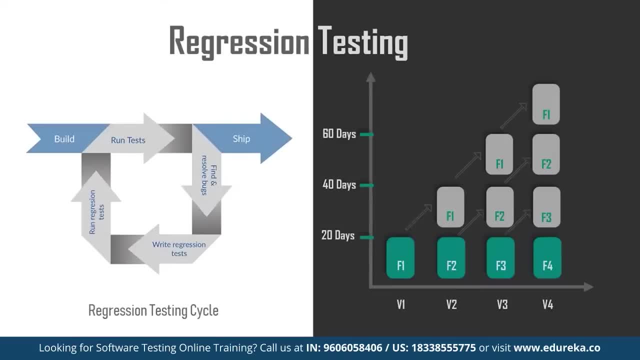 or the previous features are dependent on it If there are any errors because of the new feature. if no, then you release your product. So that's what regression testing is. So I hope, after so much explanation, you guys are clear with what regression testing is right. 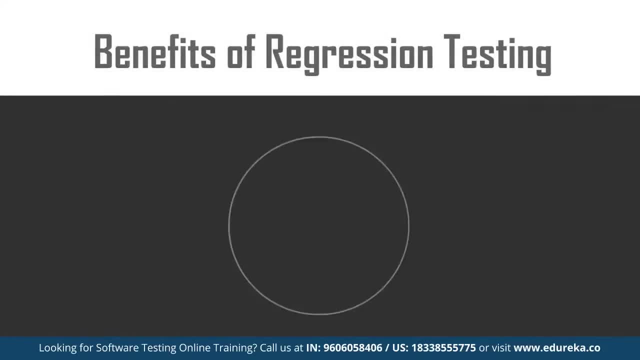 Yes, let's carry on that. Well, the basic aim behind conducting regression testing is to identify bugs that might have got developed due to changes introduced. conducting this test benefits in number of phase, such as the regression testing increases our chances of detecting bugs caused by changes. 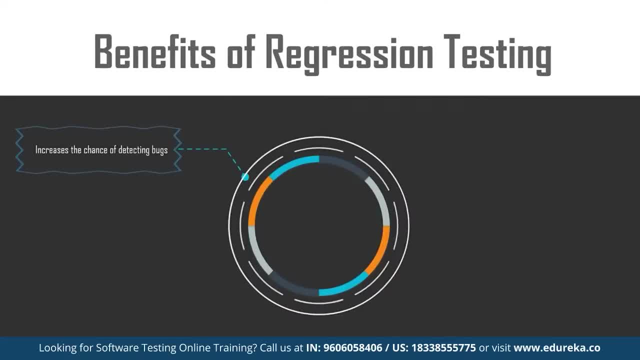 to any software or application. This changes can be anything. it could be just updates Or patch fixes or defect fixes or anything during unit and integration testing. regression testing can help catch defects early and thus the reduce the cost to resolve them. So basically it's cost-effective. it also helps. 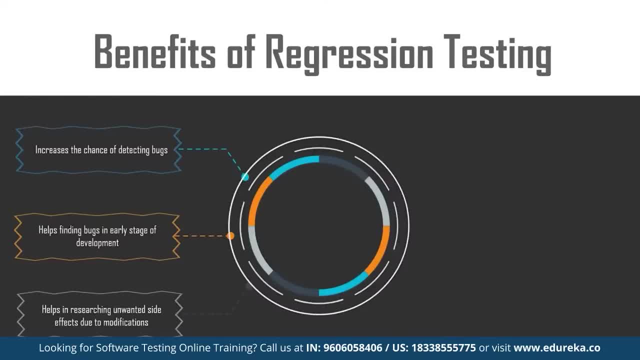 in researching unwanted side effects that might have been occurred due to new operating environment. It ensures better performance software. And why is that? because using regression testing, we can identify bugs and errors in the early stage itself. because of that, the performance your product is literally high. 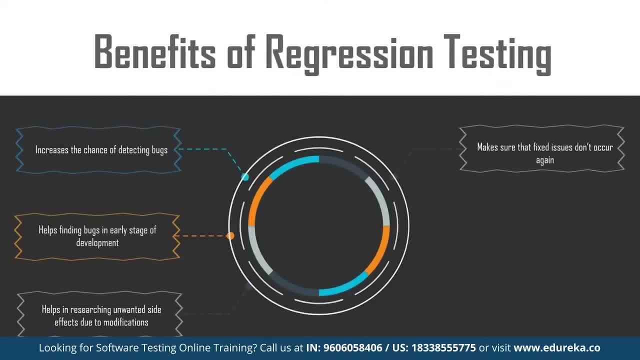 it makes sure that the issues which are already fixed do not occur again. That's one of the best thing about regression testing. Most importantly, regression testing verifies the code. changes do not introduce any old effects, improve the quality of deployed software. this way, It ensures the correctness of the program and, as a result, 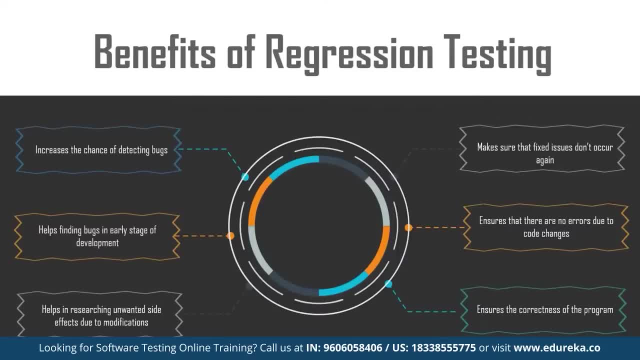 the best version of your product is released to market. So, to summarize, it reduces the amount that you have to pay on your testing. by reducing the amount of bucks and making sure that the old box don't written, it gives you the best product or the quality of product is improved. 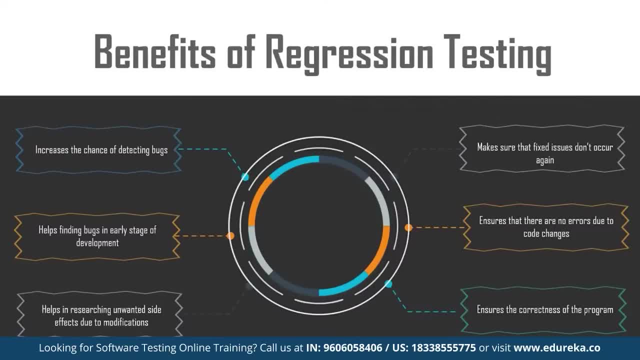 when regression testing is performed and you can actually catch the box or any kind of issues in the early stages itself. So these are some benefits of regression testing. However, in real world, designing and maintaining a near and finite set of regression test is not actually feasible. 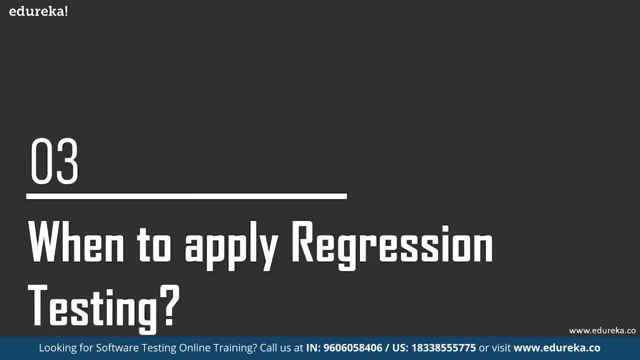 So it is important to determine when to perform regression testing and when not to. regression test are frequently executed throughout the software testing life cycle at each different level. It can be unit testing level, integration testing level, system testing level or acceptance- any level. However, it is recommended to perform regression testing. 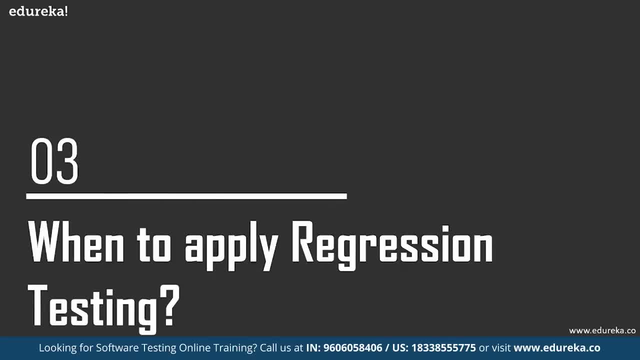 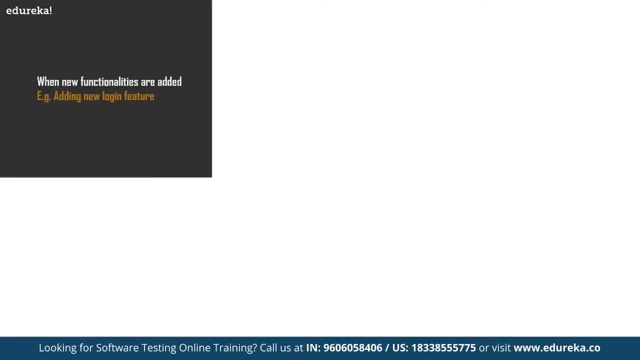 on the occurrence of following events. Let's discuss what they are. first of all, when your functionalities are added, ideally you should perform regression testing after making any changes to the code. For example, a website has a login functionality which allows users to do login only. 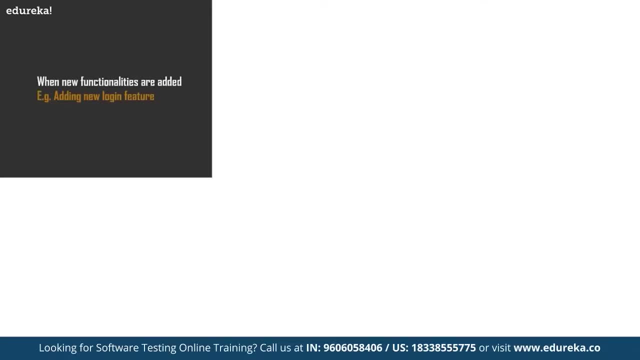 with the email. now you add a new feature like Facebook login, So you need to check the entire login functionality of the Facebook. just like the simple e-commerce website payment option which we discussed earlier, We need to make sure that the new payment option or, in this case, the new login feature, hasn't affected. 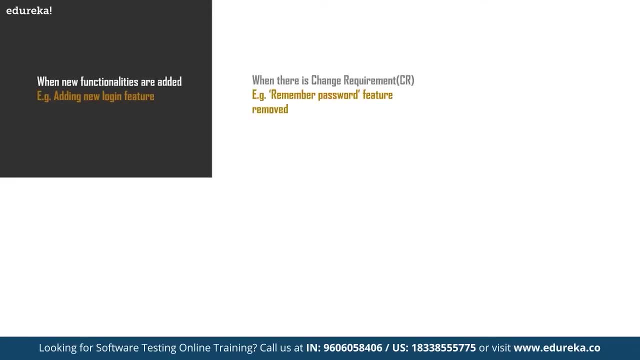 the old login functionality. Then you apply regression testing when there is change requirement, or usually you call it CR- in the market, For example, whenever you log in, does this option, which pops out, right? Do you want the system to remember your password? I'm sure you've seen that. 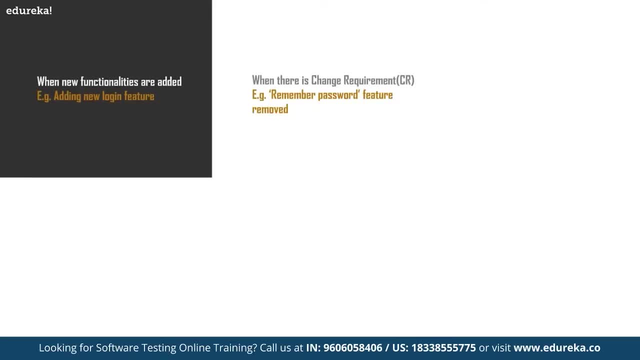 So remember, password should be removed from login page, which was available earlier. That's change requirement. It was available earlier but you want to remove it. That's when you can apply regression testing to see if the removal of thing is affected. the website. 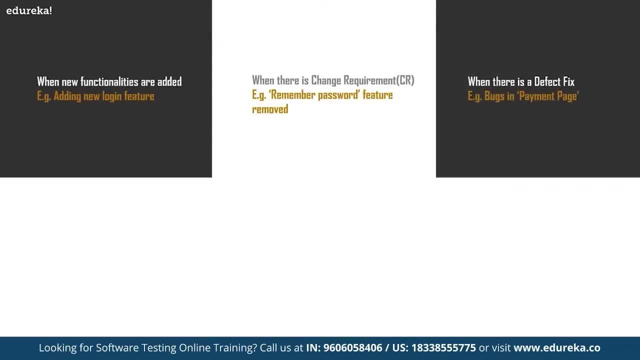 that you're using in any way and then you can apply regression testing when there is defect. fix that straightforward. You already know that. imagine: login button is not working in login page and a tester reports a bug stating that the login button is actually broken. So once the bug is fixed by the developers, tester test it. 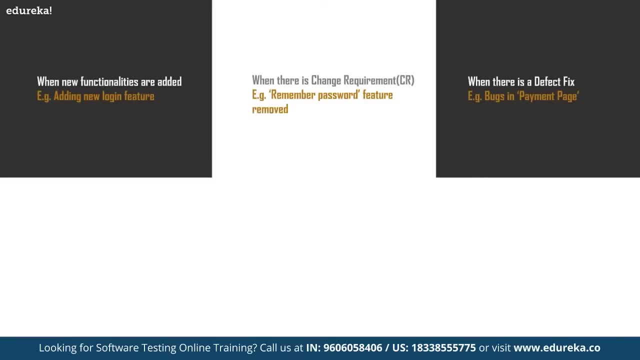 to make sure whether the login button is working as per expected results or not. simultaneously tester test under the functionalities which are related to login button and like registration or any other features which are directly related to login functionality, and then you can apply regression testing when there is performance issue fix, for example. 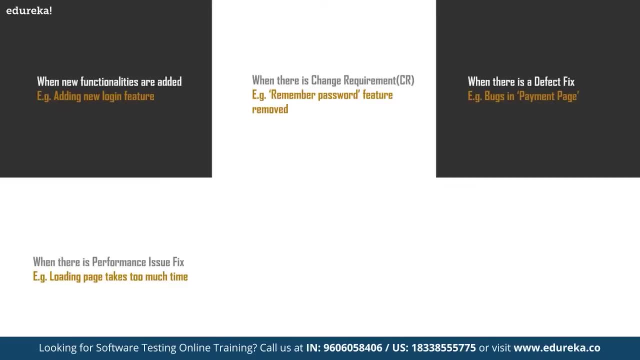 when there's modification of code based on your needs and requirements. you've made some changes to the code and since then, the loading home page, which takes 5 seconds. you want to reduce the load time to 2 seconds and you have done it, but you want to see if this has affected the functionality. 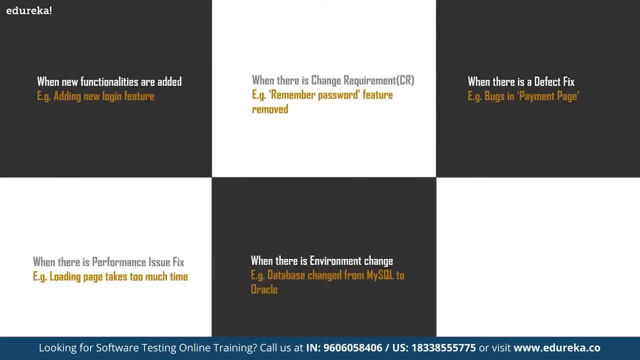 of your website in any other way. You can also apply regression testing. when there's an environment change, for example, when you've updated the database from mysql to Oracle, all the features which are dependent on your database should be tested. and, lastly, you can apply regression testing. 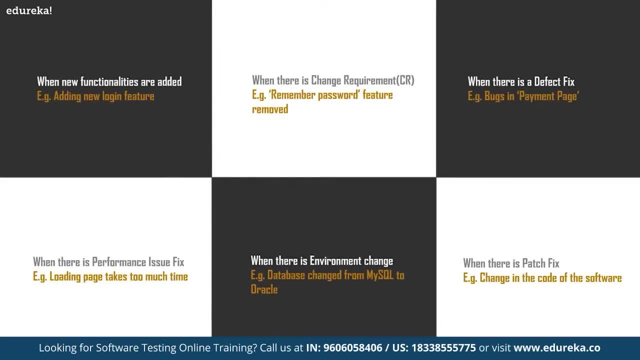 when there's a patch fix all the mental fix problems. poorly designed patches can sometimes introduce new problems, Like they can break the functionality or disable a device. So in such cases you need to perform regression testing to see if fixing a patch has actually been a profit for you or loss. 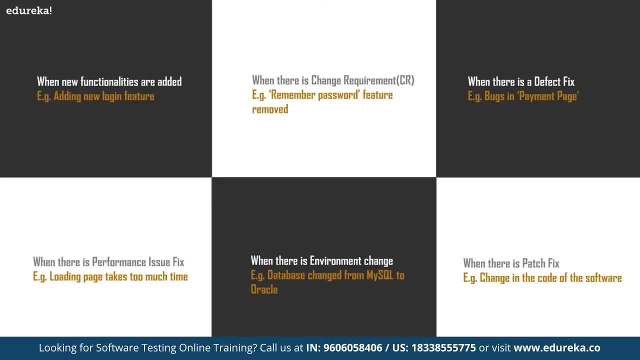 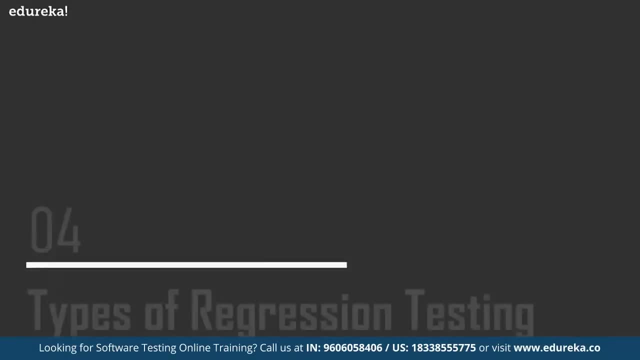 So, guys, these are some test cases, or, you can say, situations or scenarios where you can apply regression testing and that would be beneficial for you. So, guys, often regression testing is done through several phases of testing. It is for this very reason that there are several types of regression testing out there. 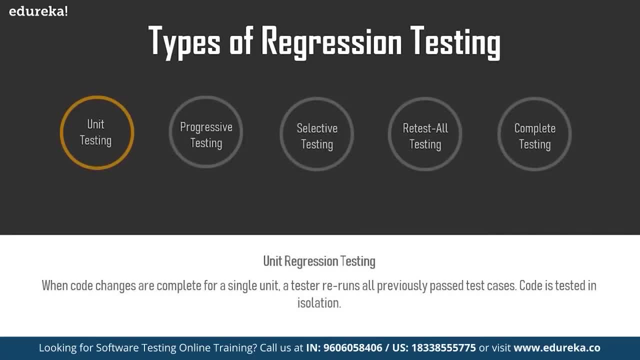 Let's check out what they are. to begin with, we have unit testing. So immediately after coding changes are made for a single unit, a tester- usually the developer who is responsible for the code- reruns all the previously passed unit tests, So test driven development, which we call it TDD. 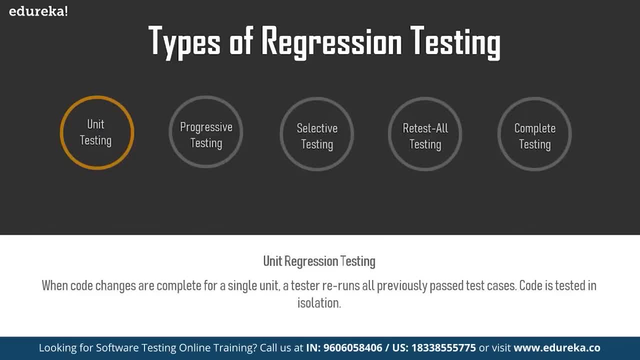 and in continuous development environments. automated unit tests are built into the code, making unit regression testing very efficient when compared to other types of testing. That's what you need testing is. then you have progressive testing. So progressive testing works efficiently when there are changes done in software. 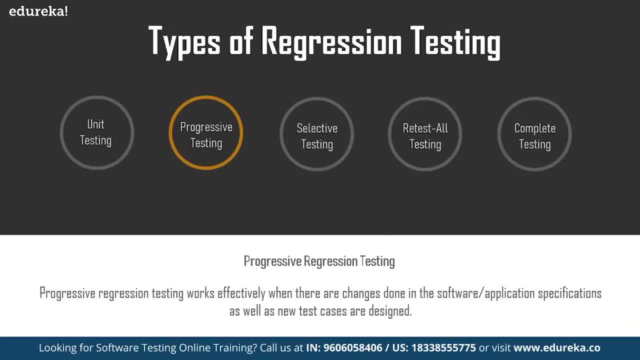 or application specifications, as well as new test cases are designed. That's when you use progression testing, and it will be more helpful for you as well. Then there is selective testing. in selective testing, testers use a subset of current test cases to cut down the cost and effort. 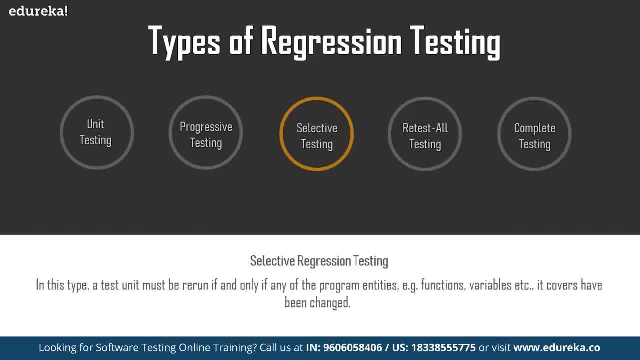 So in this strategy a test unit must be rerun if, and only if, the program entities, example, functionalities, variables, Etc. It covers, have been changed. So basically only things like functionalities, variables which are under the unit test are changed. only then you should perform testing on that unit test. 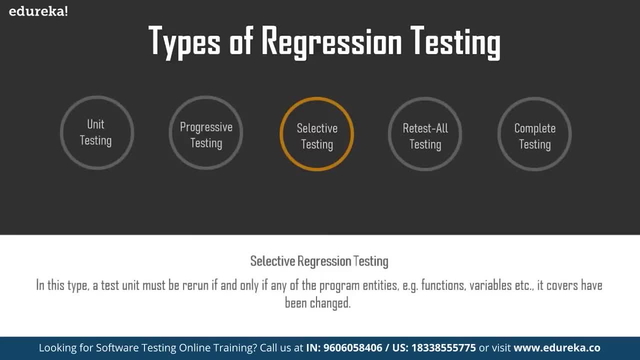 The challenge is basically to identify the dependencies between the test case and the program entities it covers. So basically, as the name indicates, you do not perform test in all units. You just select few out of those which might have affected due to change and then test those units. 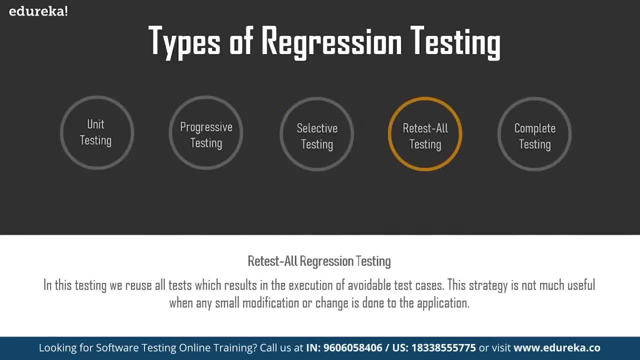 That's what you call selective testing, and then you have reset all testing. reset All testing is very time-taking because in this testing we use all the tests. This strategy is not much useful when you have small modifications or small kind of changes which are done to your code in the application. 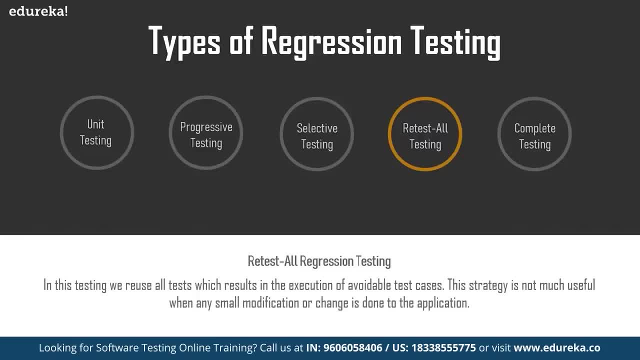 You can straight away point out: right, You have made a very small change and you are trying to retest everything because of the small change. It's literally costly and it takes a lot of effort and time on your part during small modifications or changes to your code in your application. 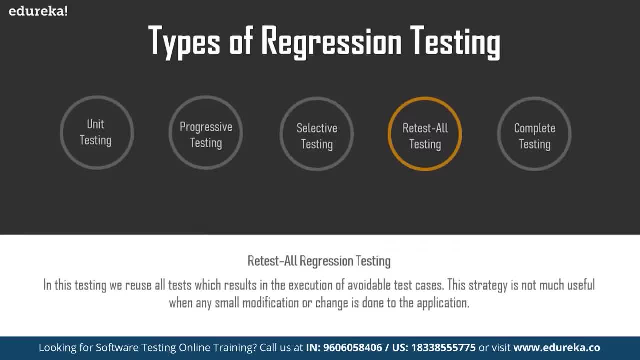 It's not effective. retest All strategy involves testing of all aspects of a particular application, as well as reusing all test cases even where the changes have not been made, So that's one of the most costliest type of testing when compared to others. 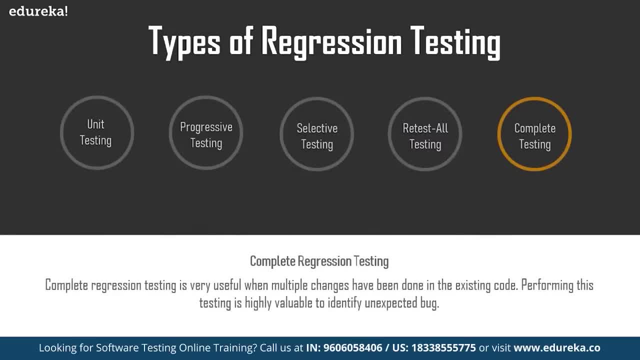 Lastly, we have something called complete testing. Don't confuse it with retest. all testing Sometimes people often refer to is both of them as the same thing? But anyway, complete regression testing is very useful when multiple changes have been made in the existing code. 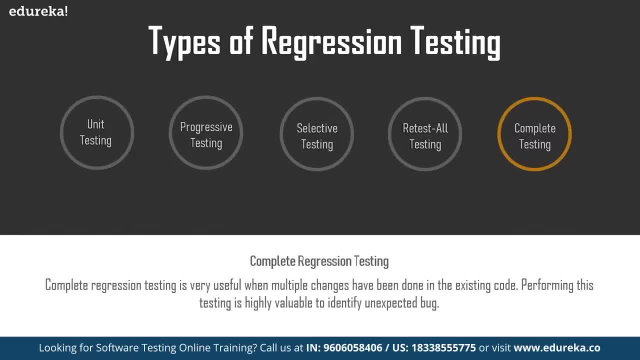 performing this testing is highly valuable to identify unexpected bugs, actually. So once the testing is completed, the final system can be made available to the user. So, guys, it is important to make sure the type of regression testing that needs to be conducted, So we should choose the one. 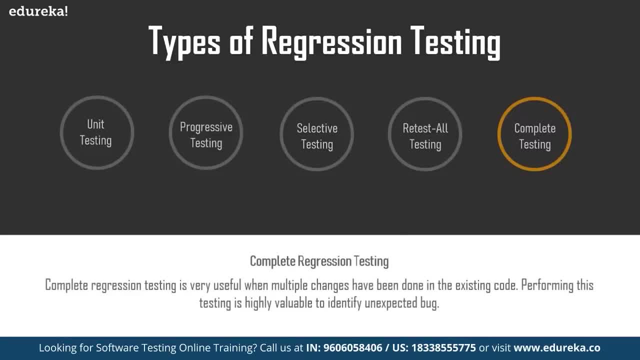 which suits your requirement properly, and how you choose, or which one you choose, totally depends on other factors such as recurrent defects, criticality of the features, Etc. But what remains on the priorities: ensuring that the software delivers the best functionality and proves to be beneficial addition. 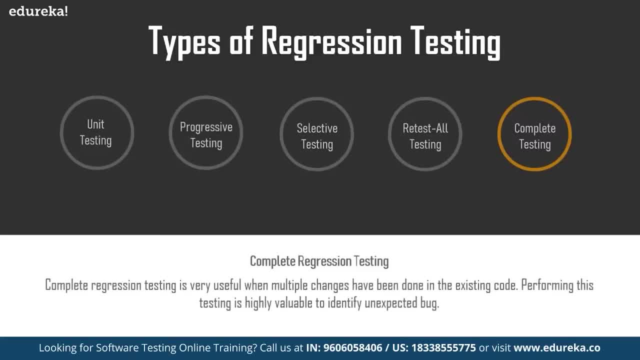 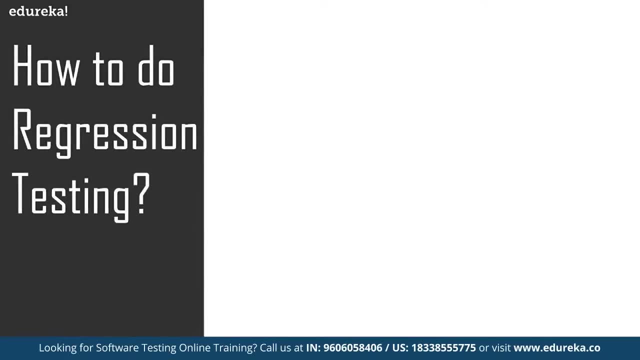 to your company or industry. So, guys, now that we have established what regression testing means, let's go ahead and check out how regression testing is actually performed. So, every time the software undergoes a change and the new version, update or release comes up, the developer 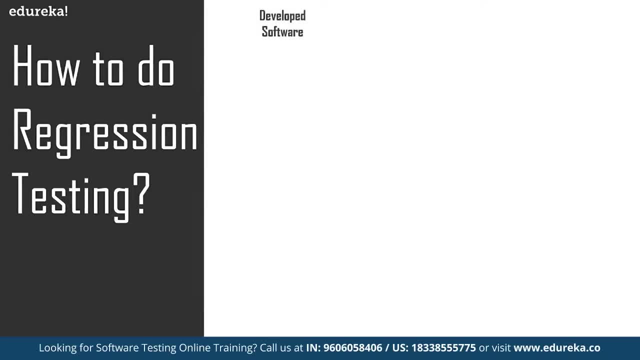 carries out these steps as a part of regression testing process. The first thing it does is developer execute unit level regression test to validate the code that they have modified, along with any new test that they have written to cover new or the change functionality. basically, whatever the changes there, made the check. 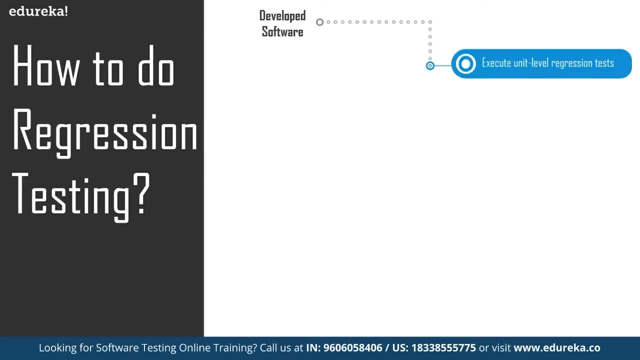 if the changes are working properly or not. So that's the first step. we did learn what unit level regression test are earlier right. So any code changes made for a single unit, a tester or basically the developer who's responsible for the code, reruns all the previously passed units as well. 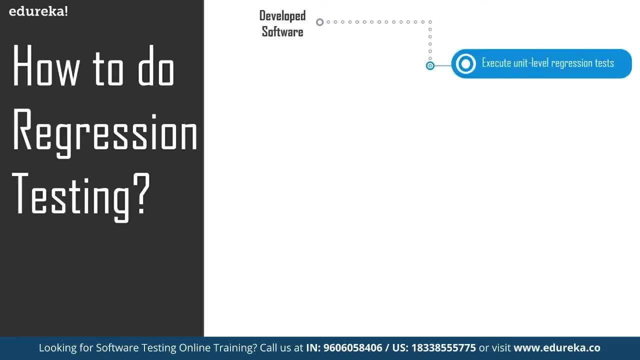 So that's what unit level regression is. once that is done, The changed code is merged and integrated to create a new build of application under test, after that smoke test are performed. These smoke tests are executed for assurance that the build which you have created in the previous step is good. 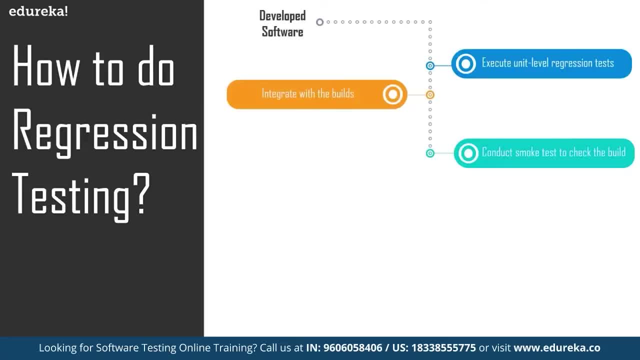 before any additional testing is performed. These tests may be automated and can be executed automatically, but continuous integration services such as Jenkins, Hudson's and bamboo. So, once the build is perfect, sanity testing confirms that new functionality works as expected and known defects are resolved before any other conducting. 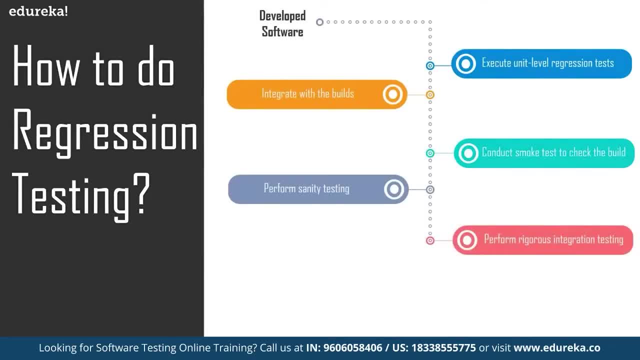 or rigorous integration testing is actually performed. So why do you perform this integration testing? to verify that the interaction between the units of application with each other and with the back-end services, such as databases, is working properly or not. for that you perform integration testing. The next step is to schedule your regression test. 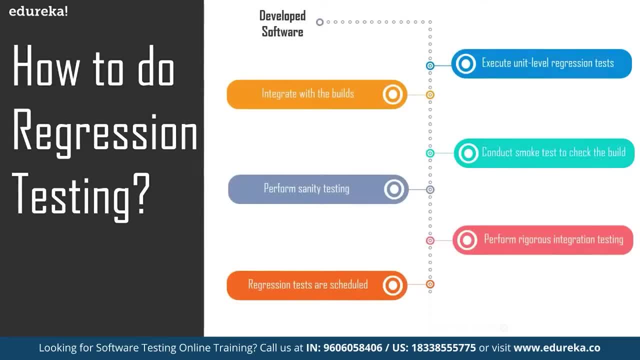 So, depending on the size and the scope of the released code, either a partial or a full regression test may take place. defects are reported back to the development team and many require additional rounds of regression testing to confirm the resolution. So, lastly, based on the reports that you've written, you analyze: 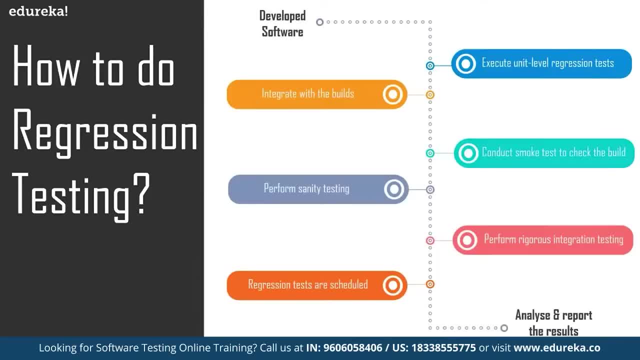 and figure out what taste cases should be added for the next checking process as well, and you create a report on that. So that's how you perform a regression testing. So, like you've seen, it's similar to any other testing. It's just that you check the functionality. 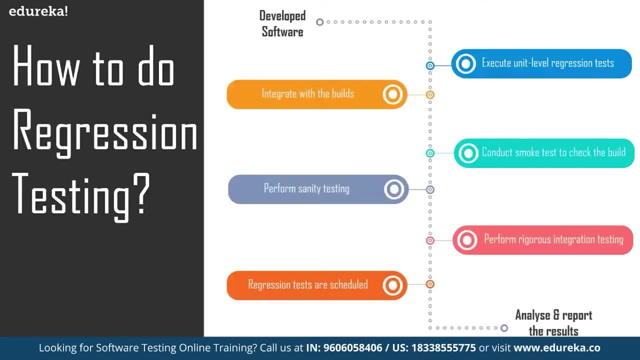 of your developed software whenever there is an update or some new release. So basically, on introduction of new feature, You check out if the previous features are working or not. So remember, guys, regression testing is not just performed in the beginning, So basically it's carried out throughout the testing process. 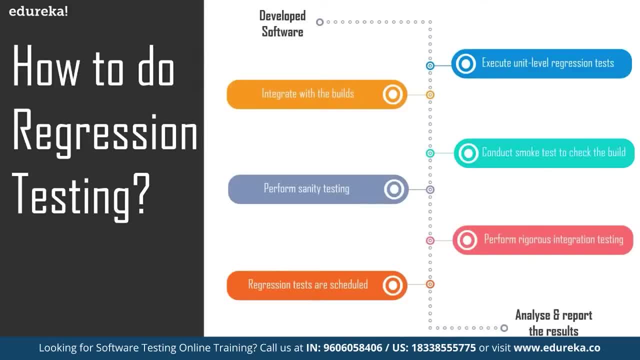 whenever a new feature is added and we discuss when to perform regression testing earlier right. So whenever one of such cases occur, we perform regression testing during the entire testing phase. So basically what you're doing here: you select the test for regression, choose a proper tool. 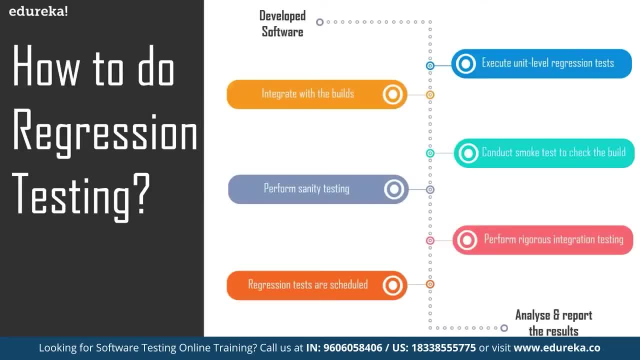 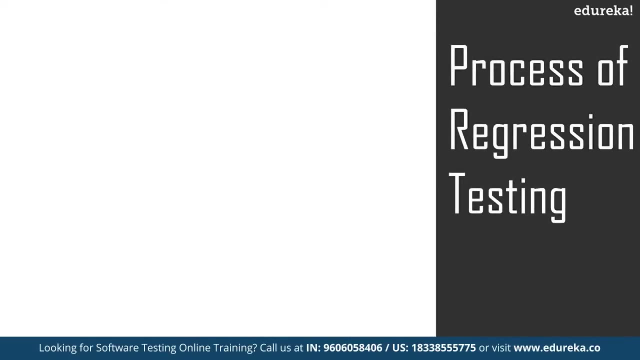 and automate the regression test, verify your application with checkpoints, manage the regression test or update when required. you schedule the test, integrate the build and analyze the result. So that's as simple as that. if that was a little theoretical and if you've not understood, here is a pictorial representation. 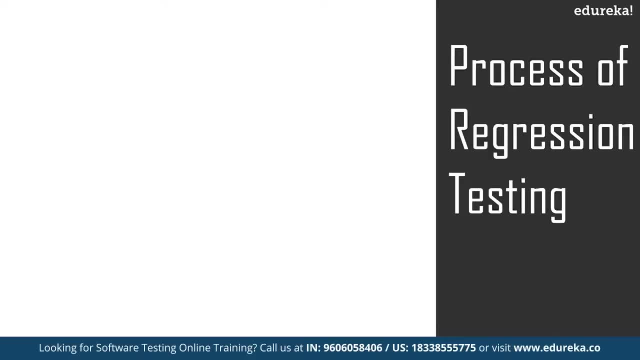 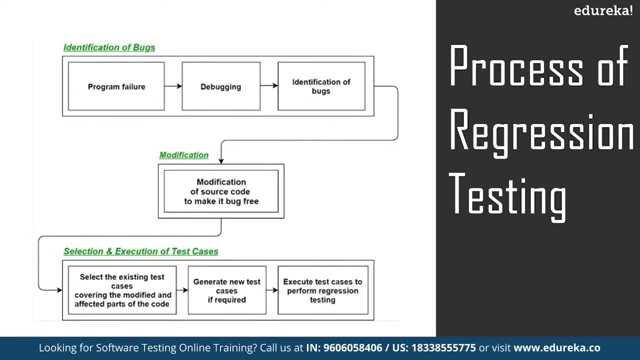 of it. So, first of all, whenever we make some changes to the code for any reasons, like adding new functionality, optimization etc. our program, when executed, fails in the previously designed test suit for obvious reasons. So after the failure, the source code is debug in order to identify the box in the program. 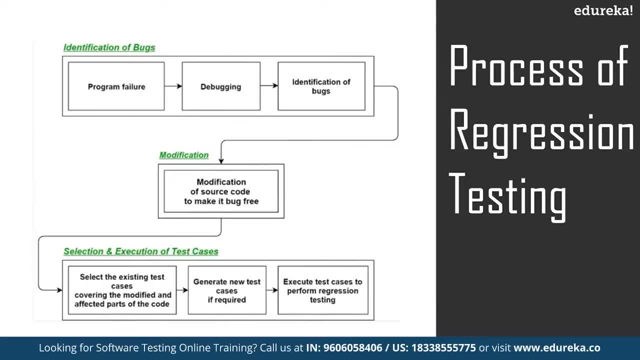 after identification of box in the source code, appropriate modifications are made. then the appropriate test cases are selected from the already existing test suit, which covers all the modified infected parts of the source code. So we can add new test cases if required. in the end, regression testing is performed using the selected test cases. 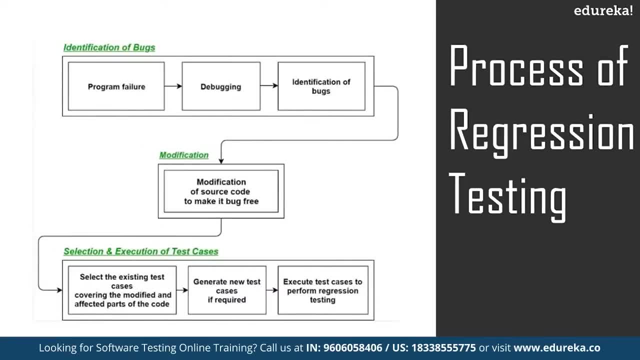 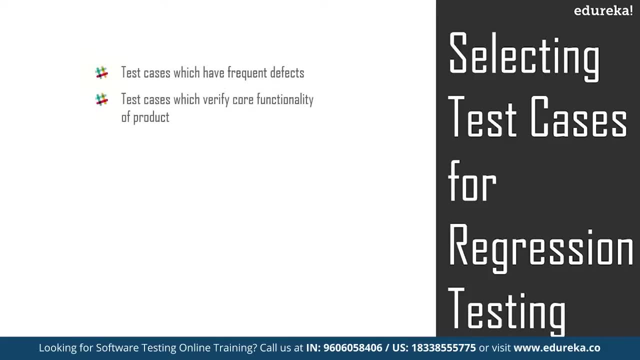 So selecting test cases is very important. effective regression test can be done by selecting the following test cases: test cases which have frequent effects. test cases which verify core functionality of the product that you're checking. the complex test cases. integration test cases. You have functionalities which are frequently used. 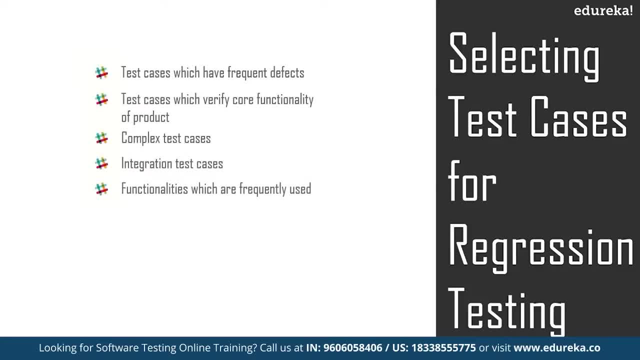 So those are the first ones that you should check out. then you have test cases which cover the module where the changes have been made. those are obvious. then test cases which frequently fail for no reason. then you have boundary value test cases. So these are certain test cases. 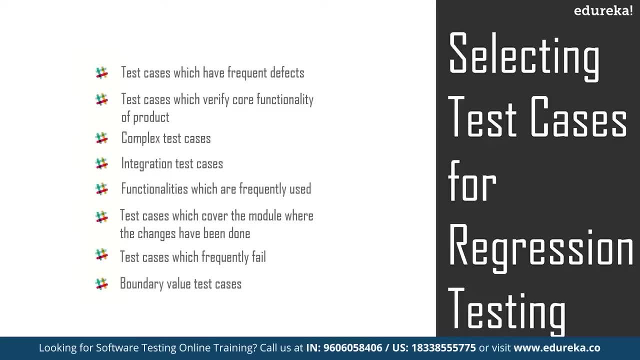 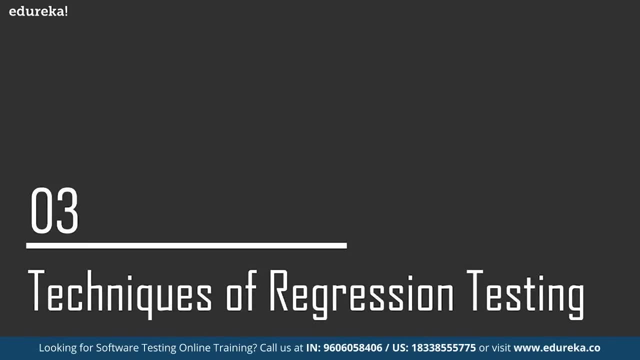 where you can apply regression testing or you can actually select these test cases for regression testing. So when you're trying to shortlist the test cases for regression testing, these are some points that you should consider. So regression testing simply confirms that modified software hasn't unintentionally changed. 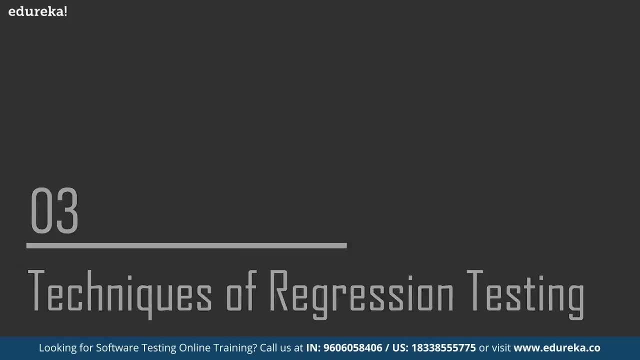 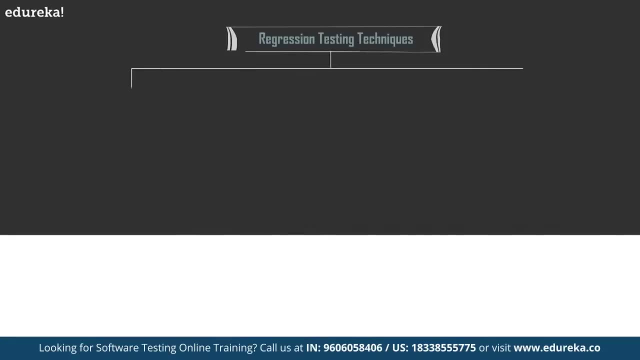 and it's typically performed using any combination of following techniques. So, basically, what I'm trying to say here is that there are three techniques that you can apply for regression testing. So the first type we have is retest. all this method of regression testing, simply retest the entire software suit. 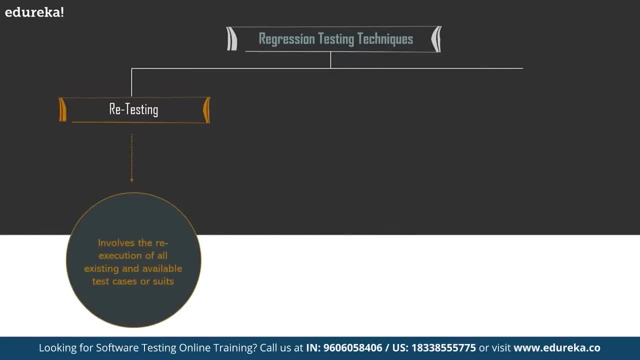 from top to bottom. in many cases, The majority of these tests are performed by automated tools and certain times automation is not necessary at all. More of all, purely using automation ignores the benefits of human testers and any change for exploratory testing. So this retest, all type of technique, is an expensive method. 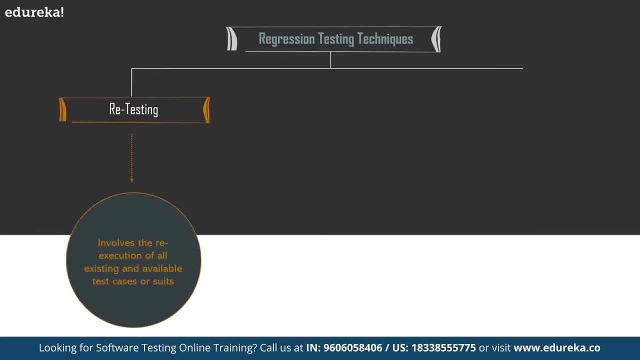 as it requires more time and resources when compared to other techniques. Well, it's all there in the name itself, right? retesting. The next is selective test cases- again from the name itself, You can guess what that is- rather than a full retest process. 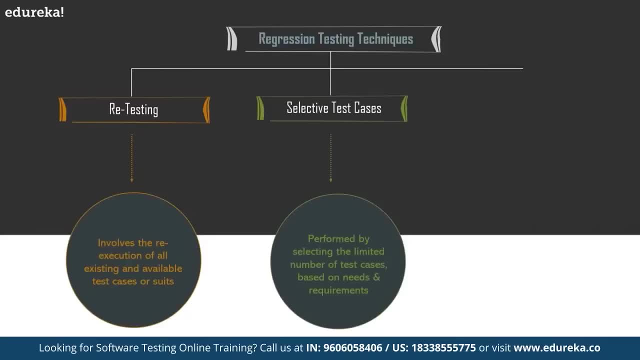 This method allows the team to choose a representative selection of tests that will approximate a full testing of a suit. The primary advantages to this practice is that it requires far less time and effort when compared to retest all method, So these kind of regression testing is usually performed. 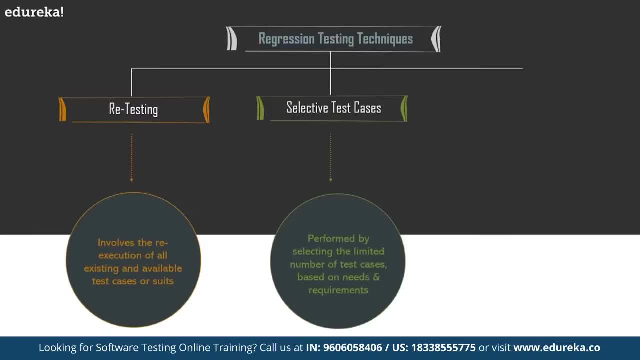 by human testers, such as quality analyst team or development teams, who will typically have better insights into the working of test cases and their unexpected behaviors. And lastly, we have test case prioritization. This is one of the popular technique. The goal here is to prioritize a limited set of test cases. 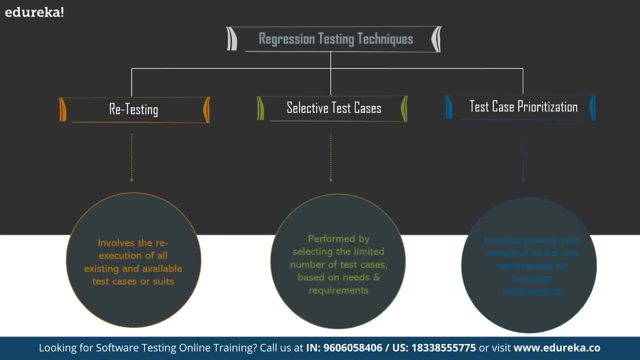 such that more potentially impactful tests are executed ahead of all less critical ones. So try to prioritize test cases which should impact both current and future bills of your software. that way, you're not wasting your time, money and effort. apart from these three, We have another one called hybrid: hybrid technique. 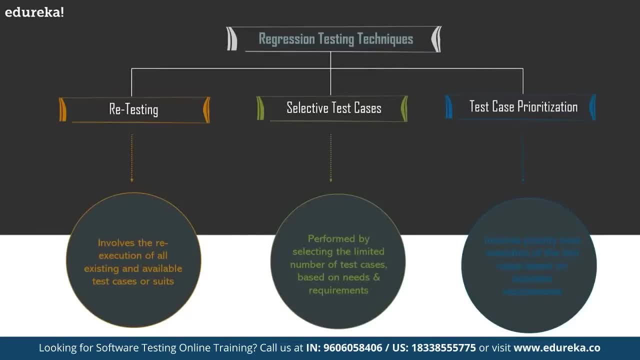 is literally a combination of regression, test selection and test case prioritization. So, rather than selecting the entire test suit, select only test cases which are executed or re-executed depending on their priority. So what are the different techniques we have? retesting, where you perform testing on the entire test cases that there are. 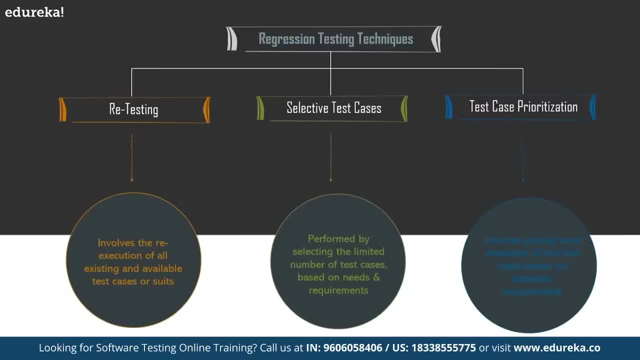 then you have selective test cases based on certain criteria. You select the few test cases. then you have prioritization: you select the more impactful test cases compared to less critical ones. And lastly, the hybrid, which is combination of selective and prioritization. So these are various ways. 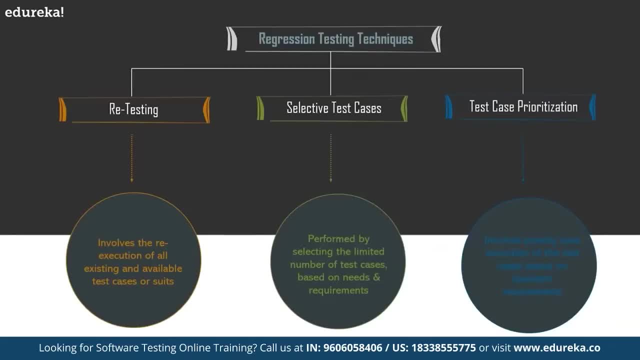 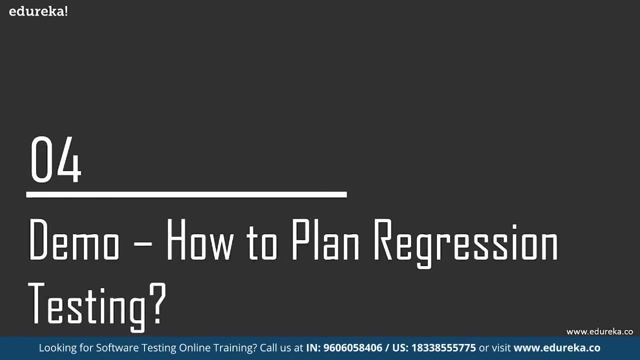 of implementing regression testing. guys, now that we know what regression testing is, its types and its techniques, Let's go ahead and do a demo on how to create a regression testing plan. for that I'll be using an excel sheet. So, guys, here we are in this demo. 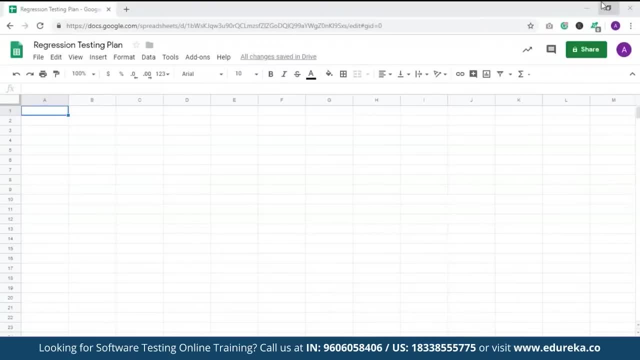 Our main goal is to actually learn how to create a regression testing plan. It's a very simple example, So with this example, I'm sure you'll be able to get started on how to perform regression testing. So, first thing, there are certain terms that you should know about, as 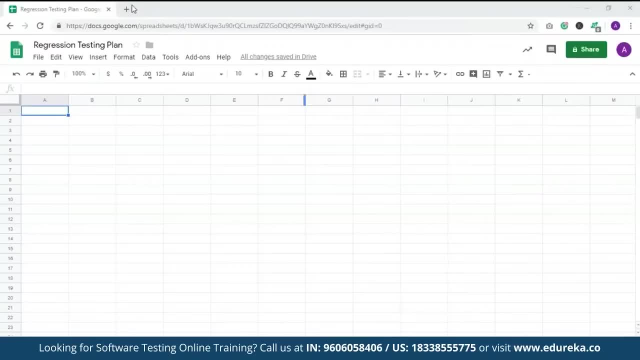 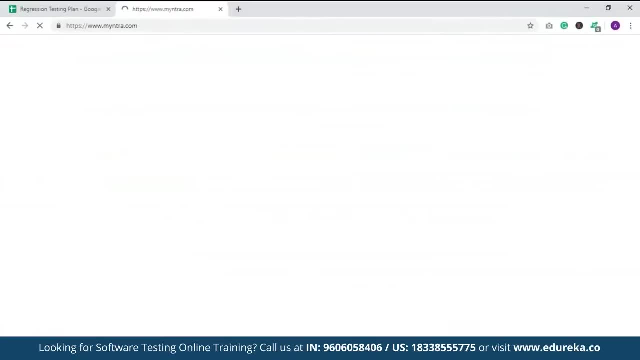 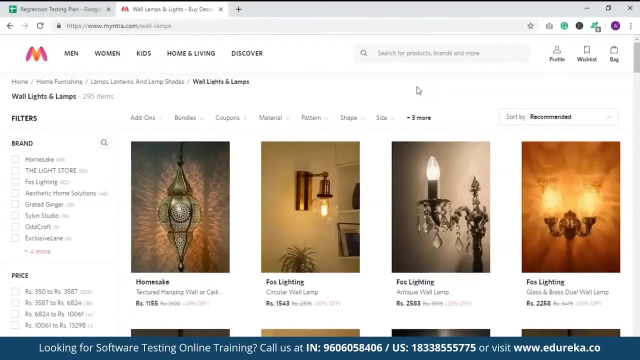 for this regression testing plan will be using an e-commerce website to test on or to create a plan actually. So let's take mantra, Here we go. Okay, what do I want to see? So we go. I'm choosing wall lamps and lights, anything just. 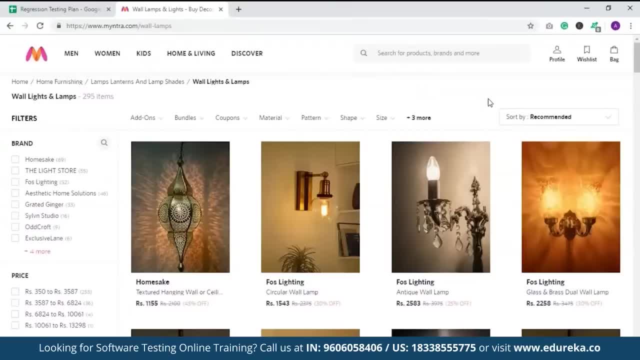 and basic example to check on. let's perform or create a regression testing plan for the sort option. here You can see right the sort here. when you click on that you have different options like sort the elements based on what's new, popularity, better discount price. high to low price. 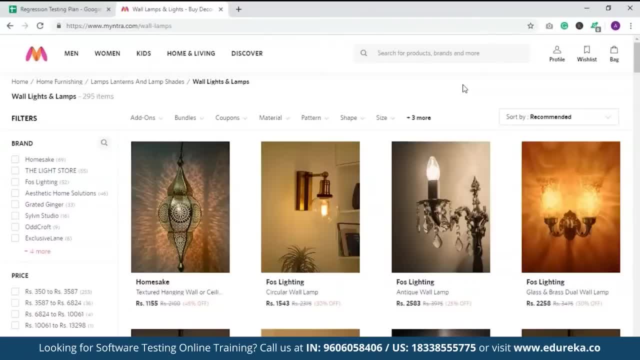 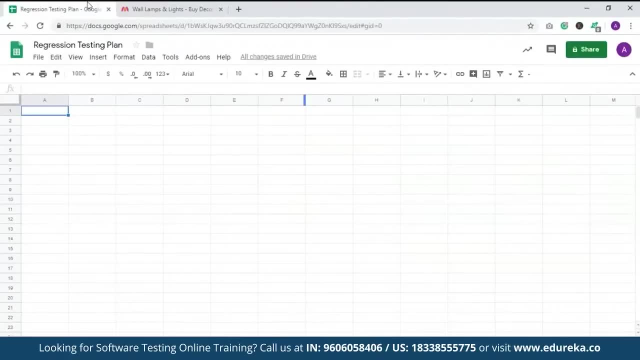 low to high and faster delivery. So we'll be creating a regression testing plan on that. Let's go back to our Excel sheet. Like I said earlier, there are certain words or terms that you should be aware of. the first thing, Let me just write the headings first. 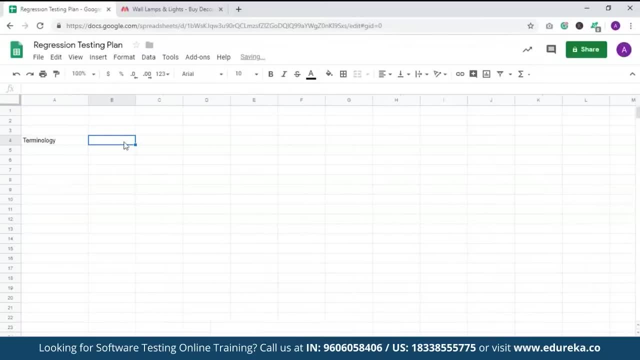 Let me increase the size. then we have what they mean. And then comes our example. Okay, let me increase the size of this one as well. Okay, first terminology is test objective. So what does a test objective mean? It's basically what you're trying to do here in this. 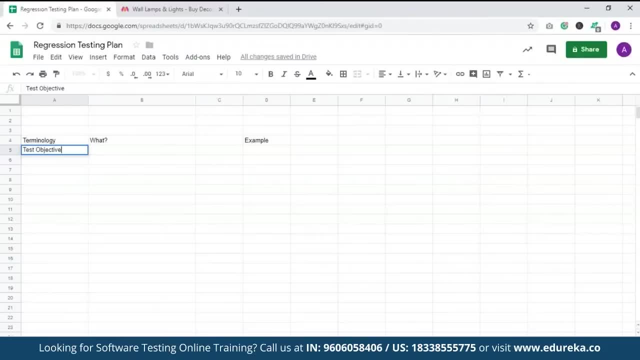 you're trying to test a functionality of your feature. That's what your objective, the goal or the objective of creating this plan. That's what we call test objective, So you can say what you are Planning to do. So what would be the example here with trying? 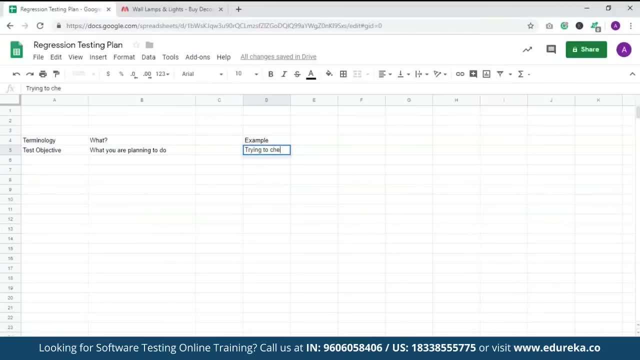 to check the functionality of a feature. here trying to check a, check the functionality, The next term is test object. So what do you mean by test object? It's basically the component which you're perfect test on, but performing test on, so component to be tested. 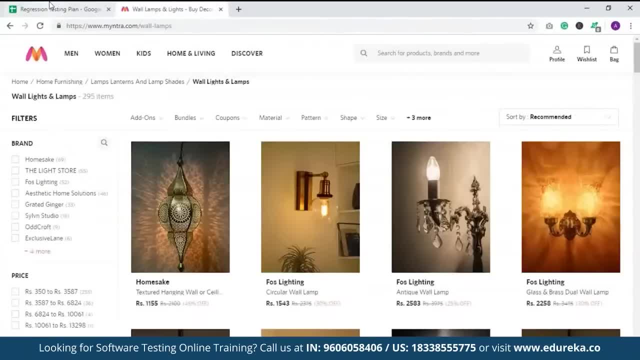 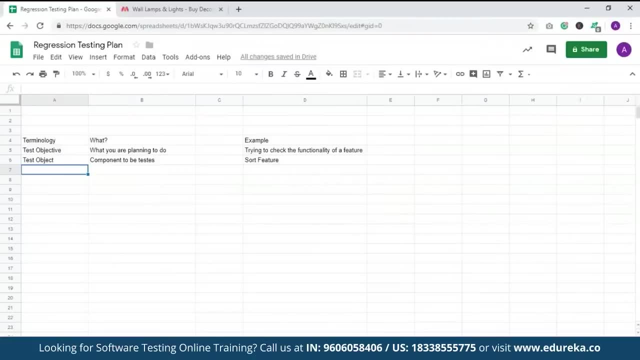 So what's the component that we're trying to test here, The sort components. So that's our test object. So I'm going to say sort feature. So we are done with test object and test objective. We have something called test item next. 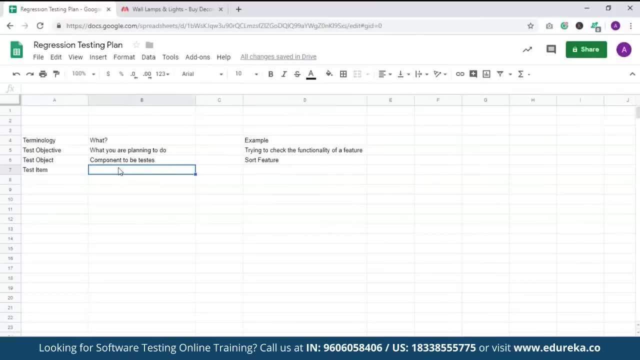 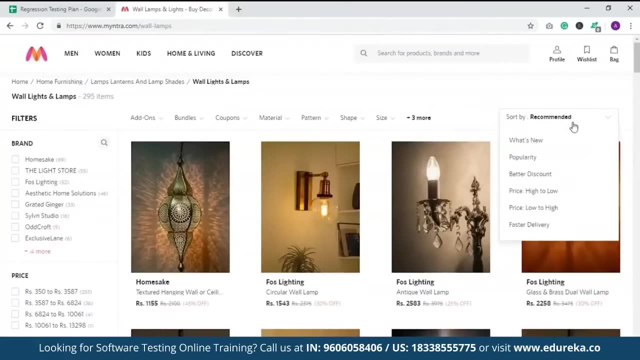 So what's in test item? This item is the subset of your test object or the item that you're performing test on. So this is the object that you're performing test on, which is sort. like I said, under sort We have multiple options. 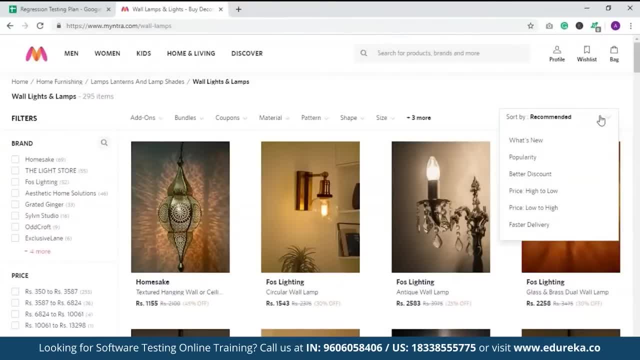 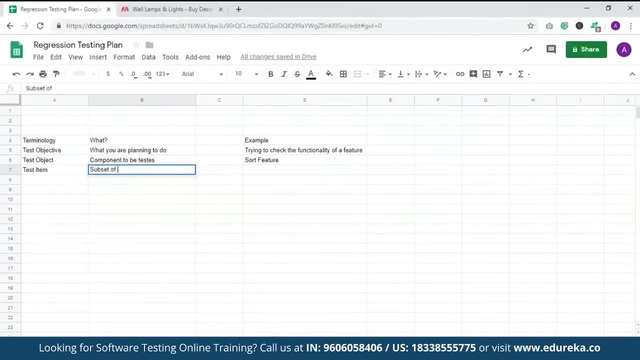 So these are nothing but test items here. So let's say, let's perform a test on this price high to low, So let me write it as sub set of test object. So what are the item that we are checking here on price from high to low. the next thing is test condition. 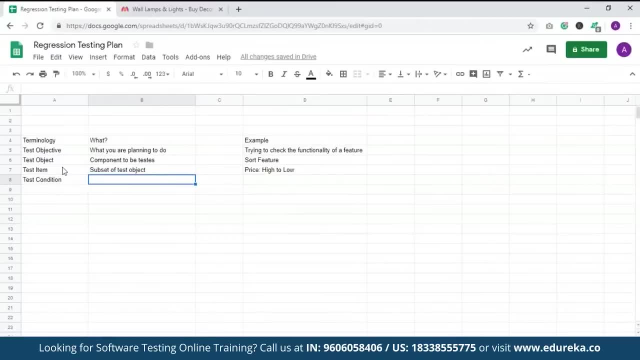 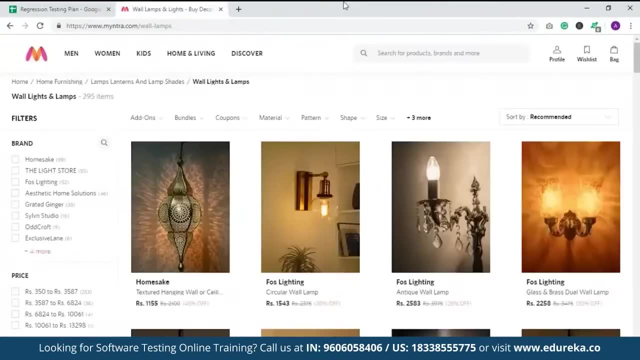 So under test items, like I said, it's a subset right. you can have any number of items or the subsects for an object, For example. like we said here, we have what's new popularity and also, let's say, if I want to select two options or two objects or items, 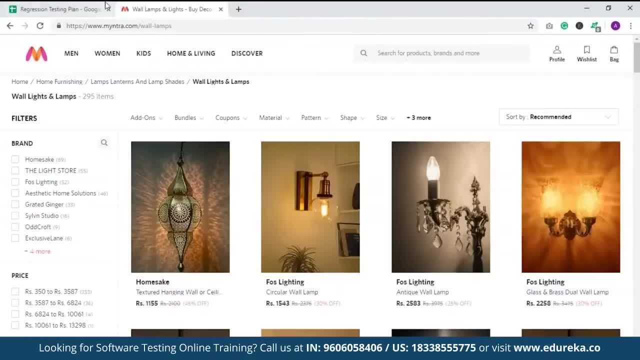 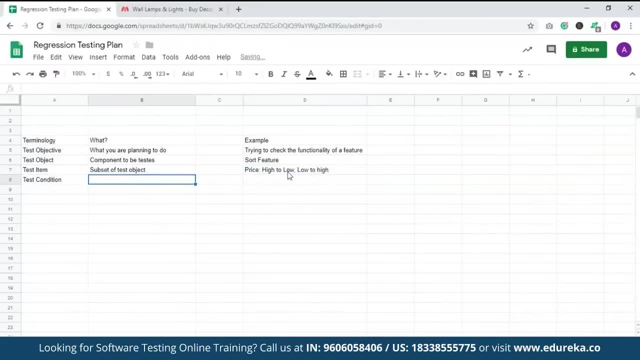 that I want to check here, which is price high to low and price low to high. I can add both of them here, high to low comma, low to high. So the test condition is the one thing which we're testing of these items. So let's say we want to check the sorting feature by price. 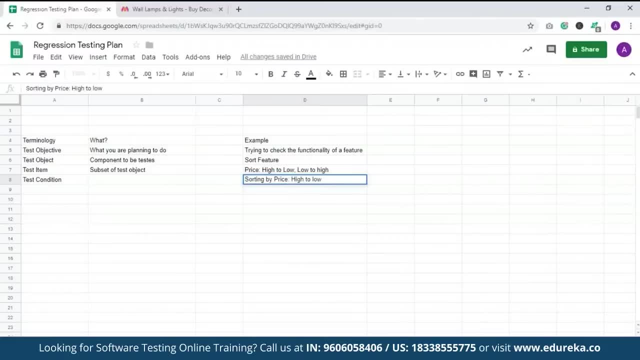 Hi to low. So you get the point right, basically the condition on which to performing testing, and then you have this case. This case are just parameters that you can relate to when you're actually performing testings. For example, you have test data that you're checking on. 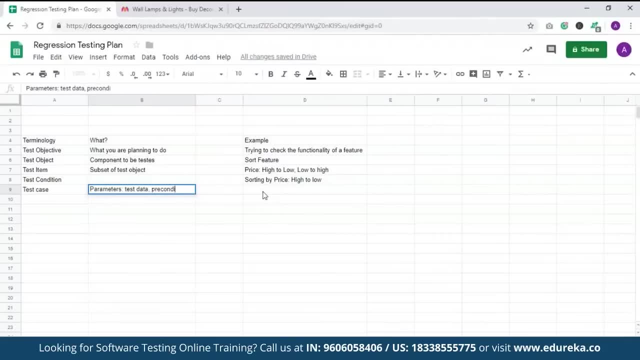 then you have preconditions. if you do have any, or you can say assumptions, and then you have expected results, actual results of testing and all that. so, guys, if you want to know more about his cases, there's separate Video by a director on test case. 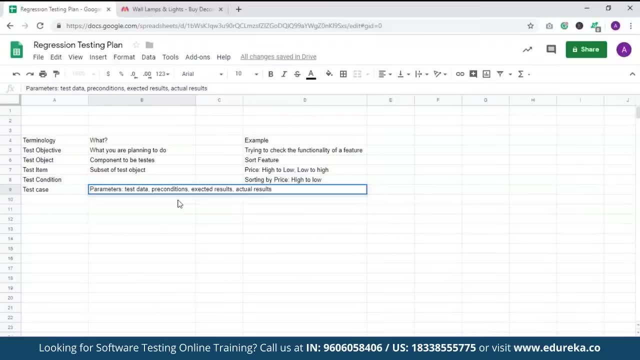 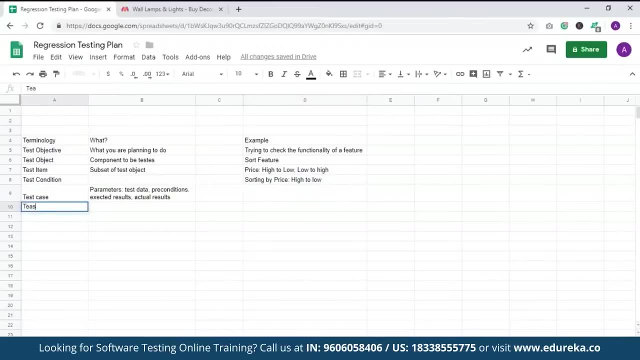 It's in the software testing YouTube playlist. go ahead and refer to that. So yeah, I don't have to give you an example, right? So I'm just leaving it blank. And lastly, you have to suit This with: is nothing but a combination or collection of test results. 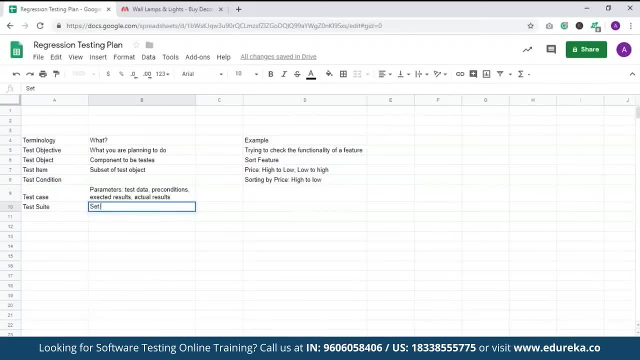 that come under test suit so I can write it as set of test cases. So these are certain terms which you should be aware of when performing a testing or writing a test case, or when you're creating a regression testing plan or anything. So the first thing is: test objective is your goal. 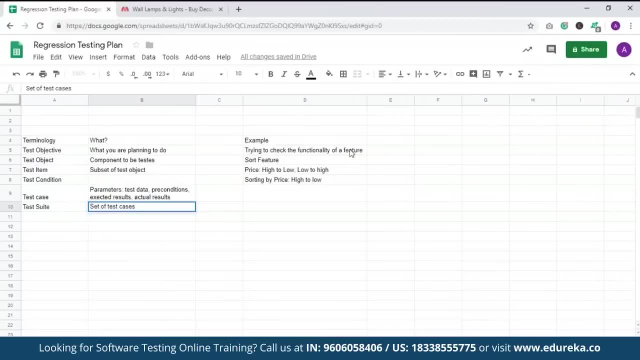 or think what you want to do. For example, you have you're trying to check the functionality of a feature. then you have something called object or the feature on which you performing test. on sort feature and the soft object, You have multiple options. those come under your test item. 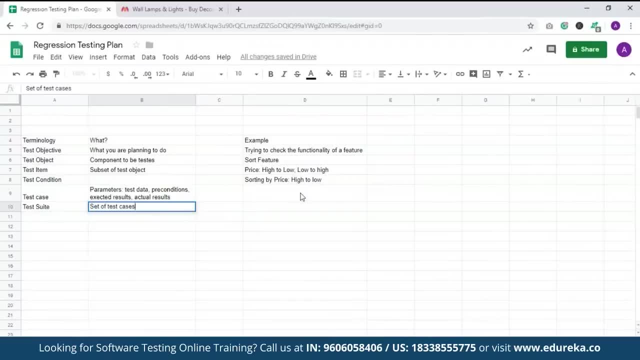 and the test condition is based on what condition you're trying to check your test object under which a test item comes. So basically we're trying to test out the sort feature based on price and high to low. So in test condition you have three things. you have your test objects. 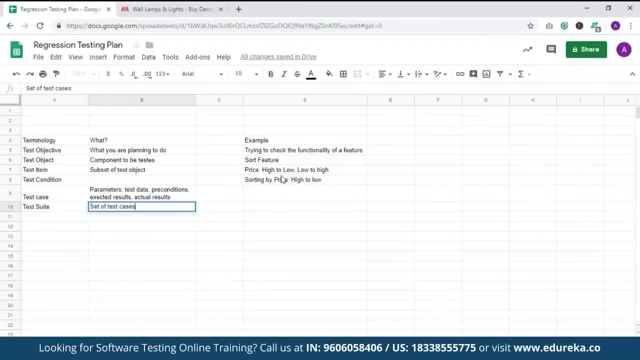 which is sorting by the item, which is price, and an item which is high to low, and then you have test cases. These are like certain parameters which are associated when you're performing a test, like test data preconditions, If you have any expected results, actual results, 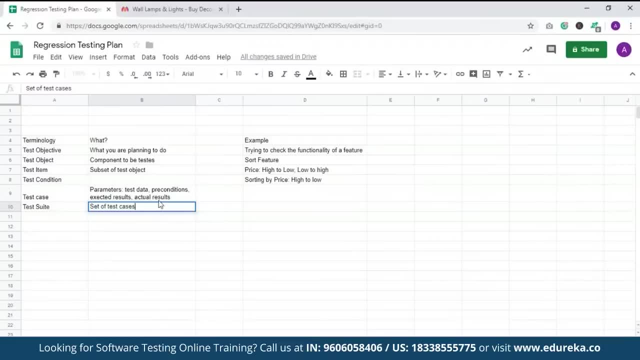 or any other comments, status and all that comes on your test cases. And lastly, you have something called set of test suit, which is set of test cases which come under the same category. you can say: So what are we trying to test your testing. 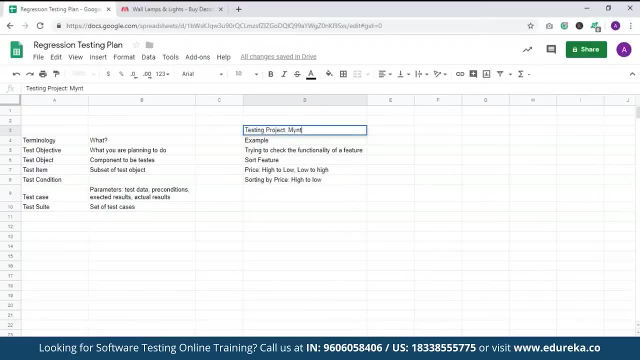 project name. Let's give it a name which is Myntra, release one. Let's say so for this first release. one: let's write something called traceability matrix. This traceability matrix basically helps you keep track of how you performing testing on and what. 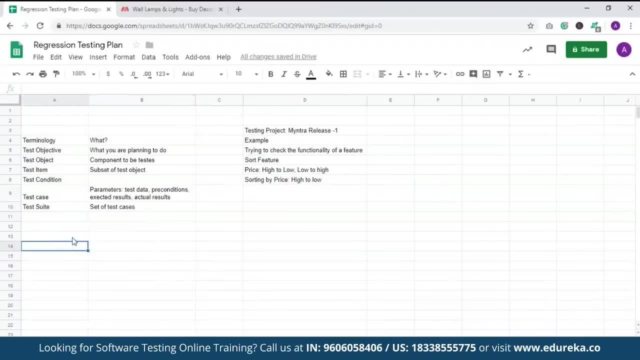 and what are the results? So here we have traceably matrix, Let's say for release one leac, release one Traceability matrix. the first one is feature, or you can just call it test item, Then you have requirement ID, Then the test suite. 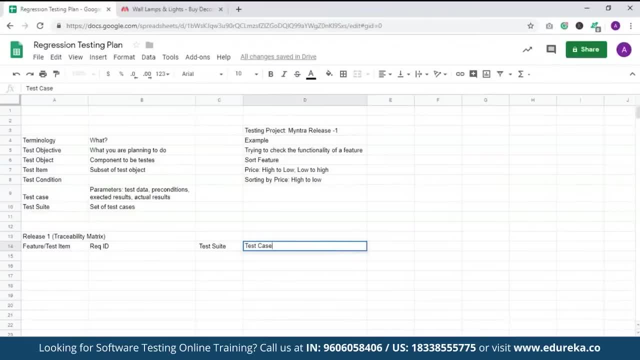 and then comes the test cases, So we go, let's try it. the first element here, So that would be: this is the website that we're testing for, and what are we testing? the sort feature That's the object and item is price, price. 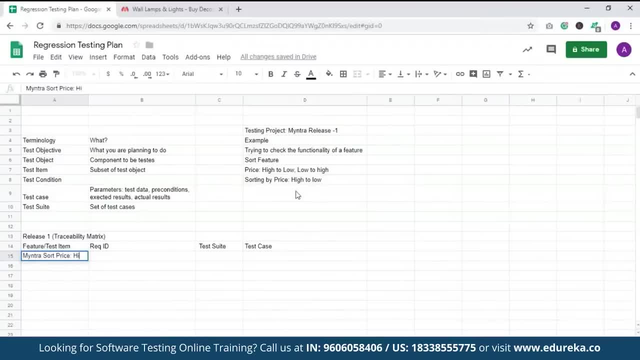 And what is that we're testing for? Let's take high to low first, Then requirement ID, some number you can give so it does things sort feature. So let me give SF and 077 test suit 20, then the test case ID. that would be Myntra sort price. 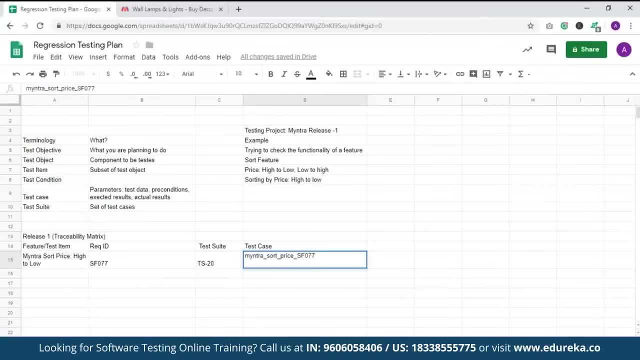 which comes under the requirement SF 077, and the test case ID would be test C 0, 1.. Let me give the this cap test case 0, 1.. So yeah, just like that, I can create multiple test cases: 2, 3.. 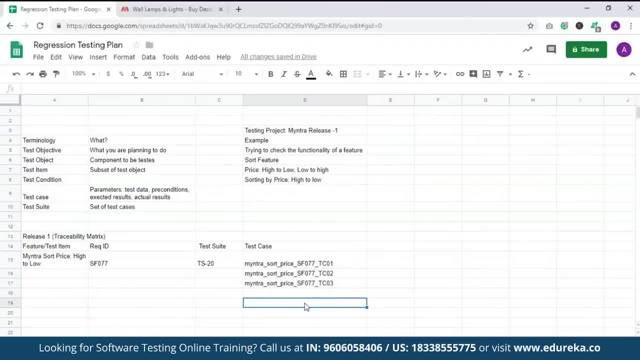 So here we go. We're done with the first traceability matrix, the first element. Similarly, you can write one more for low to high as well. I'm not going to write it, It's the same. So this is how we write a traceability matrix. 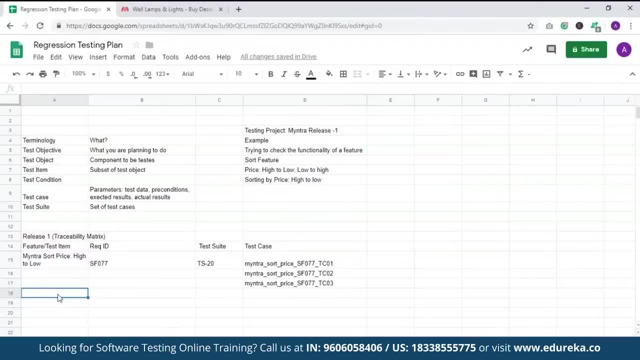 for the release one. So let's say you have performed testing by considering the filter option, which is high to low, and the testing work properly without any errors. and these are the test cases which you have checked for, high to low, and everything is working properly. 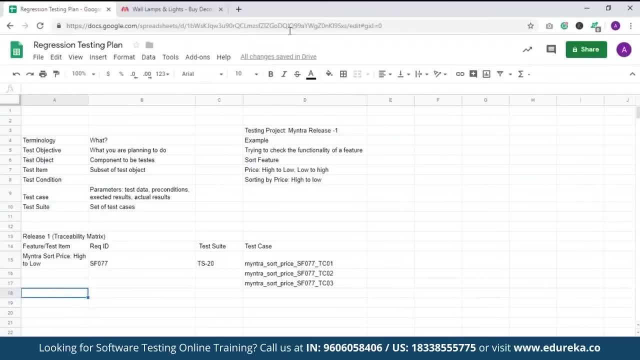 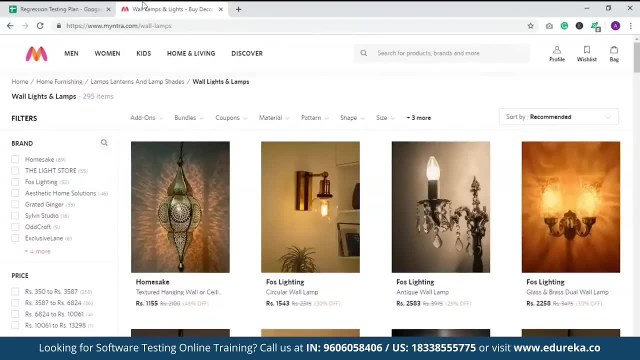 and for now it's good. now We'll move on and perform testing for other feature, Let's say under the right them actually with it, perform for high to low. Now let's go for better discount. can see the better discount option here, right? 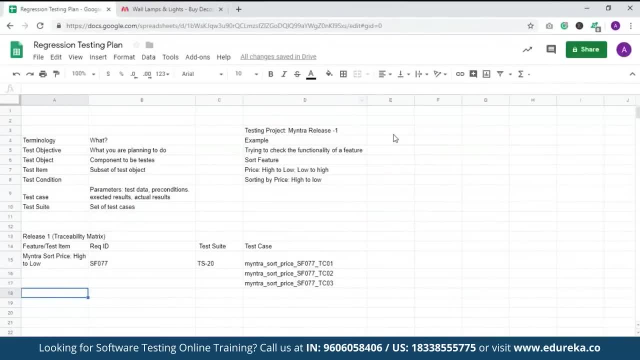 So I'm going to perform test for that. All right, it is planned for that. So it's the same thing again. So testing release. This is example as well. It's the same. So I'm trying to still check the functionality. 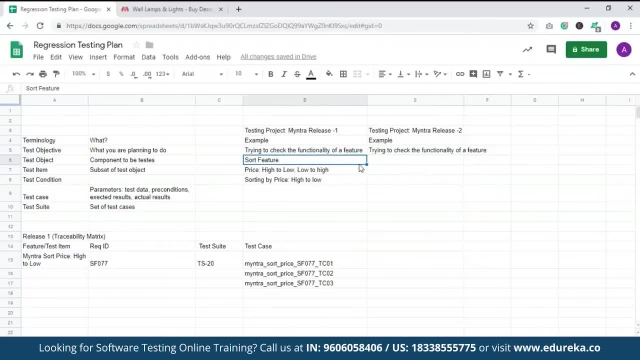 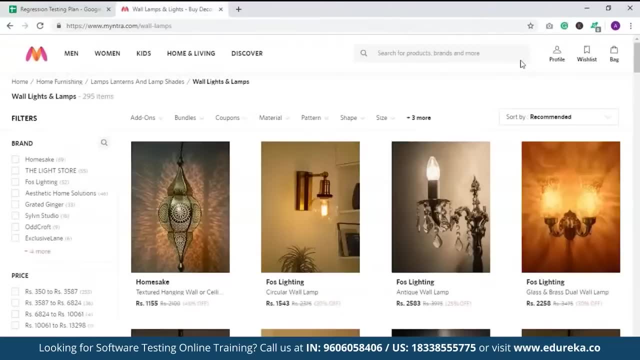 of the feature. So my objective is same. and what is the feature that I'm trying to check on? sort feature? it again, It's the same. and what is the thing I'm trying to check on? It's not price now, It's discount, better discount. 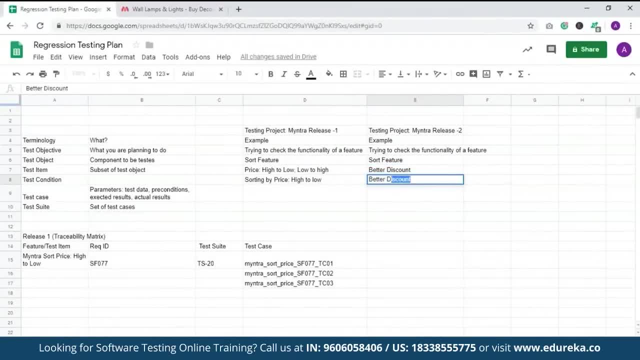 And you do not have any multiple options here, So it's just better Discount. So there we go again. We have test cases, multiple test cases and that, and multiple test use under that, So let's write a traceability matrix for that as well. 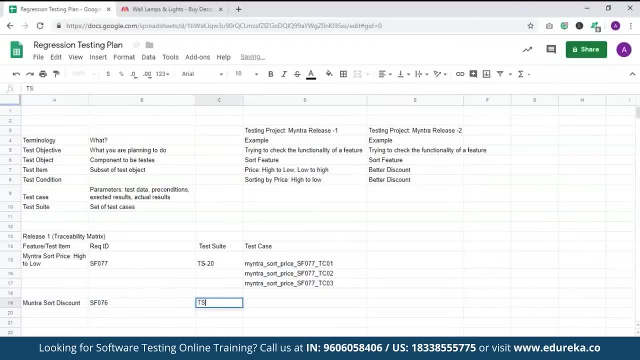 SF 076 and test suit 32. that is based sort discount And the test requirement ID, which is SF 076 in this case, and then comes the test case ID 0, 1, just like that. But here I have four test cases. So that's how you write your traceability matrix. 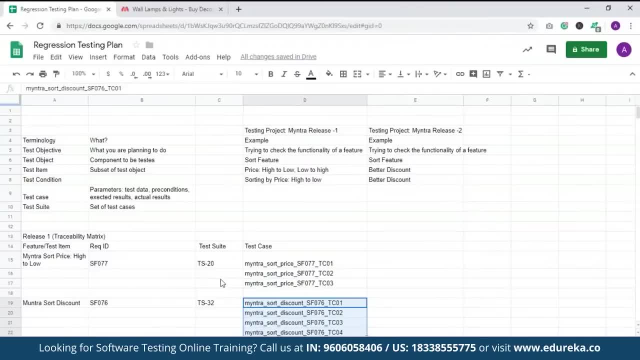 Then now you're still dealing with the normal testing process. Let's move on to regression testing Now. what happens is, when I tried to test on this feature, it's working properly. then when I tried discount option, it's working properly. But after I added this discount option, when I try to check. 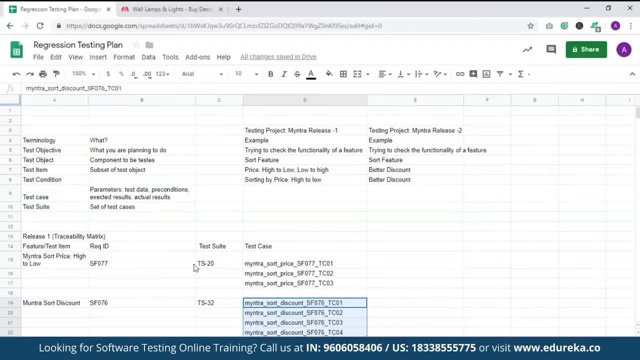 for price. again, I want the sorting being done from high to low, but based on discounts. then this option, which is high to low, is not working properly. So again, here I have a testing release which is still do. I'm just going to drag it from here. 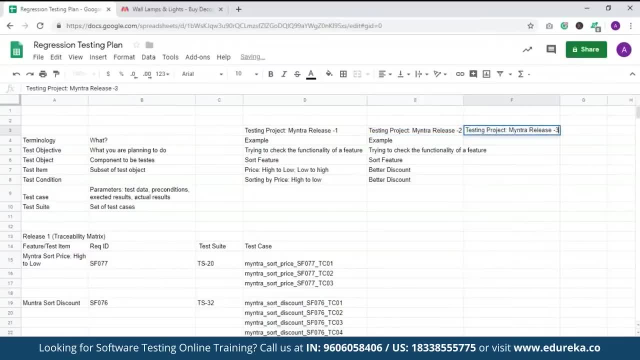 Let me increase the size of this and still into. it's just that after introducing the new feature or the new functionality, the previous functionality stopped working or I've got an arrow. So it's still example. For what is regression testing? What are we trying to do here? trying to check the functionality. 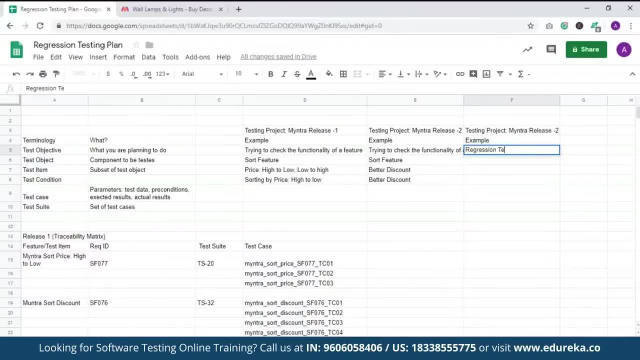 but we are performing regression testing, So that's our objective. So what's the feature that's sort? again, We're still checking out the start feature. What is the thing that's not working price? High to low and low to high. So I'm sure you're understanding, right. 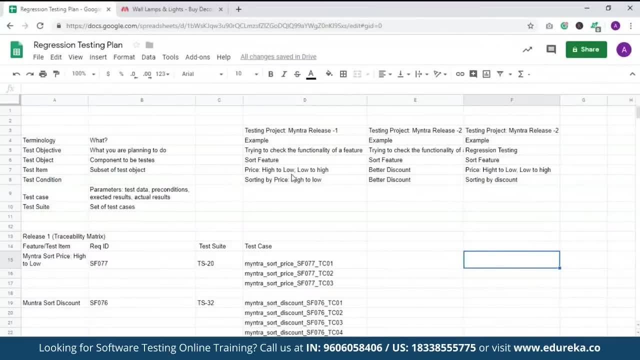 This is my only feature, which was there in the sort consider. I tested it. It's working properly. This also is working properly. the second one, which is based on discount. but I'm trying to win. combine this and see how the high to low is working based on the discount. 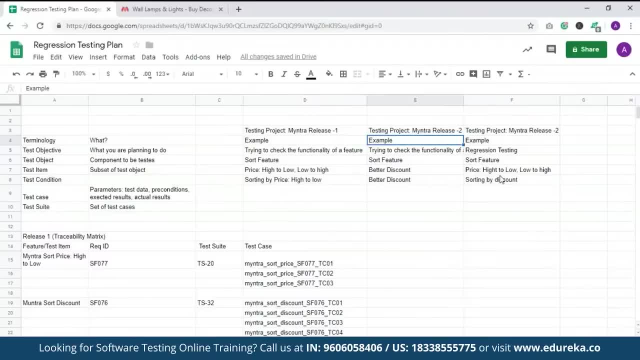 The high to low thing is not working. That's when I want to perform regression testing and check out what the test cases which are not working and what are the bucks. So that's how I perform. for that I'll be writing under the traceability. 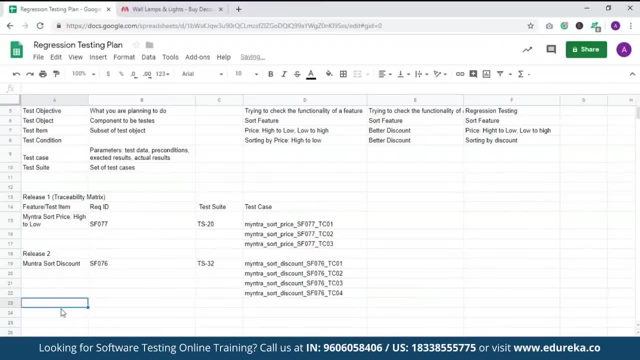 Matrix. This would be for the release to. this is again for the release to itself, but for the regression testing. Here we go. The first thing that happened was the defect that we found, So the first option would be: or the parameter would be: defect ID. 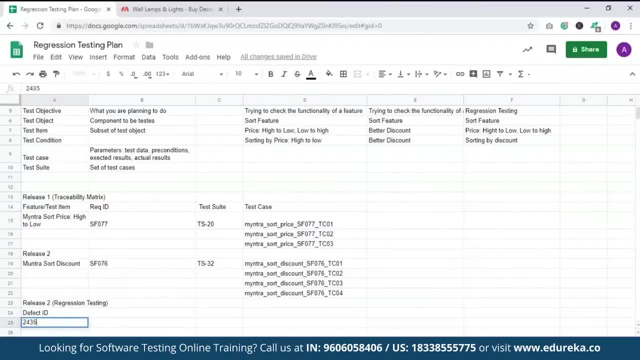 And let's say the defect was some number 245 E. So what was the test case on which the, if a defect occurred? That was Myntra sort discount. So performing the test would give it a number. Let's say it is suit 34.. 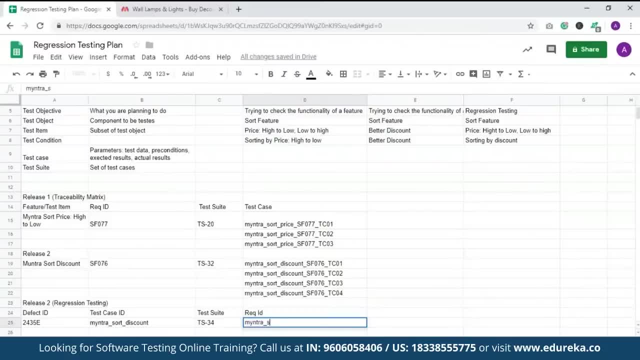 So the requirement ID, next Myntra sort. when we try to combine the price and this can't, we got that error. So that's it: Myntra sort, price discount and the requirement ID, something we should give right, Let's say SF 0 or 98.. 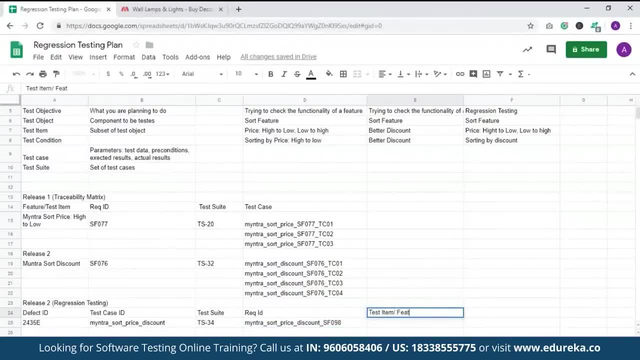 So then comes the test item or the feature. Now you might be a little confused, because the format which I've used in the first and the one which have used now is totally different. and it seems a little weird. and let me go through it again. 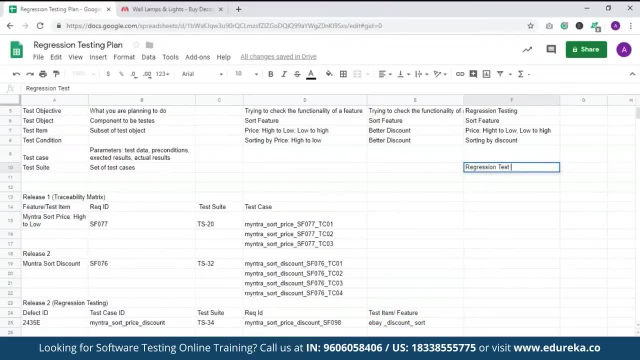 So here you have something called a regression test cases and regression test suits. So basically, guys, these Matrix, we call it a bi-directional traceability Matrix. So the first one, let me just go through it again. The first one: we have your item on which we are sorting the requirement ID, the test suit. 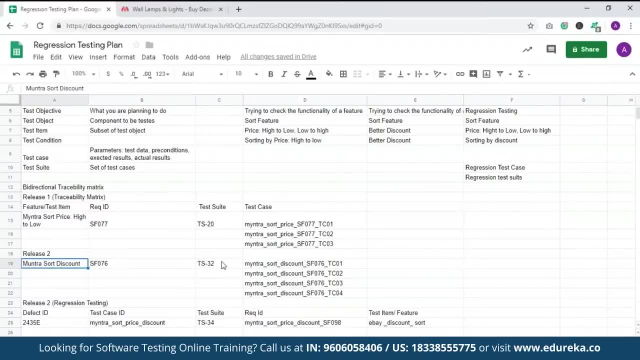 which the test case belong to, and these are the test cases which come on the test test suit. Now, what we did is we perform testing for both the features and when we try to check if combining this features or the functionality of high to low is working. 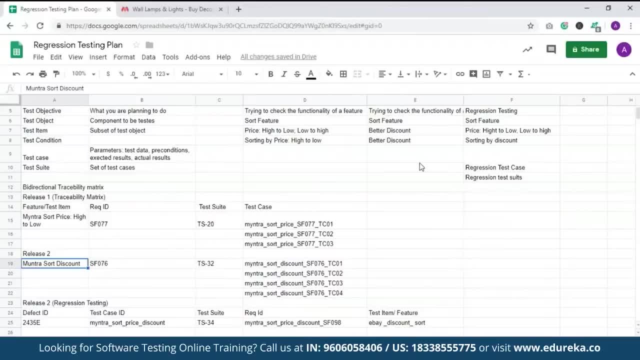 after the discount feature is added, It's not working. We are getting an error or a defect and that effect as a Heidi, that defect ID we representing here. So, but when did we get that here? So what is the test case that we did test for here? 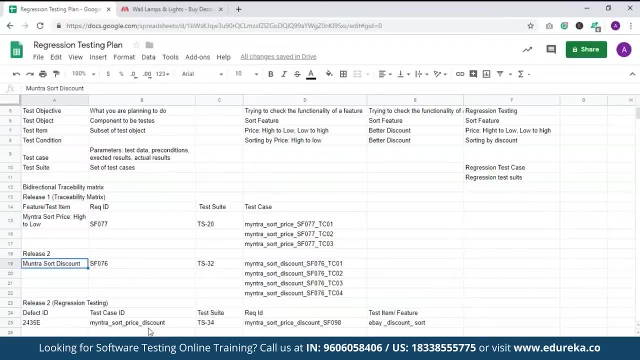 when we try to sort first based on the price and then apply, the discount thing is not working. So that's the test case ID. and which test case does this test case ID belong to this particular test suit, and what is the requirement of this particular test case sought? 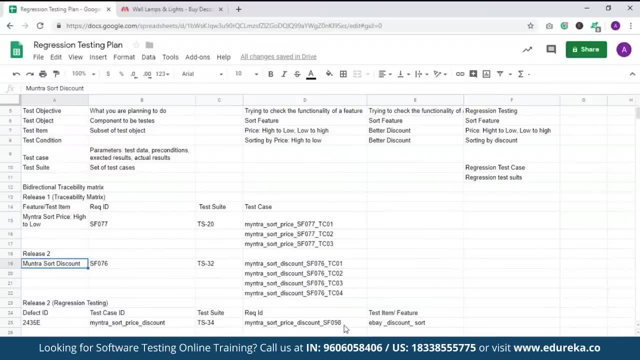 based on price and then on discount and this is a requirement ID. So what is the item or the, basically the feature or the object that we're checking here on sort. So from the defect we try We're tracing back and coming back to a feature. 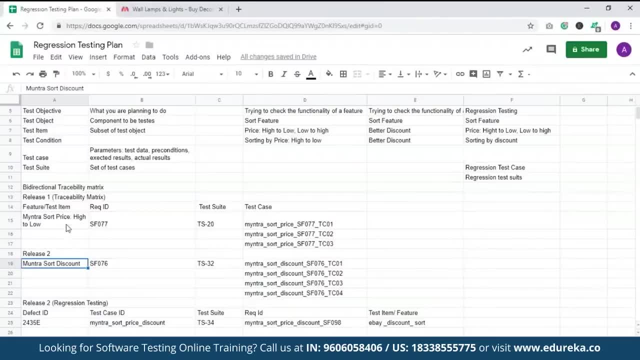 which we're testing on. you got my point right here We started with our feature or item and then we traced back to test case. But here we started with the defect and then we came back to a feature. so defect, which is the test case ID that we're checking on the suit. 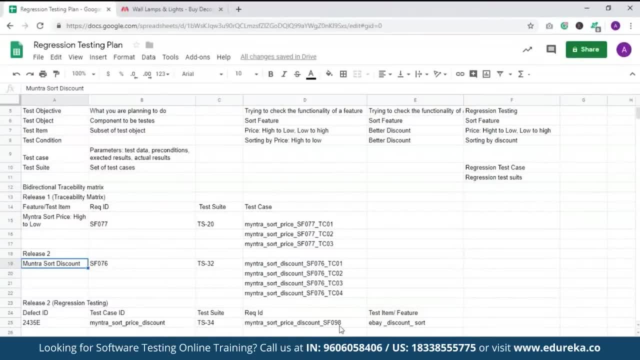 which test case belongs to and was the requirement of the test case, and then the item on which it's being tested. So this is bi-directional traceability Matrix. Well, this is just a small part of- you can say a million small part- of what you can perform in testing. the very simple example. 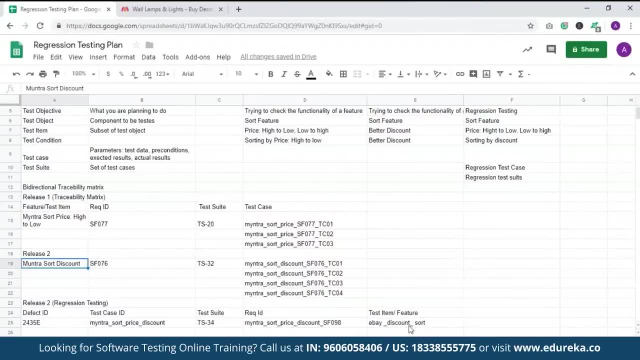 like that. You can perform multiple traceability mattresses, multiple releases and, in one release only, multiple tests. So basically, what I'm trying to say here is that this point- this item- is dependent on other features, like the discount option, is dependent on high to low and low to high. 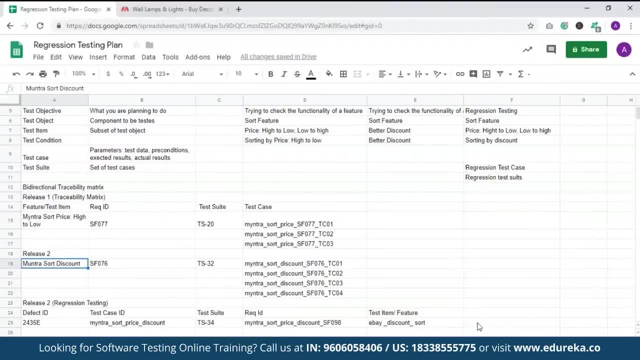 So whenever you trying to make any changes to discount option, your high to low or low to high option, They're not working, or either they're working or not working. from that You can tell these two things, or the two items are related to each other. 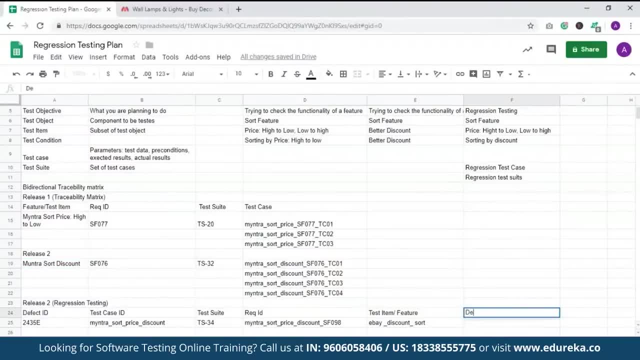 or dependent on each other. for that you have, or you can add, another parameter called dependent features. So what are the features which are dependent on our discount? It's price High to low, similarly mantra, sort, price. and what are the test cases which are dependent on this defect ID of the test case. 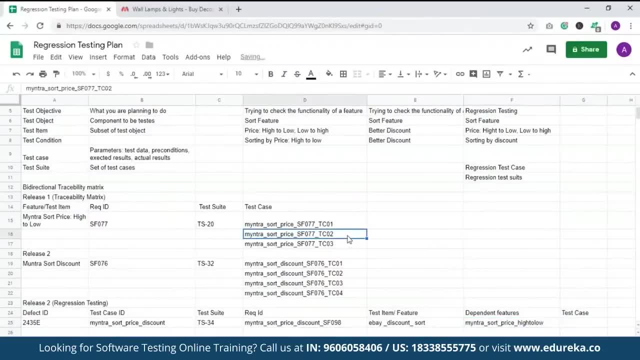 That also you can represent here. Maybe this test case is not dependent on it and this test case is dependent, So what you can do is going to copy it and paste it here. So this is the one test case which is dependent on the discounting. 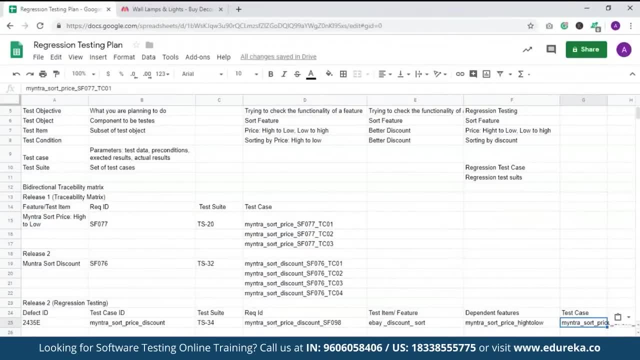 So that's how you write your traceability matrix. I hope the thing is clear for you guys. So we just started with the basing testing as in one feature. everything work Well. we have certain test cases and the test suit and proper. then you have another feature. 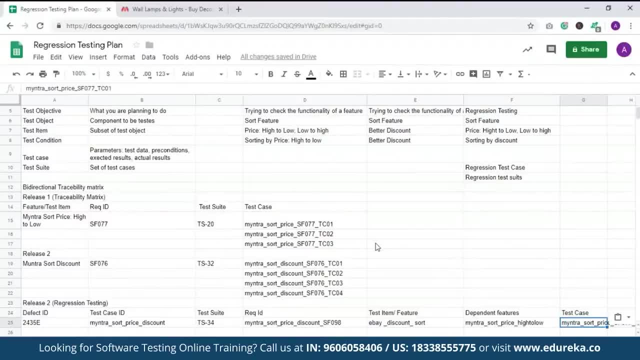 which is better discount. based on that, you perform test. It's working Well. now you try to arrange everything from high to low and then apply discount. then you're getting in defect. based on that defect, We created a traceability matrix. We traced it back to our feature, which is sort. 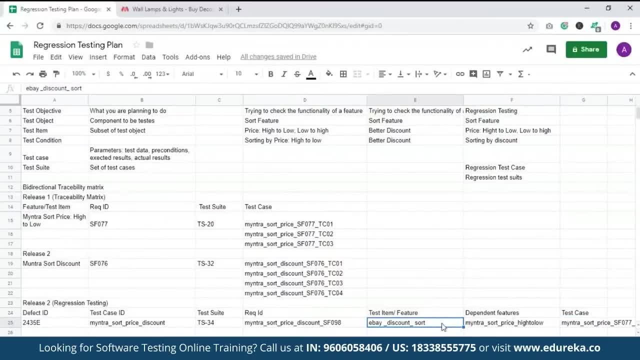 and the sort feature is our other features are dependent or interrelated to each other, So that's how they're affecting each other. So for that we need to perform testing from the beginning again, check out what are the errors and find out the defects and fix them. So that's what regression testing is all about, guys. So any changes that I'm added or made- it could be adding new feature, updating the existing feature- you should check if it's affecting the already existing functionality of your application or software. That's what regression testing is all about. 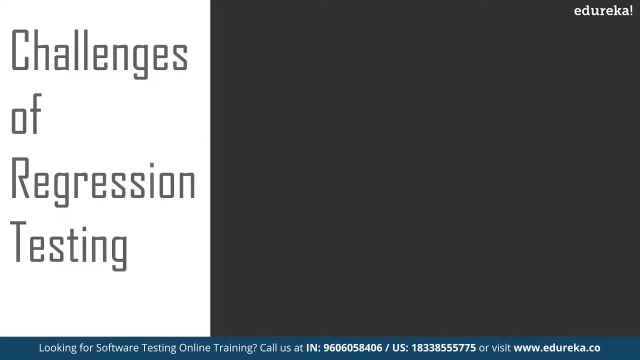 So that's all with the demo. Let's move on to the next part. So regression testing is easy to define and understand, but baffling when it comes to performing regression testing of a software product. One reason is the dynamic nature of software product. 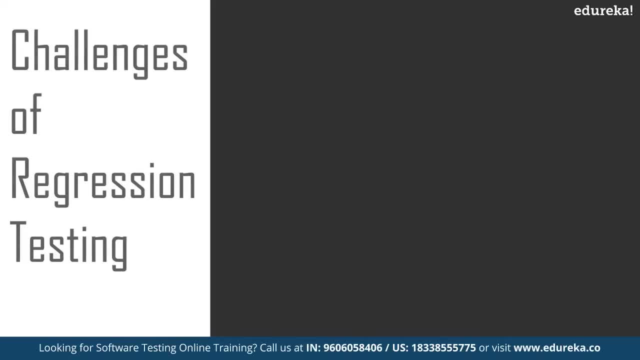 It keeps changing. You need to understand the challenges well before you can craft a counter strategy for these challenges. So let's have a look at common challenges of regression testing. So the first thing: regression testing is often considered as a drain of resources and manpower. to test again: 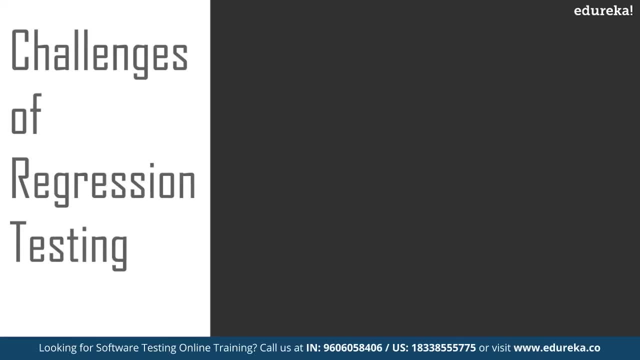 and again something which has already been developed, tested and deployed at early stages. So when testers are told to perform regression testing, that tempted to perform exhaustive testing of the software product quality assurance manager needs to make sure, or he needs to devise an intelligent methodology for regression testing. 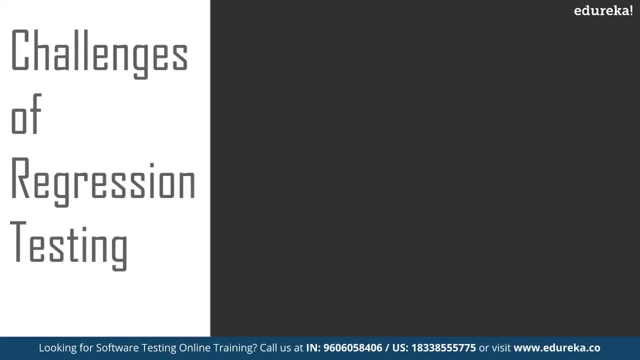 to assure that every required test case has been executed within the limited span of time and the amount of money that he's assigned with. so, basically, the first challenge that you'll encounter is it's time-consuming and expensive. So, as a Q analyst or manager, 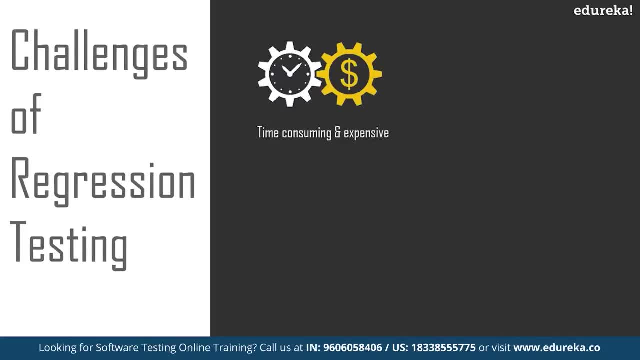 you need to devise an intelligent methodology for regression testing. next is it's complex and challenging. as new features and changes are implemented in software product, more test cases are added to regression test suit. as the product functionalities expand, testers are overwhelmed by the regression test cases and the fall victim to lose track of test cases. 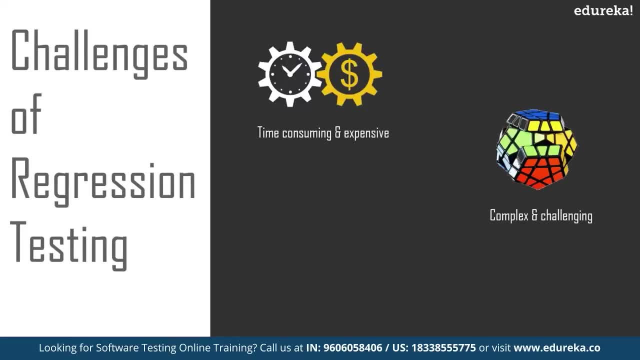 and when they lose track of the test cases, they overlook the important test cases as well, right, So regression testing is a complex process. This can be prevented by regularly monitoring the regression test suit and deleting the obsolete test cases. It is also important to avoid any duplication of test cases. 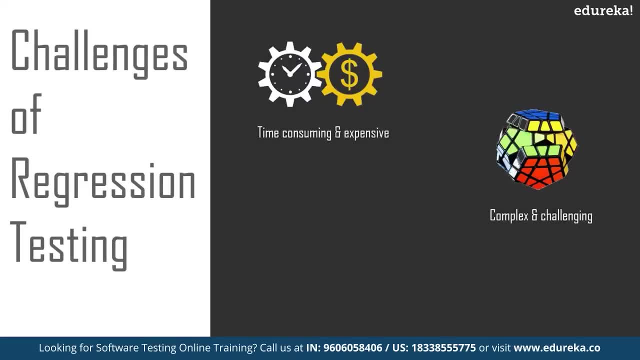 as they lack, to unnecessary effort and frustration for testers. Lastly, it's the communicating business value, and regression testing is usually tough. regression testing, as you know, in just existing product features are still in working order. communicating the value of regression testing to non-technical leaders of your company within your business: 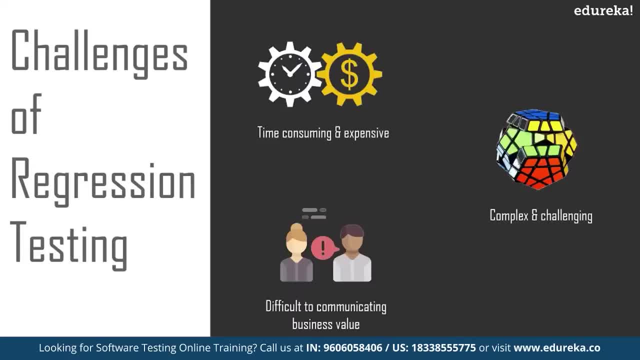 can be a difficult task. Executors most of the time want to see the product move forward. making a considerable investment in regression testing to ensure existing functionality is working can be a hard task. So these are certain challenges that you'll come across when you're performing regression testing. 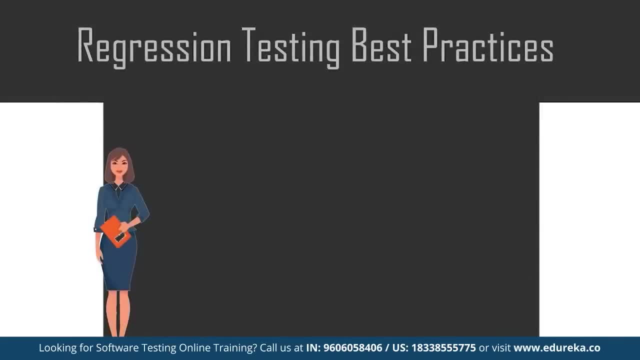 So, regardless of the method of implementation that we discussed earlier, that is, retest, all select and prioritization, There are a handful of general best practices that you can follow while implementing regression testing. that way, you can overcome the challenges which we discussed earlier. So the first thing is you need to maintain a schedule. 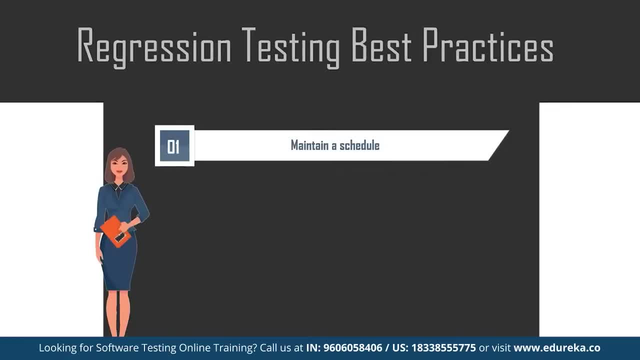 choose a schedule of testing you can maintain throughout the software development lifecycle, So testing is never placed on back burner. Secondly, use a test management tool in order to properly keep track of all the tests that are being performed a regular basis, and have the records of their performance over time. 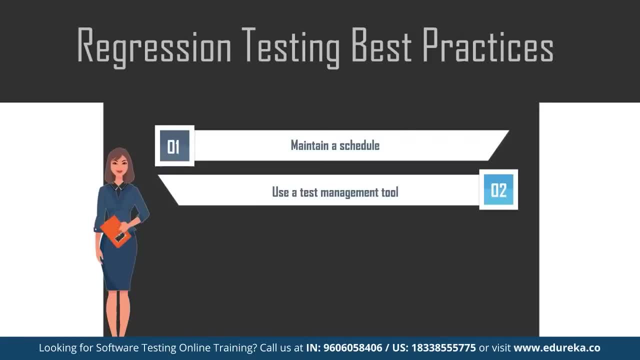 It's better to use a simple kind of test management tool that does all the tasks for you, instead of you spending long amount of time and efforts on keeping track of all these test cases. You can break down and categorize your test. tests are often considered to be easy to understand. evaluate. 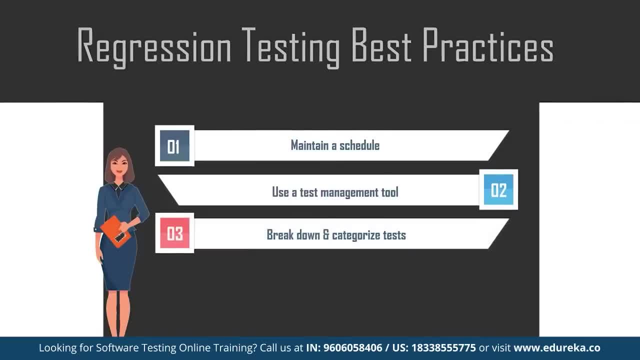 if they are broken down into smaller pieces. It's not just with testing anyway, right, If the thing is huge and complex, it's difficult to understand, but if it's broken down into pieces and then you try to understand, it's easy. So try to refactor your test cases as often as necessary. 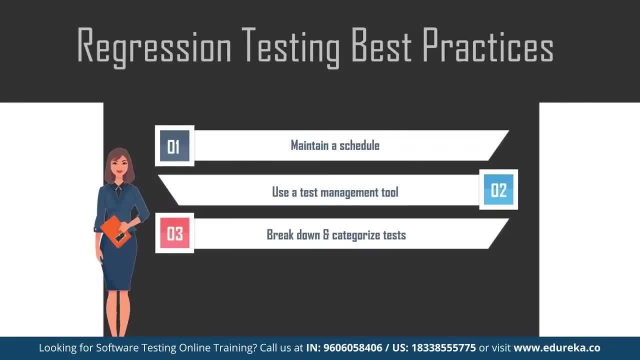 then categorize them such that the categories of smaller tests can be prioritized over the others. So this makes sorting and execution much easier and future for you. You can also consider customer risk not also? you must and should consider customer risk. basically, the product is made for customer right. 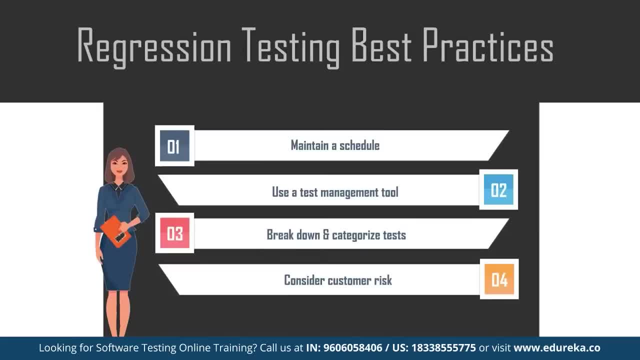 So when developing and prioritizing regression test, keep track about considering the effects the test cases will have on the customer or the business as a whole. So try to design such test cases that they cover as many test cases as possible And, lastly, evaluate test prioritization. 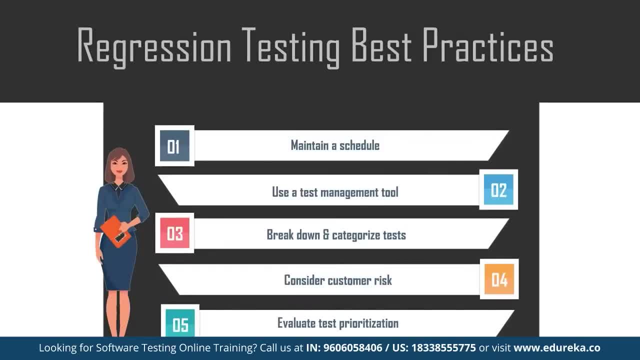 So, when using any form of prioritization to order your regression test, try to find a sensible way to order them such way you know what you're actually doing. don't mess it up. So, while these are certain things that you can follow to achieve better regression testing results, 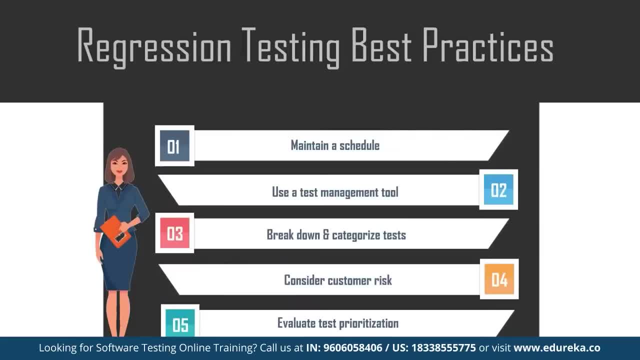 so failure to perform effective regression testing can cause a lot of needless suffering. It might happen that everything required in the new Sprint is working fine, but the previously implemented features and functionalities got messed up. If this happens, the client would not appreciate you for the new functionality. 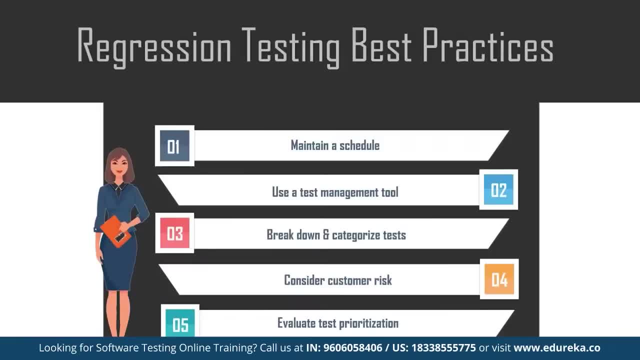 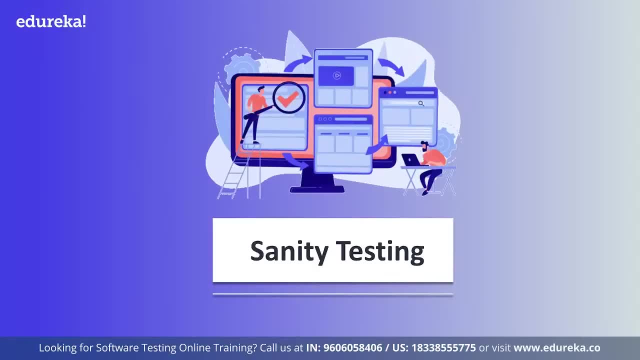 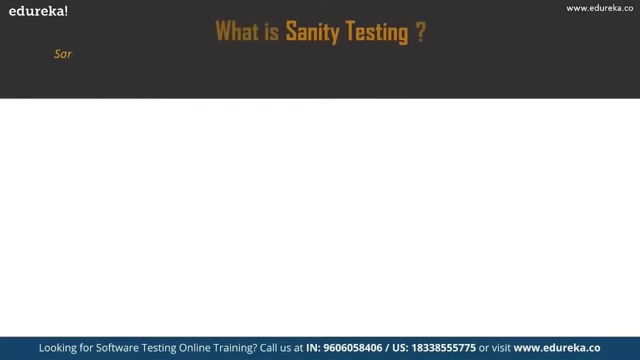 it would become angry, irritated and can be real trouble to handle. So, guys, regression testing is really important. So what is the first thought that comes to your mind when you hear the word sanity testing? if you make a guess by its name, then, as the name implies, sanity testing aims at checking. 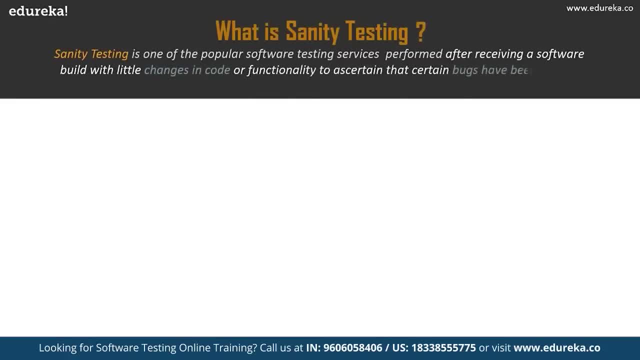 whether the developer has put some same thoughts while building the software product or not. It's quite close to actual meaning of sanity testing. Sanity testing is a software testing technique which does a quick evaluation of quality of the software. will is to determine whether it is eligible. 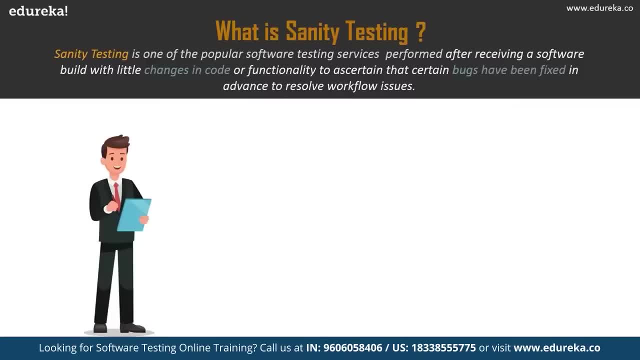 for further rounds of testing or not. So sanity testing is usually performed after receiving a fairly stable software build- and sometimes the software build might have minor changes in code or functionality- and it is sent for sanity testing to check if the books have been properly fixed. 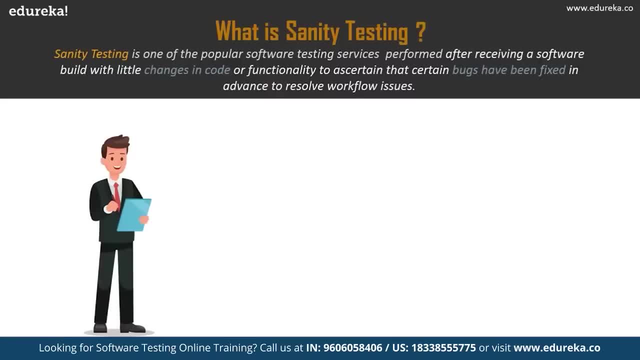 So what exactly is the intention of performing sanity test? Let's discuss the objectives. first thing is to verify and validate the veracity of newly added functionalities and features. Secondly, to evaluate the accuracy of new features and changes, if they are added. and thirdly, to ensure 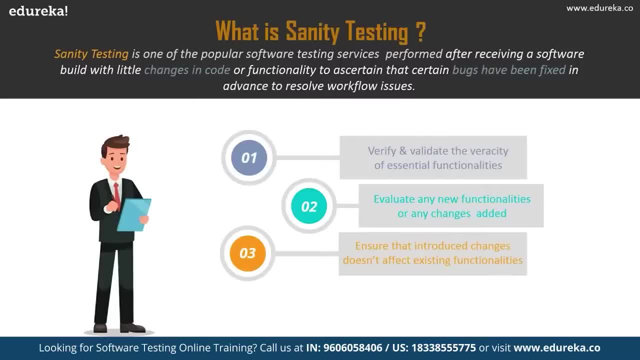 that introduced changes doesn't affect other existing functionalities of the product. Lastly, test rational thinking and logical implementation of the developers. That's the core and basic purpose of sanity testing. So basically, sanity testing is surface level testing which helps in deciding if the software build is good enough to pass it. 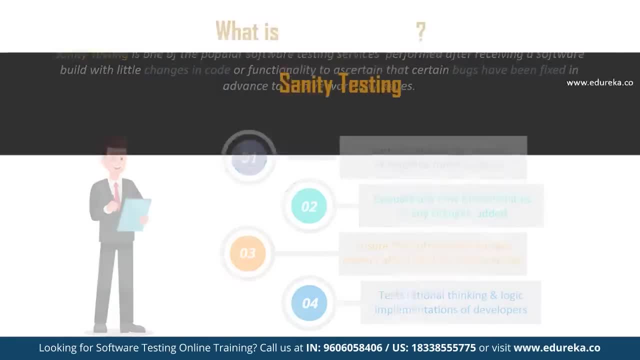 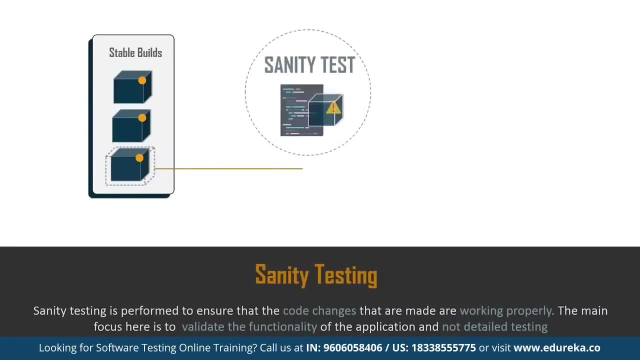 to next level of testing or not? Well, that's clear, right? So here's a basic representation of sanity testing. as you guys can see, I have three bills here and I want to send these table bills for sanity testing and, once they are centered, sanity testing, sanity testing. 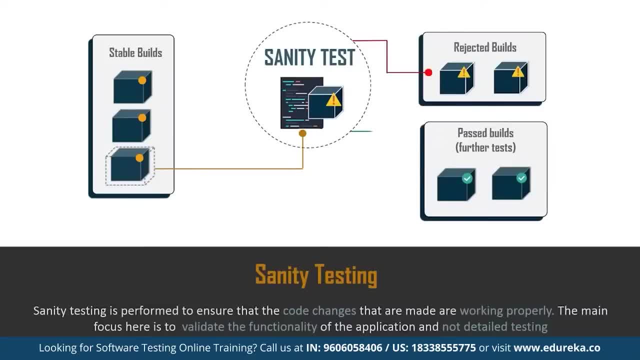 is performed on them to see if any new features or changes are made. if yes, then if they have affected the existing features in any way and if there are any bugs, were they fixed? and all that are checked or performed under sanity test and the bills if they pass the sanity test. 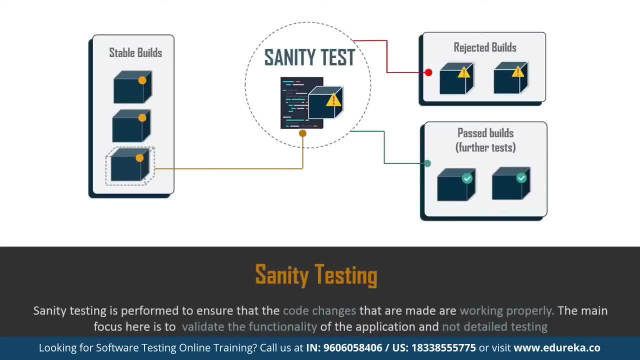 then they're sent for further rounds of testing, else they're rejected, or you can say they're added to the rejected build list. It's simple, right? That's all there is about sanity testing. Well, it's very simple and basic form of testing. 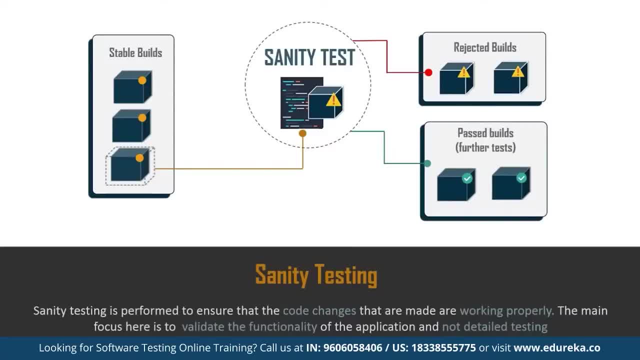 That's performed before any product is sent for further rounds of testing. So to make it more presentable and simple, Here's an example. Let's say the build, which are just subjected to sanity test, is a new feature which is added by Gmail. 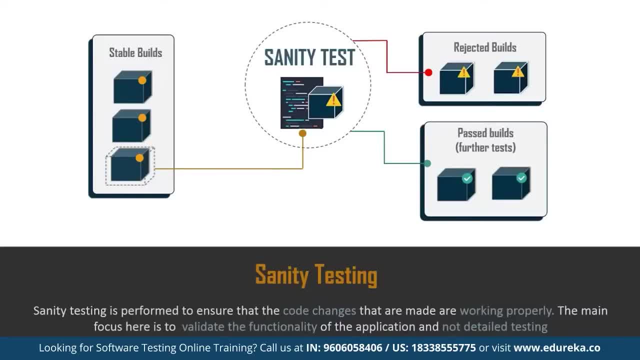 That's nothing but auto acknowledgement feature. What is this auto acknowledgement feature do? it sends a written email that the email which you tried to send is delivered successfully. Now, this is a new feature and it's fairly developed, So we already have a built that stable, sanity test. 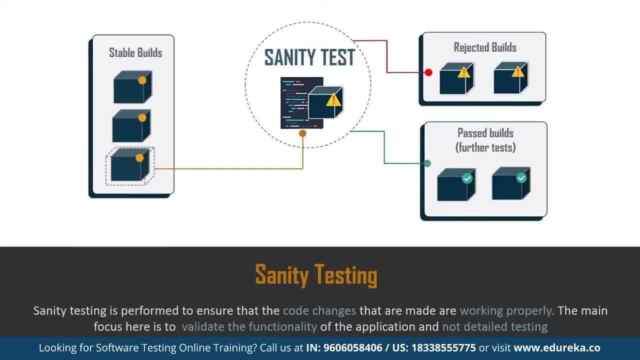 testing is performed to see if this new feature, that's auto acknowledgement feature, is working properly or not and, because of this feature, if any other features are affected. if not, it means that it is successfully passed the sanity testing and the auto acknowledgement feature is sent for further rounds of testing. 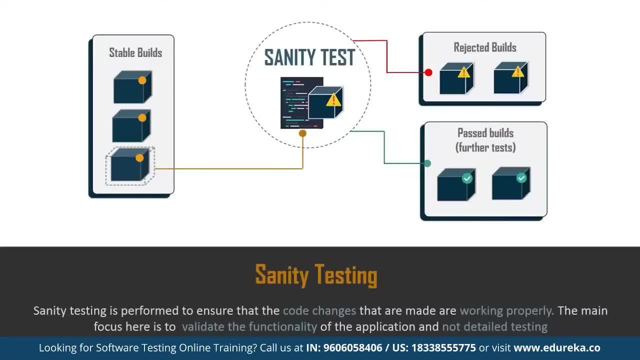 It's as simple as that. So to summarize, sanity testing is performed when a new product or functionality or change is implemented to see whether the software product is working correctly or not. It determines if thorough testing of software product shall be carried out or not. 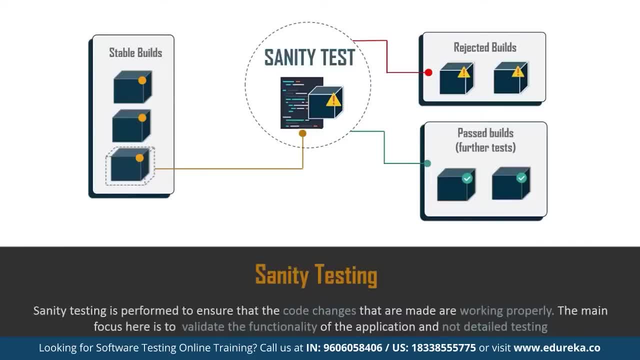 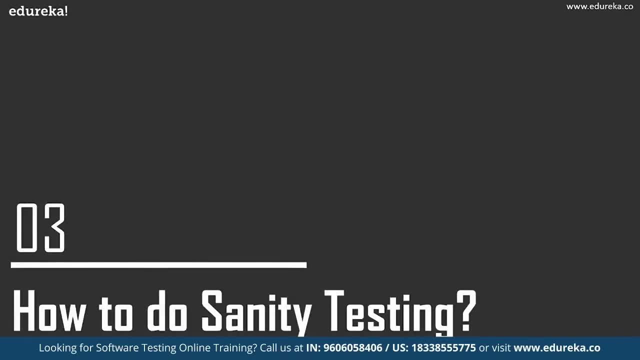 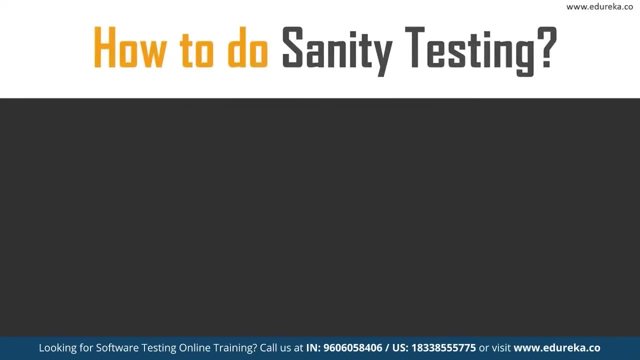 So if sanity testing fails, rigorous testing is not necessary to be conducted. Well, that's well and good, But how do you perform sanity testing? Is there a specific procedure that you need to follow? Well, unlike other types of software testing, sanity testing does not come with handful of techniques. 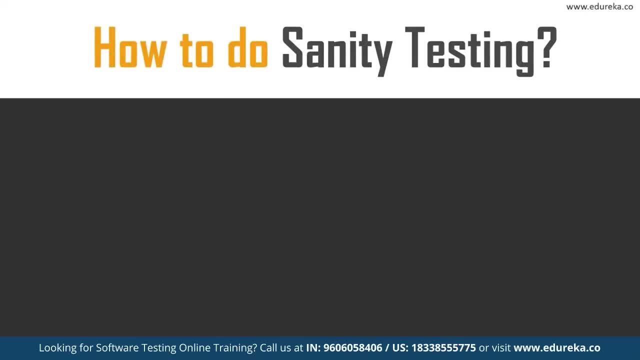 You do not need to script the test cases for sanity testing because you want to perform very quick and speedy testing. So what I want to say here is that the sanity testing is a very speedy and quick process of testing the application, as it does not involve the scripting of test cases. 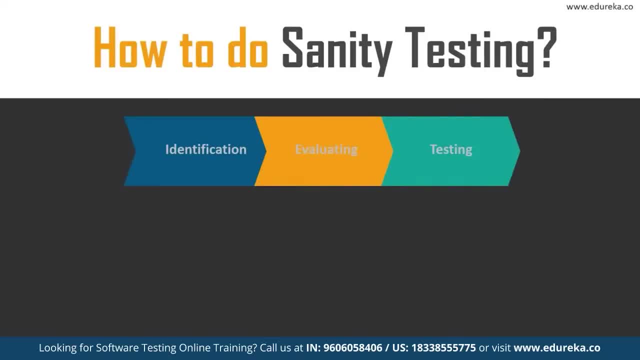 So, guys, the thing that you need to remember here is the main purpose of performing sanity testing, like have been saying from the beginning of the session- is to verify if the newly added changes and functionalities have affected the existing functionalities. are they working properly or there any software bugs? 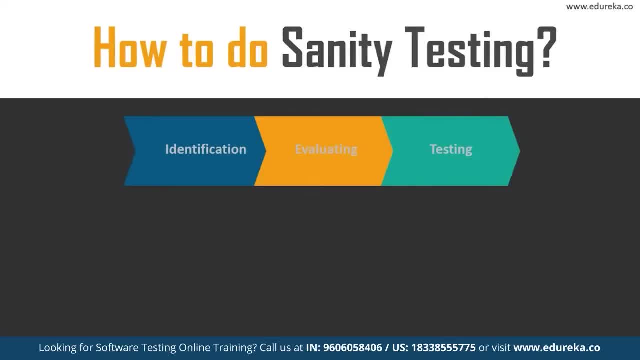 So that's the main purpose. Now, how do you perform sanity testing? It's quite simple. Well, just three steps. The first step is to identify the newly added functionalities and features, along with the modification or changes introduced in the code when you're fixing bucks. 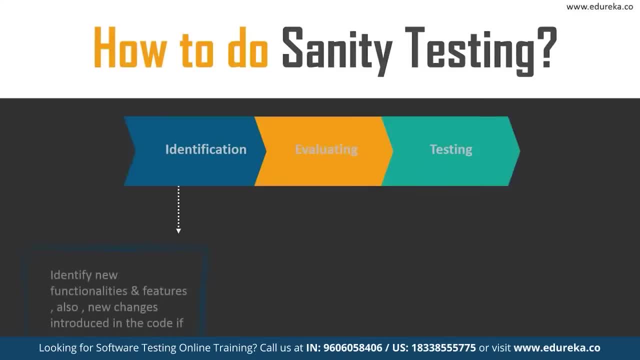 or you can say buck fixation process. So the first step is to identify all the box new features or any changes made to the code. second step is to evaluate this identified features and changes to ensure that the working as intended and the properly working, and that's what we call evaluation. 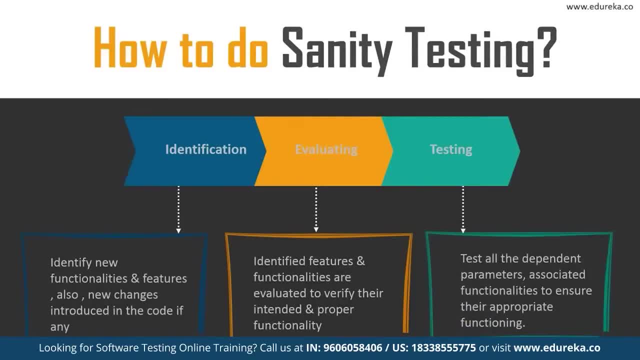 and the last step is testing. that is, we consider and test all the related parameters, associated functionalities and elements of the above evaluated features and changes to ensure that the related features are working properly as well. What I mean to say is that the new changes or the functionalities 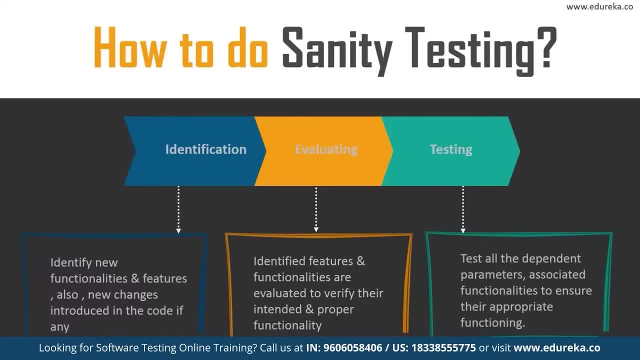 or the box which were introduced did not affect the existing features. That's what you do in testing. So very simple, right? Just the three steps. first you identify if there are any new changes to the features and functionalities, then you evaluate them and then you test. 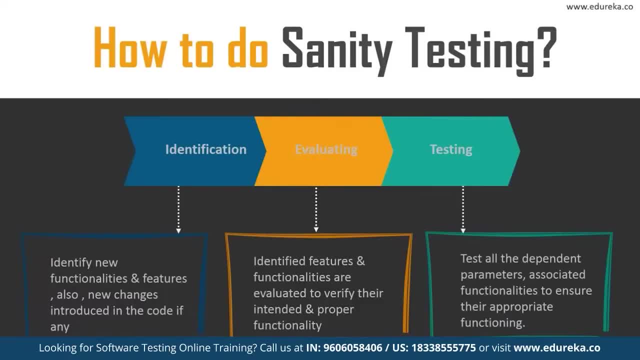 if they are affecting the existing features in any other way. if all these three steps goes well, then the bill can be subjected to more thorough and strenuous texting. So if all these three steps go well, then the build has successfully passed the sanity testing. 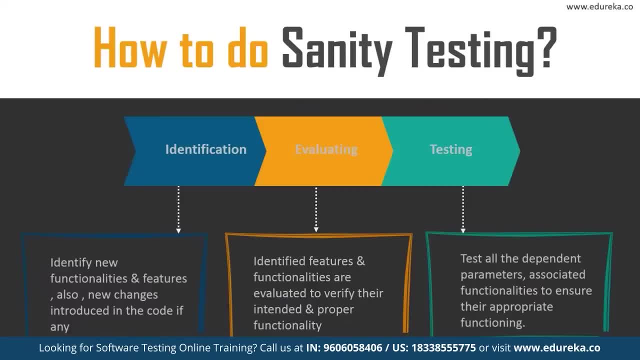 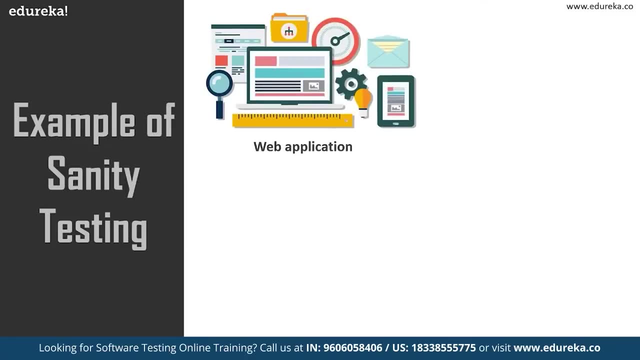 and it can be sent for further rounds of rigorous testing. So that's how you perform a sanity testing. Imagine the following scenario: You have several modules in your application. You have a user registration form in module X that allows user to enter data and submit it. 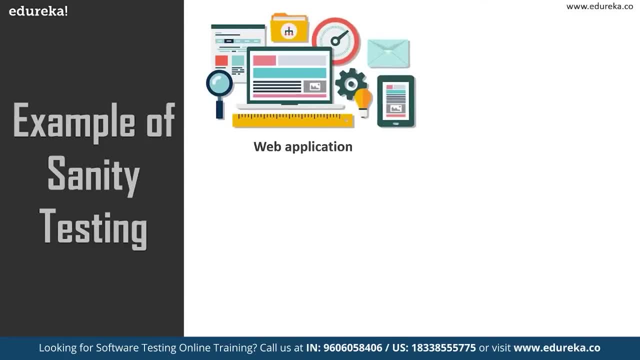 The client has now requested to add preview my profile button in the user registration form, which enables the user to preview his profile before he actually submits the details. You got my point right. You have an application, multiple modules and you have a module called X. now the client is requested. 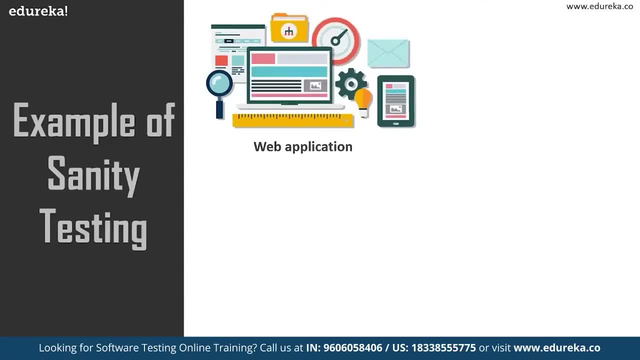 for additional feature called preview my profile, before he actually submits his profile or the details. So now the development team has implemented the request according to the clients requirement, the release in your hands and the build is sent to you. So the release is in your hands. that is testing team. 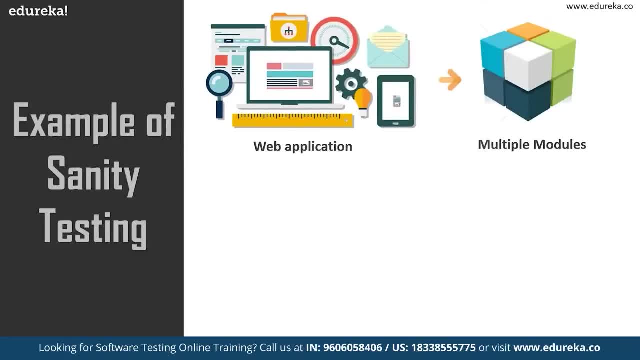 and you want to perform sanity testing. So first you will ask the development team or the manager What's the new feature that's been added to the release. then you'll get to know that preview- My profile- is the feature that's been added and according to that the code has been modified. 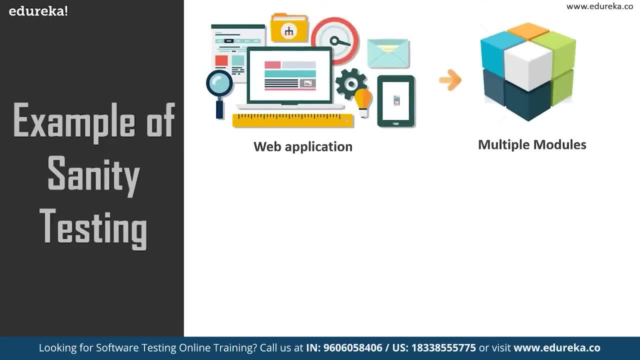 So then you go through the code, you test that particular feature which has been added and check if it's working properly or not. That's what we call evaluating. So once you check that the preview- my profile feature is working or not, then you come to testing feature there. 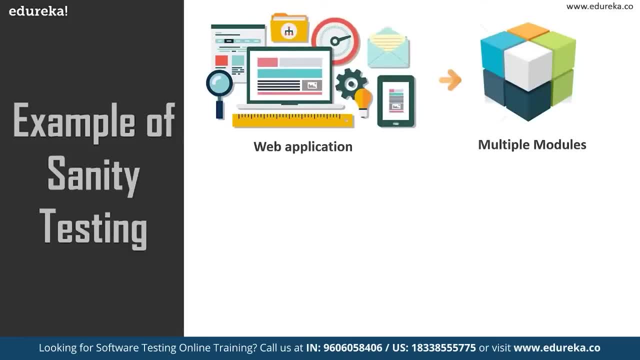 You see if, on adding that, if it has affected the submit button in any way, if it has, it means that the software build has not passed Sanity test. else It means that the software product or the software change which is being made to the build has worked properly. 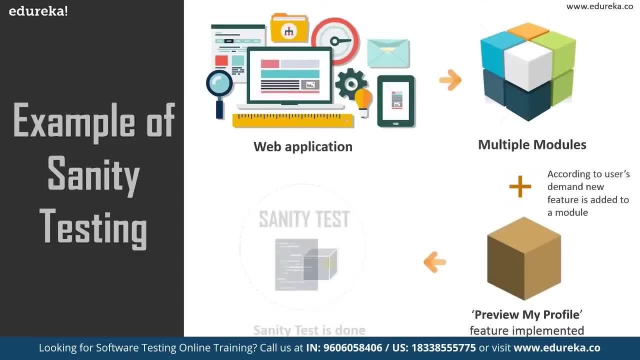 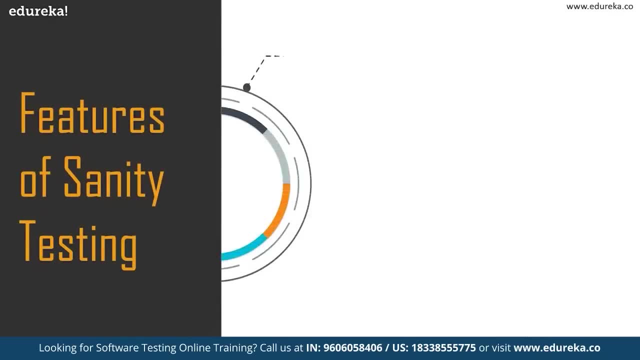 and it can pass to further rounds of testing. simple right. So by now you might have figured out certain key points of Sanity testing. If not, don't worry, I've got them covered. first of all, Sanity testing is carried out on relatively stable bills. 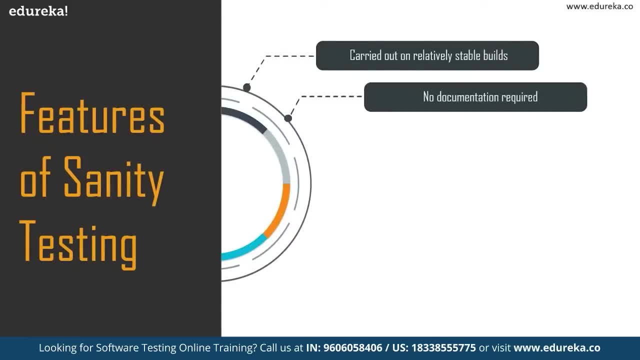 Secondly, it doesn't require any documentation, like I have been saying, and obviously it's performed without any scripts, unlike smoke testing, which is performed from end-to-end. Sanity testing is just performed on limited functionalities, which we will discuss about later by discussing the differences between smoke testing. 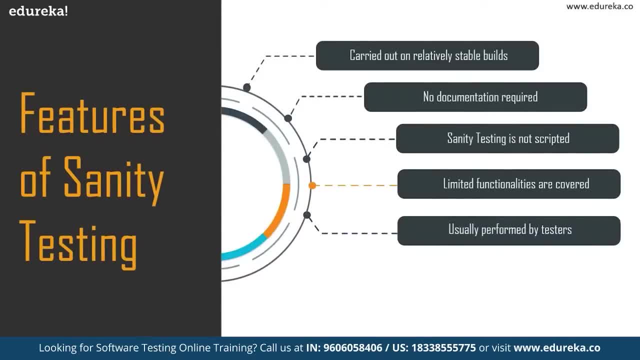 and Sanity testing, and usually it's performed by the testers, not the developers, So developers are not involved here. Well, if I have to Define Sanity testing in simple terms, it's a narrow and deep type of regression testing, and yet it's performed on limited functionalities, not from end-to-end. 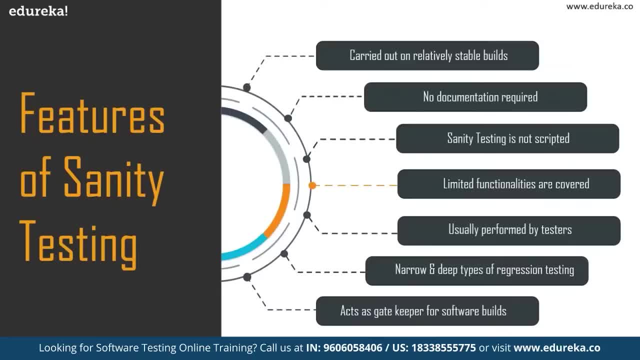 Lastly, it acts as a gatekeeper, as in. it helps the testers to decide if the software bill is worthy enough or stable enough to be sent for the further rounds of testing. So these are some important features, if have to summarize. it doesn't require documentation, less scripting carried. 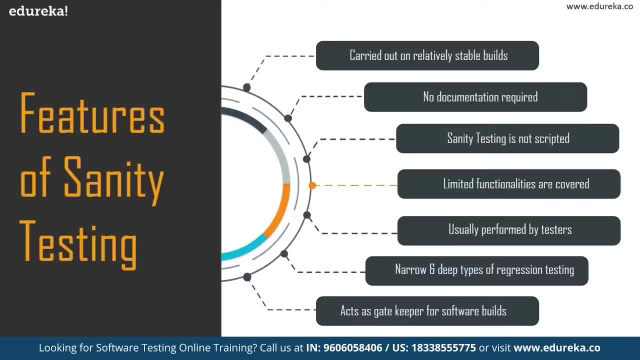 out on relatively stable bills. limited functionalities are covered in this testing, usually performed by testers. It's a very narrow and deep type of regression testing and it helps decide if the software bill is to be passed for next level of testing or not. So these are some basic features of Sanity testing. 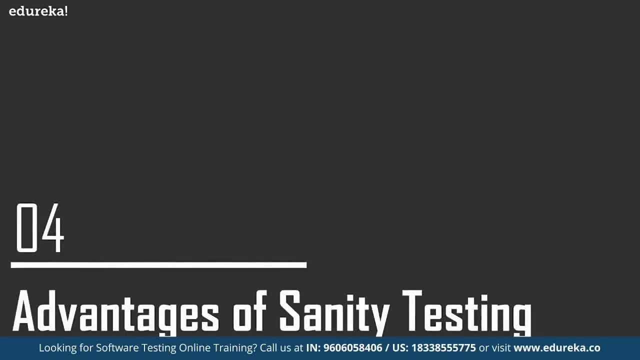 So what would you consider would happen if Sanity testing is not performed? So when a new release comes in, the tester would put entire effort in preparing test cases and executing them. and all that, the testing to him would thoroughly test each test case, each functionality of the application and its user friendliness as well. 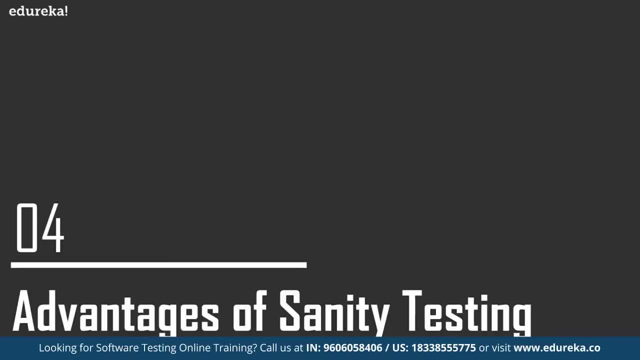 Well, do you see any problem in here? No, right, But there is a problem. The scenario sounds good only as long as new and old functionalities are working well and fine. What if the changes and the newer code have messed up your previous functionalities? 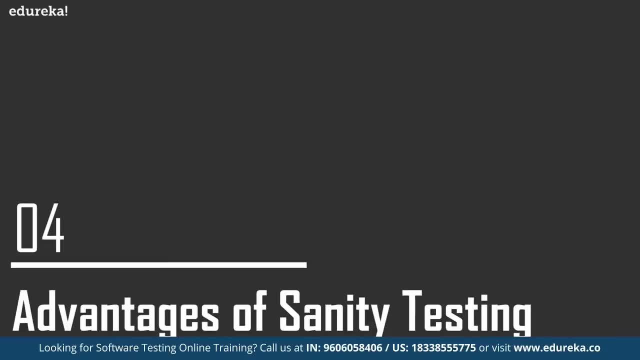 What if the newer release is crashing down at every other action? Do you still consider it's wise to undergo such a list through the full testing cycle? No right. This is where Sanity testing comes in. It's really important phase of testing. 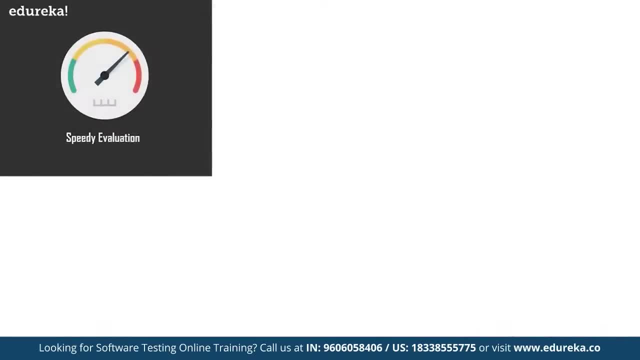 So what are the advantages of Sanity testing? First of all, it offers you speedy valuation. It offers speed. Sanity testing has a very narrow focus for functionalities or areas to be tested. Like I said, it's not end-to-end testing. It's performed on limited functionalities. 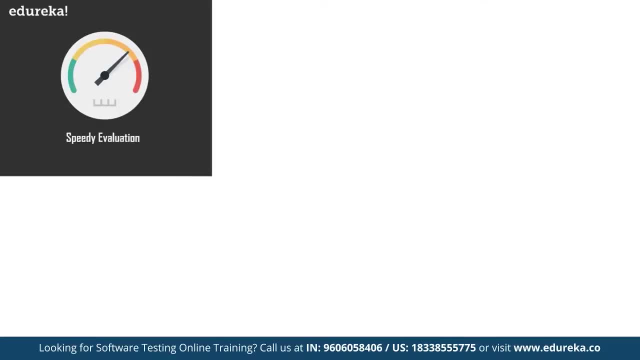 So you don't need to script the test cases before carrying out Sanity testing that the you can say it's very unplanned or intuitive approach to perform Sanity testing. next, It saves a lot of time and effort on testers. part Sanity testing: It determines whether the application should be further tested. 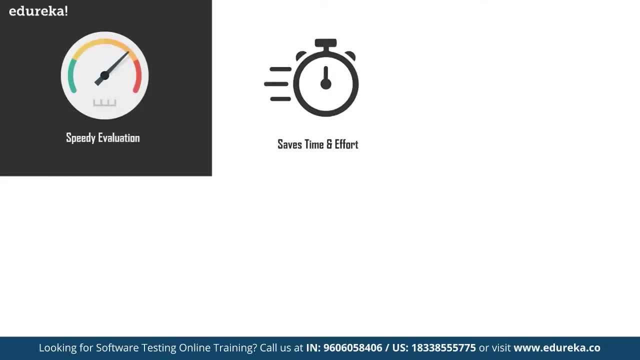 or not. like I said, it acts as a gatekeeper. this saves testers time if the release is in a very poor condition to meet the rigorous rounds of testing. also, testers do not need to report the issues or lock down them anywhere. This saves a lot of reporting time as well. 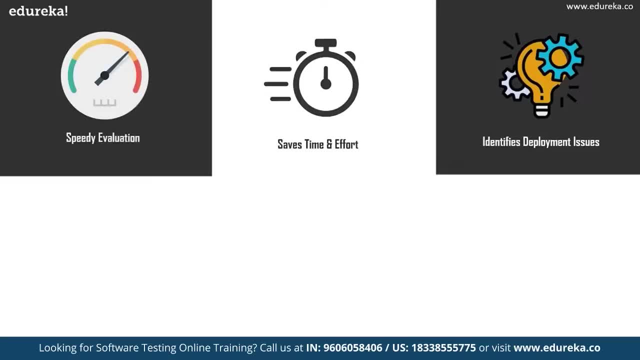 Secondly, Sanity test identifies deployment and compilation issues as well. Suppose a tester may face inaccurate user interface if the developers do not check all the resource files and the compilation. Sanity testing also identifies deployment and compilation issues. a tester may face inaccurate user interface If the developer did not use all the resource file. 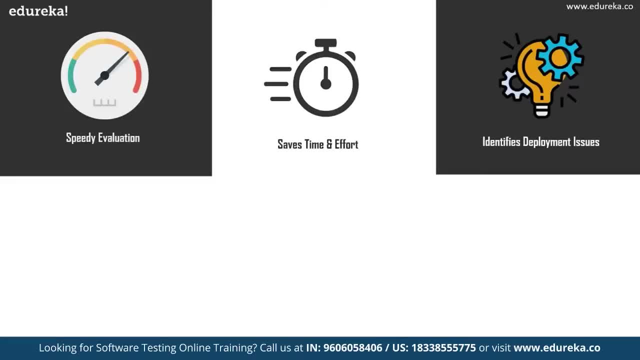 in the compilation. also, developers may not specify some important features to make them visible for testers. a sanity check detects any such problem and it offers a quick solution for well-functioning release and obviously, like we discussed earlier, It does not involve any documentation. Well, you can say very less documentation. 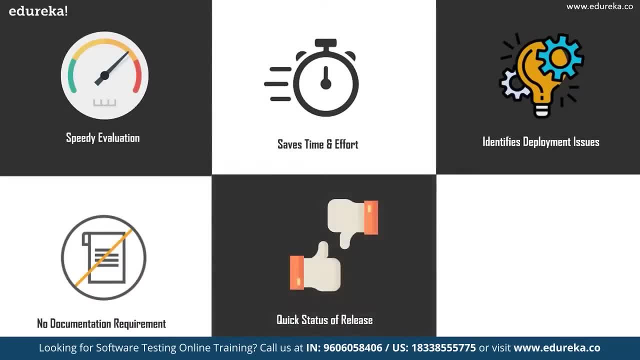 So that's one more Merit in. the other one is Sanity testing gives you a quick state of product which can help you plan your next step accordingly. So if Sanity test fails, you might plan your development team or you can tell your development team to postpone the next task. 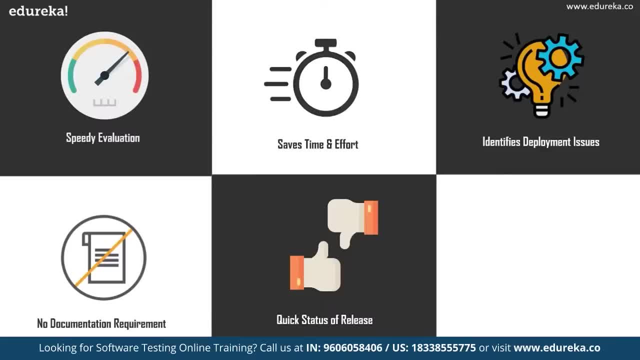 and fix the found-out issue under the hand of Sanity test is passed, You might ask your team to go ahead with the next release and spend less time on fixing bugs. So that's how it is. lastly, compared to other types of testing and Sanity testing is really cost-effective. 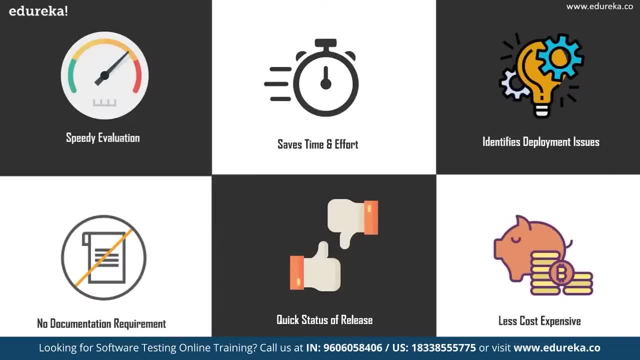 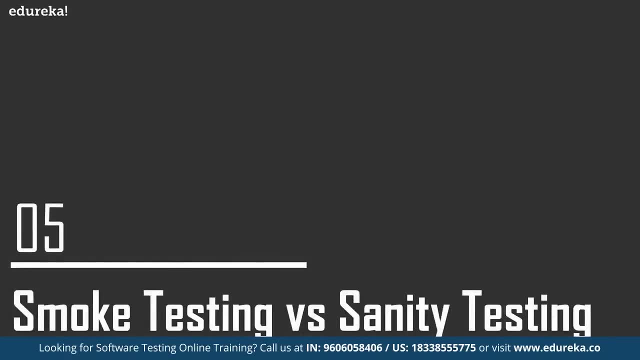 Well, guys, now you know how important Sanity testing is right. with this, We have almost reached the end of the session. last topic of today's session is how smoke testing and Sanity testing differ from each other. smoke testing and Sanity testing are two very different practices. 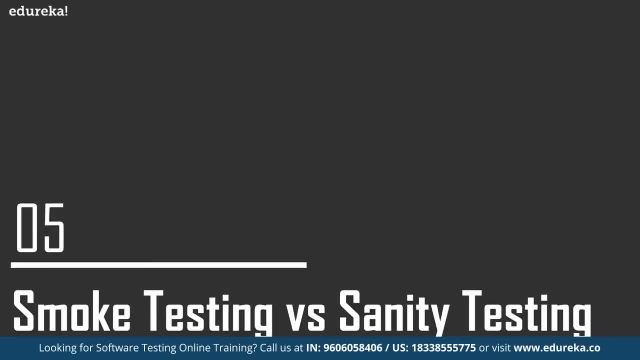 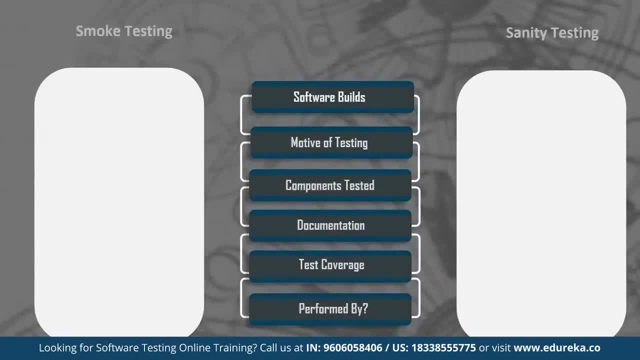 but people still get confused because the distinction between them is somewhat subtle. So let's discuss few key differences between them. So the first difference is the software build your. we already discussed what software builders. well, if you're not sure, the term build is the process. 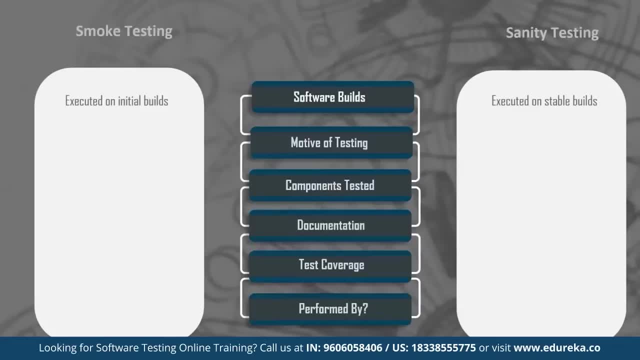 by which source code is converted to a standalone form that can run on any system. the smoke test are executed on initial build of software product, Whereas Sanity tests are performed over the bills which have passed the smoke test and gone through rigorous testing cycle, or you can say regression testing cycle. 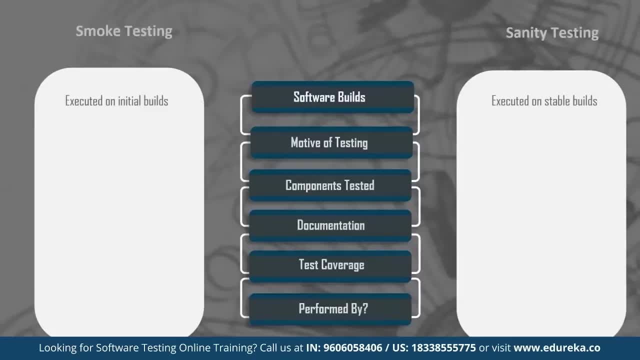 What I mean to say here is: smoke testing is usually performed on very initial bills, Whereas Sanity testing is executed on slightly stable bills than they are in smoke testing. moving on to motive of testing, smoke testing- Make sure that the core functionalities of your program are working absolutely fine. 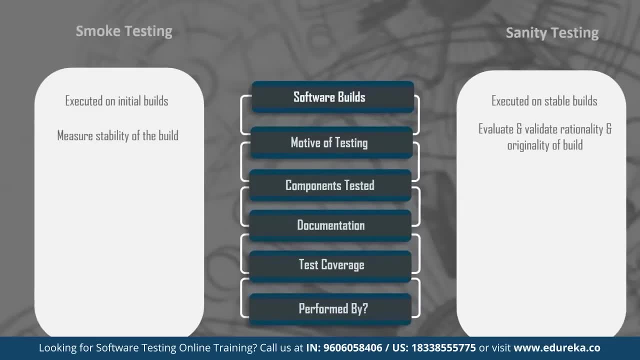 So the motive of smoke testing is to measure the stability of newly created build so that you can move on to the next round of rigorous testing, whereas Sanity testing is to check if the new functionalities or the box have been fixed properly, I believe, without going any deeper, 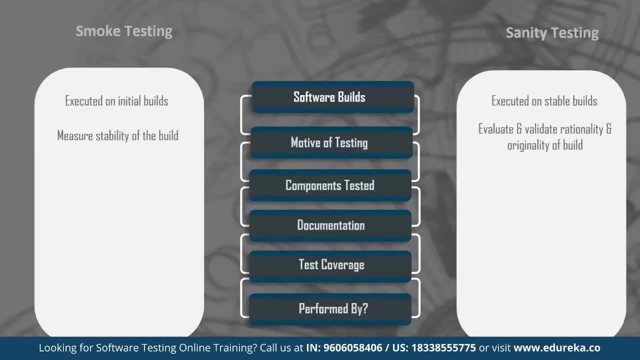 So the objective here are in the Sanity testing is to verify the rationality and the originality of core functionalities to proceed with further rounds of testing. talking about competent tested, throughout the session I've been telling that smoke testing is performed from end to end, that a sanity testing is a narrow testing. 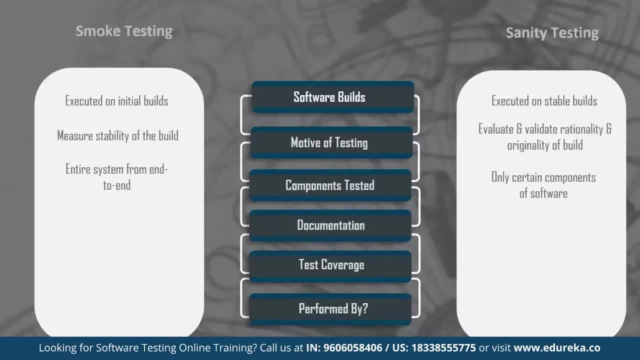 which is performed only on limited functionalities or you can say, certain components of software that's required. next up is documentation. usually smoke testing is documented and well scripted, compared to Sanity testing where, as Sanity testing is not that documented and it's usually not scripted at all, test coverage- smoke testing. 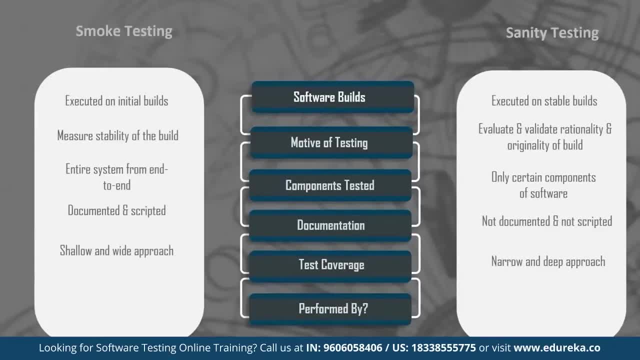 is shallow and wide approach to include all the major functionalities without getting into detail. Well, it may be seen as a general type of testing covering all basic functionalities, but Sanity testing is a narrow and deep approach involving detailed testing of functionalities and features. It's more focused on certain features rather 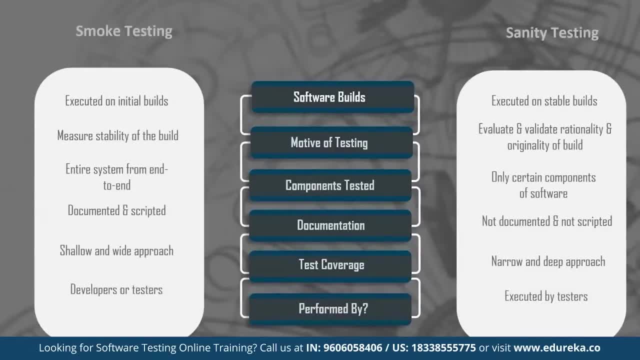 than from end to end and, lastly, performed by. smoke testing is usually performed by developers as well as testers, because it's usually performed on initial bills and initial bills are passed on from developers to testers and it's quite possible that sometimes developers themselves perform the smoke testing. 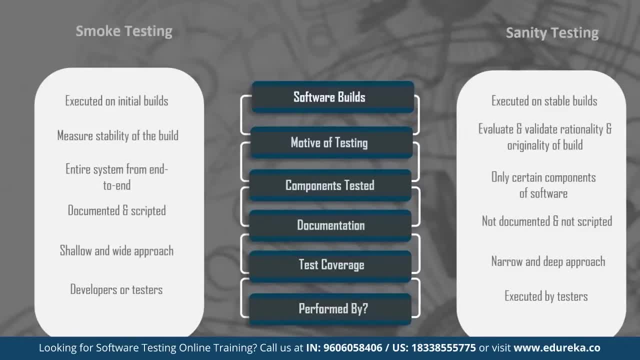 before sending it to testers. But when it comes to Sanity testing, it's usually done in between the development of software product as a not on the initial bills, So it's usually executed by the testers. Well, that's it, guys. with this we have come. 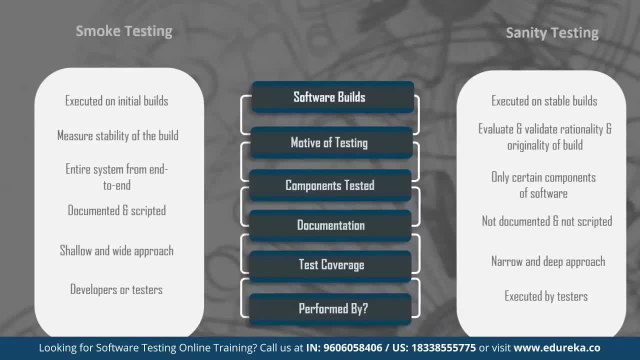 to the end of the session, So let's wrap up the discussion and quickly take a recap of what we have discussed so far. Well, we did discuss what Sanity testing is. It is a tool to tell whether your software release meets the merit to go to further rounds of testing. 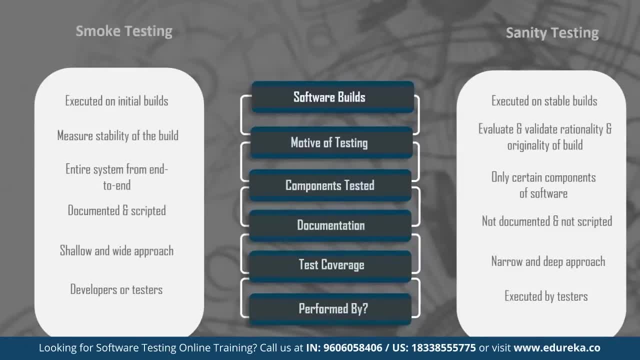 or it's too flawed to be tested. It's performed in a new functionality. change request or buff fix is implemented in the code. Its scope is narrow and it's focused on only functionalities that have been implemented or impacted by the change. and, lastly, many people confused. 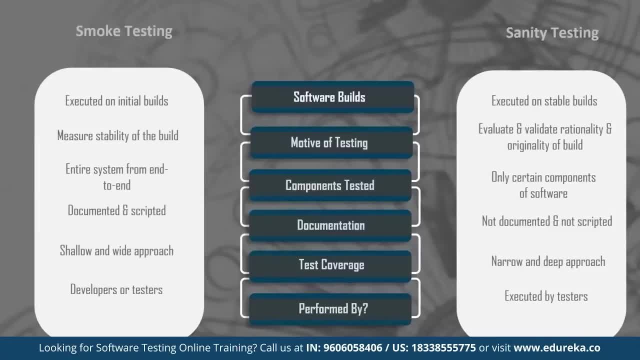 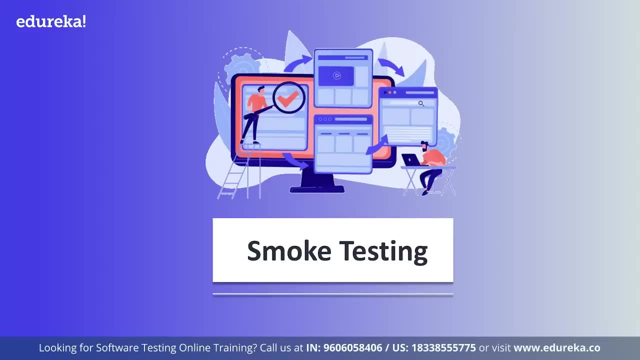 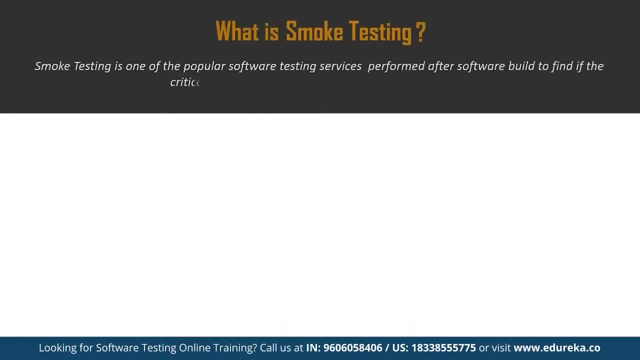 between Sanity testing and smoke testing. So we did discuss the key differences between them. So smoke testing is a high-level test performed on initial software build to make sure that the critical functionalities of the software or the application that you're testing on is working properly. 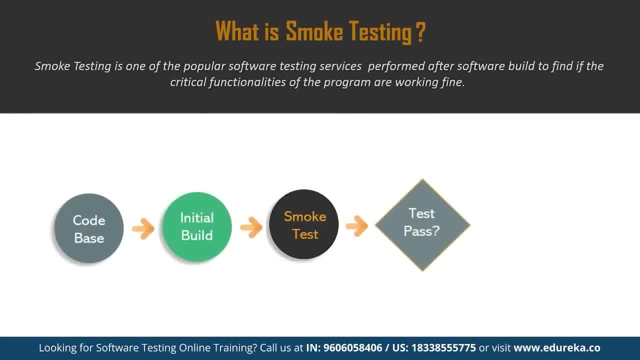 It is executed before any detailed functional or regression test are executed on that particular software built. So the process of smoke testing targets all key features and it's often considered a cost-effective approach because you're just checking the basic functionalities and you do not have to spend much effort, time and cost on that. 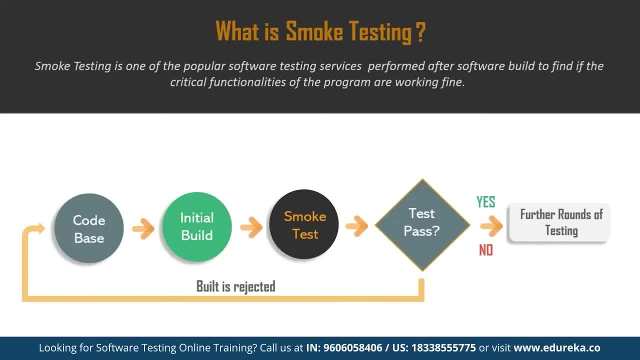 So if key features are in walking or major bugs haven't been fixed, There's no reason to waste time and further rounds of testing light. So smoke test should be scripted. this ensures that you're touching all the major components of the software and no key. 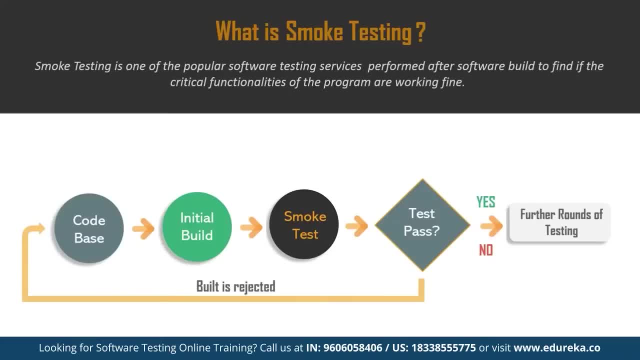 Features or the core functionalities are missed by you and most of the time all the high-quality smoke tests share common characteristics and area of coverage. like it involves clicking or navigating through many, or sometimes all, screens of an application, testing the key functionalities, such as sign-up forms, adding 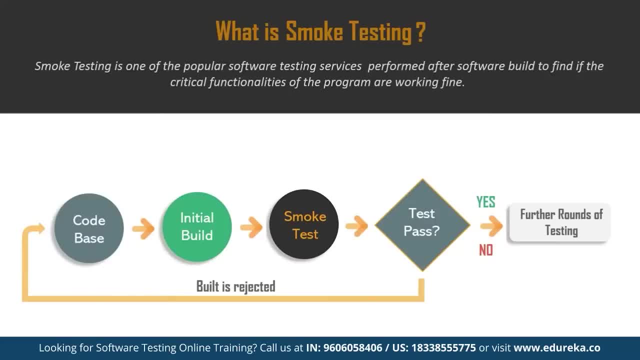 to the shopping cards, exporting files, moving data and rest of other things, verifying correct layout of the graphical user interface and visual correctness. So all these are the basic features which we check during any smoke test. but it's optional that even after checking these features, you can add on other features to check. 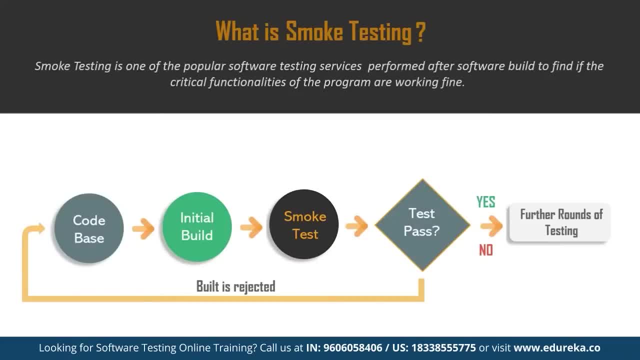 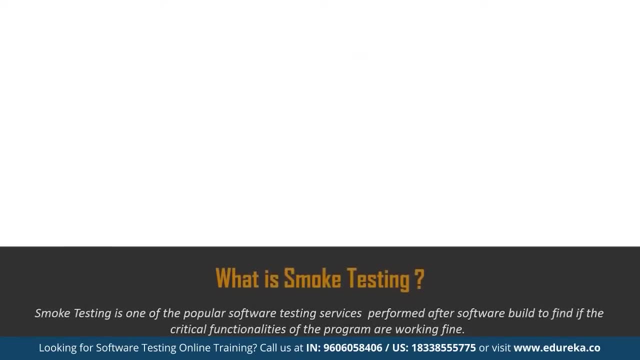 on according to your requirements. But the question here is: how important are these? smoke test. Let's consider a simple example to understand smoke test. Suppose if you're given a Gmail application to test what are the important functions that log into Gmail, compose, main and set correct. 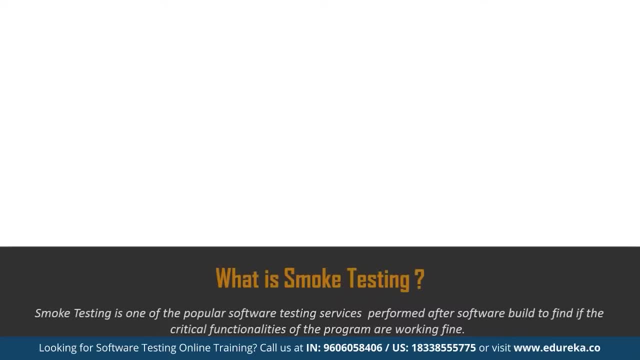 Yeah. So, for instance, if there's an error in sending an email, does it make sense for you To test sent mail drafts, folders and other features? no, right, which means you are rejecting the build without further testing or without testing other functionalities. That's because your basic functionality 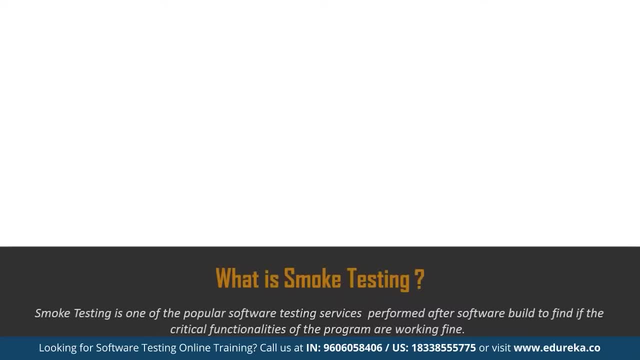 or the core functionality of your application is not working properly. That's what smoke testing is all about. Of course, thoroughly testing your application is really important for ensuring the good quality, but performing a suit of smoke test is even more important, since it's sensible to get answer to preliminary questions. 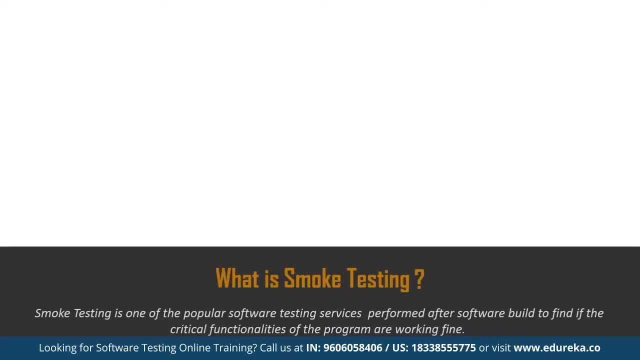 like can the application that you're testing will be successful without any error. Does the login process function correctly? What happens when you click on the primary buttons or the menus? So a major benefit of running the smoke test is that it provides quick feedback within a matter of few minutes. 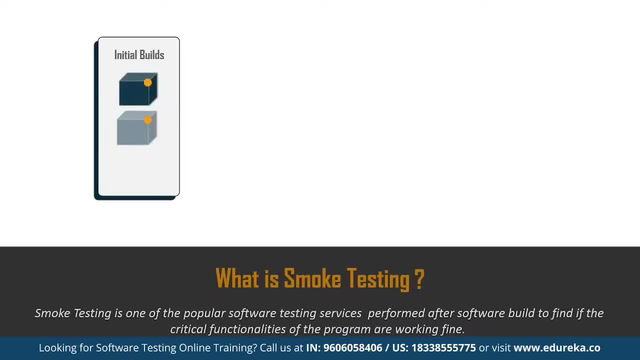 and, as a tester, you do not have to wait for house to get the results. as you can see, I have like about three bills on the screen and I want to check the functionality of my last bill, So I have subjected it To smoke test. if all the functionalities are working well. 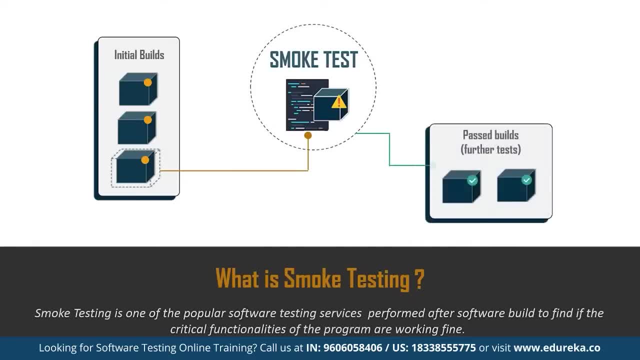 as an. if it passes the smoke test, it will be passed on to next rounds of testing. If it doesn't, the bill is either rejected or it's subjected for further development to remove the errors or the bugs that we have fun. So that's what smoke testing is all about, guys. 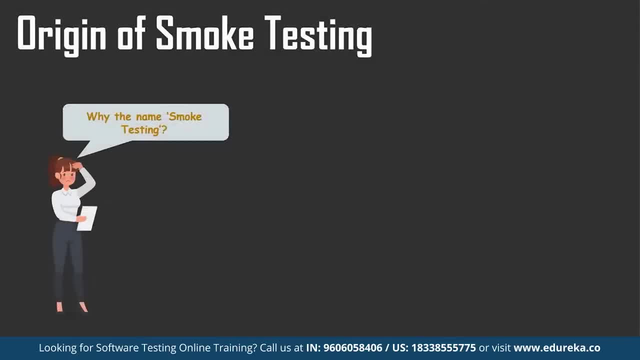 Have you ever wondered why the name smoke testing? since smoke testing came into existence? There are a lot of theories and studies associated with the nomenclature. However, out of all this, only two of them seem appropriate. One theory is that, according to Wikipedia, 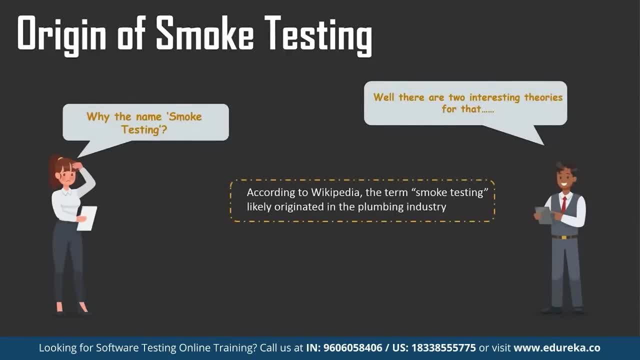 the term smoke testing likely originated in the plumbing industry. plumbers would use smoke to test for leaks and cracks in the pipe systems. Sometime later, the term was applied to testing of electronic things as well. Another theory states that the term smoke testing is originated. 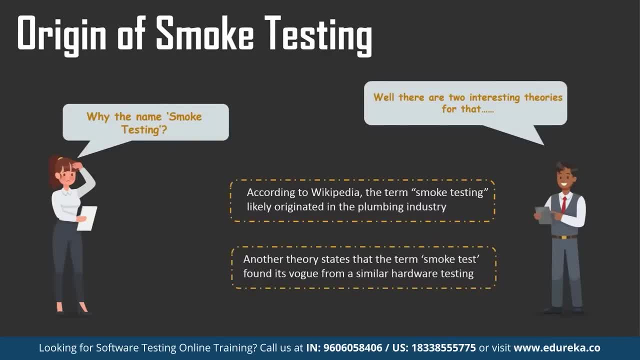 from hardware testing, where a device, when first switched on, is tested for the smoke or the fire from its components, like power device, and if you see a smoke, then well, that's bad right. So these are like the two most popular theories about a smoke testing. 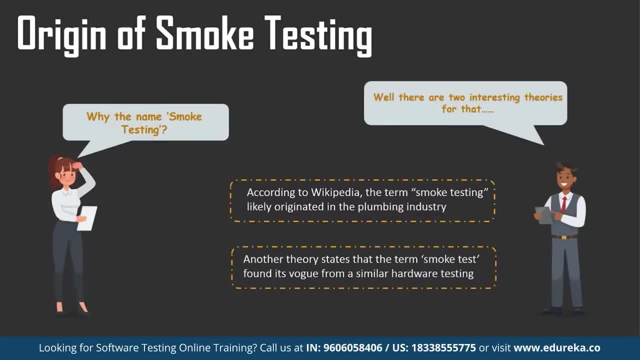 But today the concept of smoke testing is widely used in software development. Well, actual smoke may not be involved. the same principles are applied in smoke testing software as well. but to get a better insight into this process, It's important for us to understand various features. 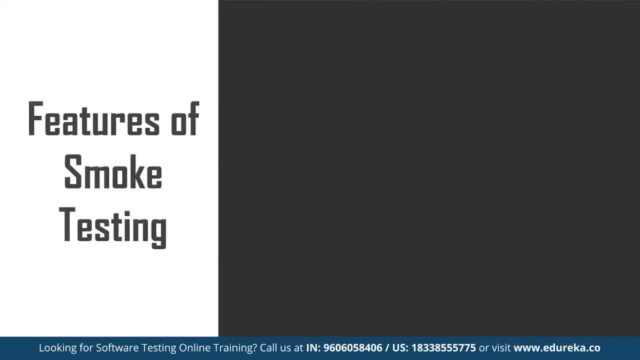 of smoke testing. So let's go ahead and check them out. First of all, smoke testing is often referred to as build verification testing. So next time you hear someone telling build verification testing, it's nothing but smoke testing, It's known as build verification testing. 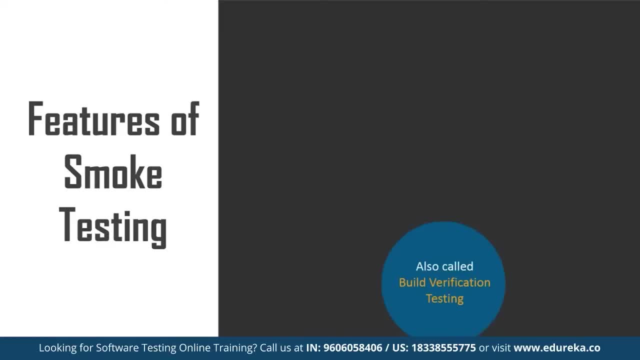 or build acceptance testing, where the build is verified by testing the important features of the application and declaring it as good for further detailed testing. It delivers quick and decisive answers on the viability of the particular build that you're testing on smoke testing is an integral part of the software development life cycle. 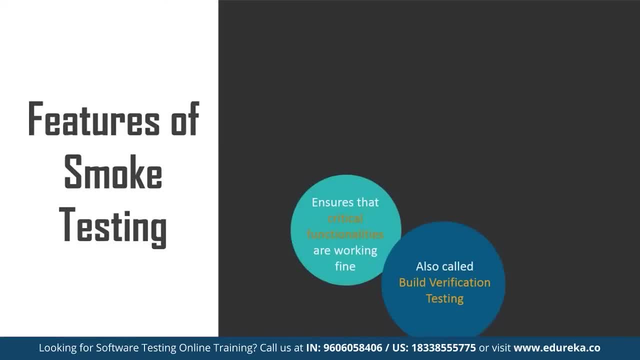 which ensures that the critical functionality of an application are working well and fine. this you already know, because that's the main definition, or the concept or the objective of smoke test. as smoke testing decides the path of the build for further testing process, It's often referred to as intake test. 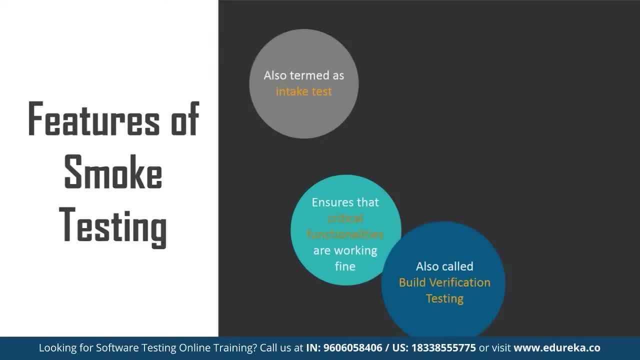 So, with the help of automation, test, developers can check built immediately whenever there's a new build ready for deployment. smoke testing can be done manually or it can be automated. Usually it's the testing team begins manually and then later on they automate the entire process. 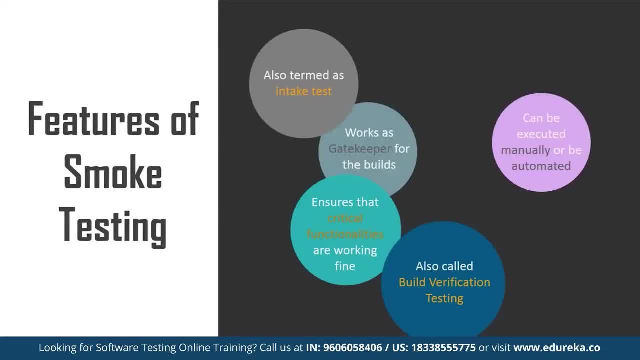 It also works as a gatekeeper to accept or reject the build based on its stability to undergo through further rigorous and in-depth testing activities. So you can say it's called build verification test or build acceptance testing. It ensures critical functionalities are working fine. 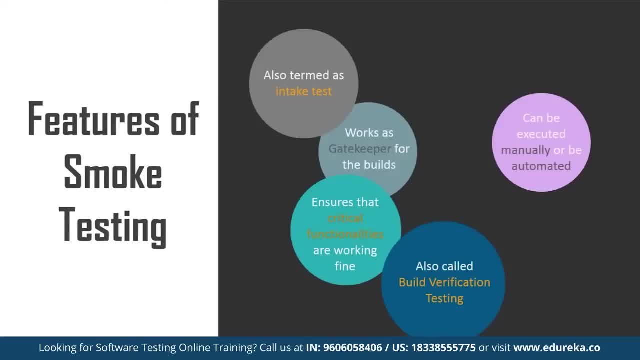 It can be referred to as intake test because it decides on the next level of testing. It's often refers to as gatekeepers- well smoke testing, as you guys know, as subset of regression testing. but it's not a substitute for regression testing and it's applicable to different levels of software testing. 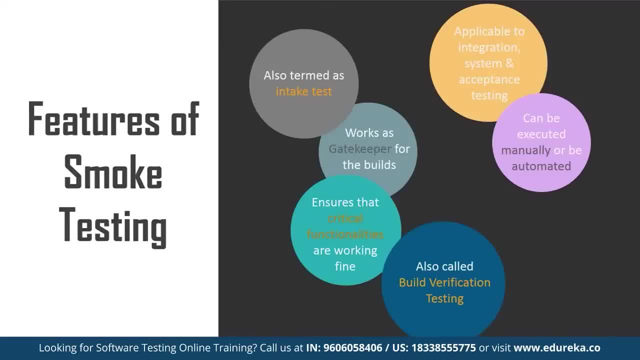 like integration testing, system testing and acceptance testing as well. Finally, it's a non-exhaustive testing with very limited number of test cases. You don't do testing here very deeply, You just check the basic functionalities, and usually smoke testing is performed with positive scenarios and with valid data. 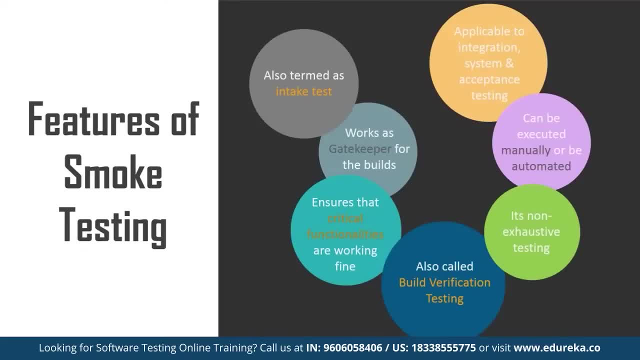 and then that process is usually documented for referring later on. So these are the basic features. Well, in conclusion, you can think of smoke testing as a normal health check on the build of an application. So, guys, now that we're aware of what smoke testing is, 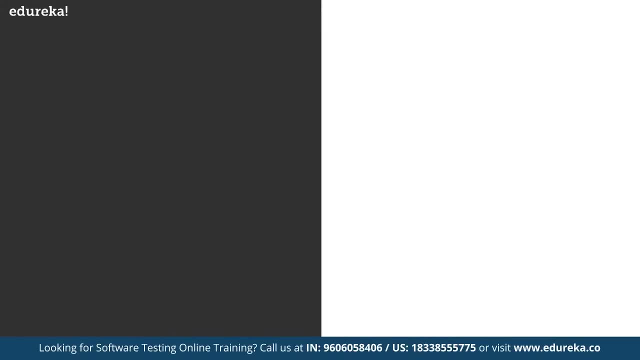 and its key features. Let's go ahead and answer some important questions about smoke testing. Well, the first question is: when is the right time to perform smoke testing, or when do we do smoke testing? First of all, smoke testing is done whenever the new functionalities of the software are developed. 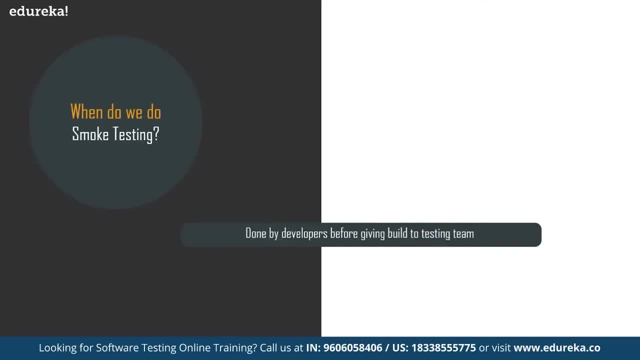 and integrated in the build that's developed in QA team. It ensures that all critical functionalities are working correctly or not. It is done in a development environment on the code to ensure the correctness of the application or the build before releasing it to QA team. 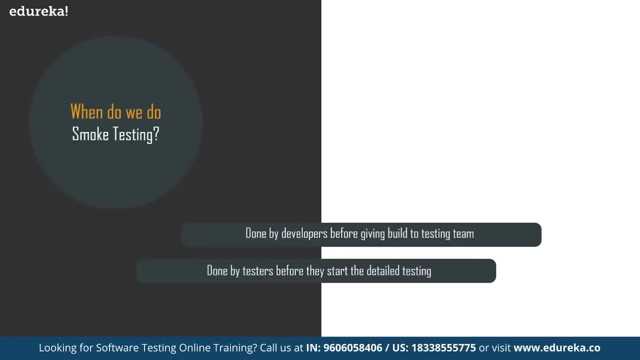 After the build is related to QA environment. smoke testing is performed by QA engineers or QA lead. So whenever there's a new build, QA team determines the major functionality in the application to perform smoke testing. These actually answers our second question as well, which is: who performs smoke testing? 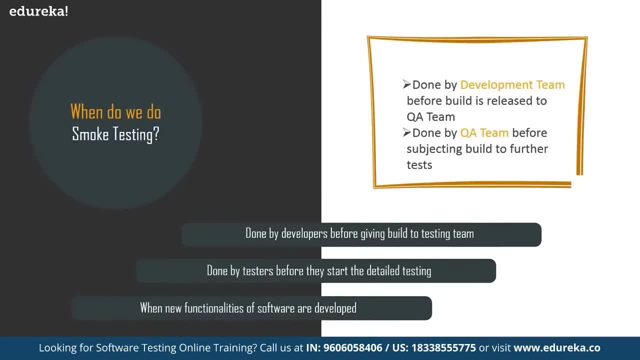 Like I said, it's done by development team before build is released to QA team. It's done by QA team before subjecting the build to further rigorous testing. So smoke testing, basically, is performed either by developers or testers, or both sometimes. Moving on to our next question, 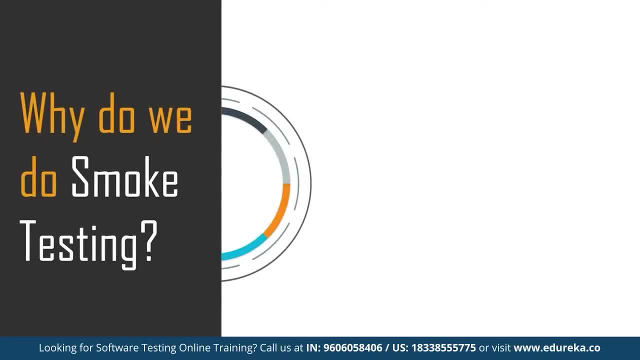 Why to do smoke testing? What are the benefits or advantages of performing smoke testing? Smoke testing offers various advantages to team of testers and allows them to effectively evaluate various aspects of the software. So let's check out what those benefits are. First of all, it helps you in finding the bugs. 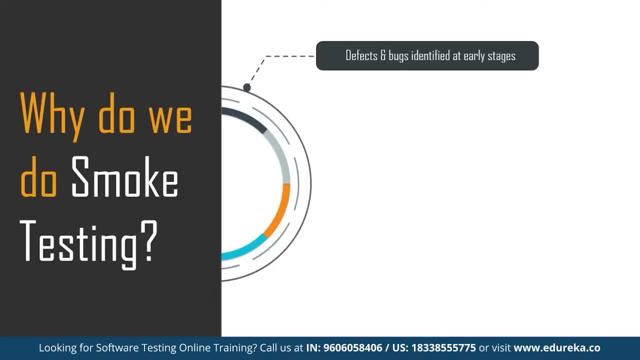 and defects in the early stages of testing itself. You can uncover and fix as many as 80% of the bugs that discover simply by configuring or executing a simple smoke test. So with smoke test you might be covering only 20% or less than that of your test cases. 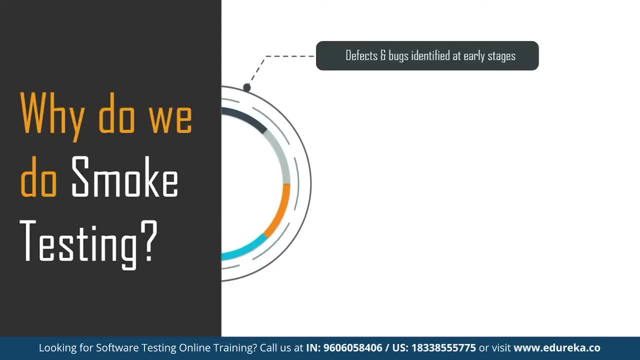 and yet you can catch up to 80% or more of the box. Secondly, it minimizes the integration risk and help in finding the issues that get introduced. whenever you integrate the components of the unit testing, Smoke testing can be carried out in small time. 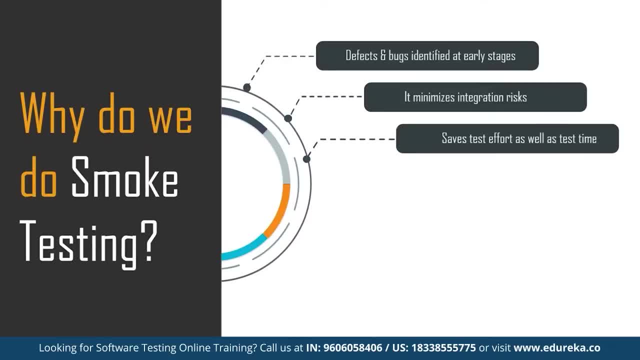 It can be executed within few minutes for every particular build. Smoke testing also improves the effectiveness of the QA team. Instead of spending and wasting test cycles by attempting to run a large test suit when there are issues, QA team can simply opt for smoke testing. 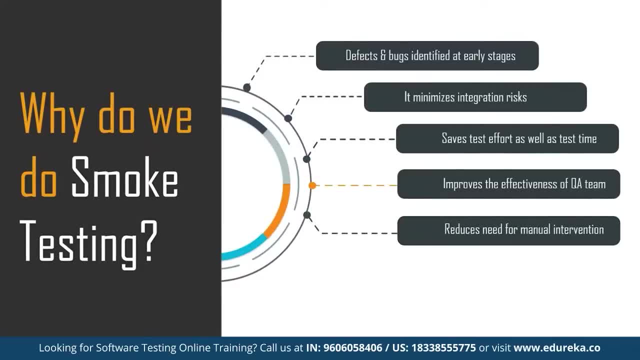 Smoke testing also reduces the manual intervention because you can easily automate the entire process and the test cases are not many here. It helps in verifying the issues fixed in the previous build and not affecting the major functionality of the application currently. This way, it improves the quality of the system. 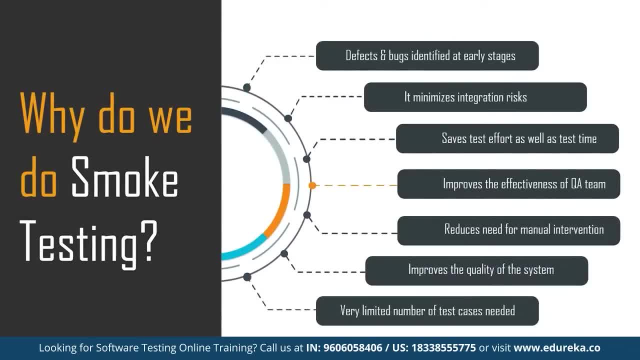 that you're testing on as well. And lastly, very limited number of test cases are needed to perform smoke testing, and it also offers the advantage of getting faster feedbacks, as it's frequently run very quickly. So these are the advantages Let's list out. 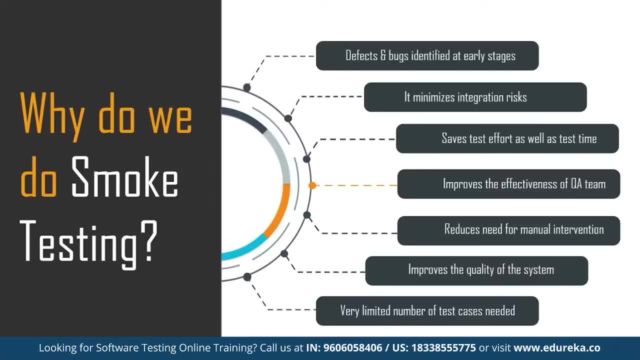 First of all, you can find defects and bug in the early stage of testing. Integration risks are reduced when the components are combined. There's no need for manual intervention. You can opt for automation. It improves the effectiveness of your QA team. It saves a lot of time and effort on testers part. 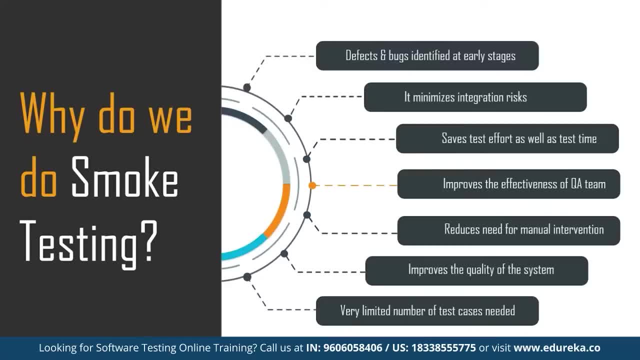 It improves the quality of the system as a whole and, the most important thing, is very limited number of test cases are needed to perform smoke testing of entire application. So smoke test, take your code, build it, run it And verify a thing or two. They will not verify. 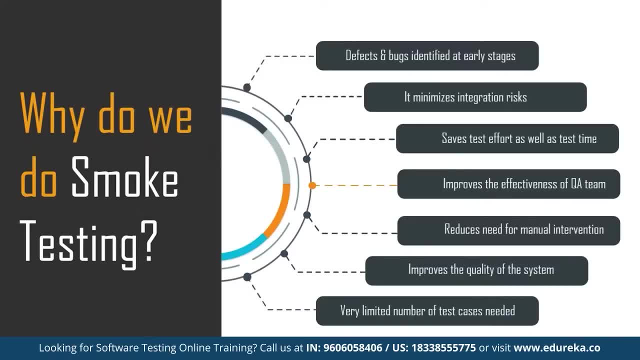 that your software is under percent functional or not in a production app. They will act as a quick bailout. If the smoke test fails, then the whole build is failed and the entire process is so quick that you do not have to waste a lot of amount of time here. 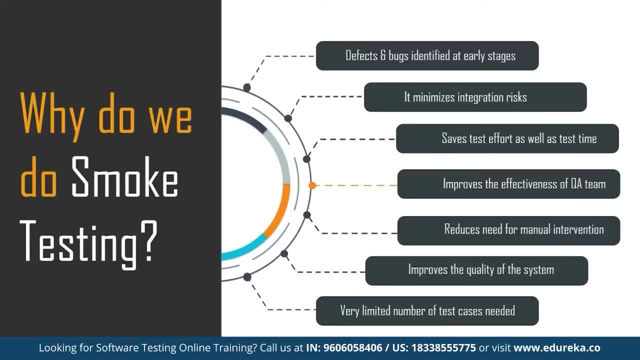 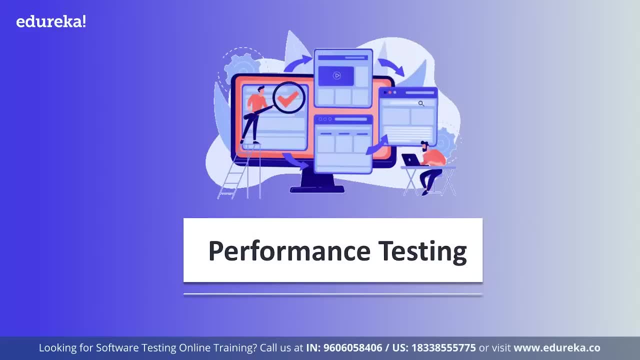 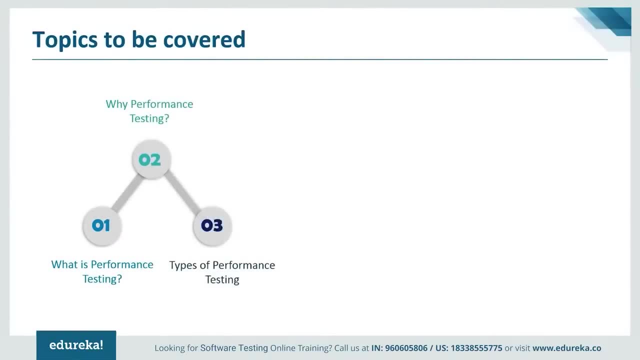 So my point is that for a simple application, smoke test is often all you need. First, I will talk about what is performance testing And why it is important. next I will discuss different types of performance testing and will also tell you some of the common problems. 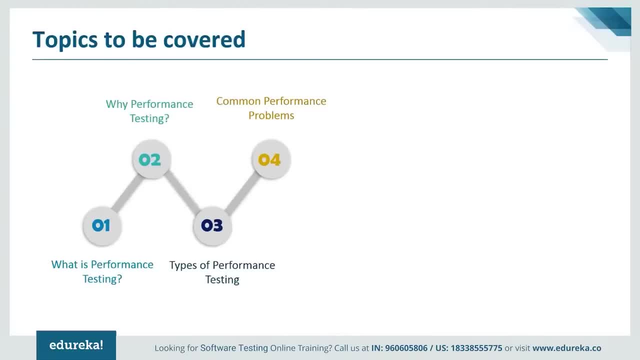 that are faced while performing performance testing. and moving further to the discussion, We'll see in depth about the process of performance testing and once you understand the performance testing process, then I will tell you some metrics used for performance testing. After that we'll see some example test cases of performance testing. 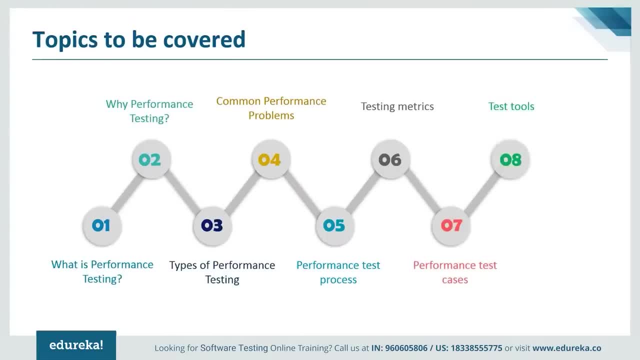 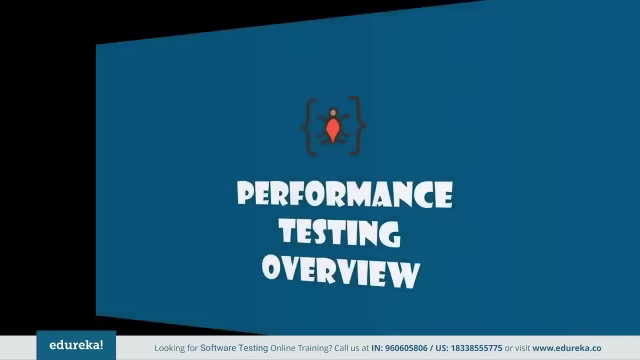 and finally, I will wrap up the session by talking about the tools used for performance testing and why Jmeter is considered as a preferred tool for performance testing. So these are the topics that we will be covering in today's session without any further ado. Let's get started first. 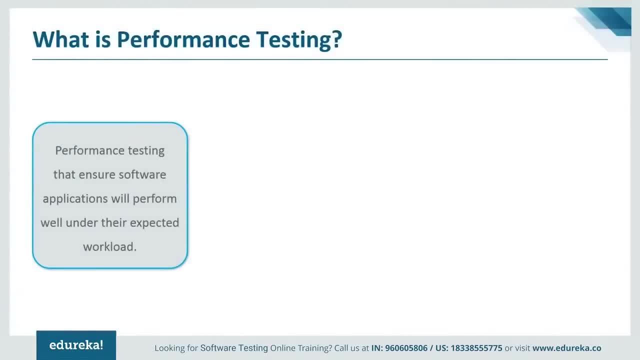 Let's understand what performance testing is. performance Testing is defined as a type of software testing to ensure software applications will perform well under their expected workload. features and functionality supported by a software system is not the only concern a software applications performance, like its response time, reliability, source usage, scalability, do matter a lot. 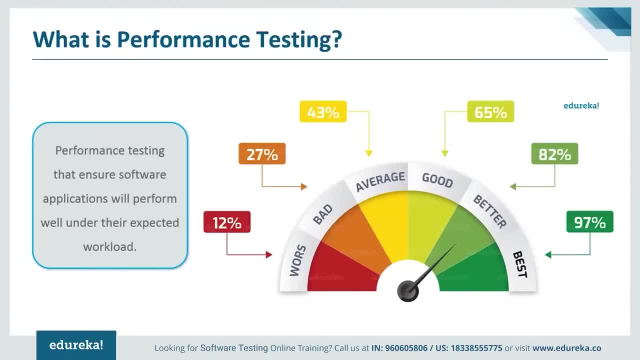 The goal of performance testing is not to find bugs but to eliminate the performance bottlenecks, and the main focus of performance testing is to check a software program speed, scalability and stability. Performance testing is popularly called as perf testing as a subset of performance engineering. 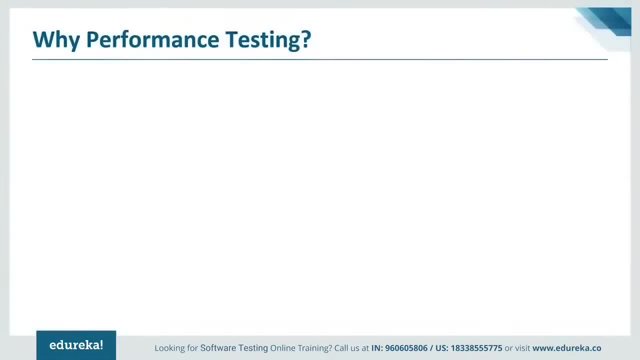 So why do we need performance testing? performance testing is done to provide stakeholders with information about their application regarding speed, stability and scalability. more importantly, it uncovers what's need to be improved before the product goes to the market. without performance testing, software is likely to suffer from issues such as running low while several users use it. 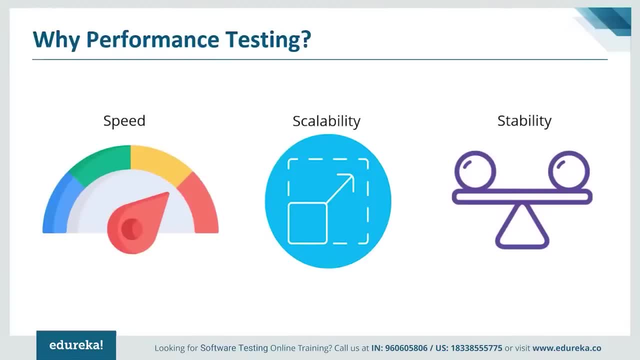 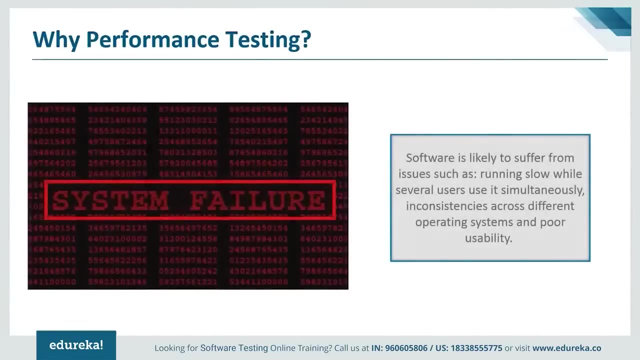 simultaneously. inconsistencies across different operating system and poor usability and performance testing will determine whether the software needs speed, scalability and stability requirements under expected workloads. applications sent to market with poor performance metrics due to non-existence or non-performance testing are likely to gain a bad reputation. 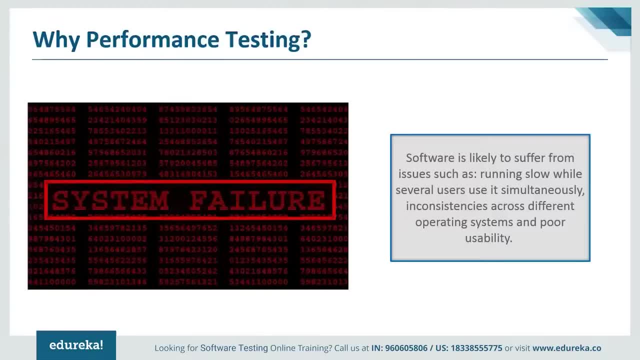 and fail to meet expected sales goals. Also, mission-critical applications like Space Launch programs or life-saving medical equipment should be performance tested to ensure that they run for a longer period without deviations, and that's why performance testing is more essential. having understood this now. 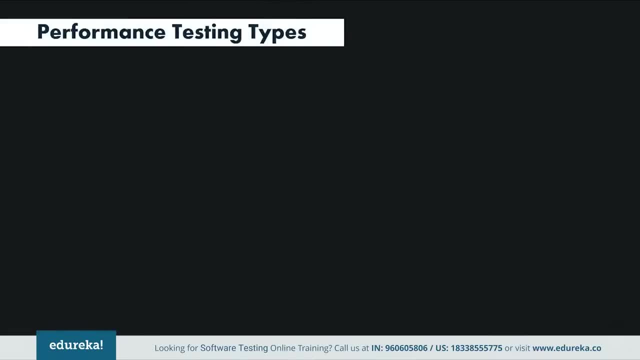 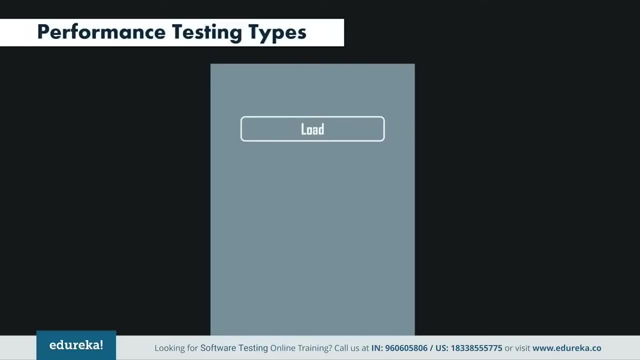 Let's move further and see different types of performance testing. first, load testing. It checks the application's ability to perform under anticipated user loads. The live objective is to identify performance bottlenecks before the software application goes live. Next, stress testing. this involves testing. 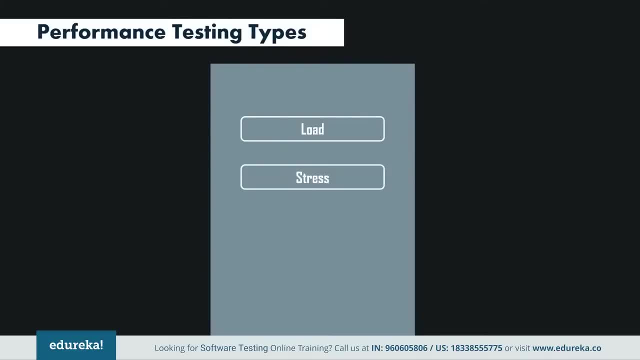 an application under extreme workloads to see how it handles high traffic or data processing. The objective is to identify the breaking point of an application. next, endurance testing. This is done to make sure that the software can handle the expected load over a long period of time. 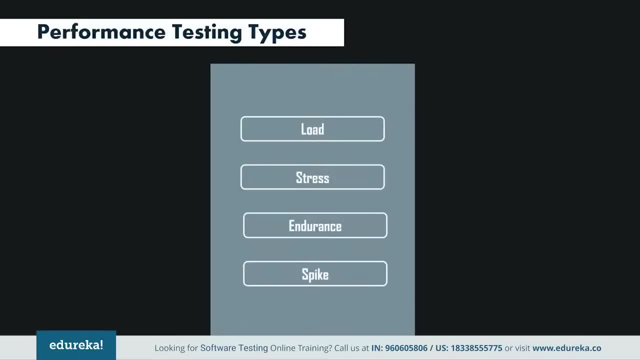 and next we have spike testing. This is used to test the software's reaction to sudden large spikes in a load generated by the users. And also we have volume and scalability testing as a type of performance testing. Now let's move further and see some of the problems. 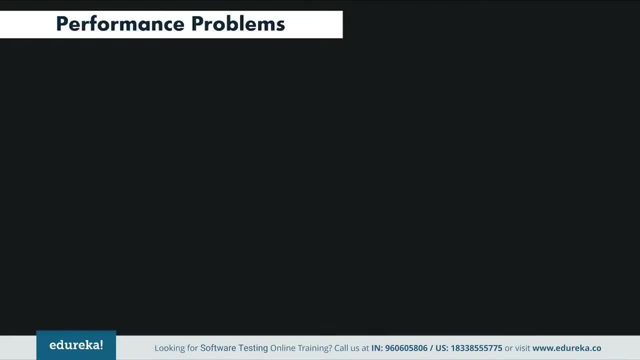 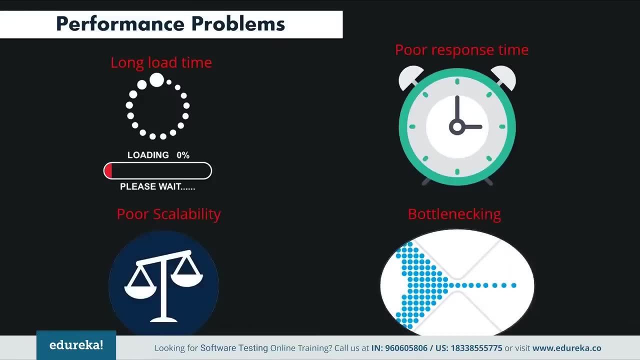 caused by performance testing. Most of the performance problem revolve around speed, response time, load time and poor scalability. Speed is often one of the most important attributes of an application. A slow running application will lose potential users. Performance testing is done to make sure an application 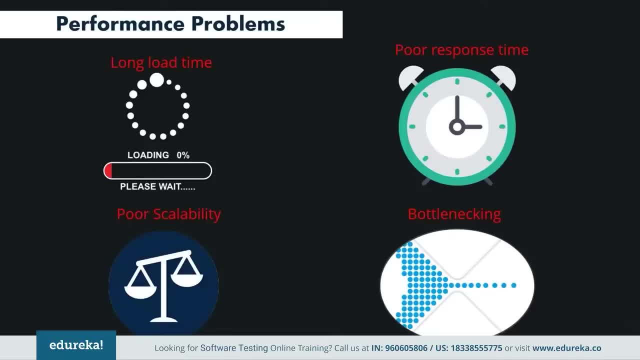 runs fast enough to keep a user's attention and interest. So these are some of the four main factors. that is, long load time, poor response time, poor scalability and bottlenecking. So first let's see what is long load time. Load time is normally the initial time. 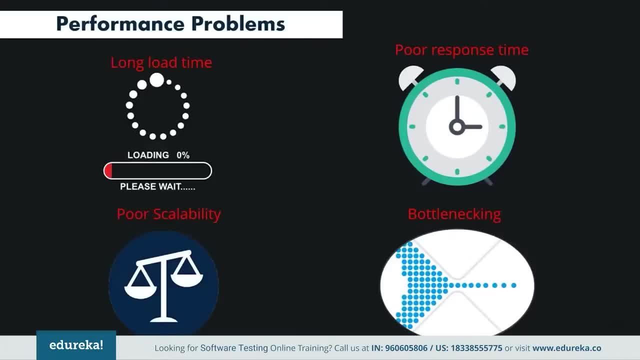 it takes an application to start. This should generally be kept to a minimum. while some applications are impossible to make it load in under a minute, and load time should always be kept to a minimum, It should be kept under a few seconds if possible. Now talking about the poor response time. 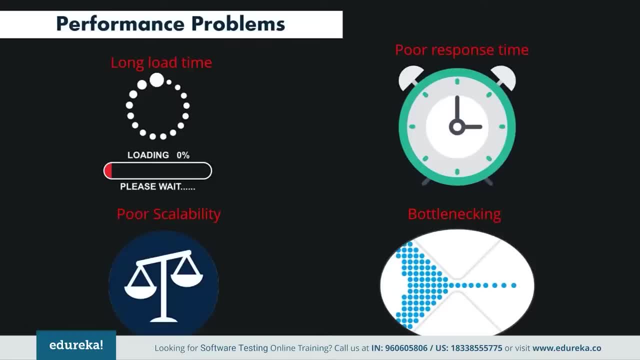 it is the time that takes from when a user inputs data into the application until the application outputs a response to that input. Generally, this should be very quick. Again, if a user has to wait it too long, they lose the interest. A software product suffers from poor scalability. 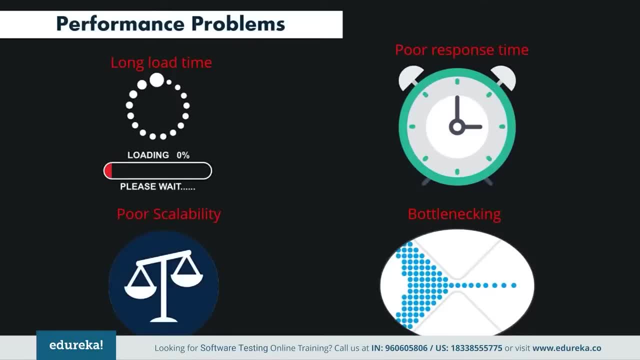 when it cannot handle the expected number of users or when it does not allocate a wide range of users. And last, bottlenecking: Bottlenecks are obstructions in a system which degrade overall system performance. Bottlenecking is when either coding errors or hardware issues cause a decrease. 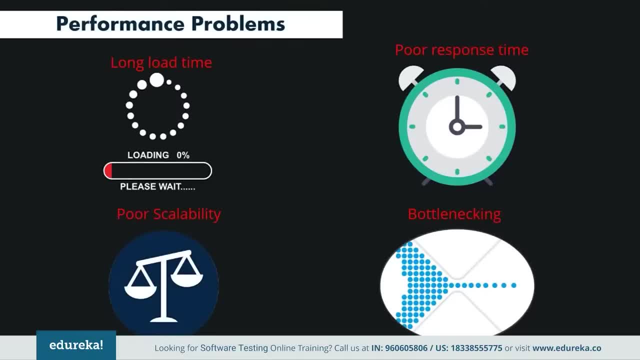 of throughput under certain loads. Bottlenecking is often caused by one faulty section of code. The key to fixing a bottlenecking issue is to find the section of code that is causing the slowdown and try to fix it there Bottlenecking is generally fixed. 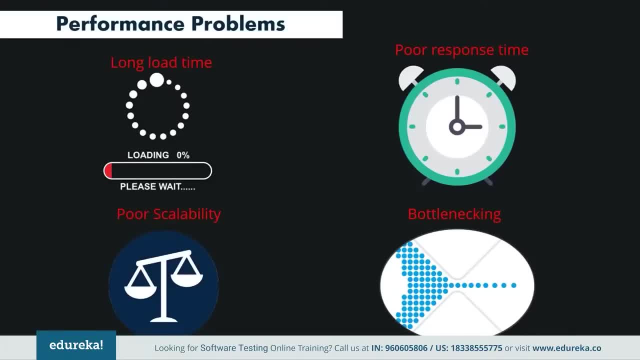 by either fixing poor run processes or adding additional hardware. Some of the common performance bottlenecks are CPU utilization, memory and network utilization, disk usage and operating system limitations. So these are some of the performance problems that should be handled then and there. 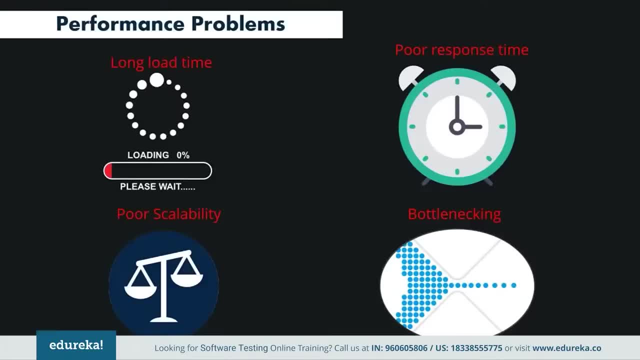 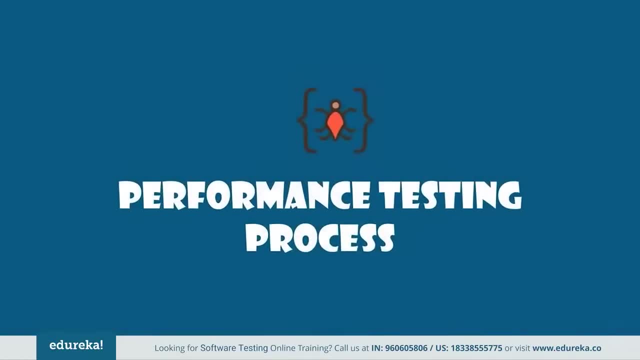 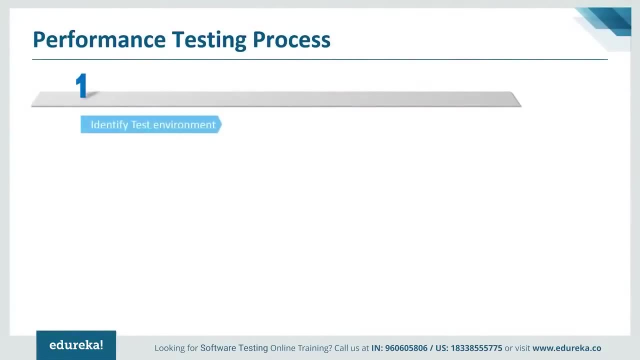 Else, they might lose potential users and also it may cause some failures as well. Now let's move further and see the performance testing process. This is a generic process on how to perform performance testing, So there are various stages involved. First one is identify your testing environment. 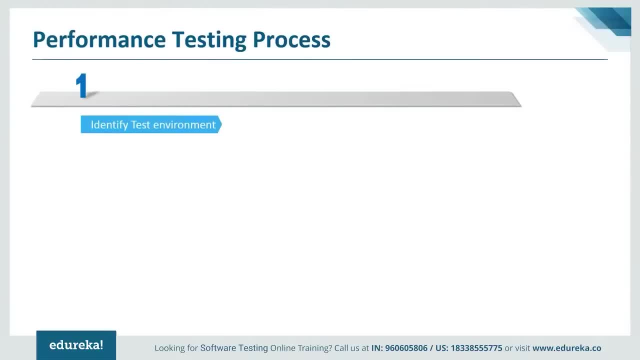 So, basically, you should know your physical test environment, production environment and what testing tools are available, and you should also understand the details of the hardware, software and network configurations that are used during testing, before you begin the testing process, and it will help the testers to create more efficient tests. 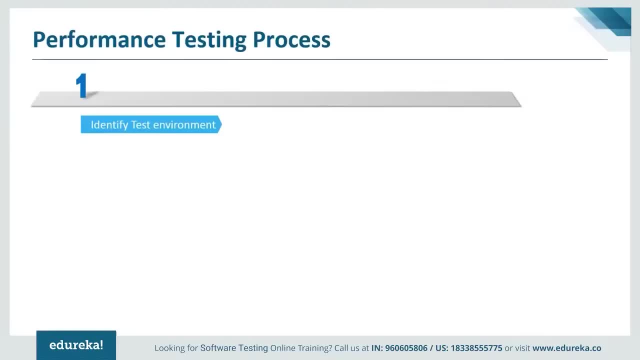 It will also help to identify the possible challenges that testers may encounter during the performance testing procedures. Next, identify the performance acceptance criteria. This includes goals and constraints for the throughput, response time and resource allocation. It is also necessary to identify projects, such as criteria, outside of these goals and constraints. 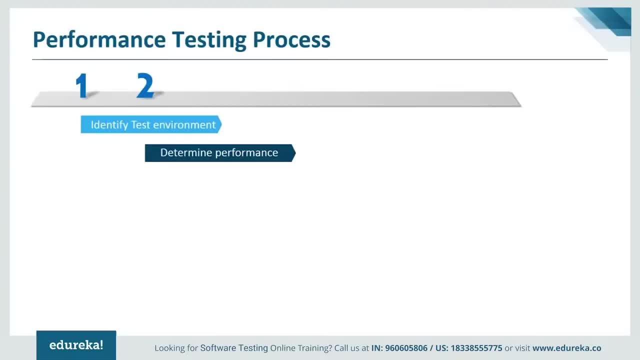 Tester should be empowered to set performance criteria and goals, because often the project specifications will not include a wide enough range of variety of performance benchmarks. Now talking about the next stage, that is, plan and design performance test. Here you have to determine how usage is likely to vary amongst end users. 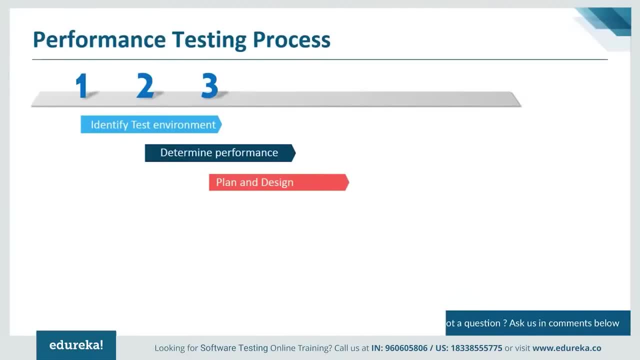 and identify key scenarios to test for all the possible use cases. It is necessary to simulate a variety of end users, plan performance test data and outline what metrics will be gathered Next, configuring your test environment. So in this phase you have to prepare. 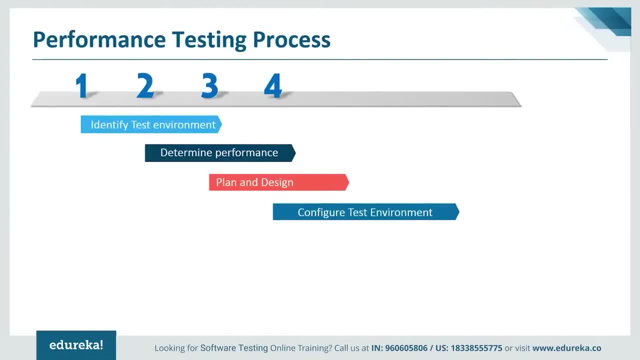 the test environment before execution. Also, you have to arrange the tools and other resources as well. Next, implement test design and run the tests. So, basically, you have to create the performance test according to your test design and execute and monitor the test. and last step is to analyze, fine-tune and retest. 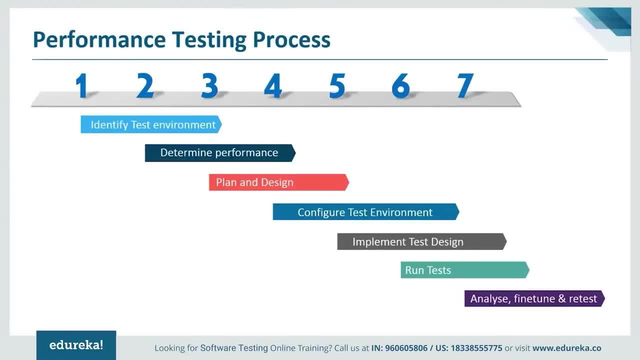 So in the last step you have to consolidate, analyze and share test results. After that you have to fine-tune and test again to see if there is an improvement or decrease in the performance, Since improvements generally grow smaller with each retest. 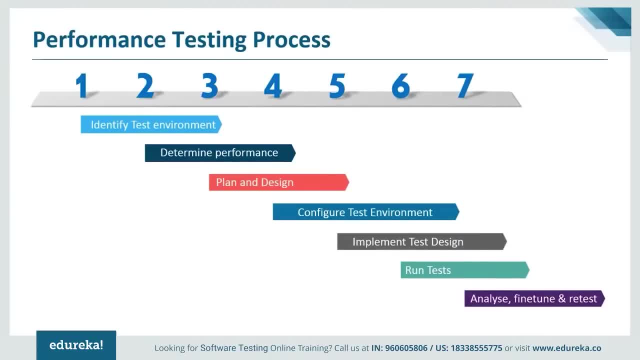 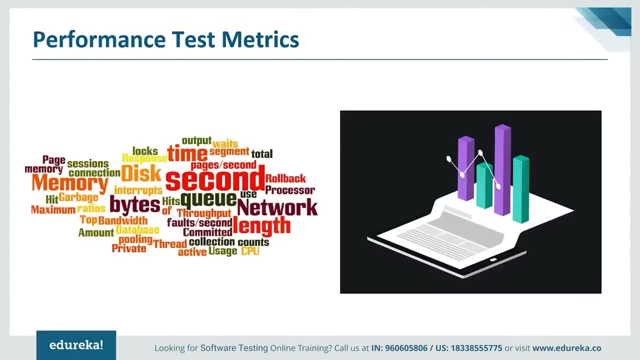 stop when bottlenecking is caused by the CPU. Then you may have the consider option of increasing the CPU power. So these are the various steps that are involved in performance testing process. Now let's move further and understand some important test metrics. So you can see in this figure: 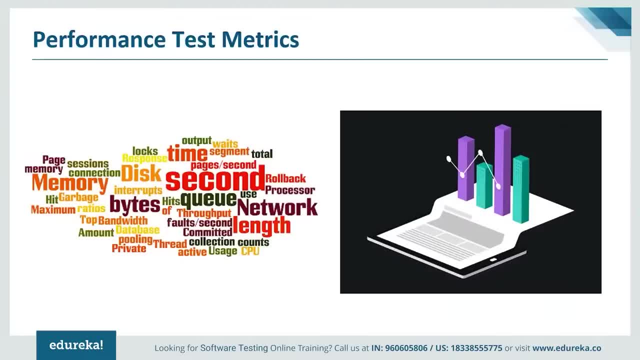 that it comprises of memory, second network length, throughput, thread active time, many more right. So I will explain you few of the important concepts, like processor usage, That is, an amount of time that processor spends on executing non-idle threats. 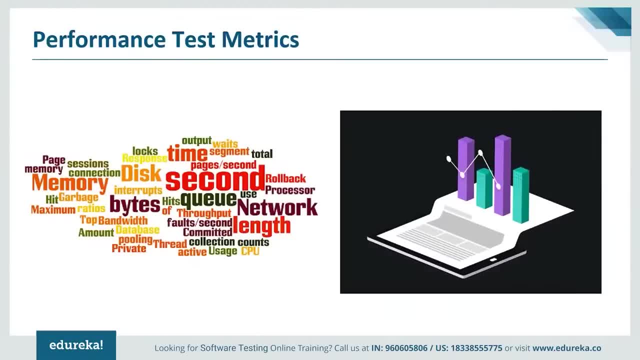 Next, memory usage, That is an amount of physical memory available to process on a computer. Next, disk time: That is the amount of time disk is busy executing a read or write request. And also there are many more like top bandwidth, CPU collection counts. 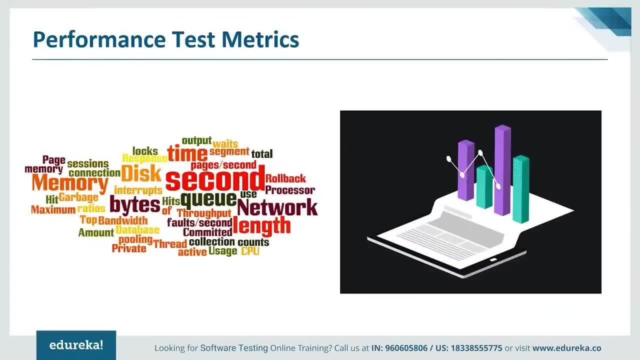 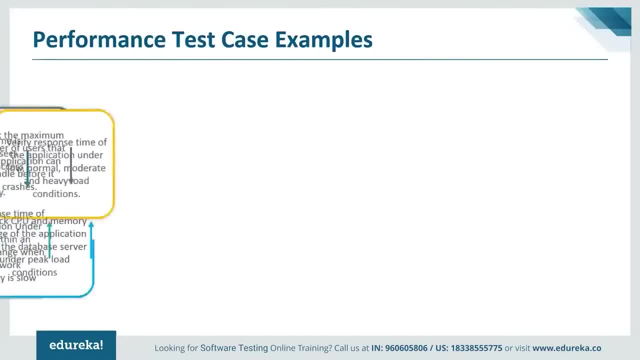 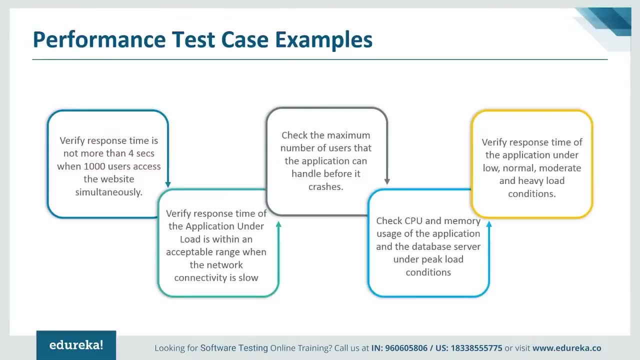 rollback processor, etc. Having understood this, let's move further and see some of the examples of performance test cases. So some of the examples are: you have to verify that response time is not more than 4 seconds when thousands of users access the website simultaneously. 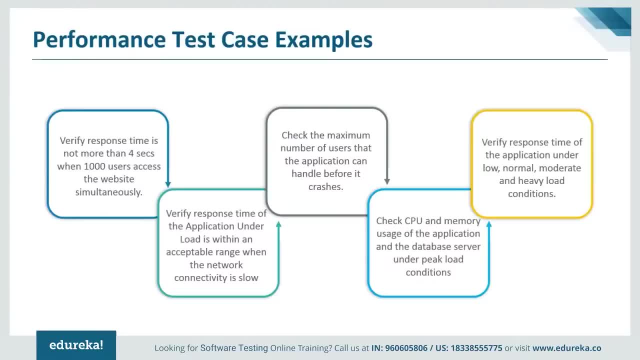 And you should also verify the response time of the application under load is within an acceptable range when the network connectivity is slow. Next, you have to check the maximum number of users that the application can handle before it crashes and also check the database execution time when 500 records are read and written simultaneously. 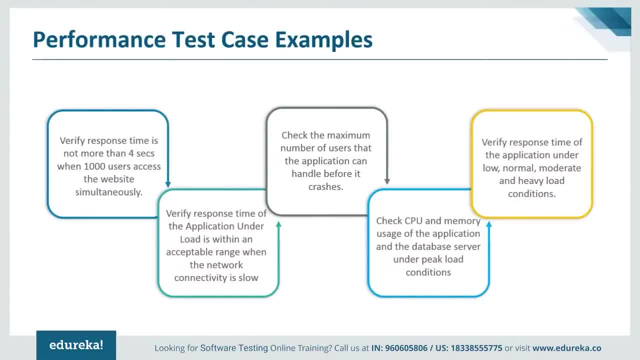 Also check CPU and memory usage of an application and the database server under peak load conditions and you have to verify the response time of the application under low, normal, moderate and heavy load conditions During the actual performance test execution. vague terms like acceptable range. 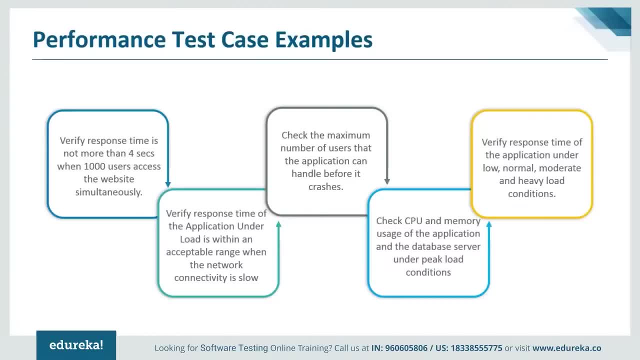 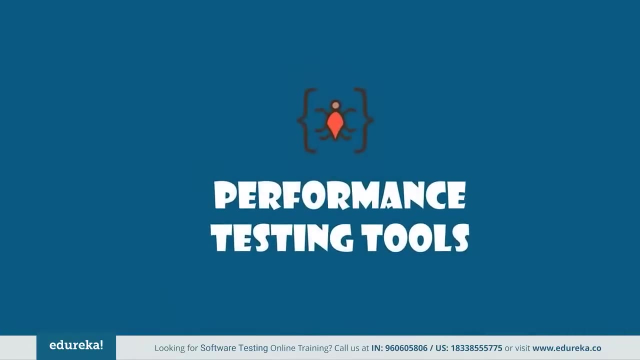 heavy load are replaced by concrete numbers. Performance engineers set these numbers as per business requirements and the technical landscape of the application. So these are some of the examples of performance test cases. Having understood this, now let's move further and see some of the performance testing tools. 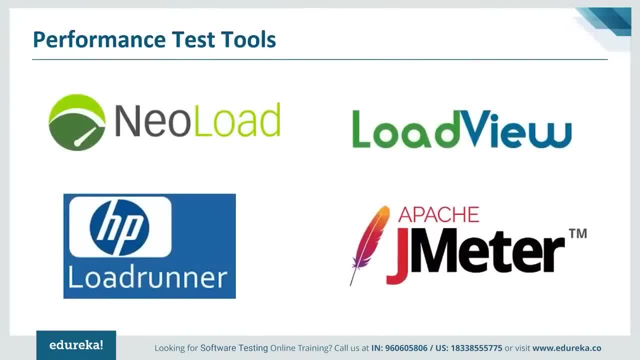 There are a wide range of performance testing tools available in the market. The tool you choose for testing will depend on many factors, such as types of protocol, supported license, cost, hardware requirements, platform support, etc. So these are the four main used tools. 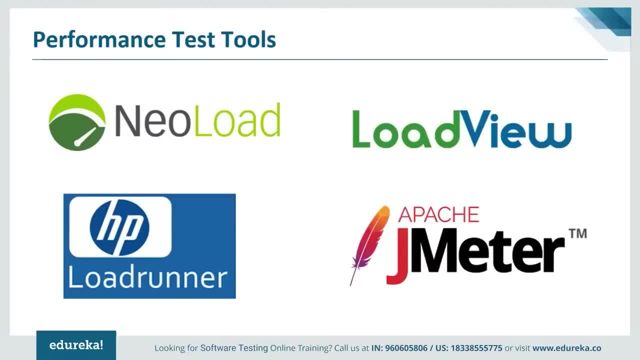 like NeoLoad. that is the performance testing platform designed for DevOps that seamlessly integrates into your continuous delivery pipeline. With this tool, teams test up to 10 times faster than with the traditional tools to meet the new level of requirements under full agile software development lifecycle. 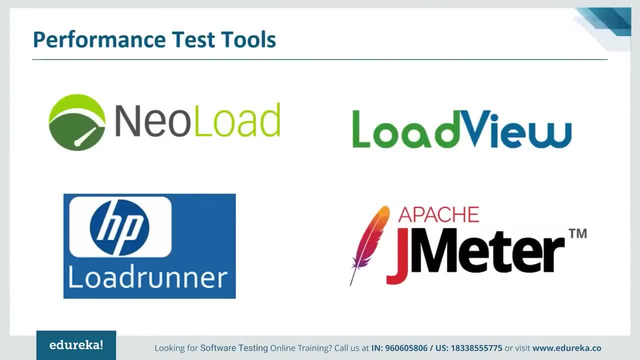 from component to full system wide load tests. Next, LoadView testing. This is used to test your infrastructure at any scale, from small targeted test to millions of users, and to find performance bottlenecks and adjust your capacity plan accordingly. LoadView offers on demand. 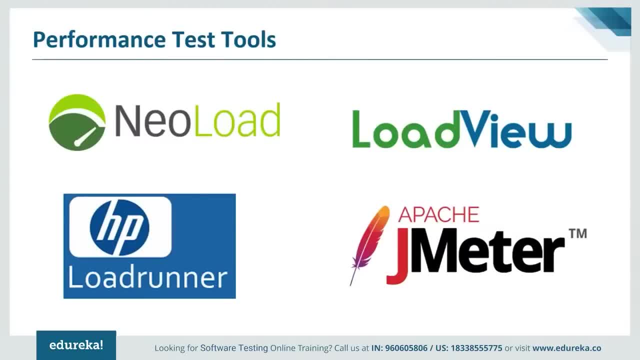 100% cloud-based load testing and you can also test user experience with real browsers for a complete performance picture. And you have one more tool, that is HP LoadRunner. This is the most popular performance testing tool on the market today. This tool is capable of simulating. 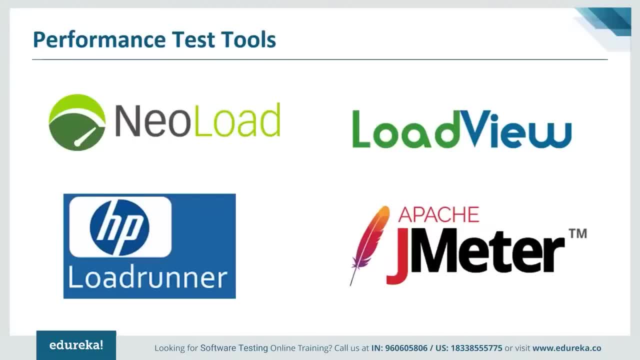 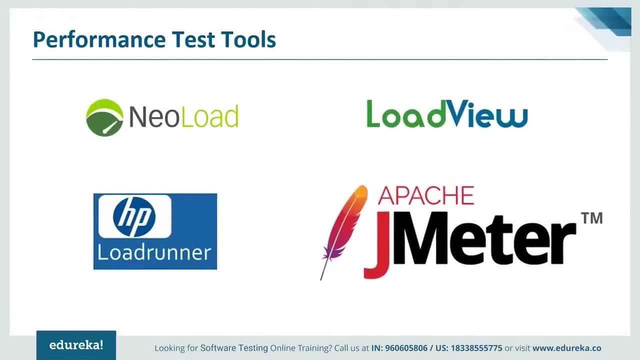 hundreds of thousands of users putting applications under real-time loads. to determine their behavior under expected loads, LoadRunner features a virtual user generator which simulates the actions of live human users. The next tool is JMeter. This is one of the leading tools used for load testing of web and application servers. 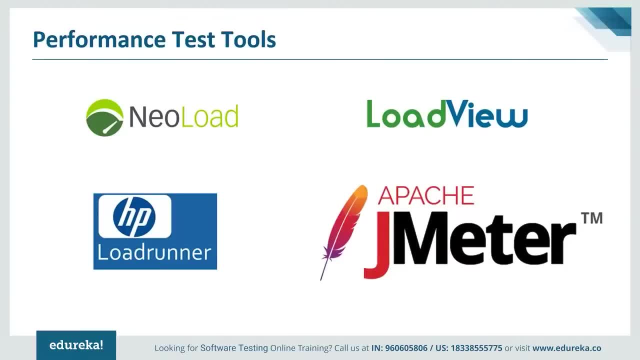 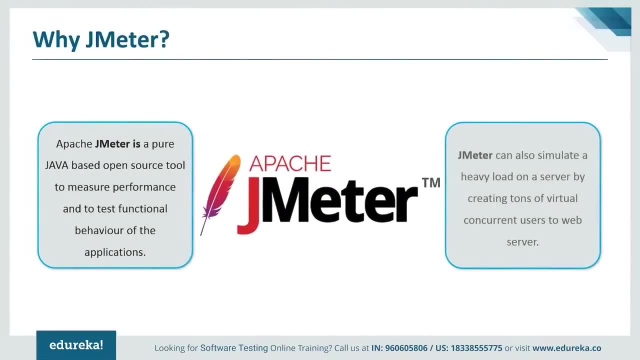 Among these tools. now let's understand why JMeter is considered as preferred tool for automation testing. Apache JMeter is a great open source application with awesome testing abilities. Web server is a platform that carries loads of numbers of applications and users, so that it is necessary to know how it works. 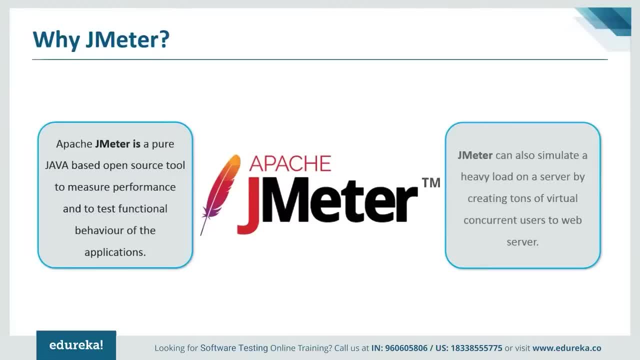 performs. that is, how effective it is to handle simultaneous users or application, And JMeter is the best suited tool to carry out all these actions. and it can also simulate a heavy load on the server by creating tons of virtual concurrent users to web server. So these are some of the advantages of using JMeter. 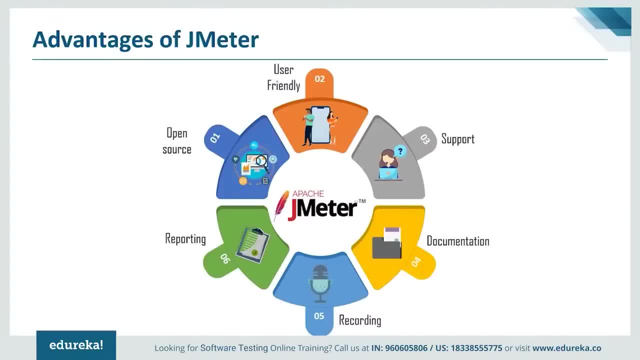 like it is an open source, It is user friendly, It has a wide support, It maintains a proper documentation and it provides proper recording of the test data, and it provides a well-structured report as well. So these are the main reasons why JMeter is considered a preferred tool. 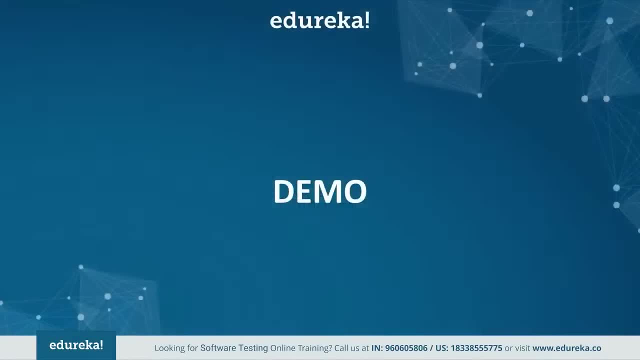 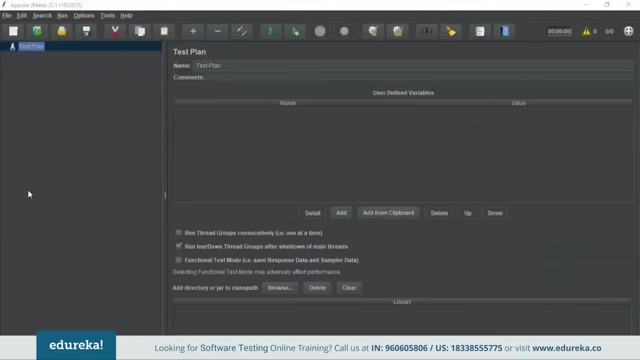 for performance testing. Now let's understand how to perform performance testing with the help of JMeter tool. Now let's move further and understand the working of Apache JMeter and let's see how to do the performance testing with the help of Apache JMeter tool. 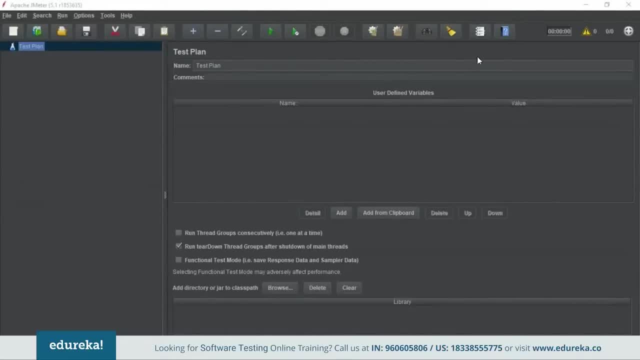 So this is my Apache JMeter tool. So this Apache JMeter tool comprised of two frameworks, that is, the left side and the right side. The left side of the framework consists of all the test plans that you're going to write, and the right side framework consists. 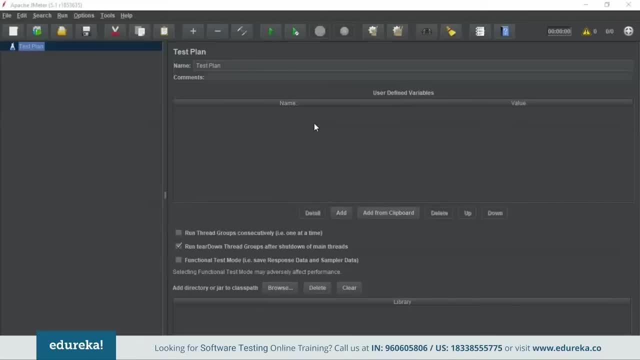 of the configurations that we will be changing and modifying as per the requirements. So here you can see the configuration of a test plan window. Now this test plan is like a container that contains all the test plan that you are going to perform, like whatever you add, like, say, your thread group. 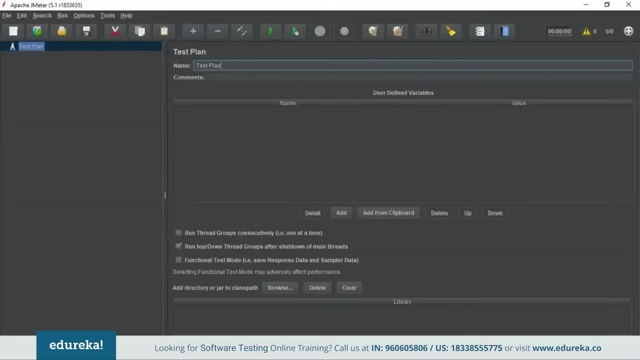 your results, your listeners, your samplers- everything comes under the test plan. Let's say I will change the name of the test plan to Edureka, So I'll save it. On changing the name of the test plan, You can see it got reflected over here. 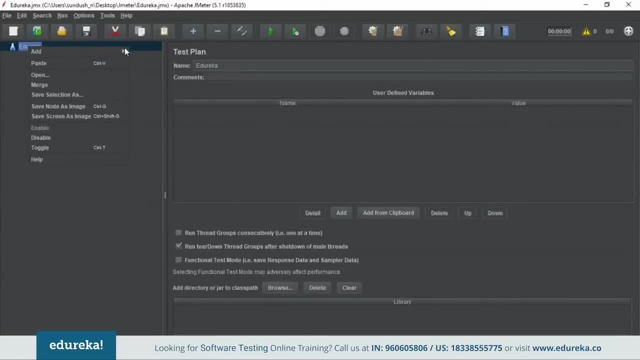 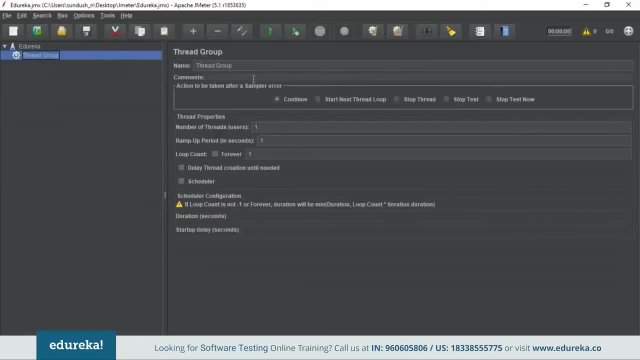 Now the basic thing that you have to do is you have to add the threads, that is, your thread group. So now I would like to tell you one thing here: If you want to know about the elements of JMeter, the basics of JMeter and the working of JMeter, 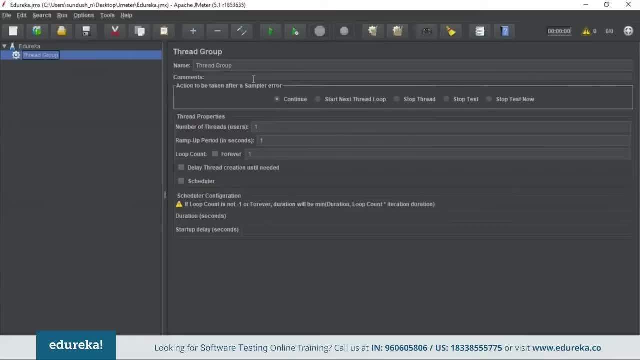 you can check out the video on JMeter tutorial on our Edureka playlist, will understand everything about JMeter: its installation, its basics, its elements, how to configure JMeter- everything in that video. So basically, thread group is nothing but a collection of threats and each thread represents the user. 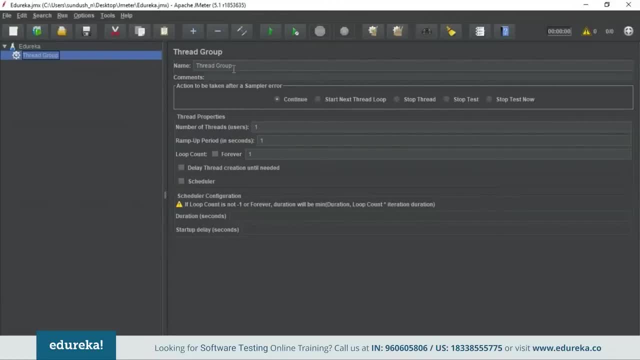 using application under test. So first I will be adding one thread group and I will rename this as users. So now we have something called as action to be taken after a sampler error and there are options like continue, start next thread loop, stop thread, stop test and stop test now. 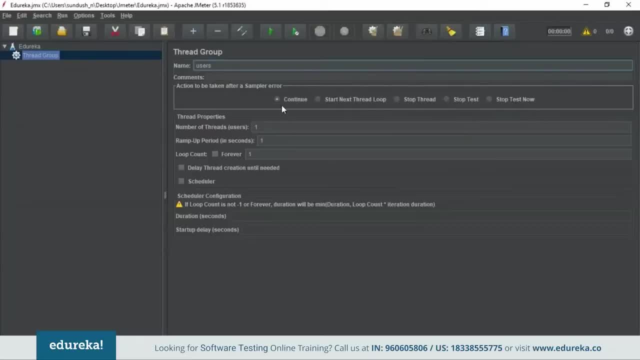 So I am going to choose the continue option, even if there is a sampler error. and thread properties is one of the important one, where you have the number of threats, the ramp up period, the loop count. even if you want to count it forever, You can give it that, so say. I want to specify. 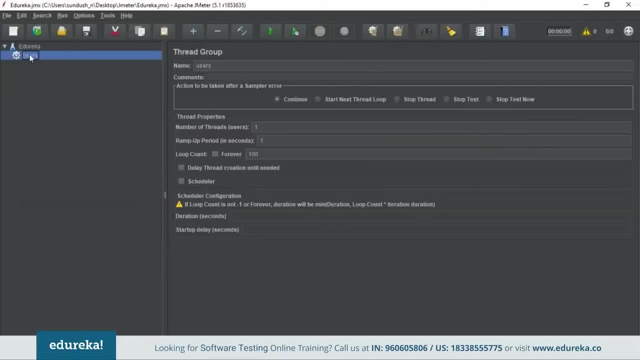 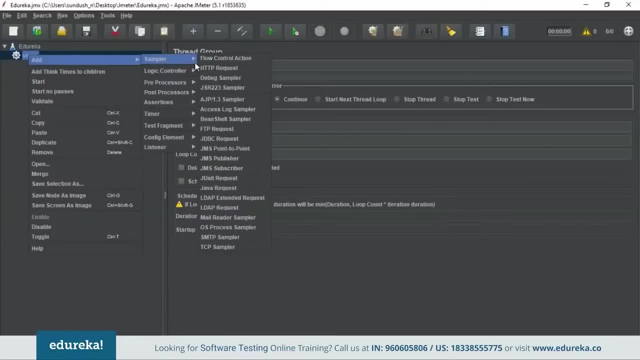 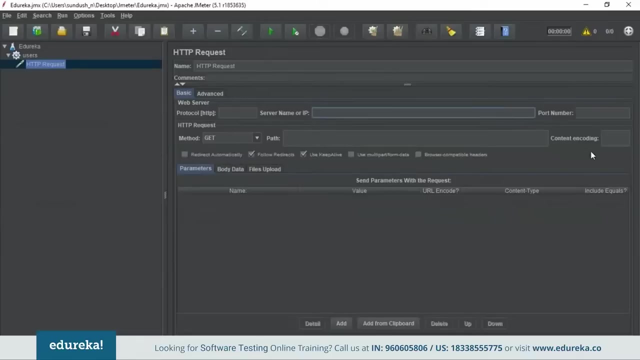 the loop count for hundred. Okay, So next what I'll do? I'll click on this thread group and I will add a sampler. as you all know that JMeter supports HTTP request, So I will be adding HTTP request under sampler. So here this is a HTTP request framework. 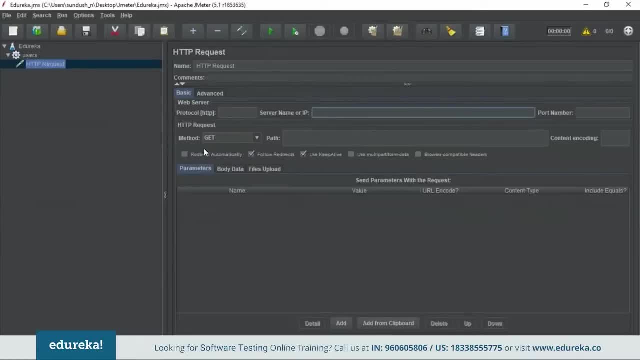 wherein there's a web server, the protocol, the HTTP request method is get, and you have to specify the server name or IP and the path as well. So now let's do one thing. So now let's launch the Edureka blog website. So I'll copy this path. 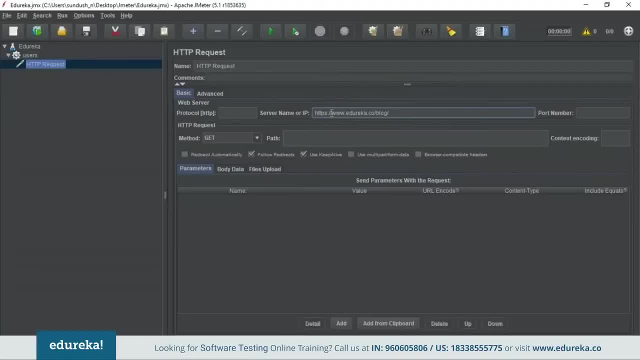 and I will paste it away. So, as this is a server name, I need not specify this, and also there shouldn't be the path, So I will just specify it as this. So this is how you have to specify your server name or IP and the path. 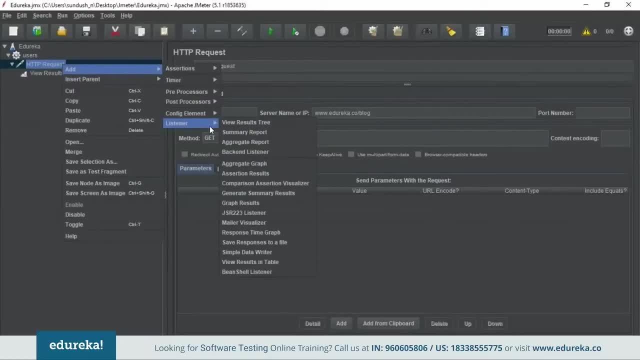 Now I will add the listener and as soon as I click on listener you can see there are options like view results, tree summary report, view results in table, etc. So now I want to view the results in table. Okay, I'll run the program now. 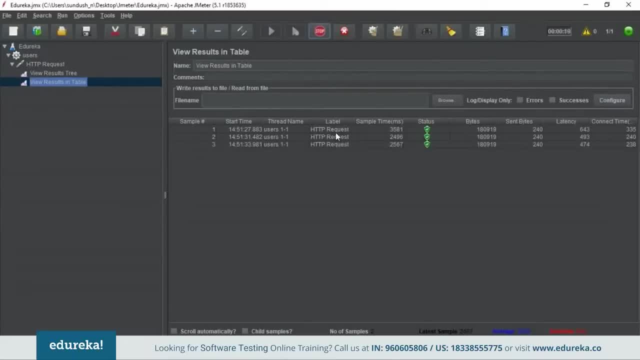 As soon as I run the program- HTTP request was submitted- You can see there's a start time, the sample numbers, the thread name, the sample time, the status bytes and bytes, latency, connection time, many things right. So basically what is happening over here? These are all the parameters for my performance testing. 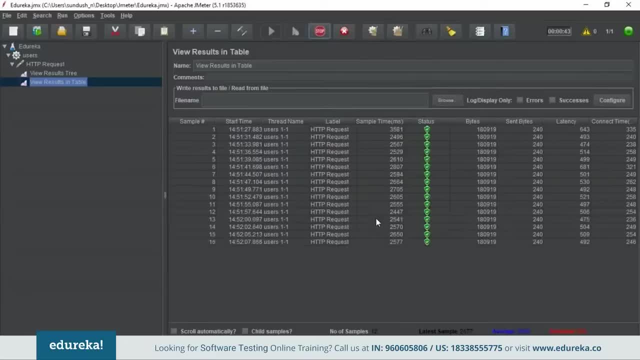 So it just calculates whether the server is able to respond to the client request or not. as I have given the count in the thread properties as hundred, it will read the results up to hundred threats. So it's go on reading it. So that's the reason it's reading the results up to hundred. 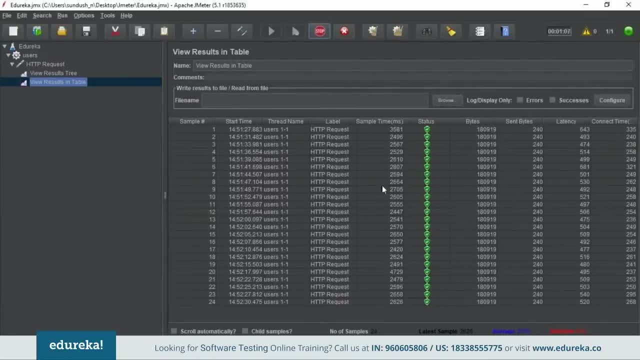 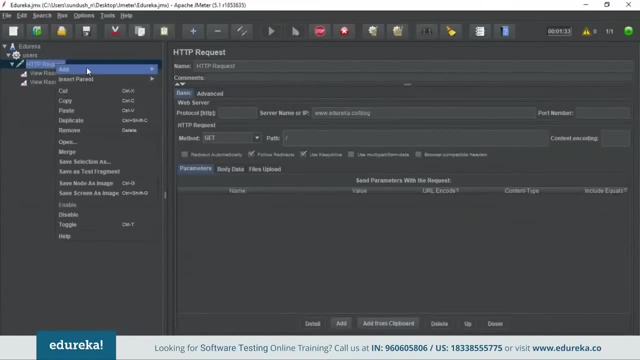 So this is a sample time: the status, the bytes, everything. Now, if you want to view the results entry, you can see that here as well. and again, if you want to add a listener for viewing the results in terms of graph, that is also possible. 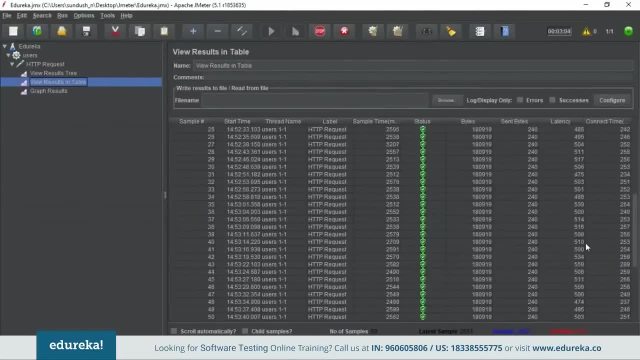 Now it will plot the graph over here So you can see here the count is getting increased and this gives the proper format of the output where you can actually see the start time, the sample time, the status. if there is any failure it will Mark as read over here. 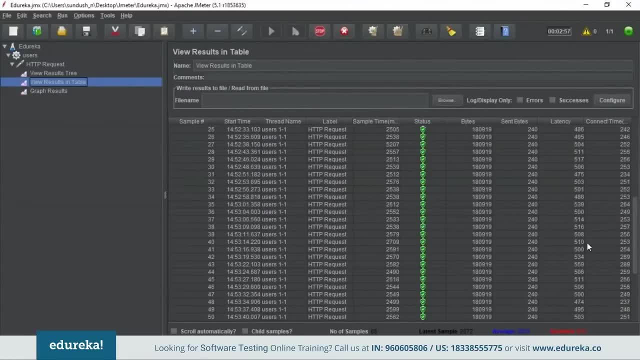 and you can see the bytes, the bytes and the latency, everything. So this is all about the performance testing using Apache Jmeter. If you wish to know how to perform load testing using Apache Jmeter, then please stay tuned because we will be coming up. 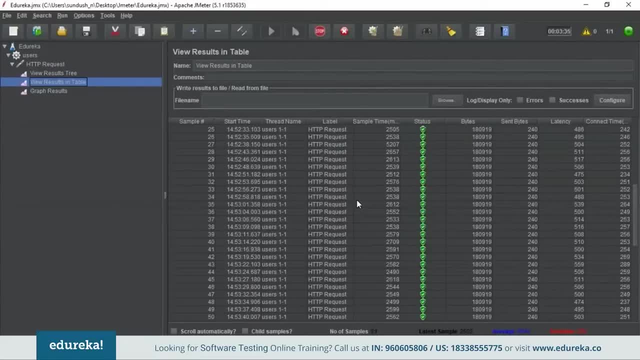 with a video on load testing using Apache Jmeter in the next few days and you can learn that as well. So that's all for the session. I hope you learned what is performance testing, how it works, What is the performance testing process, the test metrics. 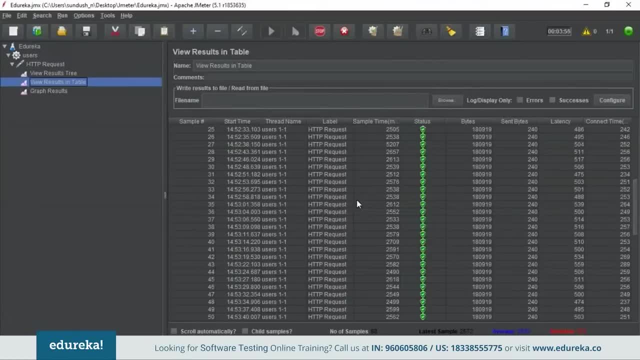 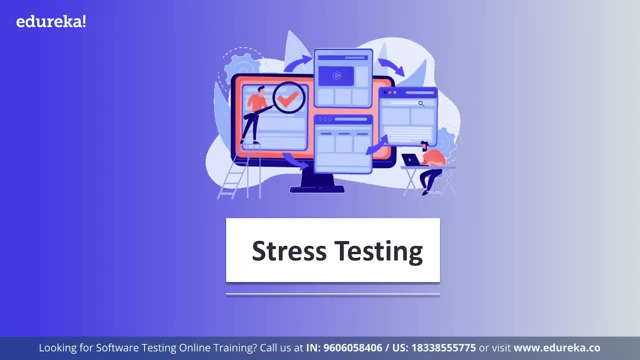 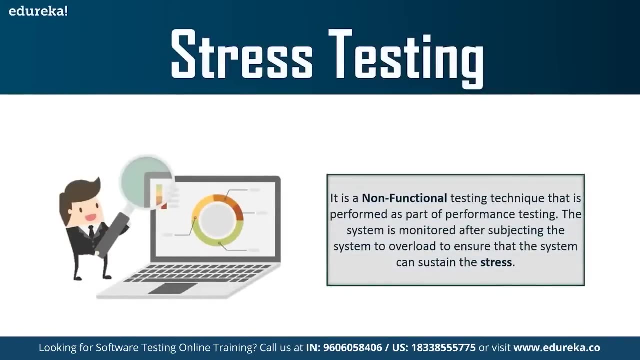 and how. Apache Jmeter is useful for performance testing of a website. So what is stress testing? now, stress testing is basically defined as a type of software testing that verifies the stability and reliability of the system. Now, this test mainly determines the system on its robustness. 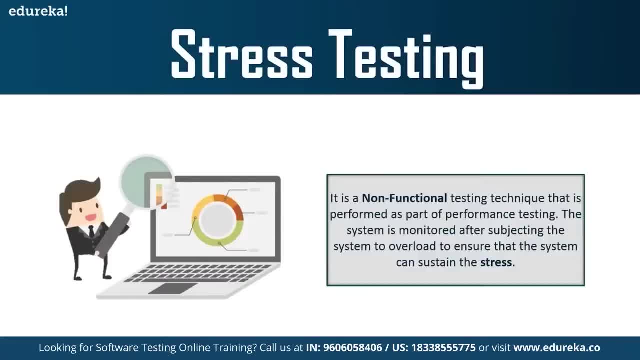 and error handling under extremely heavy load conditions. It even tests beyond the normal operating point and evaluates how the system works under those extreme conditions. Now, stress testing is done to make sure that the system would not crash under crunch situations. So in software engineering, stress testing. 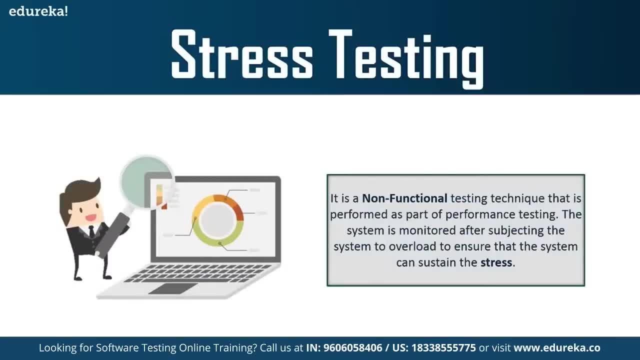 is basically known as the endurance testing, and a most prominent use of stress testing is to determine the limit at which the system or software or hardware breaks. It also checks whether the system demonstrates effective error management under extreme conditions. Now why do we need stress testing? 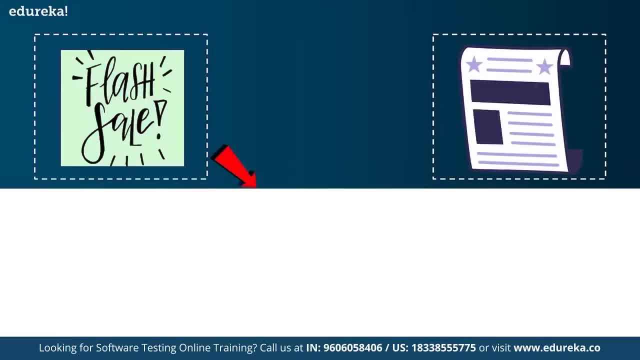 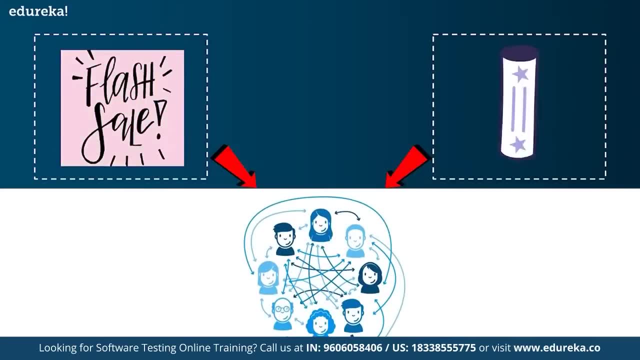 So whenever there is a festival going on or any online sale going on, an online shopping site may witness a spike in traffic, or when a blog is mentioned in a leading newspaper, it experiences a sudden surge in traffic. Now it is imperative to perform stress testing to accommodate such abnormal traffic spikes. 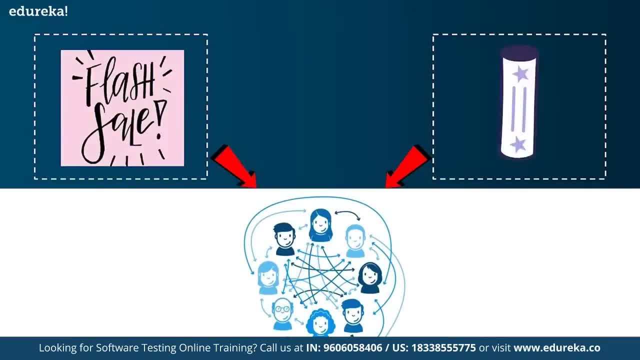 Now, failure to accommodate the sudden traffic may result in loss of revenue and repute. So we need stress testing in order to check if the system is working fine under abnormal conditions, also to display appropriate error message when the system is under stress. Now it is better to be prepared for extreme conditions. 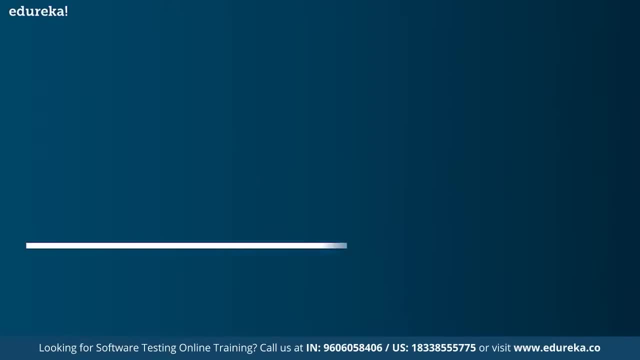 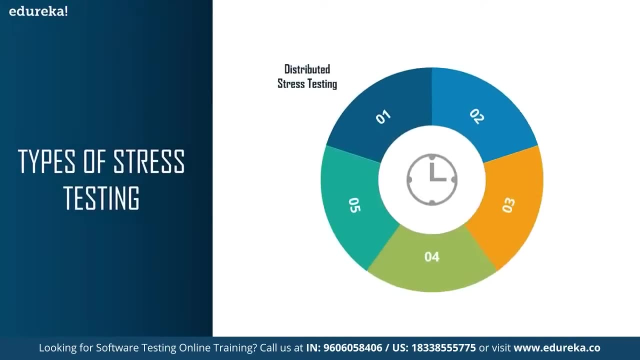 by executing the stress testing. Now let's have a look at the different types of stress testing. So first we have the distributed stress testing. Now, in distributed client-server systems, testing is basically done across all clients from the server, and the role of stress server is to distribute. 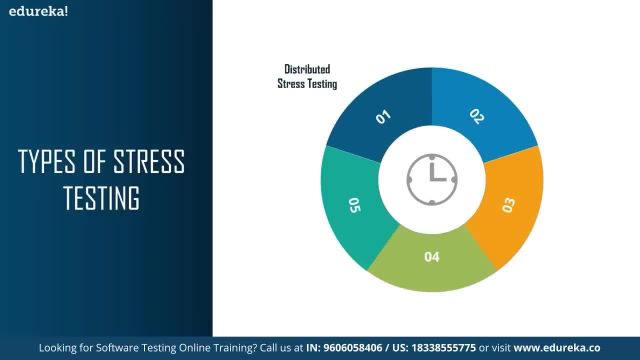 a set of stress tests to all stress clients and track on the status of the client. Now, after the client contacts the server, the server adds the name of the client and start sending data for testing. Now the large server farms need a more efficient method for determining which computers have had stress failures. 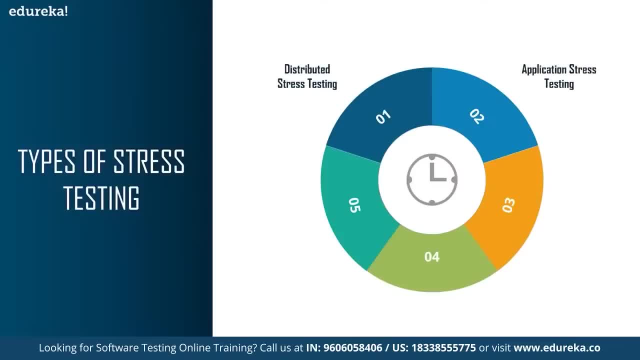 that need to be investigated. Moving on next up, We have the application stress testing. So this testing concentrates on finding defects related to data locking and blocking, network issues and performance bottlenecks in an application. Then we have the transactional stress testing. 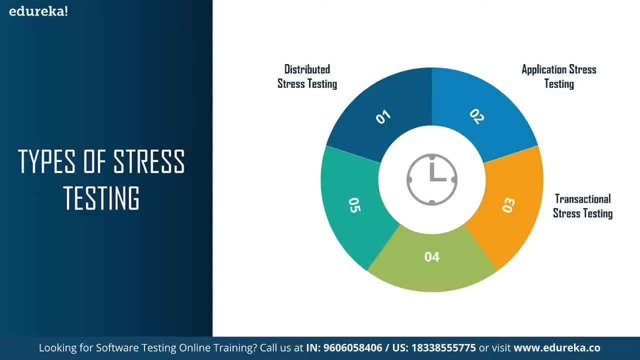 Now it does the stress testing on one or more transactions between two or more applications. It is basically used for fine-tuning and optimizing the system, and then we have systematic stress testing. Now this is integrated stress testing, which can be tested across multiple systems running on the same server. 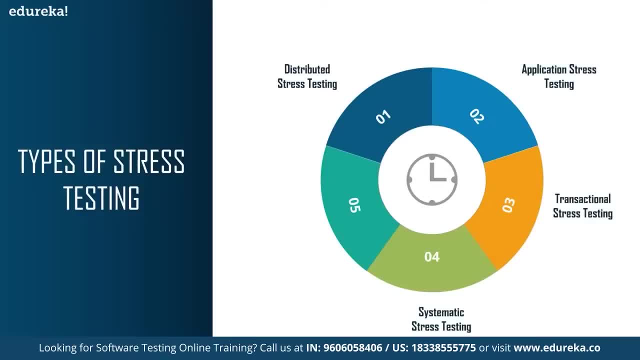 It is also used to find defects, where one application data blocks another application. And finally, we have the exploratory stress testing. Now, this is one of the types of stress testing which is used to test the system with unusual parameters or conditions that are unlikely to occur in a real scenario. 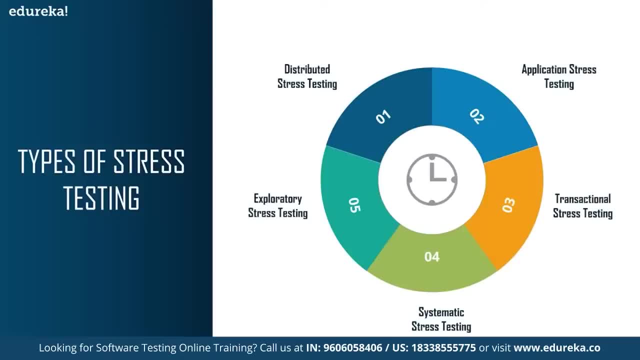 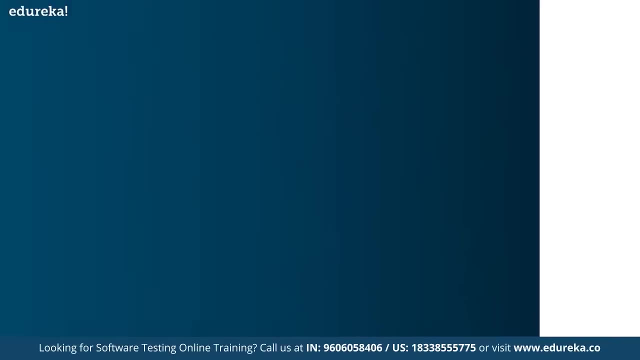 It is used to find defects in unexpected scenarios like a large number of users logged at the same time, or if a virus scanner started in all machines simultaneously, or if the database has gone offline when it is accessed from a website. So these were some of the types of stress testing. 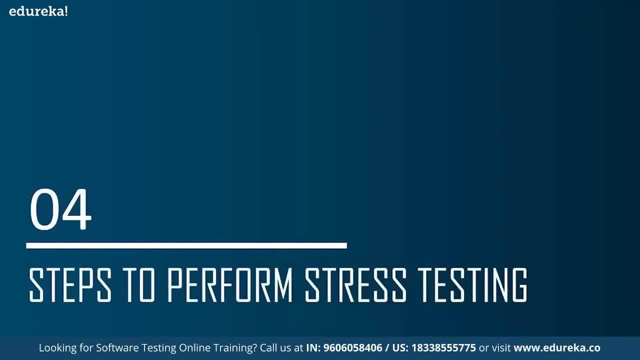 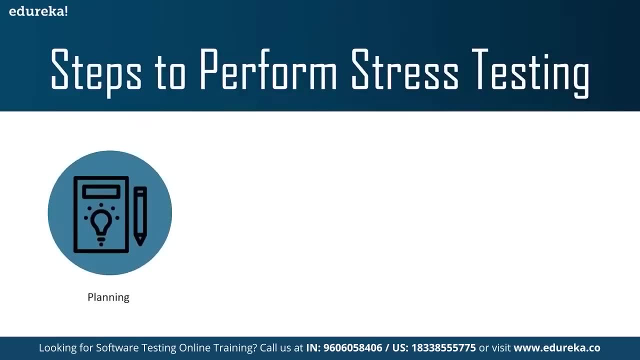 Now let's have a look at the different steps involved in performing stress testing. So stress testing can be done in five major steps. The first one is planning the stress test. So here you basically: gather the system data, analyze the system and define your stress test goals. 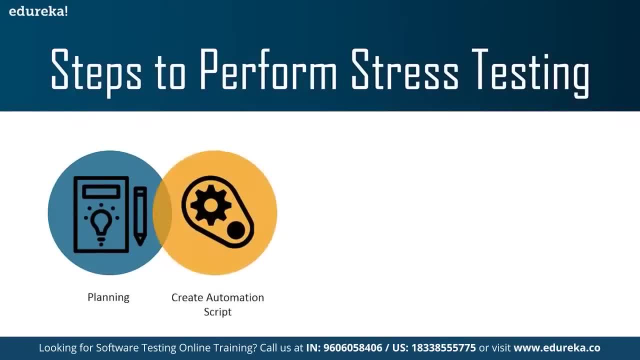 and then we have the create automation scripts. Now, in this phase, you can create the stress testing automation scripts, generate the test data for the stress scenarios. Next up is the script execution. Now, in this particular stage, you run the stress testing automation scripts and store the stress results. 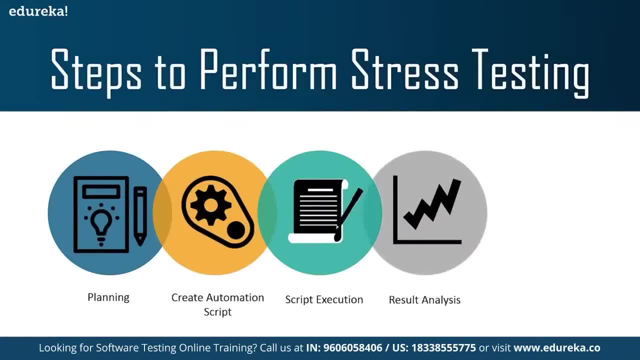 The fourth step is the result analysis. Now, in this particular stage, you analyze the stress test results and identify the bottlenecks. and finally, we have the tweaking and optimization. Now, in this stage, you fine-tune the system, change the configurations, optimize the code and meet the desired benchmark. 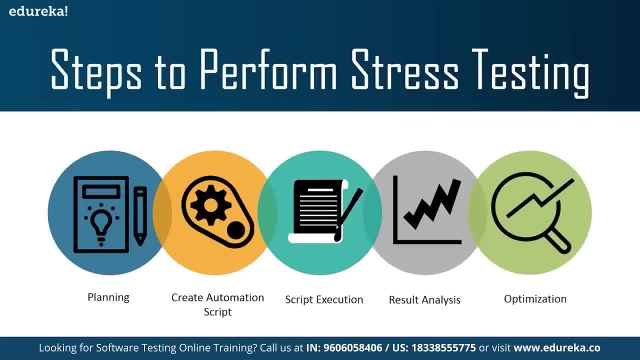 Now, finally, you again run this entire cycle to determine that the tweaks have produced the desired results. For example, it's not unusual to have three to four cycles of the stress testing process to achieve the performance goals. Now, these were the main steps that are required. 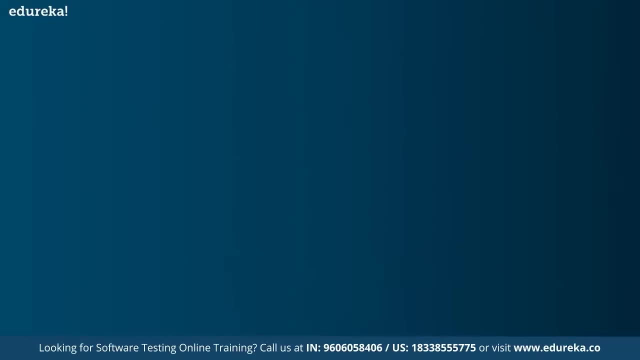 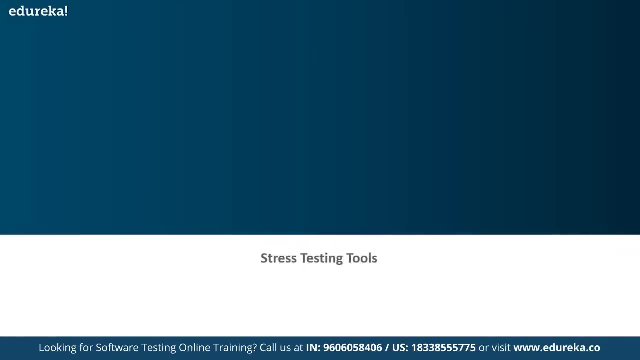 in order to perform stress testing. So let's move on and have a look at the different tools that we use for stress testing. Now, here we will talk about some of the major tools that are commonly used whenever we need to perform stress testing on any website. 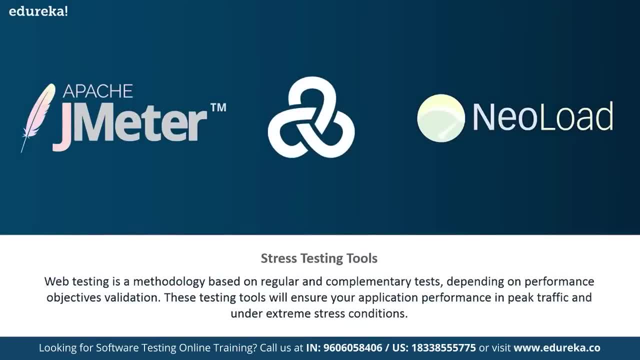 Now web testing is basically the methodology, based on regular and complementary tests depending on performance objectives validation. So these testing tools will ensure your application performance in peak traffic and under extreme stress conditions. First we have the Apache JMeter. Now JMeter is basically an open-source testing tool. 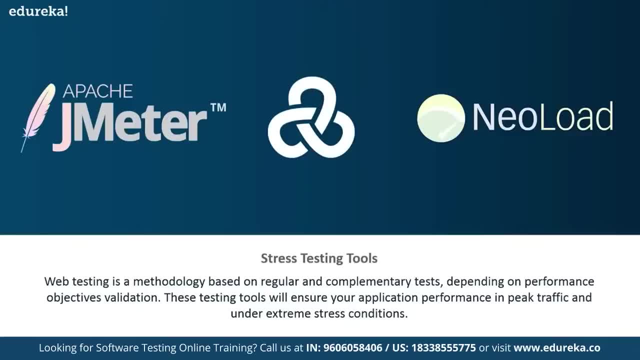 So it is a pure Java application for stress and performance testing. Now, JMeter is intended to cover types of tests like load testing, functional testing, stress testing, etc. It also needs a JDK5 or higher to function. Now you can also go back to our channel. 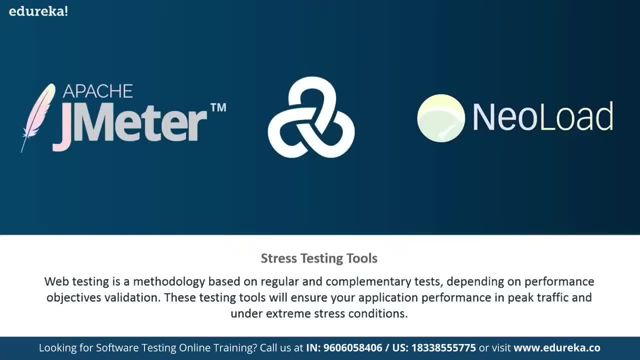 and have a look at the different videos on Apache JMeter. You can have a look at the Apache JMeter tutorial and also how to install JMeter. Also, you can have a look at the video on load testing using JMeter. Next up, we have load runner. 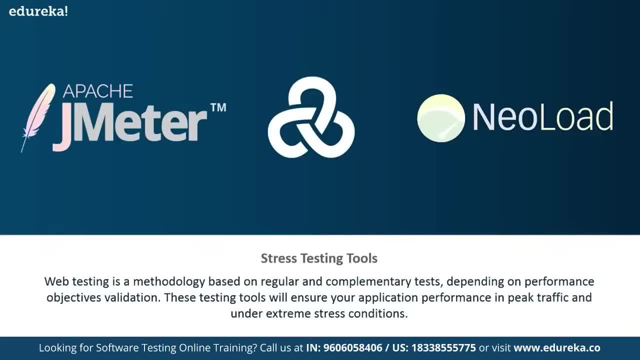 So load runner from HP is basically a widely used load testing tool. Now load test results shaped by load runner are considered as a benchmark. It is also quite efficient when it comes to stress testing. and then we have the Neo load. Now this is a popular tool available in the market. 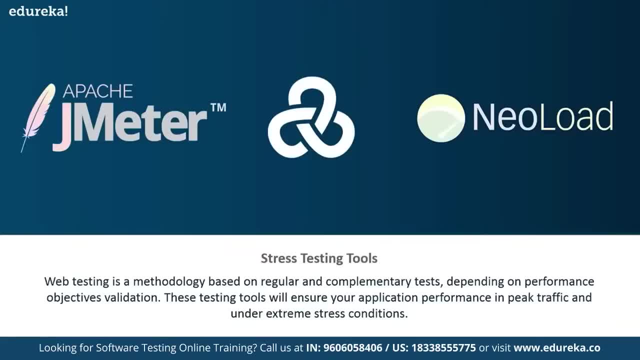 to test the web and mobile applications. Now this tool can simulate thousands of users in order to evaluate the application performance under load and analyze the response times. It also supports cloud integrated performance load and stress testing. It is easy to use, cost-effective. 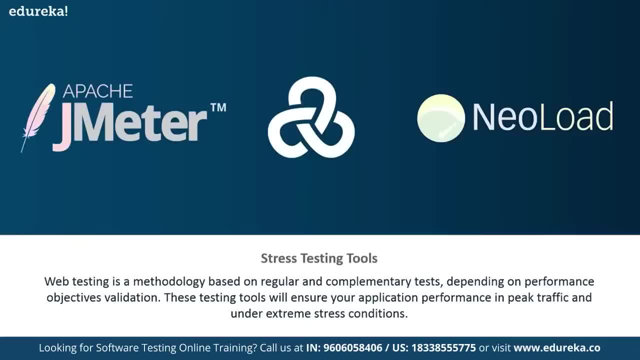 and provides good scalability. Now, stress testing's objective is to check the system under extreme conditions. It monitors system resources, such as memory processor, network, etc. and checks the ability of the system to recover back to normal status. It checks whether the system displays. 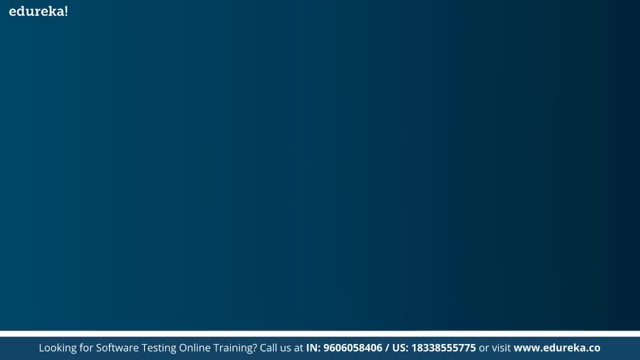 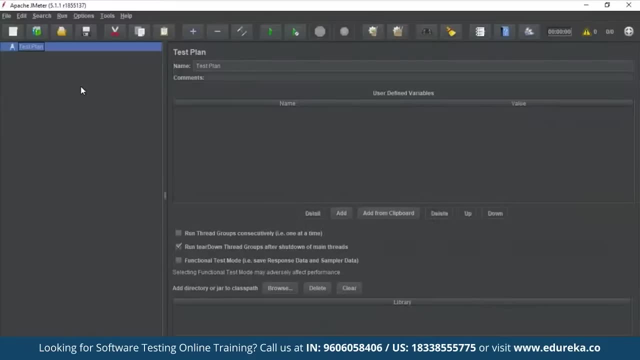 appropriate error messages while under stress. So let's have a look at how stress testing can be performed with the help of JMeter. So in my previous videos I have already shown on how to create a test plan in Apache JMeter. Also, if you want to know how to install, 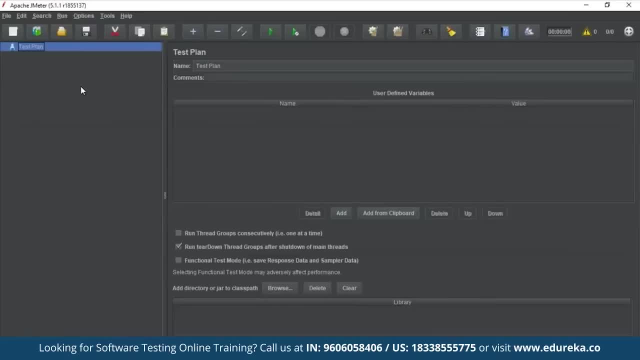 this particular tool in your system. you can go back and have a look at the video on how to install Apache JMeter Now. this is the user interface of JMeter. Now here we will create a test plan and perform our stress testing on a particular website. 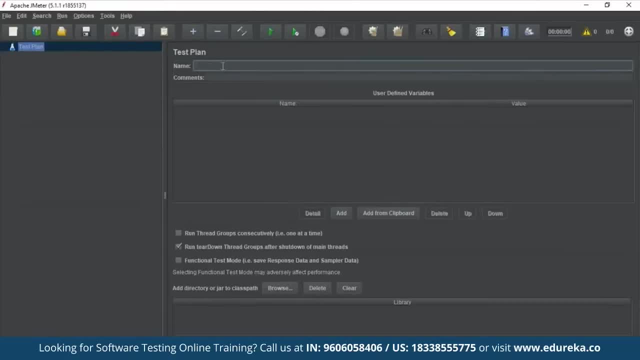 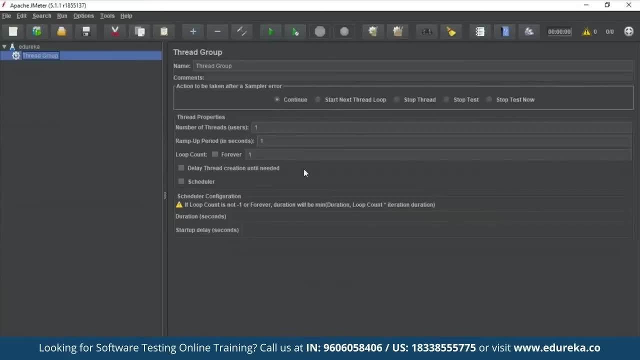 So for that we first have to create a test plan. So let me just name this test plan as Edureka. Now, inside this test plan, I'm going to add my thread groups. So let's take the number of threads as 5 and also let's have our loop count as 2.. 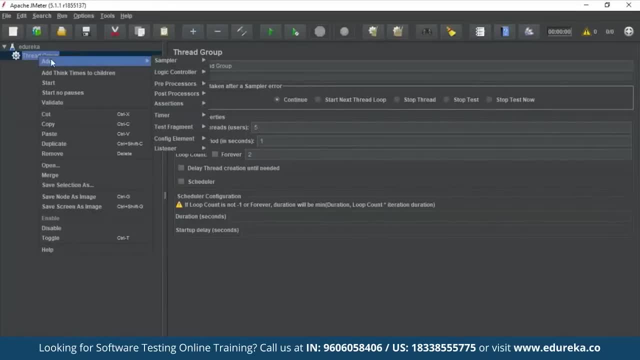 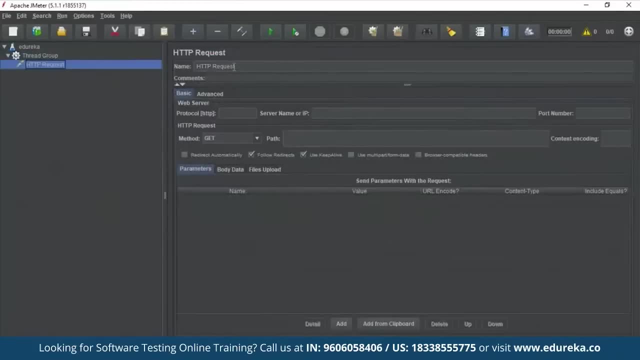 Now inside a thread group, we are going to add the HTTPS, so we go to add, then we go to sampler and inside sampler we have the option as HTTP request. Now, inside HTTP request, we provide our server name or the IP address and also specify the path to our website. 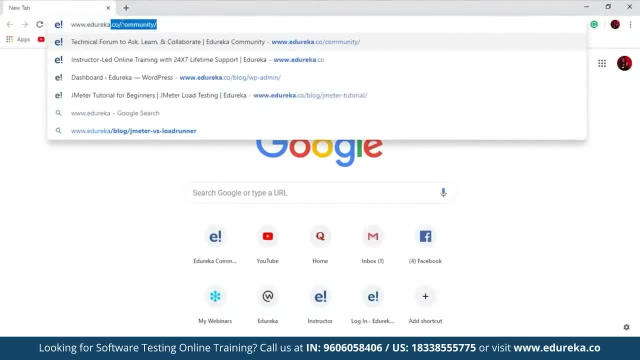 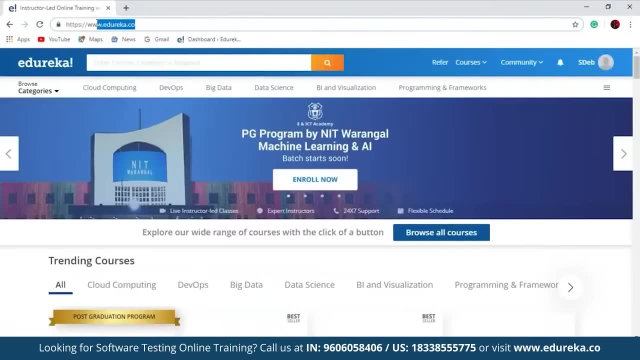 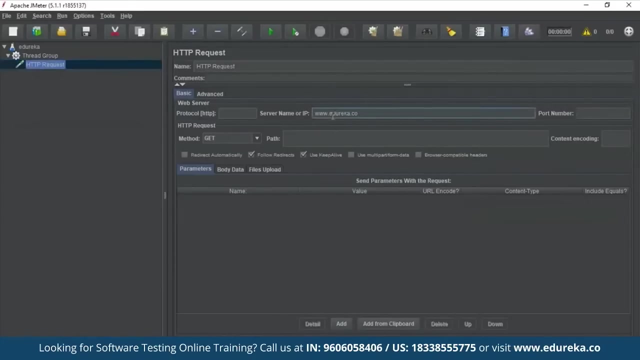 So here we will take the example of our Edureka website itself. So this is the Edureka official website. I'm just going to copy this server name and use it in my test plan. So here in space of server name or IP, I'm going to put wwwedurekaco. 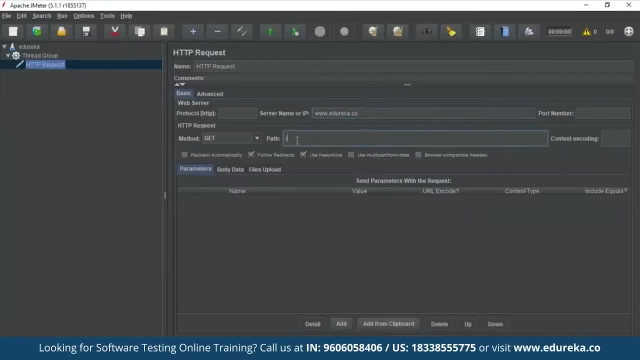 and I'm just going to specify the path with a slash. Now, for this particular website, we would want to add a listener and see how our results are viewed. So once we go to add and go to listener, we have various options So we can select view results and table. 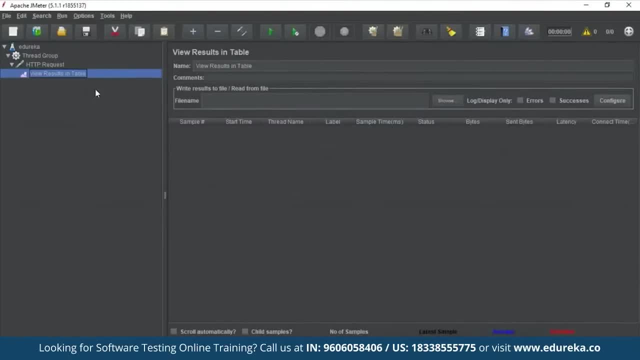 where we will get our results in the form of a table. Now, before running the test, we have to save it. So I'll just first save this test plan. so let me just name it as stress test and then it has the extension as dot: jmx. 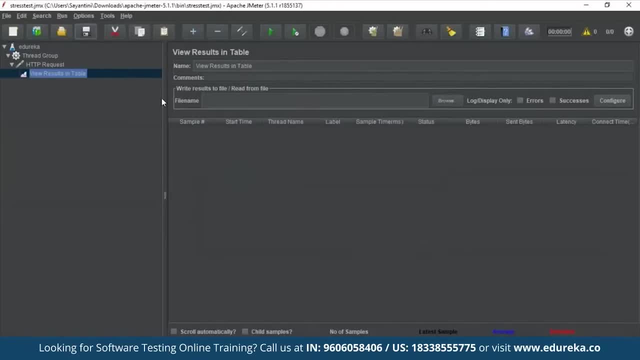 and let me just save this test plan Now. once it is saved now we can run this test and see the result. So now, once I've run this test, you can see that it's viewing the result in this table and you can also see all our thread groups. 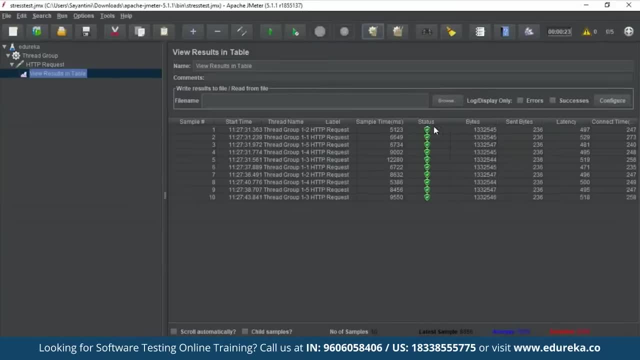 and the number of loops that I have given. So you can see that the status is green means the website is working fine And all the thread groups have been working well and it has shown the status as okay. Now, if you want to check any particular element, 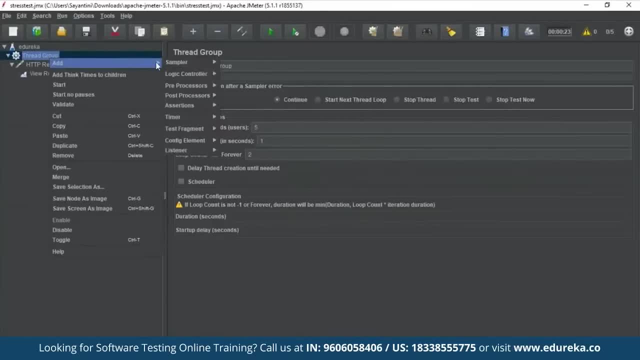 inside your website you have to add a response assertion. So in the thread group we are going to add one response assertion. So here I go to add, and inside assertions I have response assertion. Now our response assertion in Jmeter is most important element. 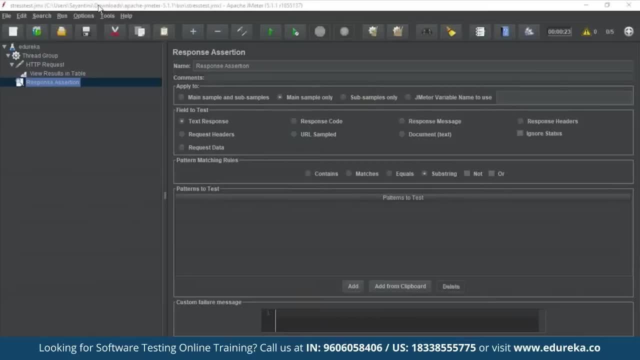 as it helps you to assert the response of request in your software load test plan. Now it will show the request result failed if response of request is not as expected, and show pass if response of request is as expected. So you can verify your software load test result. 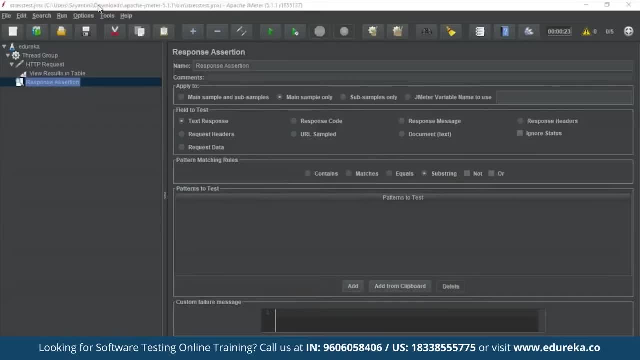 using the response assertion. So here we have added the response assertion inside our thread group. So we are going to check for the response code and we will have the pattern matching rules as contains, and here I'll add the response rate. So I'll put 200. 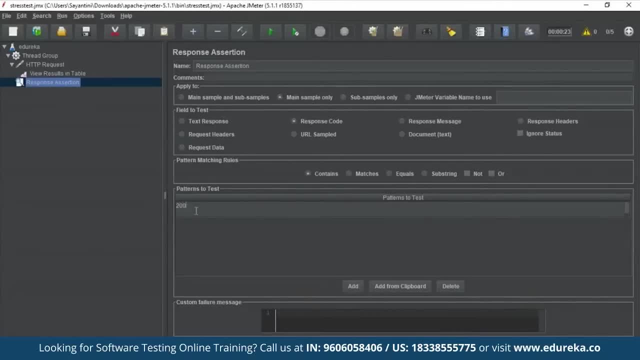 because 200 is equal to 100, used for the success response. Now the response code 200 represents the HTTP request which has succeeded already. So we will add this in our patterns to test and we will save it. So now, once we run this again, 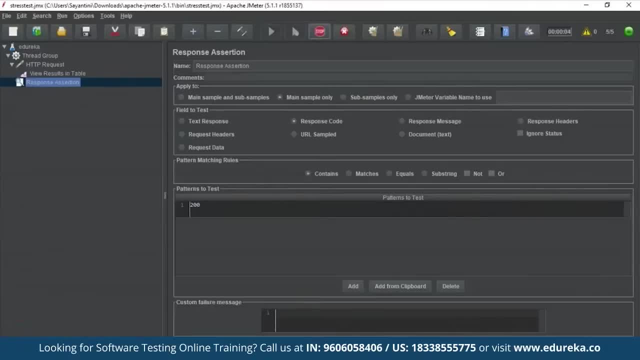 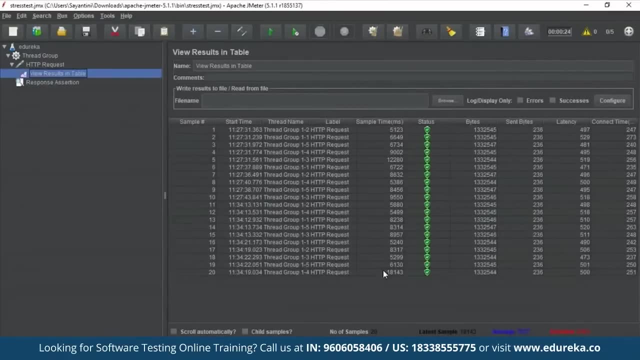 you can see that the status would be viewed in the table again. So you can see that the assertion is taking place and now we can go to our view results and table and see that more number of samples have been added here and you can see the status is still green. 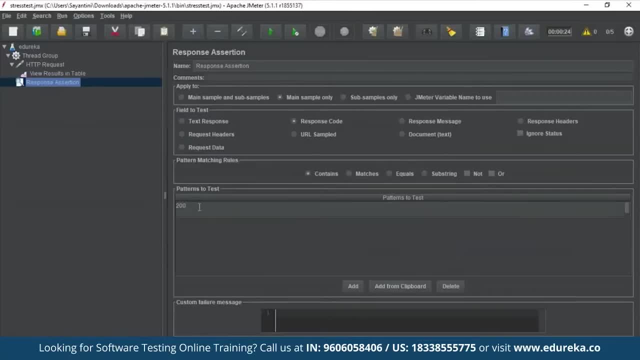 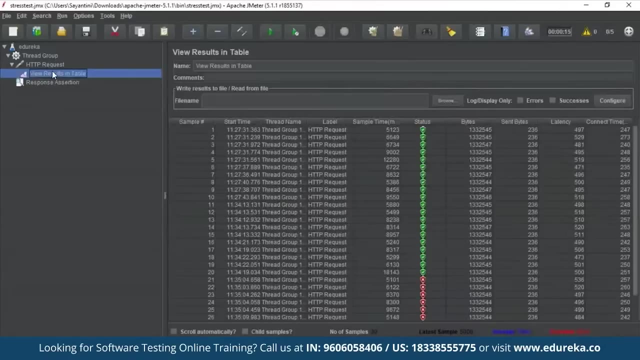 But now if we go back to our response assertion, and in case we change this number to 201 and again save it, and now if we run this again, let's see what happens. So you can see that the test is taking place, So you can see that it is complete. 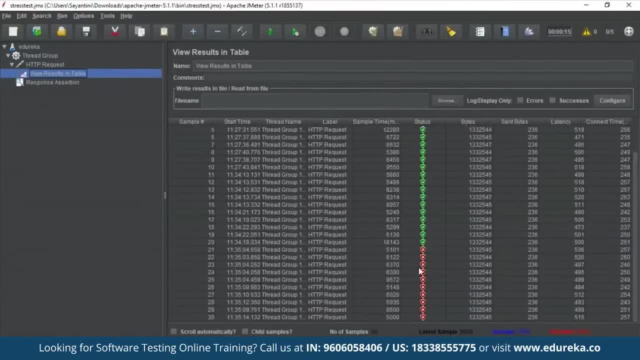 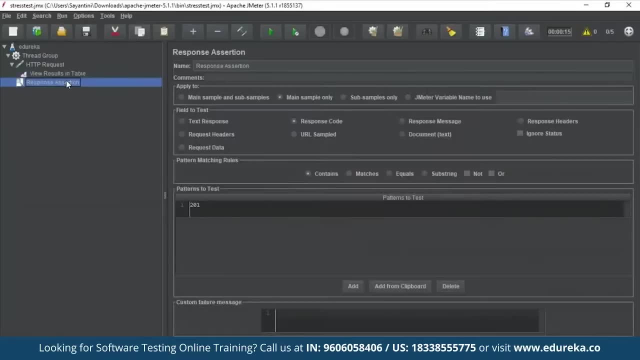 and once we go back, you can see that the status has changed to red now. So you can see that it means our HTTP request did not succeed because we put our response assertion code as 201.. So now let me just change it back to 200. 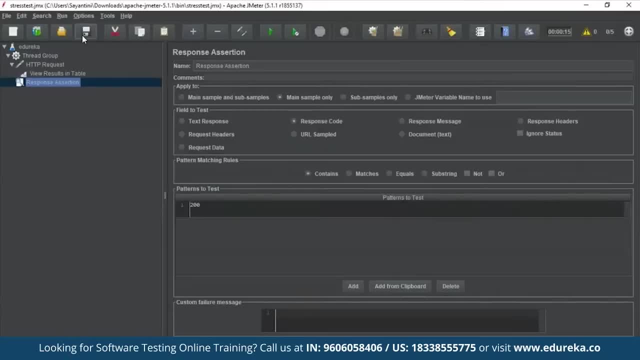 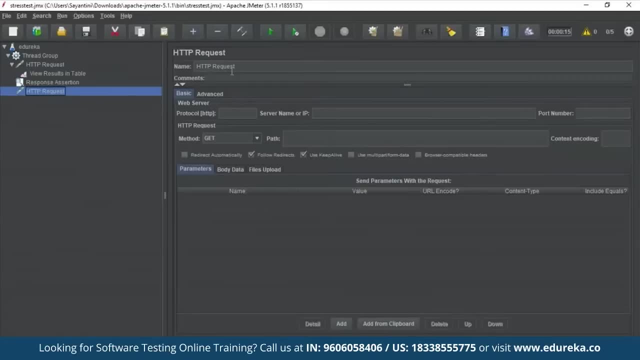 and save it, because that's the code used for the request to succeed. Now, if you want to add more pages, you can just go back to your thread group and add another HTTP request. So here I can again put my website as wwwedurekaco. 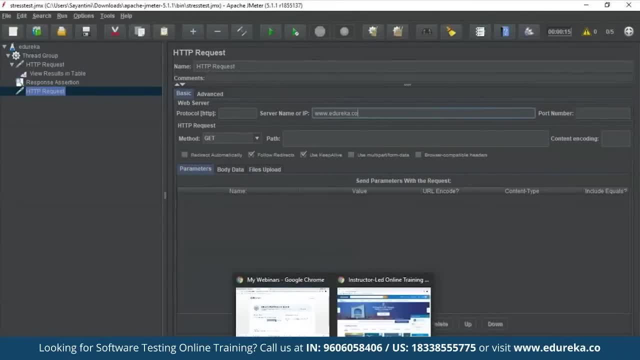 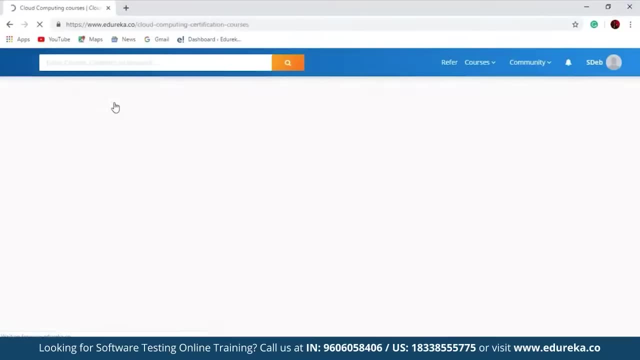 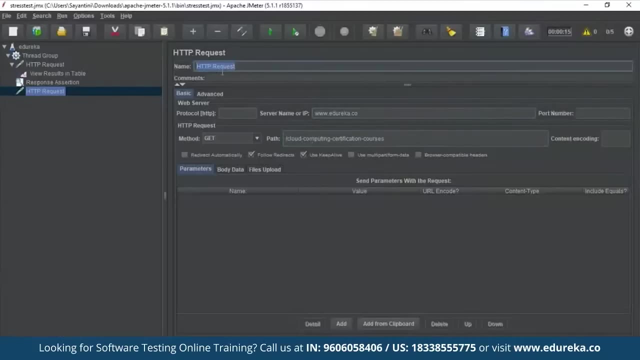 and if I want to access any other link inside this particular website. so suppose I want to get inside the class without computing page of edurekaco. I just have to copy this path and paste it inside the path section of my HTTP request. 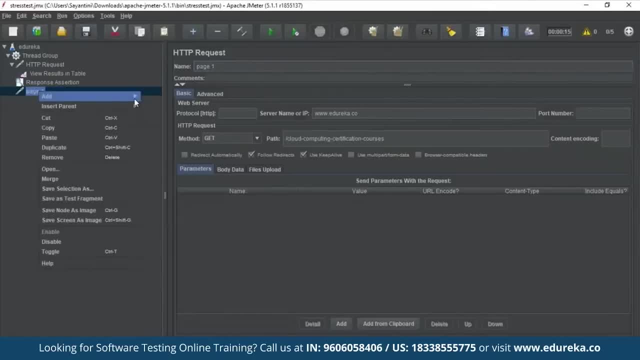 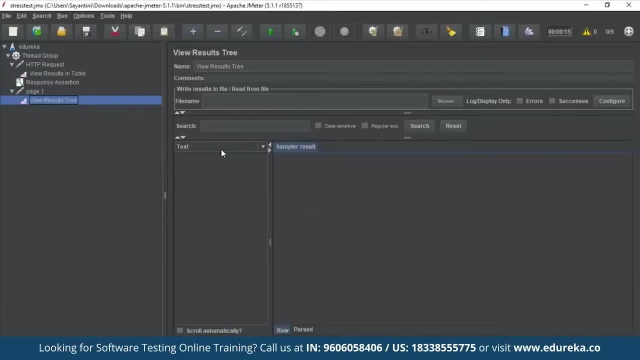 I can save it as page 1 and also add another view results and table, or in the tree format. So I'll go to listeners. So let's view this result in the form of a tree. So let me just save this test plan and run this code again. 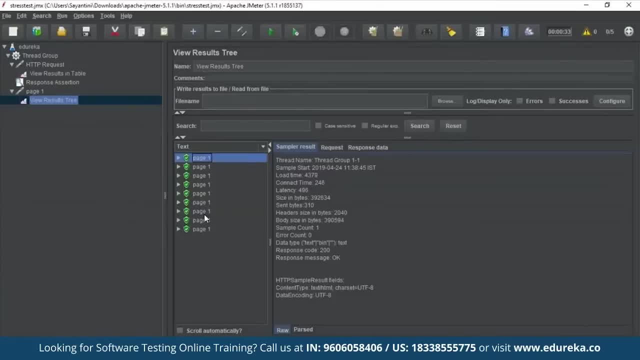 So now you can see that your test is taking place and the number of threads and users that you have provided are going on now in the tree format. Once you go and click inside this page one, you can see your thread group and you can also see your response code. 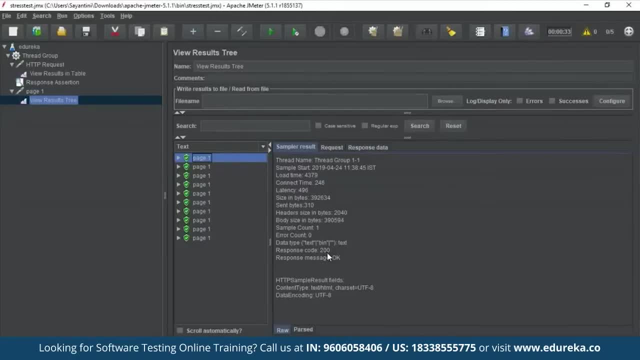 and response message. So your response code is 200,, which means your website is working fine. Also, you've got the response message, is okay, So you can also change the number of threads and the loop counts and check if your website is working fine. 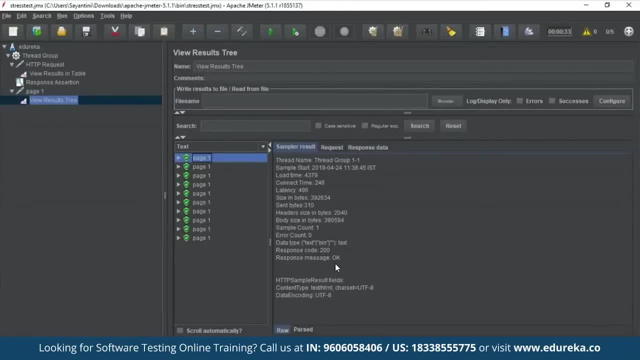 and this way you will get to know, no matter how much stress you put on your website or the number of threads you keep on adding, if it is working completely fine or not. So the response code 200 will tell you if your website is working fine. 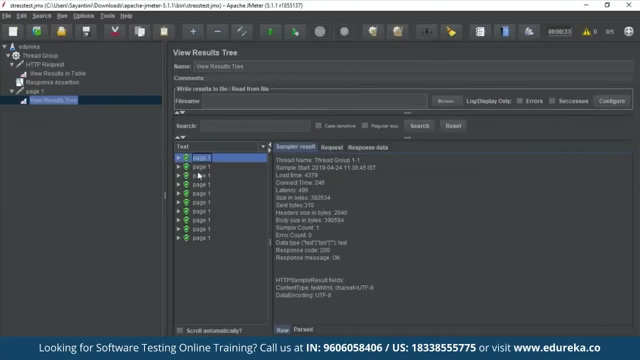 or if it has succeeded the test or not, and also when you view this result. you go to any of these page and you can check your response code and response message and also check the status of your website or any element that is present in your website. 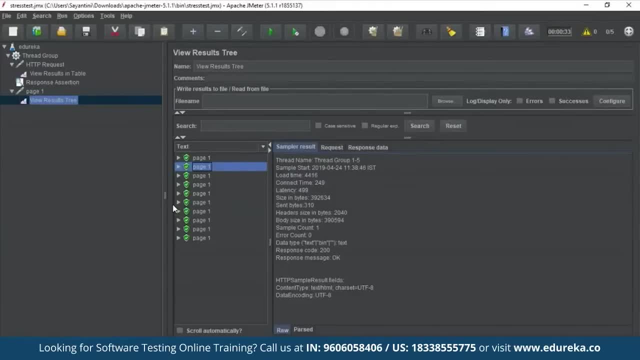 So in this way I can add as many elements as I want to and also increase the number of threads and also the number of loop counts. This will increase the stress and also you can check the time that it takes for the test to happen. You can check the load time here. 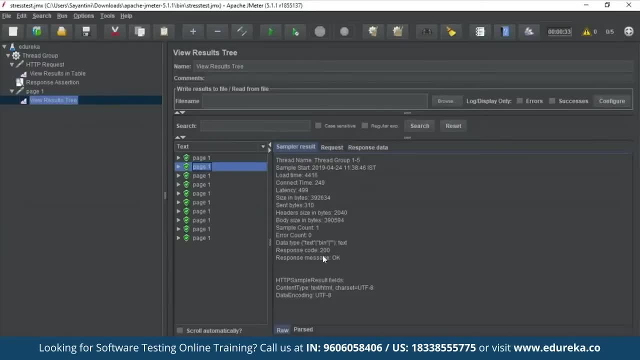 and also the connect time latency and everything is visible here, So you can check if your website is able to handle the stress and, no matter how much load you put on it, if it's working fine or not. So this was a type of performance testing. 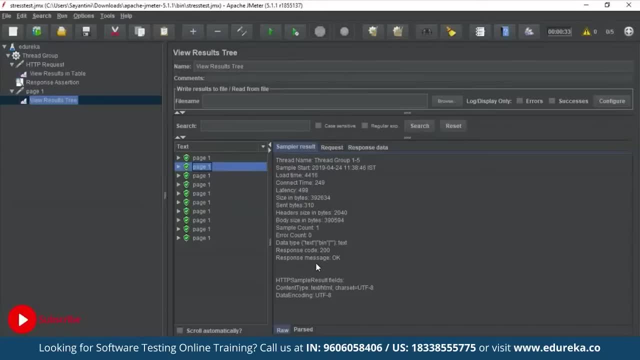 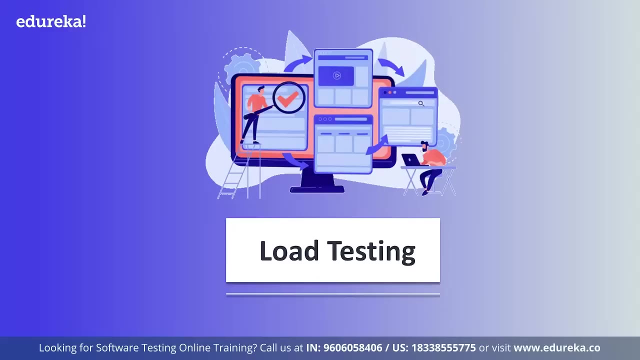 that you can perform on any website to check if it's working fine, and you can also check for the different elements present inside your website and check their performance. What is load testing? So, basically, load testing is a kind of performance testing which determines a system's performance. 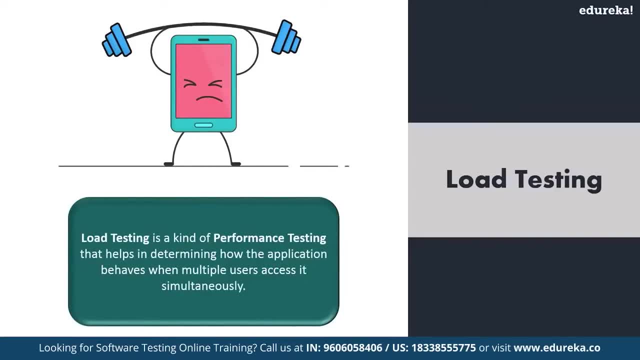 under real-life load conditions. Now, this testing helps determine how the application behaves when multiple users access it simultaneously. Now, this testing usually identifies the maximum operating capacity of an application. It determines whether the current infrastructure is sufficient to run the application. sustainability of application. 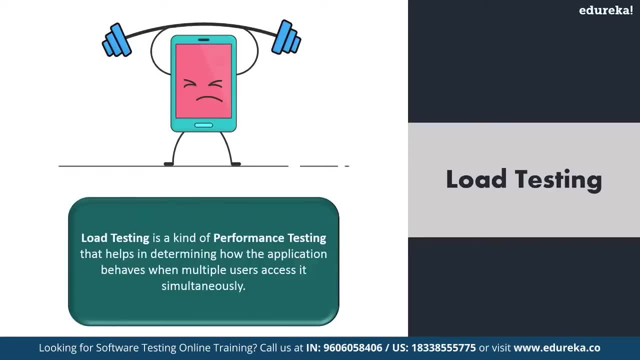 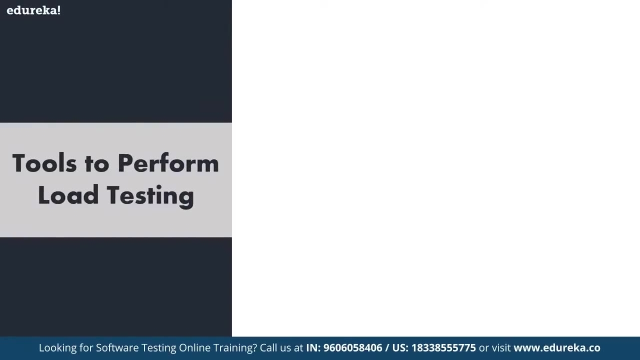 with respect to peak user load and also the number of concurrent users that an application can support, and scalability to allow more users to access it. Now there are various tools that are available in order to perform this testing, So load testing is significant in real time. 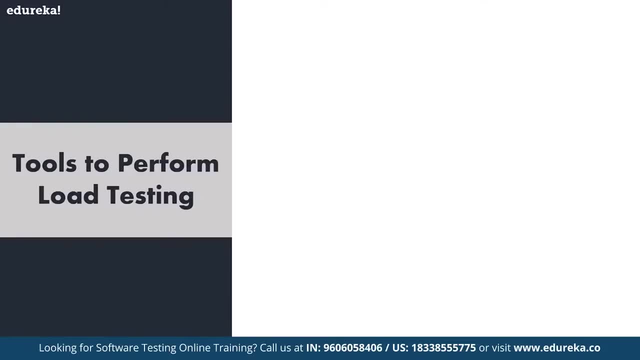 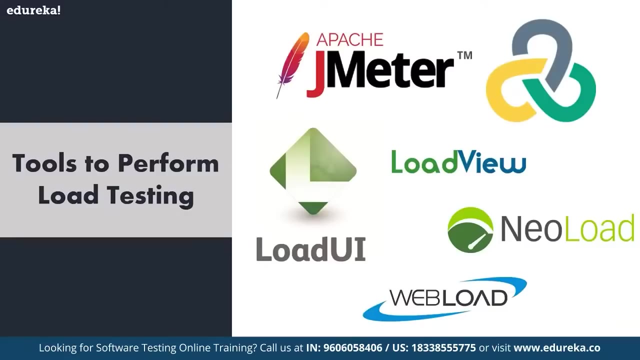 particularly from a point of view of customer satisfaction. Now there are several performance testing tools available, such as the Apache JMeter load runner, web load load UI, Neo load and web load, But JMeter is one of the most preferred tools for testing. 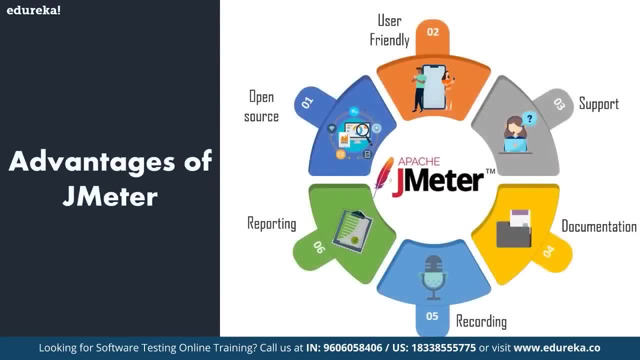 So let's have a look at some of the advantages of JMeter. that makes it the most preferable one. First of all, it is an open source and also built-in Java platform. It is highly extensible and platform independent. JMeter is also very user-friendly. 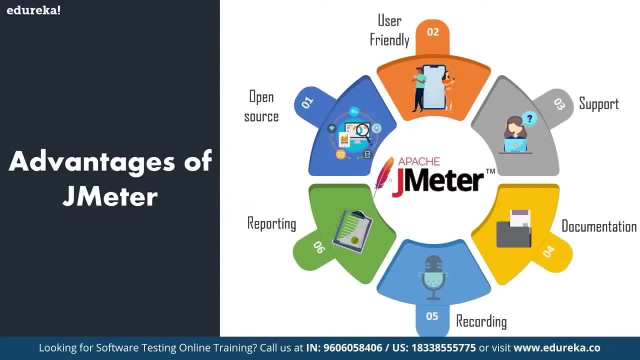 Now JMeter has a comprehensive GUI which helps to create test plan and configure the elements. Now adding elements is easy on JMeter: Just right click on the tree scenario and add what you need to do. Next up is the support. Now, basically, it is designed for performance testing. 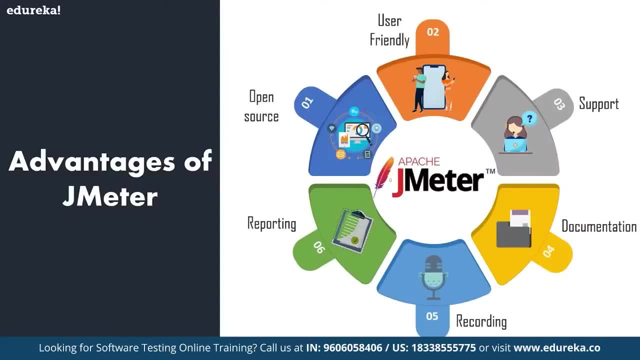 but also supports other functional tests, such as the stress testing, distributed testing, web service testing, Etc. by creating test plans. It also provides supports for protocols such as the HTTP, JDBC and FTP. Next up is the comprehensive documentation. Now, this is one of the most important things to be highlighted. 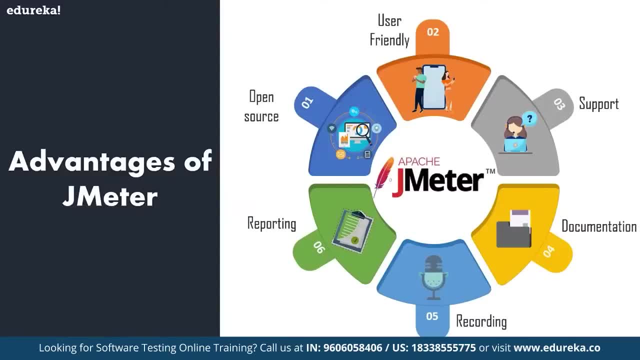 Now, because of its robust documentation, user can have a clear idea on each and every step, starting from scratch, Including installation and configuration of the test settings and generating the final report. Next up is the recording. Now JMeter allows user to record the HTTP or the HTTPS to create test plan. 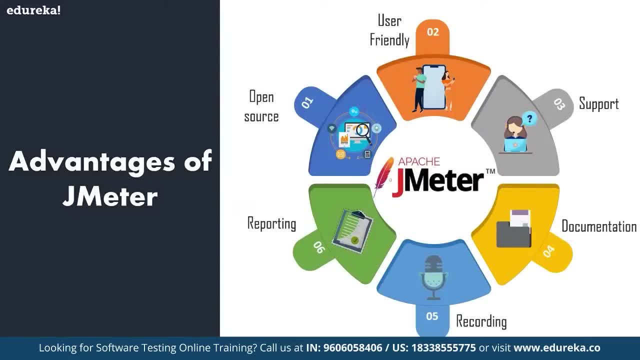 using recording facility. We use the proxy server that allows JMeter to watch and record your actions while you browse your web application with your normal browser. Finally, there's this reporting. Now. JMeter supports dashboard report generation. A host of reports are generated through JMeter. 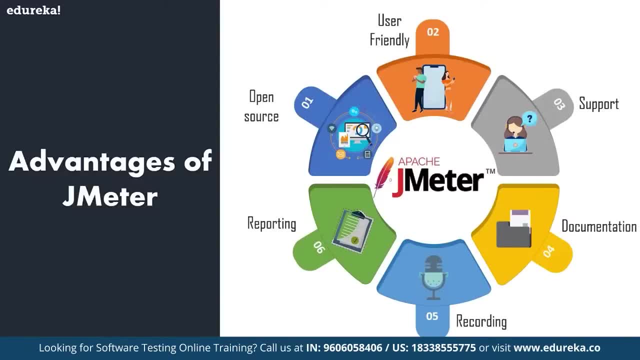 which helps the user to understand performance test execution results, And in today's session, I will teach you how to generate a report in the dashboard. Now, in the previous JMeter tutorial, I have taught you how to install JMeter and I have also showed you how it actually looks like. 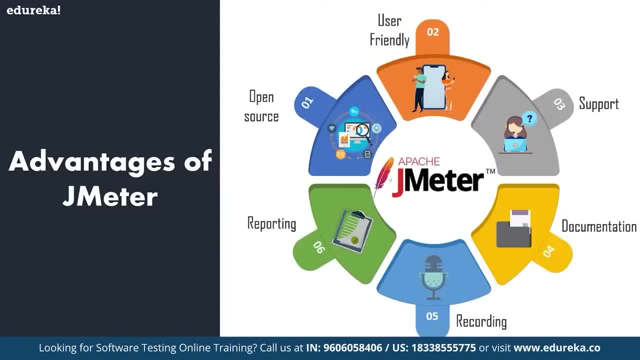 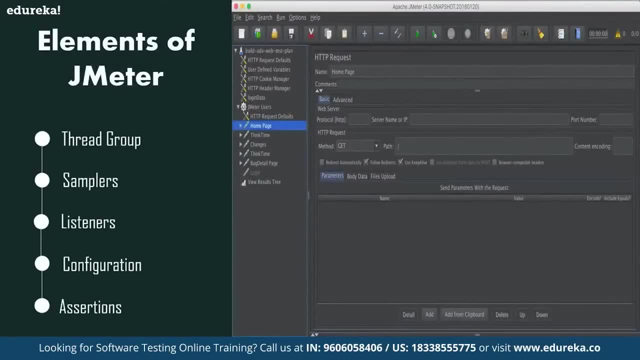 I've also discussed about some of the important elements of JMeter. Here I have added another important element in the JMeter, So let's revise about all these elements again. First of all, we have the thread group Now. the thread group is a collection of threads. 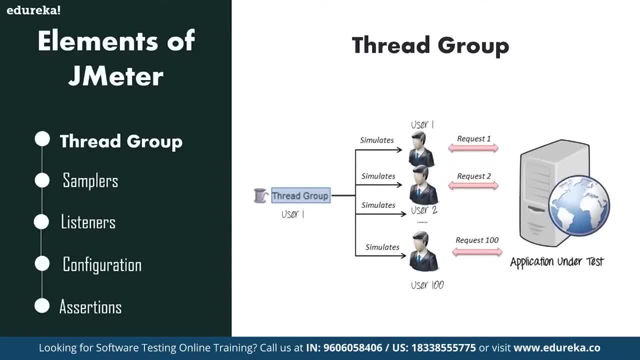 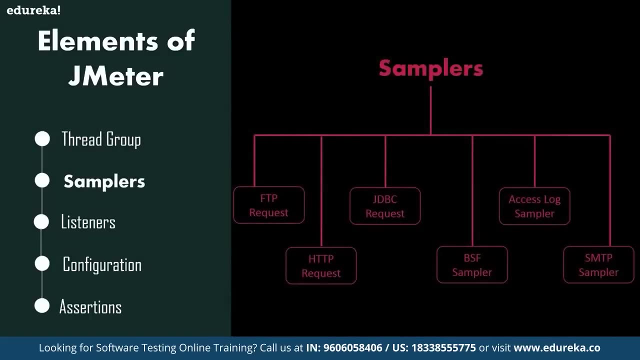 Each thread represents one user using the application under test. Basically, each thread simulates one real user request to the server. The controls for a thread group allow you to set the number of threads for each group. The next element is the samplers. Now, as we know already, 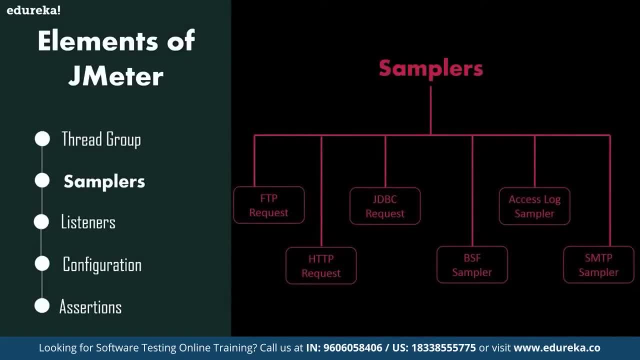 that JMeter supports testing HTTP, FTP, JDBC and many other protocols. We also know that thread groups simulate user requests to the server. But how does a thread group know which type of requests it needs to make? The answer is samplers. Now the user requests could be: 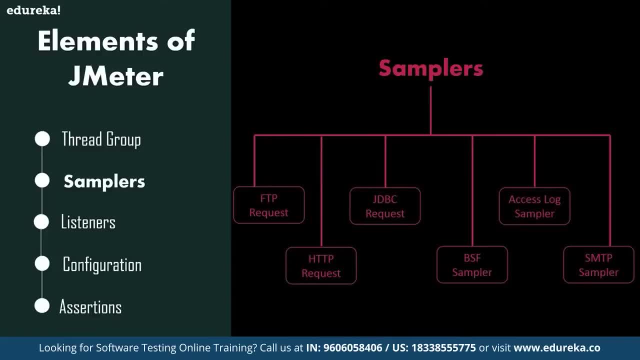 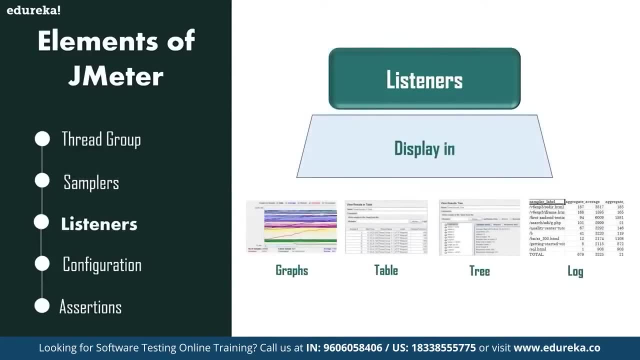 FTP, HTTP, JDBC, etc. We have also discussed about all of these requests. Next up is the listeners. Now listeners shows the results of the test execution. They can show results in a different format, such as a tree table, graph or log file. 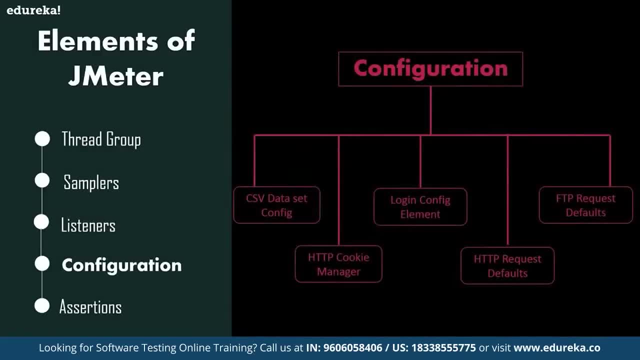 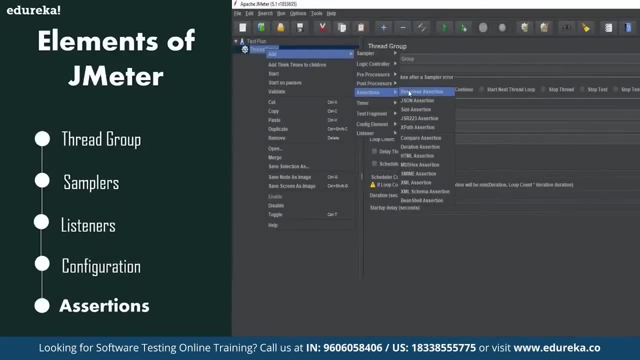 Then we have the configuration elements which set up defaults and variables for later use by samplers. Now here is another added element of JMeter for the load testing. So assertion in JMeter is used to validate response of the request that you have sent to the server. 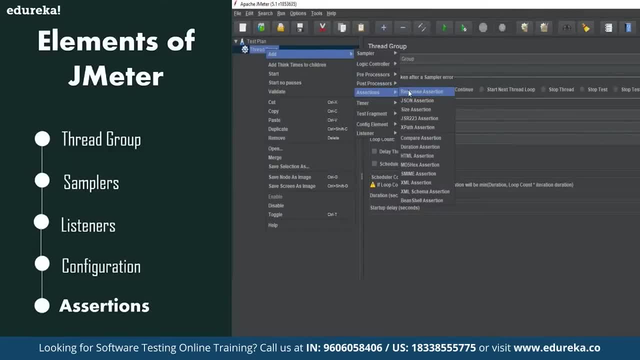 Now, assertion is a process where you verify expected result with the actual result of the request at runtime. Now if you need to apply assertion on a particular sampler, then add it as a child of that sampler. You can view assertion results by adding assertion. listener to the thread group. 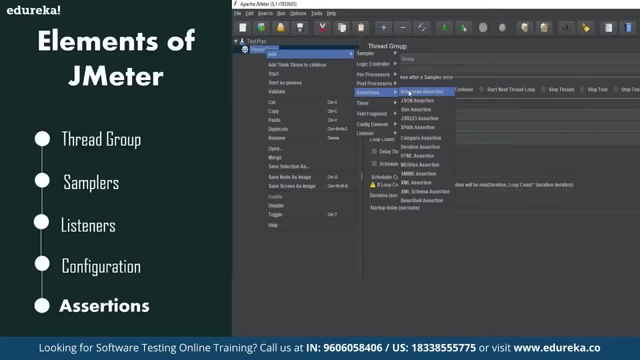 Failed assertions will be displayed in other listeners as well. So here we will be using the response assertion. So response assertion can be used to add and compare pattern strings against one or many values of server response. So here you can verify the response by using the response assertion. 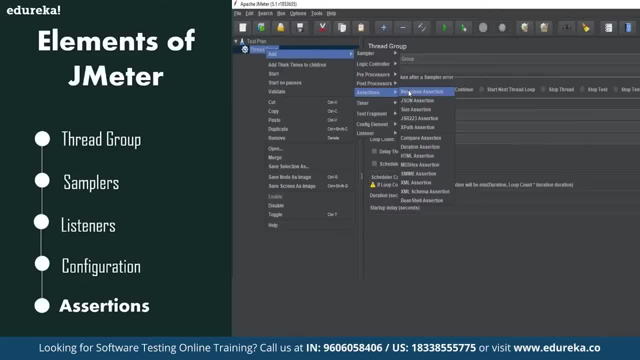 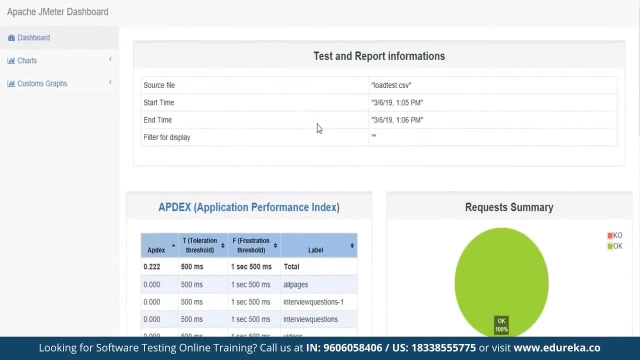 Now, these were the elements that we will be using in our load testing. Next up, I'll tell you how to generate a report on a dashboard. So this is exactly how a dashboard looks like and also the report generated here. Now, JMeter supports dashboard report generation. 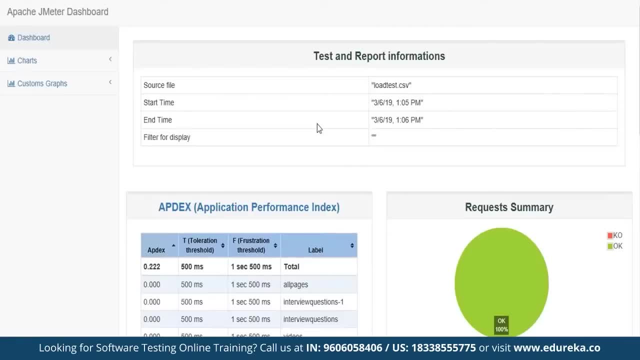 to get graphs and statistics from a test plan. The dashboard generator is a modular extension of JMeter. Its default behavior is to read and process samples from CSV files to generate HTML files containing graph views. it can generate the report at end of a load test. 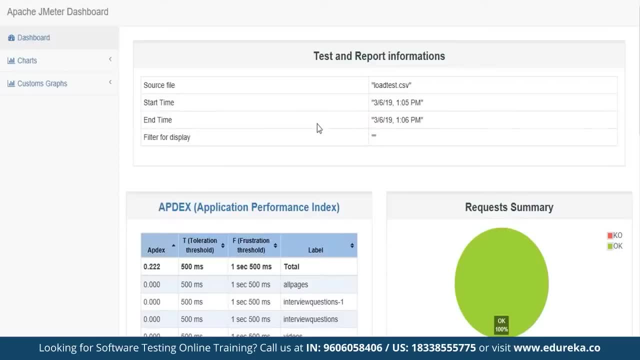 or on demand. So in my previous JMeter tutorial I have already taught you how to install JMeter and also how the test plan works. So here I'll be doing the testing in the non GUI method. So first of all I'll show you again how to create a test plan. 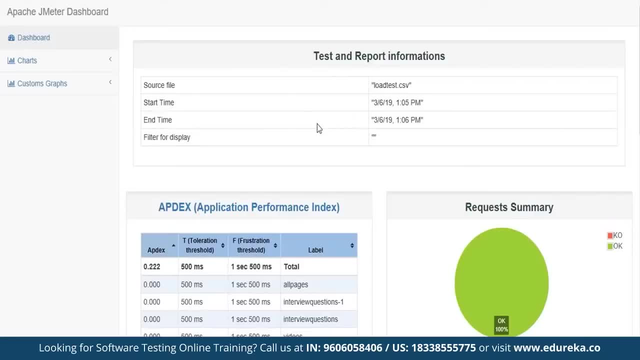 and then we will be running that particular test plan in our command prompt. in the previous one We have done it in the JMeter itself. here We will be using a non GUI method, So let's see how this works. So this is our Apache JMeter tool. 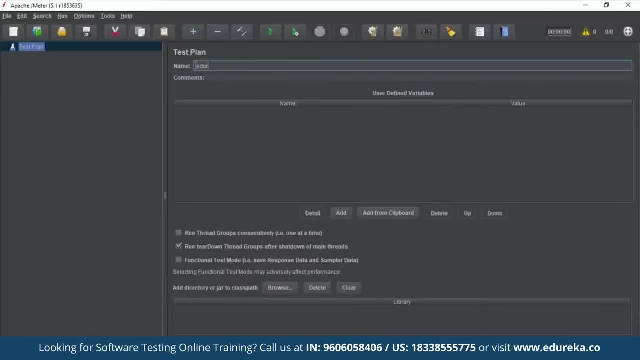 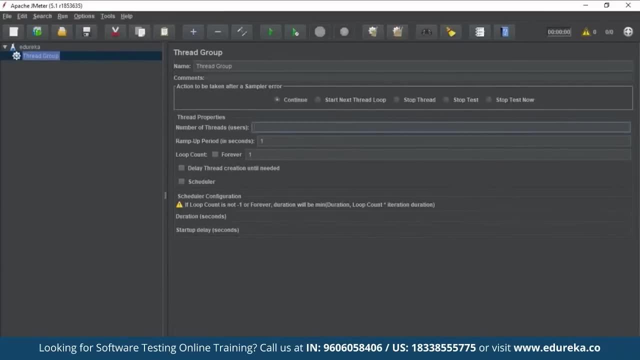 and we have a test plan here. So first of all I'll rename the test plan to edureka and then I'll create a thread group. Now, inside the thread group I'll put some number of threads and also increase the loop count. 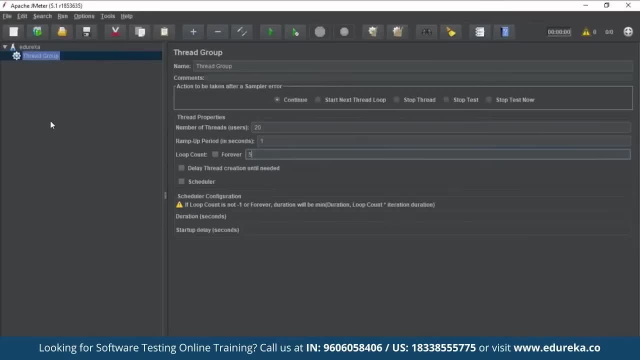 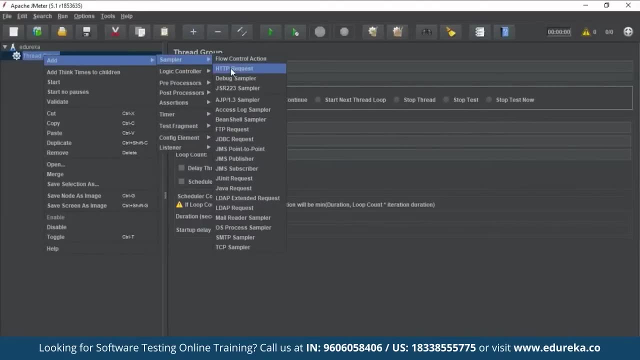 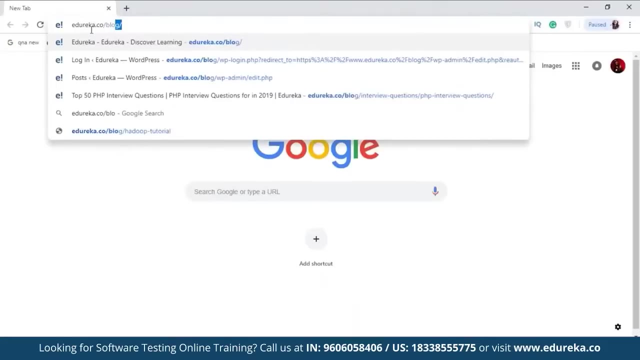 So here I have added the number of threads or the users as 20 and have increased the loop count to 5.. Now I'll add another sampler, that is the HTML HTTP request. So let's open our edureka blog website. So here we go to the edurekaco slash blog. 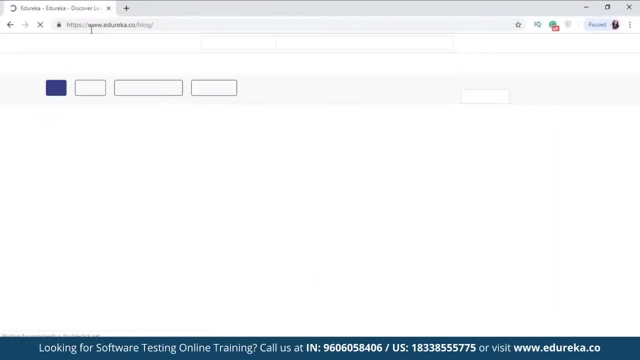 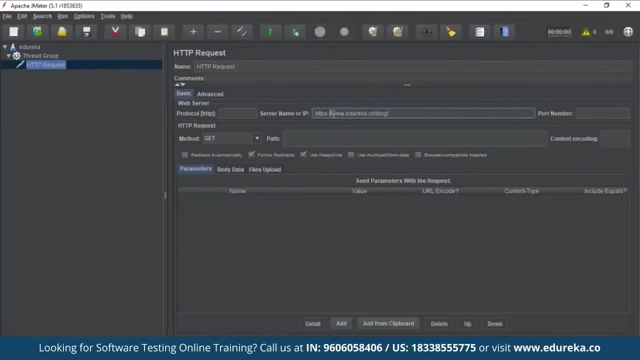 So this is the website for all the edureka blogs. So this is our server on which we are performing the testing, So we'll copy the URL and put it on the IP address Now, as you know that we are not supposed to put the HTTPS. 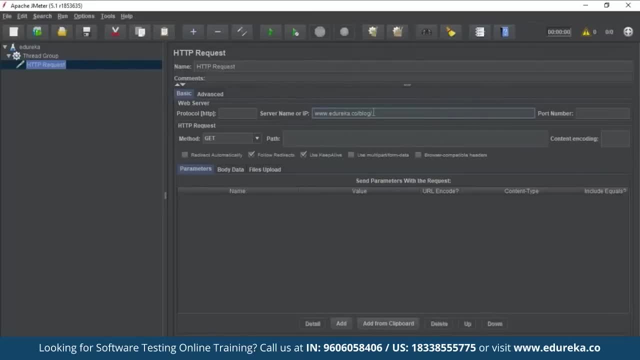 So we will remove this from here and also the path will be added in the path section. So we'll copy it from here and put it in the path section. Next up, I'll create another HTTP request now inside our edureka blog website. 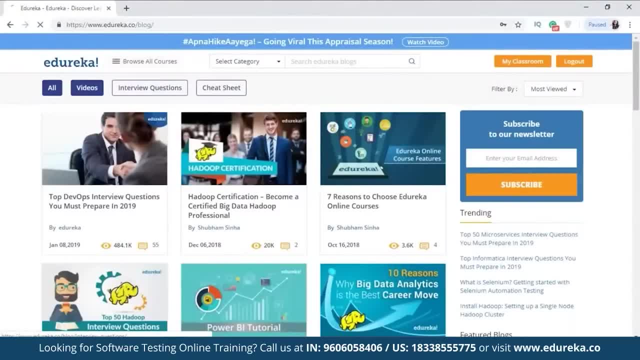 We have different sections, such as the all videos, interview questions and cheat sheet. So these are the different paths that lead to different sections inside the website. So I've added one path that goes to all the blogs next up. I'll just add another HTTP request. 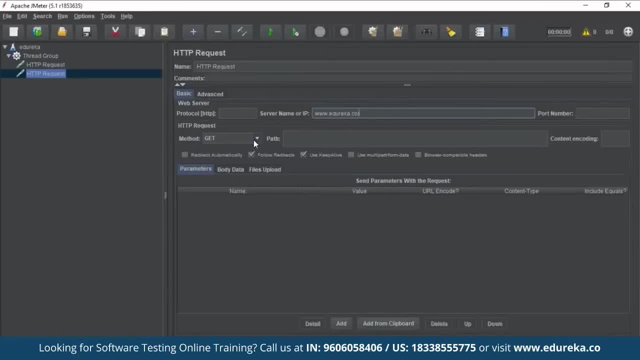 where I'll put the website as edurekaco slash blog and the path I'll set to the videos. So I will copy the path from slash videos and put it in the path section and save it as videos. I'm also saving the first one as all pages. 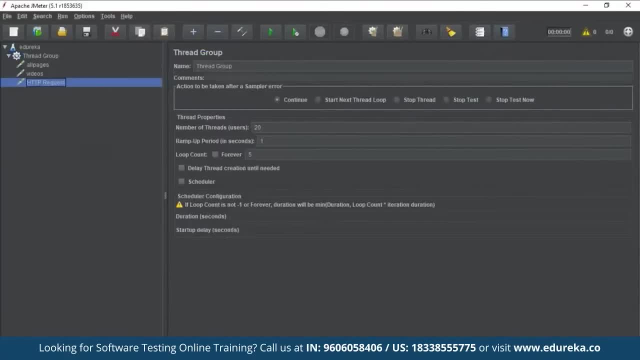 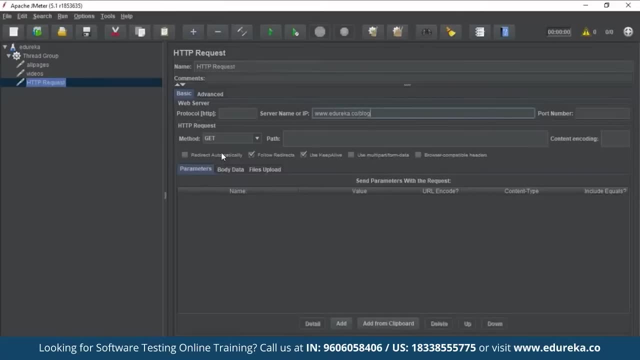 Next up I'll add another HTTP request and here I'll add the path to all the cheat sheets. So here I'll add the server as edurekaco slash blog. So I'll add the path as the interview questions. I'll also change the name of this HTTP request. 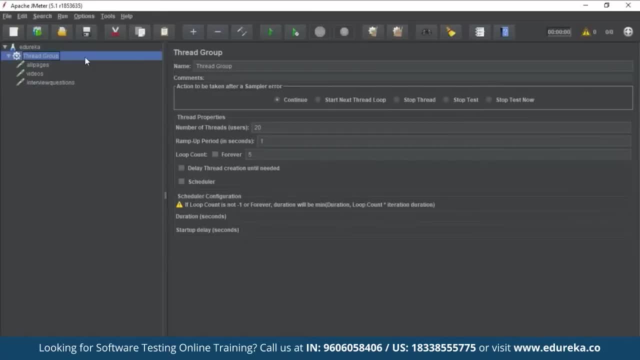 to interview questions. So once we have added all the HTTP request, we will save this as our edureka dot jmx file. So I'm saving it inside my load test folder. So I'll rename it as edureka edureka dot jmx. 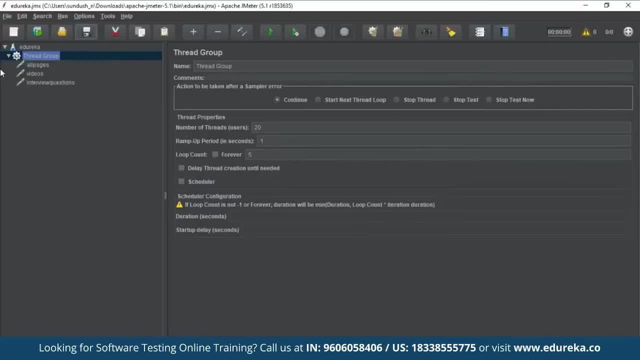 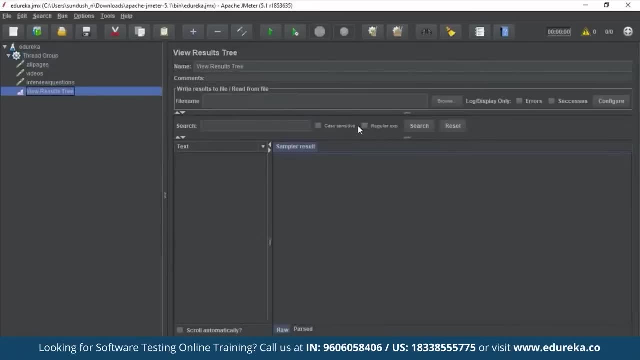 and I'm saving it inside the load test folder. Now, in order to check if the test is running properly, Let's add a listener where we show the results in the tree format. So once I've created this view results tree and if I run this test, 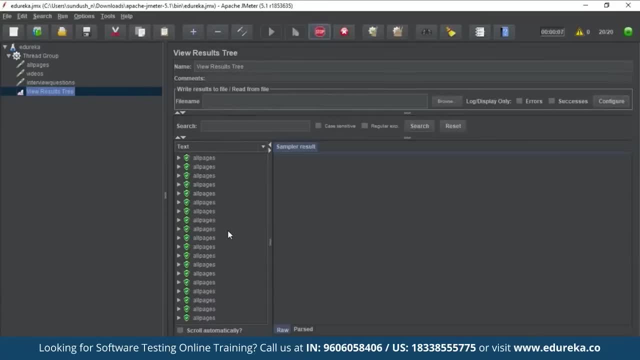 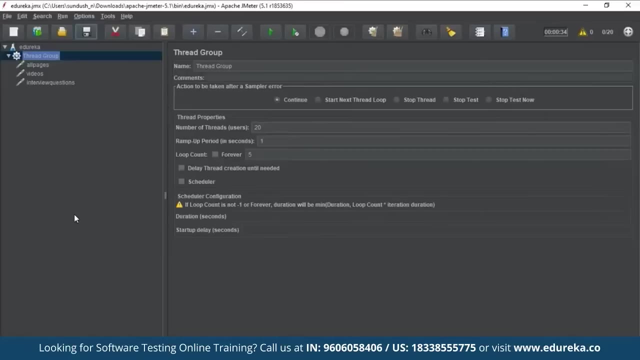 I'm going to see that all the tests are running perfectly and the status is okay for all of these pages, So you can see that the test is running completely fine. So now let's remove this and run this test in the non GUI mode, and for that we have to clear this view results tree. 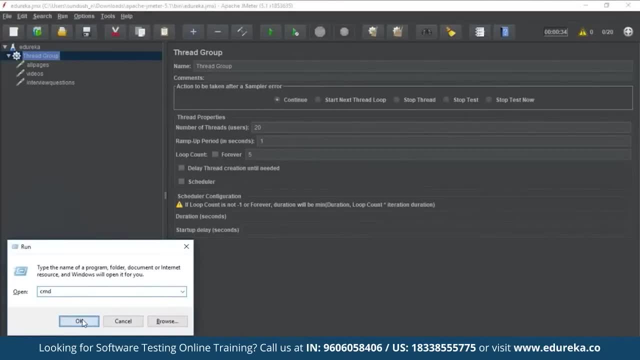 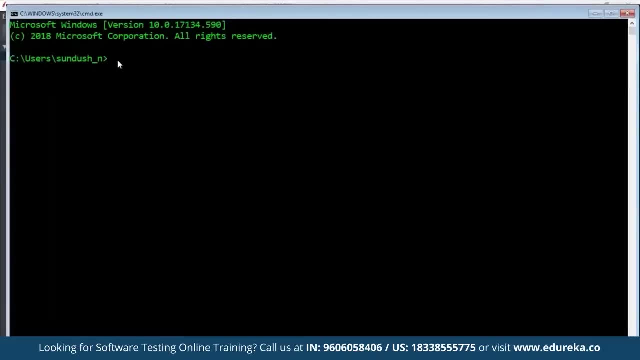 and also we have to go to the command prompt and check how we can run this test in the non GUI mode. So now that our test plan is ready, We will be shifting to our command prompt Now, inside command from. the first thing that you need to do is specify the path. 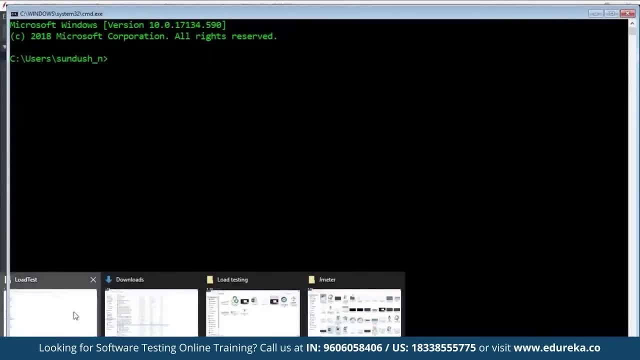 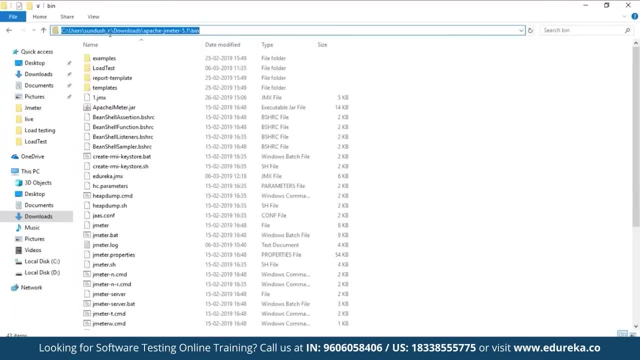 So first you have to go inside the J meter bin. Now this is the path that takes me inside my J meter and the bin folder. So now I'm inside my J meter bin folder and here I'll be running the command line for performing the test. 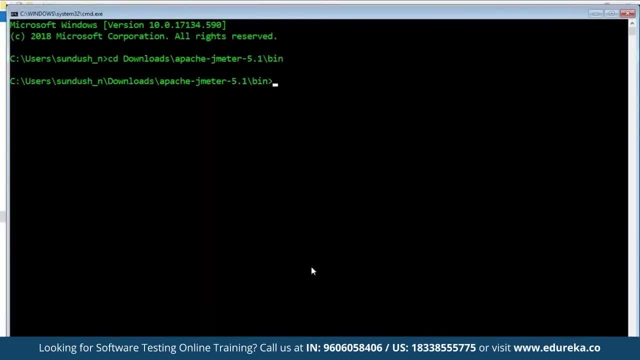 Now the command for performing the load testing is J meter. hyphen n, hyphen T. Now what is this? hyphen n? the hyphen n represents the non GUI mode and the hyphen T is used in order to specify the location for your test script. 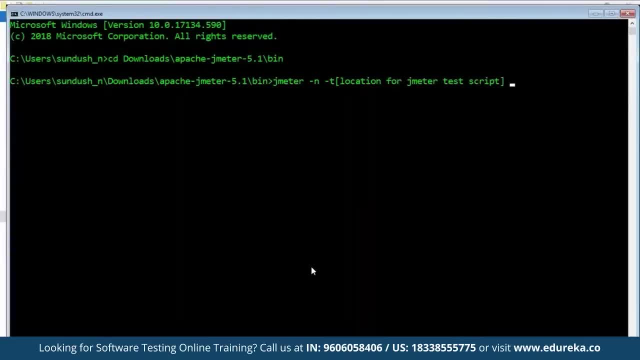 So once we have specified the location for our test script, then we have hyphen L. Now this hyphen L is used to specify the test location for our output result. Now the minus L is used for the location of the result file. Now, here we have the minus N for the non GUI minus T. 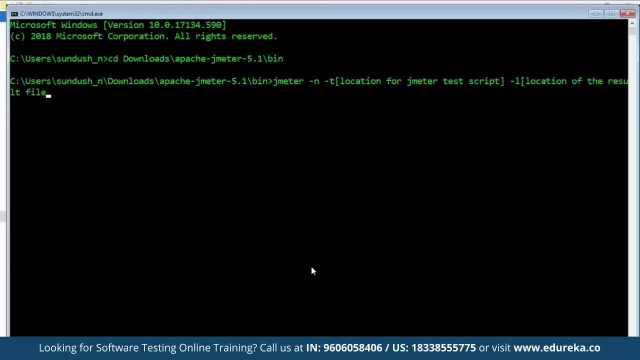 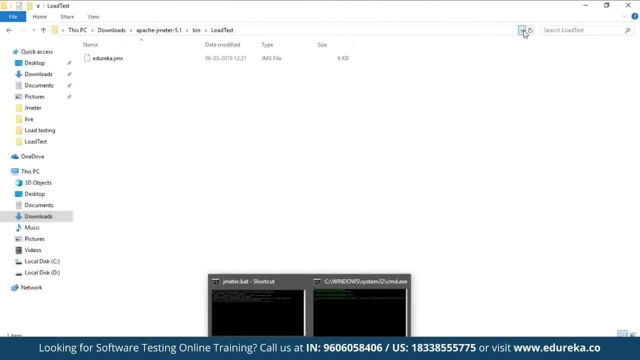 for location for J meter test script and the L for the location of the result file. So now here we have to specify the location for both. So inside the load test folder I have my edureka dot JMX, So I have to copy this path and specify it after hyphen T. 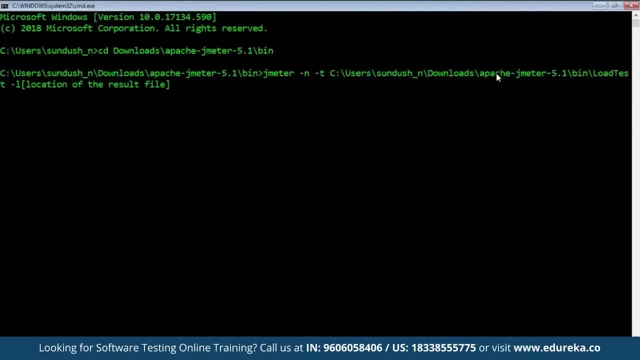 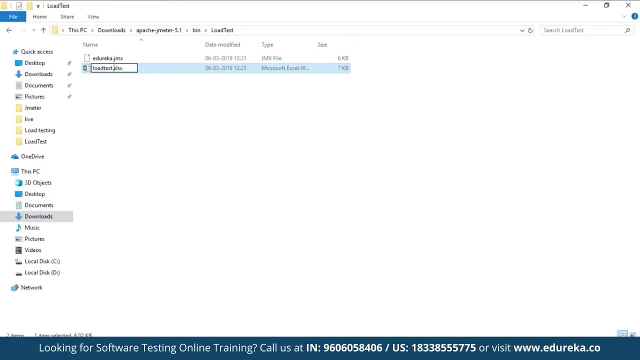 that is, specify the test script location. So here I have specified the test script location and the name of the file would be edureka dot JMX. Now, inside my load test, I have created a dot CSV file which I'll name it as load test dot CSV. 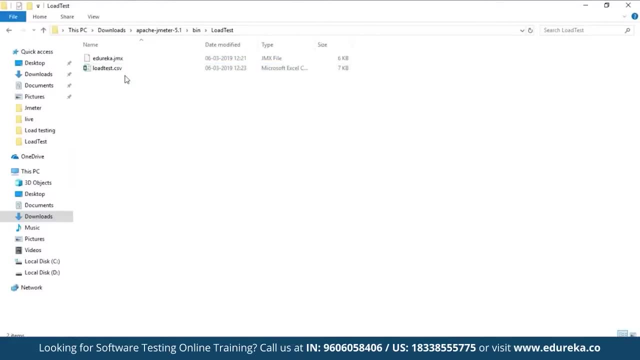 Now this load test dot CSV file will hold all my test results. So now I have to specify the location for my result file, which is the load test dot CSV file. So after hyphen L, I'll be specifying the location for my result file. 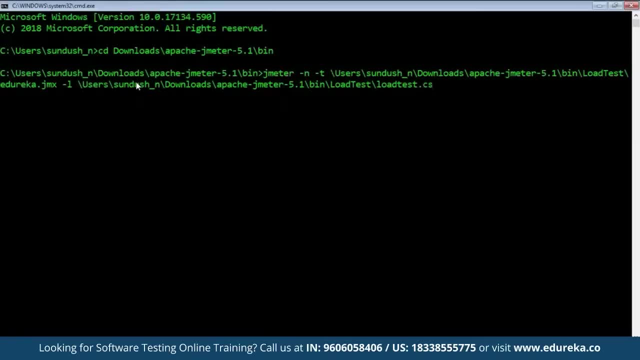 So now this is the command for running the test in a non GUI format, where I'll be using the test script file and also the result file location. So now, once we run this command line, we can see that the tree has been successfully created and the test has started. 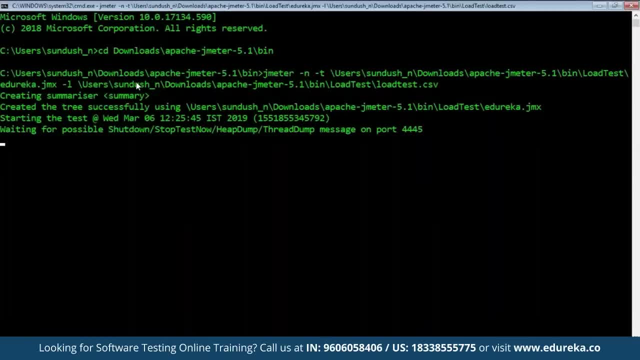 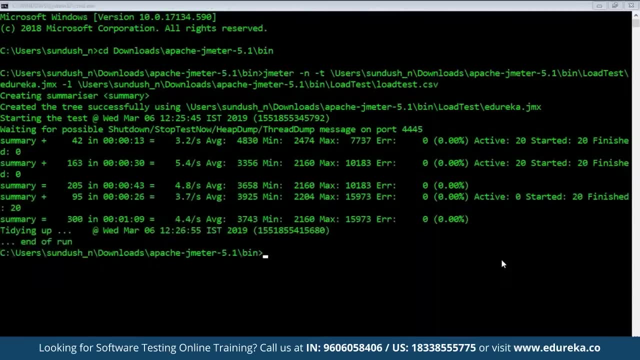 So now this will take some time and the process will continue because we have used 20 users and also the loop count will go on for five times. Now, once you see end of run, it means that the test is completed. Now, when we go back to our load test folder, 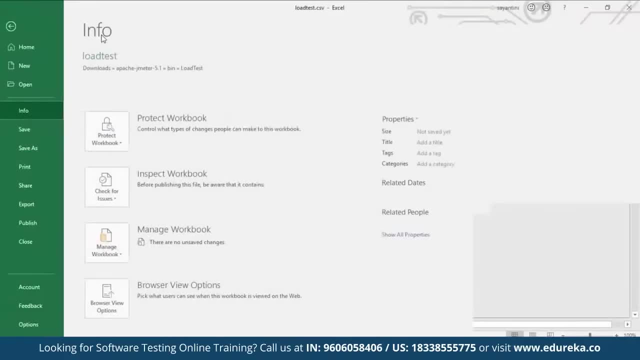 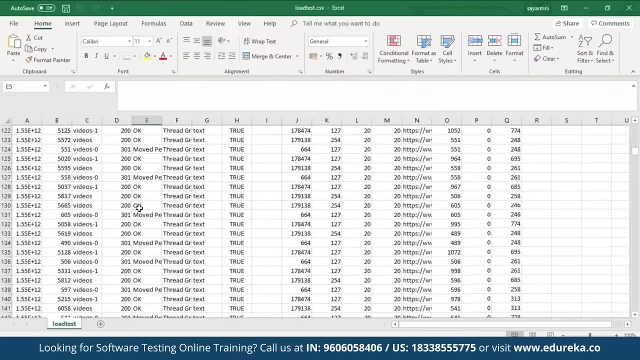 and open our load test dot CSV file. So now here you can see that the entire test results has been generated inside our load test dot CSV. So it shows that the test has been performed successfully and it's all okay. So it has been completed successfully. 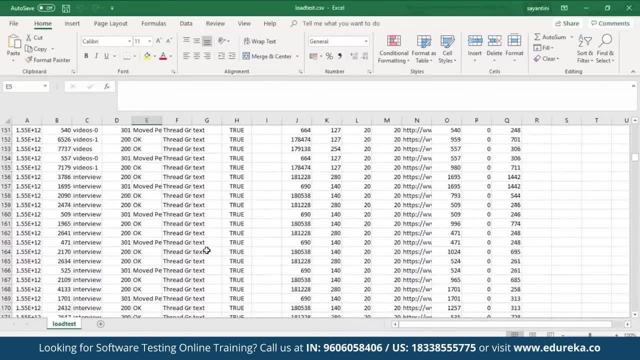 and there has been no error generated either. So now this is exactly how you perform your testing in the non GUI method. So we have just used our command prompt in order to run the test. finally, and also, we have got the entire results output in the dot CSV file. now 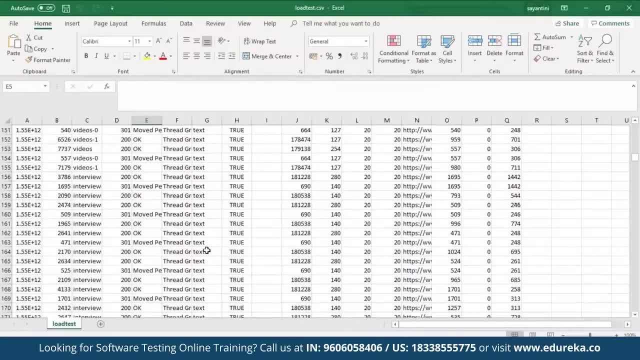 in order to have a better understanding of the output of your test, You would need a dashboard. now, in dashboard, We will be creating different sorts of graphs that will help you understand the performance of your website even better. So now let's move on and see how we can generate a report on our dashboard. 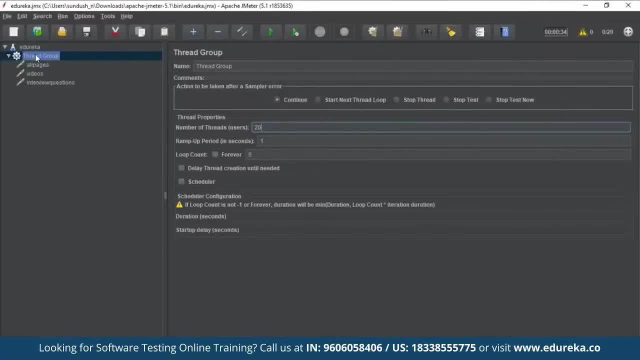 Now, in order to generate a report in our dashboard, we follow the same procedure. We go to the J meter, create a test plan. here I'll be using the same test plan where I have used the edureka block for our website and also all the three HTTP requests. 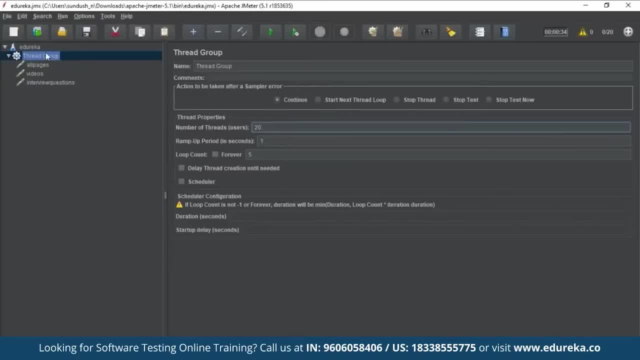 that have created for our all pages, videos and interview questions separately. Now, these are some of the elements that we had already added. now, for the dashboard, We will be adding another new element known as the assertion. Now, basically, it will help us to add. 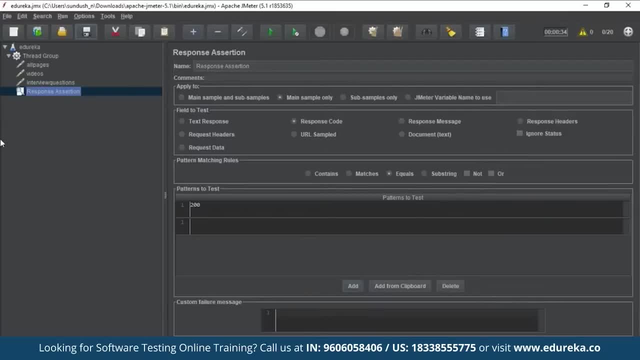 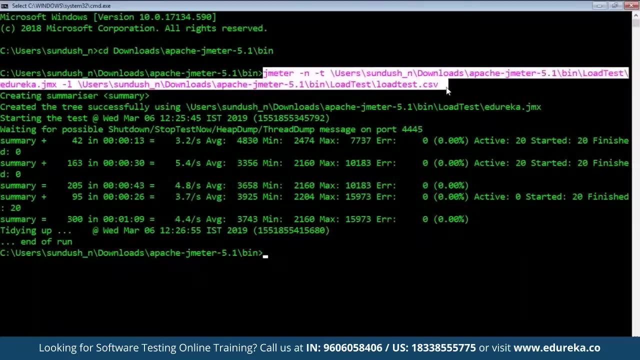 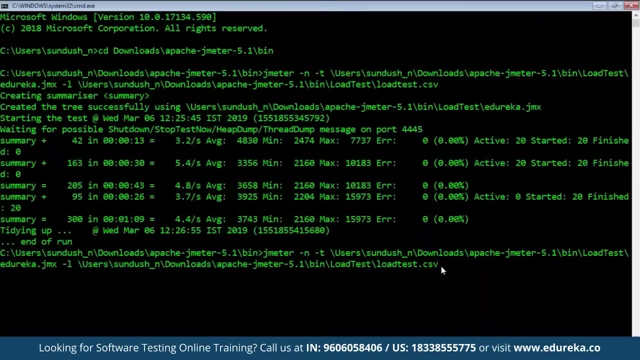 and compare the pattern strings against one or many values of server response. Now, in order to run the test and generate the report on the dashboard, The command line is almost similar, with two more added elements here. So initially we had J meter, hyphen n, hyphen T and hyphen L. 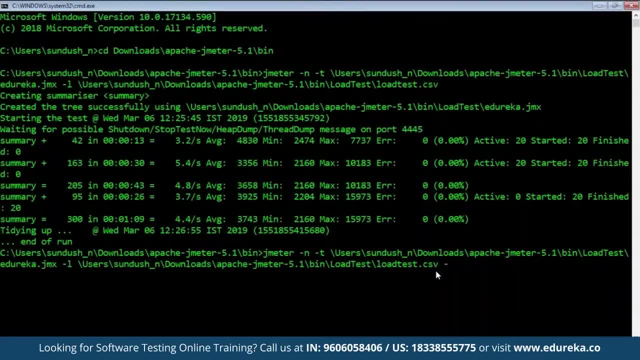 Now, here we will be adding two more extra things, that is, the hyphen E and the hyphen O. Now the hyphen O is used for the output file. Now for the output file. we will go back to our load test folder and create another folder. 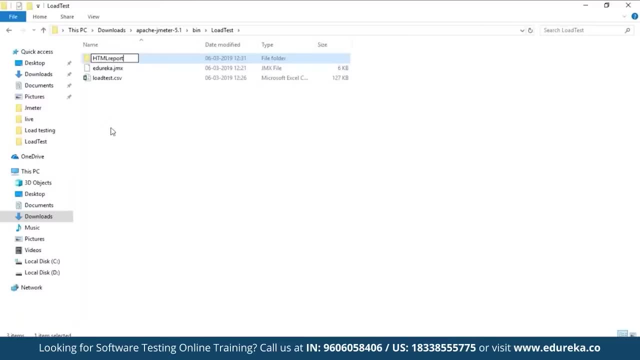 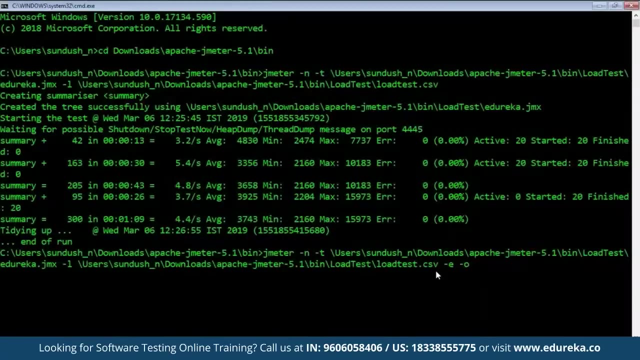 Suppose I'm naming the folder as HTML report. Now this will give us my dash port report, So I'm creating this output folder here. Now we have to specify this path after the hyphen O. Now the command remains the same. where we have J meter, hyphen n for the non GY. 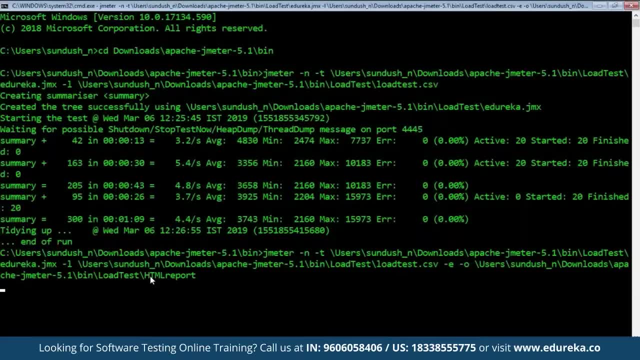 then we have hyphen T for our test script location, which is our edurekajmx, and then we have the hyphen L for our dot CSV file, and then we have hyphen E, hyphen O and we specify the location for our HTML report. 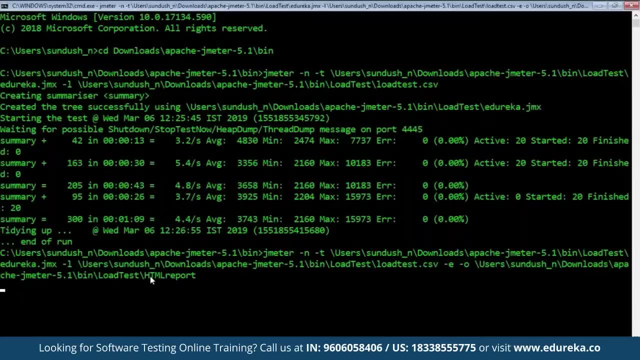 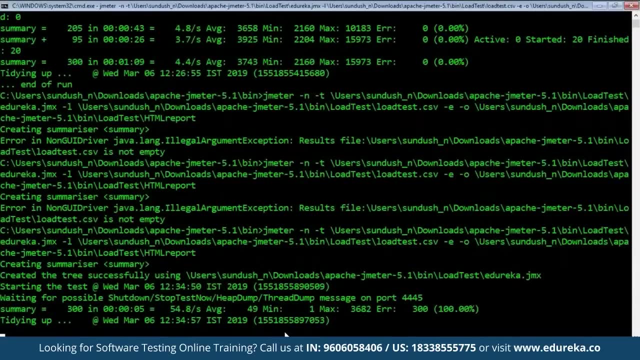 So this is the location for our HTML report. Now, once we run this command, we can see that again, we are successfully creating the tree and then starting the test. Now, this will also take some time for the report to get generated. Now, once we run this command line. 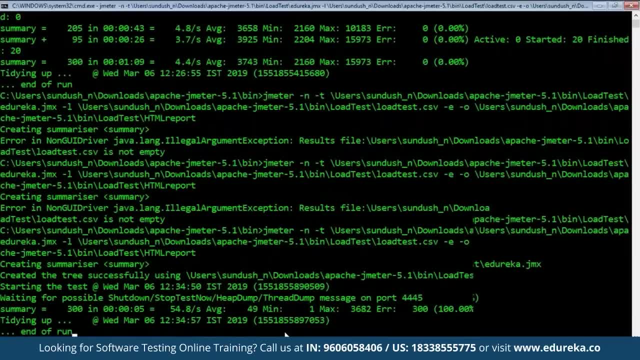 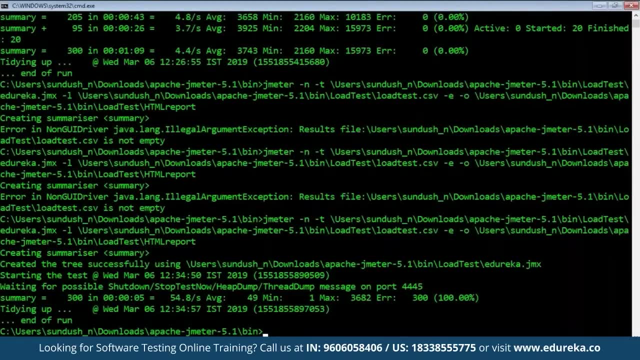 we will also get the CSV file where the report is generated in the tree format, and also we will have a separate dashboard created where we will have the entire output generated in the form of graphs. Now the J meter supports the dashboard report to get the graphs and statistics from a test plan. 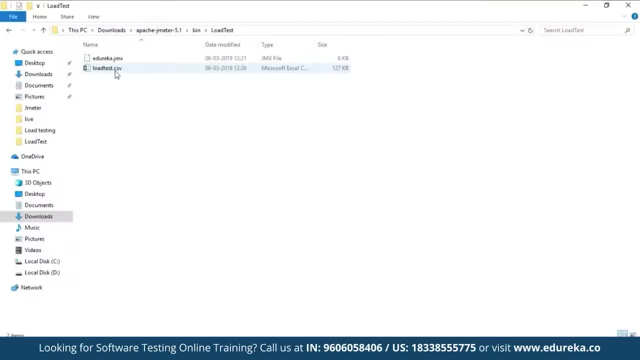 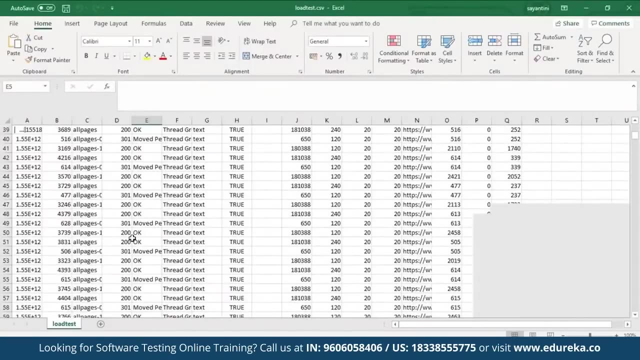 So now that the test is done successfully, once we go back to our load test folder and we open our dot CSV file, we can see that the report has been generated here. Now, moving on, if we go back to the folder and open our HTML report folder, 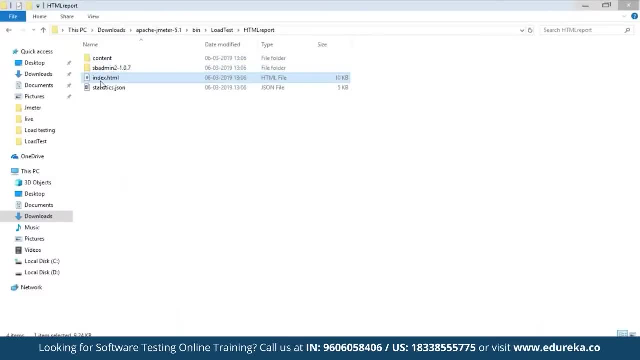 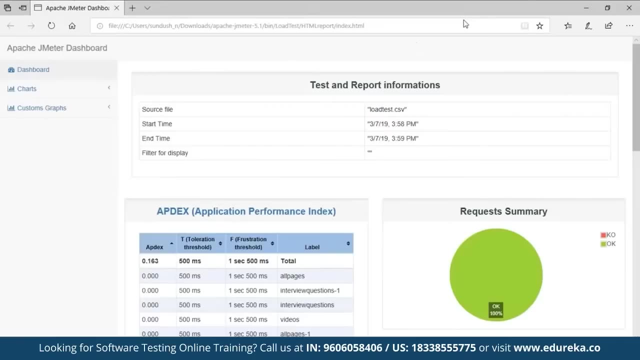 we can see that there is an index dot HTML created. Now this is the dashboard that has been generated. So in this dashboard we have our entire report of our test, generated in the form of graphs and statistics. So you can see that we have the output of our test plan. 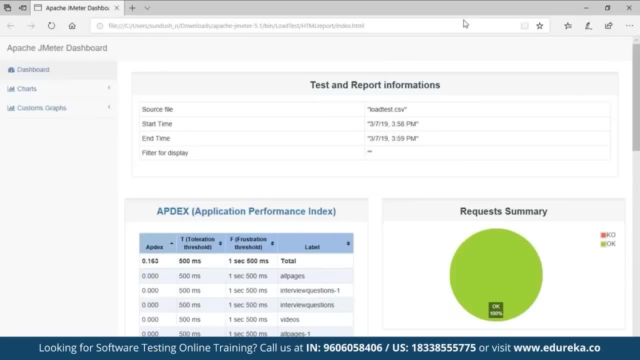 which shows that it was all okay, because there was no error inside our test plan. We have specified the paths correctly and thus the test plan has occurred successfully. Now the dashboard generator is a modular extension of the J meter. Its default behavior is to read and process samples. 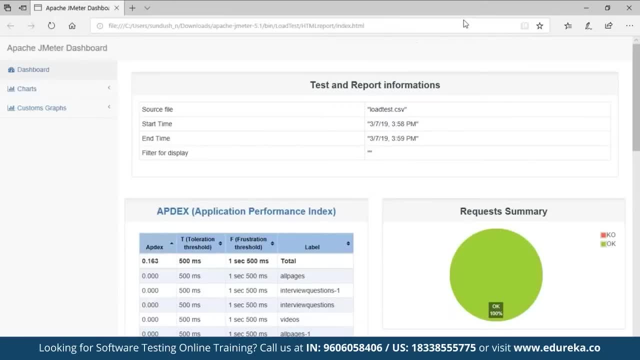 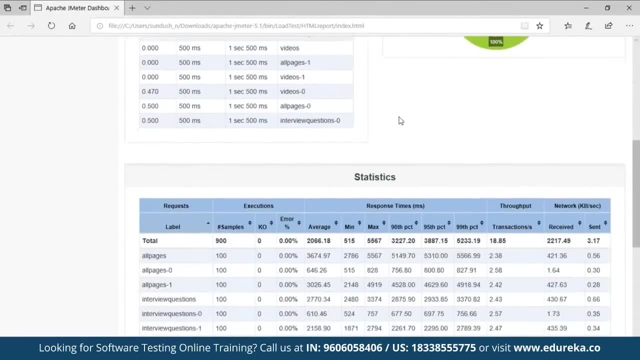 from CSV files to generate HTML files containing the graph views. So here you can see the graph that shows 100%. okay, because there has been no error in our testing. We also have a statistics table, providing one table, a summary of all metrics per transaction. 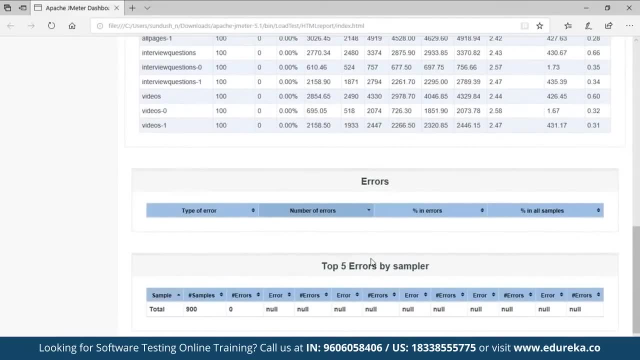 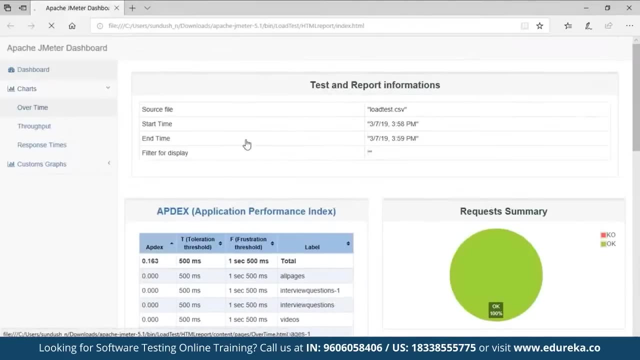 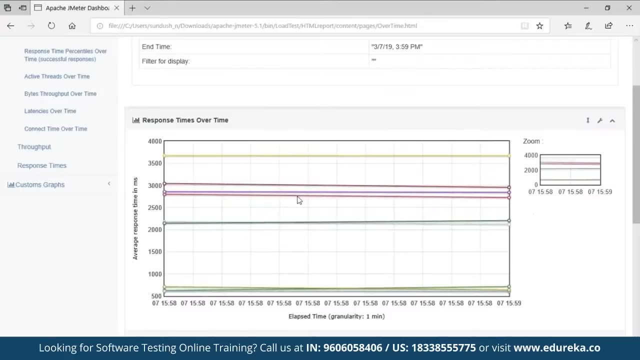 and then we have the error table, providing a summary of all errors and their proportion in the total request. Here we do not have any particular error. Now, not just that, we also have zoomable chart where you can check or uncheck every transaction to show or hide it. for like the response time, 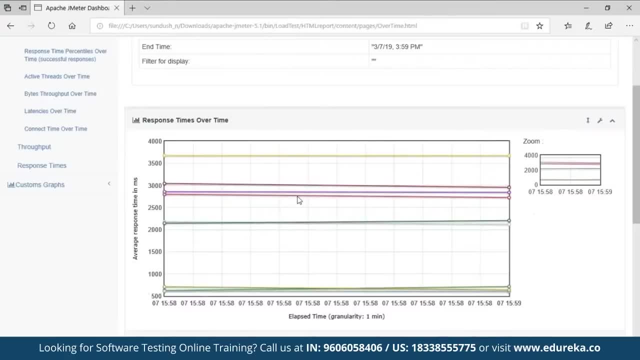 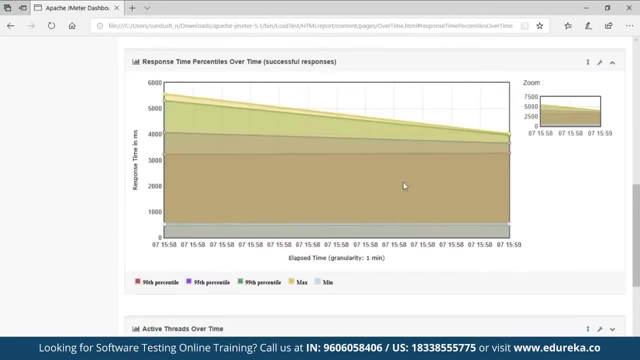 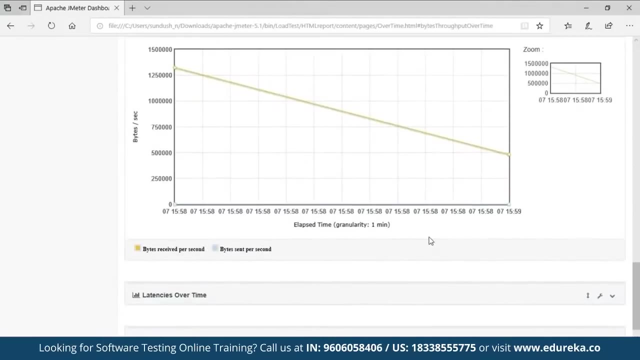 over time, where it includes the transaction controller sample results. We also have the response times: percentile over time, which shows the successful responses only. then we have the active threads over time, bytes throughput over time, which ignores transaction controller sample results. Then we have latencies over time. 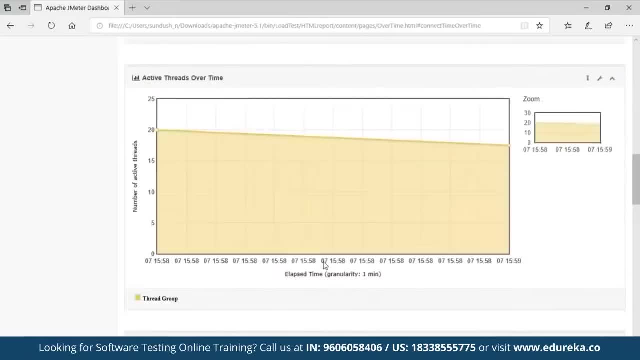 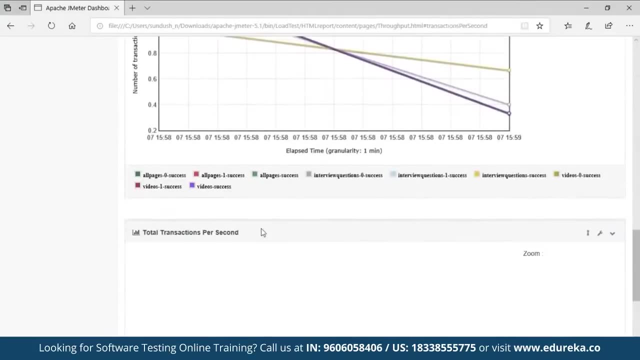 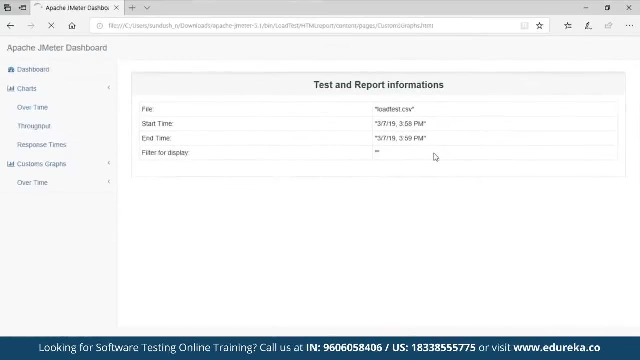 connect time over time, which includes the transaction controller sample results. Then we have the hits per second, response codes per second and transactions per second. We also have the latency versus request per second and response time over. So we have all these different forms of shots available. 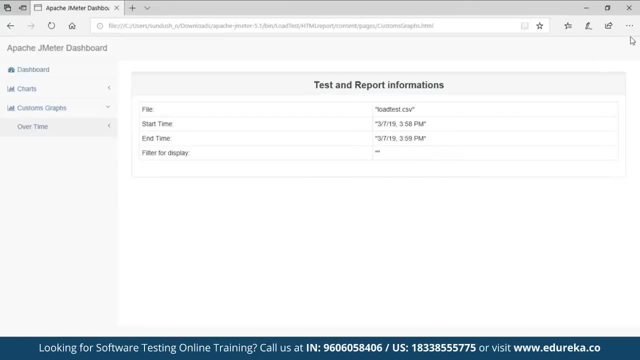 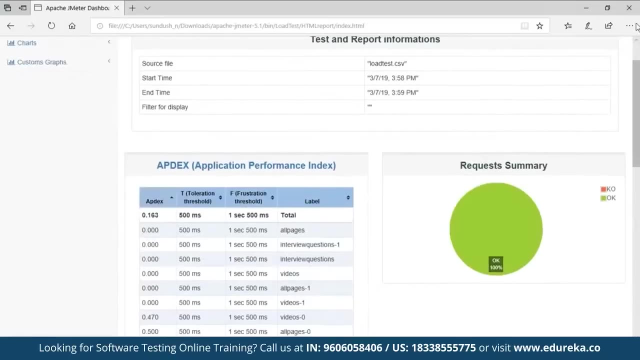 in our dashboard that will give you a detailed report about the test that has been performed on your website. This actually gives you a visual satisfaction of whatever test you have performed and it's always easy to understand with the help of these graphs and statistics. and you get to easily understand. 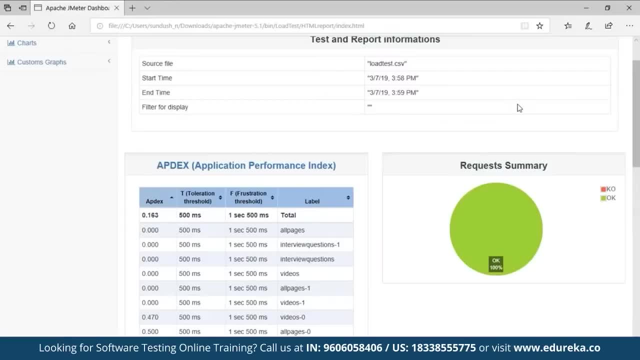 how well your website have been performing. not just that, we also have custom graphs here, which will let you have the graphs the way you wanted to, according to the report that has been generated. So this is exactly how Apache JMeter helps you in performing load testing on any such website. 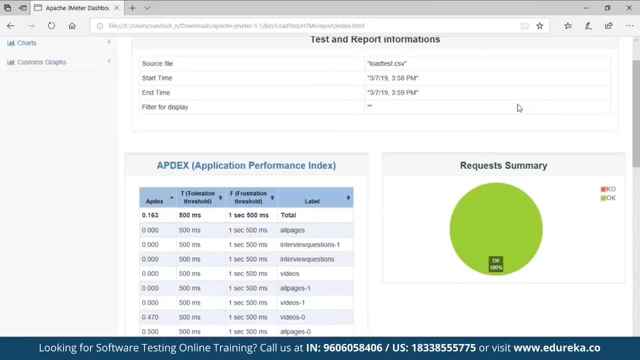 So this was the non GUI method of float testing with the help of Apache JMeter, and also we have seen how we can have a better version of outputs generated in the form of a report in the dashboard. here We have graphs and statistics that will easily help you know. 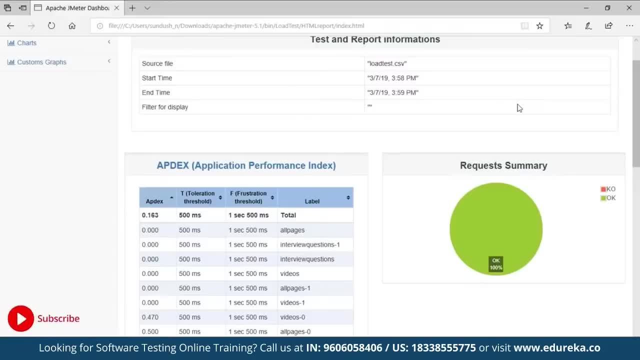 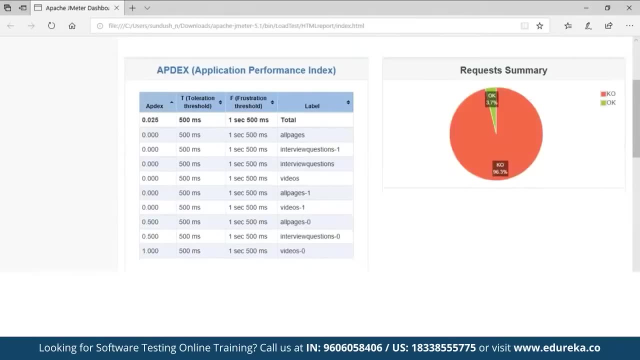 about what kind of status you are getting after the test has been completed. It completely shows you if there is any error or if the status is completely okay. now, in case there is any error, there will be false in place of true, and also you will get to see a red and green graph. 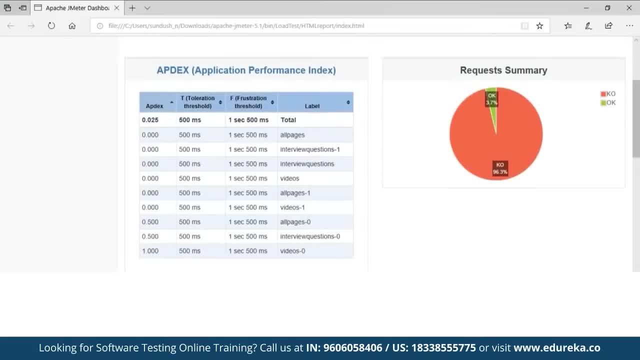 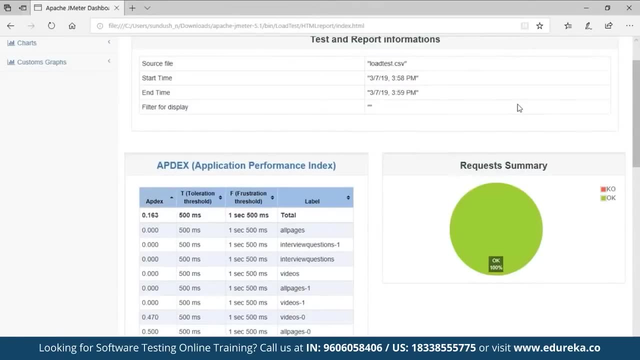 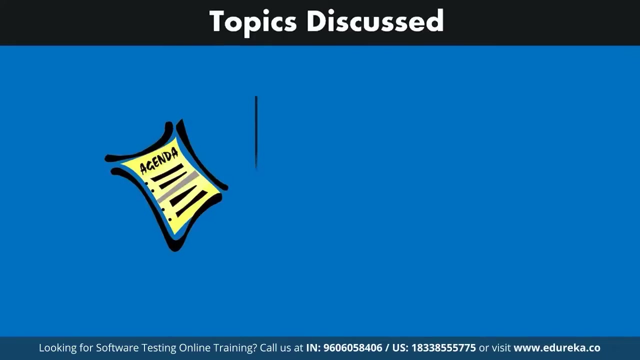 wherever there is an error, It will show you something like this, where you'll also get to see the error in the test. So now this was all about performing load testing using the Apache JMeter tool. So first of all, we will be going through an introduction. 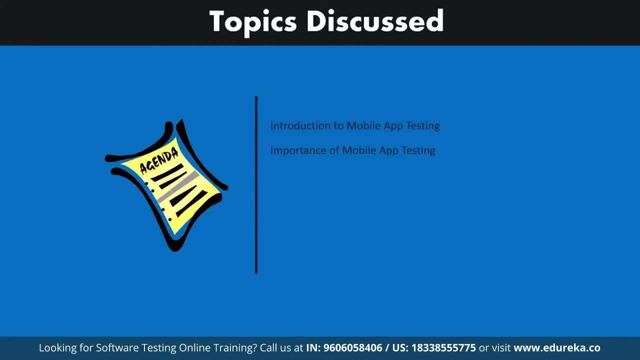 to mobile application testing, and we will also discuss the importance of the same. next, We will be actually discussing the approaches to mobile application testing, which is basically manual testing versus an automation testing comparison. next, We will be also discussing the advantages of mobile application. 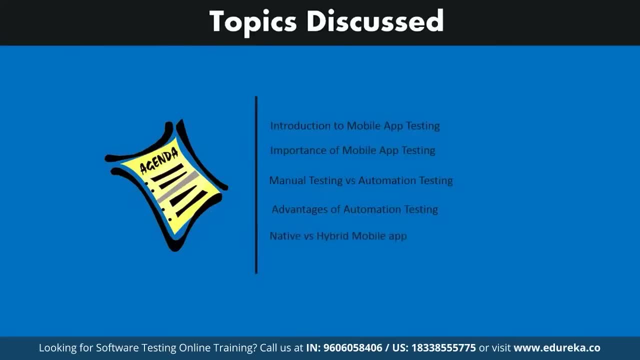 Testing to an automated approach and in the end, we will be discussing the differences between native, hybrid and web applications. and in the end, I will also give you a small demonstration as to how mobile applications are tested using the small tool called Appium in this demonstration. 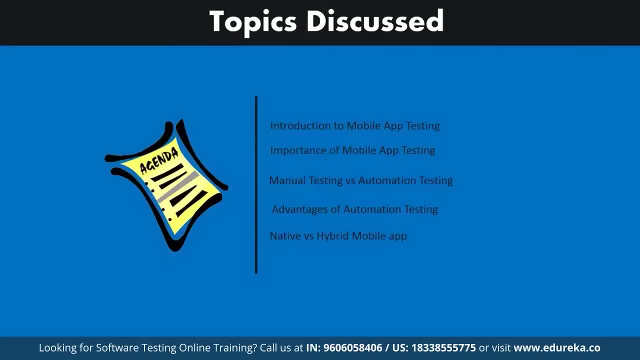 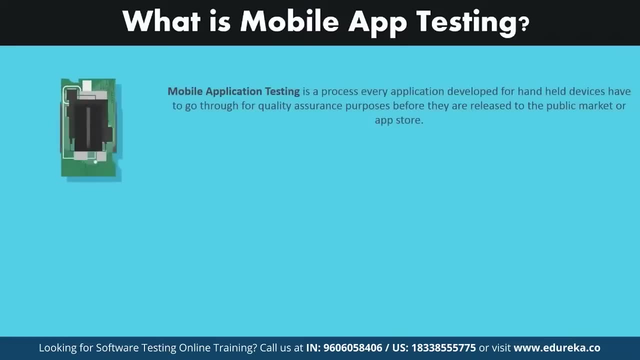 I will not teach you how to install Appium. that is for a tutorial sometime later. Okay, Now let's get started. So what exactly is mobile application testing? Well, mobile application testing is the process every application developed for handheld devices It has to go through. this, obviously, is to assure 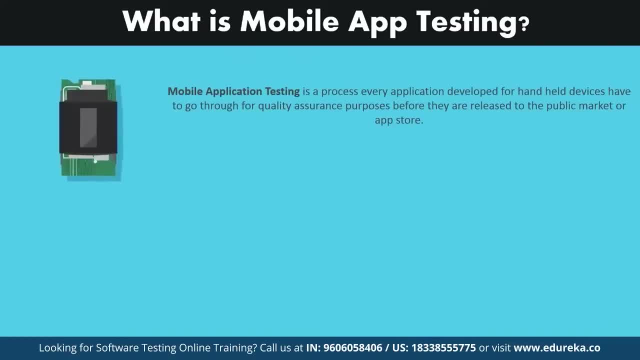 a certain level of quality before an application is released into the marketplace, also commonly known as the App Store. Now, this App Store is known in different names on different operating systems. For example, on all Google based operating systems for handle devices, that is, Android, the App Store is known. 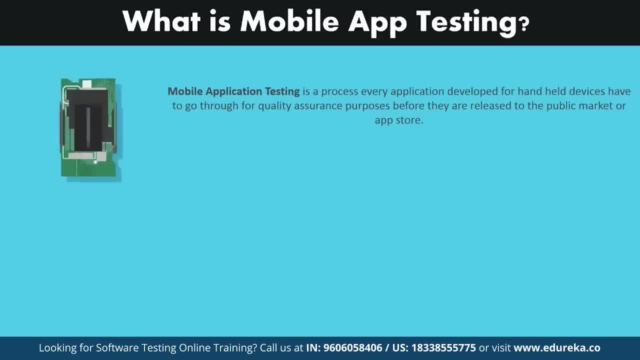 as the Play Store, while on iOS devices It is simply known as the App Store. now, mobile application development life cycle generally tends to be much shorter than the others, Like desktop apps. Hence these applications heavily depend on mobile application testing for their success. applications get tested on the basis of various parameters. 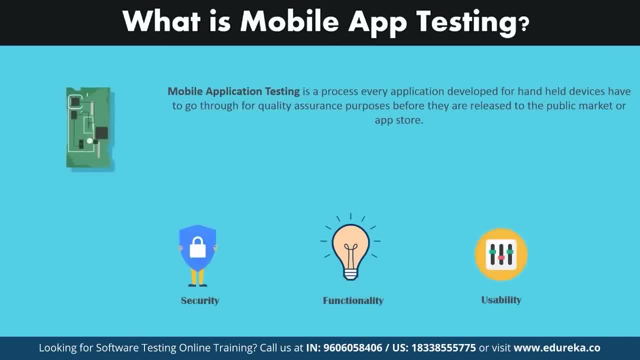 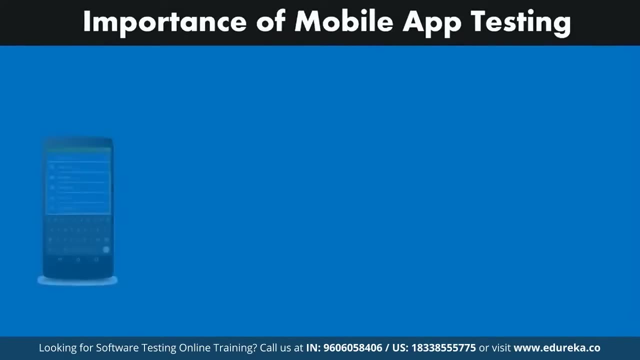 like security, their functionality, usability, etc. This increases the general efficiency of the application on all fronts, while also increasing the reliability factor amongst users that use them. Now let us discuss the importance of mobile application testing in today's era. How does a user generally decide which app to download? 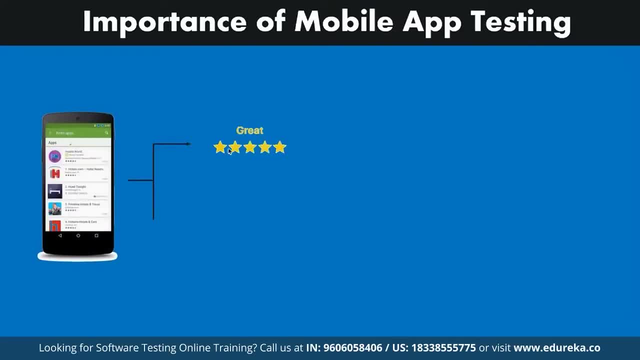 for a certain purpose? 10 years ago, this question could have generated a host of answers, depending on personal choice and what not. today, It depends on two things, the first being ratings and the second being reviews. daily, mobile phone users install new applications on the basis of ratings and reviews. 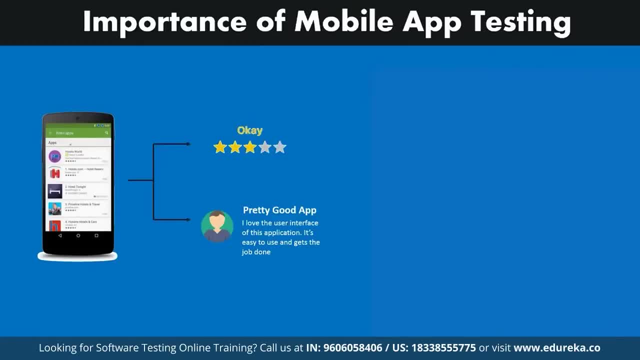 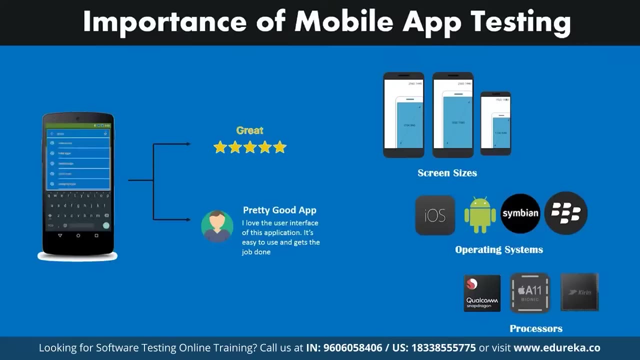 which are directly related to how well your application performs. This has made mobile application testing ever so important. with the host of mobile phones out there, with the different operating systems, screen sizes, processing capacity testing has evolved into a mandatory process And the software development process. now new features keep users. 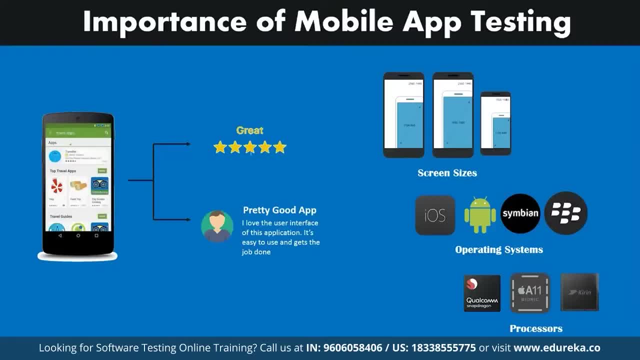 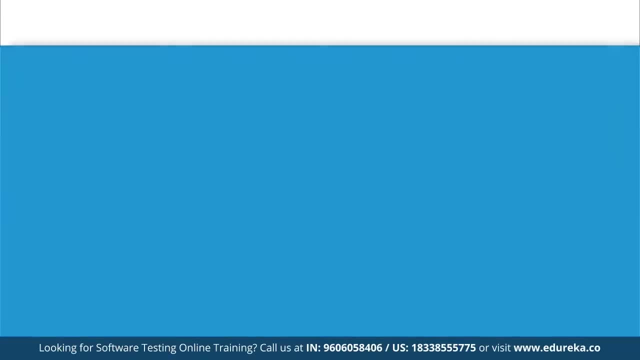 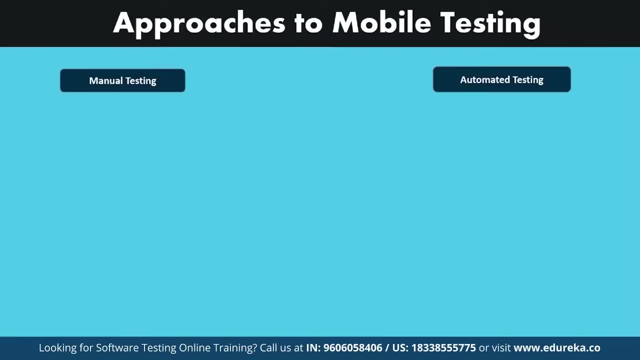 entertained, while quick bug fixes make sure that nobody uninstalled your app, making testing an essential process for an app survival on the said Marketplace. Now let us discuss the approaches to mobile application testing. Well, there are two different approaches for testing mobile applications on the basis of how they performed. 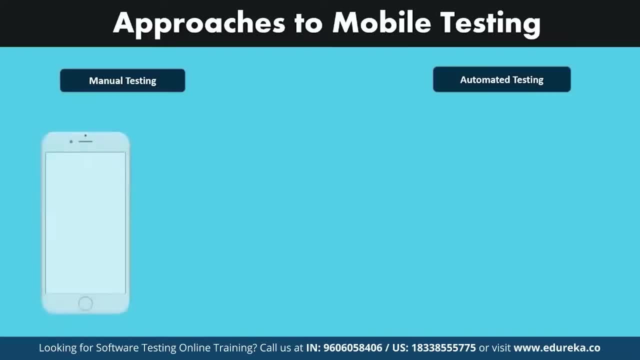 namely manual testing and automated testing. manual testing, as the name clearly suggest, is a human process majorly focused on user experience. analysis and evaluation of the application- functionality, security, usability- are done through the medium of a user in an explorative process. This ensures that your application lives up to a standard. 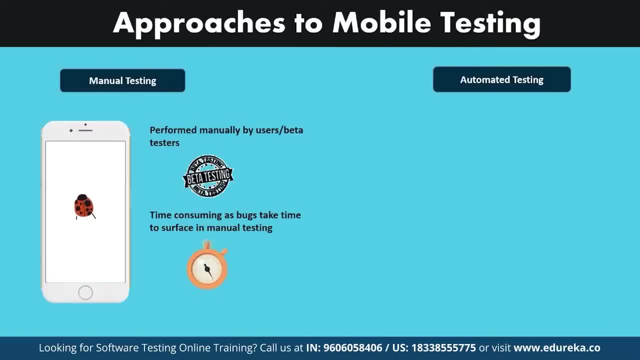 of user friendliness, and this type of testing is generally time-consuming, as bugs tend to take time to get recognized. Therefore, as a rule of thumb, 20% of an application testing should be performed manually to the help of Alpha and Beta releases, while the rest should be automated. 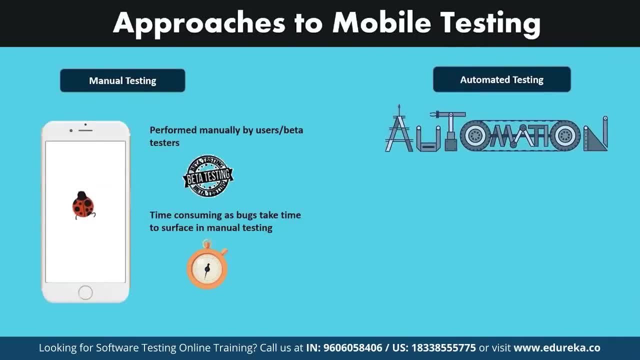 Now Let's move on to automation testing. now, automated testing is the second approach to mobile application testing and in this process an array of test cases are set up, which would generally cover 80% of the testing process. The percentage is not rule, but generally a guideline followed in the software industry. 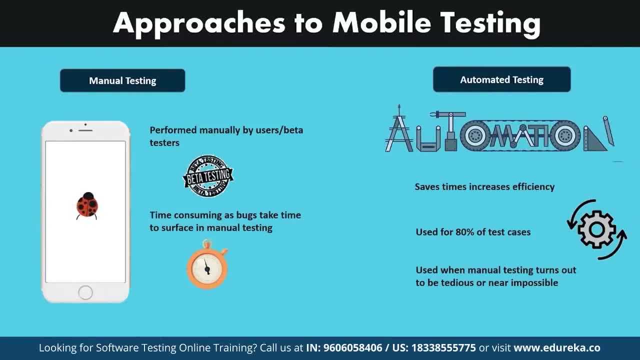 Now let me list down a number of test cases that are generally performed through this particular approach. So, firstly, we could automate most tedious manual testing cases. Then we can automate test cases that can be easily automated. We should always do them. thirdly, 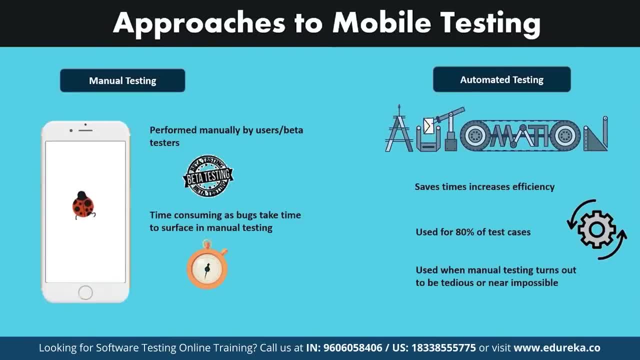 We should always automate test cases for most frequently used functionality. fourth, We should always automate test cases that are impossible to perform manually. and, last but not the least, We should automate test cases with predictable results. Okay, so that was about the two approaches to mobile testing. 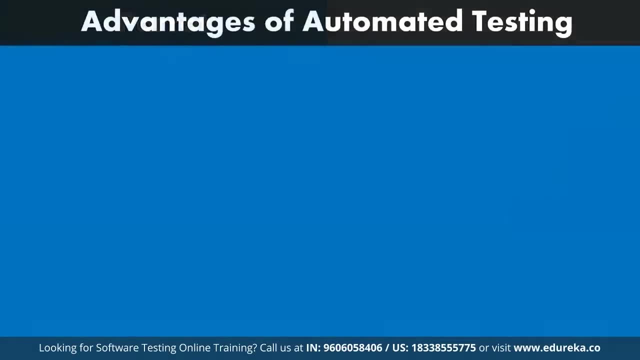 on the basis of how they are performed. Now let me just list down the key advantages of automated testing. So, firstly, automation of mobile testing has proven to be really helpful. So here are a few advantages that come along with automation of mobile application testing. 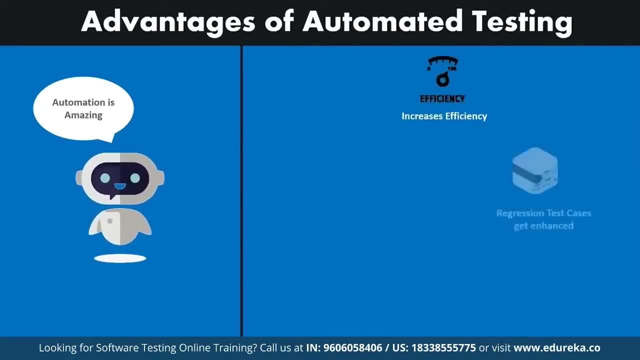 Firstly, it increases testing efficiency. Secondly, it enhances the regression test case execution. third, It saves a bunch of time while also executing more test cases, for the same test cases can be performed again and again on multiple devices. and, last but not the least, test scripts. 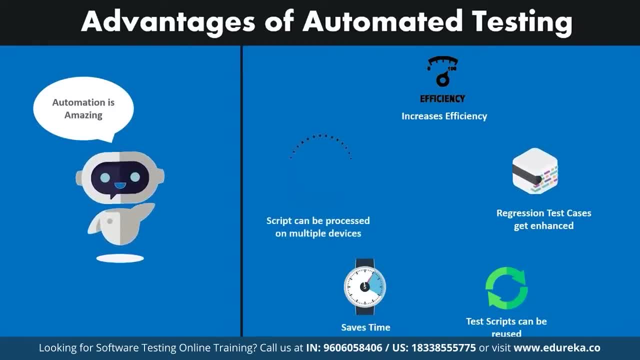 can be run parallelly on multiple devices. So these are a few advantages that come along with automated testing of mobile applications. Okay, So, now that we have discussed the advantages of automating your test cases and basically following an automated approach to mobile application testing, 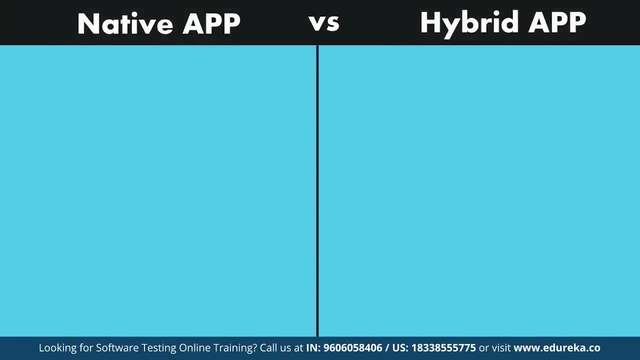 Let us now move ahead and discuss the various kinds of applications for mobile devices that are available in today's world. So these are native applications, hybrid applications and web applications. Now, I have excluded web applications because they are very simple. You can Google them out and what web applications are. 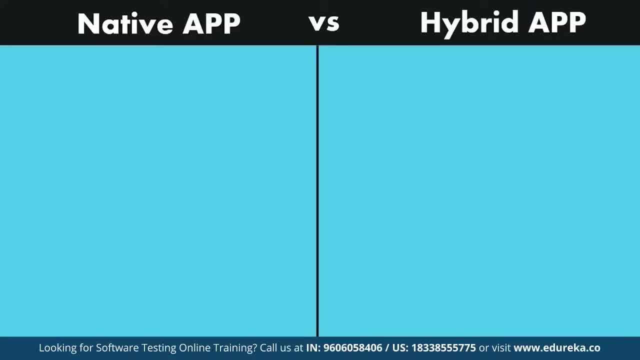 I think native applications and hybrid applications deserve an explanation of their own. So native applications Are considered to be the most reliable, showing extraordinary performance when compared to something like in hybrid or web applications. native applications are developed for a specific mobile platform using particular programming languages. 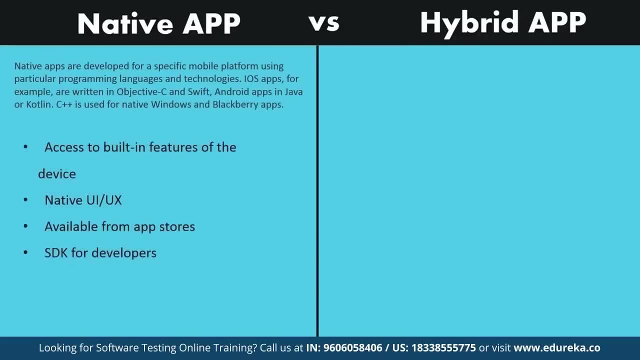 and technologies. iOS apps, for example, are written in Objective C and Swift, and Android apps are written in Java or Kotlin. C++ is used for native Windows and BlackBerry apps, and native app development is preferred for high-performance app. Now, the following are the advantages of having a native application: 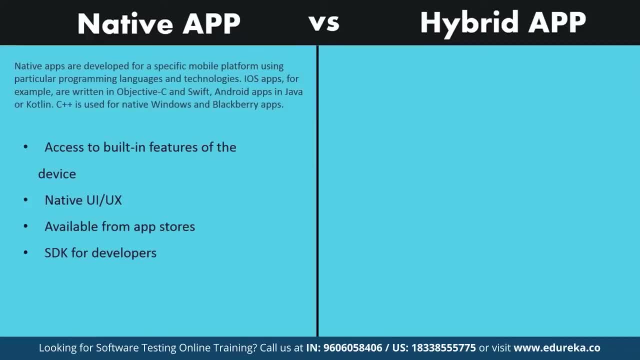 So the first one is access to built-in features of the devices. Then you will also have a native UI and UX, then the application is directly available from app stores. And the last advantage is that you will have a specified software development kit for your development purposes. 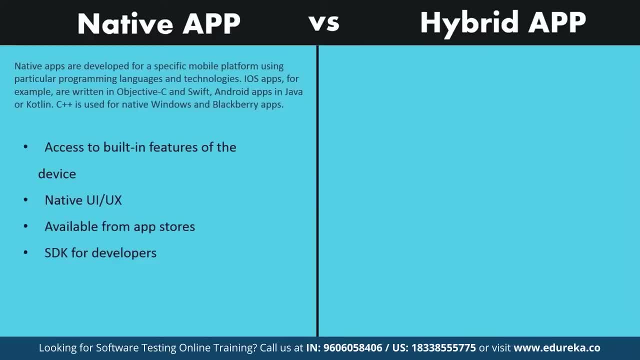 This is not to say that native applications don't come with their disadvantages, So some of them would be like high price and long development time. It's complicated and expensive. maintenance and support, content not seen by search engines and support of multiple versions of the application. 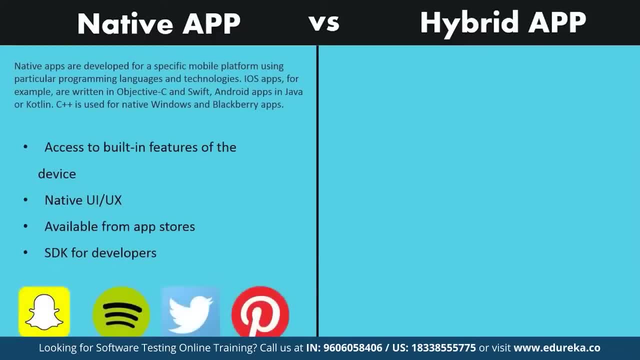 Now. native apps are popular solutions nowadays and they deliver an exceptional user experience and are perfect for solving complicated tasks. really good examples of native apps include Google Maps, for both iOS and Android, Facebook, for both iOS and Android, Snapchat, for both iOS and Android, again Spotify, Twitter and Pinterest. 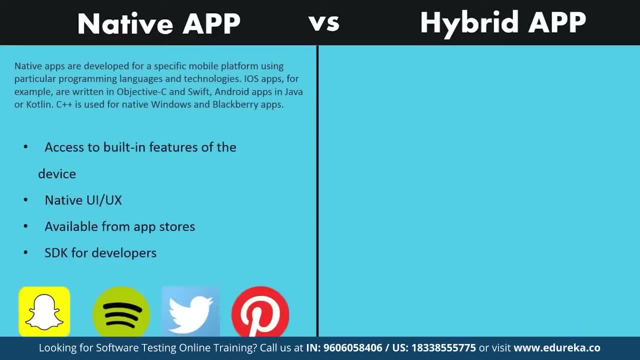 Now you'll definitely appreciate the exceptional performance delivered by the application on both the platforms. now moving on to hybrid apps. a hybrid app is, in a way, a compromise Between a web and a native app development. It combines the advantages of both types of app development. 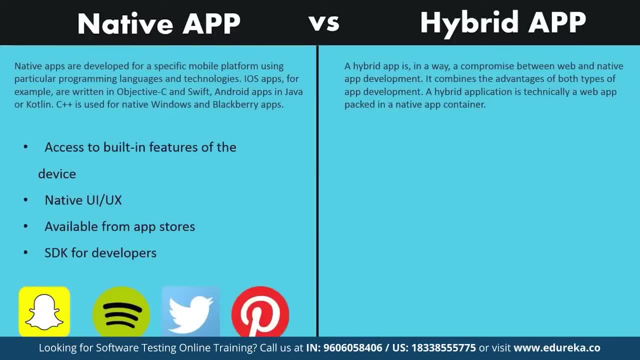 a hybrid application is technically a web app packed in a native app container. like the web app, It is written in HTML, CSS and JavaScript. unlike the web app, It is distributed through the App Store or over the air for iOS devices. Another difference is that the hybrid app is reliant. 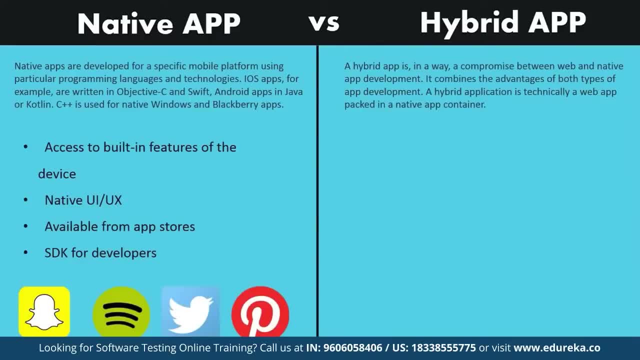 on the web view and not the mobile browser. hybrid apps are good for banks, news media and content delivery Platforms. now, some advantages of hybrid apps are that they are cross-platform. they use the web development technology. They're mostly lower in price when it comes to support maintenance. 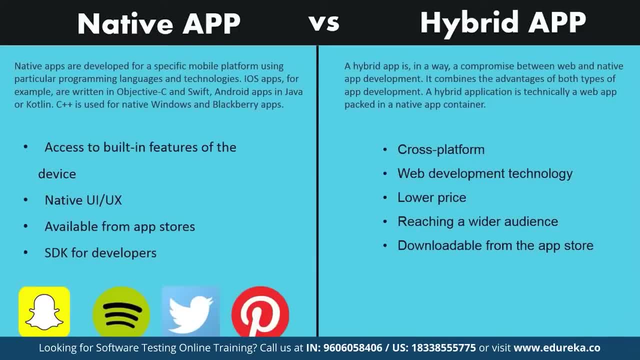 and development. also, it helps in reaching a wider audience, and they're also downloadable from the App Store. Also, another big plus point is no ad blockers. Now, This is also not to say that they don't have the disadvantages, so their disadvantages would be something. 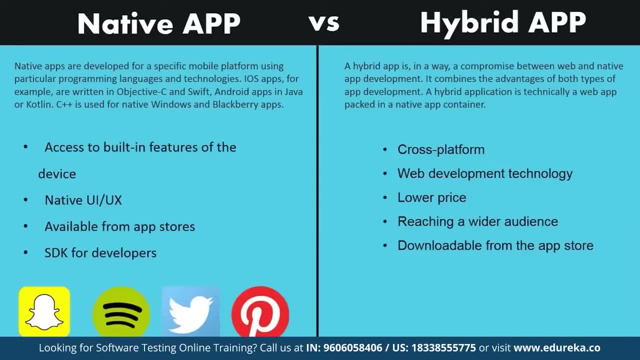 like they have very limited performance scopes and they don't have the whole clean Look of a native app. Now let's talk about a few examples of hybrid applications. So for many it is surprising to learn that some of the world's most popular mobile apps turn out to be hybrid. 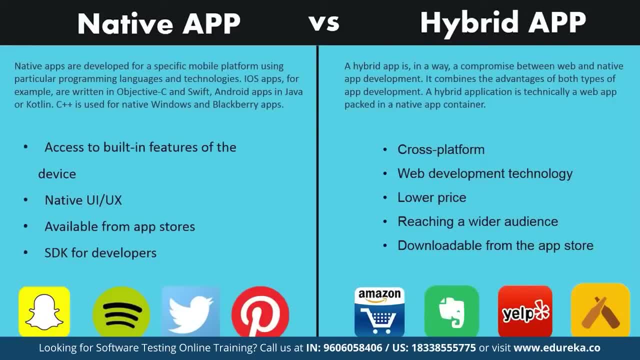 This includes stuff like Amazon, for both iOS and Android, Netflix used to be a hybrid application until a very good time And now it's a native application- and also stuff like Yelp and untapped. untapped is a beer service which will help you find the best beers in town. 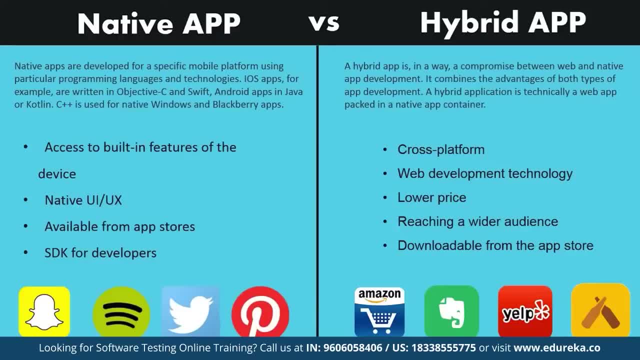 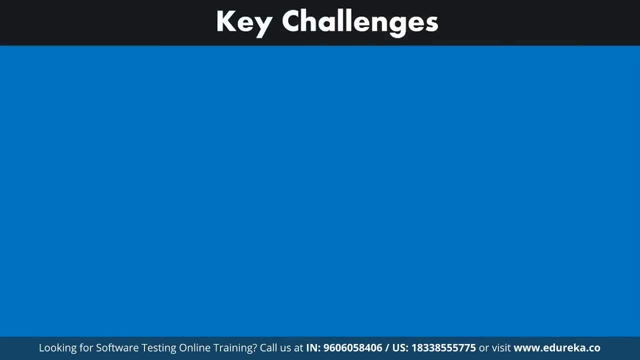 So that's a really nice app. So all these really cool apps like Amazon, untapped, Yelp and Evernote are all very good examples of hybrid apps. Now let us look at the key challenges that are faced by application testers in the mobile application testing world. 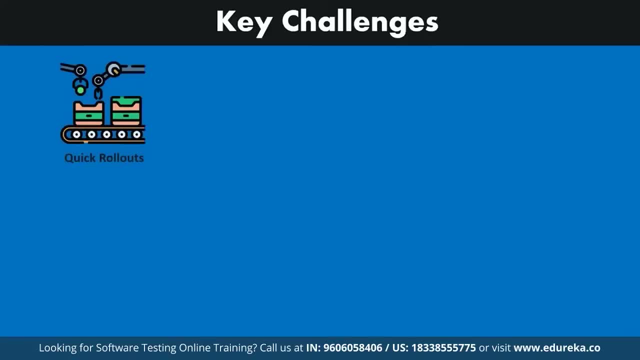 Now, mobile application testing differs from traditional process of testing desktop or web applications. This means it comes with its own host of challenges. The major challenge is due to diversity of mobile devices. today There are a bunch of screen sizes, operating systems, hardware options, software versions. 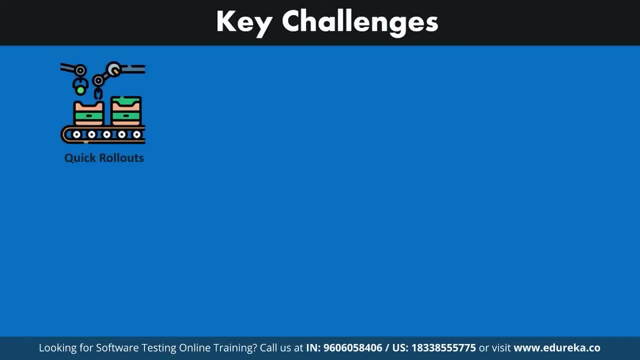 etc. as of 2017, there are more than 60,000 Android devices on the market, And some of them have even started adopting the whole notch fashion which is brought about by iPhone 10.. Now let me list down the major issues faced. 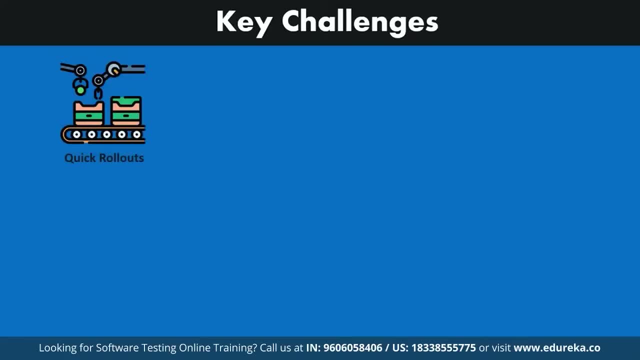 in mobile application testing. So the first key challenge is quick rollouts. now, mobile applications industry is one that acts upon bugs quickly and they're always thinking about new features. the faster these get rolled out, the longer an application remains trending on its respective Marketplace. The second key challenge is the multi-platform. 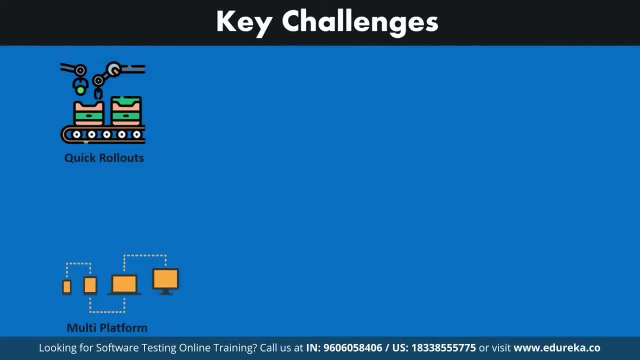 activity. apart from Android and iOS, There are a bunch of operating systems executed across a multitude of platforms. this only increases the time taken to test a certain application. thirdly is that mobile applications should work on a bunch of connectivity modes. mobile phones are subjected to different modes of connectivity. 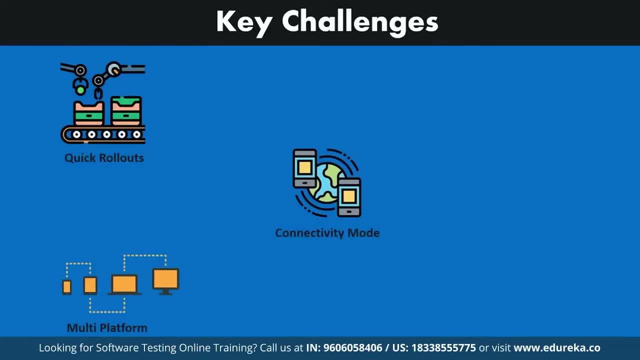 For example, roaming, 4g, 3g, Edge, Etc. Now applications must be tested in all these various connectivity modes and to see if they're working efficiently. the fourth point is end-to-end testing. the mobile phone industry demands that applications integrate seamlessly and be able to access data from the back end to be produced. 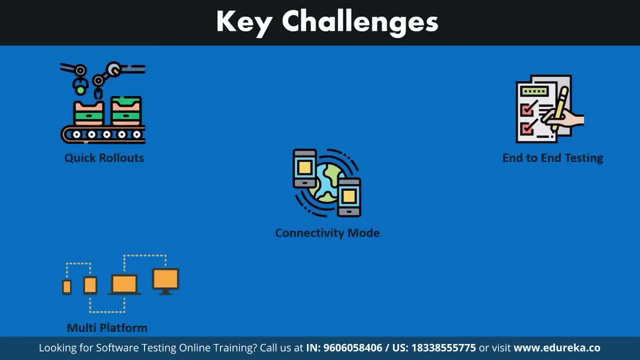 on the front end without any problems. due to the diverse nature of mobile phones, This becomes a Herculean task. last but not the least is the availability of tools. Now, There are a number of tools today that automate mobile applications. choosing the right one. 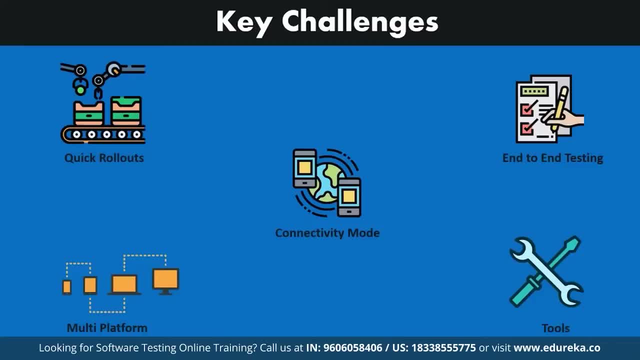 for your application is essential to the success and the efficient testing of the application. Okay, guys, so this brings us to the theoretical end of this introductory session on mobile application testing. Now, as you guys know, none of the edutech, our videos, are ever without a demonstration. 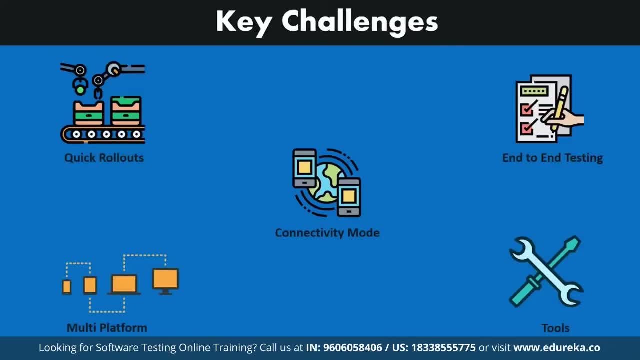 So for today's videos demonstration, I will be giving you guys a quick sneak peek into what we will be doing ahead in future videos. So in the future videos, you will be introduced to a tool called Appium, which is an open source tool that is used for mobile application testing. 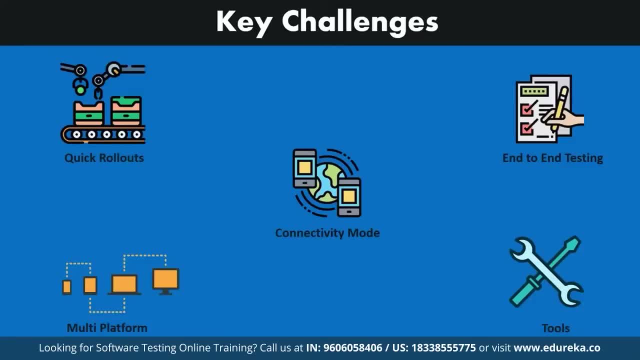 just to give you guys a sneak peek into what it looks like. So what we have done is, firstly, I have installed Android studio, I have installed Appium and I have installed a few drivers To get them both integrated and running seamlessly. So let me just show you this is what I have done. 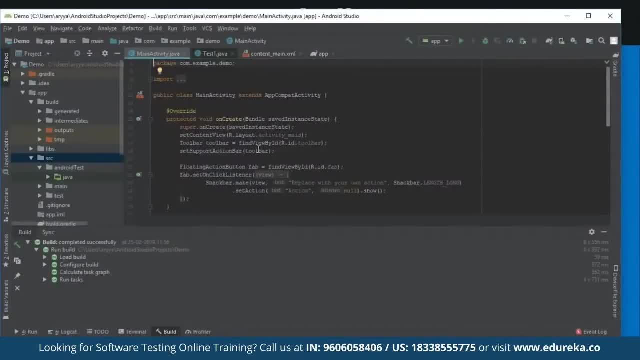 I have made a small application that absolutely does nothing, and this is very easy to build, and you can check out our Android development videos for the same, and what we have also done is I have also downloaded the calculator app, which is provided by Google, and you can download this from apkprcom. 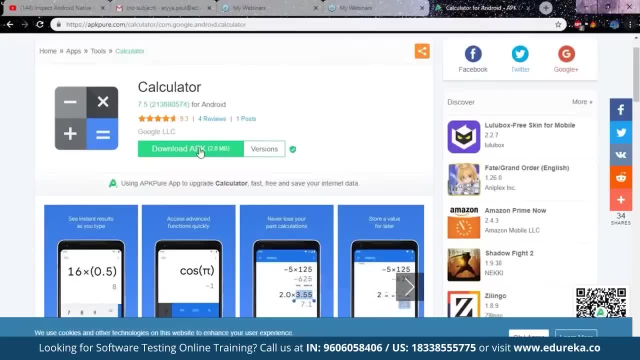 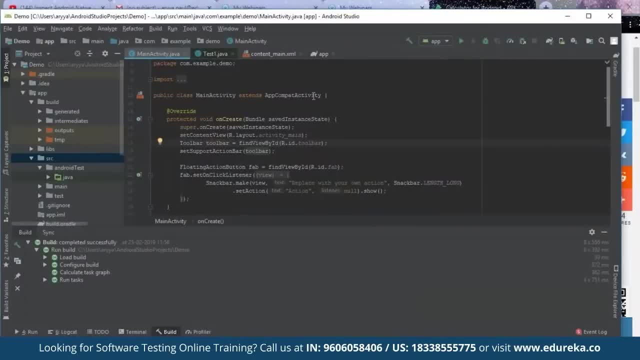 and you can just search for the calculator out there and download it. It's a 2 MB APK. Now what you want to do first is: we want to install this APK. So the question arises: where do we install it? Well, you can install it on your local device. 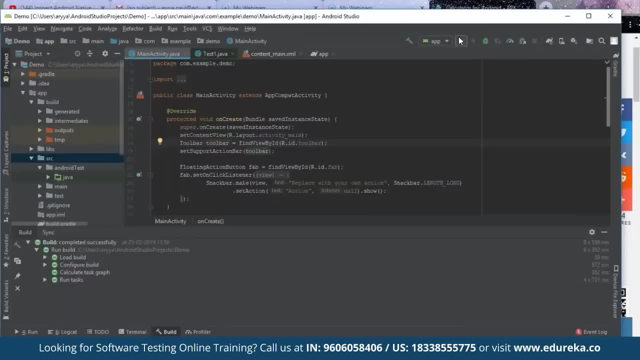 but if you don't really have an Android phone, then what you can do is start up an emulator. Now I have a Nexus 6 emulator that I have set up through Android studio, So Android studio is going to be the primary medium of writing our apps and writing our test cases. 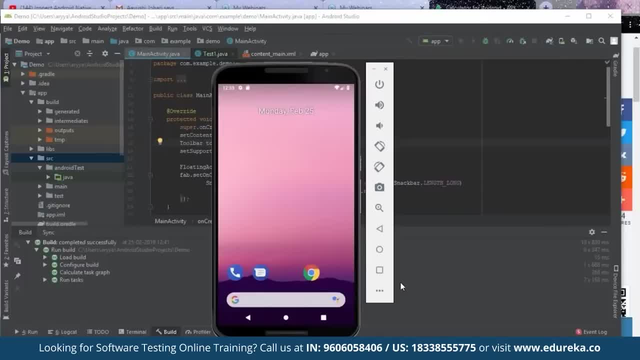 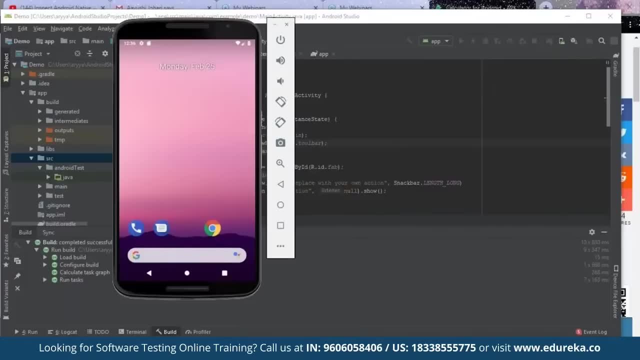 So I highly recommend that you go ahead and install that on your device or your system. So what do you see out? here is an emulated device that looks like a Nexus 6. next, What we want to do is also install ADB. So to install ADB. 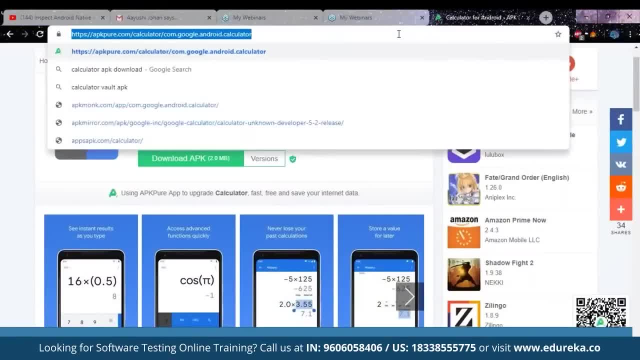 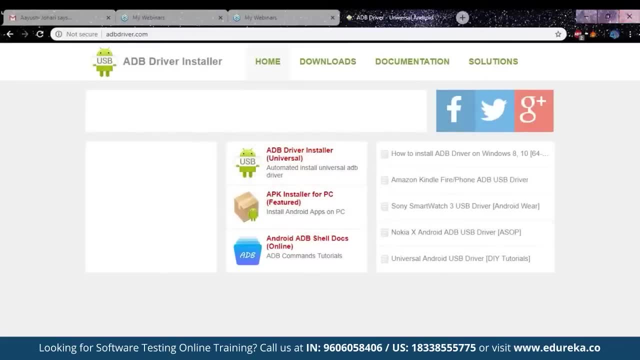 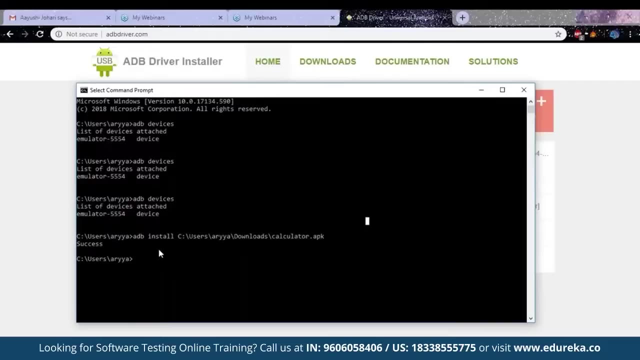 you have to go on Google and just type in ADB. So if you type ADB out here, you can follow these download links and install them Now. ADB is used for checking our Android devices and installing apps. Now, as you guys can see, I have already installed the APK. 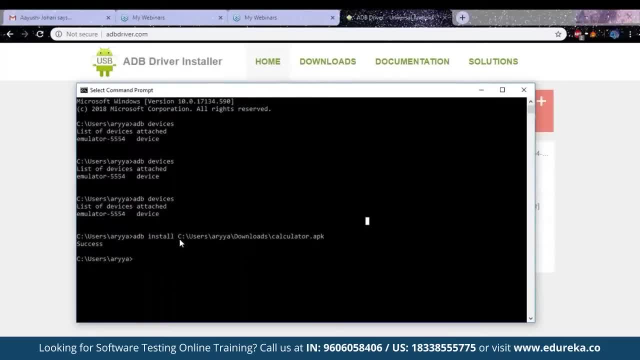 on my device. You can simply do it by going ADB install and then putting the part of the APK on where it is stored on your system or device, and if it is successful, it'll show success out here. Now you can also check. 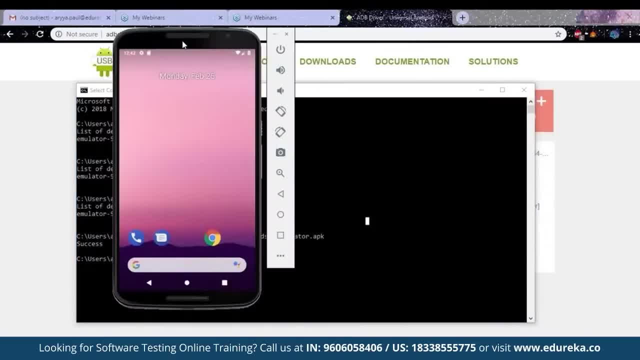 if the device has successfully installed your application by going into the app drawer and just checking it out there Now, I will always recommend that you use a local device, because the emulator that comes along with Android studio is not up to the mark. It kind of takes a lot of time to install stuff. 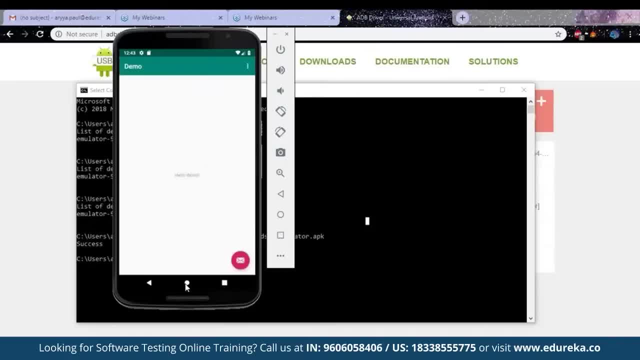 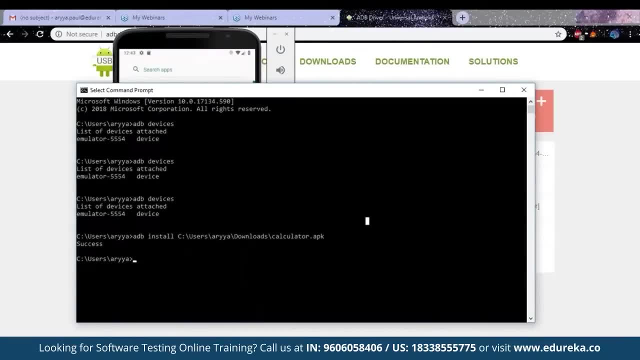 and it generally takes up a lot of time that could be used in testing. Okay, So, as you guys can see, our calculator has been installed out here, So what we want to do is now: you want to go ahead and start up Appium. 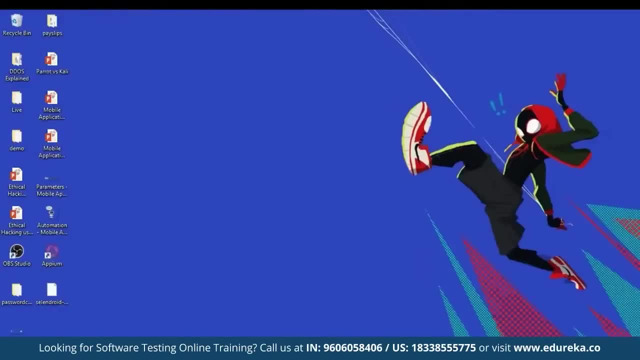 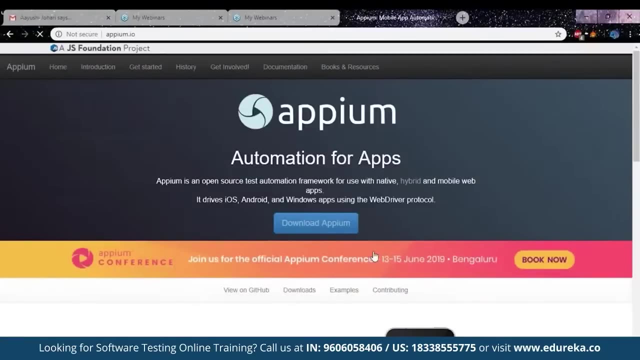 Now I have installed Appium from the Appium official site. that can be easily found out by going Appium and going to Appiumio. So out here you can see that you see this download button, which is the Appiumio desktop version. 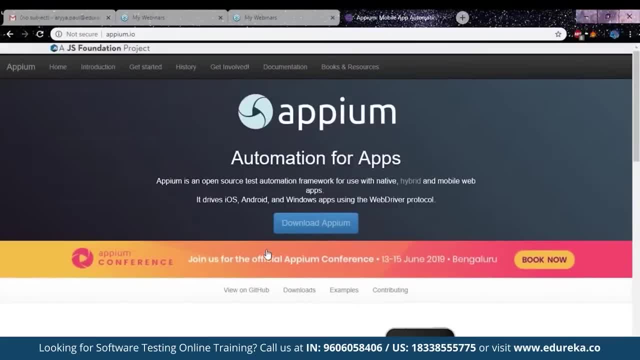 Now Appium also has a command line interface version, but I highly recommend that you use the desktop version, because this is what we are going to be using in future videos to actually test our applications. Now let's just wait for Appium to start up. 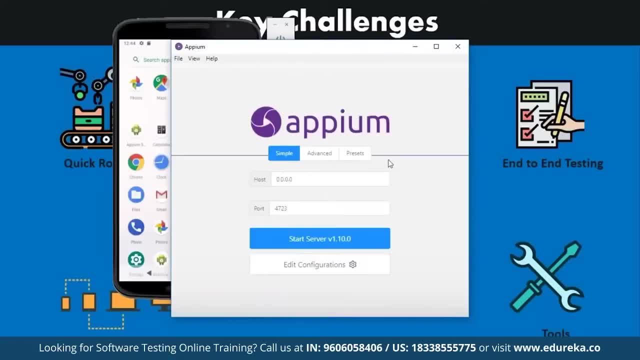 Okay, so Appium has started up out here And, as you guys can see, Appium is just a server. It is a server for testing purposes and it is not much more than that. You will need a bunch of things other than Appium. 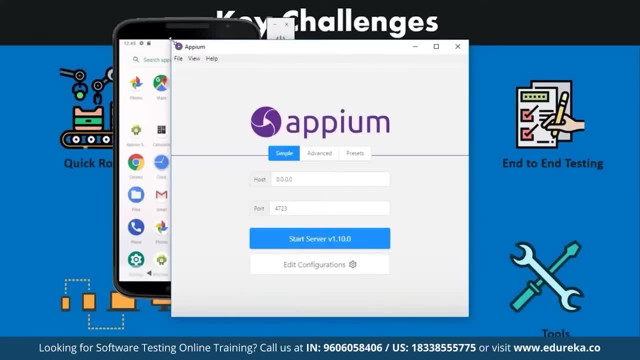 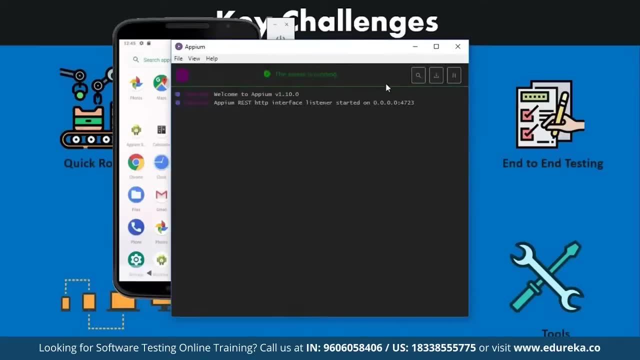 to actually test your applications now, just to give you guys a sneak peek into how applications are tested using Appium. This is going to be the general process every time. So what do you want to do is start your server now. after you have started the server, you want to go ahead. 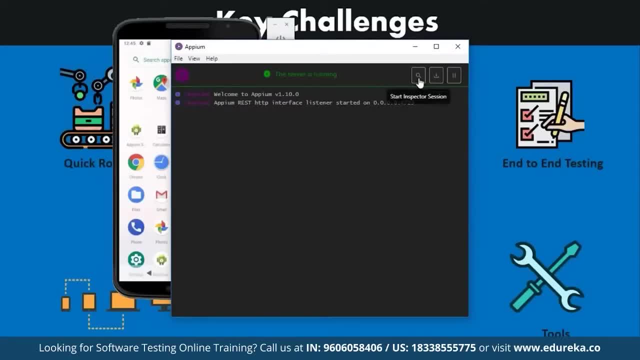 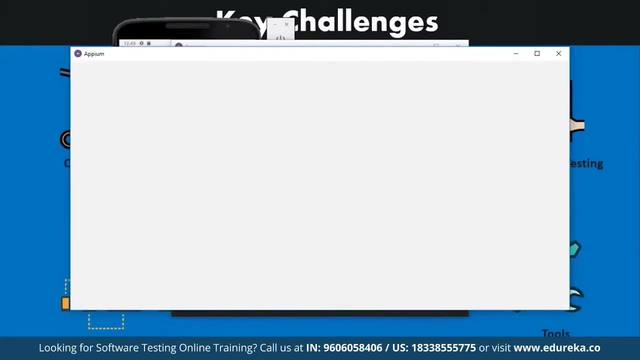 and press this search icon which says start inspector session. Now the inspector session is where you generate your test script that you can run on various devices. now to generate your test script, We will be first setting up our desired capabilities. I will explain what desired capabilities are in our next video. 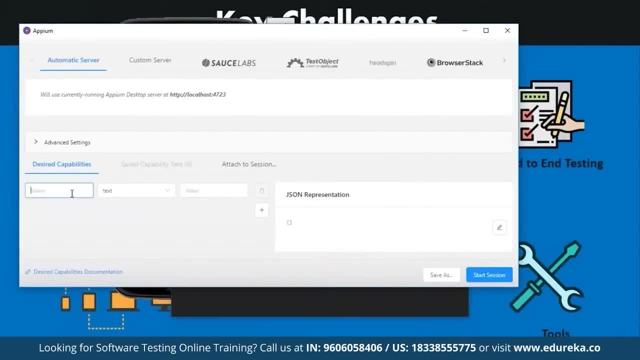 which is going to be Appium tutorial, where I will also show you how to install Appium along with its various dependencies. So, first of all, the first desired capability that we want to set up is the app. Now, to set up the app only have to do in the value section. 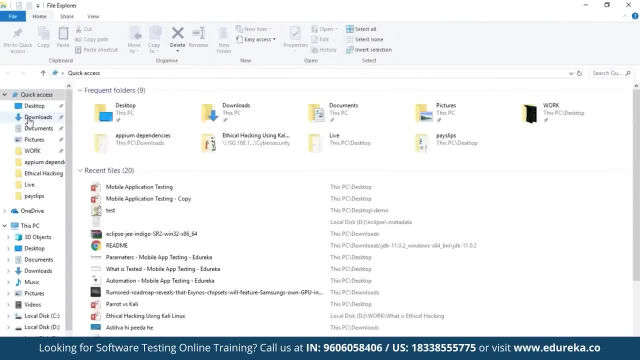 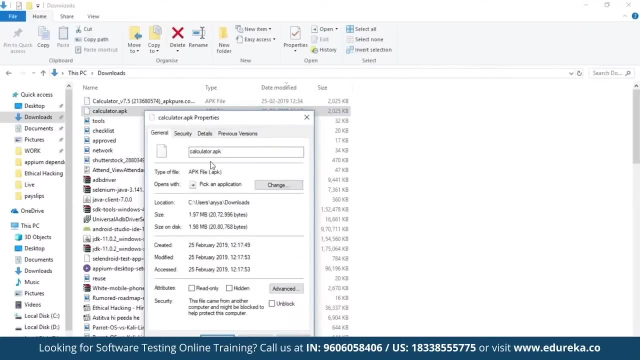 is go ahead and paste in the address of the app that is stored on your device. So, as you guys can see, I have calculated APK going on out here. All you want to do is go into properties and copy down the location control. see that put out here. 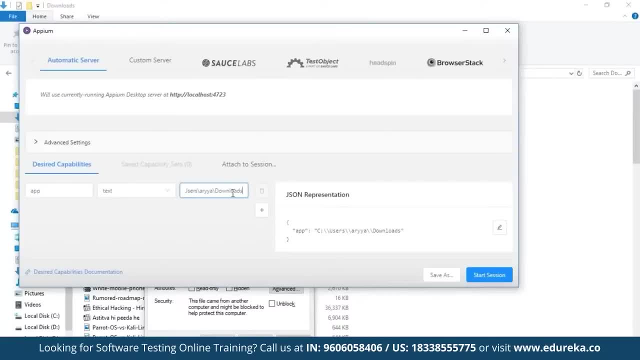 Paste it and you also want to put in the name. So go ahead, at the end of this put a slash and put in calculator dot APK. So that serves as the app path. So, as you guys can see, it generates a JSON representation out here. 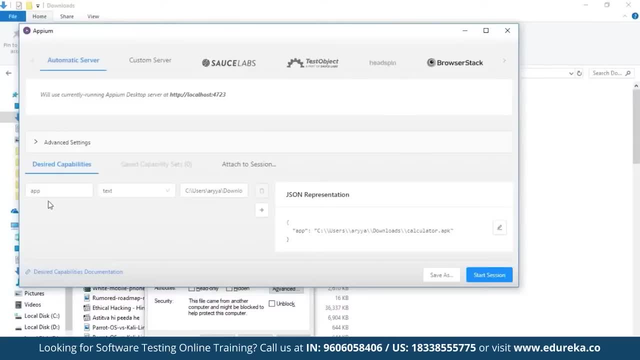 So it's basically mapping key value pairs and sending them to the server to react upon. now We need a couple more desired capabilities. One of them is device name. So for device name you can go into your command prompt again and you can go ADB devices. 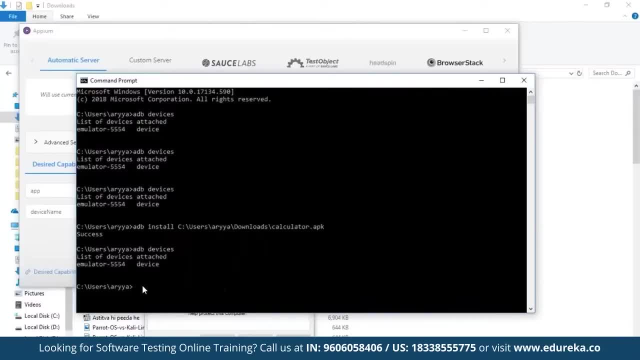 and this will show you the list of devices. when it comes to Android, that is connected to your computer at this moment. So for us, we have our emulator that is running. So this is emulator 5554, and all you want to do is copy this and then paste it out here. 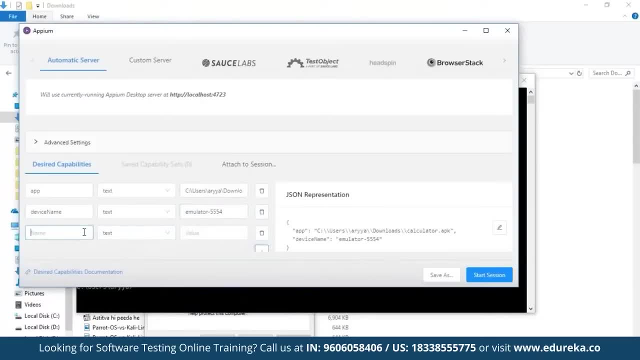 So that will set up our device name, and we also need to specify the platform name. So once we've set up the platform name, it's going to be Android. All you want to do is go ahead and hit start session. Now, when you hit start session- another interesting thing- 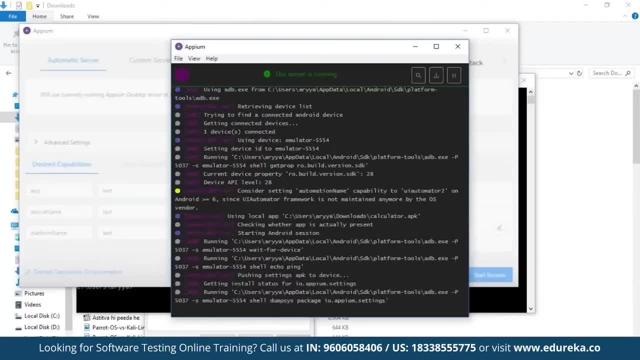 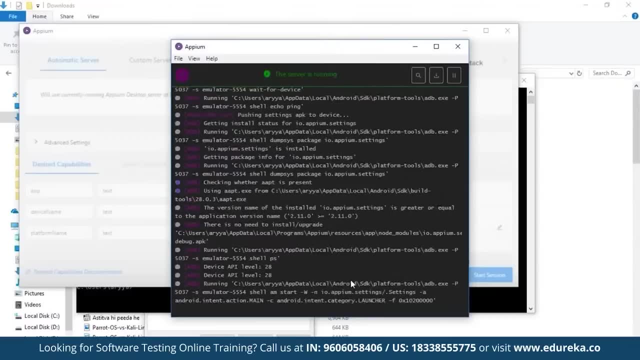 to note is in this page So, as you guys can see, it will give you a complete log of what is actually happening in the background. So you need not worry. if you go through any error, it'll show up out here. Suppose it can't find your device. 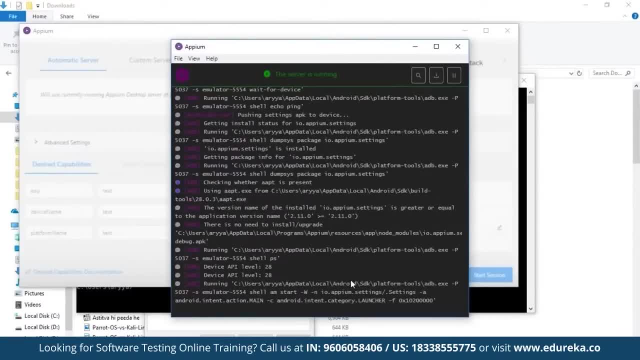 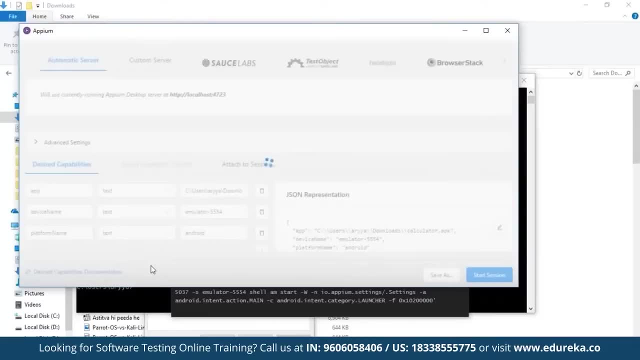 and it'll show that device not connected or Appium couldn't find the device. But if everything goes correctly, you should see a screen that pops up here. that will let you begin your testing process, and let's just wait for the screen to come up. 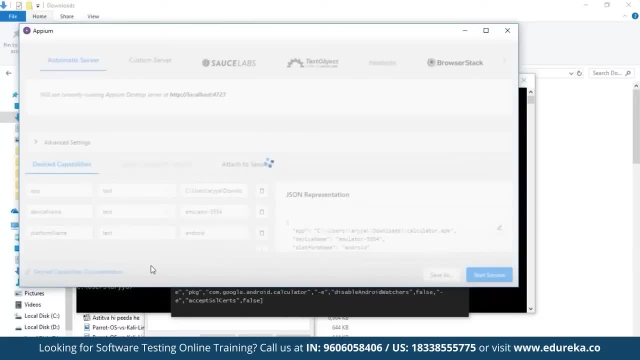 without me explaining much Now. I always recommend that you use a local device because of this reason, because emulators take a long, long time, especially the Android studio emulator, and this being an i3 device with only about 8 gigs of RAM, This is going to be a slow process for most of us. 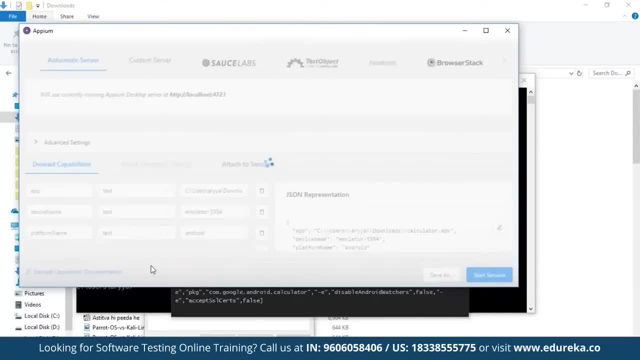 I normally recommend around 16 gigs of RAM and i5 device with least 16 gigs of RAM for any sort of heavy testing procedure that you might want to follow If you go ahead and go on our calculator out here. Okay, so our server has started up. 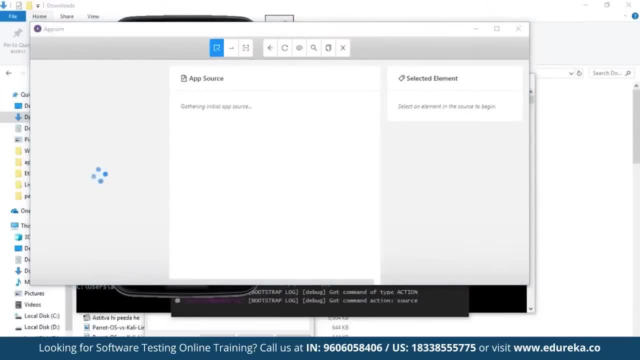 after a long period of waiting, and what you see out here is the interface that will be used for testing of our application. So let the interface just load up properly. So, if you guys can see, our calculator has actually launched on our emulator without us even invoking it. 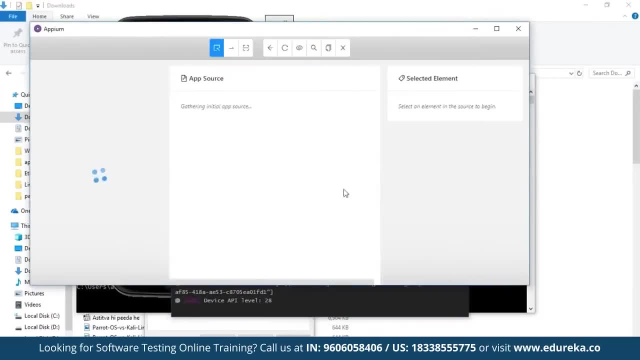 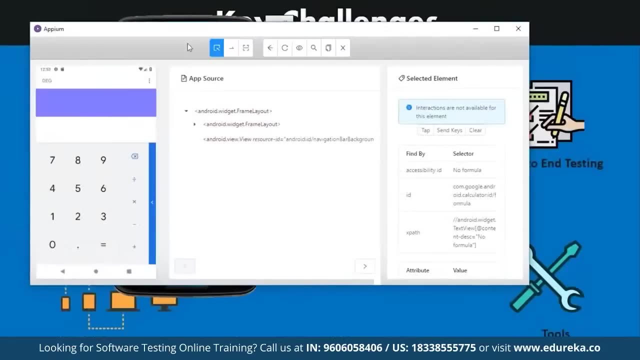 and that is because Appium has invoked it. Now let us just wait for the slow process to actually end and the screen out here to appear. So, as you guys can see, our interface is loaded up. That means our calculator has also been invoked on our emulator. 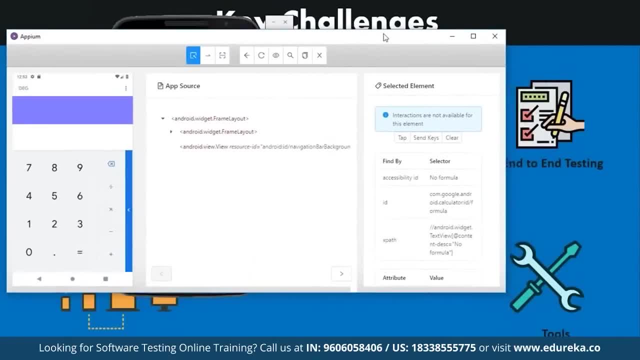 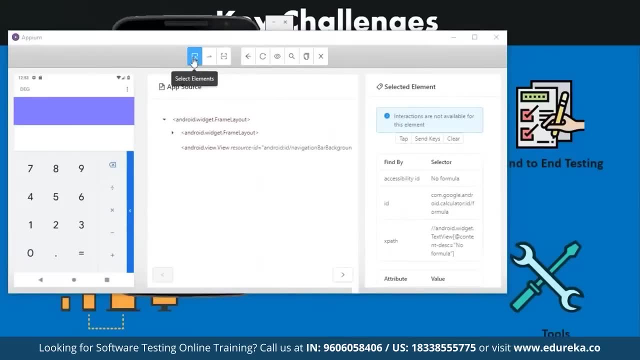 Now, what this is is the element selector, and I will tell you more about this in our Appium tutorial video. Now, what you can do out here is you see these bunch of buttons. So first is select element. So this allows us to select an element like this: 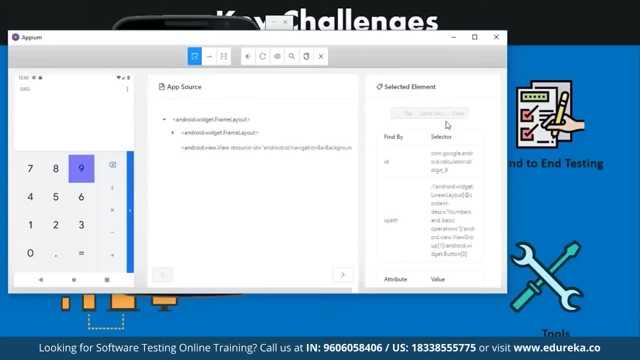 and out here you see a bunch of options like tap, send keys and clear. so tapping is basically you can tap that button and test it for the interactions that it has. You can also send values. that is basically send keys. and the best part about Appium is that you can start a recording. 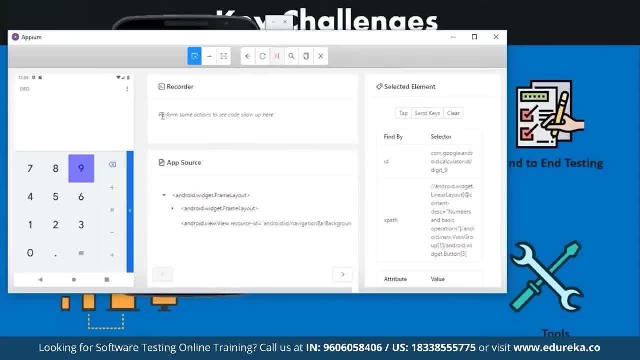 Now, if you start recording out here, what it will do out here is generate a test script. So suppose I were to go on nine. I selected nine as an element, So the stop part takes a little bit time. So, Appium, lets us record our test scripts that we can paste. 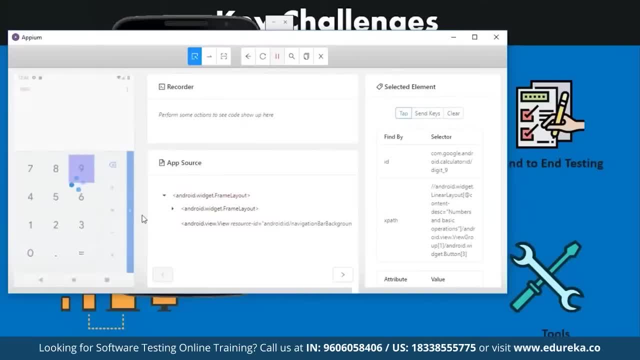 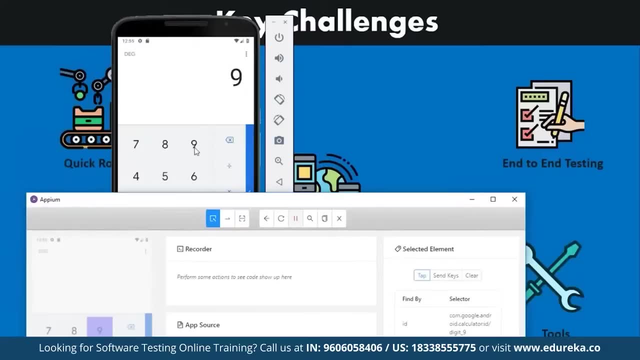 so you can tap it and you'll see that nine pops up out here. It's a little slow process, but you'll see it happen and you can also see it happen out here On the emulator. Now you see that nine got tapped and nine actually got output on the display. 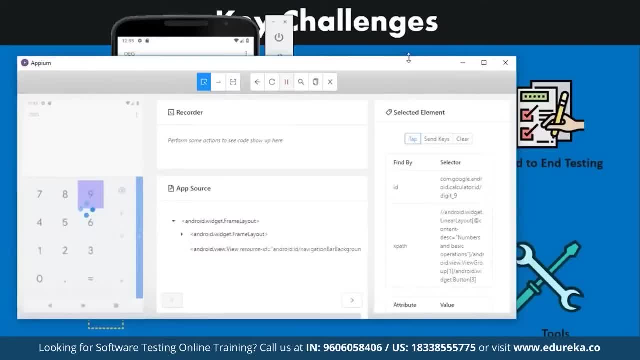 So that's how you actually test your applications. We will get to the testing phase of this application in much more detail in upcoming videos, But for now, this is how you can set up an application on an emulator and also start that application on Appium for testing purposes. 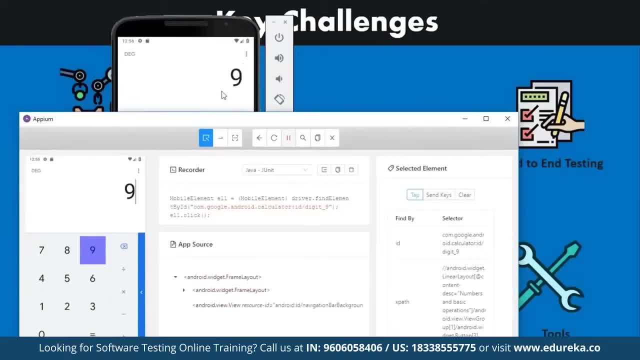 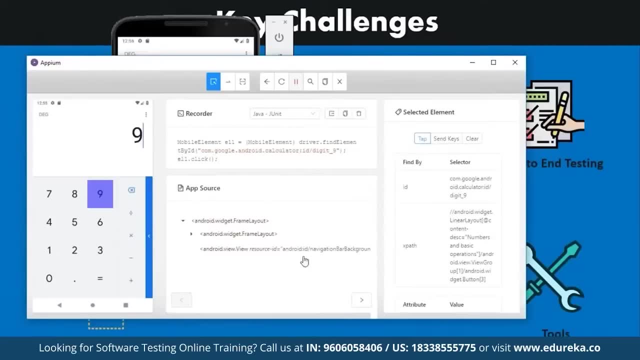 Okay, So now that nine has been pressed- and it both appeared on the screen of our emulator and the screen Of our testing interface- You can see a little bit of code that comes up now. This code is basically your test script that you are generating. 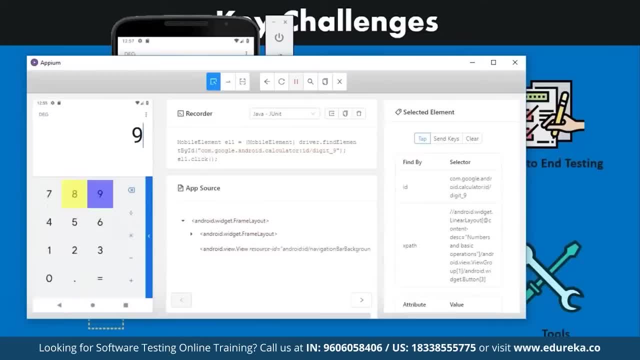 and basically, you can go ahead and select a bunch of elements and you can send them keys. You can tap on them and it will constantly generate a test script in a bunch of different languages. You can choose the language of Java, Python, Ruby, and there's also the robot framework. 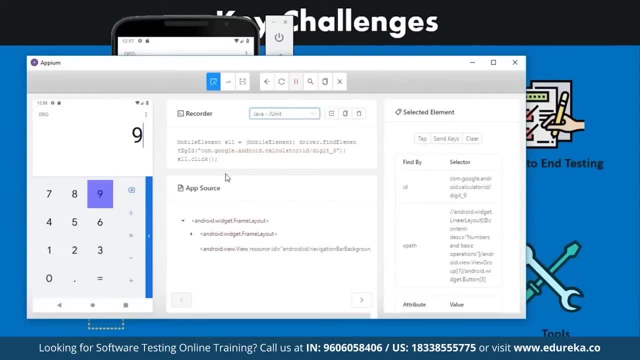 So that was it for today. I showed you guys how to set up an application on an emulator Out here with the help of a DB. in the upcoming videos, which is Appium tutorial, I will showing you how to install Appium from scratch. 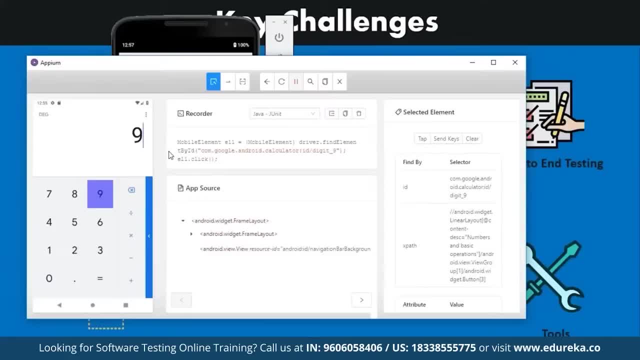 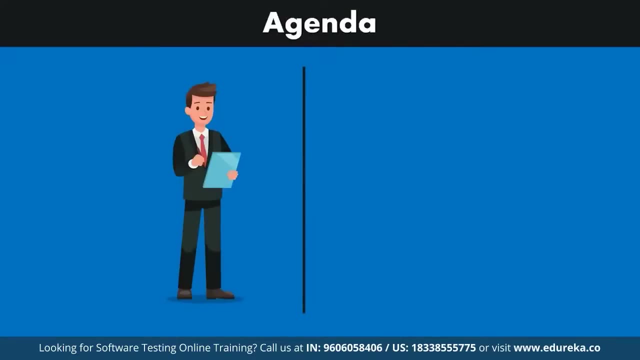 And then we will also dig deep into the testing of any sort of application. We will be mostly testing native applications, as native applications are much more robust in performance. So firstly we will be looking into tool called Appium. So the first topic that we're going to be tackling is called: 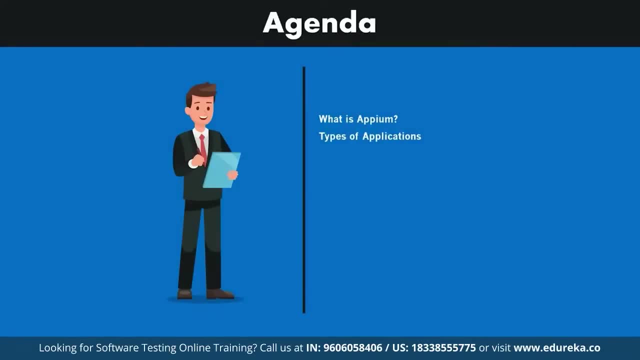 What is Appium? Then we are going to go into the types of applications that are there for mobile industry. Then we will also discuss why you should choose Appium by comparing Appium to its market competitors. Then we will go ahead and discuss the Appium architecture. 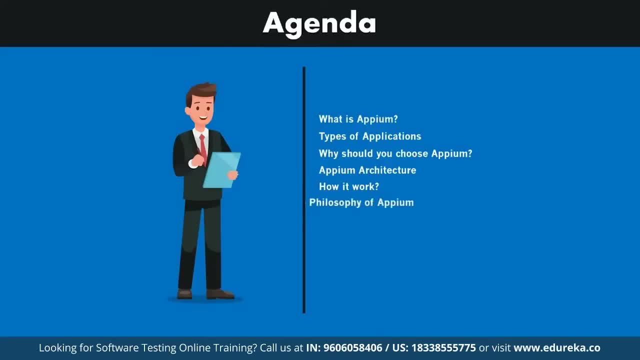 and how, of course, how it works. after that, We will be discussing the philosophy on which Appium was built on, and we will also be discussing the pros and cons of actually using Appium. in the end, I will be talking about the dependencies that Appium actually depends on. 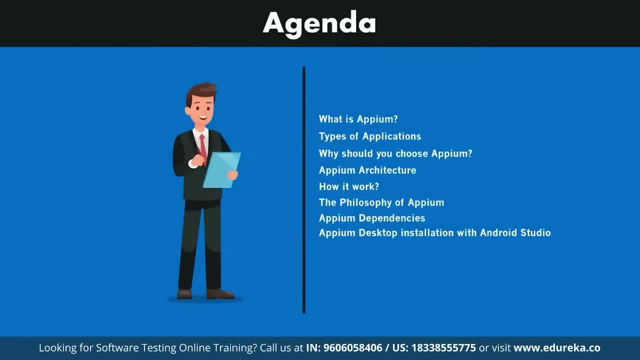 and we will also be doing a installation of Appium desktop version, that is, Appium 1.10, from scratch using Android studio, and we will also be integrating it in the end. I'll also give you guys a brief introduction to the desired capabilities, part. 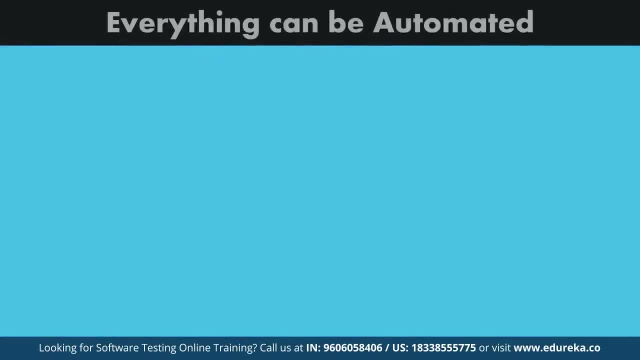 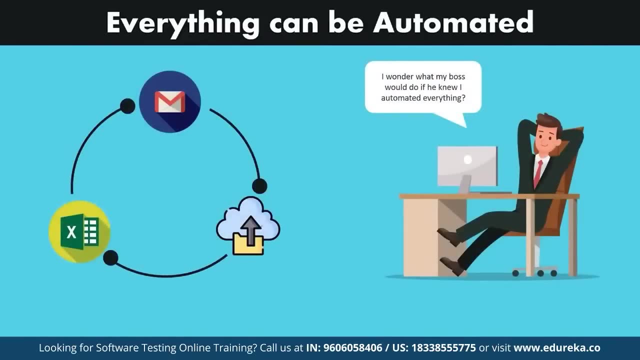 which is there in the Appium documentation. Now, the first topic for today is: what is Appium? now, if you guys have seen, today there is a general trend of automating almost everything that has a pattern in it, whether it be emails or whether it be Google Forms. 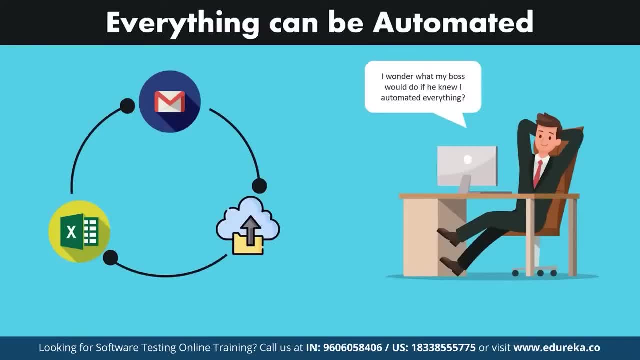 or whether it be uploading files, tasks like web scraping or anything that can be put into a pattern, like there are particular steps that you are following. like step one for writing an email is: go ahead and hit the compose button on Gmail, And then there are a few steps that you have to follow. 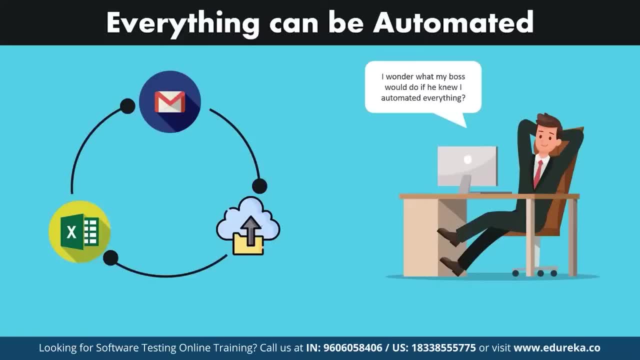 and everybody knows how to send an email. So the point I'm trying to drive across here that if you can tell an automating tool that these are the steps to follow for every single email that there is there, then a tool can very well automate what you want to do now. the same Crux. 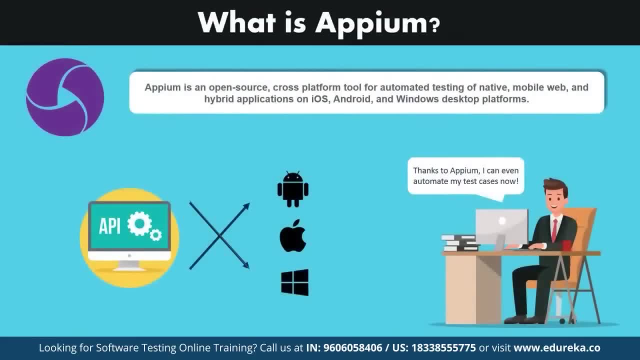 or you can say: the same fundamental is being used in the mobile software industry. now, in the mobile testing industry, especially in the testing area, automation has become quite the norm. now, today We are going to be talking about Appium, So Appium is basically. 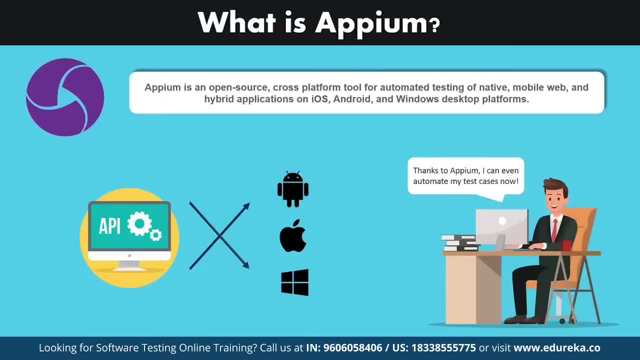 a tool that is being used for automated testing of native application, web-based application and even hybrid applications. Now let me give you guys much more refined introduction to what exactly Appium is. Appium is a freely distributed, open-source mobile application UI testing framework. 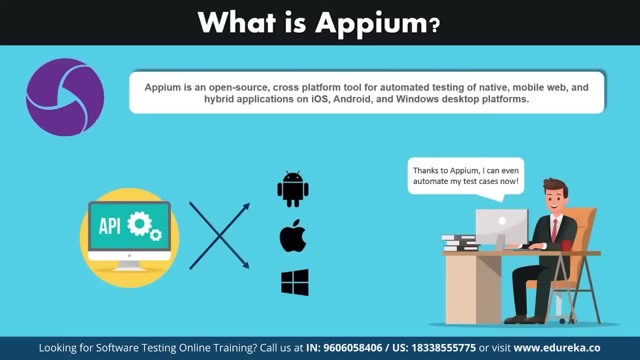 Now, Appium allows native hybrid and web application testing and supports automation test on physical devices, as well as an emulator or simulator or both. above that, Appium also offers cross-platform application testing. that is, a single API that you guys can see out here on this part of the screen. 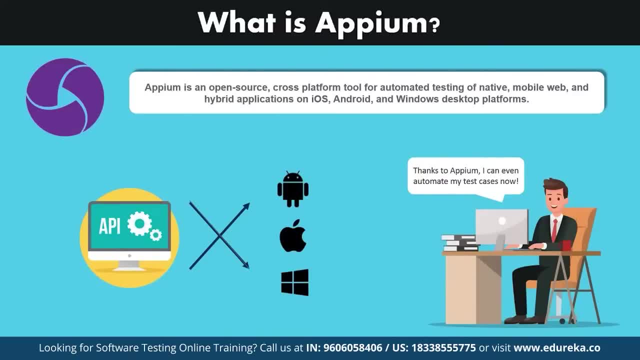 a single API is actually going to work for both Android and iOS now. recently, Appium only was restricted to the mobile application testing domain, but with recent updates, especially Appium desktop since Appium 1.8, Appium has also moved forward into the domain of test. 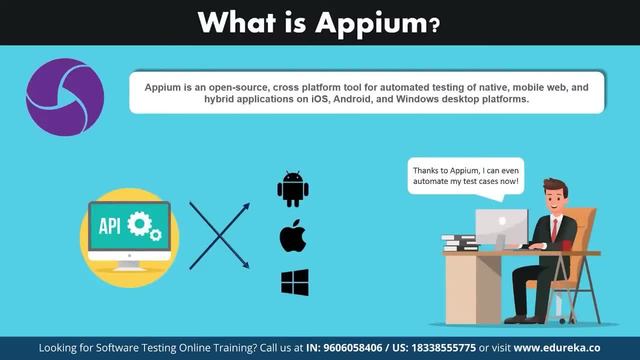 of application testing. So currently Appium visit single API. It allows us to test applications for Android, for iOS and for Windows OS, and when I say Windows OS, I don't mean the OS that would be running on phones, I mean Windows 10 and Windows 7 and Windows 8 that kind. 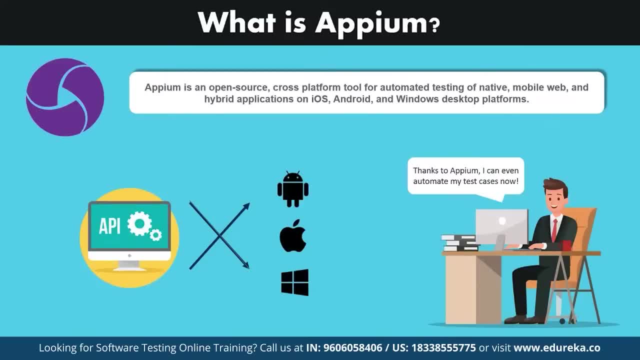 of stuff and applications that are built for them. So, basically, it's one tool for testing various applications, whether it be native application, whether it be hybrid application or whether it be web-based application. So, as you guys can see out, here our character, Bob, is really 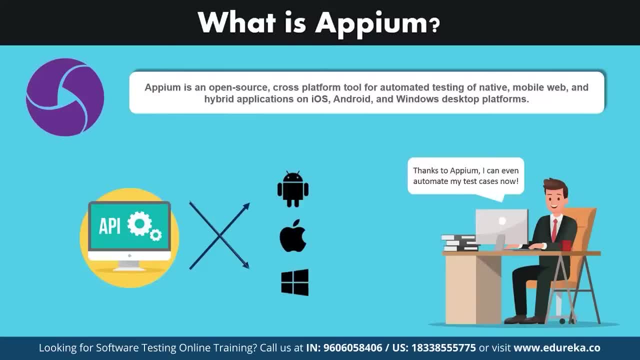 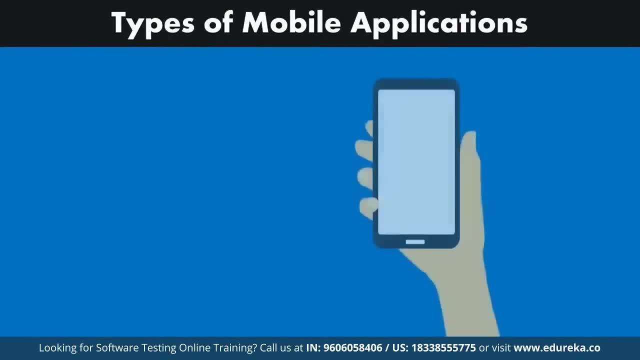 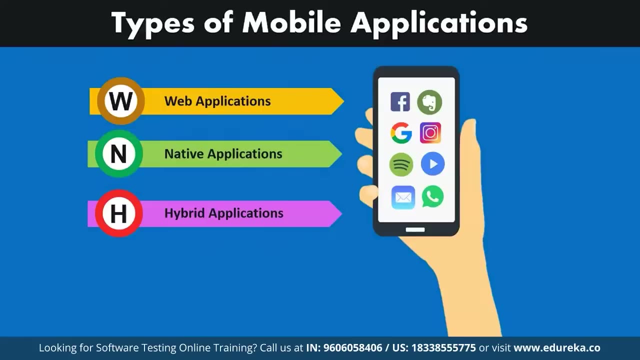 happy that he can now automate all his test cases and save a bunch of time doing much more productive stuff. Okay, now moving on. I just told you guys that Appium is used for native apps, hybrid apps and web apps. So what exactly are these? 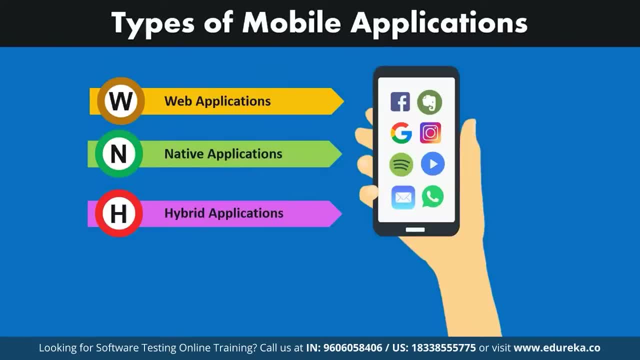 Well, these are just types of mobile applications. They are classified into three types, as you guys can see, and as you guys have already heard that they are web applications, native applications and hybrid applications. Now let's take a look at them one by one and also try. 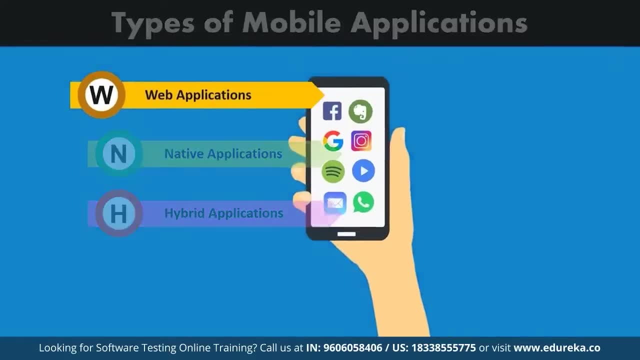 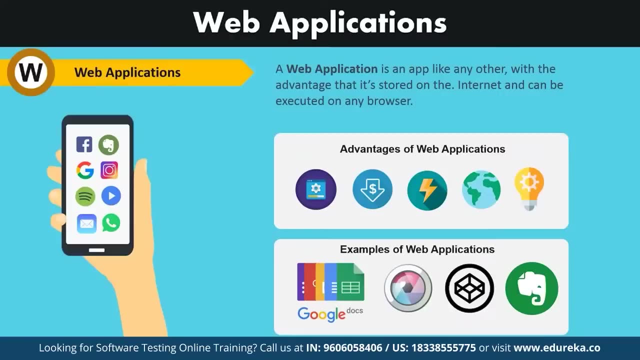 and understand the differences between these types of applications. Okay, so the first kind of applications that we're going to discuss are called web applications. Now, web application is an application like any other. It's just that it's stored on the internet and to actually use app you'll be going. 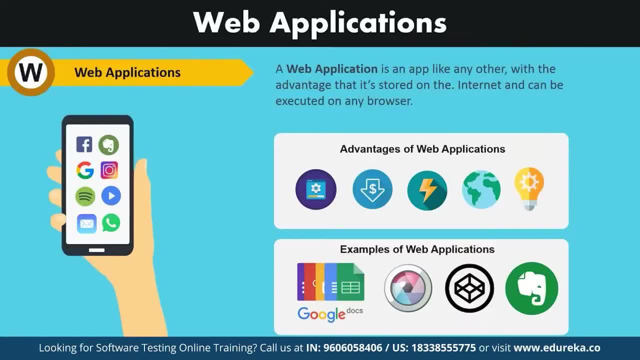 through a browser sort of interface. So how are web apps different from a website? Well, a website typically provides users with a lot more information than is practical to display in a mobile site, Whereas a web app condenses this information. to improve functionality, web apps: 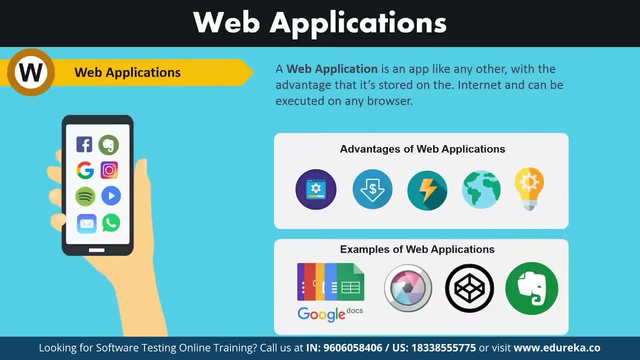 However, do not need to be downloaded from the app stores. like mobile apps, web apps load in browsers like Chrome, Safari or Firefox. a web app also doesn't take up storage on the user's device. Now people classify web apps as new technologies which blurred the lines between web native and hybrid apps. 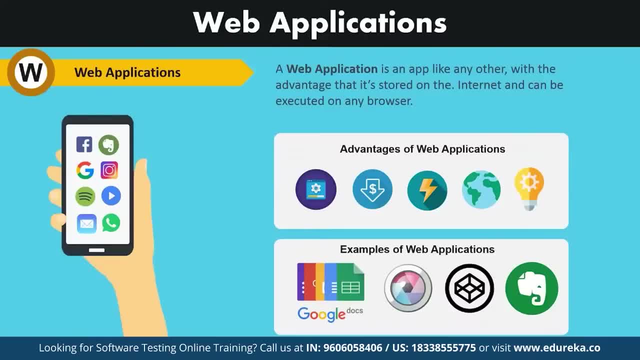 It's kind of difficult to distinguish which apps are web apps and which are hybrid apps and which are website built with a responsive design. Sometimes, what seems like a native app downloaded from the App Store is actually an app in a web view which is written in the native language containing the URL. 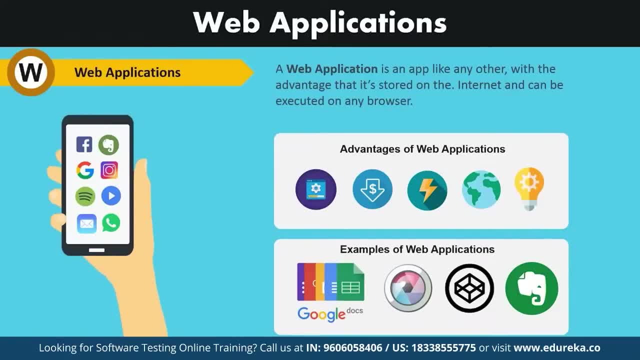 to the web app. the majority of the code is handled outside of the native language. to some, that satisfies the requirement of a native application, and to others It's just another format for a web application. web apps are essentially websites that look like native application but instead of being installed on the home screen, 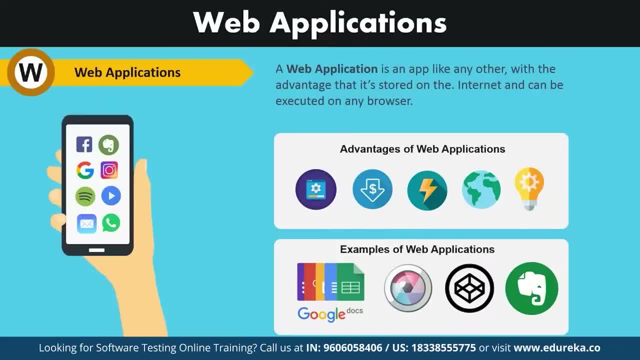 that users create a bookmark to. it's basically on your bookmarks in your web browser. Now the question comes: how do you build a web app? So typically, web apps are built using JavaScript, CSS and HTML and run inside a browser like Safari or Chrome, and there is no software development kit. 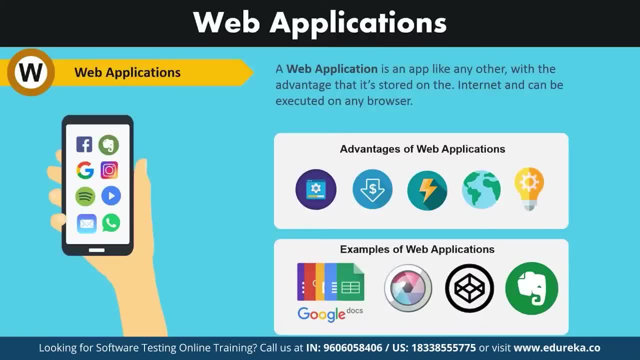 for developers to use. However, there are templates that developers can work with if you choose to develop a web app- a fast forward and a quick to build. However, they are often oversimplified and don't offer the same features of native mobile applications. now web applications do come. 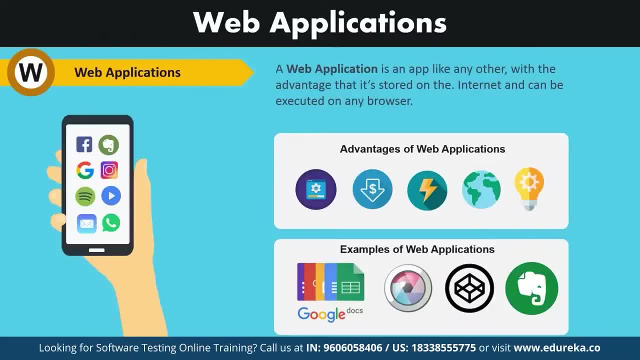 with their host of advantages. One is that you do not need to install anything. The second is that they are really cheap to actually develop and maintain. above that, they're kind of fast, depending on the speed of your internet, but in today's day and age almost everybody has super fast. 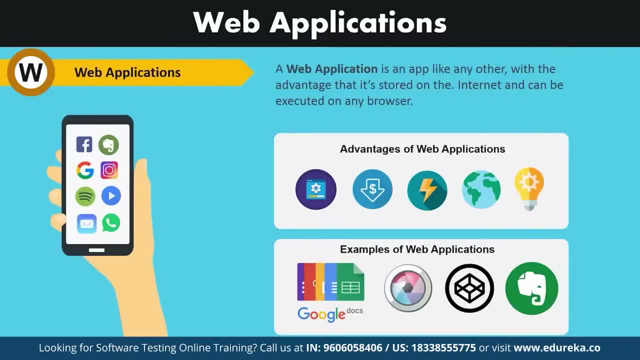 internet. So web applications are kind of the way to go If you are looking for speed over the internet. above that, they have a global access because you're not restricted by a Play Store or a marketplace of applications that is only catering to a certain operating system and above that setting. 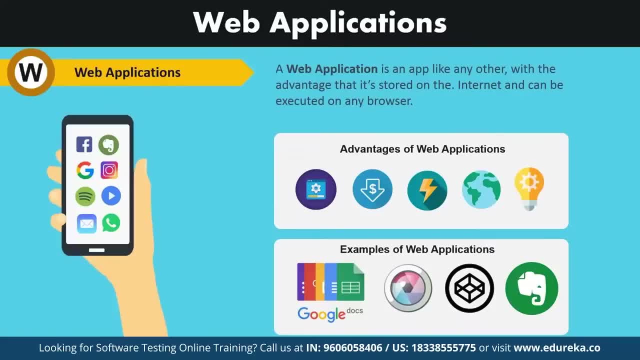 and maintaining them is really, really easy. Some examples of web applications include: pixel are Google documentation's, CodePen, dot, IO and Evernote. now, Google applications, or Google Docs, as you might know, is like an office suit and it's online. pixel are is just picture editing application that runs. 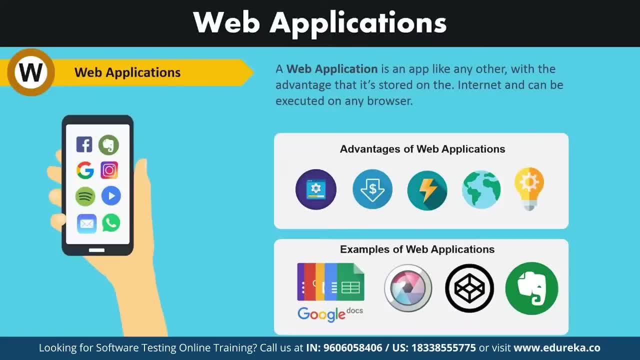 on your browser CodePen dot IO. It's like a repository of code, like GitHub, but it also lets you see how your code is being developed, and it's mainly used for web development purposes. Evernote, as you guys know, is everybody's note-taking app. 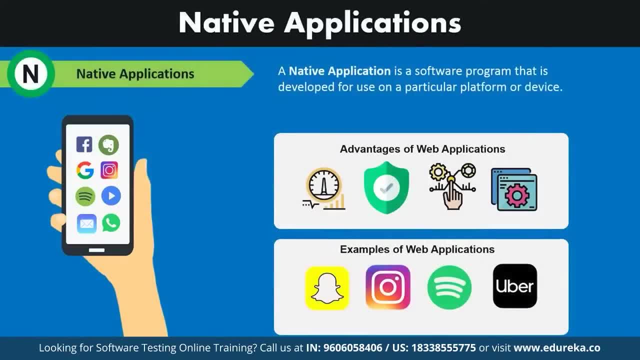 and you should definitely use it up. next, We have native mobile applications. now, native mobile apps are the most common type of application. They are built for specific platforms and are written in languages that the platform accepts, For example, Swift and Objective-C for iOS Java. 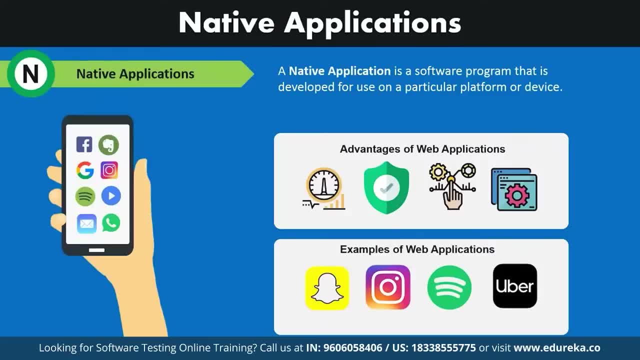 or Kotlin for native Android apps. native apps are also built using the specific integrated development environment, or IDE, for the given operating system. So both Apple and Google provide app developers with their own development tool and interface and elements and SDKs. most companies will invest in native mobile application development. 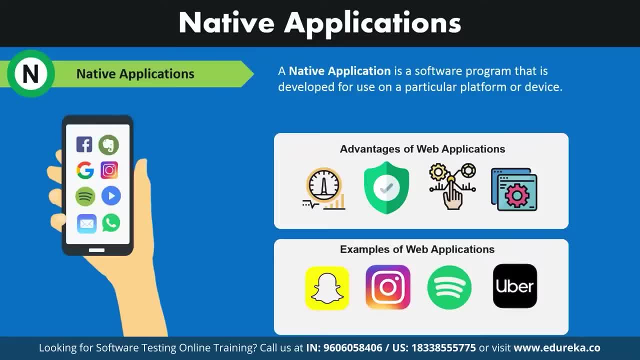 because there are a host of benefits offered in comparison to other types of applications. So let's go over a few of the advantages That come with native applications. So, firstly, native apps are very fast and responsive because they are built for that specific platform. 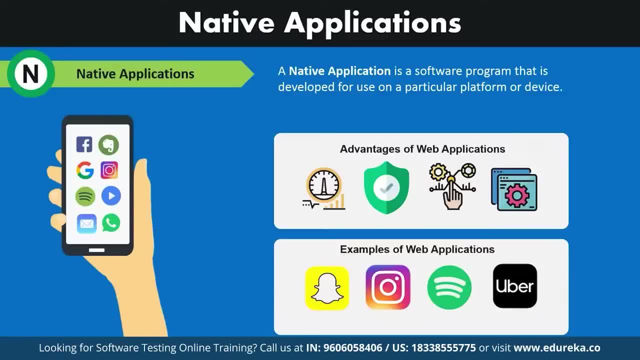 Secondly, they have the best performance that an application could offer. They are also distributed in the App Store, So you have the whole legitimacy aspect going on for them. Then they are more interactive, intuitive and run much smoother in terms of user input and output. 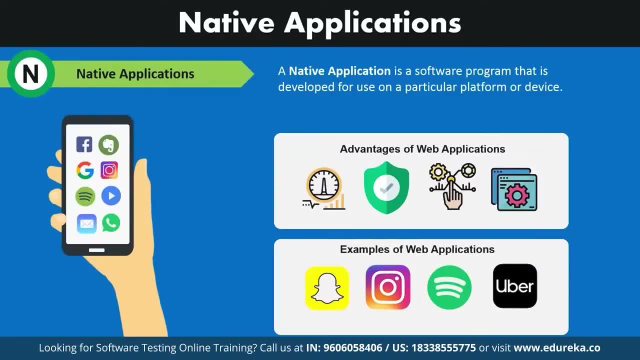 Above that, native applications allow developers to access the full feature set of their given platform, with whatever performance optimizations the native system has, but that internet connection is not required, Although it depends on the functionality. last but not least, overall better user experience is offered by native applications. 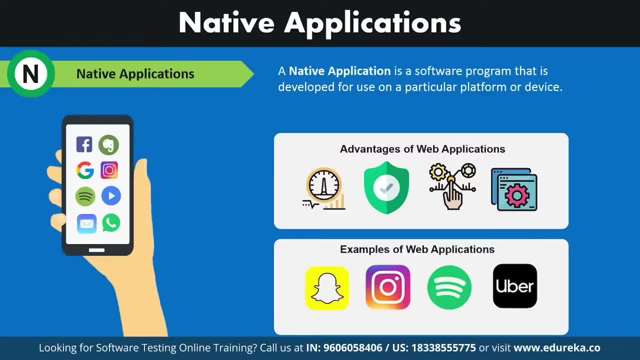 So to the user, the flow is more natural as they have the specific UI standards for each platform. Now, this doesn't mean that native applications don't have some disadvantages. For example, native applications can be difficult to develop as their difficult languages are being used. 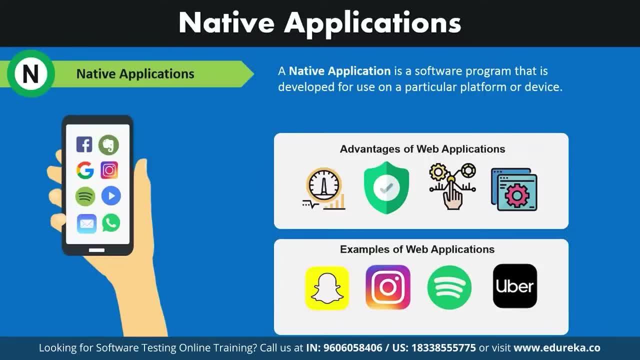 to actually develop them, So there might be a learning curve involved, unlike HTML, CSS and JavaScript. Also, they tend to be much more expensive because, for the people that you will be employing to develop your native apps, they will be charging you for their education. 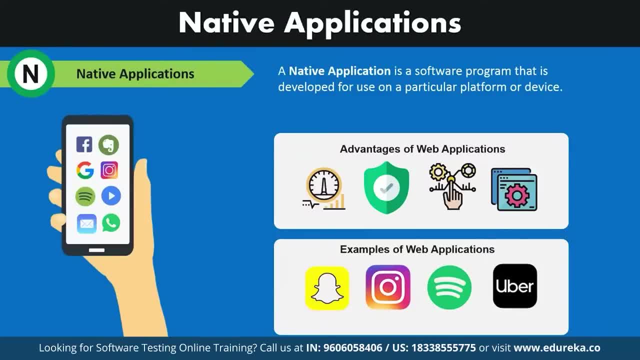 that has gone into actually learning how to deal with native apps, like how you would be paying a Swift developer or IO or a generic Android developer or Kotlin developer, Java developer. So web apps can't access device features, which many view as a major disadvantage. However, on contrary, mobile apps need to keep downloading updates. 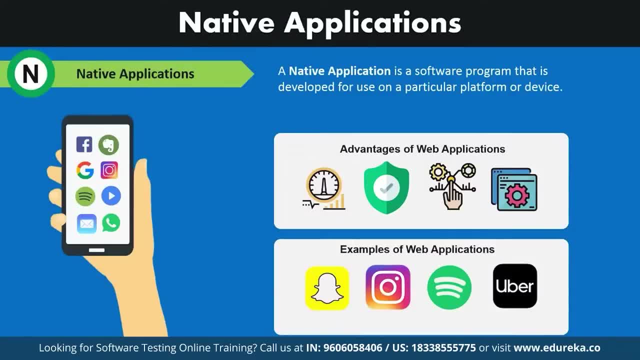 to improve accessibility, while web apps can update itself without any involvement of the user. Additionally, with native mobile application development, you get direct access to all native frameworks which otherwise may not be available, Although the initial cost may be higher with a native app. 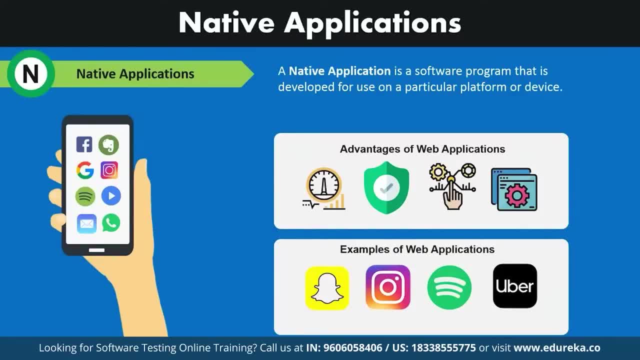 You'll end up saving a lot of time and money in the long run. by offering a great user experience, better performance and leveraging the device features, You're able to offer your user a more personalized experience. The combination of native mobile applications advantages will result in higher conversion rates. 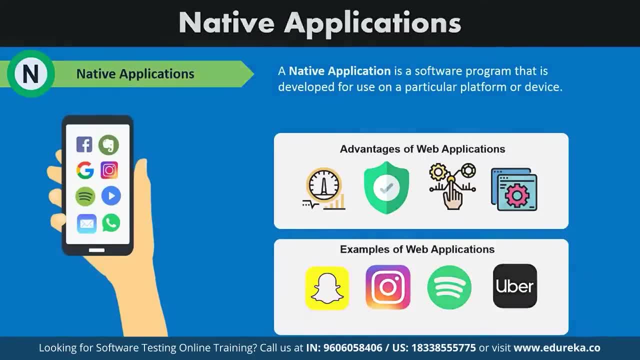 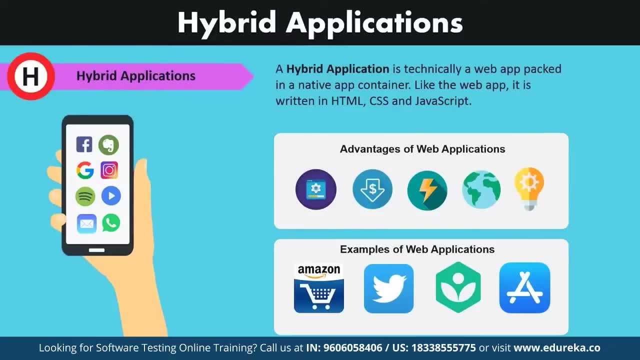 and will ultimately boost customer loyalty for your app. Now, the last kind of applications that we are going to discuss are called hybrid applications. Now, hybrid application work across platforms and behave like native applications. A hybrid app is essentially a combination of native application and a web app. users can install it. 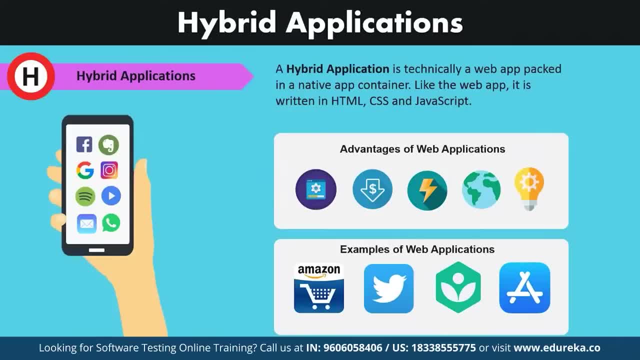 on their device like a native application, but it is actually a web application, and these types of applications are built with JavaScript, HTML and CSS and run in the web view. Hybrid app development can essentially do everything HTML 5 does, except it also incorporates native app features. 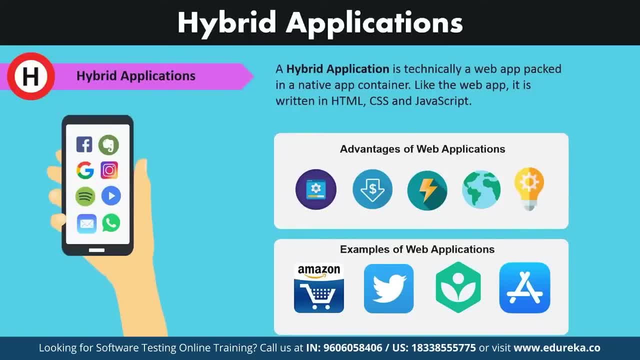 This is possible when you deploy a wrapper to act as a bridge between the platform to access the native features. So basically, it's a web app that is wrapped around the native app features. now, hybrid app consists of two parts. The first is the back-end code built using languages. 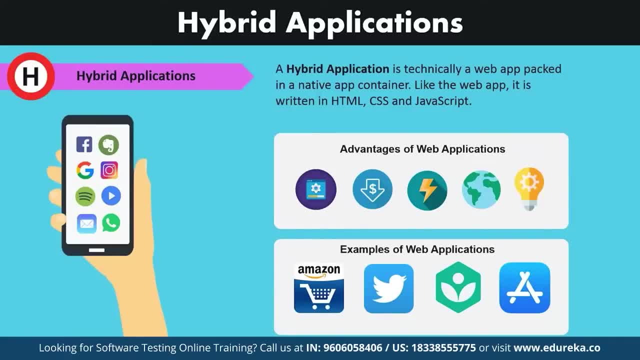 as HTML, CSS and JavaScript, and the second is a native shell that is downloadable and loads the code using a web view. now, hybrid applications come along with their own advantages too. So, first of all, they're built on web technology, that is, HTML, CSS and JavaScript. 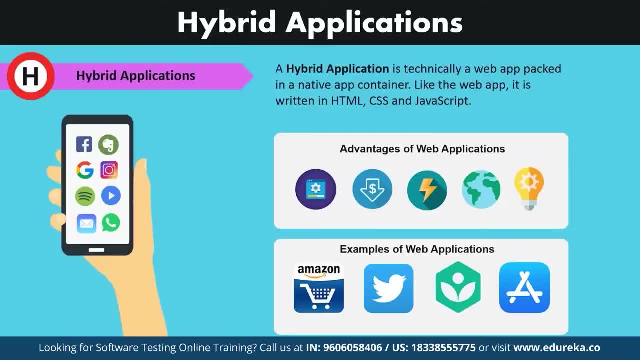 So it's much easier to build. They're also a cheaper alternative to native applications, and one app for all platforms is a thing that hybrid application developers are going for. So it's basically one app and it works on every single platform, So it uses technologies like Cordova above. 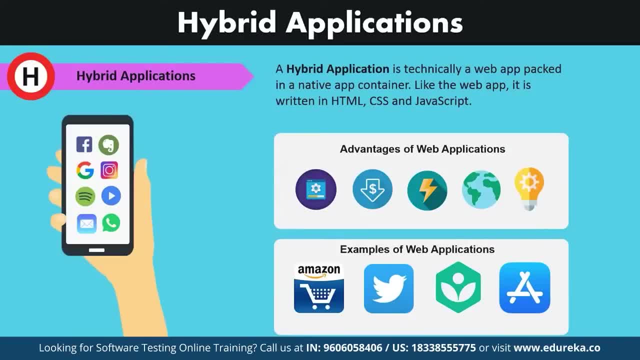 that no browser needed as opposed to a web app. So I like a web app which makes it quite ugly by introducing the whole browser view. hybrid apps completely negate that, even though they are indeed using a web app in its core. above that, hybrid apps can access to the devices internal APIs. 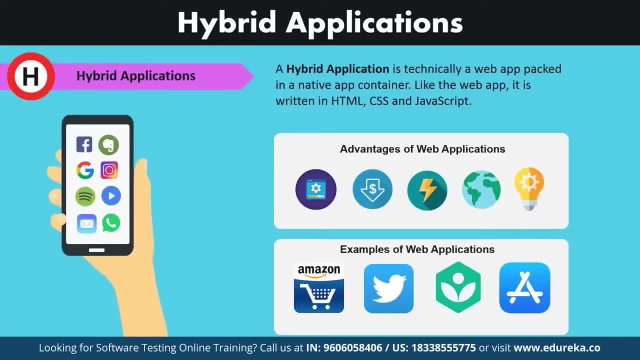 and can access storage cameras etc. above that, it's faster to develop the native apps because you have a single code base. This also doesn't mean that they don't have the disadvantages. For example, they are slower than native apps. They're also more expensive than web apps. 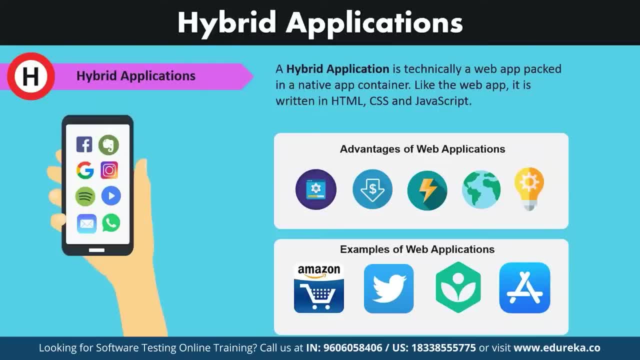 because you are require a wrapper essentially are dependent on third-party platform. They're also less interactive than native apps and customizations will take you away from the hybrid model, in which you may as well go native. So with hybrid, you have to contend with issues. 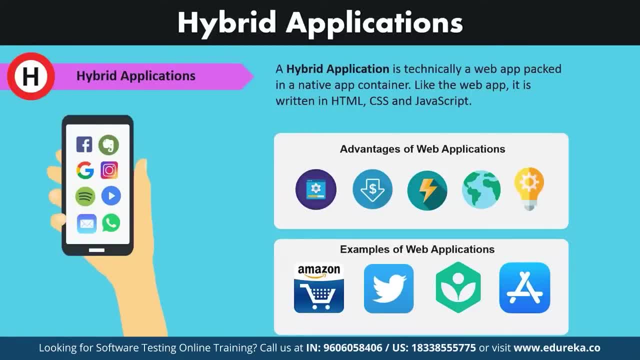 that stem from both native systems and hybrid systems, which makes bug fixing more difficult. The performance is also a disadvantage because hybrid apps load in web view. the user experience is often sacrificed with a hybrid app, as you cannot customize the app based on the platform. 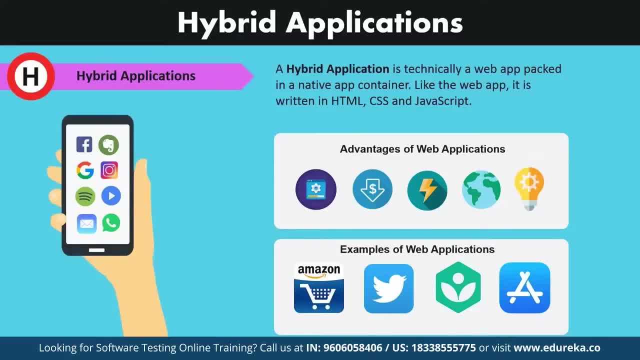 Another disadvantage is that you can customize your app the way you would be able to do with a native app. In fact, the more customizations you do, the more you're steering towards a native solution, So you might as well take the native approach. 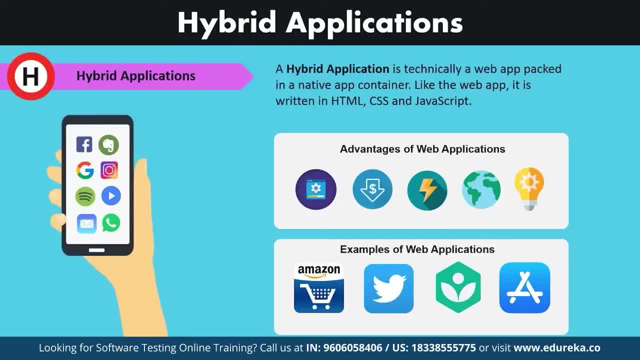 Additionally, the more customizations you want within your hybrid app, the more expensive, and therefore a native solution will end up being a more cost-effective one. So if you do choose to customize your hybrid app, you will end up spending A lot more money and time. 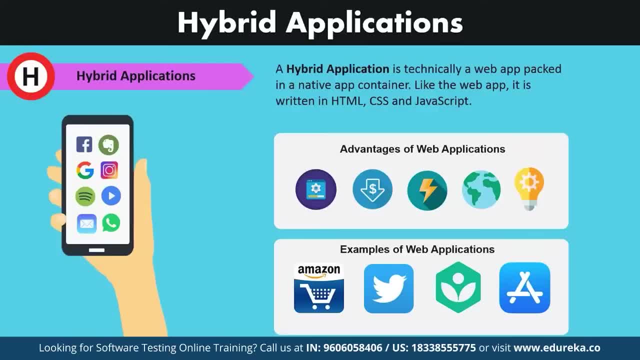 So, when it comes down to a web application versus a native application, was a hybrid application? which approach is the West? well, the decision to build either a web, native or hybrid mobile app should be based on your business objectives. before jumping into development, You should consider the following factors. 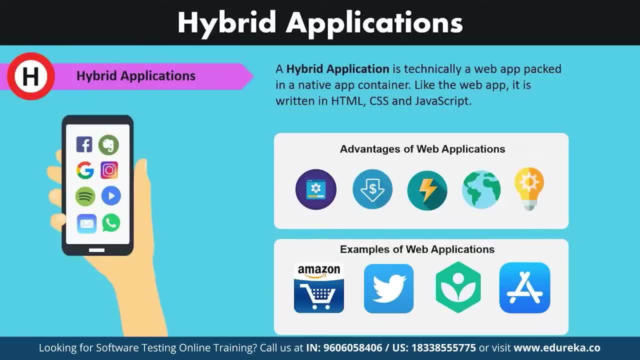 like how fast you need the app, the quality of the user experience you want your app to have, the complexity of the features you need for app to work, and your budget. So, keeping all these things in mind, you can very well decide whether you need a hybrid application, a native application. 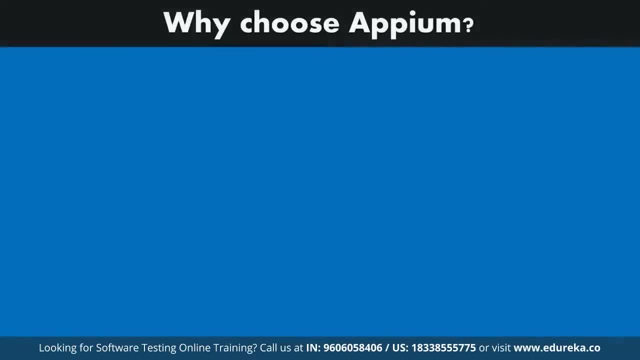 or just a simple web application. Okay, So now moving on, let's get back to Appium. and now let's discuss why you should choose Appium when there are so many other competitors in the market. Okay, So, now that we have discussed the three different types, 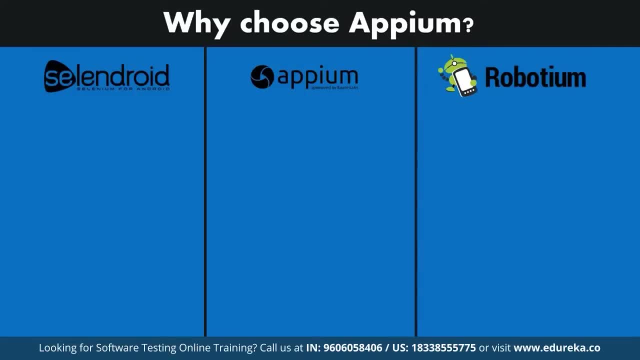 of applications when you should try and develop them, in what use cases and the different advantages, along with their few examples, let us move forward to the spotlight of today's tutorial, and that is the tool called Appium. now, the topic that we are going to currently discuss is why you should choose Appium. 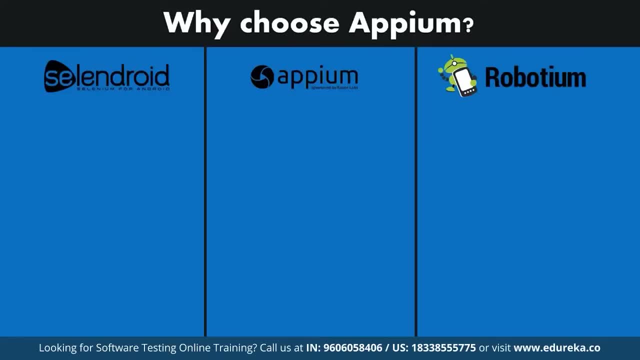 So the best way to convince somebody to choose a certain tool is by comparing it with its market competitors. for this particular comparison, I have kept the comparison between free and open source tools instead of paid Enterprise versions. So since Appium is free and open source, 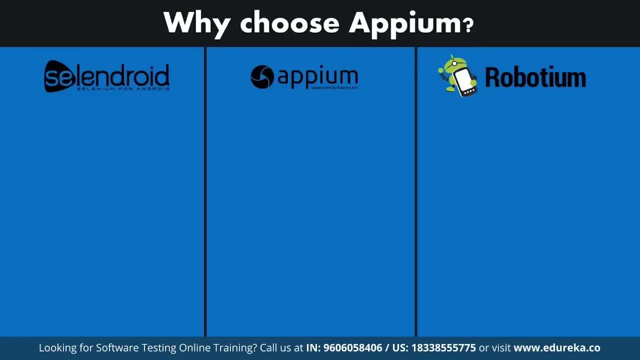 it is only fair that we compare them to other free automation testing tools. Okay, so the tools that we are going to test: Appium against our cell, Android, which is basically selenium for Android, and Robotium. So firstly, let us go ahead and see the features of Appium. 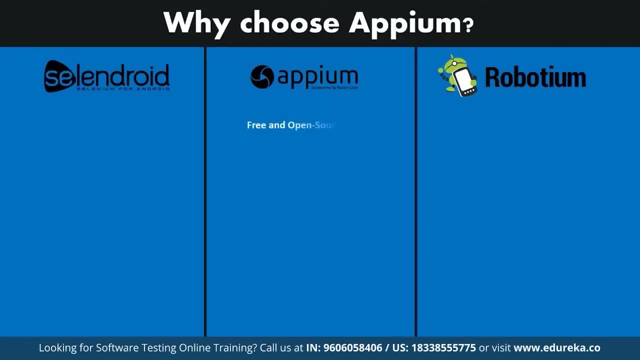 that make it such a beautiful choice. So, firstly, Appium is free and open source. Secondly, it supports both iOS and Android apps for testing purposes. above that, when you use Appium, there is no need for the app source code to be available to the tester. 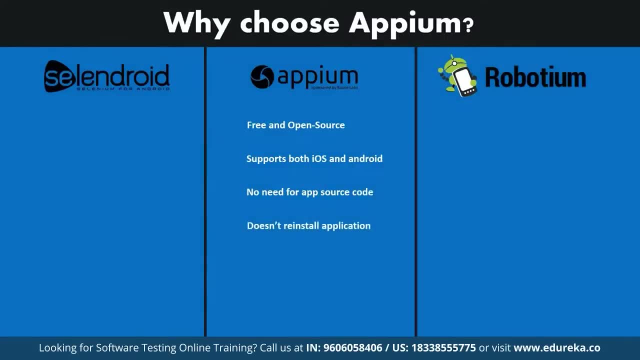 as he can just test the app without reinstalling the application. which brings us to the fourth point, that Appium never reinstalls the application again and again because Appium actually believes in testing the app that you will actually release to the marketplace. So when you reinstall an application, 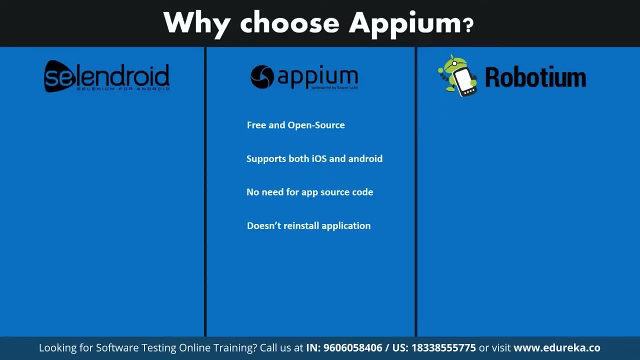 with third-party agents for automating purposes. it kind of beats the purpose above that. Appium supports multiple frameworks and programming languages like Ruby, Scala, Kotlin, Java, Python and a bunch of other different languages. last but not the least, Appium has a strong, active and budding community, which means any help that you need. 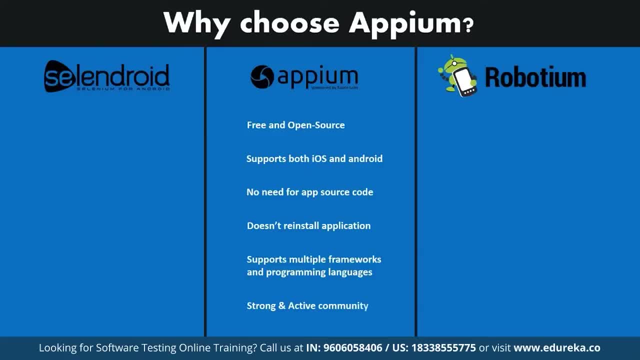 will be actually given to you by the community itself because it's such an proactive one. Okay, Now let's discuss how Cylindroid compares with Appium. So Cylindroid is lenient for Android, which is also free and open source automation testing tool. 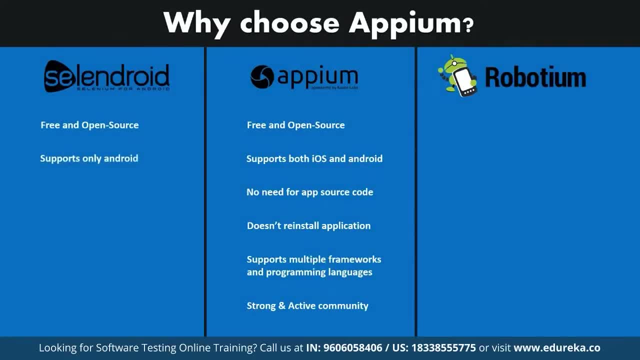 Unfortunately, as the name suggests, Cylindroid can only be used for testing Android apps. above that, Cylindroid also needs the app source code or the app library that has been used for development. also, the thing that actually puts Cylindroid guide quite back. 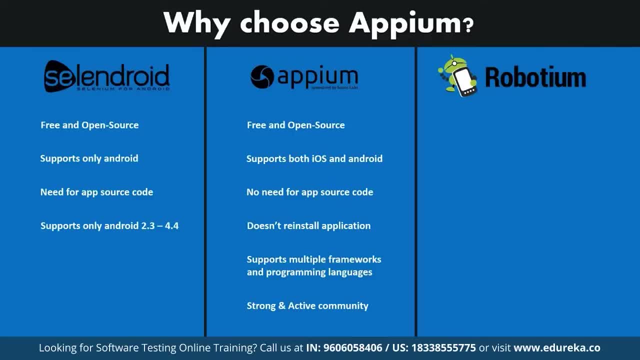 is that it only supports Android 2.3 to Android 4.4 and we are currently at Android 8.. I guess I might be wrong. We could be an Android 9.. I'm not really up to date with how Android is going about. 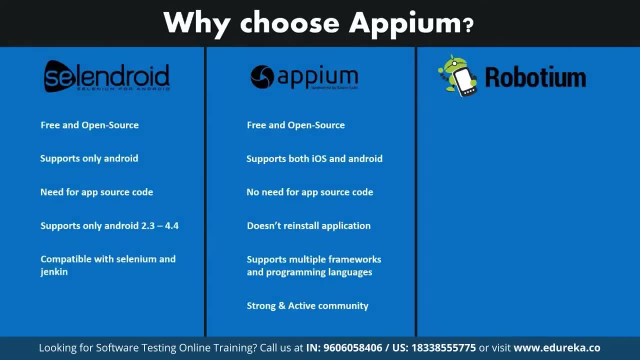 about that. Cylindroid is also compatible with selenium and Jenkins, which is great, and a Cylindroid also has a community going for it, but it's not as strong As Appians. now let's get down to discussing about Robotium. 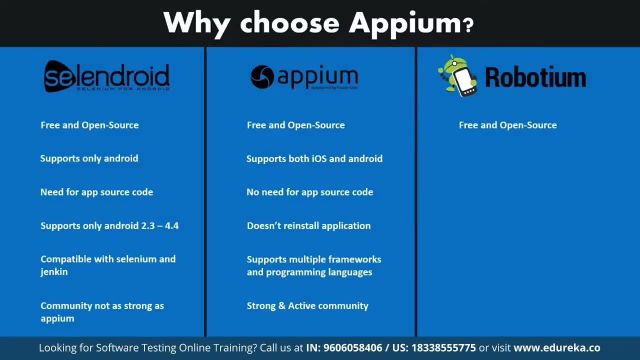 So Robotium is also free and open source automation testing tool. Unfortunately, it only supports Android. It also needs the app source code and library. above that, small changes in the Robotium code could actually lead you to completely rebuild the application. above that, Robotium only supports Java. 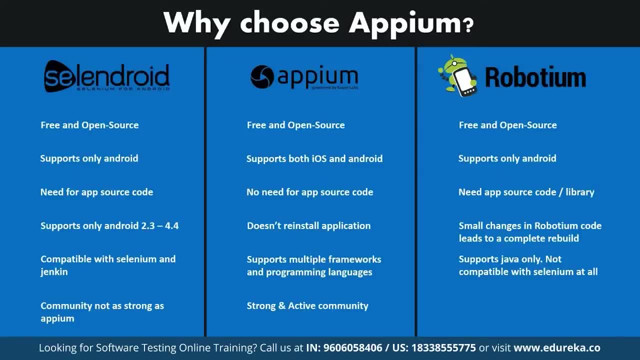 So other languages that are used to develop applications like Kotlin, for example, which has become really famous in these days, It will not be actually supported by Robotium. above that, It is not at all compatible with stuff like selenium and Jenkins. also, Robotium doesn't really have 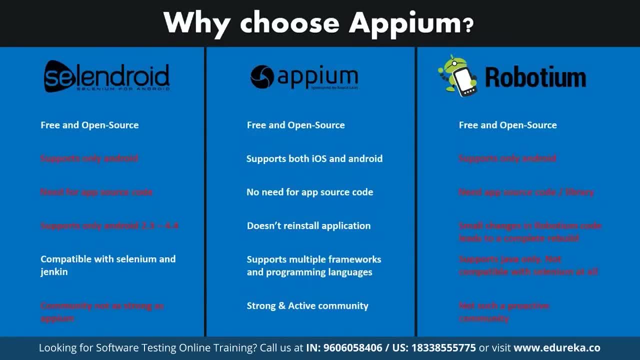 that greater community. So, as you guys can see, these points that have become read now are kind of what draws them back when compared to Appium. Appium, On the other hand, out shines in front of its market competitors, that is, Cylindroid and Robotium. 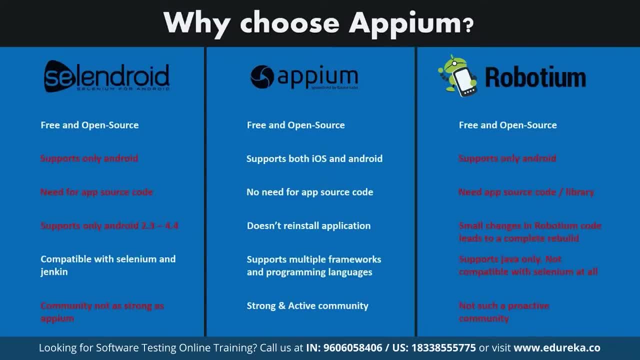 You guys can also compare Appium with other free and open source automation testing tools and I assure you Appium will stand out to be the best. It is with good reason that Appium has such a strong and budding community and such a wide scale acceptance. 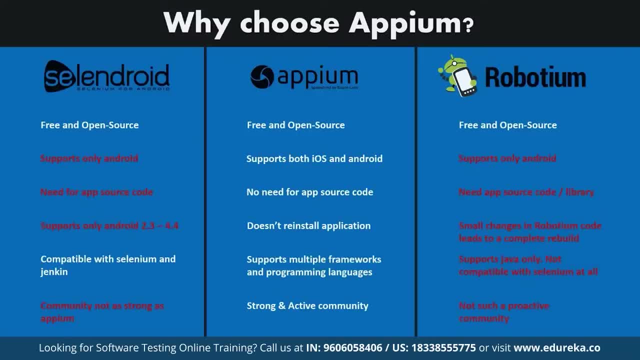 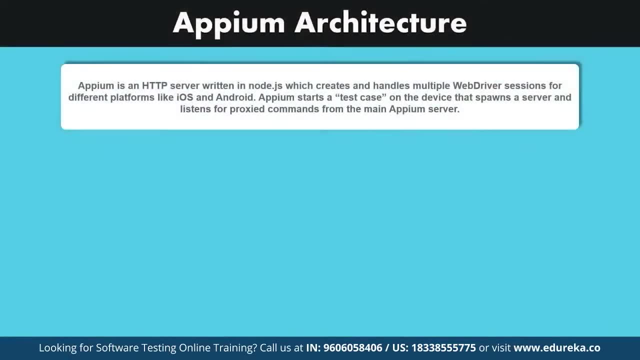 around the globe amongst automation testers. So now that we have discussed why Appium stands out to be the best automation testing tool, Let us go ahead and discuss the architecture that makes this tool So brilliant. So Appium is basically an HTTP server written in nodejs. 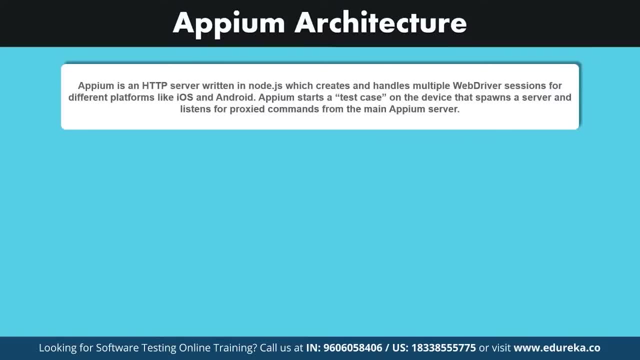 which creates and handles multiple web driver sessions for different platforms like iOS and Android. If that didn't make any sense to you, let me just simplify it a bit more. So what Appium does is it follows the client server architecture. Now on your left hand side of the screen. 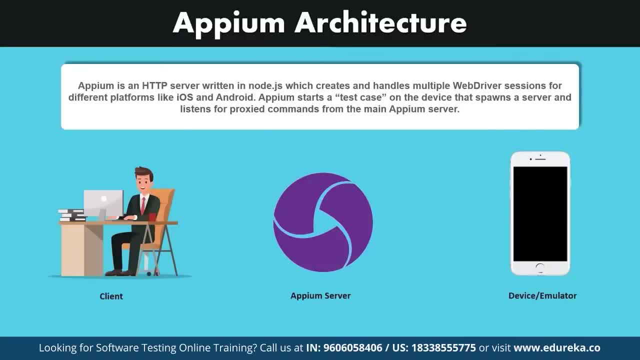 What you see is the client, who is also the tester. Now, what this guy will do is send some requests to the Appium server. Now, these requests are the green arrows that you see. So, first, the request is sent to the Appium server. 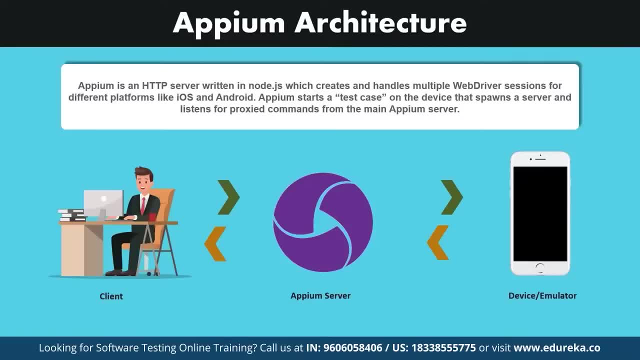 Now the Appium server, along with its brilliant API, decides how to actually handle the request and then, with the appropriate decisions being made by the server itself, without any complications that you might need to worry about as a tester, It sends these requests to the device and the emulator. 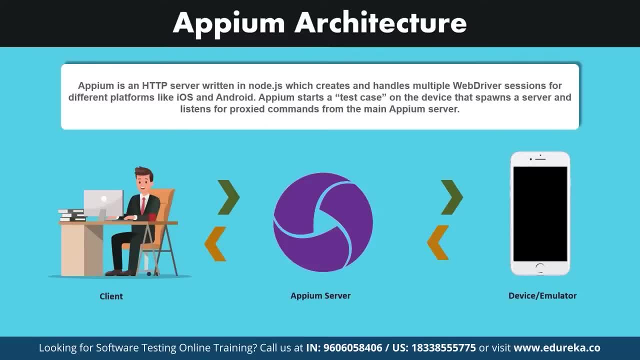 So the device or the emulator runs the test cases according to how they are written and then sends back the response to the Appium server, which in return sends it back to the client. So Appium starts a test case on the device that spawns a server. 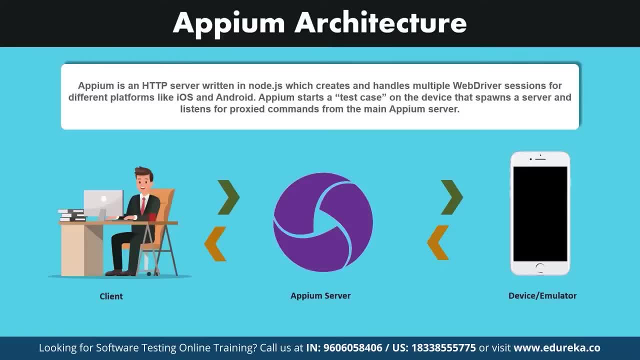 and it listens for proxy commands from the main Appium server. It is almost same as a selenium server which perceives HTTP requests from selenium client libraries and it handles those requests in different ways depending on the platform. each vendor, like iOS and Android, have a different way and mechanism to run a test case. 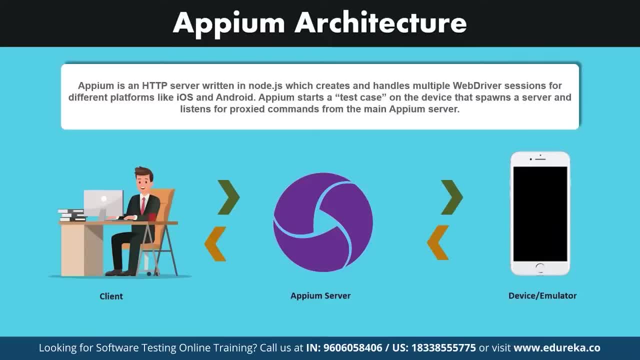 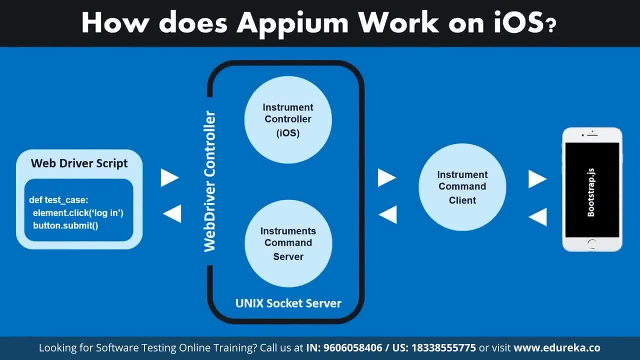 and so Appium kind of hacks into it and runs these test cases after listening commands from the Appium server. So first of all, let's discuss how Appium works on an iOS device. On iOS, basically, Appium proxies commands to a UI automation script running. 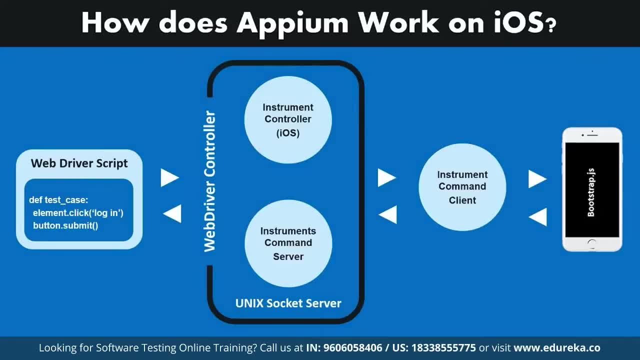 in Mac instrumentation environment. Apple provides this application called instruments, which is used to do lots of activities like profiling, controlling and building iOS apps. but it also has an automation component where we can write some commands in JavaScript which uses UI automation apis to interact with the app: UI Appium. 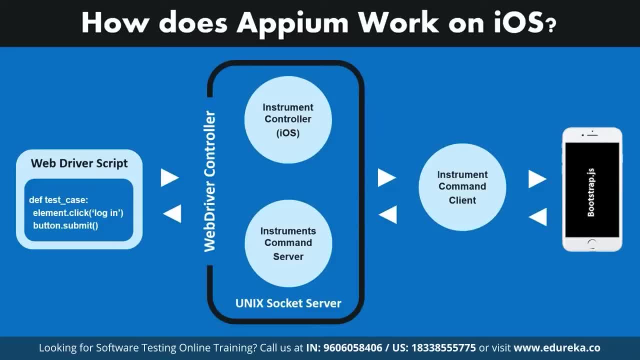 utilizes these same libraries to automate iOS apps. So in the diagram there that you see on your screen, we can see that the architecture of Appium in context to iOS automation. If we talk about the command life cycle, it goes like selenium web driver. 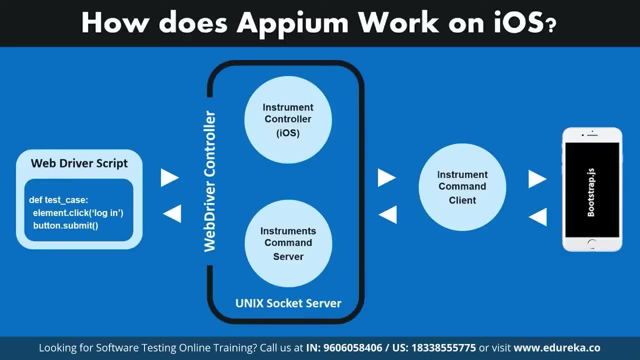 It picks up a command from the code like element dot click and sends it in the form of a JSON representation via an HTTP request to the Appium server. Now Appium server knows the automation context, like iOS and Android, and sends this command to the instrument command server. 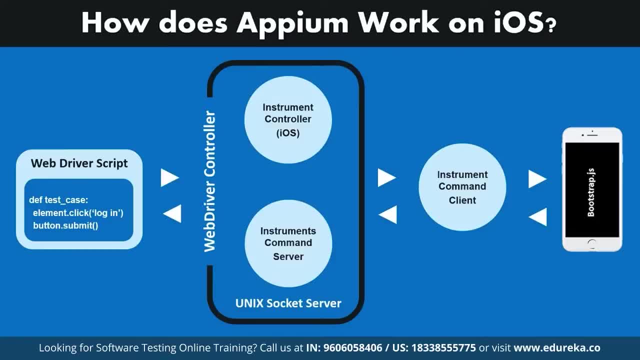 which will wait for the instrument command client, written in nodejs, to pick it up and execute it in bootstrapjs with in the iOS instrumentation environment. Now, once the command is executed, the command client sends back the message to the Appium server, which logs everything related to the command in its console. 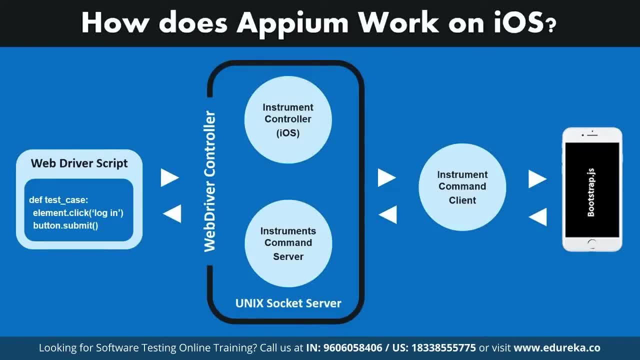 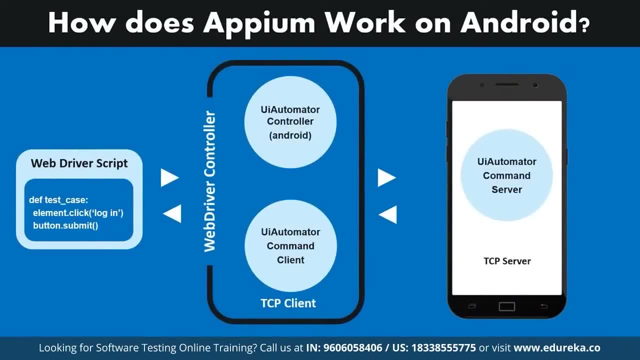 The cycle keeps going till the time all the commands get executed. Now let's move forward and see how Appium works on Android. Now the situation is almost similar in case of Android, where Appium proxies commands to a UI Automator test case running. 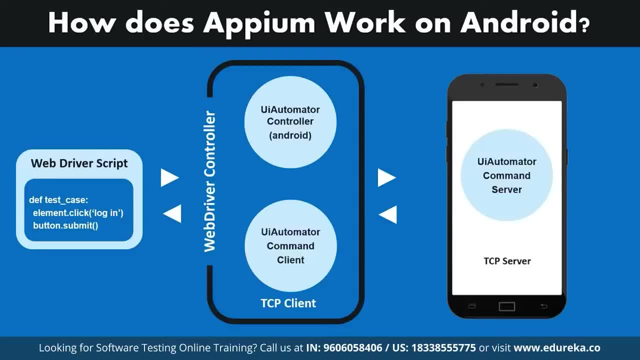 on the device. So UI Automator is Android's native UI automation framework which supports running JUnit test cases directly into the device from the command line. It uses Java as a programming language, but Appium will make sure it runs from any of the web driver supported languages. 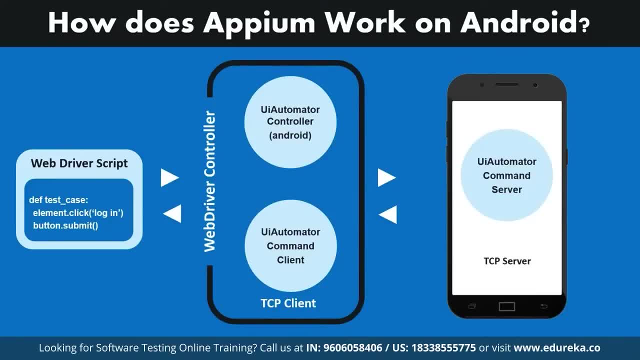 So in the diagram that you see, we have the bootstrapjar in place of the bootstrapjs, which represents our test case. when compiled in Java, As soon as it gets launched it spawns a TCP server. Here, the TCP server resides inside the device and the client is in the Appium process. 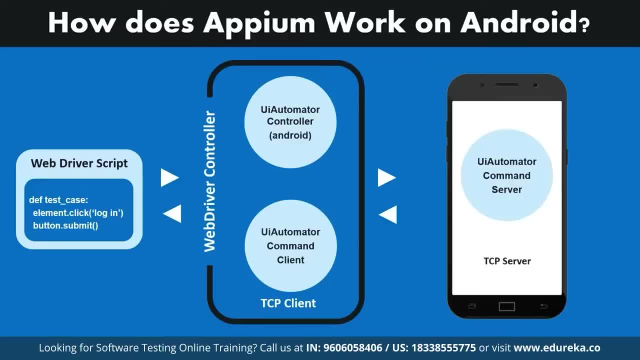 which is just opposite to the way it is in iOS. Okay, So that was all about how Appium works on both iOS and Android and the small nitty-gritties that make out the difference between the two systems. Now let's move ahead and discuss the philosophy of Appium. 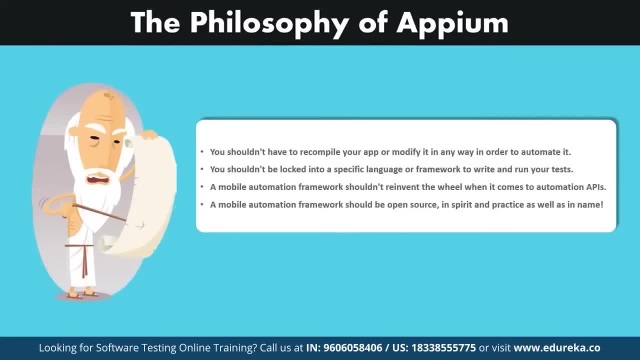 So Appium is a rising star in the mobile test automation landscape and since a few of the developers here at SauceLab are regular commuters to the project, It's pretty close to their heart. Now you'll often find SauceLab developers hanging out at the Appium Google group answering questions musing. 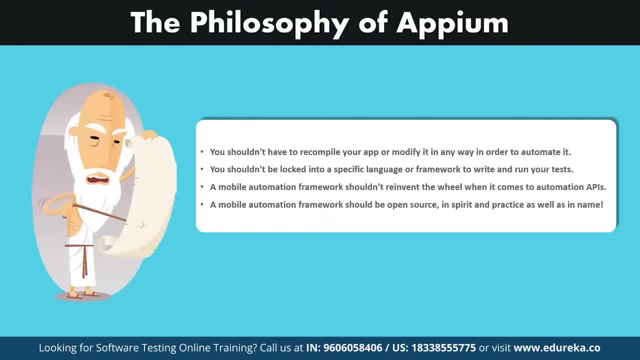 about testing strategies and helping folks tweak their configuration or hunt down bugs When it comes to mobile test automation, in many ways they're still figuring out the best approaches and, with Appium, the benefits of lessons learned from early automation solution that didn't quite work as well. 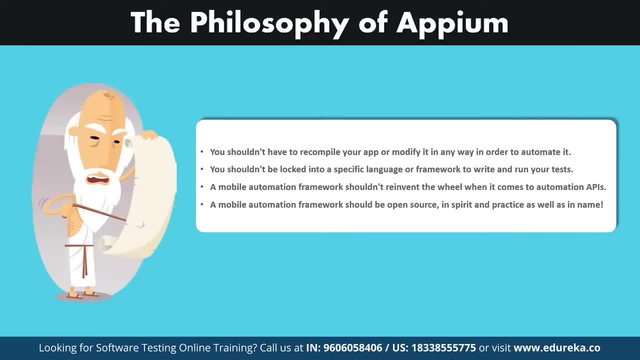 So these guys actually put up something called the four-point Appium philosophy. So the philosophy is as it goes. So, firstly, the first philosophy is: you shouldn't have to recompile your apps or modify it in any way in order to automate it. The second one is: you shouldn't be locked. 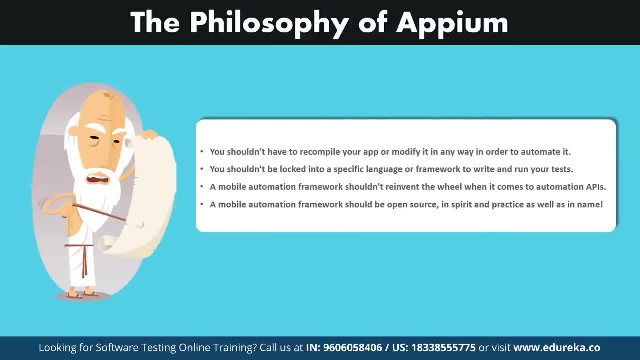 into a specific language or framework to write and run your tests. thirdly, a mobile automation framework shouldn't reinvent the wheel when it comes to automation api's. and fourth is that a mobile automation framework should be open source in spirit and practice, as well as a name. 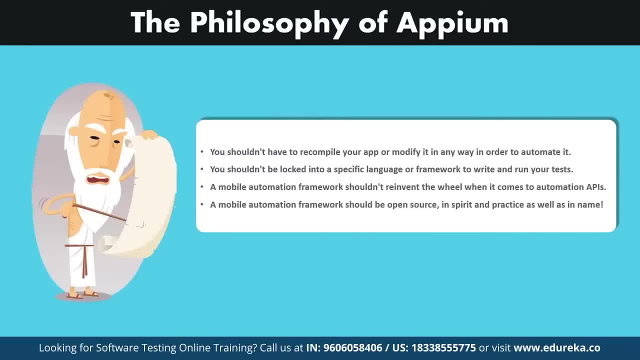 So let's explore these four points, shall we Now? you shouldn't have to recompile your app or modify it in any way in order to automate it, So some earlier attempts at mobile test automation were based around OCR and pixel based interaction. 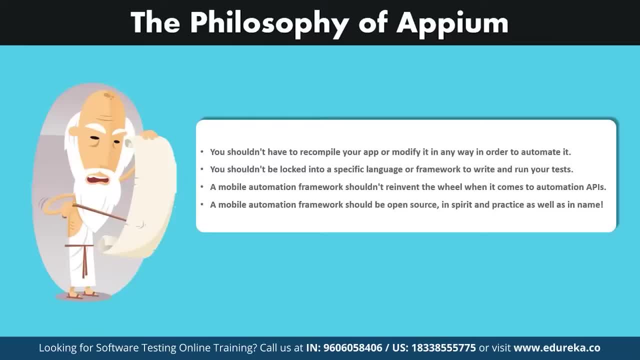 which history tells us are never very reliable. after that, We saw the introduction of in-app agents that can execute the underlying code that would otherwise be triggered by a user interacting with the application. These agents then make calls to the same code, triggering user actions like swiping. 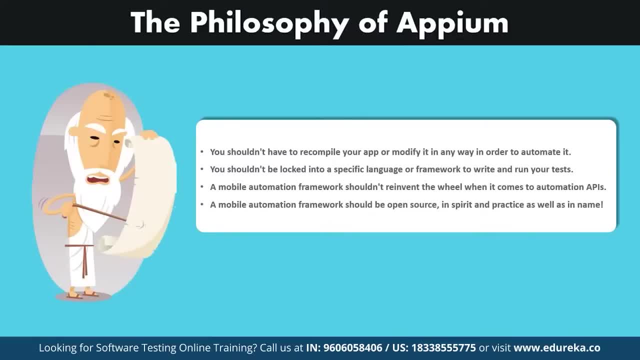 and taps and pinches. It's not a bad solution, but it's that it's got you to have to compile these agents into your app while it's being tested and you probably want to take it out after testing is done. the result: You're not actually testing the code that you release. 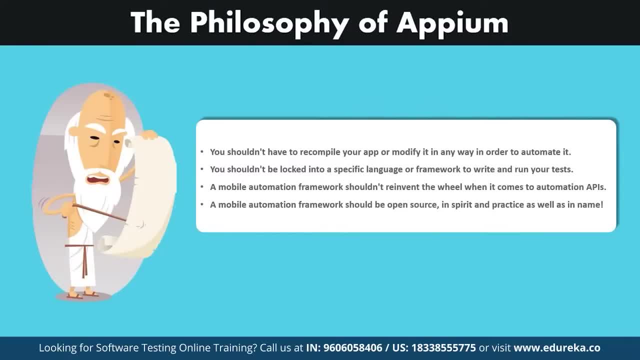 So the agent approach is a bit odd, since the real world user actions are always from outside the app itself, And so if you are simulating those actions inside code rather than triggering them by the corresponding UI actions, you're that much further away from the real experience of an actual human user. in order, 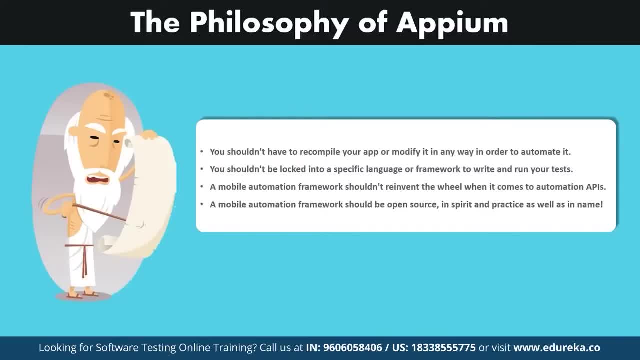 to solve the problem and provide for testing with these more real-world style users, both Apple and Google have created their interface automation frameworks for the respective development environments. Google provides UI Automator, which is a Java API for simulating this UI actions on Android devices and emulators, and Apple provides UI automation. 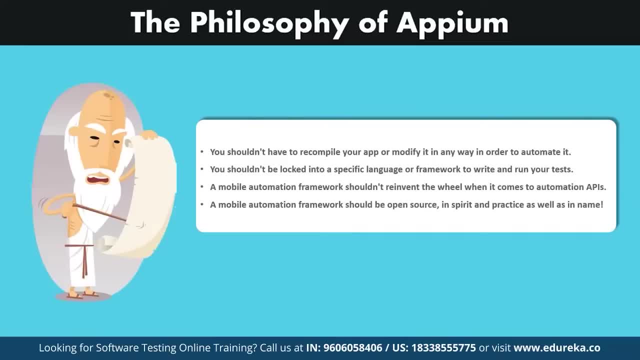 instruments, a JavaScript programming interface for use with iOS devices and simulators. So Appium works by interfacing with these vendor, provided automation frameworks, translating your test code into platform specific interactions, And I think that this is a better approach than using an agent, since you don't have to compile a test and build. 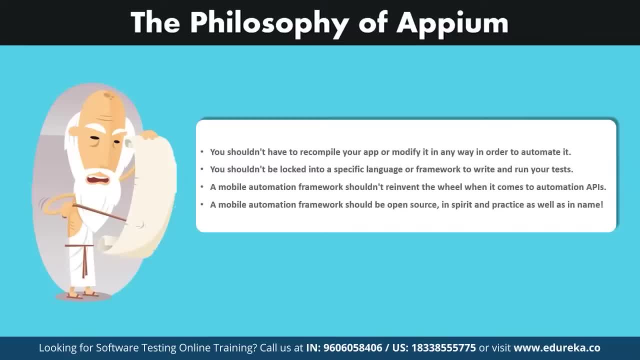 at which contains code which will not be in the production build, So you're best off testing the same code You will release. the next two points of Appium philosophy are covered together, since they both derived from the decision to implement the WebDriver API and the Jason wire protocol. 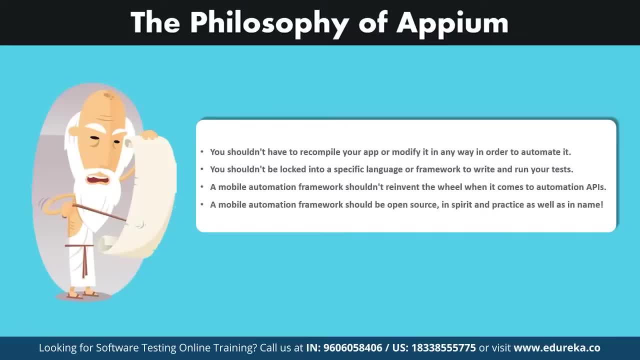 So you shouldn't be locked in to a specific language or framework to write and run your test, and a mobile automation framework shouldn't reinvent the wheels when it comes to automation APIs. So a WebDriver is already well known as the engine behind selenium to test automation for web apps. 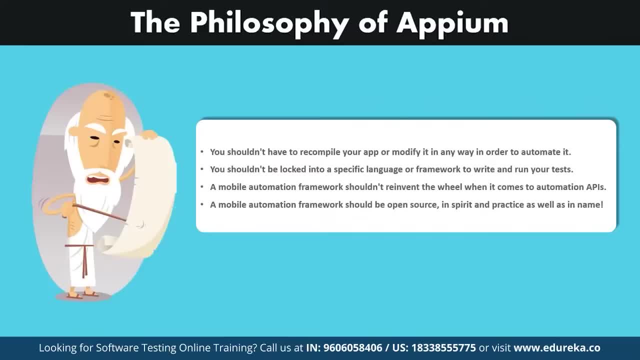 in Appium implementation instead of using a web browser on a desktop operating system, as selenium does. Appium drives native apps and browsers on mobile operating systems. Many testers are already very familiar with writing and running tests Locally using selenium WebDrivers, where you will open a web browser. run through some interactions. 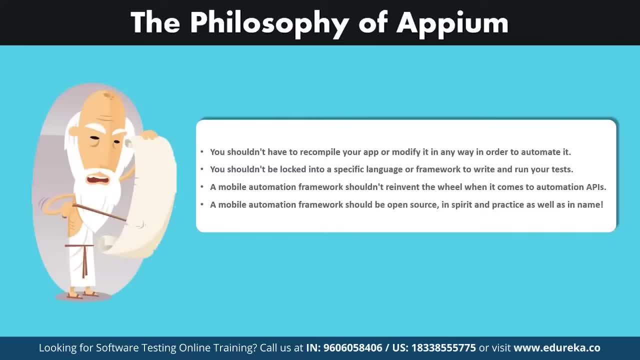 with the app and verify that the test cases passes. but the magic of WebDriver really happens when it is used in a distributed fashion. instead of making local calls directly to the browser, The WebDriver test becomes an HTTP client and makes requests to a WebDriver server, which in turn actually makes the necessary college. 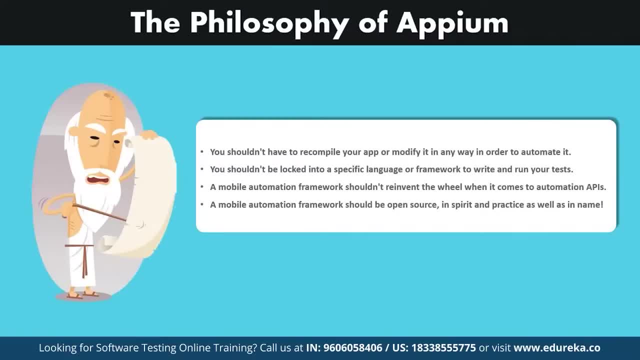 the browser and the application. the elegance of Appium is that it utilizes this framework to interact, not for the desktop browser, but with Android's UI Automator or Apple's UI automation instruments, which then performs user actions on the native app or mobile browser running in either an emulator. 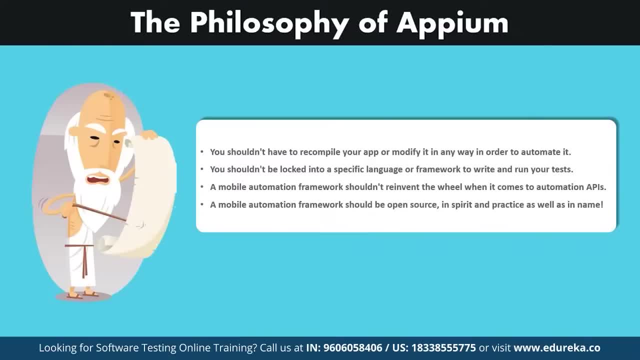 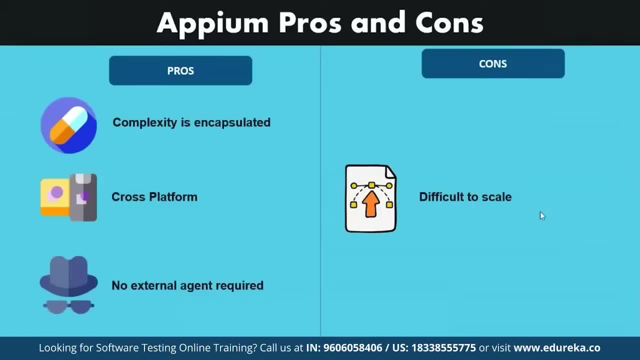 or real device and, of course, Sauce Labs infrastructure can manage all of this for you. Okay, So now, before we get on with installing Appium, let me just go over the pros and cons of using Appium as a mobile application tester. Okay, 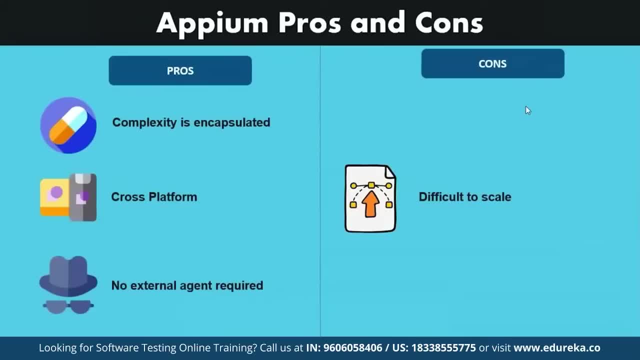 So, as you guys can already see, there are more pros and cons, because Appium is a brilliant app, So let's go the pros first, one by one. So the first positive aspect of Appium that I have pointed out is that the complexity of the testing environment. 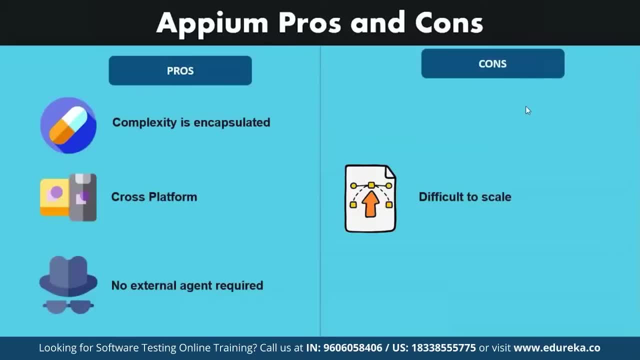 is completely encapsulated. So the beauty of Appium is that all the complexities are under the hood of Appium server and for an automation developer, the programming language and the whole experience would remain, irrespective of the platform He is automating, that is, iOS or Android. the other benefits: 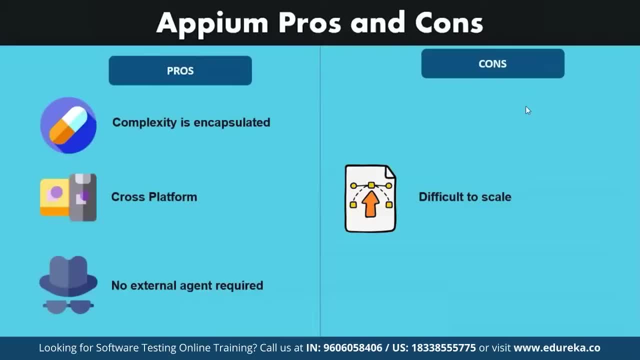 of Appium is that it opens the door to cross-platform mobile testing, Which means the same test would work on multiple platforms. above that, unlike other tools, Appium doesn't require you to include some extra agent in your app to make it automation friendly. It believes in the philosophy of testing that the same app. 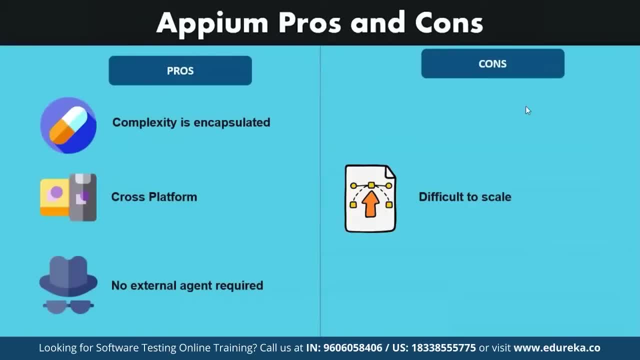 which we are going to be submitting to the application store. Also, it is developed and supported by Sauce Lab and it is getting picked up really fast within the web driver community for mobile automation and it can automate web hybrid and native mobile applications on the sides of cons. 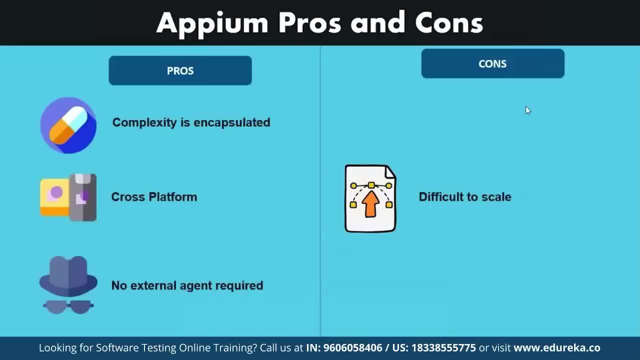 We have only one, and that is it is difficult to scale, So scaling up is an important consideration with continuous integration, and Appium comes across as a great tool to fulfill this expectation. The reason for this is a technical limitation in iOS. We can only run one instance on instruments for Mac OS. So we can only run our iOS scripts on one device per Mac machine. So if you want to run our tests on multiple iOS devices at the same time, then we would need to arrange the same number of Mac machines, which would basically be a very costly task. 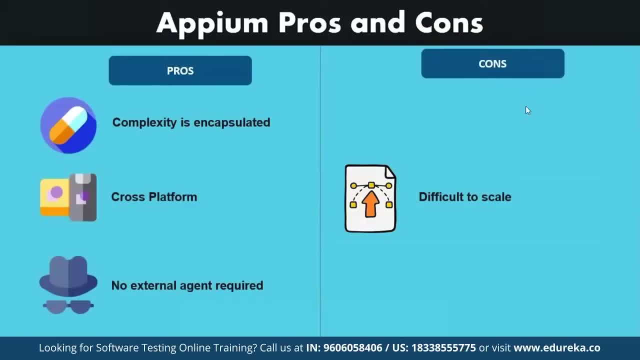 but this limitation can be resolved if we execute our scripts in Sauce Labs mobile cloud, which at present supports running scripts on multiple iOS simulators. Above that Appium uses UI Automator for Android automation, which only supports Android SDK platform, that is, API 16 or higher. 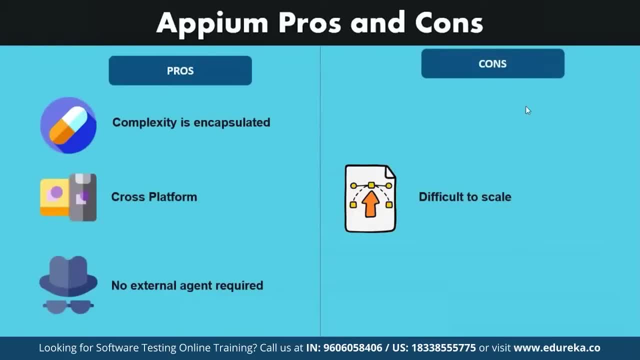 So to support the older API's they have used another open source library called Slendroid. So I would not say it is a limitation, but it is definitely an overhead on the configuration side. Okay, So that was on the pros and cons of Appium. 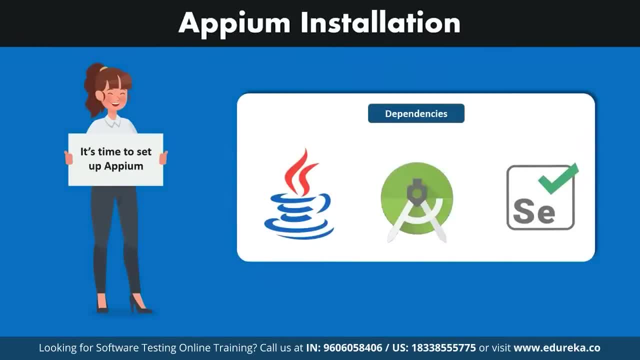 So let's go ahead and now get on with the demonstration part of our video today, and that is actually installing Appium and integrating it with Android Studio in this case. So now that we're done with the theoretical part of this Appium tutorial, it's time we actually go ahead. 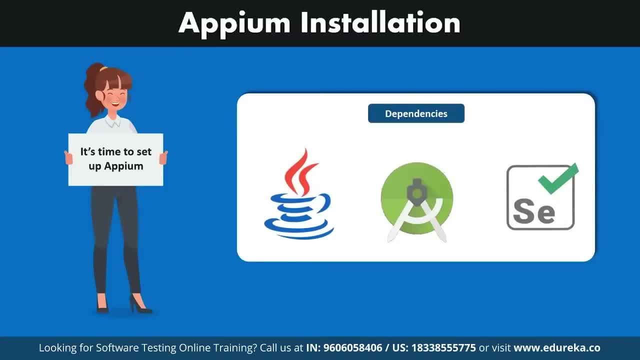 and install Appium on our own systems. Now Appium has a bunch of dependencies that it depends on for running seamlessly on your system and they're pretty easy to install. I know there's a buzz in the community that Appium can be a real pain to install on your system. 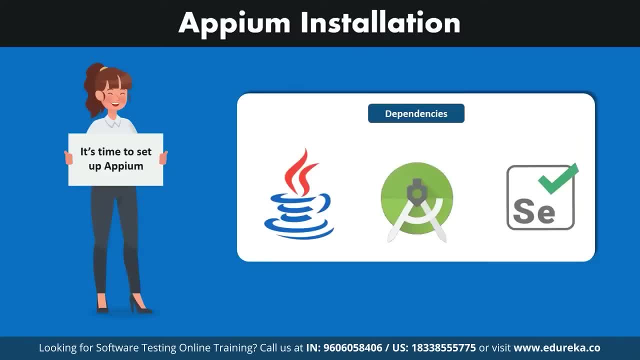 but that's all a myth, because I can assure you that it's a very simple process, and all you have to do is follow me step by step Now. first of all, we have to install Java onto our systems, if it's not already installed. 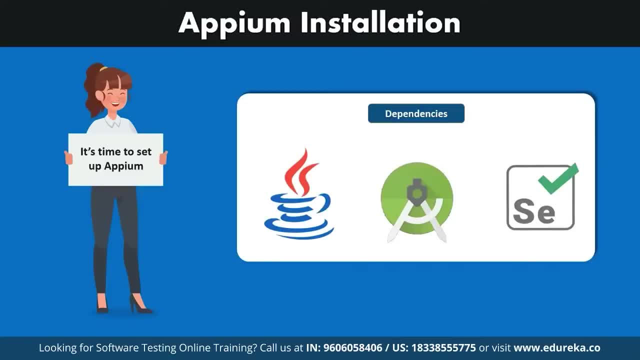 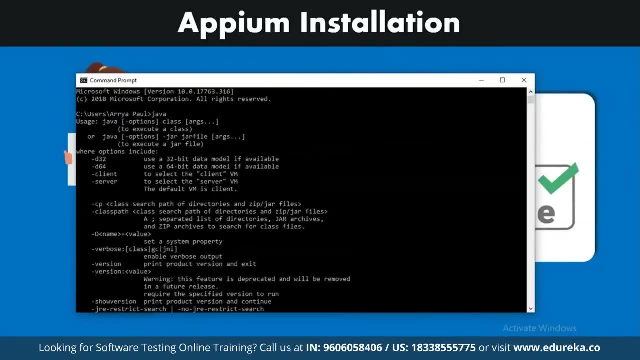 Now, if you want to know if Java is already installed on your system, all you have to do is go into your command prompt and just type in Java. Now, if you have Java installed, it should show up a help menu that shows something like this: 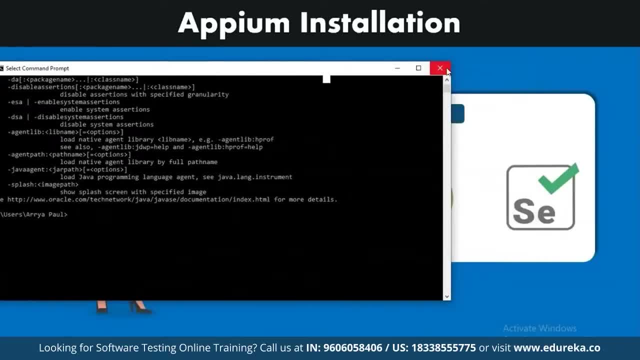 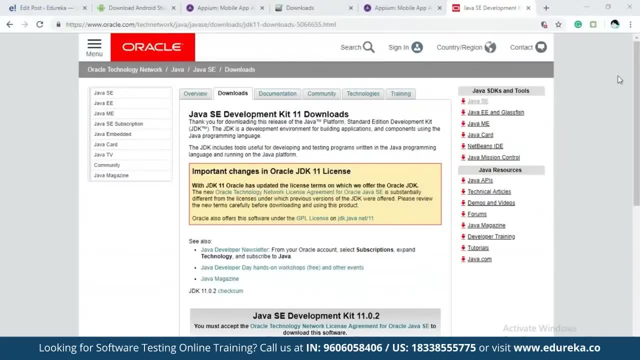 So Java has already been installed on my computer and I'm going to show you exactly how I did it. So first of all you have to go to the Oracle page out here. Now you can really do that by just going to Google and typing in Java and space download. 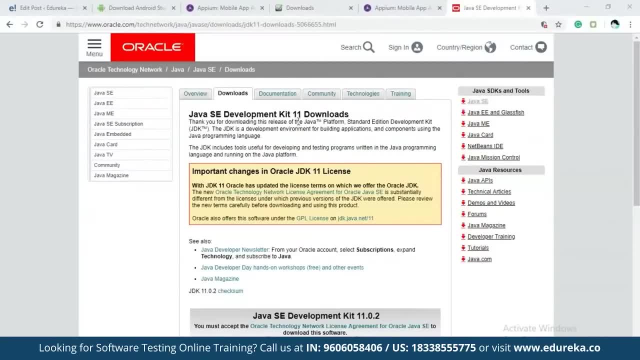 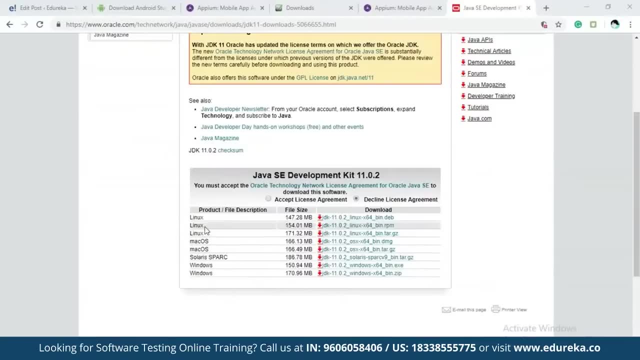 Now you will be redirected to the Java SE Development Kit 11 download, which is basically Java 11.. Now what you want to do is, according to your system, whether you were running Linux, Mac or Windows. Personally, I'm running Windows 10 right this moment. 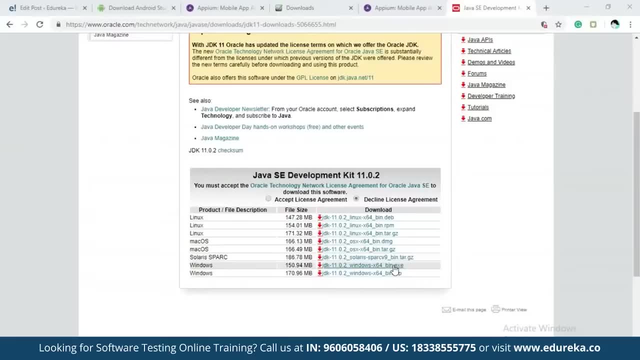 I am going to download this one, So this exe file that you see out here. So go ahead and download it. Okay, so it seems that I must agree to the license agreement before downloading, So you can do that by just checking the radio button out here. 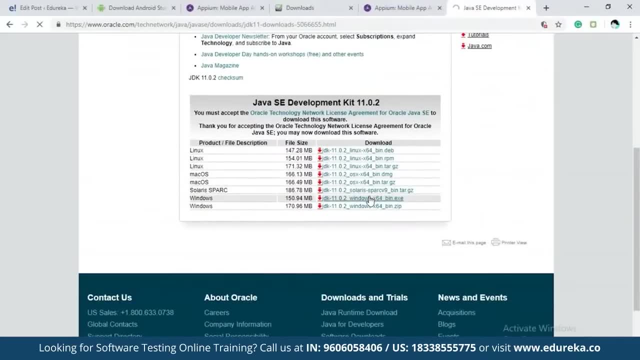 and all you have to do is then click on this link and it will start up your download. So, as you guys can see, this is downloading. I'm not going to actually download this file because I already have Java installed, But after you download this file. 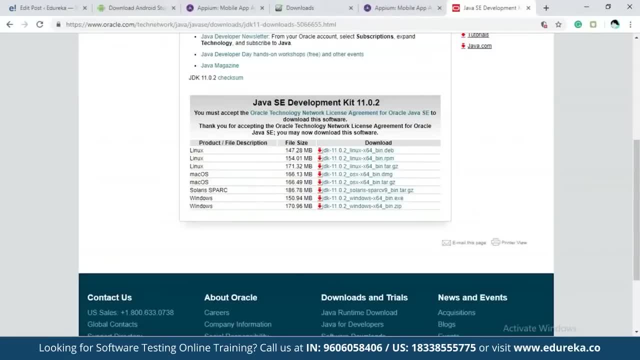 all you have to do is double click and follow the instructions that come onto the screen. So the tricky part is: well, it's not actually tricky. All you have to do is set the environment variables so that your computer knows where you've actually stored the Java SDK. 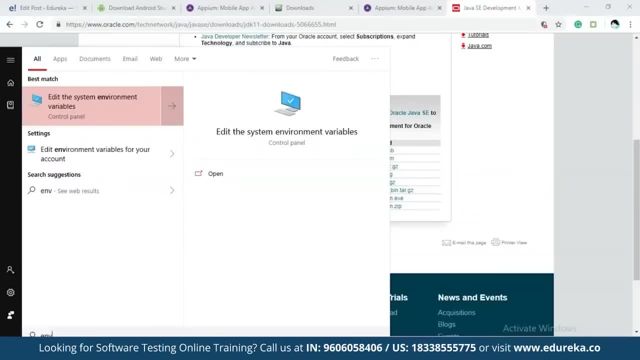 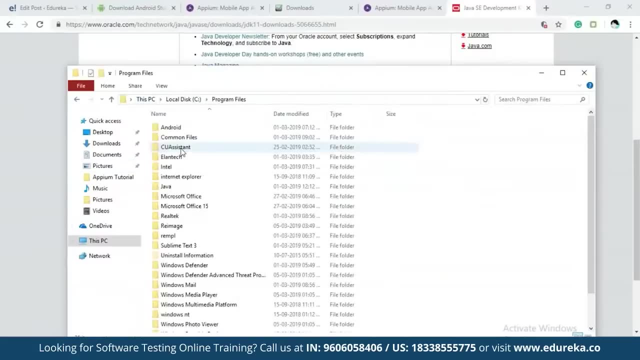 and the Java runtime environment. So after you've installed Java with the exe file, you can go ahead into this PC, going to local this C and going to program files. Now, program files should have a Java file which will have your Java JDK. 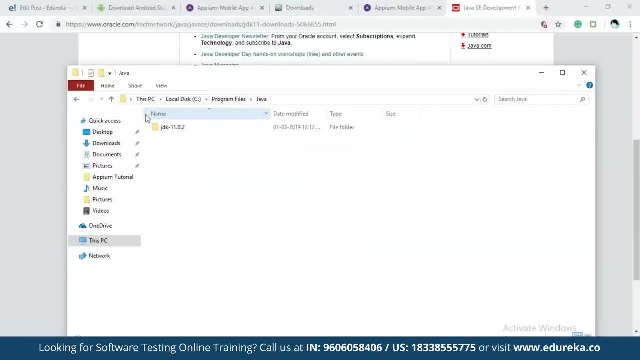 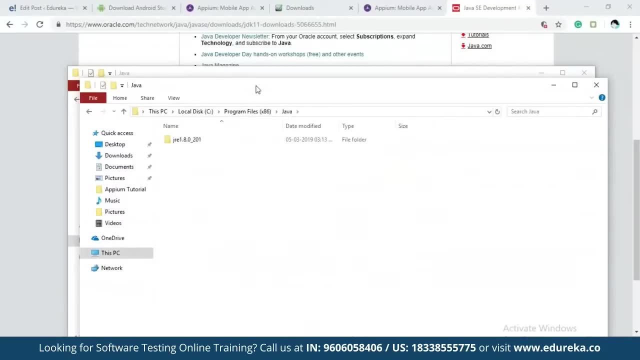 which is your Java Development Kit, and open up a new window of this PC, going to program files x86, and you will also see a Java file out here. So this is your JDK, So let's keep these open once you have installed or run the exe file that we just downloaded. 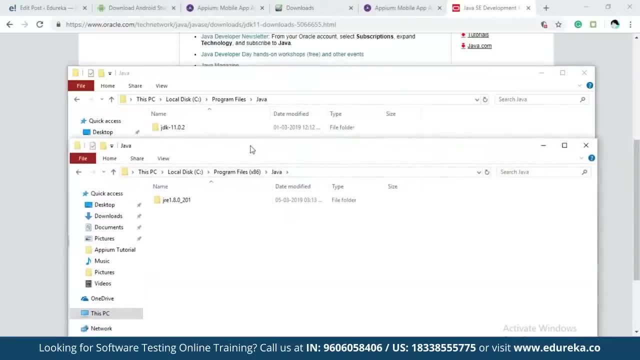 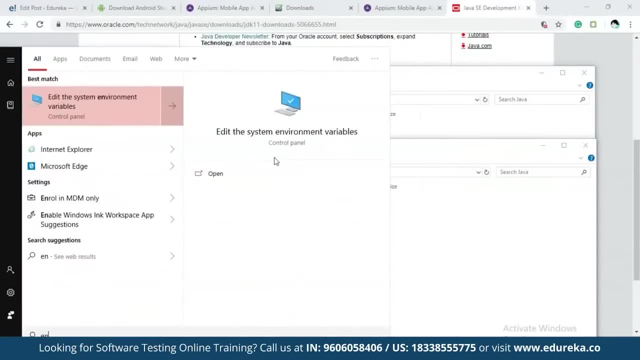 You should have these two files that are going for you. Now all you have to do is copy the path of these files and set that environment variables. Now all you have to do is go into your search menu and type for environment variables. 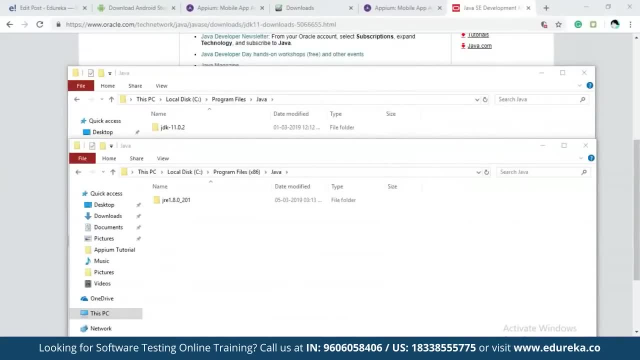 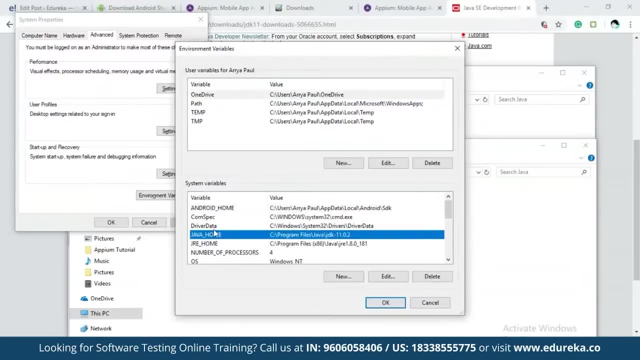 It might ask you for your password. It looks like this, So let me just enter my password. Okay, so out here you have to click on environment variables. So, as you guys can see, I have set my path out here for Java home and Jari home. 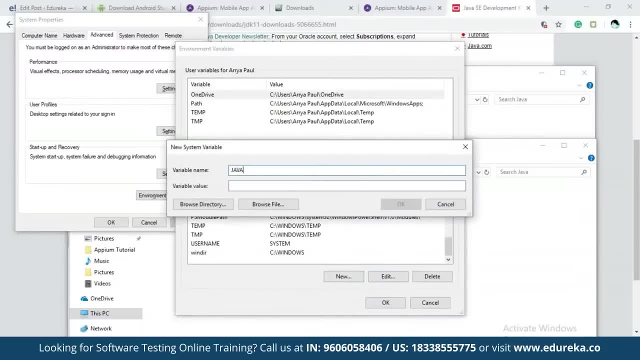 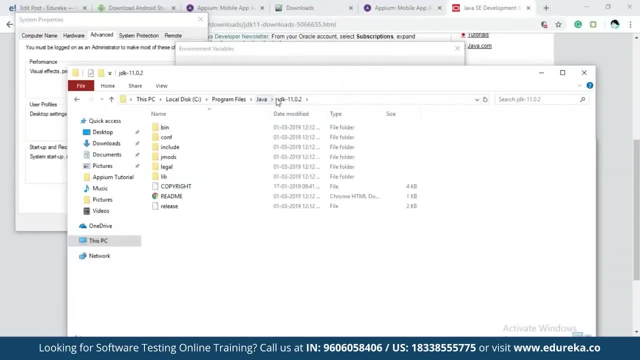 So to do that out here, all you have to do is go in and type Java underscore home and you give the variable value as the JDK file. So you're going to JDK, you copy down this entire path and you just paste it out here. 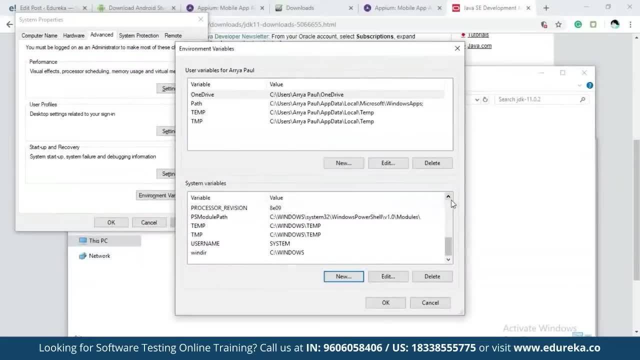 Now I'm not going to really add this, because I already have that added. You have to do the same thing for Jari. So once you have that going on, you should have something like this: Java home and Jari home. Once you have that set up. 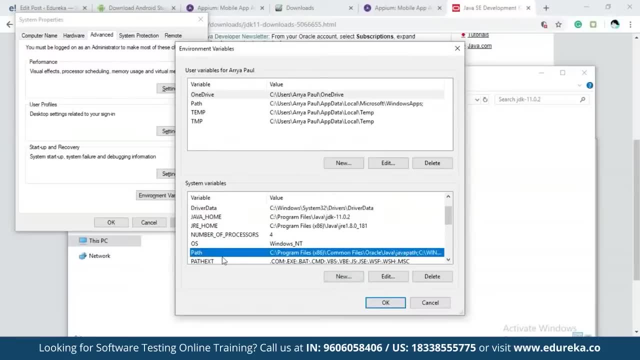 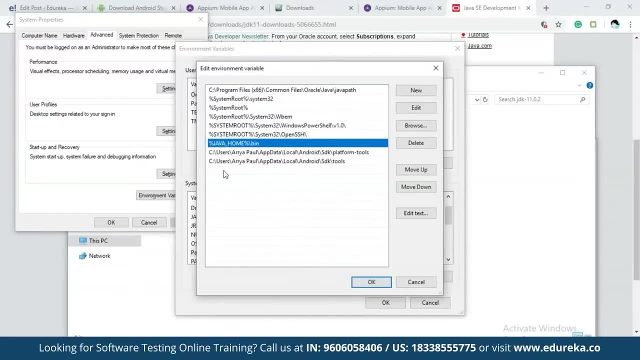 all you have to go and do is, under system variables, find this thing called path, going to edit, and you should see something like this audio. So all you have to do is type in a percentage sign, Java underscore, home percentage sign and the bin. So basically what you're doing out here. 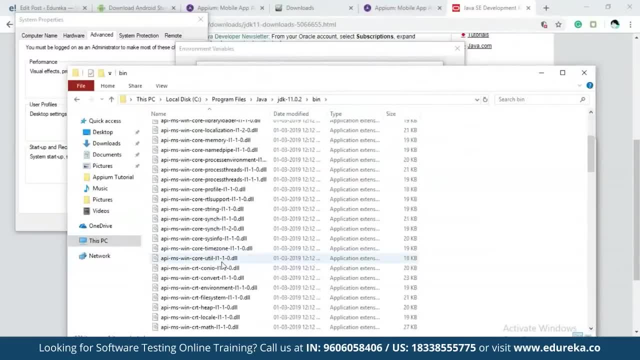 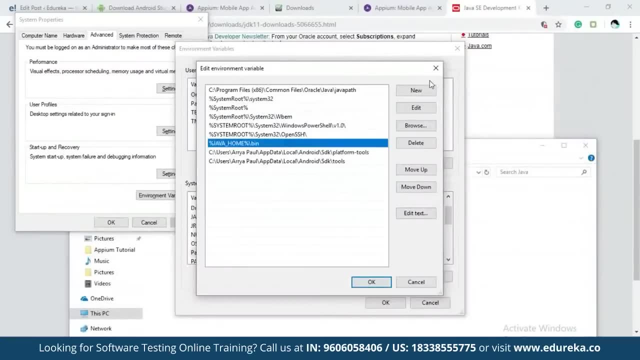 is giving your computer access to the bin folder which has all the DLL files which is necessary to run Java on your machine. Okay, so that takes care of Java for now. So, once you have Java installed on your computer, as I just said, 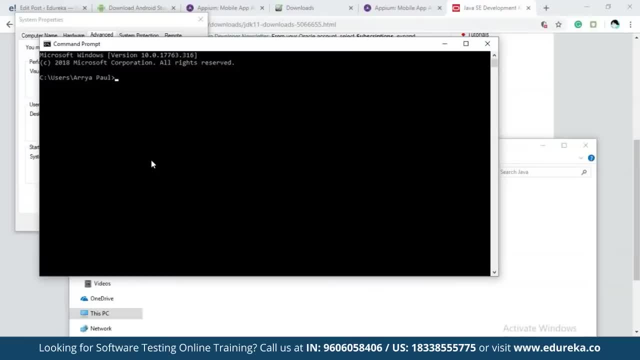 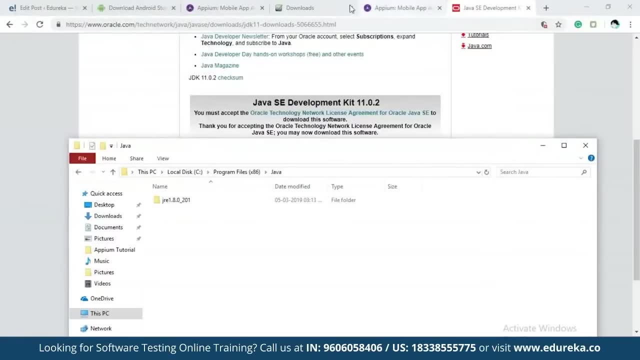 all you have to do is going to command prompt and just type in Java, and it should give you up this menu. So if that menu comes up, you're well and good. Now the next thing that we actually need to install is out here. 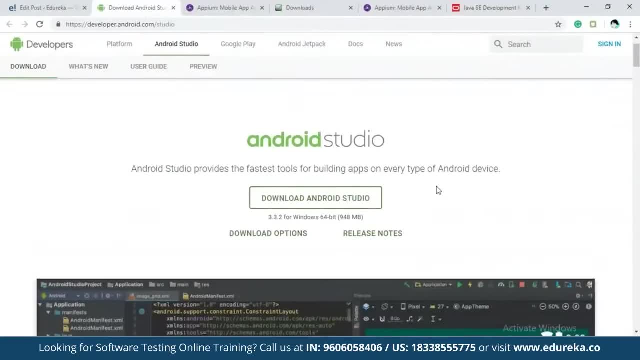 and that is Android studio. Now. all you need to do to install Android studio is go ahead and download Android studio Now. it's a pretty big file. It's 948 MB, That's around gig of data. So I'm not really going to download this. 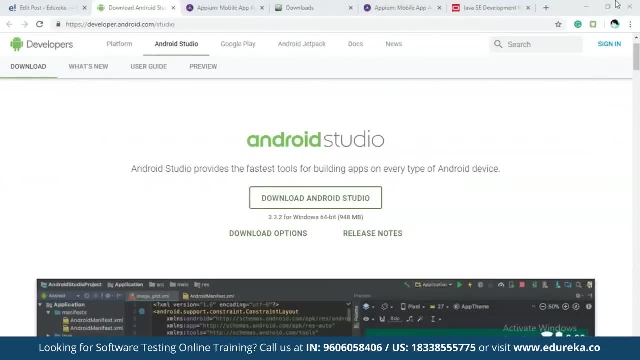 because I already have it downloaded. But once you download it it's basically a exe file and you have to just go ahead and read the onscreen menu and just install it. It's like installing any other tool or game that you write to on your computer. 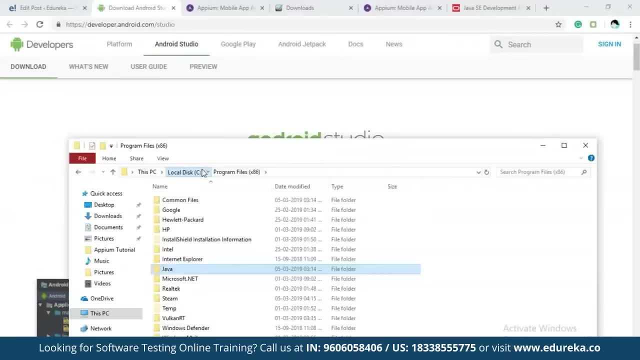 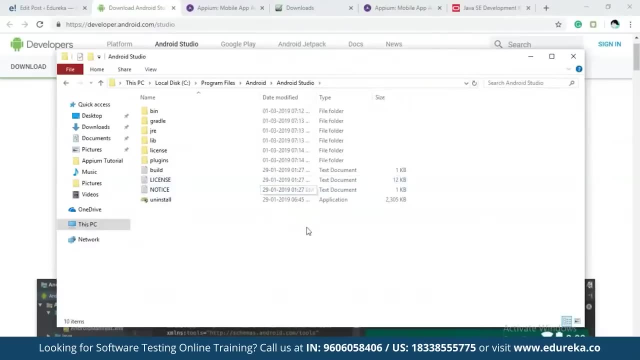 Now, once that is installed, you should have something like this on your computer. So, going to program files, and you should find Android and Android studio. now for Android studio Also, we need to set up the environment variables. So to do that again. 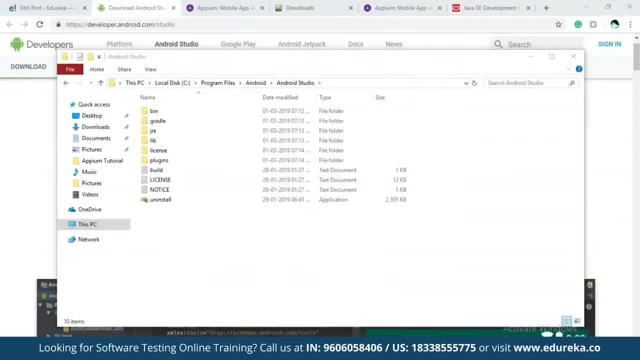 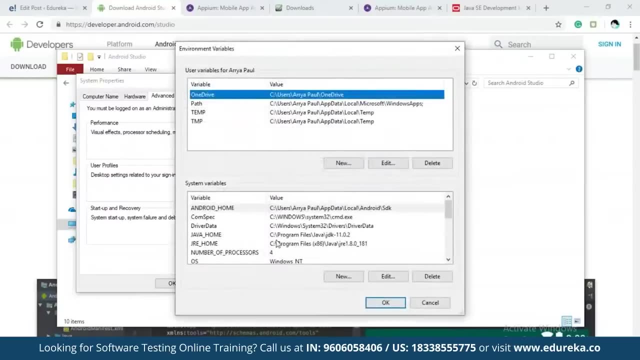 we have to go in and get the environment variables part up, So let me just get in my password in. Okay, so that does it. Now you're going to environment variables and what we have to do is put in this thing called Android home. 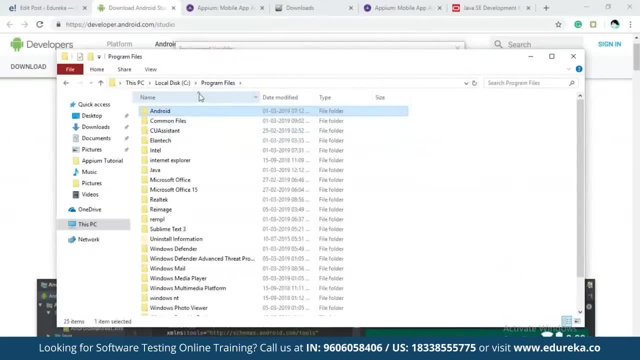 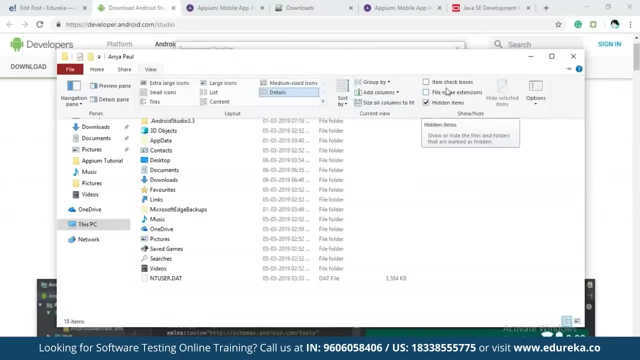 Now Android home is set in your local to see it going to users, going to your user that you're using. That's our Apple, and out here You see app data. Now, if you can't see app data going to view and all you have to do is take this hidden items checkbox out here, 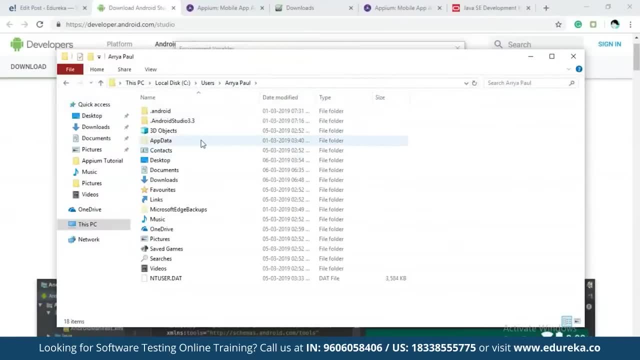 and it will show you all the hidden files and folders. So you're going to app data, going local, go to Android, go to SDK and all you have to do is copy down this path. going to environment variables, say new, give it a name. Okay, 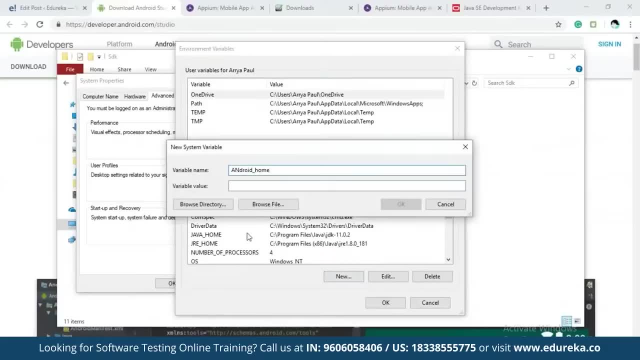 Give it name of Android home. as you guys can see, It doesn't really matter what you name it, to be honest, and then just given the value, and that is, let me just go back again, copy this and all you have to do is paste that so, as you guys can see, it's. 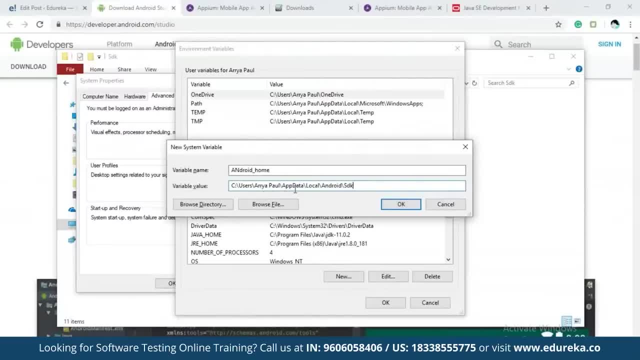 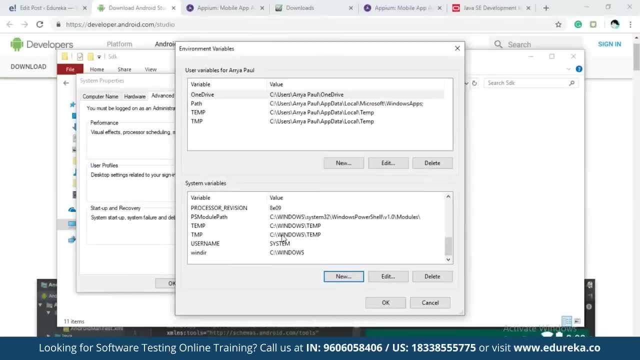 under see users and the particular user that you're using: app data, local Android and then SDK. not going to set it, because I already have that set out here and after that all you have to do is going to path again. So let's go down to the path. 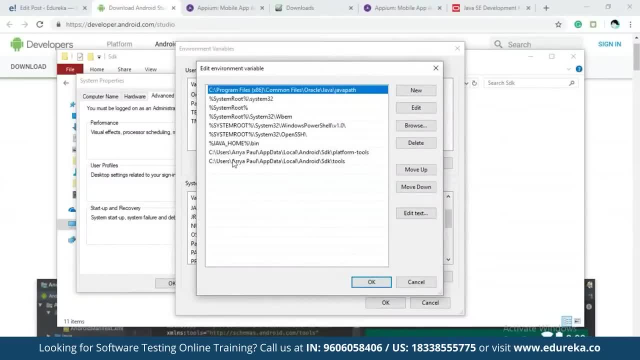 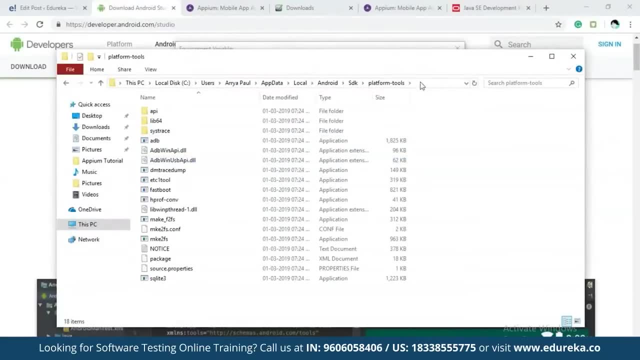 and you have to edit the path and, as you guys can see, I've added two new things. So one is the platform tools address and one is the tools address, so you can find them out here. So go to platform tools and copy down this address. 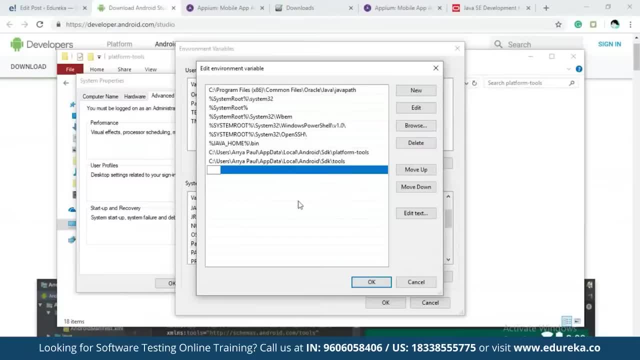 and going to path, say new and just paste it out here. Now I'm not going to do anything because I already have that pasted. So you have to do this for platform tools and tools port Now. once that is up and running, you also have to install the ADB drivers. 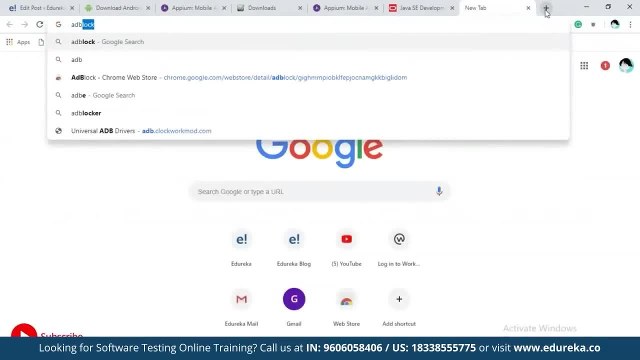 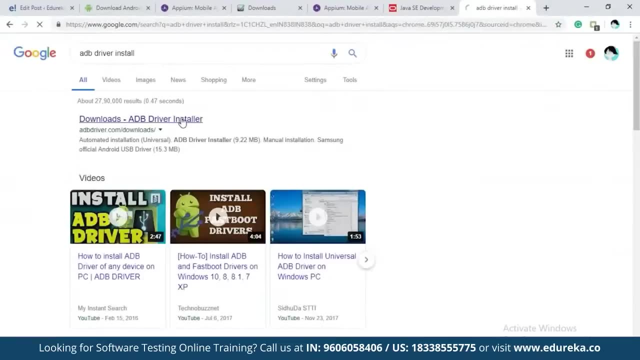 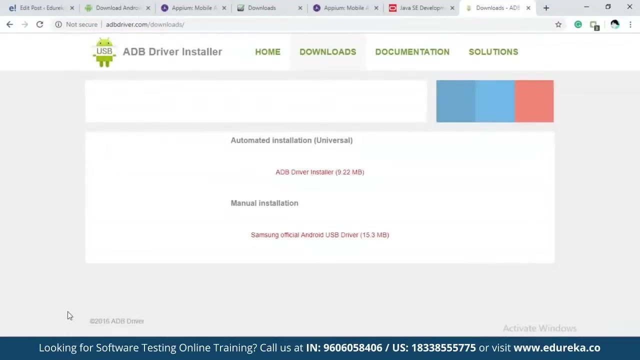 So for ADB drivers, All you have to do is go ahead and type in ADB driver install. So ADB driver install. the first link that you see out here should be the one that you have to install. Now. you click on ADB driver Universal and that should get it downloading. 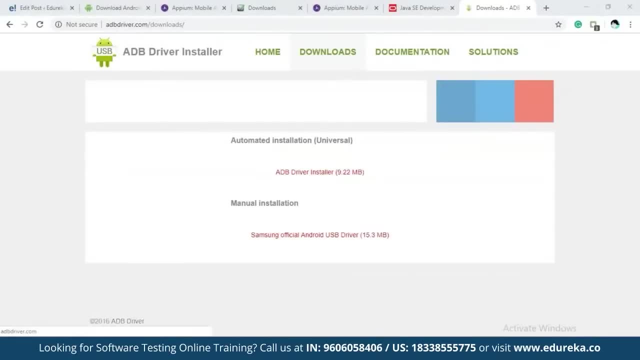 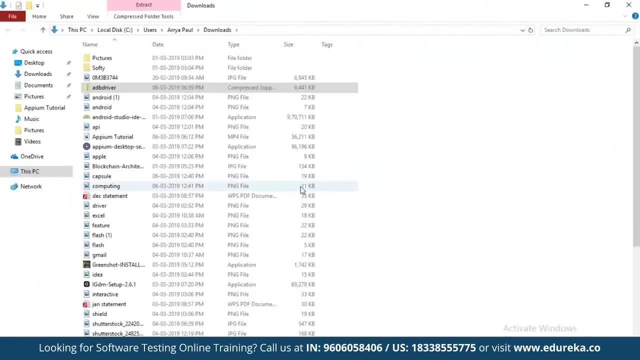 Okay, So once that has been downloaded, going to show in folder and, as you guys can see, we have this thing called ADB driver out here. Let me do that, Let me paste that, Let me put this in a view that can make sense. 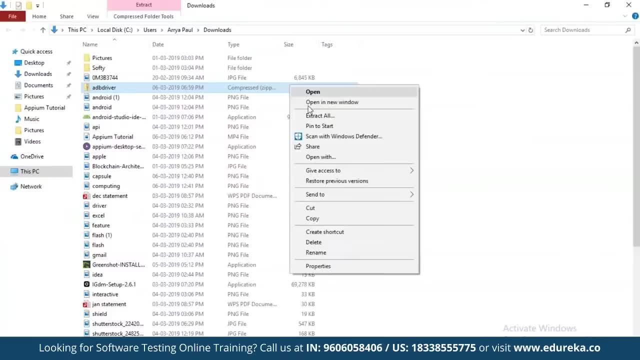 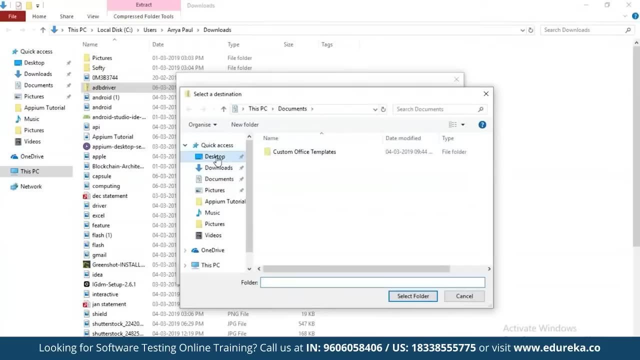 So ADB driver. So it's a compressed file. now, since it's a compressed file, All you have to do is extract all. now you can extract it to somewhere. So I'm going to go ahead and extract it to my desktop. So let's go ahead and extract that. 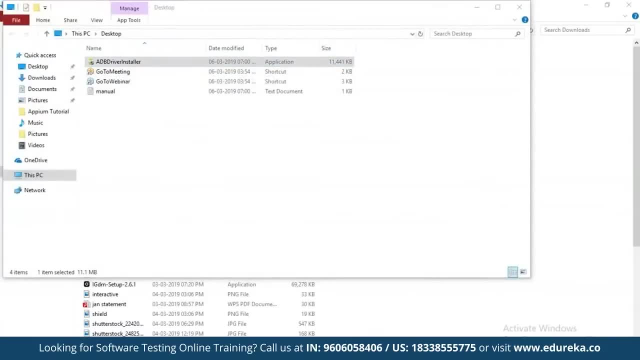 Okay, So now we have ADB driver installer out here. All you have to do is just click on the installer and let us do its job. So I'm just going to put in my password again So it installs it. Okay, So, as you guys can see, ADB driver installer. 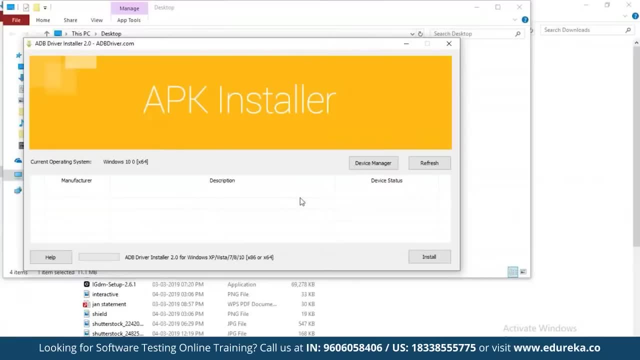 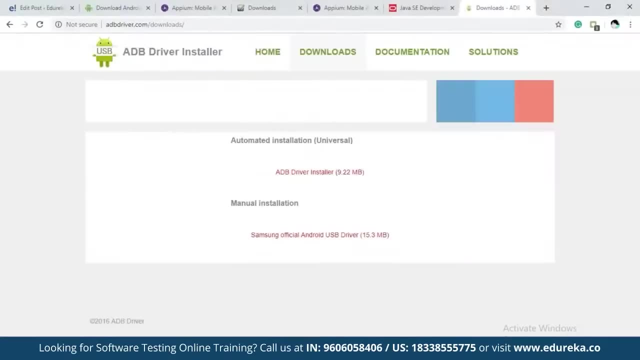 and if you have a device that is connected, it should actually go ahead and install the ADB driver for that. So that was all about ADB. Now the next thing that you need to download is a few more things. So firstly, we need to download Appium itself. 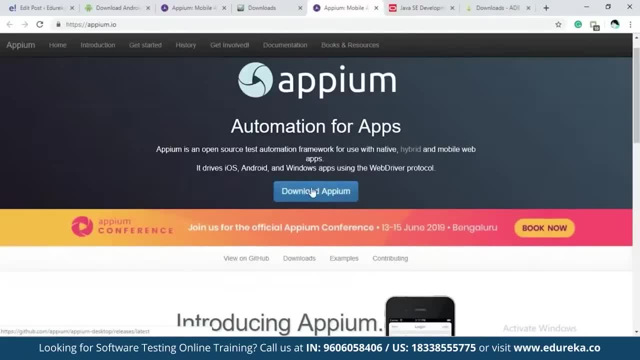 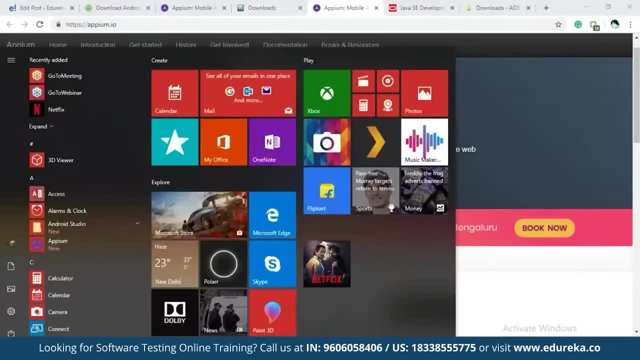 So that's pretty simple. All you have to go ahead and download is download Appium. So that can be found at Appiumio. So go ahead and download that, and till then, let's open up our Android studio. Okay, So once Android studio has been actually opened up, 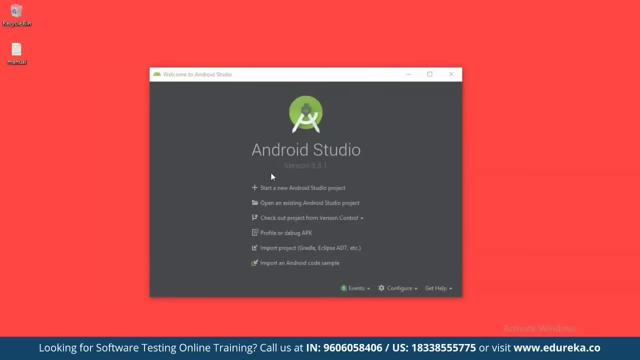 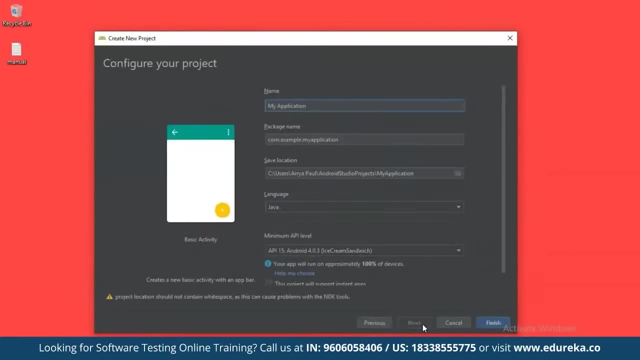 and you should get the screen on out here. So all you have to do is say start a new Android project and you should get the screen. You can choose a basic activity for now, because we are not really going to do any sort of development. 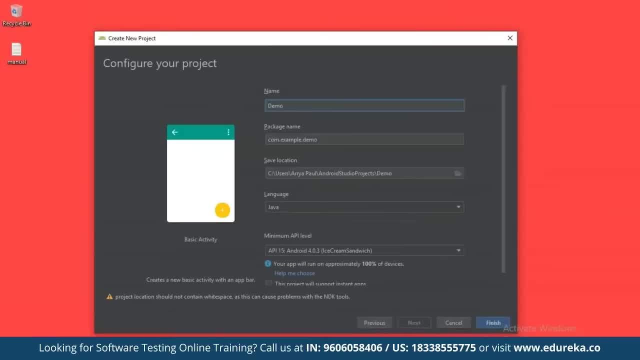 We are only interested in testing. So I'm going to name my project demo and all you have to do is say finish. You can also choose a minimum API level. I'm going to choose it to be API, So let's see, put it at API 24,. 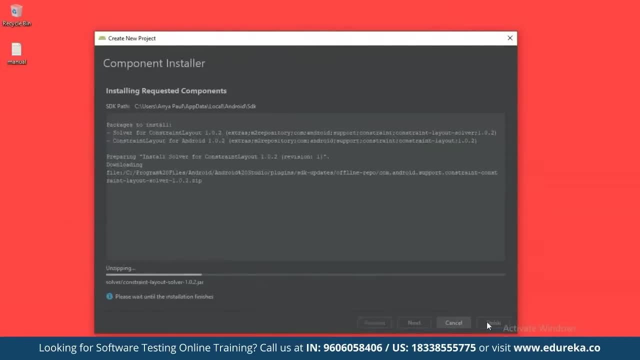 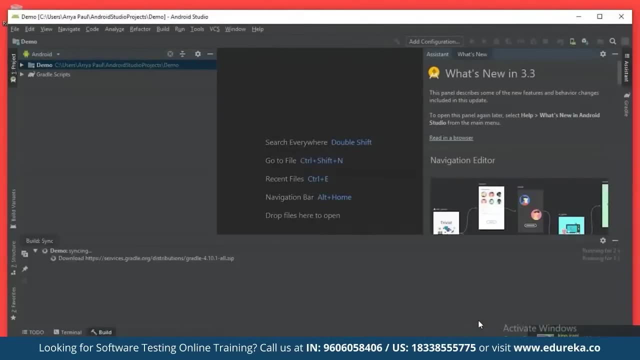 which is Android 7 Nougat. So let's finish that, Okay. So our project is now loading up. So what we have to do is get our Android studio to get integrated with our Appium server. So what do you guys can see out here in this demo part? 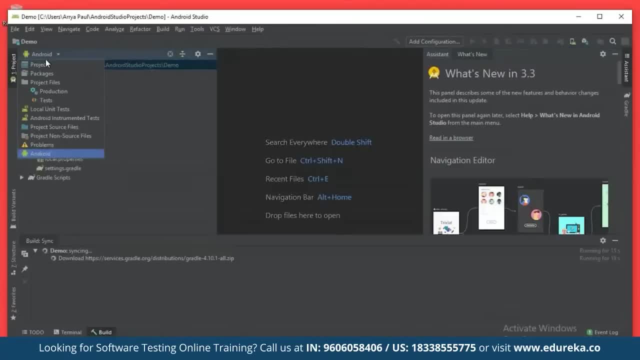 is the project structure. Now you can go out here and go into project and going to demo and all you see is app file out here. Okay, So now we are really interested in the app file and the lips folder. Now for the lips folder. 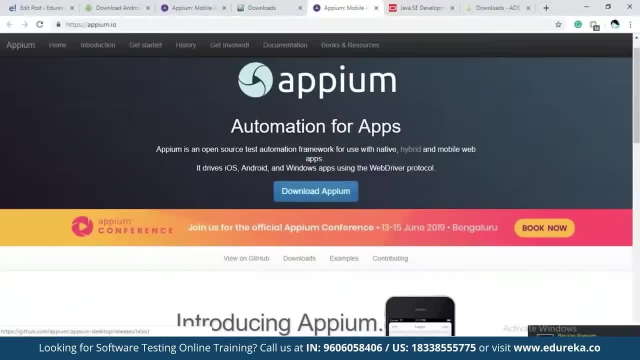 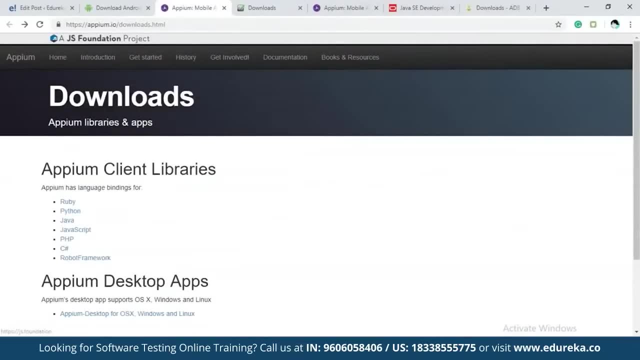 we need to put some stuff in. So let's go back to our page. and now we need to download a few stuff. So out here you can see that I have the Appiumio slash downloadshtml page open. So Appium has a bunch of client libraries. 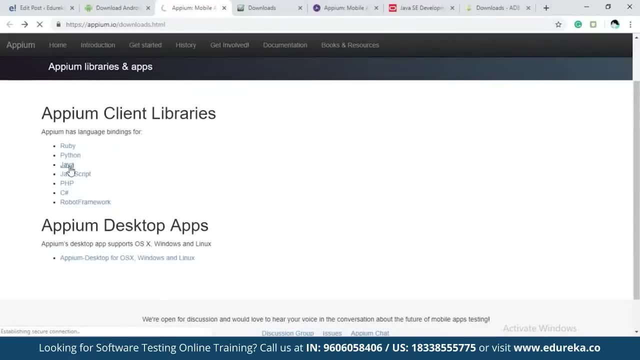 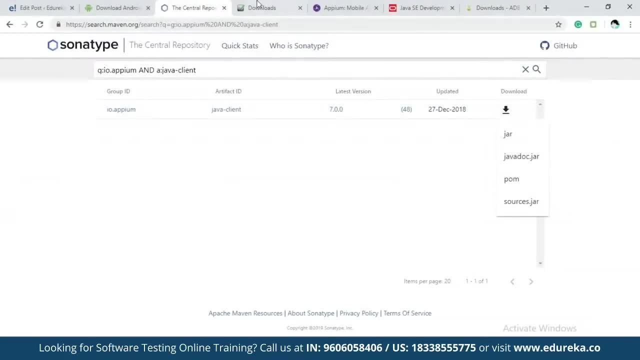 So for now, we are going to be installing the Java library, So let's go ahead and download that. So all you have to do is click on that link and then click download, And you also have to download the Selenium web drivers. So we are going to be using Java. 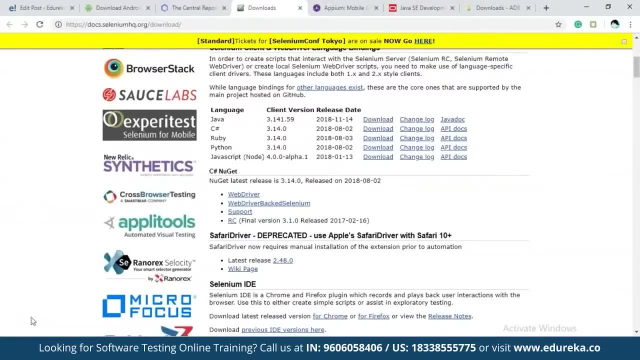 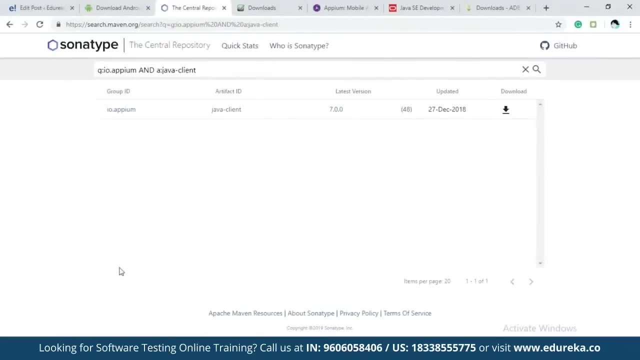 So let's go ahead and download that too. So Selenium Java is downloading while, so we need to download the jar files, So that will also get downloaded. So let's keep this file. So we have two files right now with us. We have the Java client 7.00 jar. 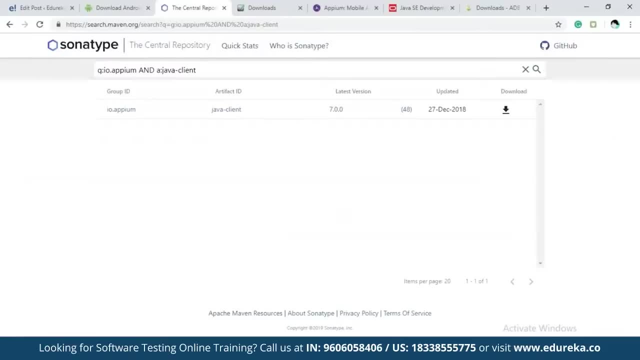 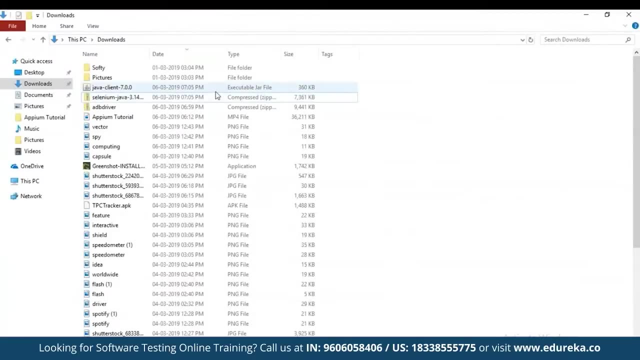 and the Selenium Java 3.0.. Okay, So let's go ahead and find these in our folder. Okay, So once you have both the files downloaded, move that to a separate folder. for now I'm going to cut them. I'm going to go ahead to my desktop. 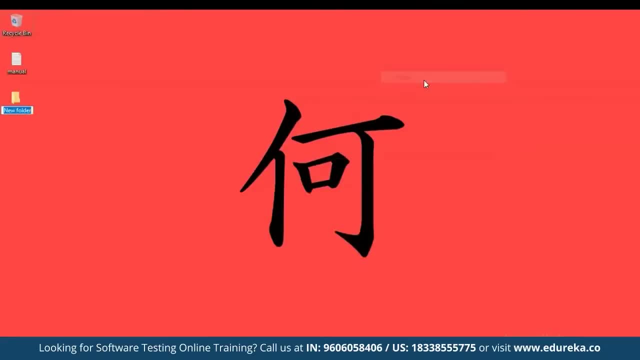 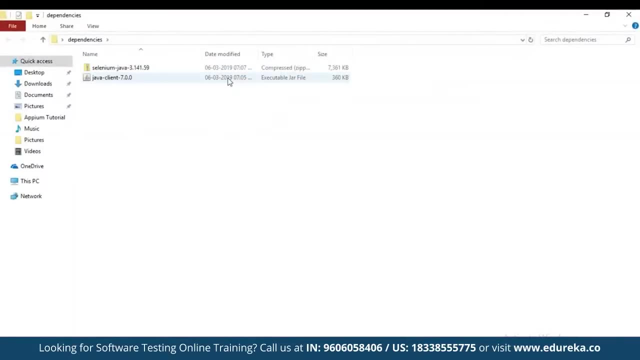 and let's make a new folder called dependencies, and you can name it for whatever you want. I'm going to paste these out here so that I can find them in a convenient manner. Now What I want to do is extract all of these out. 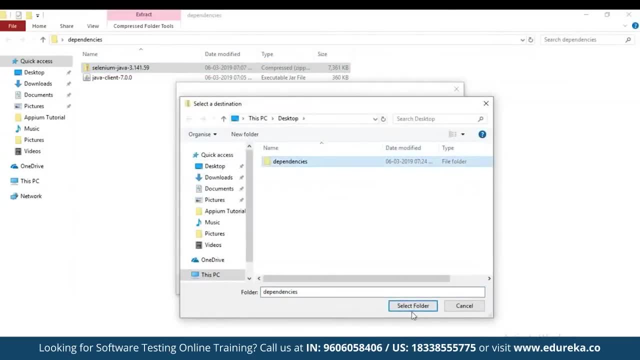 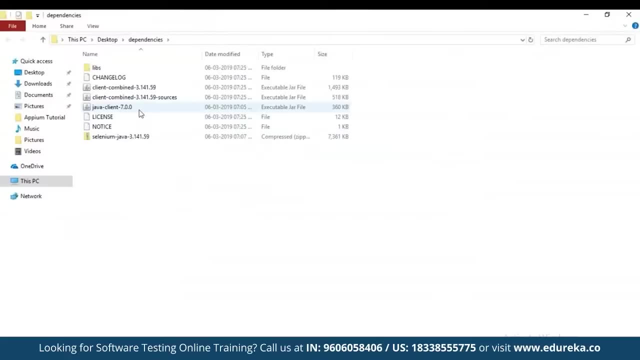 Okay, let's go and browse, and we want to do it. independency, So select folder and we want to do extract. So, once that has been extracted, what we are interested in is the Java client and these files. Okay, So, if you go back to Android studio, out here. 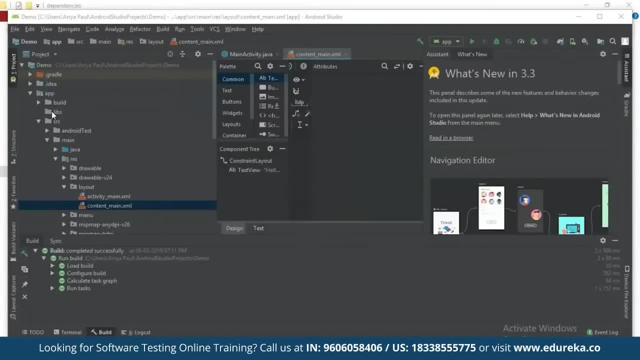 and you open the project structure, you can see your libraries folder. Now what we want to do is put in all these files into the lib folder. So if you go ahead out here and see our project is stored in under users and under our Paul under Android studio project. 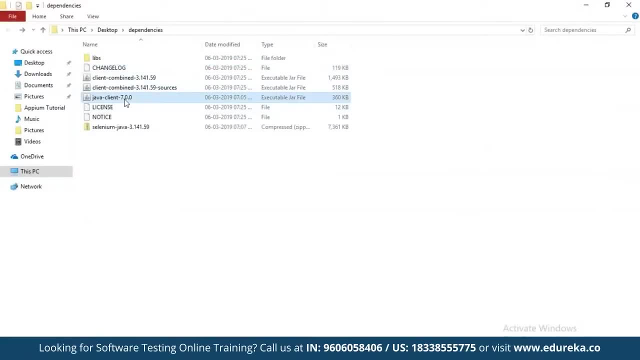 and under demo. So first of all, copy this file, the Java client. So let's copy that, Let's go to this PC, Let's go to local to see, let's go to users or a Paul, and we want to go into Android studio projects. 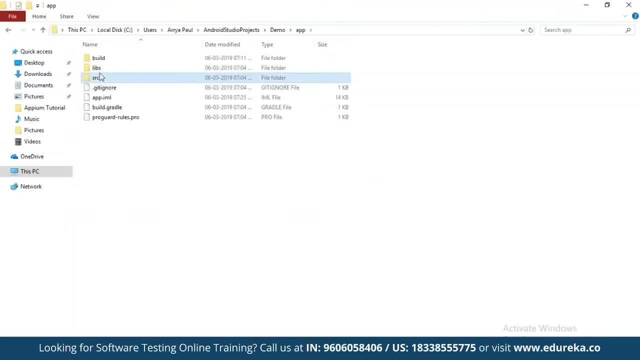 We want to go into demo. We're going to go to app libraries and just start pasting your stuff There, go back into dependencies and what we want to do is go into libs folder And copy all this and go to the lips folder of our Android project. 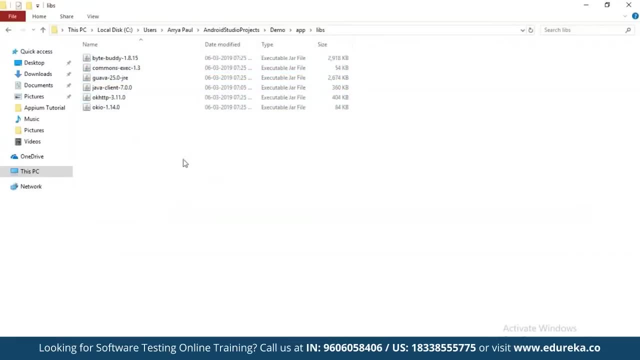 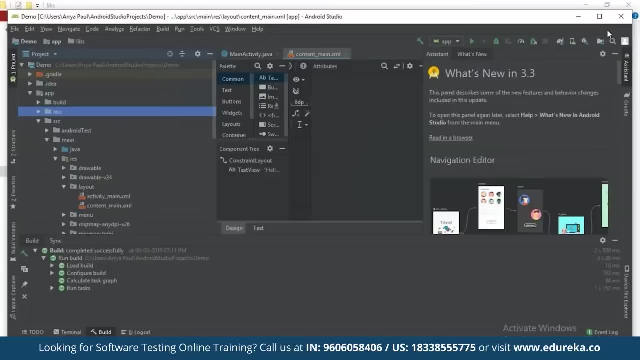 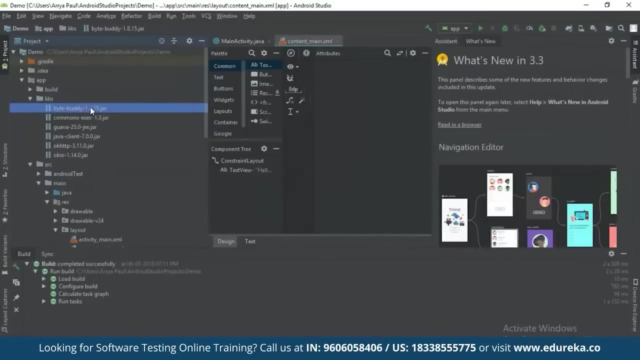 and just paste it there. So once that is done, what we want to do is go back out here and check if these things have been actually put in our lib folder. So if you see we have an arrow now and you see we have all these things out here, 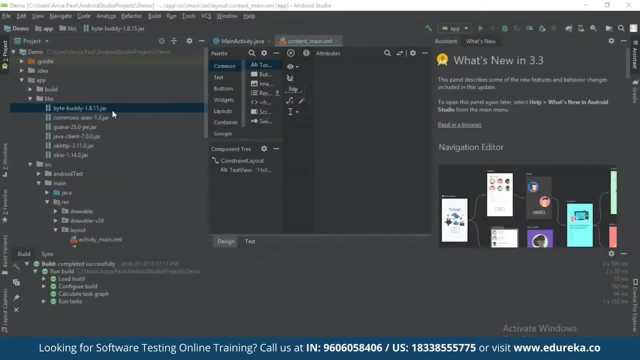 Okay. So now what we need to do is tell Android studio that all these jar files will be used in our library. So let's go ahead and select all these and right-click on them, and all you have to do is add as library. So this will be added as library to the app module. 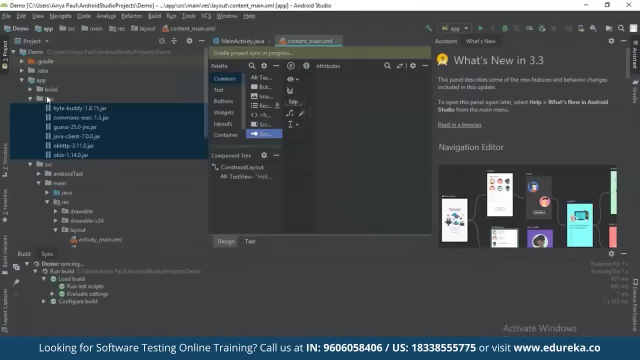 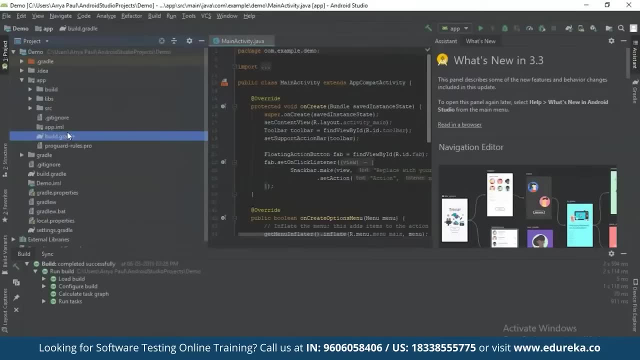 Okay, So our app module has a library now, fine, Okay. So after you've added those files as a library, should get a build out gravel file under your app folder. So let's go ahead and open that. Okay. So, once that is done, 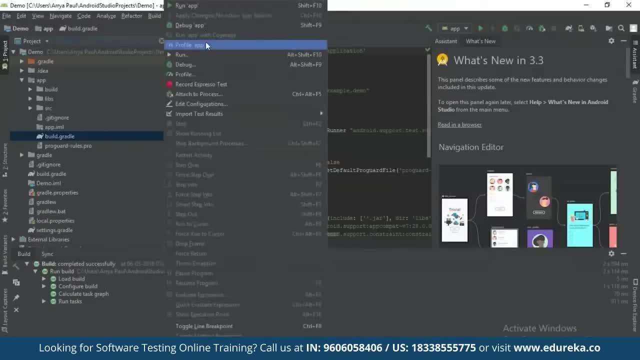 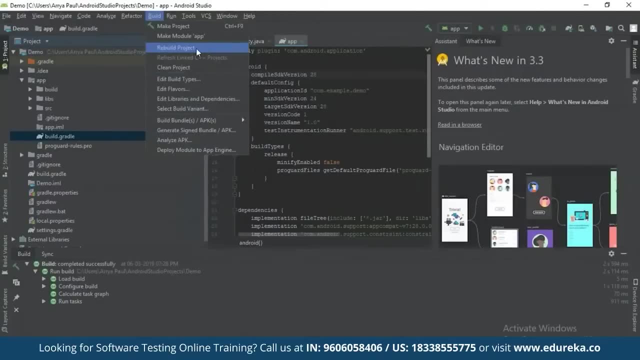 all you have to do is go in here and going to run and all you have to say is rebuild project. I don't think it's in run. Okay, It's in build. So all you have to do is open your build file and you have to rebuild your project. 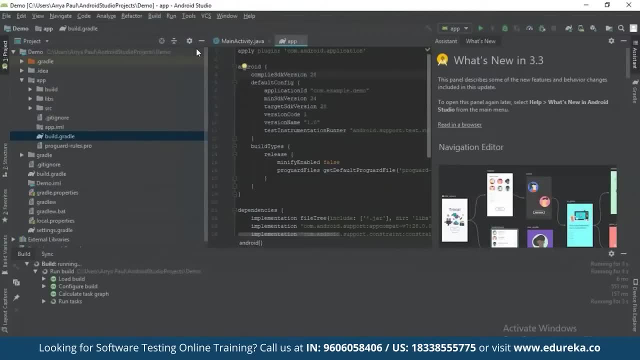 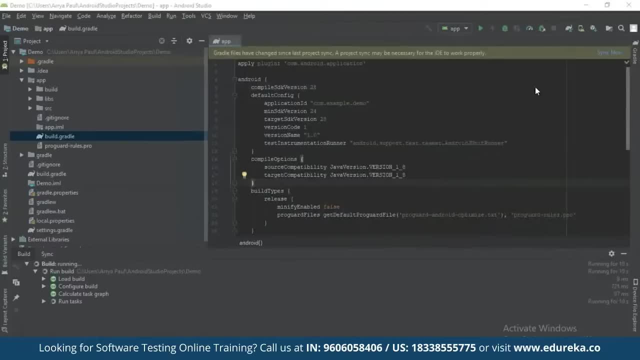 So sometimes it will sync automatically and when this build is done, it means that you have successfully integrated Appium into your Android studio. Okay, guys, So, as you guys can see, our build has successfully completed and since our build has successfully completed, This means that Appium has been successfully integrated. 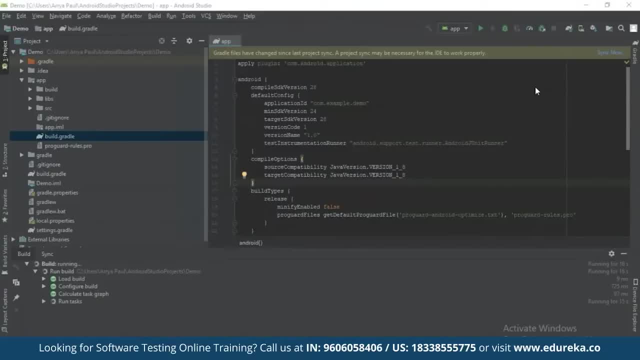 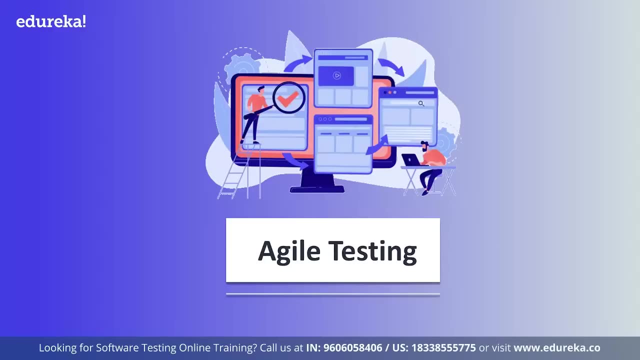 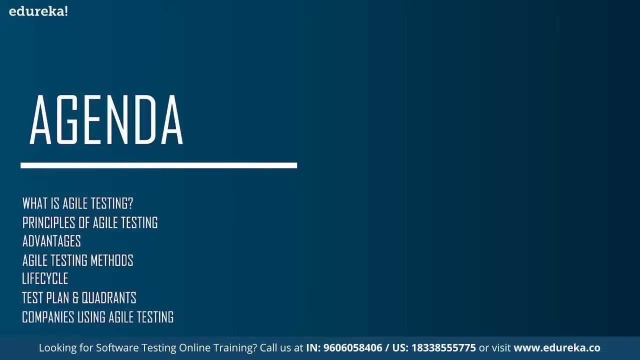 with our Android studio and now we can proceed and write our test cases. So first we will see what is agile testing, and then we will move on to the different principles and then have a look at the different advantages of agile testing. after that We will see what are the different methods involved. 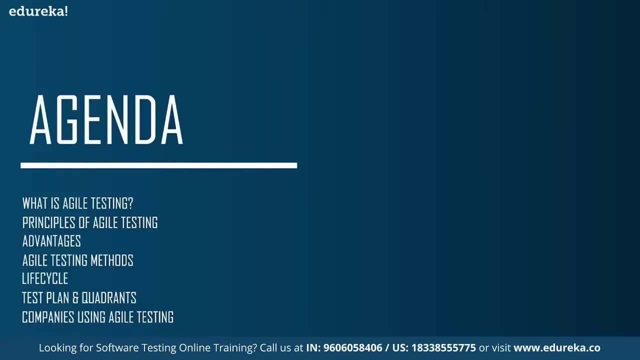 in this testing and also the life cycle. next up, We will have a look at the different test plan and quadrants of agile testing and finally, we will discuss about the big companies using agile testing in today's world. So let's get started. 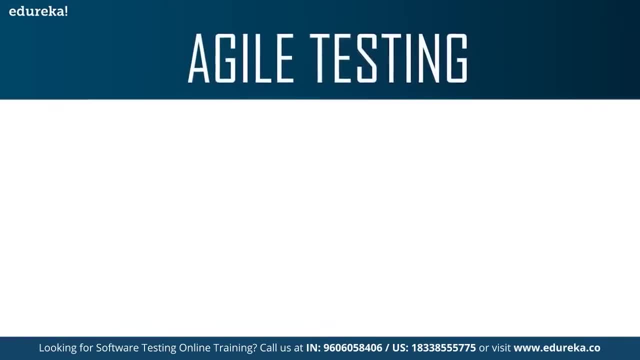 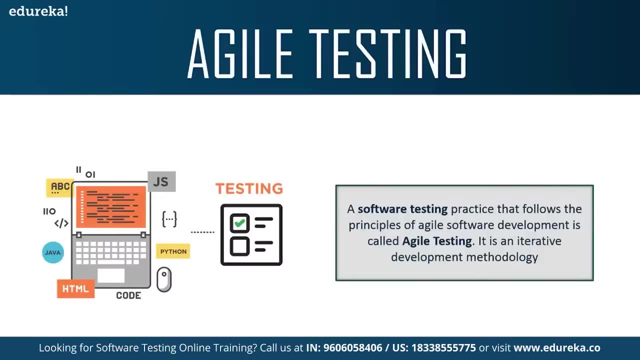 So what is this agile testing? Now, agile testing is basically a software testing process that follows the principles of agile software development. Now, agile is basically an iterative development methodology where requirements evolves through collaboration between the customer and self-organizing teams, and agile aligns development with the customer development. 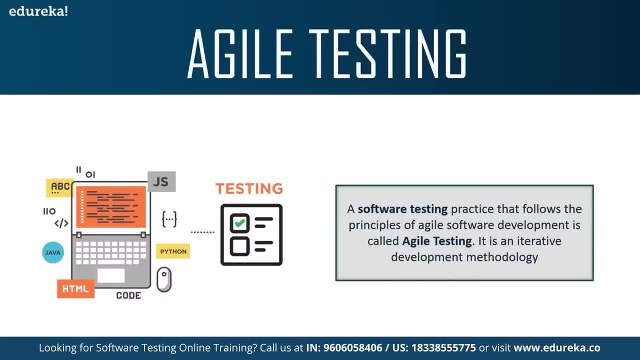 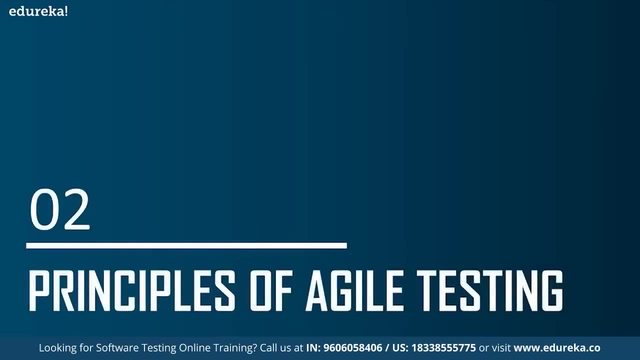 It is not sequential but a continuous process. Now this methodology is also called release or delivery driven approach, since it gives a better prediction on the workable products in short duration of time. So let's move on and have a look at the different principles of agile testing. 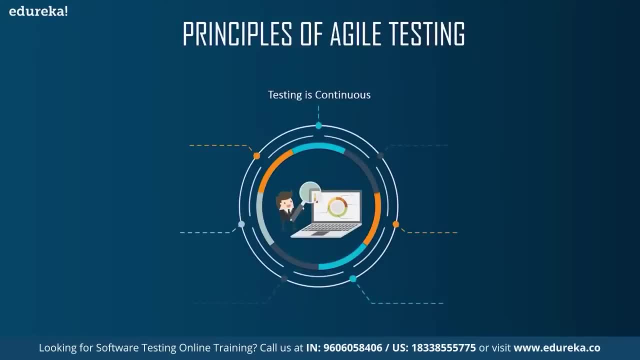 Now. the first one is that testing is continuous. Now the agile team tests continuously because it is the only way to ensure continuous progress of the product. Then we have the continuous feedback as well. So agile testing provides feedback on an ongoing basis and this is how your product meets the business needs. 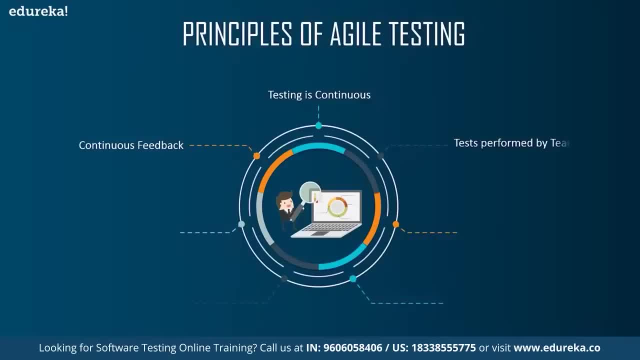 and also satisfies the customer requirements. Then we have the tests performed by the whole team. Now, in a traditional software development lifecycle, only the test team is responsible for testing, but in agile testing, the developers and the business analysts also test the application Next up. 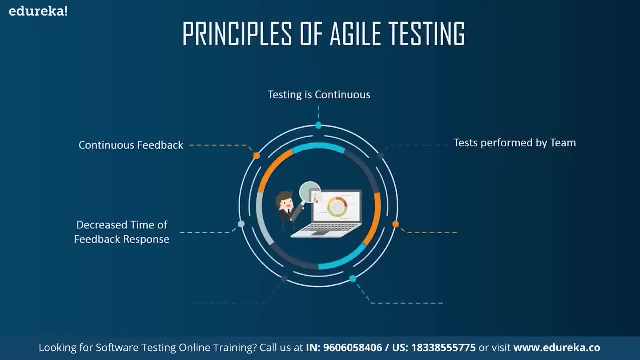 is the decreased time of feedback response. Now the business team is basically involved in each iteration, in agile testing, and continuous feedback shortens the time of feedback response. Then we have the simplified and clean code, So all the defects which are raised by the agile team. 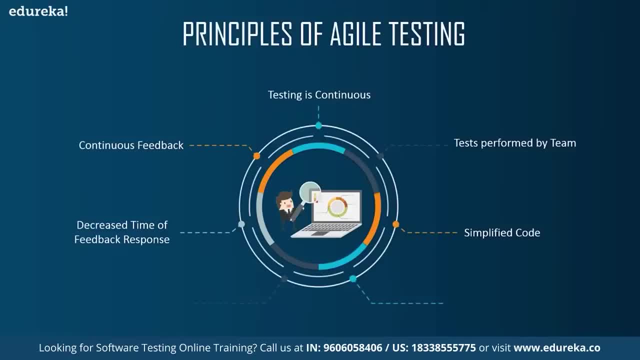 are fixed within the same iteration, and it also helps in keeping the code clean and simplified. Next is less documentation. Now, agile teams use a reusable checklist, The team focuses on the test instead of the incidental details And finally we have the test driven. 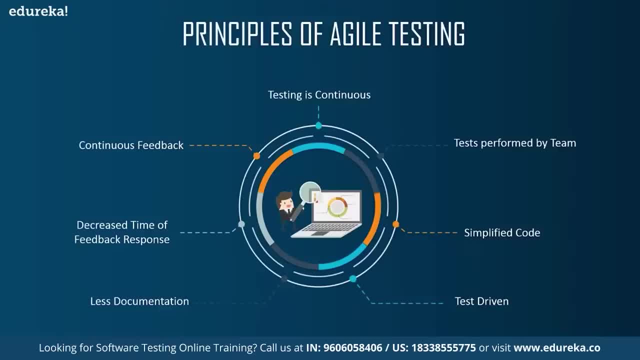 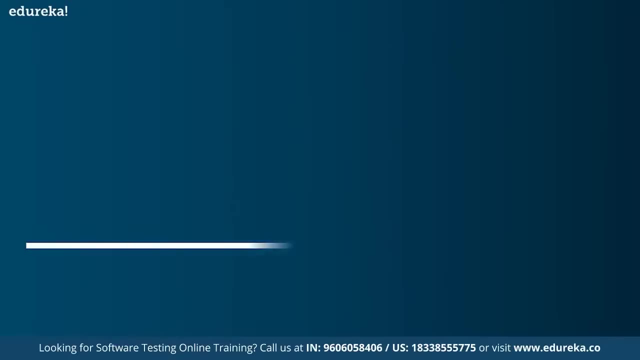 Now, in agile methods, testing is performed at the time of implementation, whereas in the traditional process, the testing is performed after implementation. So these were some of the principles that are followed while performing agile testing on any software. Now let's move on and have a look at the different advantages of agile testing. 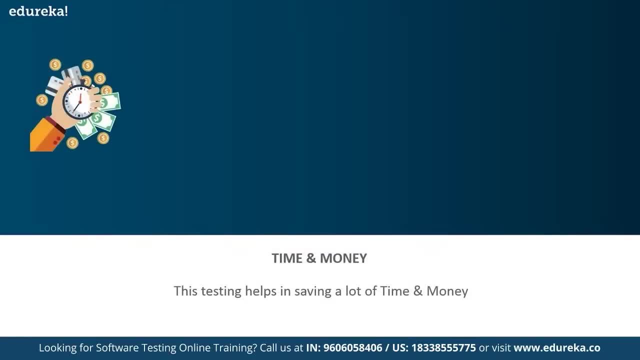 So the first benefit is that it saves time and money. Now, with the help of agile testing, you get to know about the problems in your software in the earlier stages, and this saves a lot of time and money as well. Next up is the documentation. 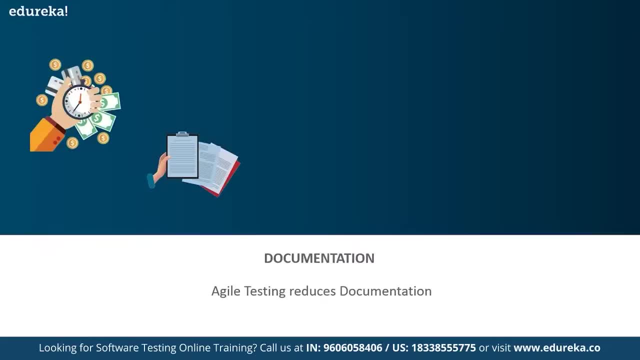 So agile testing basically reduces a lot of documentation involved in the process. Then we have the flexibility and adaptability. So agile testing is basically flexible and highly adaptable to changes. So you would not face any trouble if there are any changes that are to be made. 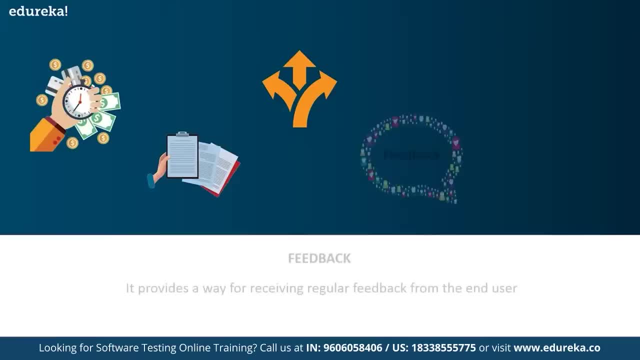 in the software during the process. It also provides a way for receiving regular feedback from the end user. So the more amount of feedback that you receive, the easier it becomes to solve the problems and also meet the requirements of the user easily. And finally, there's better determination of issues. 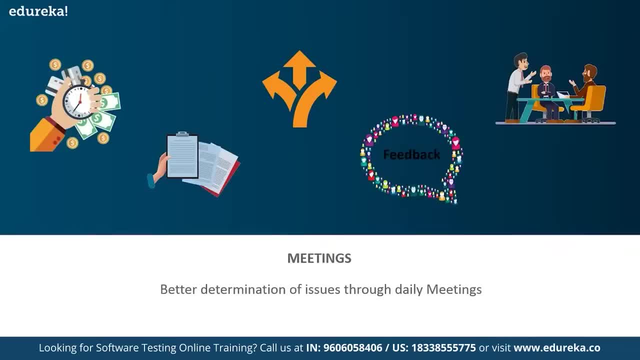 through daily meetings. So there are daily meetings happening for the agile testing. that lets you know about the whole process and also the improvement that is happening. So these were some of the advantages. Now let's have a look at the different testing methods for agile testing. 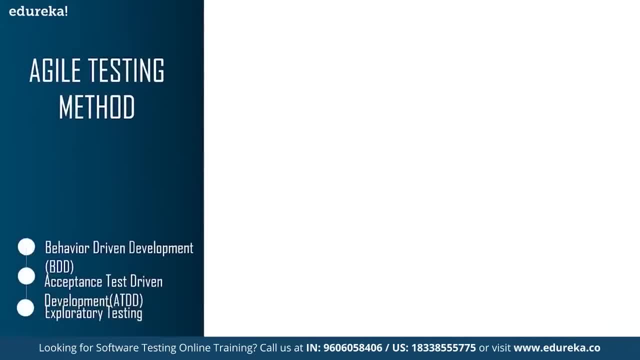 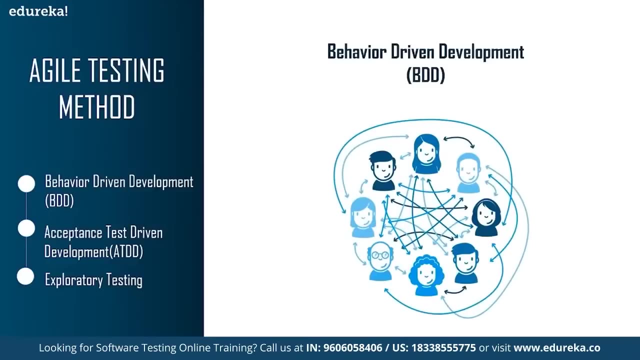 Now there are various agile testing methods. So first we have the behavior-driven development, then the acceptance test driven development and finally there's the exploratory testing. So the first one is the behavior-driven development. Now the behavior-driven development improves communication amongst project stakeholders. 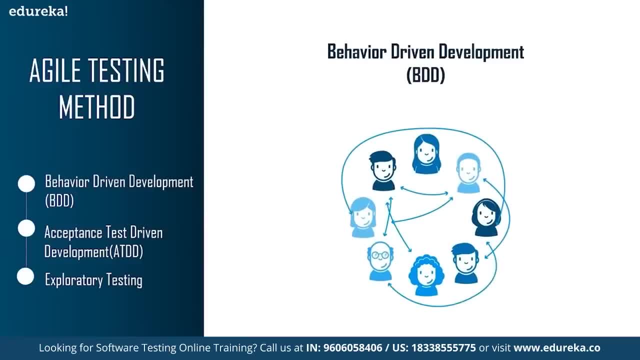 so that all members correctly understand each feature before the development process starts. Now there is continuous example based communication between the developers, testers and business analysts. Now these examples are called scenarios, which are written in a special format. The scenarios hold information on how a given feature should behave. 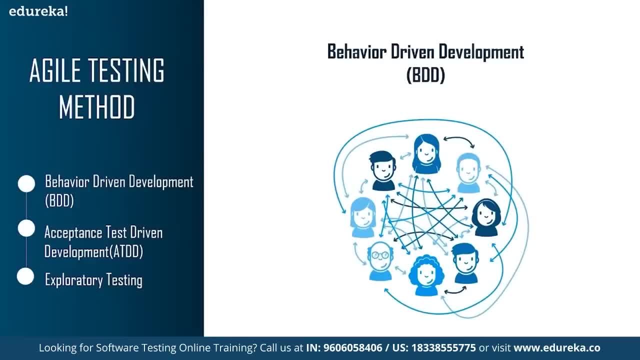 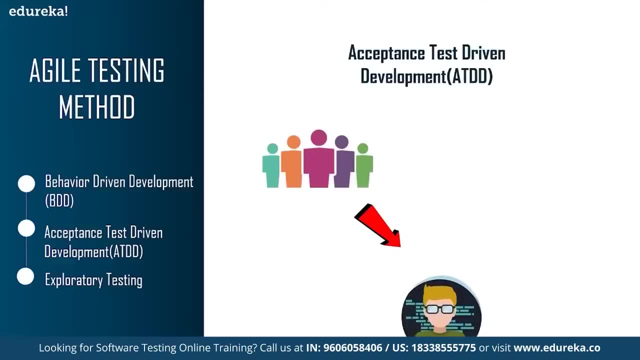 in different situations with different input parameters. These are called executable specifications, as it comprises of both specification and inputs to the automated tests. Next up, we have the acceptance test driven development that is the ATDD. Now the ATDD focuses on involving team members with different perspectives. 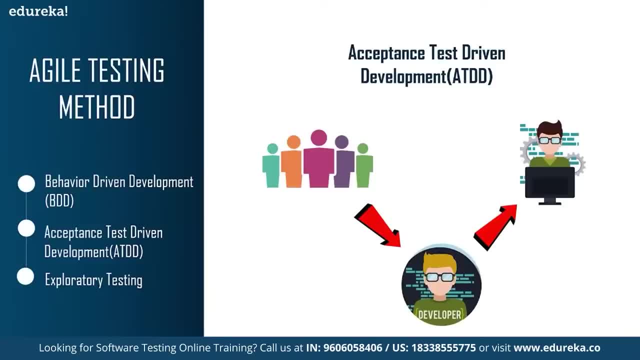 such as the customer, developer and tester. So the three amigos meetings are held to formulate acceptance tests incorporating perspectives of the customer, development and testing. So the customer is focused on the problem that is to be solved, The development is focused on how the problem will be solved. 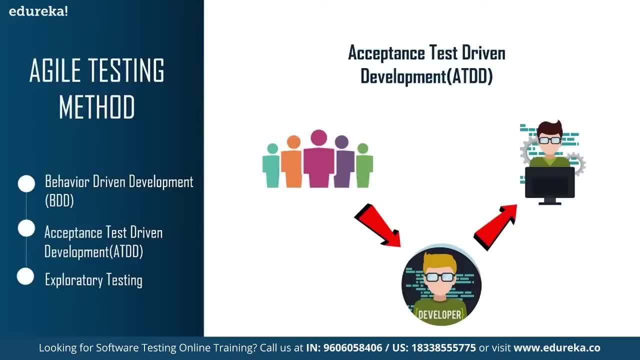 whereas the testing is focused on what could go wrong, The acceptance tests are a representation of the user's point of view and it describes how the system will function. It also helps to verify that the system functions as it is supposed to. In some instances, acceptance tests are automated. 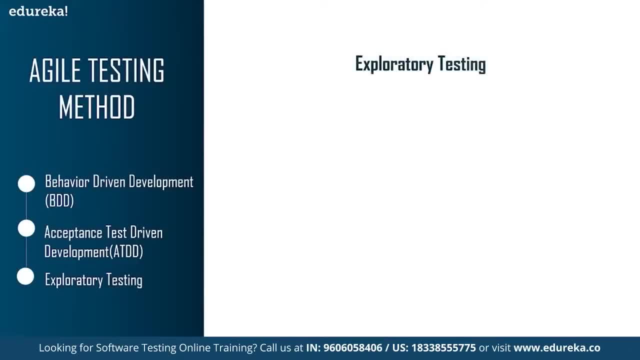 Now moving on. the final one is the exploratory testing. Now, in this type of testing, the test design and test execution phase go hand-in-hand. So the exploratory testing emphasizes working software over comprehensive documentation. The individuals and interactions are more important than the process and tools. 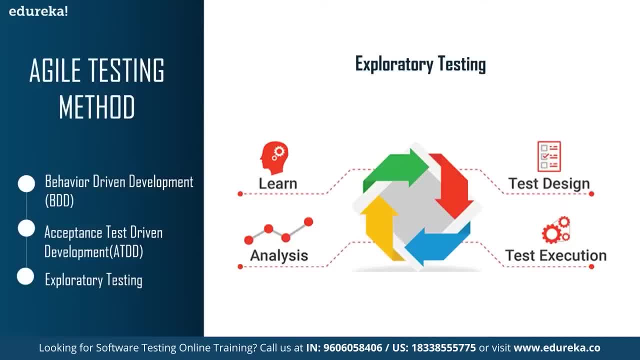 So the customer collaboration holds greater value than contract negotiation. Exploratory testing is more adaptable to changes as well. Now, in this, testers identify the functionality of an application by exploring the application. So the testers try to learn the application and design and execute the test plans. 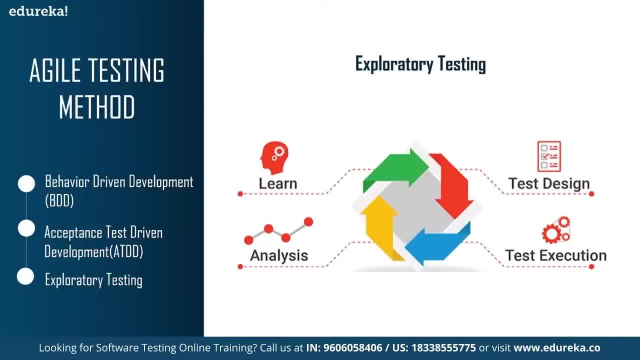 according to their findings. So the process goes like this: first you learn, then you design a test and then execute that particular test, and then, finally, you analyze the test results. So these were some of the agile testing methods that you need to know about Now, moving on next up. 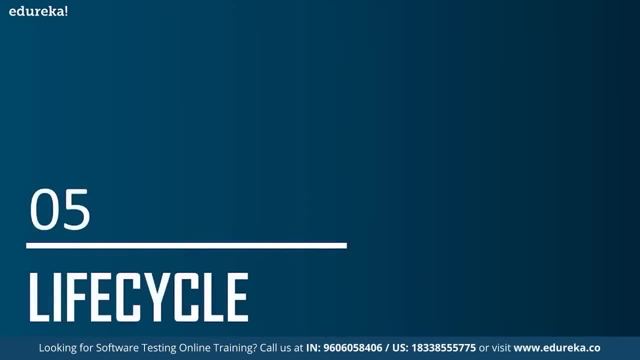 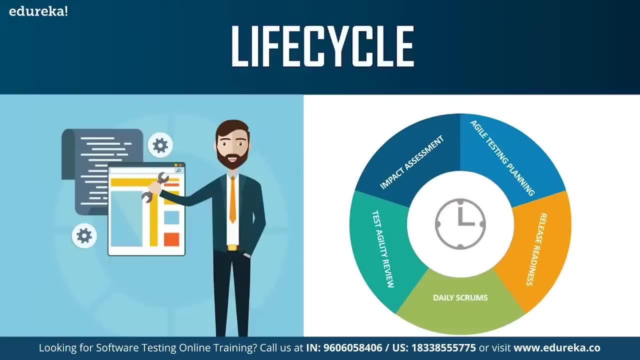 Let's have a look at the life cycle of agile testing. So the life cycle of agile testing consists of five different phases. So first we have the impact assessment, then agility test planning, then daily scrums, then agility review meeting and finally release the readiness. 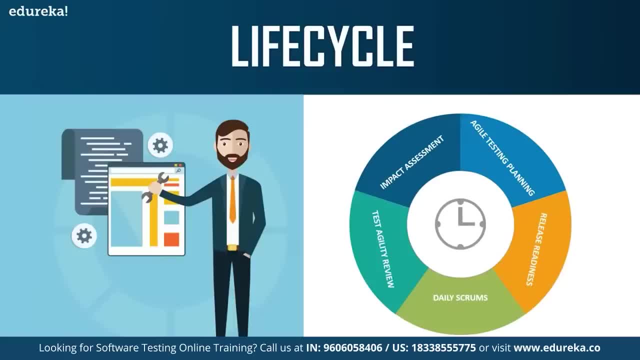 So in the first phase we gather the input from the stakeholders and users, and this will act as a feedback for the next deployment cycle. The next phase is the test plan meetup. Now, here all these stakeholders come together to plan the schedule of testing process: meeting frequency. 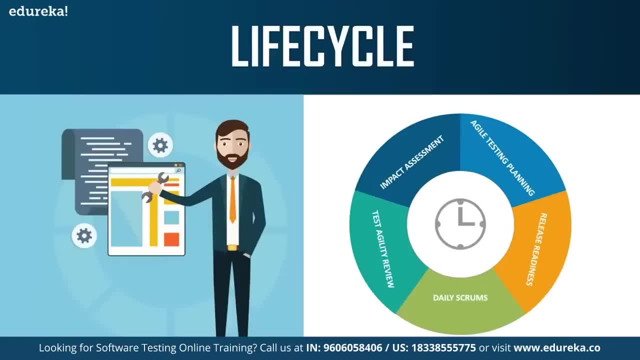 and deliverables. The third phase is the daily stand-up meetings. Now this includes the everyday stand-up morning meeting to catch up on the status of testing and set the goals for whole day. Next up is the agility review meeting, So weekly review meetings with stakeholders. 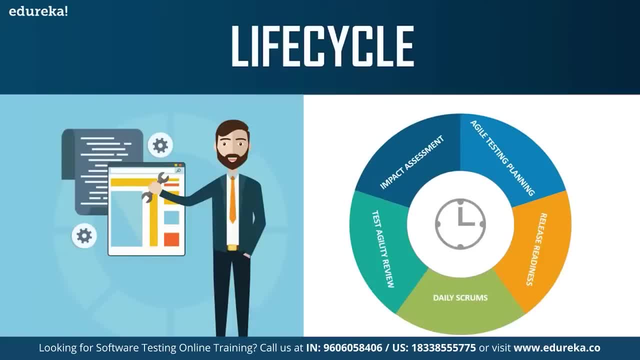 meet to review and assess the progress against milestones. and finally, the last stage is the approval meetings for deployment. So at this stage you review the features that have been developed or implemented and are ready to go live. So this is the life cycle that is followed. 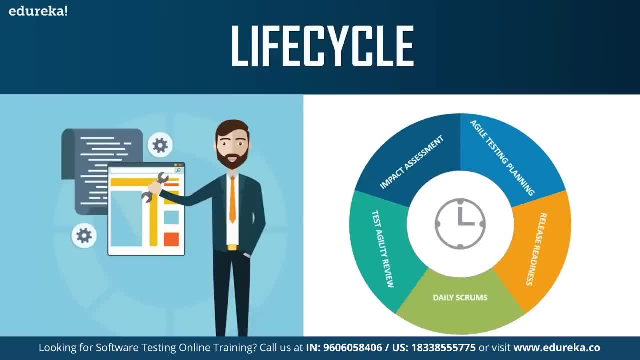 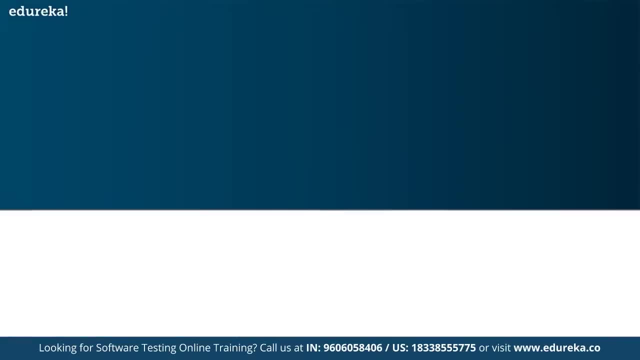 in the process of agile testing in case of any particular software. So now that you know what is agile testing and also the different advantages and how it actually works, Let's have a look at the test plan for agile testing and also the quadrants. 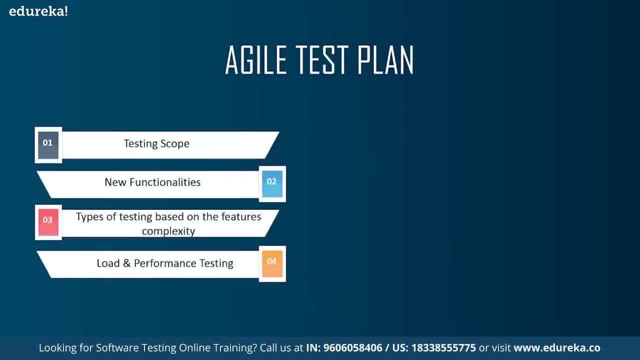 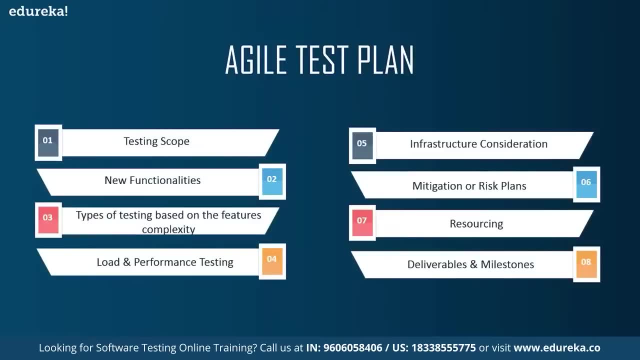 So first let's talk about the agile test plan. Now, in agile testing, the test plan is written as well as updated for every release. So the test plan in agile includes the scope of the testing, then the consolidating new functionalities that are to be tested. 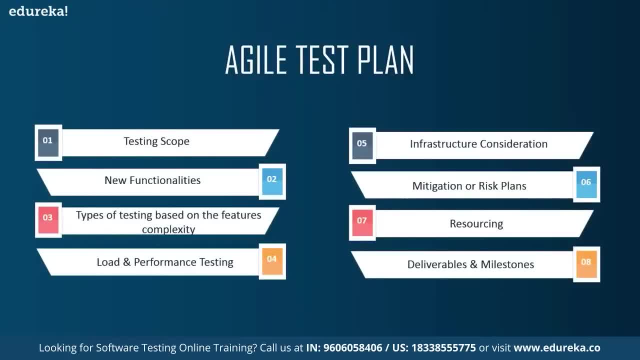 Then we have types of testing or various levels of testing, and next up we have performance and load testing that needs to be performed on your software. Next, we have the consideration of infrastructure, and then we have mitigation, or the risk plans, where you have to know about the risks. 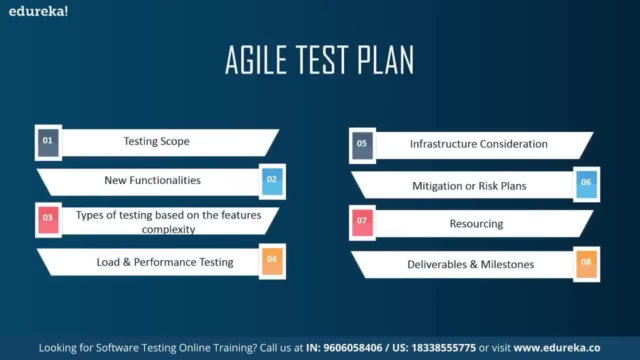 that might occur during the testing. Then we have the different planning of resources and, finally, deliverables and milestones, because you need to deliver your product as soon as possible in order to meet the requirements of your customer. So this is the plan that you must follow. 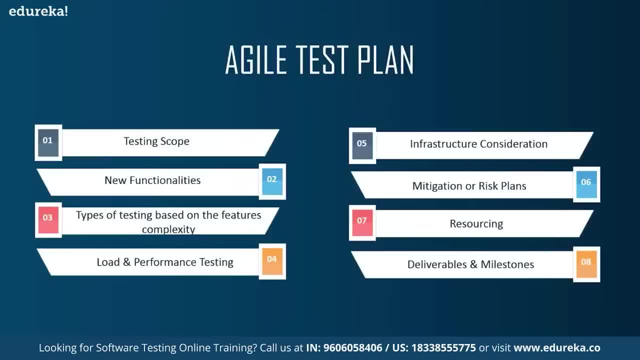 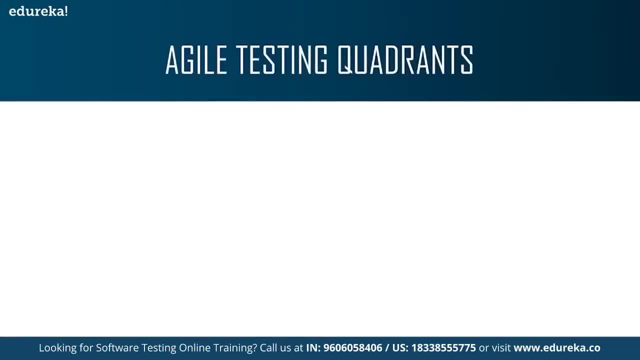 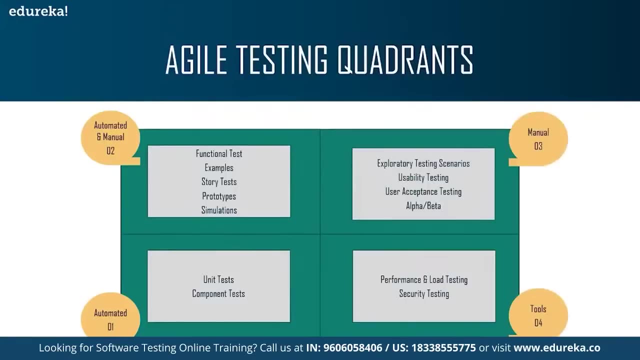 while performing agile testing on your software and also in order to deliver an error-free software. Now talking about the agile testing quadrants. these basically separate the whole process in four quadrants and help to understand how agile testing is actually performed. Now for the first quadrant. 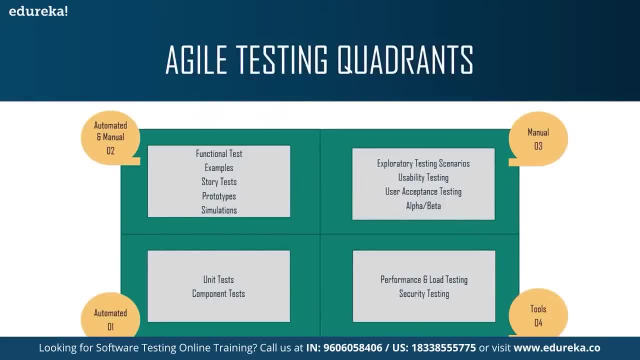 that is the agile quadrant one. the internal code quality is the main focus in this quadrant. It consists of test cases which are technologically driven and are implemented to support them. So it basically includes the unit tests and the component tests. So here we have the various unit tests. 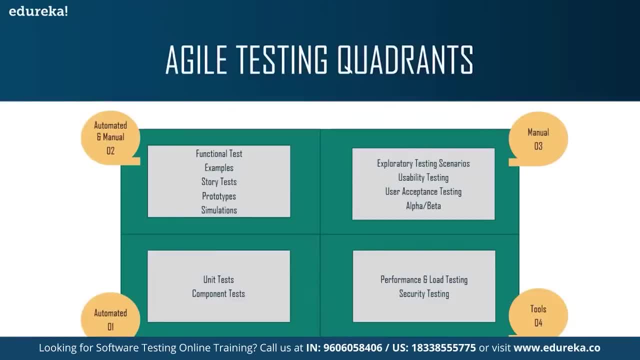 and component tests, and also this is the automated quadrant. Now the agile quadrant 2 contains test cases that are business driven and are implemented to support the team. Now this quadrant focuses on the requirements. The kind of test performed in this phase is the testing of examples. 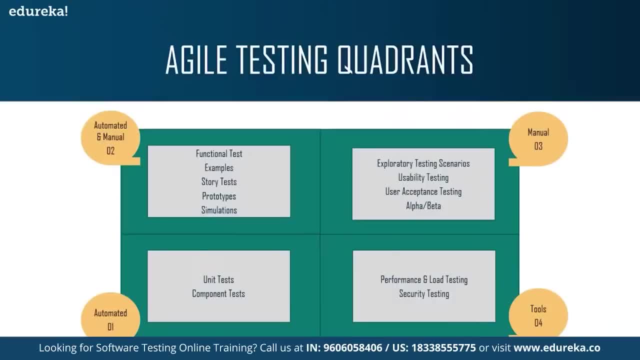 of possible scenarios and workflows, testing of user experience, such as the prototypes, and also paired testing. This can be automated and manual as well. Now, the agile quadrant 3 provides feedback to quadrants 1 and 2. The test cases can be used as the basis. 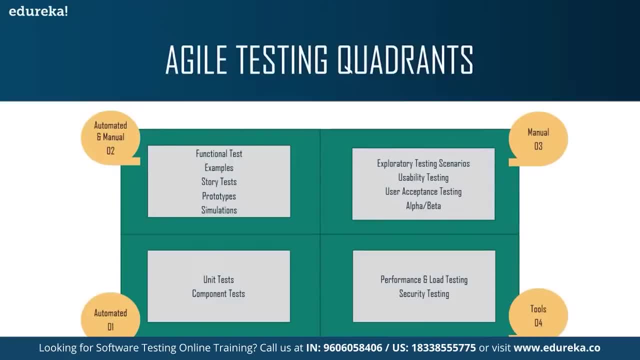 to perform automation testing. Now, in this quadrant many rounds of iteration reviews are carried out, which builds confidence in the product. So the kind of testing done in this quadrant is basically the usability testing, exploratory testing, paired testing with customers, collaborative and also user acceptance testing. 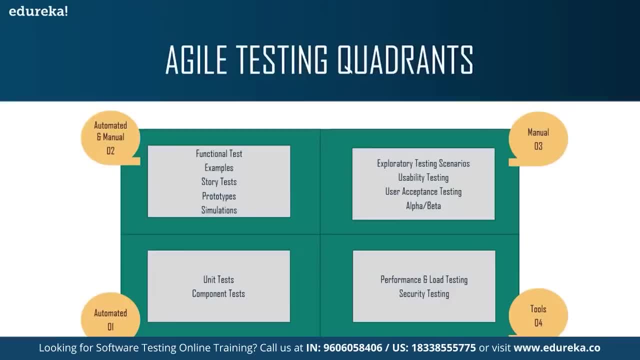 Now moving on to the final quadrant. the fourth quadrant basically concentrates on the non-functional requirements, such as the performance, security, stability, etc. Now, with the help of the agile quadrant, the application is made to deliver the non-functional qualities and the expected value. 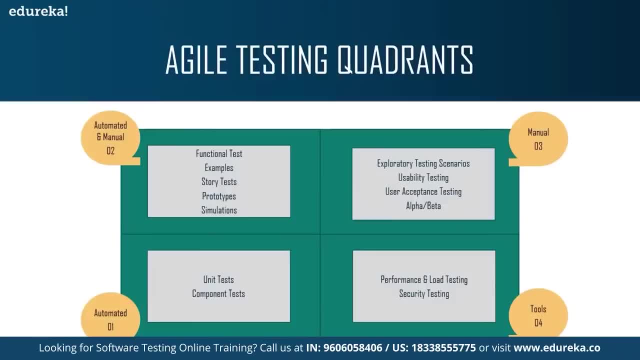 Now, in this quadrant, the kind of testing done is the non-functional tests, such as the stress and performance testing. Then we have the security testing with respect to authentication, hacking and also infrastructure, data migration, scalability and load testing. So now that you know why we need to perform agile testing, 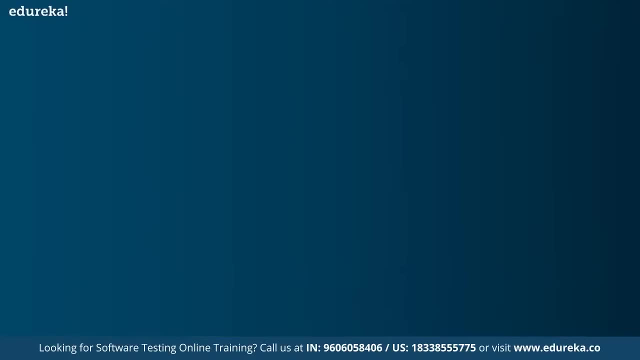 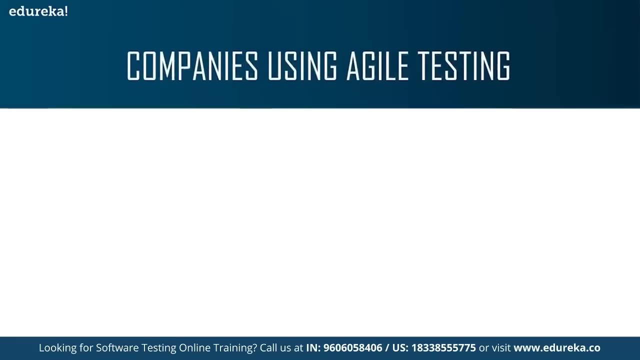 in our everyday lives. let's move on and have a look at the big companies that actually use agile testing for their software. So let's have a look at some of the big names. So there are Cisco, Sky, Philips, Vistaprint. 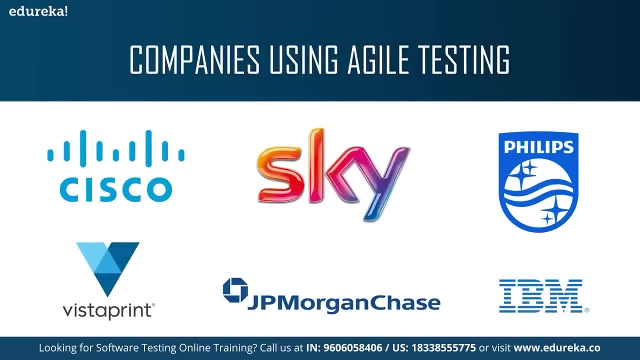 JPMorgan Chase, IBM and many more such companies that use agile testing as one of their methodologies. Now, Sky might be a household name, famous for its satellite TV, broadband and telephone services, but the media provider is almost making a name for itself in software development. 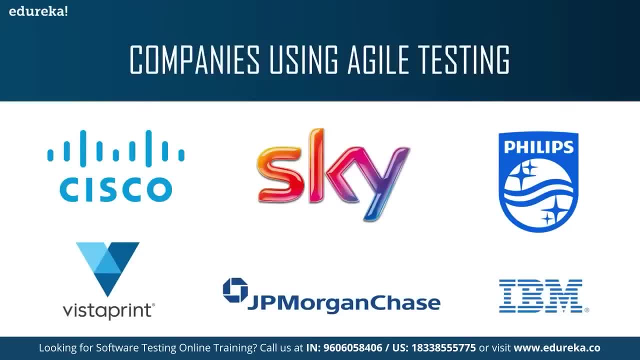 So the company which has launched products to combat the likes of Apple's TV box has been placing agile methodologies and open source at the center of the software development approach. Not just that, Philips has also adopted the agile principles Now, after numerous changes to management structure. 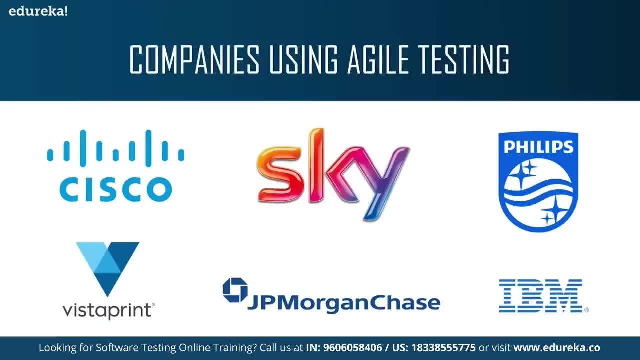 the firm introduced several agile coaches that went to deploy scrum principles, such as scrum boards and breaking down teams into smaller ones. As a result of changes like this, teams could react to situations quicker, bureaucracy was removed and it was ultimately easier for these smaller teams. 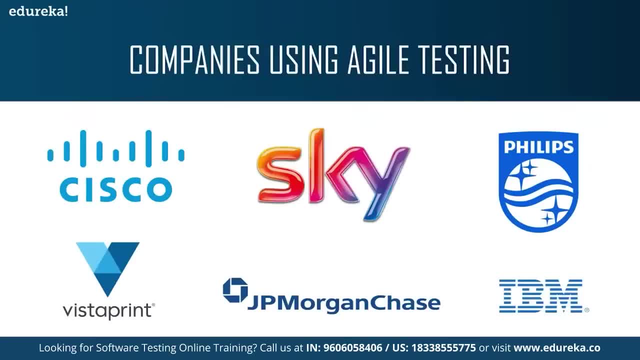 to take responsibility for their respective products. Not just that, Vistaprint is also the go-to marketing company for small businesses. Now the company performs some analysis of their existing waterfall methodology and found that teams were taking more than 60 days to move from the ideation phase to product delivery. 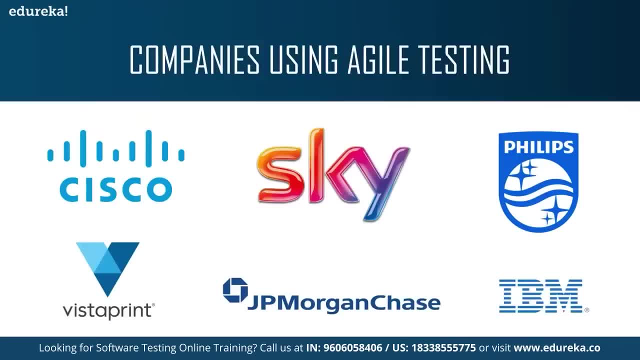 Now, the 60-day cycle only amounted to 40 hours of actual work. The company looked further into why this was the case. It transpired that unclear decisions and long creative lead times were to blame, all of which resulted in feedback loops. That's when they moved to the agile testing. 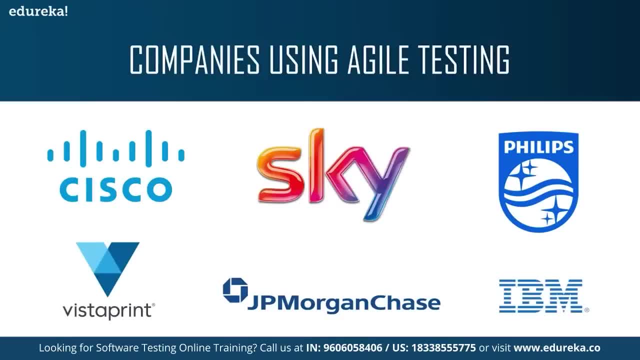 This is also the case for JPMorgan Chase Now. a few years ago, the baking giant overhauled their business processes to help improve product development and simultaneously slashed the cost of training as part of a high-profile IT initiative. Now, agile methodologies were a key part. 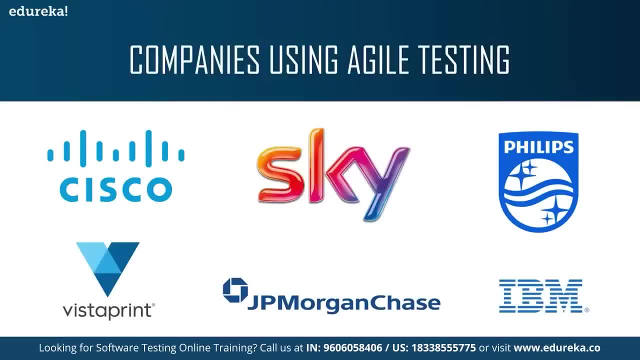 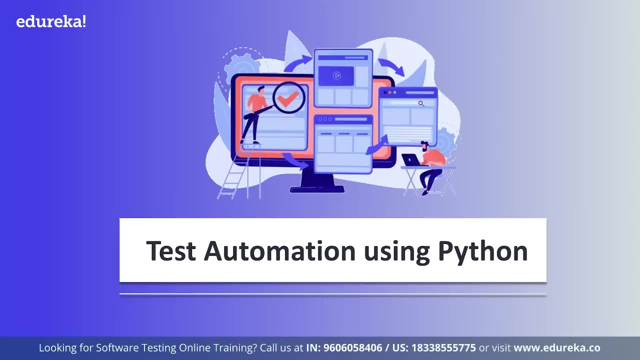 of that particular initiative. So that is all about what is agile testing and why exactly you need to perform agile testing on your softwares and also how it works in our daily lives. First, let's understand what is selenium and why it is required. 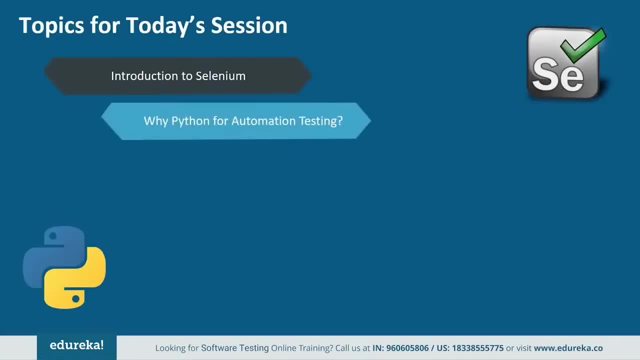 Next we will see why Python is preferred for automation testing. Once you understand this, we will move further and understand the binding between selenium and Python. After that, we will discuss about one of the important tool to write selenium script in Python, that is, PyCharm. 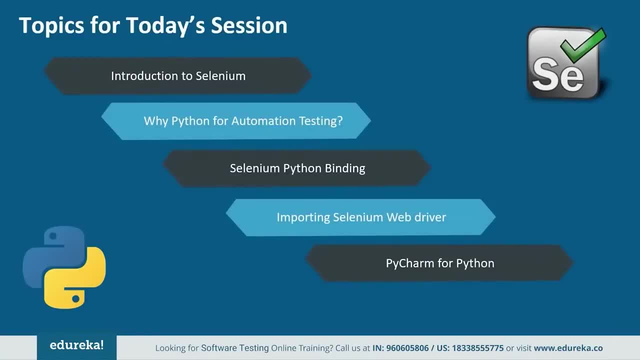 and we will also understand how to locate elements in selenium. and finally, I will wrap up the session by automating hotstar website in selenium using Python. So I hope you guys are clear with our agenda. Kindly give me a quick confirmation so that I can proceed further. 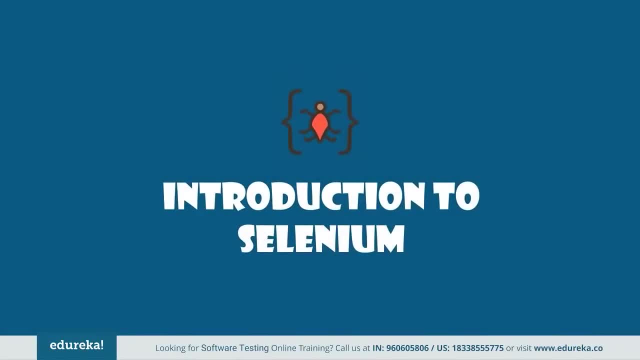 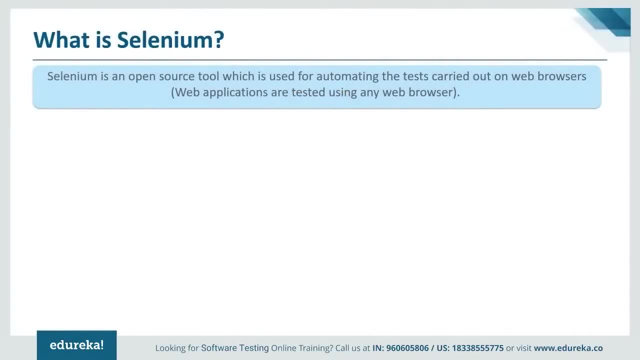 All right, So let's get straight to the point. Let's integrate with the module. first, Let's see What is selenium. selenium is an open source tool which is used for automating the tests that are carried out on web browsers. wait before you get carried away. 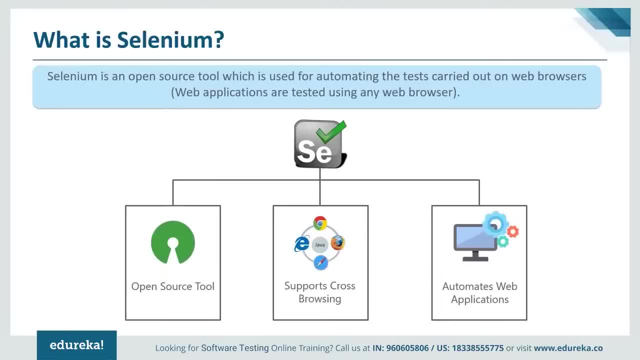 Let me reiterate that only testing of web applications is possible with selenium. We can neither test any desktop software application nor test any mobile application using selenium. So it is an open source tool that supports the cross browsing and automates web application Simple. 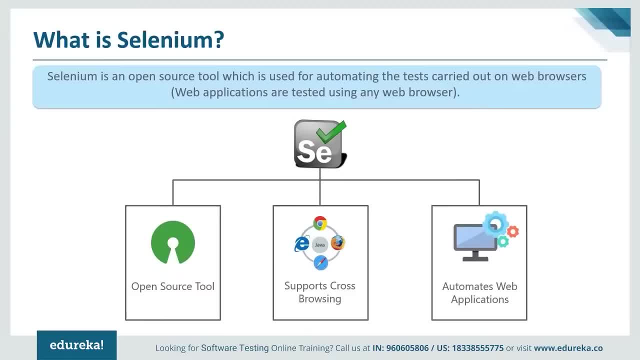 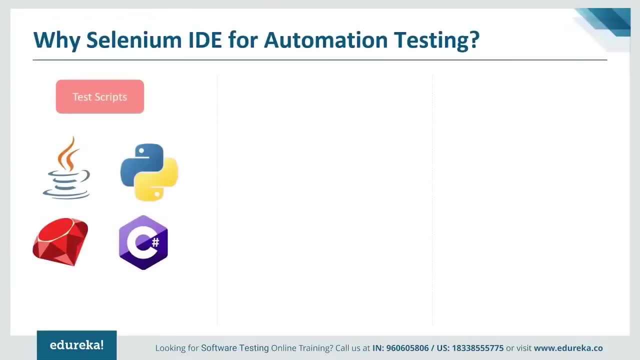 Okay, enough moving ahead. Now let's see. Why do we need selenium for automation testing. The main reasons are: the test scripts can be written in any of the programming languages, like Java, Python, Ruby C, sharp, dotnet, Etc. and test can also be carried out in any. 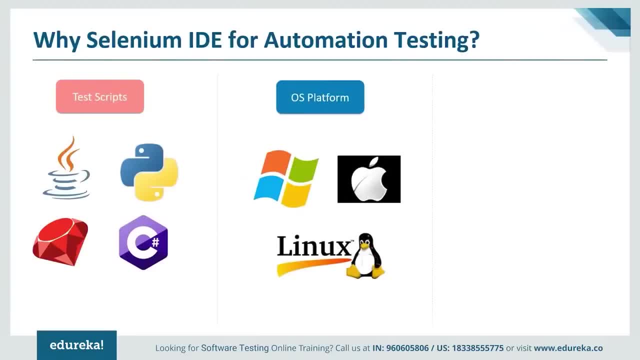 of these operating systems like Windows, Mac, Linux, Etc. and test can be carried out using any web browsers like Google Chrome, Internet Explorer, Mozilla Firefox, Safari, Opera, Etc. Not just that, it can also be integrated with tools like test ng and G unit for managing the test cases. 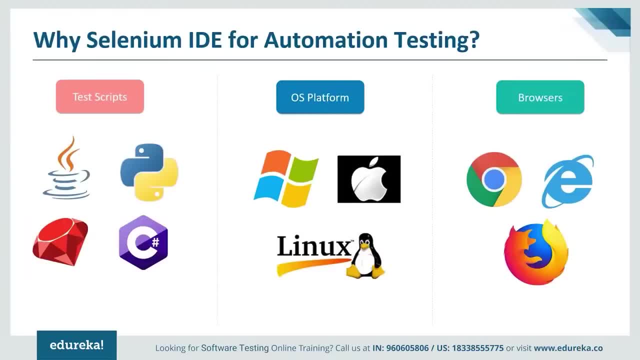 and generating the reports, and it can also be integrated with Maven, Jenkins and Docker to achieve continuous testing. So these are some of the reasons that keeps selenium at the top when compared to other automation tools, and that's why it is a preferred tool for testing. 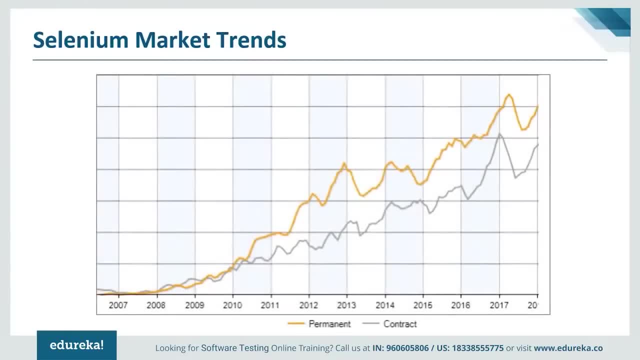 Now let's see the market trends of selenium. You can see in this figure the market trends from the past 10 years and you can easily make out the growth rate from 2007 till date. by this you can understand the demand for selenium in the testing domain of the IT world. 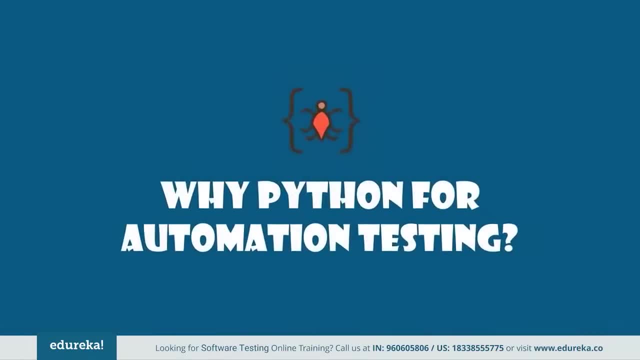 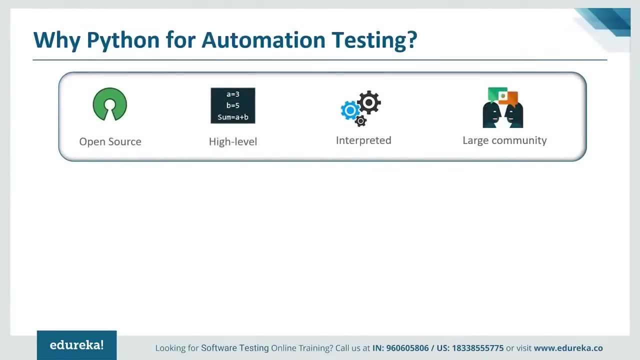 Now let's move further and understand by. Python is a preferred programming language for automation testing. Python is extremely simple and easy to learn. It's a very powerful language and it closely resembles the English language. So what contributes to its simplicity? Python is free and open-source. 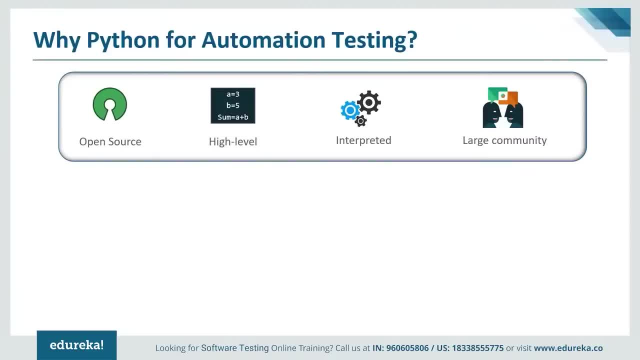 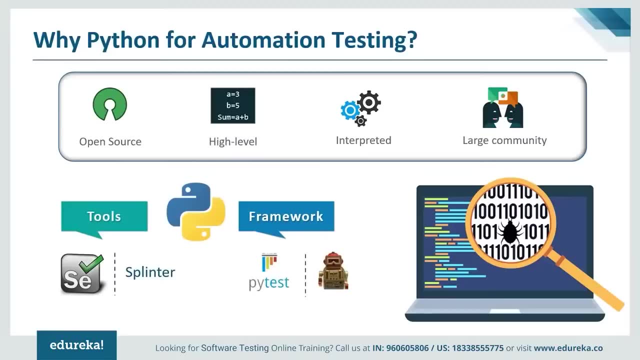 It is high-level interpreted and blessed with a large community, and Python also has many built-in testing frameworks. that covers debugging and fastest workflows. There are a lot of tools and modules to make things easier, such as selenium and splinter, and it also supports testing with cross-platform. 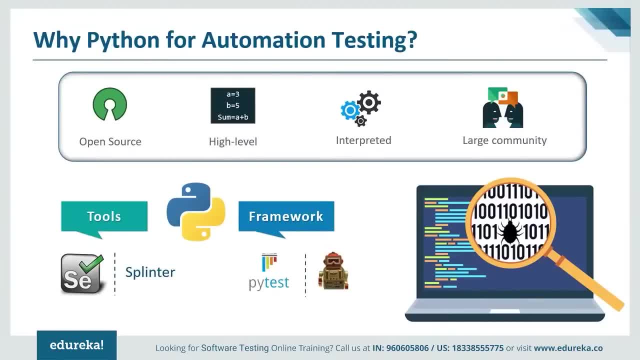 and cross browser with frameworks such as pytest and robot framework. So testing is a tedious task and python is a booster for it, So every tester should definitely go for it. with respect to that, Let's have a look at the market trends for python programming language. 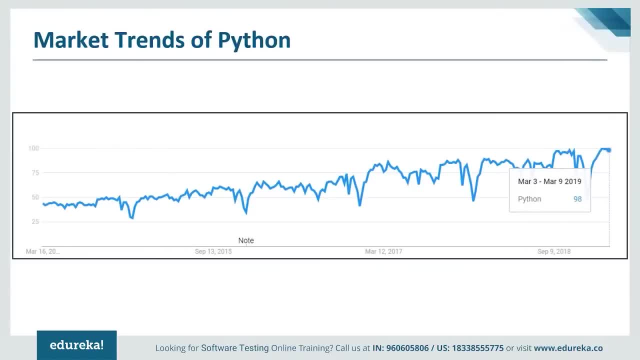 This graph depicts the market value of python since past five years and you can see the growth rate where it reads the peak maximum in the last year and recently. you can see the python count as 98 in the recent day of March 9.. So this implies the market value. 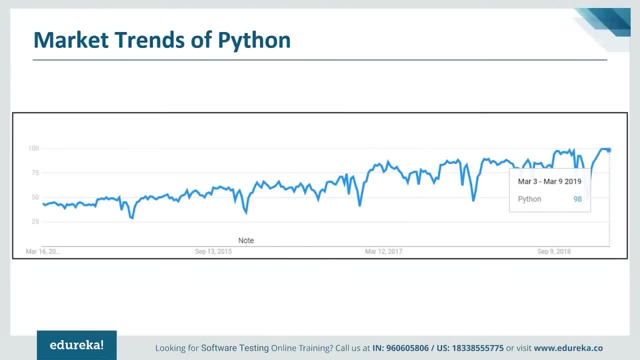 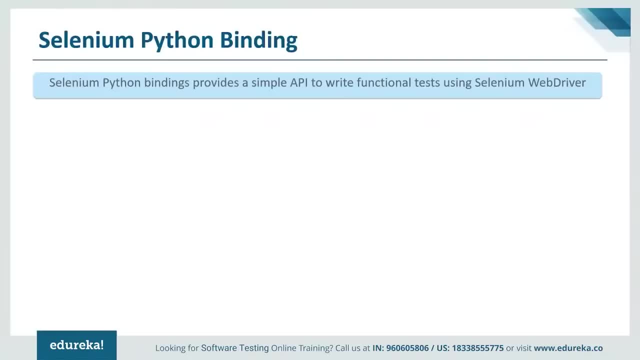 and demand for python that is growing at a higher rate. So let's move further and understand the binding between both of them, that the selenium and python- selenium- python bindings provide a simple API to write functional test using selenium web driver. here What you can do is you can simply write: 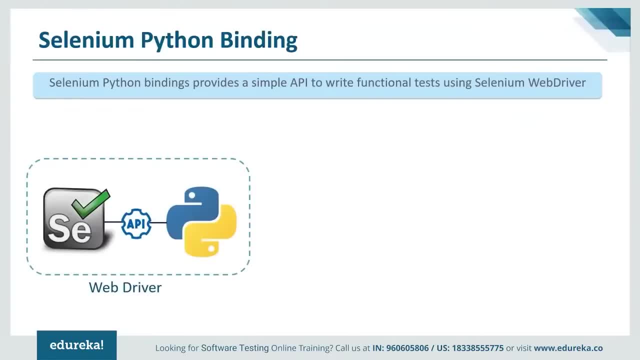 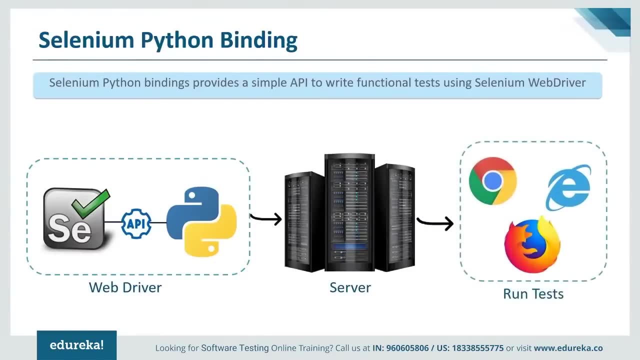 your functional test cases using selenium web driver. After that, you send a request to selenium server, and selenium server then runs the test cases on various browser. It can be Google Chrome, Internet Explorer or Mozilla Firefox. So this is how it works Now, in order to implement the python with selenium. 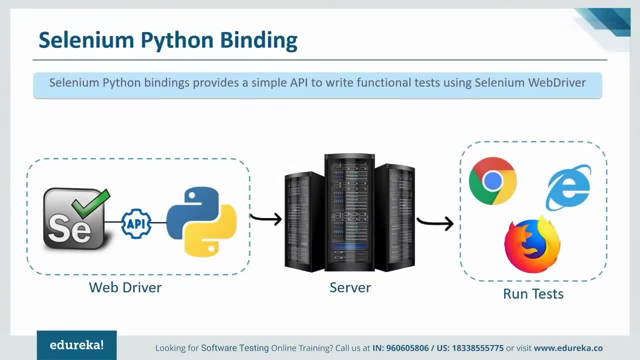 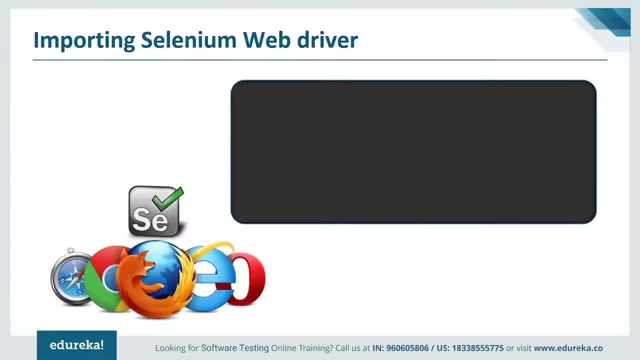 We first need to import the selenium web driver. So let's see How can we import selenium web driver. before that, Let me tell you what a selenium web driver. selenium web driver is a web-based automation testing framework which can test the web pages that are initiated on various web browsers. 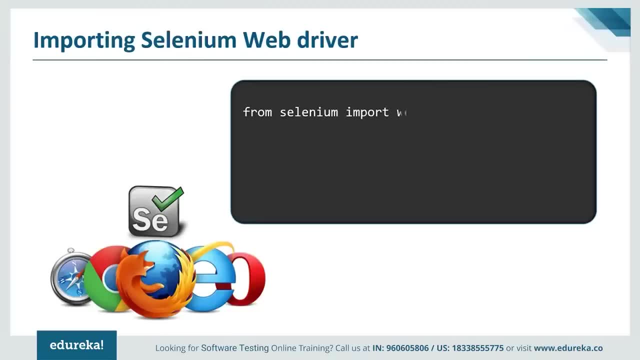 and various operating systems. You can import the web driver with the help of these two commands or just simply use the asterisk. that is this one, And that helps you to import all the dependencies that are required for a project Now, without wasting any further time. 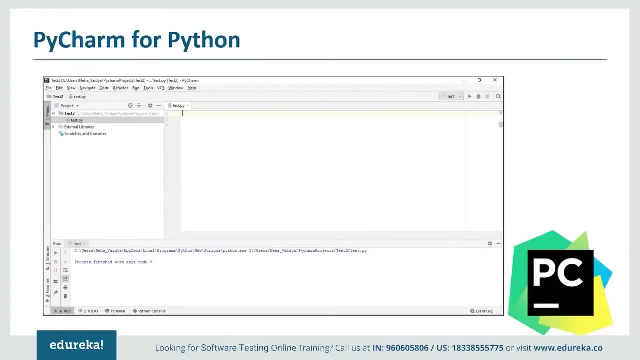 Let's talk about PyCharm. So this is an ID where you can write the python code or scripts in order to execute the test cases. You can use any other ID for the same, like you can use Jupiter, notebook, shell, etc. Over here. 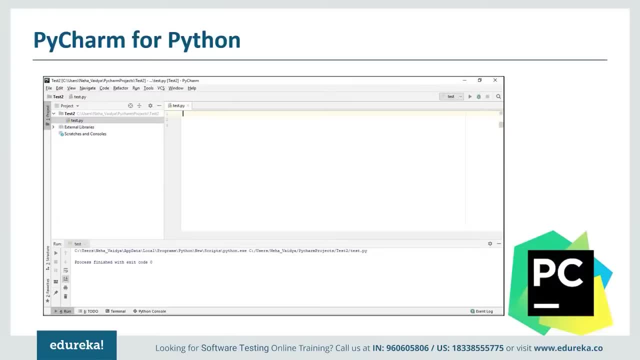 I'm using PyCharm, So this is how it looks. Python is an amazing language which has various frameworks like Django, flask, etc. You can also customize it with themes and plugins, and it also lets you to enhance the productivity while coding by providing some of the features. 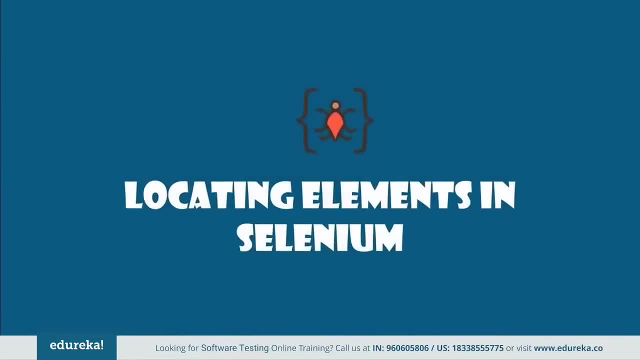 like suggestions, local VCS, etc. Now let's see what are locators in selenium. The locator can be termed as an address that identifies a web element uniquely within the web page. Locators are the HTML properties of the web element, which tells selenium about the web element. 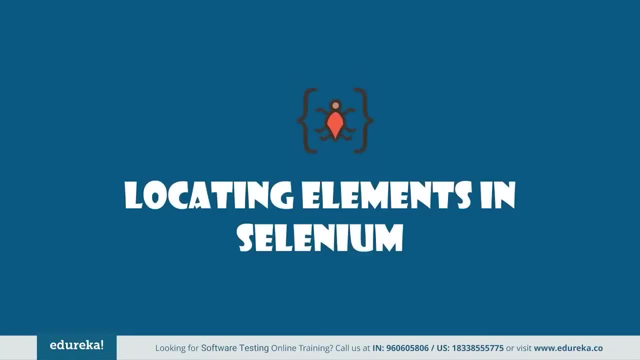 that needs to perform the action on, and selenium uses locators to interact with the web elements on the web page. Now there are diverse range of web elements, like text box, ID, radio button, etc. and identifying these elements has been a very tricky subject, and thus it requires an accurate 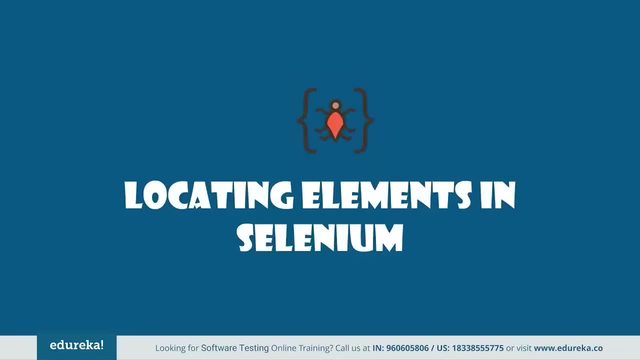 and effective approach, and thereby we can assert that more effective locator is more stable, will be the automation script. Essentially, every selenium command requires locators to find web elements. Thus, in order to identify these elements accurately and precisely, We have different types of locators. 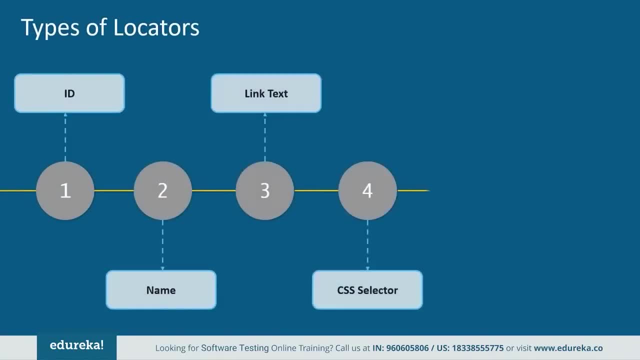 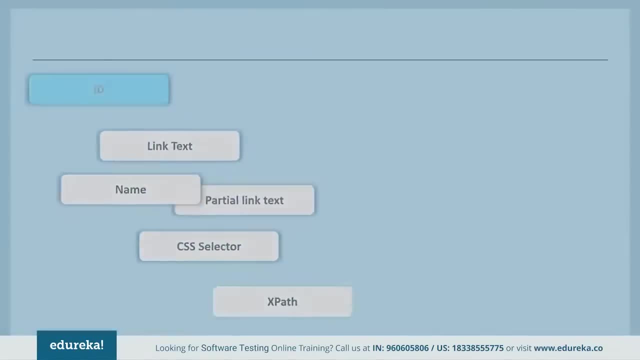 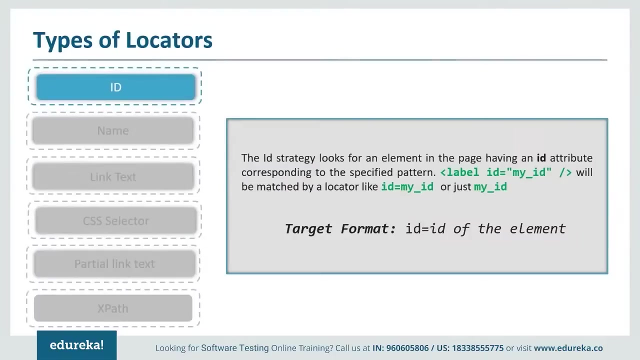 like ID, name, link text, CSS selector, partial link text and XPath. So let's get into the details of all these types. first, ID locator: the best and the most popular method to identify web element is to use ID. The idea of each element is alleged to be unique IDs. 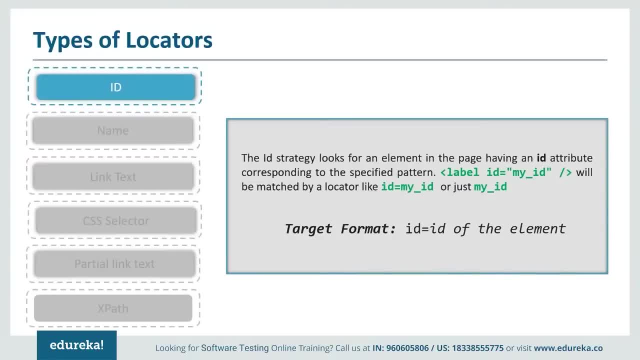 are the safest and fastest locator option and should always be the first choice, even when there are multiple choices. For example, it is like an employee number or account number which will be uniquely identified. Now let's see how to use ID locator with the help of example. 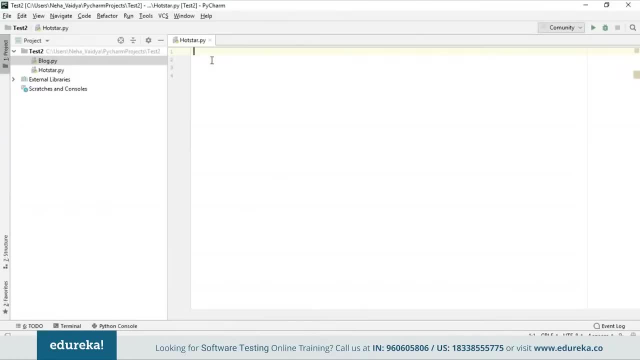 So first I have created a simple file in Python that is hot star, and the very first step that I'm going to do is I'm going to import the web driver. So I'm going to write it like from selenium: Import web driver simple. 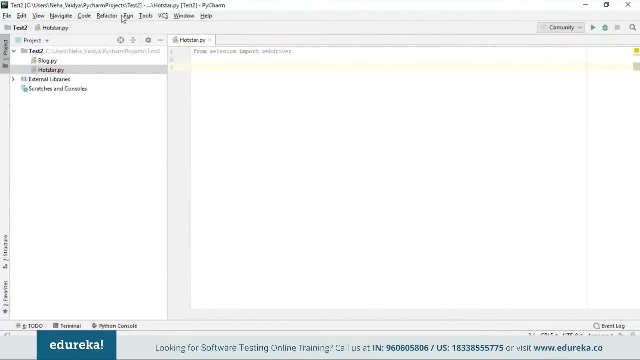 So, once I import the web driver, the next step is to launch the Chrome driver, So I'll create a new element called. driver is equal to, so my web driver will be Chrome, And this is the path where I have saved my Chrome driver. 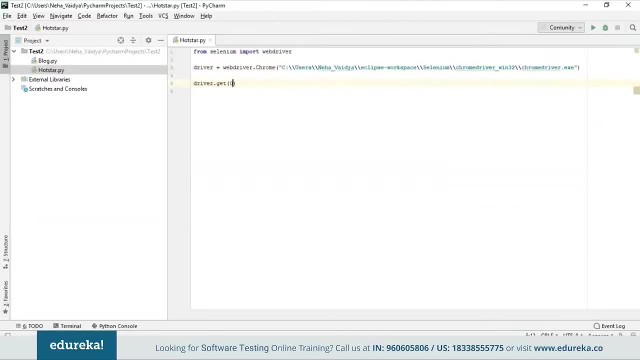 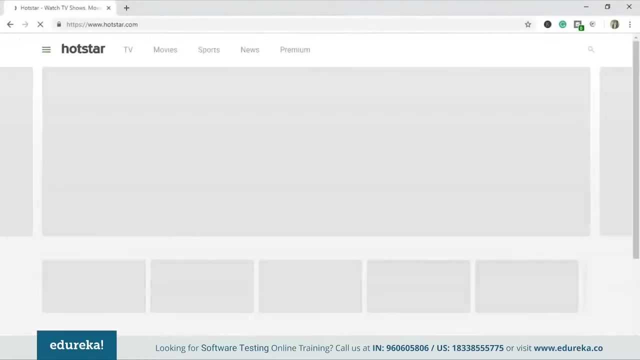 Okay. Next I will use driver dot get method and give the link of hotstarcom because I want to locate the elements that is present in hot star. So that's the reason I'm giving this link. So here I will navigate to hot star website. 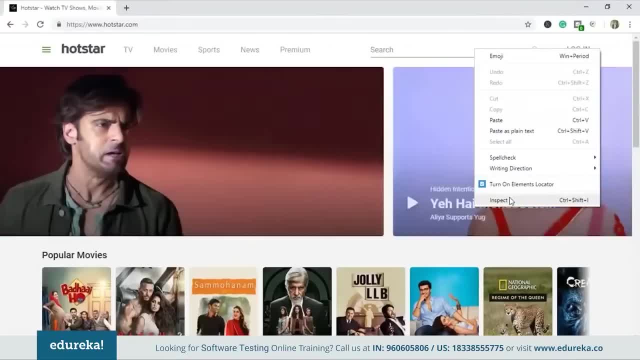 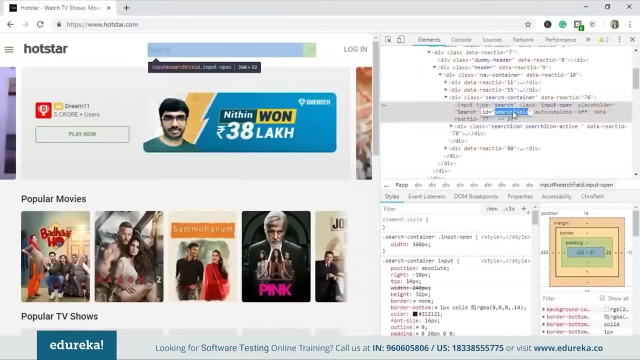 and locate the search box first, what I will do. I'll inspect on this and you can see it has a ID attribute whose value is search field, So I'll just copy this value now. The next step is to write the script in PyCharm. 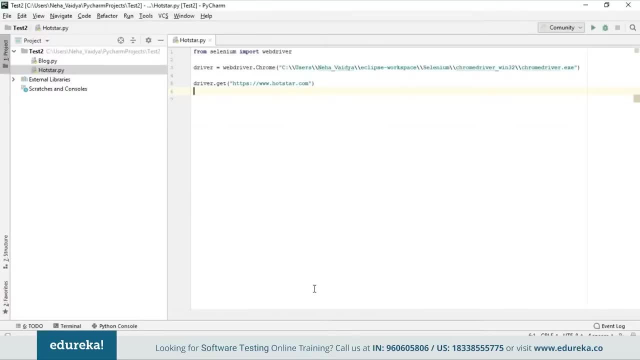 So I have already imported the web driver and I've launched the link and also have registered my Chrome driver. So once this is done, the very next step is to locate the elements and perform action on it. So what I'll do? I'll use driver dot find element by ID. 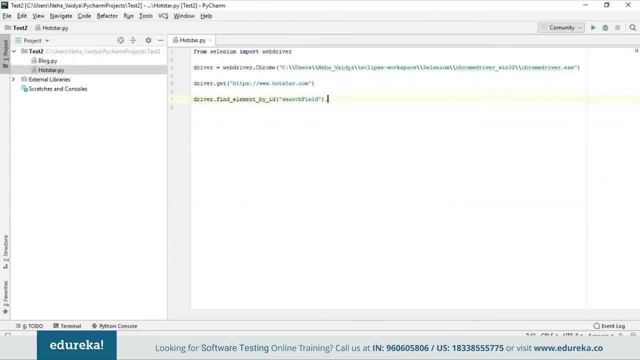 and the value of ID is search field and I want to send keys as movies. Okay, what I'm doing here is I'm finding the element by ID attribute whose value is search field, And I'm sending the value to that search field as movies. 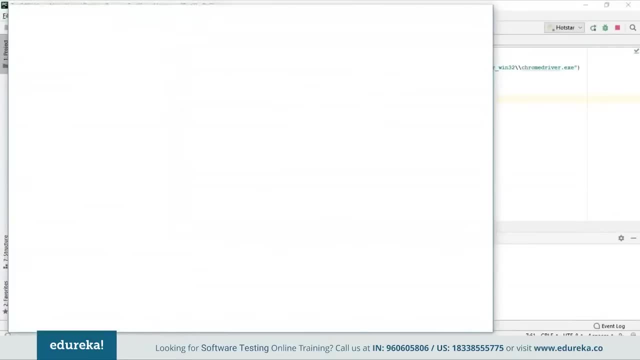 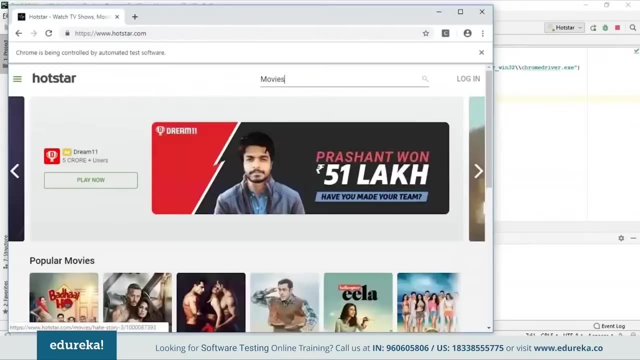 So I'm going to run the program. Let's check what will be the output. So Chrome driver launched. Google Chrome navigated through hotstarcom and entered the value as movies in the search field, So you can choose from any of these movies. 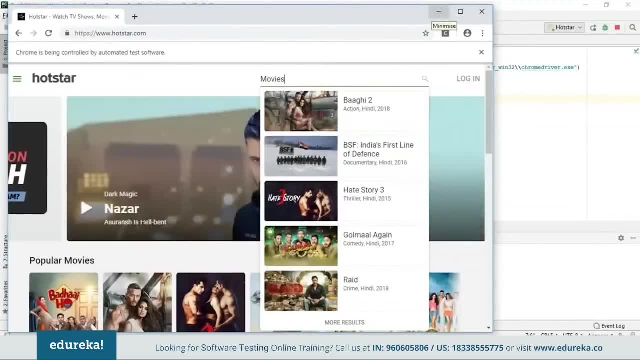 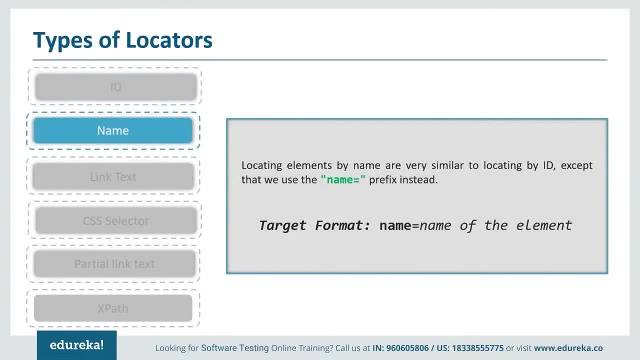 Okay, sounds much simple, right? So this is how you can locate the elements using ID attribute. Next one is name locator. This is also an efficient way to locate elements with the name attribute After IDs. you can give it your second preference. 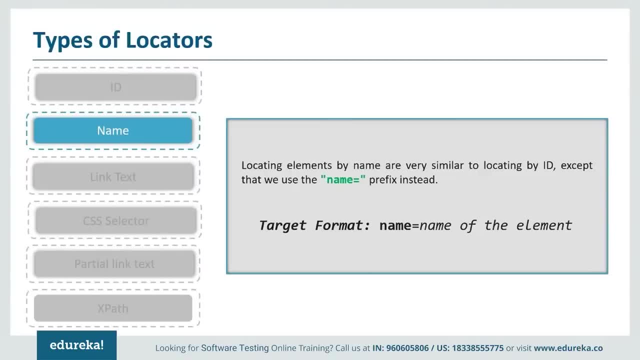 But likewise name attributes don't have to be unique in the page. With the strategy, the first element with the name attribute value that is matching the location will be returned. If no element has a matching name attribute, then no such element exception will be raised. 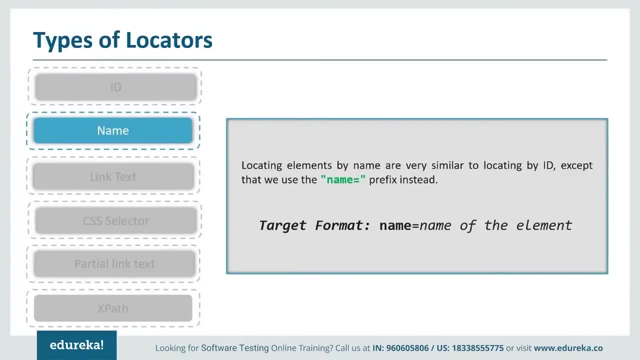 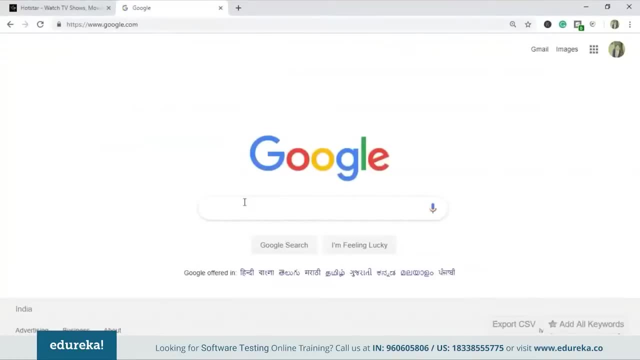 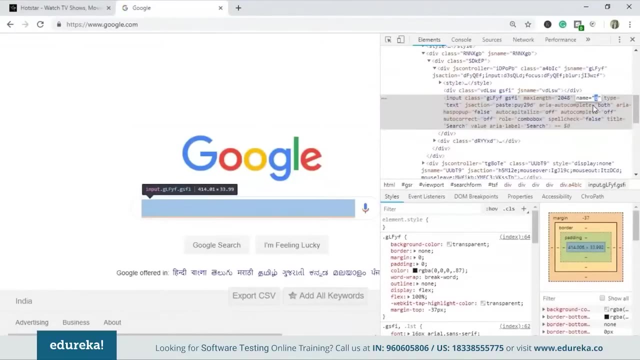 Let's see it's working. It's almost same like ID attribute, but the difference here is that instead of ID you have to use a name attribute. So what I'll do? I'll just navigate to googlecom and inspect the search box and you can see it has a name attribute whose value is Q. 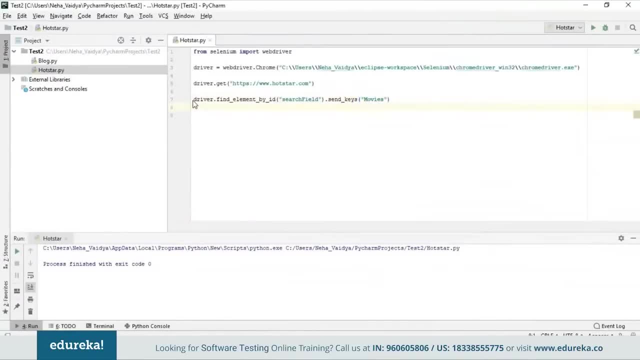 So I'll just copy this: open my pie charm. I'll just comment this first and I will write: driver dot- find element by name whose value is Q dot. I want to send keys as selenium And also I want to give this search as well. 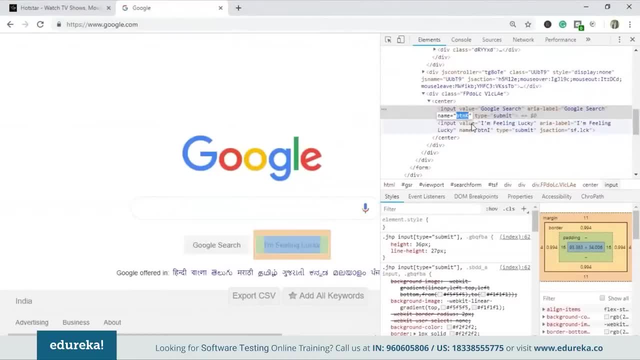 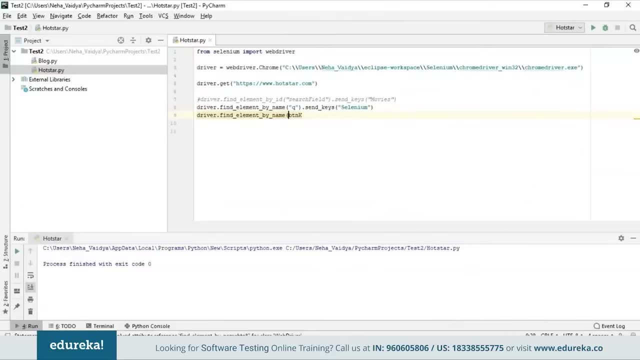 So again, that has a name attribute. whose value is this? So I'll copy this. I'll just paste it over your. as it is a button, I'll use click method because it is not a text box to send the values to it, So I'm just using click. 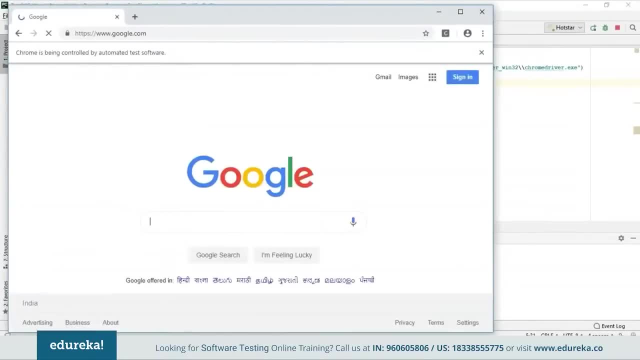 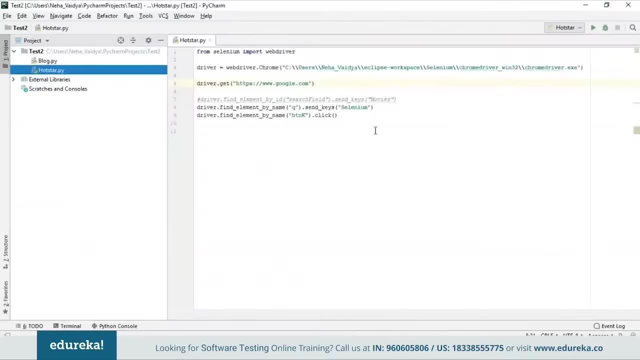 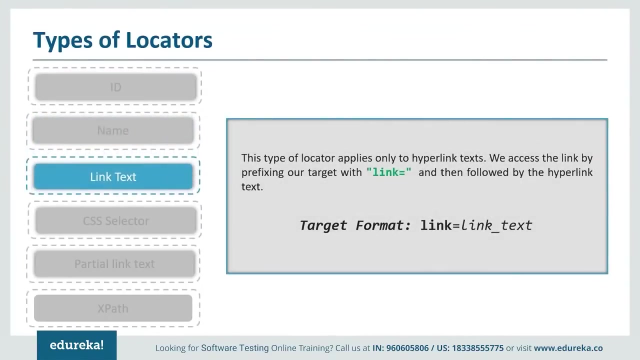 Let's run the program and check the output So you can see. it gave the search for selenium simple, So this is how you can use name locator moving forward. Next is link text. all the hyperlinks on the web page can be identified using link text. 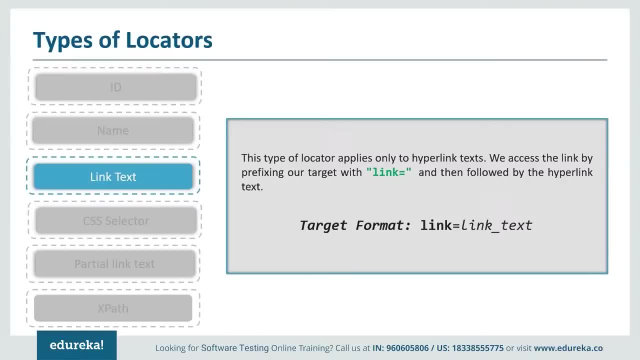 The links on the web page can be determined with the help of an anchor tag. Now the anchor tag is used to create the hyperlinks on the web page, and the text between the opening and closing of anchor tag constitutes the link text. Now let's see how it works. 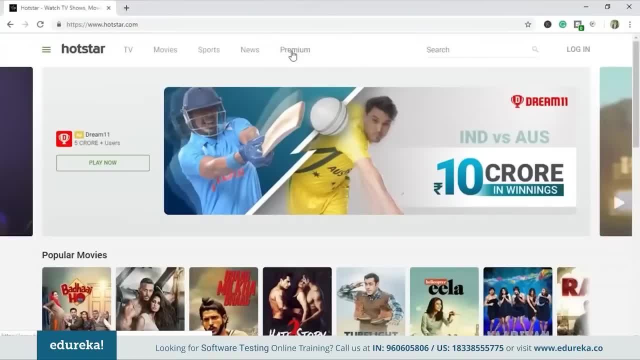 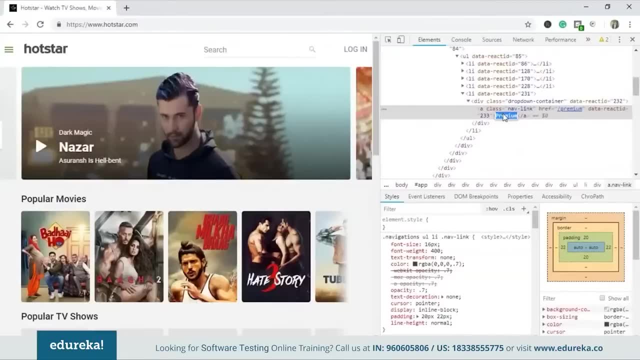 Now let's switch back to hotstar and try to locate on this particular link that is premium. As you can see, it consists of a link text called premium, So I will write my python script and search element by link text as python and click on it. 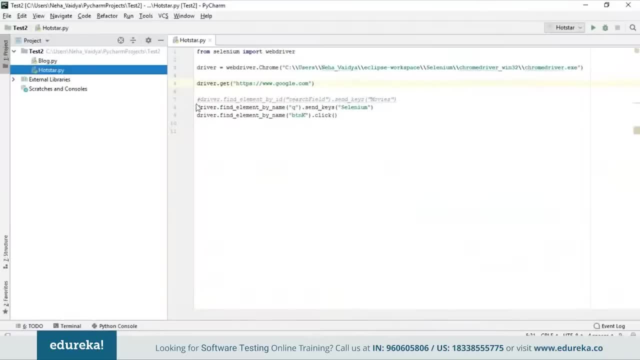 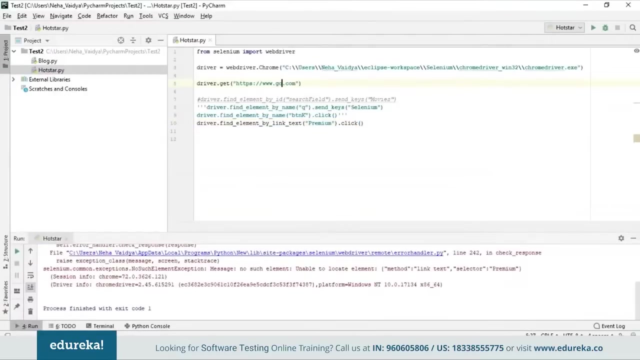 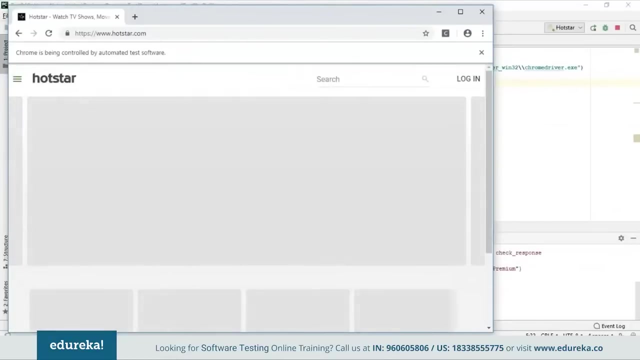 So I'll copy this. I'll open my pycharm and write driver dot find element by link text and the value is premium Dot click because it is a link. So let's run the program and check the output. On executing the program, it clicked on the premium link. 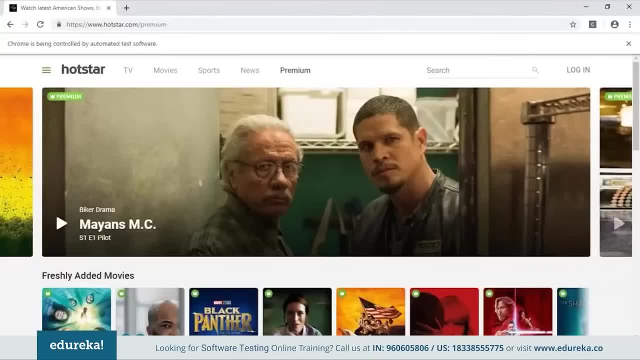 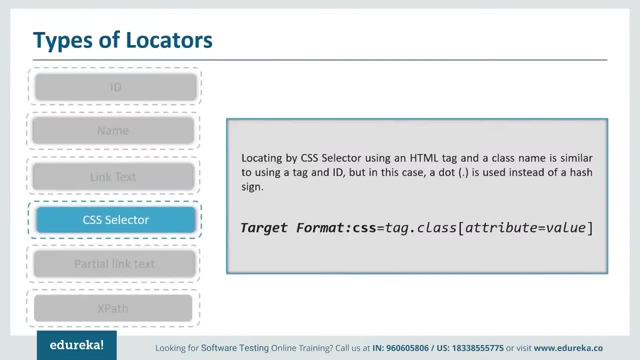 and gave the result. So this is how it works. Next, Let's see What are CSS selectors. CSS is mainly used to provide the style rules for the web pages. We can use CSS for identifying one or more elements in the web page. 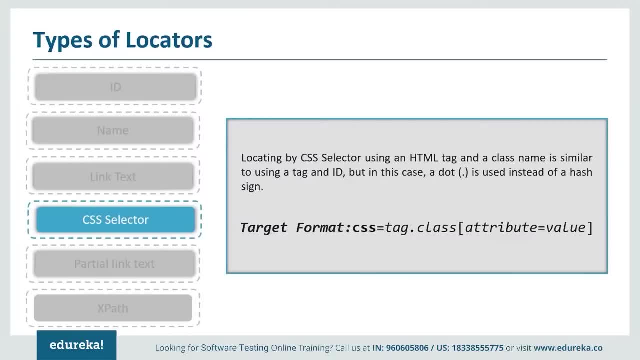 If you start using CSS selectors to identify elements, you will love the speed when compared with XPath. Now we can also use CSS selector to make sure that the scripts run with the same speed in all the browsers, So CSS selectors becomes the best possible way. 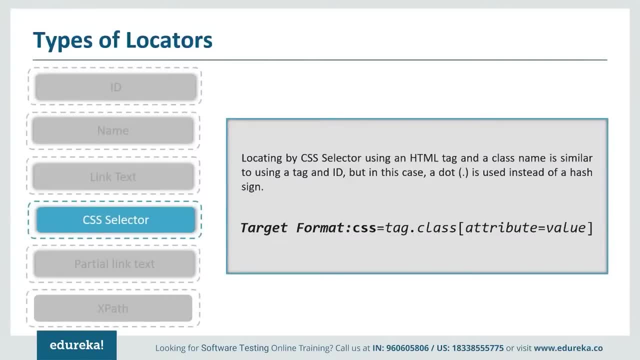 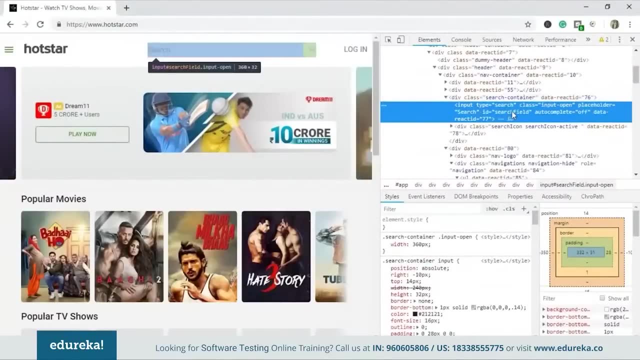 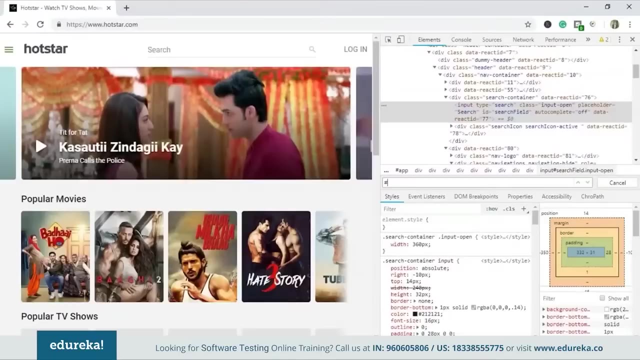 to locate complex elements in the web page. Let's locate the same search field using CSS selectors. So I'll inspect on this, As it has the ID attribute whose value is search field. I'll just copy this and you all might know that CSS selectors starts with hash. 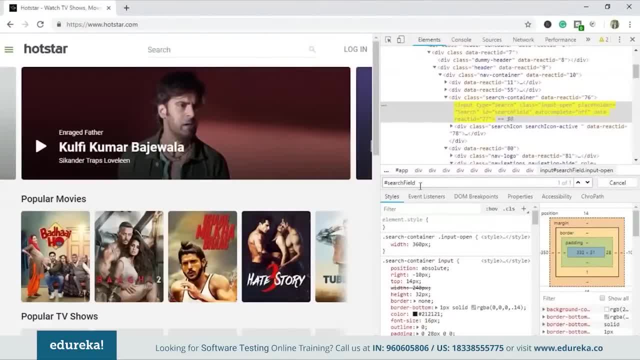 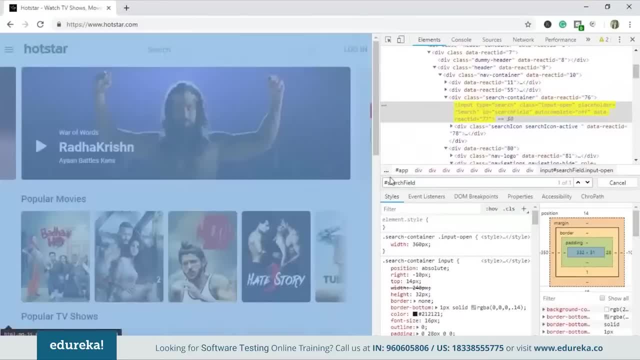 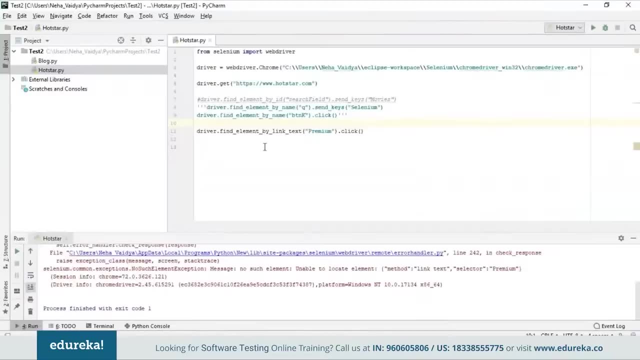 So I will give hash, followed by this ID attribute value. as you can see, it highlighted the element on writing the CSS selectors, which implies it was able to locate this particular element using this particular CSS selectors. Now I will copy the CSS selector. go to my pie charm. 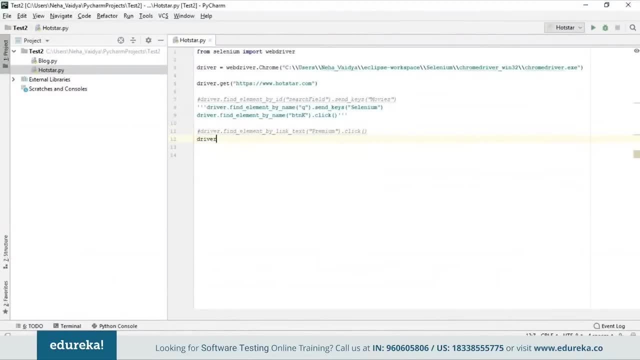 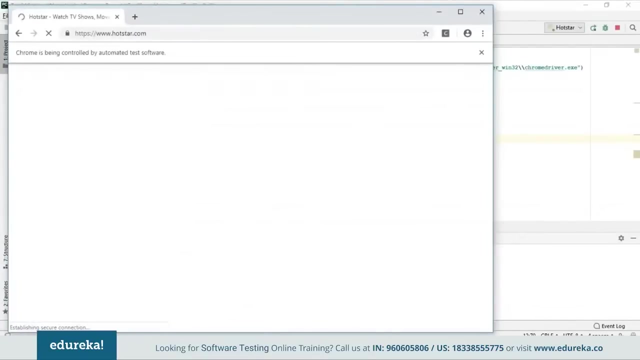 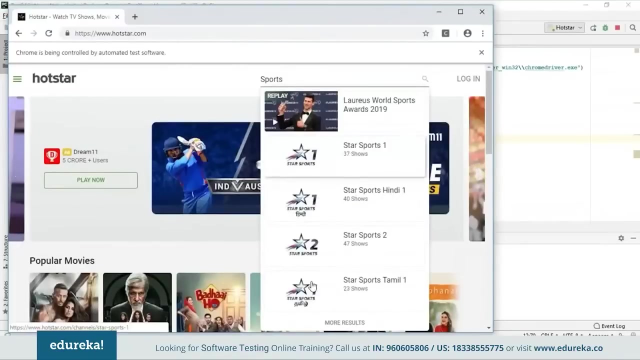 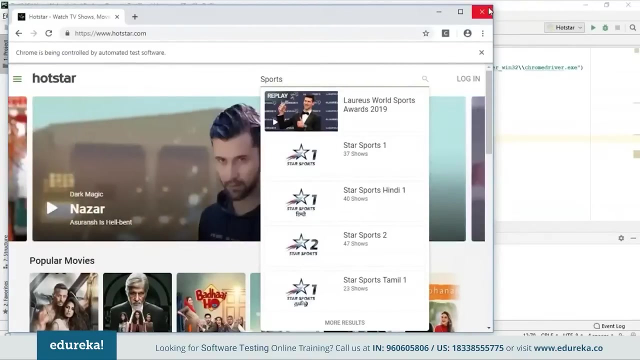 And write CSS selector: Send keys as sports. Let's check the output now. So it launched hotstarcom. enter sports: Correct, So you can choose from any of these sports channels, your awards, etc. Sounds simple, right? So that's how it works. 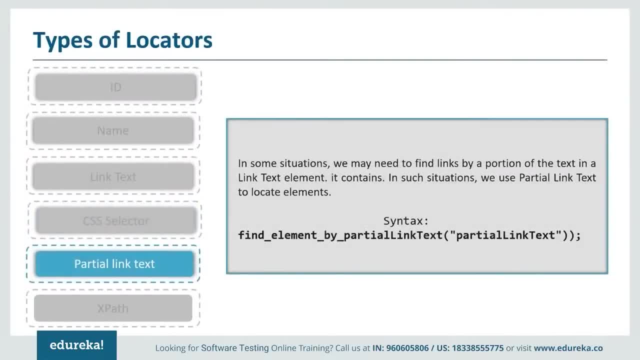 Now let's move further and see how to locate elements using partial link text. In some situations we may need to find links by a portion of the text in a link text element. in such situations, We use partial link text to locate the elements here. 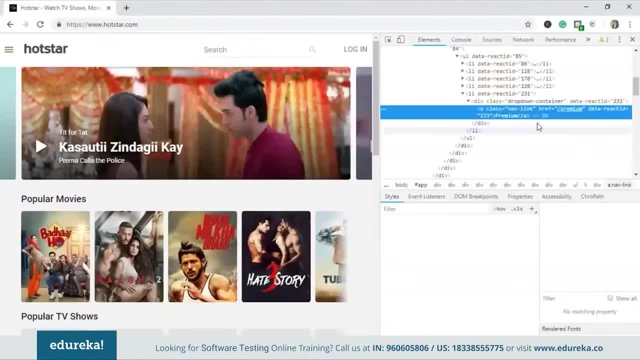 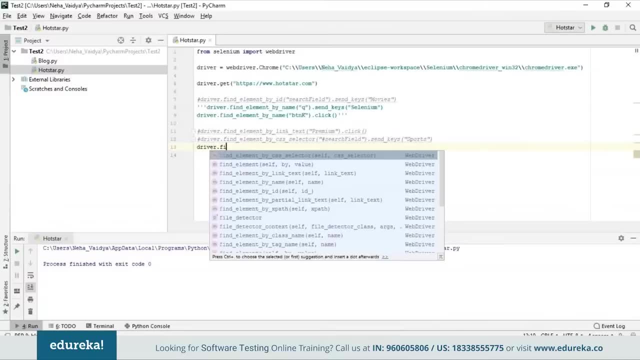 Let's try to click on this particular link itself and try to locate it. So what I'll do? I'll write Driver dot find element by partial link text and I'll place the value as. instead of giving the full value as premium, I have just given the half value. 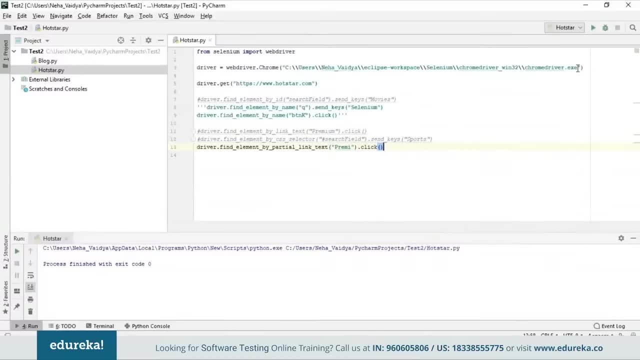 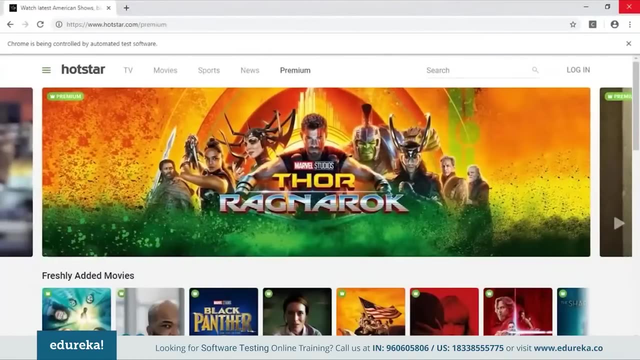 and I'm using click method to click on that simple. Let's run the program and check the output So you can see. so, even on using the partial value, it was able to locate the element. That's how partial link text locator is useful. 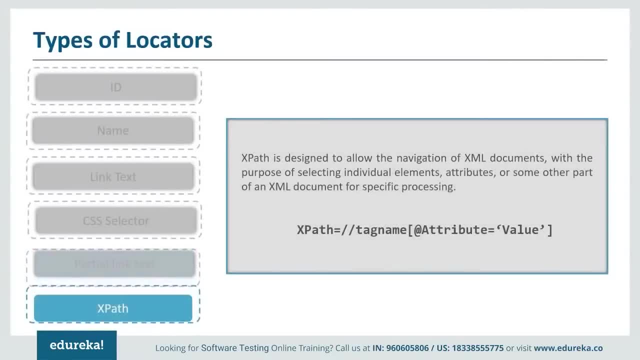 in locating the elements. Next, let's move to the last locator, that is XPath. So this is my favorite locator. XPath, also called as XML path, is a language to query XML documents. It consists of a path expression along with some conditions. Now let's understand the working of XPath. 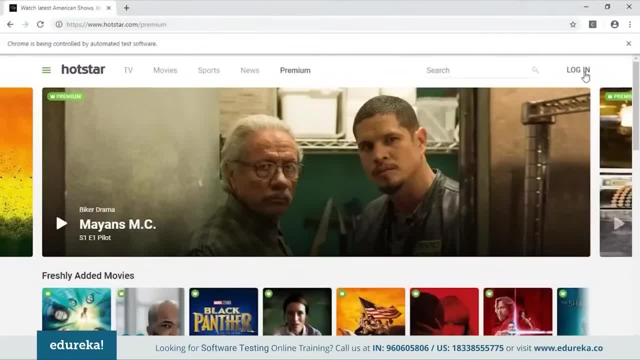 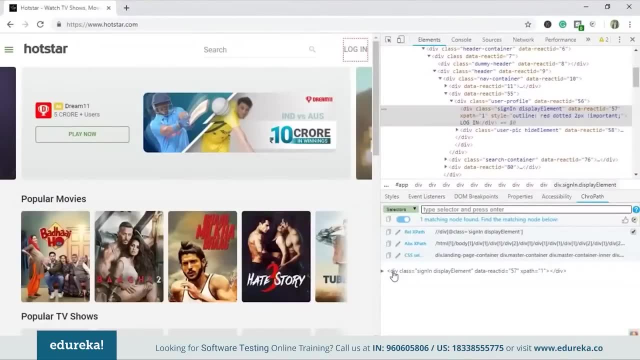 Now here. I want to perform action on this login button. So what will I do? I will write the XPath for this. as I have already added the crow path extension, I need not manually write XPath for this particular element. Instead, I will find it using crow path. 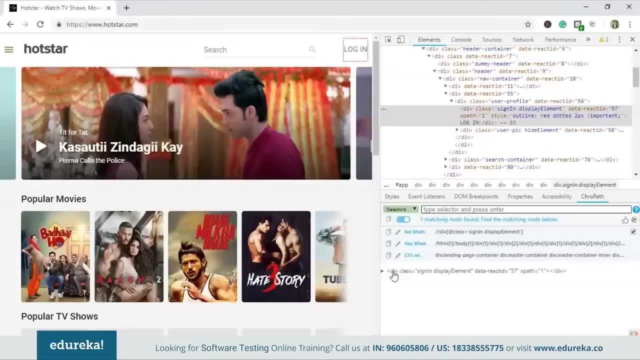 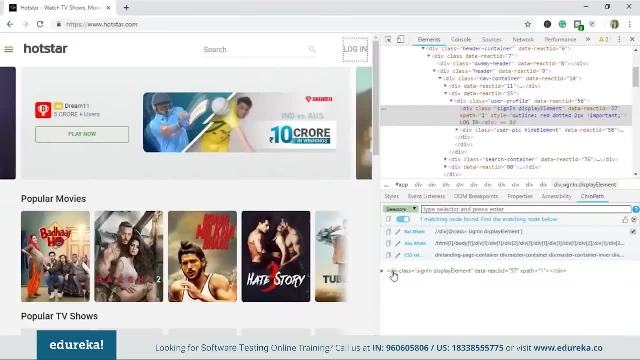 Crow path is basically a tool that is very helpful to find XPath and CSS selectors. If you wish to know more about it, you can check my video on new features of crow path in our YouTube playlist. Now I will copy this XPath and paste this value in my script. 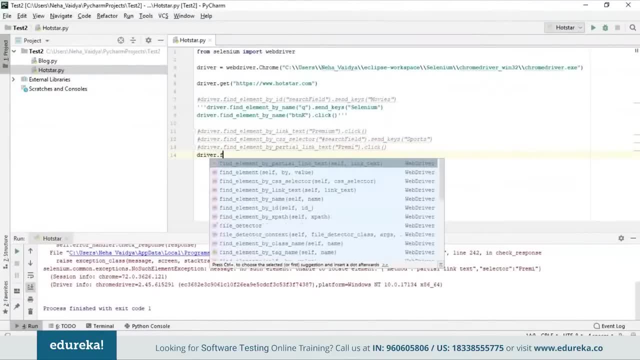 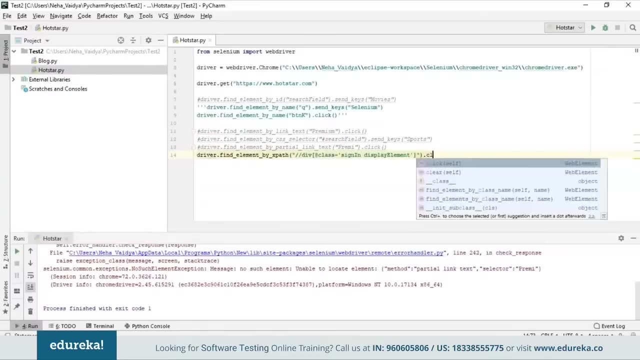 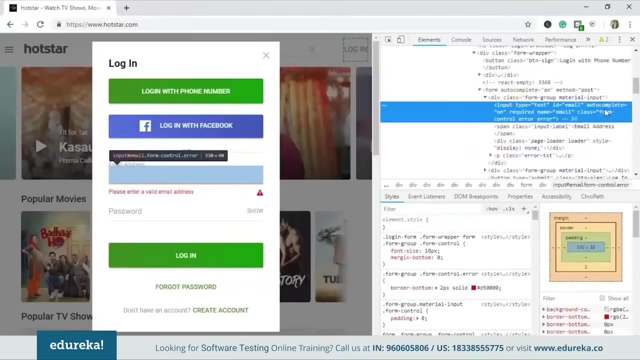 So first I will write driver dot find element by XPath. in this I'll paste the value. as it is a button, I'm just clicking on that, Okay, Next I want to enter the email address and password as well. So in case of this, 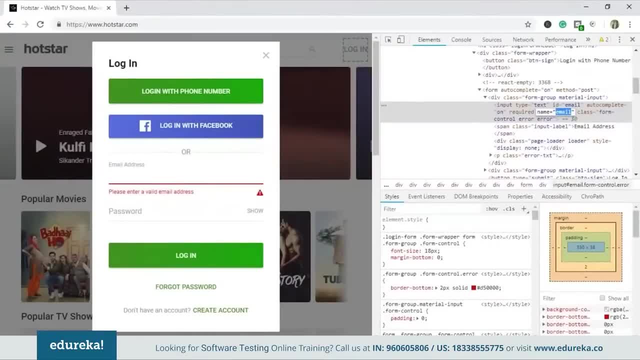 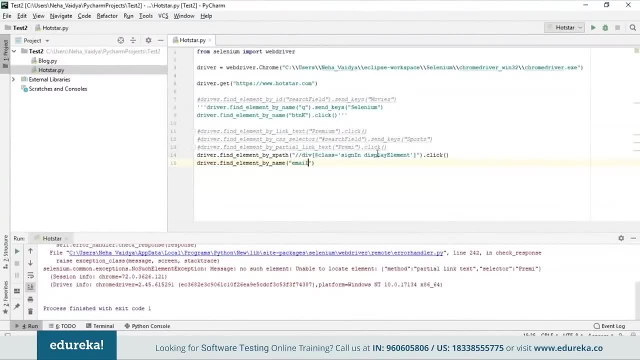 it has a name attribute whose value is email. So I'll just copy that. So I'll write driver dot, find element by name and pass the value as email and I will give send keys and pass the value of the email as I she at the rate. 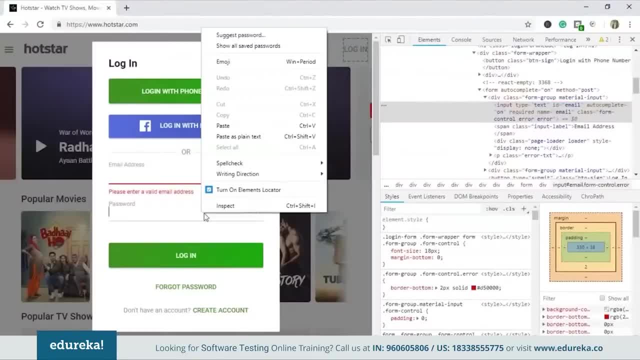 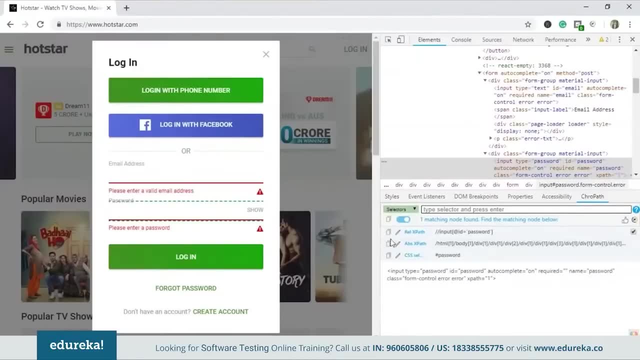 at Eureka dot co. and I'll again inspect this password field and it has an ID attribute. even I can use the crow path as well, So you can see the CSS selector. There's an absolute XPath and there's a relative XPath. So what I'll do? I'll copy the relative XPath. 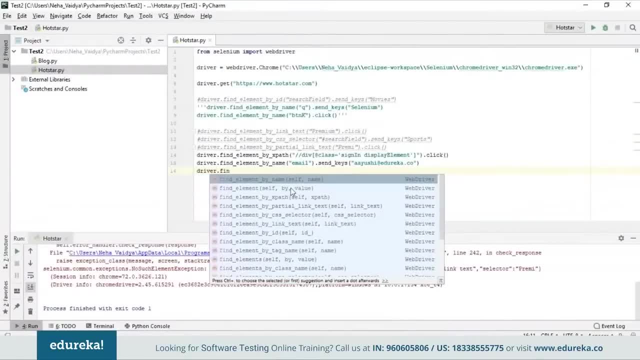 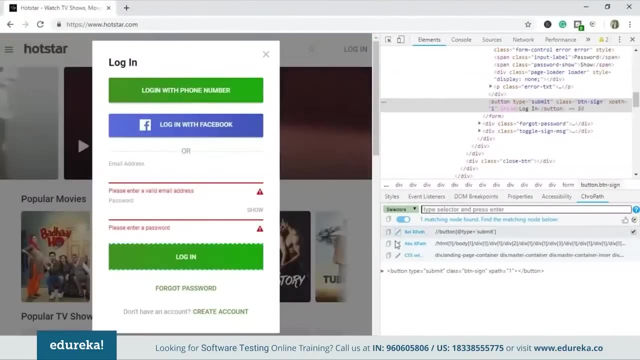 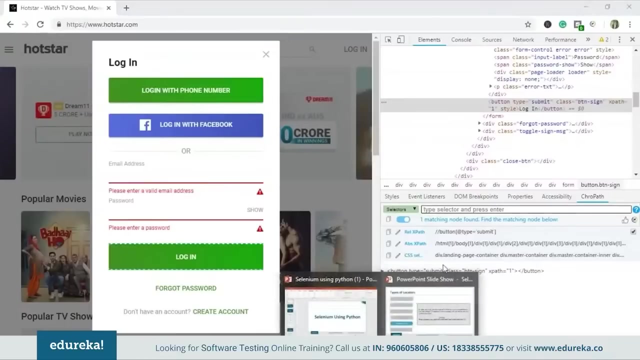 and I'll write find element by XPath and pass the value and I'll give password for that. Next I want to click on this button, So again it has a class, that is button sign. but I'll again copy the XPath for that. 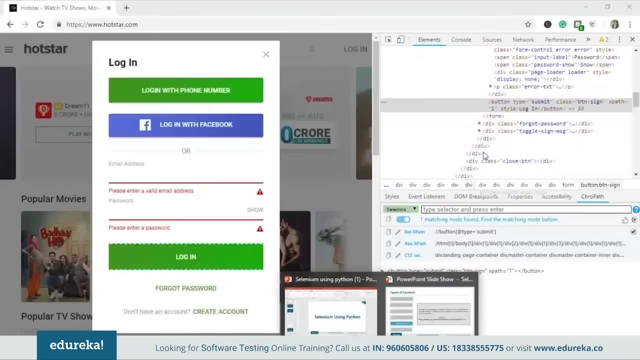 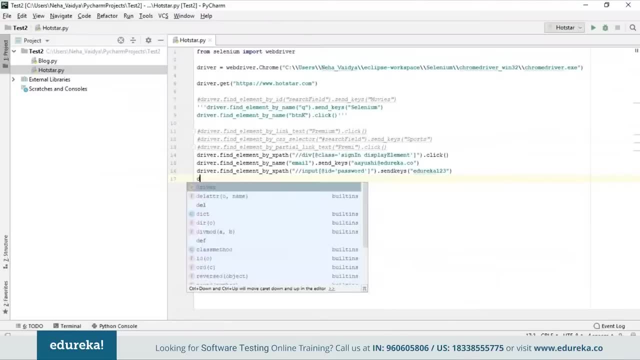 That is, it starts with the type whose value is submit. It has a button tag and attribute is type whose value is submit. So I'll copy this. I will paste it over here: Dot click Okay. So now when you run the program, 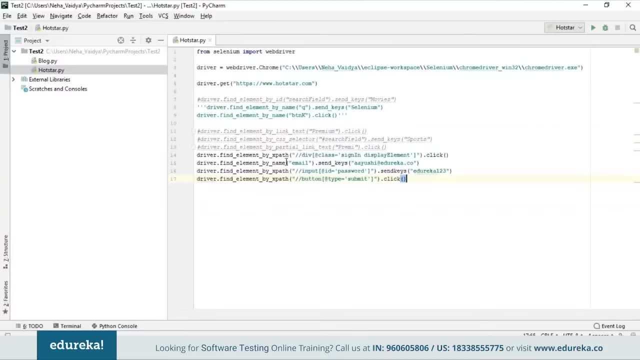 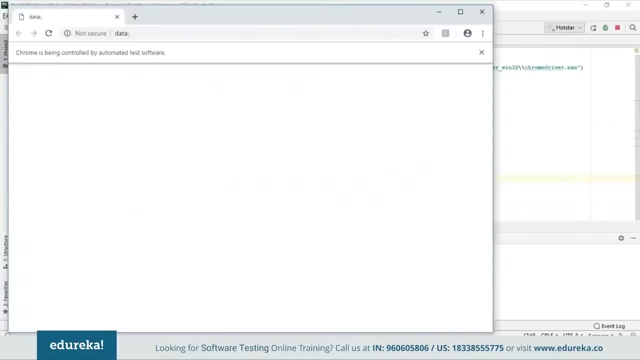 it will first click on the login icon, then enter the value for your email and password. After that it will click on the login button. Now let's run the program and check the output. So when I execute the program, you can see it navigated through hotstarcom. 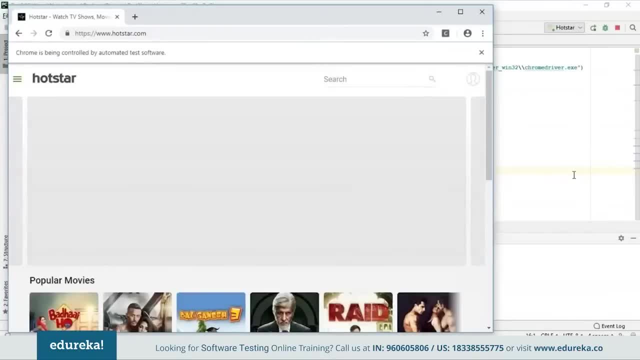 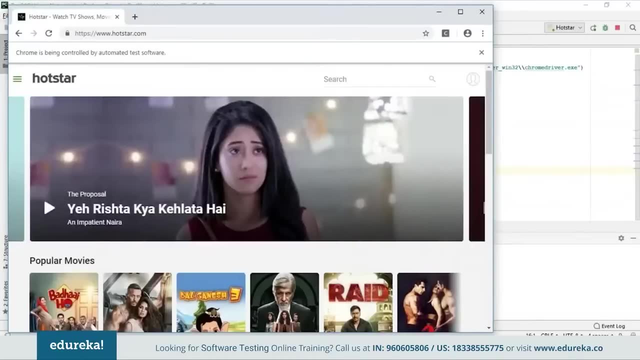 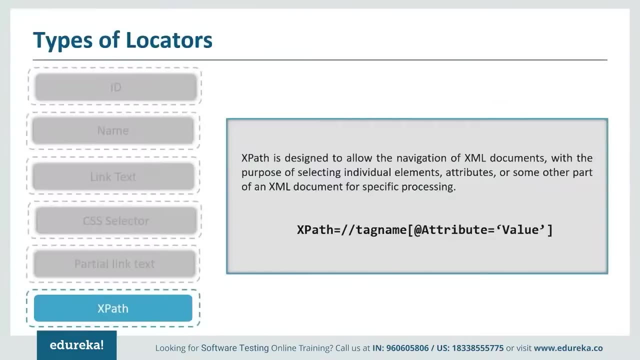 clicked on login, entered email address and password and clicked on login button- clear. much simple, right. So that's how it works. So this is all about XPath and various types of locators. Now what is a preference for the locators? So basically, ID is given the first preference. 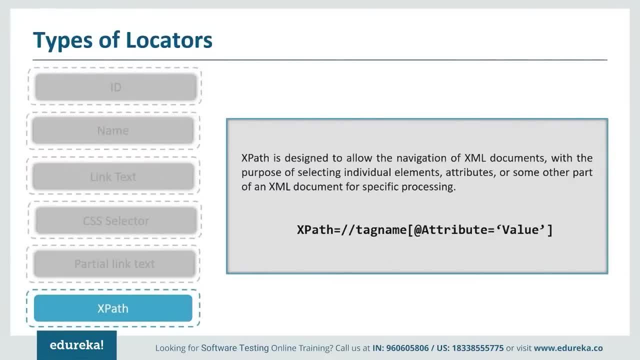 because it is unique, even name as well, because even that is also considered as an unique locator. next, XPath and CSS selectors are given the second preference. Why? Because in some complex situations where ID and name are not available, we have to create dynamic XPath. 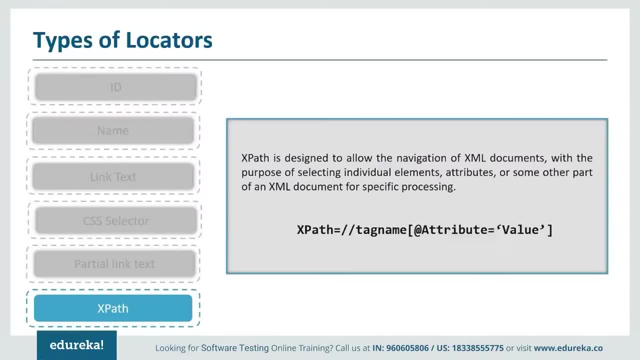 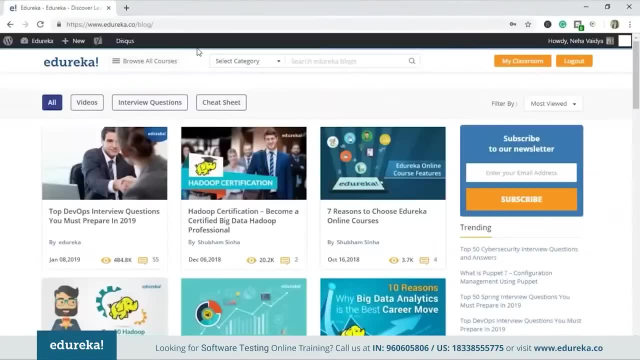 Next link. text is useful only for links, So I will give the third preference and partial links as my fourth preference. Now let's do one thing. Let's navigate through edureka blog page and perform some actions on it. So I wish to search the blogs for Python. 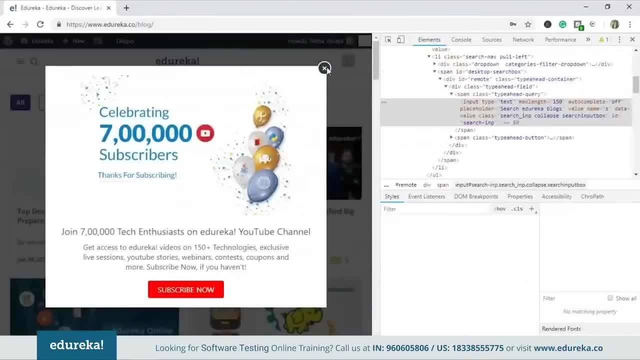 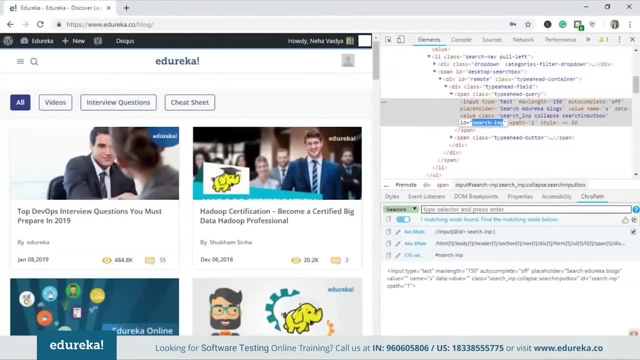 So what I'll do? I'll inspect this page and I will write it using CSS selector, because it has an ID attribute whose value is search input. So I'll just copy that and I will write the code like this. So first, basically, I will import the web driver. 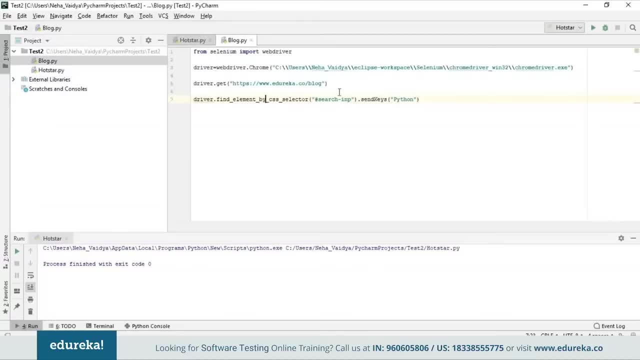 I launch Google Chrome and then I will use the driver dot get and launch the link that is edureka blog and then, using CSS selectors, I'll use the search input. I'll give the value of CSS selector as search input and send keys as Python. 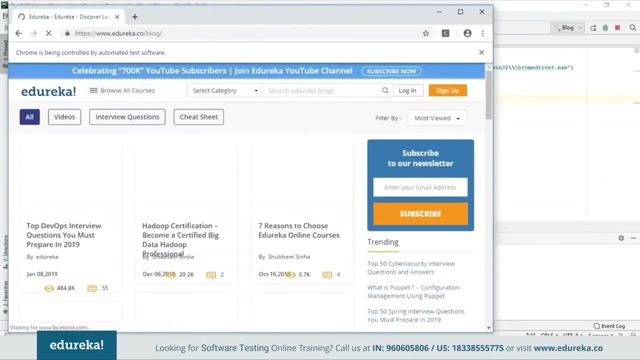 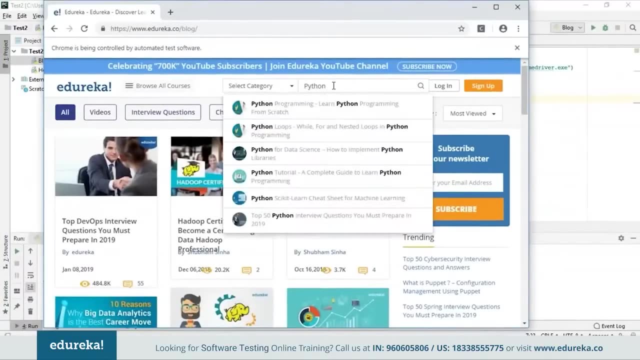 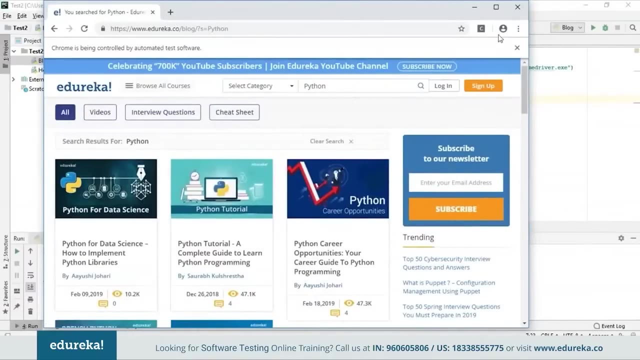 Now let's run the program and check for the output. So you can see, it launched edureka blog page and it entered the value as Python. So you can see there are so many blogs for Python, There are videos, There are interview questions, Etc. 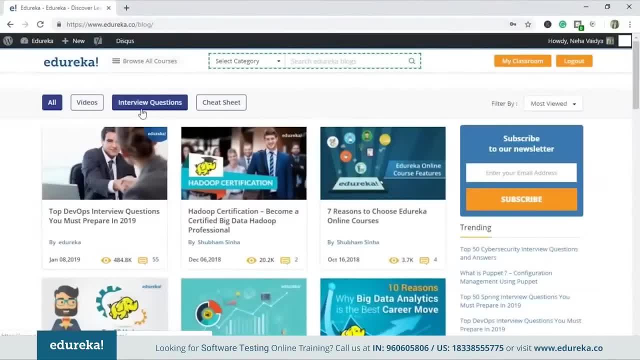 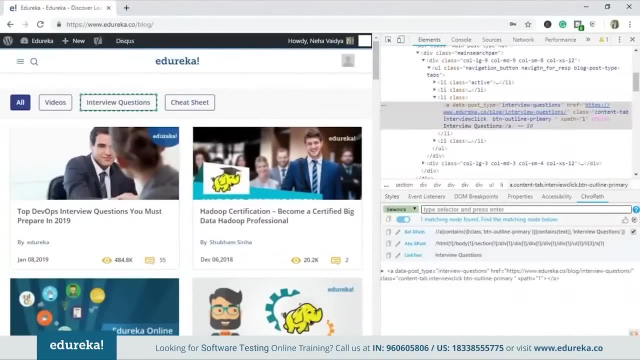 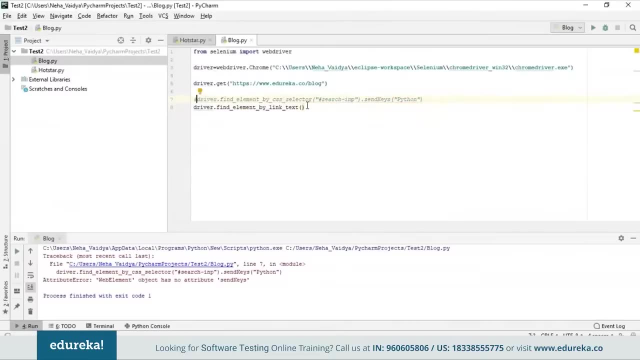 Next, what I want to do is I want to click on this interview questions link. So I'll just click on inspect, I'll copy the link text- that is interview questions, and I'll go back and write the code Dot click. Let's run the program. 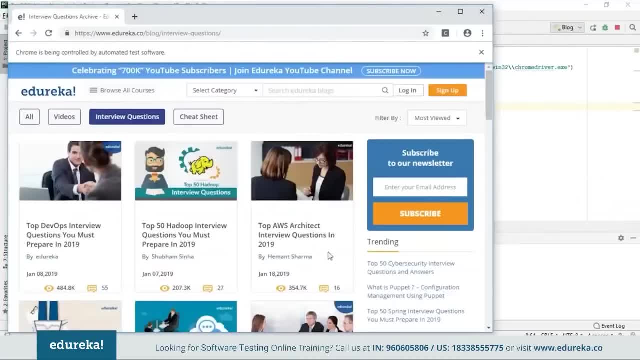 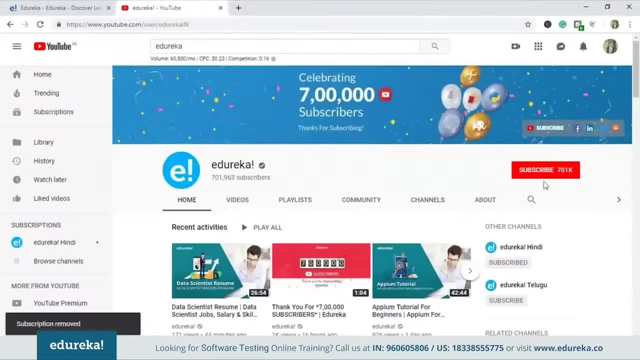 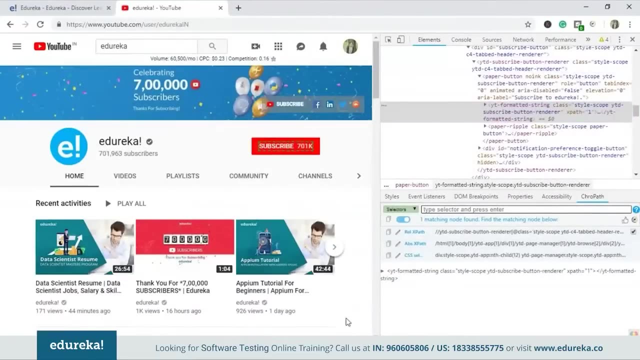 So you can see it, clicked on interview questions and you can find many of the interview questions for your preparations. if you wish to Now say I want to subscribe on this edureka channel, So what will I do? I'll just inspect this and I will copy the XPath for that. 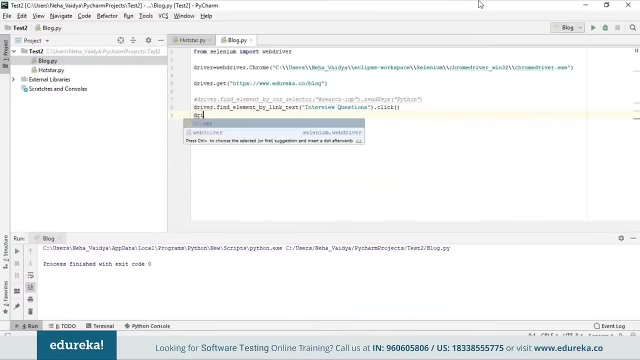 Go back to my PyCharm, Write it by XPath dot click. Okay, So as this is a very complex XPath query, So with the help of grow path, it's very simple for us to find the XPath, or else manually writing such a big XPath. 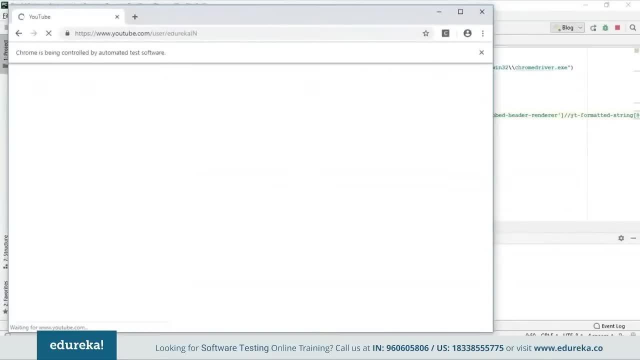 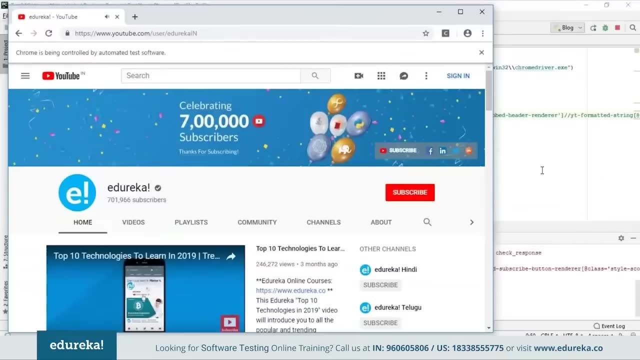 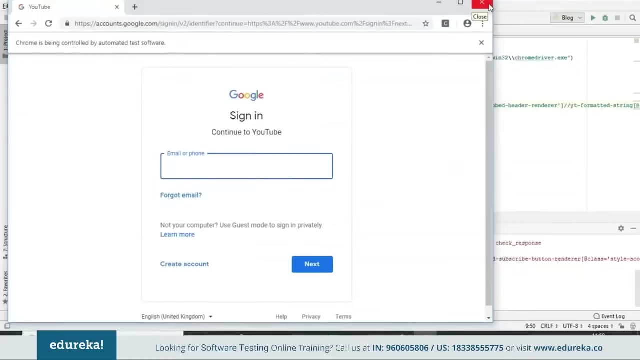 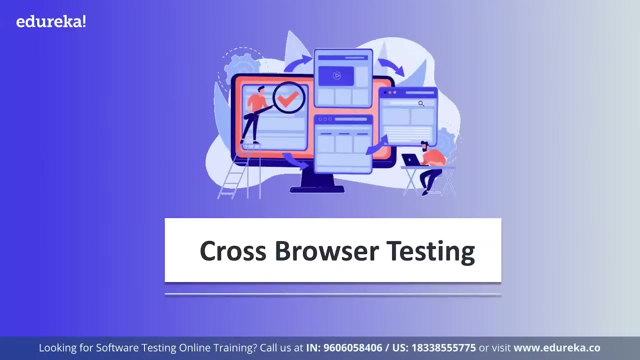 is very complicated. So you can see it launched, edureka website and it will now click on the subscribe button. Yes, I want to, So next I can proceed further with my email address, everything Okay, so that's how it works. First I will talk about what is cross browser compatibility. 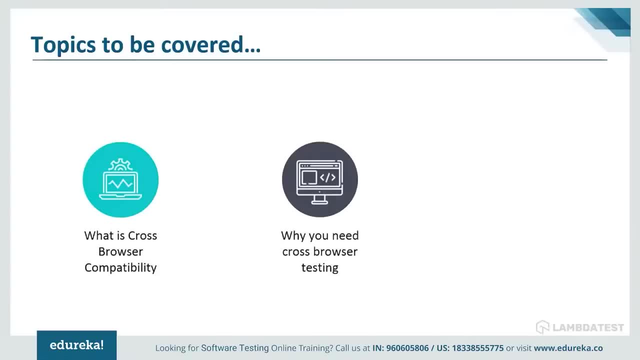 and next I will tell you why do you need cross browser testing, and after that we will be seeing how it works. in order to understand working of cross browser testing, I will demonstrate one of the useful tool that is lambda test, and showcase the demo on cross browser testing. 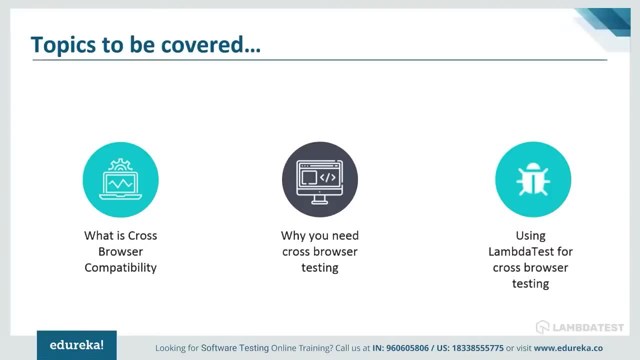 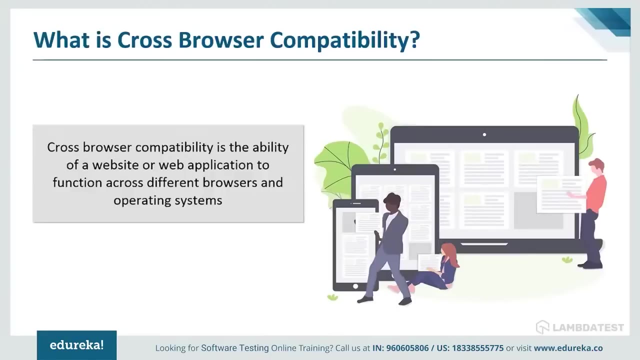 I hope you like the agenda. So before I move ahead, can I get a quick confirmation as whether I'm audible or not? So all right, let's get started. first Let's see What is cross browser compatibility. cross browser Compatibility is the ability of a website. 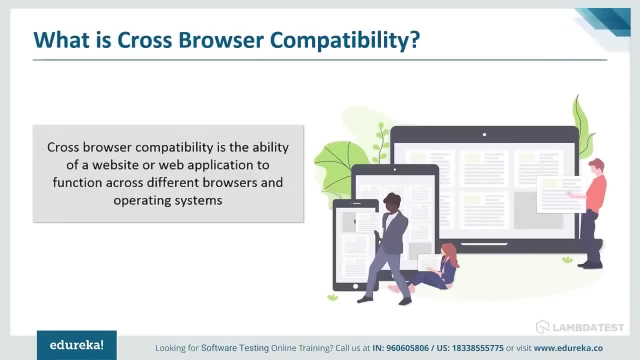 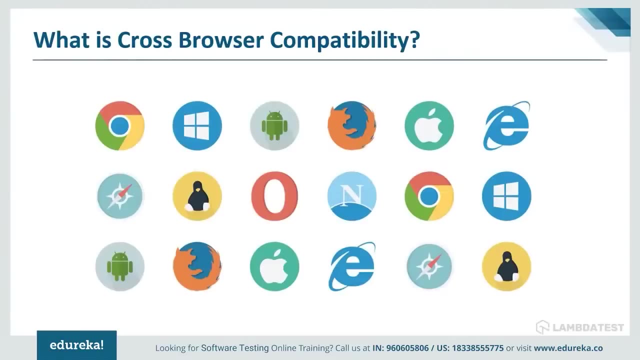 or a web application to function across different browser and operating systems, which means your web applications or website should work absolutely fine across all the browsers Like Chrome, Firefox, Safari, and even across all the operating systems, such as Windows, Mac and iOS, but at times that's not the case. 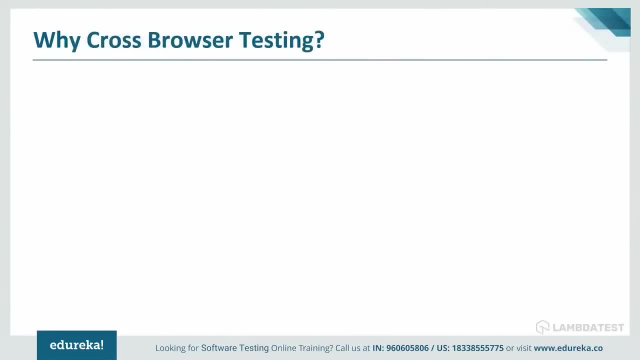 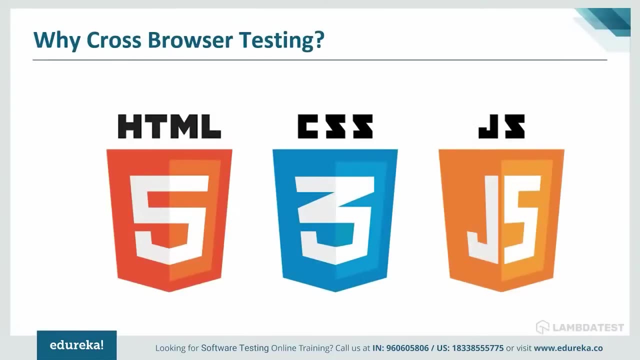 and that's where you need to understand the concept of cross browser testing. So, basically, a simple website is comprised of three major Technologies, that is, HTML, CSS and JavaScript, but there are other hundreds of Technologies that is there in the back end, like you have Python. 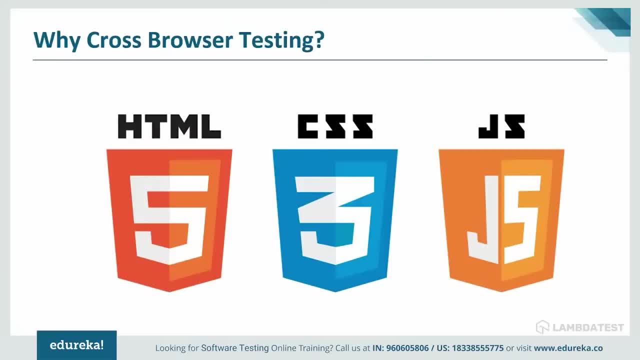 Ruby Note, and these can be used for your back-end work, But overall, in the front end, in the rendering, only these three main Technologies are used. However, each browser use a completely different rendering engine to compute these three Technologies. For example, Chrome use blink, Firefox use Gecko. 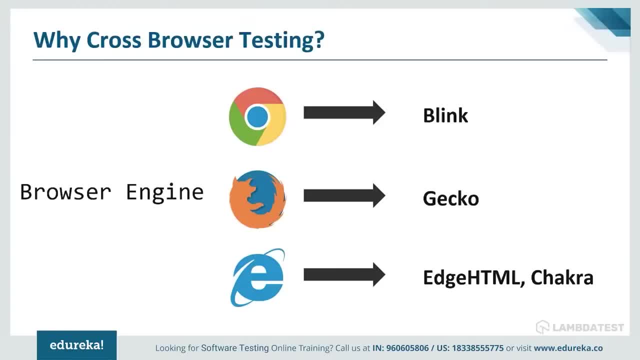 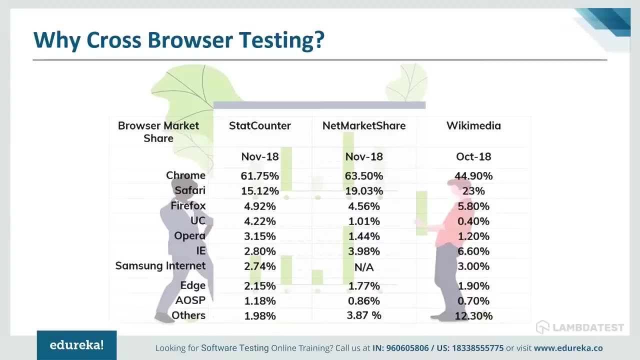 and Internet Explorer use HTML and Chakra, because of which same website would be rendered completely differently by all these different browsers, and that's why you need cross browser testing. So, in order to get a better perspective, Let's look at the stats here. Chrome is 61% popular. 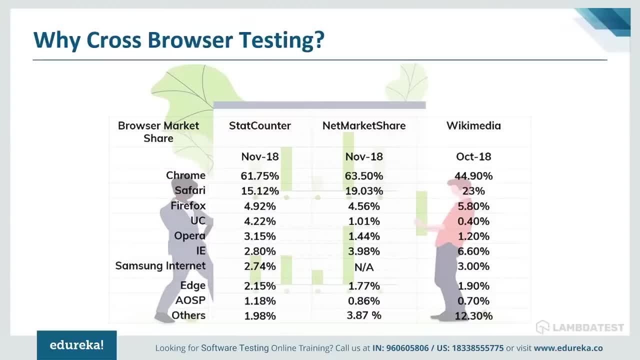 and its market share is 63.50%, which is the highest value when compared to other browsers, Whereas Safari owns about 19% of the market share, and other browsers have much less market share than these browsers. So now let's have a look at the data. 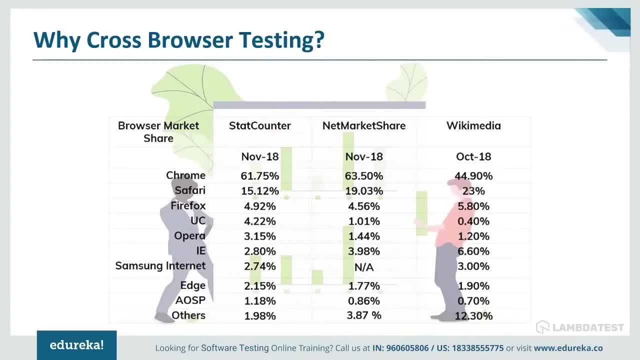 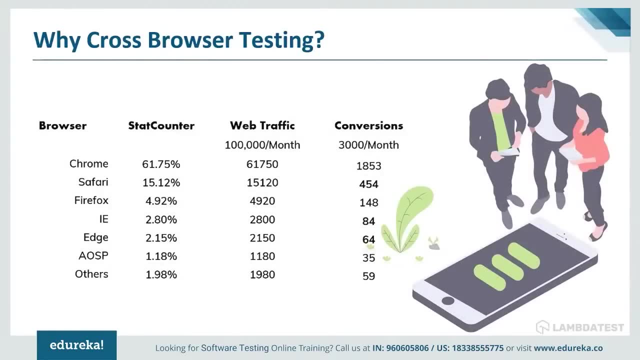 that is related to traffic that you get on these browsers. Now, let's say you get a web traffic of around hundred thousand people a month. considering 15% of the people use Safari, then only 454 people will be the paying customers for you in this month. 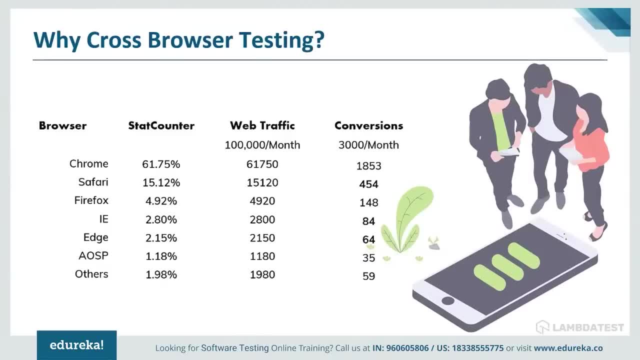 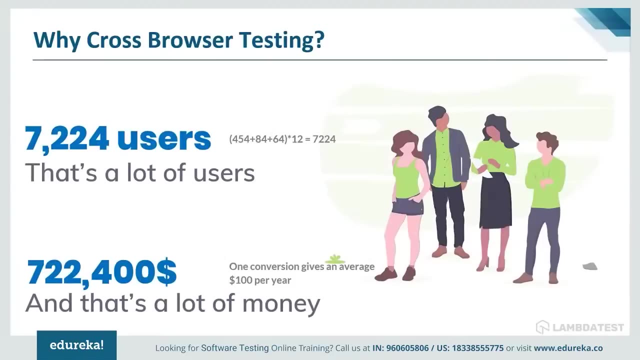 Now, if you sum up Safari, Edge and Internet Explorer, then the total number of people that will be paying for you will be 454 plus 84 plus 64. So if you have not tested your website on all the other browsers, then you would be losing around 7224 customers a year. 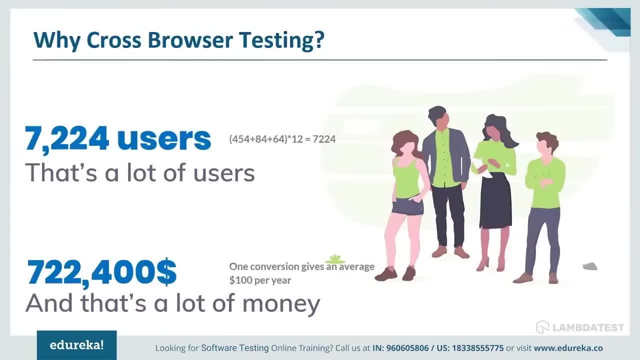 And if you can say that one customer will give you hundred dollars a year, then you would be losing around 722 thousand four hundred dollars a year, and that's a lot of money. and that's because your website is not functioning fine in all the three different browsers. 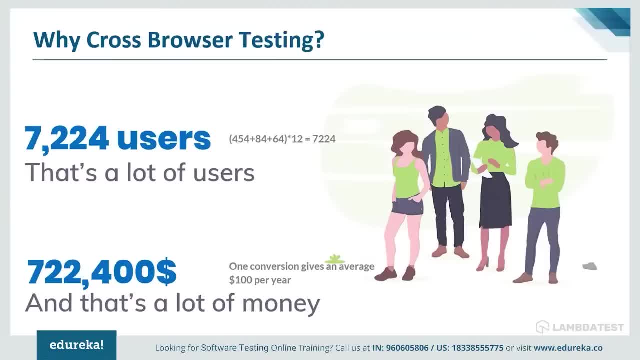 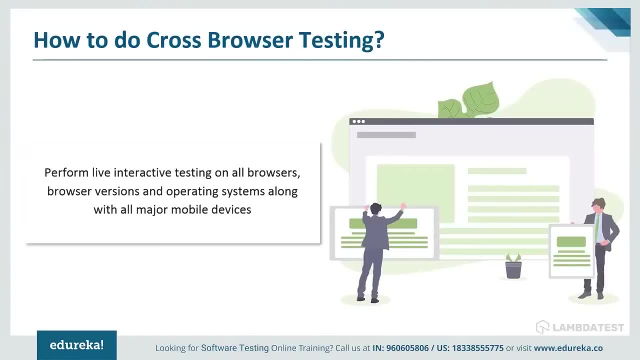 and that is exactly why you need cross browser testing. Now the next question that pops up is how to perform cross browser testing. So it is performed with live interaction testing on all browsers, browser versions and the operating systems, along with all the major mobile devices. 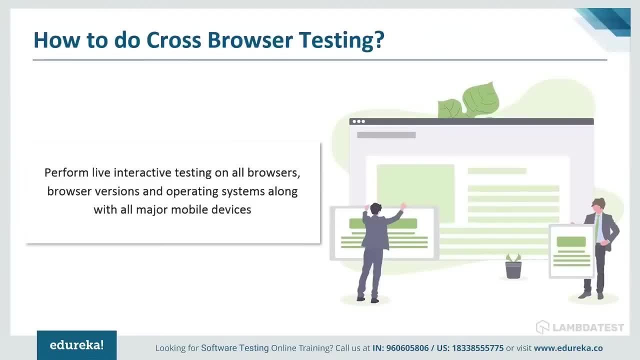 So it is basically done with two methods. that is, manual as well as automated way. It is performed with live interactions on all browsers, browser versions and operating systems, along with all the major mobile devices. It is basically done with two methods. that is, manual as well as automated way. 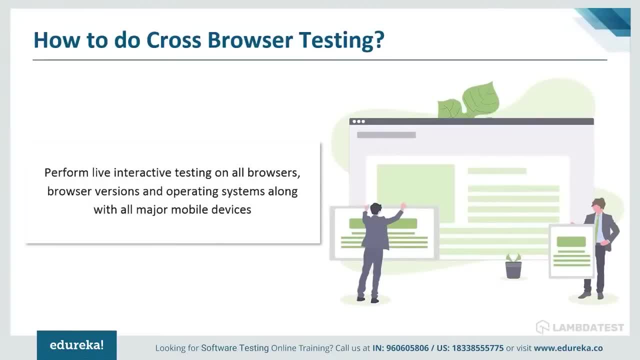 So first manual method- in this case a business identifies the browsers that the application must support. testers then rerun the same test cases using different browsers and observe the applications behavior and report bugs If there are any. in this type of testing it is not possible to cover many browsers. 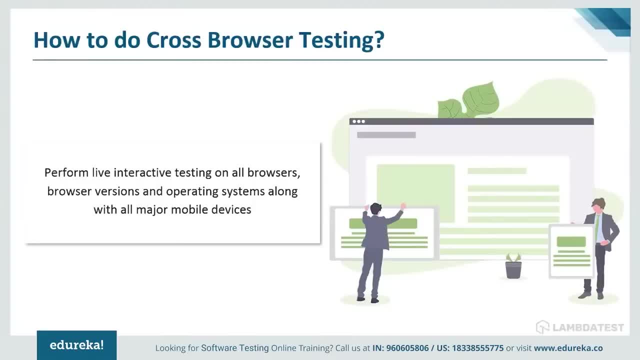 and also the application might not be tested on major browser versions. Also, performing cross browser check manually is costly and time-consuming. to next talking about the automated way, cross browser testing is basically running the same set of test cases multiple times on different browsers, So this type of repeated task is best suited for automation. 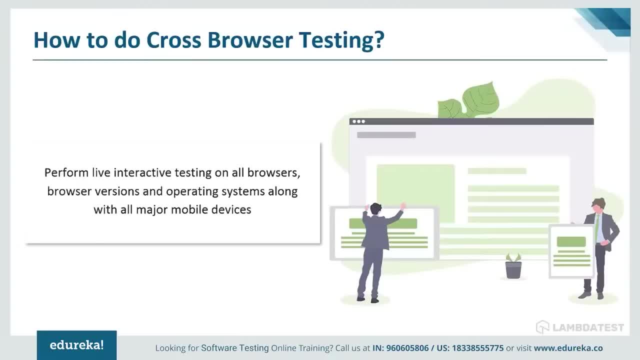 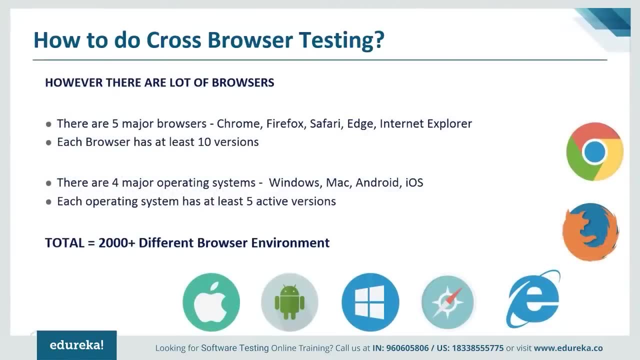 Thus it is more costly and time-effective to perform this type of testing by using tools. But again, there's a challenge over here. That is, there are lots of browsers. commonly used ones are Chrome, Firefox, Safari, Internet Explorer, Edge, Etc. And again, each browser have at least 10 versions. 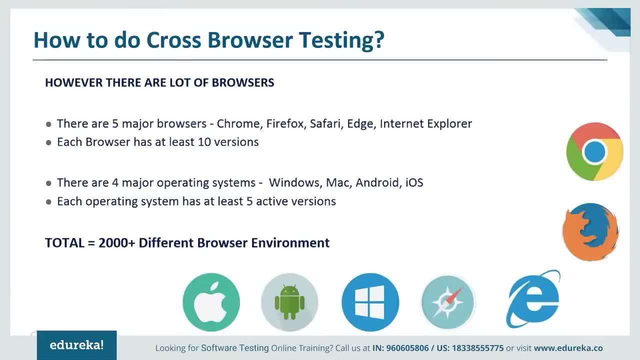 like Chrome, have Chrome 72, 70, 68 and so on. Also, there are four main operating systems and they have again five versions. like Windows, have Windows 98, XP, Windows 7, 8 and Windows 10.. So in total, there are more than 2000 browser environment. 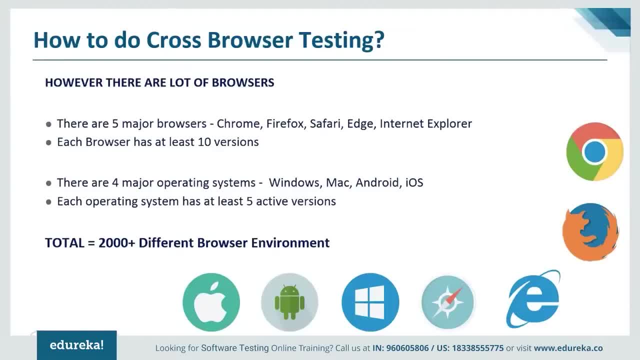 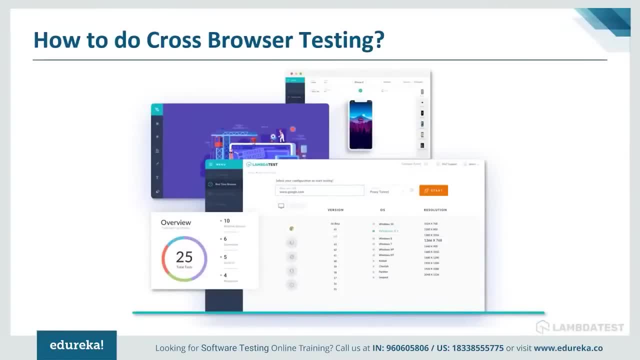 However, collecting a browser and browser environment is a challenge for anyone, and that's where lambda test comes in. lambda testing is a cloud-based cross testing platform. It is one of the amazing tool for cross browser testing. What basically was done was lambda test collected all the browsers, browser versions, operating system types. 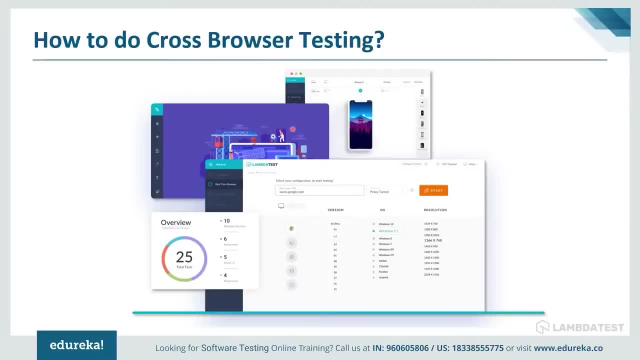 and its versions and created machines out of them. After that, they collected all those machines and deployed under a cloud-based platform. So if you want to test a website or a web app on a specific configuration that you don't have access to, lambda test gives you a solution. 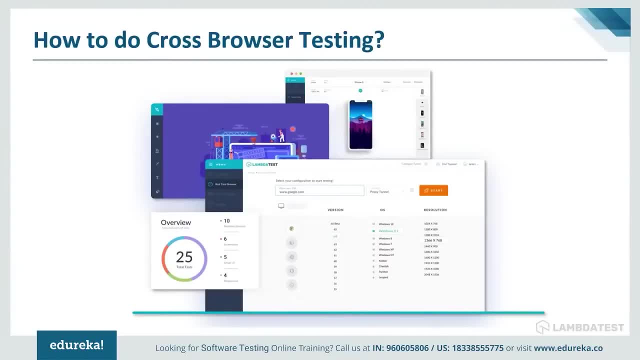 You just have to log into lambda test, enter the URL of the website that you wish to test and start off the session where you can test the website for browser compatibility issues. Now let's have a look at the demo, where you will understand how actually this lambda test works. 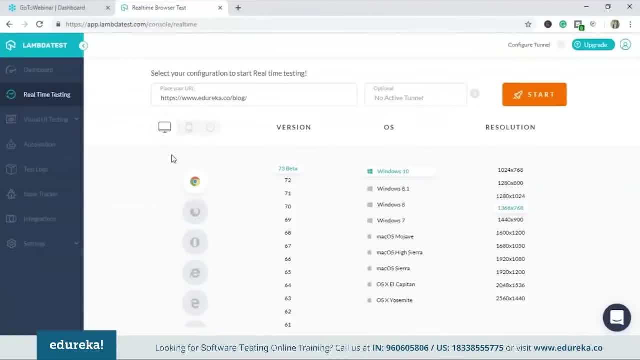 So this is a lambda test platform to see how real-time testing looks like. So real-time testing is a feature that gives you a live interaction, testing of a website or a web application. So there's a dashboard, There's a real-time testing. 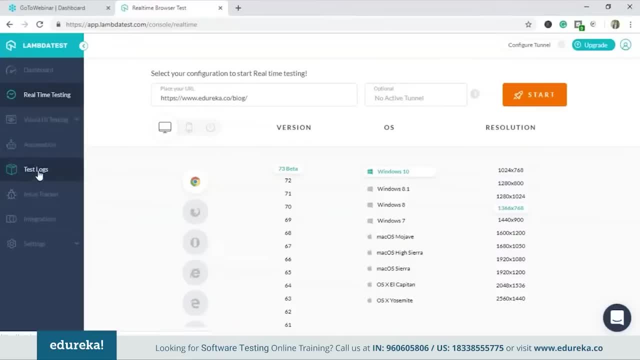 There's a visual UI testing automation. You can log your test records over here and if you have any bug, you can track it with this issue tracker. There are integrations and settings as well. Now I will tell you how to perform lambda testing of a website on this particular lambda test platform. 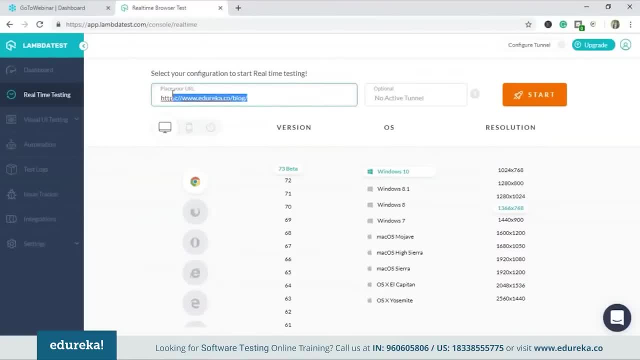 So I have placed a URL of edureka blog website and I will do one thing. I'll choose Chrome, say I want to run it on 72, or say 73, the latest version of Chrome, and I want to run it on operating system That is, Windows 10.. 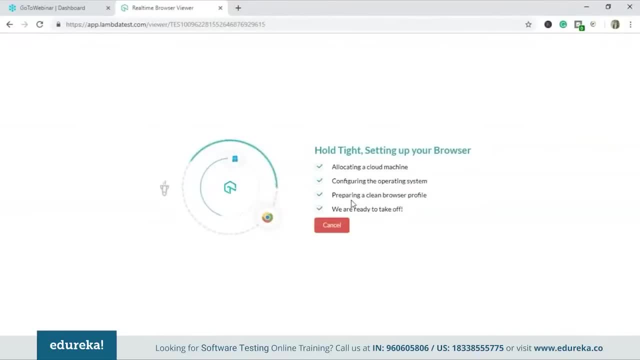 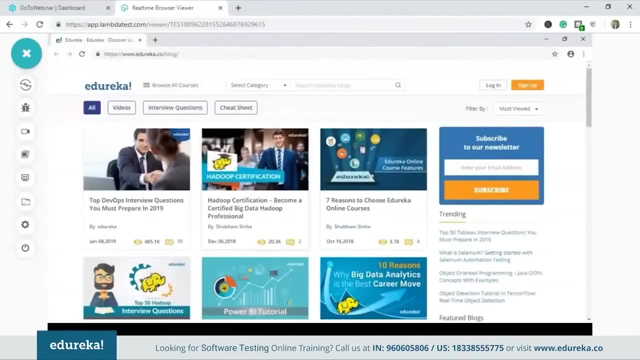 So now what I'll do. I'll start this test. So first, what happened? it allocated a cloud machine, configure the operating system, preparing a clean browser profile, and then we are ready to take off. So you can see here that edureka blog website was launched, suppose. 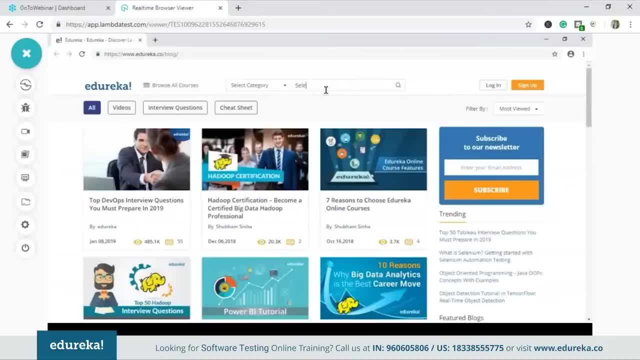 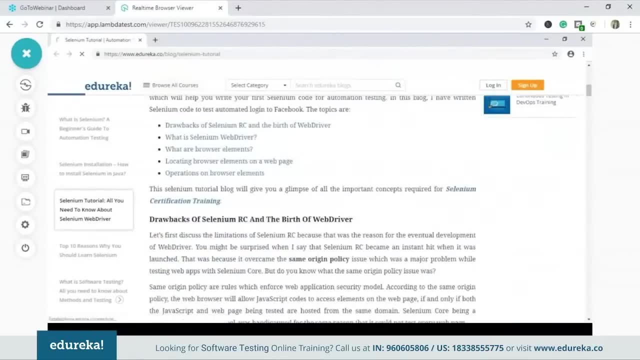 say, I want to search for selenium blocks, I'll just write selenium and choose whatever the blocks I want. and I can read the following blog and I can also browse all the courses like devops, big data, data scientists and everything. I can go back. there's BI and visualization. 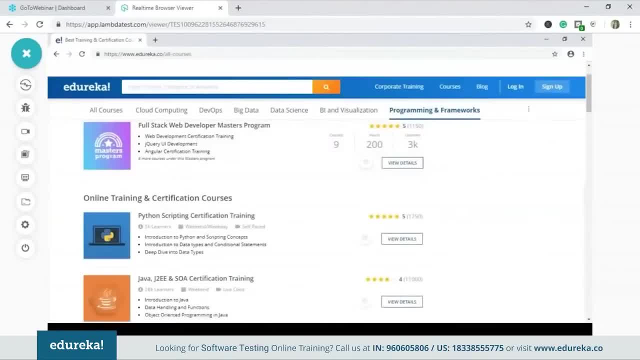 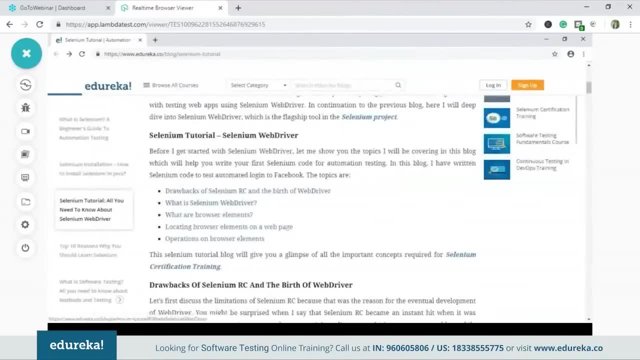 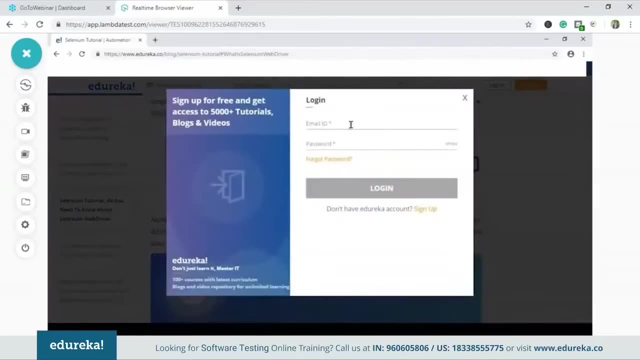 There is programming and frameworks, like you have Python scripting, Java training, You have cloud computing, Etc. Also, I can click on this hyperlink to know what is selenium web driver. I can log in. if I have the credentials to log in, I can close this. 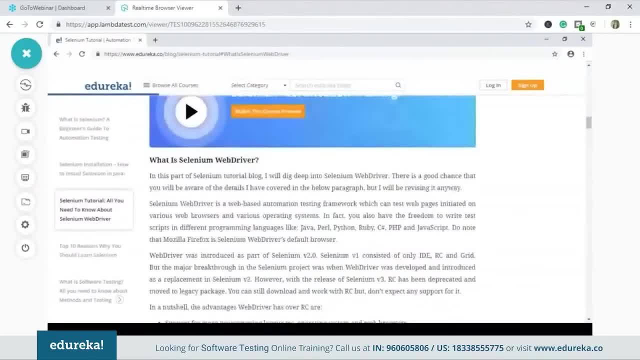 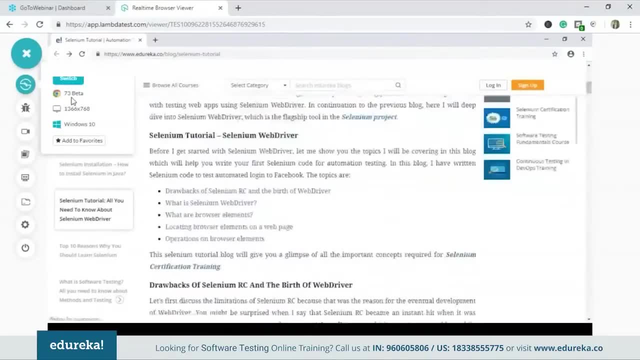 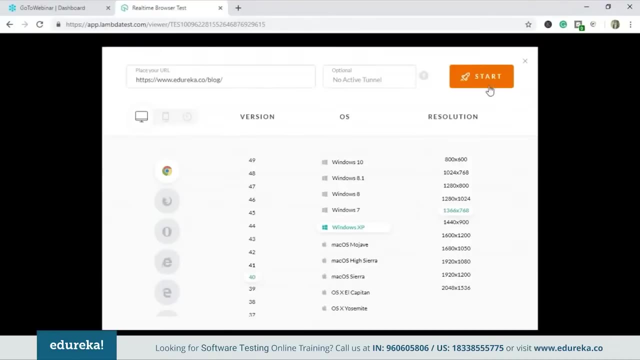 So basically, on Google Chrome version 73 and on Windows 10 platform, My website is functioning perfectly fine. Now let's do one thing. now say I want to perform the cross browser testing on Windows XP, on Chrome version 40. I'll start the test. 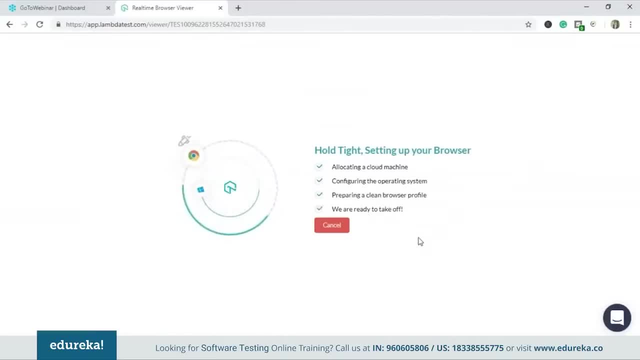 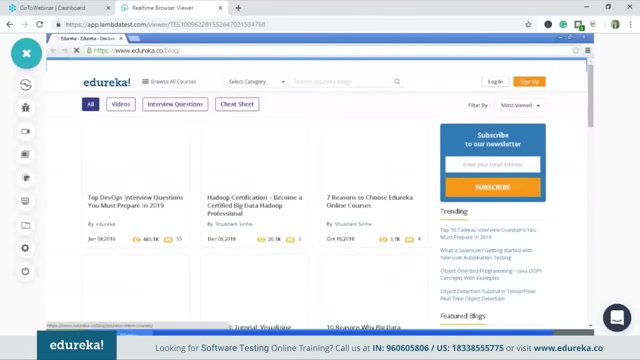 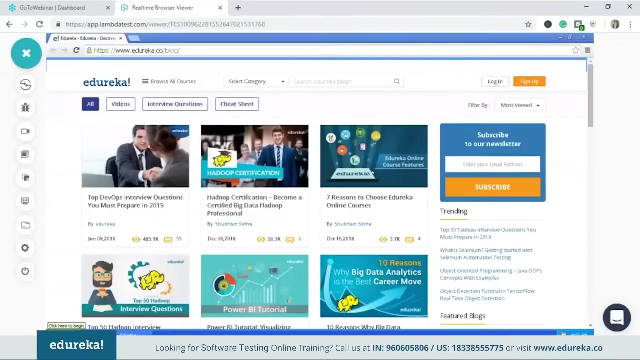 So it started allocating a machine and then following the next steps. Let's wait So you can see the older Chrome version how it looks like. So here you can see this tab. the down one shows It is Windows XP and this is the older version of Chrome. 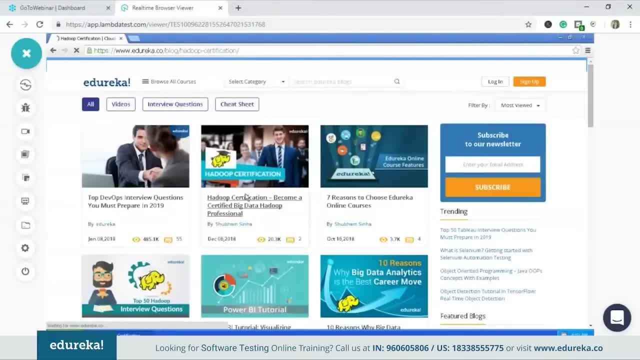 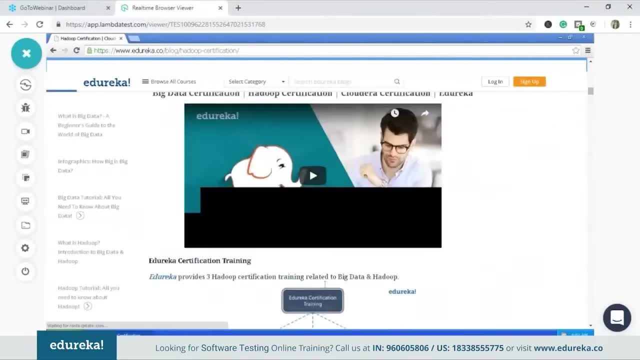 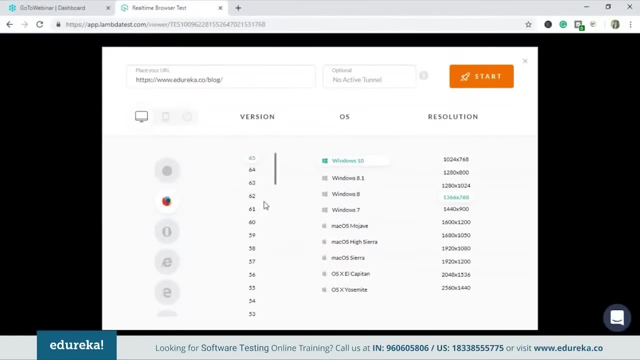 Yes, again, I can carry out all the same actions, like I can click on this particular blog and I can read this blog and many more things. So now I want to perform a cross browser testing on Mozilla version 60.. No, no, let me take up older version. 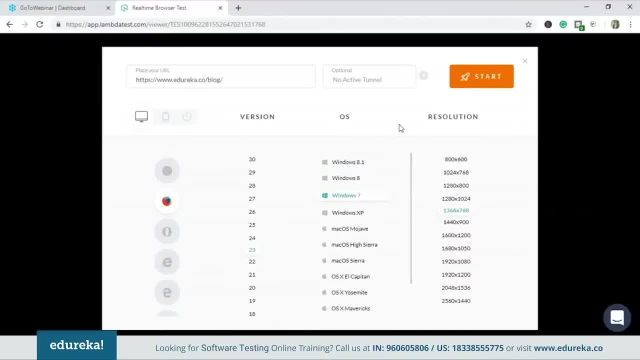 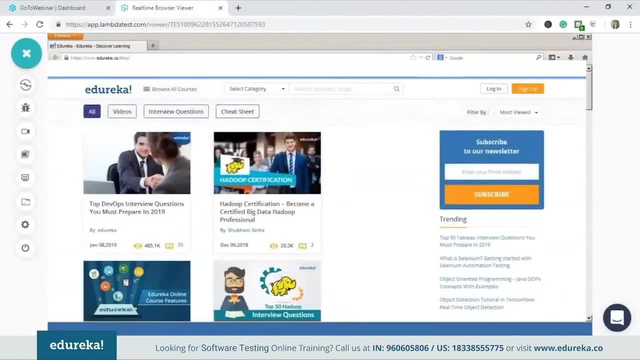 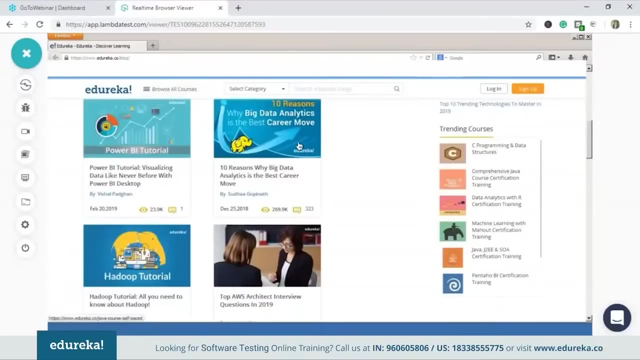 and I want to perform it on Windows 7.. Yes, let's start. So you can see here, This is older version of Mozilla on Windows 7. Platform. so I can choose a trending courses. I can click on login. I can search for the blogs. 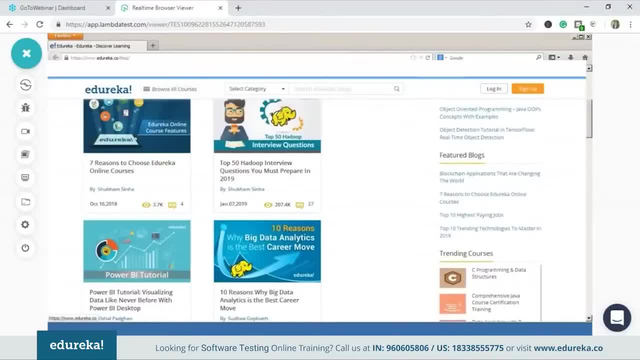 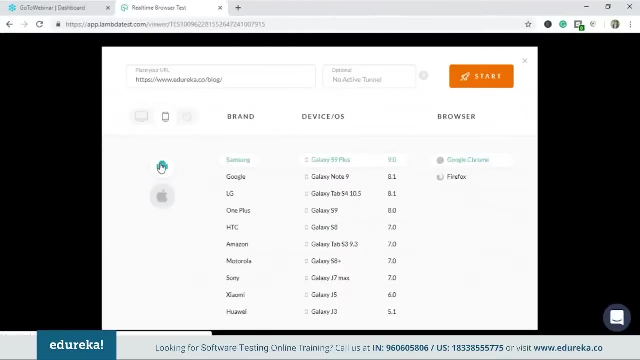 So even on the oldest Firefox version on Windows 7 platform, My website is functioning perfectly fine. That means it is compatible with even this version as well. Now I want to perform it on a mobile website, So I want to use Android and I want to use Sony experience. 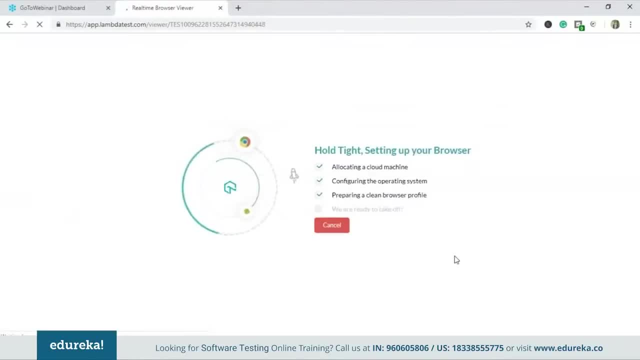 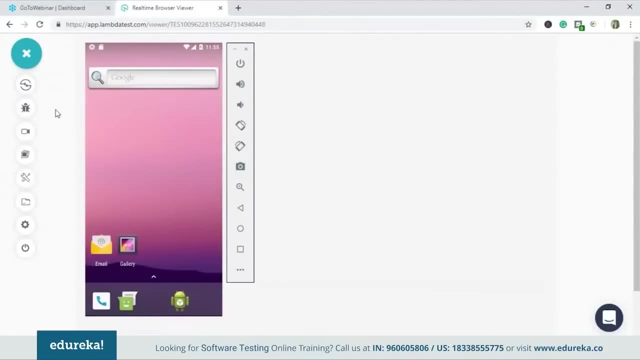 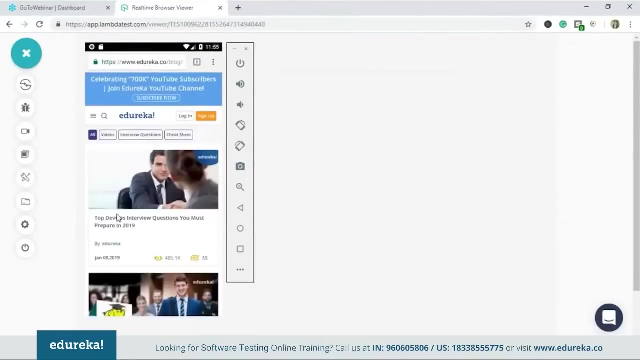 Sony Xperia on Google Chrome. Now let's see how it works. So basically this is the Xperia version. So it got redirected to Eureka blog website, Say: I want to click on the DevOps interview questions and you can see the whole thing. 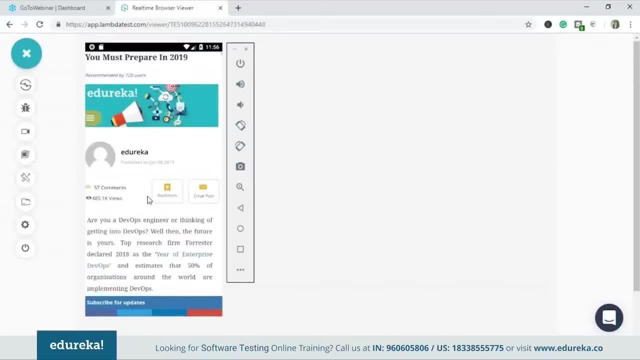 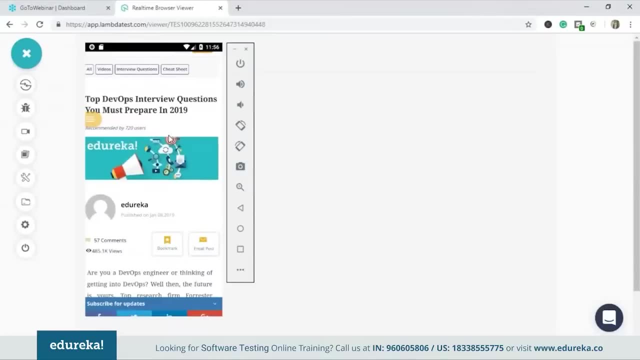 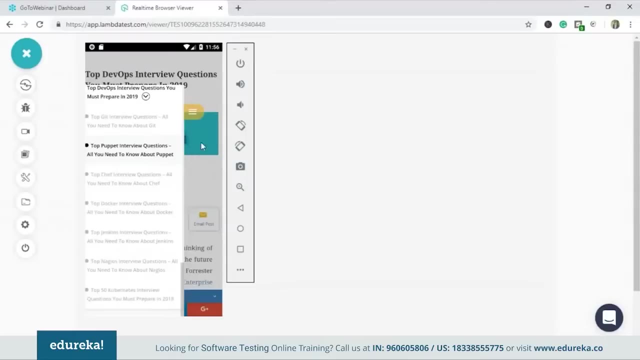 even on mobile platform as well, It's functioning perfectly fine. That means my website Is compatible with even mobile operating system as well. Yes, I can even click on this link and check for the latest blogs. I can read the particular blog as well. 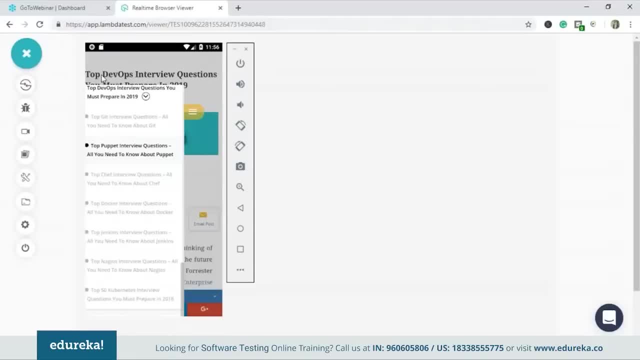 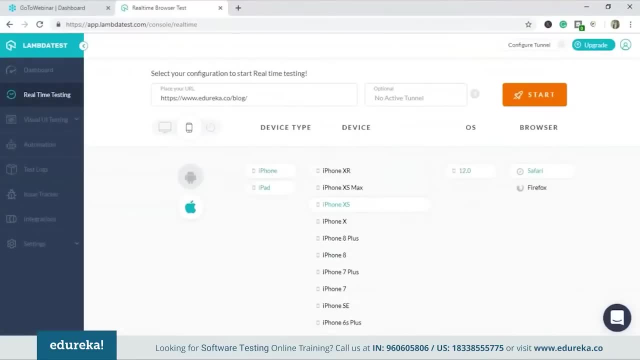 There's a screenshot option as well. It's nothing, but I'm operating on a mobile screen. That's all now say. I want to check the compatibility of the website on iOS iPhone XS device and I want to work it on operating system 12 and Firefox. 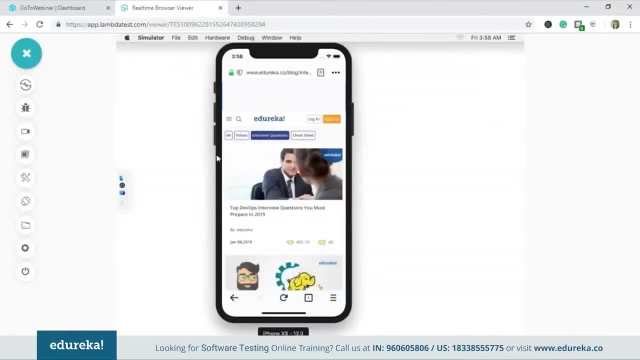 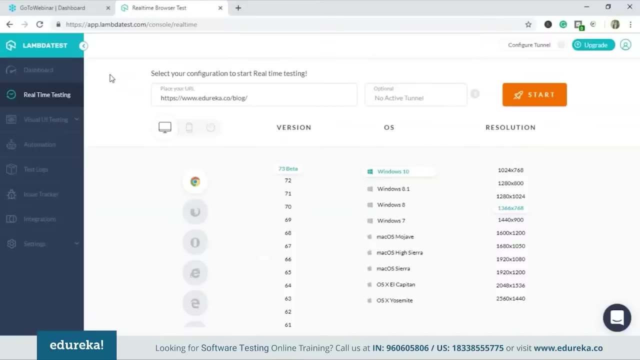 Let's start so you can see. even this is compatible with Apple iPhone as well, and I can click on cheat sheet, I can click on interview questions, I can navigate through videos, Etc. So this is how you can check the cross browser compatibility or perform cross browser testing. 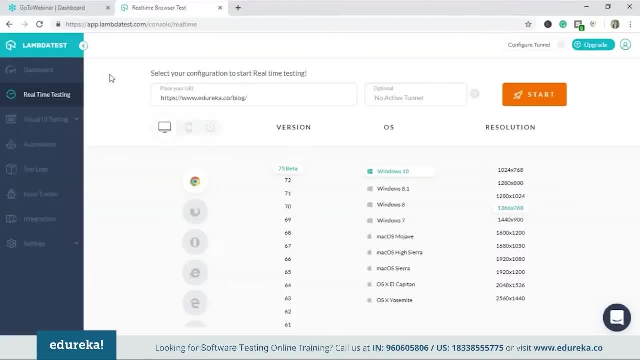 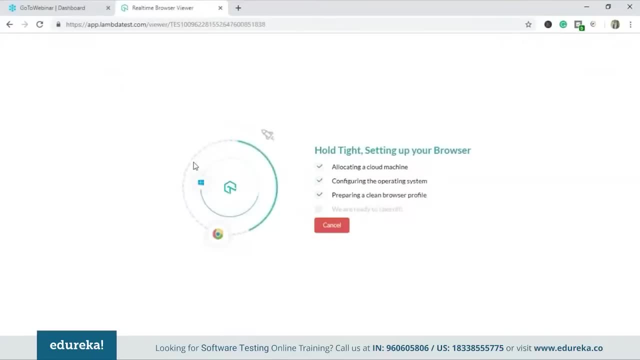 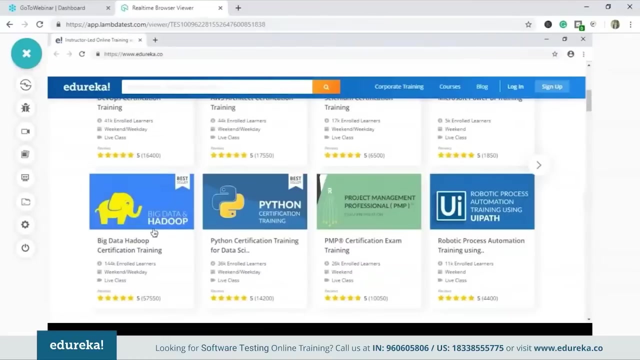 to check whether a particular website is functioning perfectly fine or not. Now, say, I just want to navigate through edurekaco website and check it. Let's see whether it works perfectly fine or not. Yes, even that's working perfectly fine. So this is the latest version of Chrome. 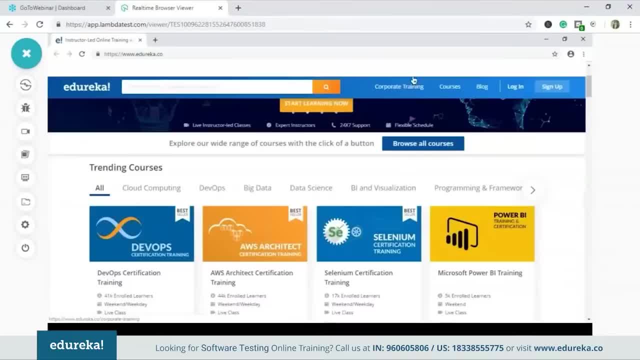 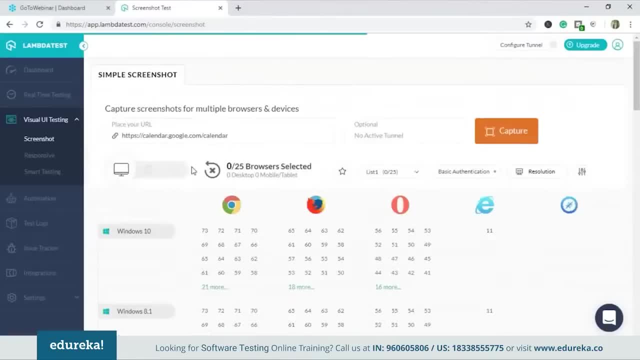 You can see various trainings over here, your blogs, your corporate training, and there's some offer as well. Now, say, I want to take a screenshot, Let's see how. so first I'll place a URL so you can see that there's option for 25 browsers. 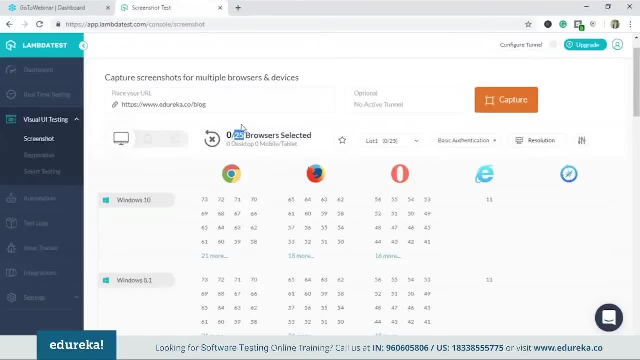 That is, you can take 25 screenshot at one particular instance, like at one shot or at one time. You can take 25 screenshots. So in Windows 10 platform, I'll choose 73.. Yes, and Mozilla, I will choose 61. in Opera, I'll choose 49. 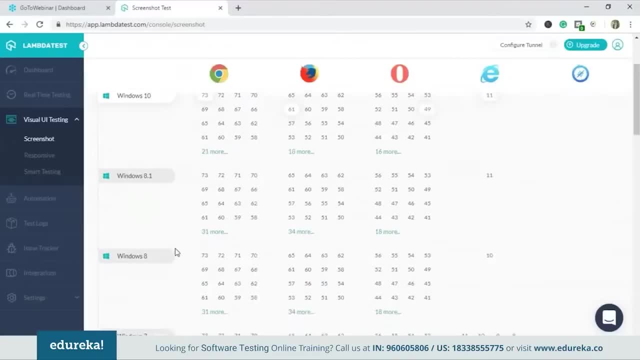 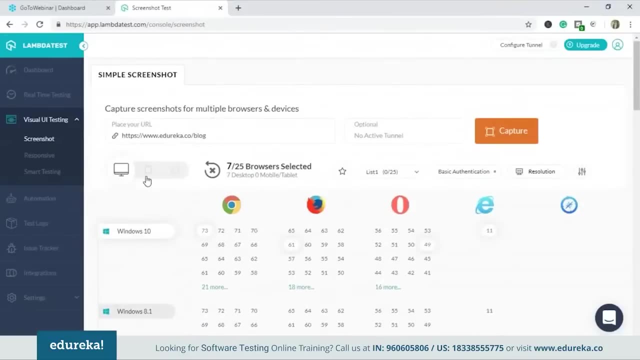 and Edge, I'll choose 11.. Yes, and coming now to Windows 7, I'll choose Chrome 69 and 58.. I'll choose Firefox and 47 Opera, and I'll go to mobile platform: I'll choose iPhone XR. I'll choose iPhone 5s. 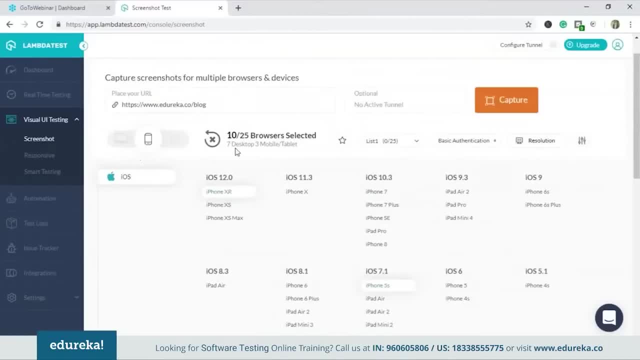 I will choose iPhone 3GS and I'll go to mobile platform. Yes, So I have basically choose 10 options among mobile and website browsers. I'll click on capture, So your test has been added to queue. it's saying so. basically, you can see that the seven desktop. 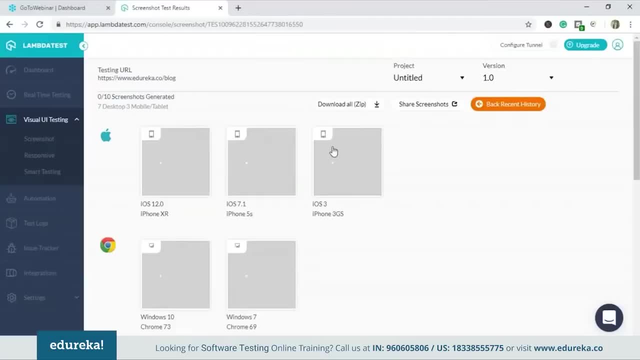 and three mobile options, that is, I have taken 10. So, basically, what you can do is you can compare the screenshots based on different browsers, different operating systems, and check how your website performs and how your website looks in either of the operating systems and browsers, and you can check the compatibility of that. 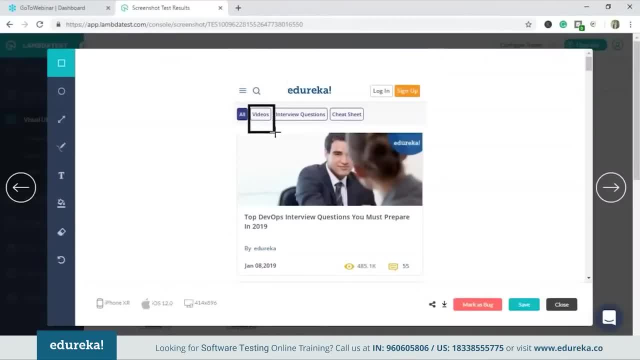 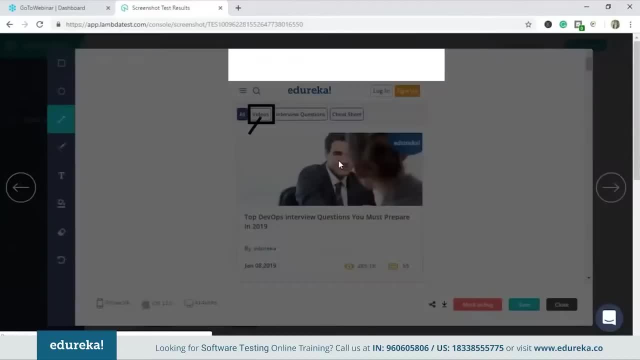 So now suppose in this video there's a bug. So what I'll do? I can just mark it. I can pin 10 arrow and say: mark as a bug. So there are tools like you know: GitHub, Asana, slack, Jira. 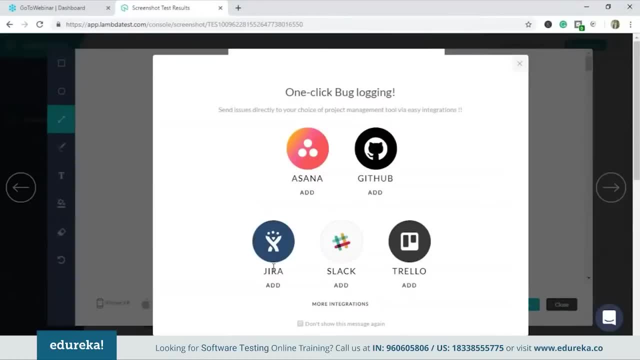 If I want to use for Jira, I'll click on that, I'll choose add. So basically I have to add all the details and generate the token and then install it So you can see the assignee, the type of issue, It's priority, say it's a low and it's summary. 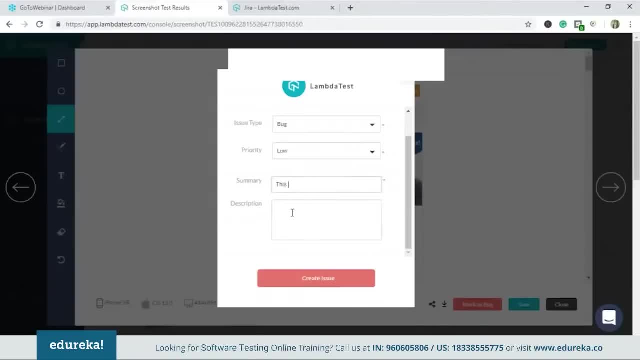 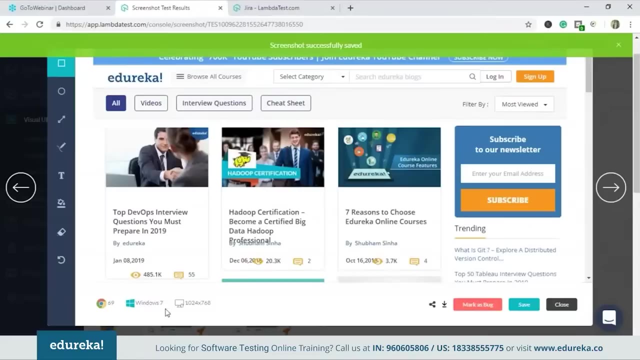 I have to write: this particular button is not functioning. fine, I can give the description and I can just create the issue. See, you can see that bug was marked successfully. If you want, you can save this. So this is all about Windows 7 and Chrome 69 version. 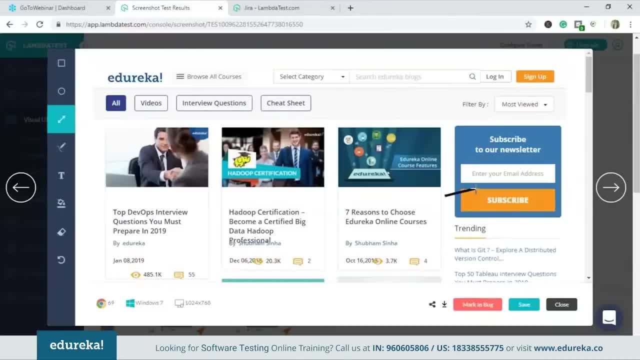 So again, you can do the same thing: mark in saying there's a bug here, You can mark it. You can write the text like text box is not working Right and I can mark it as a bug. if I have to mark it as a bug again, 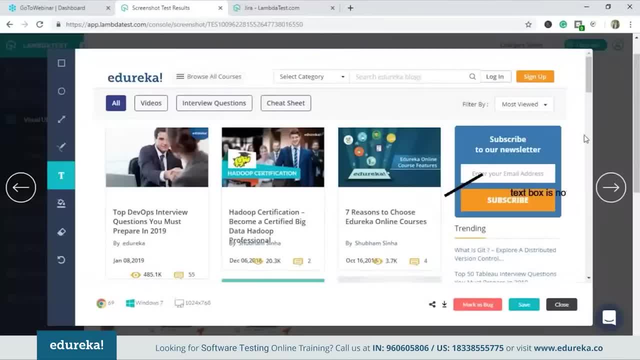 I need to give all the details and then proceed further sounds much simple: right to take the screenshots and compare it, and even if you want to market as well, gets very easy and just one click you can do everything right. So that's why I said lambda test is an amazing. 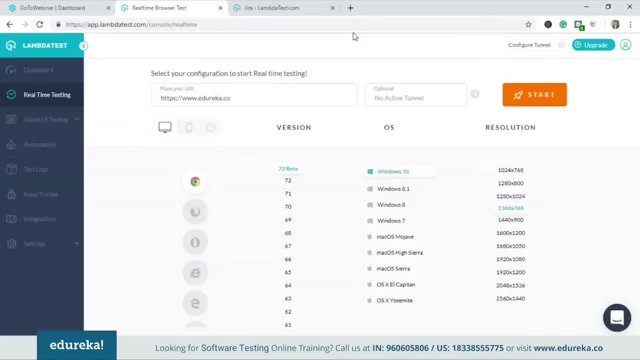 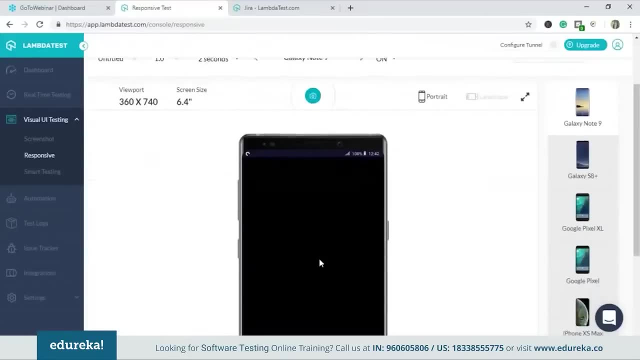 platform to check the compatibility of your website on all the different browser versions and all the operating systems as well, and this if you want to check for the responsive. So I will place the URL and I'll set the size of the monitor and there's a screen size. 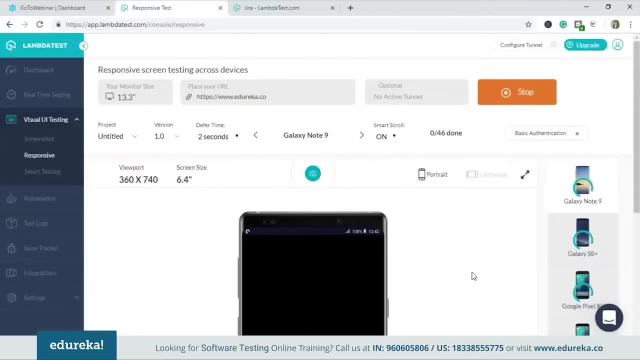 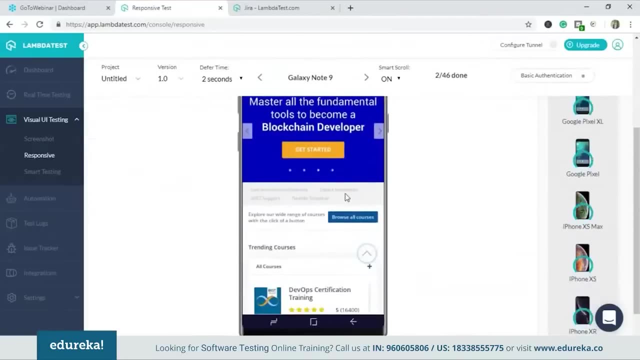 and I'm using which phone? Galaxy Note 9.. So I'll click on generate, so it will generate on this mobile platform. now, Yes, you can see the Edureka website got launched On your Galaxy Note 9 and it's working perfectly fine. 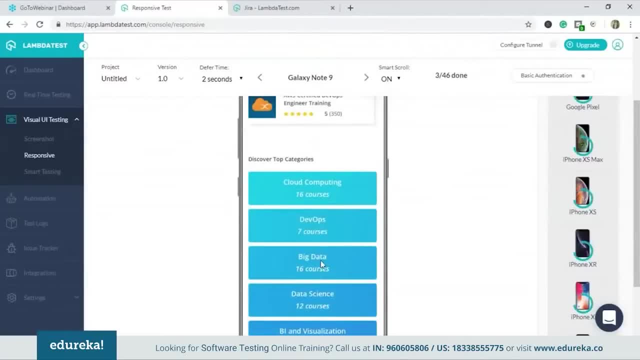 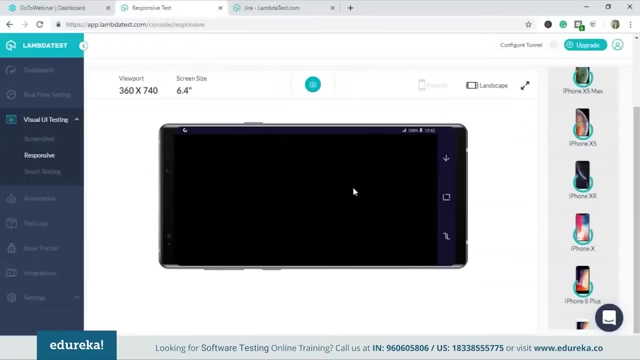 so I can click on the big data courses and I can do many other things as well, right? So if you want to check it in landscape mode, even that is possible. if you want to check it on iPhone X, I just have to click on the particular device. 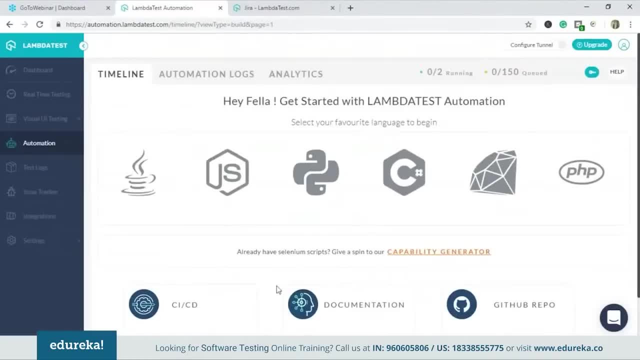 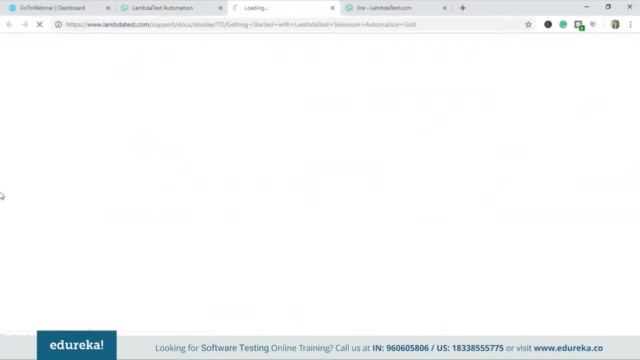 and it will be ready. So you can see, here There is something like timeline. if you want to wish to learn about it, you can click on it and you can go to the help and you can just click on getting started and you will get to know many other things. 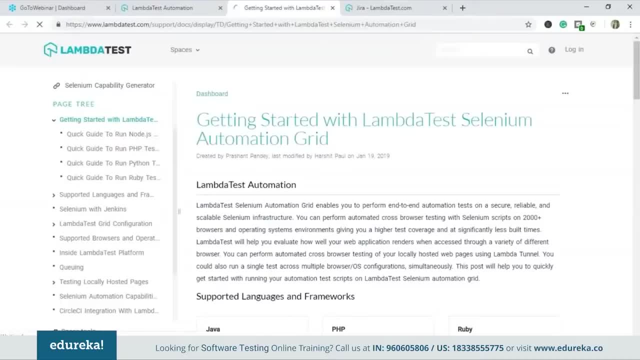 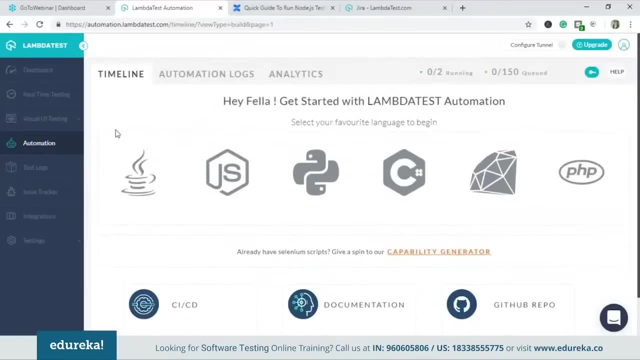 about getting started with Lambda test and any motivation grid. It's basically a free tool. You can click on Java, You can click on CI, CD and everything, and if you want to log any of the tests, then you can log it over here. 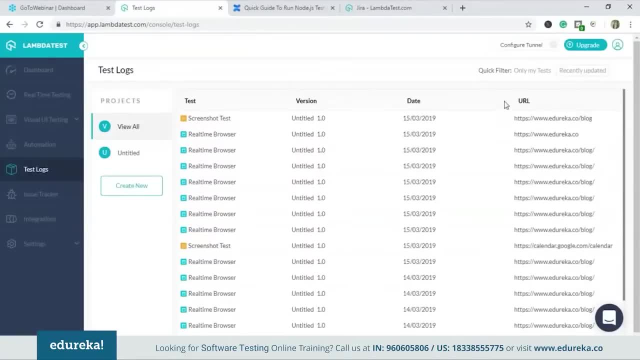 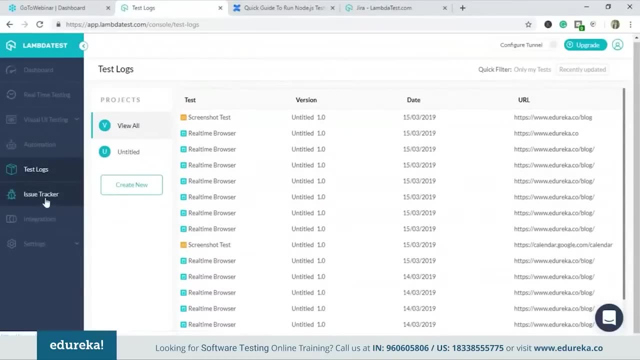 So, basically, before what I did, I took a screenshot test and I logged it, and even I have performed any real-time browser test as well. You can see that we just said in a while and there's a issue tracker. I just said the issue, that is the videos button. 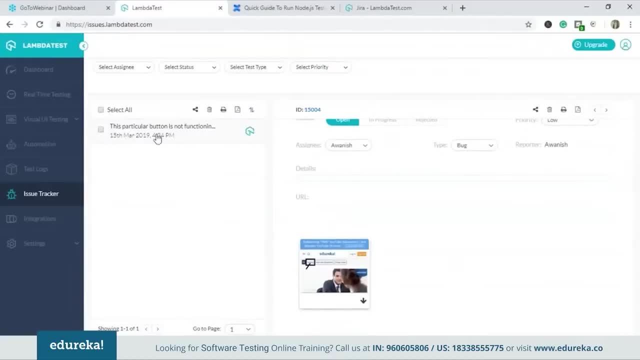 was not functioning So I logged the issue and you can see the date and time of the issue that was logged in the issue tracker. because I have logged the issue and you can see the details at this. priority is low. the reporter, the type of a bug. 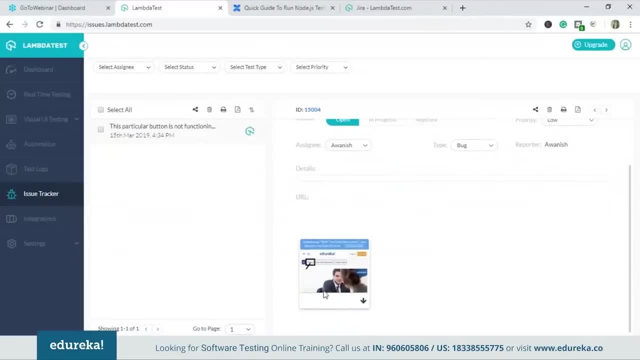 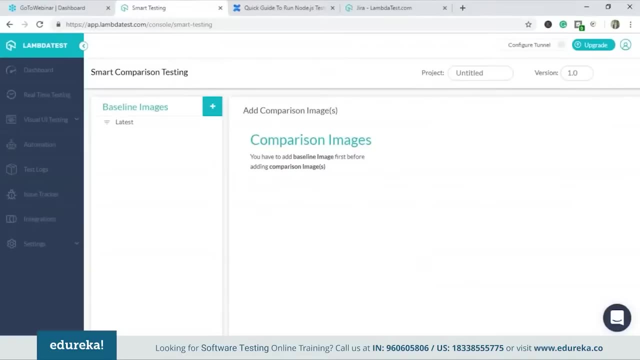 and it's in open state and there's even a screenshot of this, which implies about the bug where I have marked it, So you can add the comparison images here and check on in which browser or in which version of the browser It's functioning perfectly fine. 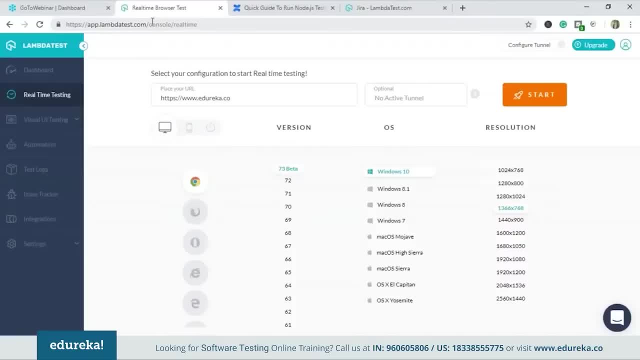 If you wish to take up Lambda test for checking the cross browser compatibility and to perform cross browser testing, then you can take up the light version of this, which is free for you, and you can test it across your platforms, your browsers. You can do many other things as well. 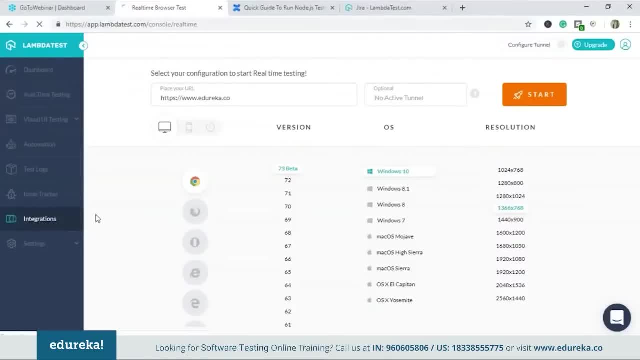 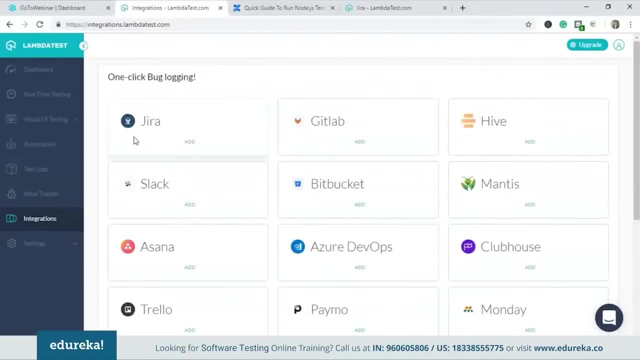 like you can track the issue, You can log the test and many more. So these are the integrations. like we have so many things for WordPress as well, for Chrome extension, plugins for Jira, git lab and many other tools, So I hope you understood. 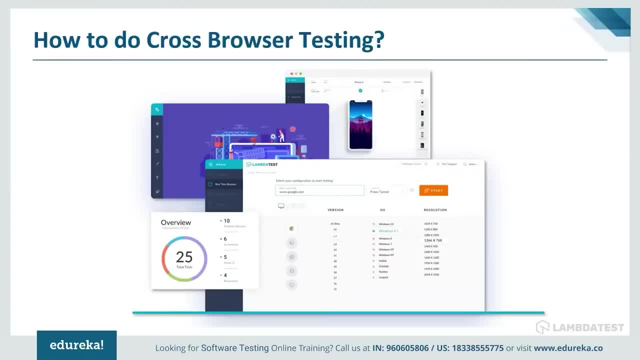 how the cross browser testing works and how to check the compatibility of your website on a particular browser and its version and operating system platform as well, And I hope you also understood how to take the screenshots, how to log a issue and how to mark it as a bug. 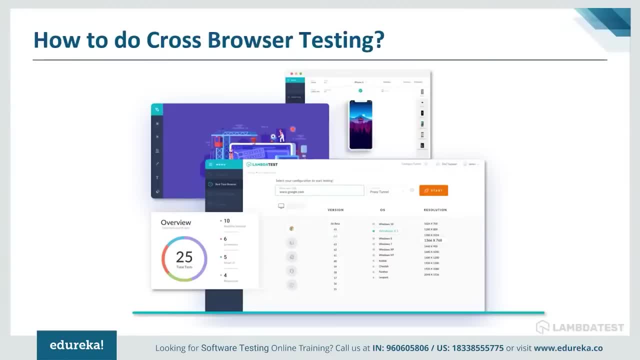 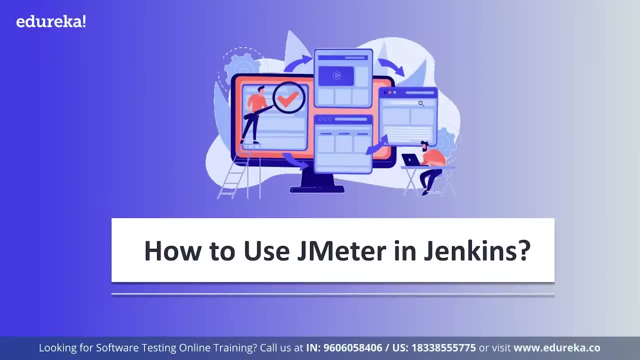 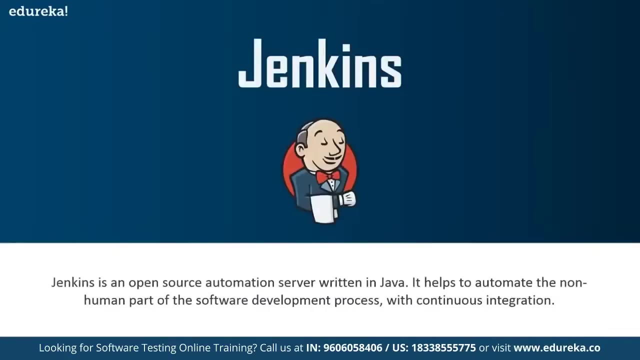 and also how you can take 25 screenshots at a stretch and compare them based on your requirements. And that's all about it. What is Jenkins Now? Jenkins is basically an extensible, open-source continuous integration server. It builds and tests your software continuously. 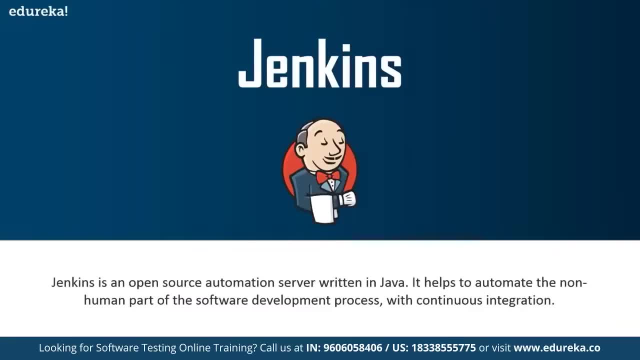 and monitors the execution and status of remote jobs, making it easier for the team members and users to regularly obtain the latest stable code. You can also refer to our Jenkins tutorial for more information on this, But today's session is about how to use JMeter in Jenkins. 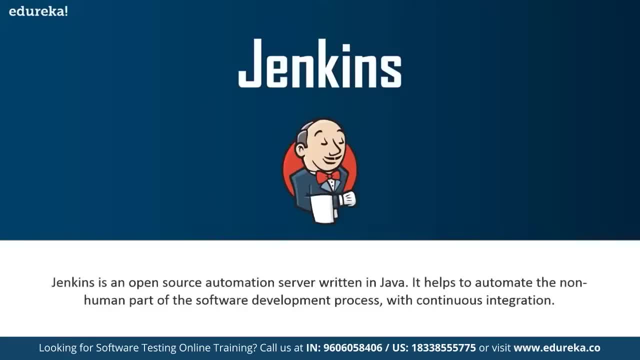 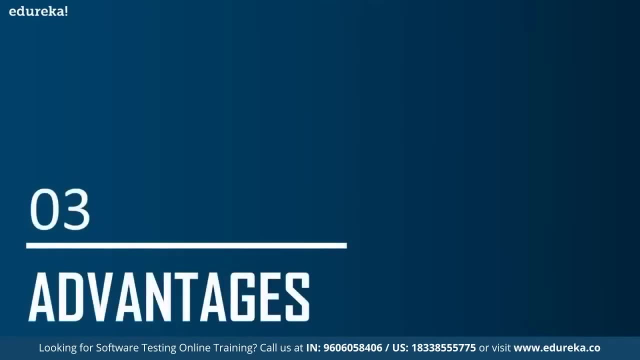 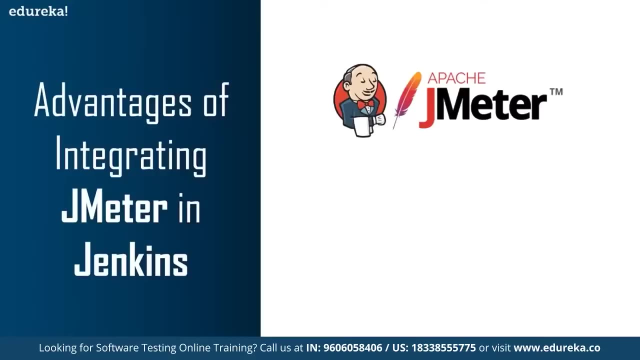 But before we move on to that, why exactly should we use JMeter in Jenkins? So let's have a look at the different advantages of using JMeter in Jenkins Now. continuous integration, test automation and shifting left are becoming the standard for DevOps developers and the QA engineers as well. 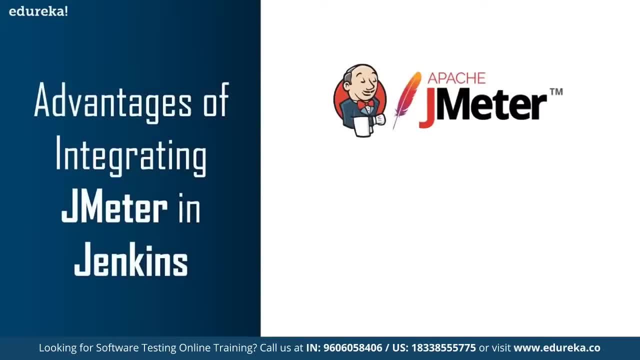 But first, despite the importance of performance and the understanding that systems are complex and it can be challenging to identify and fix bottlenecks in a short time, Load testing is still not an integral part of the CI workflow. So Jenkins easily enables user to integrate load testing into its workflow. 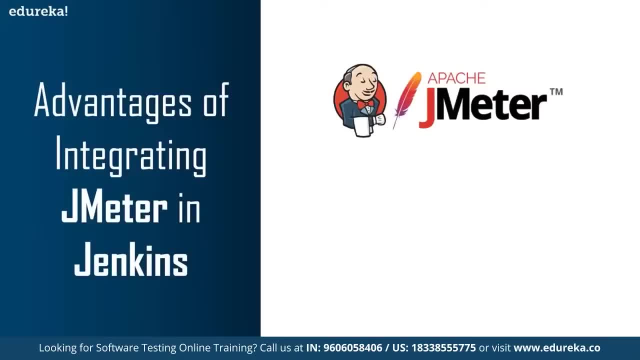 So by using Jenkins as part of the CI process and to trigger jobs by commits, users are taking advantage of automation and process speed up capabilities. So some of the advantages include the unattended test executions right after software build and deploy. Then we have the automatic build failures. 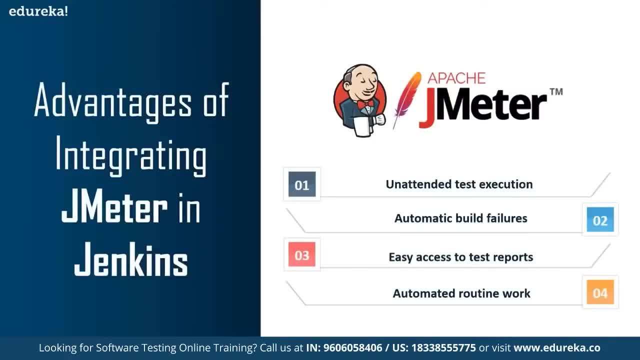 in case of performance degradation. Then we have easy access to test reports that show application metric trends. All tests are in one place and available to anybody with the correct permissions. Not just that: the automated routine work of test configuration execution and baseline results analysis. 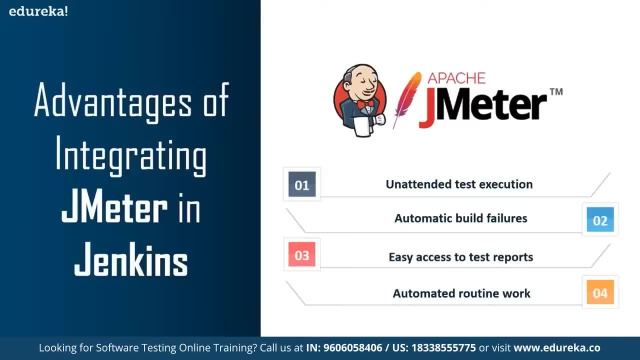 Now users hands and minds are free for more important, complex and interesting tasks. Now, these were some of the reasons why we should integrate our Jmeter in Jenkins. So now let's move on and see how we can do this. So I'll give you a step-by-step guide. 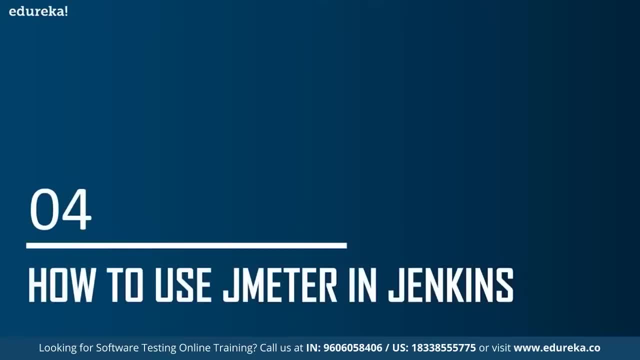 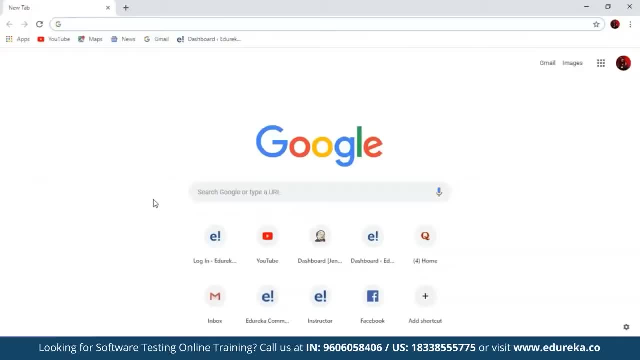 on how you can use your Jmeter in Jenkins. So in this session we will configure our Jmeter and run it in Jenkins. So basically, we will perform our Jmeter test in our Jenkins. So now, basically, in Jenkins you have plugins that support Jmeter. 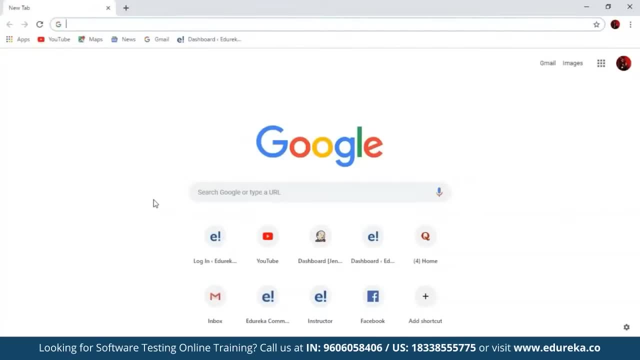 So what you can do is perform the test in Jmeter and also get your performance results report in your Jenkins. Okay, so now, before we start the session, the first thing that we would need is to install Jenkins. Now, in order to install Jenkins, all you need to do is type: download Jenkins. 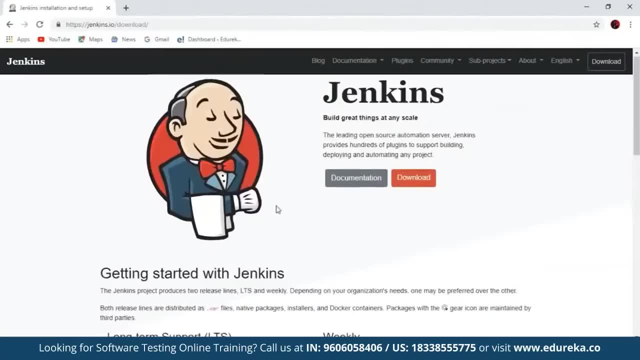 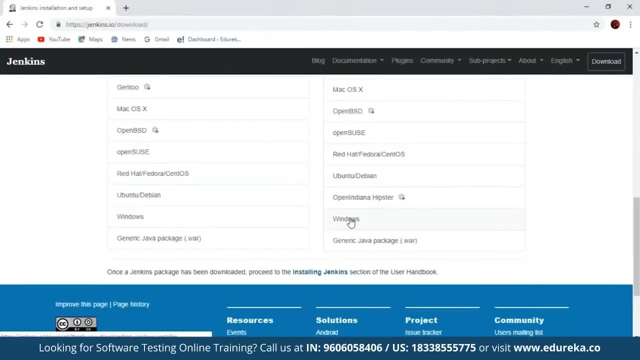 and go inside this website, And once you're inside this website, all you need to do is select your operating system. So I'm using Windows, So I'll be downloading Jenkins for Windows, So this is how you get to download your Jenkins. 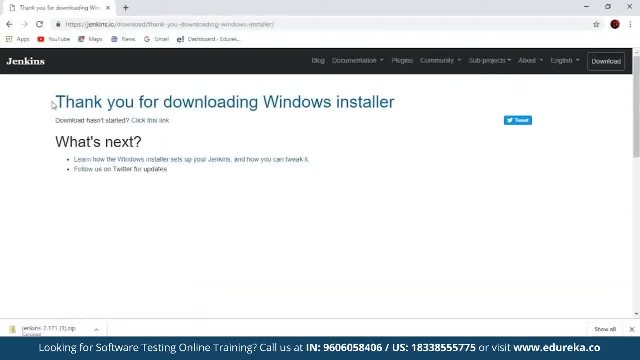 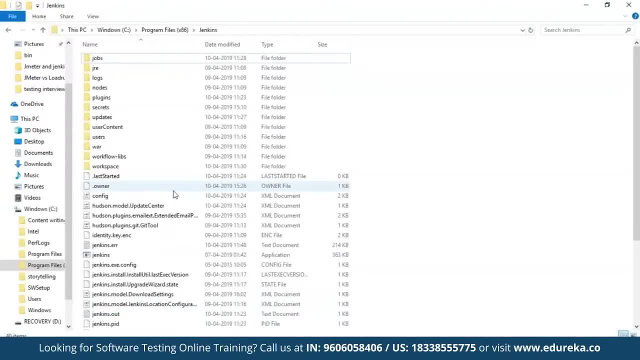 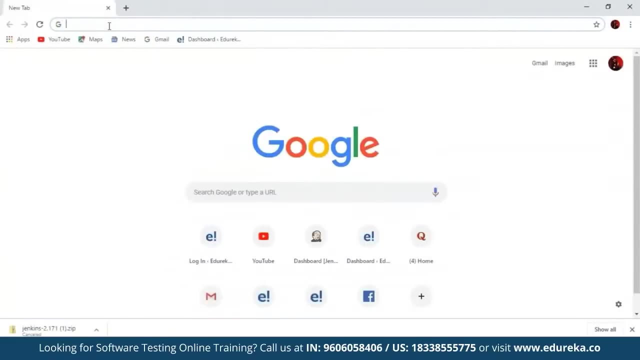 I have already installed Jenkins in my system, So I was just showing you the process on how you can do it for your system. Now, once the download is complete, all you need to do is go to your Jenkins folder and just run your application. Now the localhost ID for Jenkins is 8080.. 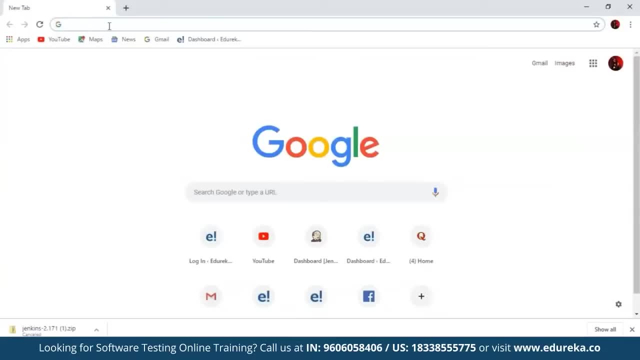 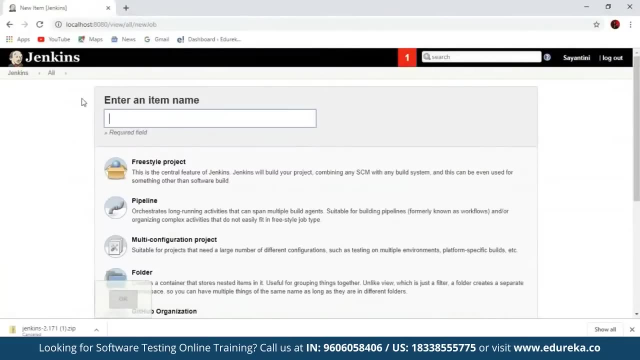 So once you have done installing your Jenkins application in your system, you can go to your localhost 8080. And you can see that your Jenkins is ready to work now. So this is your Jenkins dashboard, in which you can build your project and get your performance report as well. 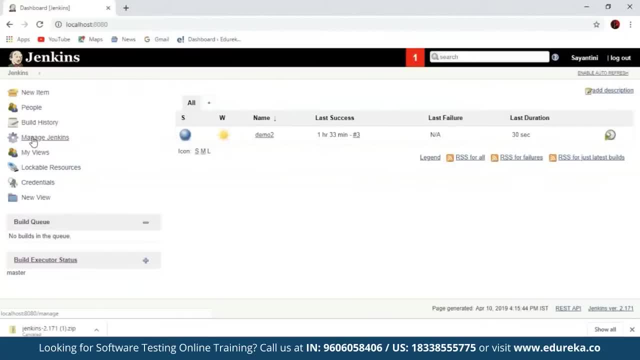 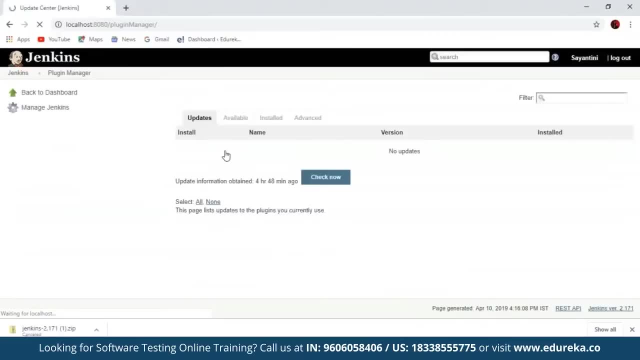 Now the next step is to get the performance plug-in Now. in order to get that, you can just go inside your manage Jenkins and here you will get an option: manage plugins Now. once you are inside your manage plugins, you will get to see your available installed. 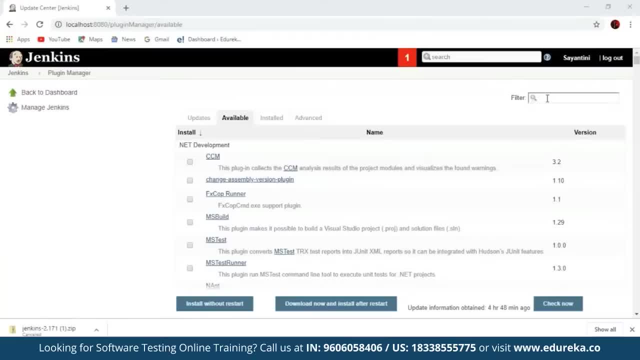 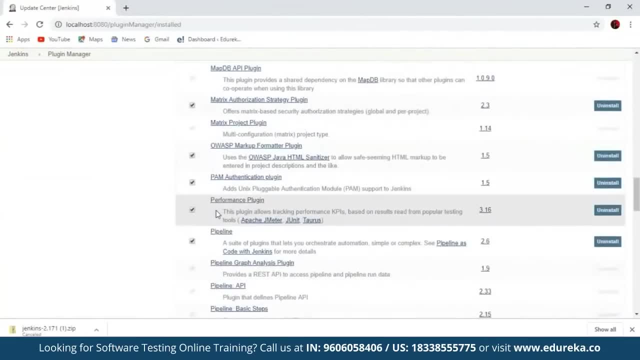 all sort of plugins that are already there. Now for the performance testing, we would need the performance plug-in, So you can just search here and get your performance plug-in and install it in your Jenkins. Now I have already installed it before, So it's already there inside my Jenkins. 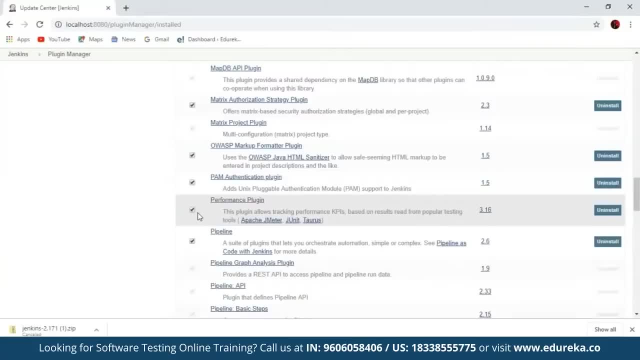 Now, this plug-in basically allows the tracking of your performance based on the results that you read from your Apache JMeter. Now, in order to get the results that you have run on your Apache JMeter, you will need this particular plug-in. Otherwise you would not be able. 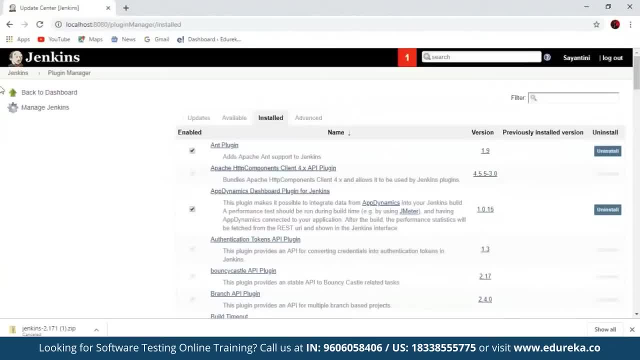 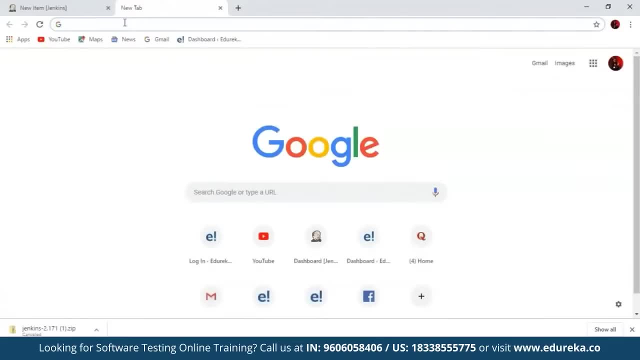 to see any of your test reports in Jenkins. Now, once your Jenkins is up and ready in your system, The next thing you would need is JMeter. now for JMeter, All you need to do is same: download JMeter, And you just have to install this performance testing tool. 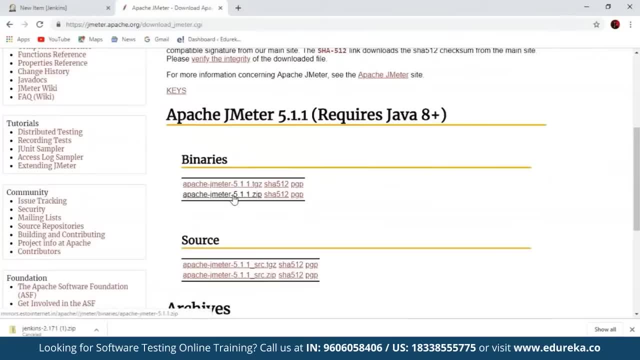 in your system, So you can just download any of these binary files and install it in your system. You can also go back and check out. There's a video on how to install JMeter, which will give you step-by-step guidance on how you can install this particular tool in your system. 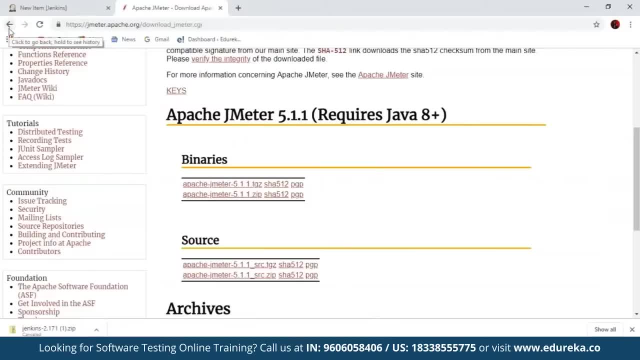 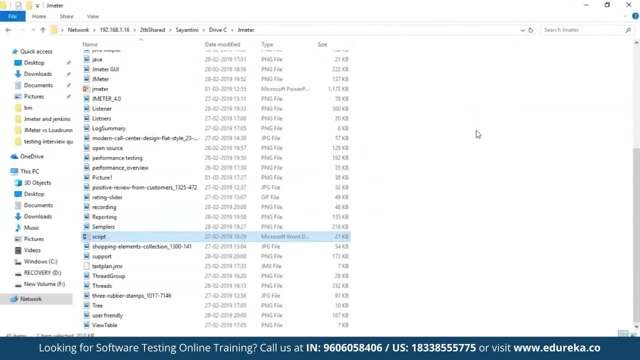 Now I have already installed Apache JMeter in my system, So let's see what we need to do Next. Now, once both Jenkins and JMeter are up and running in your system, All you need to do is go to your JMeter folder. 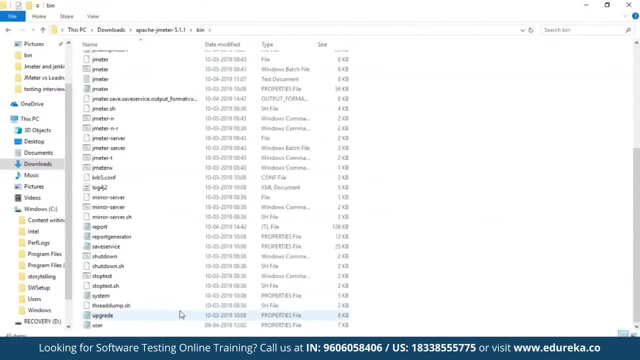 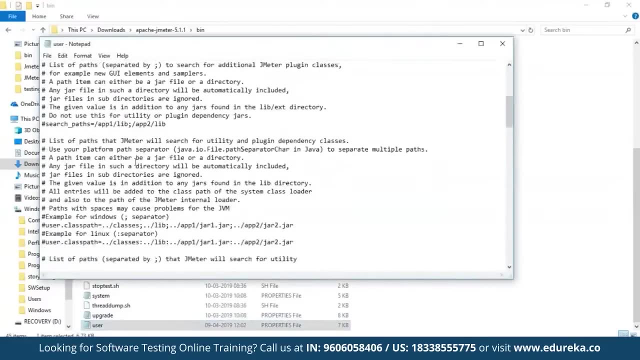 and open the bin folder inside that. Now, inside your bin folder, there would be a file named as the user properties. So here we have the user properties Now inside this file. all you have to do is go and just type this particular command. 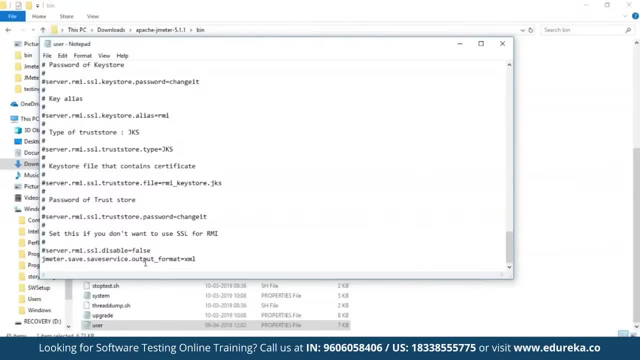 That is the JMetersavesaveserviceoutput underscore format equals to XML. Now this will just provide you your output format that will help you in your Jenkins report generation. So I have already inserted this command in this particular file, and then all you need to do is just save it. 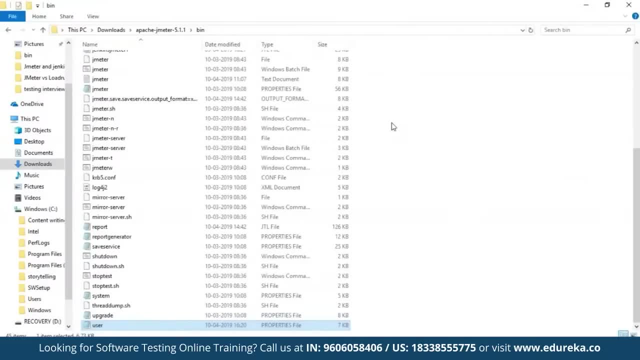 So these were the first three important steps that we need to do in order to begin with the session, That is, first you will need your Jenkins, So we have to download and install Jenkins in your system, and then we will also check if JMeter is installed or not. 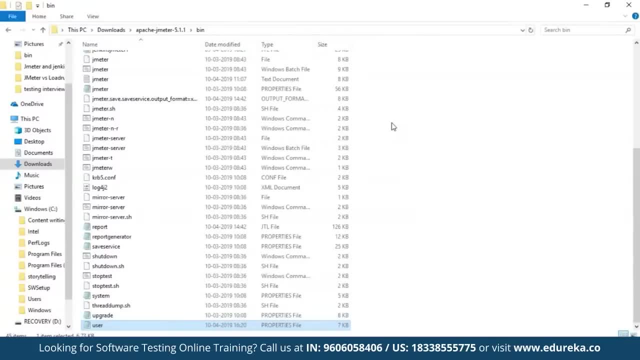 If not, you have to install JMeter as well, and then you have to add one particular command inside your user properties file in your JMeter bin. So now the three steps are completed, Let's move on and see what to do. The next step would be just using your Apache JMeter. 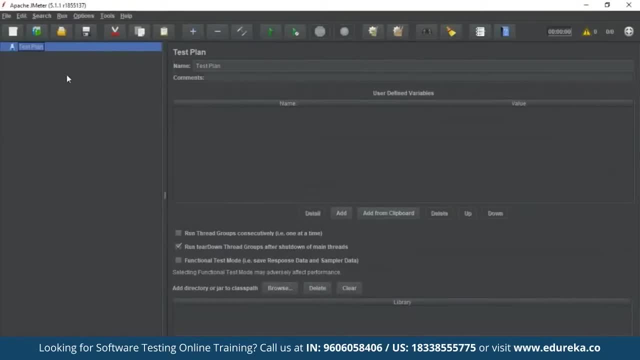 create a test plan. So this is my Apache JMeter user interface and here I'll create a test plan that will also generate the reports in my Jenkins. So let me name my test plan as edureka, and inside my test plan I'm going to add thread groups. 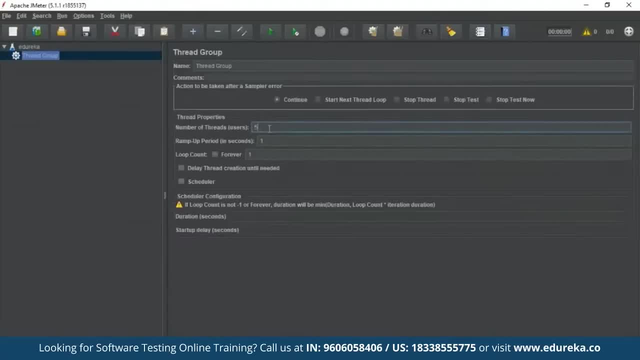 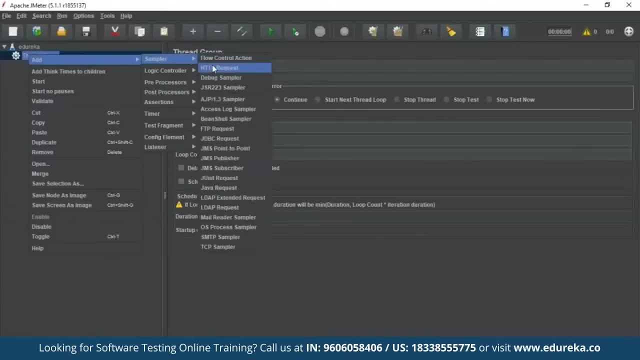 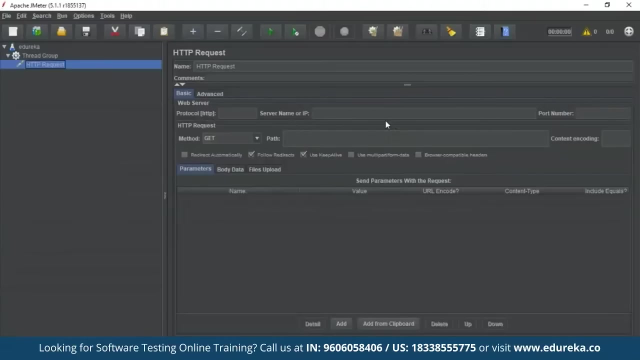 So let me just take five threads or users and let me give the loop count as 2.. Now next, inside this thread group, I'll add one HTTP request. So here we have to add our server name or the IP address for the website that we're going to perform our testing on. 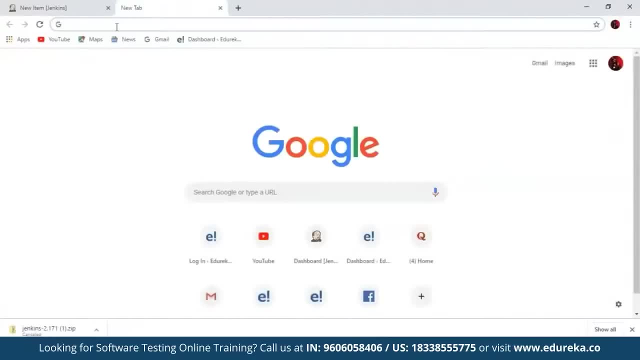 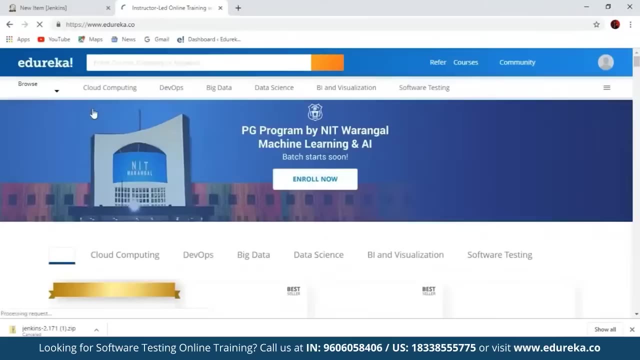 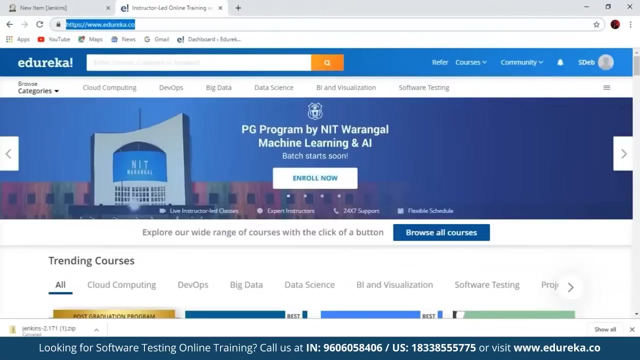 So here I'll be taking the example of the edureka website, that is the edurekaco. So this is our edureka website, on which I'm going to perform the test on, so I'll just copy this IP address And I'll paste it here in JMeter. 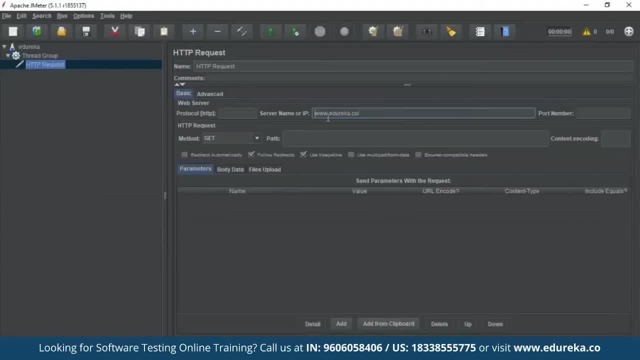 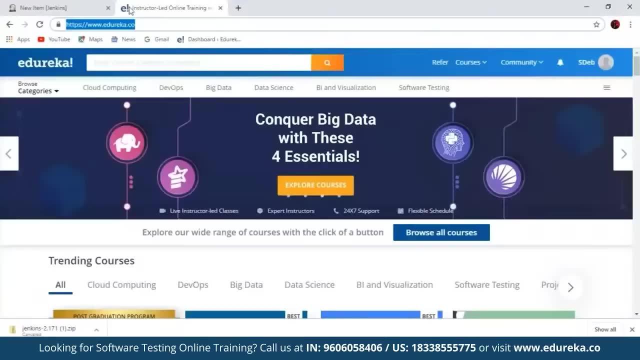 We don't put the HTTPS, So the server name or the IP would be wwwedurekaco. Now I have to set a path inside this So you can see that inside the edureka website We have different paths where we can get into that. 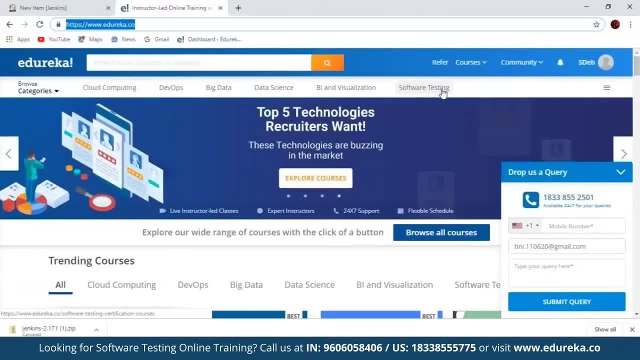 as we have a cloud computing devops, software testing and all these parts take you to all these courses that we provide and it gives you a brief description about what these courses are and what you get to learn. So let me first take the course on cloud computing. 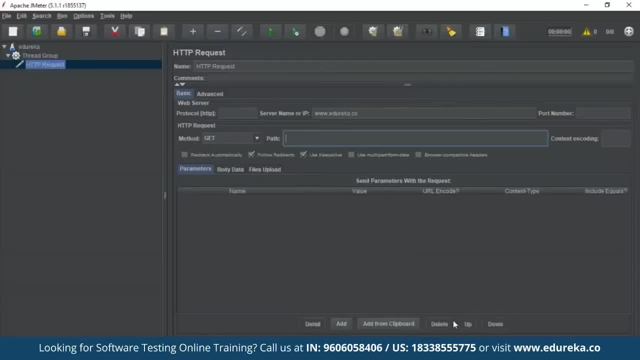 So let me set a path to this particular course. So here I'll just paste the path to my cloud computing server. This is the certification courses, and let me just rename it as cloud. Now let me create another HTTP request, So the server name will be the same as wwwedurekaco. 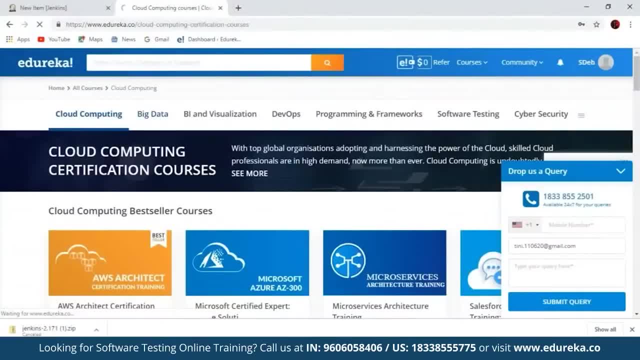 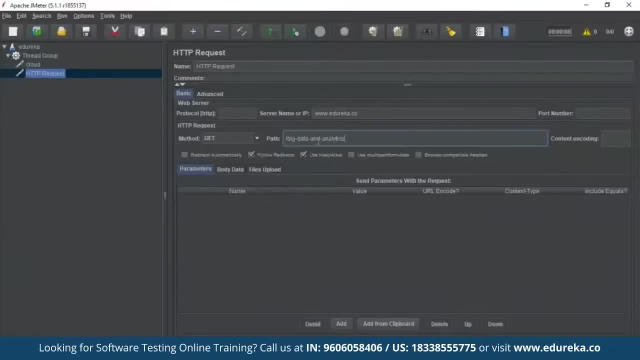 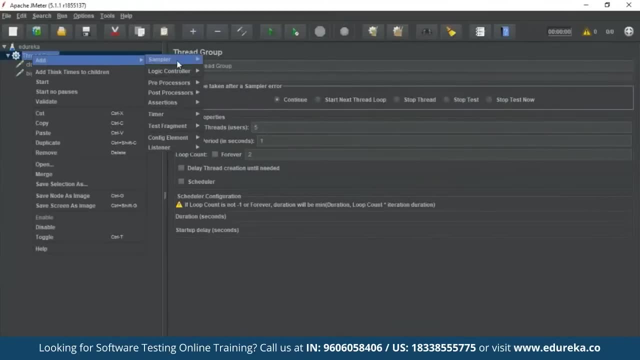 Now let me travels to another path. So let's just take big data as our second path. So here I'll copy this particular path and use it here. Now let me just rename this one as big data Again. Let me just take another HTTP request, same way. 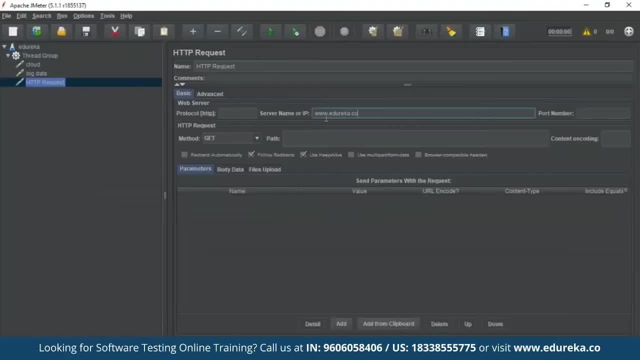 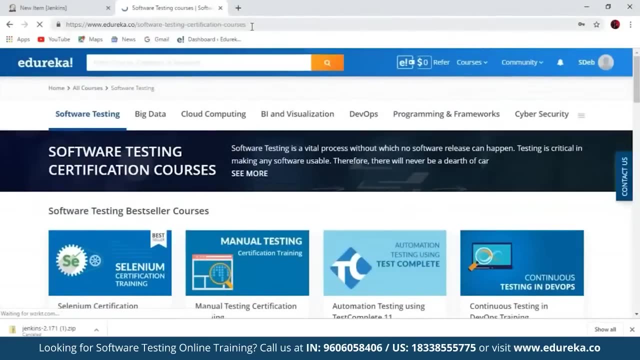 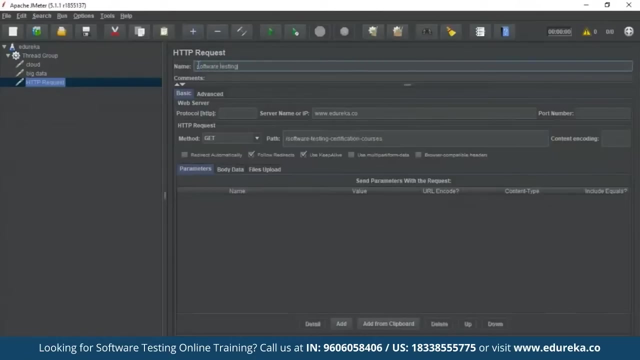 I'll just type wwwedurekaco, And this time let me take another path. So this time let's go inside our software testing course And I'll rename this one as software testing. Okay, so now that we have created all the HTTP request. 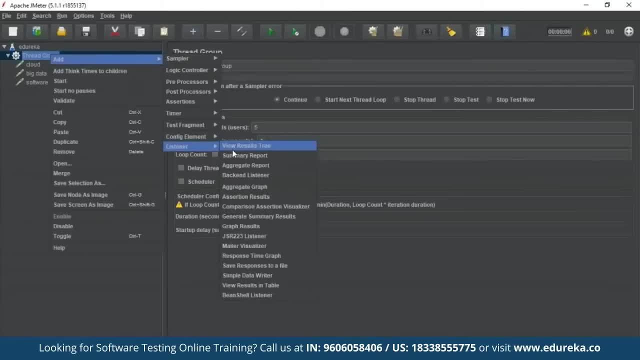 now next up I'll add a listener. that is where I can view my results, so we can select the option on how we want to view our results. So there are view results, tree view results and table. So let me just select view results and table. 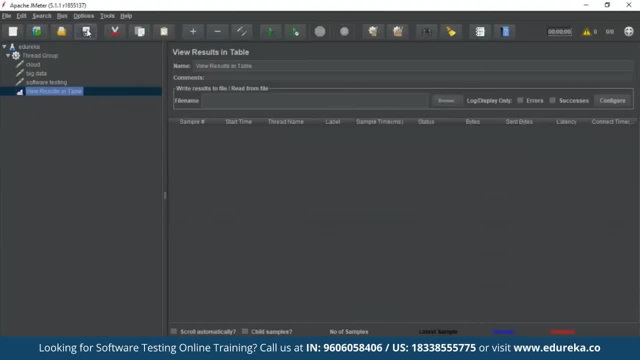 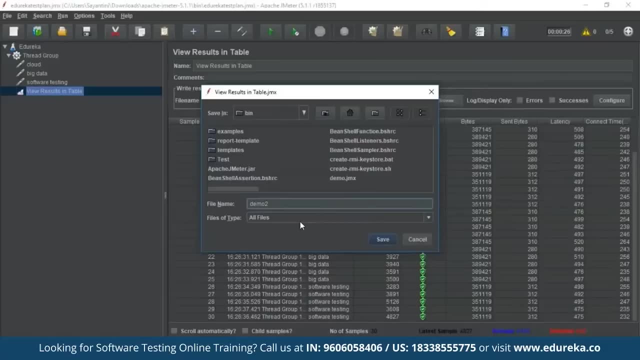 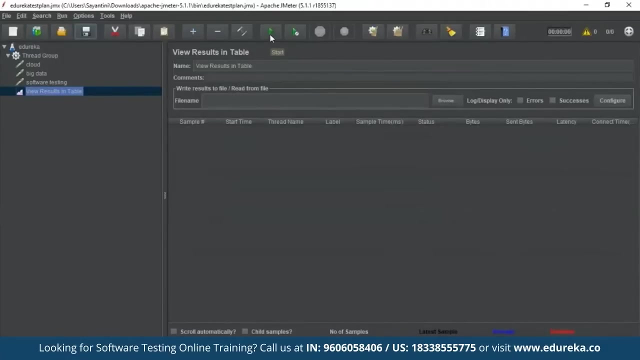 Now, before we run our test, we always have to save our test, So let me just save this test as demo2 and the extension is always jmx. Now I have saved this test plan. Now let's run this test And see what happens. 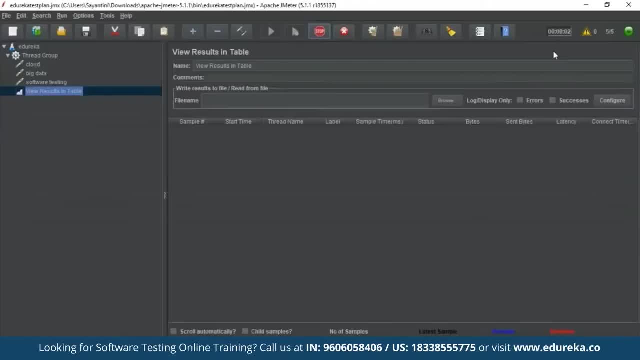 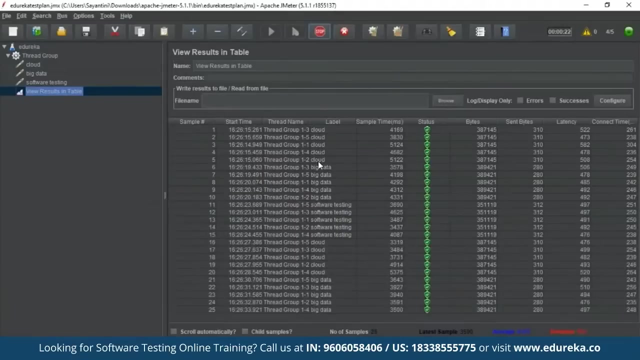 So once I start this test, you can see that it's going on. So yeah, the test is happening and you can see that the number of thread group for cloud big data and software testing takes place first. It takes place five times because I have taken the thread user number as five. 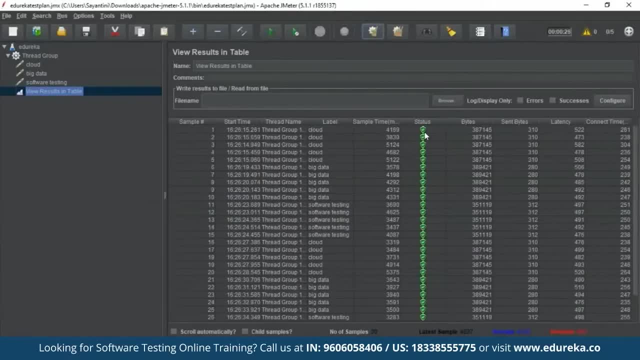 and the loop count will go on for two times. So you can see that the status here is green. That means the test is going on fine and there is no error that has occurred in this test yet. So now in the JMeter user interface. 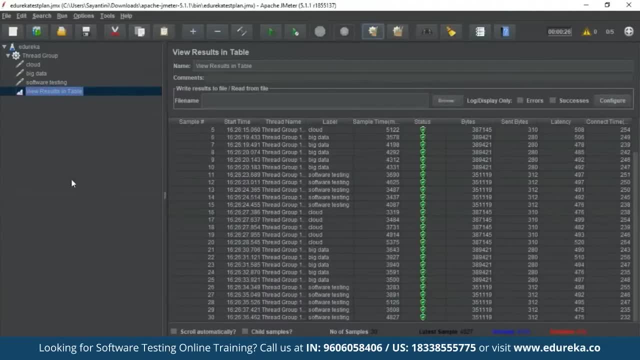 you can see that the test is going on perfectly, all right, and the website is functioning perfectly. Now, in order to generate our test reports in our Jenkins, we would need to run this test in the non GUI method. So now, in order to run this test in the non GUI method, 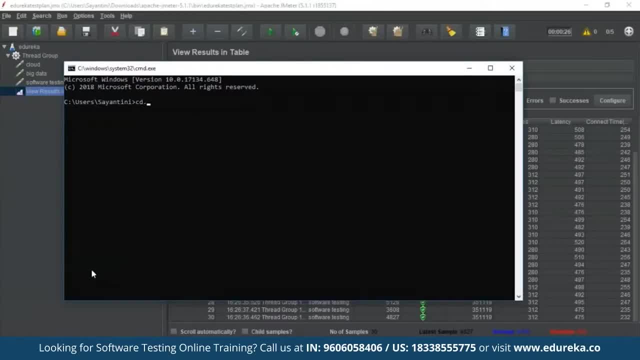 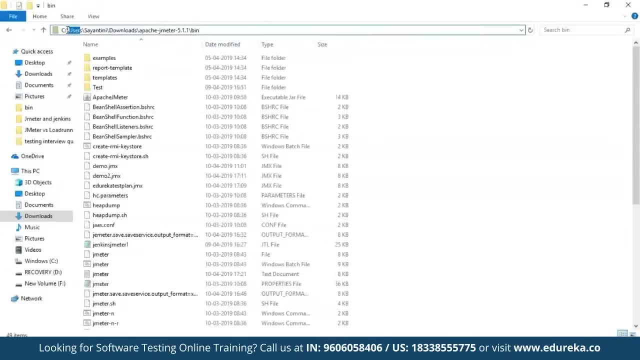 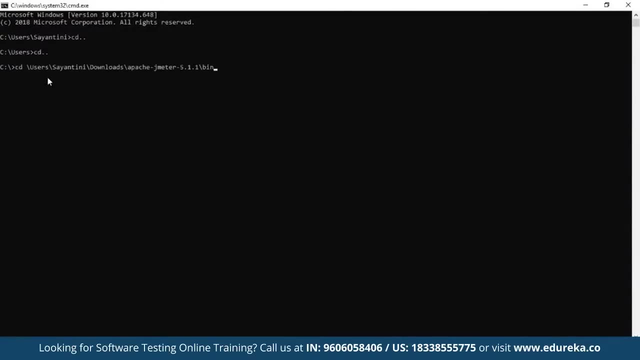 we'll go to our command prompt And here we just have to specify the name of the path inside our JMeter folder. So I'll specify this particular path And now we are inside our Apache JMeter bin folder. Now you can also go back and check out our video. 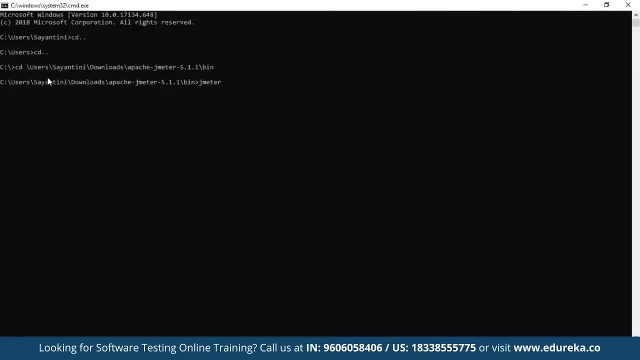 on load testing using JMeter in the non GUI mode, which will give you a step-by-step guide on how you can perform your testing in the non GUI mode as well. So now let's have a look at the command in order to run our test plan. 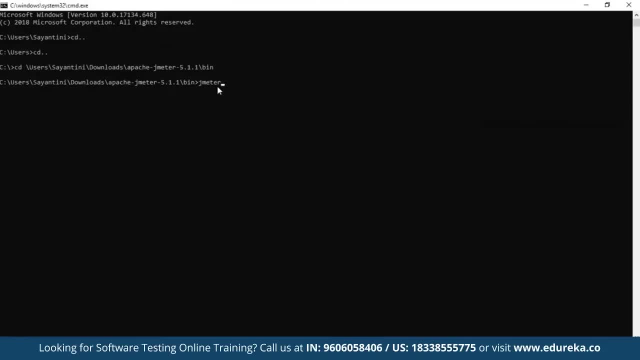 in the non GUI mode. So first we have to write JMeter, and then we go for minus N. Okay, Now in this one we can also go for minus J, That is, if you want to send any parameter. So here we will be sending a parameter. 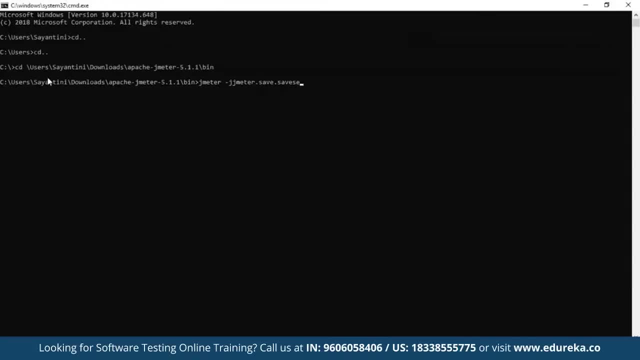 as JMetersavesaveserviceoutput underscore format equals to XML, just to ensure that this format is up and running and we can get the output in the same format that is in our XML format in our Jenkins as well, So we'll just pass this parameter. 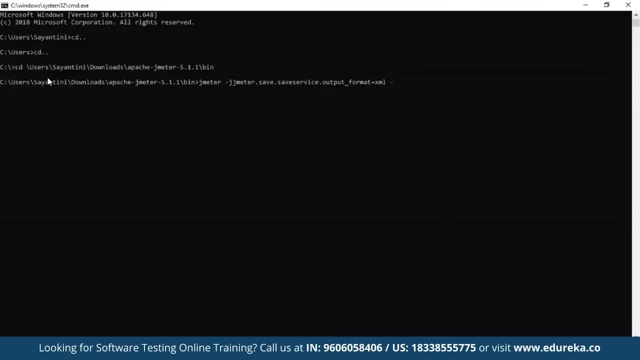 in order to ensure that this is happening. Then it's hyphen N which is used to specify the test plan to run in our non GUI mode. Then we have hyphen T, which specifies the path to our source of dot JMX file. 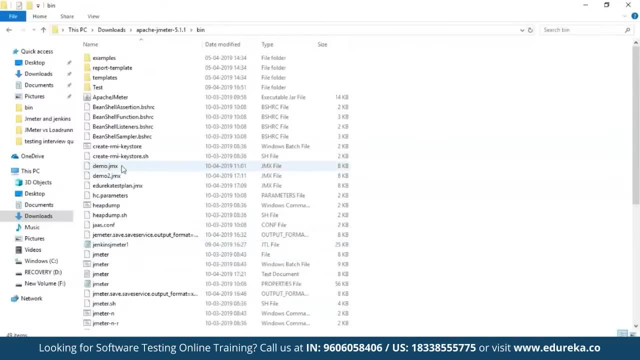 where we have actually saved our test plan. Next, we will just copy the path to our JMX file, So you can see that our JMX file is right here. That is demo 2 dot JMX. So I'll just copy this path. 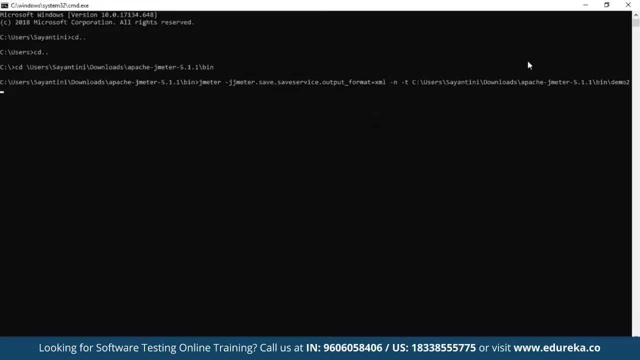 and insert my file name, That is edureka test plan dot JMX. So with hyphen L we specify the path to our output file or the file where we are getting our results. So I'll copy the path as well. We want it inside the bin folder only. 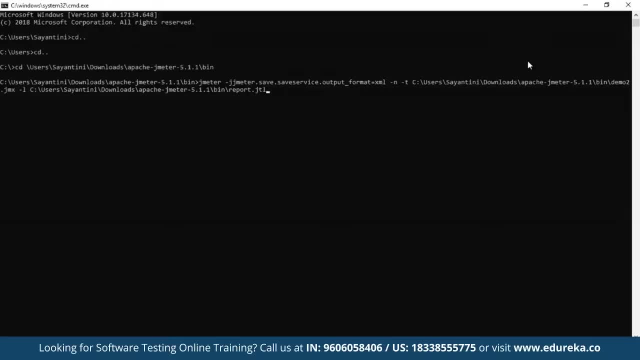 So let me just name it as report, and we want a JTL file. You can have a JTL file or a CSV file. Now let me just run this command and see what happens. So here you can see that the tree has been successfully created. 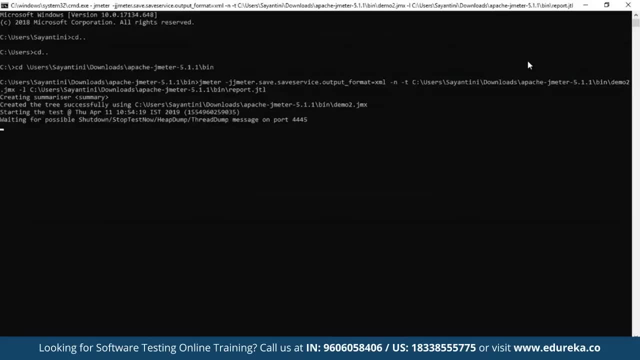 and the test has been started. So now, basically, the same test has been taking place in the non GUI mode, So this will take a certain time, and we also got to see the status in our GUI format in the form of a table. Now, in this case, 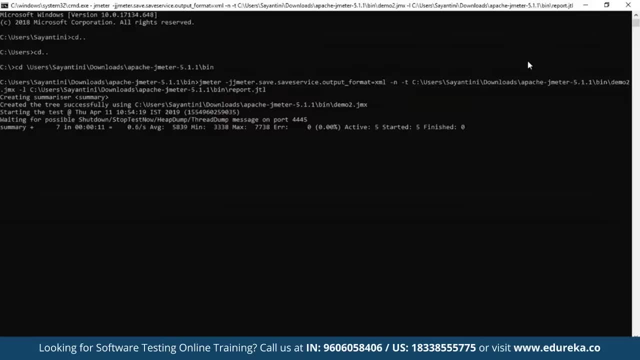 we will get it in our dot JTL file and it will show us the same status as the testing is performing completely fine or not. Now, once the test will be completed, it will show you that the test is completed and then you can go back. 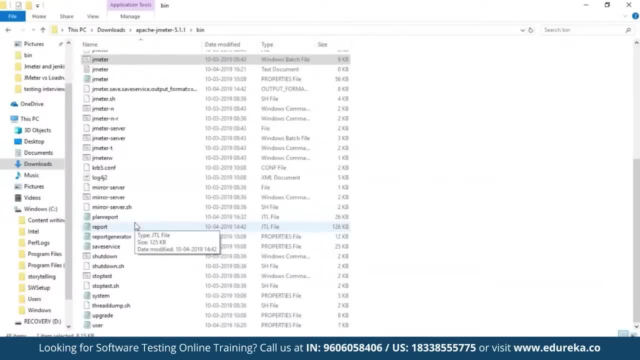 and check your result in your folder, in your bin folder, where you have saved your test report or where you have saved your test plan as well. So here you can see that it shows end of run. That is, the test plan has successfully completed the testing. 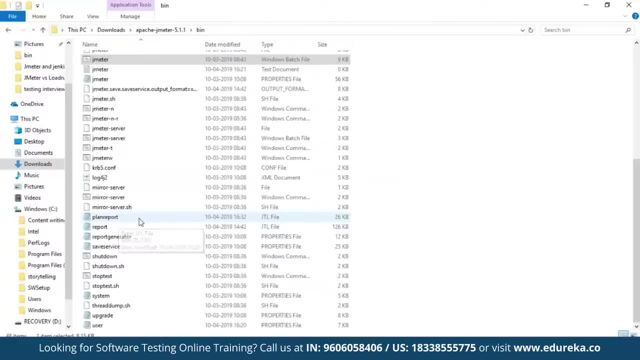 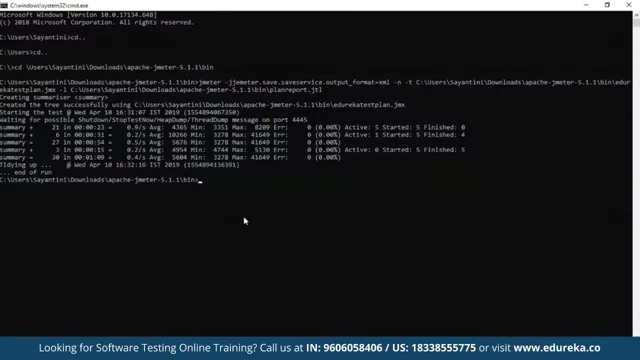 So inside your bin folder you can go back and see that your JTL file is created, where you have your report ready. So now this was about running your test in J meter using the non GUI mode. I have also shown you that the test is completely up. 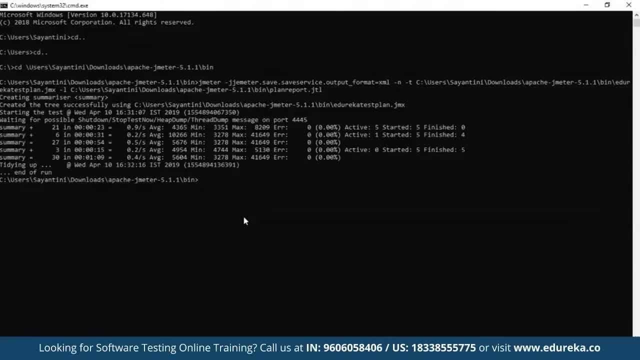 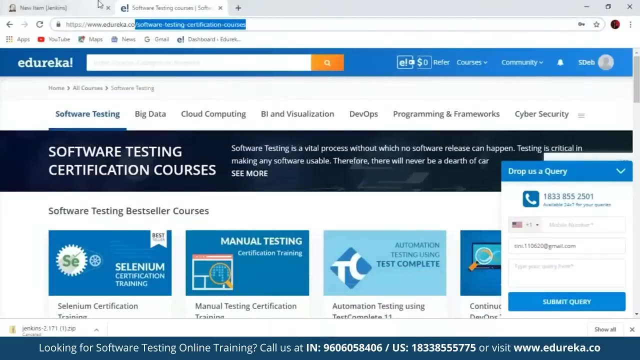 and running in the user interface mode as well. So now that the test has run completely fine in the J meter, now it's time to import this in our Jenkins and get our performance results report. Now, how do we do that Now? for that we have to go back to our localhost 8080.. 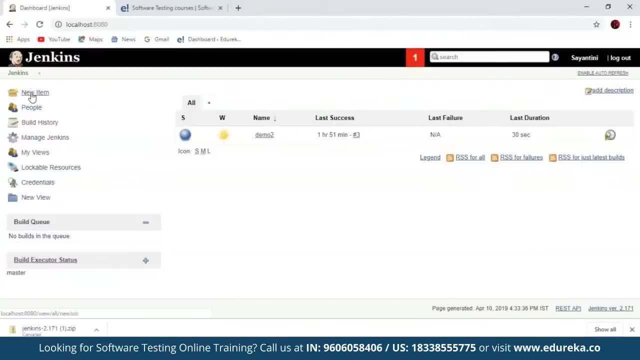 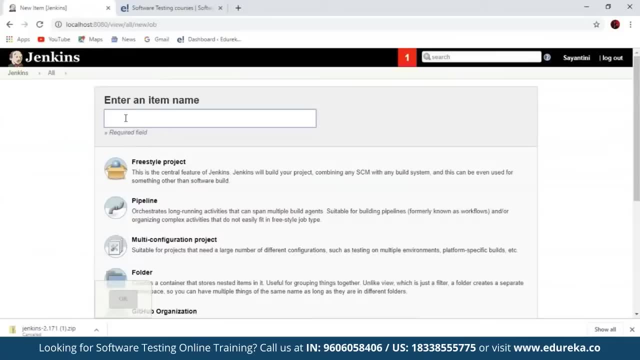 Now, once we are inside our Jenkins dashboard. so in the left side there is an option called as new item. So here you just have to enter an item for your project. So here I'll just name my project as J meter, J meter test, and I want it to be a freestyle project. 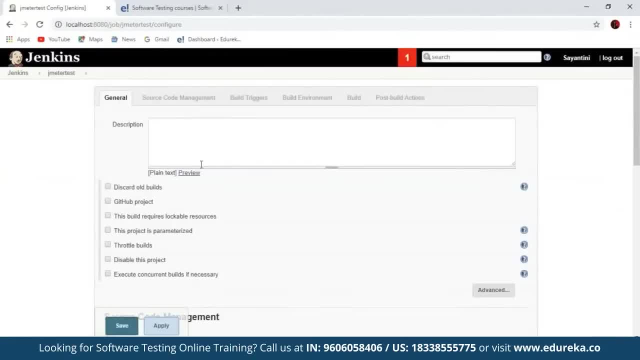 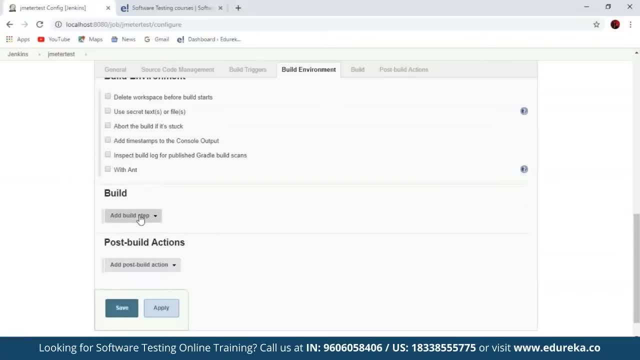 and then just click on OK. So now the project J meter test has been created. Now the next step is to add a built setup. So just to give you a quick review, We have followed quite a few steps till now. that is first. 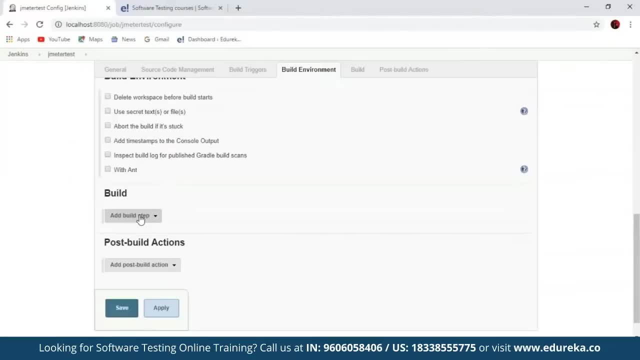 We have installed our Jenkins, that we have installed our J meter and then we have set our path as J meter dot, save, dot, save service dot. output format equals to XML inside our user properties file in J meter bin. Then we have created a test plan inside our J meter. 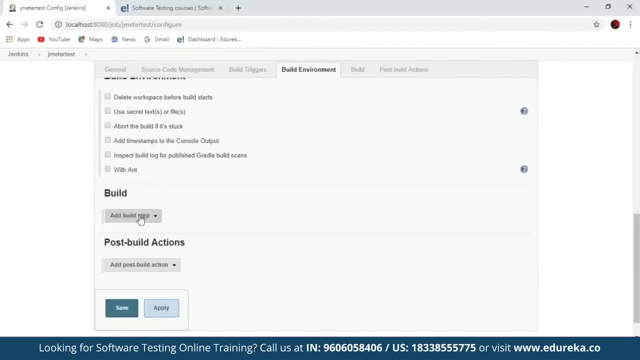 and perform the test plan in GUI and checked that it's all up and running and then, finally, we have moved on and also tested our plan in the non GUI mode. So once the test is completed and it's up and running, We have come back to our localhost 8080.. 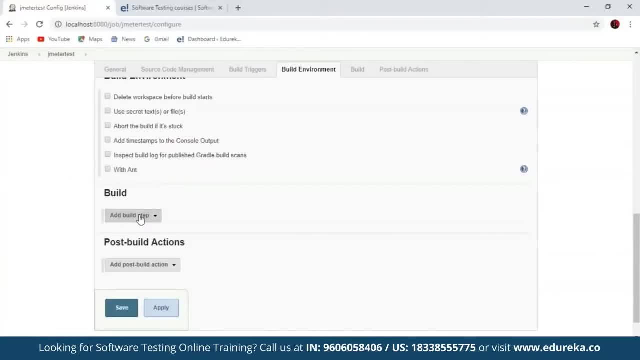 That is, it's time to get our results report in our Jenkins now. Now the next step is to add a build step. So once we click into add build step, you'll see all these options. now I'm using Windows, So I'll select execute Windows batch command. 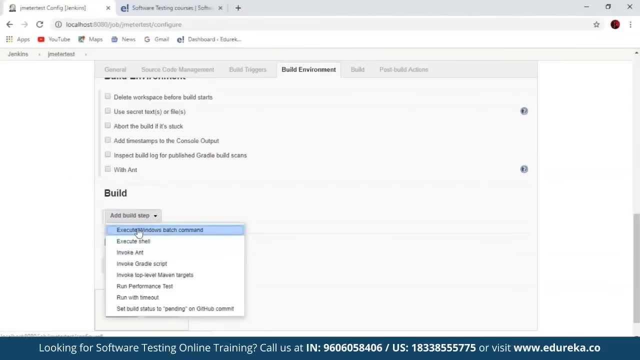 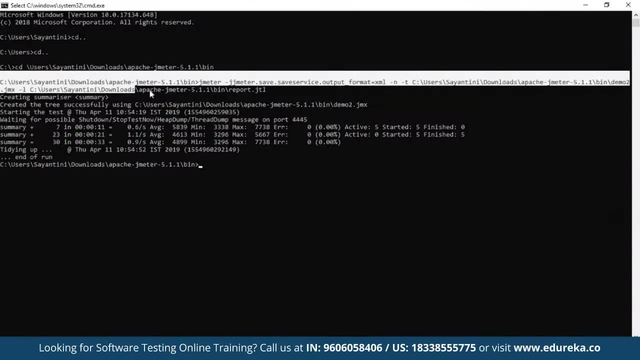 If you are using your locks, you can go for execute shell. So here I click on execute Windows batch command. So now we would be needing this particular command in our Jenkins, So let me just copy this one first and go back to Jenkins. 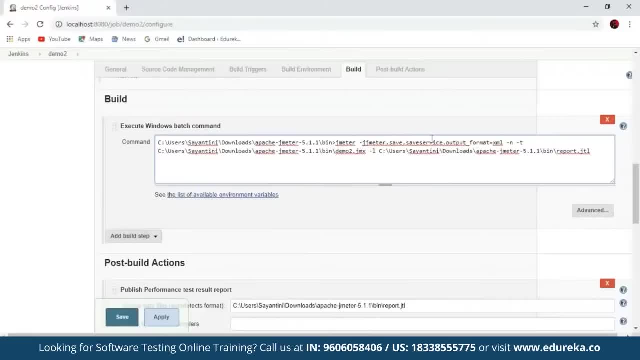 So here I'll just paste this particular command. Now here, what I'm doing is I'm importing the particular test plan in my Jenkins and giving it the path to my test report, where the test plan has already been successfully completed. Now this will give Jenkins the details about my test. 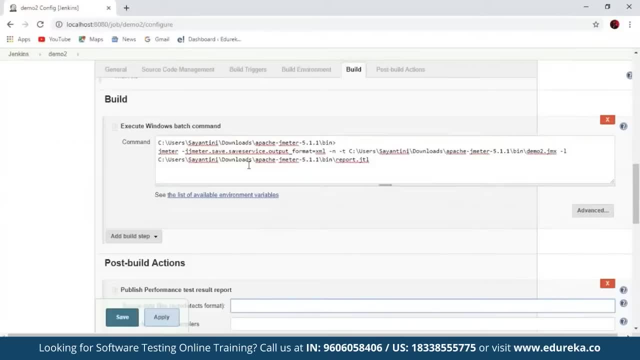 and also the report that has been generated, and thus Jenkins will take that report and give me a performance report here. So at first I have to provide the path to my J meter bin and then I have to give my path to the test report, that is, the JMX file. 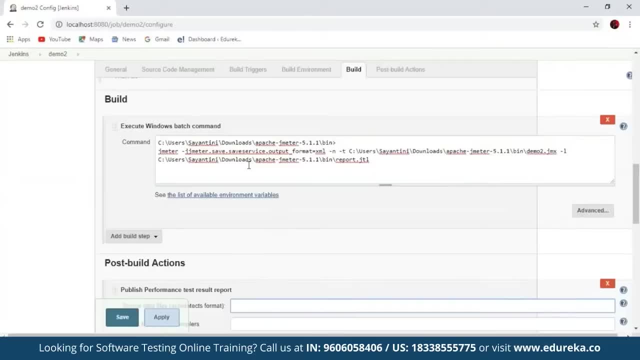 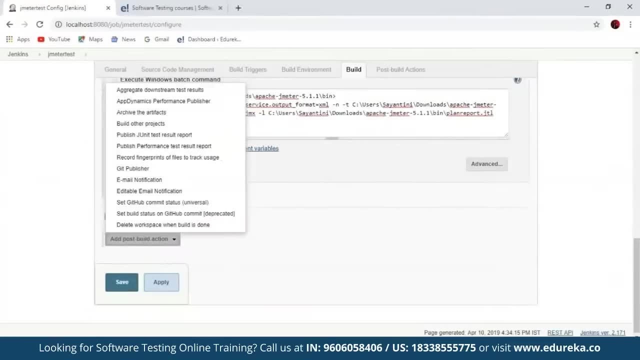 and also the report file, That is, the dot JTL file. So now, once this is done, there's another important step that we need to perform. So next is the add post build action. So once we have completed our ad built setup, next up. 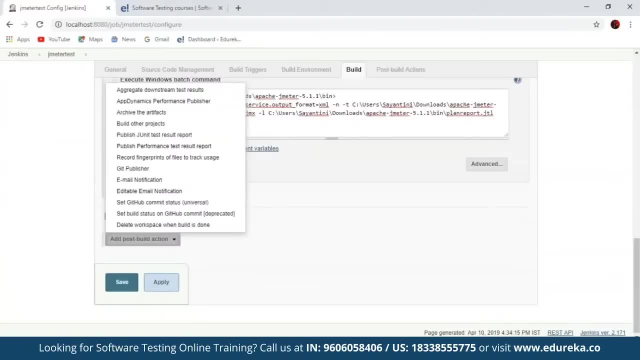 is another important step where we have to add post build action. Now here we have to select the published performance test result report. Now at the beginning, if you remember, we have installed this performance plug-in inside our Jenkins, So now that particular performance plug-in. 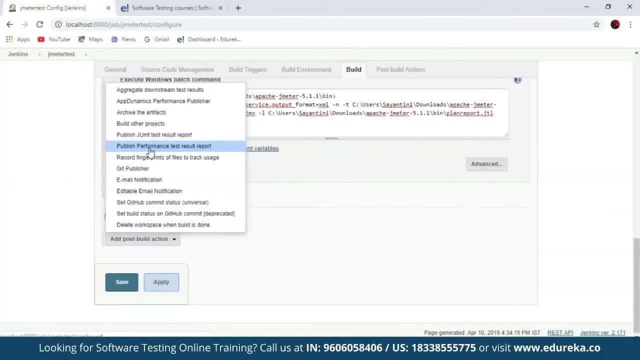 is added as our post build action, where we publish our performance test result report. Now this particular plug-in will first collect the data, then conditionally fail the build if the error threshold is exceeded, build or update the performance trend chart for the project. So now you know why we needed that particular plug-in. 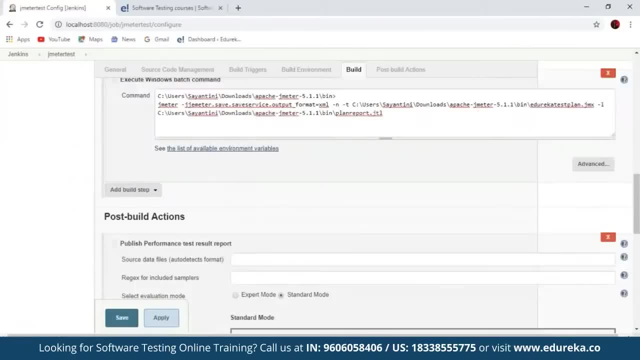 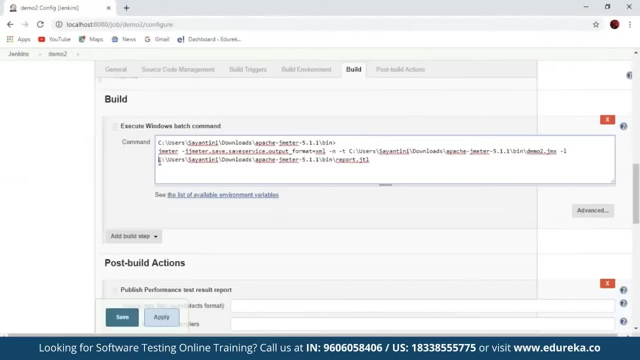 inside our Jenkins. So now here I'll select publish performance test result report. Now, here, in the source data files, you have to specify the path on where the report is saved. So this is our path where my report is saved. So I've saved it as report dot JTL. 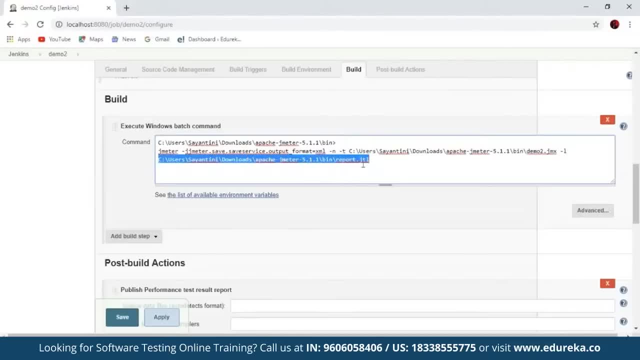 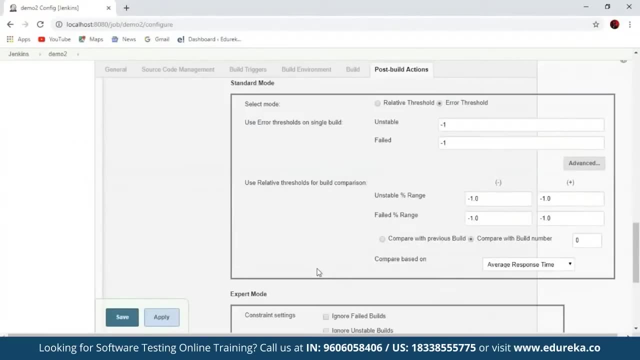 So I'll copy this particular path and I'll provide this particular path here inside the source data files. So here we have the standard mode selected. Yeah, so that's all that you need to do. First you need to build your setup and then another important step. 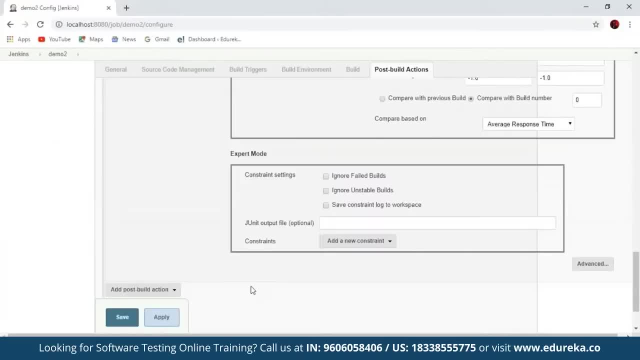 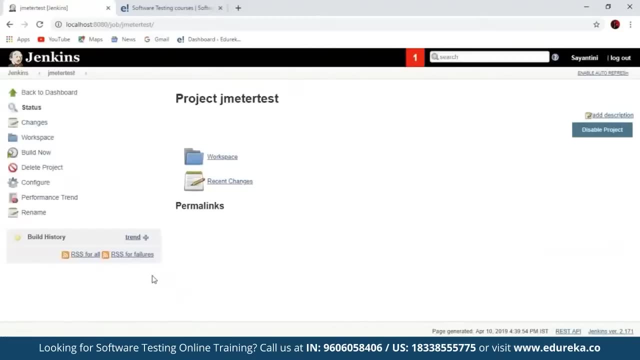 is definitely the post build actions, where you have to specify the path of your test report that will be generated here. So now that we have done all of these, I'll save. So now the project Geometer test has been created. So now, once the project is created, 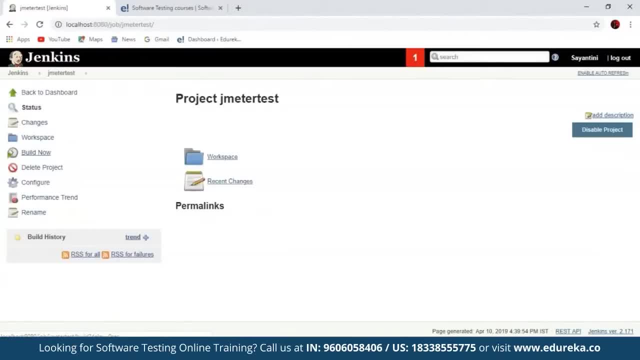 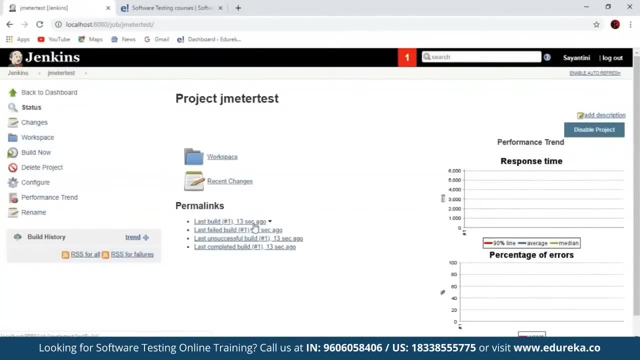 it's time that you build it and get to see the results. So once the project is created now, we will go inside build now. So you can see that the last build was 13 seconds ago. That is just now that I have performed the Jmeter test. 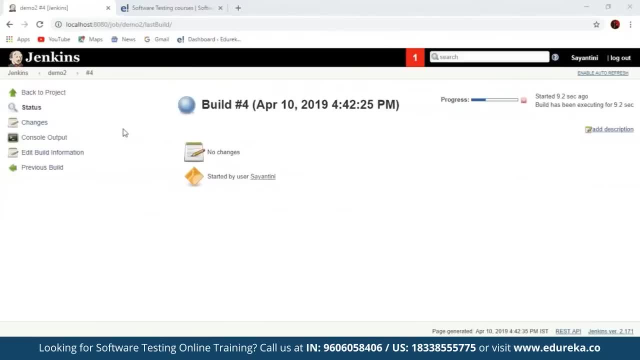 So now that this is done, So now, once we have selected the build now option, you can see that the test is building here and it's in progress. So the build goes on executing and once it is completed, you can get your performance report. 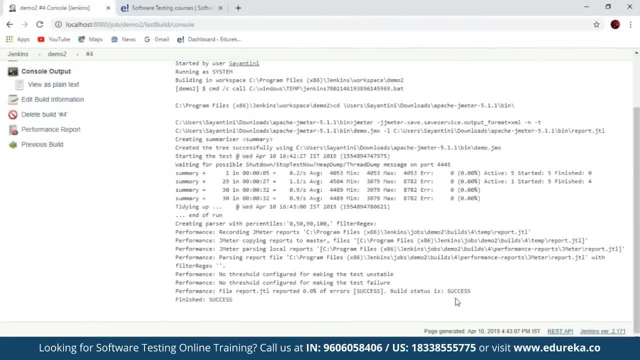 So in the console output you can see that your build status is success and your test has been completed. So you can see that your test has been successfully completed. So you have finally finished a performance testing on the edureka website. Now in order to check your performance report: 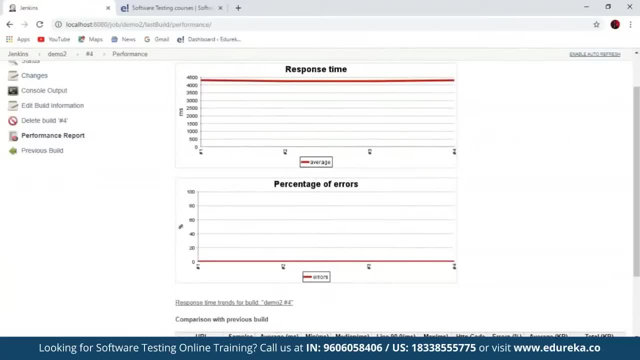 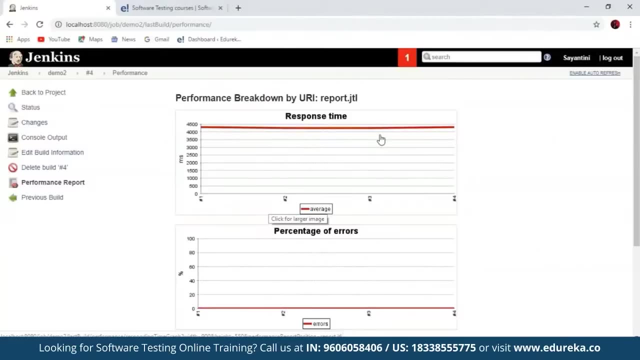 you can go to your performance report and see your response time and percentage of errors. Now we have just done the test once. So there's this one line that is visible and there's no comparison yet. But if you run the test a number of times, 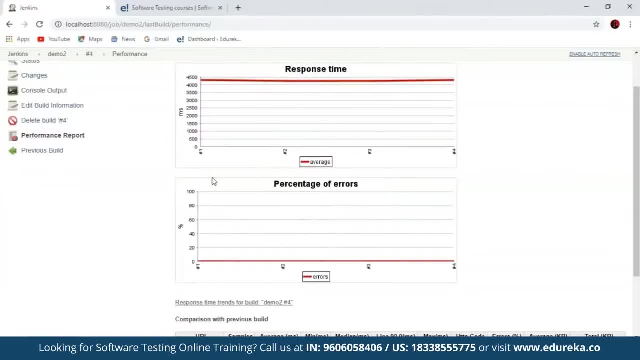 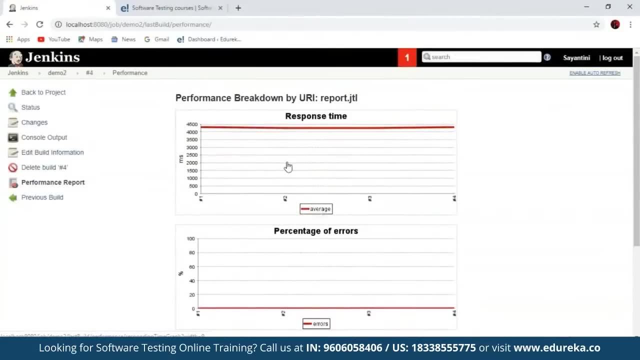 you will be able to see a graph that shows you the difference between the number of bills. So you can see there are no errors, because there has been no error in our website as of now, and you can see the response time here, and here you have all the samples. 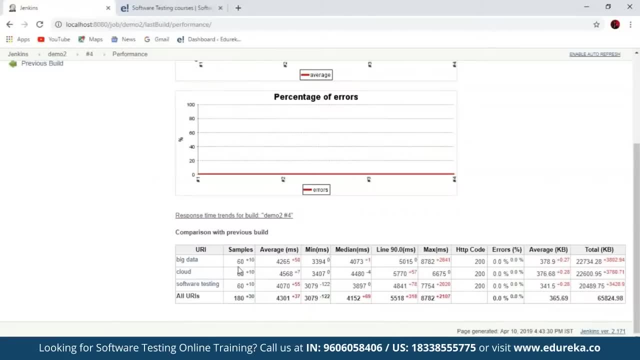 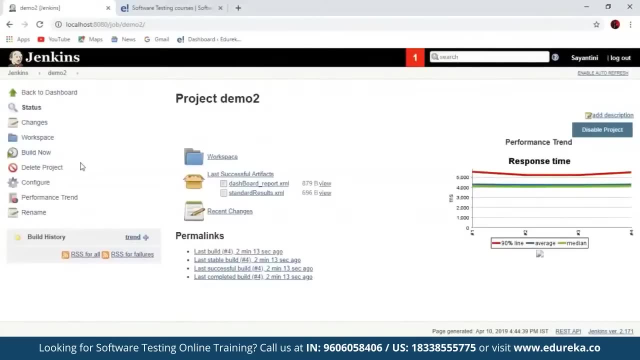 on. see, I have taken big data cloud software testing, So it provides me with all the details of the performance that has taken place. Now I can go back to my project and just click on build now, So it will create another built and I can just go. 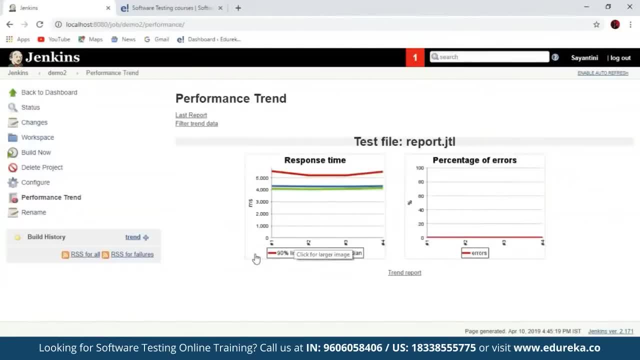 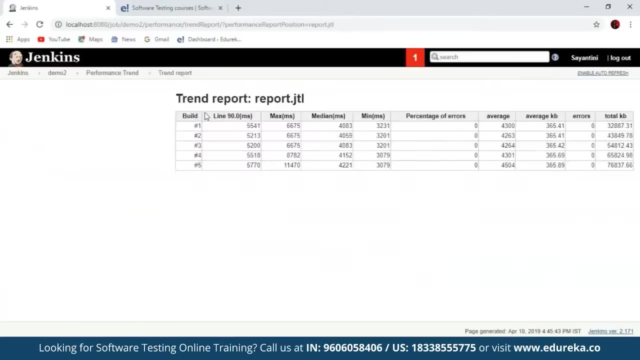 and click on build and check on my performance trend again. So now that I have built my project two times, so you can see that there's a graph you can see here on the response time and the percentage of errors is still zero, Now we can go to our trend report. 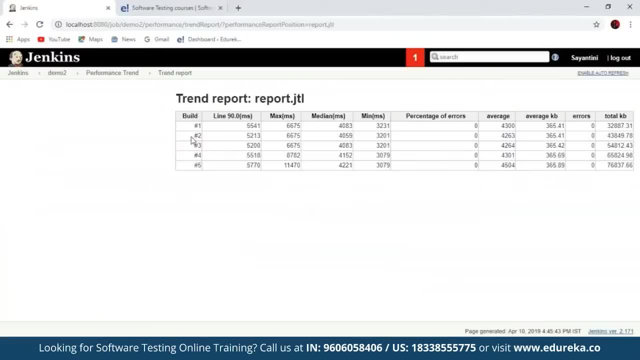 and we can see the number of bills, So the number of times you perform the built on. you can see all of those bills that has been performed here and then you can see the maximum median min percentage of errors and average errors and everything that you need to see. 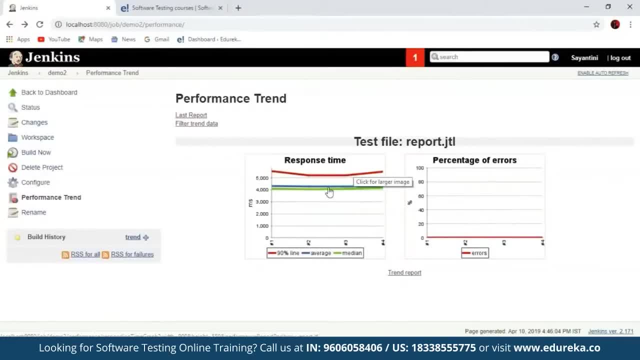 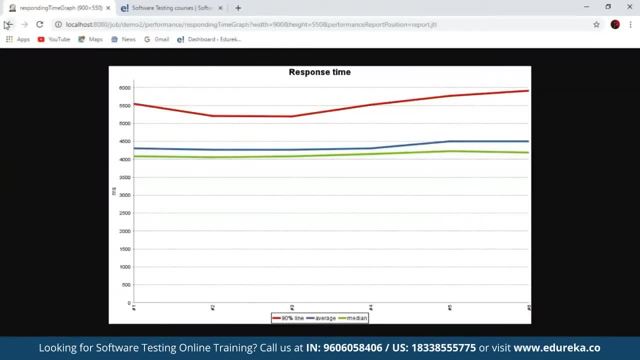 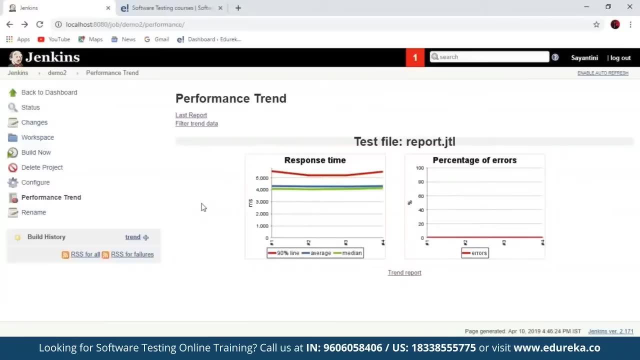 so you can definitely understand your performance trend better with the help of Jenkins. So in this particular one you can see the response time, the average, the median and all of these reports that are generated in our Jenkins. So this is one easy way on how you can use your G meter in Jenkins. 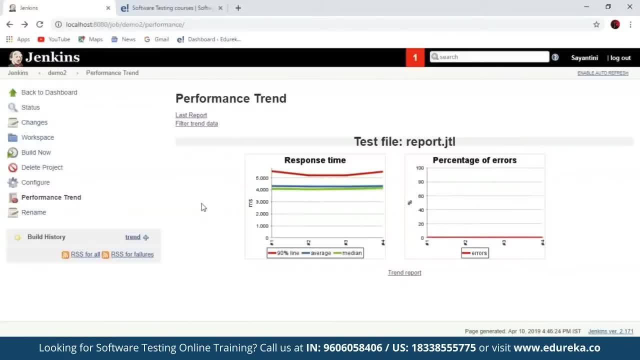 So this way you can easily enable the user to integrate load testing into your workflow. So we had saved our report in the report dot JTL file So you can see that the test file gives the report dot JTL where you have your response time. 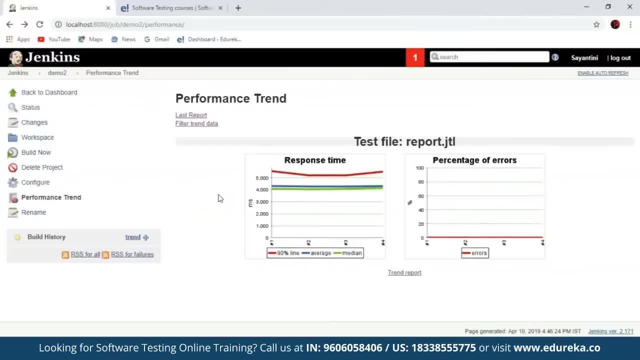 and also the percentage of errors. So this way in Jenkins you get to see the performance report of the test that you have performed on any particular website or server using your Apache J meter. So I hope now you have understood on how you can use J meter in Jenkins. 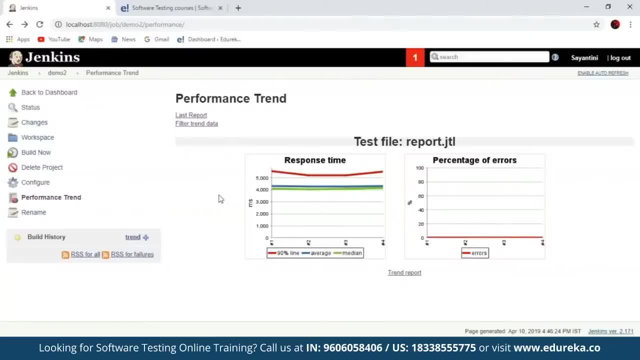 If you have any doubt about how to install Apache J meter or how you're going to use it, You can always check our YouTube channel and check the videos on J meter. that is how to install J meter and load testing in J meter in the non GUI mode. 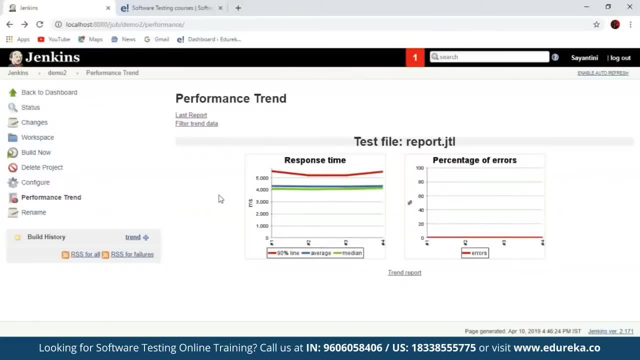 and you can also check out our playlist on Jenkins. that will help you understand these two in a better way, and I hope this session was helpful for you to understand on how you can use these two together in order to perform your testing in a better way. 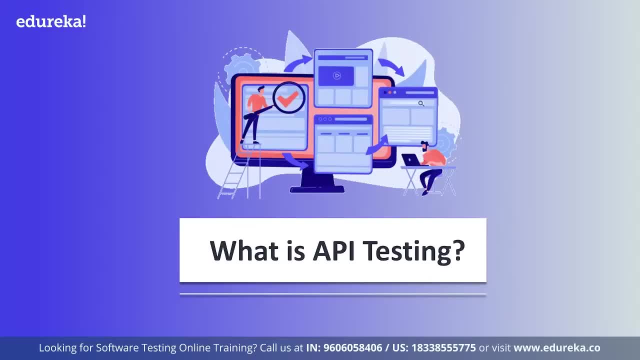 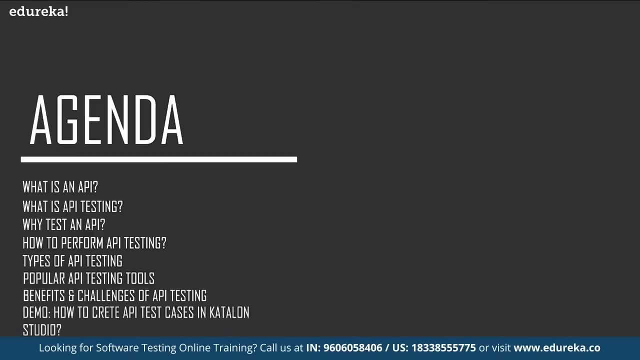 So we will begin the session by discussing what exactly is an API and what does it do. then we will move on to our today's topic, which is API testing, and there we will discuss what API testing is. Why do you have to test an API in the first place? 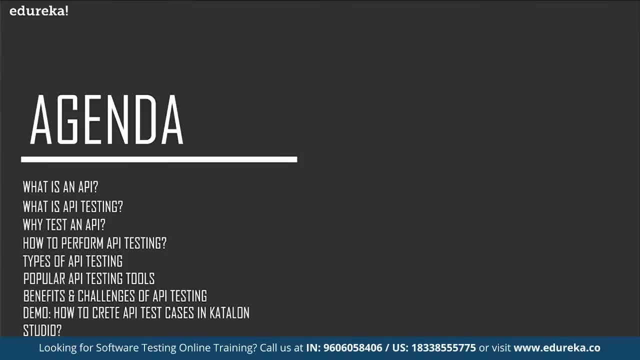 how to perform API testing, different types of API testing that there are in the market, and popular API testing tools. after that, we will discuss benefits and benefits of testing an API in the first place. So let's get started and the challenges that you might come across. 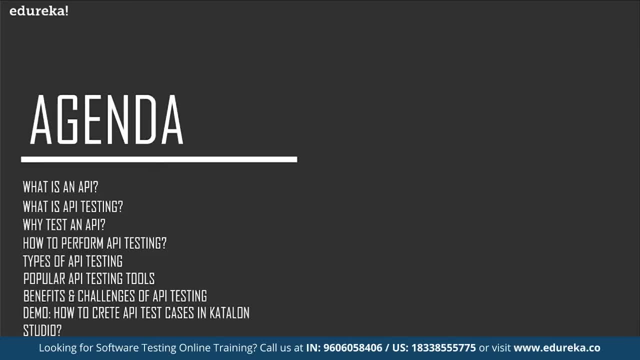 when you're performing API testing. and lastly, we will end the session by doing a demo or basically by creating an API test in a popular tool called Katalon studio. So I hope agenda was clear to you guys. Let's get started there, guys. 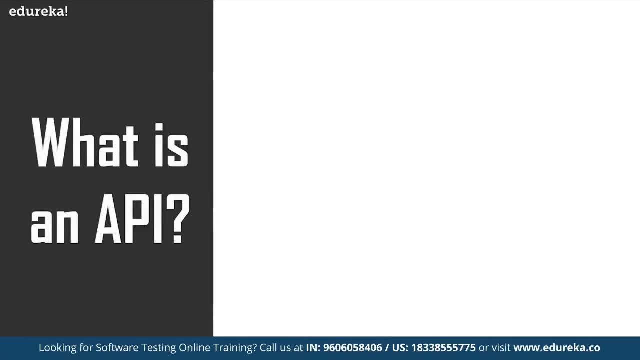 APIs have been around since 1960s, So if they aren't a new concept, why are they such a hot topic lately? Why do you think so? Because without APIs, the digital experiences that we expect every day as consumers would be different, wouldn't be possible. 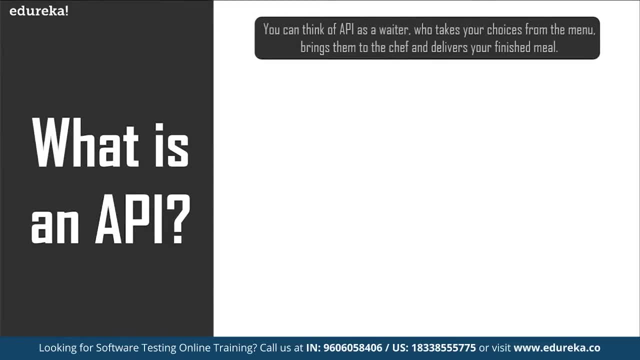 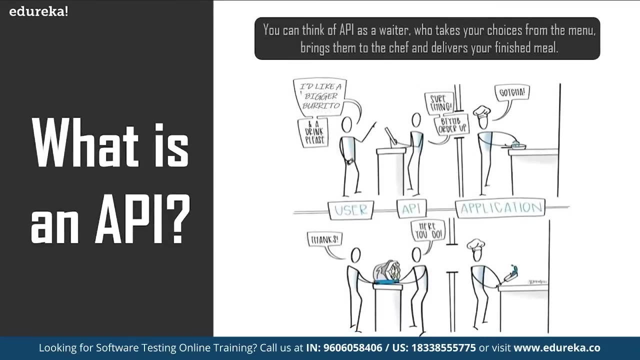 APIs are doing everything, from driving information, rich marketing campaigns to connecting mobile apps to streamlining internal operations. Well, here's a brief introduction to what APIs are and what they can do. to understand API is better, Let's consider a simple example. Imagine you're sitting at a table. 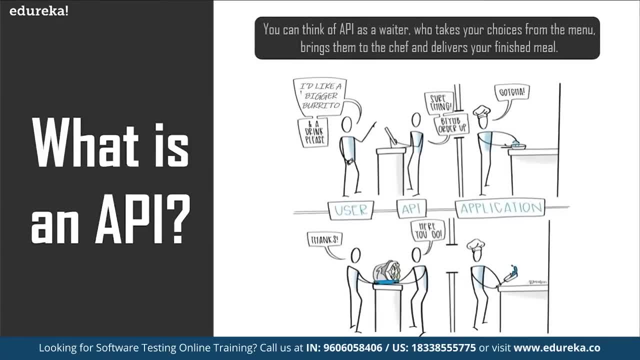 in restaurant with a menu of choices to order from the kitchen. here is part of the system that will prepare your order. What is missing here is that the critical link to communicate your order to the kitchen and deliver your food back to your table. That's where the waiter 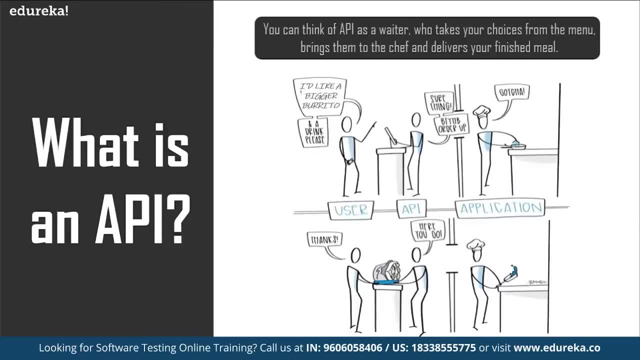 or an API comes in, The waiter is the messenger or an API that takes your request or order to the kitchen or the system and tells them what to do. Then the waiter delivers the response back to you. Well, in this case it is the food. 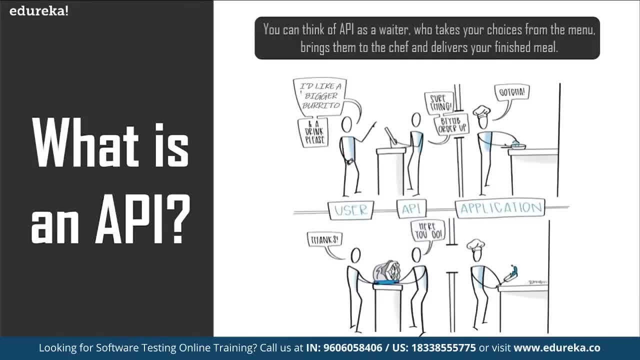 Well, put it in that way, It's easy to understand API, just like a waiter is a messenger between you and your application. Well, that being said, let's take a look at real-world example of an API. Let's see how we are using. 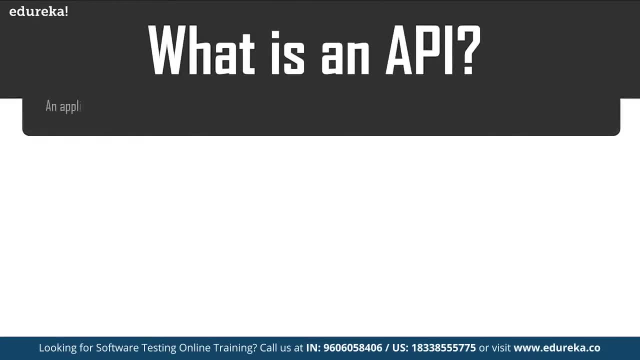 APIs in our daily life. Let's say you are searching for a hotel room from an online travel booking site. using the site's online form, You select the city you want to stay in, fill in the check-in and check out dates. number of guests, number of rooms. 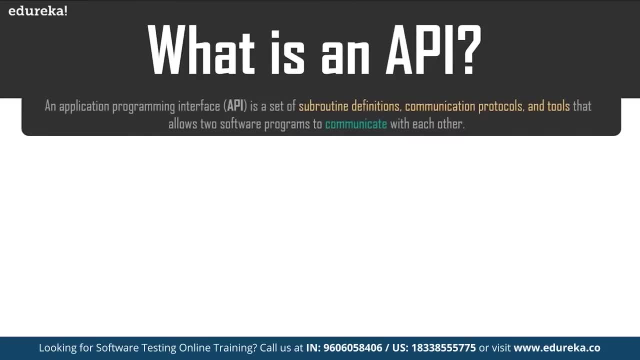 and other information. Then you click the search button. So what's going on between you entering your information and the application displaying you the choices APIs? That's what. so, as you know, the traveling site aggregates information from many different hotels. So when you click search option, 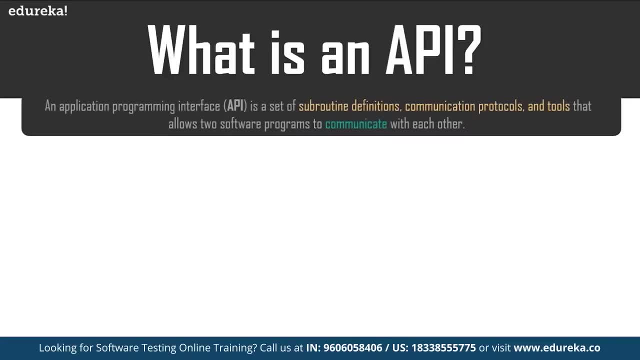 the site, then interact with each hotel's API, which delivers the result for variable rooms that are available according to your choice. This can all happen within seconds because an API which acts like a messenger and runs back and forth between your application database and devices. Now you understand. 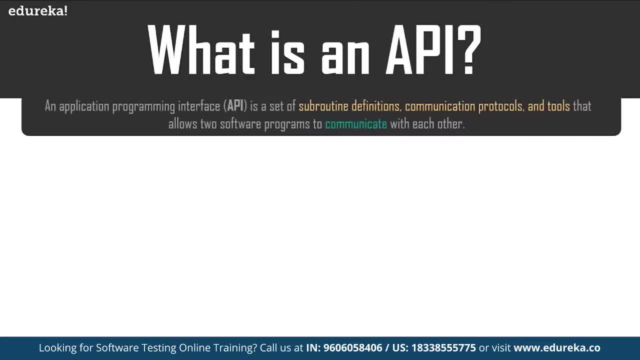 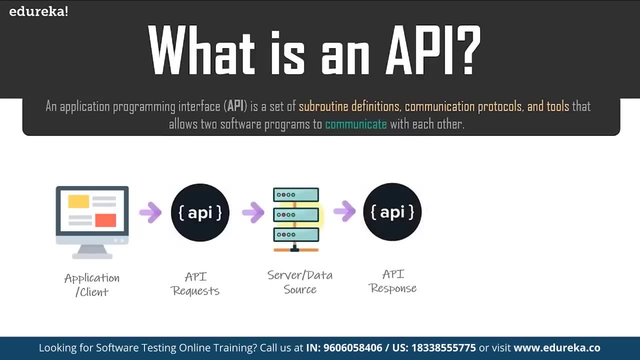 what I meant when I was comparing API with a waiter. So it's basically a messenger. API is an acronym for application programming interface, which is a software intermediary that allows two applications to talk to each other without any glitches. So every time you use 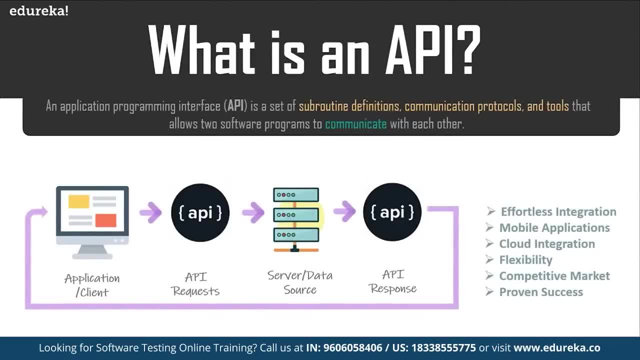 an app like Facebook to send an instant message or to chat with your friend whenever you check whether on your phone you're using an API. So why use an API? What are the main reasons? First of all, it offers effortless integration. It allows customers. 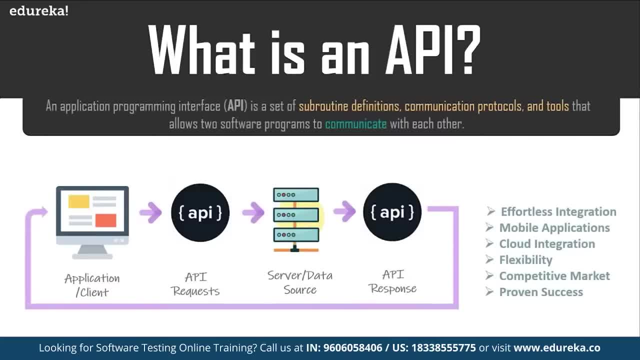 to access data server or any other application in very stable and secure way. Secondly, mobile phones and devices embedded with sensors fit perfectly with the service-based structure of API. So, as you know, cloud computing is already in rise. APIs are mainly needed for both the initial migration. 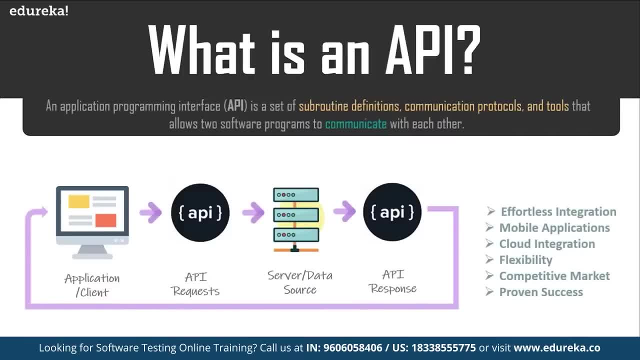 and integration with other systems in the cloud and next APIs offer flexibility That allows you to quickly leverage and use your desired services on mobile and web, and the IT market is rising, So everyone wants their product to be best, which depends on how intuitive and usable. 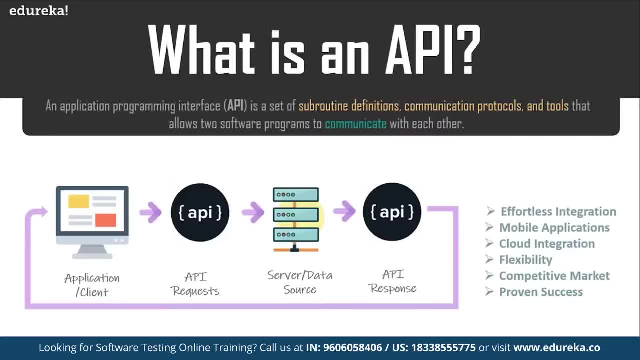 their API is. And, lastly, there are a number of applications and, lastly, the huge success of APIs. If any company has employed or deployed API and has been successful using that, then other companies also want to do as well. So because of these reasons, 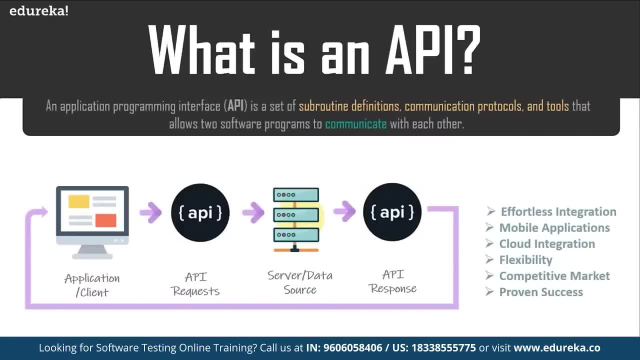 API is very popular these days. as you know, software is exactly not perfect every time. So, guys, now you know why is this so much hype about APIs. APIs of what gives value to your application, It's what makes our phone smart and it's what streamlines. 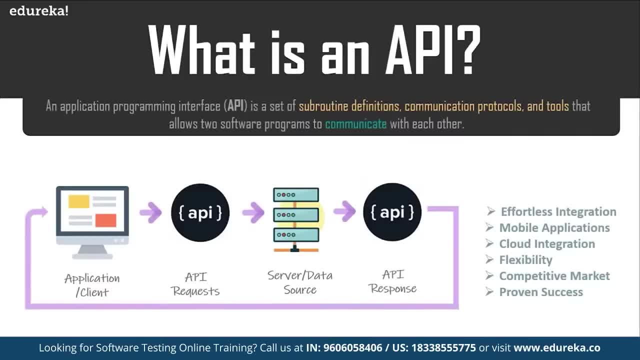 business processes. So if API doesn't work efficiently and effectively, it will never be adopted, regardless if it is free or not. Also, if an API breaks because errors weren't detected, there's a threat of not only breaking a single application, but an entire chain of business processes. 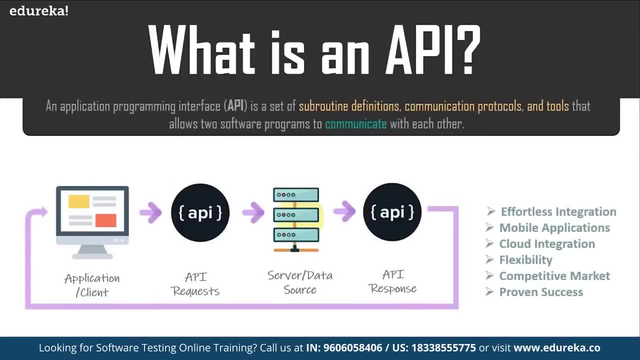 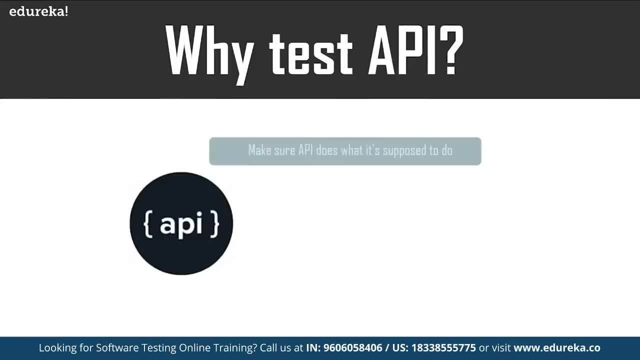 hinged with it. So the solution: to test APIs before they're put to use. here are the most common reasons as to why you should test your APIs before putting them to use. First of all, you want to be sure that they're doing what they're supposed to do. 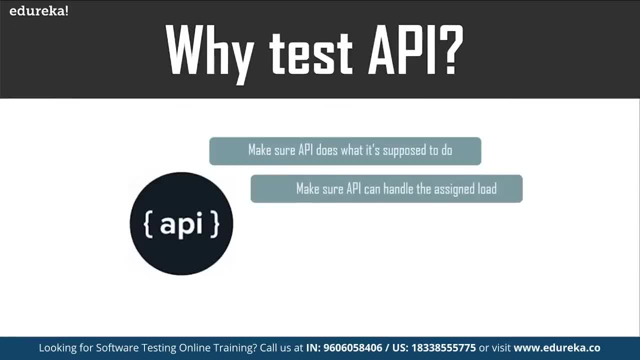 you want to make sure the APIs are handling the maximum load or the amount of load that's been assigned to them, and you want to find all the way users can mess things up when they're using the applications that are linked with API. You also want to make sure 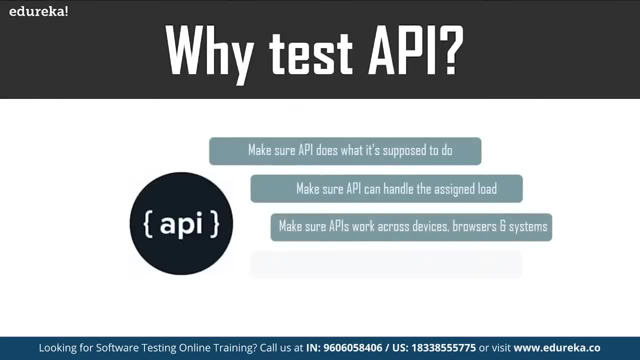 your API is work across different devices, browsers and operating systems. and, lastly, if you don't test your API, it can be costly for you later on. So these are the simple reasons as to why you should test your APIs before putting them to use. So basically, 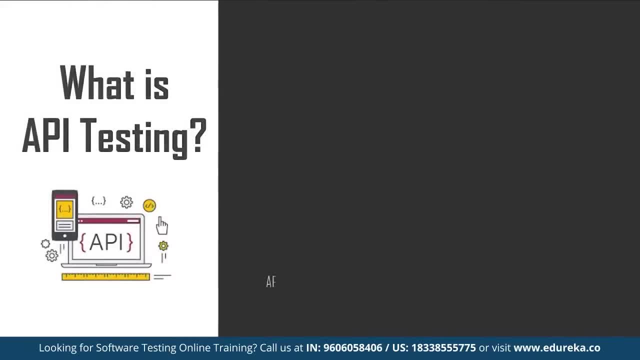 the entire process of testing these APIs is what you call API testing. It's a type of software testing that involves testing your application programming interface, or APIs, as a part of integration testing, to see if the meet expectations for functionality, reliability, performance and security. So, as you can see, 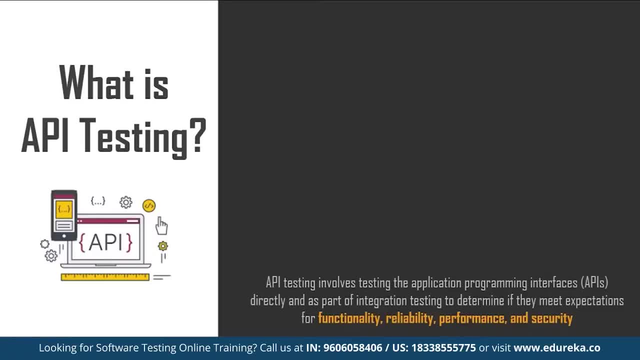 I'm stressing on four words here. So basically an API testing: you check if API's meet expectations for functionality, reliability, performance and security. most basic level API testing is a test that is intended to reveal bugs, inconsistency or derivations or deviations from the expected behavior of an API. 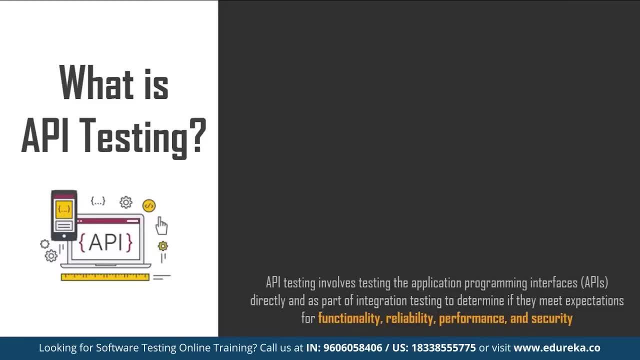 and obviously the next question that follows, after knowing what API testing is, where do you perform API testing? since APIs lack a graphical user interface, API testing is usually performed at the message layer and can validate application logic very quickly and effectively. there sort of putting it that way. 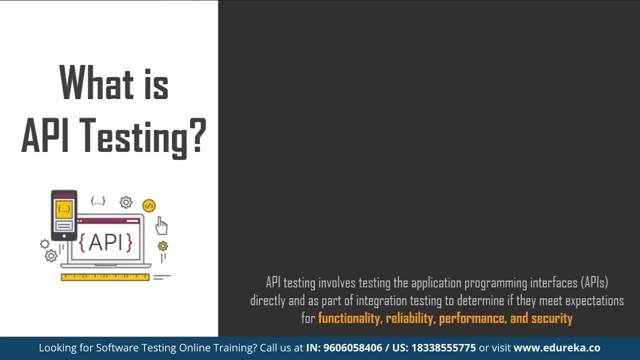 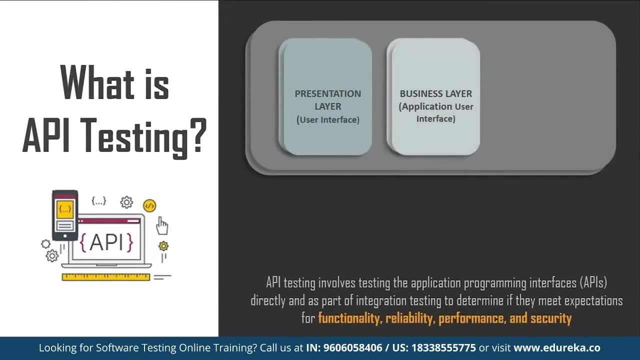 Let me make it more simple to you guys. commonly applications have three steps of plate layers or tires. You can say: first comes is presentation layer or user interface. Then you have business layer, application user interface. or you can say for business logic processing, and then you have database layer. 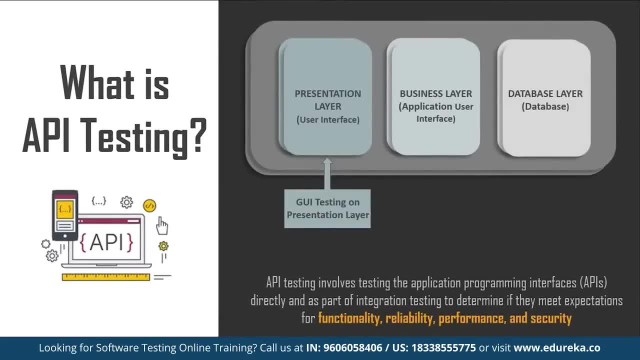 for modeling and manipulating your data. So application programming interface testing is performed at the most critical layer, which is the business layer, where business logic processing is carried out and all the transactions between user interface and the database happen. So basically, an API testing, our main focus. 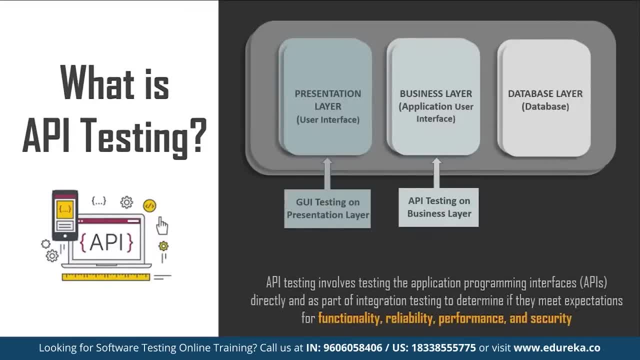 will be on business logic layer of the software architecture. and I have to tell you guys, API testing, like graphical user interface testing, won't concentrate on the look and feel of the applications. So it's entirely different from graphical user interface testing. and API testing also requires: 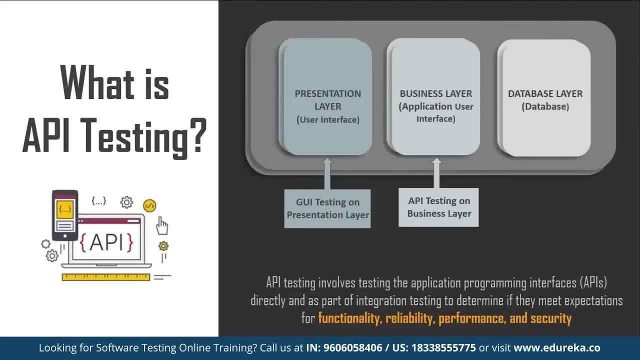 less maintenance and effort when compared to GUI testing, which makes it perfect choice for agile and devops teams. So making sure that API offers complete functionality allows for the easy future expansion of API testing, which is the easy future expansion of the application, if you want to do so. 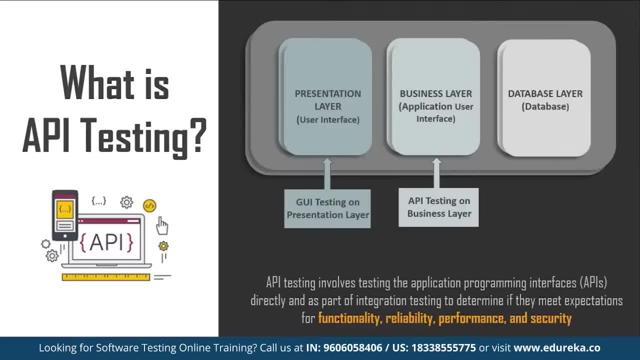 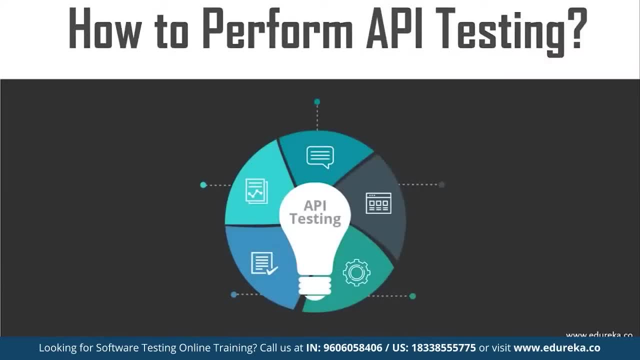 later on in the future. So that's what API testing is all about. So, now that you know what API testing is and where you perform API testing, how do you actually go ahead and proceed or perform API testing? Well, it's a five-step process. 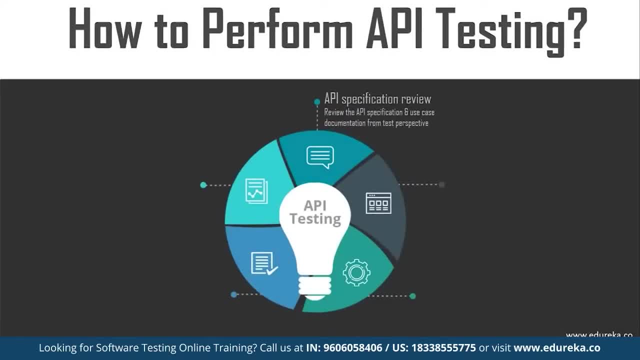 First step is documenting the API testing requirements, like: what is the purpose of API? What is the workflow of your application? What are the integration supported by the API here or in your application? what are the features and functions of the API that you have included in your application? 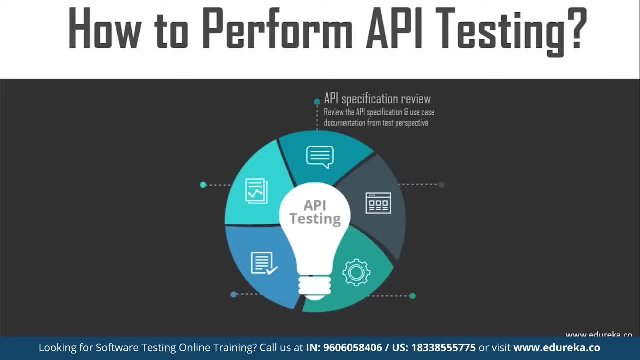 Documenting all these API testing requirements is the first thing you need to do. This will help you in planning API test throughout the testing process. So the first step is just preparing a plan. Next step is setting a test environment according to your plan. 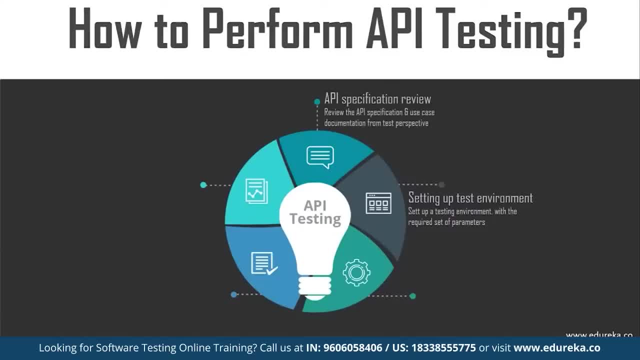 So you'd set up testing environment with the required set of parameters around the API. This involves configuring the database and the server for the applications requirements. Next step is setting up test environment according to your plan. So once the setup is done, it's good to make an API. 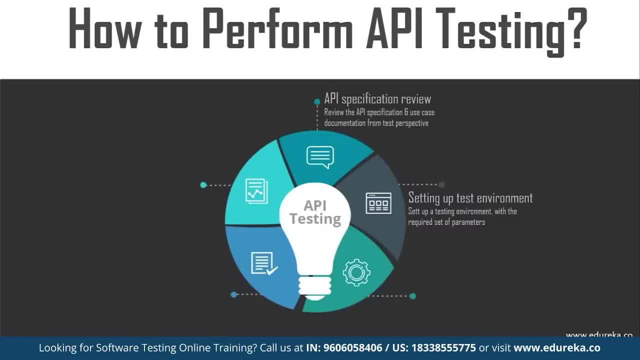 called right away to make sure nothing is broken before we move forward with any kind of testing. So the next step is to combine your application data with your API test to ensure that API is functioning as it is expected to, under different or basic conditions. or you can say: 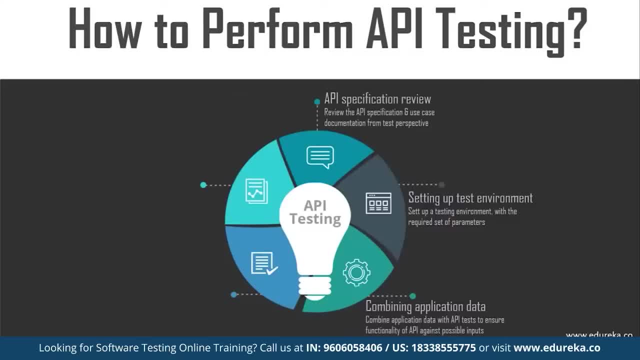 different input configurations, and then you need to organize yourself around the API test. for that You need to start asking questions like: who is the target audience here? Who is your API customer? What aspects are you testing? What problems are we testing for? What are your priorities? 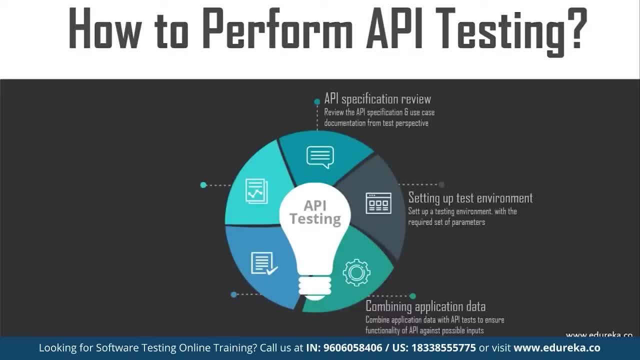 to test What could potentially happen in such circumstances. Now, after performing the test, when you should consider test as a pass or a fail, What other APIs could this API interact with? and so on. like that, many different questions. So, after you have created these testing, 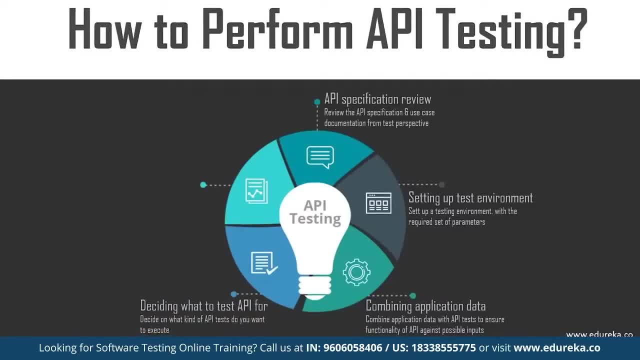 boundaries and requirements. you need to decide what you want to test on your API for while. we will look into what kind of API test we can perform in the next part of the session, So I leave that step blank for a while, which is our fourth step. 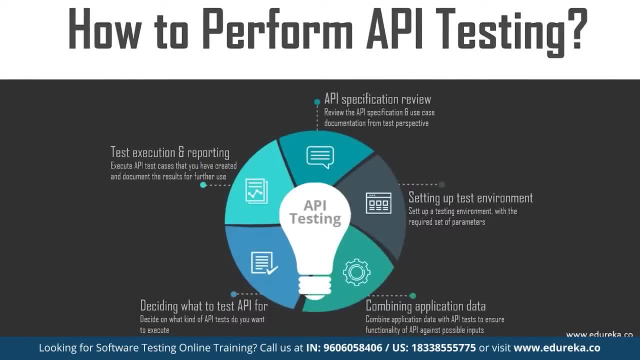 designing on what to test API for. and finally, once you have decided, the next step obviously is to create test cases around the requirements and execute them. a basic guideline is to identify the most common parameters and conditions that an end developer will use when calling the API and, based on that, 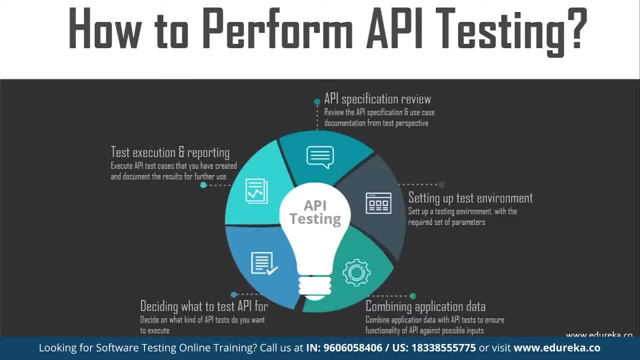 you should create your test cases and execute the test, and I'm sure the last step is the common step. So you create the test results and give it for review. So let's just summarize what are the steps. the first step is preparing a documentation or a plan. 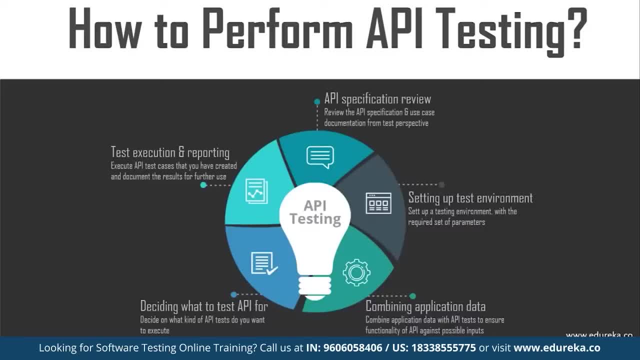 on what you're doing or you're trying to do, then, according to the plan, you set up your test environment, then you combine your application data with your API test to make sure that your API is working perfectly under different input configurations, and then decide on what kind of API test. 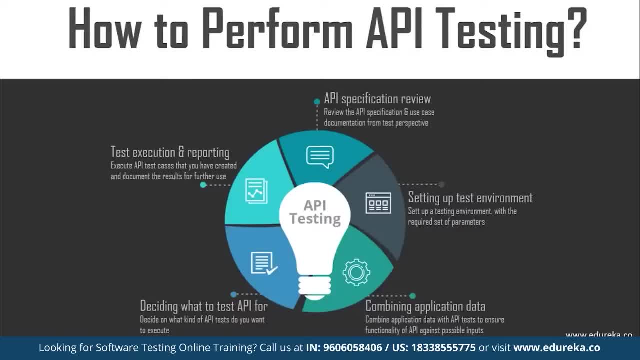 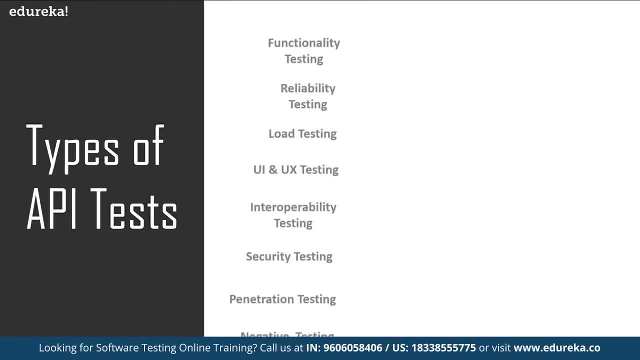 you want to perform and, lastly, create the test cases based on your requirements and execute the test. and create the test. and it's that easy. So one of the most important step while performing API test is to decide on what kind of test you want to perform. 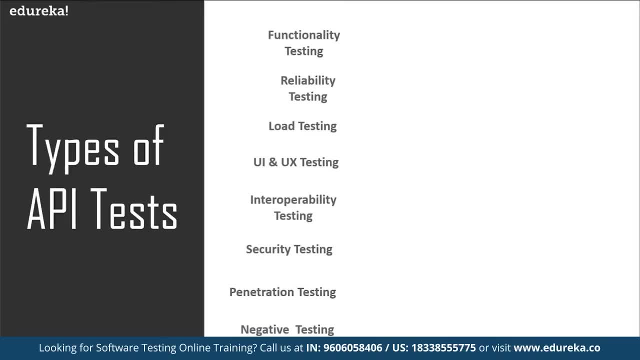 for that you should be aware of different types of API testing. as you can see, there are multiple types of API testing. first you have functionality testing, the basic testing. so you perform functional test to check if the API works and does exactly what it is supposed to do. functional testing: 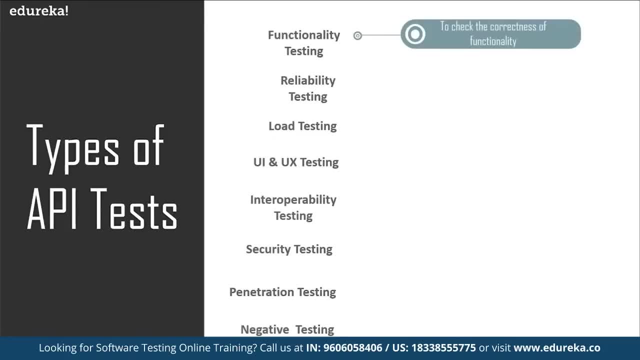 includes testing of a particular functions in the code base. So that's what functional testing is. it's all in the name. then you have reliability testing. basically, here you're checking if API can be consistently connected to whenever you want and lead to consistent results always. and then you have 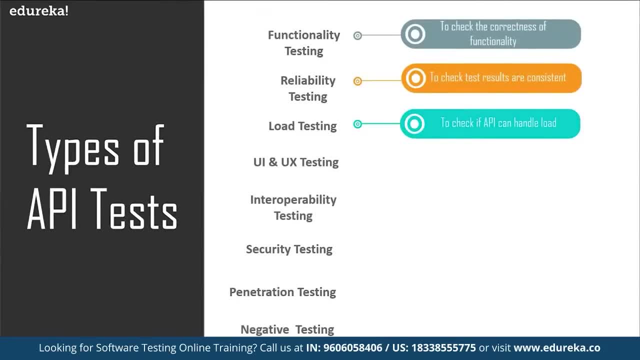 load testing. well, load testing, you can say, is a test which is obsessed with reality. here you ask yourself: you test your API on different scenarios like: does this code of my API work in theory? will this code work with 1k requests, 10k requests and 100k requests? 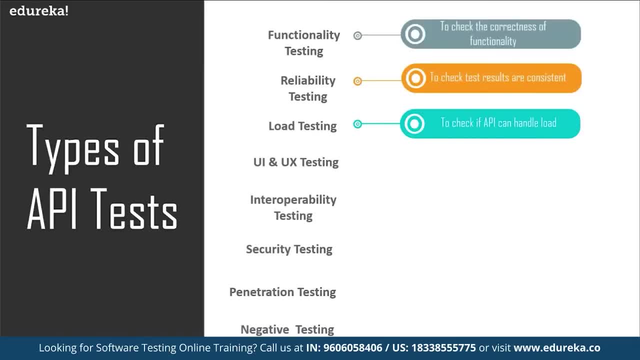 so basically you're trying to check if API can handle the load. load testing is basically performed to ensure that the performance under both normal and at peak conditions is normal for an API. you have different scenarios under that. for example, you have baseline scenario. it tests the API. 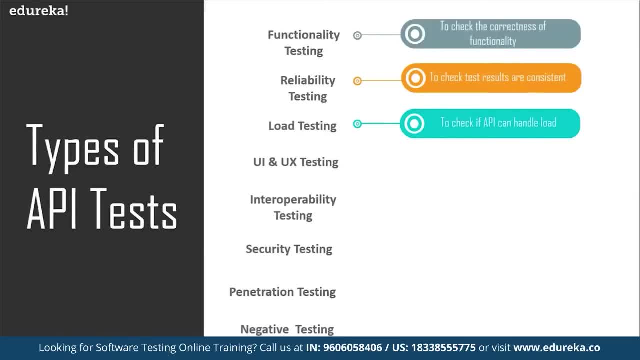 against textbook values, regular traffic that API expects in an ordinary usage. then you have theoretical maximum traffic, that is to make sure during the full load periods the solutions respond to the request properly. then you have overload test to test the maximum capacity according to the theory. maybe then add: 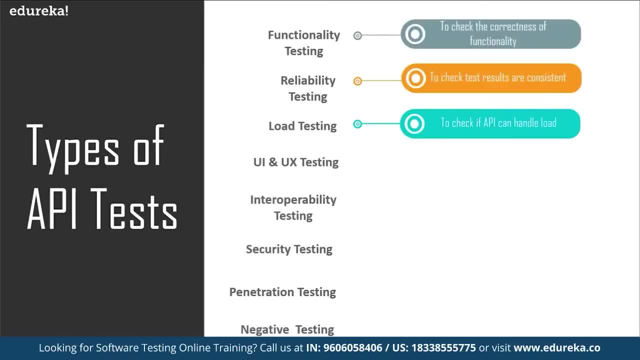 20% more to the peak traffic. So this way you have different kind of load testing and then you have end-to-end testing or UI and UX testing. it involves testing user interface for the API and other integral parts. interface here naturally can be graphical user interface. 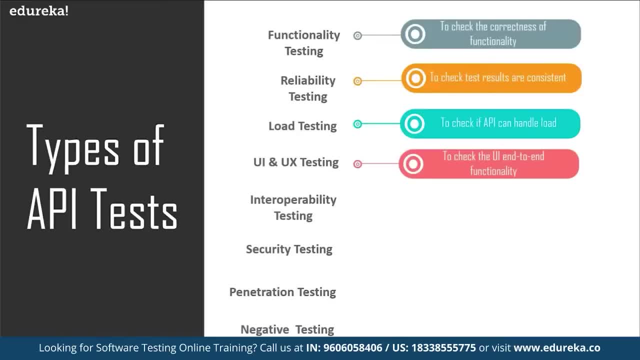 to GUI, or it can rely on the command line endpoints as well. and then you have interoperability testing and compliance testing. this type of testing applies to SOAP APIs. it ensures that the predefined standards of your API is met. and then comes security testing. security testing, penetration testing. 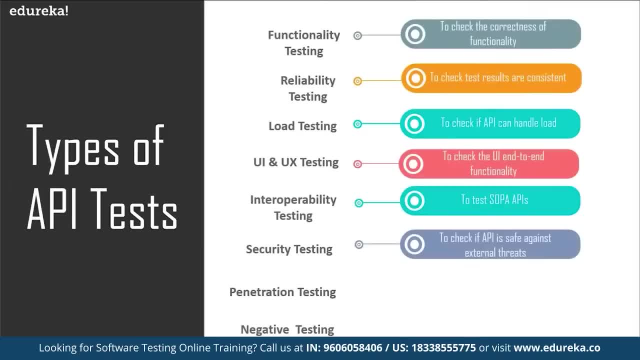 and first testing are the three separate elements of security auditing process. they are used to ensure that the API implementation is secure from external threats. that's the common point for all security: penetration and the first testing. so besides enclosing with penetration and first testing, security testing also includes. 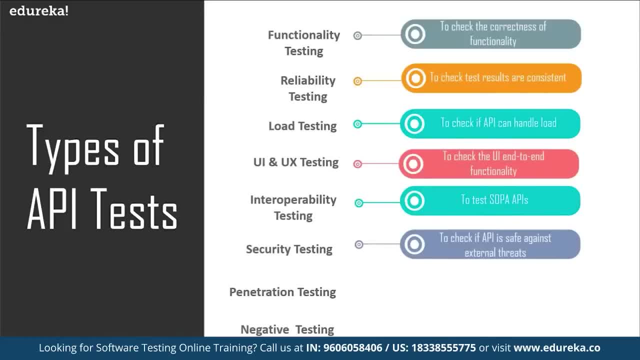 additional steps like validation of encryption methodologies and of design of the access control. and then comes penetration testing. it's considered the second step in the security auditing process. in this testing type, users with limited API knowledge will try to attack to access the threat vector from outside perspective. 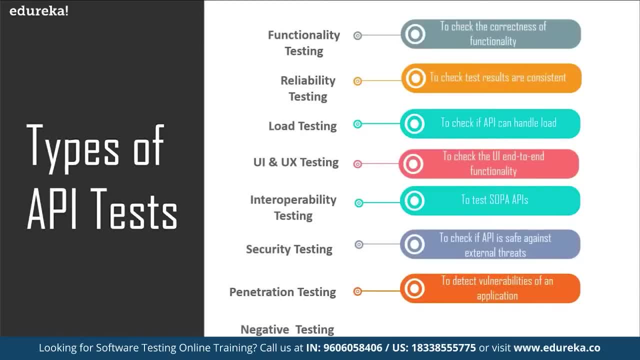 while it's all about functions, resources, processes, or sometimes it can be an entire API from the outside perspective. and then comes first. testing is another step in the whole audit process. in this testing type of vast amount of random data which you usually refer to as noise in the system. 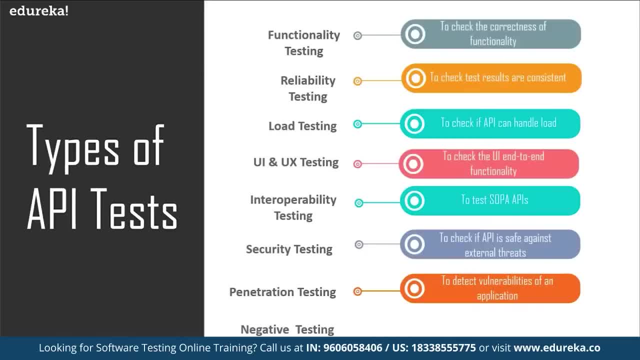 with the aim that they want to forcefully crash the system and see what happens. this way, when there's an actual threat from the outside, they can react back to it very quickly. that's what first testing is all about. so, basically, first testing will help the API in terms of. 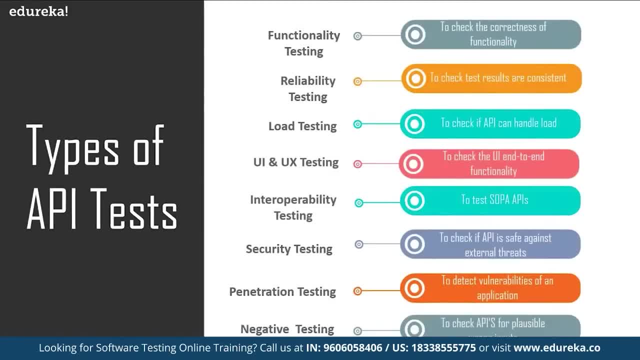 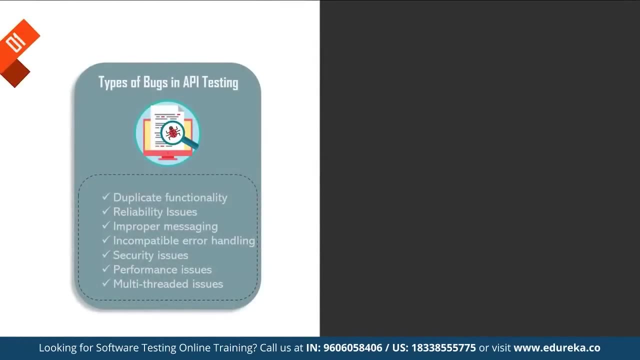 limit to prepare for the worst case scenarios. with that said, these are the most frequently performed API tests. so, by performing this test, what are you trying to test for and what will you find? so, basically, by performing this test, you are looking for duplicate or missing functionality or improper messaging. 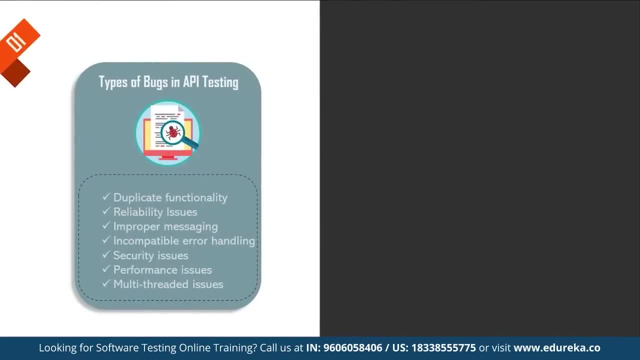 multi-threaded issues, or performance issues, or it could be about incompatible header handling, or it could be about reliability issues. so, basically, by performing all this different kind of API test, you are trying to find these kind of bugs. since API testing is gaining popularity, we have many tools. 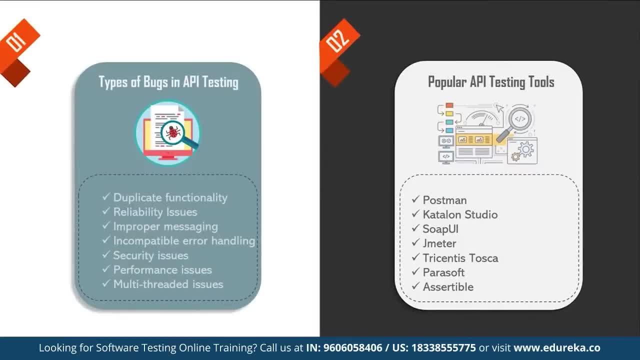 available for performing the same. here are some of the top API testing tools that you can use for rest and soap, for example. you have postman. you have Kataloon studio. Well, will be using one of these, which is Kataloon studio, to see how to create. 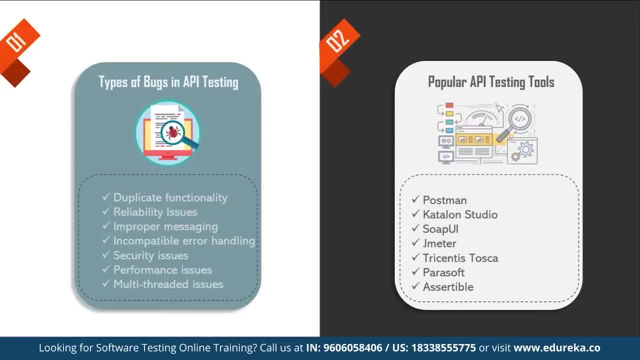 API test. then you have soap UI, then you have Tosca, Parasoft, assertable. Well, these are very few. basically, I just listed the most popular ones. apart from these, there are many other tools outside, while you can choose any one of them according to your 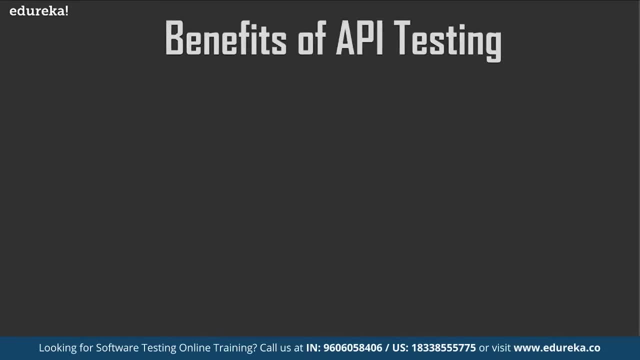 requirements and comfort. now let's discuss benefits and challenges of this important activity The testing team should focus on. it offers a number of advantages over other kinds of testing. For example, first of all, it's language. independent data here is exchanged via an XML. 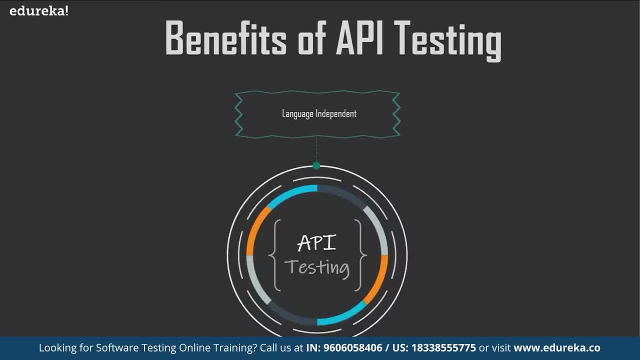 or Jason format, So any language can be used for automation, independent from the languages used to develop the application. XML and Jason are typically structured data, So the verification is literally very fast and stable in these XML without comparing data in different data formats. So the first reason: 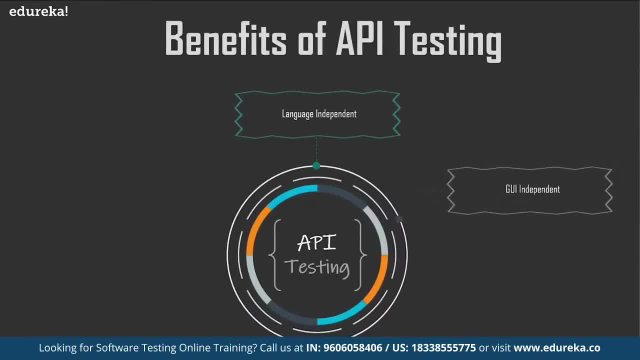 is its language independent, then its graphical user interface independent or GUI independent. we can perform API testing within the application prior to GUI testing, and this early testing will help you get feedback sooner and so that you can improve the team's productivity. core functionality can be tested to expose small errors. 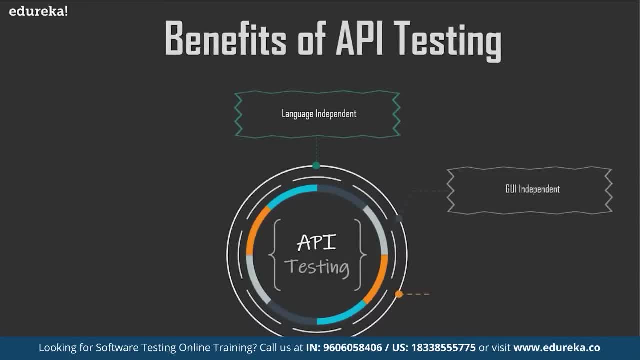 and evaluate team strength or your application built strength, then it offers improved test coverage. Most API services have specifications allowing us to create automated test with high coverage, including functional testing and non-functional testing as well, and nowadays there are multiple techniques which are available, using which you can find: 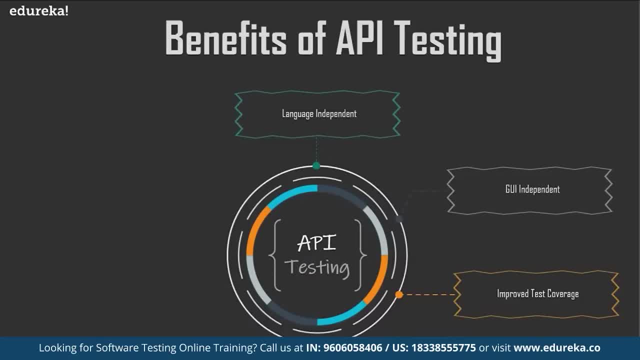 API test cases that could not be automated. So this way you can improve the test coverage by using either manual API testing or automated API testing. and another most important benefit of API testing is it reduces testing costs. API testing helps us to reduce the testing costs with API testing. 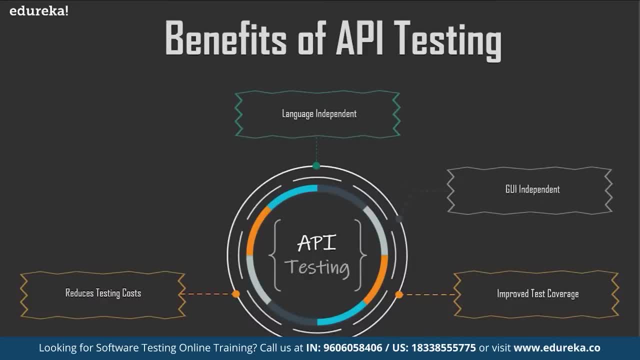 We can find minor bugs, Like I said before graphical user testing. these minor bugs will become bigger during graphical user interface testing. So finding this bug in early stage itself is a very good process and will beneficial. and, lastly, API testing is a step for faster release. 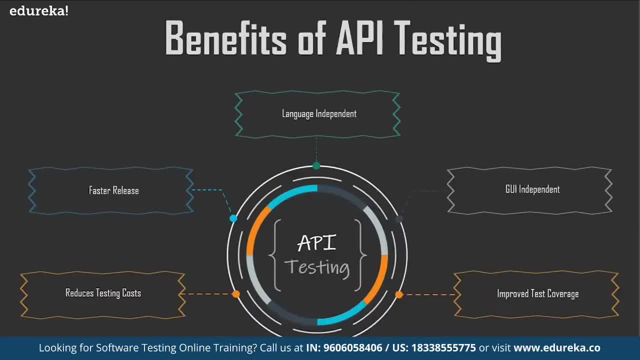 It's common that executing a UI regression test takes about 8 to 10 hours, while the same scenario with API testing takes only 1 to 2 hours. You see the difference there, right? The effectiveness of API testing is also lower than that of UI testing. 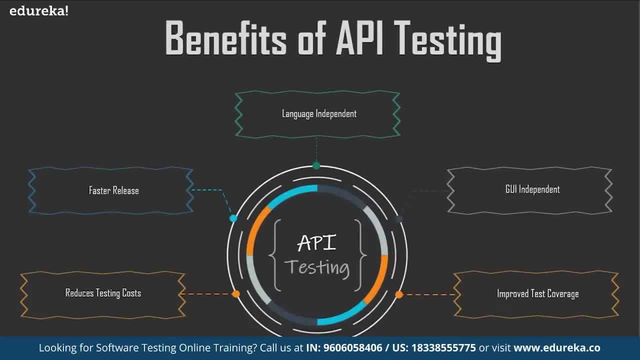 All these allows to release are built faster with API testing. So these are certain benefits that you get out of performing API testing before putting your API to use its language independent. So, basically, you can use any language, irrespective of the language the application is developed on. 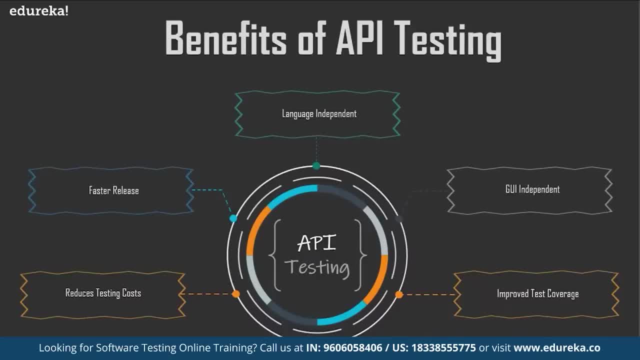 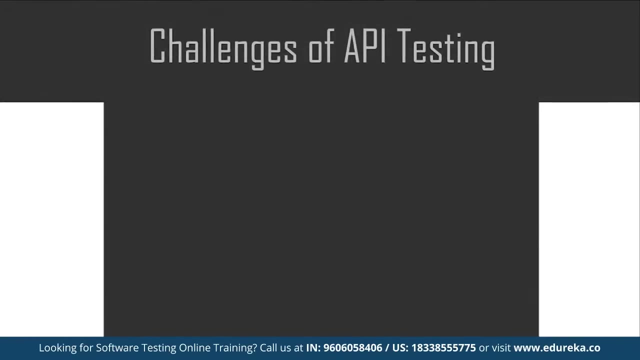 its graphical user independent. You can find out the bugs in early stage. because of that, the testing costs are also released. I mean reduced offers, improved test coverage and faster release as well. Well, that's about the benefits, but again, like any other testing process, there are certain 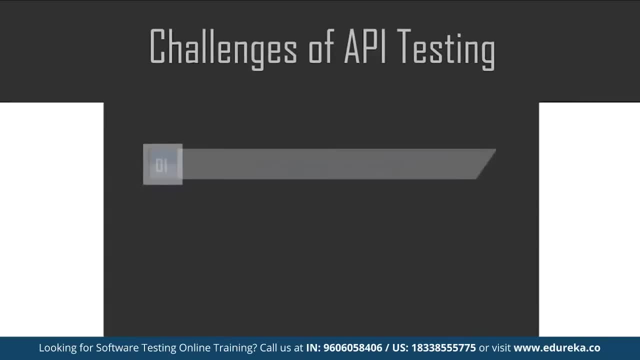 things that you will come across or you will feel difficult when you're performing just in API testing as well. The point of not having graphical user interface can be a benefit as well as a challenge. We discussed why it is a benefit. now let's see. 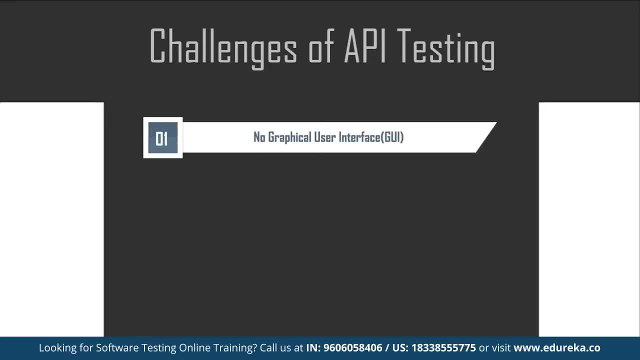 why it's a challenge. APIs are primarily intended for computer to computer communication. A computer doesn't need an user interface. This is a challenge if you're a tester who is used to testing applications designed for end users with a graphical interface where you can click. 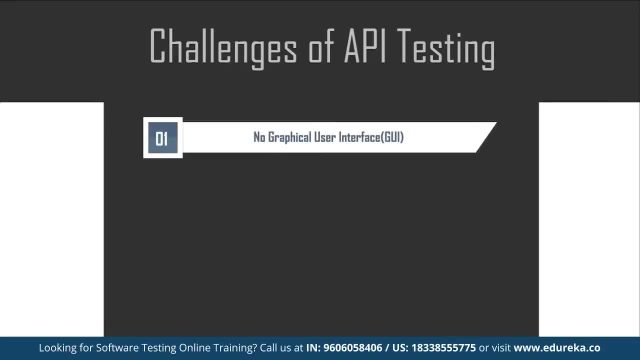 drag and in general manipulate an application or data visual. So, basically, if you are familiar with all those graphical user interface features, it might be difficult to jump into API testing. and then you have synchronous and synchronous dependencies. So often APIs rely on other APIs or other backend systems. 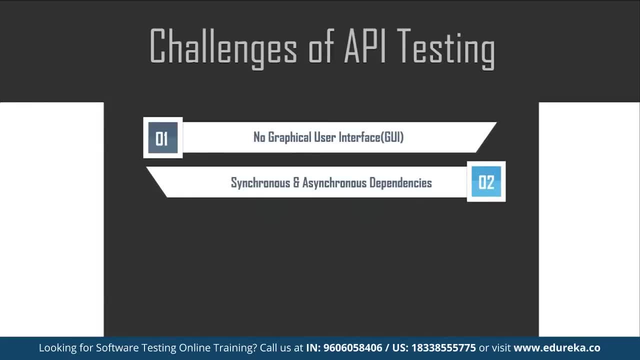 to function properly. So if any of these steps or systems are out of place, all the assertions connected to it will fail. So this way, when your API is connected to other APIs or any back instance like synchronous and asynchronous dependencies are there, then it might pose a problem. 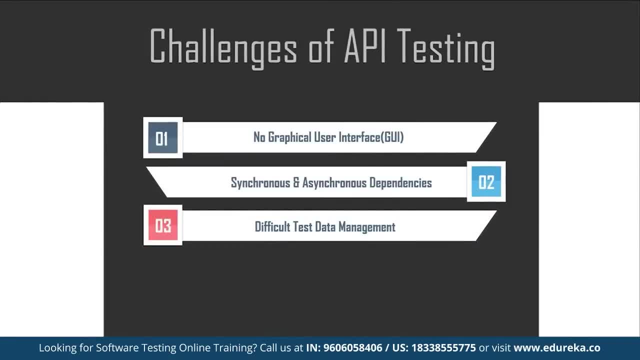 and during API testing it's difficult to test data management. So, basically, API testing verifies the business logic of an application layer which often has millions of permutation and use cases. So it can be difficult to propagate scenarios that sufficiently test your API boundaries. and then there's 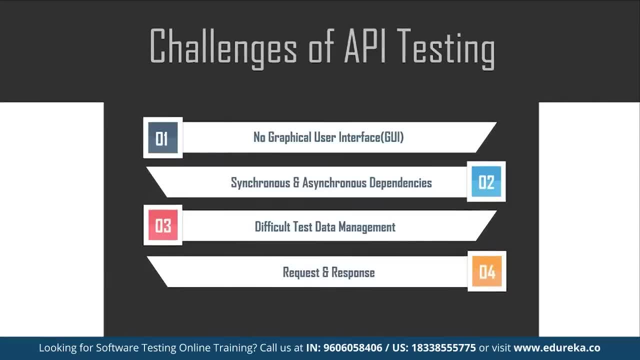 a problem of request and response. As stated before, APIs work on a request and response relationship. SOAP and REST APIs have different standards for the request and response calls that you will have to be familiar with before you actually start performing API testing, and that task can be difficult. 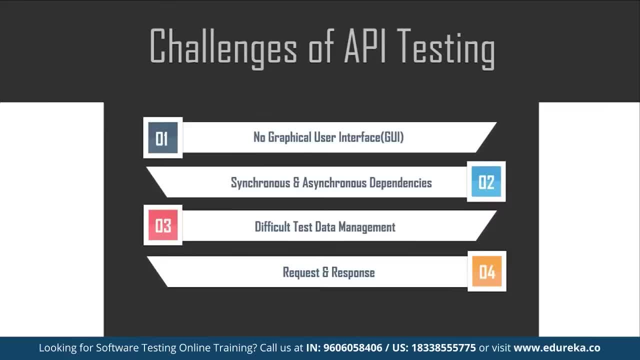 SOAP based API use XML as a communication protocol. that means, as a tester, you must be able to read, understand, create and update XML documents With REST based services. the request- for the most part, it only involves sending an URL to the service. Thing here is. 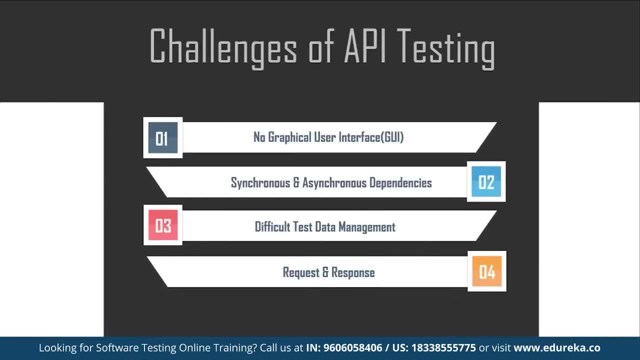 you need to have certain technical knowledge before you actually jump into API testing. that's very necessary. and lastly, there's no documentation and there are a lot of time constraints in API testing. The API is developed will hardly have any documentation. without the proper documentation, it is difficult. 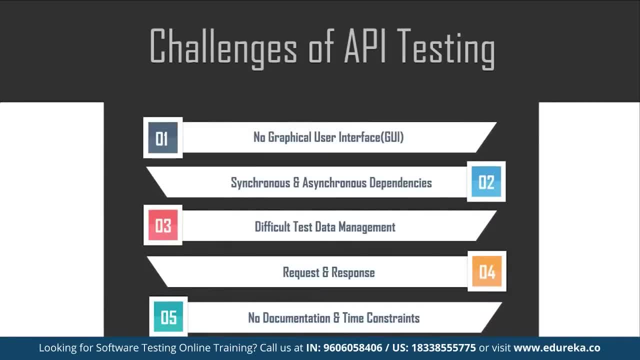 for the test designer to understand the purpose of these calls, parameter types, the possible valid and invalid values, the written values, the calls it makes and usage scenarios. to avoid that, like I said earlier, the first step of your API testing should be documentation. thorough testing of API is. 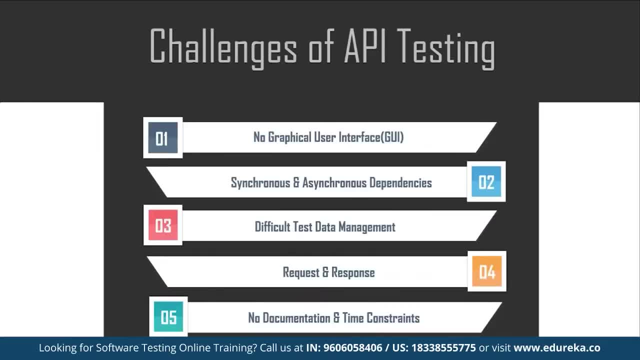 almost time-consuming. It requires a learning overhead and resources to develop tools and design tests that will suit your requirement. So these are certain challenges that you might come across while performing API testing. So, guys, that's all with the theory part, I hope at this point of time. 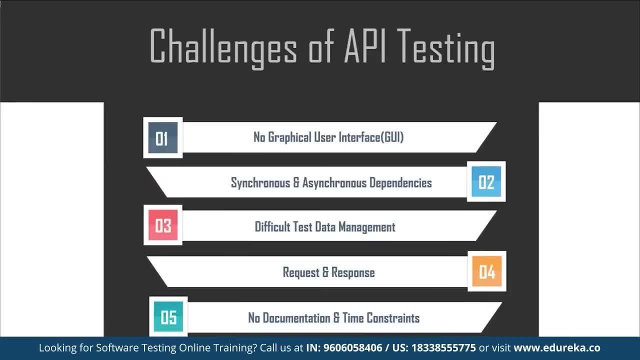 you're aware of what API is and why do you need to test your APIs before you put them to use and how to put them to perform API testing? Like I said, there are different tools which you can use to perform API tests, like you have Postman. 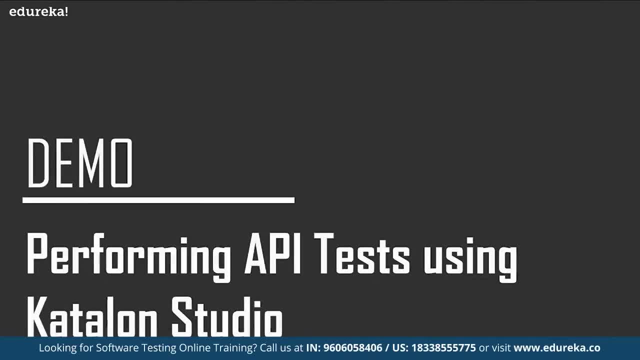 Katalon Studio, Parasoft, Assertable and many others. Now that we're aware of the theory part, let's go ahead and use a tool called Katalon Studio to see how to create API test cases and how to perform tests on API. 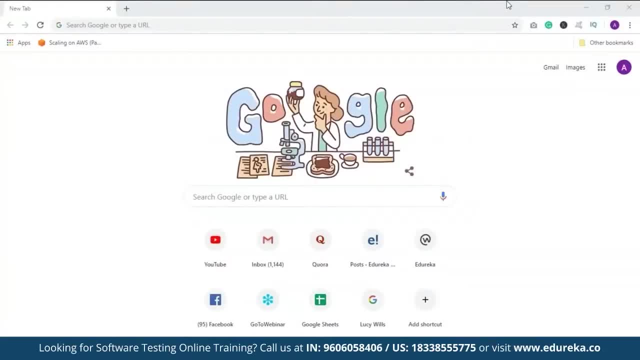 So, guys, in today's session, or demo, we'll be using a tool called Katalon Studio. So basically, Katalon Studio is a robust and comprehensive API's web and mobile testing. I already have it downloaded and installed on my PC. All you have to do. 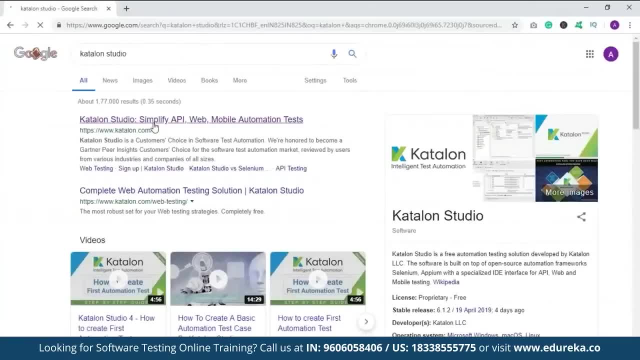 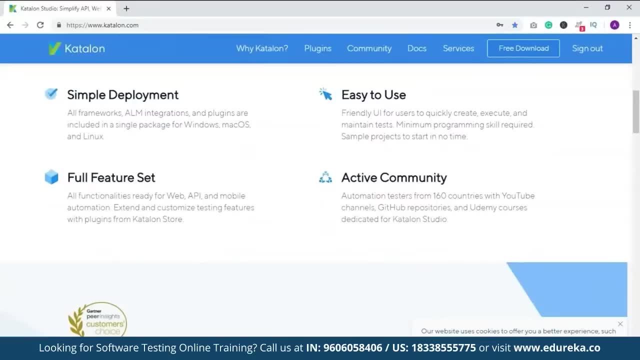 is search for Katalon Studio and you can just go for the first link that you find. So this Katalon Studio provides easy deployment by including all frameworks, ALM, integrations and plugins in one package. It has a unique feature, which is combining: 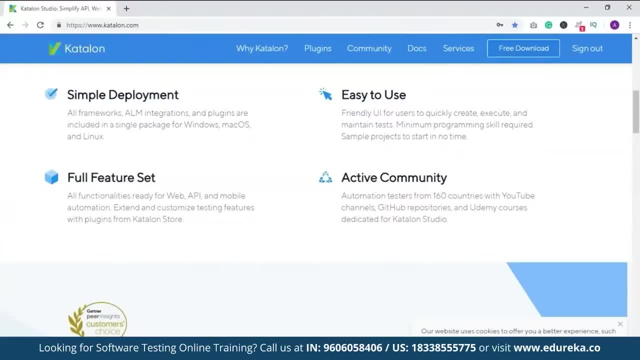 UI and API web services for multiple environments. Another thing is that it's a free tool and, apart from that, Katalon Studio also offers paid support services for small teams, businesses and enterprises. As you can see, the most benefits of using Katalon Studio. 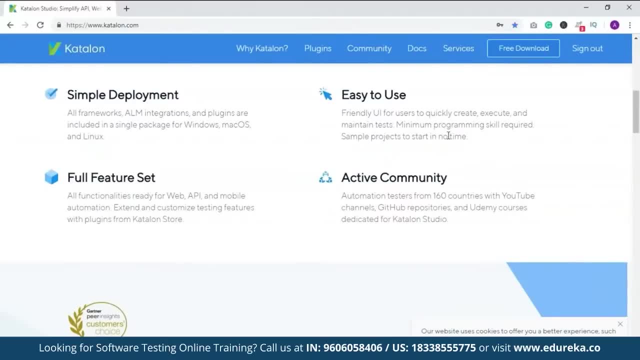 are listed here: simple deployment, It's easy to use interface and, like I said, it has a full feature package and it has active community of about people from different 160 countries across YouTube channels, GitHub repositories, Udemy courses. So if you face any problems or if you have anything, 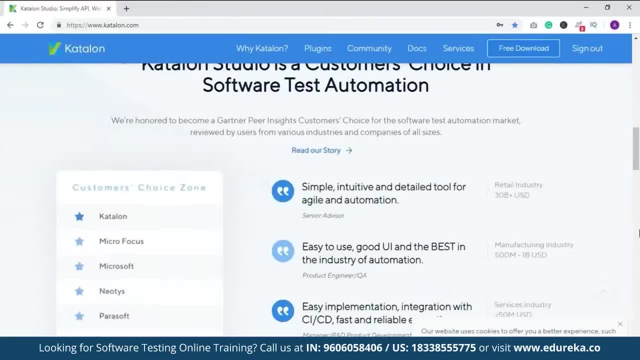 to contribute. you can go ahead and discuss your queries there. So the things that we might are interested today or we would be interested today about Katalon Studios that it supports both SOAP and REST request. SOAP and REST are two different kind of APIs. It also supports 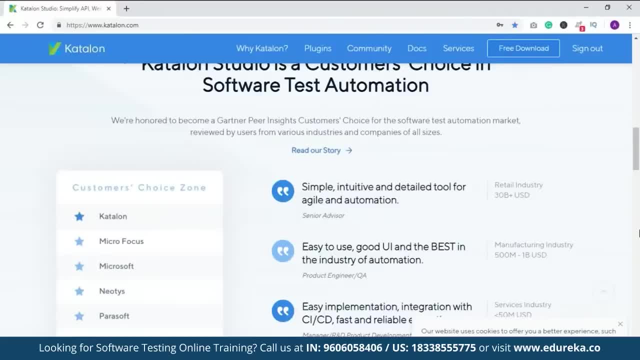 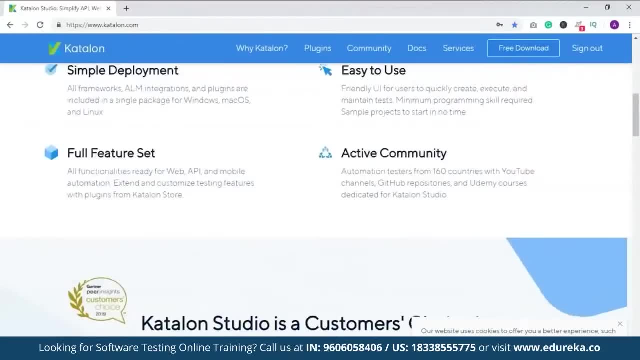 data-driven approach and it supports CI CD integration. apart from this, it has many other cool features that you can go ahead and research on. so I, like I said earlier, already have it installed. If you do not, you please go ahead and click on this download button. 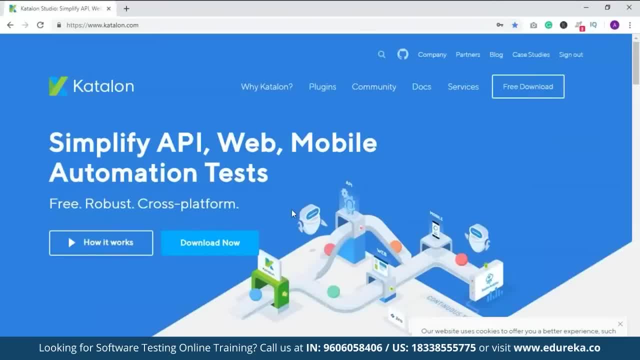 a zip file will be installed on your computer, or download it on your computer, can unzip it and install the application. Well guys, I am using this tool for no particular reason. There are many other tools which might suit your requirement and you're free to go ahead. 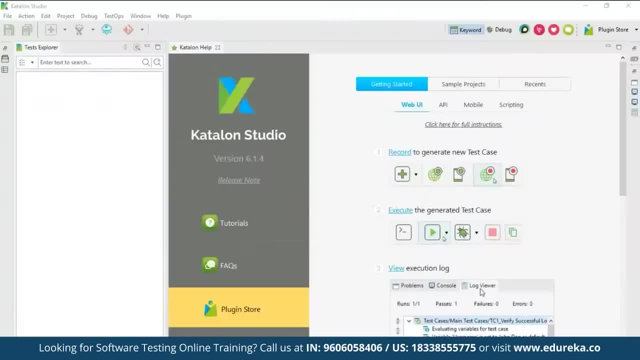 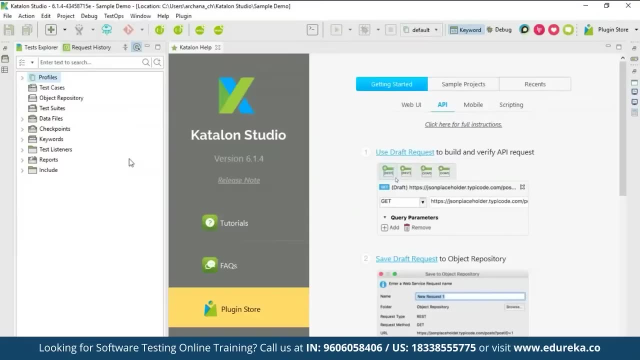 and use any of these. So let's proceed with the demo part now. So, guys, if you have installed Katalon Studio perfectly, then this is the home page where you will land on. So, as you can see, this page is basically what is known. 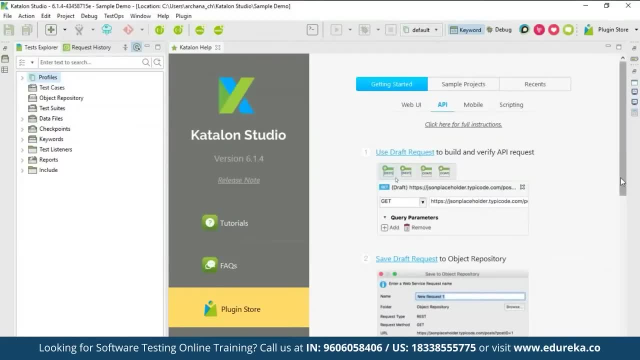 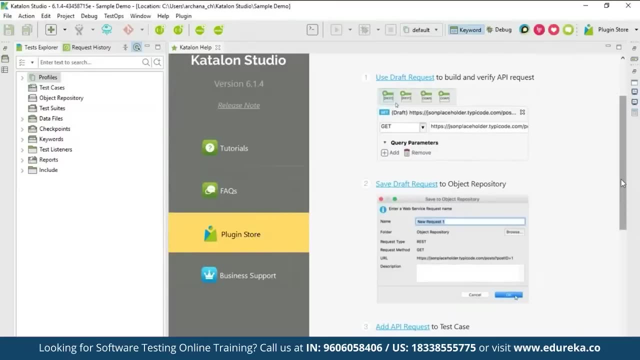 as Katalon help or you can say the documentation part. here You have the tutorials on how to use different features of this application. when you have different FAQs and different plugins that you can add, like I said earlier, you can use Katalon to perform test. 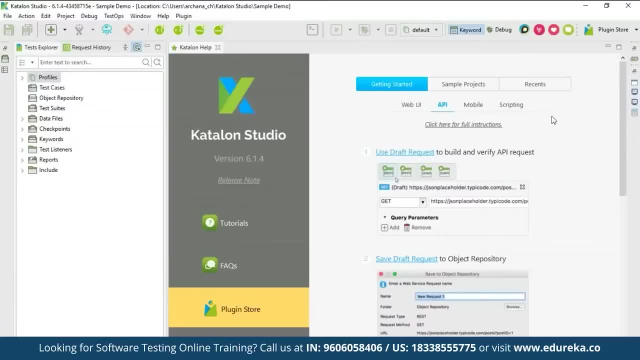 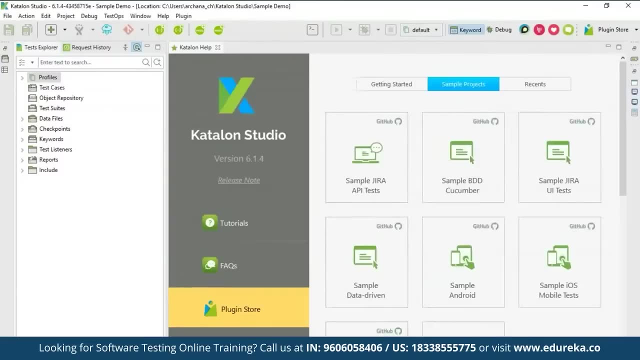 on web user interface, API, mobile testing and scripting as well. But as for today's demo, we are interested only with API. So you have getting started, as in the tutorials. here You have the sample projects that you can go ahead and start with if you're not familiar. 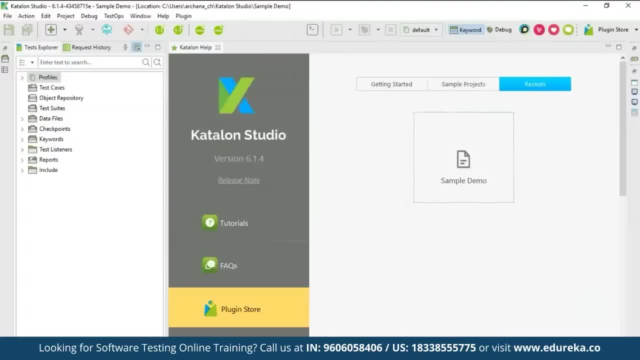 with the tool. then you have the folder which shows the reasons project that you might have done. So, as you can see, I've done a sample demo, so you can see it's showing a sample demo here. But if you have missed the page, all you have to do 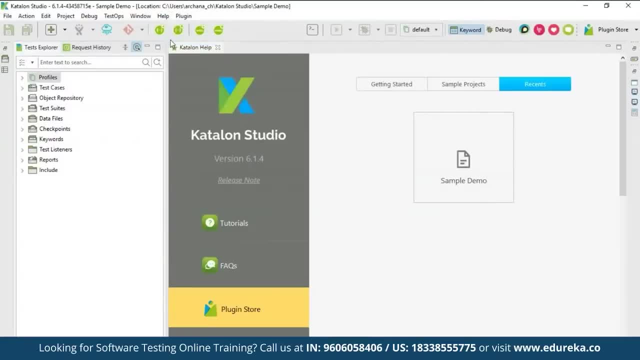 is go for help and you have Katalon help here. You can click on that and you'll land on this page again. So let me close the top. So if you have gone for API, the page will land on. is this page? 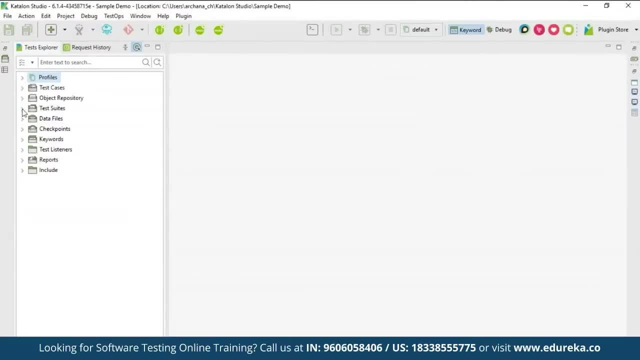 You can see the test cases object repository. You have tests, you data files, checkpoints, different keywords and you have test listeners, reports and other features or other plugins. We won't be using all these today for few, So the first thing you need to do is go ahead. 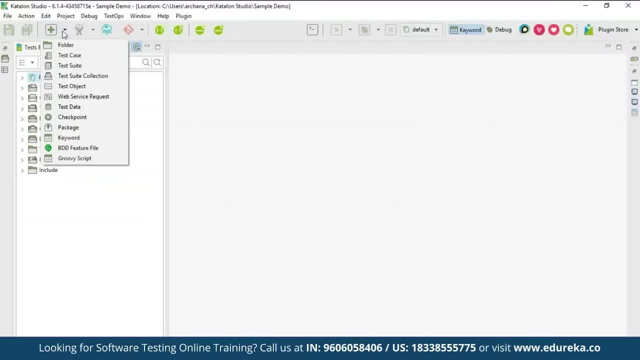 and create a project. You can see the plus a symbol of the new symbol. your click on that and go ahead and create a folder, Let's say testing API, and okay. So the first thing here is we need to have an API to perform tests on right for that. 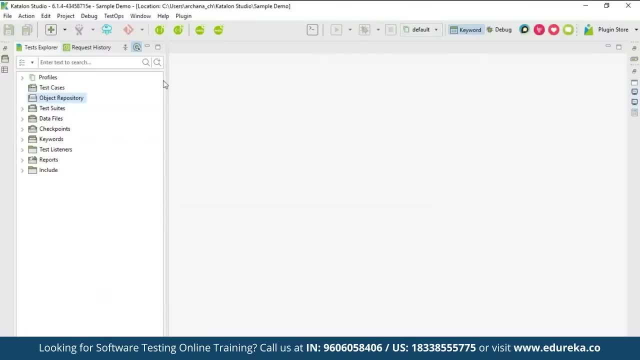 You can go ahead and search for sample APIs that are available on the net before. that will create a folder in object repository where you actually store your APIs. So go for new, create a folder, Let's say API testing, and okay, under this you can go ahead. 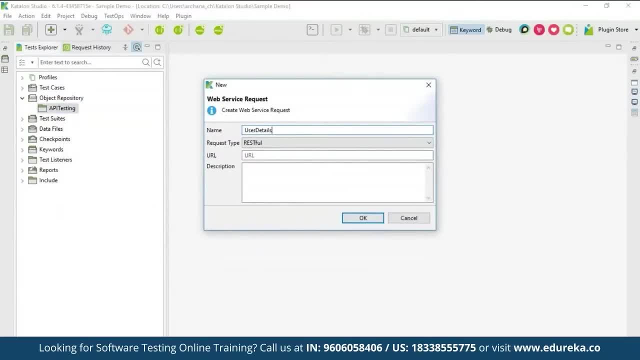 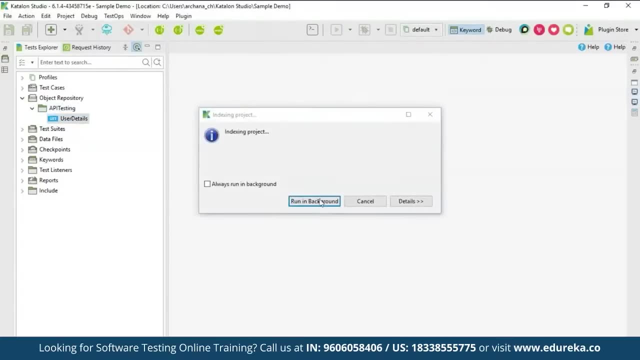 and create web servers request user details. It's a restful API for now. since we don't have URL, Let's just leave it blank and click OK. So, as you can see, it's ready here, but the only thing that we need here is an API. 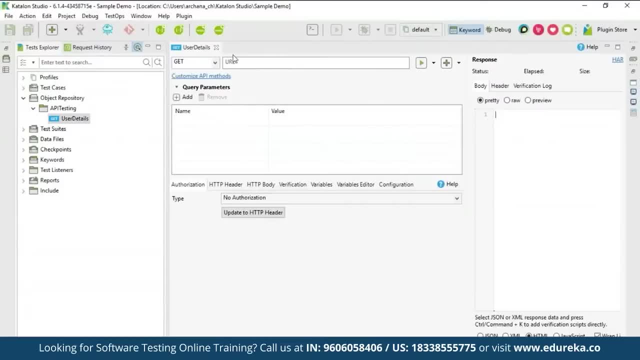 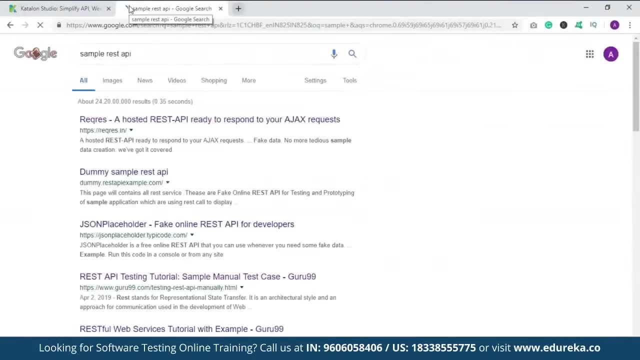 or sample API to perform tests on. for that We have a Google. all you have to do is I'm going to search for sample APIs. So, like I said, guys, there are different APIs: rest API, So PA API, but for today we'll be checking out. 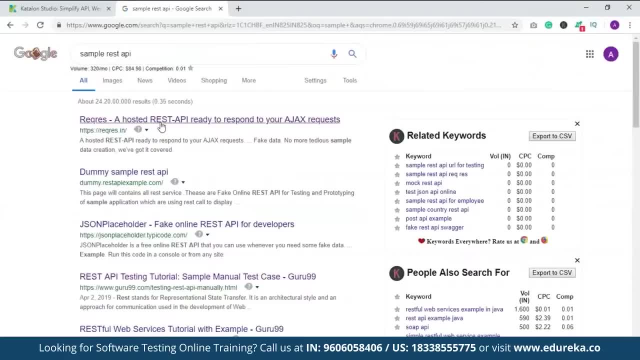 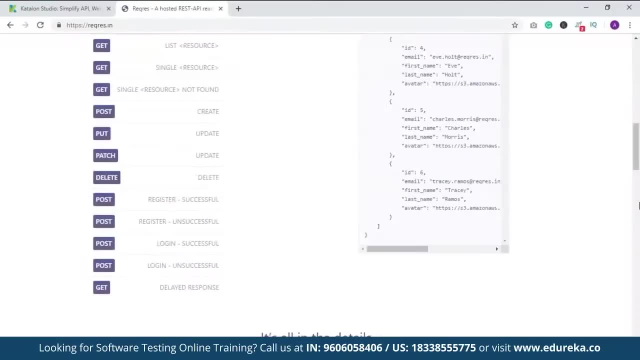 how to perform tests on rest API. So I'm basically going for the first link. that's here. You can go ahead and use any of these fake online rest APIs, or the sample rest API is available online. So, as you can see, I have different kinds of APIs here. 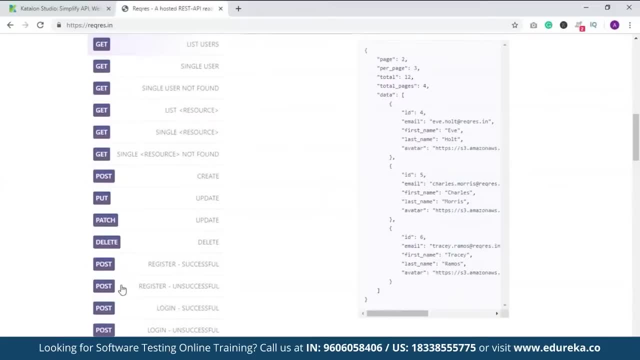 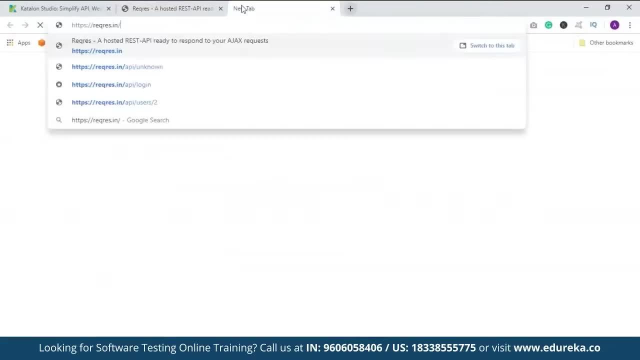 I have get have post put, then I have delete patch post and all that. So let's go ahead and take one list users and all you have to do is copy this Lincoln and paste it in a new folder and copy the request Control C. 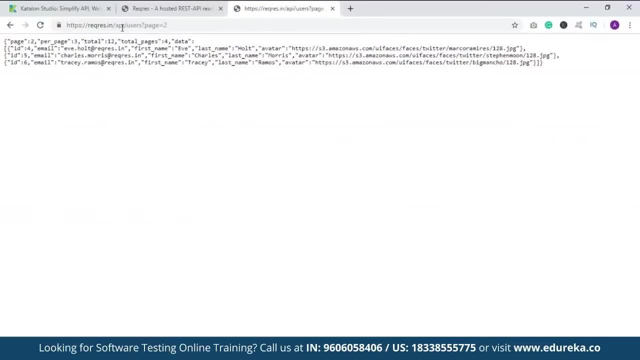 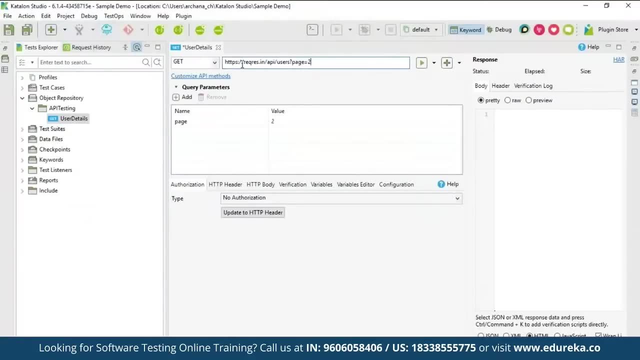 So, as you can see, here is our API, but it's in different format. All you have to do is copy this URL, go back to Catalan studio and place it here and click on this test request button, and it's asking if I want to save the changes, and okay. 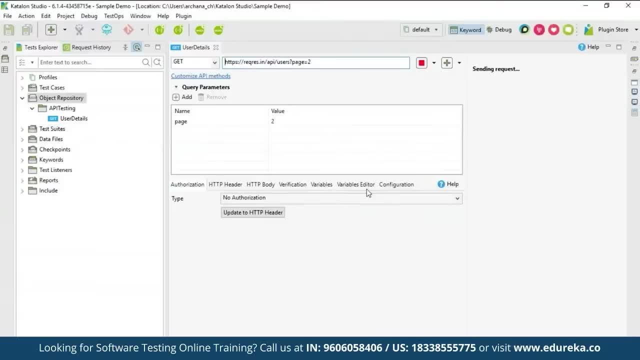 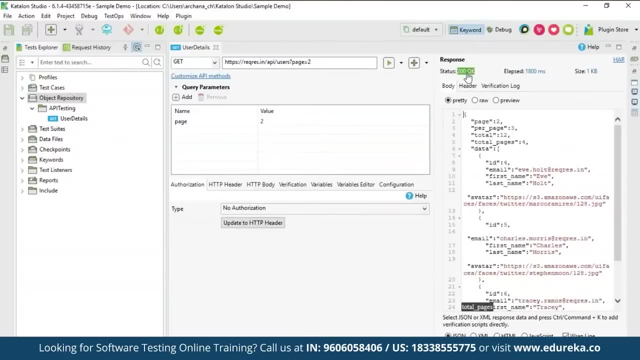 So request has been sent and we're waiting for the output. Let's see. So here it is. So, as you can see, the status of this response is 200.. Okay, it has taken so, and so time, and the size is about 1 KB. 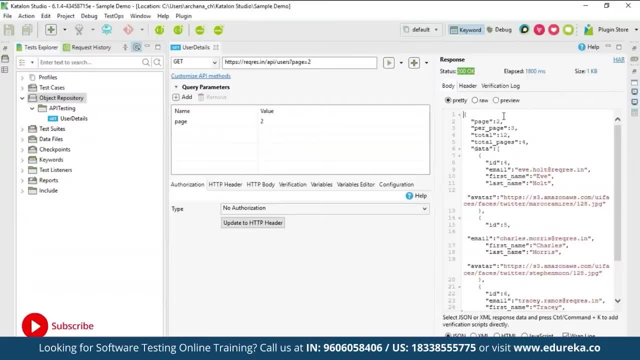 You have different formats of representing your API request. your for now It is in Jason format. You can opt for XML or HTML or JavaScript and all that. So let me get back to Jason and you have something called pretty format. as you can see, it's better to understand. 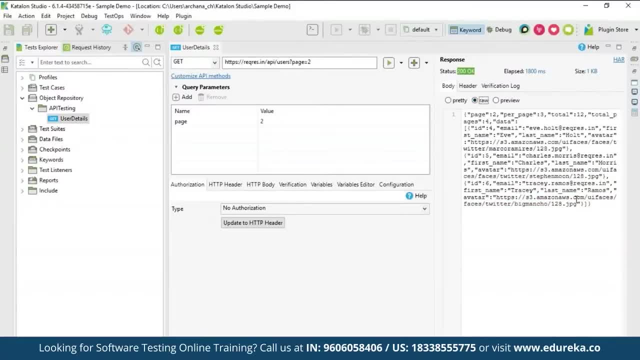 and easy to figure out. You have something called raw format, which we saw when we just copied the URL right. This is the raw format. going back, You have preview, and that's how it's supposed to look in the preview, and all that. so any of these you can choose. 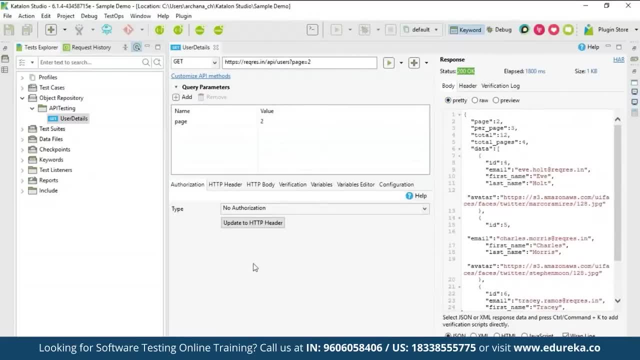 according to your comfort. So right now we have created a folder under object repository called API testing and we have a get API or the get command. This is the URL. We have pasted it here. So now that our API is ready for testing, 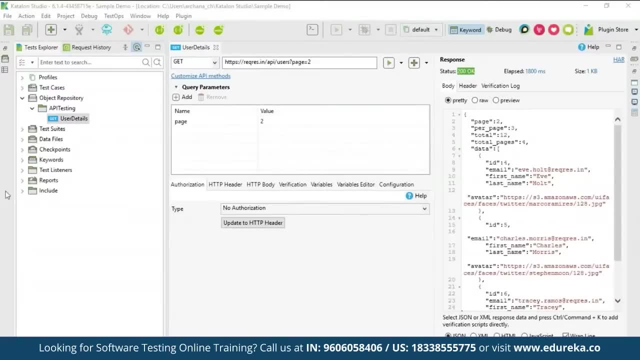 The next thing is to go ahead and create test cases. So guys have directly started doing all that stuff here, but you have an option to go and start with the sample project, where the sample test cases and the sample API will be provided to you and the Catalan studio. 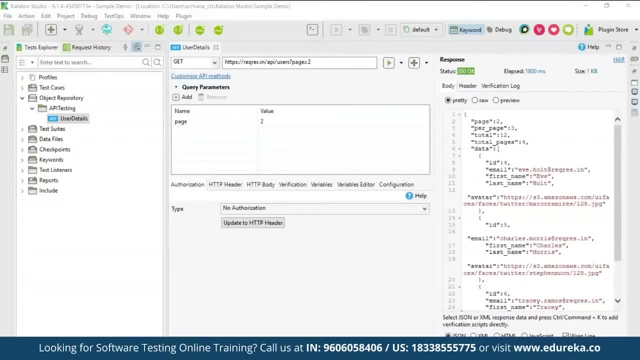 Go ahead and explore the Catalan studio application. You'll find it. So, now that we are done with our object repository, as in we have our API, Let's go ahead and create few test cases. So the good practice to follow is always a creative folder. 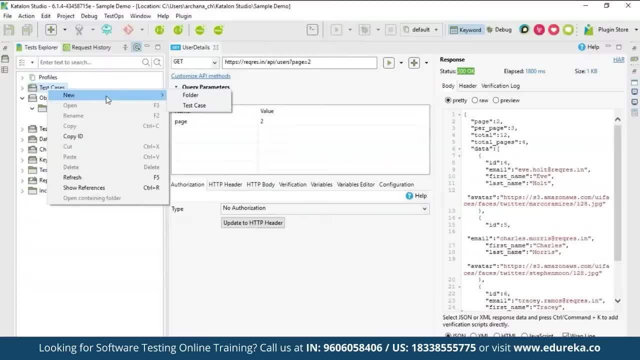 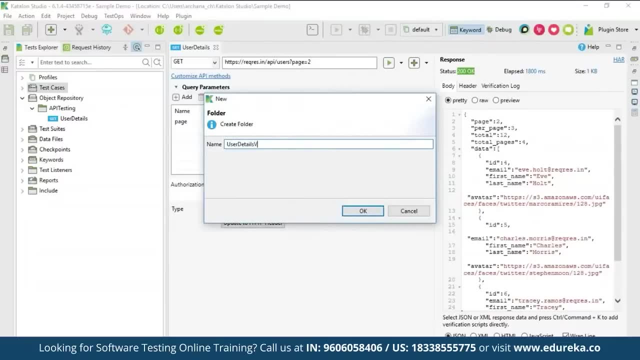 and create test cases under that, so that your test cases are not jumbled or placed here in there. So let's create a folder, Let's give it a user detail verification, Details verification, and okay, Now under that new and create a test case verification. 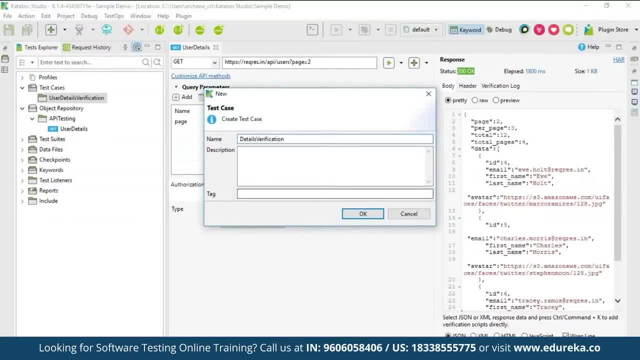 Let's say, details. verification tags are really important because right now I have only one test case, So it's very easy to search, but when you're doing an actual project of performing an API testing, you'll have multiple thousands of test cases. like I said earlier, 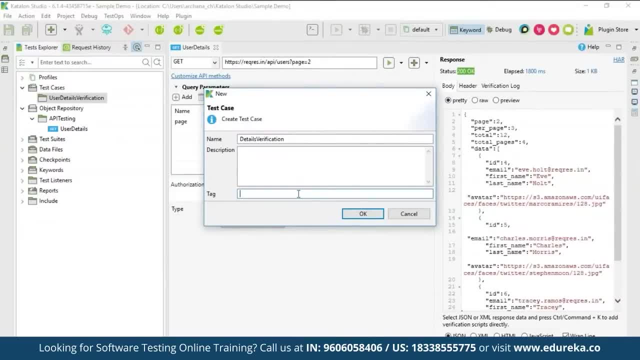 when we were discussing the challenges that you come across when you're performing API testing. You'll have multiple test cases for multiple scenarios, So it's better to attack so that whenever you want to search a particular test case and if you just type the tag related to it, 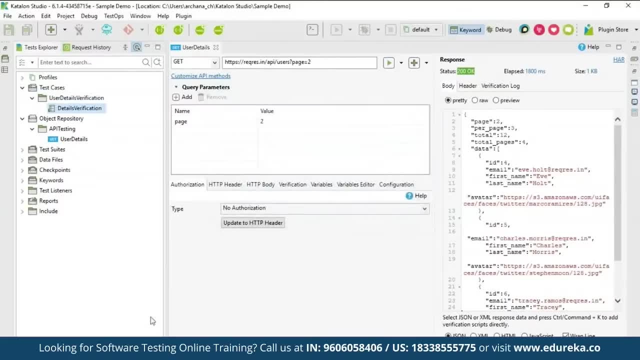 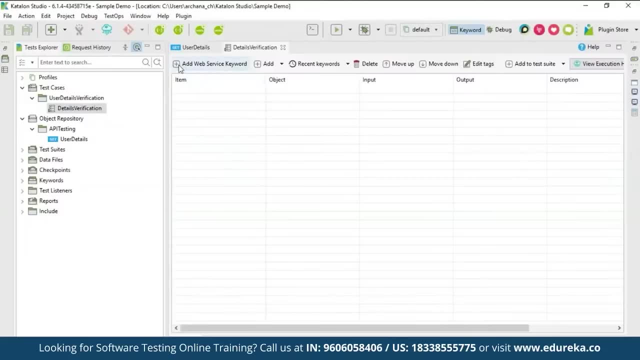 you'll be easily able to find where the test cases details. and okay, So here we go. As soon as you create a test case, you'll land on this page where you can add your service board. There's a option that it says add web service keyword. 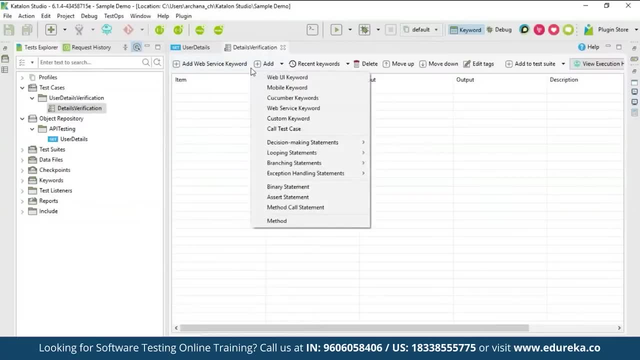 Then you have just add option. This is for the web service keyboard, because we are doing a simple project or the sample project on web service testing here or API testing. but you can go ahead and do it for mobile testing, cucumber keywords or custom keyword. 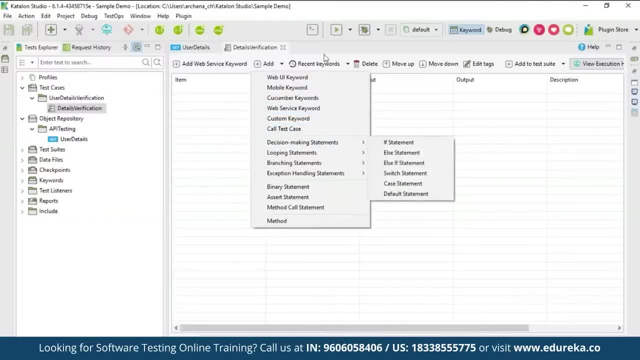 If you create one, you can add different kind of decision-making statements and all that. That's way too complicated for this video, So let's go ahead with our demo. So anytime you're performing an API test on web services, the first thing you need to do is send a request. 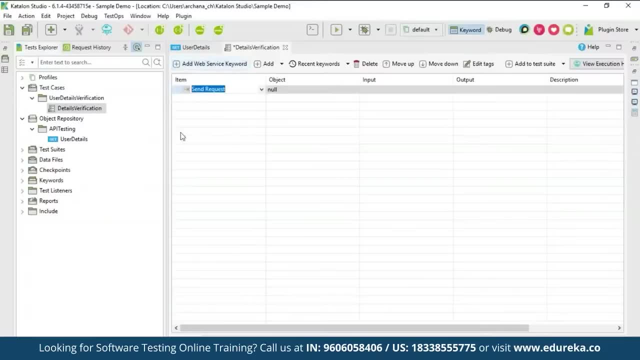 You have that here as well, So click on this, add web request. The first thing that pops out is send request and the object repository or the API which we're performing test on, or for the API request to get. all you have to do is copy, drag and drop it here. 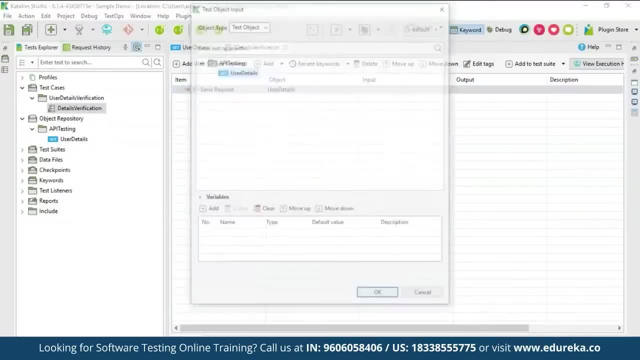 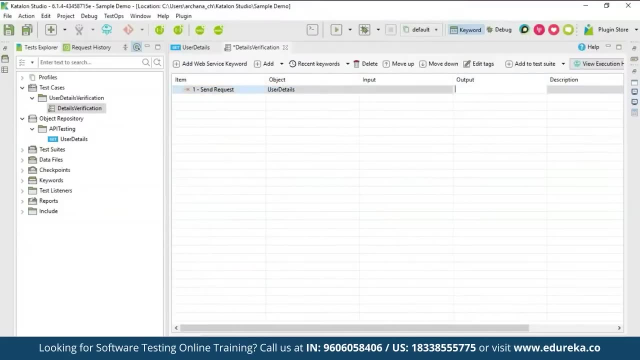 or you can just double click on the folder and we'll take your page where you have list of APIs and you can choose on the one you want and you need to assign a name to the output which you get for the object. So let's just say response. 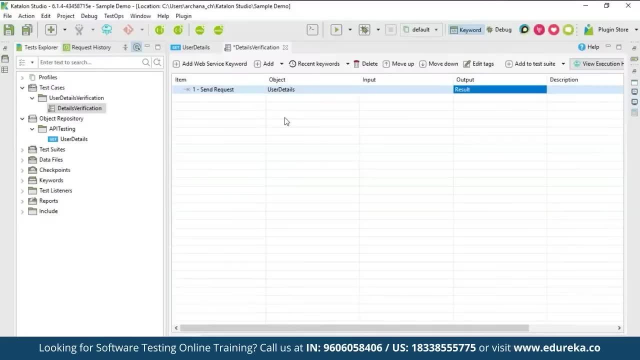 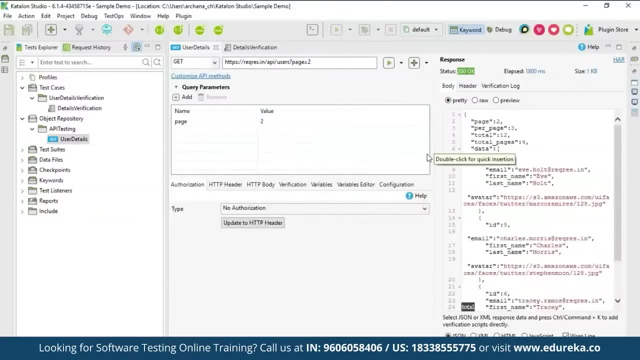 Let's say result one. So you have, you've added a first command and let me save it. So what I want to check for here? let's go back to the view. So let's go back to the view. I want to check if the status code. 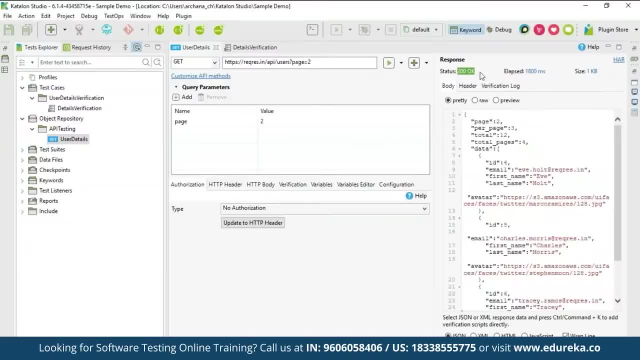 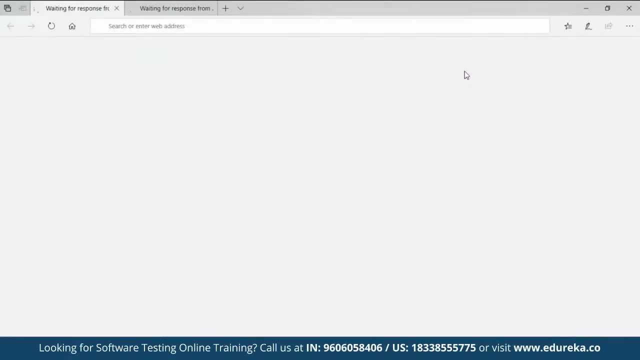 is 200 or not in the while testing. So what I'll do is I'll add the web service commander, but before that you have different status values here. You can just click on this and it will take you to a page where you'll be shown with what each respond code means. 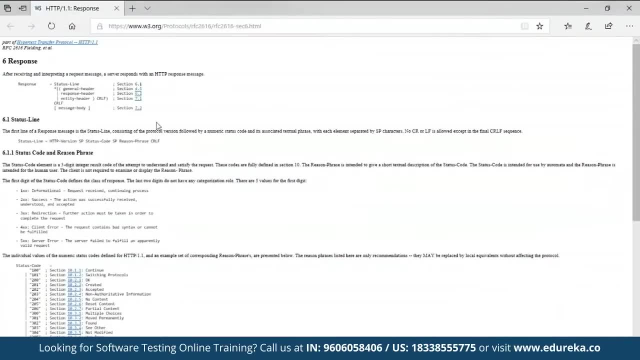 for as for now, we have something called 200. Okay. Similarly, you have different things like hundred, 101, 201 and all that. What does it say? for now It's 200 and then you have to not do, which is the request is accepted. 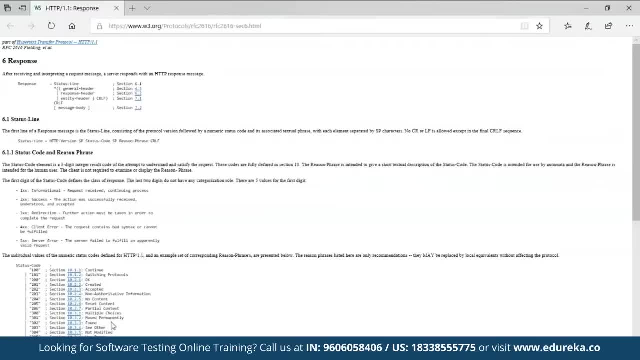 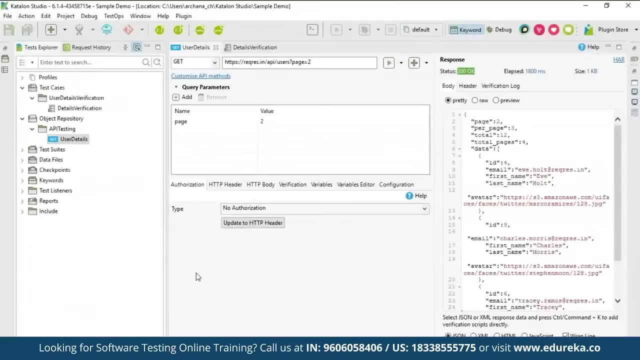 Then you have to, not six for the partial content, Then you have 303 for see other. then you have to use proxy 305, like that multiple every request has and state is associated with it, right? So if you want no more, you can just double click on that will be taken to that page. 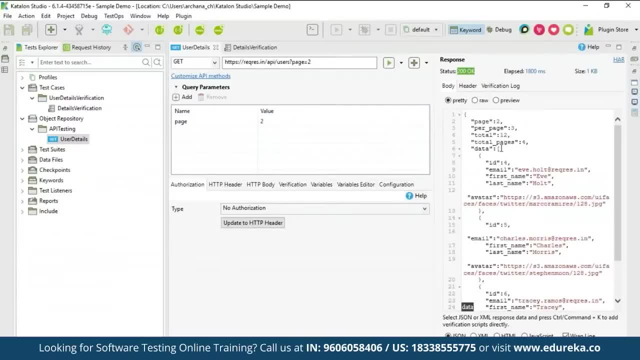 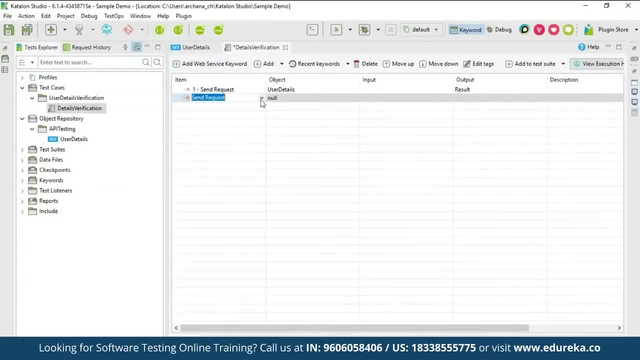 So where was I getting back to? what to test? Let's test if the status code is 200 or not. Let's go back to our test case and I'm going to add a new web service. You have a drop-down command here. 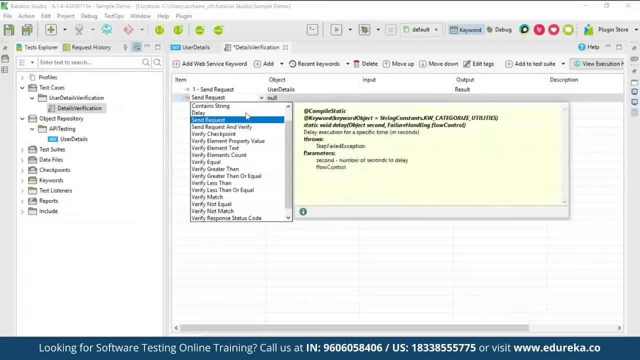 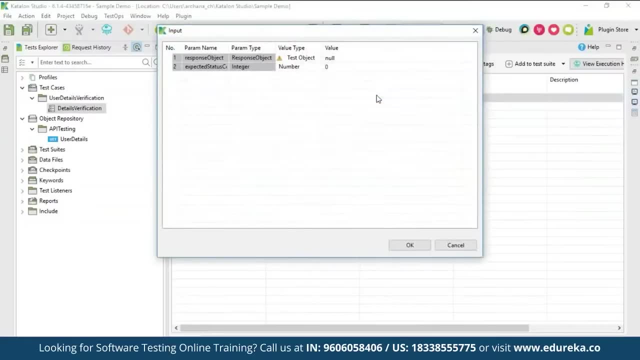 You can just click on that and what I want to check? I want to check: verify response status code. click on that. So input to test. you need to give the input right so you can double click on that and it's the response object with a variable. 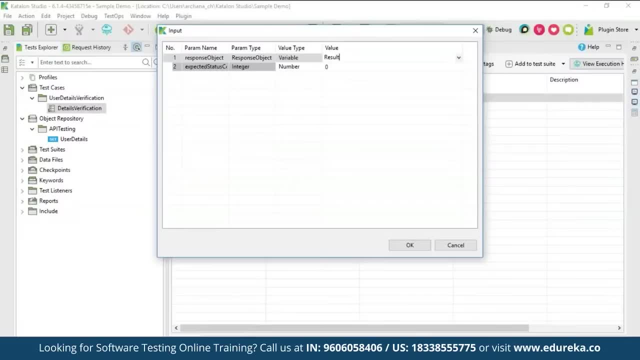 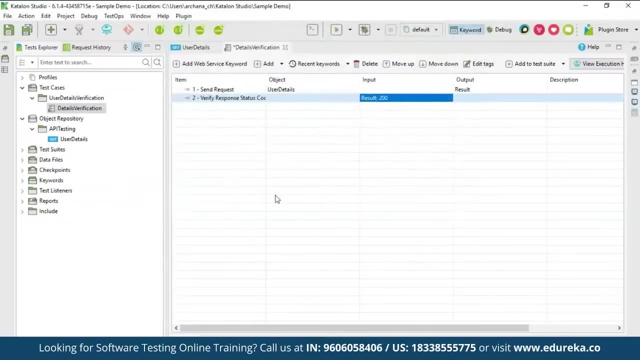 What did we give its result? So type that here and obviously the value which you want to test it for, let's say 200, and okay, that's done. Let's add one more command. Let's say: for now, I know that this request supposed to be 200 status. 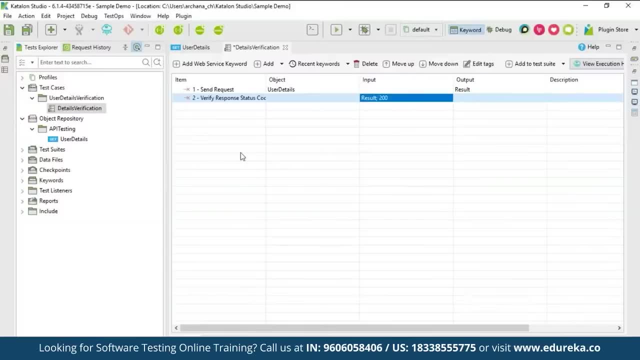 But what if I want? if I don't know the status, I just know the range of it, Then I want to check if the status of my request lies within the range. You have that option as well. You can go and add web service again. 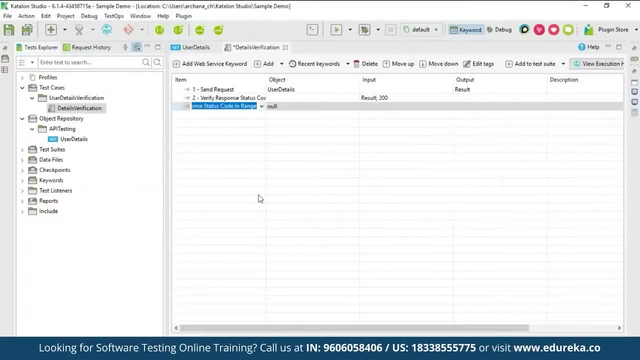 and you have something say is verified response status code in range, again, You can just go ahead and add the input here. So again, guys, if you are new to web service keywords or this API testing, and if you have no idea what keywords choose, what do you want to test for? and all that, you have an option. 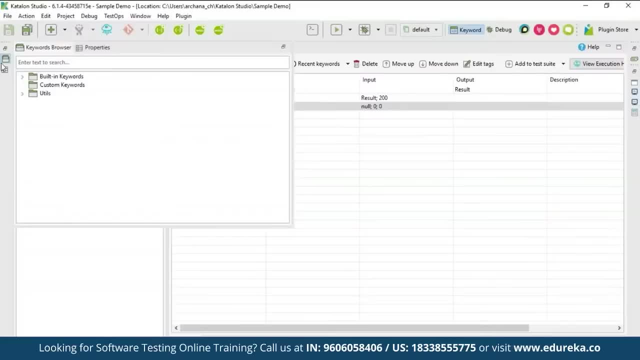 which says keywords, browser, and there you have different kind of options to browser. you can say documentation- You can actually go for official document station in the Catalan studio website, but you also can do that here. You have built-in commands for web UI keywords. 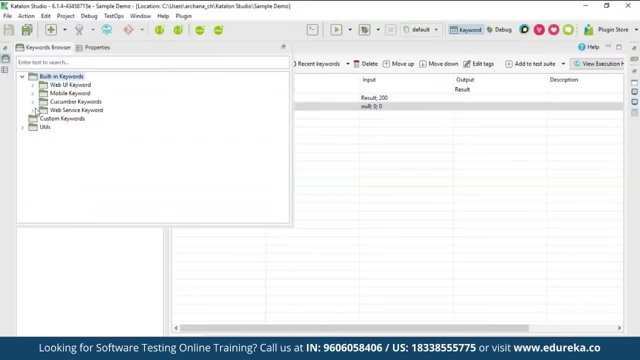 You have mobile keywords, You have cucumber keywords, You have web service keyboard. So the thing which is related to the demo which you're doing right now is web service keywords. So you have different options for element number request test and it leads, let's say, for request. you have 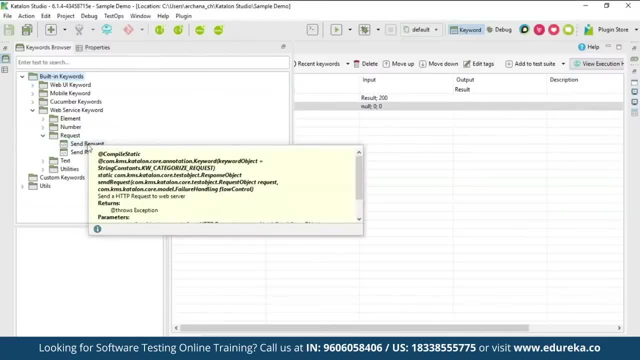 we just use the send request. So when you click on that dialog box, it pops up which says: what exactly does that keyword do? It sends an HTTP request to web server. That's what this send request does. and what if the error pops out? it throws an exception. 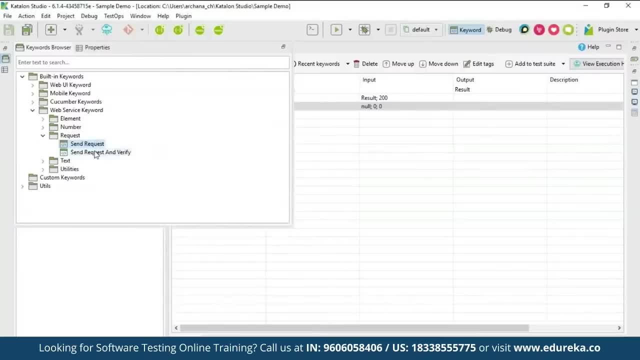 So what are the parameters that you need to mention for that keyword and all that? There's something called send the request and verify as well. It sends an HTTP request to web server and verifies the response. It does the both. you will check that out later. 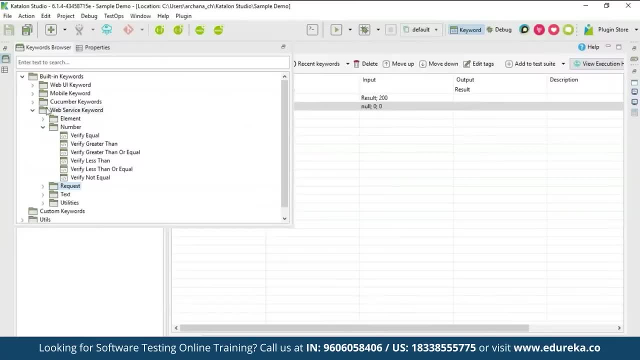 And then we have something for number, basically, or equal to, greater than, less than, and all that. you can go ahead and check that. then you have element features which you want to check. We'll do that right now in the demo part You have an option to check: verify element property value. 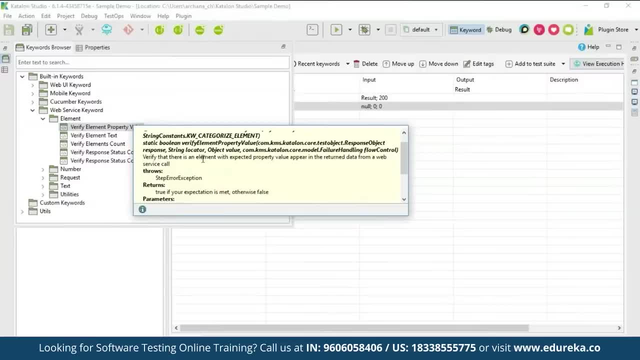 Let's see what that is. So if I scroll down it says verify that there's an element with expected property value appear in the return data from a web service call. Basically you're checking if the particular value which have given in the input is there or not. 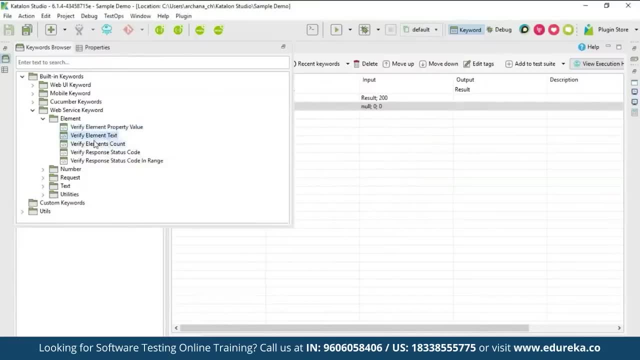 for that particular element using this element keyword. You have text: verify element text. verify element count. Then you have verify element response code, which we just did, and verify response code range that we're using. So if you're not familiar with the keywords, you can go ahead and use these. 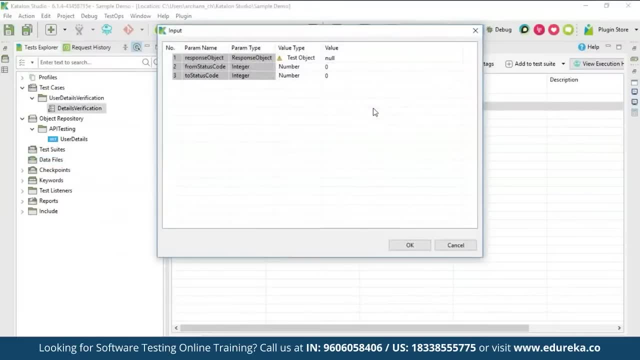 I mean refer to that, or in the documentation. Getting back to our command, We have three options here. The first one is basically the object variable which you've assigned. So it's a variable. and what is that? It's result? It's a number. 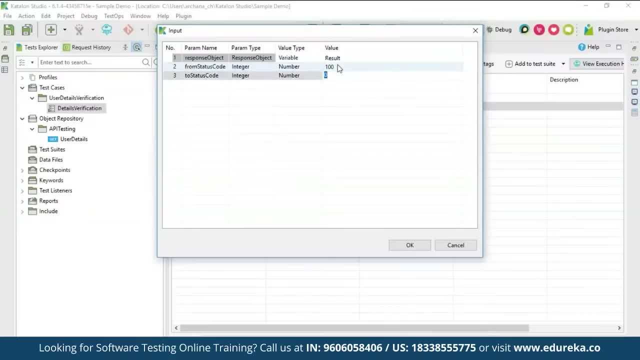 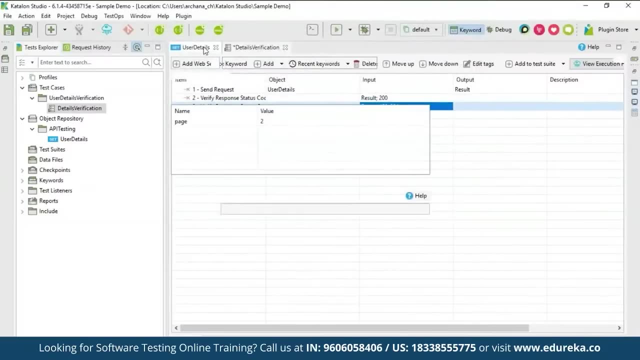 I want to check if it's between 100 and, let's say, 150 and 201.. And okay, So let's get back to our request Format and see what else we can do. As you can see, under this data, I have three elements. 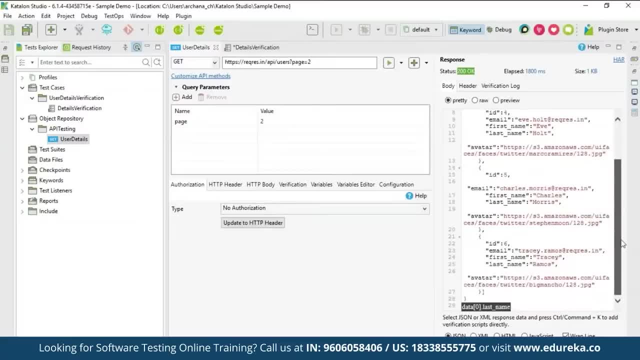 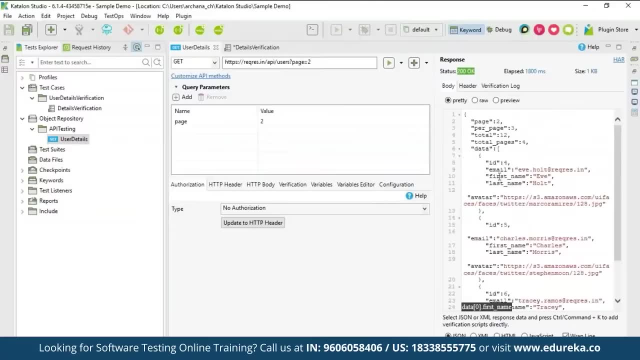 I have one which is related to id4 and one id5 and id6.. So basically I have three elements for this data. So I want to check if for the id4, the first name is Eve or not. So what do I do? go for the detail verification. 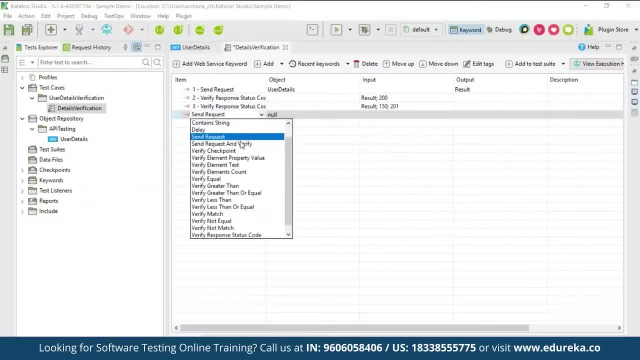 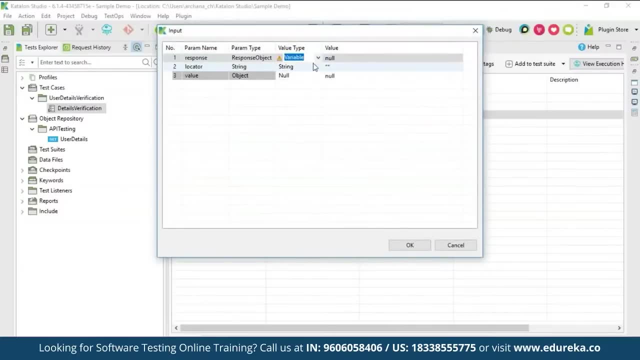 and click on add web service keyword here, verify element property value and, as you can see, we have three inputs that we are supposed to provide. Obviously, the first one is the waiting variable name, which you've given its result. Next is locator. locator is something which is basically telling the application. 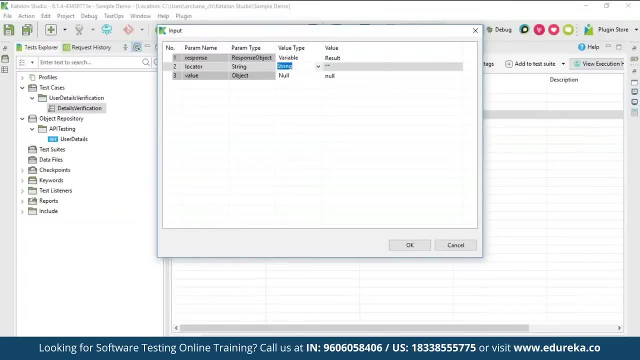 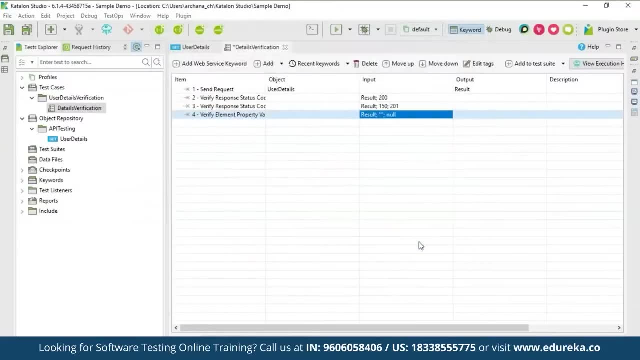 or the Catalan studio application here that please go there, to that particular location, And that's the element value that I want to check on. It's like a path. So what do you do for that? Let's just click for okay, For that you can find something called Jason Pathfinder. 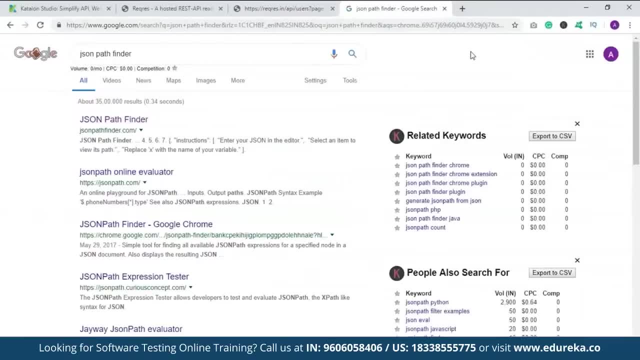 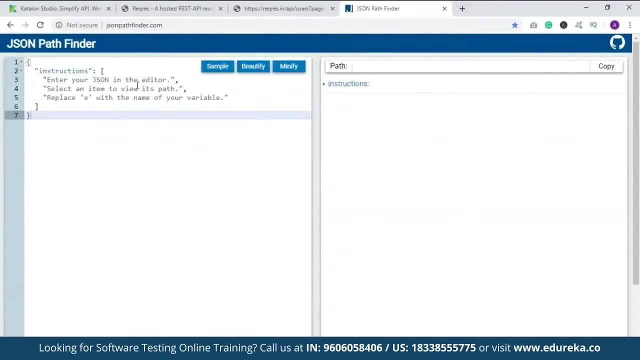 You have a Chrome plug-in as well that you can add to your plug-in, So you can just use an online JSON in Pathfinder and just using the first one I found. So what you have to do is here: enter your Jason in the editor, select the item to view its path. 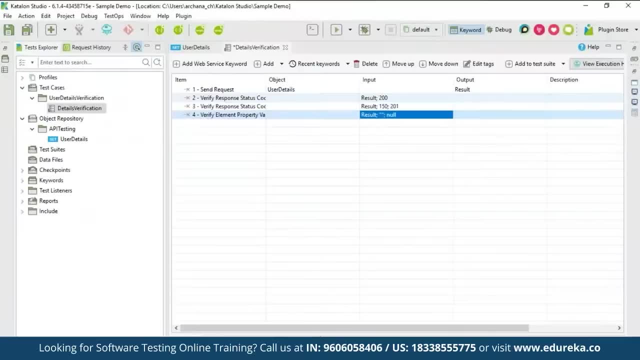 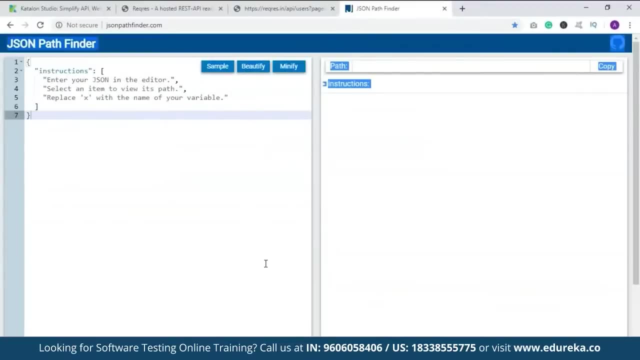 and replace X with the number or the name of your variable. So that's what I'm going to do. user details. This is my Jason input, So I'm going to copy the entire thing and paste it over here. So, as you can see, the details are shown in the third page. 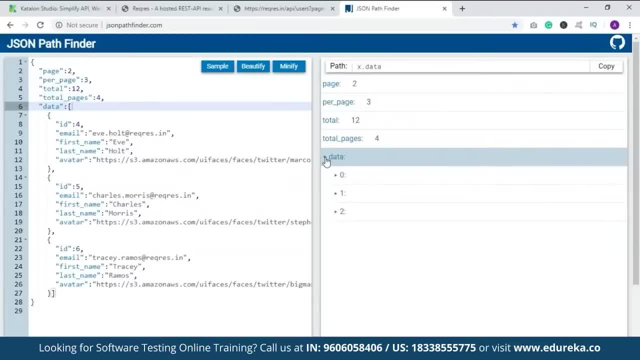 I mean the next part of the screen. So, as you can see, under data I have three elements. What I want to check is if the first name is Eve or not, So click on that. You can see a locator here in the path variable. 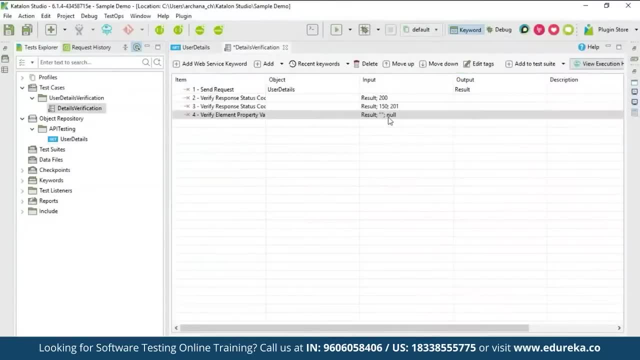 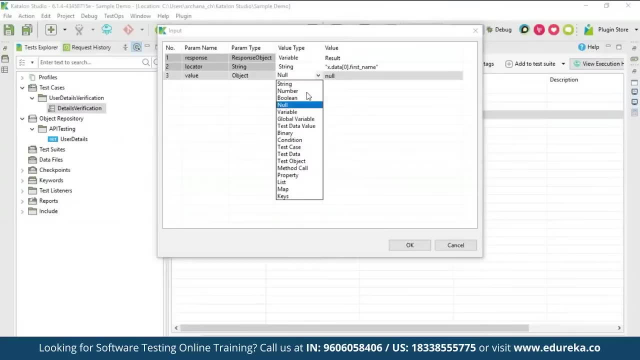 So copy that, Go back to the Catalan studio and the string. I'm going to paste it here. And next is obviously again the string that I want to check for. right now I'm giving the right value, which is Eve, right? So again the string Eve and click on OK. 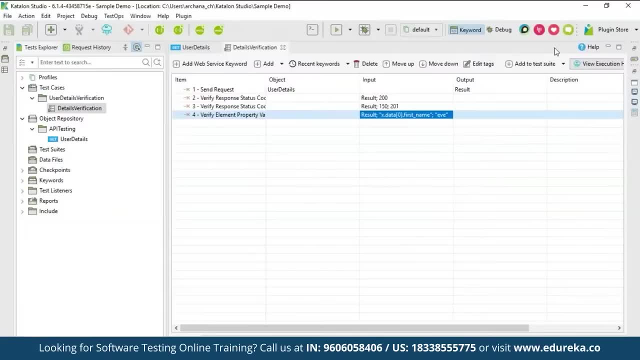 So guess this is enough for now. Let's go ahead and check. the test is running. All you have to do is click on the run button here. So, guys, this is what you say, the manual format, As in you manually entering using different drag. 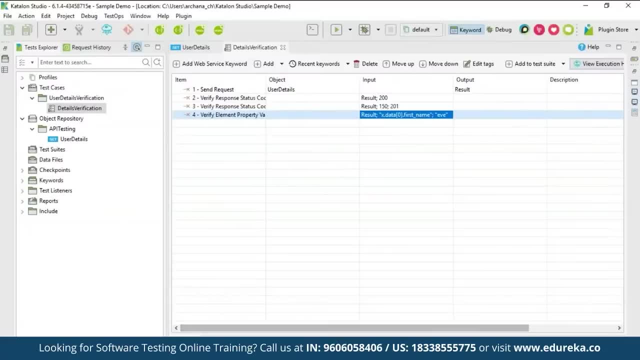 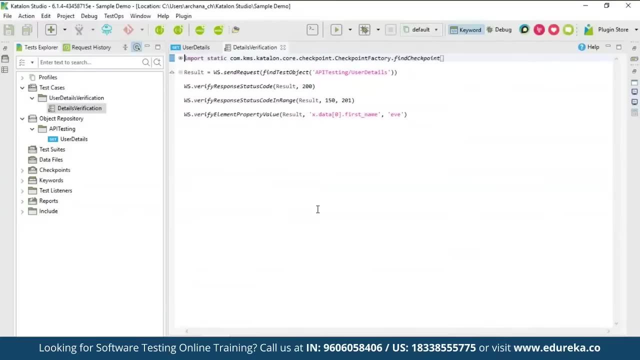 and drop options and all that. You have something called script format as well. You can go for that. As you can see, this is a script format. Let me just minimize this. So these are the commands that we just added. First of all, we sent a request for the web server. 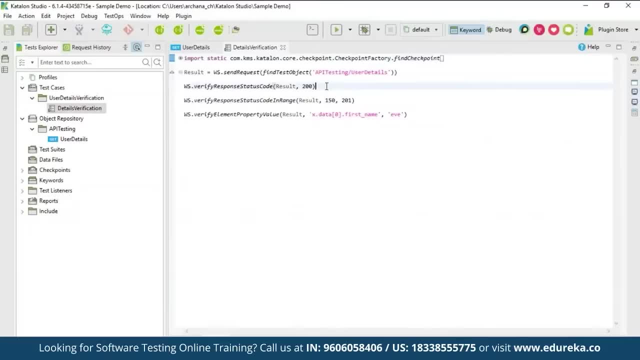 Then we added a command to check if the response code is 200 or not. Then we had the same thing: to find out the range of it as an- if it lies within the range, and to check the property value. now. So, guys, what I'm trying to tell you is that 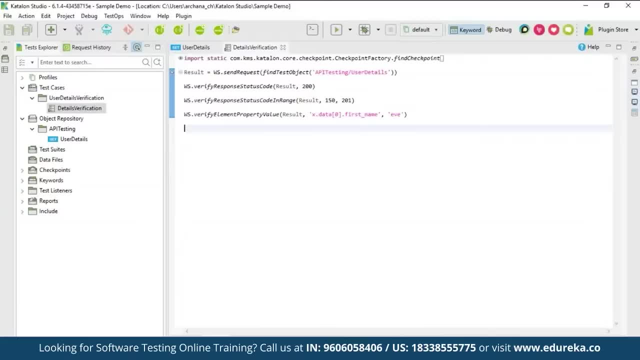 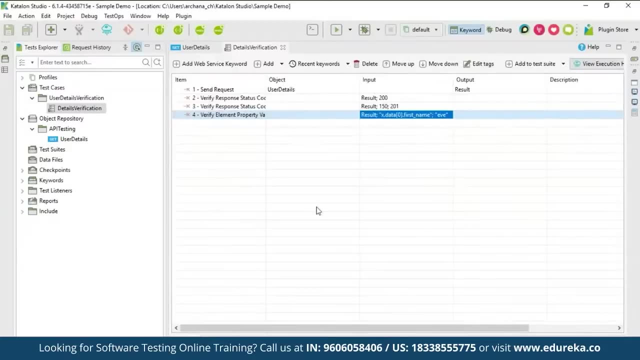 you can either use the manual format of it or the script format of it. If you are most familiar with the script, go ahead and use that. So again, let's go back to manual. And now I want to check if the test is performing well or not. 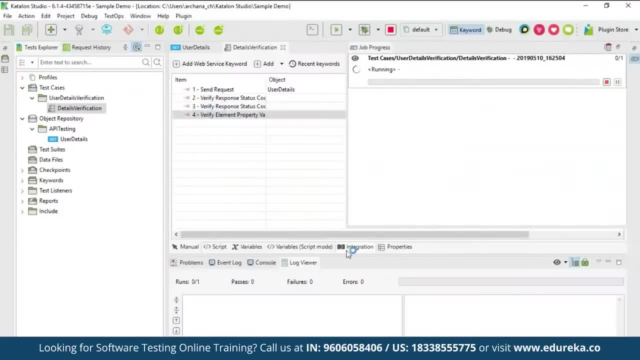 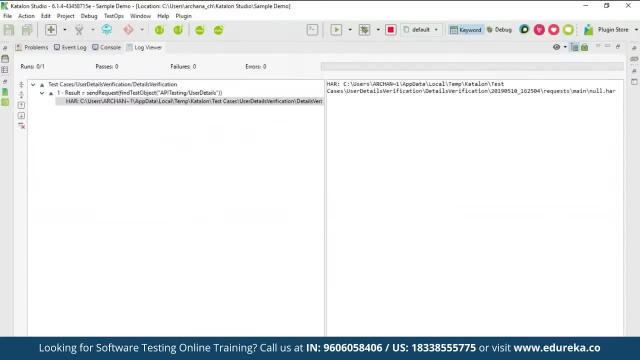 All you have to do is click on this run button and to view the output, You can just go for this log viewer. As you can see on the screen, the test is being performed. the output for every step or the every keyword that we've added will be shown here. 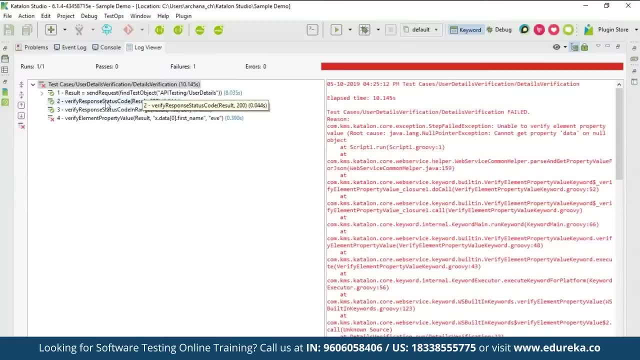 It says the first step is a success, as in the request has been sent and the data scored is 200 and data scored range is 200, which lies between 150 and do not want. but then there's a failure with the last one which says: unable to verify element property value root. 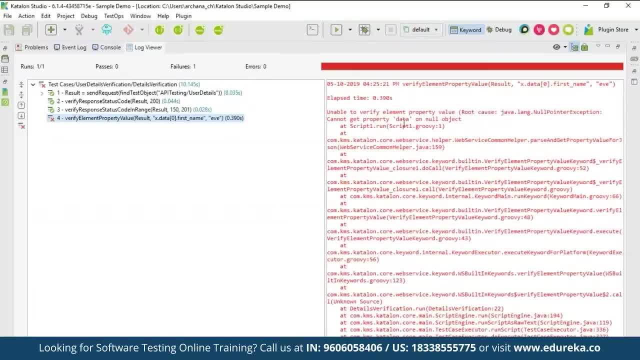 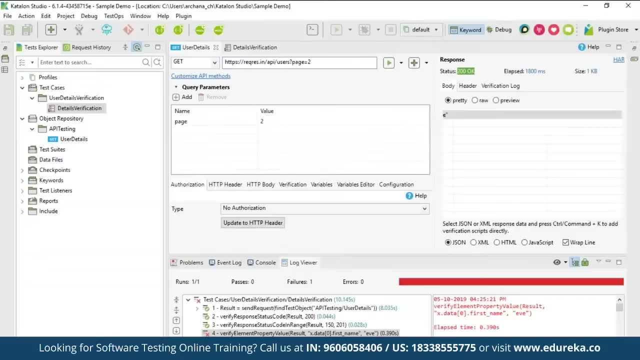 cause null pointer exception: cannot get property data in the null object. Give me a minute, guys, I'll figure out the wrong. So, guys, so what do you think the error is? Let me check the user details again. Okay, The first name is Eve, but it's in capital. 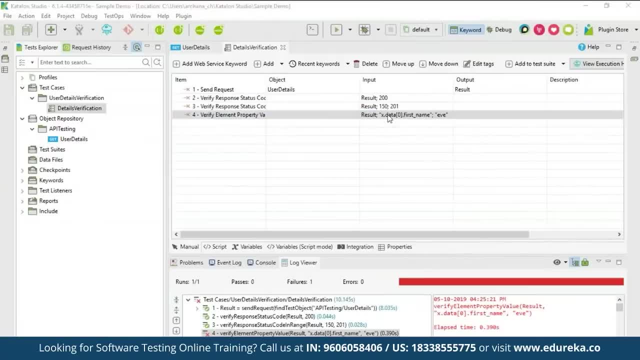 So, as you can see, that is why the test has failed. Now let me edit the string value here and see if it works- capital Eve- and click on OK. Let's save it and try to run the test. Now I'm going to go for the law viewer for the full thing. 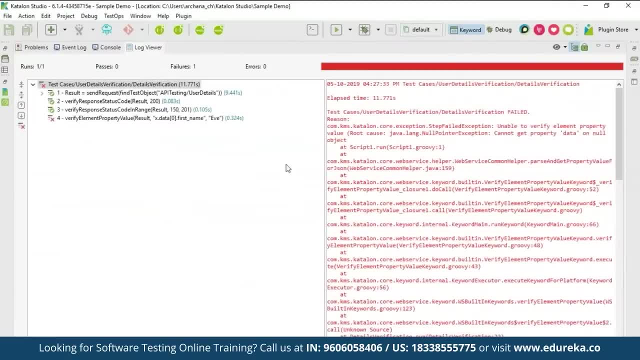 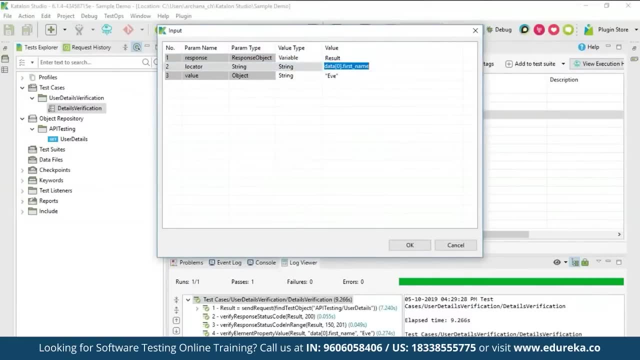 So again the test connected, again It's wrong. So it's not the problem. So sorry about that guys. The error was that here in the JSON path I had another variable, which is X dot data, the copy thing. I mean there was an extra letter in the JSON path. 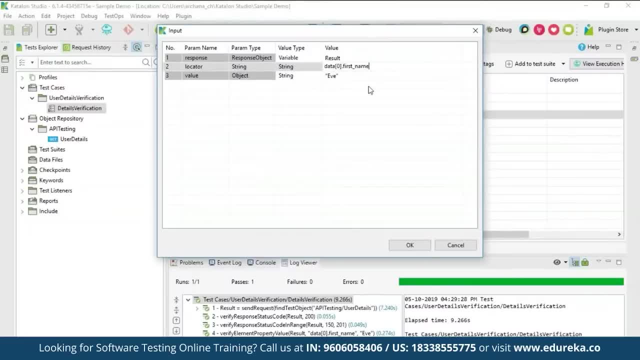 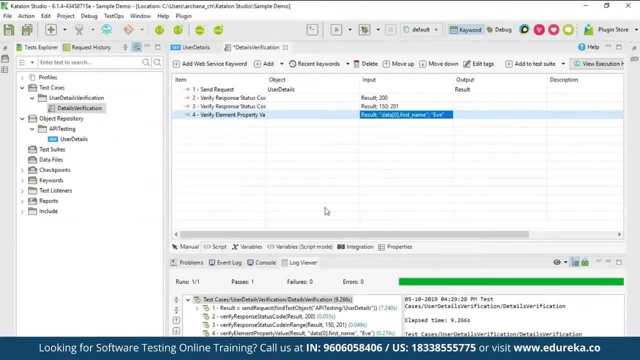 which I pasted here. So I did paste the current part. right now It is the zero to the first element of data and the first name that I want to check is Eve or not. So after doing that I did, and then if I click on run button, 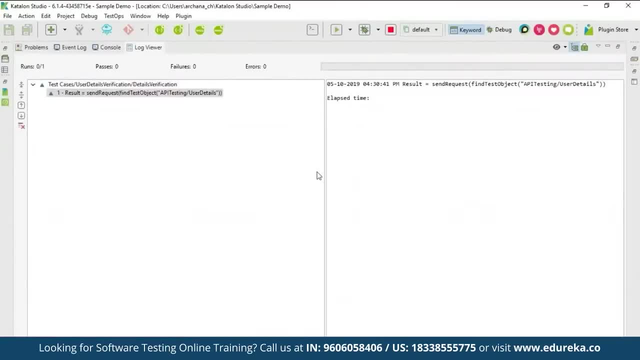 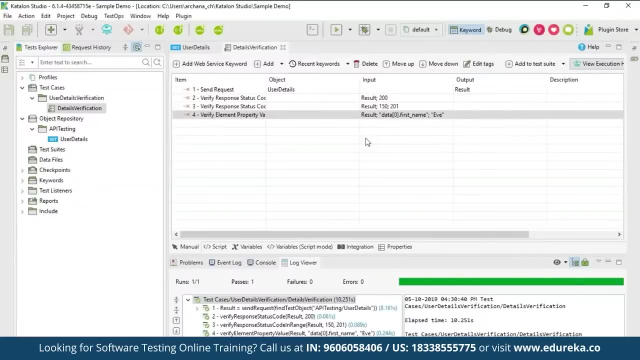 so here we go, the log viewer. So, as you can see, all the four steps are correct. by mistake, I've shown you the result of giving the ROM input as well, So that way you can make sure you API testing is working well by giving different options. 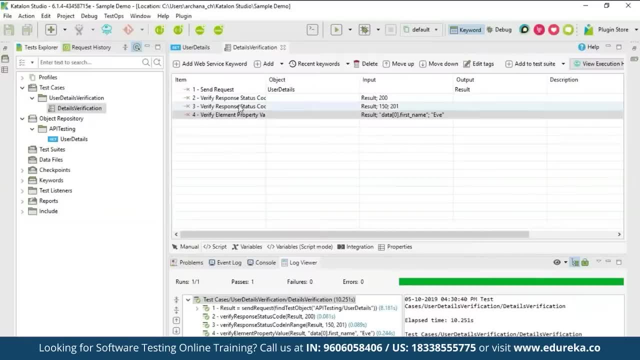 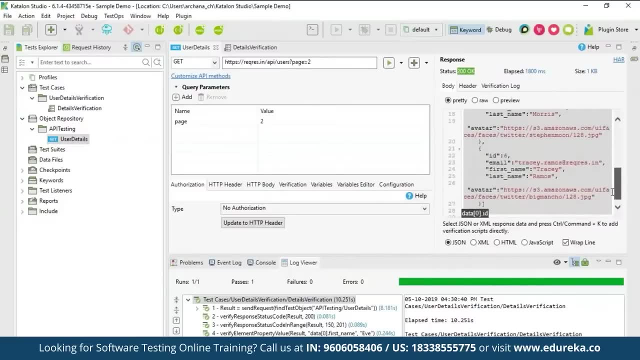 for different web service keywords here. Well, we have checked few, Let's go ahead and add one more. So, as you can see in the user details, I have three elements under the data elements, as you can see: the one with ID, one with ID, five. 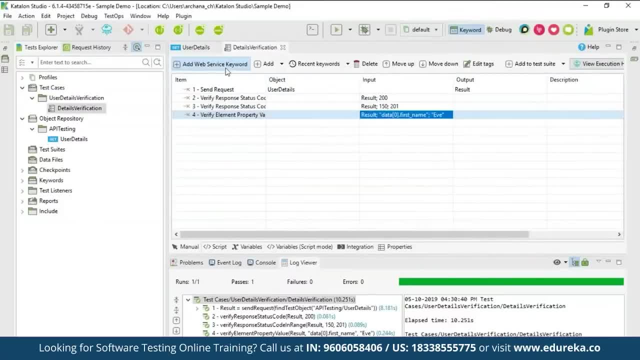 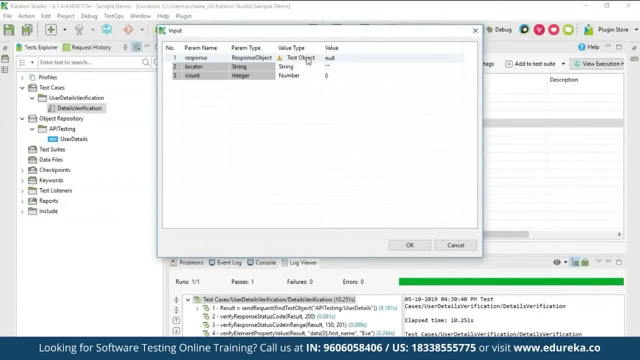 and one with ID six. So I want to go ahead and add one more command, add keyword. I want to check the elements counter. It checks the number of elements present. Well, again, the variable is result. So I'm going to enter that and again. 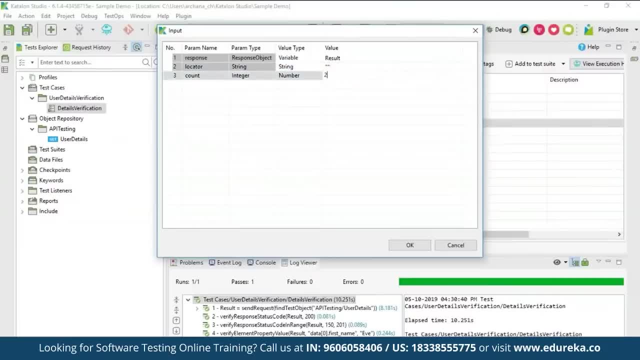 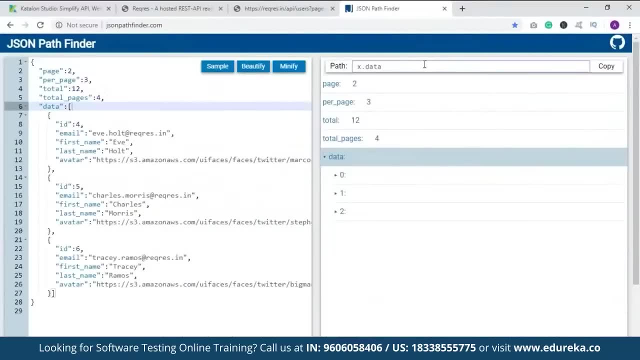 I need a JSON path and let's say, I want to check. if it's to, it should basically give me a row, because there are three elements. So let's go ahead with the negative case and okay, so data, and I'm going to copy this. 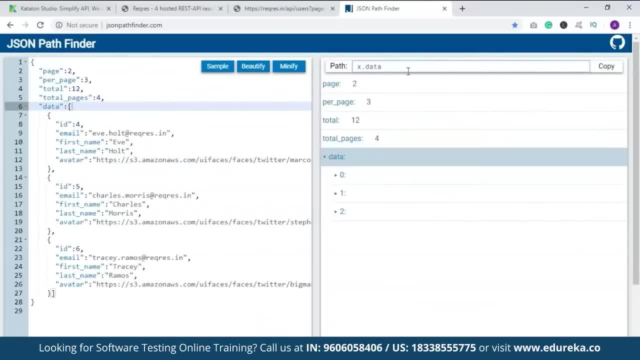 So, as you can see, the error which I did earlier was I copy the X as well. I don't need to do that, I just copy data from data, whatever it is. So then I say first name. I just have to copy from this data to the first name right now. 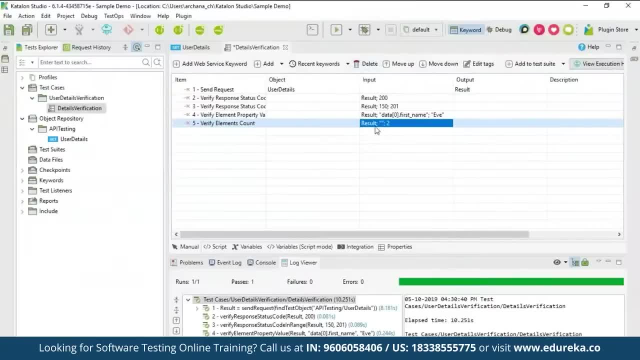 I just want the part of this. So that's just data. We can just type it here, So data, and enter. Well, it should show us an error. But how about we give positive keys, Anyway, with testing so going to say: save it. 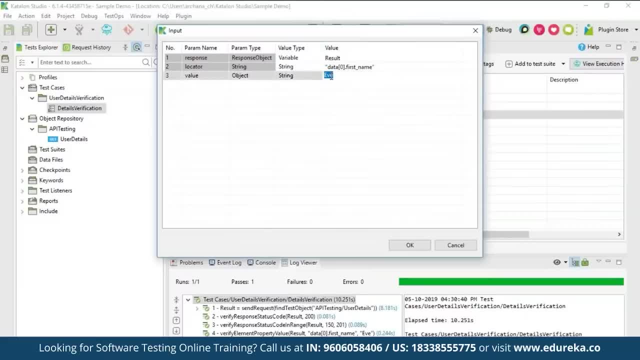 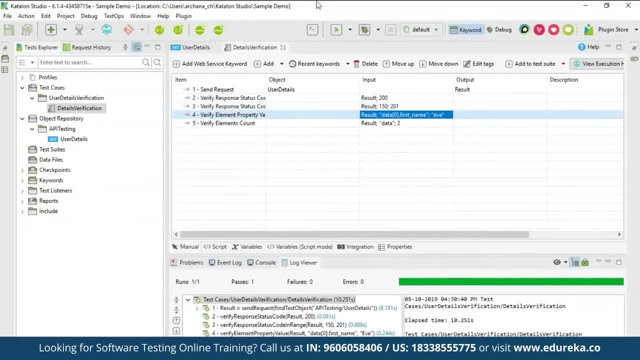 So what do we do? before that, I'm going to show you another thing. Let's make it negative case. Let's say Eve. and okay, now after saving if I run the test. So it's basically checking for the every step. The request has been sent. 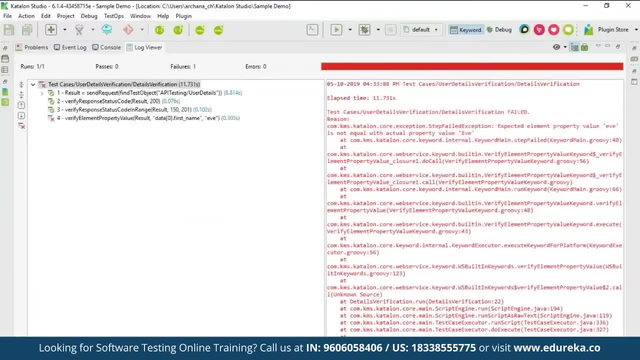 The next step is to check for the response code. That's done. response code range: That's also done. But since the fourth keyword, which is to check the element property value, since we have a negative case, the program stop executing there. I didn't, it didn't go beyond that. 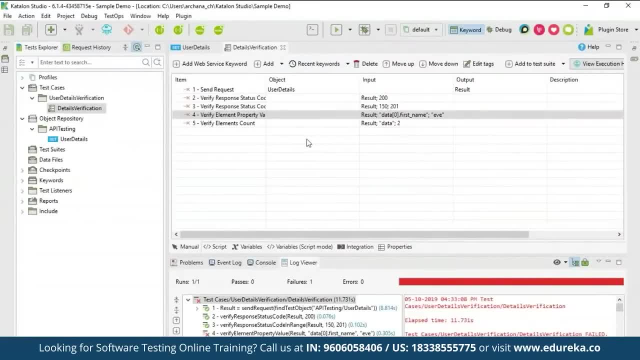 But after that we do have another keyword for which it has to check to, so for that we have different properties. to go ahead and change how this keyword has to behave, can right click on that. you have something called change failure handling here, So you have different option. 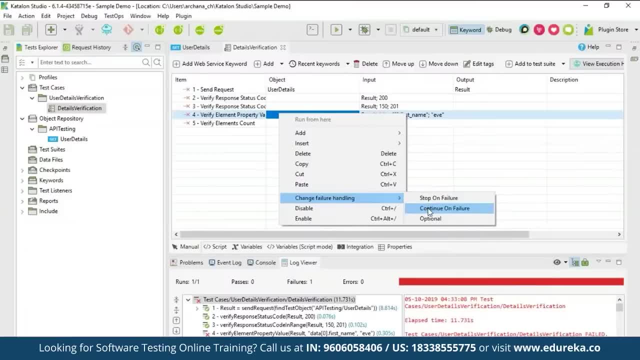 which says you have to stop on failure or continue on failure. Let's say we have given continue failure, So it will stop. I mean it will execute the step even if it's there and I chose an error and go to the next part. 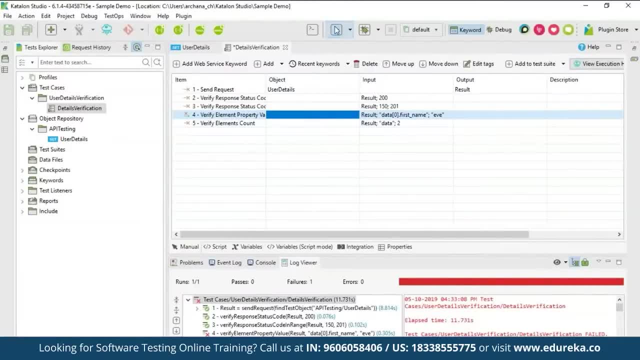 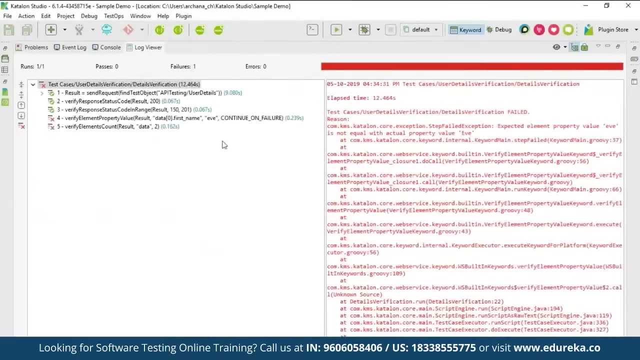 Of it, Let me save it, And if you click on run again, let's go for the log viewer. Here we go, guys. It didn't stop there. It went for the next step as well, And since that was also a negative case, 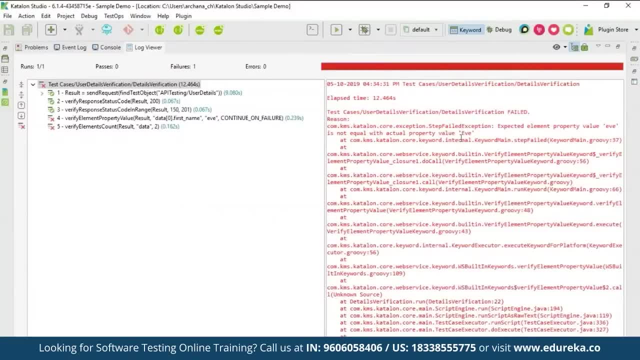 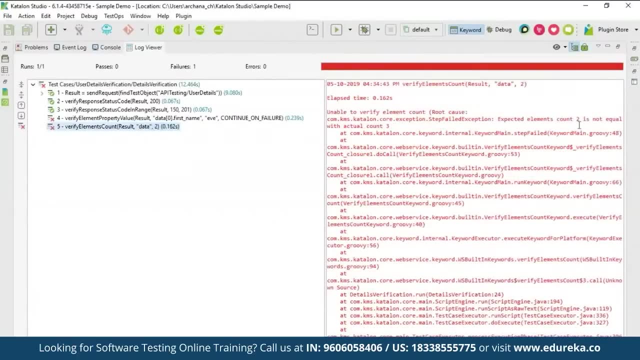 it's shown that there's an error. It says it's not equal with the actual property value, Eve. and there's one more error right When you click on that particular step. it says expected limit count 2, which is not equal to the actual count 3.. 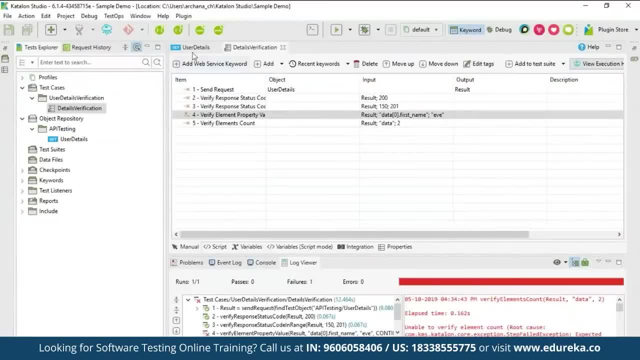 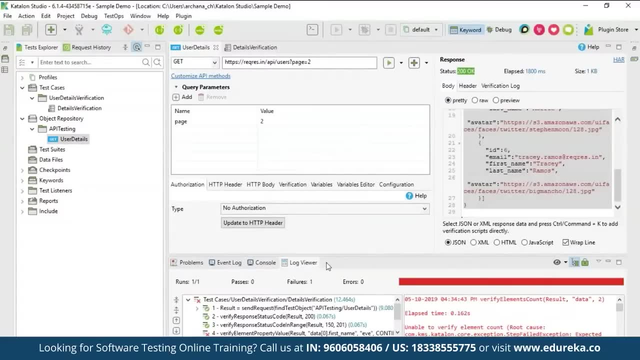 So that's the error. That's how you perform tests on API. Apart from this, if I click on the objective or the API request, your, which is get request, Basically, you have different options here as well to check out. You have something called authorization. 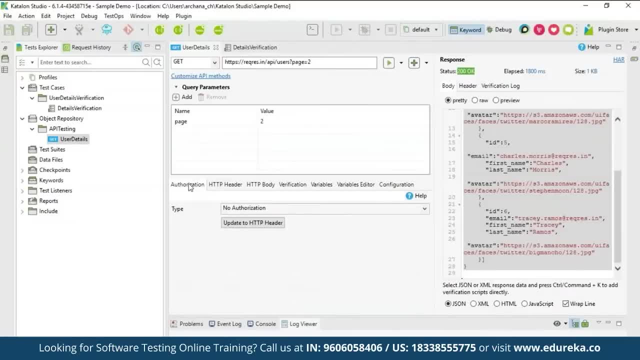 If you are actually providing some email ID and all that, you have a resin, your testing for the login page and all. you have authorization. right now, We do not have any authorization. You have multiple authorization options as well: basic or one not zero to not zero, and all that then. 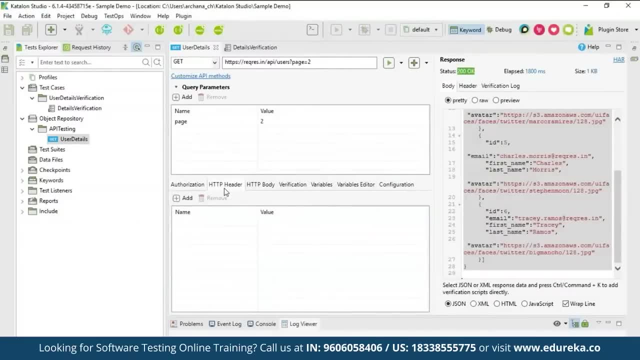 you have something called HTTP at the right now. We do not have an HTTP header. If you do, you can add to your. same goes for the strip body, but the important thing here is something called verification. So, as you can see, there are already some snippets here. 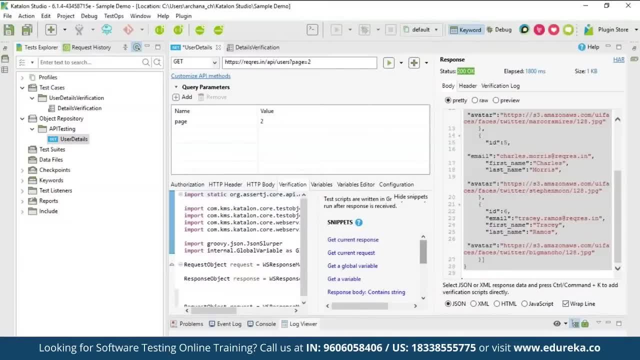 or the test skips which are already written for this. for which response is received? you have get a variable response. body contains string. then you have converted: Jason is equal to a string or not? status code. So if I click on that, you can see a command being added. 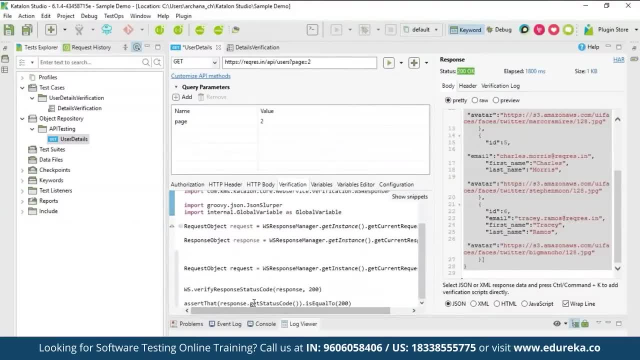 Let me hide this and let me expand this for you. as you can see, when I clicked on that, This was added. assert that the entire thing to verify if the status code is 200 or not, and to assert that it's equal to 200. 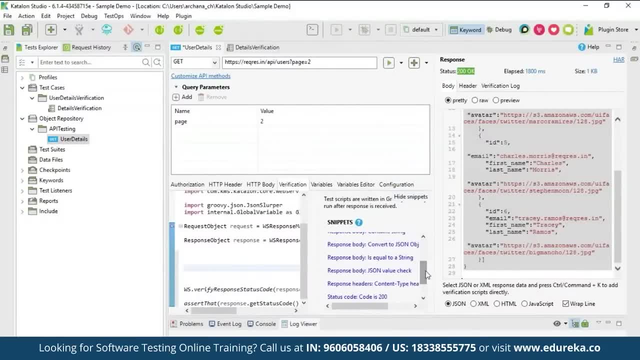 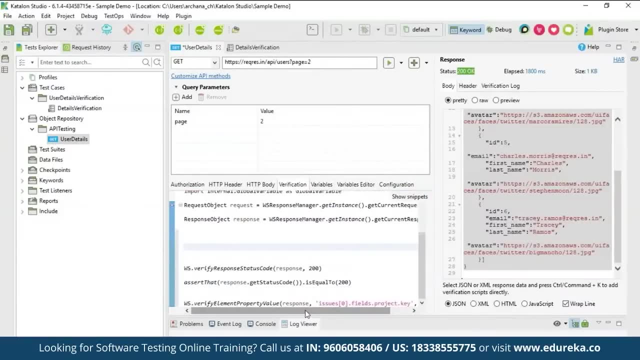 Similarly, let's check out on the snippets. I clicked on Jason, value check. Let's see What does that have to add? So it says the verify element property value is so and so, but right now the actual data is not put here. 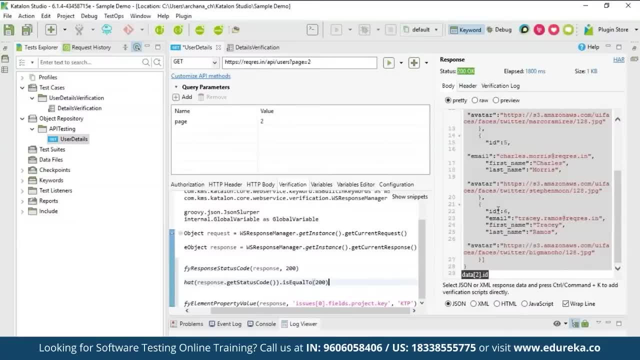 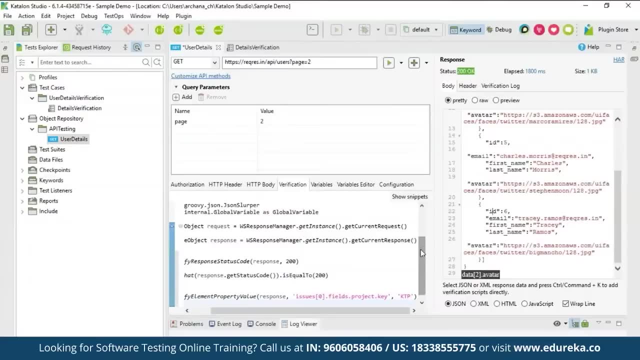 It says the random data. Let's say I want to check if the ID is six. All you have to do is place the cursor on the option that you want to check on and press control key. You can see command or the verification command being added to it. 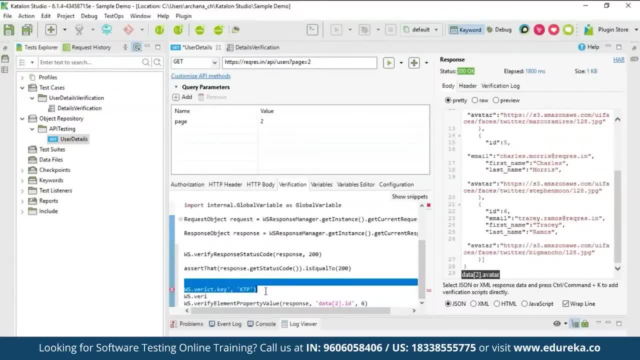 You can see a fly command property value. So it says verify element property value data to, as in the for second element, if the ID is six or not. So that's another way of adding verification snippets. Once you've added, all you have to do is click on this test request. 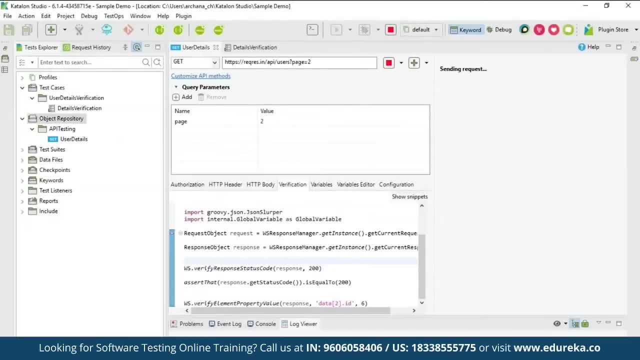 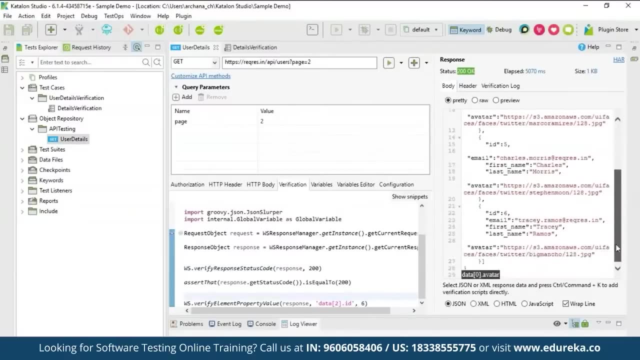 and do you want to save changes? Okay, So the request has been sent again. Now you can go for something called verification log here. So, guys, as you can see, when I place the cursor on ID 6 and press control key, the command has been added to my script. 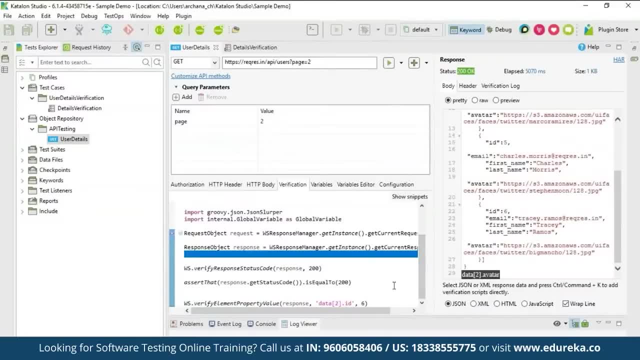 which is verify element property value, if the ID is 6 or not. for the second element, Now that I've added it, I want to check if the verification is passing. What if we do is test click, not just click on the run button. click on that and say test request and verify. 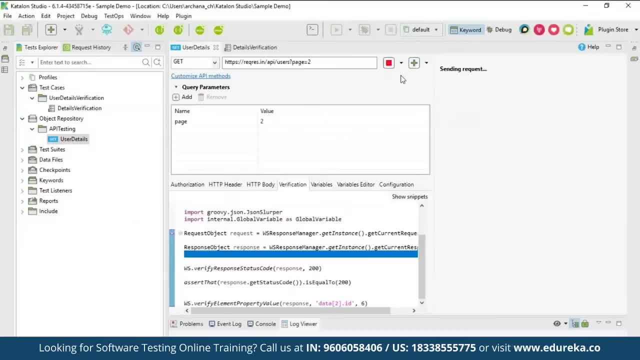 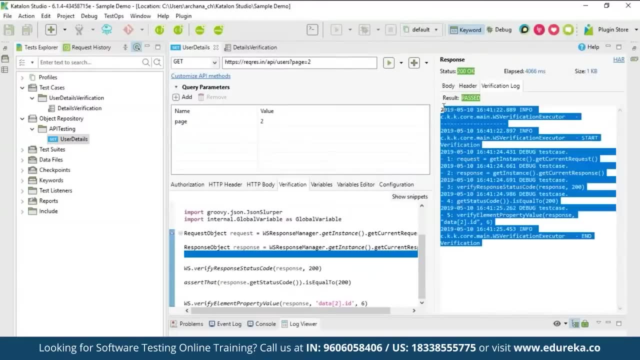 if you do that again, a request will be sent And you have something called verification log here, As you can see, when you see that it says the result has been passed. So that's another way of doing it. Now let's go back to details: verification: 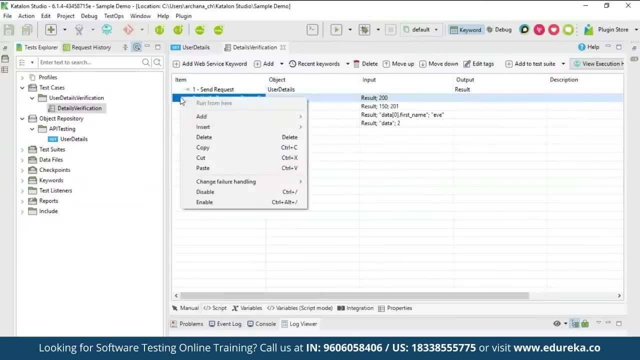 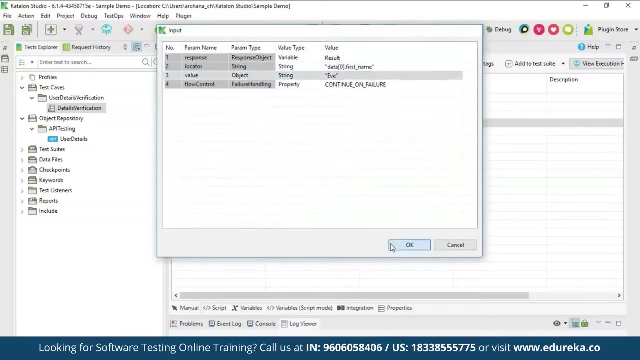 and after send request, Let me add one more command. I want to send request and verify for the same thing. result one and click. then let me make all this right. I want to give the right data, if- and I'm going to make it three- 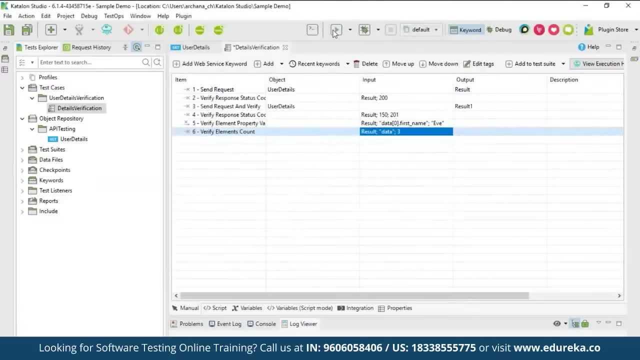 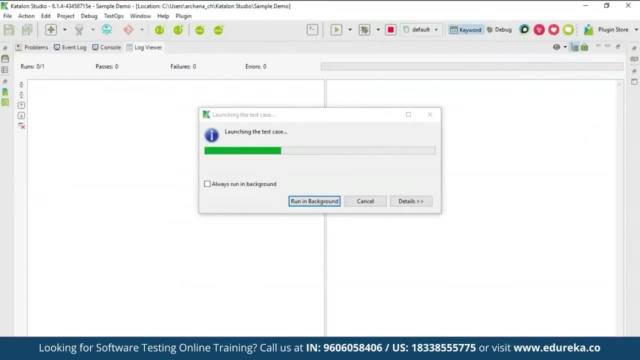 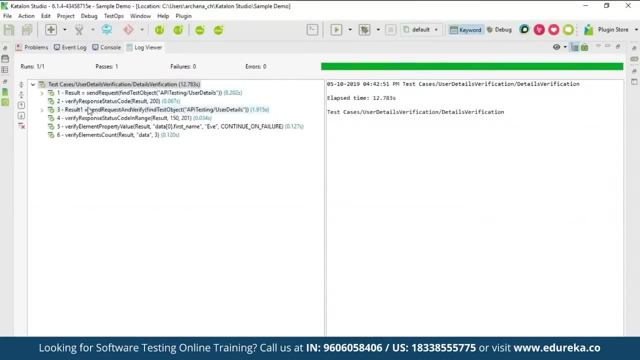 So now, if I run, everything should be green because we have given the right data right. So I've clicked on the log viewer. It's maximize the screen. So, as you can see, the first is those opposed to send the request. It's walk and verify. the status code is 200. 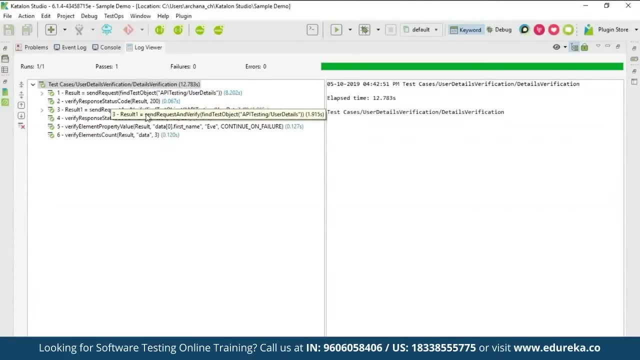 Yes, the result one: send request and verify. So it will verify the verifications which we just added. that also work. Then you have a status code range 200 lies between 150 and 200.. So it work. then the property value for Eve. 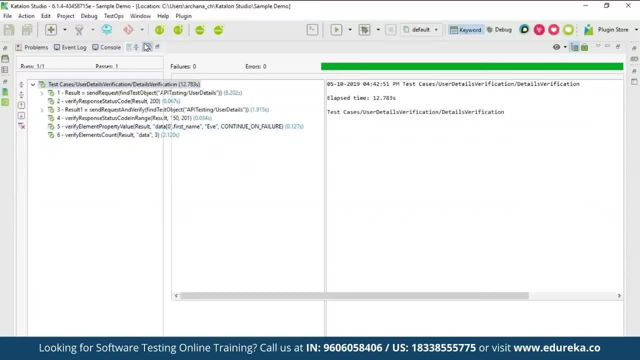 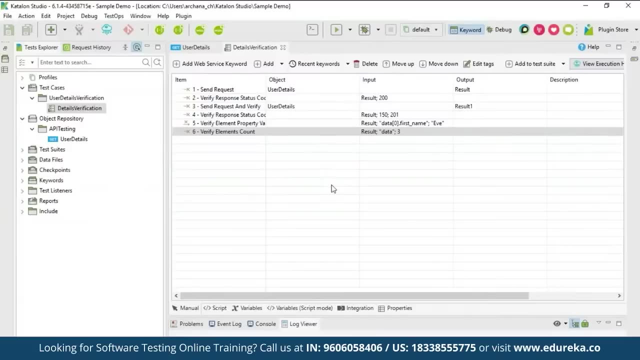 and result data is three. So, as you can see, everything is passed properly. So, guys, that's as easy it is to perform testing using Katalon studio. Well, what I've done is really basic because, since we're learning the basics here, 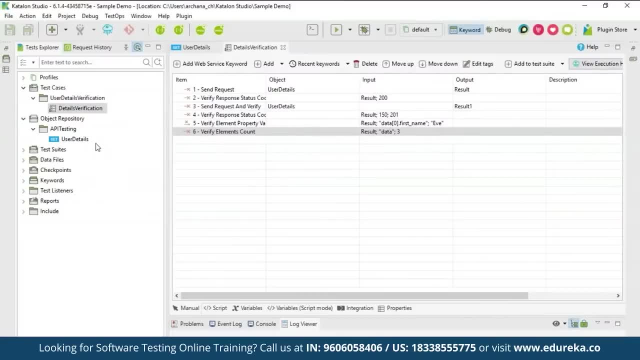 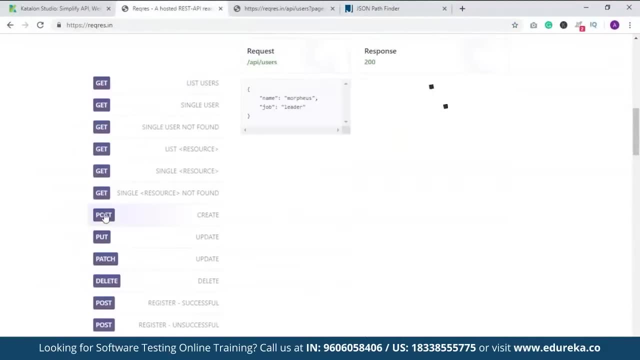 so we have just performed testing only for the get request. So, like I showed you guys earlier, we have different kind of request here. We have post request, patch request. but when you go for the post you have two things: you have response and request here. 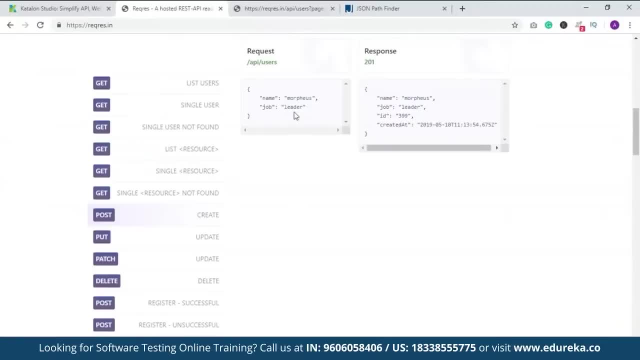 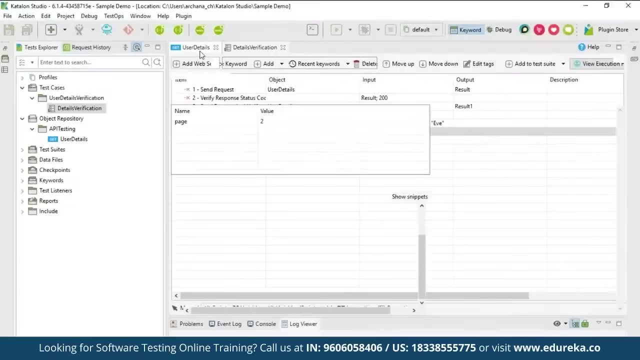 So you have two things. You have an HTTP body as well that you will have to add. Well, obviously, this is your JSON format API request, but this is the body where you have to add. I did show you here in the user details. 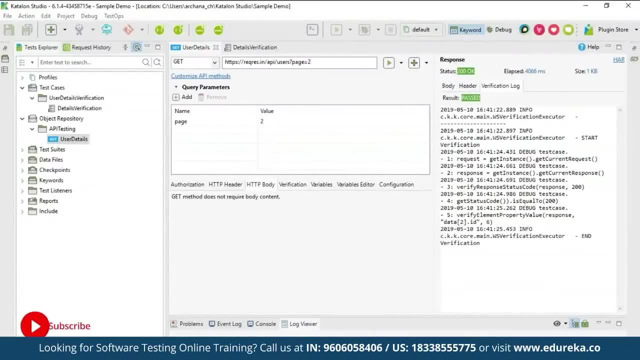 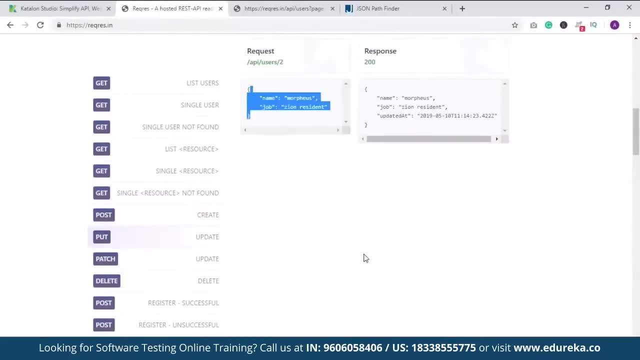 You have something called HTTP body. So when you are trying to test for post or port and all that, you'll have two things. You'll have to paste this thing in the body part and then proceed with your testing. then same goes for the get, for the get. 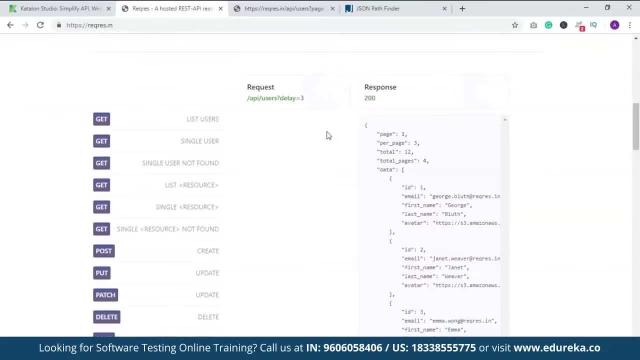 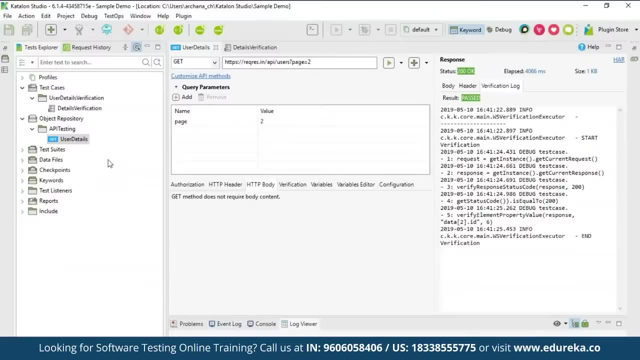 We do not have any body, So that's it. So, guys, that's all about it. and one more thing. This is for the rest API. You also have something called soap API. for that as well, You have an option to go ahead and perform tests. 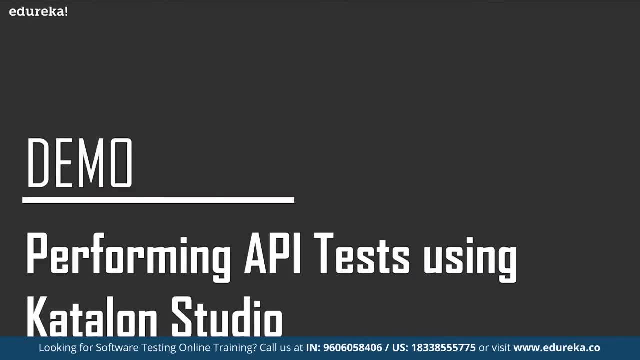 So, guys, that's about it. We did see how to use Katalon studio to perform API test. Like I said, it's a very basic testing which we did earlier. You can go ahead and use the Katalon studio for performing soap test and add your test cases to test studio. 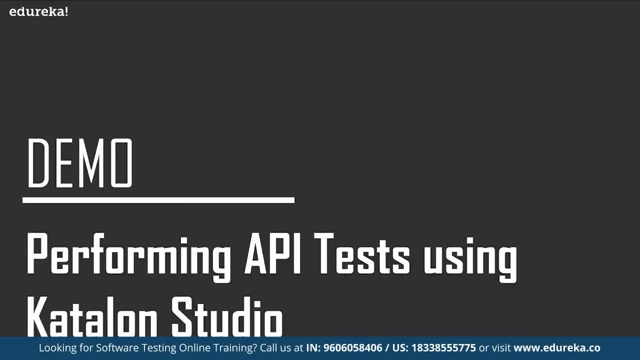 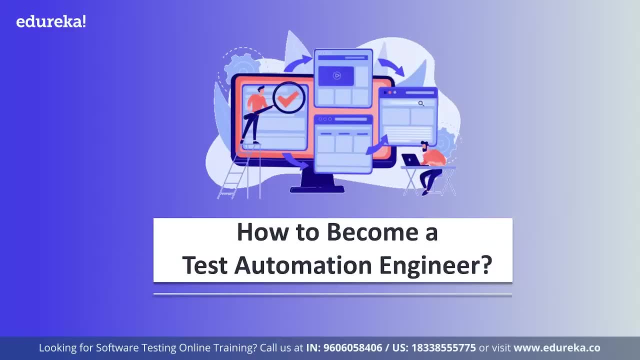 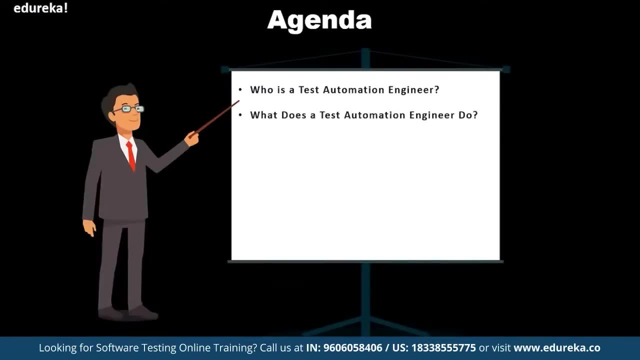 so that you can view your reports and all that. How to become a test automation engineer. So first we will see who is a test automation engineer and then we will see what do they exactly do. Next up, we will have a look at the roadmap. 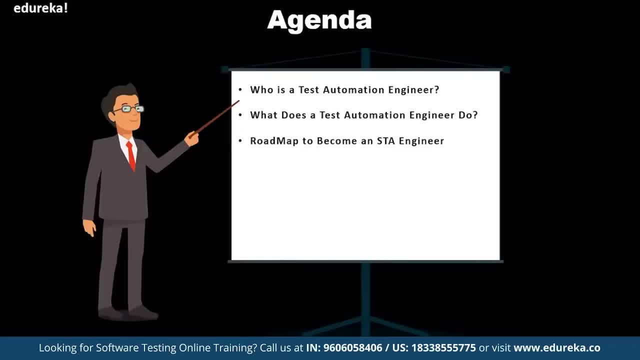 to become a test automation engineer, and then we will know about the various job roles and the required skills for an automation engineer. Then we will move on to the roadmap, to the various roles and responsibilities, and also know about all the skills that you must have in order to become a test automation engineer. 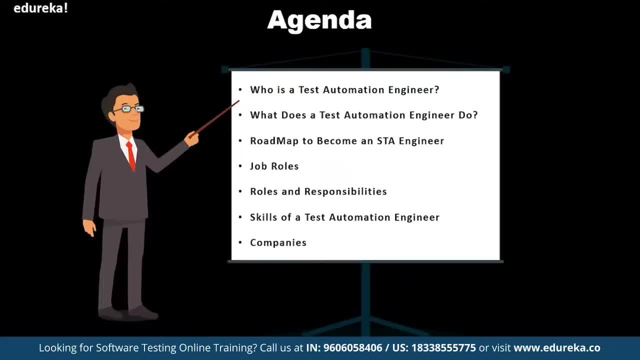 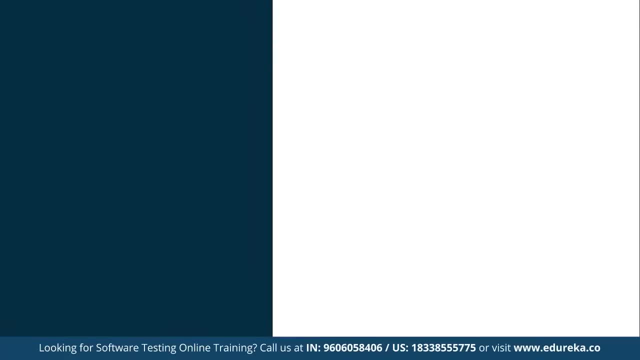 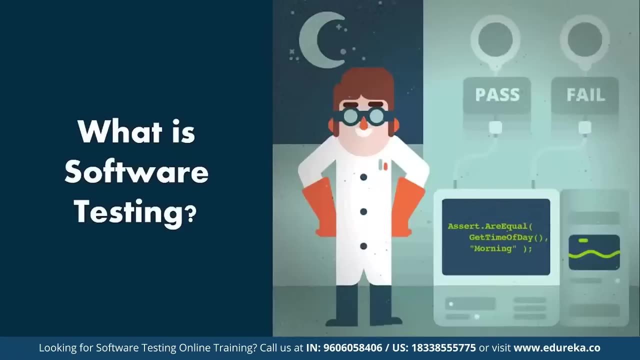 Finally, we will have a look at the various companies hiring test automation engineers. So let's get started Now. before I tell you who is a software test automation engineer, let us first know what is software testing. So software testing is basically a process of evaluating the functionality. 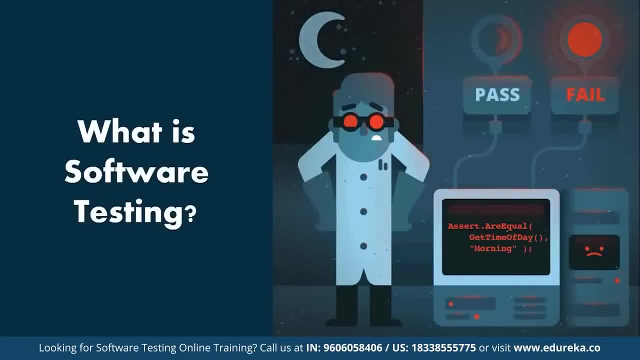 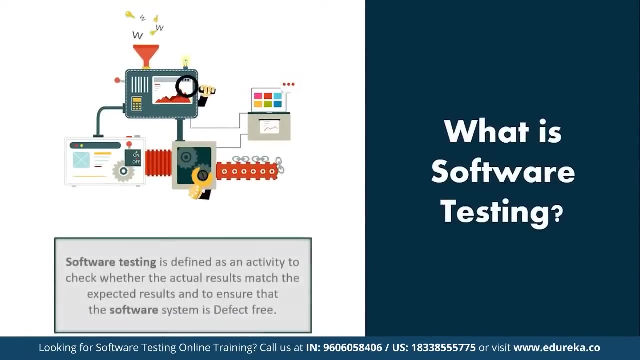 of a software application to find any software bugs. So it checks whether the developed software met the specified requirements and identifies any defect in the software in order to produce a quality product. It is also stated as the process of verifying and validating a software product. 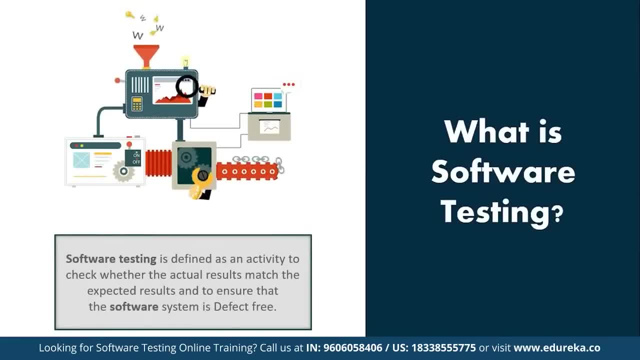 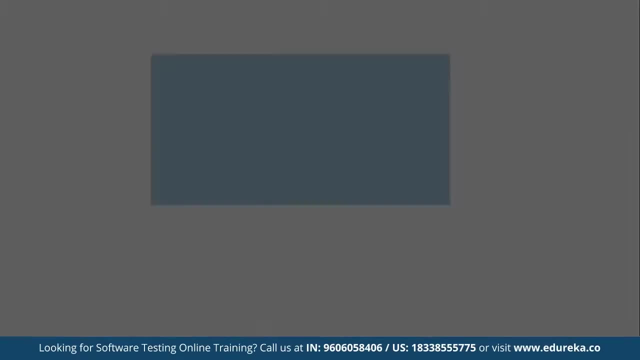 So it checks whether the software product meets the business and technical requirements that guided its design and development. It works as per the requirement and can be implemented with the same characteristics. So now that you know what is software testing, let's see who is a testing automation engineer. 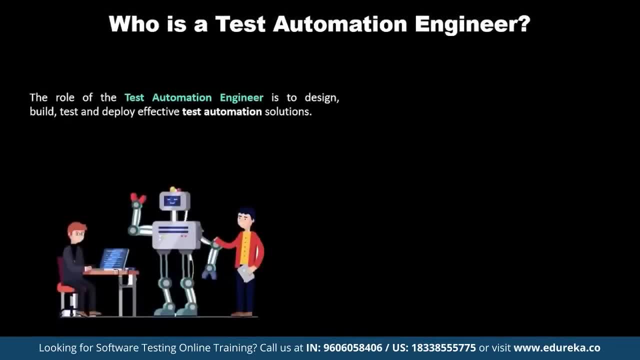 So the role of the test automation engineer is to design, build, test and deploy effective test automation solutions. Now, to fulfill this role, the automation engineer applies appropriate automation technologies to meet the short and long term goals of the testing organization. So now, what does automation engineer actually do? 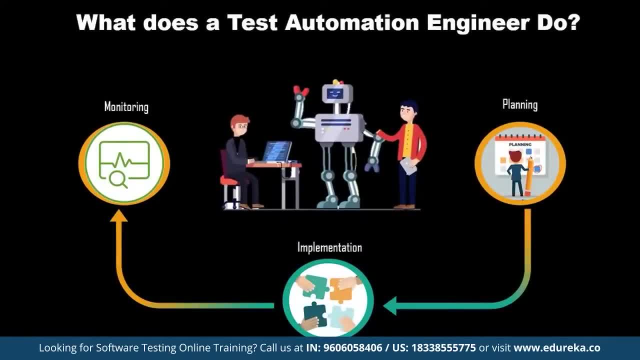 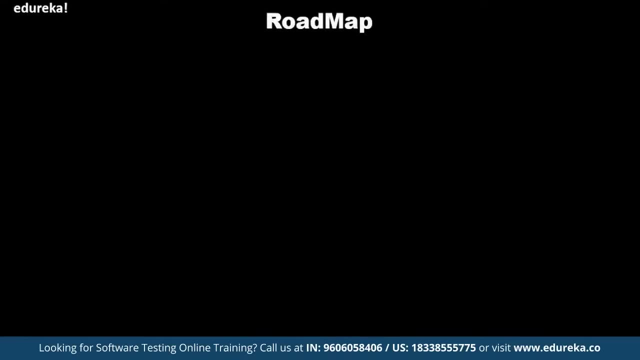 An automation engineer basically utilizes technology to improve, streamline and automate a manufacturing process. They are responsible for planning, implementation and monitoring of such technology. So now let's move ahead and have a look at the road map that will lead you to become a successful test automation engineer. 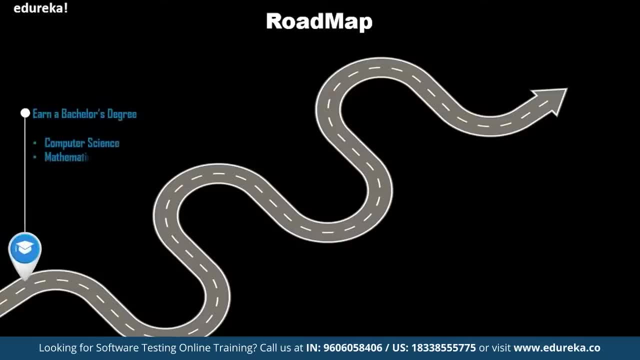 So, first of all, in order to become an automation engineer, you need to have a bachelor's degree. You will likely need to earn a bachelor's of engineering degree related to the field in which you want to work, For example, if you want to become a software testing engineer. 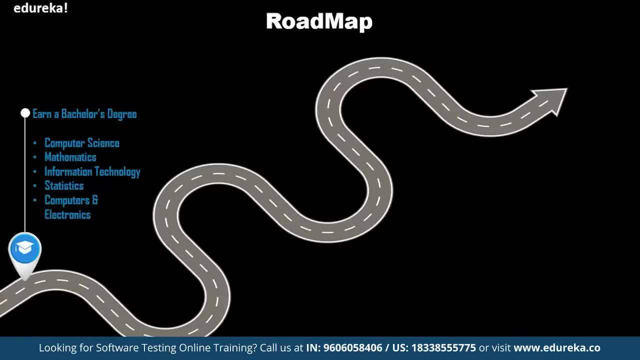 you will need a bachelor's degree in software engineering Now to work in this field. you must be comfortable working closely with other professionals. You also need mathematics and science, and also a little bit of computers and electronics. Now, next up, we will need to know about. 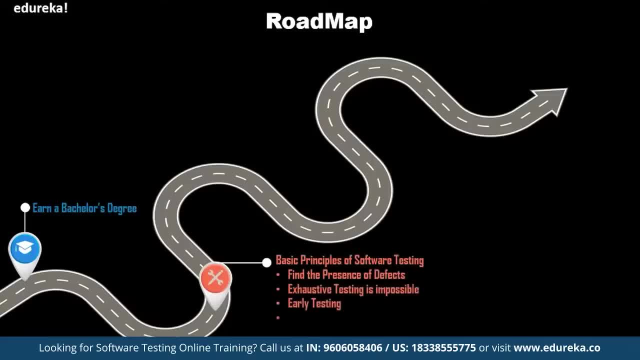 the basic principles of software testing, such as finding the presence of any sort of defects, how to determine the risk without exhaustive testing, early testing, defect clustering and how to make a product fulfill business requirements without any error. Now, if you are new to the testing industry, 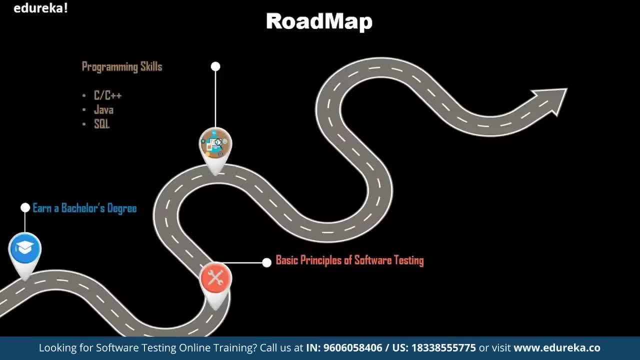 one needs to have knowledge of programming language such as C, C++, Java, SQL, Python, HTML. Now, along with this, if you also have a master's degree in computer science, machine learning, statistics or any such certifications related to automation testing, 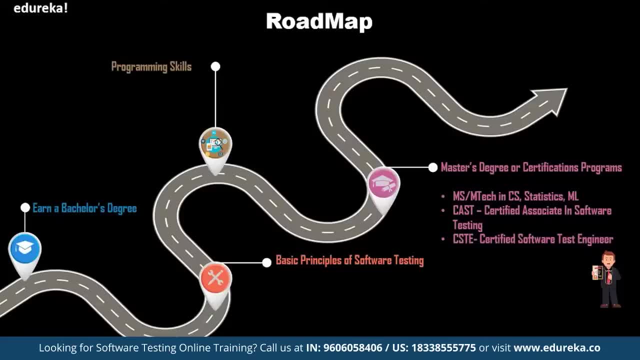 it is just an added advantage. Now, some of the best certifications for a test automation engineer are CAST, that is the Certified Associate in Software Testing, CSTE, that is the Certified Software Test Engineer, and there are many more such certifications. So now let's move ahead and have a look. 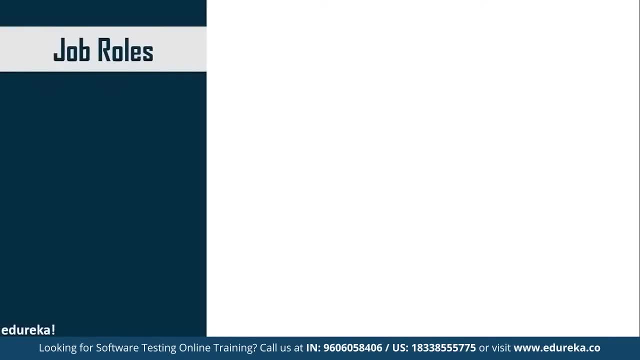 at the job roles for a test automation engineer. Now, some of the most common job profiles include Test Automation, Performance Tester, Test Analyst and QA Engineer. So let's have a look at some of the statistics provided by LinkedIn on these top profiles. So here you can see the graph. 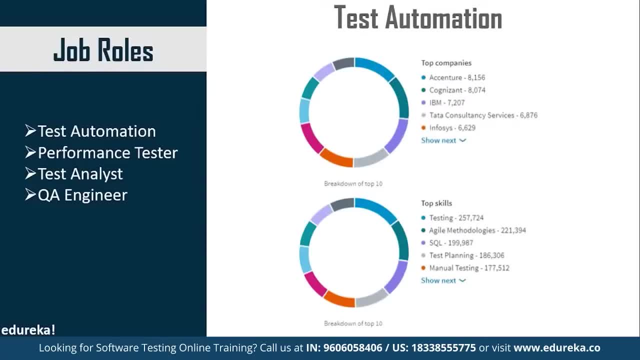 for the top companies in test automation, and some of the big names are Accenture, Cognizant, IBM, TCS and Infosys. Now, the top skills that are required to become a test automation engineer include the knowledge of testing agile methodologies, SQL test planning. 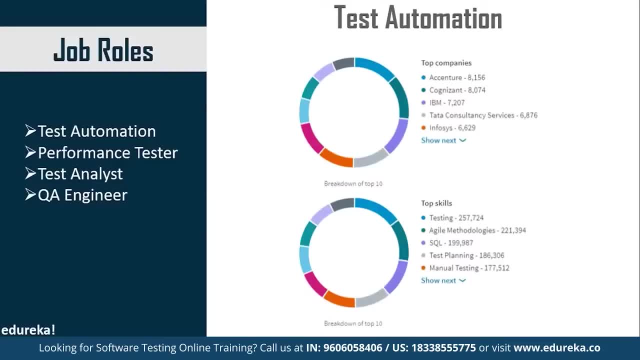 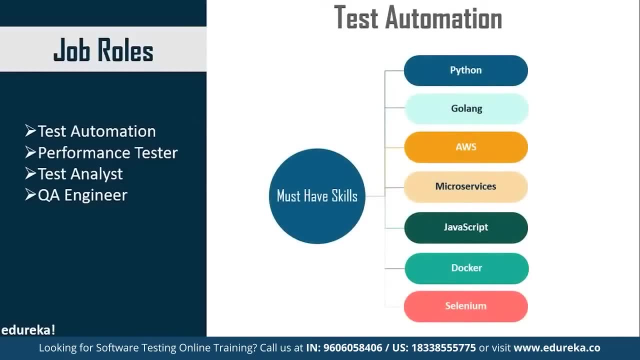 and also you need to be well acquainted with manual testing. Now, apart from these, you need to be well acquainted with programming languages like Python, Golang and JavaScript. You also need to be well versed with AWS, Microservices, Docker and Selenium. 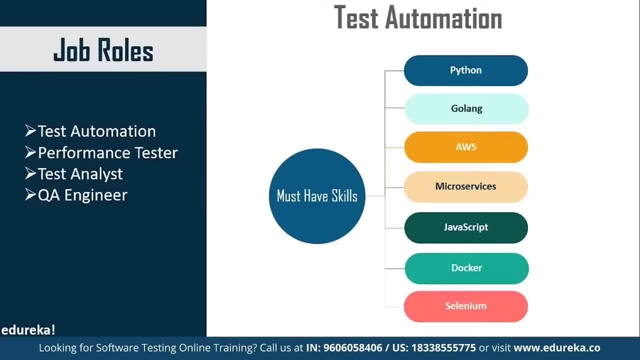 Now these skills will basically help you move to a higher position as a test automation engineer and also adapt your appraisal. Okay now talking about appraisals in Hike. Edureka has released a small video just a few hours back on Hike and appraisal. 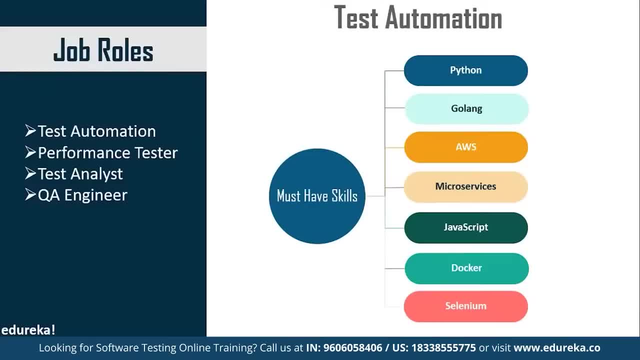 during this season of the year, which is essentially the appraisal season. So do check out our latest video, named Apna Hike Aayega. I'll leave the link in the live chat and also in the description box. Hope you guys will enjoy it. Now moving on. next up is the performance tester profile. So some of the top companies for this job role are IBM, Accenture, TCS, Cognizant and Capgemini. Now some of the top industries for performance tester are the IT services. 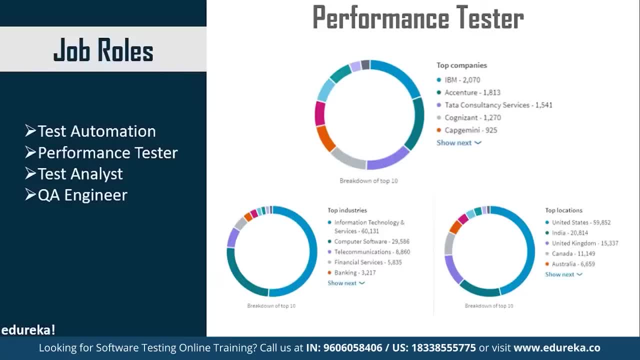 computer software, telecommunications, financial services, as well as banking. Now United States is considered to be the best preferred location for a performance tester, followed by India, UK, Canada and Australia. Now some of the must have skills to become a performance tester include the knowledge of Selenium. 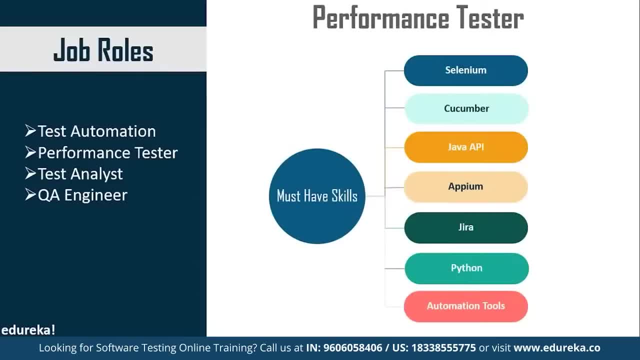 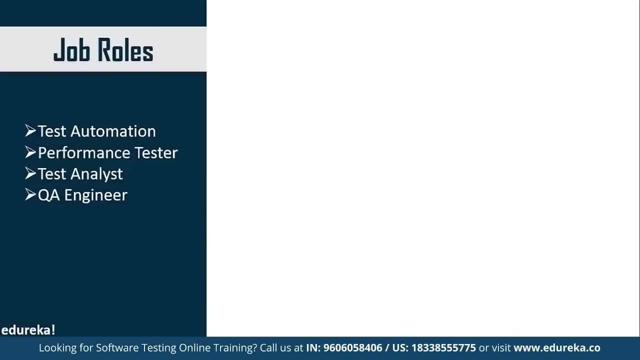 Cucumber, Java, API, Appium, Jira, Python, and also you must be profound with automation tools. So next we will talk about the test analyst job profile. Now for this particular role, Bangalore is one of the top most preferred locations after US, UK and Australia. 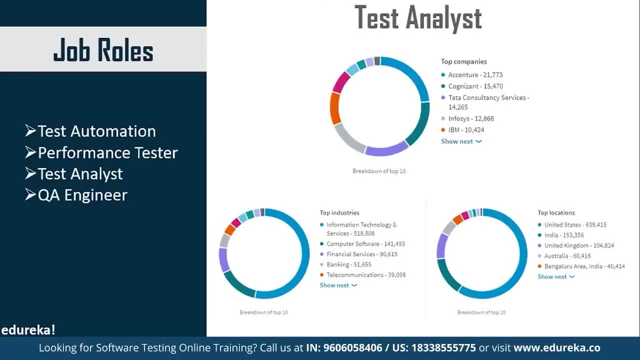 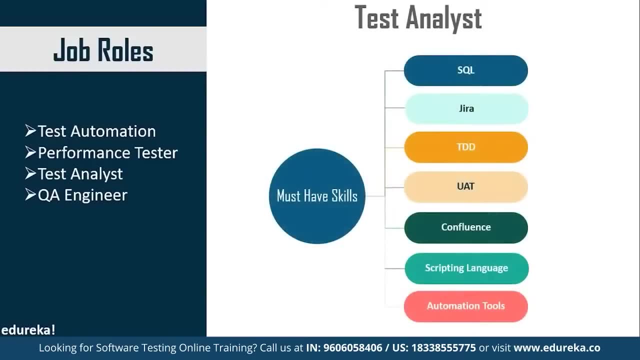 And similarly, companies like Accenture Cognizant TCS are one of the top recruiters. Now, talking about some of the skills: you must be well versed with SQL, Jira, UAT, TDD, Confluence and some of the scripting languages. 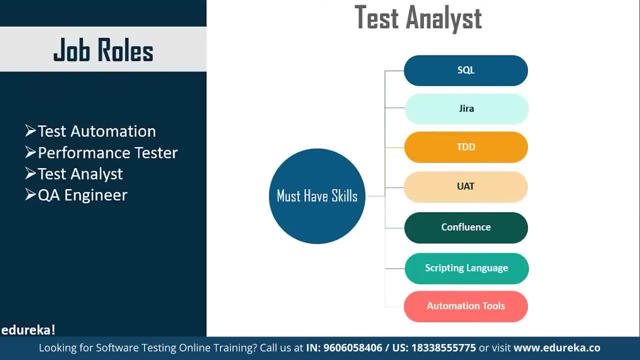 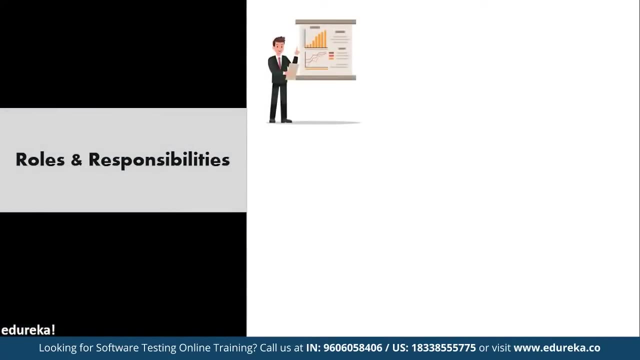 like Python, JavaScript. Also, you would need some of the automation tools. So now that you know about the different job profiles, let's have a look at the roles and responsibilities of a testing automation engineer. Now, in case of software testing, every company defines its own level. 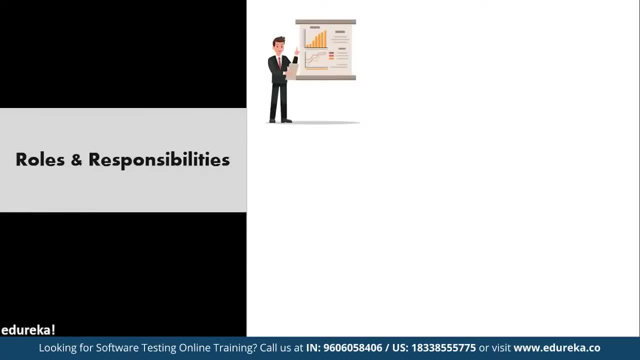 of hierarchy, roles and responsibilities. But on a broader level, if you take a look at software testing, you will always find two levels in a software testing team. The first one is the test lead, or manager. Now, a test lead is responsible for defining the testing activities. 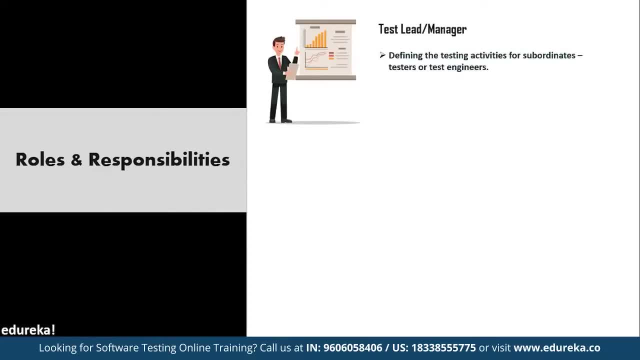 for subordinates, testers or test engineers, All responsibilities of test planning. To check if the team has all the necessary resources to execute the testing activities. To check if testing is going hand-in-hand with the software development in all phases. And finally, 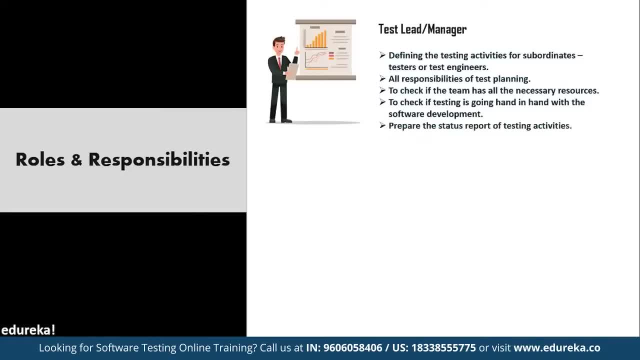 to prepare the status report of testing activities. He is also responsible for required interactions with customers and updating project manager regularly about the progress of testing activities. Next up, we have the test engineers or the QA testers. Now they are responsible to read all the documents. 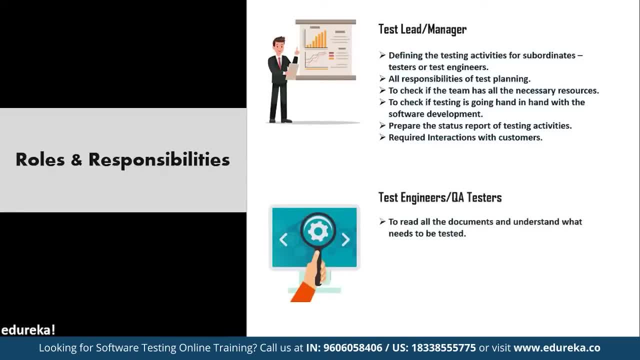 and understand what needs to be tested. Now, based on the information procured in the above step, decide whether or not it is to be tested And inform the test lead about what all resources will be required for software testing. Then develop test cases and prioritize testing activities. 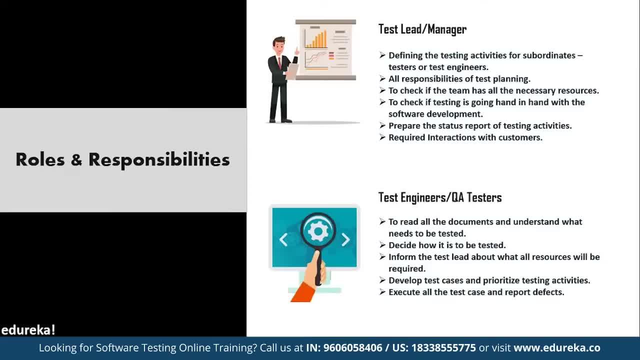 Then we finally execute all the test case and report defects, define severity and priority for each defect and carry out regression testing every time when changes are made to the code to fix defects. Now, how a software application shapes up during the development process depends on how the software engineering team 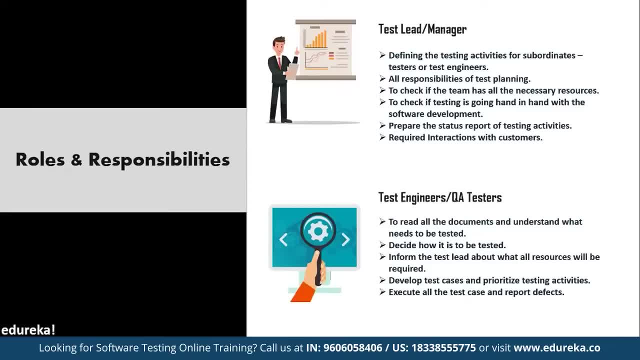 organizes work and implements various methodologies. Now test automation engineers can save you from the world full of codes. Enterprises completely agree with this statement, and this is the reason why you see a lot of job opportunities in automation testing industry. So here I am going to explain. 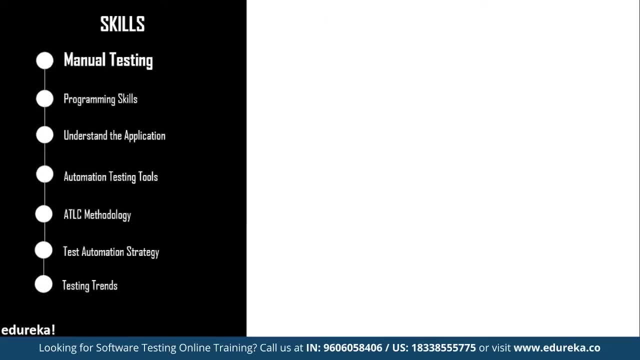 in detail the seven most important steps to becoming a test automation engineer. It will also help you if you are planning to switch your career to automated testing Now. the first one is manual testing Now, while I understand that companies are moving towards codeless automated testing tools, 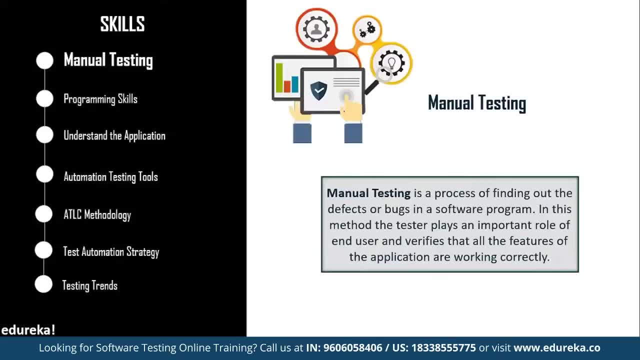 to reach an expert level and to keep up with the competition of automation test engineers in the industry, it is highly important to focus on manual testing concepts initially Now. manual testing is basically a process of finding out the defects or bugs in a software program. 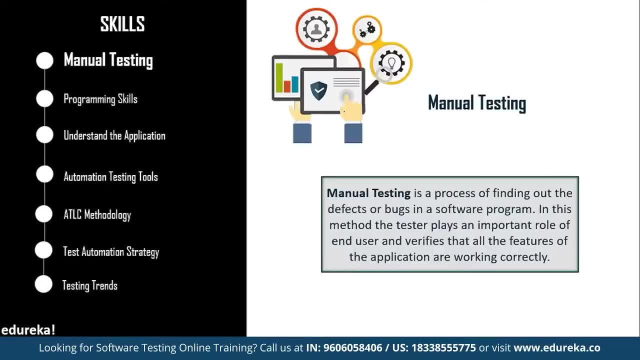 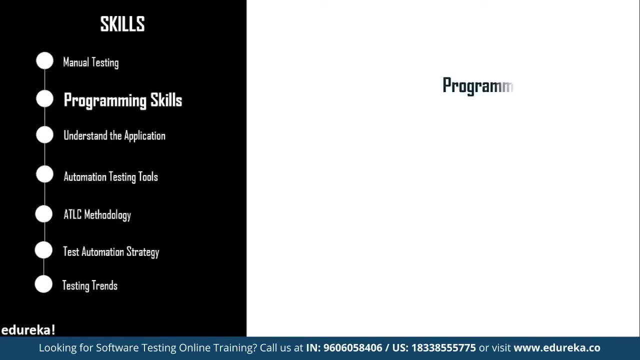 Using this method, the tester plays an important role of end user and verifies that all the features of the application are working correctly. Now this makes a point very clear that automation testing is for experienced manual testers. The next skill is the programming skills. Now it is very important to possess 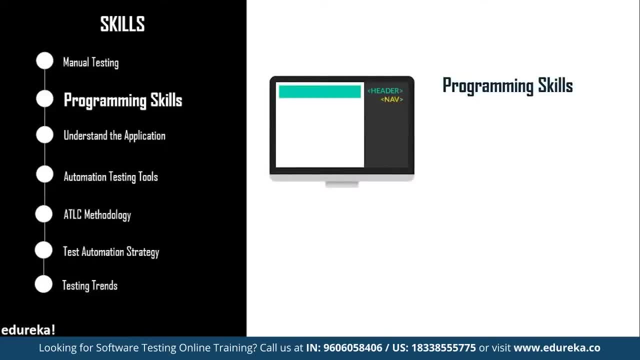 excellent technical programming skills. Now most newcomers ask that if they need programming skills for automated testing. Now, most of the people who come up with the idea of automated testing wish to skip the coding part. Either they don't have programming knowledge or they hate coding. 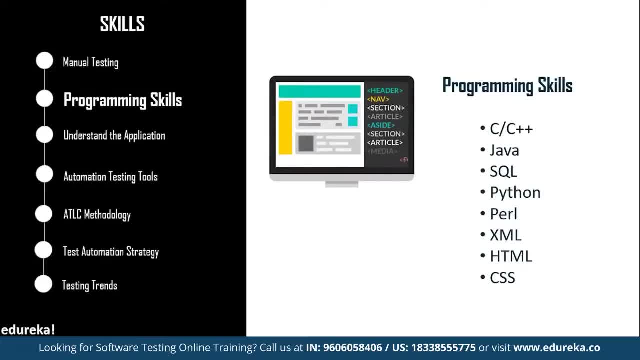 However, that one needs to be very proficient with manual testing skills to become a great automation testing engineer. for a long lasting career in the software testing industry, And if you are new to the testing industry, you need the following programming languages, such as C, C++. 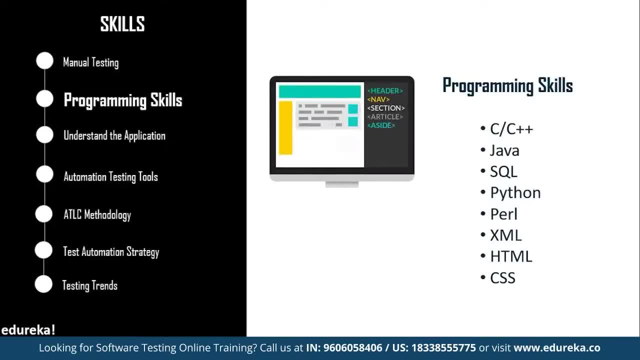 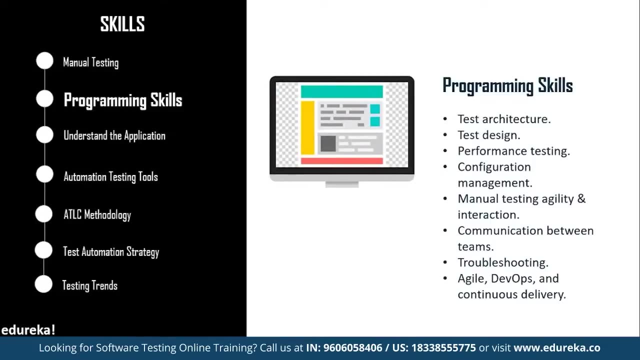 Java, SQL, Python, Perl, XML, HTML and CSS. Now there are also a few technical skills a manual tester should master to become a brilliant automation testing engineer, such as the test architecture, test design, performance testing, configuration management, manual testing agility. 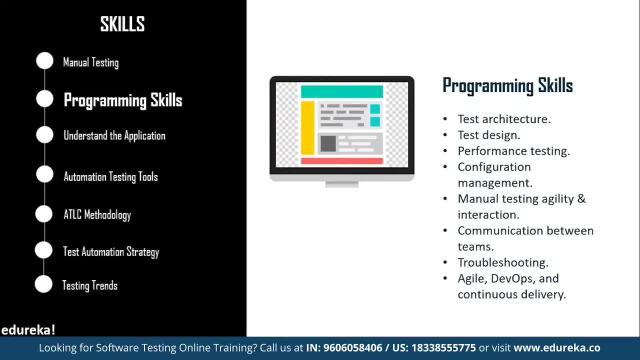 and interaction, communication between the teams, troubleshooting, agile devops and continuous delivery: Now the combination of all the above mentioned skills can help you transit to automated testing easily and smoothly. Now, next up is understand the application. Now the common application details that every automation tester 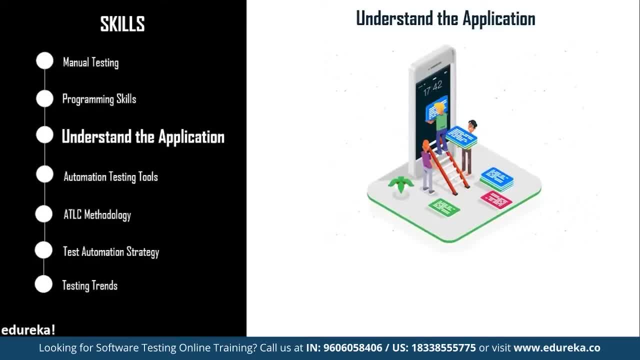 needs to take care of are which programming languages have been used while developing the application. on what platform is the application built, which databases are involved, are there any web services or APIs connected to different parts of the system, and how, and many more such questions. 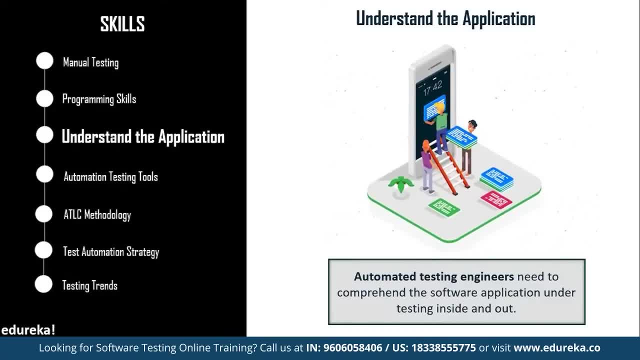 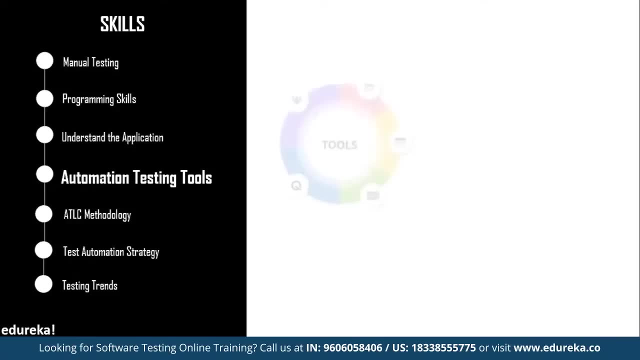 Now, these are just few points and it may vary based on the complexity of the applications. So make sure you are completely thorough with the application that you are going to test via automation testing Now. next up, we have the automation testing tools Now. when learning to become a. 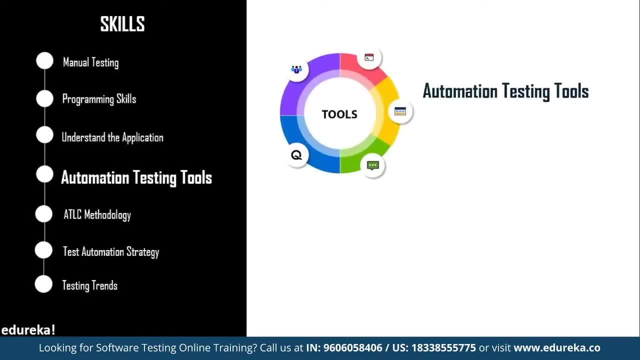 smart automation testing engineer. if we don't talk about the test automation tools, then we are doing an injustice to the industry. A major part of the companies have already started using automation testing tools. Now, the main reason behind using them is to provide benefits to the enterprises. 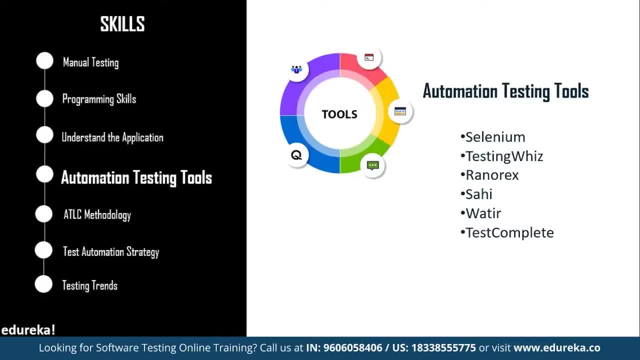 Some of the famous testing tools are Selenium TestingWiz, Ranurex, Sahi Water and TestComplete. Now, next up is the ATLC methodology. Now, ATLC stands for Automation, Testing Life Cycle. Now, the way we follow the life cycle of software development. 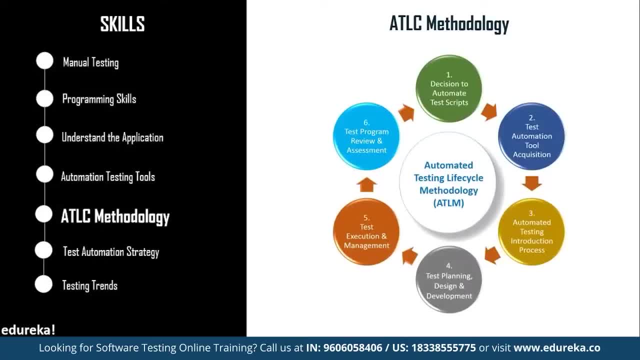 and testing. same is the way for automation testing as well. To understand and follow the ATLC, one needs to have experience of the following, such as the decision making in automated testing, then the test automation tools, automation testing process, then test planning design. 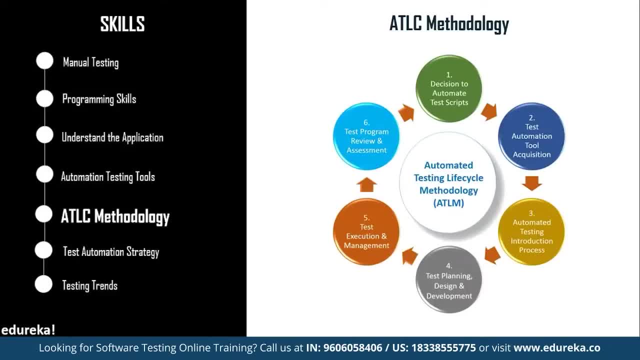 and development, test script execution and management and, finally, review and assessment of test programs. Now for each test automation requirements. a test automation engineer follows the life cycle and to be a successful automation test engineer, you need to understand the ATLC methodology and execute it in your each test automation. 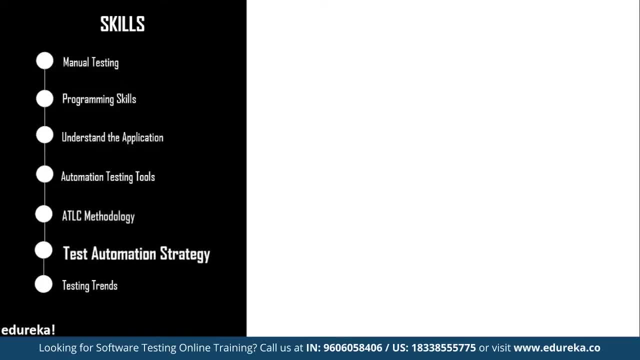 project Now moving on. the next one is the test automation strategy. So once you are through with the ATLC methodology and the automated testing tools, you are well prepared to create your test automation strategy for your clients or employer. Now to become a great automation. 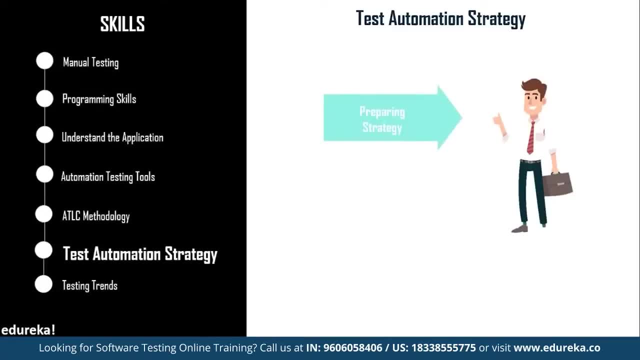 test engineer, you would be the right person to initiate with preparing the test automation strategy, finalizing the tools, overall cost and ROI calculation. Now automation strategy creation is considered to be a very crucial part, as you would need to define and develop the path that will help. 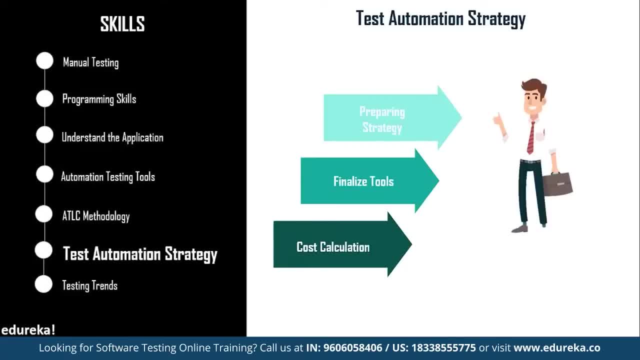 you to reduce the manual testing hours and offer justice on the ROI of the clients. Now let's move on to the final skill, which is the testing trends. Now, for this, you have to stay updated with the testing strengths, and this is the most important part of this industry. 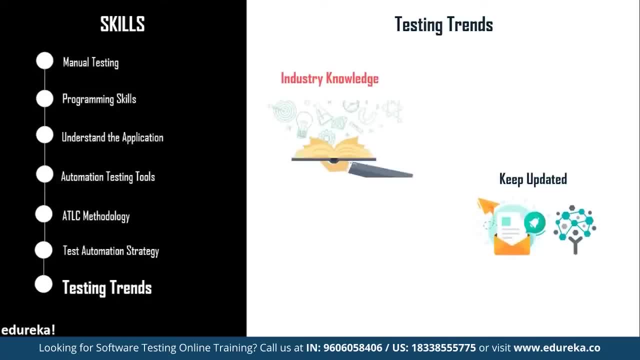 The most trending best practices, tools, techniques, tips and tricks will help you and your team to achieve the success in optimizing your test automation strategies and methodology. Now this generation is moving towards automation everywhere. However, there has been a lot of debate around test automation tools replacing 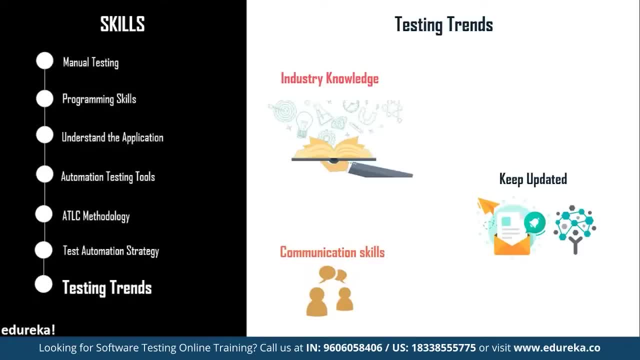 the manual testers. But remember, the creators of test automation tools are the testers like you. So to become a smart automation testing engineer and to be successful in this industry, you would need to really work hard, with passion and dedication. So once you have mastered these skills, 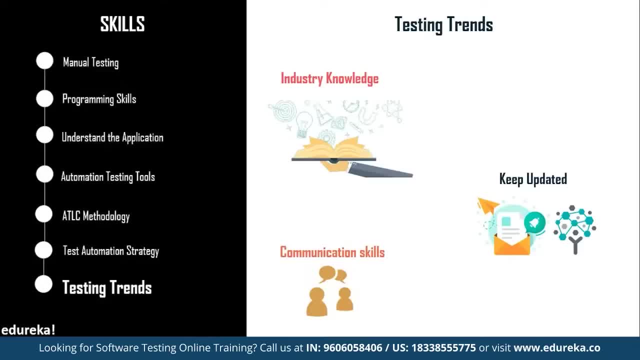 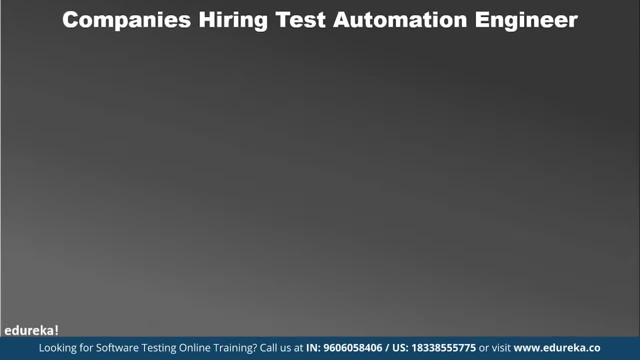 you are now on your way to become a successful software test automation engineer. Now let's see some of the top most companies that are hiring for a test automation engineer Now. these companies are Accenture, IBM Cognizant, Infosys, TCS. 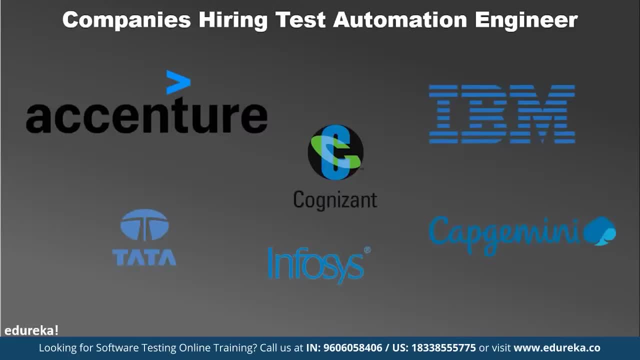 and Capgemini. So do keep an eye for an opportunity and utilize your skills to grab the offer. So that was all about today's session, and I hope this will help you in the long run to prepare yourself and get well versed with all the skills. 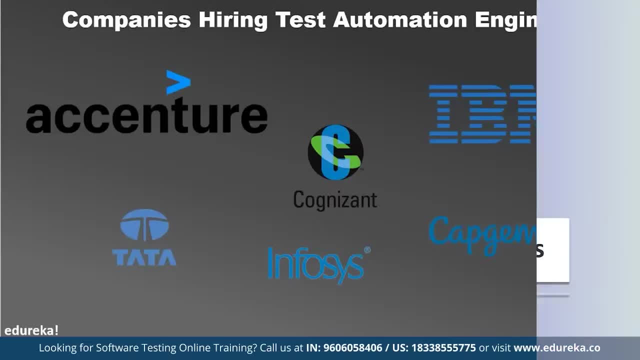 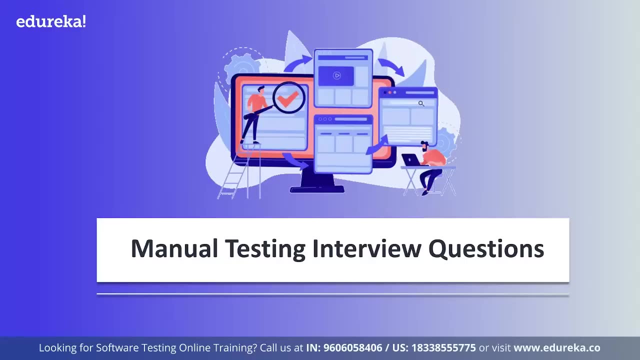 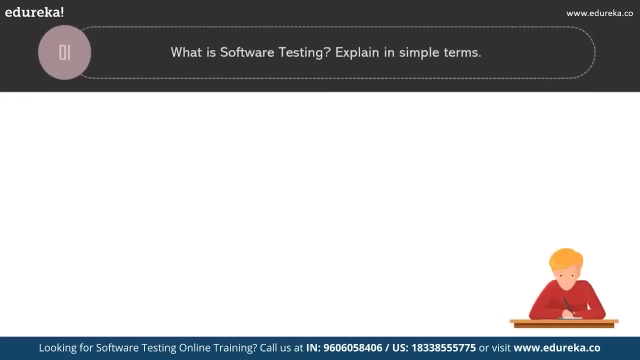 in order to become a successful test automation engineer. So here we go. Let's begin with the first category of questions, which are beginner level questions. The first question that we have here is very basic: What does software testing explain in simple terms? Do you guys agree with me when I 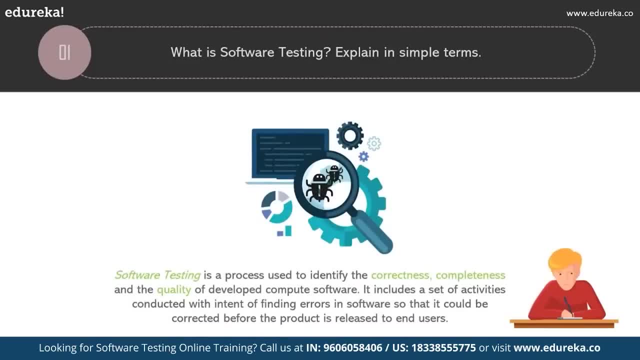 say every system has software bugs. Well, it's true, right, It's impossible to design and bring out a perfect software product. So software testing, basically, is the process of executing any sort of software or an application to find out if there are any bugs or 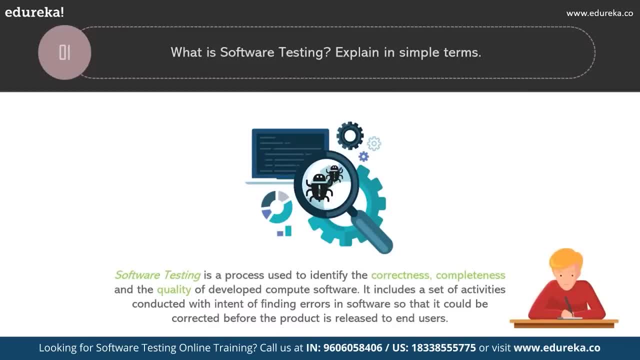 some sort of errors in it. So before actually goes public, programmers spend hours trying to iron out every little bug there is. They check for any mistakes and problems in the design and the functionality of the software. Well, until then product won't be available. 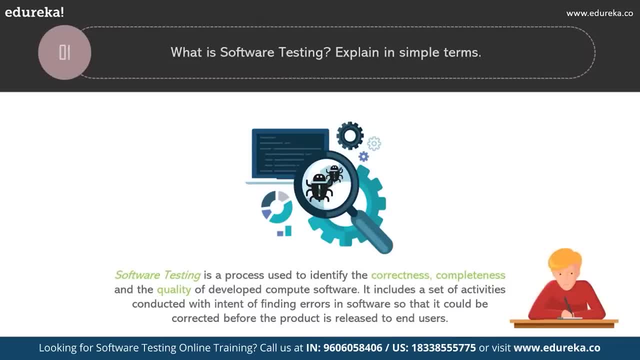 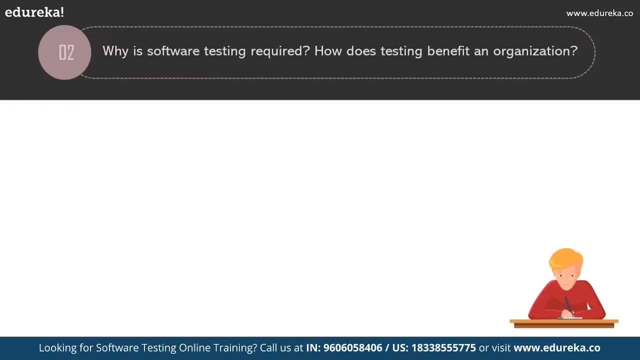 for commercial use in the market. So, as that name already suggests, software testing means checking the developed software for any mistakes and problems in the initial design. Next up we have a following question, which says why is software testing required and how does testing benefit? 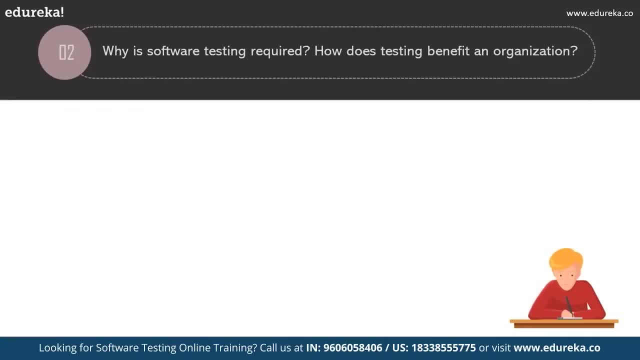 an organization. Software testing is really a mandatory process which guarantees that software product is safe and good enough to be released to market for public to use it. Well, here are some compelling reasons to prove why testing is really needed. First of all, it points: 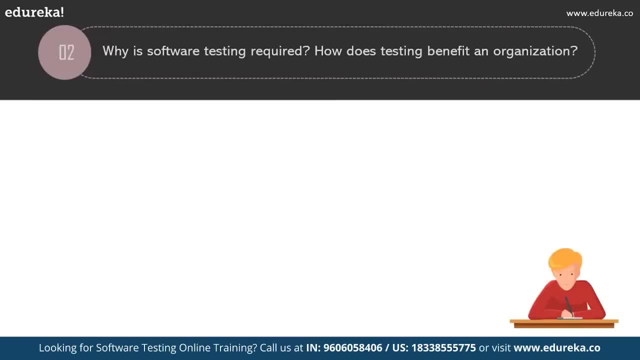 out the defects and errors that were made during the development phase. So, basically, it provides a quality assurance, It reduces the coding cycles by identifying issues at the initial stage of development, It ensures that software application requires lower maintenance costs and it results in more accurate. 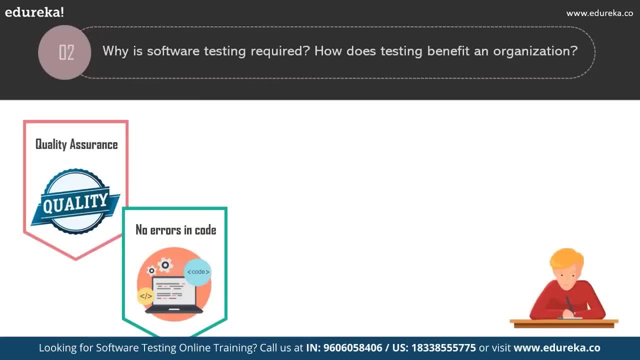 consistent and very reliable results. Testing ensures that customer finds the organization more reliable and their satisfaction in the application is maintained continuously. Testing also makes sure that software is bug free and the quality of the product meets the market standard. And, lastly, it ensures that the 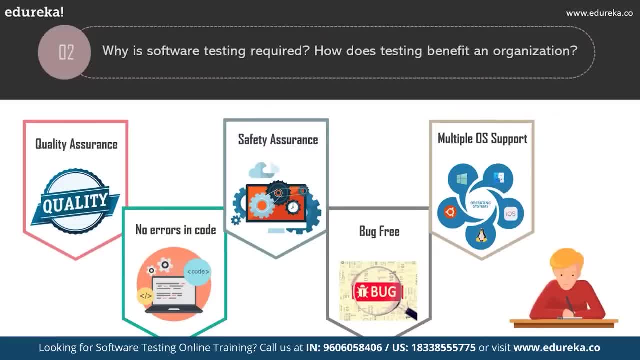 application doesn't result in any failures that could be of some harm to people who are using it. So in this way, software testing is really required to bring out a high quality and safe product to market. Moving on to next question, we have: what are the 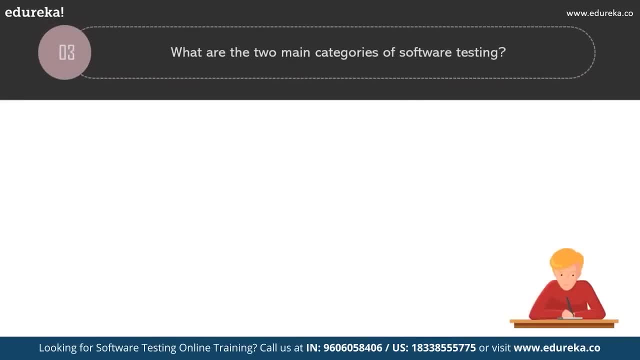 two main categories of software testing. Well, software testing can be divided into multiple categories based on different scenarios, but mainly you can divide software testing into two types, which is manual testing and automation testing. So manual testing, it's pretty self explanatory. which is testing of a web. 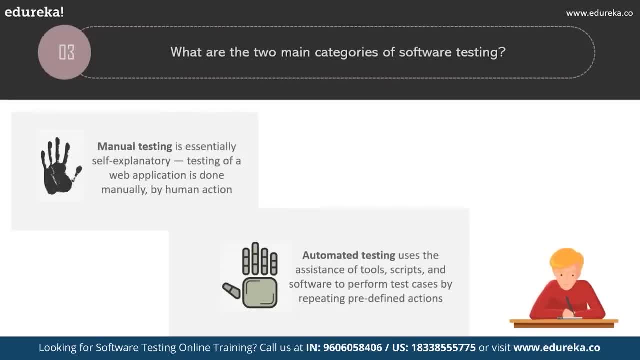 application is basically done by human action. That means someone actually goes on a device to evaluate numerous components like design, functionality and performance of the application. but a testing to find defects or bugs manually is really time-consuming, right, It's expensive, It's often. 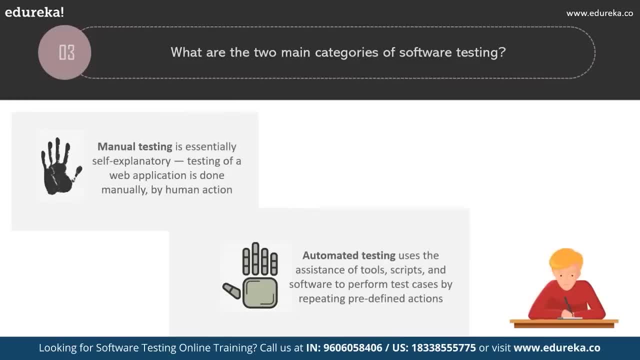 repetitive and it's subjective to human error, and that is why automation testing comes into picture. Automation testing is well automated, if I have to tell. automation testing uses the assistance of tools, scripts and software to perform test cases by repeating predefined actions. So these are two main 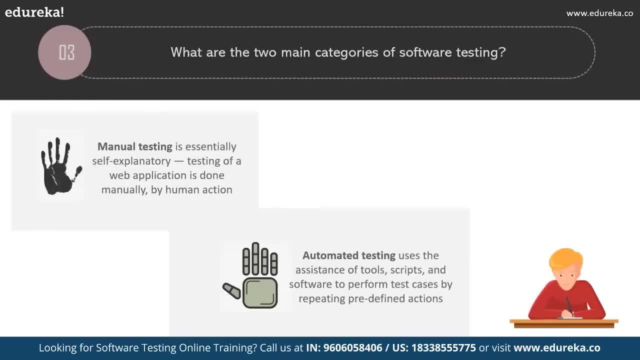 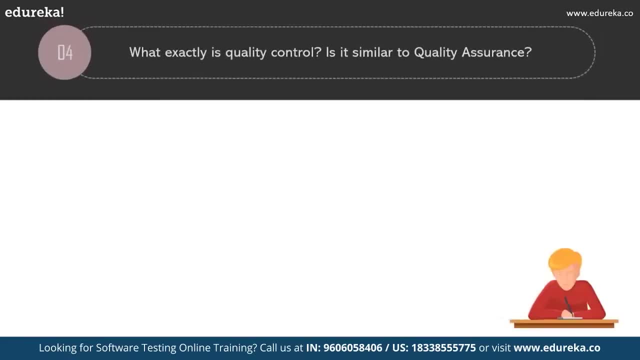 categories of software testing: manual testing and automation testing. Next question that we have is: what exactly is quality control? There are different terms that are associated with quality when we are referring to software. You have quality control, quality assurance and many more. So what exactly is quality control? 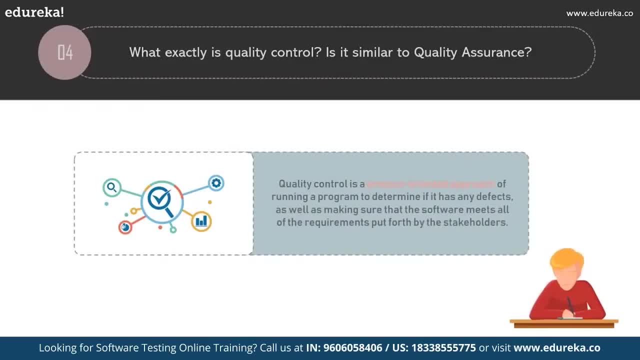 Well, quality control is the product-oriented approach of running a program to check if it has any defects. The key point that you have to remember is it is product-oriented approach. So, using quality control testers, make sure that the software meets all the requirements, which are: 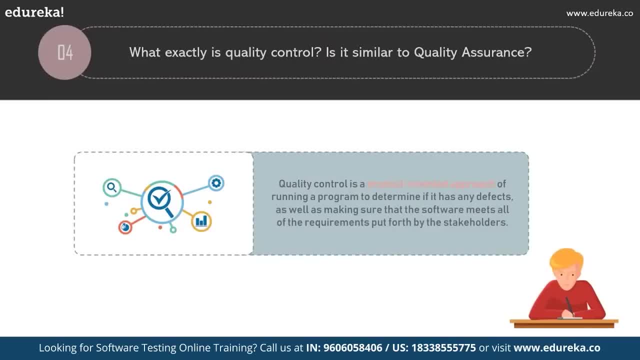 put forth by stakeholders and end users. It includes different type of testings, like you have functional testing like unit testing, usability and integration testing. You also have non-functional testing, like compatibility, security and performance and all that. So quality control is a product-oriented approach of. 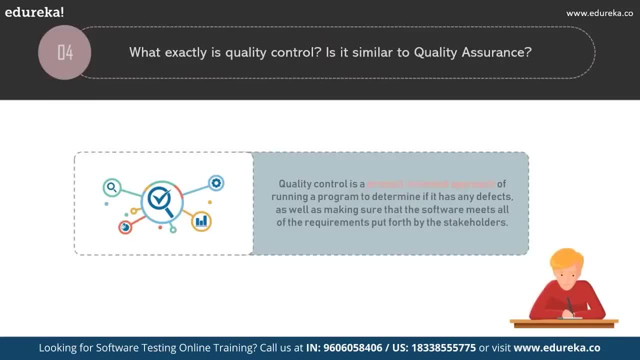 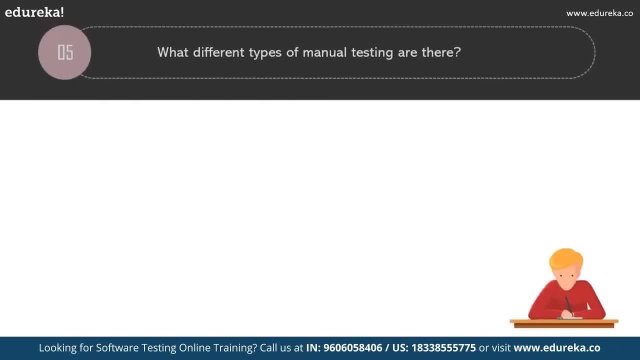 running a program to determine if it has any defects or not. Moving on to our next question, It says what different types of manual testing are there? Well, basically you have six types of manual testing, which are: black box testing, white box testing, unit testing, system testing acceptance. 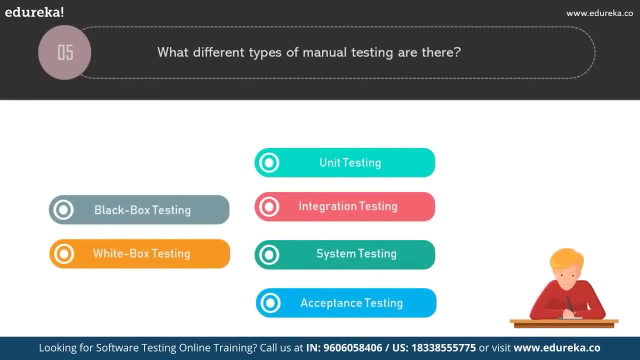 testing and integration testing. Well, let me explain you all of these types in a very brief manner, But if you want to know more, you can actually go to our website at goahead and refer to Edureka YouTube playlist on software testing. So what exactly is black box testing? 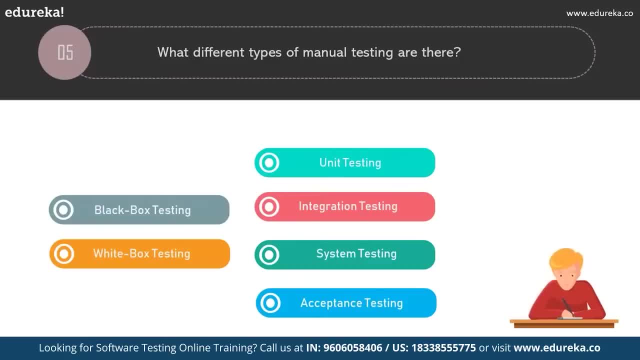 in black box testing, testers analyze the functionality of the software or an application without actually knowing much about the internal design or structure of the application that they're testing. talking about white box testing, and like black box testing, white box requires a profound knowledge of code, as it includes testing of some 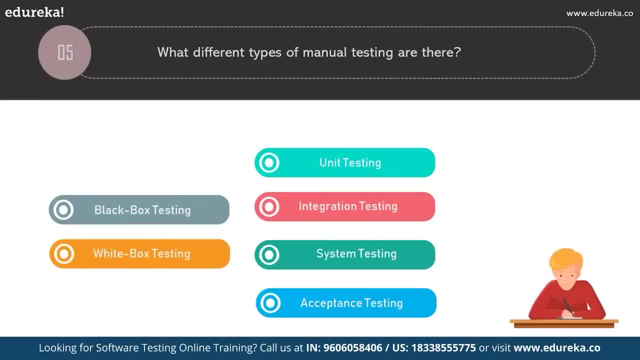 structural part of the application. Next question is about the unit testing. It's a way of testing the smallest piece of code, which we usually refer to as a unit. then there's integration testing, where you test the interface between the units. after that we have system. 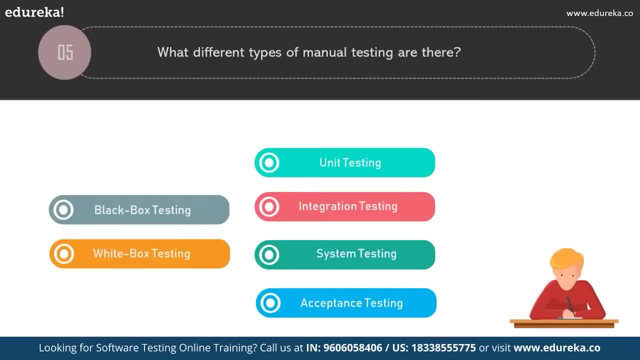 testing, which is done to examine the fully working of an integrated software system against the user requirements. and lastly, we have you 80, or acceptance testing. It's a formal testing that's performed based on user requirements and function processing. this type of testing that we call 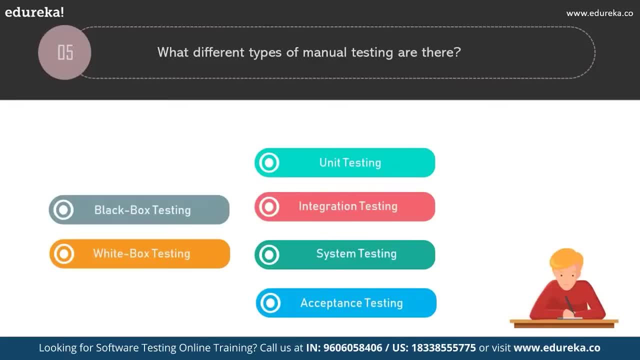 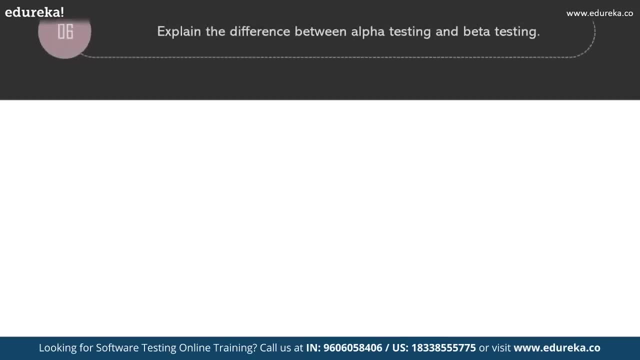 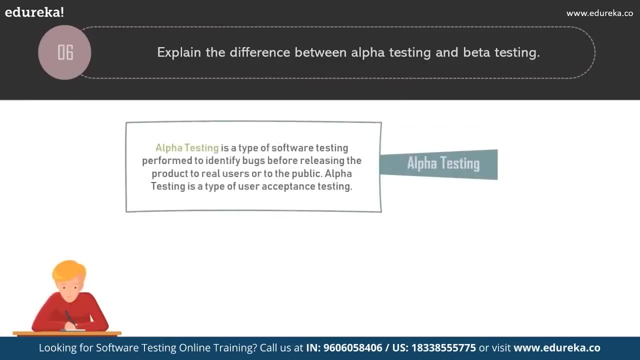 acceptance testing. it covers end-users, real-world scenarios. So yeah, these are six typical types of manual testing. moving on to the next question, explain the difference between alpha testing and beta testing. well, both alpha and beta testing are customer validation methodologies. on top of that, both of our acceptance testing 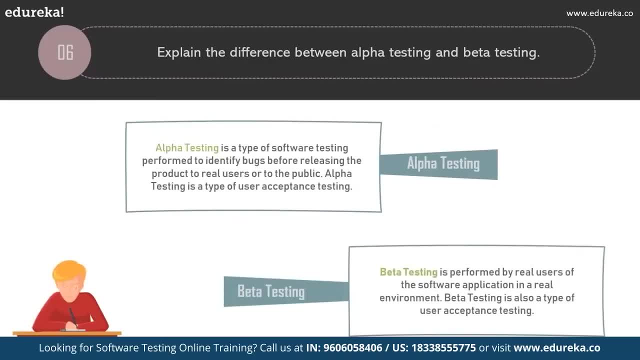 types. they help in building confidence to launch the product in the market and that's how they result in success of product in the market. So what exactly is alpha testing? alpha testing is internal acceptance testing which is performed to identify all possible issues and bugs. after. 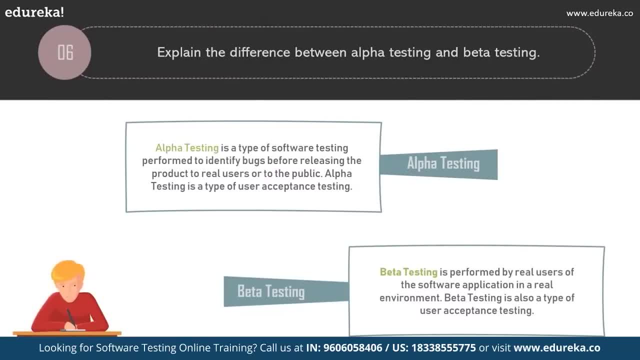 acceptance testing, but before releasing the software for beta testing. So the focus of this testing is to simulate real users by using black box and white box technique. The key point is you perform it after acceptance testing, but before actually releasing the product for beta testing. now beta. 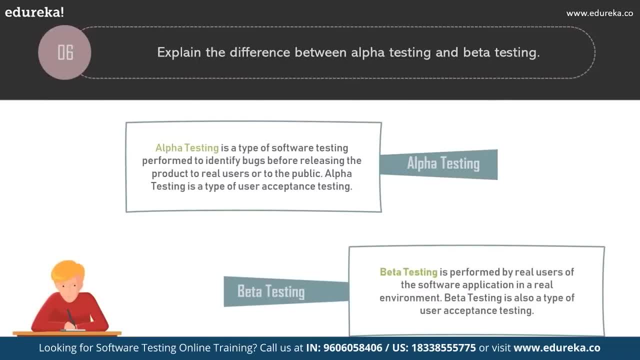 testing of a product is performed by real users of software application in real environments. It allows the customer an opportunity to provide inputs to the design, functionality or it could be usability of a product, though companies like do rigorous in-house quality assurance with dedicated test teams. 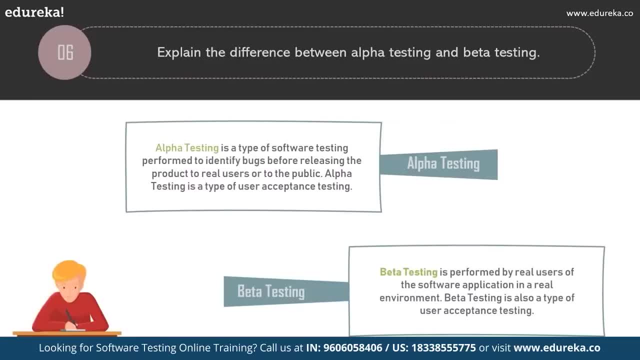 It's practically impossible to test an application for each and every possible combination of test cases. right, and that is why beta releases make it much more easier to test the application on thousands of test machines and fix the shoes before actually releasing the product to market and alpha testing. 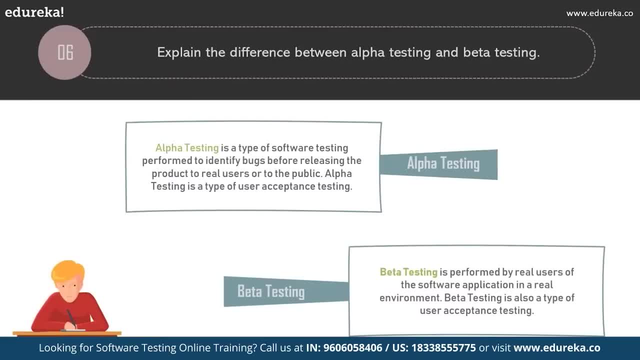 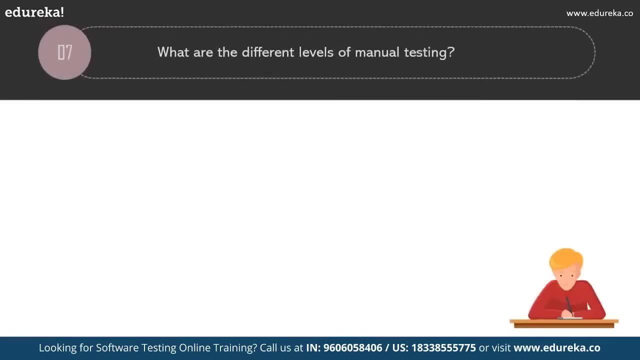 is performed before beta testing. So yeah, that's the difference between alpha and beta testing. I hope the difference is clear. Let's move on to next question. What are the different levels of manual testing? so beat a manual testing or automation testing, or 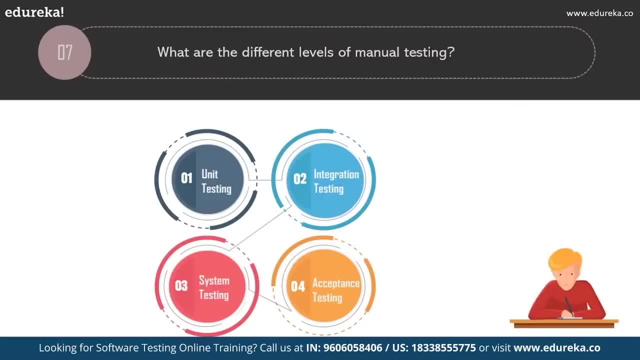 software testing in general. There are like four levels. first up, you have unit testing, then there's integration testing, after that system testing and lastly you have acceptance testing is a way of testing the smallest piece of code, which is referred to as unit. a unit is something that can be. 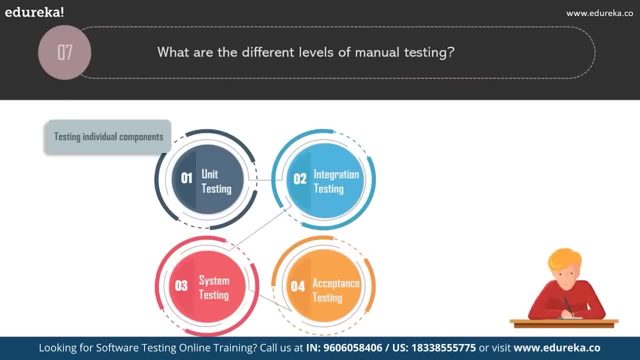 logically isolated in a system. It can be anything that you want. It can be a specific piece of functionality, or it can be a program or a method in a program- anything. So the main focus here is on the functional correctness of the standalone modules or units. 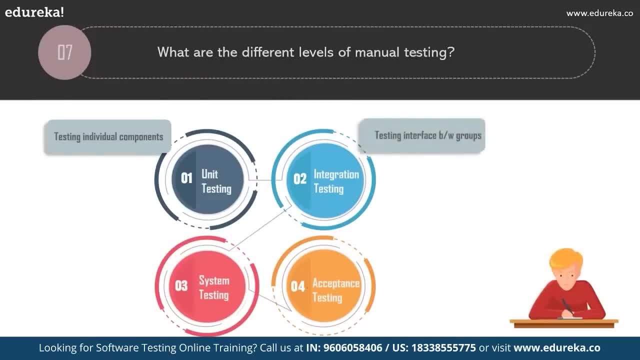 next up there's integration testing. It's performed after unit testing, when different units, components and modules are integrated together. The focus of integration testing is to check the correctness of communication among all the modules. So in simple terms, you can say that you are checking. 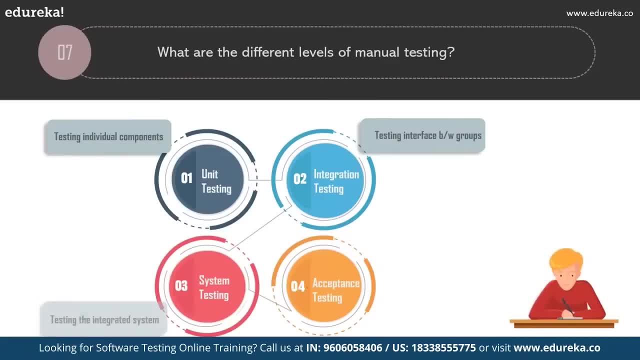 the interface that's there between the different units or modules. after that the system testing is carried out on a complete, fully integrated software product to evaluate the behavior of the system and then to examine the fully working of an integrated software application according to user requirements. On the system testing, we have different 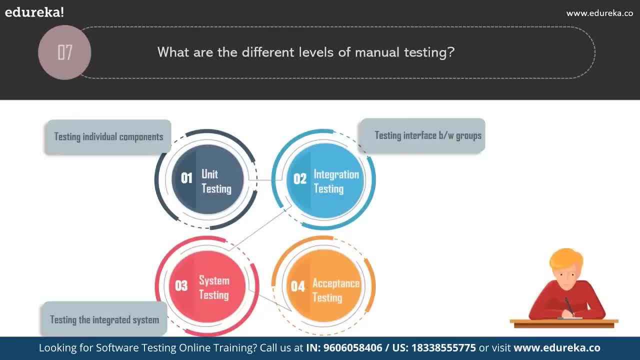 techniques like functionality testing, performance testing, scalability testing, load testing, stress testing, regression testing and many more. and the last level that we have is UAT, or user acceptance testing, or, in simple terms, acceptance testing. It's the formal testing that's performed based on user requirements and function. processing this. 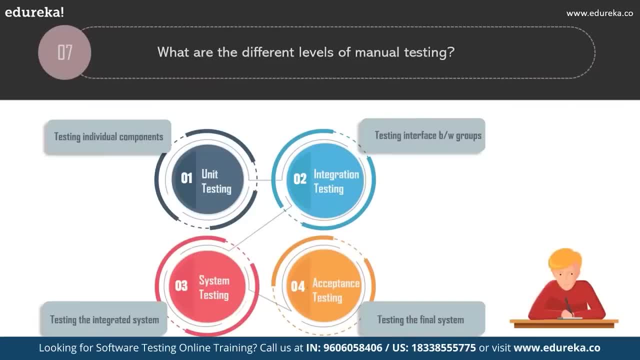 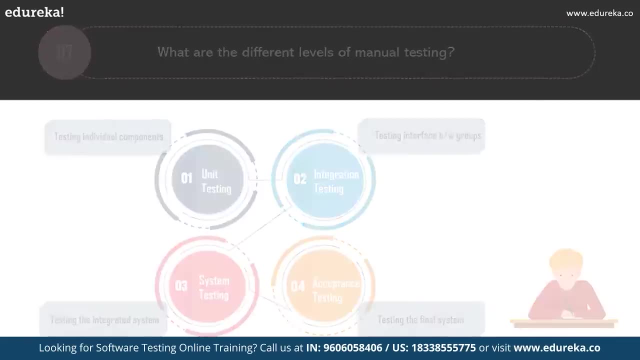 acceptance testing actually covers end users, real-world scenarios. and this last level needs to be done to correctly because it provides you with the result on the basis of if the software product is fit to be released to the market or not. So yeah, these are four levels of. 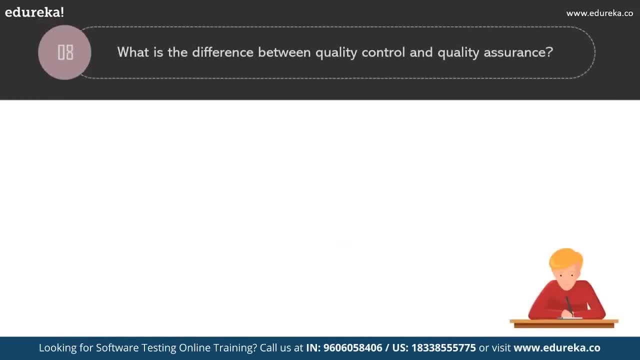 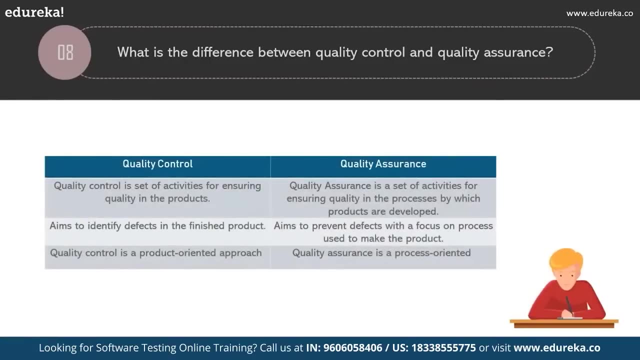 manual testing. So the next question that we have is: what's the difference between quality control and quality assurance? We did already talk about what quality control is. quality control a set of activities for ensuring quality in the product, So the activities focus on identifying defects in 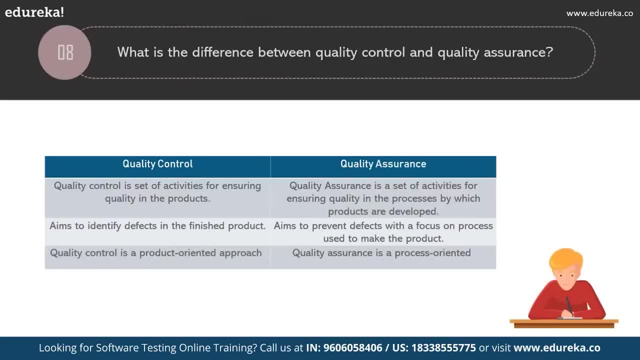 actual product produced, Whereas quality assurance is set of activities for ensuring quality in the processes by which product are developed. So you get my point right: quality control is a product oriented approach- You're checking the quality or defects in the product- whereas quality assurance is a process oriented. 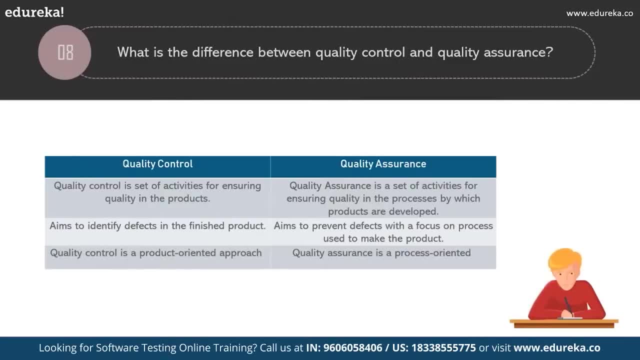 approach, You're checking the quality of the process by which products are developed. So quality control aims to identify defects in the finished product. Therefore it's a reactive process, whereas quality assurance prevents defects, with the focus on processes which are used to make the product. Therefore, it is a 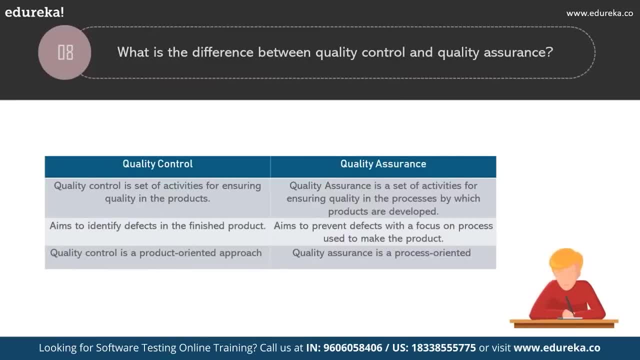 proactive process. I hope the difference is clear. Let me summarize: quality control is a product oriented approach of running a program to determine if it has any defects, as well as making sure that software meets all the requirements put forth by end user and stakeholder, Whereas quality 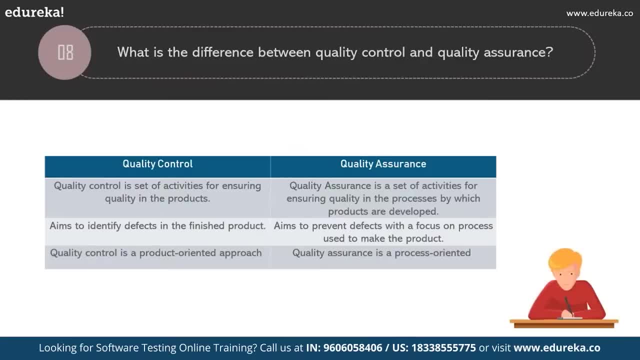 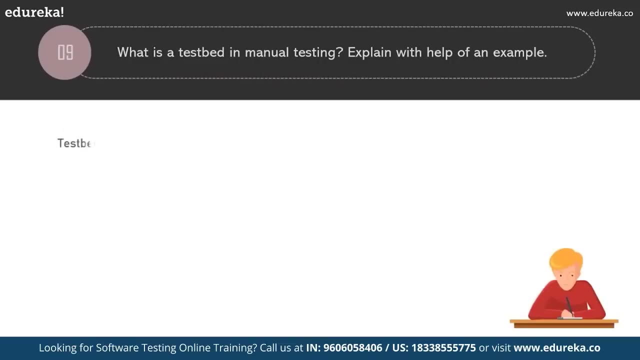 assurance is a process oriented approach that focuses on making sure that methods, techniques and processes which are used to create the product meets the quality standard. The next question that we have is: what is a test bed in manual testing? explain with help of an example test bed. 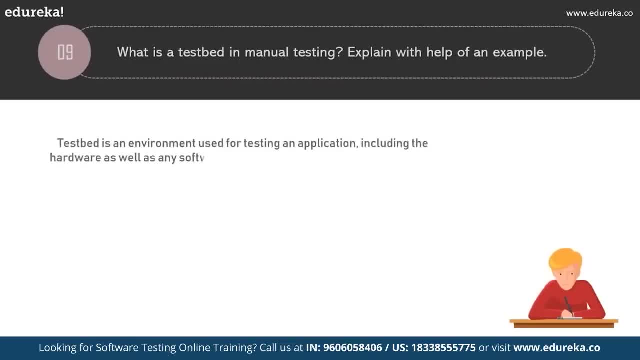 in simple terms, is a test execution environment which is configured for testing. It consists of hardware, software, network configuration application which is under test, operating system settings, software configuration, test terminals and much more. So, in simple terms, it's a test execution environment which is 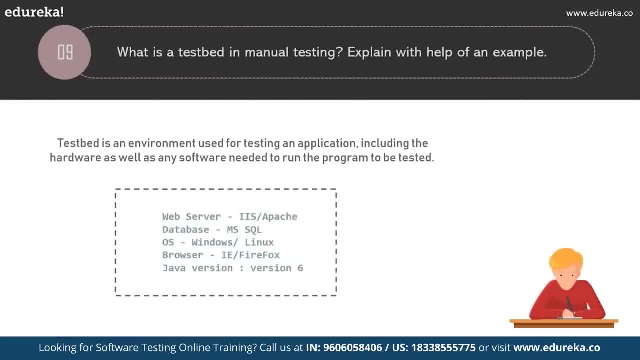 configured for testing. Well, a typical test bit for a web-based application looks something like this: You have Java version listed out. You have the browser that you're using listed out operating system settings like Windows or Linux in the database that you're using- web server, Etc. It. 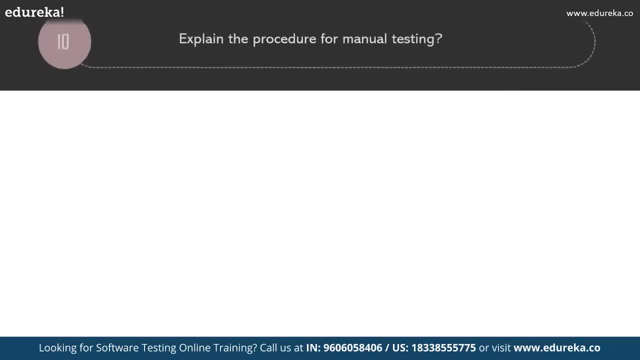 has all the details which are required for you to perform testing. Next question is: explain the procedure for manual testing. Well, it's quite simple and similar to any other standard software testing. First of all, you start by understanding the requirements which are put forth. 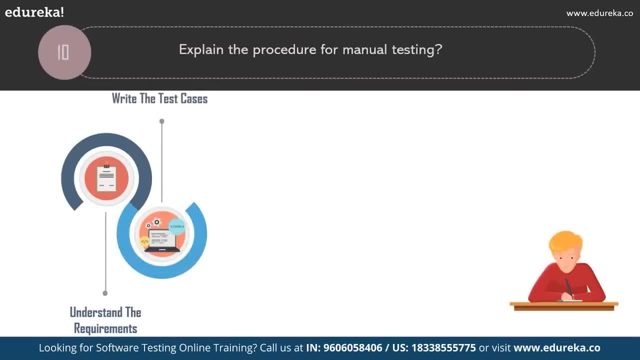 by the users. based on the requirements, you write the test cases and after that you conduct the test cases that you have written and categorized. once you've conducted the test and you have your result, you create good bug report which you will have to submit to your manager or 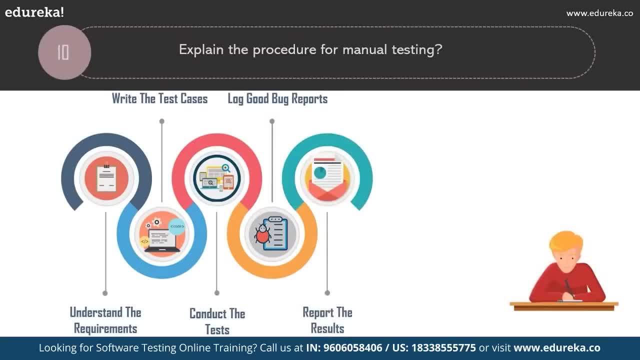 higher-level people in the next stage. simple enough, right? You start with understanding the requirements put forth by the users. you categorize the requirements and write test cases and separate them into different groups to make it much more easier to identify. once you have your test cases, you execute them and 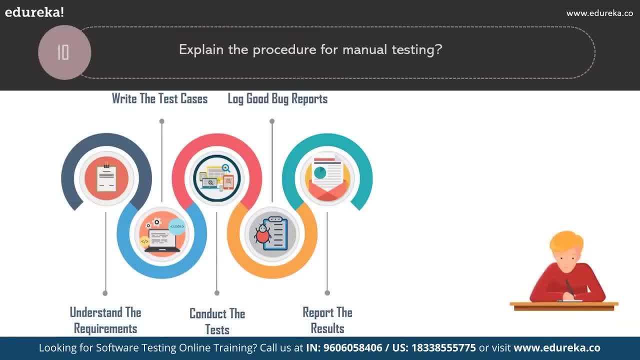 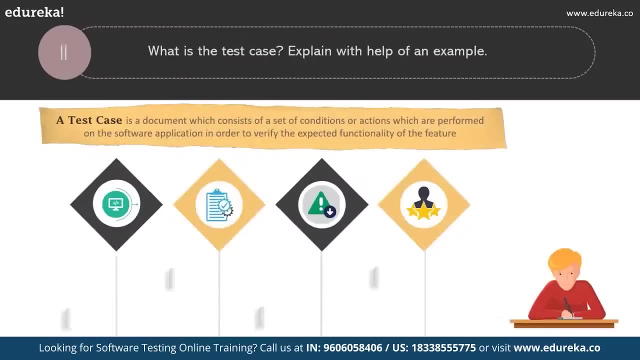 once you get the results, you create reports and submit the reports to higher authorities. So that's the general procedure that you follow when performing manual test. The next question is: what exactly is test case? explain with an example, guys. documentation plays a very important role in testing. beat manual testing or. 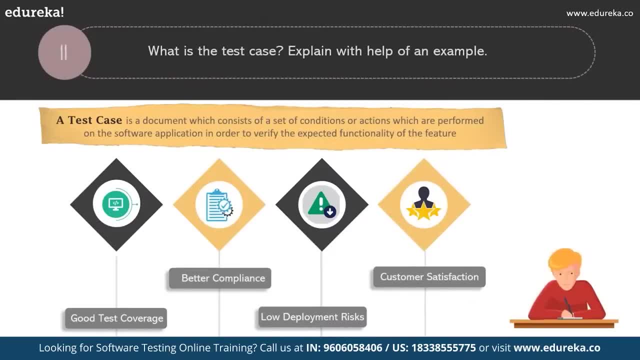 automation testing. a test case is very important because it is one of the documentation used. It's a document which has set of conditions or actions that are performed on software application in order to verify the expected functionality of a feature. So, basically, test cases describe a. 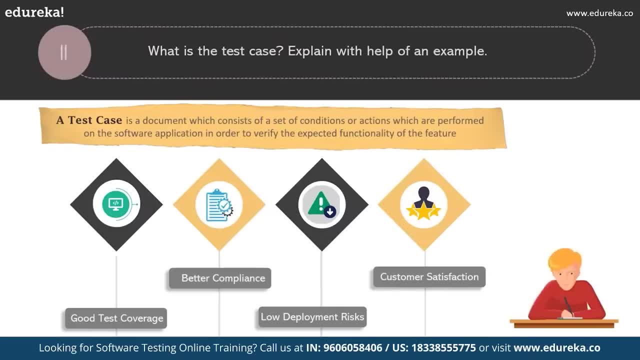 specific idea that is to be tested, without actually detailing the exact steps to be taken or data to be used. For example, let's say in a test case your document looks something like this quotation test: if coupon is used in a test case. So in a test case, your 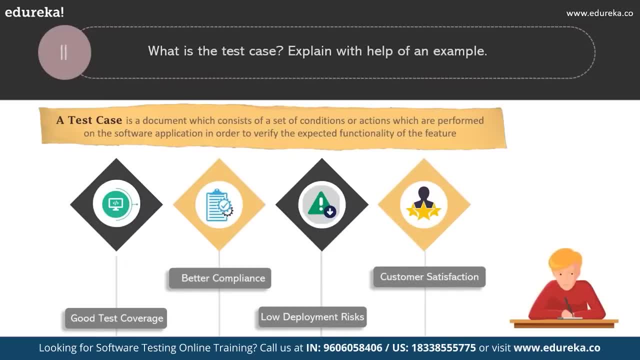 document looks something like this: coupons can be applied to actual price. quotation close. So that's your test case statement. Let me read it again: test if coupons can be applied on actual price. So, as you can notice, this statement doesn't actually mention how to apply. 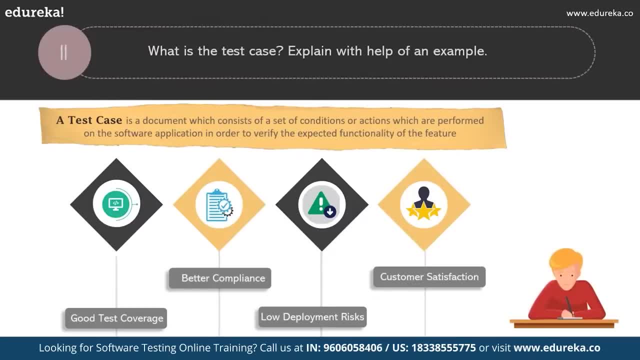 the coupons or whether they are multiple ways to apply or not. It doesn't mention if tester uses a link to apply discount or does he enter a code or does he have a customer service to apply it. It doesn't go into much details, It just specifies the major. 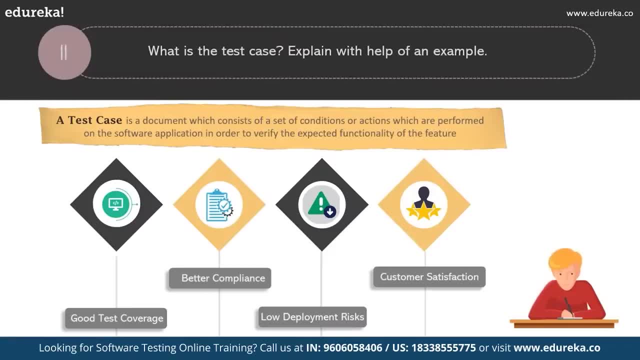 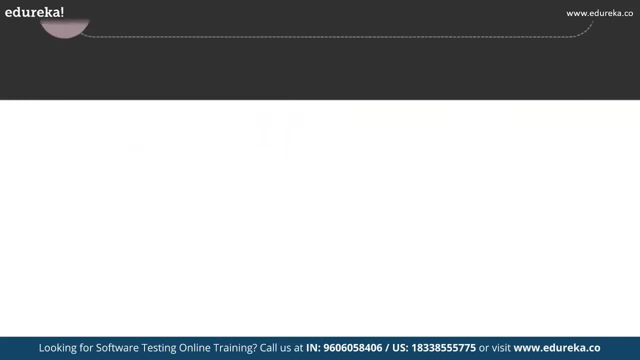 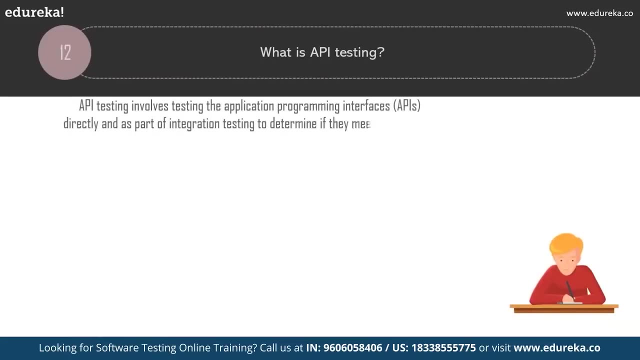 objectives of testing in simple terms. So these test cases, they give flexibility to tester to decide how they want to execute the test. Next question that we have is: what is API testing? API, as you guys might know as an acronym for application programming interface, which is a software. 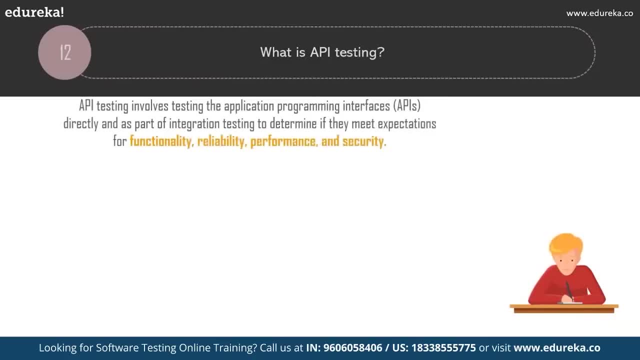 intermediary that allows two applications to talk to each other. So API testing is a type of software testing where APIs, or application programming interfaces, are tested to check if they meet expected functionality, reliability, performance and security. API testing is really needed to reveal bugs, inconsistencies and deviations from the 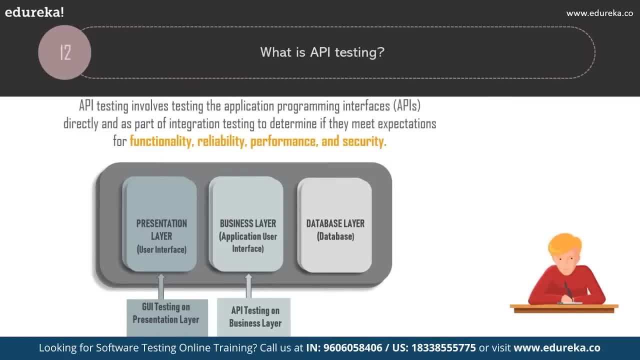 expected behavior of an API. Well, to be honest, API testing offers lot of advantages, like its language independent, first of all, and its graphical user interface independent. It offers improved test coverage, It reduces the testing cost, It enables faster releases, and all that On top of that, one more thing that 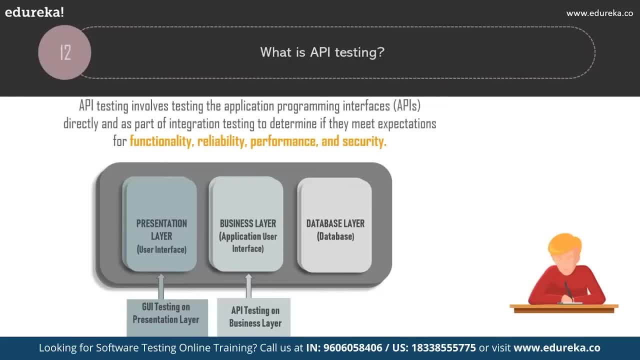 you should remember is basically: application is divided into three stages. You have presentation layer, then you have business layer and database layer. So API testing is usually performed in business layer. Let's move on to the next question. Let's see what that is. 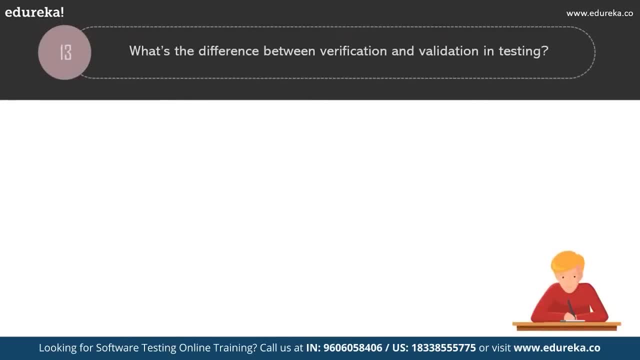 So what's the difference between verification and validation and manual testing? In software testing, verification is a means to confirm that the product development is taking place according to the specifications and using standard development procedures. It consists of different activities, like you have reviews, inspection, walkthroughs, demos and all. 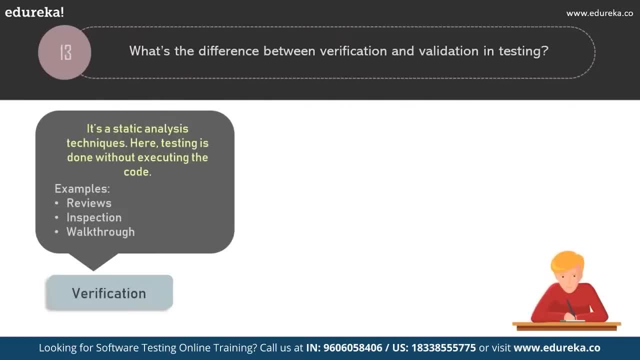 that. So, basically, you're confirming that the product development is taking place according to the requirements, specifications and using standard procedures. Now coming to validation: It's a means to confirm that the developed product doesn't have any bugs and it's working as expected. It consists: 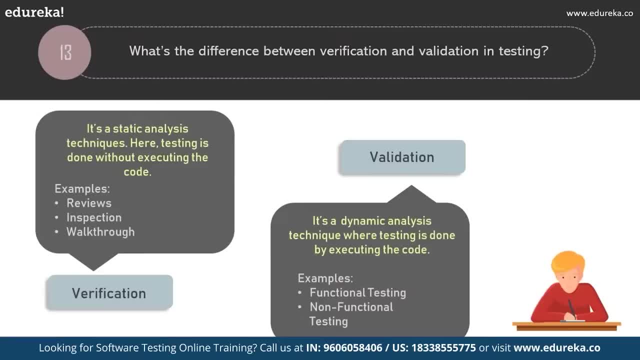 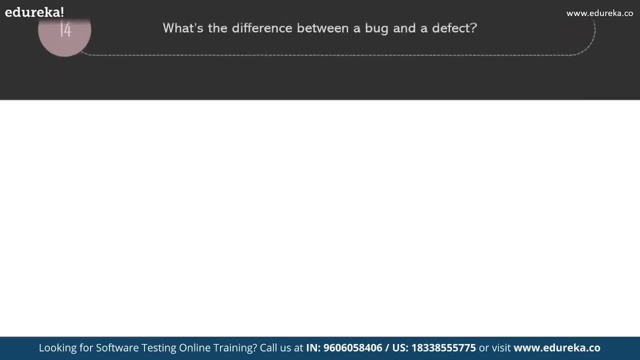 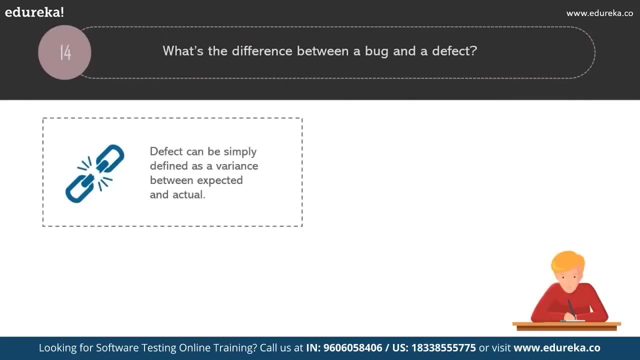 of activities like functional and non-functional testing techniques. So that's the difference between verification and validation. moving on to next question: What's the difference between a bug and a defect? So a defect is simply defined as a variance or difference between expected and actual result. 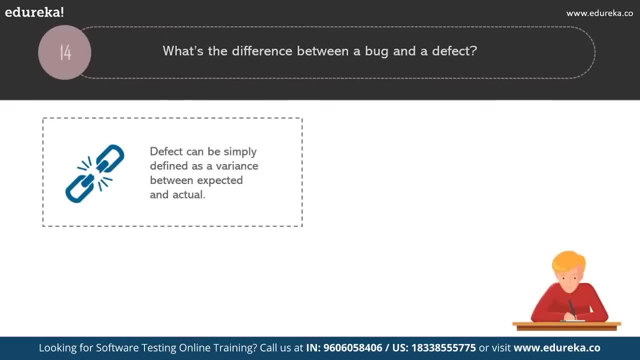 It's an error found after the application goes into production. It commonly refers to several troubles with software products, with its external behavior or with its internal feature. So the key point is: defect is an error which is found after the application goes into production. Coming back to bug, bug is a result. 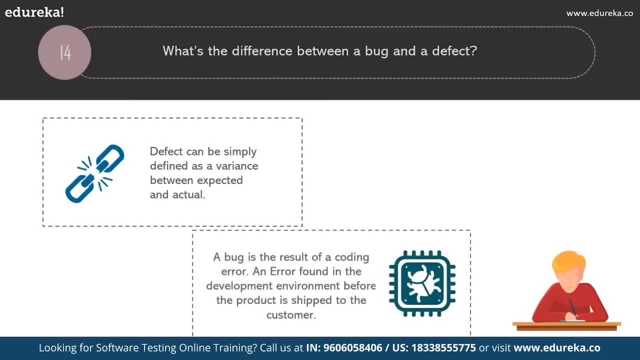 of a coding error, an error which is found in the development environment before the product is shipped to the customer. a programming error that causes a program to work poorly, produce incorrect results or crash the system. That's a park, or it can be an error in software or hardware that causes a 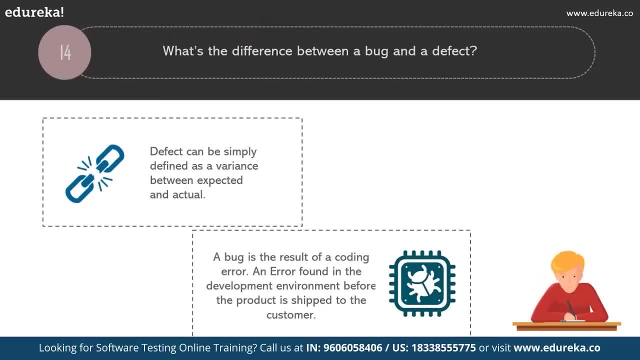 program to malfunction entirely. Bug is the terminology of a tester. Now you understand the difference. right, defect is an error in software or hardware that causes a program to malfunction entirely- The difference between expected and actual result. and it occurs after the application goes into production. 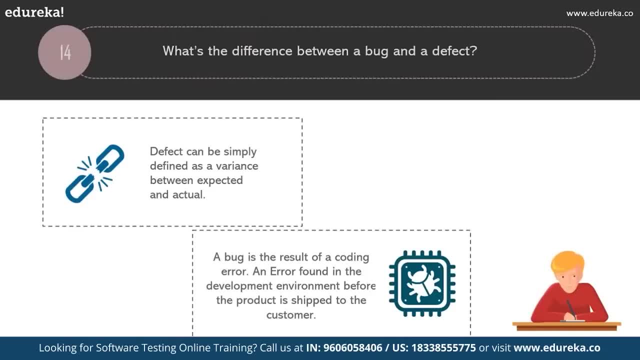 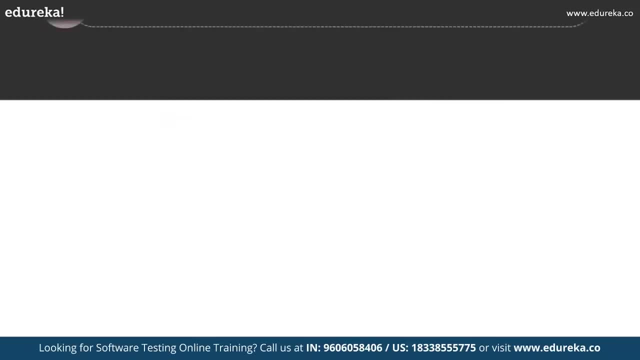 There is bug is result of a coding error. Like I said, it can be anything, So it's error that's developed before the product is shipped to the customer. moving on, the next question that we have is: what are advantages of manual testing? manual testing is lot of. 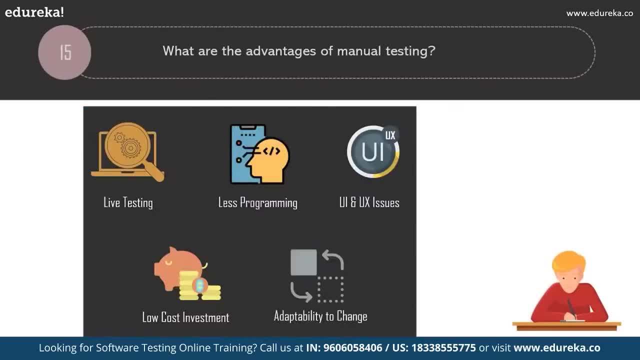 advantages to offer. First of all, you have life testing. So with manual testing, tester can test the application under similar condition, which means that the application, when your application goes live, So any bugs or glitches which occur when application is life, can be easily tracked with help of manual testing. 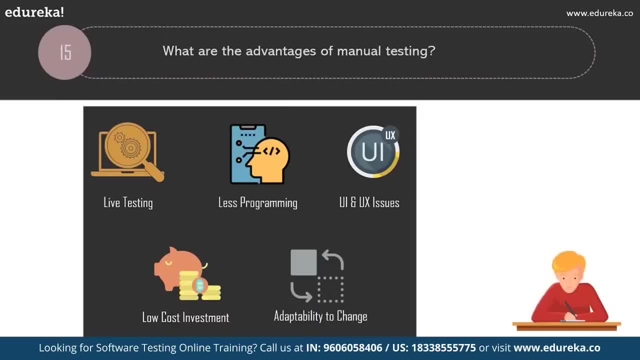 Secondly, in manual testing, less programming knowledge is required. basically, when you're testing on an application manually, your main focus is on understanding requirements, documenting the test cases and executing the test cases. Then there's this case of UI and UX issues when it comes to automation testing. 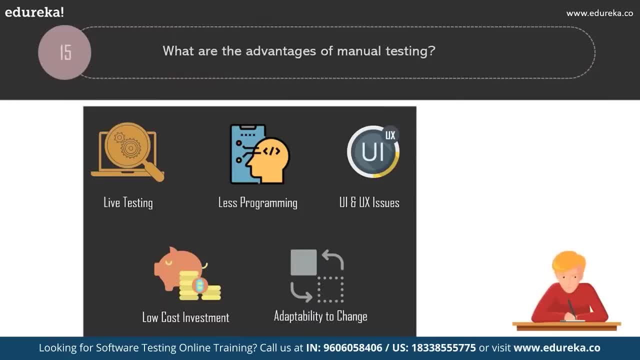 So, basically, automated tests are quite literally robotic. right, They fail to act as a real end-user would, but manual testing helps test you to identify any issues which are related to look and feel of the application. It also helps to find out the usability issues in the application. on top, 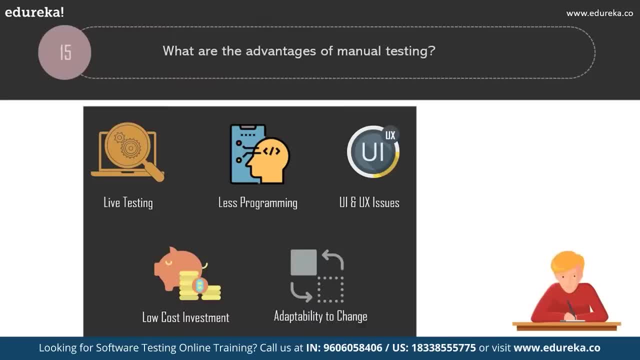 of all that manual testing requires really low investment, as it doesn't require any costly tools or highly skilled people to be hired. So what I meant to say is: initial investment in manual testing is very low and manual testing is cost effective for short-term projects. 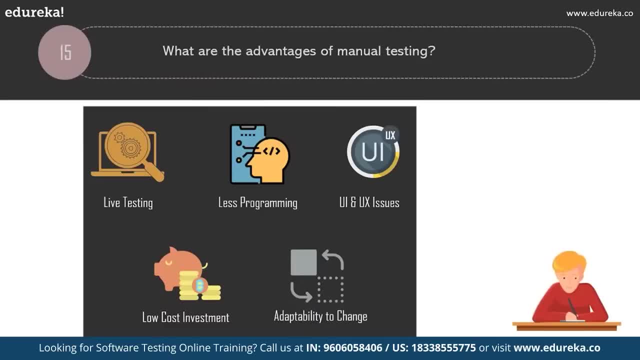 Lastly, in manual testing you can Swiftly test and see the outcomes, So it's well suited in cases when you're making lot of unplanned changes to your application and also your application needs to be tested immediately after implementing these changes. in such cases, 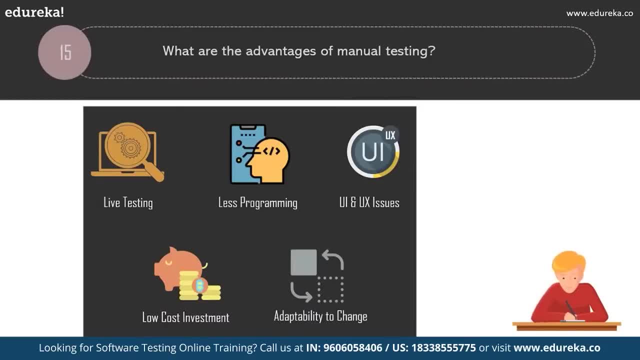 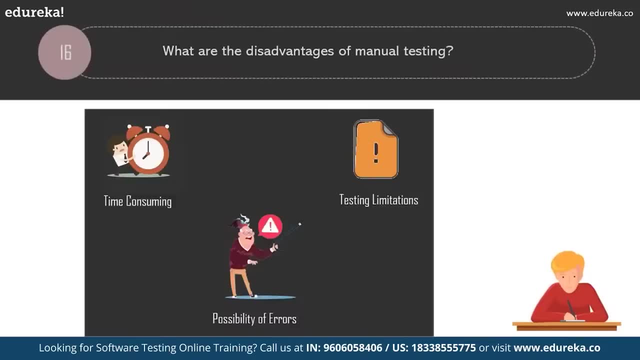 Manual testing is really effective. Let's move on to our next question, which is: what are disadvantages of manual testing? apart from the pros it offers, It has a lot of demerits as well. First of all, it's really time-consuming manual test. 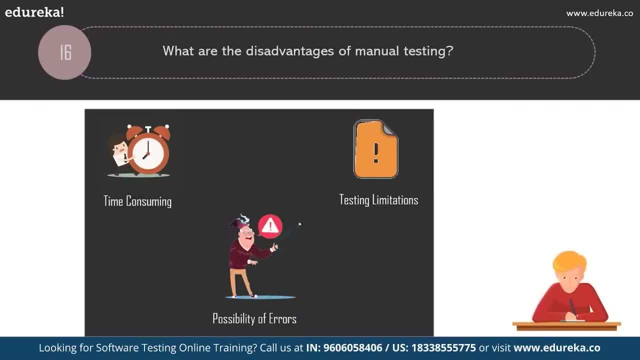 cannot be reused manually, Which means every time there's a change in your application, the tester need to run all the test cases again. Well, this is rather time-consuming activity, and that is why manual testing is really time-consuming. then you have like testing limitations. 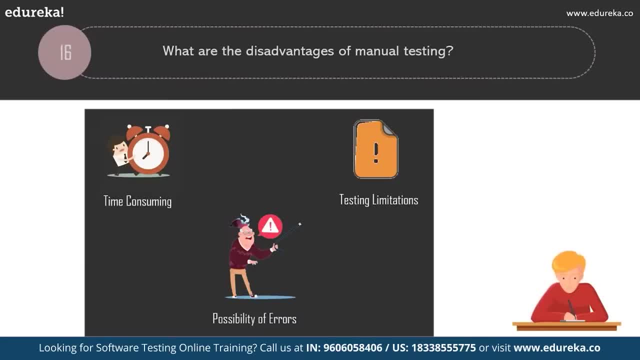 You can't go and apply manual testing. for performing load and performance testing, See, to check the performance of an application using manual testing, You require a lot of users and gadgets, which again increases the cost of the testing. So it's better to go for automation. 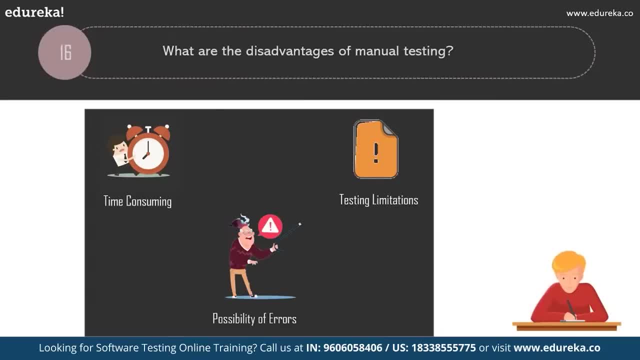 in that case- And obviously since manual testing is performed by humans, There's always this possibility of errors. The testing results will be as good as the tester performs the test. That's it. You can't guarantee the quality with a manual testing. 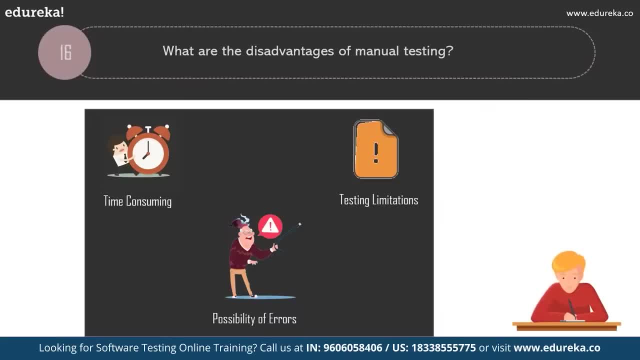 There are chances that the tester may miss out the same box on retesting the application. because it's being performed by human. There's always possibility of that human making an error. So yeah, these are certain disadvantages of manual testing. moving on the next question, 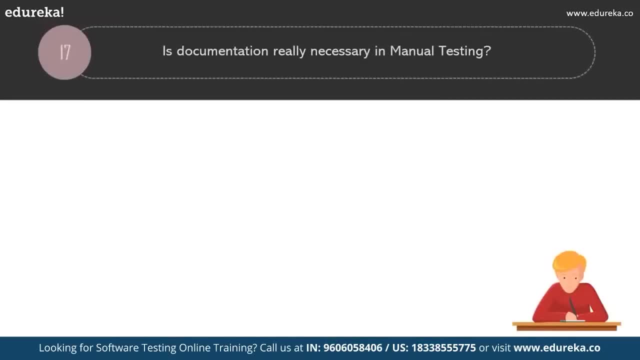 Is documentation really necessary in manual testing? Yes, documentation plays a critical role in achieving effective software testing. Well, details like your designs, business rules, requirements, specifications, inspection reports, configurations, code changes, test plans, bug reports, etc. All should be documented. documenting the test cases will facilitate you. 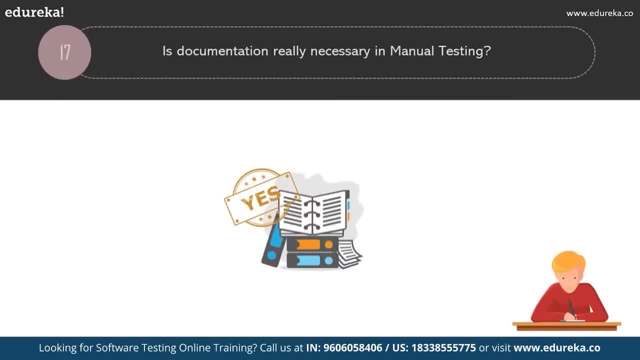 to estimate the testing efforts that you will need, along with your test coverage. It will help you to track and trace your requirements, as well as some commonly applied or used documentation. artifacts that are associated with manual testing are: we did discuss one earlier, which is test case after that. 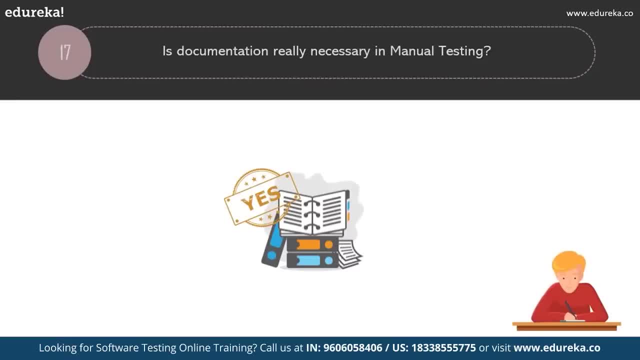 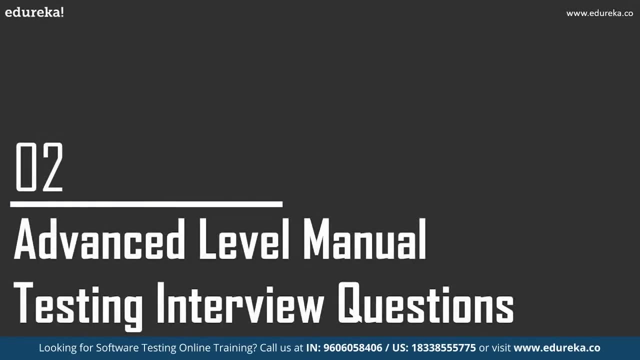 We have test plans to scenario, traceability, matrix and many more. Well, guys, with this we have completed the basic level questions, So let's move on to next level, which is advanced level manual testing interview questions. So let's see what's the first question and advanced level category. 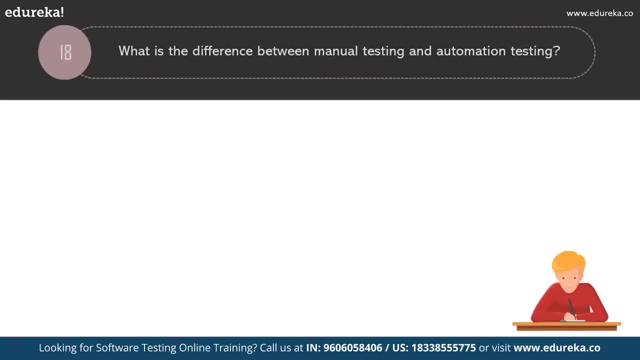 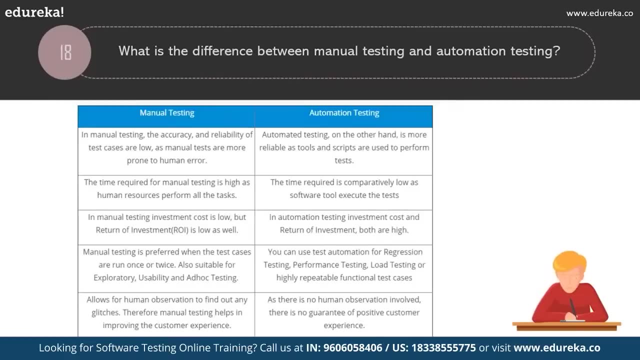 So what's the difference between manual testing? interview questions. so what's the difference between manual testing and automation testing? you guys all know the basic difference. while manual testing is literally performed by humans or human action, whereas automation testing is performed by human, but with the assistant of. 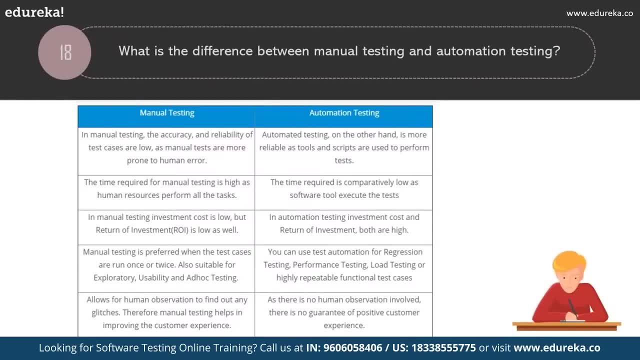 tools, scripts and other things. that being the main difference, Let's go ahead and discuss other differences as well. So manual testing, since it's performed by humans, the accuracy and the reliability of test cases are low, whereas automation testing, on other hand, is performed with test cases. 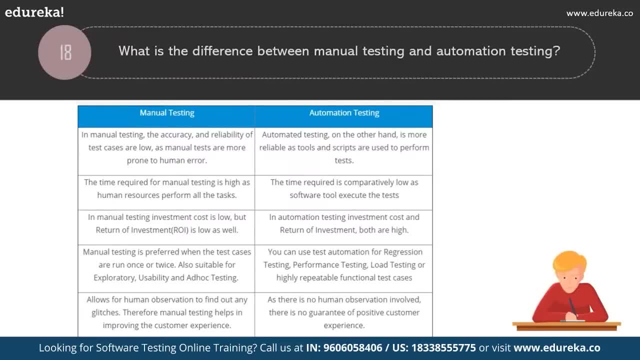 tools and scripts, the reliability and accuracy is literally high. the time required for manual testing is literally high as you and resource perform all the task, whereas time required for automation testing is comparatively low, as software tools execute the test cases. in manual testing, the initial investment which you make is low because you don't use 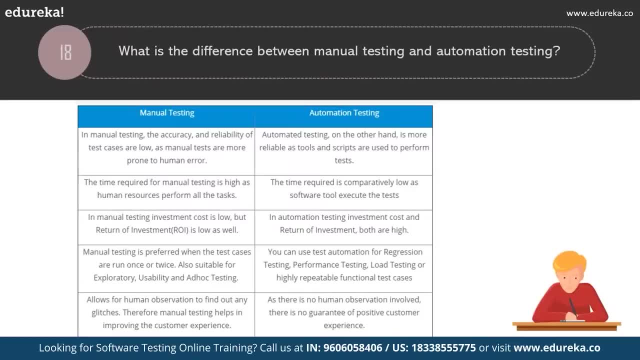 any kind of tools and all that here, but the written of investment is low as well. But as an automation testing, initial investment is literally high, but you written of Investments is also high. manual testing is performed when you have test cases that need to be learned only once or twice. also when you have 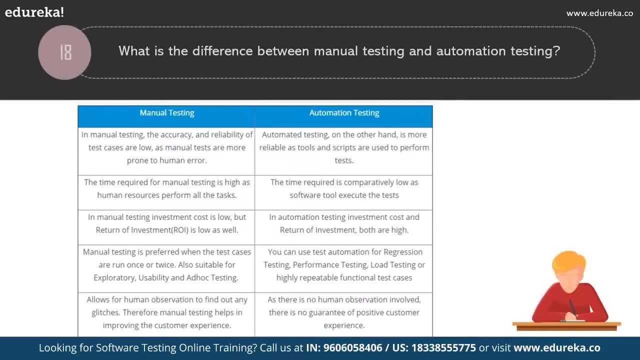 test cases suitable for exploratory testing, usability testing or ad-hoc testing. you can use automation for performing regression testing, performance testing, load testing or when you have cases that need to be tested multiple times. Now, one best thing about manual testing is that it Hallows for human observation. 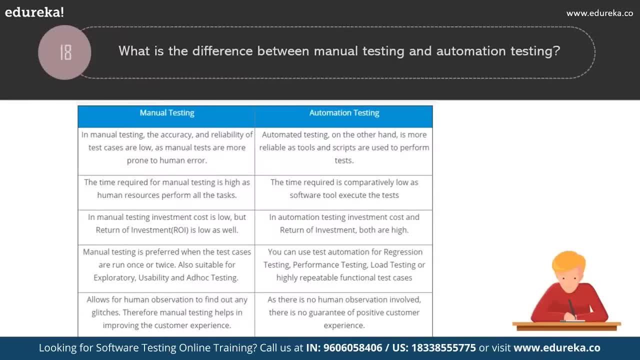 to find out if there are any glitches, and that's what automation testing is, why manual testing helps in improving the customer experience. when it comes to automation, testing is no human observation involved, and that is why it doesn't guarantee the positive customer experience that a manual testing. 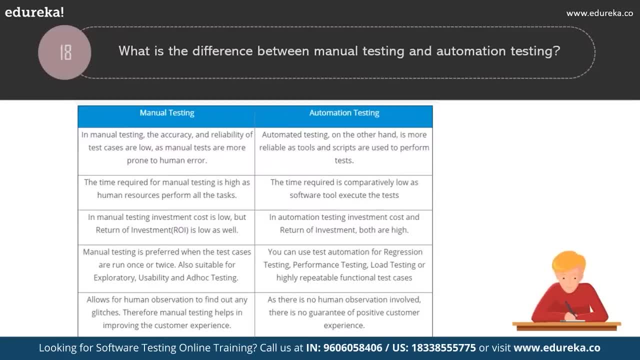 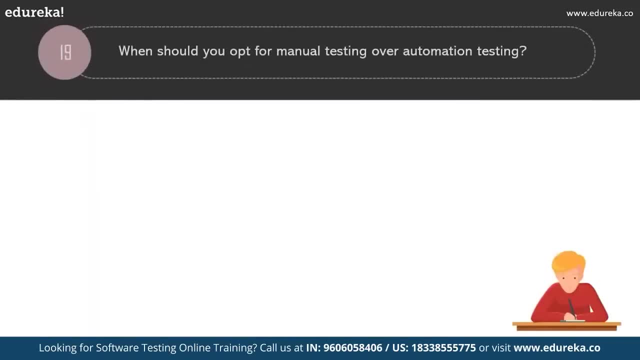 guarantees. So these are certain basic key differences between manual testing and automation testing. Now let's move on to our next question: When should you opt for manual testing over automation testing? There are certain key cases or scenarios when manual testing should be preferred. 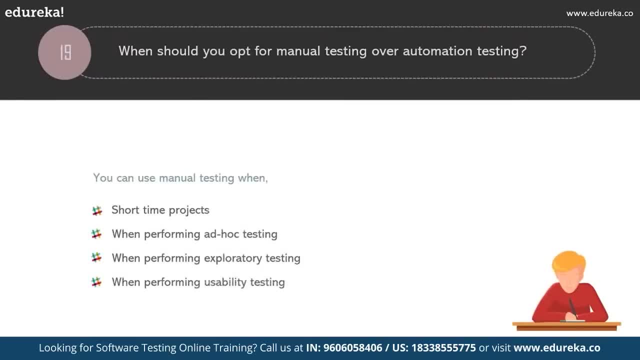 For example when you have a short time projects. automated test are aimed at saving time and resources, and yet they take a lot of time and resources to design and maintain them. For example, if you are building a small promotional website, it can be much more efficient to rely. 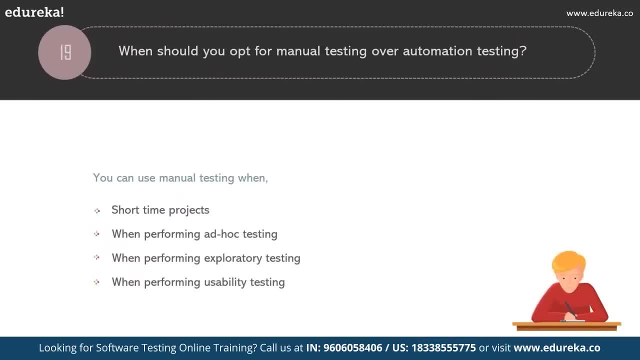 on manual testing rather than go ahead and create all those automated test cases. Well, it takes time, right. So in such cases, when you're working on small scale projects or projects which take small amount of time, you could go for manual testing also. 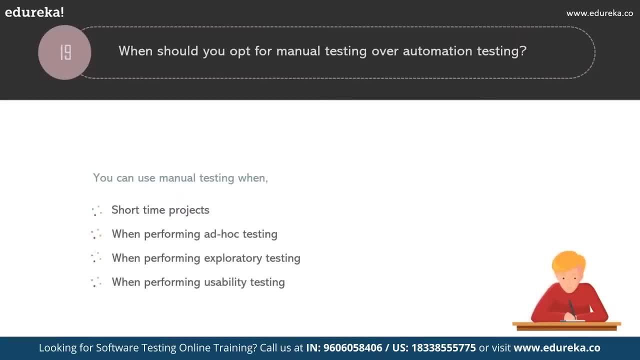 when you have ad-hoc testing. in ad-hoc testing There's no specific approach. as in, there's no fixed approach. It's a totally unplanned method of testing where the understanding and the insight of the tester is the only important factor. Well, again, manual testing sounds good. 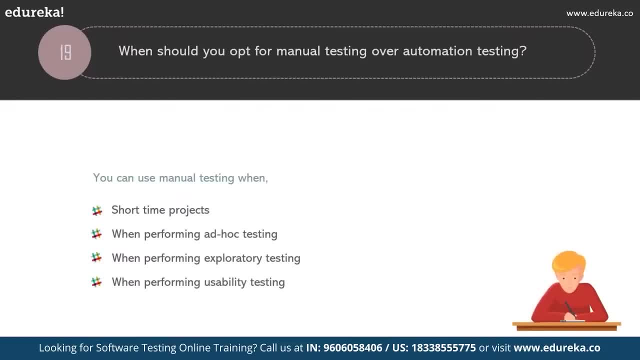 Then there's the case of exploratory testing. even then manual testing is preferred, because in exploratory testing it requires testers knowledge, experience, skills, analytical skills, creativity and mainly intuition. So human involvement is really important here. Lastly, you have usability testing. So when performing usability testing, 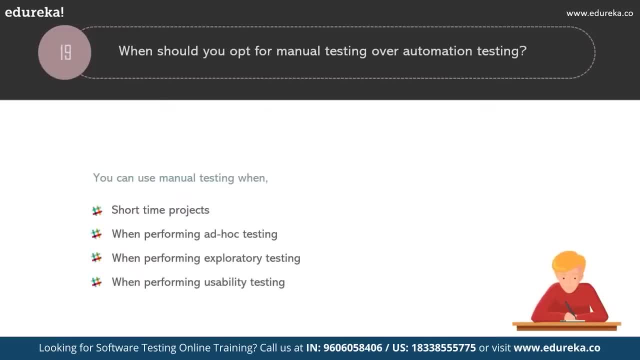 go ahead and use manual testing. So when performing usability testing, usually the tester needs to measure how user-friendly, efficient or convenient the software, the product is to end-user. So you should think in terms of end-user. for that again, manual testing is preferred. So these are certain scenarios. 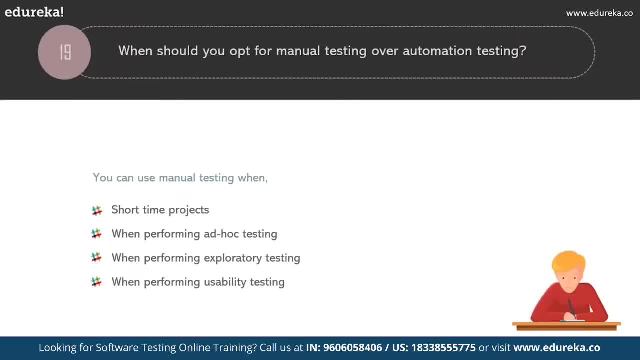 where you can prefer manual testing over automation testing. The next question that we have is: what are the features and cases involved in software testing life cycle? Well, it's quite simple. It begins with requirement analysis, where you figure out or categorize the user requirements. 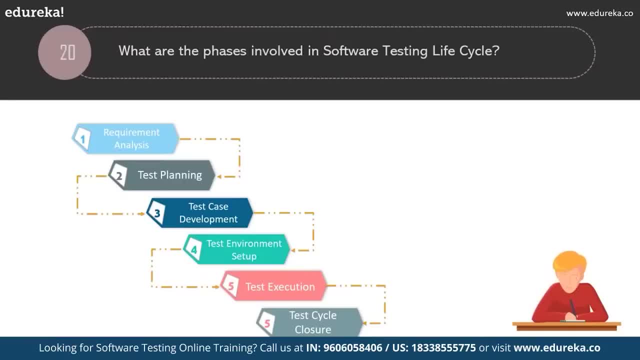 Next up. based on the requirements that you've gathered, you plan your entire test life cycle. Once you're sure as to what you're performing testing, on which type of testing you have to perform and all that, you start developing your test cases. then set up the entire test environment. 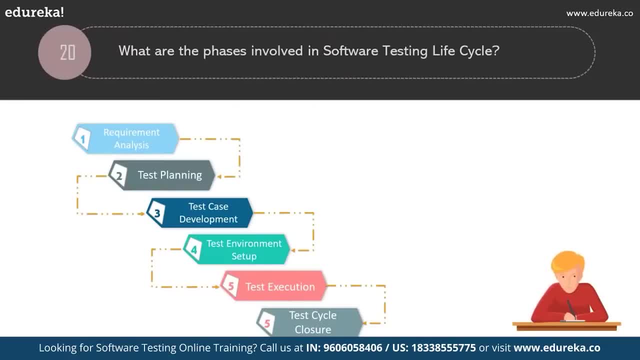 which will make your testing more effective after that, So that you can start your test execution and, lastly, you have test cycle closure. So let me repeat it again: You begin by analyzing the requirements put forth by the end-user, then you start planning your entire test cycle. 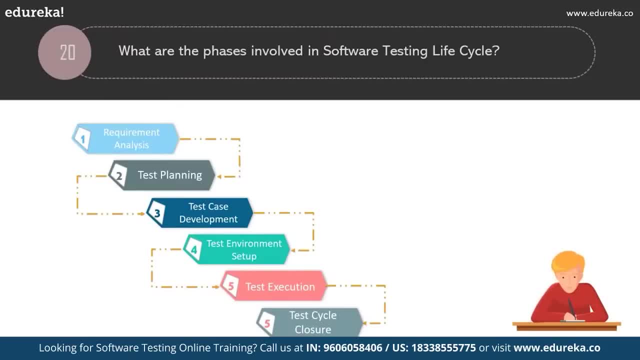 then you develop your test cases, categorize them, design your test environment. after that, Basically, you design and different kind of test that you want to perform, what you want to test on, and all that. then you execute the test cases that you've created And, lastly, then there's just cycle closure. 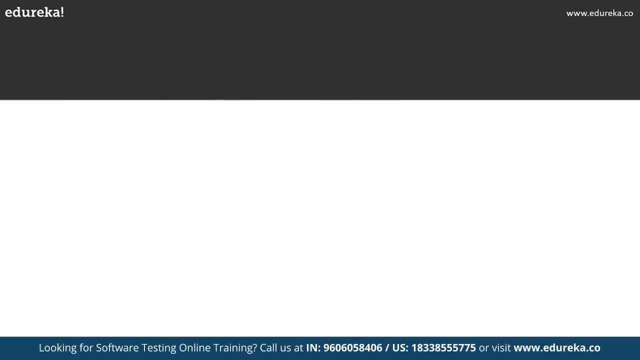 which indicates the end of your testing cycle. Next question that we have is a really interesting one: What's the difference between a bug or defect and an error? We did already discuss the difference between a bug and a defect. Let me go through it again. 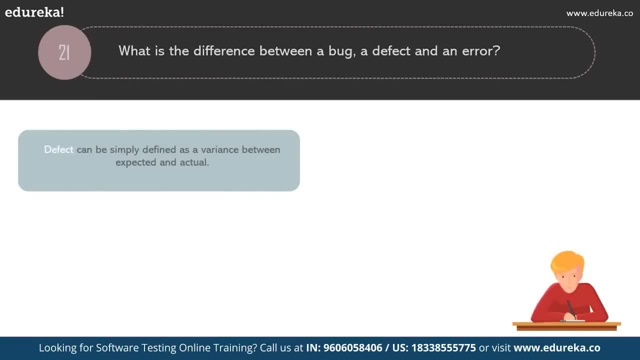 So defect is a variance or difference between expected results and actual results detected by the developer after the product goes live. So defect is an error which is found after the application goes into production and, simple terms, it refers to several troubles with the software product, with its external behavior. 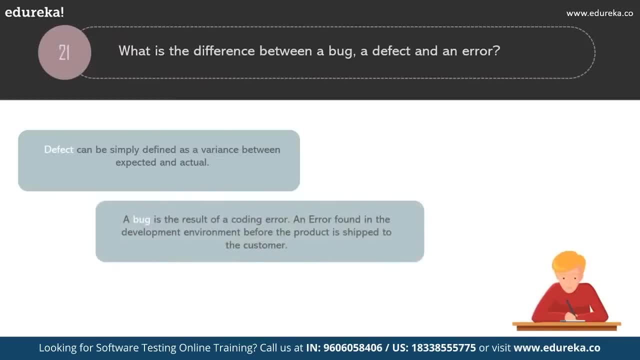 or with its internal features. Next up this bug? It's a fault in software that's detected during test time. They occur mainly because of some coding error, which might lead to the entire malfunctioning of a program. They may also lead to a functional issue in the product. 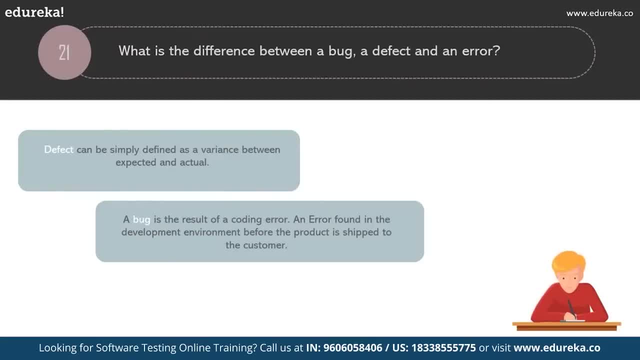 So basically, bugs are fatal errors that could block a functionality or result in a crash or cause performance bottleneck. Now what exactly is error? Error is a mistake, misunderstanding or misconception on part of software developer. So when I say software developer, it includes software engineers, programmers. 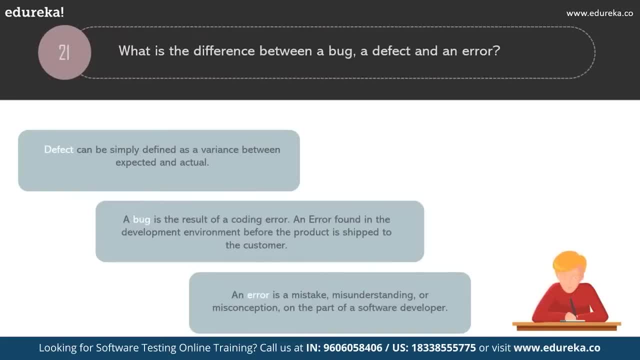 analysts, testers, whoever is in contact with the software. So, for example, a developer may misunderstand a design notation or a programmer might just type a wrong variable name, which might lead to an error. Error normally arises in software and it leads to change the functionality of the program. 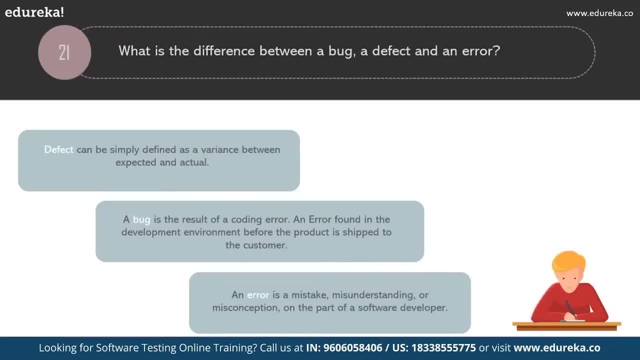 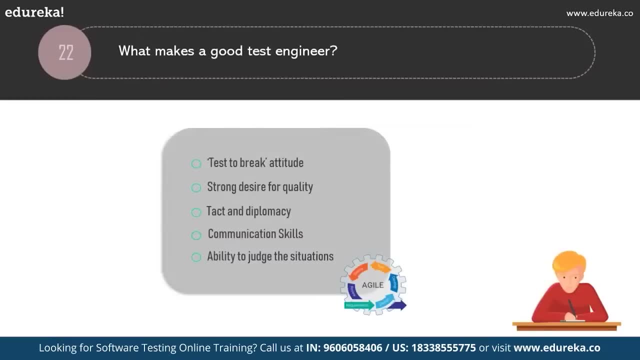 So that's the difference between a bug or defect and an error. Moving on to the next question: What really makes a good test engineer? First of all, a good engineer should have a test to break attitude, That's an ability to take the point of view of a customer. 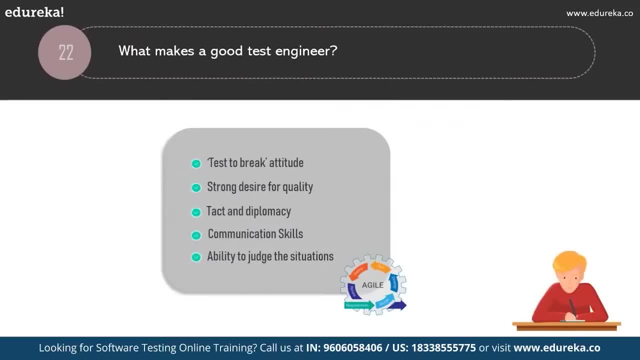 You should have a strong desire for quality and keen attention to detail. Also, tact and diplomacy are also needed, which is to maintain a cooperative relation with rest of the developers that is involved to it, And obviously you should have an ability to communicate with both technical people, non-technical people as well. 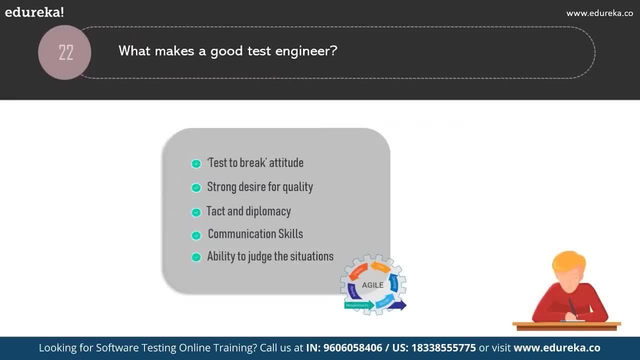 So you should have excellent communication skills And you should have ability to judge the situations and make important decisions, to test high-risk areas of an application when the time is actually very limited. Along with all this, it's always best to have an experience in software development or testing field. 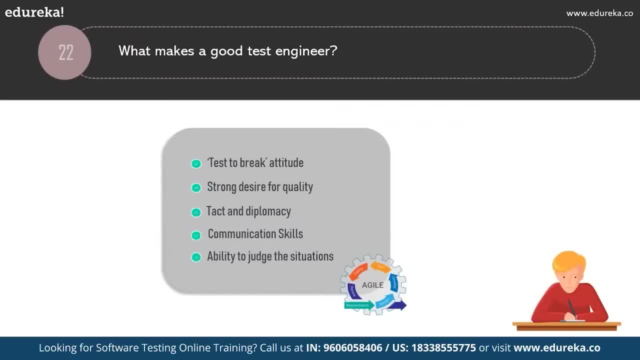 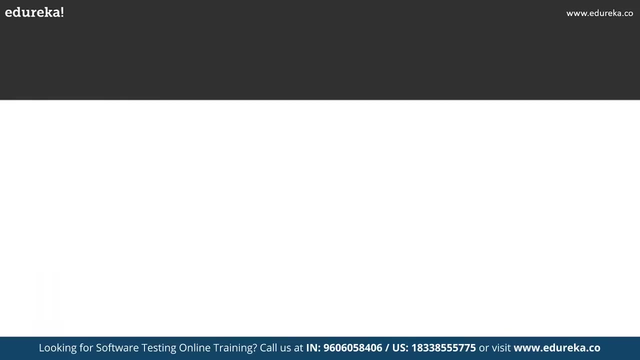 because previous experience can be helpful, as it provides a deeper understanding of software development process and it gives the testers an appreciation for the developer's point of view. So these are certain qualities that you look for when you're hiring a good test engineer. Moving on to our next question, 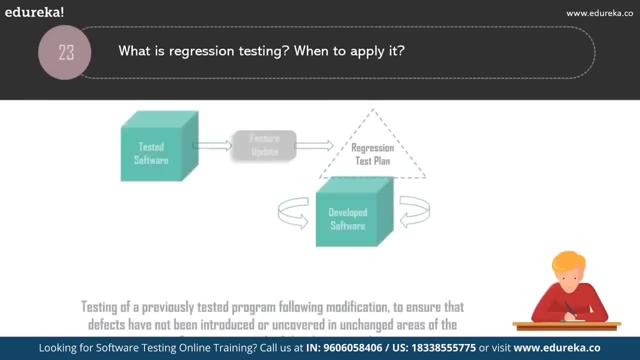 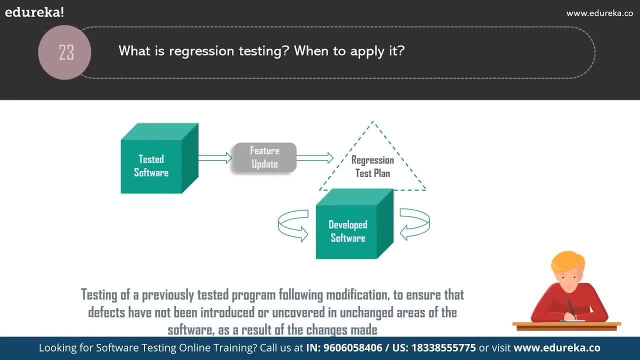 what is regression testing and when to apply it? A regression test is basically a system-wide test whose main purpose is to ensure that small change in one part of the system doesn't break the existing functionality elsewhere in the system. So if you consider regression testing, 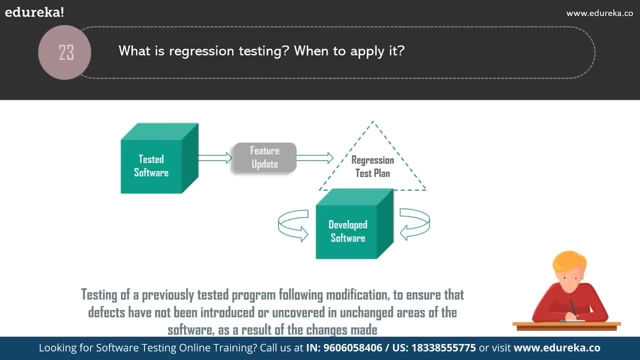 as an unintended change, then this type of testing is the process of hunting for those changes. So, in simple terms, it's all about making sure that your old box doesn't come back to haunt you. Let's take a look at fixitious example. 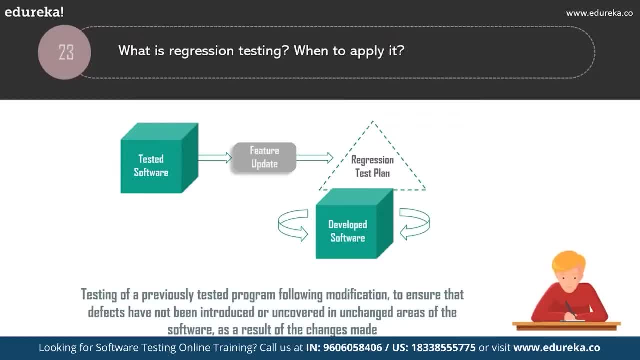 that illustrates the concept. So when adding a new payment type to shopping website, you have to rerun the old test to ensure that new code hasn't created any new defects or it hasn't introduced or reintroduced any old ones. So regression testing is really important. 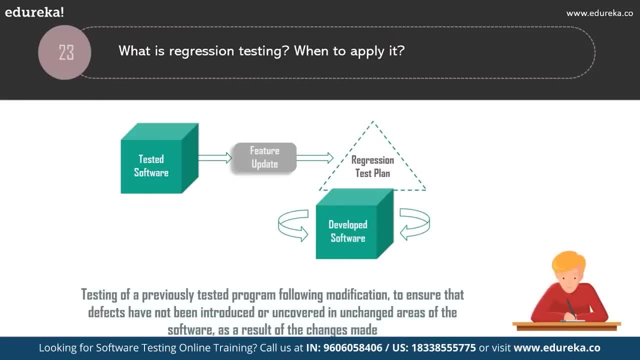 because without it, it's quite possible to introduce intended fixes into system that create more problems that they can actually solve. So regression testing. so how do you actually apply regression testing? It's quite simple: You have tested software, but you'll have to add a new feature. 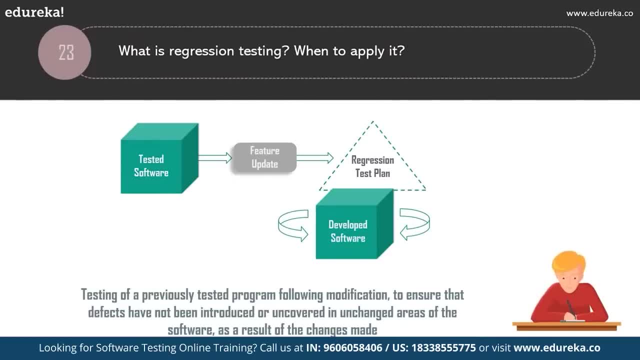 So a feature has been updated. Now you want to check if the new feature is affected or brought out any old bugs, or if it has introduced any new bugs. for that you perform regression testing. All you have to do is create a regression test plan, just like how you perform. 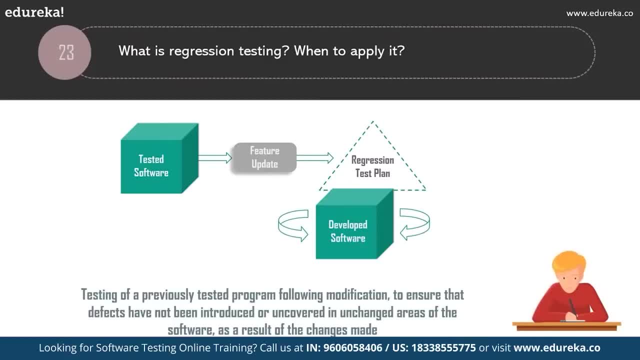 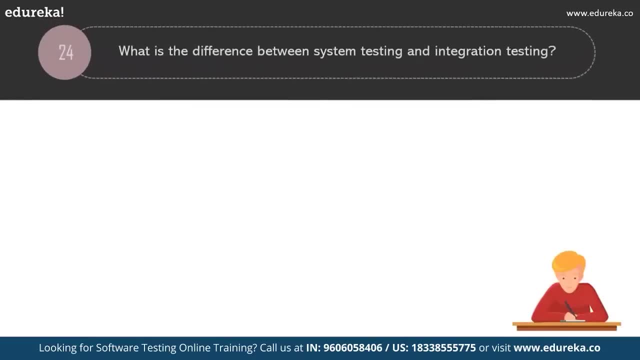 the entire software testing lifecycle. You carry that and you'll have newly tested software with updated feature. Well, that's regression testing. The next question That we have is: what's the difference between system testing and integration testing? It's quite simple: system testing. 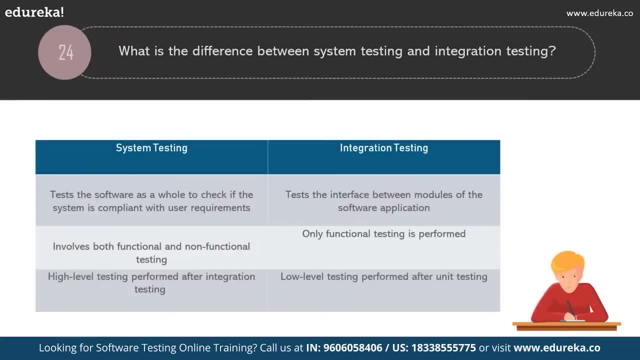 It tests the entire software application to see if the system is compliant with user requirements and stakeholders requirements. but integration testing: it test interface between the modules or units of software application system testing. It involves both functional and non-functional testing like sanity, usability testing, performance testing, load testing. 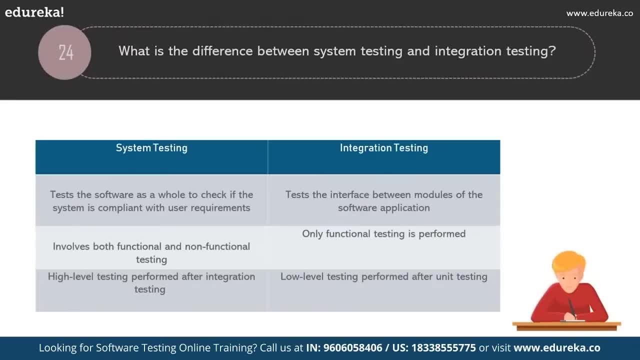 and all that, whereas only functional testing is performed in integration testing. It is performed in integration level or integration testing to check if two modules, when combined, give the right outcome, or if they are able to communicate properly through the interface or not. Well, system testing is a high-level testing. 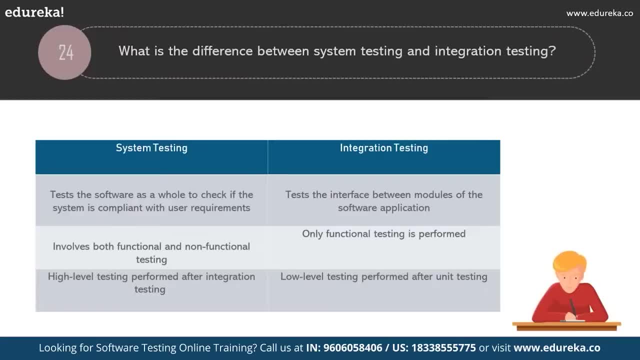 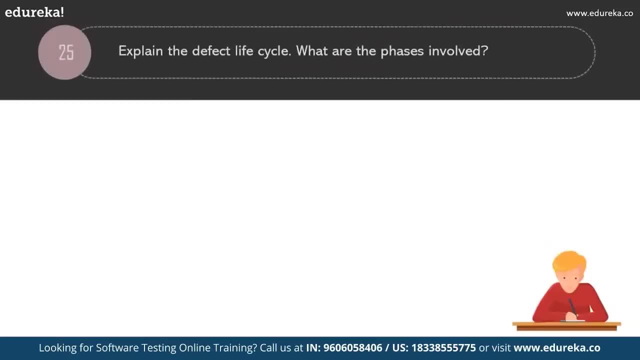 which is performed after integration testing, Whereas integration testing is a low-level testing which is performed after unit testing. The next question that we have is explain the defect lifecycle. What are the different phases involved? So you guys already know what bug is. We already discussed this many times. 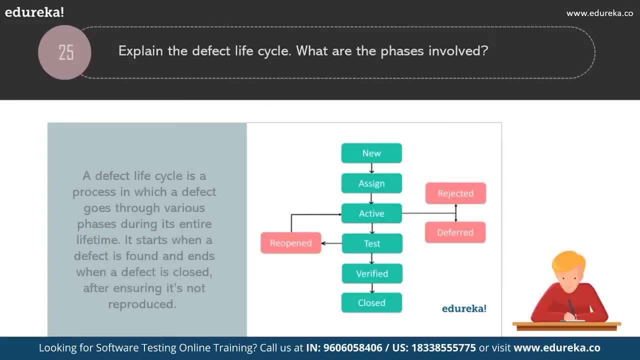 a work is actually an error that could have been introduced in the due course of software development life cycles. due to multiple reasons, The common sources of bugs are: it can be ambiguous requirements, programming errors, unachievable deadlines and much more. every reported bug actually follows a life cycle till its closure: a bug life cycle. 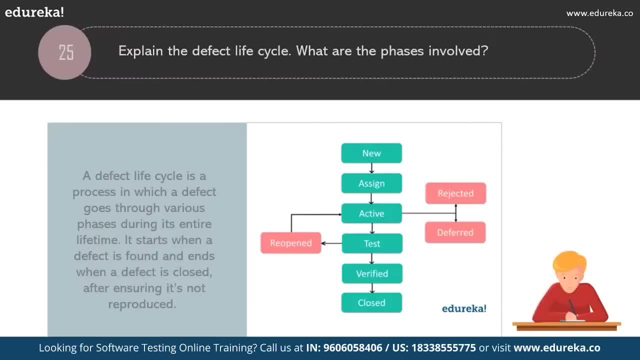 basically illustrates the journey of a bug from the time it is reported to the time it's fixed and closed. So let's quickly go through the steps that are involved in defect life cycle or bug life cycle. First, if we have something called new state, 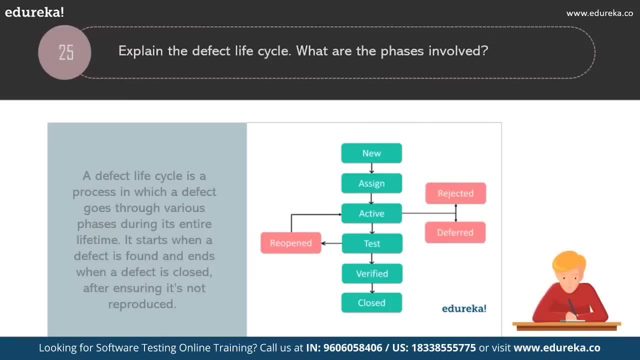 Well, in this step, if a defect is locked and it's posted for first time, its state is given as new. then you have assigned state. So after the tester is posted the bug, the lead of the testing team approves that the bug is genuine and he assigns the bug to corresponding developer. 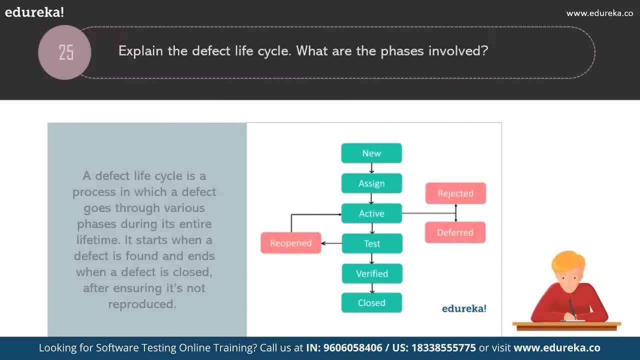 and the developing team to solve it. Then it's said to be in assigned state. After that you have two other status which says open and fixed. So in open state developer actually start analyzing the bug and start fixing it Once he's sure that is fixed, the defect. 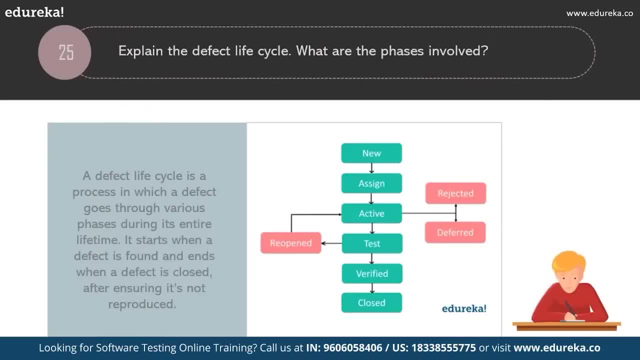 he changes the state of the bug to fixed Next up. we have test date, So at this stage tester does the testing of change code which the developer has given back to him. So basically here the tester is checking if the bug which he has assigned to developer. 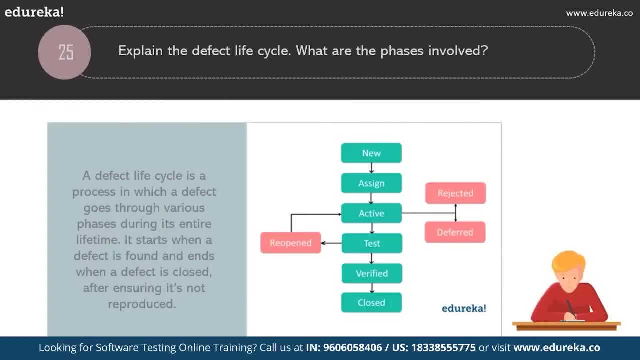 has been fixed or not. So once he is verified he changes the status of the bug to verified. Now, in case of the bug still exists, even after the bug is being fixed by the developer, the tester might decide to reconsider the bug. in such state it goes to reopen state. 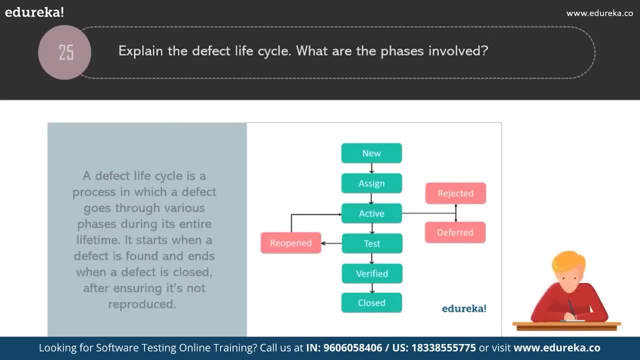 Now if the tester thinks that bug is fixed, he marks the status as closed. There's another state called duplicate in the bug-like cycle. if bug is repeated twice or there are two bugs which deal with the same concept, then one bug status is changed to duplicate. 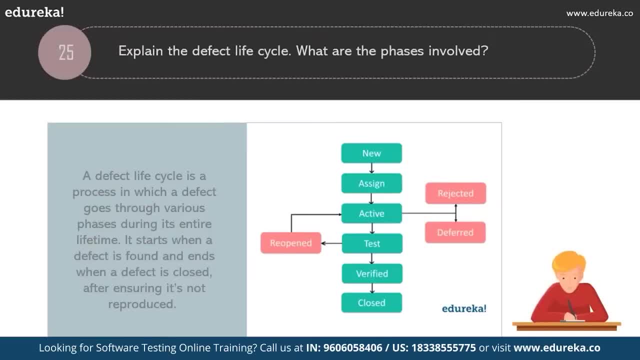 After that you have rejected and deferred. Rejected is: if the developer feels that bug is not genuine, he rejects the bug and the status of the bug is changed to reject Deferred. if the bug is changed to defer state, it means that bug is expected to be fixed. 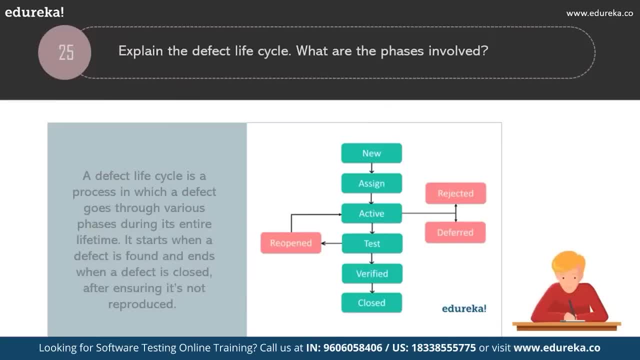 in next few releases. It's quite simple. If you have any queries in this defect lifecycle, you can actually go ahead and refer to software testing tutorial by Edureka. The entire lifecycle is explained in detail, So I expect this concept is much more clear. 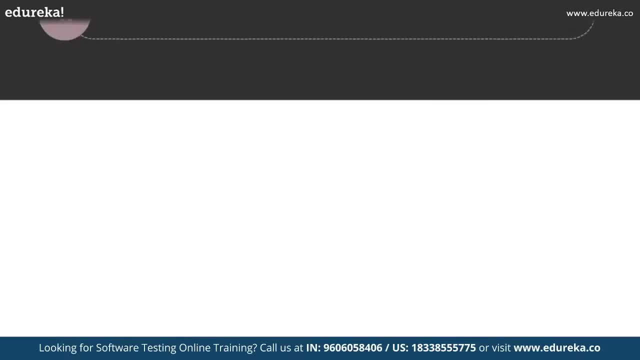 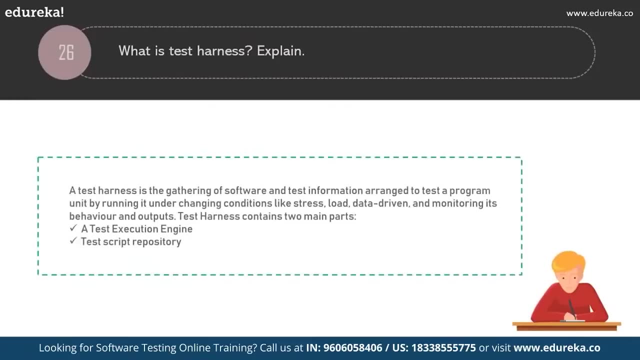 for you guys. now Let's move on to next question. What is a test harness in testing? Explain In software testing? a test harness, or automated test framework, is a collection of software and test data configured to test a program unit by running it under multiple conditions. 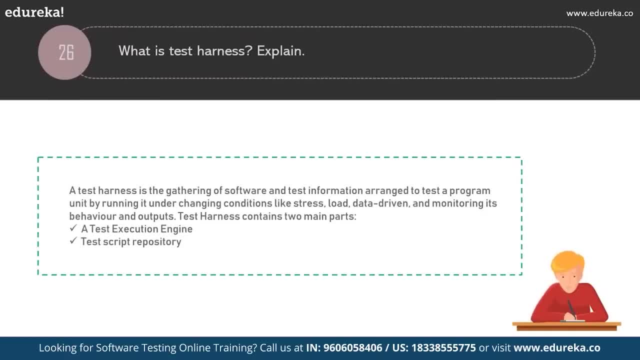 and monitoring its behavior and output for all these conditions. So basically, it's a collection of software and test data configured to test a program under multiple conditions by monitoring its behavior and its output. Test harness has two important parts: test execution engine and test script repository. 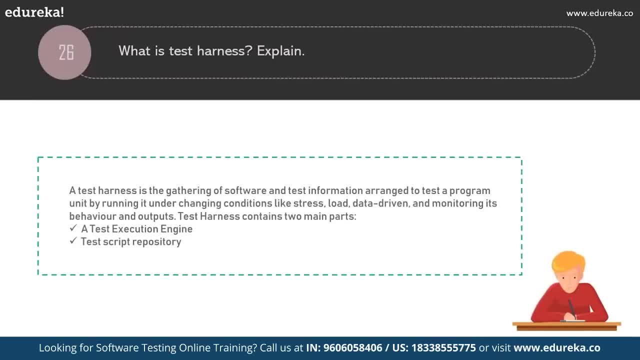 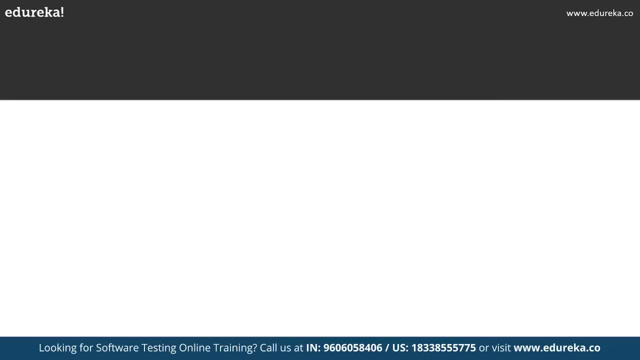 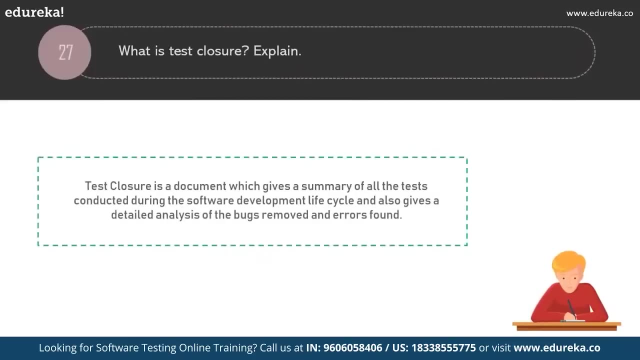 A test harness should allow specific test to be run, It should orchestrate a runtime environment and it should also provide a capability to analyze the results. Moving on to our next question, What is test closure? Well, test closure is a document which gives a summary of all the tests. 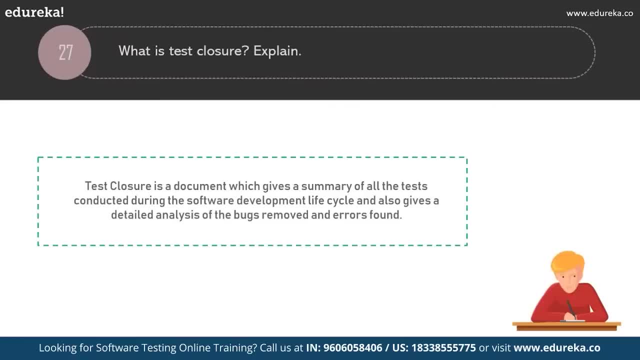 which are conducted during the software development lifecycle, and it also gives a detailed analysis of bugs removed and their as far. So this document, or memo, actually contains the total number of experiments, total number of experiments executed, total number of imperfections found and total number of imperfections settled. 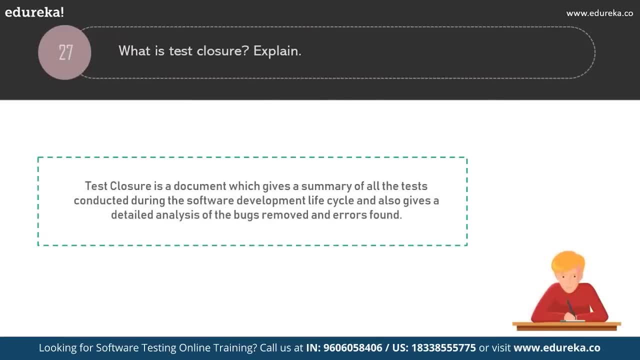 total number of bucks or imperfections not settled, total number of bucks rejected, total number of bucks differed, and so forth. So, in simple terms, test closure as a document which has like summary of all the tests that are conducted during entire software development and testing life cycle. 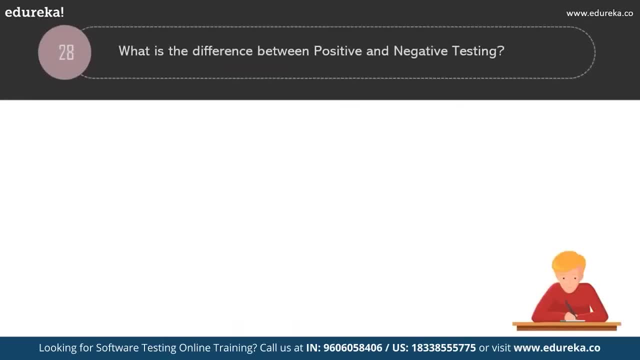 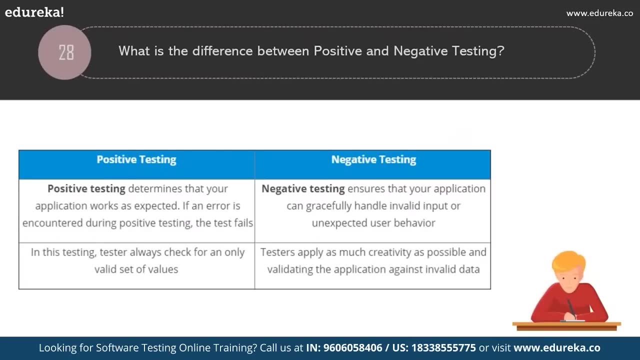 Next question that we have is very basic question: What's the difference between positive and negative testing and manual testing? So positive testing means actually testing the application or system by giving valid data, whereas negative testing means testing application or system by giving invalid data. So positive testing it determines. 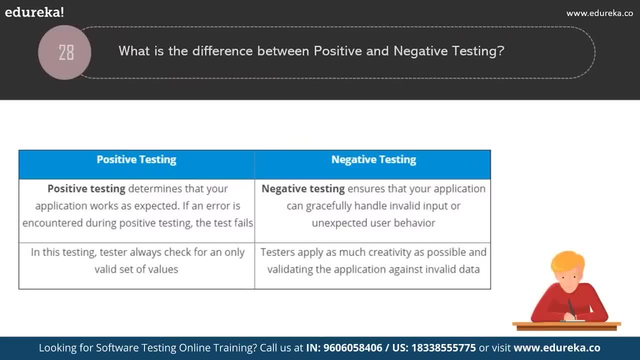 that your application is working as expected, whereas negative testing it ensures that your application can run gracefully and it can handle invalid input and unexpected user behavior in a very proper manner. Positive testing is always done to verify a known set of test conditions, whereas negative testing is always done. 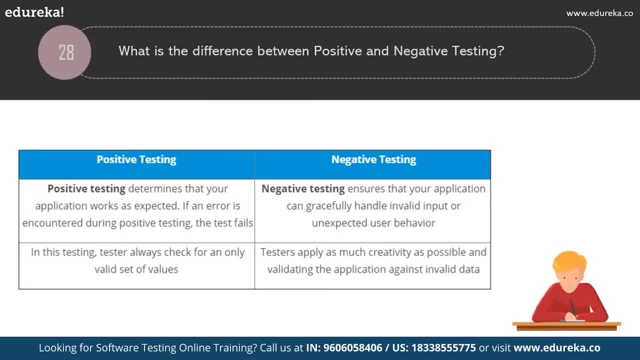 to break the project and the product with unknown set of test conditions. Positive testing checks how the product and the project behave by providing the valid set of data, whereas negative testing checks how the application will actually perform if we provide the invalid output. Will it actually deal with it? 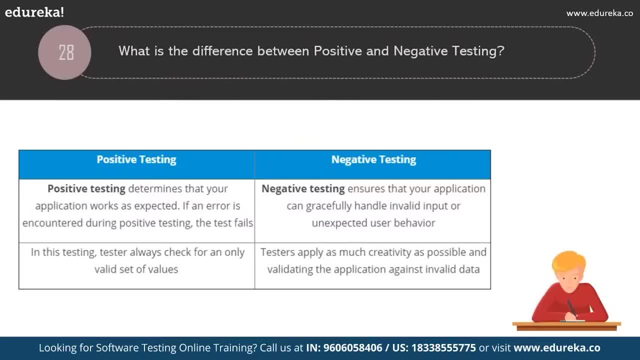 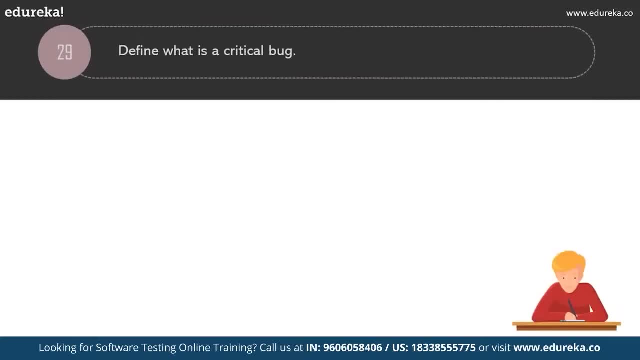 or give the wrong output, or what would be the result? That's negative testing. So that's the basic difference between positive and negative testing. So next question that we have is define what's critical bug. Well, a critical bug is a bug that's got tendency. 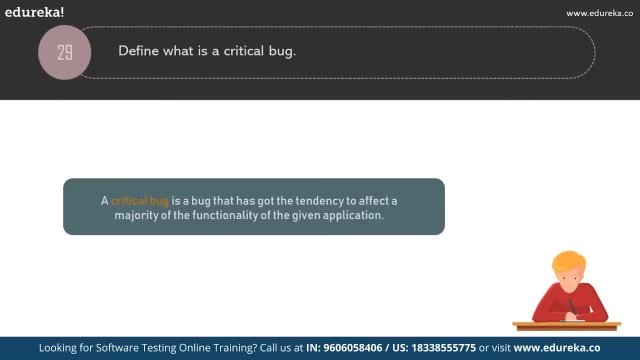 to affect majority of functionality of a given application. It means that a large piece of functionality or a major system component is completely broken and there's no way to work around it. Application cannot be distributed to end-client users If the critical bug has not been issued. remember that. 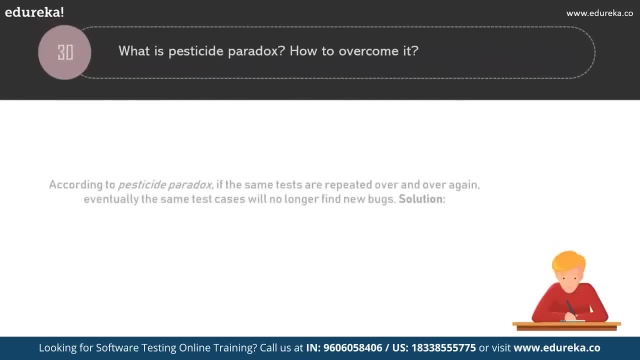 Moving on to our next question: What is pesticide paradox and how do you overcome it? If same test cases are repeatedly run over and over again, eventually they will no longer will help you find new bugs, and this concept is called pesticide paradox in testing. After certain number of iterations of testing, 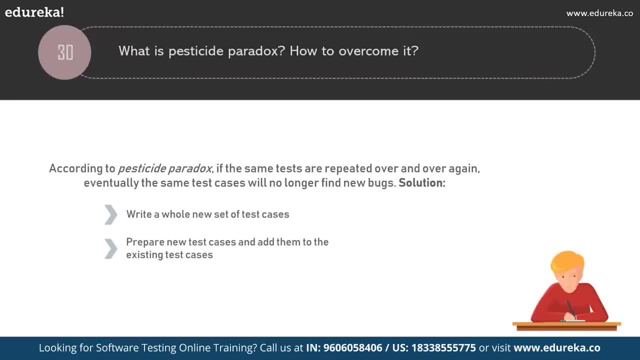 as the testing improves, the defect number actually starts dropping and most of the bugs will actually be fixed. So developers will be extra careful in only those places where testers found more defects, and they might not look in the other areas. This is what you call pesticide paradox. 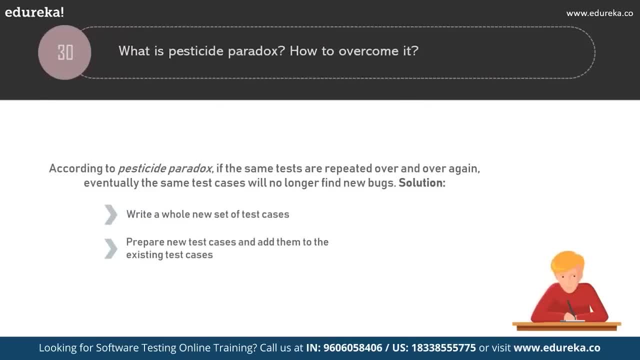 So how do you actually go ahead and overcome this pesticide paradox? Do you have any solutions? Well, yes, you can go ahead and write whole new set of test cases to exercise different parts of the software, and you can prepare new test cases and add them to your existing test cases. 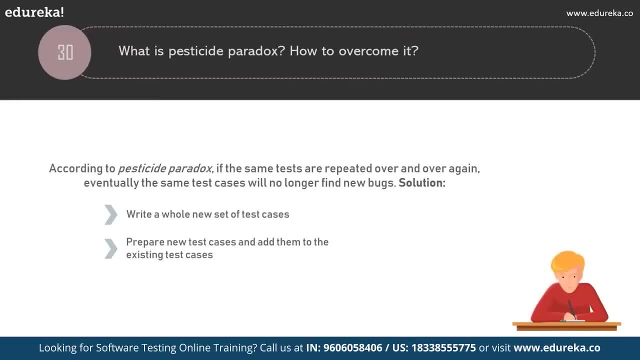 So by following above two methods of prevention, it's possible to find more potential defects in the area where you might have actually missed previously or where you might have neglected before. So that's what pesticide paradox is and how you overcome it. Moving on to the next question, 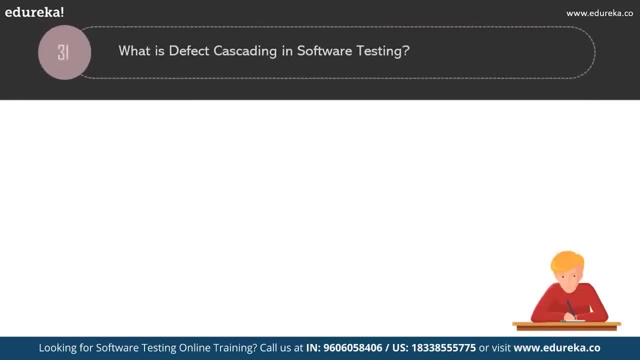 What is defect cascading in software testing? So defect cascading is process of triggering other defects in application. Simple, right, It's just triggering other defects in application. When a defect goes unnoticed while testing, it invokes other defects. Well, as a result, 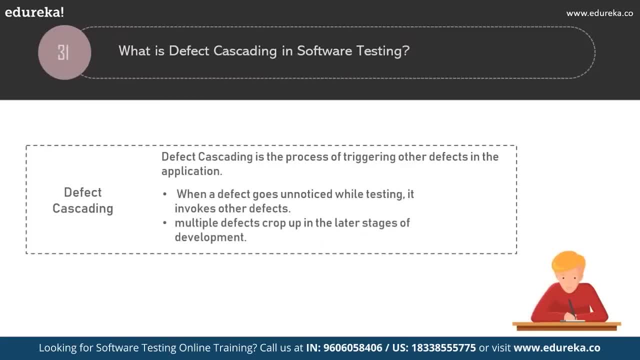 multiple defects crop up in later stages of development. If defect cascading continues to affect other features in your application, identifying the affected- actually affected- feature becomes very challenging. You might actually go ahead and take different test cases to solve this issue, even when it's difficult and time-consuming. 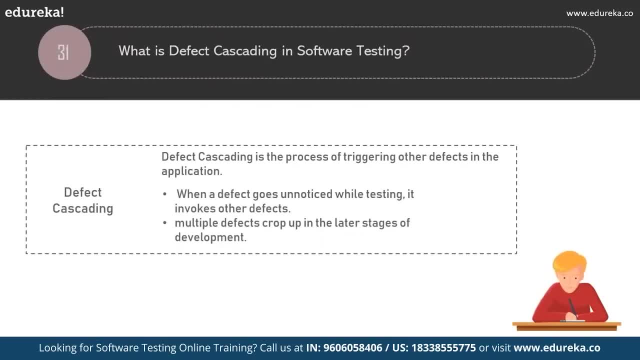 Let me give you a simple example to understand the concept. So an application is being deployed to calculate a monthly salary of the employees. The module which is responsible for calculating salaries is having an unidentified defect. As a result, it's wrongly calculating the salary. 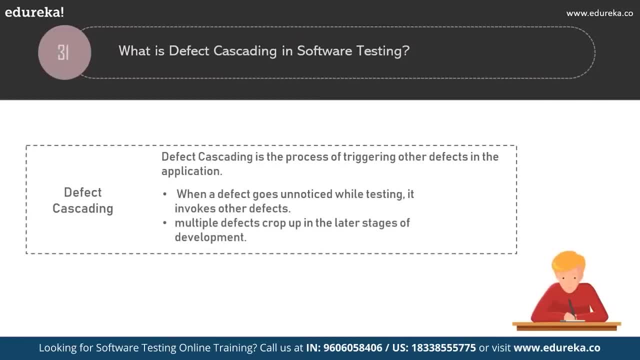 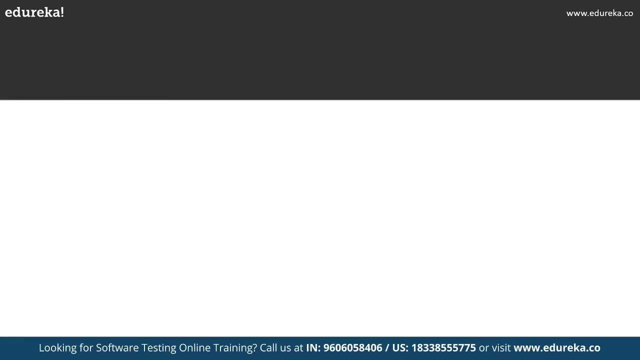 This prompts the database to transmit incorrect salary numbers, which are further reflected in your balance sheet tax calculations and wherever the salary part is used. So one defect is triggering other defects in application. That's what defect cascading is. Let's move on to our next question. 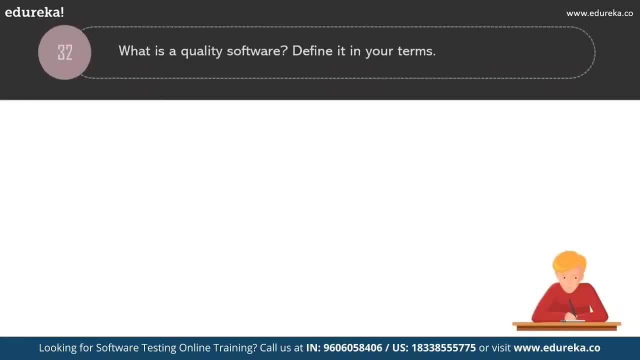 which is what do you actually mean when you say a quality software. So, in general, quality software is reasonably bug-free, It's delivered on time and within budget, It meets the given requirements or expectations and it's highly maintainable. But again, 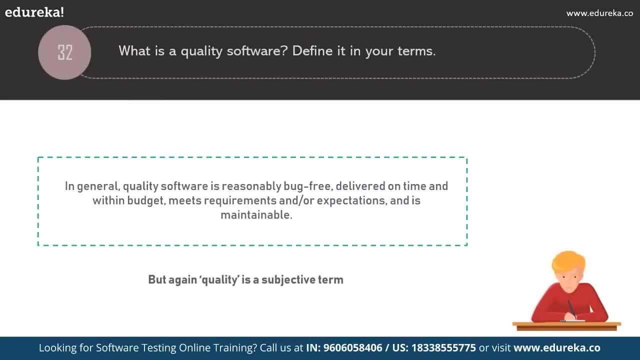 quality is always a subjective term. It will depend on who the customer is and their overall influence. in the schema of your testing, For example, each type of customer will have their own slant for quality. The accounting department might define quality in terms of profit. 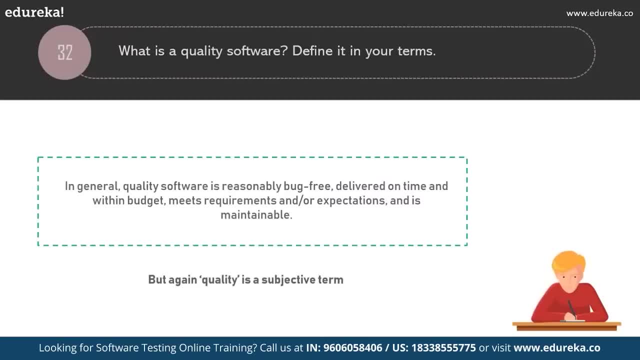 whereas if you ask a general end user, he might define quality as user-friendly, safe and bug-free. So, again, quality is a subjective term. The next question that we have is: what is black box testing and what are various techniques that come under black box testing? 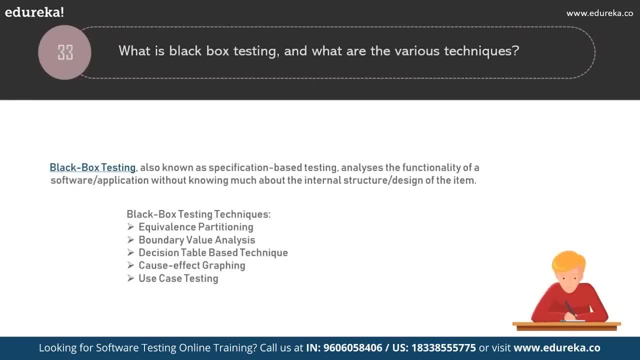 So black box testing is also known as specification-based testing. It analyzes the functionality of the application without knowing much about the internal structure or design of the application that's being tested. So what's the purpose of black box testing? Well, it's to check the functionality. 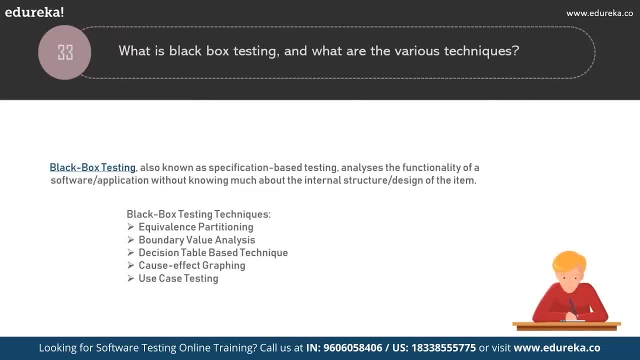 of the system as a whole to make sure that it works correctly and it's meeting the user demands. You have various techniques that pop up under black box testing, like you have equivalence partitioning, use case testing, cause-effect graphing and many others. 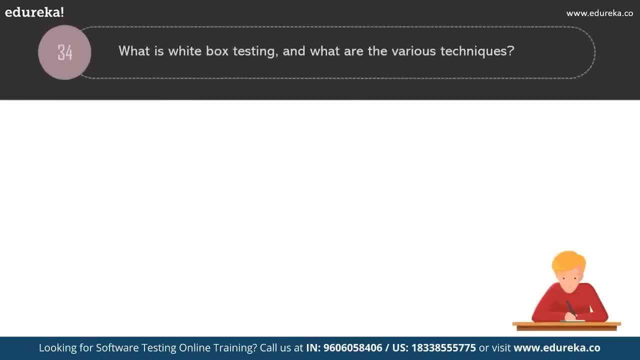 The next question is also somewhat similar to that. What is white box testing and what are various techniques? White box testing is also known as structure-based testing. It requires a profound knowledge of code, as it includes testing of some internal structures a part of application. 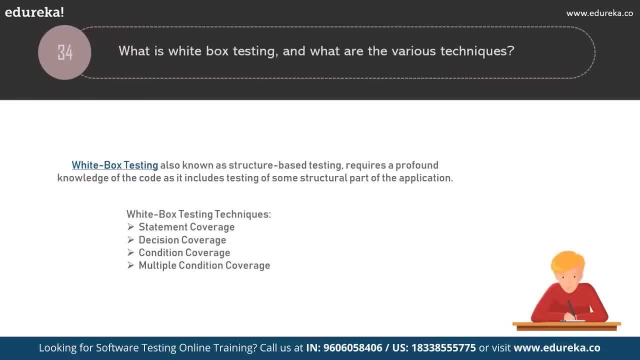 So, unlike black box testing and white box testing, the tester need to have some sort of knowledge regarding the internal architecture of the application that he's testing. The purpose, if you ask, is to enhance the security, check the flow of input-output through application to improve the design, usability and all that. 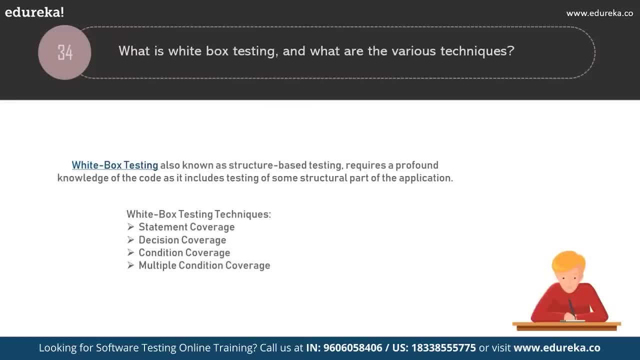 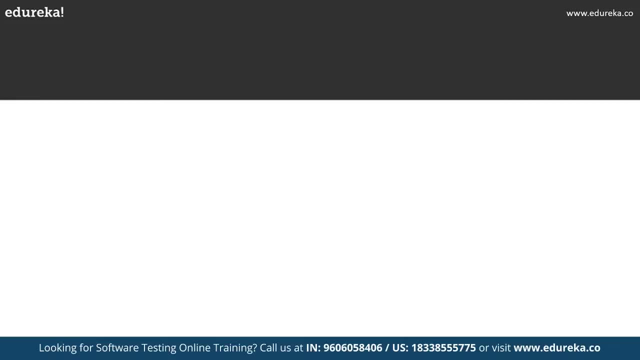 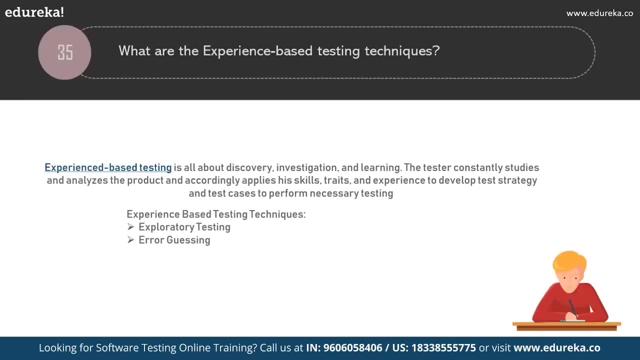 Various techniques that come under white box testing are you have decision coverage statements, condition coverage, condition coverage, multiple condition coverage and many others. Another question based on the same concept is: what are experience-based testing techniques? Experience-based testing is all about discovery. 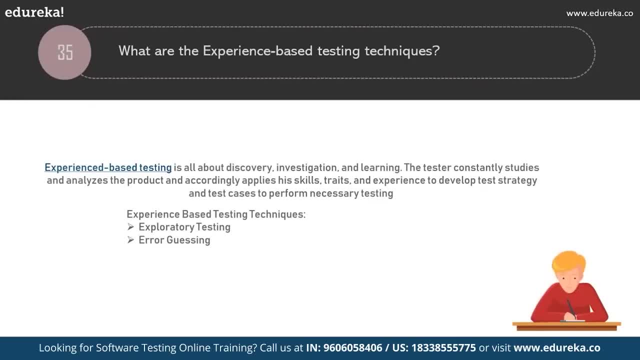 invention, intuition, and it's all about learning. So the tester constantly studies and analyzes the product and accordingly applies the skills, traits, experience to develop a test strategy and design test cases. So various techniques that come under this category are exploratory testing. 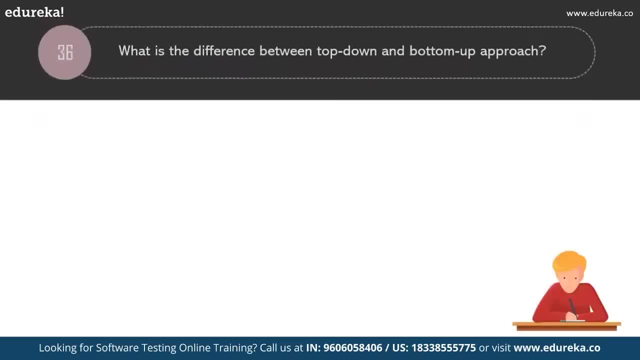 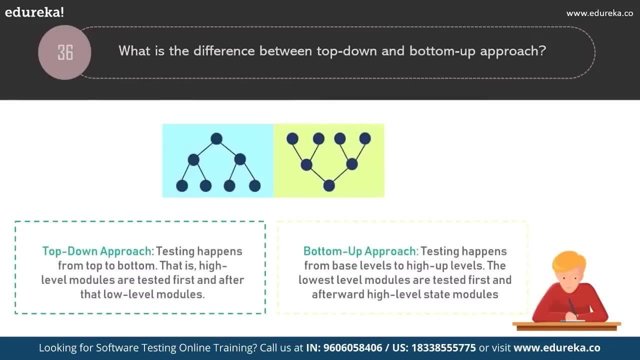 and interrogation. The next question that we have is: what's the difference between top-down and bottom-up approach? Well, it's all there in the name of the term itself. In top-down approach, testing happens from top to bottom, That's, high-level modules are tested. 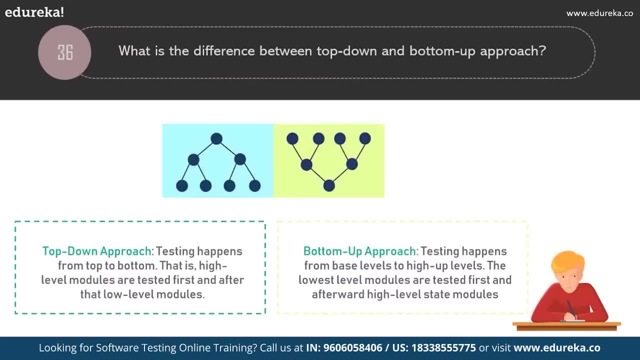 first, and after that, low-level modules And lastly, low-level modules are incorporated into a high-level state to guarantee that framework is working as it's supposed to do. Similarly, in bottom-up approach, testing happens from base levels to high-up levels. 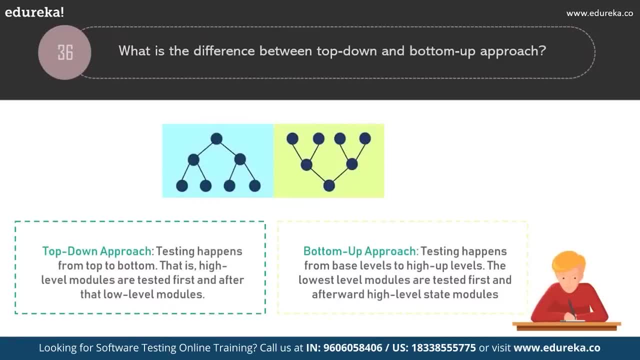 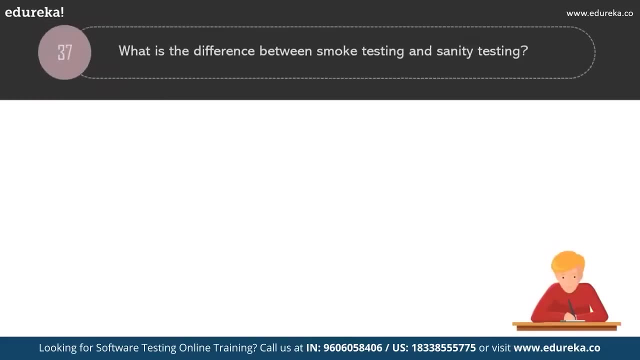 The lowest-level modules are tested first, and after that high-level modules. And lastly, high-level modules are incorporated to low-level state to see if the framework is working as expected or not. Moving on, we have what's the difference between smoke testing and sanity testing? 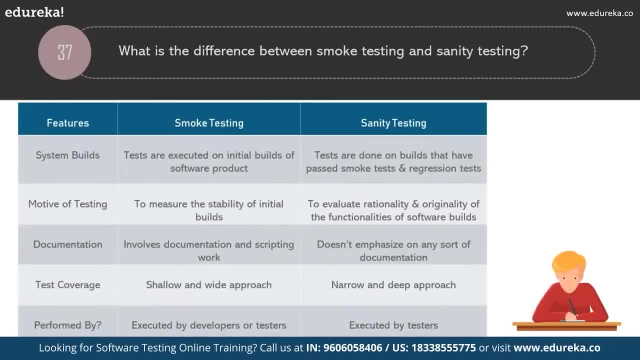 It's quite simple. The concept of smoke testing and sanity testing is very similar, except smoke tests are executed on initial builds of software product, whereas sanity testing are tests which are done on the builds that have passed smoke test and other rounds of regression test. 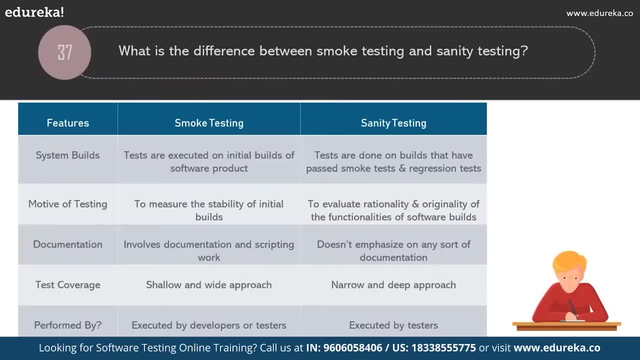 So what's the motive of smoke testing? It's to measure the stability of newly created builds so that it can go for more rigorous rounds of testing. What's the motive of sanity testing? That's to evaluate rationality and originality of the functionalities. 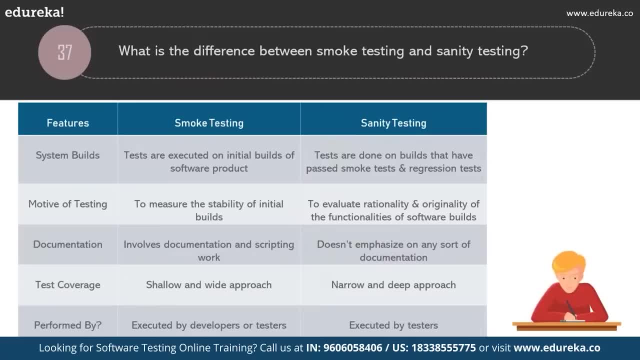 of software builds. Another main difference is that smoke testing involves a lot of documentation and scripting work, whereas sanity testing doesn't emphasize any sort of documentation. Smoke testing is a shallow and wide approach to include all major functionalities without actually going much deep, whereas sanity testing is narrow and deep approach. 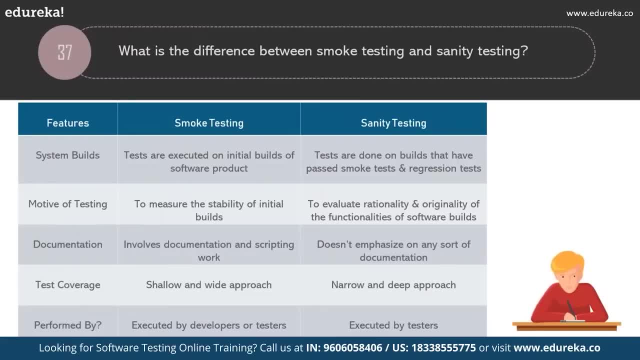 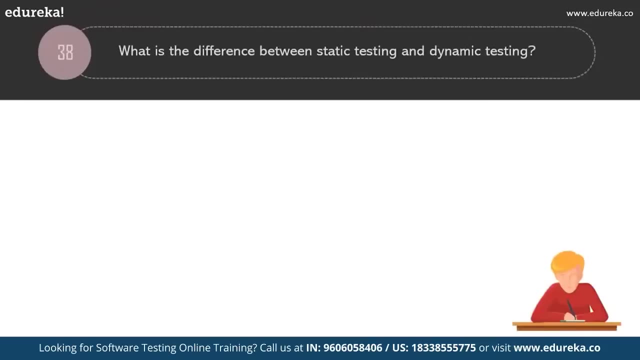 and it involves detailed testing of functionalities and features. Smoke testing is executed by developers as well as testers sometimes, whereas sanity testing is executed only by testers. We have another difference-based question, which is the difference between static testing and dynamic testing. So static testing is a white box testing technique. 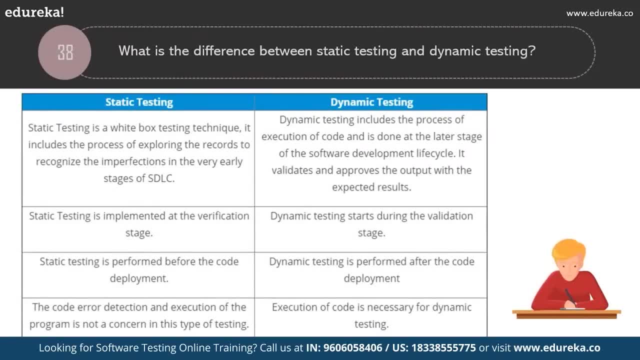 It includes the process of exploring the records or documents to recognize the imperfections in early stages of software development lifecycle. The key point is: static testing is performed in the early stages of development lifecycle to recognize imperfections. Dynamic testing: it includes a lot of execution of code. 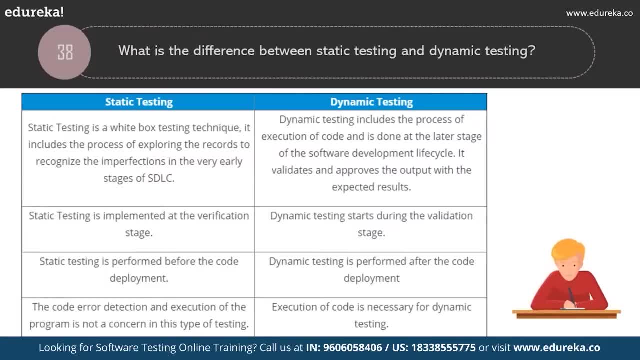 and it's done at later stage of software development lifecycle. It validates and it approves the output with expected results. Static testing is usually implemented at verification stage, so that's early stages, whereas dynamic testing usually starts during validation stage. Static testing is performed before the code deployment. 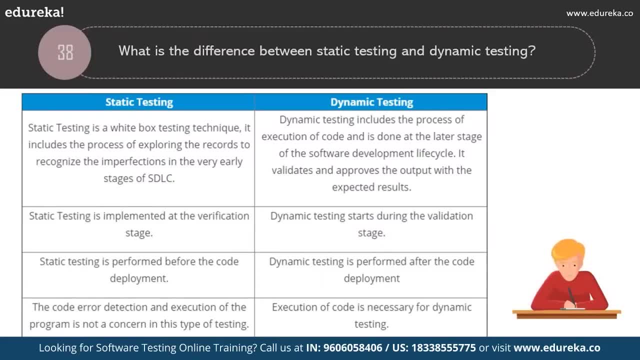 and dynamic testing is performed after the code deployment. Another important thing is code error detection, and execution of program is not much of a concern when it comes to static testing, whereas execution of code is really necessary when you're performing dynamic testing. So these are some key differences. 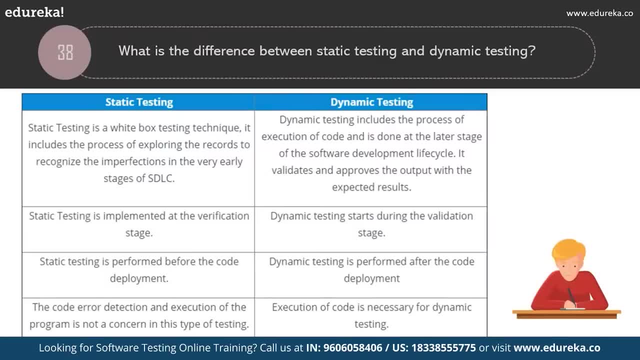 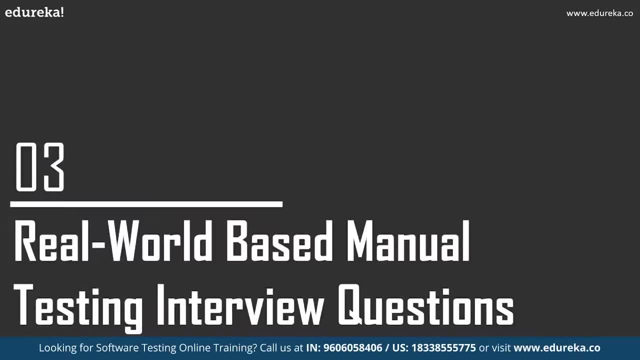 between static testing and dynamic testing. So, guys, with this we have come to the end of advanced level questions, or you can say theory-based questions. Now let's go ahead and deal with some real-world scenario-based questions. So the first question that we have under this category: 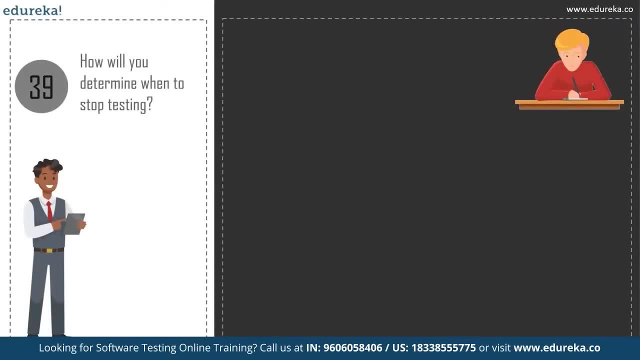 is: how will you actually go ahead and determine when to actually stop testing? Deciding when to stop testing can be really difficult. Many modern software applications are so complex and they run in such interdependent environment that complete testing can never be done. You agree with me there, right? 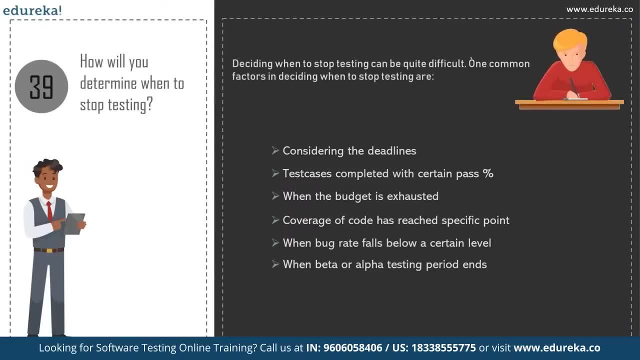 So some common factors that you can consider when you're facing difficulty to decide on when to stop your testing are that you can go ahead and consider the deadlines which are release deadlines, testing deadlines and all those and suppose if you have test cases which are completed. 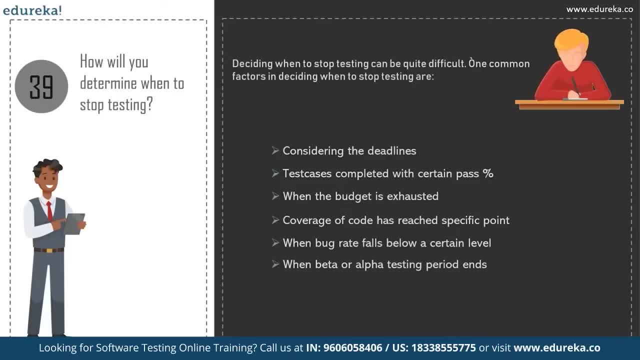 with certain pass percentage, then maybe you can go ahead and stop testing after you think that the amount of pass percentage is enough, or when your test purchase is completely depleted- Well, again, that's another reason to stop testing- or when coverage of code or functionality. 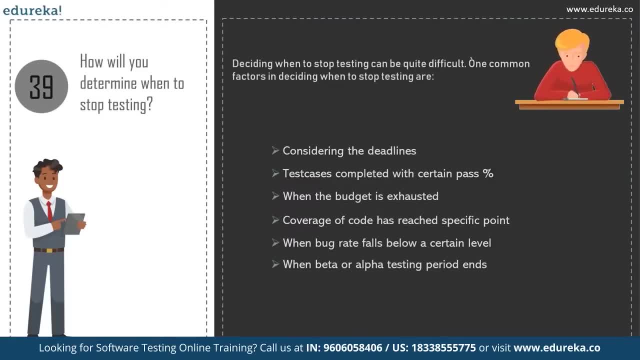 or any other requirements reaches a specific point, or when your bug rate falls below a certain level that you can no longer proceed with testing, or when your beta or alpha testing period actually ends. Well, these are certain simple ideas that can help you decide when to stop testing. 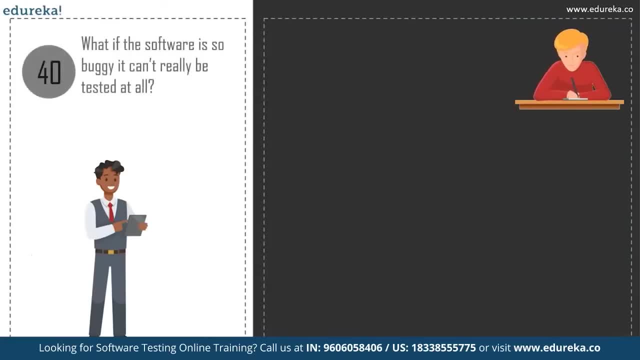 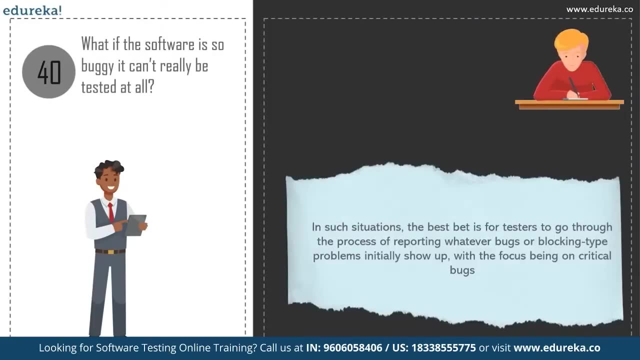 Moving on to next question: What if the software is so buggy that it cannot be tested at all? Often testers encounter a bug that cannot be resolved at all. In such situations, the best thing is for testers to go through the process of reporting whatever bugs they find. 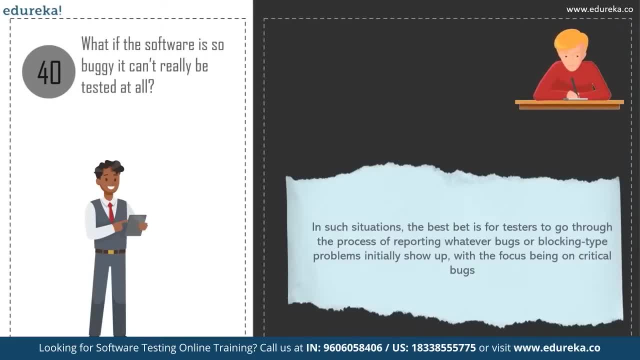 and focus mainly on critical bugs. Well, since this type of problem can cause other issues like insufficient unit testing or insufficient integration testing, poor design of an application, improper build or release procedures, etc. The higher authorities or managers should be notified and they should be provided with some sort of documentation. 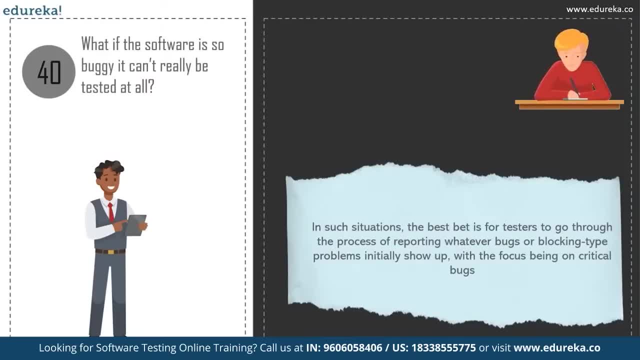 as a proof or evidence of the problem, saying that so-and-so bug has come up and we are facing an issue where we're not able to solve this bug at all. So in that way, they should provide some sort of documentation as an evidence of proof to their higher authorities. 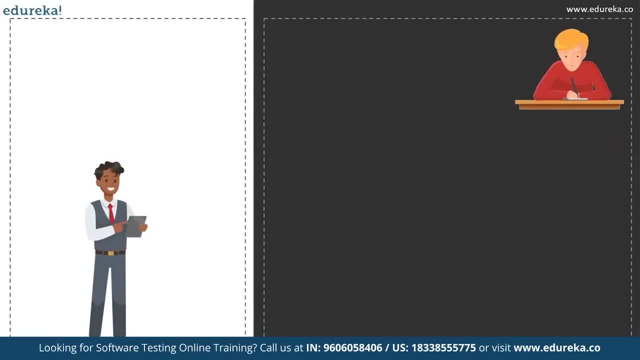 saying that bug is really not testable at all. Moving on to next question, How you actually test a product. if the requirements are yet to come, Do you freeze? It's possible that a requirement stack is not exactly or not available for a piece of product. 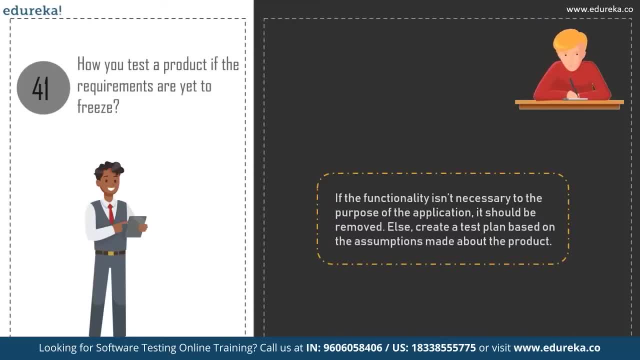 Sometimes it might take serious effort to decide if an application is significant unexpected functionality and obviously it would indicate deeper problems in software development process. So what do you do in such situations? So if the functionality for this, for which requirements are not there, isn't necessary for functioning of your application, 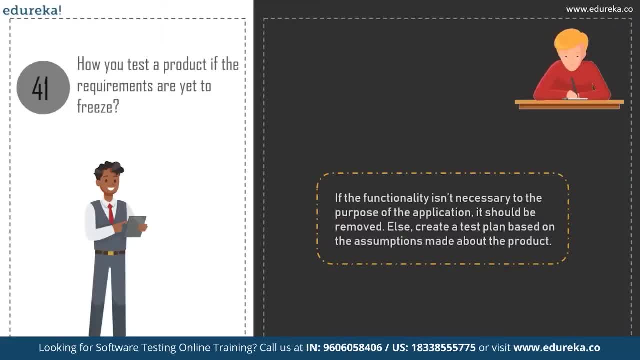 maybe you can actually remove that functionality. Well, if you think that functionality is really necessary, then go ahead, create a test plan based on the exceptions that you have made about the product, But again make sure that all the assumptions that you've made you get it right. 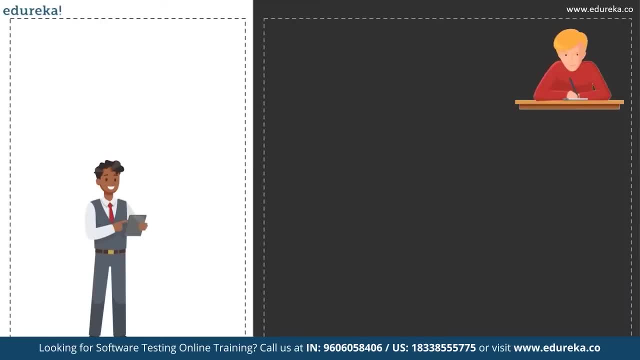 and they are well documented in the test plan. Moving on to next question: What if an organization is growing so fast that fixed testing procedures are impossible? What do you do in such situations? Well, this is a very common problem which is faced in software industry. 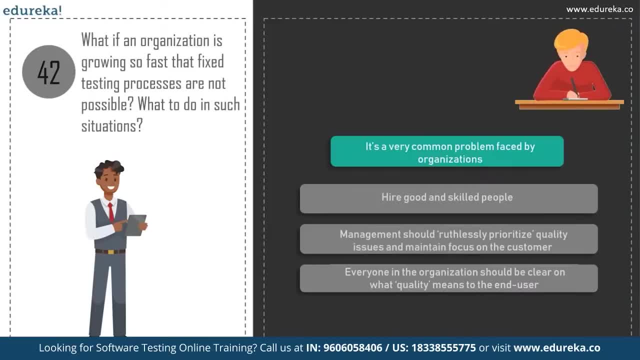 especially considering the new technologies that are being incorporated and some that are being popped up very now and then. so there's no easy situation or solution for the scenario. You can actually go ahead and I very skilled and good people to deal with the situation or management. 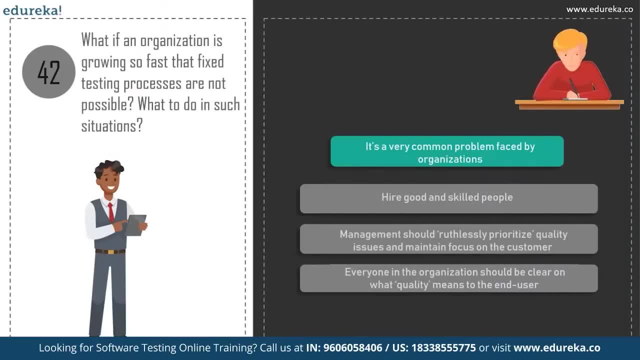 should actually ruthlessly prioritize quality issues, and their main focus should be put on customer, and everyone in the organization should be clear on what actually quality means to them. So these are certain solutions that they can adopt in situation where they actually think that the fixed testing procedures. 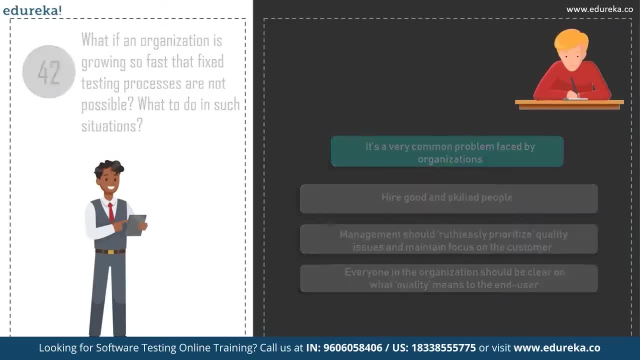 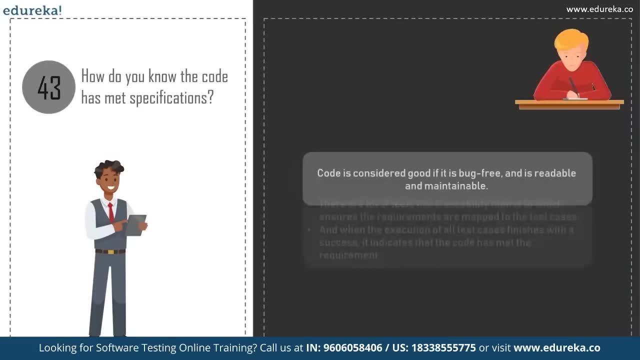 are no longer plausible or can be applied. Next question that we have is: how do you know that the code has actually met the specifications? So when I say a good code, it doesn't have any particular definition. in simple terms, Good code is code that works. that's bug free. It's readable and highly maintainable. So most organizations have their own coding standard that all the developers and testers are supposed to stick to, but everyone has different ideas about what's best, What's too many rules and what's very few rules, So there's no fixed thing as good code or anything. 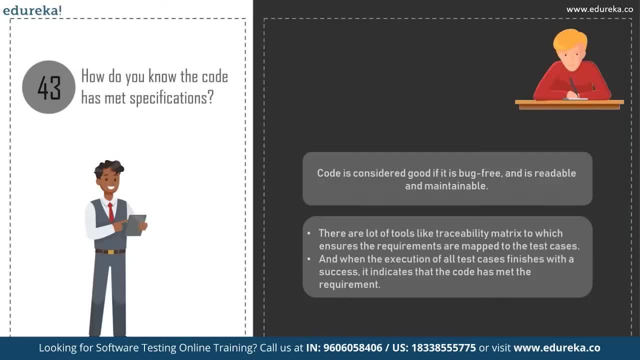 Well, honestly, there are a lot of tools these days that can help you check if your code is sustainable, if it's good or if it is met specifications. For example, you have something called traceability matrix, which ensures that all your requirements are mapped to the test cases. 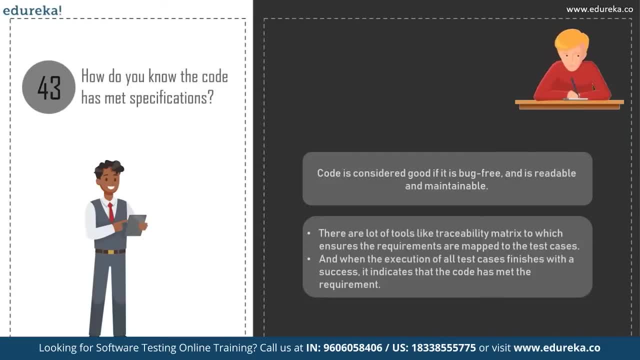 and when the execution of all the test cases finishes with success, it indicates that the code is met to requirement. So you can go ahead and use such tools to see if your code is met the specifications or not. Let's move on to our next question. 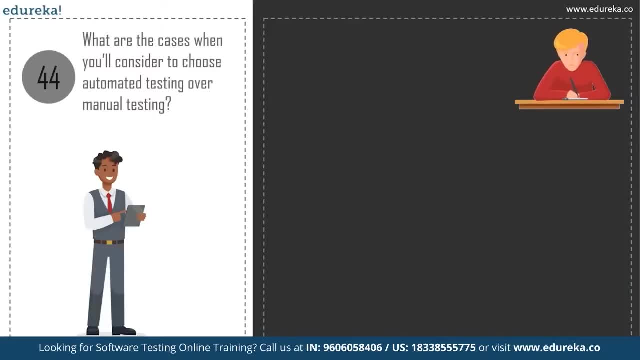 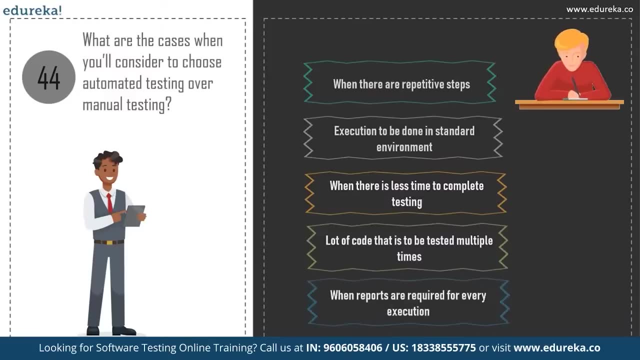 So what are certain cases where you consider to choose automated testing over manual testing? Automated testing can be considered over manual testing during multiple situations. For example, when you have test cases that require periodic execution. when the tests include repetitive steps. when tests need to be executed. 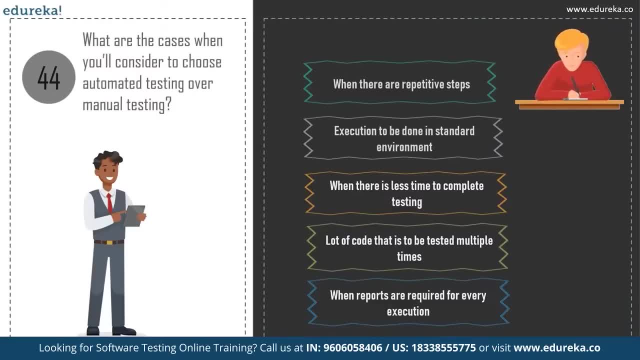 in a standard runtime environment, you can go ahead and adopt automation testing rather than manual testing. Also, when you have very less time to complete the test phase, when there's a lot of code that needs to be repeatedly tested and when there are reports that are required for every execution. 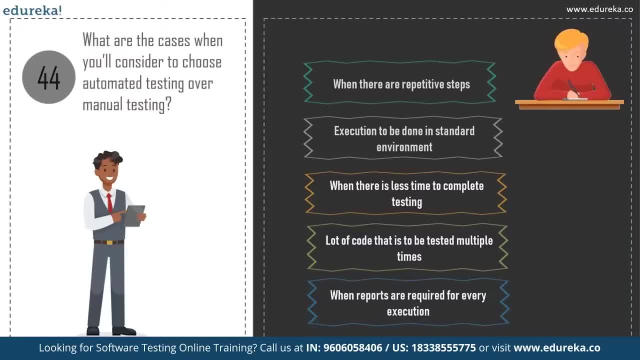 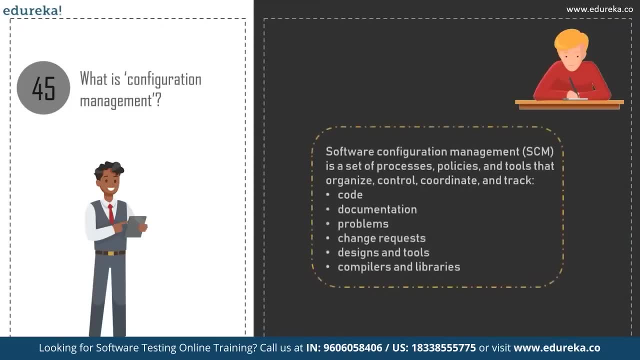 then actually you can go ahead and use automation than manual. So the next question that we have here is quite interesting: What's configuration management? So every high-functioning organization has a master plan right That details how they're supposed to operate and how they're supposed to achieve their goals. 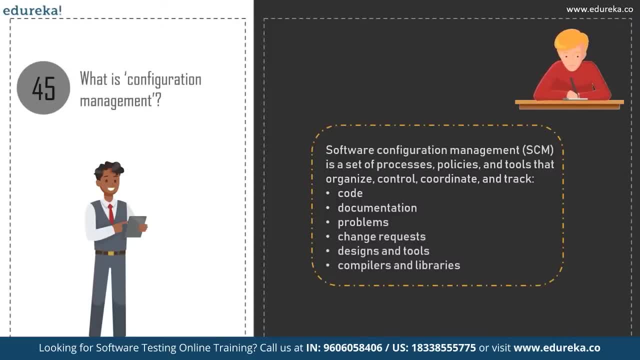 and all that Well. software development and testing are no different. Software Configuration Management, or SCM, is set of processes, policies and tools that organize, control, coordinate and track code: different documentations, problems, change requests, designs, tools, compilers and libraries. 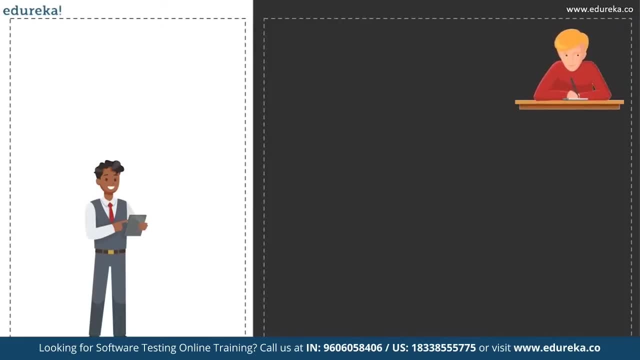 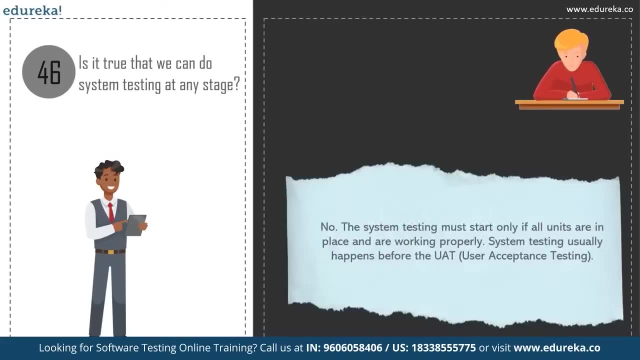 Well, you can call it as a master plan for testing. Next question is: is it true that you can actually go ahead and do system testing at any stage? System testing: all the components of software are tested as a whole in order to make sure that overall product. 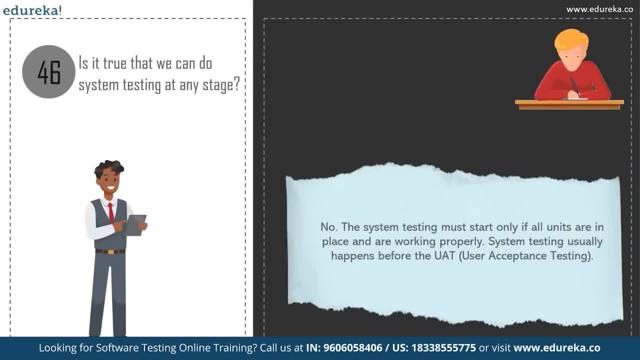 meets the requirements specified. So no, system testing cannot be performed at any stage. It can only start if all the units or modules are in place and are working individually properly. Another thing is that system testing actually happens before you perform user acceptance testing. 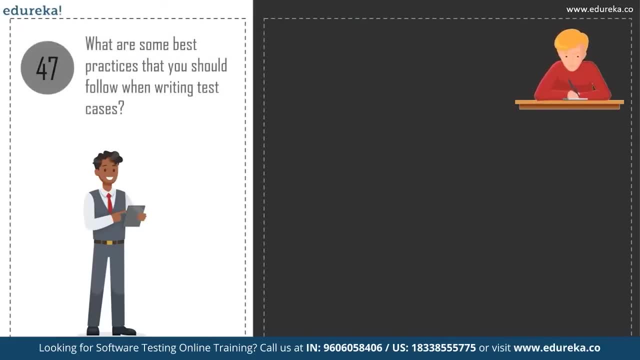 Next question is: what are certain best practices that you should follow when writing test cases? When you're performing testing on a large scale, you have like thousands of requirements to consider, And if you go ahead and write your test cases randomly, it will become difficult for you to track later on. 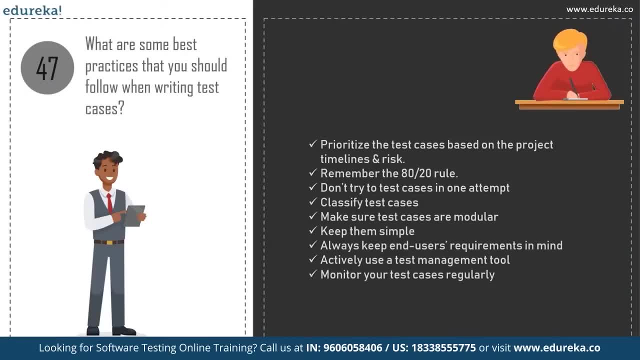 For that very reason, you have some practices that you can go ahead and follow, and it will make you much more easier to keep track of your test cases. So, first of all, prioritize which test case to write, based on the project timeline and the risk factor of your application. 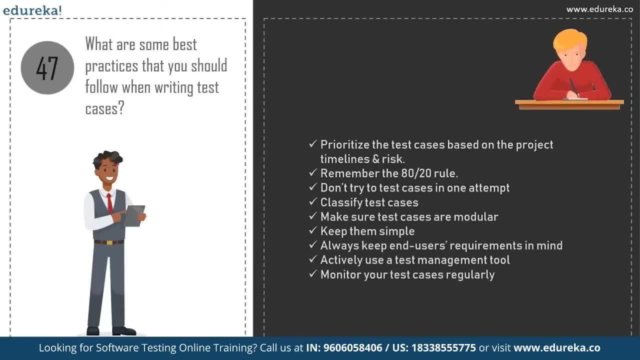 Always remember the 80-20 rule. So to achieve best coverage, 20% of your test should cover 80% of your application. That's 80-20 rule. So don't try to test all the cases in one attempt. 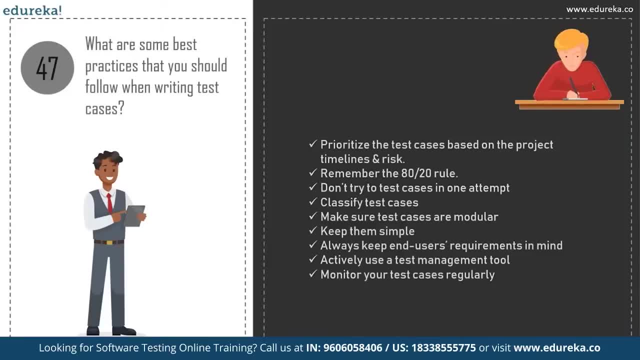 Instead, improvise them as you progress, List down your test cases and classify them and separate them based on your business scenarios and different functionality. Make sure your test cases are modular and your test case steps are as granular as possible. Another thing is that 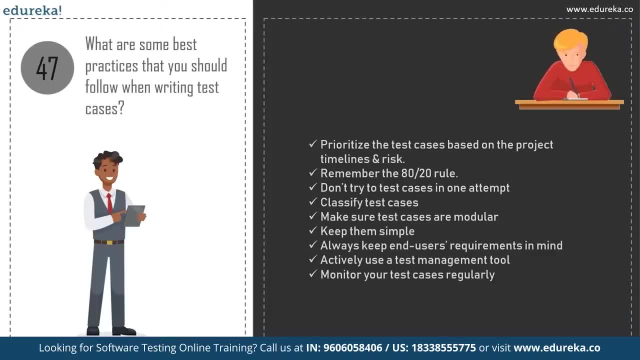 write your test cases in such a way that others can easily understand them and modify them if required. Always keep end users requirement in back of your mind, because, ultimately, the software product that you're testing or designing is for the test end users. Well, always remember using a test management tool. 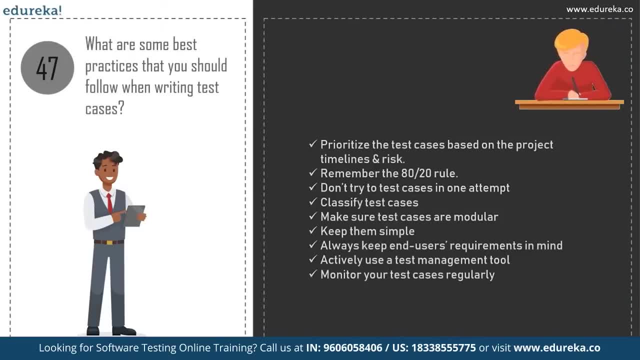 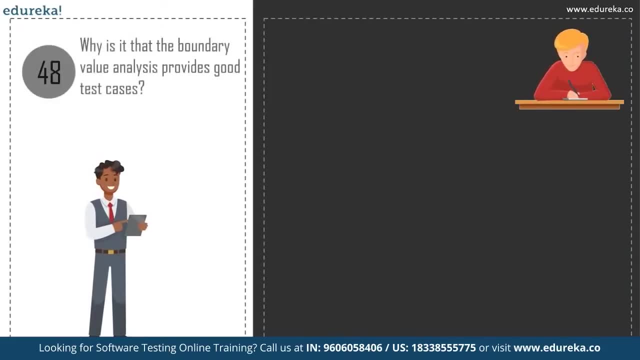 to manage stable release cycle. Monitor your test cases regularly, Write unique test cases and remove irrelevant and duplicate ones. Moving on to our next question: Why is that boundary value analysis provides very good test cases? So the reason why boundary value analysis provides good test cases is that 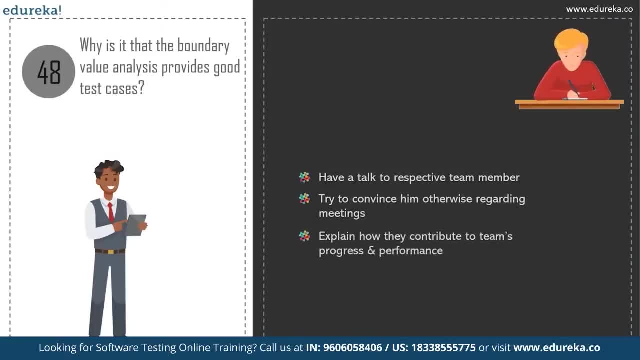 a greater number of errors actually occur at boundaries rather than in the center of the input domain for any test. So basically, in boundary value analysis, test cases are designed to include values at boundaries, and that's why boundary value analysis provides very good test cases. So if the input is within the boundary value, 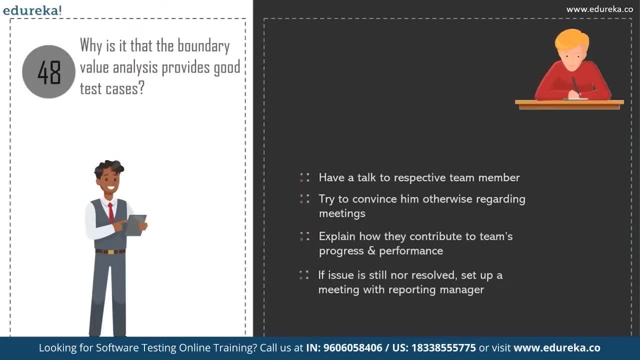 it's considered positive testing and if your input is outside of your boundary value, it's considered negative testing. So when I say boundary value analysis, it includes different values like maximum minimum, inside or outside edge, typical values or error values. Next question that we have is: 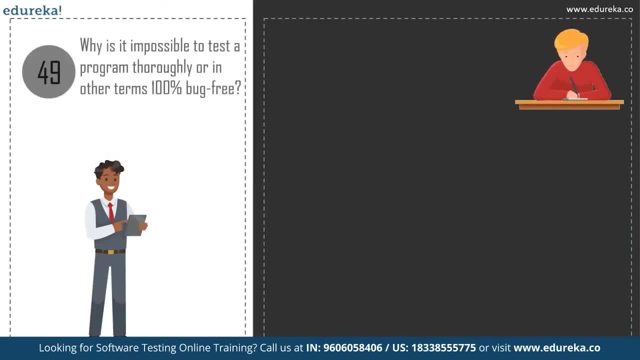 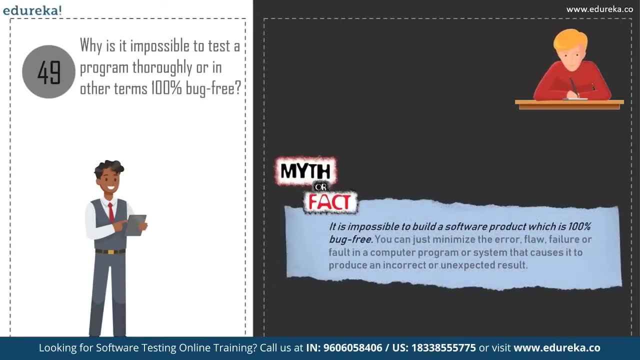 why is it impossible to test a program thoroughly, or in other terms, 100% bug free? Because it's impossible to build a software product which is 100% bug free. You can just minimize the error, flaws or failures or faults in your computer program. 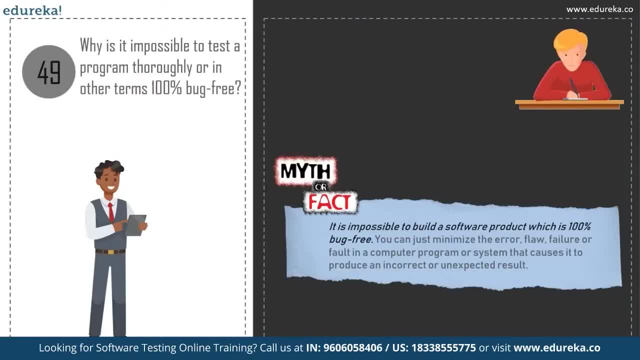 or system which cause it to produce an unexpected result. but it's impossible to make it 100% error free. Well, here are some two principal reasons that make it impossible to test a program entirely. First of all, software specifications and requirements can be subjective. 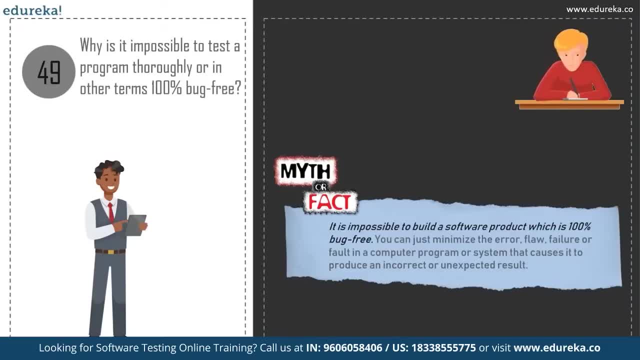 and they can lead to different interpretations. Secondly, a software program might require too many inputs, too many outputs and too many path combinations to test. Well, these reasons make it impossible to test a program entirely. So the last question that we have is: 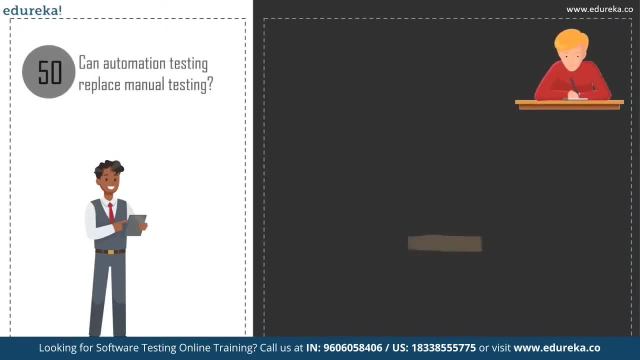 can automation testing replace manual testing? Automation testing isn't a replacement for manual testing. No matter how good automation tests are, you cannot actually go ahead and automate everything right. Manual tests play a very important role in software development and they come in handy whenever you have a case. 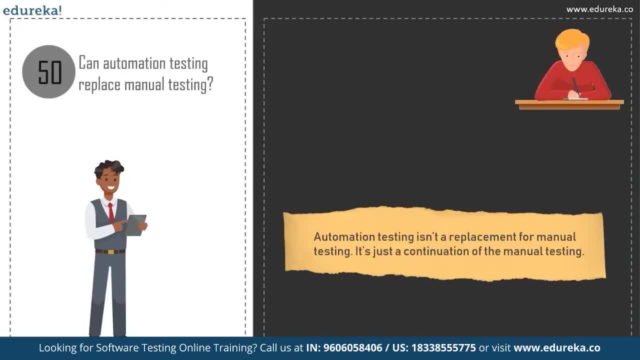 where you cannot apply automation. So automation and manual testing each have their own strengths and weaknesses. In simple terms, manual testing helps you to understand the entire program or problem and explore the functionality of a feature or applications from users perspective, or in other words, with more flexibility. 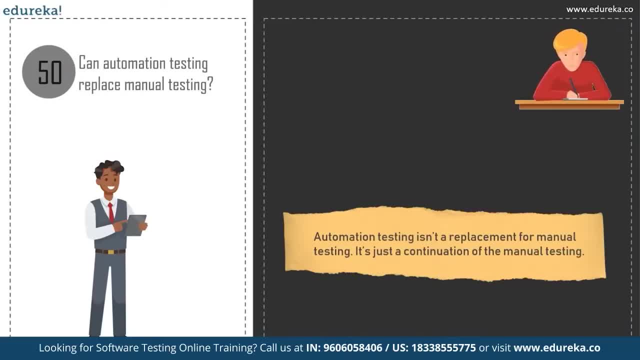 On the other hand, automated testing helps save time in long run by using a lot of tools and techniques and scripts. So, like I said, both of them have their pros and cons. So automation testing isn't actually a replacement. It's another way of performing software testing. 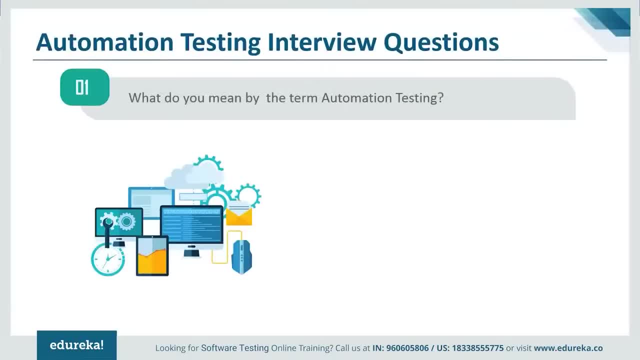 So let's begin with the basic questions. So here goes our first question: What do you mean by term automation, testing? Well, we've already discussed this. Anyway. automation focuses on replacing manual human activity with systems or devices that enhance the efficiency of our work. 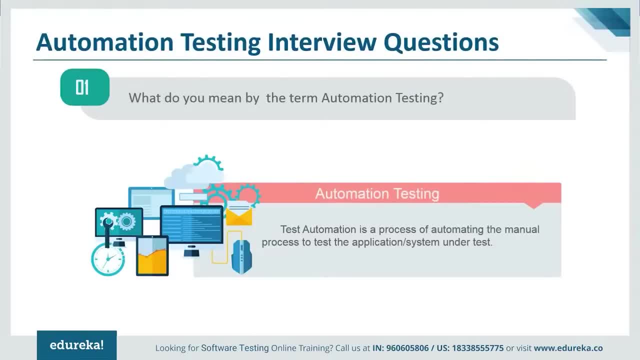 The process of using special software tools or some sort of scripts to perform testing tasks, such as entering data, or it could be executing the test steps or comparing the results with the expected results- is known as automation testing. So basically, in automation testing you're trying to replace the human. 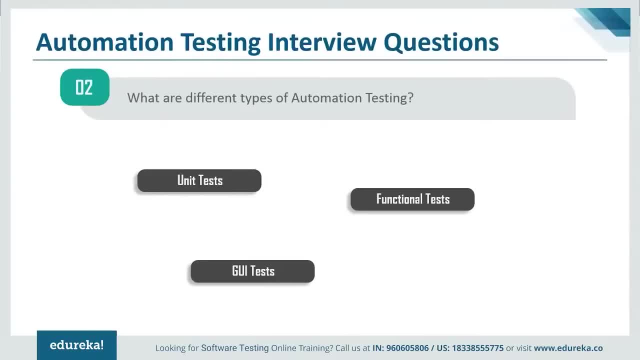 who is performing the testing? Moving on to our next question, What are different types of automation testing, guys? Automation testing is basically divided into four to five categories, but the most popular ones are So: unit test, graphical user interface test and functional test. 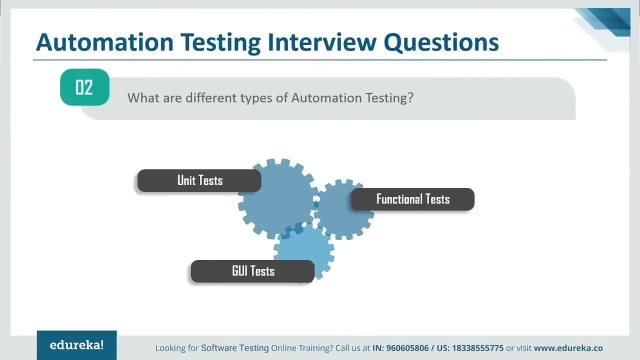 So unit test. These are usually done at the development phase and the help reduce the box in the initial stage of development of software itself. Then we have graphical user interface test. These tests are usually done at testing level and these tests are mainly written to focus. 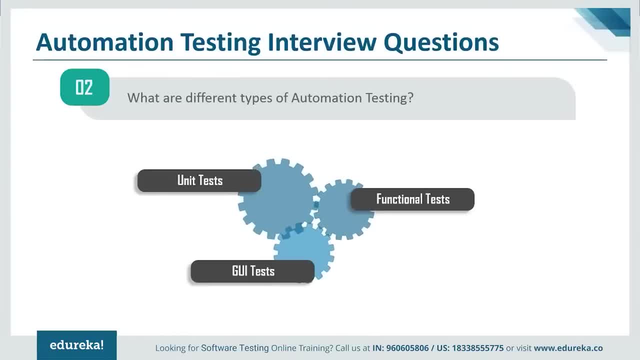 if the test interface or the interface of an application or software that you're testing on is working properly under certain conditions or not, Then we have functional test, just like graphical user interface test. These are also done at testing level. This simulate the functional scenarios. 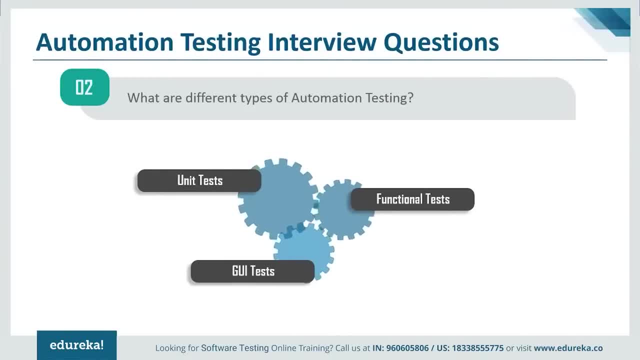 to test if the application works properly or not for the provided input at different conditions. So basically, here we are checking the functionality of an application or software or any item that you're performing testing on. Apart from these three, we also have something called web service testing. 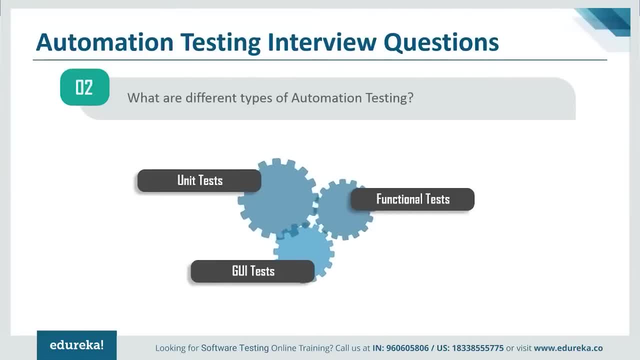 Web service testing is testing of web services and its protocols, like SOAP protocol, dress protocol and all that. So automation testing is divided into about four to five categories, but the most important ones are unit test, graphical user interface test and functional test. So, guys, now moving on to our third question. 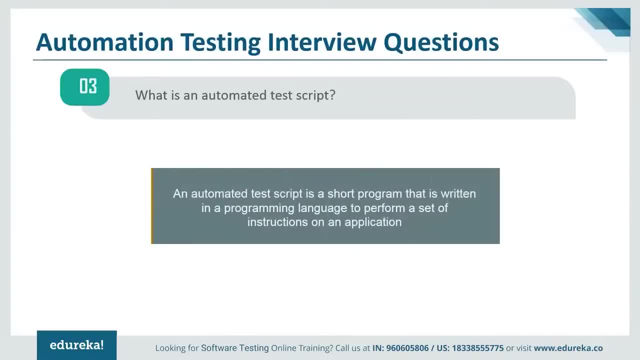 What is an automated test script? and automated test script is basically a short program which is actually written in some sort of programming language to perform a set of instructions on the software or the application that you're testing on. So when you run this program, 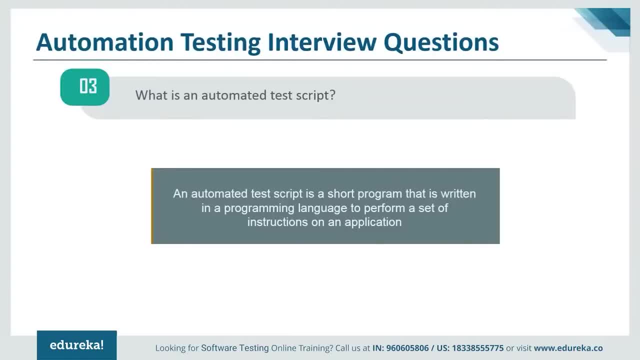 it gives the test results as pass or fail, depending on if the application is working as per your expectations or not. So, basically, whatever test you want to perform on the application of the software, you writing it as a program or in form of program in the test script. 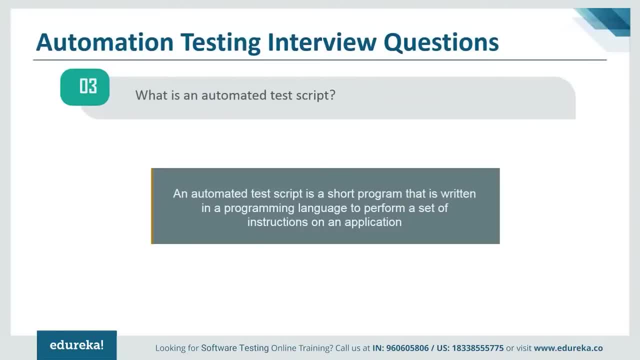 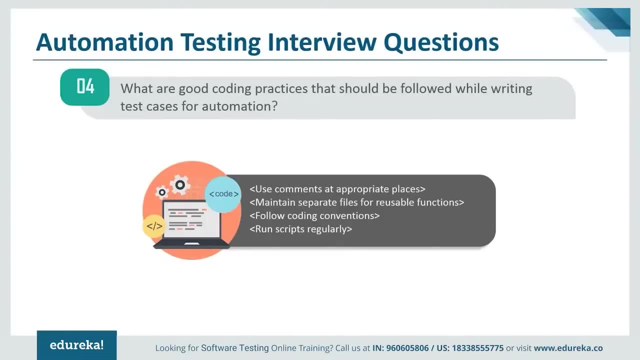 and that's what we call automated test script. Next question: What are good coding practices that you should follow while writing test cases for automation? So, guys, before you actually go ahead and write code for your testing, you need to follow certain coding standards. 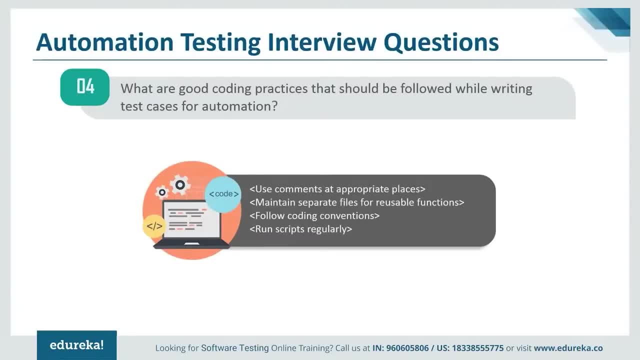 For example, you need to use comments at regular paces, You need to maintain separate file if you have functions that you want to reuse and there are certain coding conventions that you have to follow, like colon and all that, and, most importantly, you should regularly run your scripts. 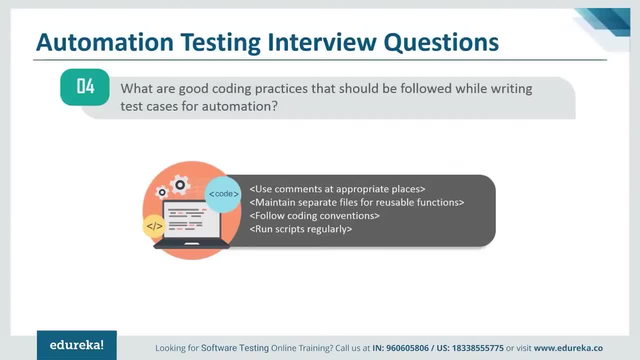 to make sure that you do not make any error or there are no box in the code that you've written. So these are certain coding practices that you need to follow when you're writing code for your automation. This way, you will be sure that if you get an error. 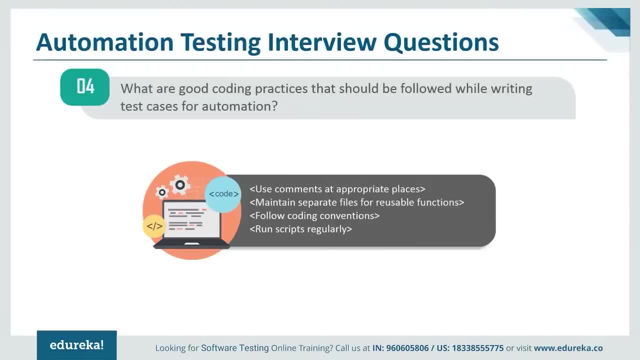 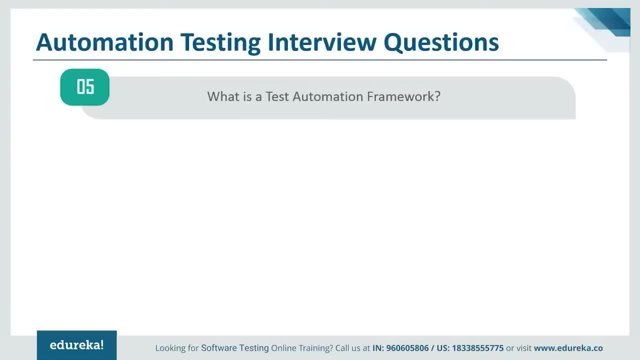 it's not because of your code, It will be because of the box which are in the application. Next question, guys, This is most frequently asked question: every interview, every test automation interview. This is a must or definite question, guys. which is, what is a test automation framework? 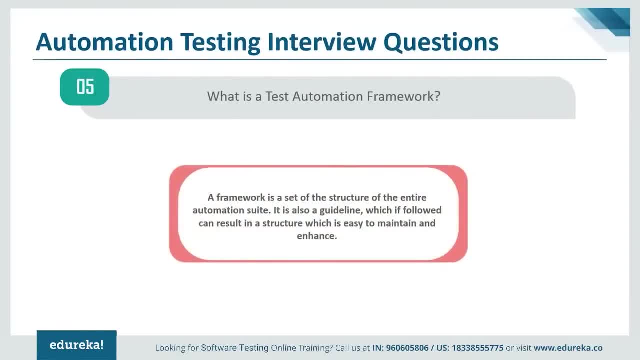 a test automation framework is a set of guidelines used to produce beneficial results of automation testing activity. So basically, in simple terms, it's set of guidelines and rules that every tester follows universally. the framework brings together function libraries, test data sources, object details and other reusable modules, functions and methods. 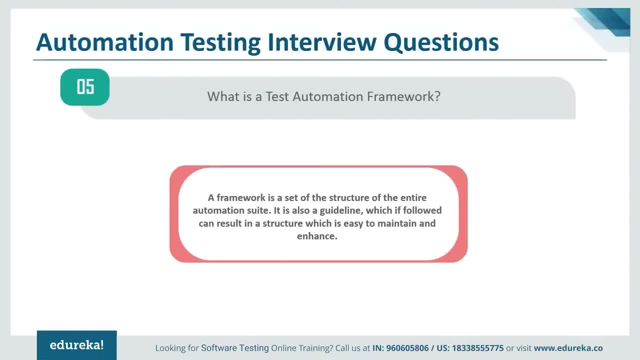 So once you've adopted any kind of test framework, you can even extend the framework. For example, the guidelines which are set in any framework would be rules for writing test cases, coding guidelines for creating tests and test handlers, or it could be input test data templates. 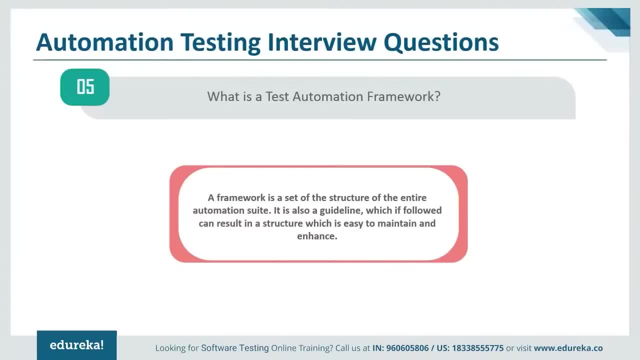 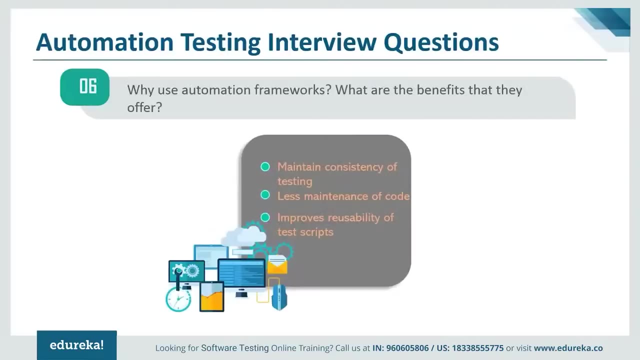 or object repository management, log configuration, test results and reporting usage. All of these are the guidelines which are listed in any framework, So make sure you get to know more about automation framework before you attend any testing interview. next question: Why use automated frameworks? What are the benefits that they offer? 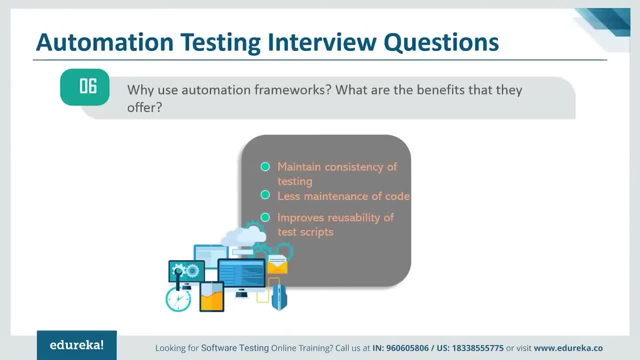 First of all, guys, they established a universal standard for testers to achieve the specific goals of automated tests. They maintain consistency of testing. So, basically, these are the rules which are followed by every tester all around the world. This way, they maintain consistency of testing. 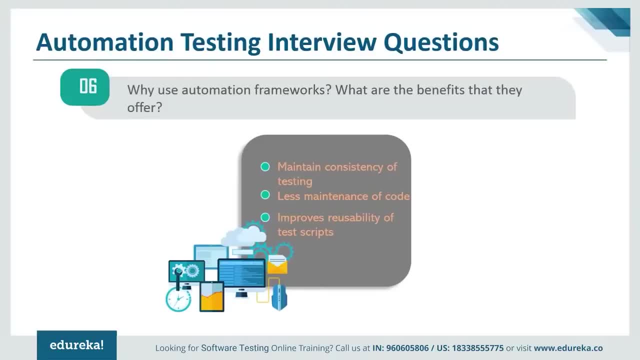 You are also provided with commonly used methods. This way it improves the efficiency of automated task and framework and even with the limited knowledge of how the test case is set up, a tester can easily depend on the framework to refer to simple statements and implement the test cases. 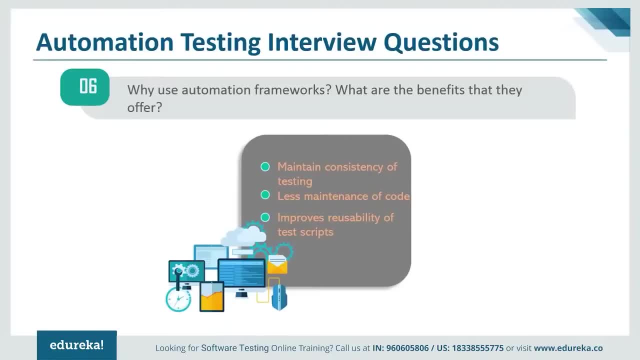 You can easily reuse the test scripts for future purposes. So with a proper framework, the code is easier to maintain and often reusable. So, technically, automation framework: when designed and implemented correctly, they deliver frequent and stable automated test code. So basically, in simple terms, is automation frameworks. 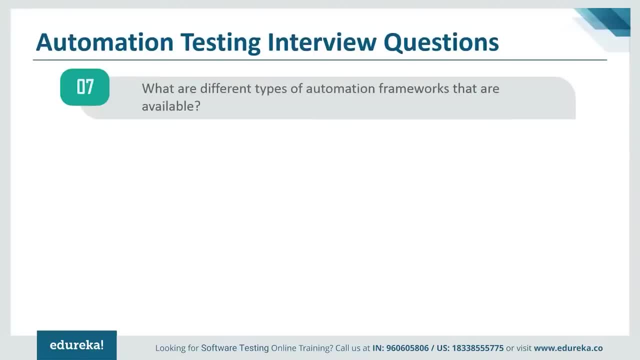 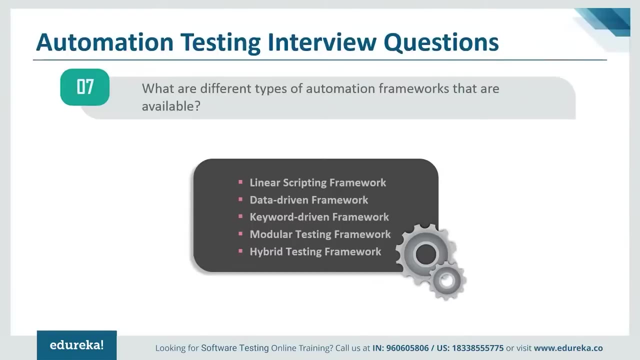 make the life of a tester much more easier, guys. One more question about automation framework. What are different types of automation frameworks that are available right now? So first we have linear scripting framework. linear scripting framework is basic level test automation framework, which is basically in the form of record. 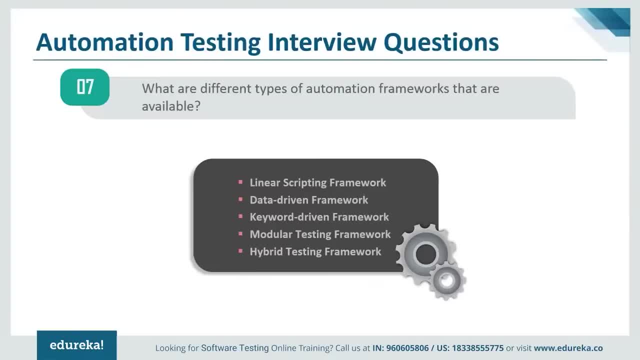 and playback in a linear fashion. This framework is also known as record and playback framework. This type of framework is used to test small size applications. in this type, creation and execution of test script are done individually for every test case. So this is the basic level test automation framework. 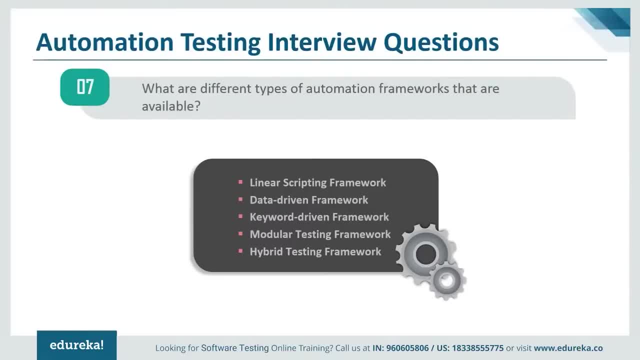 Then there is data-driven framework. data-driven test automation framework is focused on separating your test scripts that you have written from the test data that you want to test on. So it allows us to create test automation scripts by passing different set of data types. The test data set is kept in external files. 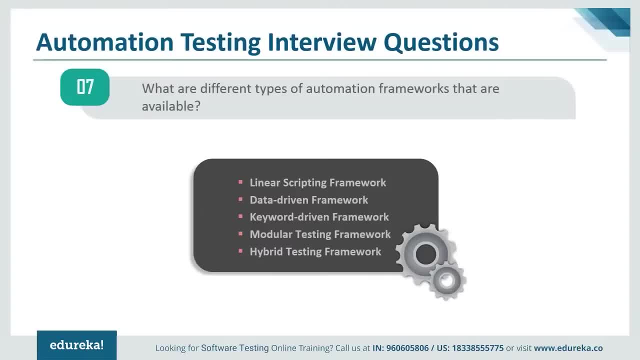 or resources such as excel sheets, or it could be access tables or SQL database or XML files, Etc. Then you have keyword driven framework. This keyword driven framework is also known as table driven or action word based testing. in keyword driven testing, We use a table format to define some sort of keyword. 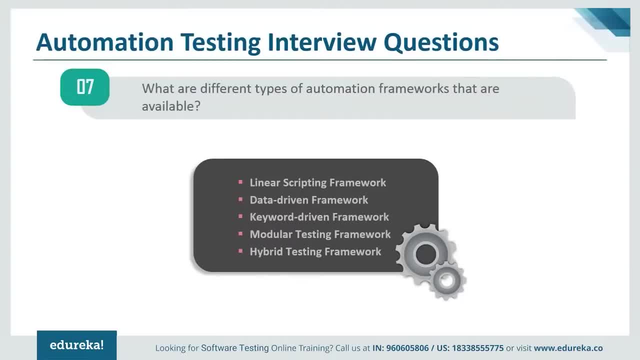 or action word for each method that you could execute in your code. now, based on the keywords or action words which are specified in the excel sheet, that scripting is done and test are executed by using this framework. since we are using keyword and action words, programmer need not know much. 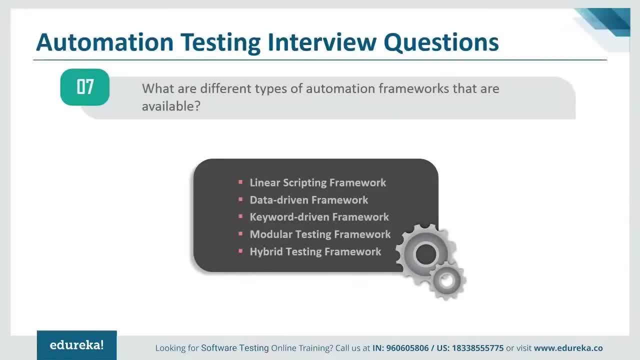 about the scripting language here. Then we have modular testing framework. here, tester divides the application into multiple modules and creates test scripts individually for each module. these individual test scripts, which are written for each module, are then combined to make larger test scripts by using a master script. 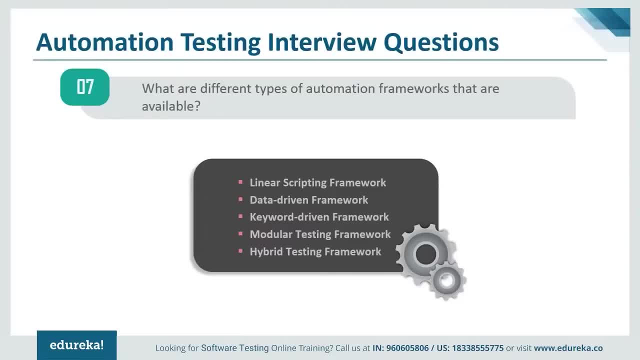 This master script is used to invoke the individual modules to run end-to-end test scenarios. So basically, you divide applications into multiple modules, then for each module you write down a test case and then combine this test case according to your requirements using a master test script. 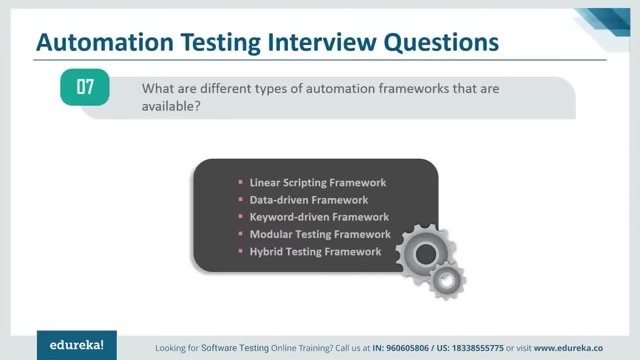 and the last one is hybrid testing framework. hybrid test automation framework is literally a combination of two or more frameworks that we just discussed. it attempts to leverage the strength and benefit of other framework for particular test environment It can manage. apart from these five, you also have others. 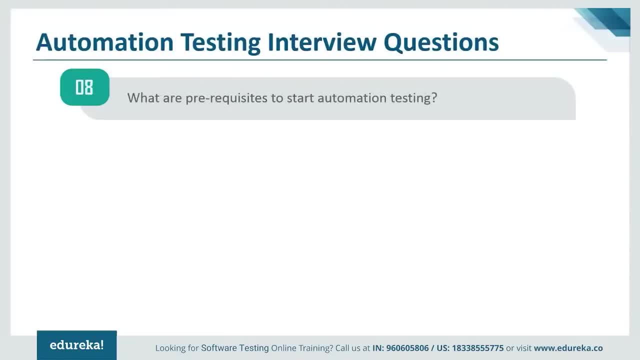 but these five are the most popular ones. next question: What are prerequisites to start automation testing? So, guys, before you actually start automation, you need to be aware of certain things. For example, you should make sure that the bill for your framework is stable. 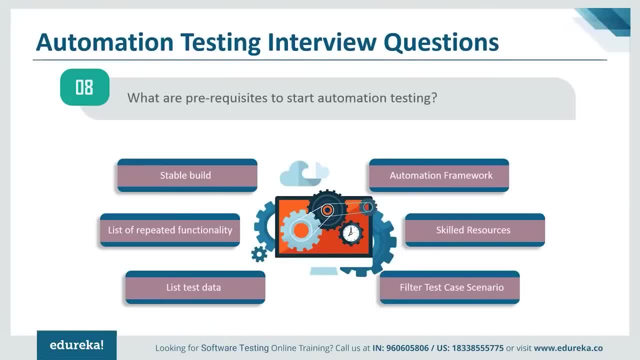 You should make sure to filter the test cases which you need to automate, as in, you should be sure as to which test cases you want to automate and which not. you need to separate the functions which you will use repeatedly and if you have certain functions which you want. 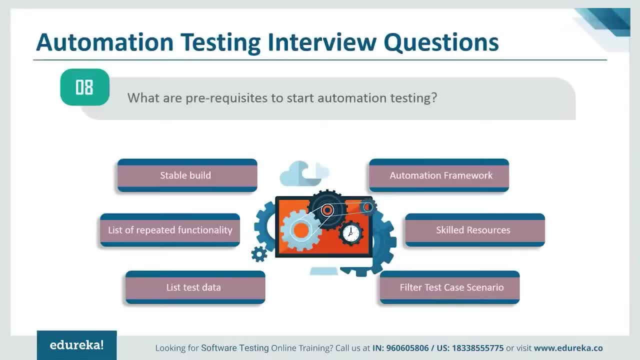 to use repeatedly. make sure you storing in separate files. Make sure you have your application modules in such a way that their requirements do not change frequently. in such cases, automation becomes difficult. and the most important one: make sure you have skilled and experienced resources. This makes your automation much more easier. 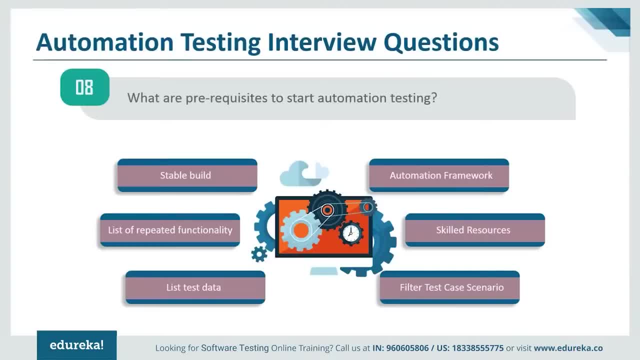 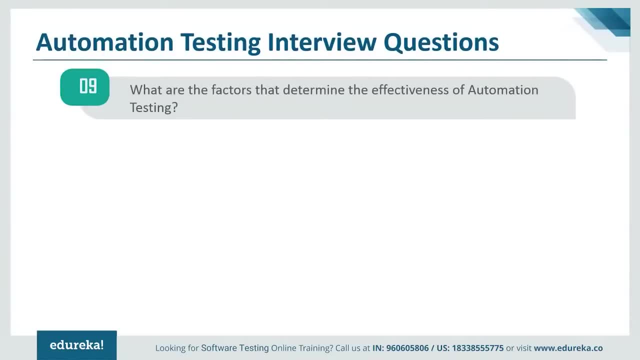 So these are certain things and points that you should keep in mind before you actually start automation. moving on to next question, What are the factors that determine the effectiveness of automation testing? There are certain key factors which help you decide if your automation was successful or not. first of all, 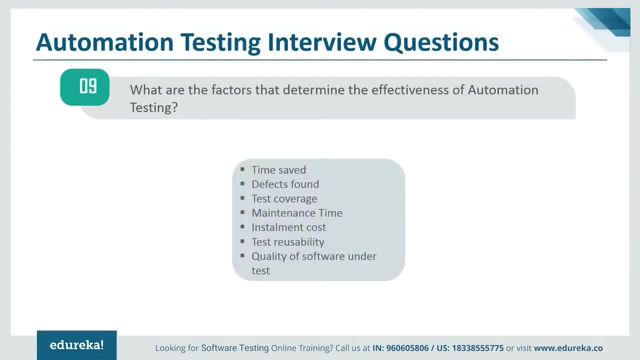 obviously the amount of time saved. then you have the number of defects or bugs found after automation. the test coverage, as in literally one test covers how much data or how many cases like that. then you have maintenance time that you've spent on maintaining the automation software. then installment cost the amount of money. 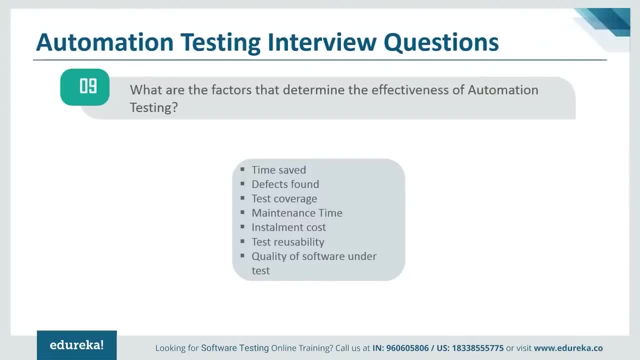 that you spend before actually starting your automation. then the test case readability- as an easier test cases usable or the just not reusable as such, and lastly, the quality of the software that you're actually performing. test on. these determine if your automation was successful or not. and here we go, the most common question. 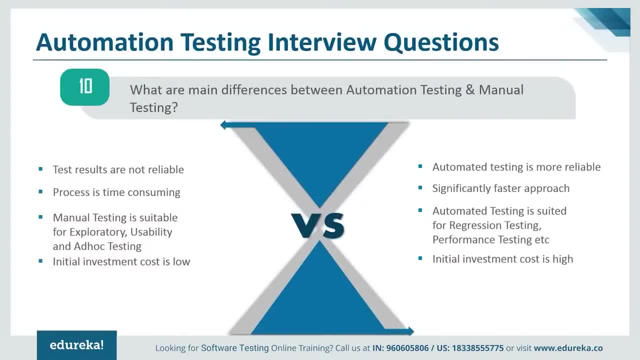 What are the main differences between automation testing and manual testing? So when you begin testing, one of the primary decisions that you'll have to make is when you're going to test manually or use automated testing. So you have to be aware of distinct differences between manual testing and automation testing. 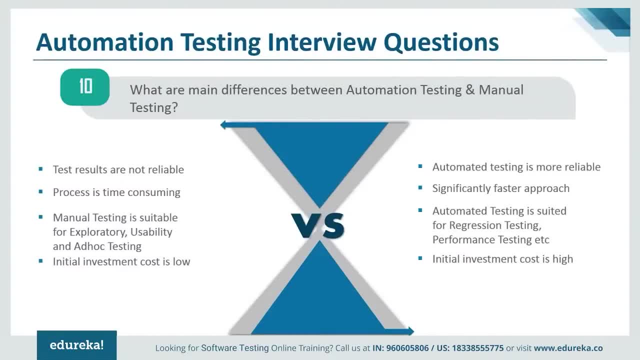 The first point is obviously reliability for a testing phase which is very long. Let's say it's very long. There are high chances of an undetected error when testing is performed manually. So when you perform testing manually, you have to do test repeatedly again and again. the task becomes boring. 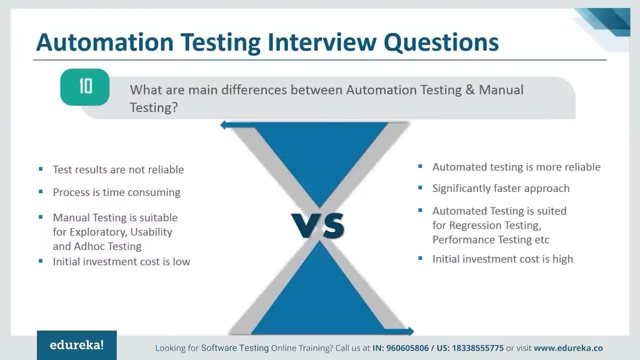 and it's quite possible that you might overlook some errors. So in such cases reliability is really less, whereas in automated testing you use different kind of tools and scripting to perform the test and find the box, So there's no chance of making any errors. 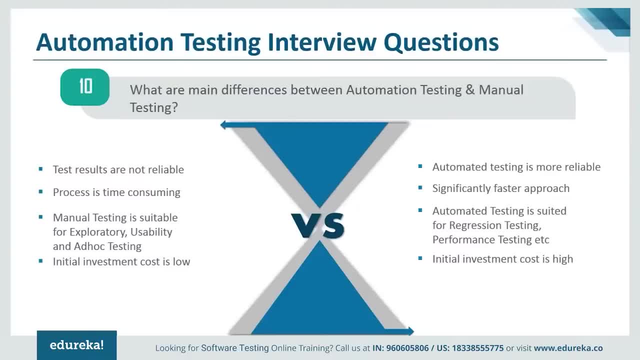 So the reliability in automation testing is literally high and again and manual testing, It's humans who are performing the testing and obviously humans are little slower when compared to machines, right? So the processing time is more in manual testing while compared to automation testing. 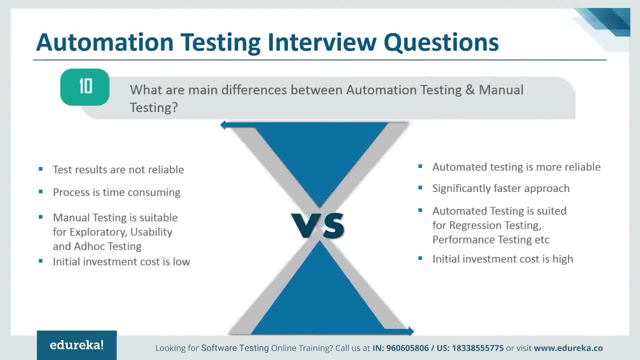 And the important point is, you cannot use manual testing and automation testing everywhere. There are certain cases where manual testing is suitable and there are certain cases where automation testing is suitable. For example, manual testing is suitable for one-time task or exploratory or usability and Haddock testing. 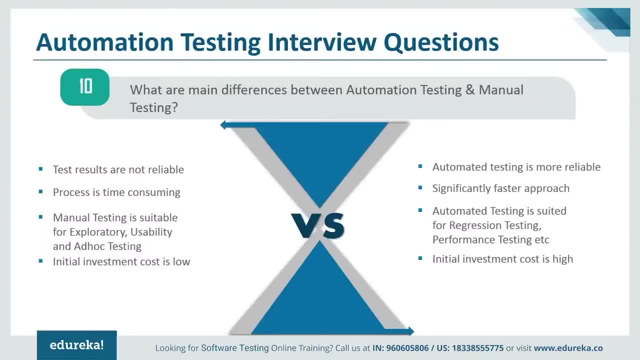 Whereas automated testing is suited if you want to perform test repeatedly for long run, or for regression testing or performance testing, Etc. Apart from that, initial investment costs in manual testing is low, but the return of investment, as in the amount you get as a written after you perform your automation, is also less. 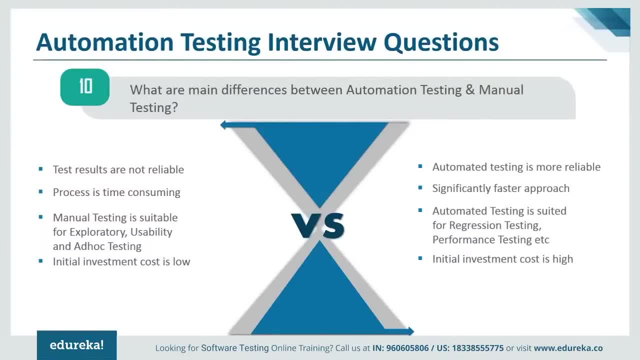 in manual testing, But when it comes to automation testing, initial investment cost is high and the return of investment is also high in longer run. So these are some basic differences between automation testing and manual testing. Let's move on to a next question. So is it possible to achieve hundred percent automation? 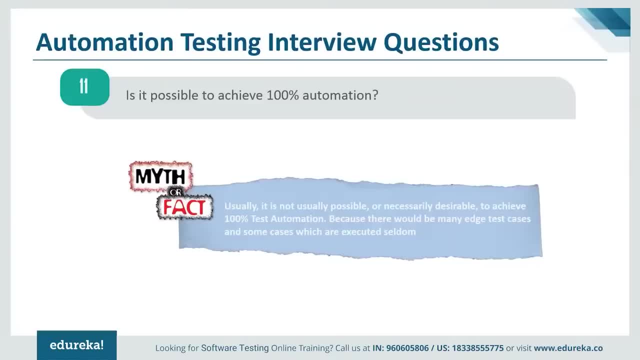 hundred percent automation is definitely not possible, guys. There are certain test cases that cannot easily be automated, For example, checking the background color of an window or a delock box. Well, why would you do that Right? It's a very simple task. 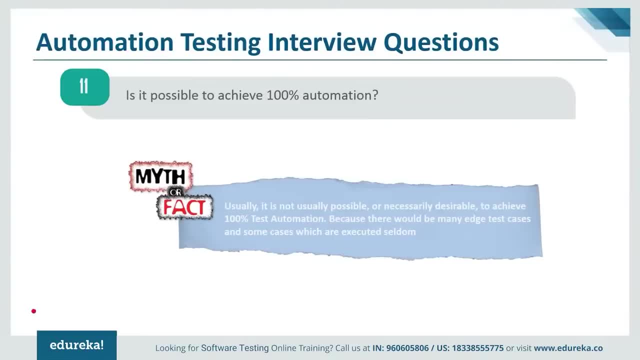 Why do you need to automate our use machines here to perform the task right? It's a waste of time and effort. just like that. while we were discussing the differences, We also discuss certain cases where you actually cannot use automation testing. So hundred percent automation is definitely not possible. 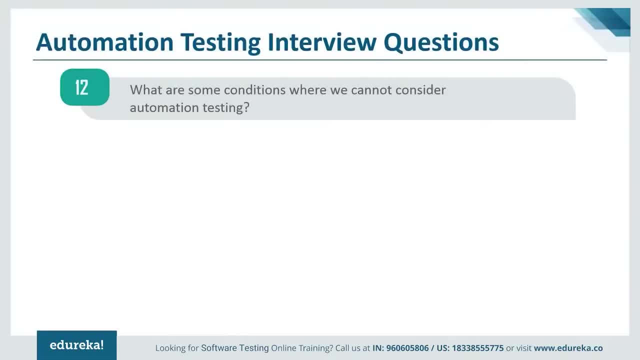 Next question: What are some conditions where we cannot consider automation testing? So just in case, just before discussing this question, we discussed a question where I said a hundred percent automation is not a possible thing. It means that there are certain cases where you cannot apply automation. 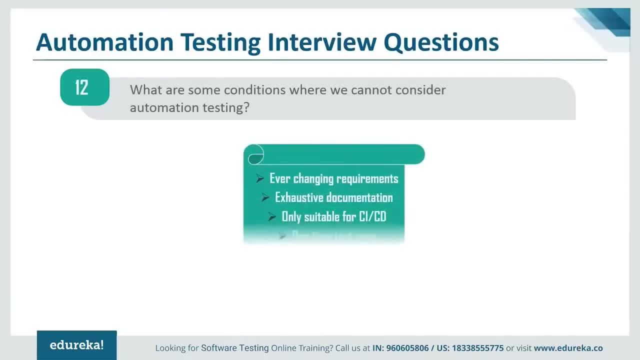 So what are those? So if you have a situation where the requirements of your software or an application keeps changing, in such cases automation becomes difficult because every time requirement change you need to change your test scripts as well, right? So it becomes difficult in such cases. 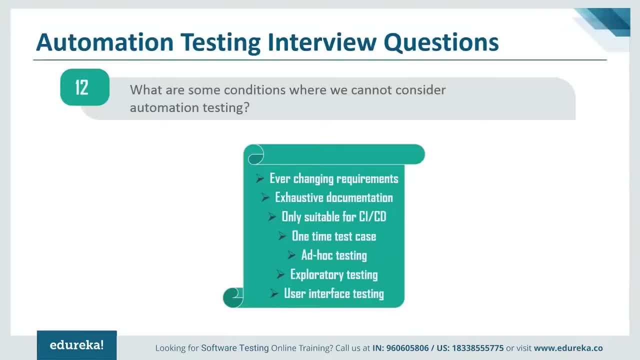 It's suggested not to use automation testing. similarly, if you have exhaustive documentation or if you have a requirement where you can apply only continuous integration at continuous delivery concept, then it's slightly difficult to apply automation testing. Then of the case is when you have one-time test cases. 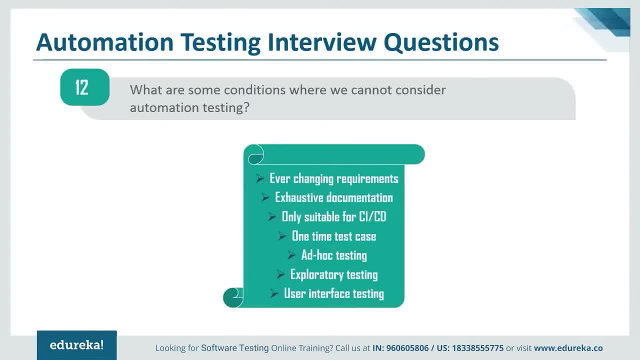 as in, you need to test these test cases only once. So what is the point of using automation? because it doesn't require much effort to test or test case only once, right? in such cases, Manual testing is much more preferred. apart from that, You also have ad hoc testing, exploratory testing. 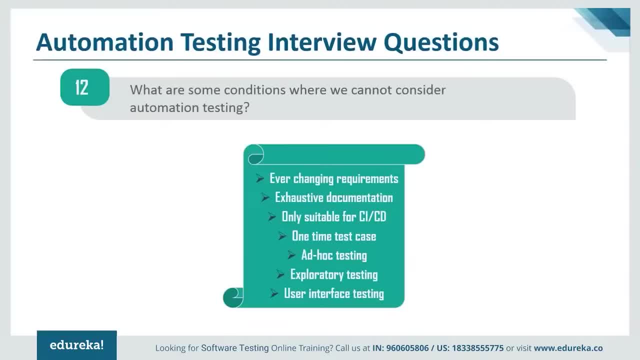 and user interface testing, So don't worry about them for now. We'll discuss what those three are as we progress. There's another question based on that, So for now I'm just going to list them and leave them like that. Here we go. 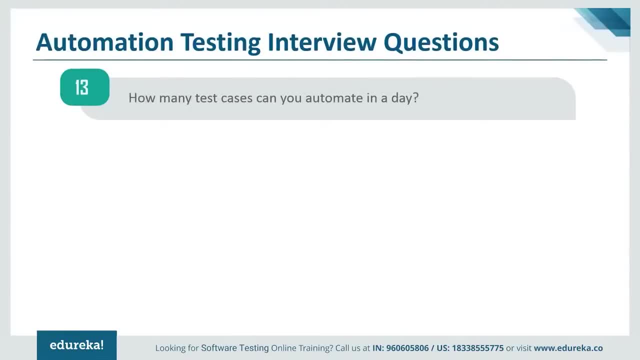 Our next question: How many text cases can you actually automate in a day? guys, It totally depends on test case scenario complexity and the design and the length. So, generally speaking, given the standard complexity of test cases, It's usually possible to automate a minimum of six test cases in a single day. 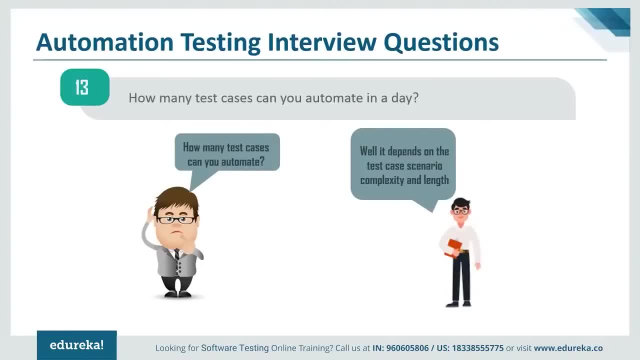 Well, this is for me. So when I perform testing, I realized that I could test six test cases in a day, depending on their complexity. But again, it depends on you. It depends on individual. If you are asked this question, you just have to talk based on your experience. 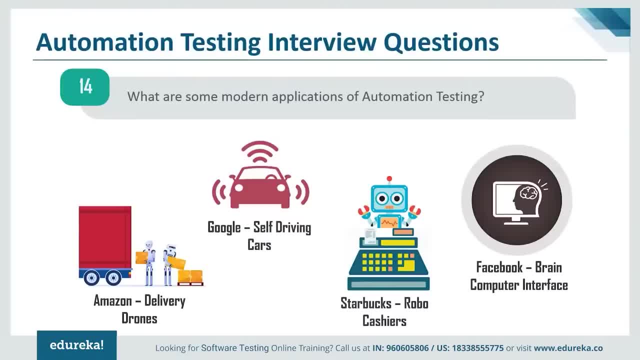 and the next question: What are some modern applications of automation testing? So, guys, like I said in the beginning, automation is literally everywhere. Every company is implementing automation and one or the other way. For example, Amazon is testing delivery drones that pick up warehouse orders, which are sorted by robots. 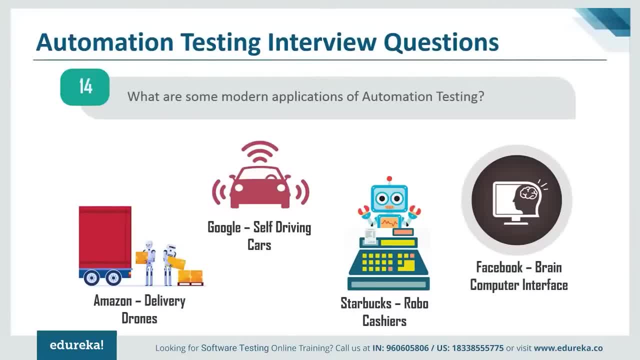 Whereas Google is testing self-driving cars. Then you have Starbucks, which is testing cashier free stores dedicated to mobile ordering and payment, and Facebook is testing a brain computer interface that may one day translate your thoughts into digital text. Well, these are some mundane versions of automation technology. 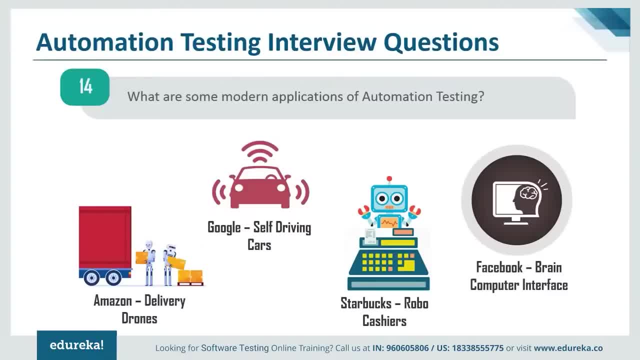 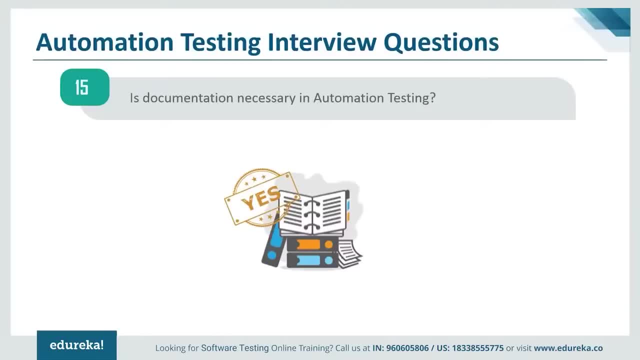 Apart from this, there are other innovative ideas that are coming up regarding automation. Fascinating, right, So let's move on to our next question: Is documentation actually necessary in automation testing? because documentation plays a critical role in test automation. So, whatever the practices that you follow while automation, 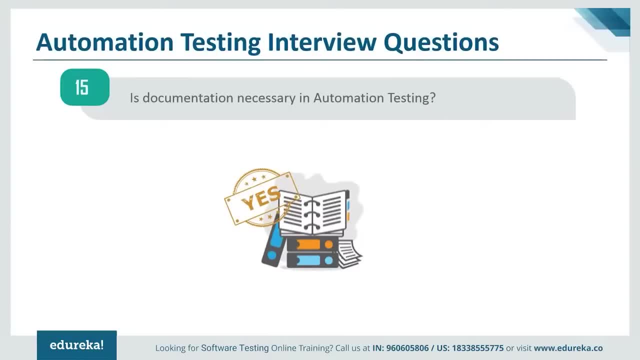 should be documented so that they are repeatable, as in you can refer to them later on. if they are documented somewhere like specifications, designs, configuration code changes, automation plan, test cases, bug reports, user manuals- all should be documented so that later on you have somewhere where you can refer to if you have forgotten. 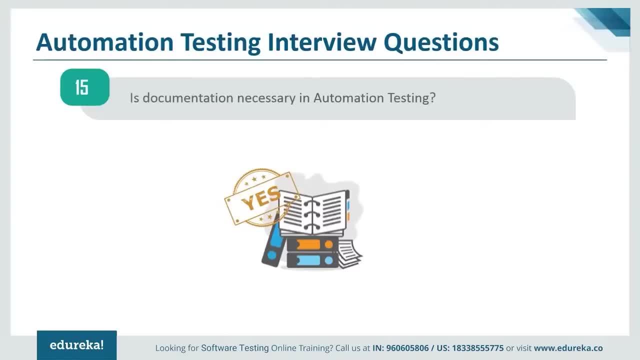 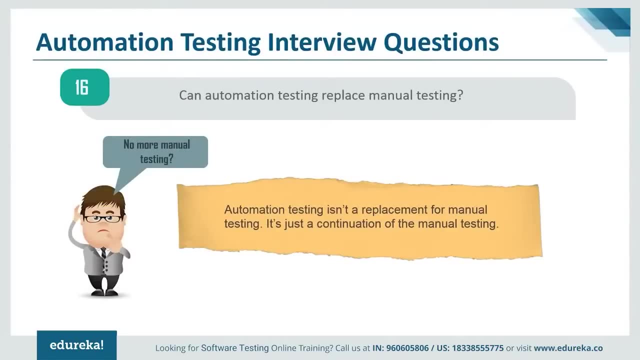 or, if you have made any mistake. this way, documentation plays a very important role in automation testing. So here goes one more tricky question that you might be asked, guys: can automation testing replace manual testing? Well, according to me, automation testing isn't a replacement for manual testing. 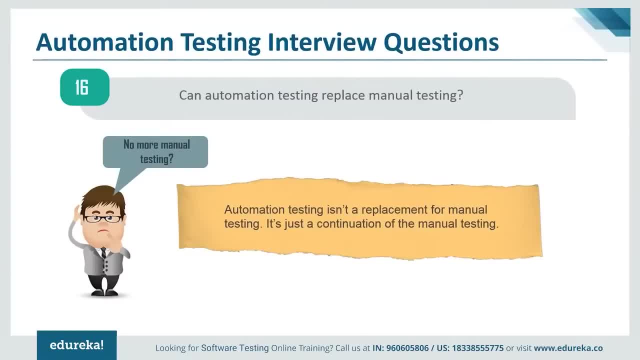 It's just a continuation of manual testing. So no matter how great automated tests are, you cannot automate everything right. We even discuss the cases where you cannot apply automation. manual test play important role in software development and come in handy whenever you cannot automated test cases automated. 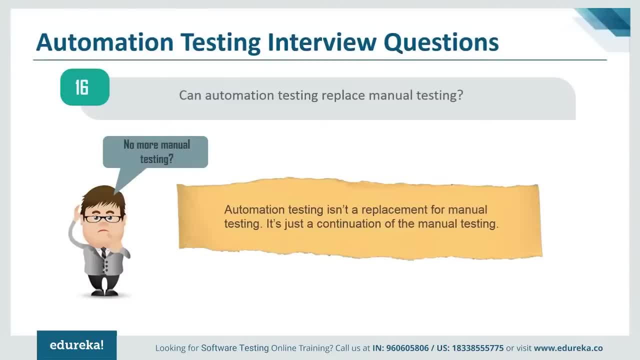 and manual testing. each of them have their strength and weaknesses. manual testing helps us understand the entire problem and explore other angles of test with more flexibility when compared to automation. but automation testing helps save time in long run by completing a large number of surface level test in very short period of time. 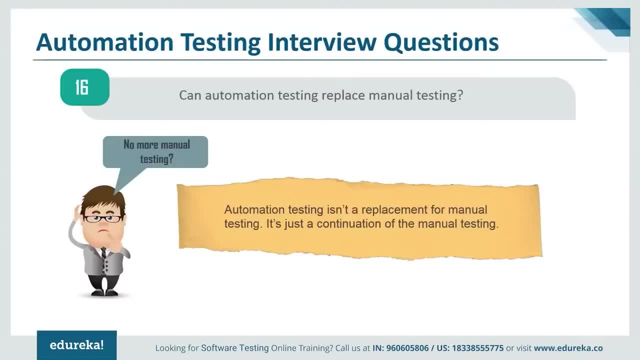 So what is automation testing? So what I want to stress here is that automation testing is actually not replacing manual testing. moving on to a next question: What are some popular automation testing tools that are used worldwide? So in the definition itself we have automation testing. 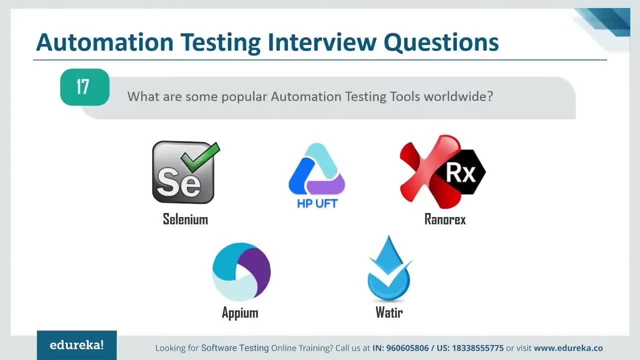 is process where it uses assistance of tools and scripts to perform testing, So obviously there are a whole lot of tools that can be used in automation for different purposes. Some of the most popular ones include selenium. It's a popular testing framework to perform web application testing across multiple browsers. 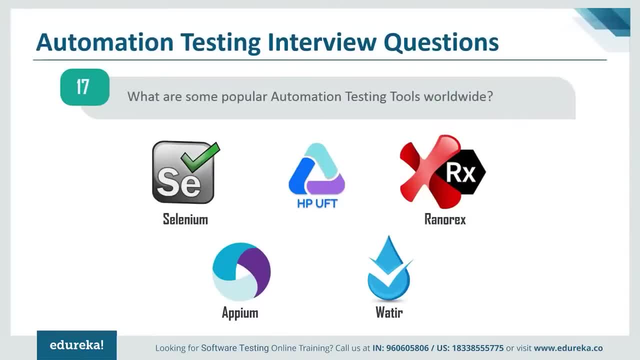 and platforms like Windows, Mac, Linux, you name it. Then you have water, which is pronounced as water. It's an open source testing tool made up of Ruby libraries to automate web application testing. Well, don't get confused with the spelling. 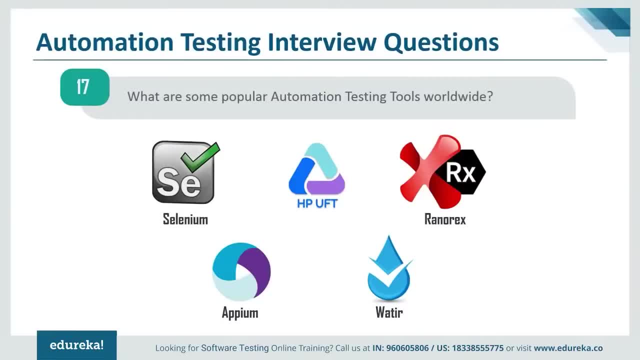 It's w-a-t-i-r but still it's pronounced as water. Then you have ranorex. It is flexible, all-in-one GUI testing tool which you can execute automated test flawlessly throughout all environments and devices. then you also have APM. 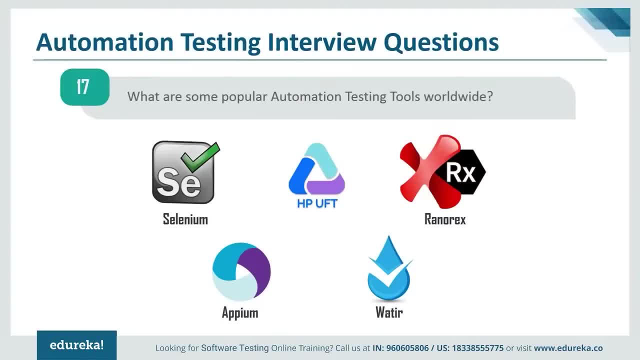 It's an open source mobile testing automation software. It's free and it supported highly active community of developers and experts. Well, these are just this creep, or I can say, very few, of the tools which I've listed here. There are multiple other tools. 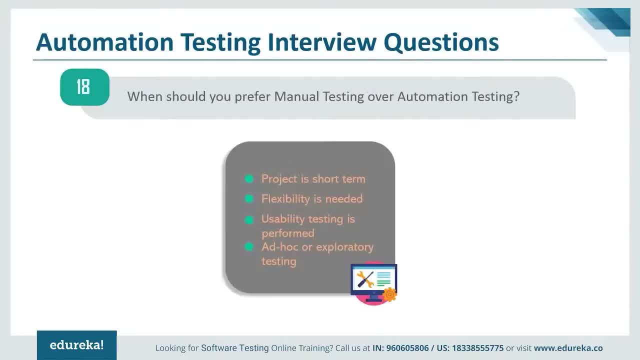 that are popular for different purposes. Our next question: when should you prefer manual testing over automation testing? Well, earlier we discussed when you cannot use automation testing. Now let's discuss when can you actually prefer manual testing over automation testing? First of all, when you have short-term projects. 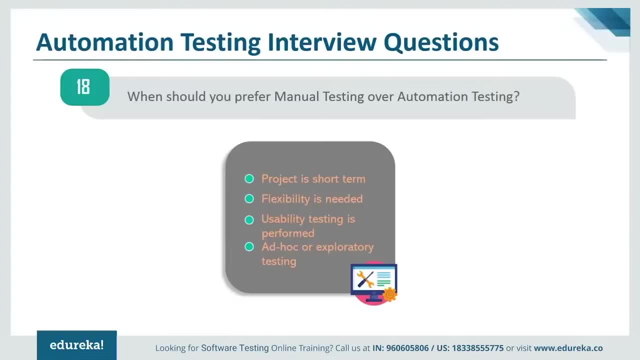 even the automated tests are aimed at saving a lot of time and resources, It still takes a lot of time and resources to design and maintain an automation test case or any such automation, So in some cases, such as building a small promotional website, it can be much more efficient to rely. 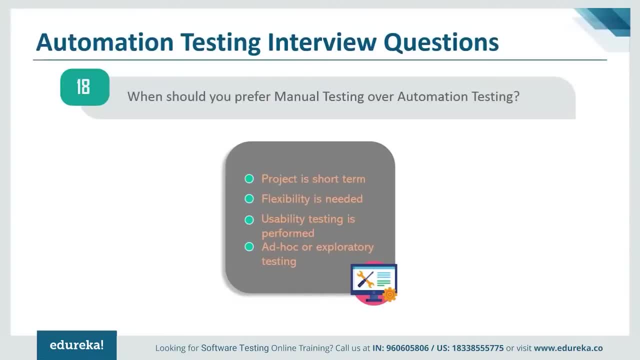 on manual testing rather than automation testing. It saves a lot of effort and time on your part. Other one is user testing. This is an area in which you need to measure how user-friendly, efficient and convenient the software or the product is for end users. 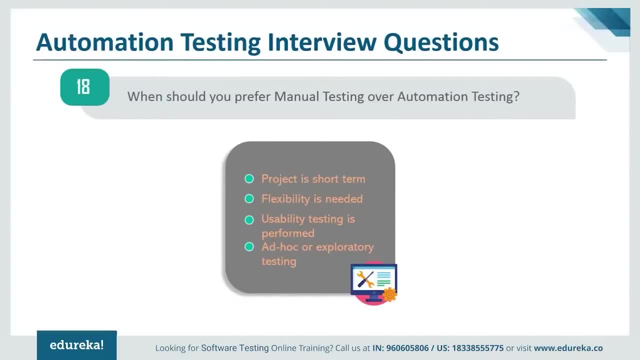 So basically, here you're representing an end user. Well, it's not possible by machines, right? Human observation is the most important factor, So manual approach is much preferable in that such cases. Then you have ad hoc testing. in this scenario, There's no specific approach. 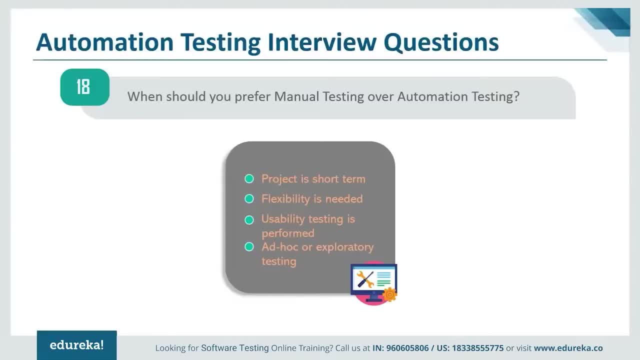 It's totally unplanned method of testing where the understanding in the inside of the tester is the important factor. So again, manual testing is much more preferable and ad hoc testing. apart from that, We also have exploratory test. this type of testing requires testers knowledge, experience, analytical. 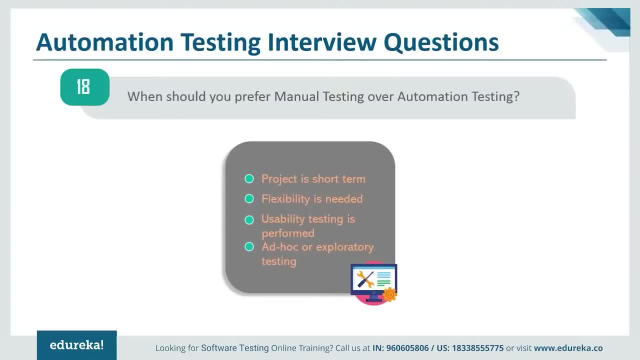 logical skills, creativity and intuition, and all that which is definitely not possible by machine. So yeah, even here manual testing is preferred. So we are done with the first set of questions, which are the basic questions that you might come across in the interviews. 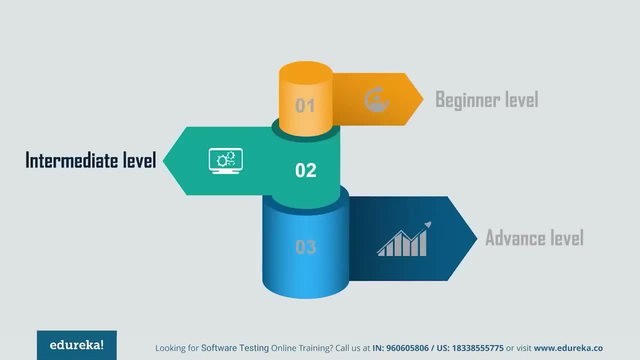 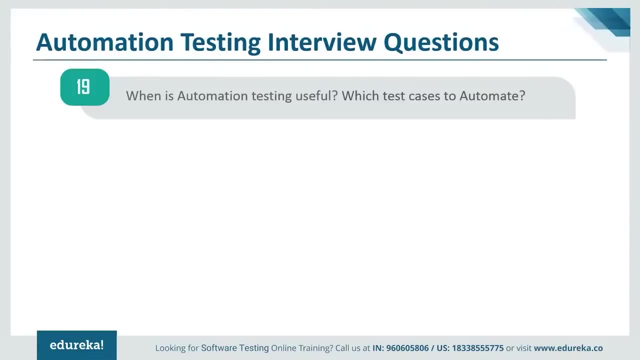 Now let's move on to the next level of questions, which I call it intermediate level. Here we go: When is automation testing useful? which test cases to automate? so, guys, like I said earlier, it's impossible to automate all testing, So it's important to determine which test cases. 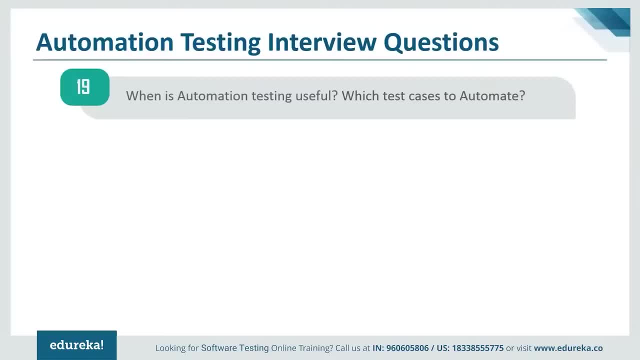 Should you actually automate? when it comes to figuring out where to start automation, There are some top candidates like. first of all, repetitive tasks are primary candidates for automation because if you are implementing manual testing here, it takes a lot of time and the task becomes boring. 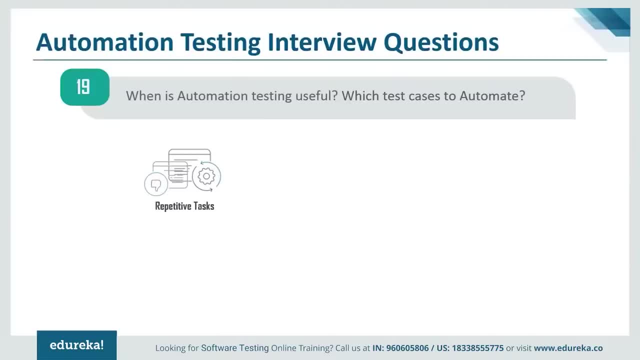 because when you do the same task again and again, it definitely becomes boring and you will make mistakes. So in the creative task, automation is much better. Then you have certain cases where you might have to capture results and share it with other people. So rather than manually exporting your data, crunching the numbers, 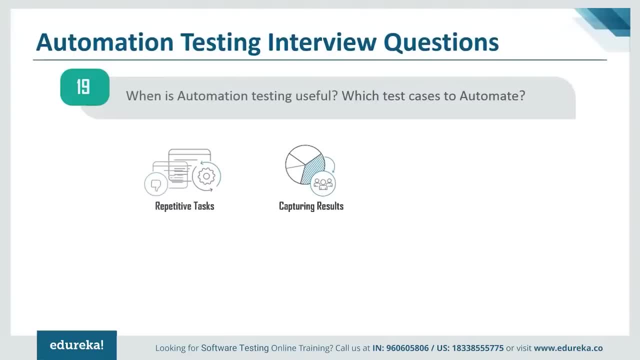 and making such pretty complex graphs. you can invest in a tool or automation strategy that will do this task for you. You can also use automation and the tasks that require multiple data sets, So, rather than manually typing an information into forms or fields, or automate this process. 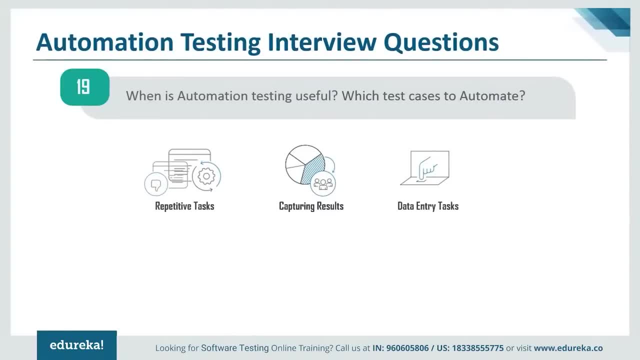 to read an information from a data source and automatically type into the respective forms. this way, Your time is saved. then you have certain cases where you have to screen the response as in how the interface is performing, or such cases. You do not have to just sit and stare at the screen. 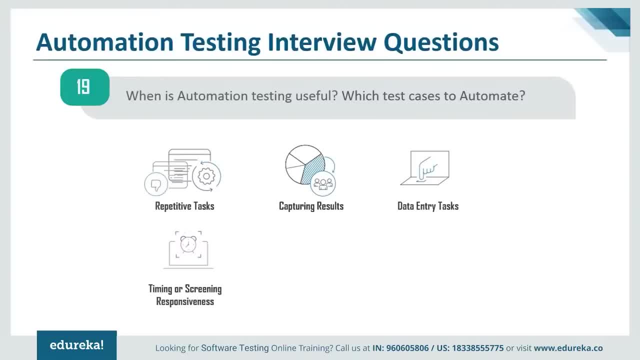 as in how the interface is behaving. You can just automate and look for the box later. Another example where you can apply automation is your non-functional testing types, For example load testing. suppose let's say you're testing a software and you are testing it. 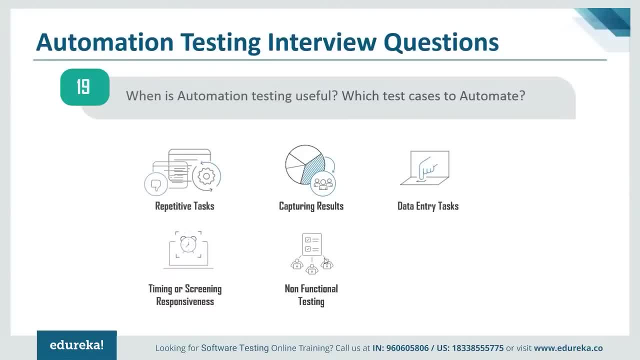 for some 10 cases, then manually it's preferable. But suppose if you have to test for 10,000 cases then it's better you use automation. and you can also use automations for the test cases that run on several different hardware or software platforms and configurations. 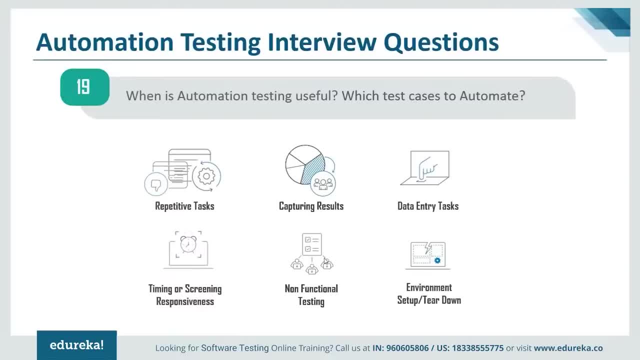 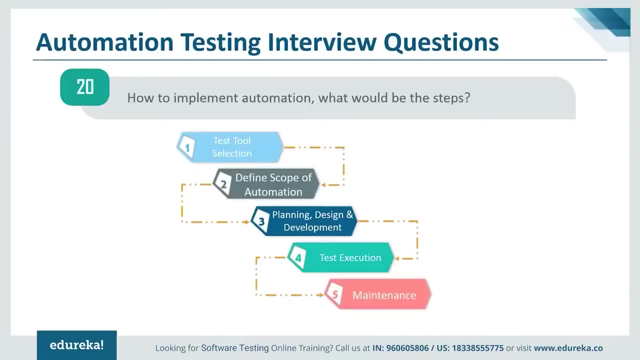 So, guys, these are certain test cases that you should consider for automation. Another important question, guys: How do you actually implement automation and what would be the steps that you need to follow? first of all, you should define your goal for automation testing and define which types of test cases are you going to automate. 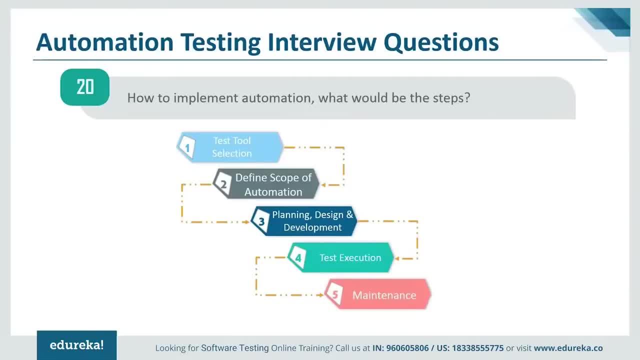 So once you're sure of what kind of test are you actually performing, you need to select the right, appropriate tool according to your requirements. Next, you define the scope of automation, as in you decide which test cases to automate, which not to automate, separate repetitive functions, and all that. 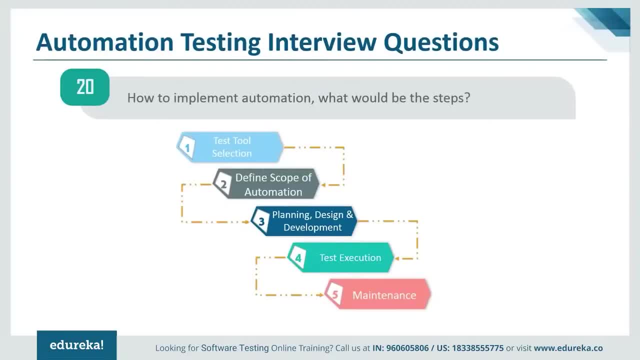 So, after determining your goal, defining the scope of automation and selecting the type of tool according to your requirements, You should start planning, designing and development. as in, you should start writing your test scripts So you create your test scripts and develop test suits to hold your test scripts. 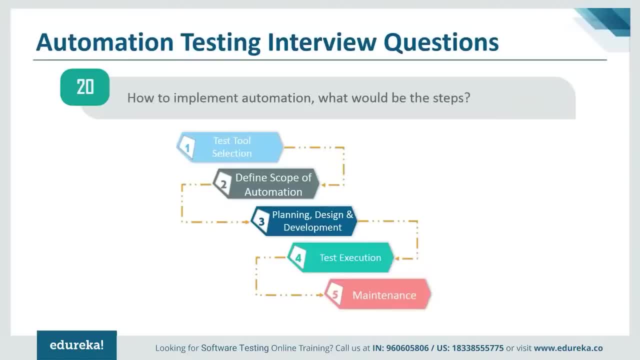 Next step is execution. You can execute the tests that you have written using an automation tool, directly or through test management tool, which will in turn evoke the in automation tool. So this way you can execute the test cases which you have written. The other important thing is: once you have done, 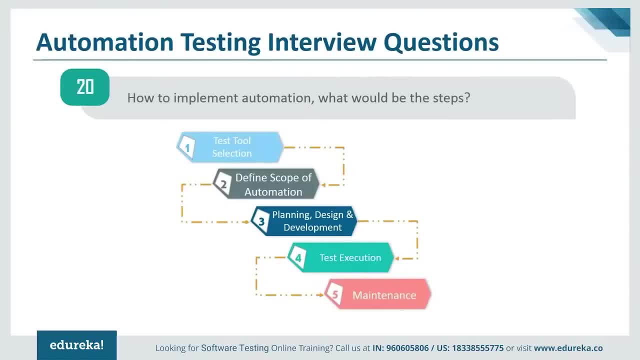 with your automation. the case doesn't end there. as you keep adding new features to your application or software, automation scripts also need to be added, reviewed and maintained for each release cycle, So maintenance also plays a very important role. It becomes necessary to improve the effectiveness. 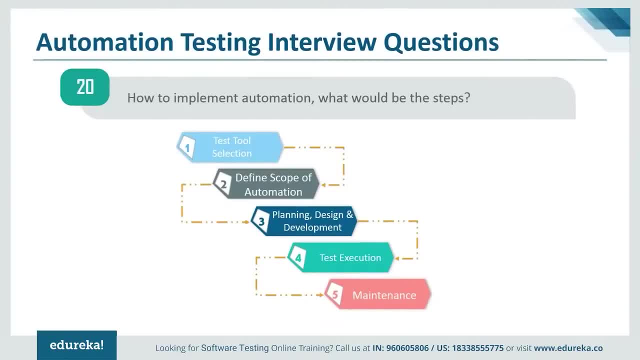 of your automation scripts. So these are the basic steps that you follow while implementing automation. So you need to know why you're actually performing automation. Then you select the right tool. Then you decide on which test cases to actually automate, based on all this requirement tool and which test cases. 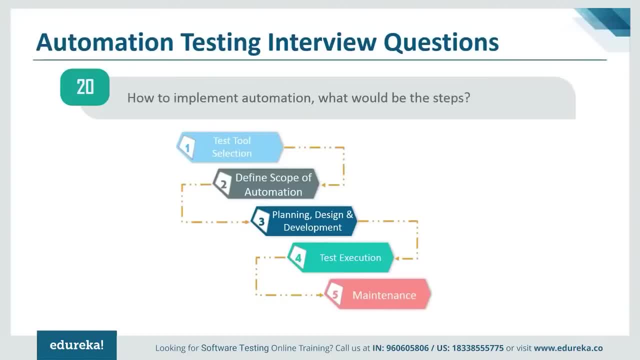 you need to develop a test script. Once your script is ready, you need to execute the test scripts, note down the results and, as soon as your application keeps changing, you can keep updating your automation scripts as well. So these are the steps that you follow. 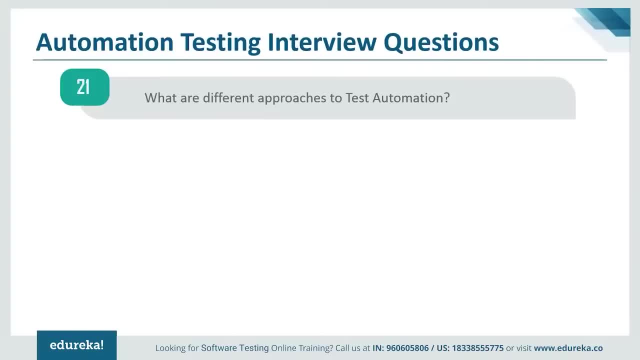 So, guys, here's another important question: What are different approaches that you can take to test automation? You have something called code-driven approach here. The focus is mainly on test case execution to find out if various sections of the code that you've written a performing as per expectations. 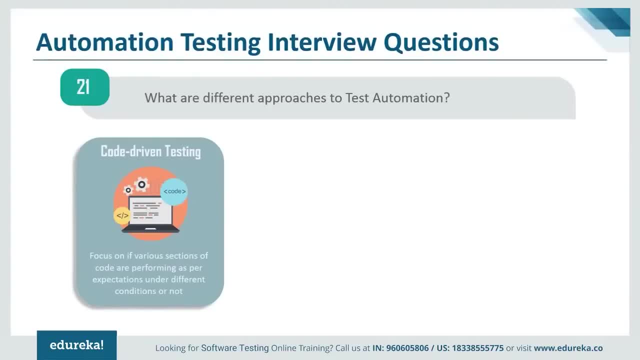 and the different conditions or not. So basically here you're checking if the application of the code that you've written to test the application is performing right or not under different conditions. Then you have graphical user interface testing, or GUI testing as we call it. 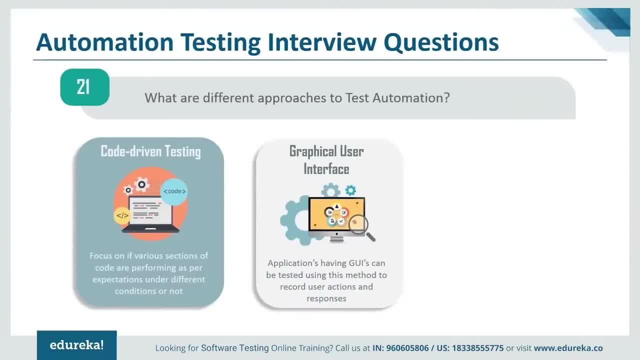 So applications that have graphical user interface may be tested using this approach. It allows the testers to record user actions and analyze them any number of times. For example, let's say you want to test a website. you can use framework like selenium that provides you with a record. 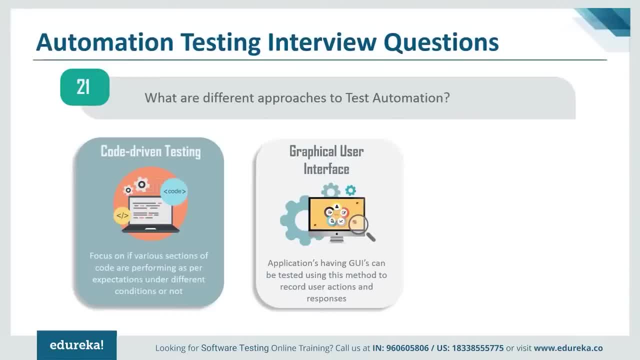 and playback tool using which you can authorize your test without having any knowledge of scripting language. So test cases here and graphical testing can be written in number of programming languages like C, sharp, Java, Pearl, Python and many others, and then you have test automation framework. We already discussed this. 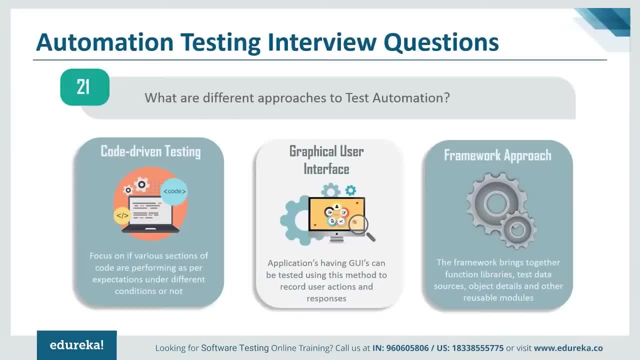 But anyway, framework is set of guidelines which are used to produce beneficial results of automated testing activity. The framework brings together function libraries, test data sources, project details and other reusable modules. Basically, it sets up a universal standard that all testers can actually follow. moving on to next question, 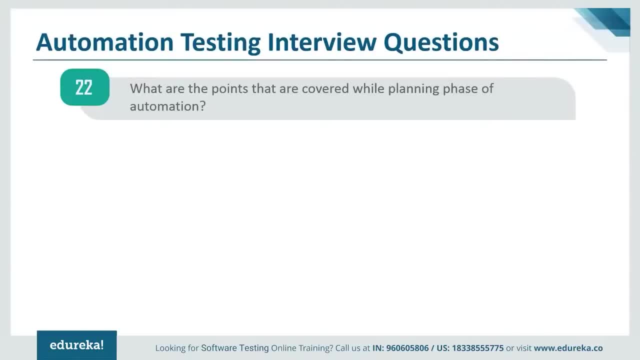 What are the points that are covered in the planning phase of automation? So earlier we discussed different set of steps that you need to follow while performing automation light and there's one phase called planning phase and the points that you have to keep track of in this phase. 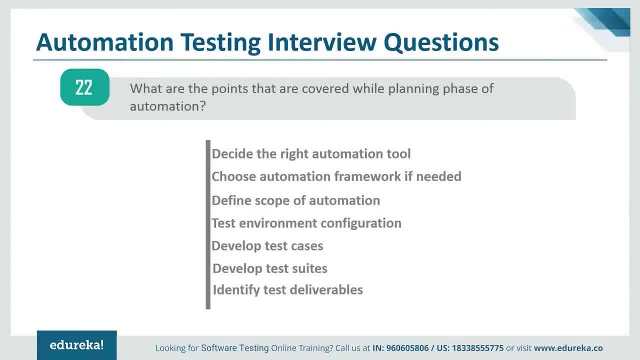 include deciding on the right automation tool, deciding if you want to actually use automation framework as the approach to automation or not, defining the scope of your automation, configuring your test environment- details develop in test cases, developing test suits and identifying test deliverables. So all these are the points that you should consider. 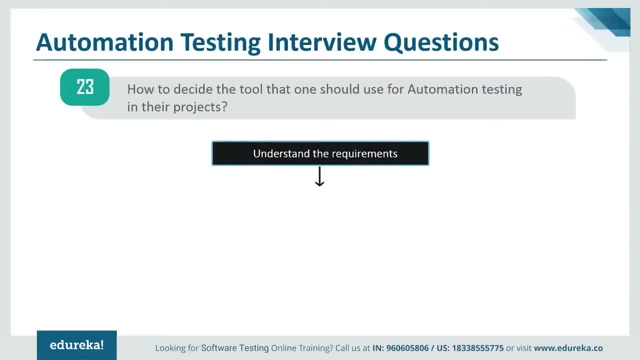 in the planning phase of automation. The next question: how to decide the tool that one should use for automation testing in their projects. So, guys, the first step in automation testing is to select a proper tool that suits your requirements. But how do you actually go ahead and select a tool? 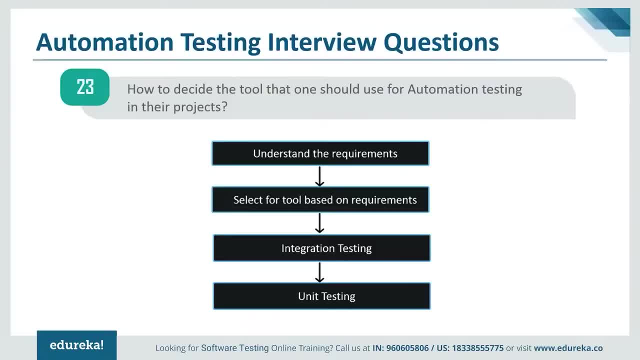 based on what criteria? first you need to know, you need to understand your project requirements thoroughly, and then you need to identify the testing scenarios that you actually want to automate. based on these requirements, you make a list of tools. Once you've made the list, for each tool, identify the budget. 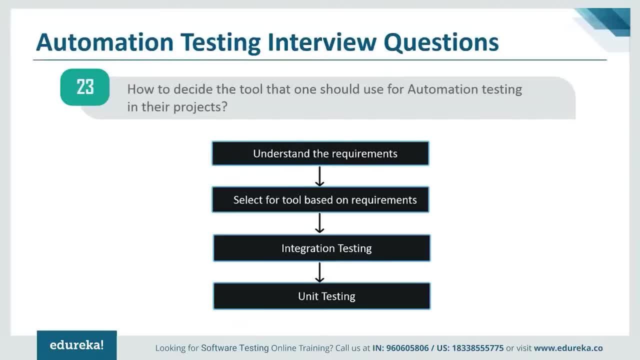 and select the tools which are within your budget. after that, compare the tools which are remaining in the list, using some criteria like: is it easy to develop and maintain the script for that tool or not? Does it work on platforms like web, mobile desktop and other platforms? is it based? 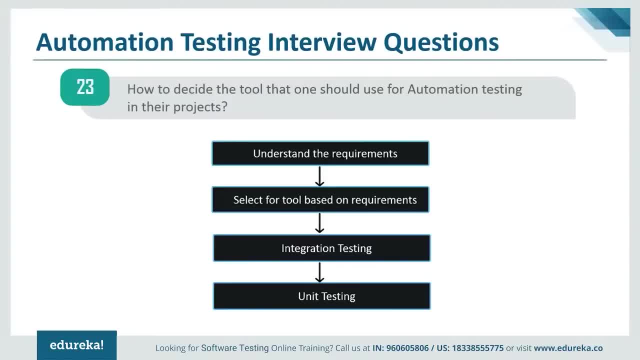 on your project requirements. does the tool have a test reporting functionality? how many different testing types can this tool support? how many other languages does the tool support? So, once you've compared different tools based on these criterias, select the tool which is within your budget and supports your project requirements. 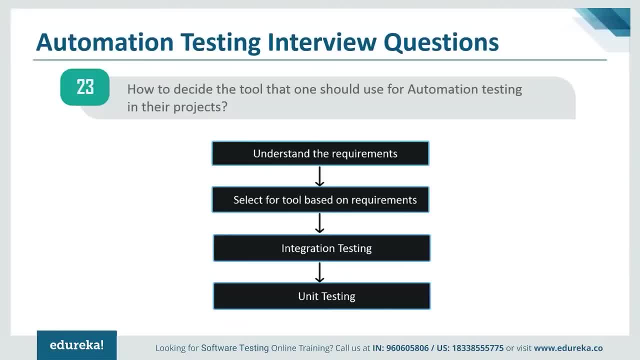 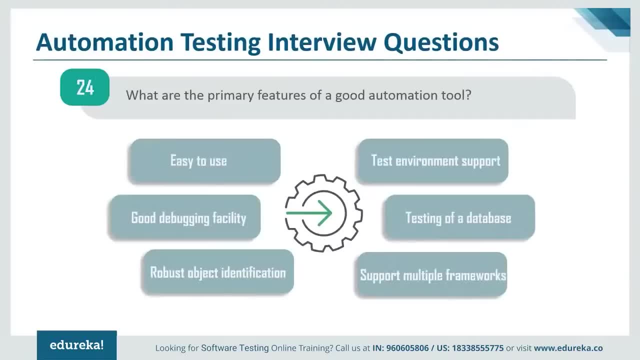 and gives you more advantage based on your key requirements. So that's how, actually, you select a tool which suits your requirement. guys, Now, what are the primary features of a good automation tool? first thing you need to consider is if or not the tool is easy to use. 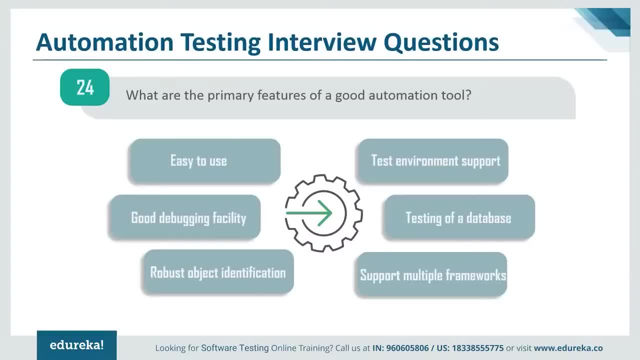 because if you choose a tool which is difficult to use, then there's no point in using automation. automation is implemented to make our task much easy so that we don't spend much effort on our part, right? So you need to select tool which is easy to use and understand. 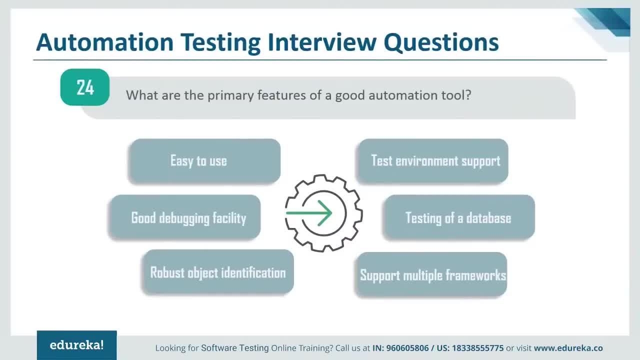 and you need to check if the tool is compatible with platforms and technology that you're using. it should also include features like implementing checkpoints to verify values, databases or key files, Functionalities of your application at definite points and also check if the tool does have a record and playback support apart. 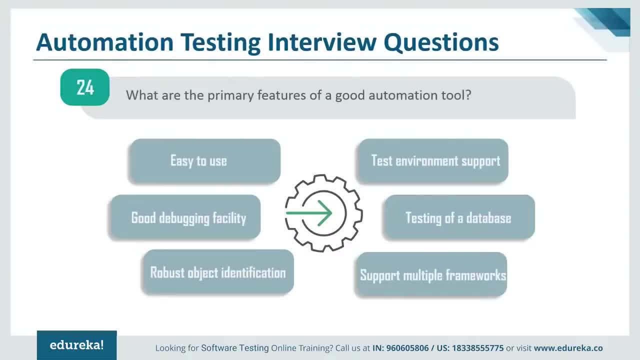 from these. it can also check if the tool has good debugging facility, robust object identification, object and image testing and all that. one more point: You can also see if the tools that you're using supports automation framework or not. So these are certain features that very good automation tool has. 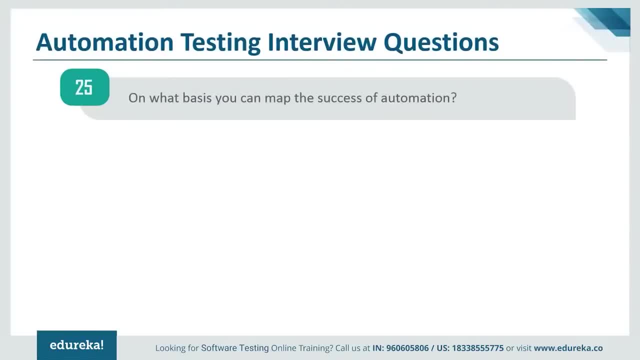 moving on to next question: on what basis you can map the success of automation? So on what basis can you actually decide if the automation is successful or not? We did discuss few points earlier, but let me just repeat them. The main points are the defect detection ratio. 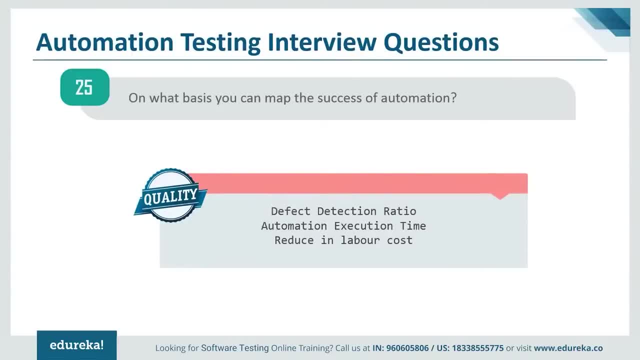 You can say the number of defects that you have found out after your automation. second, the amount of time that you've taken to execute the automation. and finally, the amount of reduction in the labor cost. These are the three key points or strategies or criterias that you should consider. 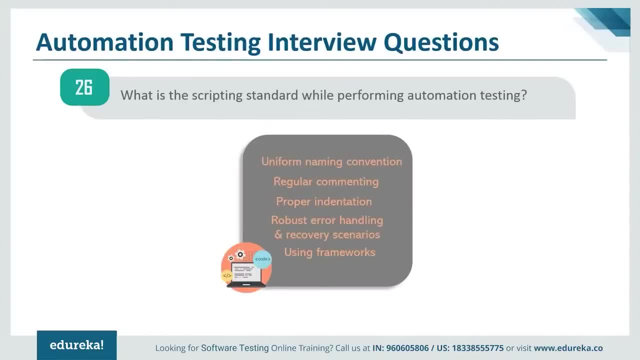 while evaluating the success of your automation. Now, what are the scripting standards that you should follow while performing automation testing? just like you have certain coding standards that you should follow, There are something called scripting standard that you should follow while writing your scripts, For example. 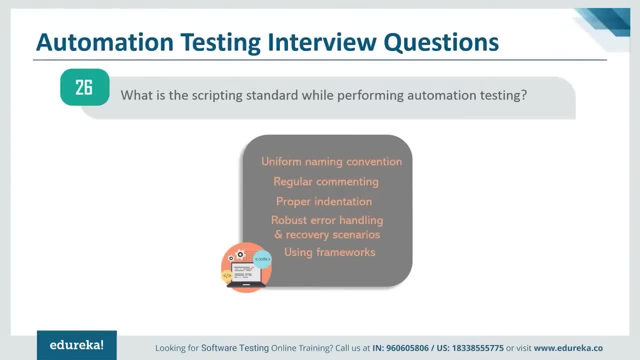 you need to maintain uniformity. naming convention, commenting the functionality whenever and wherever it's necessary. adequate indentation: indentation is really very important concept. It changes the meaning of your code entirely if you have done it in the wrong way. robust error handling and ability to recover, use of frameworks- and all this. 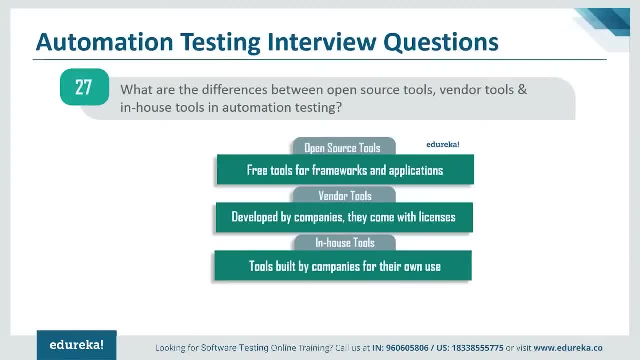 What are the differences between open source tools, vendor tools and in-house tools in automation testing? very simple guys. open source tools are free to use frameworks and applications. engineers build these tools and have the source code available for free on the internet for other engineers to use. so such tools. 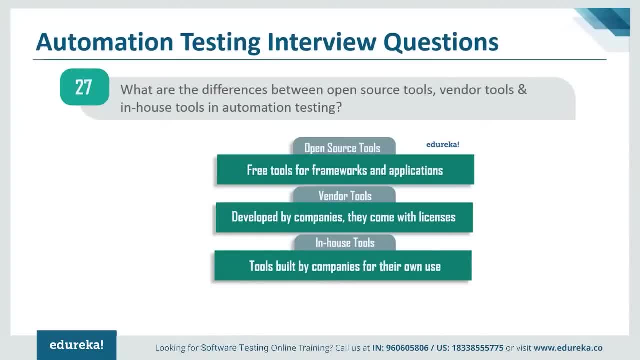 We call them open source tools. Then we have vendor tools. These are developed by companies that come with license to use, so they cost money very often. And because they're developed by an outside source, technical support is often available If you have employed the tool. better examples: 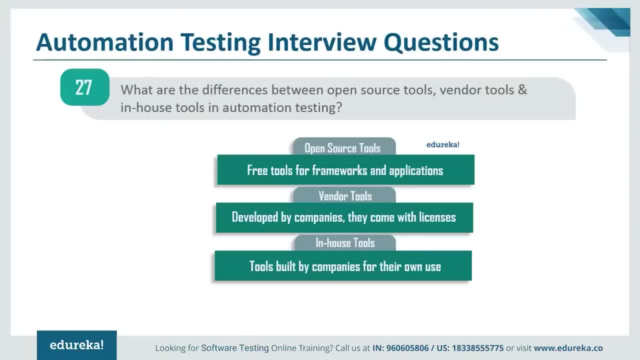 for vendor tools include win runner, silk test, rational robot, QA director, QTP, RPT and many others. and as for in-house tool, it is a tool that a company builds for their own use. rather than purchasing vendor tools or using open source tools, a company builds a tool. 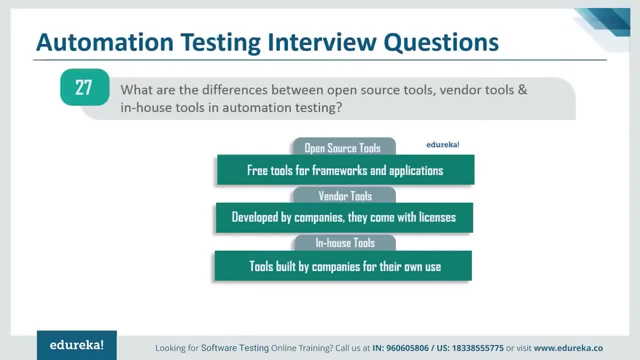 for its own purpose. those tools we called in-house tools- So open source tools- are free and available on internet. You can go ahead and use the source code. as for vendor tools, You need to have license to use and you often have to pay a lot. 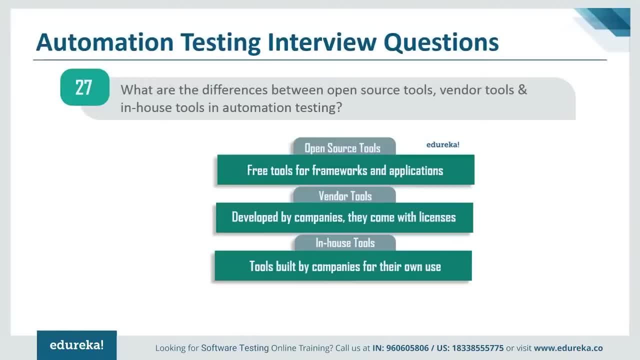 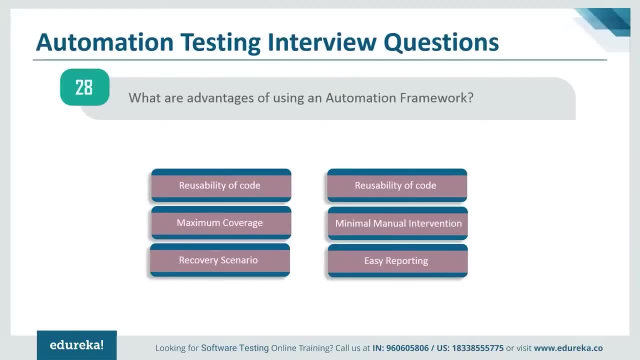 of money. then you have in-house tools, where companies build those tools for themselves for they use. moving on to next question: What are the advantages of using an automation framework? So here we go, guys. another important question about automation frameworks. So what are the advantages of using framework? 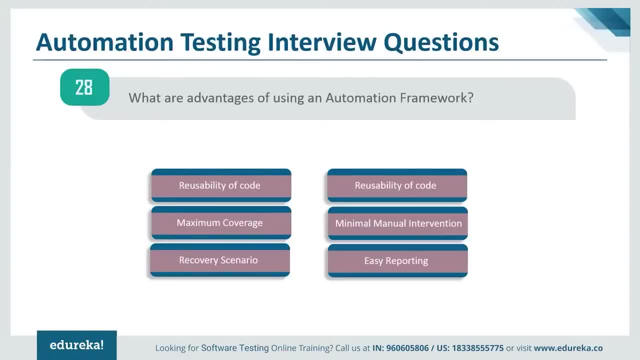 First of all, they save you a lot of time. You can reuse the code any number of times and they offer you maximum test case coverage automation framework. They come with a proper recovery scenario and debugging facilities and obviously minimal manual intervention as well, and they also provide you with easy reporting features. 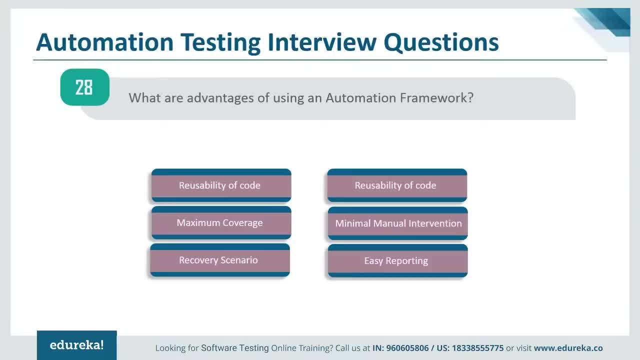 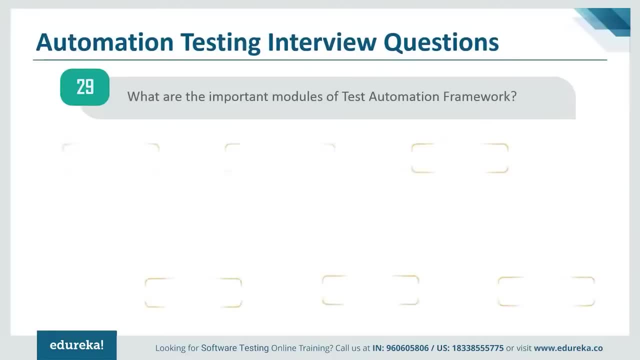 as in our. once you're done with automation, you can easily create reports and share it with other people in your company. So these are some advantages of using automation framework. Next question: What are the important modules of test automation framework? Every test automation framework? 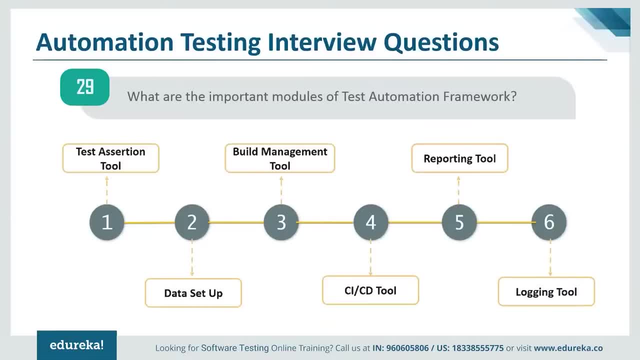 has some important modules. For example, you have test assertion tool. This tool will provide a search statements for testing the expected values in application which is under test- an example for test assertion tool. You have test NG J unit and many others. Then you have something called data setup. 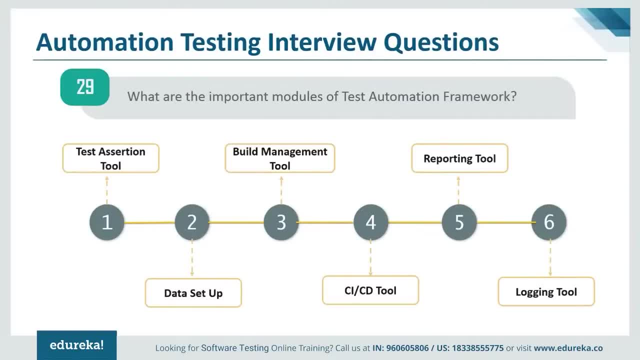 So whenever you have written a test script, the test script works on some sort of data right And you need to actually take the data or you need to have a source of data. So each test case needs to take the user data, either from the database. 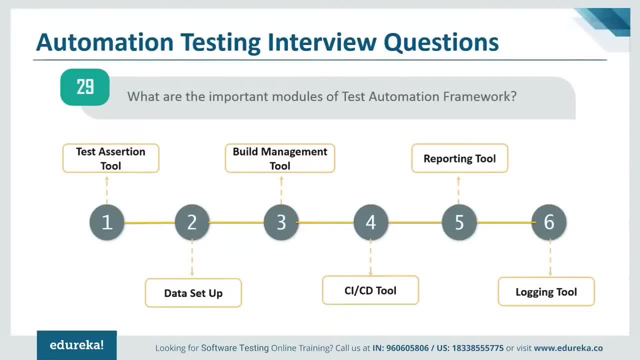 or from a file or embedded in a test script. to manage all this, We have a module called data setup. then comes build management tool. using this tool, You can actually manage how to build your framework according to your requirement. this way, You can easily write your test scripts and manage them. 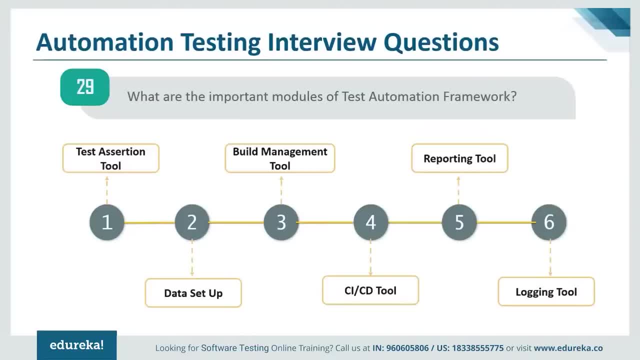 Then you have continuous integration tool or CI CD tool. These tools are required for integrating and deploying the changes which are done in framework at every iteration. Then you have reporting tool. a reporting tool is required to generate readable report after the test cases are executed. 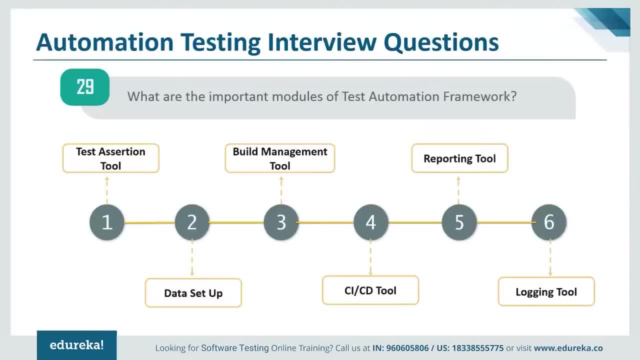 This way you get better view of the steps, results and the failures of your automation. And lastly, we have something called logging tool. The logging tool and framework actually helps in better debugging of error and bugs. So if you have the log of whatever you have done, 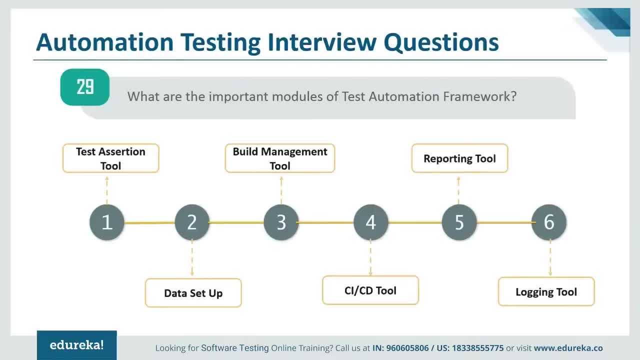 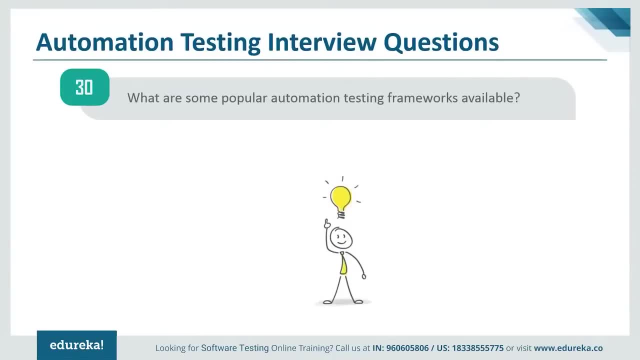 throughout the course of your automation, it will be easier for you to find out that bugs and debug them. Here comes our next question: What are some popular automation tests and frameworks available? So let me list out few popular framework testing frameworks. Well, to name the most important ones, 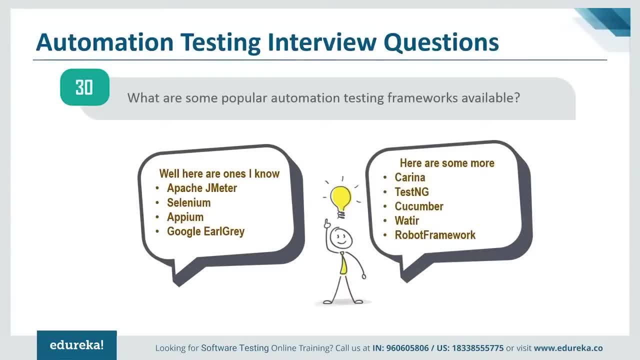 I have Apache, G meter, selenium, Appium, Google or gray. apart from this, you also have test energy, cucumber, water robot framework and many others. make sure you go ahead and refer to other lists on internet so that you will remember many names as possible. So as what I meant to say is there are other popular frameworks. 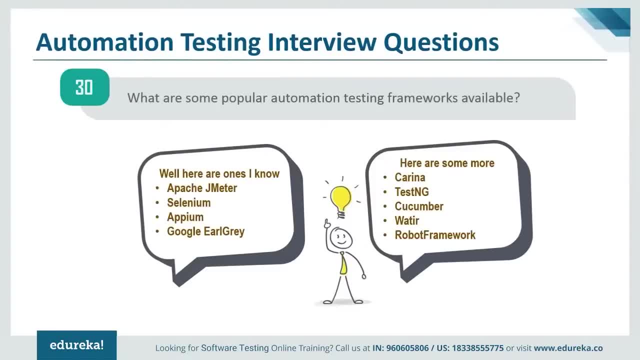 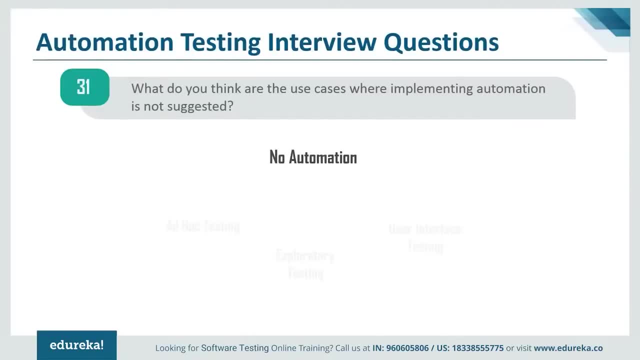 as well, apart from the just once which are just listed. now, moving on to the next question: What do you think are the use cases where implementing automation is actually not suggested? Well, we already discussed this, but let's go a little deeper. One of the key testing principles is: 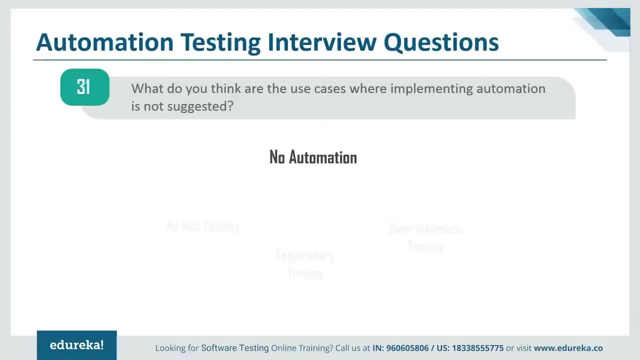 that 100% test automation is definitely not possible, but discuss this as well. So manual testing is still necessary. Let's see which test cases cannot be automated, or I could say would take too much effort to actually automate. We did discuss about test cases. 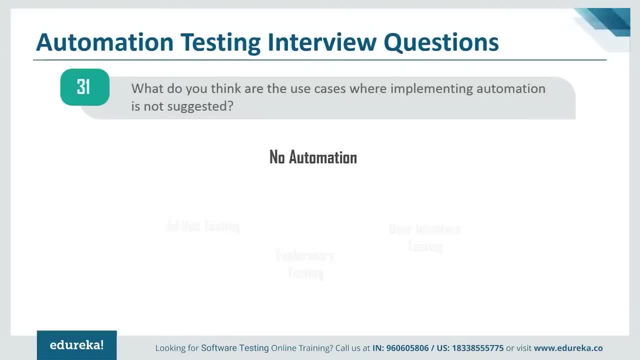 which you need to execute only once, when you have exhaustive level of documentation. and all that apart from this, I listed out three other cases, if you remember, which is ad hoc, exploratory and user interface testing. Let me explain these three concepts to you guys. So, first of all, you have ad hoc testing here. testing is done. 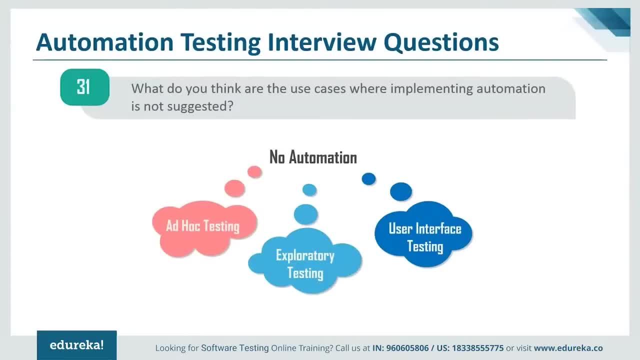 without actual preparation and you do not have any written test cases. So during ad hoc testing, a specialist randomly test the functionality of system. basically, his goal or his aim is to be creative And break the system and discover flaws, which might be not possible when you're actually using a machine. 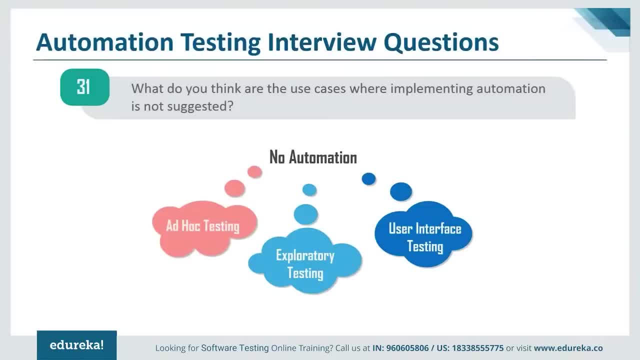 I mean in case of automation. So in such cases it's better to use manual testing rather than automation testing. Then we have something called exploratory testing. during exploratory testing, a specialist or a tester tests a product like an Explorer, as in. he relays on his personal experience. 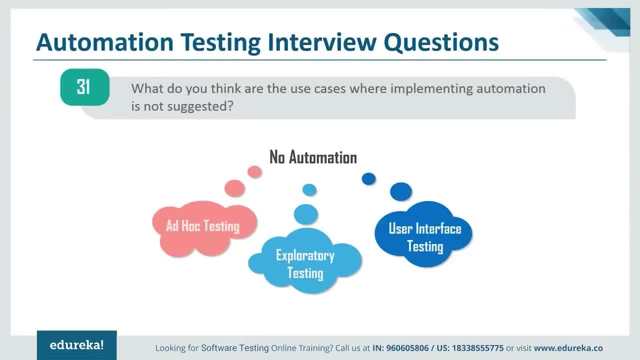 after getting the full picture of products functionality, He designs test cases which he seems right. So in exploratory testing you have to rely on your personal experience and design test cases. So it's definitely not suggested you to use automation testing here. Then comes user interface testing, one problem. 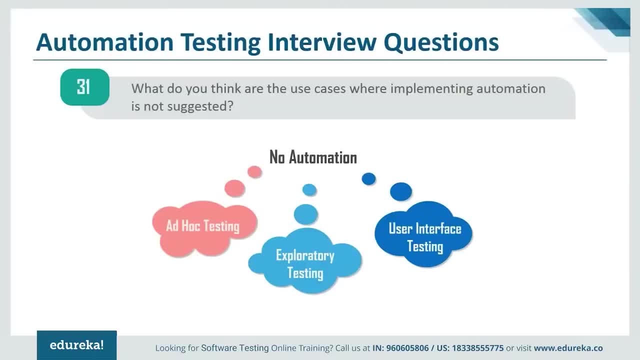 with user interfaces is that the requirements for user interface keep changing. Well, like I said earlier, it's not suggested to use automation when the user requirements keep changing, because you might have to change your automation script again and again, which will be a hard task. 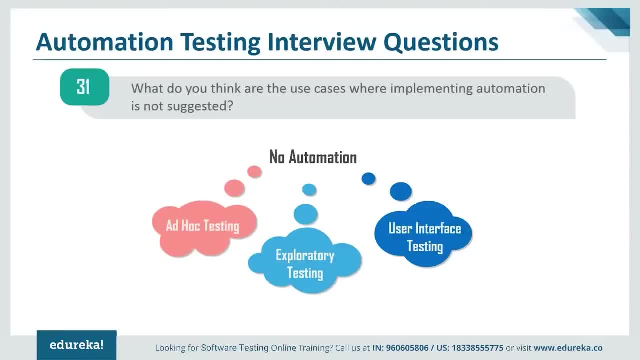 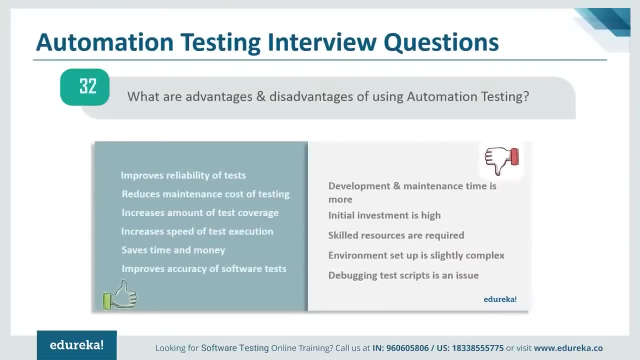 So, although we could automate basically everything, manual testing still provides an effective and quality check of bugs and inappropriate in some situations. Now, what are the advantages and disadvantages of using automation testing? Well, after listening so much about automation testing, I'm sure you guys can list it out. 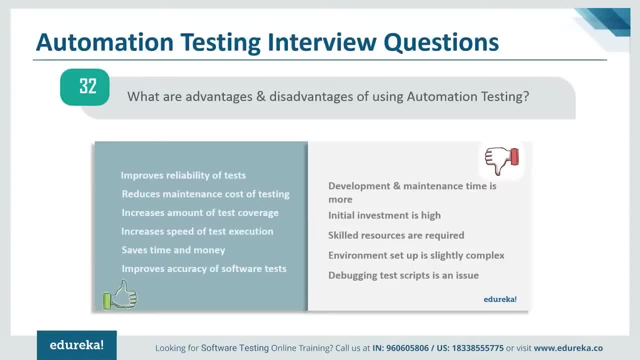 So automation test is: simplify the test case execution. They save a lot of time and money on you part. They improve the accuracy and reliability of your software test. They increase the amount of test coverage. also the speed of test execution as well. They reduce the maintenance cost. 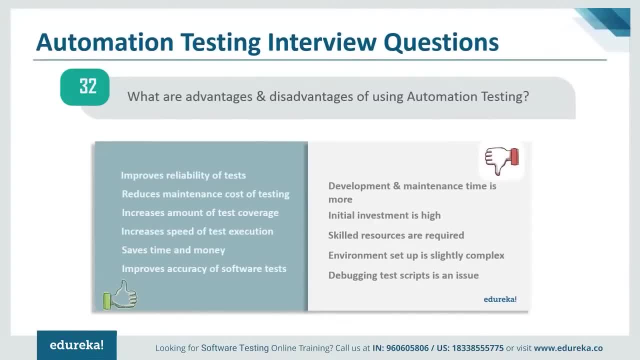 and they give you a high return of invest in case of long run. Talking about disadvantages, maintaining developing test cases is little difficult. initial investment is high. You need to have skilled resources. this way, They can actually make proper use of the automation tool that you're implementing. your environment setup is 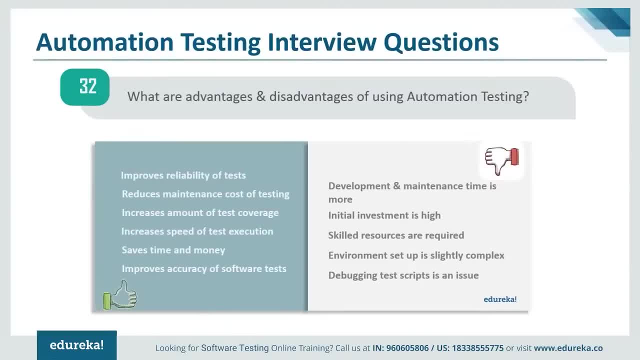 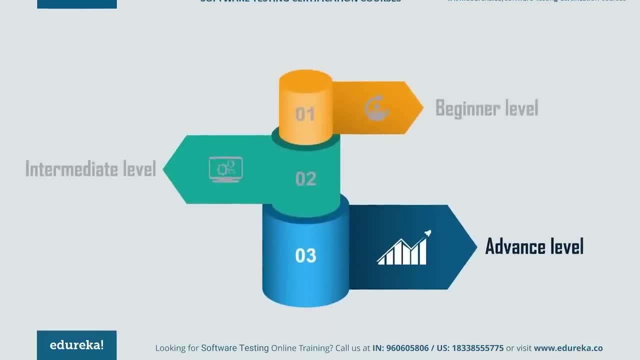 a little complex, while automation debugging test script is also an issue sometimes. So these are certain advantages and disadvantages of using automation testing. So, guys, here we're done with the intermediate level questions, and then we have advanced level questions. meant when I say advanced doesn't mean 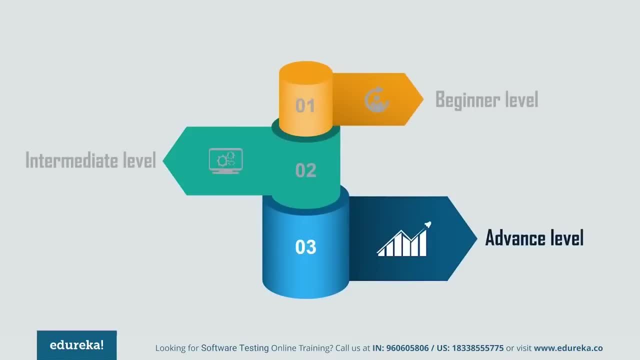 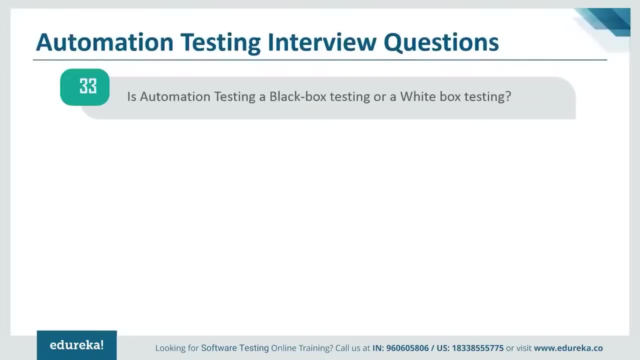 they have very long answer or something like that. It's just that they're little tricky and you need to have proper knowledge to answer these questions, or in-depth knowledge to answer these questions. So let's continue. So the first question in advanced level is: is automation testing? 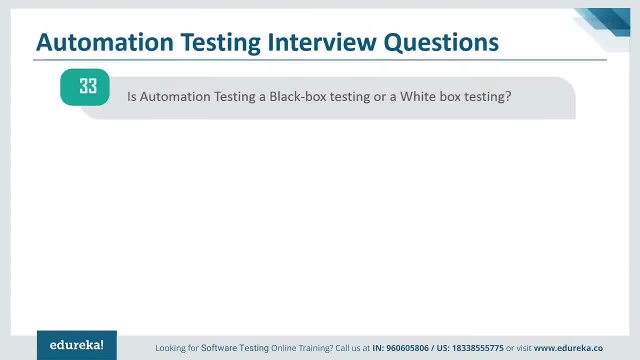 a black box testing or a white box testing? before I go ahead and answer this question, Let me explain you what black box testing is, and white box testing is first about black box testing. here, in black box testing, internal structure, design, implementation of any software product or an application or user interface. 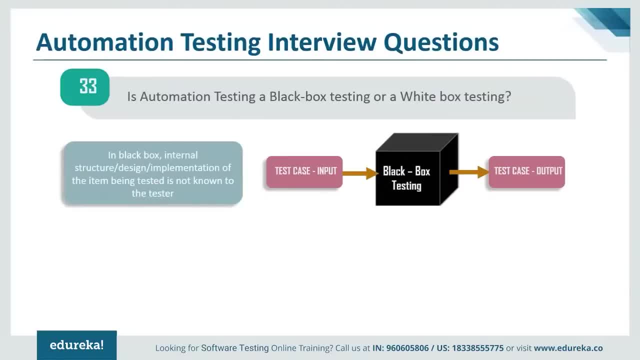 that you're testing on. the user will not know any of these details prior to testing in black box testing, but when it comes to white box testing, details like structure, design, implementation and all this the user will know about. So, basically, black box testing you are actually performing. 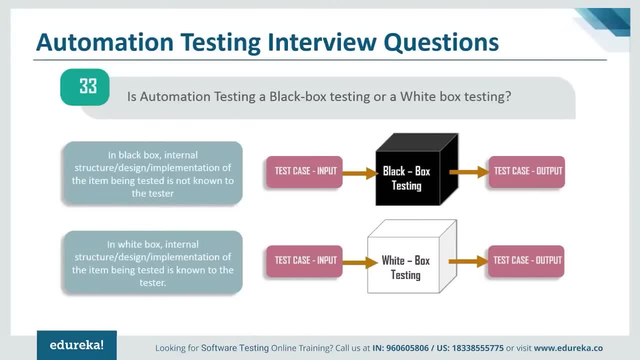 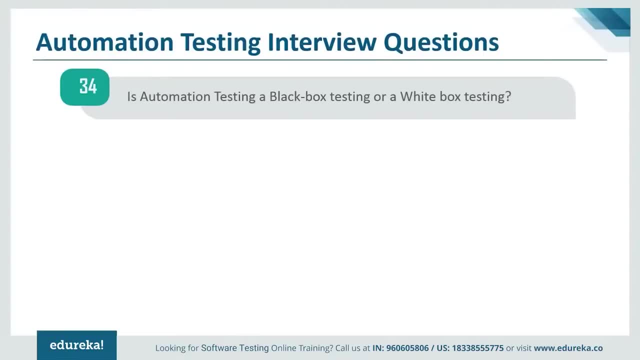 test without any prior knowledge, Whereas in white box testing you do have certain idea of what actually you performing tests on. so now is automation testing a black box or a white box testing? guys, automation testing is mostly a black box testing, as we just program the steps that a manual tester usually does. 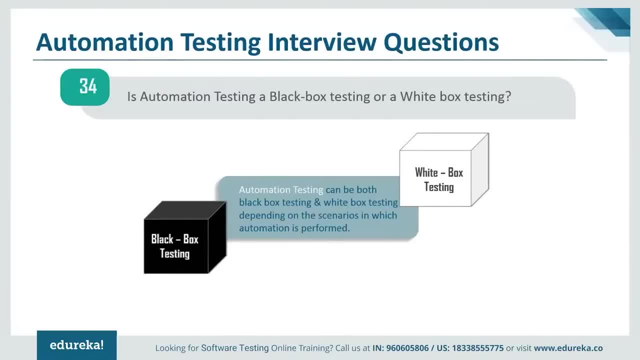 without any prior knowledge of application. but sometimes automated test scripts need access to database details as well, which are used in the application. in that case it again becomes a white box testing. so automation testing can be both black box or white box, depending on the scenarios. 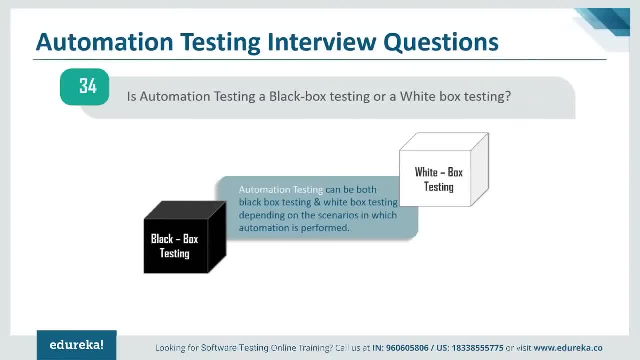 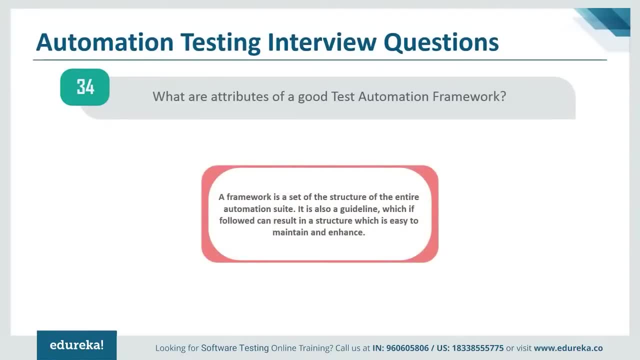 in which automation is actually performed. moving on to our next question, What are the attributes of a good test automation framework, or test automation framework which is considered to be good? should be modular, as in it. should be adaptable to change. tester should be able to modify the script as per the requirements. next, 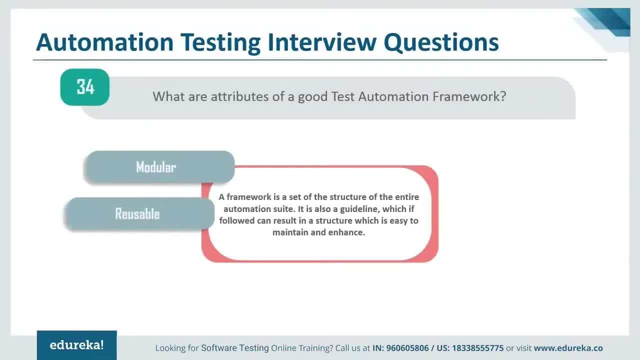 It should be reusable. Suppose, if you have any methods or functions which you want to reuse, make sure you put them in a separate file so that you can access them later, and your framework should support this feature. next important feature is it should be consistent, the suit. 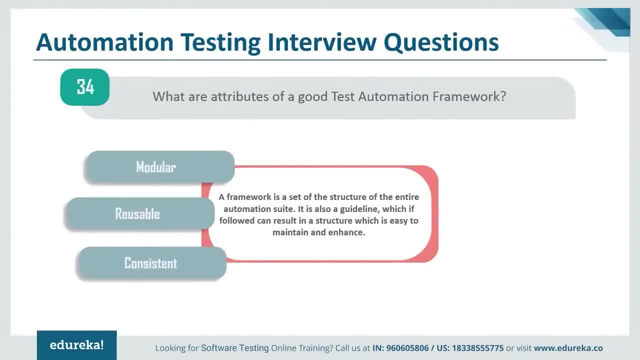 that you're developing for your framework should be written in a consistent format by following all the coding practices and the scripting practices which we discussed earlier. then obviously independent. the test script should be written in such a way that they are independent of each other, So in case of one test fails. 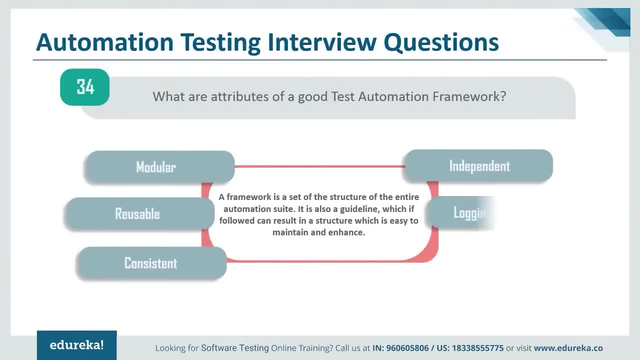 it should not hold back the remaining test cases. Then you have a lot of logging feature, as in your automation framework should have a login and reporting feature. Like I said earlier, logging feature helps you to find the bugs in the earlier stage itself and easily debug those books. 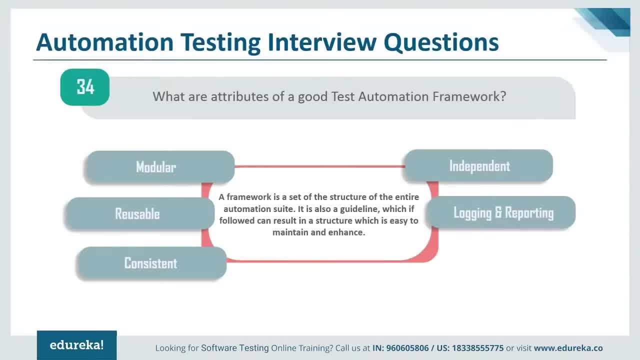 For example, let's say, if the script fails at any point of time, having the log file will help you detect the location along with the type of error that you're actually encountering here. Similarly, it should also have a reporting feature. It's good to have a reporting feature. 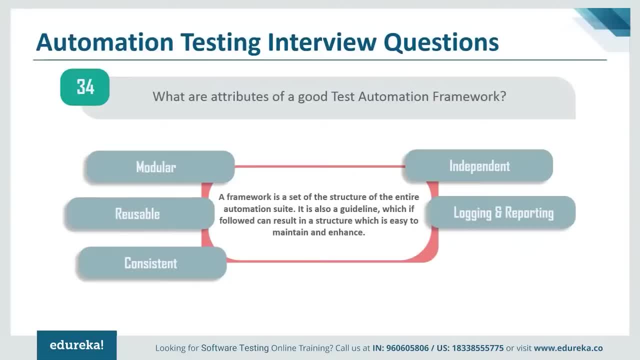 So once the scripting is done, we can have the results and report sent via email. Lastly, it should also support integration. automation framework should be such a way that it's easy to integrate with other applications like CI, CD. So these are some features that a good test automation framework. 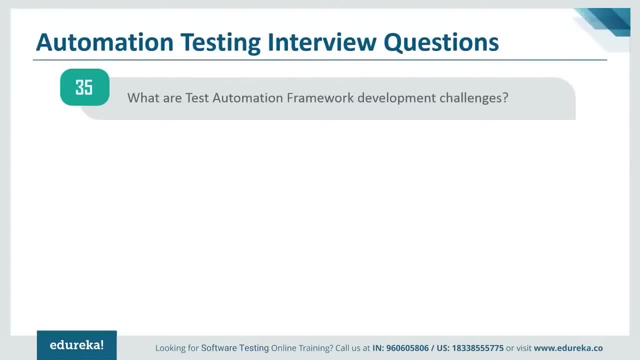 must and should have. moving on to next question: What are test automation framework development challenges? Obviously, while developing a framework, you will come across certain challenges. first of all, setting the scope of automation might be a difficult task. that is, you need to know properly which test cases to actually automate. 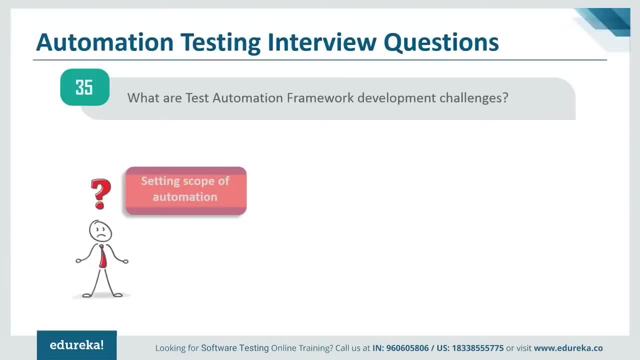 and where to use automation framework, If or not you should use your automation framework for such test cases. So deciding on that part is little difficult. then identifying the requirements of your test case is also a difficult part, because, since your application or software keeps changing, you need 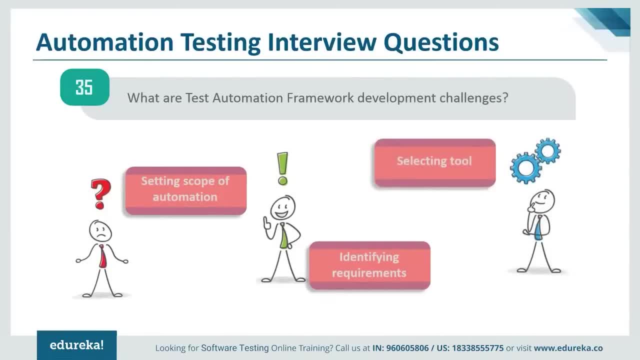 to be aware of your requirements. Lastly, selecting the tool. There are a plethora of tools out there, So choosing a tool out of them which suits your requirement will be difficult. So in such cases, you can follow the rules which we discussed earlier or the steps to select a proper, appropriate tool. 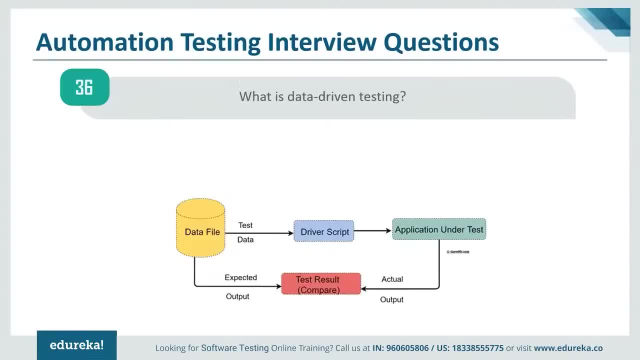 which suits your requirement. moving on to next question: What is data-driven testing? If you remember, this is a type of automation framework we discussed. So major use of automation testing is to simplify the testing process, which involves complex and huge data sets, by documenting the same details. 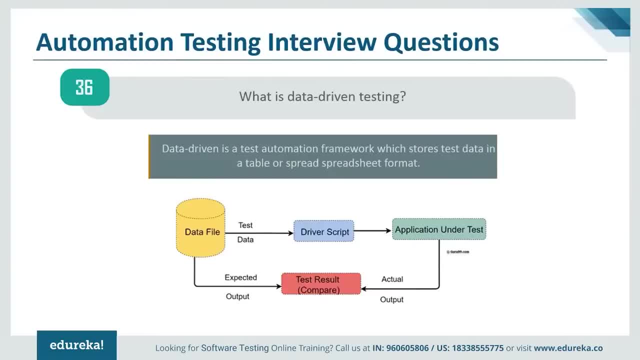 as in data-driven test, is used when you have large or huge amount of data sets that you have to deal with while testing. So in data-driven testing framework, the test data includes input files, output files and the result field, and these fields are included in files. 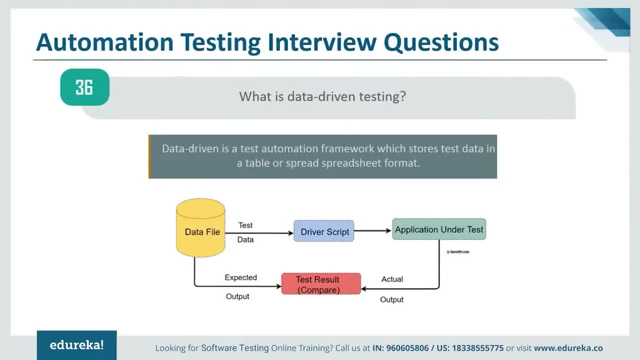 like CSV, Excel sheets, XML files, etc. So once you have all the test data in these files, these files are fed to an automation tool for execution which in turn compares the expected and the actual data. then it documents the result of each test data into resulting field in those files. 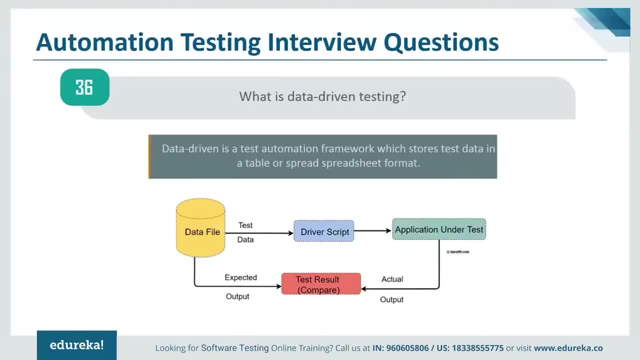 So that's what data-driven testing is all about. as you can see, you have a data file and you have an expected output which is compared to actual output, But before that you have test data and all your input, and all that that's fed into your driver script or the automation script. 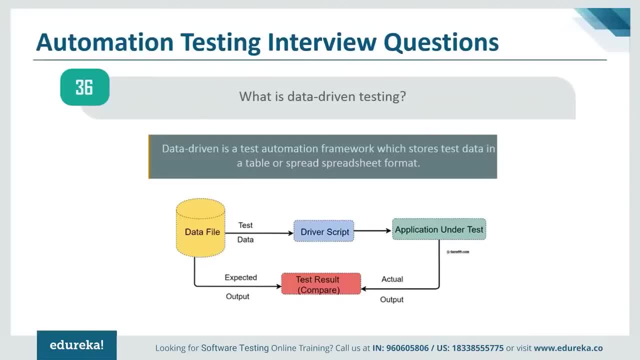 which you write and the script is implemented on your application. this way you get the results and then you compare the expected output with your actual output. This is how data-driven testing is done. Next question: What is test energy? Let's list out some of its prominent features. 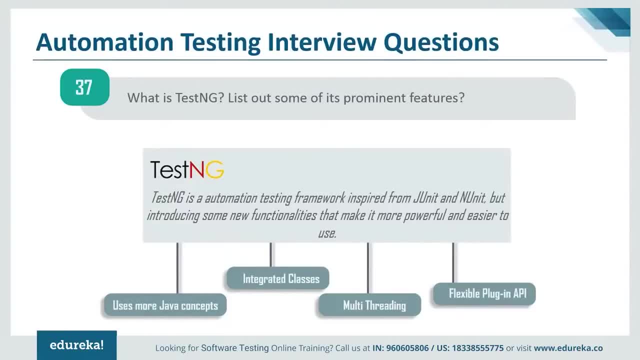 So, guys, if you remember, while listing out some of the most important test frameworks, I listed test energy as well. So, basically, test energy is an open-source automation testing framework where energy actually means next generation. It is inspired by another kind of framework called J units and N unit. 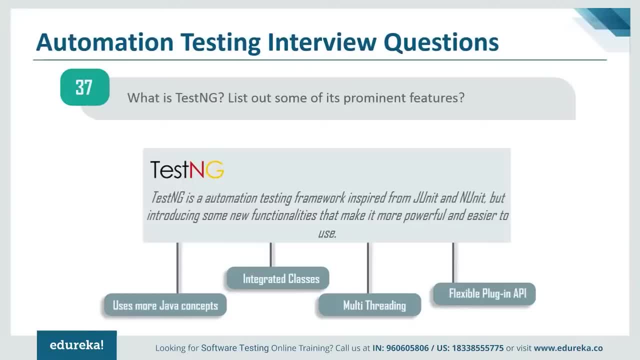 It is designed to be better than J unit actually, especially when it comes to testing with integrated classes. The creator of test energy is Cedric Bust. Test energy gives the developer the ability to write test more flexibly and more powerfully, And some of the most prominent features. 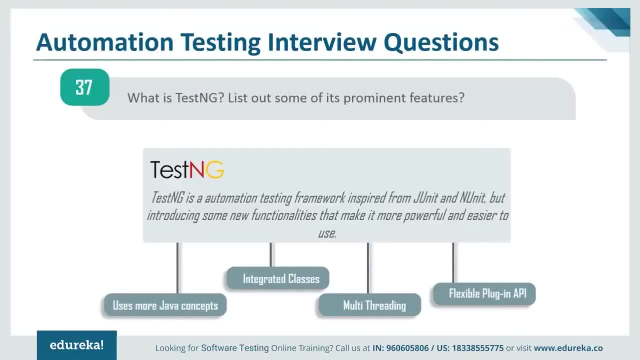 of test engine included supports annotations. annotations play a very important role. It also supports Java and oops concepts. It's supposed testing integrated classes, For example. by default you do not have to create a new test class instance for every test method that you use. 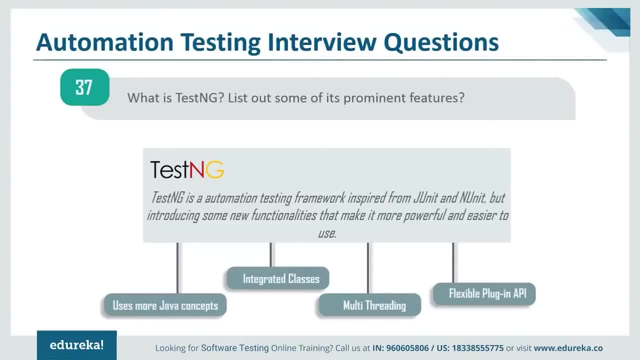 It also has flexible runtime configuration. It introduces a concept called test groups, So once you have compiled your test, you can just ask test energy to run your friend and test or fast or slow or database test, based on the way you have listed them. 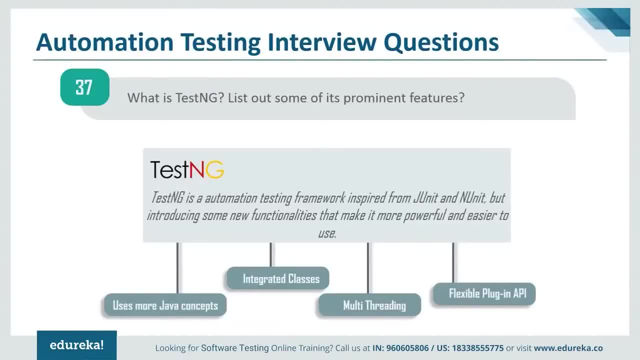 It also supports dependent test methods: pallet testing, load testing and partial failure. apart from this, it offers plug-in API and supports multi-threading as well. cool right, It has a lot of features. So what are the features of the advantages test energy has over J unit? 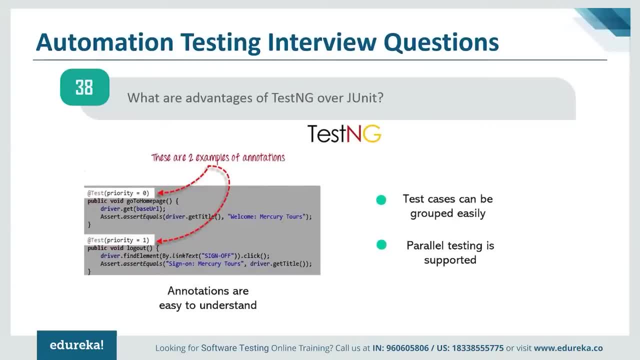 First of all, the most important feature is annotation. annotation and test energy are very easier to understand. They're just lines of code that can control how the method below them will be executed, For example. as you can see- I have a image there on the screen- 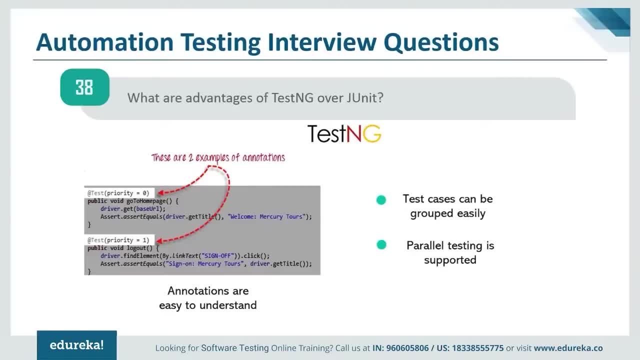 You can see I have two annotations here. First one is with priority 0 and next one is priority 1.. So basically, using these annotations and priorities, I'm saying that execute this method before you actually go in and execute other method. apart from annotations, other features include test. groups can be grouped. 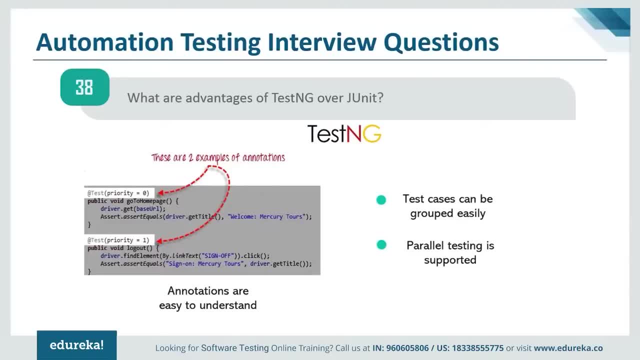 very easily. Like I said, you can just go ahead and ask test energy to run your friend and test fast or slow or database test, based on the way you have listed them, and it supports pallet testing, which is not there in J unit. Moving on to the next question, in what conditions? 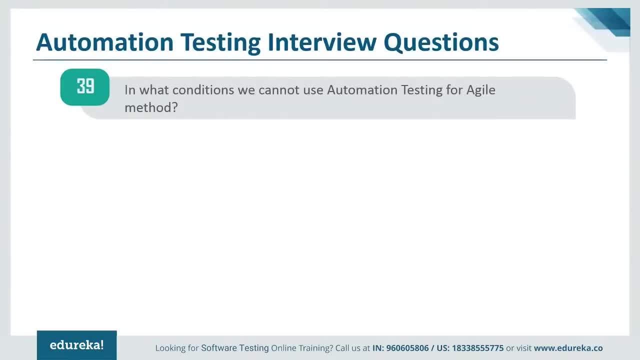 we cannot use automation testing for agile method guys. the Titans of information technology like Google, Amazon, Facebook, the develop software at very rapid phase So to meet the demand for their products and services They mostly use agile practices. test automation is fundamental part of agile. 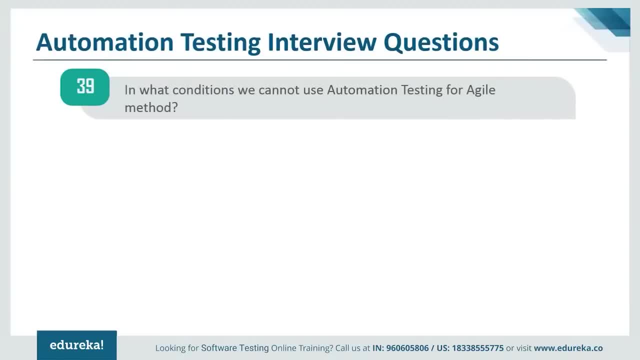 but there are certain times where automation testing in agile is useless. for example, when you have exhaustive level of documentation, when the requirements of your application of the software you're testing keeps changing. in such cases automation is definitely not suggested. Also, if you have one-time task, 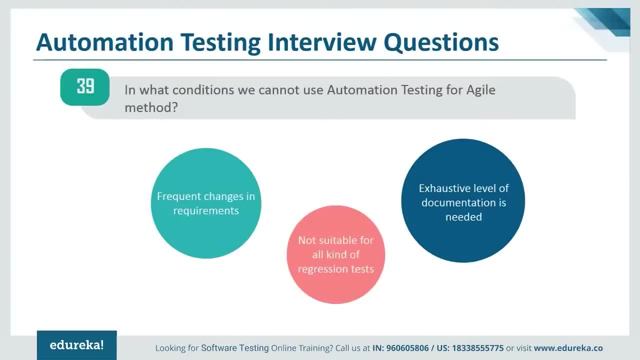 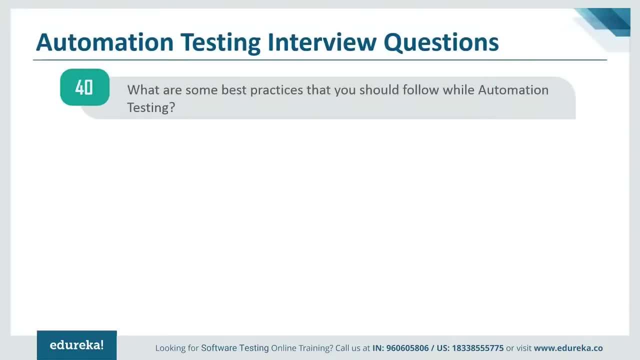 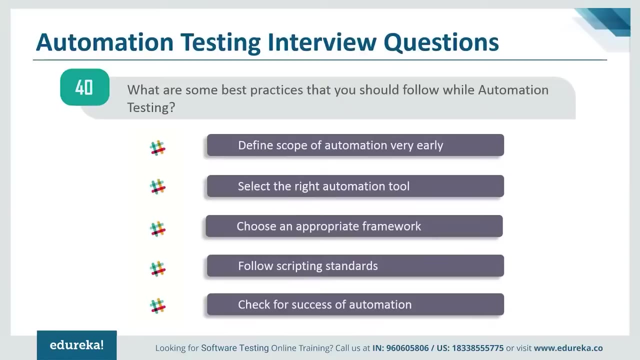 and exploratory test edge cases, automation should not be implemented. So these are certain cases where automation testing becomes useless in agile methods. a next question: What are some best practices that you should follow while automation testing? so, guys, to actually get maximum return of investment, you need to keep track of certain points. 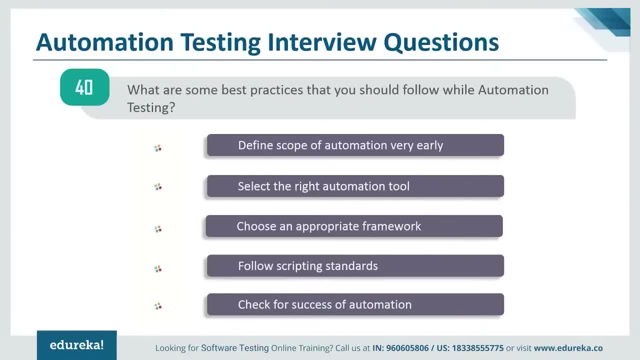 while actually performing automation testing. For example, the scope of automation needs to be determined in detail before the start of automation. So this way you actually know what you're actually automating and what you're expecting from the automation. next off, You should select the property tool. 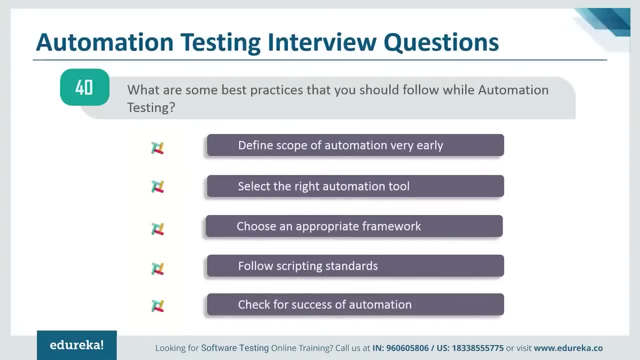 that meets your requirement. a tool must not be selected solely based on its popularity. You need to select this only because it fits your requirement. You need to decide if you want to use framework in your automation or not. So, apart from selecting framework tool and define the scope of automation, 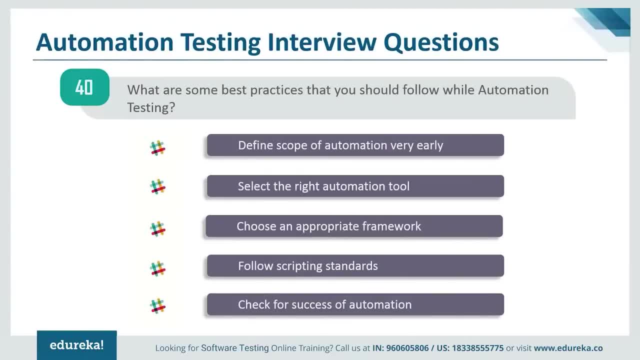 you need to follow certain scripting standards. standards have to be followed by writing the scripts for automation. We discussed them earlier. the standards like regularly including comments, proper indentation, adequate exceptional handling, Etc. Next, you need to check if the automation that you performed is successful or not. 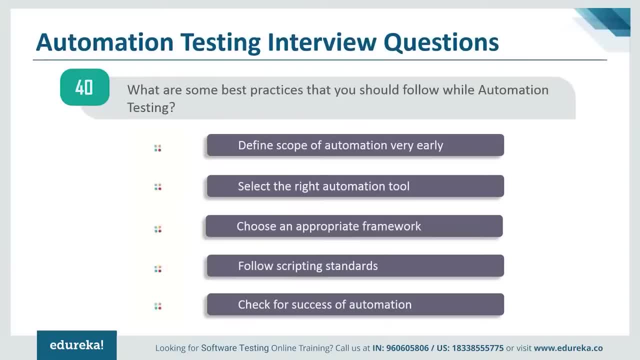 to check that. you can use criteria like the number of defects found, the number of time taken to actually perform the automation and the time required for automation testing for each and every release cycle, customer satisfaction index, productivity improvement- all the switches you can consider. So these are certain points that you should keep in mind. 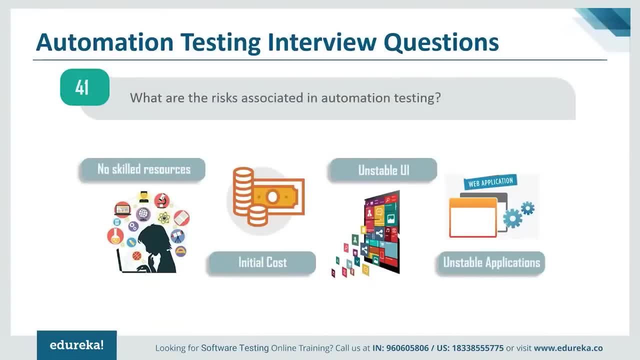 when you're actually performing automation. So the last question: what are the risks associated in automation testing? So, guys, just like manual testing, automation testing also involves risk. First of all, you need to ask yourself if or not you have skilled resources. automation testing demands resources. 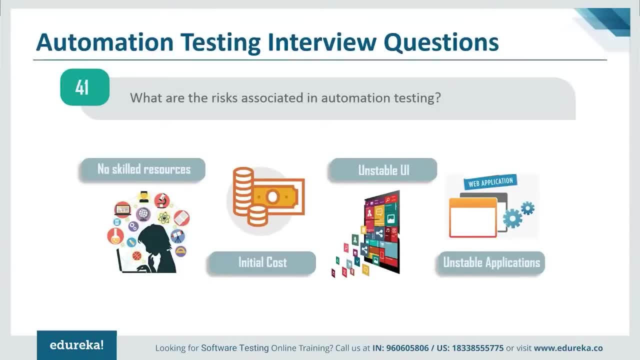 with some proper knowledge about programming. So if the people that you're actually automating or writing descriptive doesn't have any knowledge of programming, then definitely there will be some sort of error in your test cases, right? So you need to make sure that you have skilled resources. 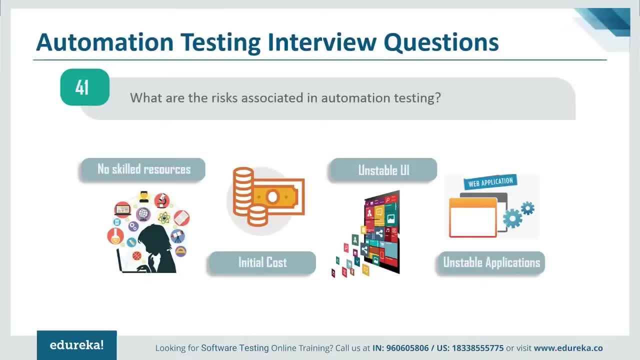 when you're actually starting your automation, and you should also ask yourself: are the resources which are wired capable to adapt easily to new technologies or not? and the second risk is the initial cost for automation is literally high because you have to buy a lot of tools and a lot of other things. 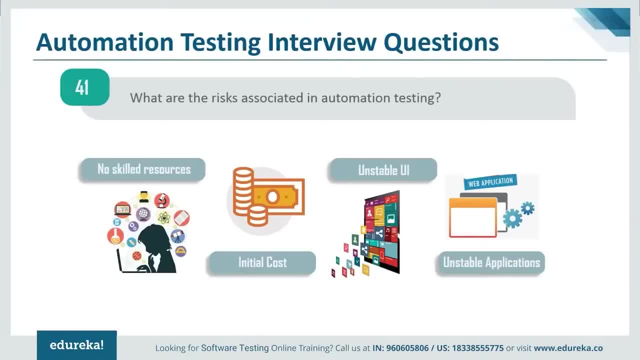 So make sure that the amount of money you spend compensates the testing results. and it's suggested not to use automation if you are using it for user interface because, like I said earlier, when you are testing and user interface, the requirements keep changing and it's difficult to keep updating your automation scripts. 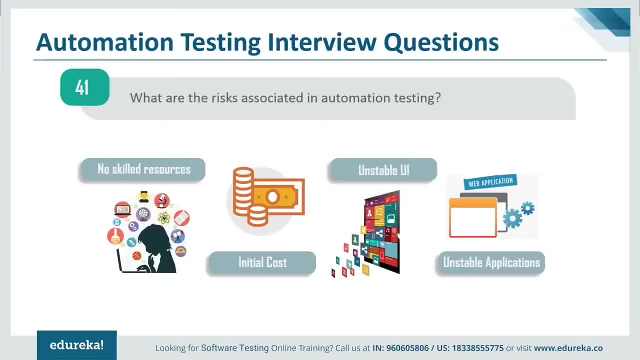 based on the changes. So if your UI is not fixed, do not use automation and next, make sure that the application you're testing is stable enough, else You might encounter a lot of errors while automation testing and it will take a lot of time. So refer to debug those errors and, lastly, stop automating. 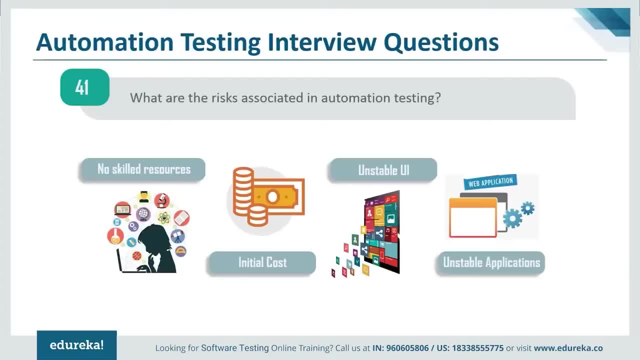 the test which run only once, because it does not worth the time and effort on your part, because you're running those tests only for once. So what is the point of applying automation here? So avoid automating such test modules. So these are certain risks which you might encounter. 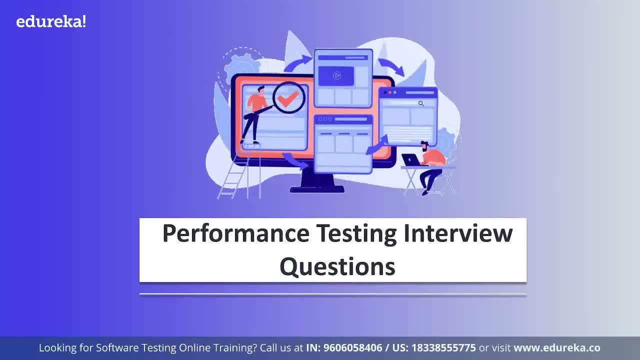 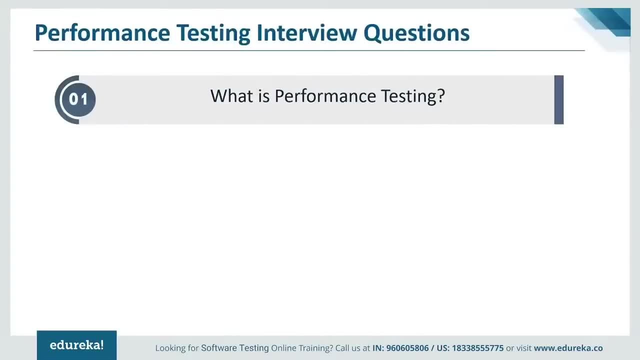 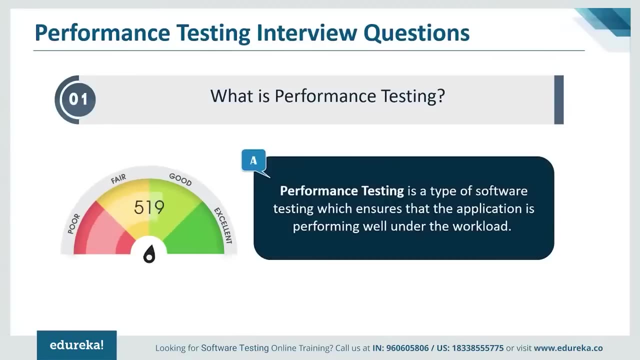 when you're performing automation. So the first question is: what is performance testing? now, performance testing is based on, basically, a type of software testing that ensures that the application is performing well under the workload. Now it is mainly done for quality assurance. It involves testing software application. 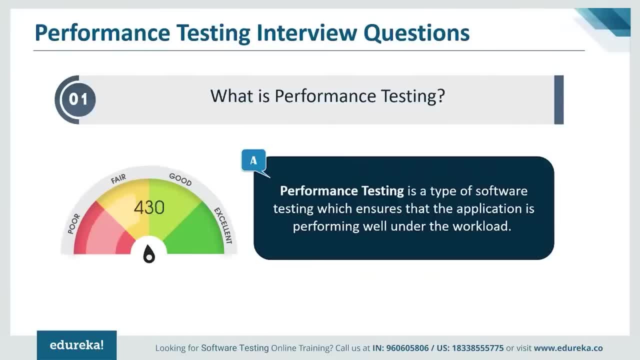 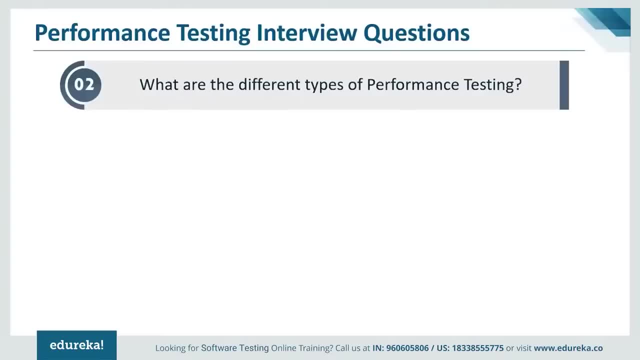 in order to provide a better performance of your product. This also helps you in gaining the confidence of your customers. The next question is: what are the different types of performance testing? Now, performance testing has mainly six types. First, We have the load testing. 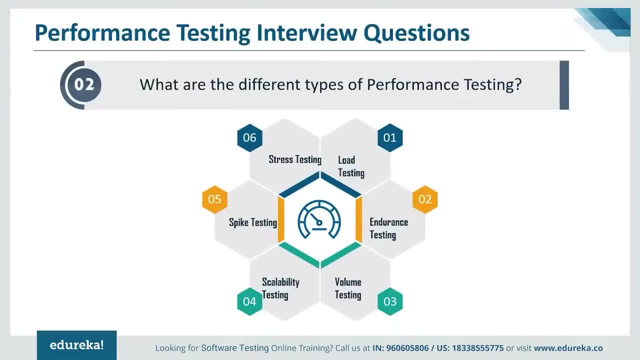 Now this checks the applications ability to perform under anticipated user loads. The objective is to identify performance bottlenecks before the software application goes live. Then we have the endurance testing. Now it is done to make sure that the software can handle the expected load over a long period of time. 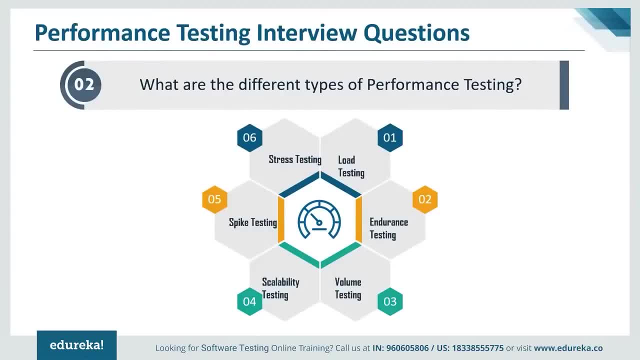 Then we have the volume testing. Now, under volume testing, large number of data is populated in a database and the overall software systems behavior is monitored. The objective is to check software applications performance under varying database volumes. Then we have the scalability testing. So the objective of scalability testing is: 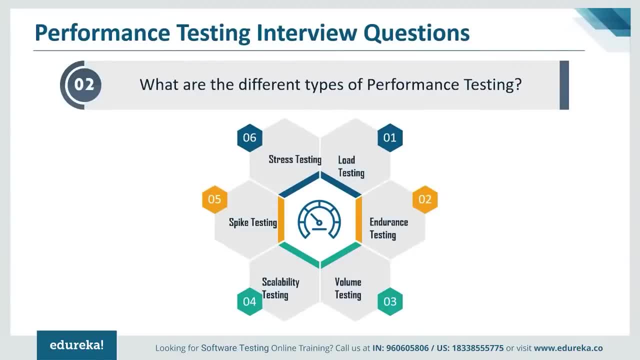 to determine the software applications effectiveness in scaling up to support an increase in user load. It helps plan capacity addition to your software system. Then we have the spike testing. Now this tests the software's reaction to sudden large spikes in the load generated by users. 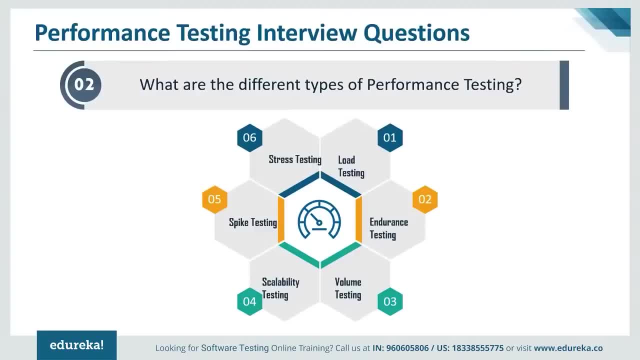 And finally, we have stress testing. Now this testing involves testing an application under extreme workloads to see how it handles high traffic or data processing. The objective is to identify the breaking point of an application. Now the next question is: what are the common performance? 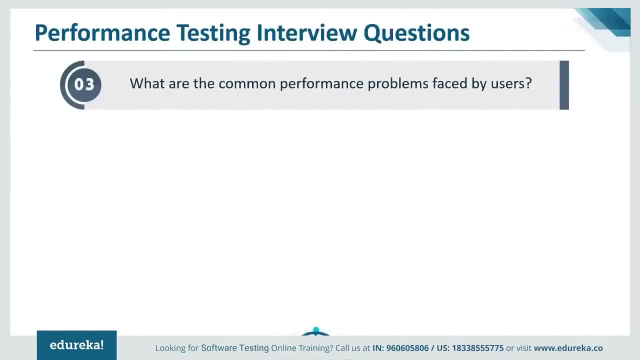 problems faced by users. So there are certain common problems that the users face in everyday life, which is exactly why we need performance testing in order to solve these issues. So the first one is longer loading time. Certain softwares might take a longer loading time. 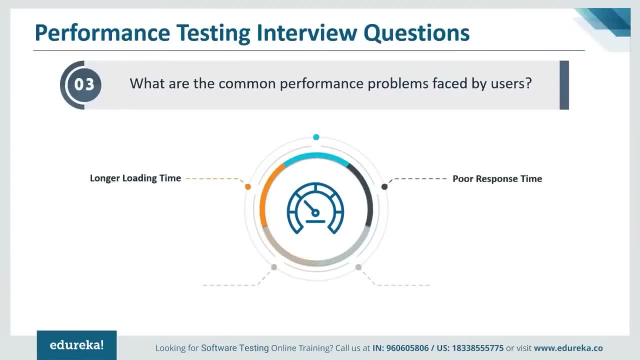 than expected. Also, there can be poor response time from the product. Then we have poor scalability and also bottlenecking, in which there might be coding errors or certain hardware issues, And to solve these problems faced by users, performance testing is used. Now moving on, the next question is: name some. 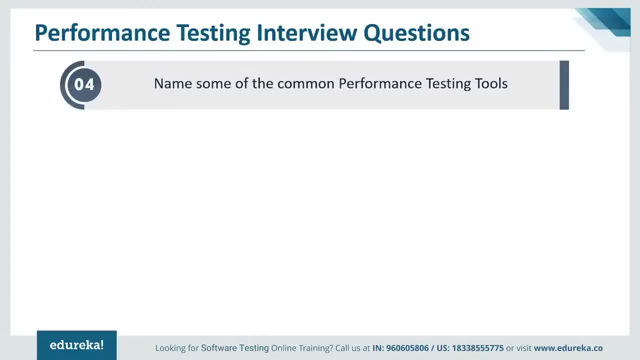 of the common performance testing tools. So there are a lot of performance testing tools available in the market and you have to select your perfect tool according to the requirement of the product. But some of the common performance testing tools are the load view, load UI, the web load Apache, JMeter. 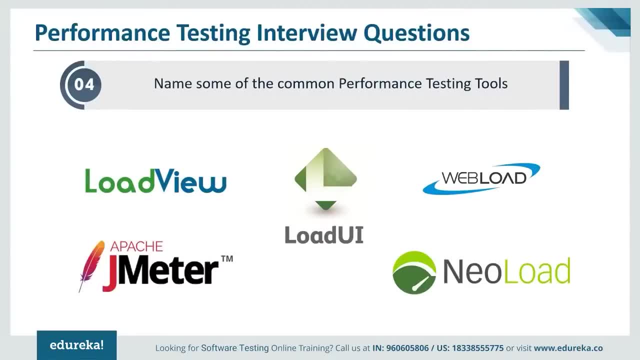 new load, and there are quite a few more. So there is no best tool in the market. All you need to do is find the best tool for your performance project goals. moving on, the next question is list out some common performance bottlenecks. So there are five common performance bottlenecks. 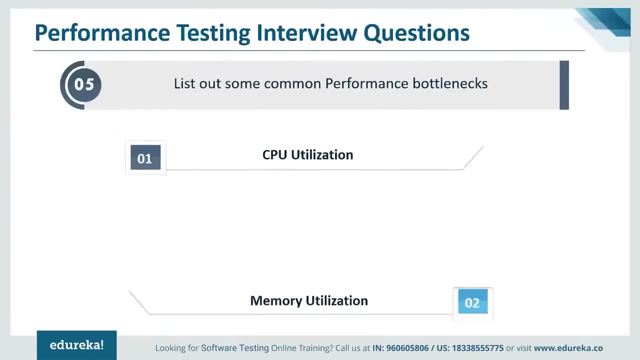 such as the CPU utilization, the memory utilization, Then we have the networking utilization s limitation and disk usage. next up, What are the parameters considered for performance testing? now, before the performance testing Takes place, There are certain parameters that we must consider, So let's have a look. 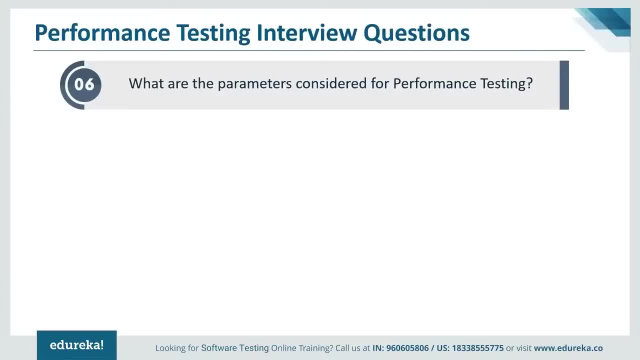 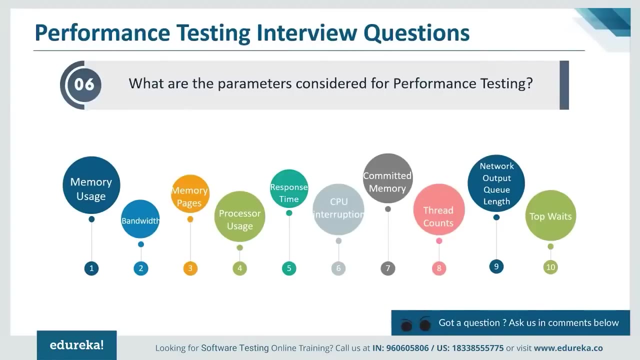 at all of those parameters that we must keep in mind. So first we have the memory usage. how much memory is being used here? Then we have the bandwidth. We must calculate the bandwidth of our product as well. Then we have memory pages, processor usage, response time. 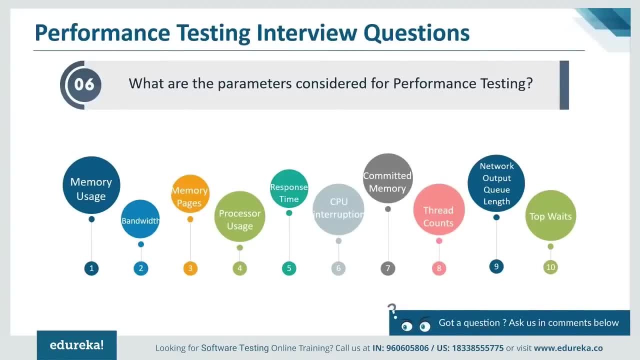 CPU interruption, committed memory, threat counts, network output, queue length and the top weights. There are certain more parameters that are to be considered, But these are some of the main parameters that must be taken care of before the performance testing takes place. next up, What are the factors? 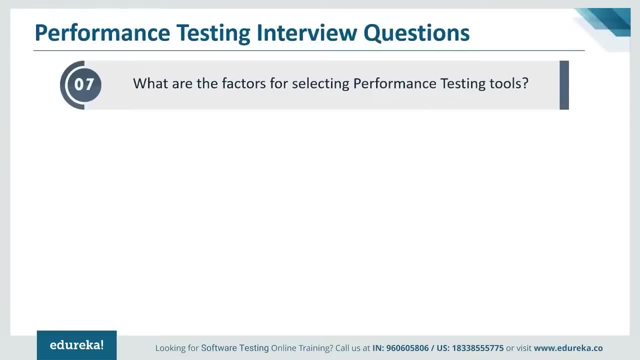 for selecting performance testing tools. now, as I've already told you, there is no such thing as the best tool. You have to find out the tool that suits your project goals. So I selecting your performance testing tools. There are certain factors that you must consider. 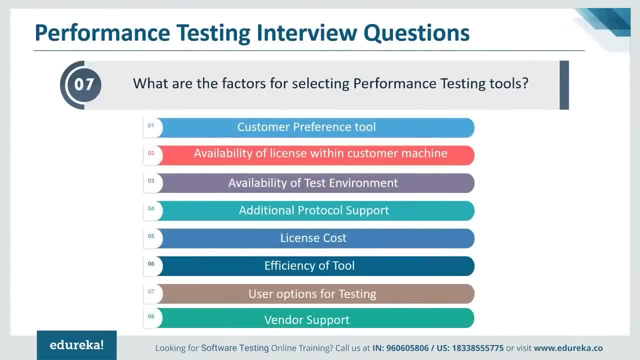 Some of these are the customer preference tool, the availability of license within customer machine, the availability of test environment, additional protocol support, license cost, efficiency of tool user options for testing and the vendor support. So you must check all of these things before you consider selecting any of the performance testing tools available. 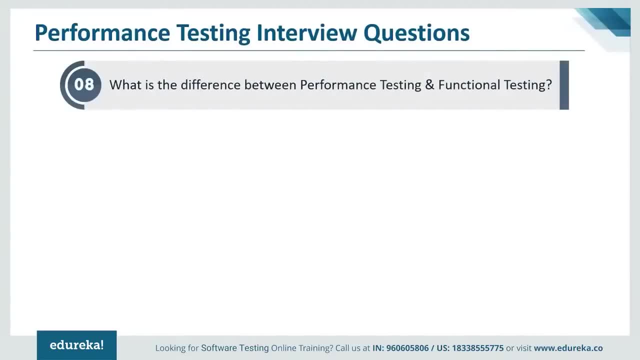 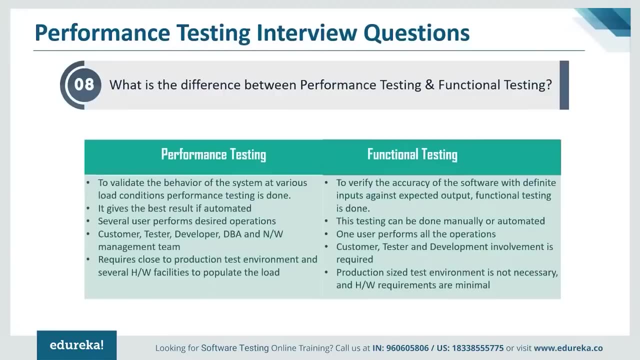 in the market today. The next question is: what is the difference between performance testing and functional testing? now, in case of performance testing, to validate the behavior of the system at various load conditions, performance testing is done, Whereas to verify the accuracy of the software with definite inputs against expected output. 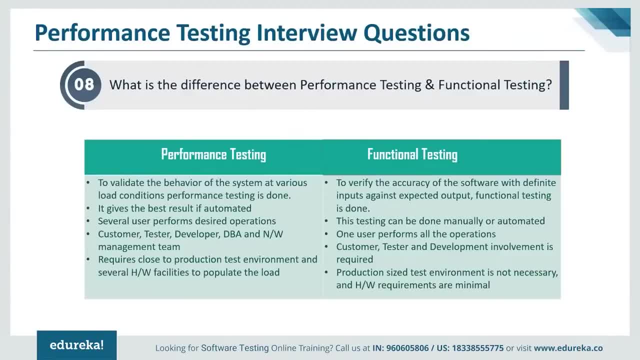 functional testing is done. Also, performance testing provides the best results when it is automated, but functional testing can be done manually or automated. now, in performance testing, several user performs the desired operations, but in functional testing only one user performs all the operations. in performance testing, 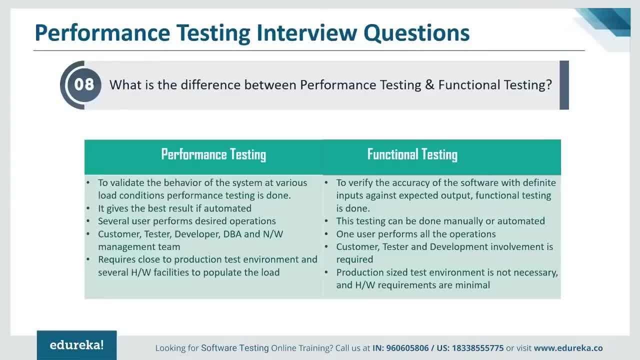 We would need a customer, a tester, developer, DBA and a management team, Whereas in case of functional testing, we would need a customer, tester and development involvement. Now, performance testing requires close to production test environment and several facilities to populate the load, Whereas in case of functional testing, 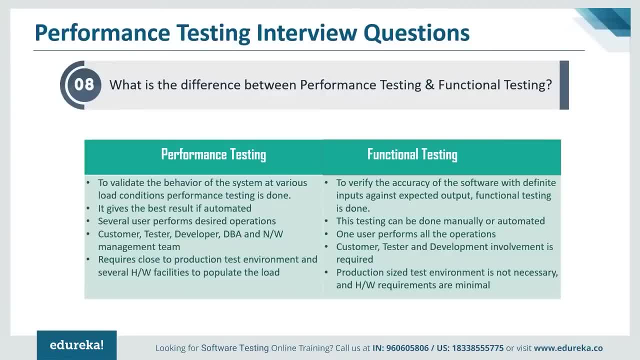 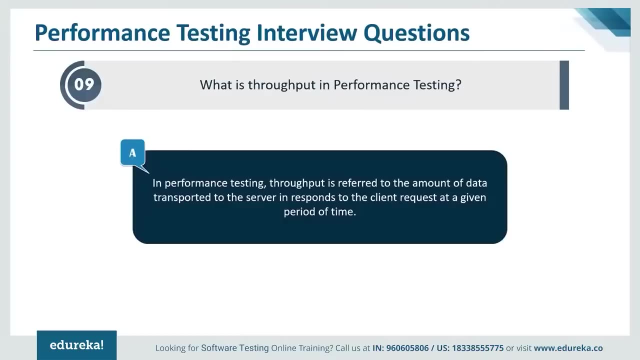 production sized test environment is not necessary and hardware requirements are minimal. So these were some of the differences between functional testing and performance testing. Now next question is: what is throughput in performance testing? Now, for every application, There are lots of users performing lots of different requests. 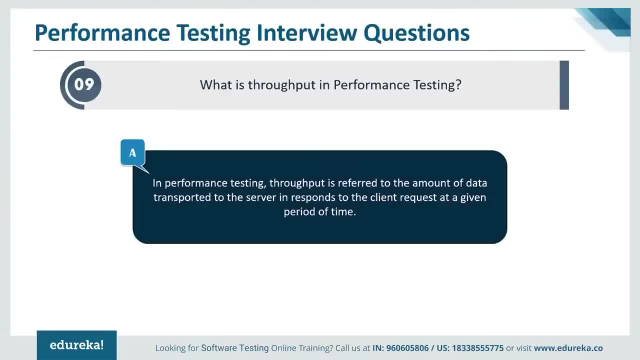 What you need to ensure is that your application meets the required capacity before it hits production or life. So in performance testing, throughput is referred to the amount of data transported to the server in response to the client request at a given period of time. Your throughput depends on factors. 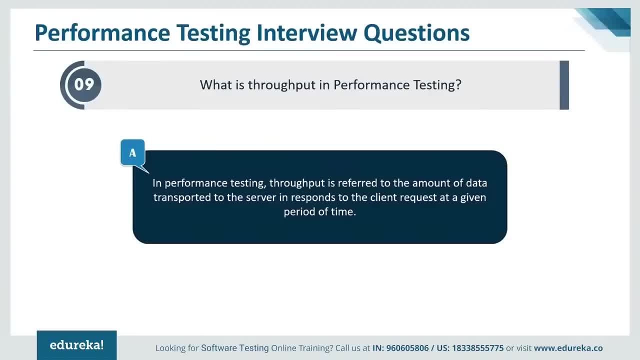 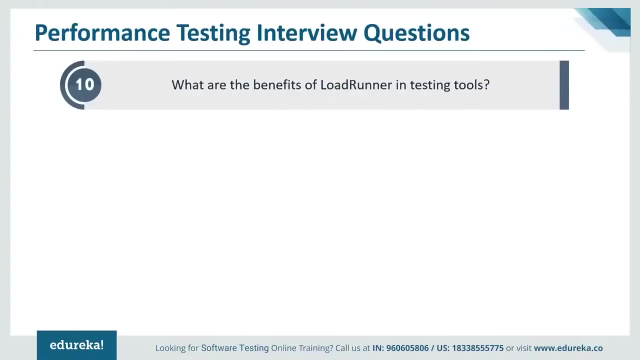 like specifications of the host computer, processing overhead in the software, degree of parallelism, both hardware and software support and types of transactions being processed. Now next question is: what are the benefits of load runner in testing tools? So, while using the load runner tool in performance testing, 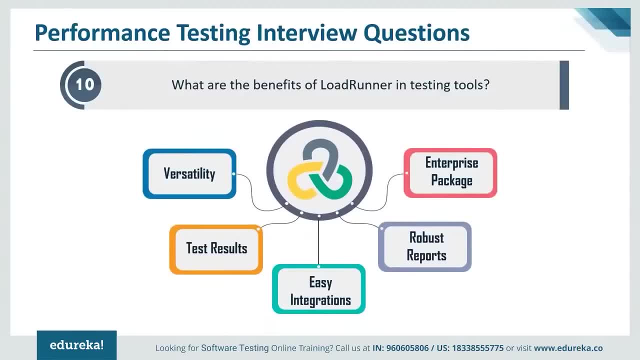 it provides a versatile result. Also, the test results are quite easy to understand and it provides an accurate result as well. With the help of load runner, we have easy integrations, There are robust reports and also it provides a complete Enterprise package. That's why load runner is also. 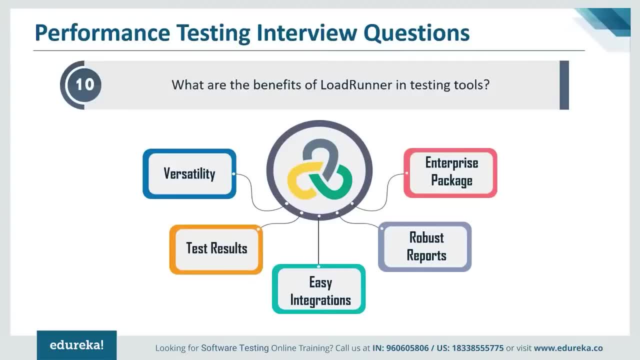 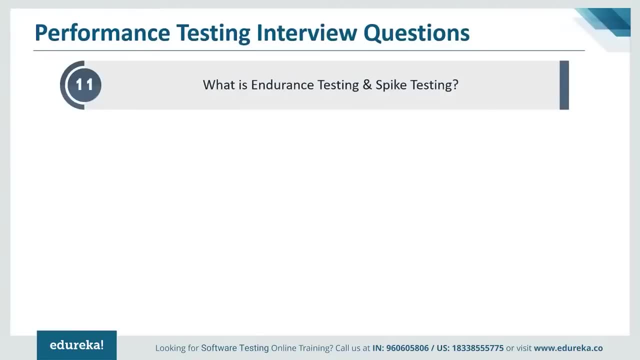 one of the most preferable testing tools when it comes to performance testing. Now moving on, the next question is: what is endurance testing and spike testing? So first let's have a look at what is endurance testing. So it is a non-functional type of software testing. 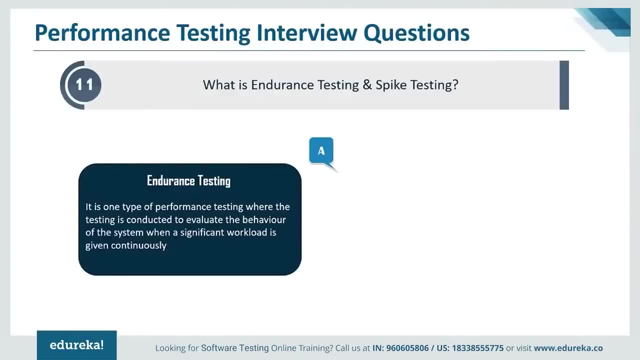 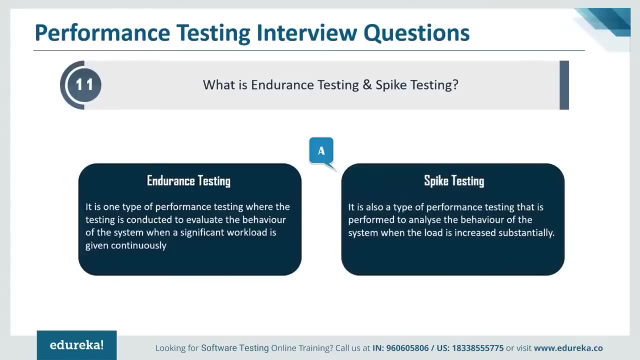 It is one type of performance testing where the testing is conducted to evaluate the behavior of the system when a significant workload is given continuously. It discovers how the system behaves under sustained use. Now, next, we have the spike testing. Now spike testing is defined. 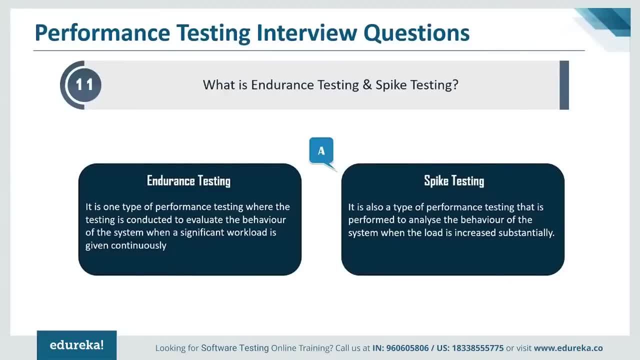 as a type of performance testing in which application is tested with extreme increment and decrements in the load. It is performed to estimate the weakness of an application. It is also a type of performance testing that is performed to analyze the behavior of the system where the load is increased substantially. 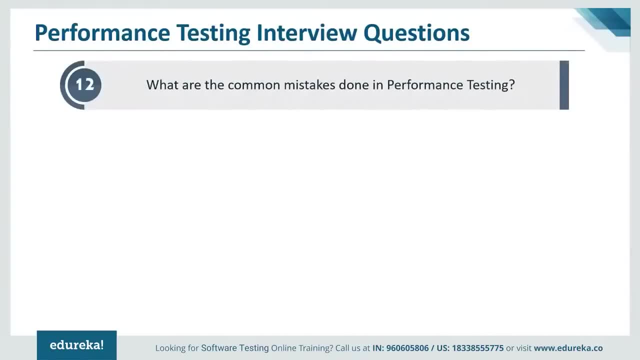 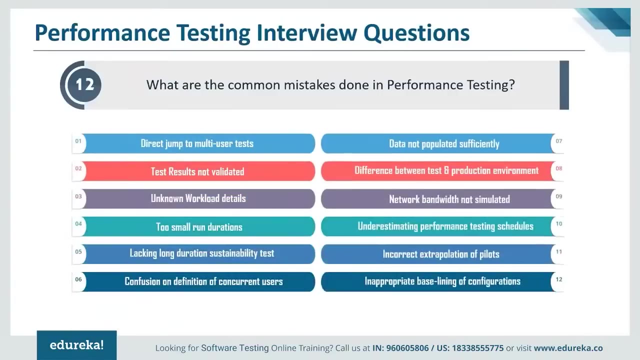 Now next up: what are the common mistakes done in performance testing? Now, during performance testing, we should always take care of certain common mistakes that are usually done by the users. So let's have a look at some of those common mistakes. The first one is direct jump. 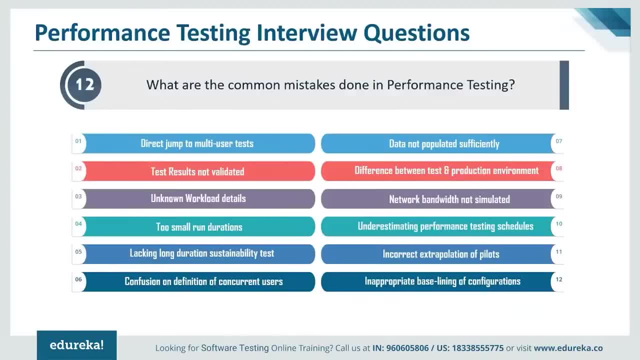 to multi-user tests. Then we have the test results not validated. It is always important to validate your test results before moving on. Next up is the unknown workload details. You should always be aware of the workload on your software. Next is too small run durations. 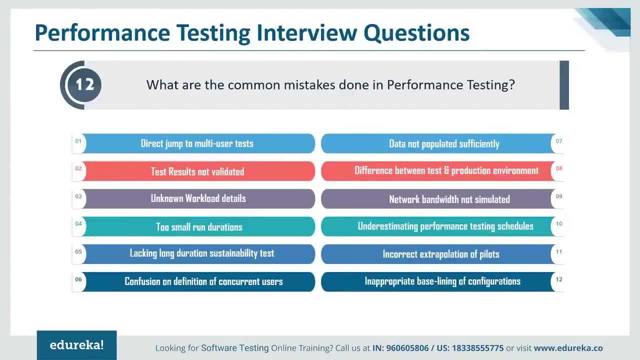 So your testing should not be too small. It should be at least of an average duration where you can figure out how is your product performing. Next up is lacking long duration sustainability test. Then we have the confusion on definition of concurrent users, Also another common mistake. 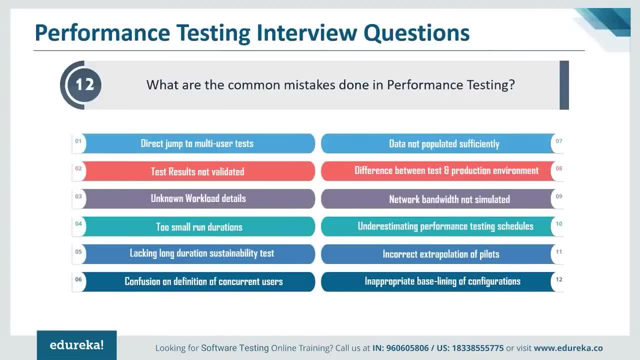 is data not being populated sufficiently. If there is too less data, the performance testing will not give you proper results. Also, you need to figure out the difference between test and production environment. Another mistake is the network bandwidth not being simulated. Then we have the underestimating. 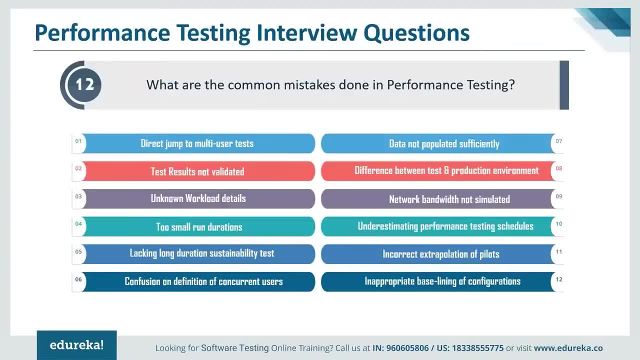 performance testing schedules and incorrect extrapolation of pilots. And finally, there's inappropriate baselining of configurations. So these are some of the common mistakes committed by the users, and you should always have a check on all of these during your performance testing. Now moving on. 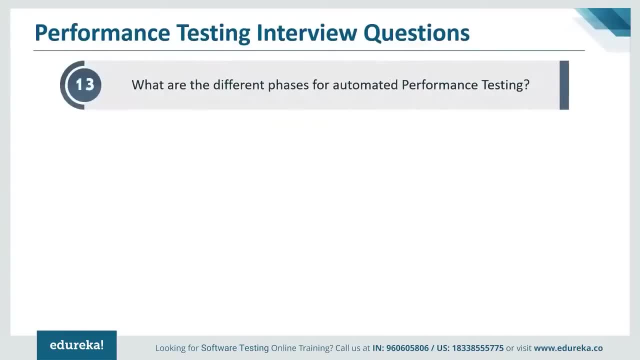 the next question is: what are the different phases for automated performance testing? Now, the first phase is design or planning. Now, what are the most important parts of the system you are testing and how do the critical components impact performance and the user experience? So a handful of API endpoints. 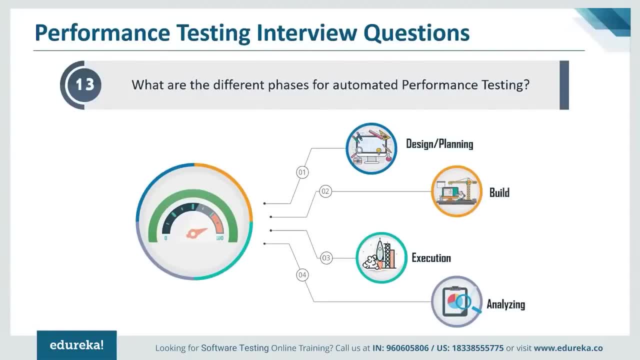 are most critical to the performance of your system. So testing your production environment requires additional planning to avoid disruption of your business. So it is very important to design or plan your performance testing beforehand. The next phase is building the structure. So according to your design, 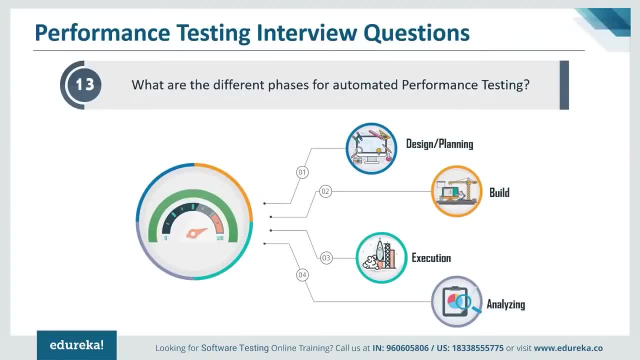 or plan of your performance testing. now you need to build your software accordingly, And once that is done, the next step is the execution. Now, once you are done with the designing, planning and building of your software, it's time you execute it. 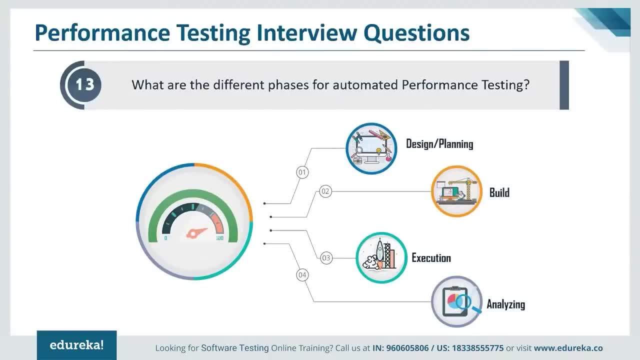 and perform testing on your software. Once the testing is completed, the final phase is analyzing the report. Now, once you have done the performance testing on your software, it's time you analyze the reports and check on how your software has been performing. So these are the different phases. 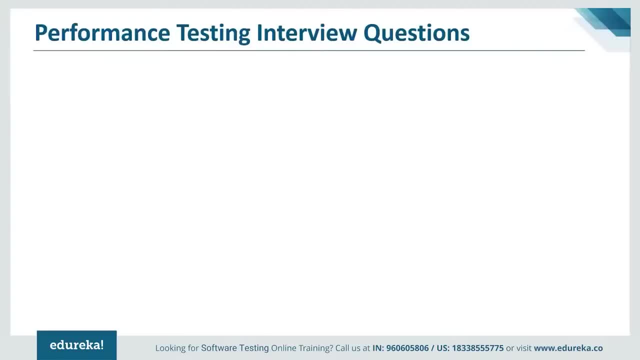 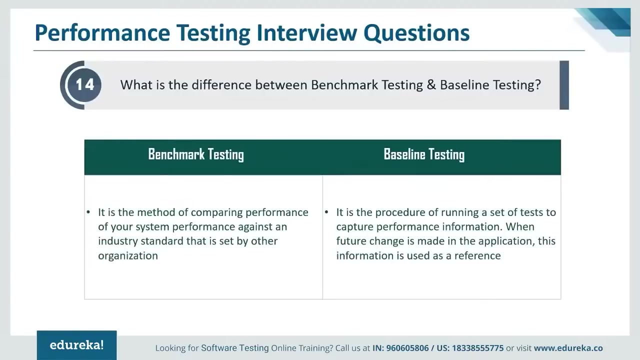 that are required for an automated performance testing. Now, moving on, the next question is: what is the difference between benchmark testing and baseline testing? So what is basically a benchmark testing? Now, it is the method of comparing performance of your system performance against an industry standard. 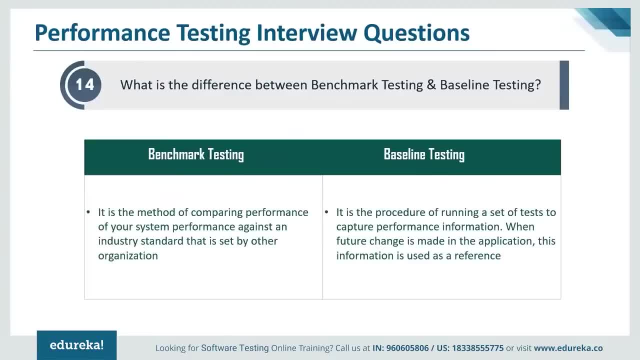 that is set by some other organization. So it will compare the performance of your software with certain industry standards that are available and it will also set a benchmark for your software that it should reach that certain level. Next is what's the baseline testing? So basically, this is the procedure. 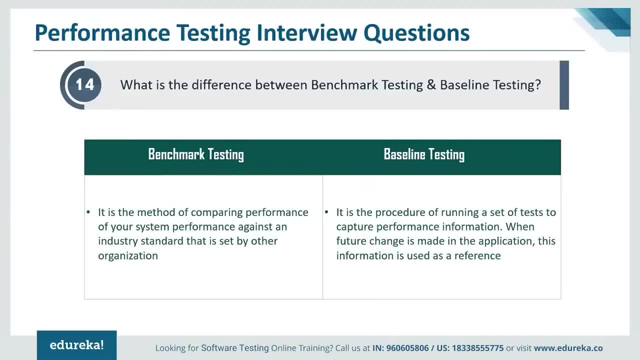 of running a set of tests to capture performance information Now, when the future changes made in the application, this information is used as a reference, It will always hold all the details if any changes have been made in your software. The next question is: 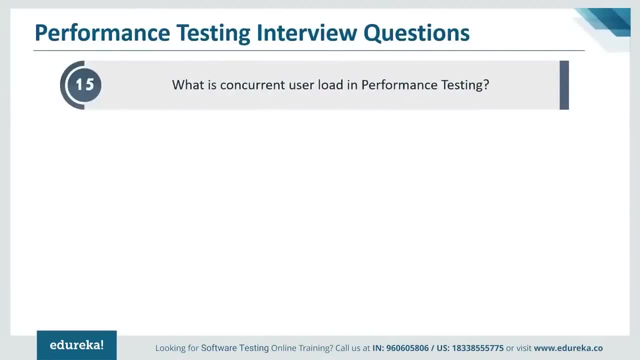 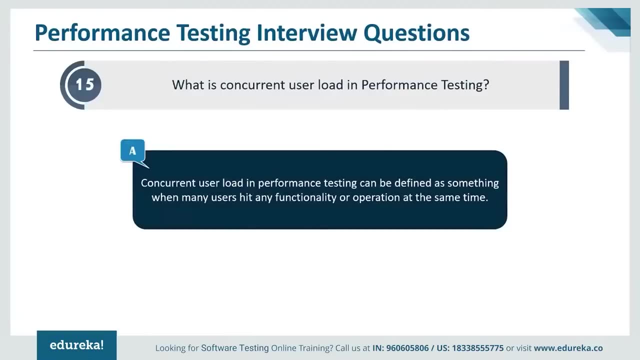 what is concurrent user load in performance testing? Now, concurrent user load in performance testing can be defined as something when many users hit any functionality or operation at the same time. It is also called a simultaneous user testing. Now, the idea behind concurrent user testing is to identify the response time of a website. 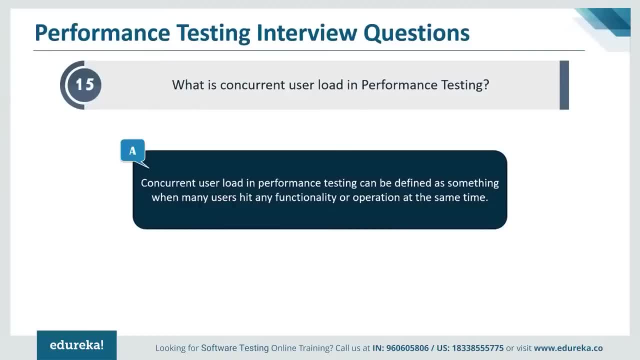 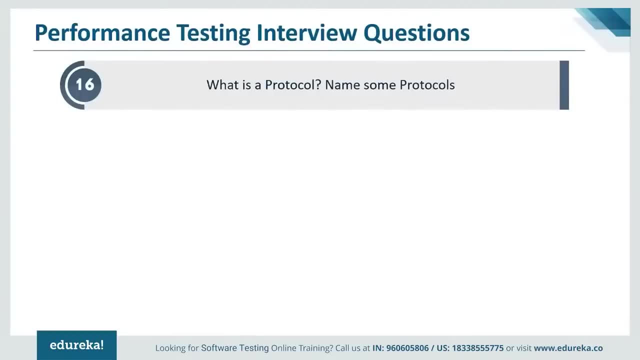 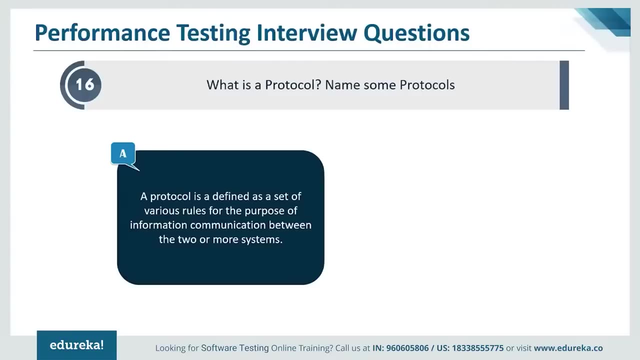 for a specified number of simultaneous users making requests to a website. Now moving on, next question is: what is a protocol, and name some of those protocols. Now, a protocol is basically defined as a set of various rules for the purpose of information communication between the two or more systems. 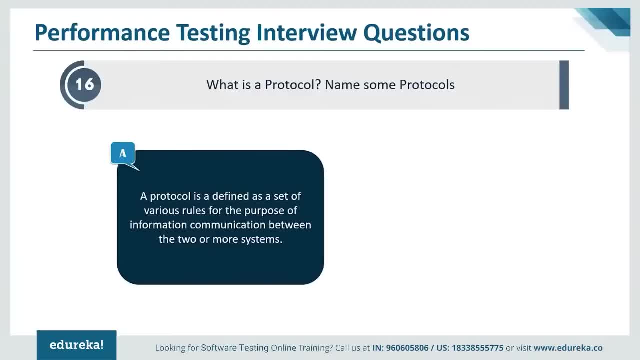 So it may be a load generator, application and web servers. Protocols include sending, receiving, authentication and error detection and correction capabilities. Some of the common protocols include the HTTP, HTTPS, FTP, the web services and Citrix. Next up, what is a performance tuning? 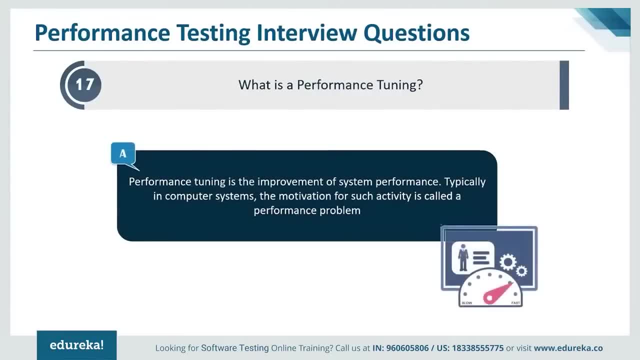 Now, performance tuning is the improvement of system performance. Typically in computer systems the motivation for such actions and activity is called a performance problem. Now this can be either real or anticipated. Now most systems will respond to increased load with some degree of decreasing performance. 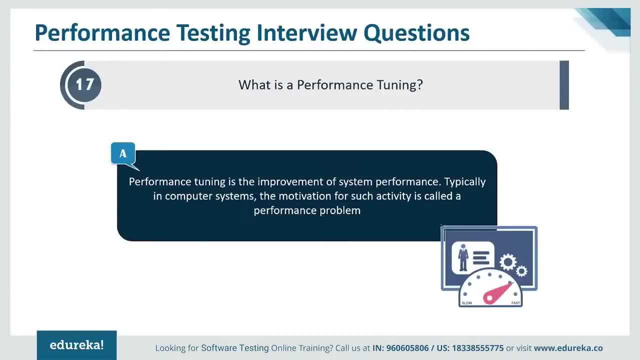 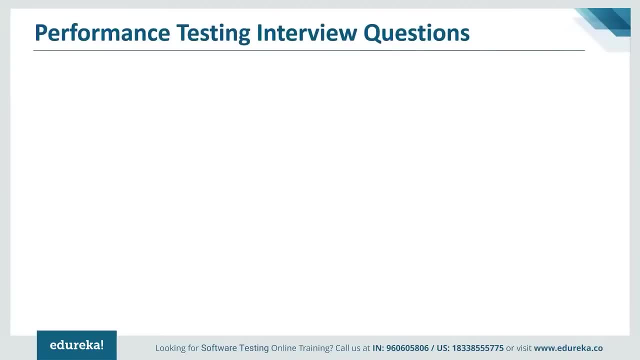 Now, as performance bottlenecks are identified during load testing and performance testing, these issues are commonly rectified through a process of the performance testing. Now moving on, the next question is: what are the types of performance tuning? So we have two different kinds. 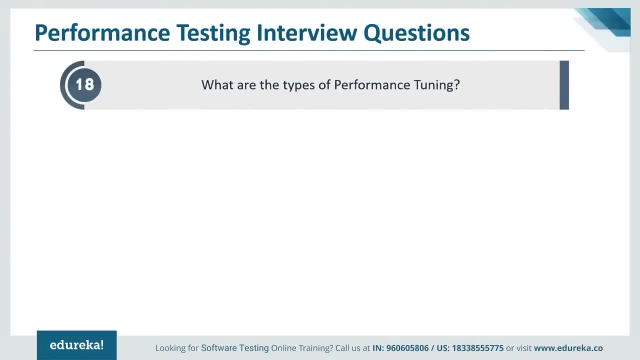 of performance tuning. First we have the hardware tuning and then we have software tuning. Let's have a look at what is hardware tuning So enhancing? adding or supplanting the hardware components of the system under test, and changes in the framework level to augment the system's performance. 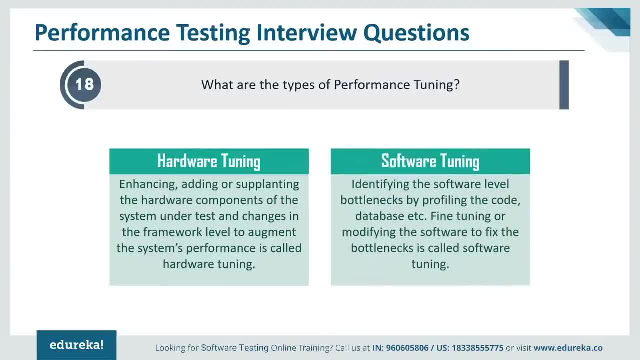 is called as the hardware tuning. Now what is software tuning? Basically, identifying the software level bottlenecks by profiling the code database, etc. Now fine-tuning, or modifying the software to fix the bottlenecks, is called as the software tuning. 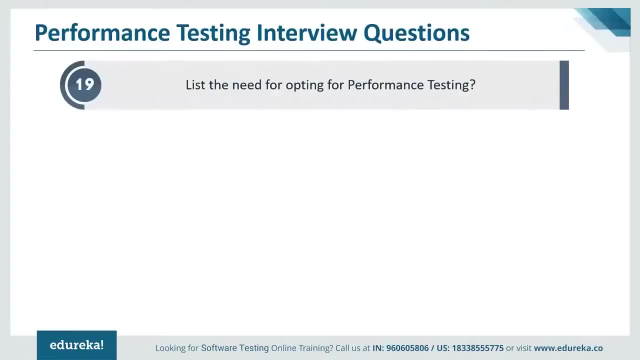 Next up list the need for opting for performance testing. Now, performance testing is generally required to validate the response time of application for the intended number of users. It also verifies the utmost load resisting capacity of an application. Next, it validates the capability of the app. 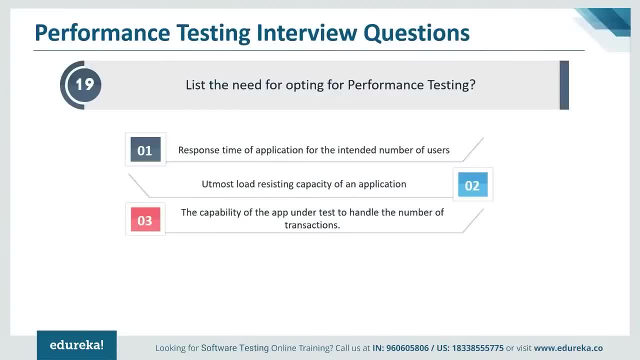 under test to handle the particular number of transactions. Also, it checks the constancy of an application under the usual and unexpected user load and finally, it makes sure that the users have an appropriate response time on production. Now the next question is: what is the reason behind the discontinuation? 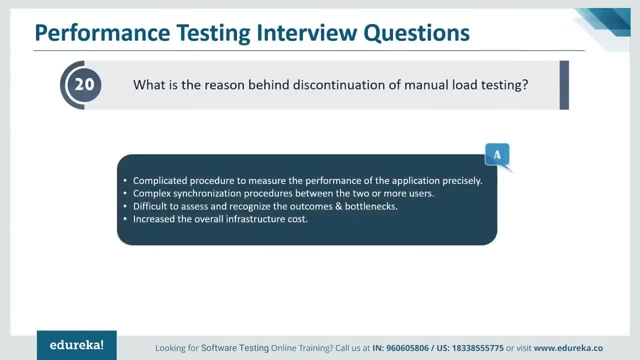 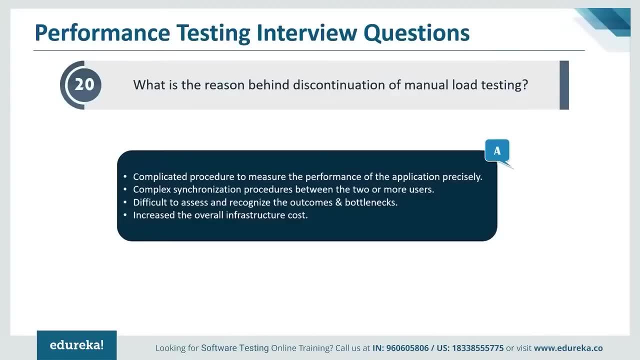 of manual load testing. So now, these days, the automated load testing is more preferred as compared to manual load testing. This happened due to the certain drawbacks of manual load testing. Now, due to those drawbacks of manual load testing, it led to the adoption of automation load testing. 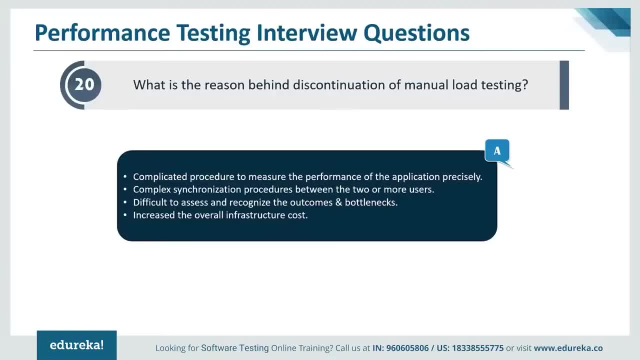 Now let's have a look at some of the reasons. First of all, the manual load testing had a complicated procedure to measure the performance of the application precisely. Then it had complex synchronization procedures between the two or more users. Also, it was difficult to assess. 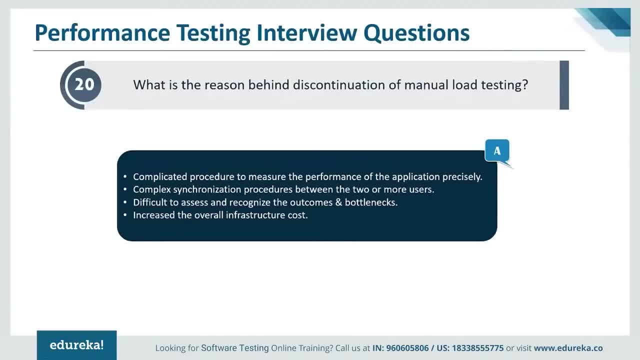 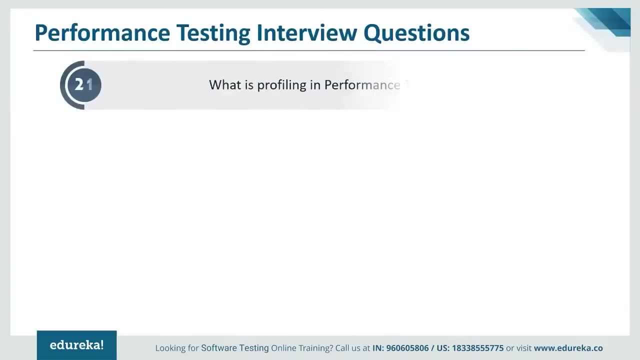 and recognize the outcomes and bottlenecks. and finally, it increased the overall infrastructure cost. So these are some of the reasons due to which manual load testing has been discontinued and now people prefer automation load testing. Now the next question is: what is profiling in performance testing? 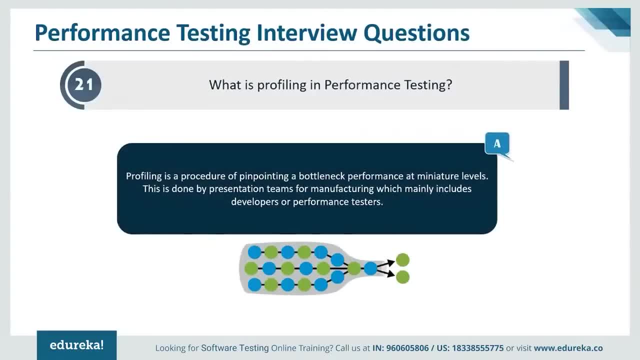 So profiling is basically a procedure of pinpointing a bottleneck performance at miniature levels. Now this is done by presentation teams for manufacturing, which mainly includes developers or performance testers. Now, profiling tools are usually only used once it has been identified that the system has a performance problem. 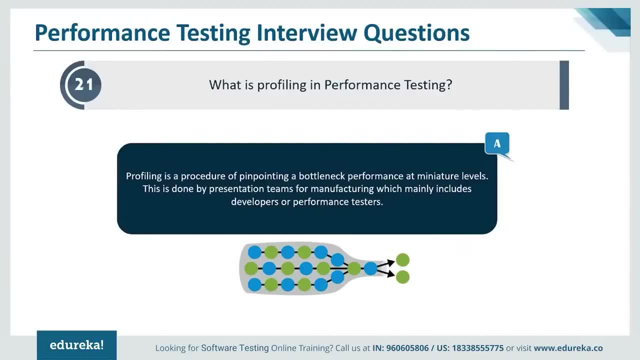 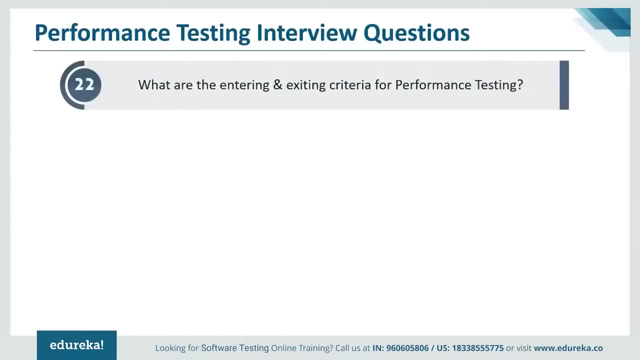 Now, if the server is taking a long time to respond and you can't identify any resource problem, profiling might be your next choice of strategy. It is best handled by a developer, while the tester applies load using the performance scripts. Next up, what are the entering and exiting? 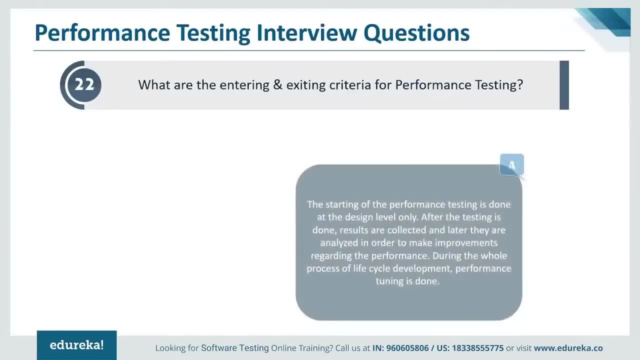 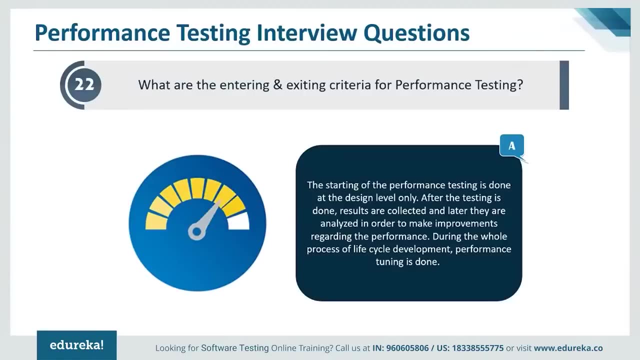 criteria for performance testing. Now the starting of the performance testing is basically done at the design level. only Now, after the testing is done, the results are collected and later they are analyzed in order to make improvements regarding the performance. Now, during the whole process of life cycle development, 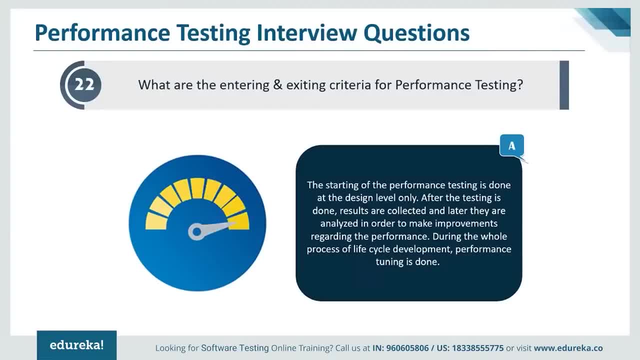 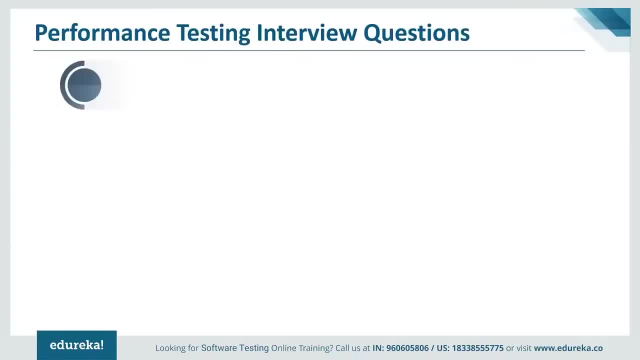 performance tuning is done. So these are the things that are need to be considered for the entering and exiting of the performance testing. Now moving on, the next question is: what are the activities involved in performance testing? So at first we have to know all our requirements. 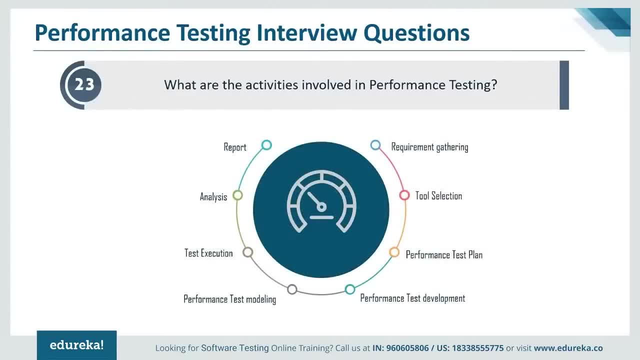 and make sure all of them are available. Next up, we have the tool selection. So, based on our requirements, we have to opt for a performance testing tool that will serve our purpose. The next activity is the performance test plan. So first we have to plan exactly. 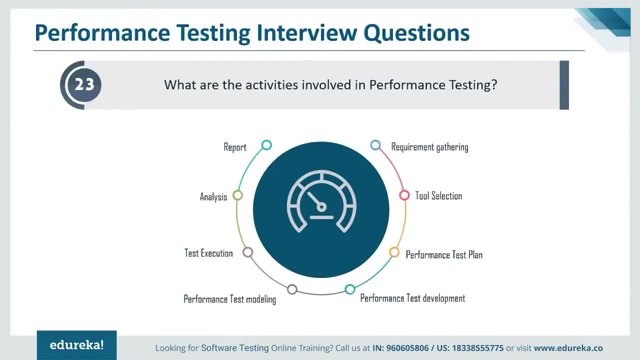 how the performance testing will take place. and then we have to check for the performance test development. Next activity is the performance test modeling. So once the test has been developed, next step is to check the performance test model. Once the idea of how the performance testing 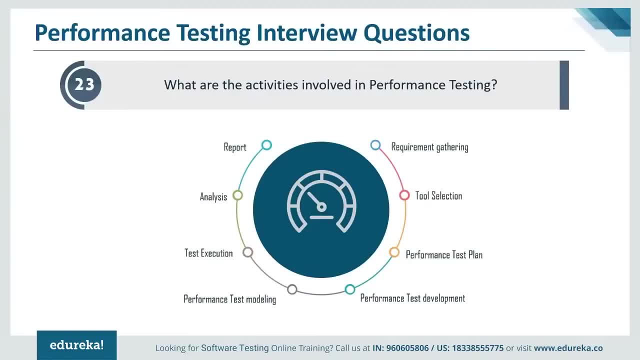 is going to take place is ready and the model is set. the next step is the test execution. In this step, finally, the testing takes place. Next up, we have the analysis. Now, once the test is completed, the next step is to analyze how the test has been performed. 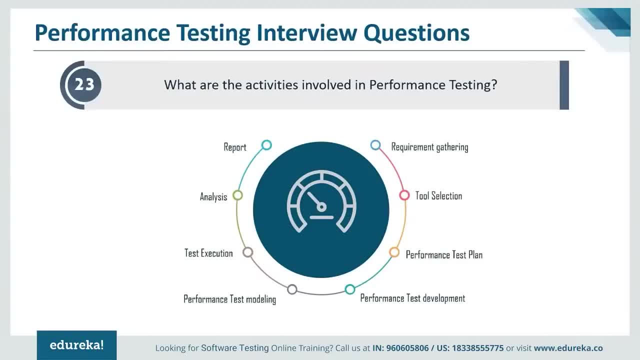 and what results does it show? and finally, we have the report of our performance testing. So the report provides you all the detailed information about your software and how the testing has performed. So these are the number of activities that are performed during performance testing. Now the next question is: 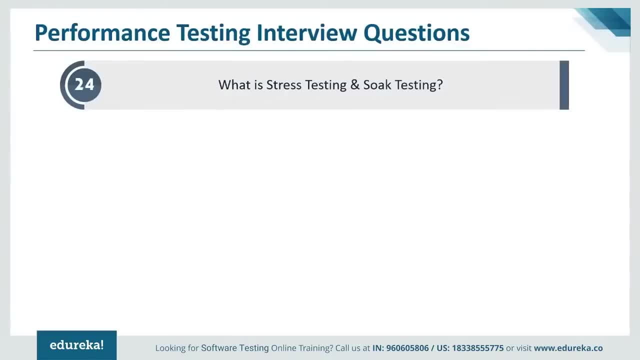 what is stress testing and SOC testing? So first let's have a look at what is stress testing Now, stress testing is a software testing activity that determines the robustness of software by testing beyond the limits of normal operation. So what is SOC testing? 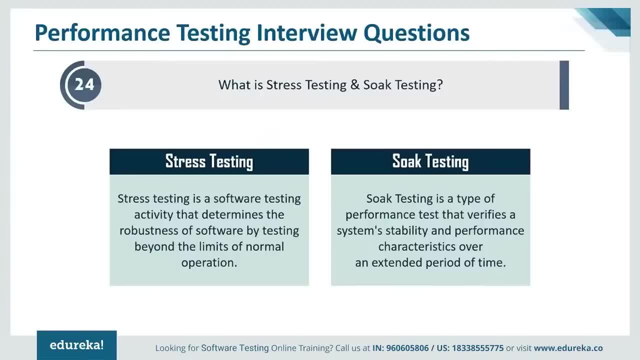 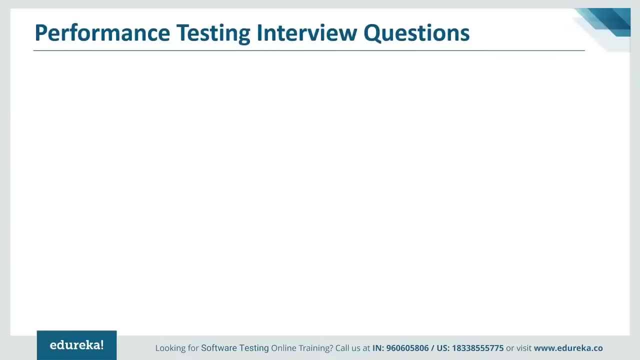 SOC testing is basically a type of performance test that verifies a system's stability and performance characteristics over an extended period of time. So now that you know what is stress testing and SOC testing, let's move on to the next question. The next question is differentiate. 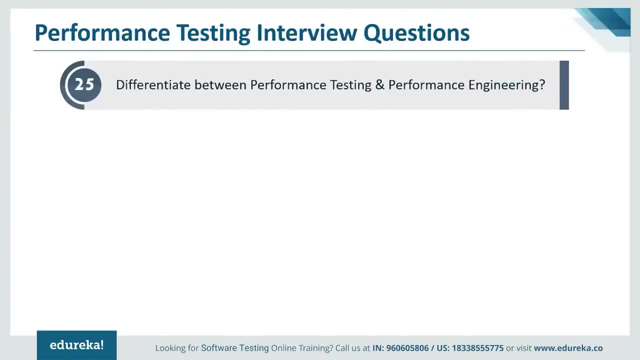 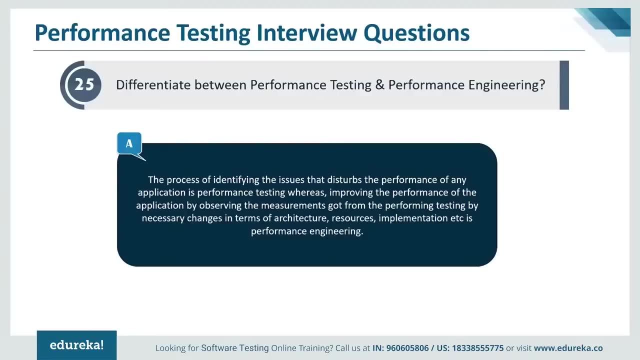 between performance testing and performance engineering. Now, the process of identifying the issues that disturbs the performance of any application is performance testing, Whereas improving the performance of the application by observing the measurements got from the performance testing, by necessary changes in terms of architecture, resources, implementation, etc. 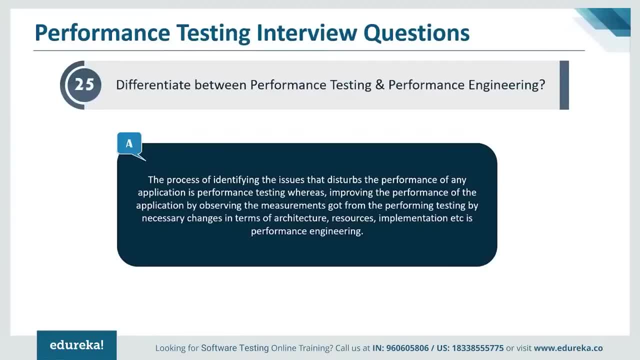 is called as performance engineering. Now, a performance test is someone who has an understanding of how to execute loads, scalability and SOC or the endurance tests. They have experience with performance testing tools like Jmeter, Loadrunner and many more, Whereas a performance engineer has skills. 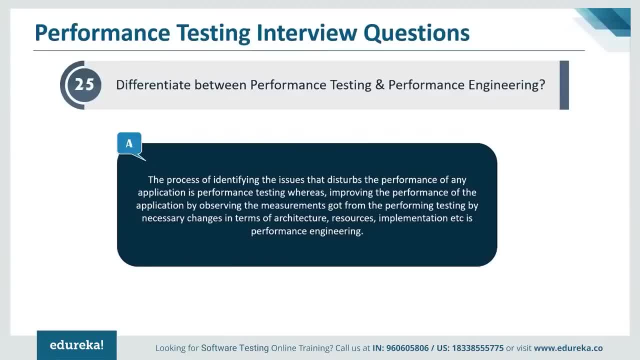 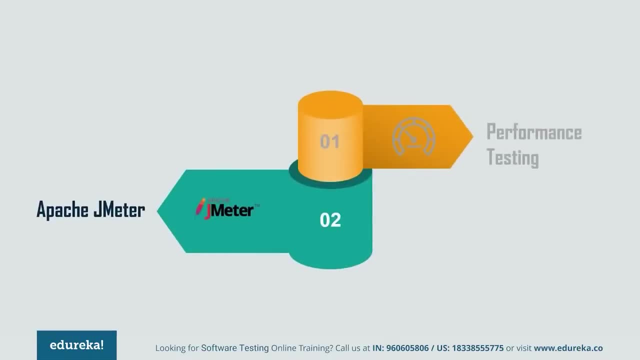 beyond that of a performance tester. A performance engineer is capable of not only identifying a performance issue, but digging in to help identify the root cause as well. So these were some of the common questions asked for performance testing interviews. Now, Jmeter is one of the most commonly used. 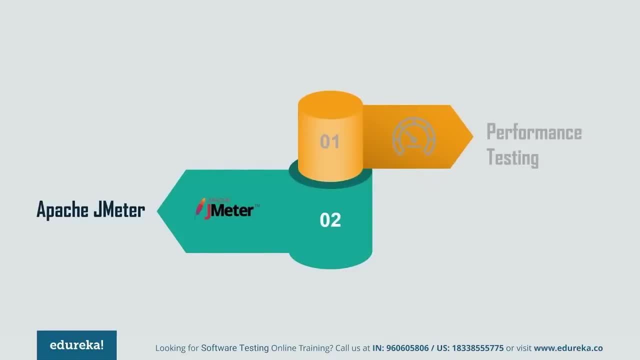 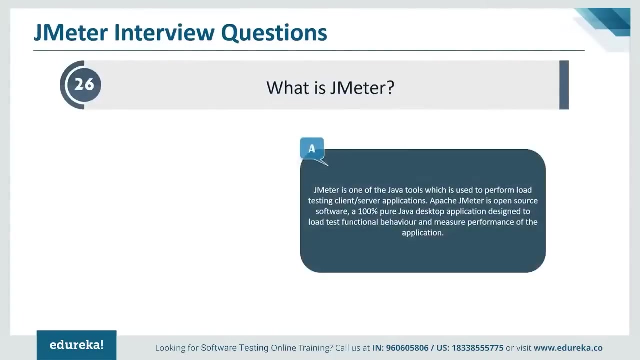 performance testing tools. So we will have a look at some of the commonly asked interview questions about Apache Jmeter. So now let's have a look at the common questions asked about Jmeter. So the first question is: what is Jmeter? Now, Jmeter is one of the Java tools. 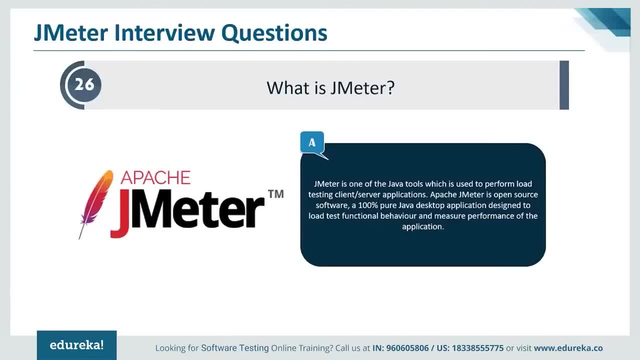 which is used to perform load testing client or server applications. Now, Apache Jmeter is basically an open-source software. It is a 100% pure Java desktop application which is designed to load, test functional behavior and measure performance of the application. Now, it was originally designed for testing web applications. 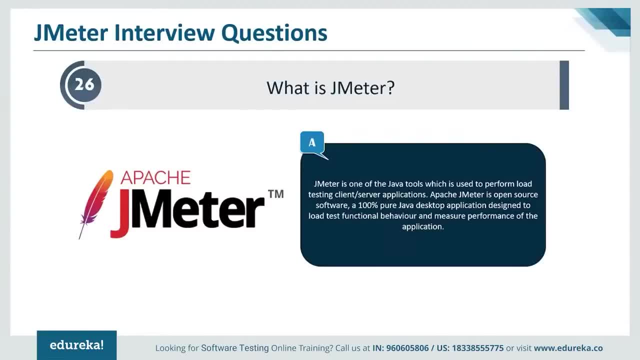 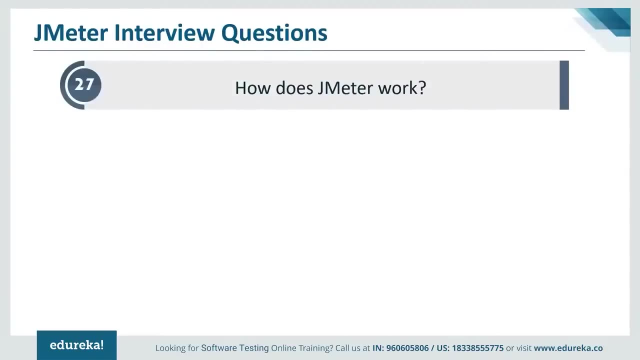 but has expanded to other test functions. It is also one of the most preferable testing tools when it comes to performance testing. You can also check out the Jmeter tutorial in order to know more about the working of Jmeter. Now the next question is: how does a Jmeter work? 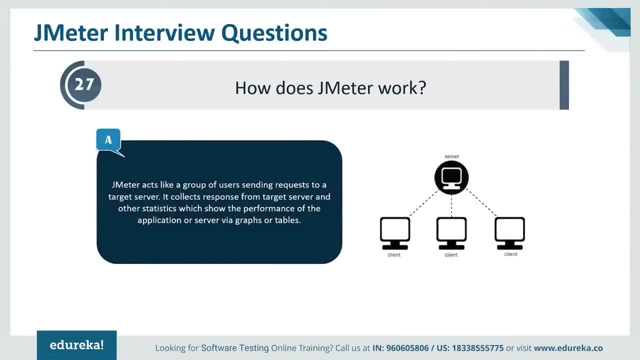 So now a Jmeter basically acts like a group of users sending requests to a target server. So what it does is it collects response from target server and other statistics which show the performance of the application or server via graphs or tables. It provides you with a generalized report. 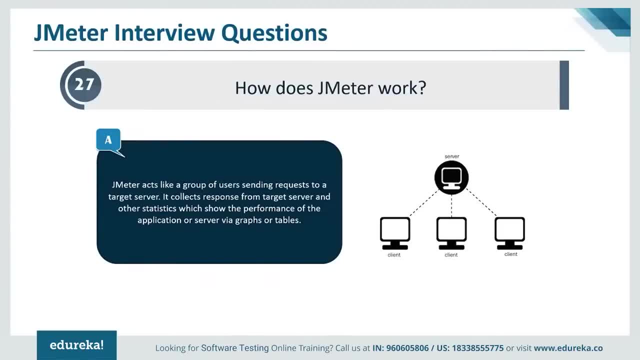 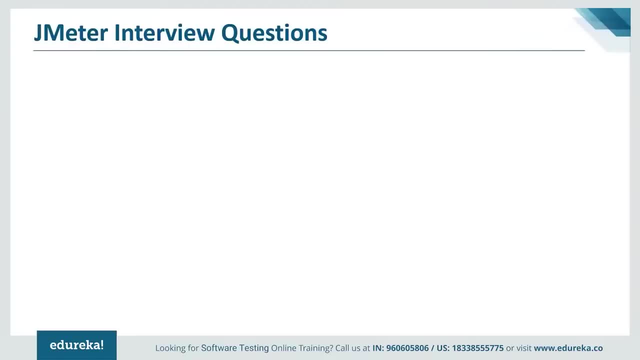 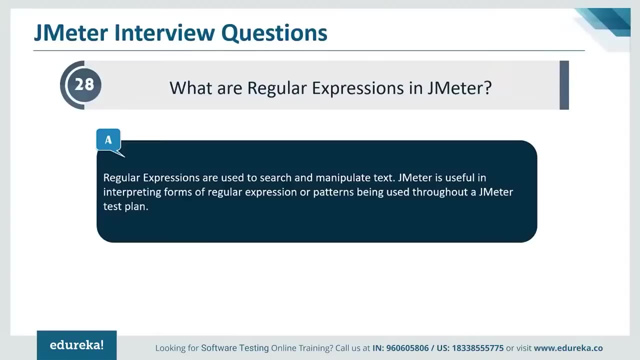 with lots of graphs and tables and trees, which will give you a proper analysis report of your testing. Now moving on, the next question is: what are the regular expressions in Jmeter? Now, the regular expressions are used to search and manipulate text. Now Jmeter is useful in interpreting forms. 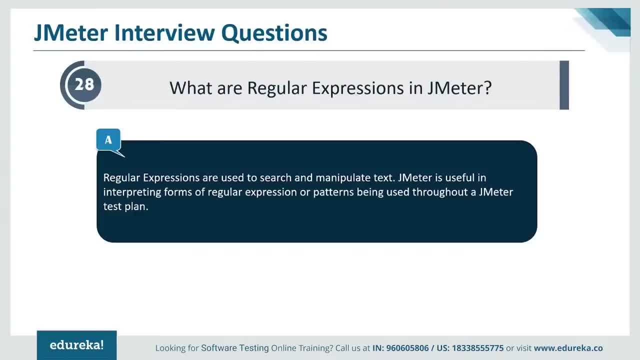 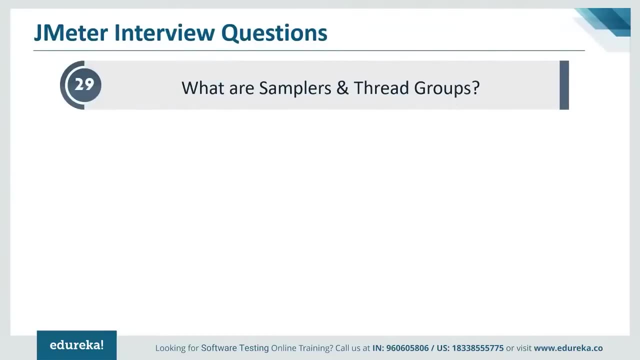 of regular expression or patterns being used throughout a Jmeter test plan. This just provides a common pattern that we use during our entire process of testing in Jmeter. Now the next question is: what are samplers and thread groups? So samplers and thread groups are basically: 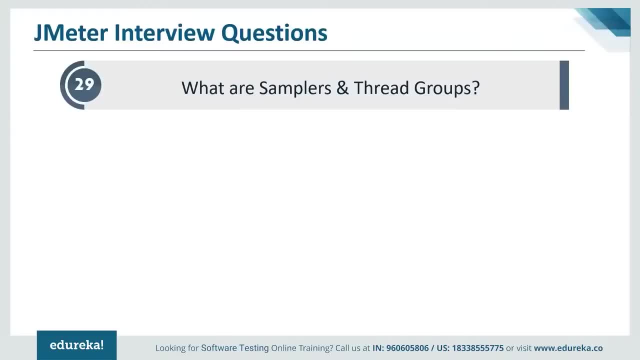 two important elements of Jmeter while we are performing any test using this tool. So let's have a look at what are samplers. So samplers basically allow Jmeter to send specific types of requests to the server. through samplers, Thread group decides which type of request it need to make. 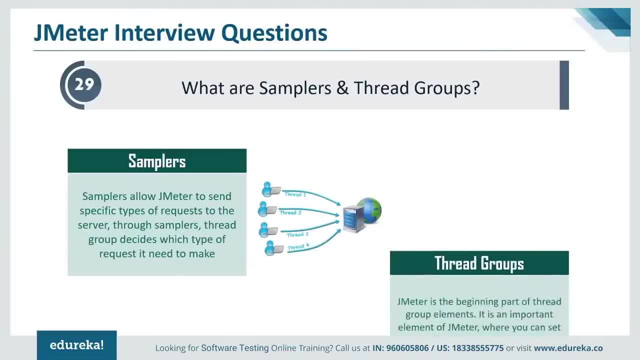 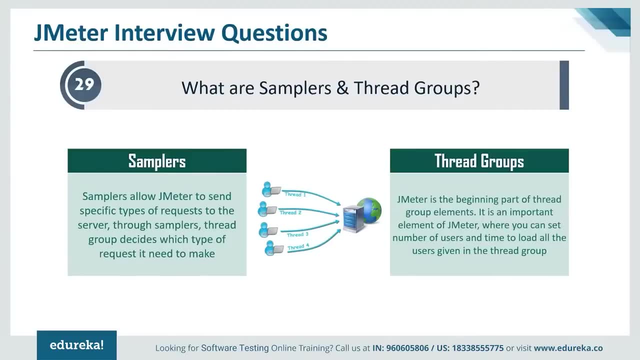 Now let's have a look at what are thread groups. So Jmeter is basically the beginning part of thread group elements. Now it is an important element of Jmeter where you can set number of users and time to load all the users given in the thread group. 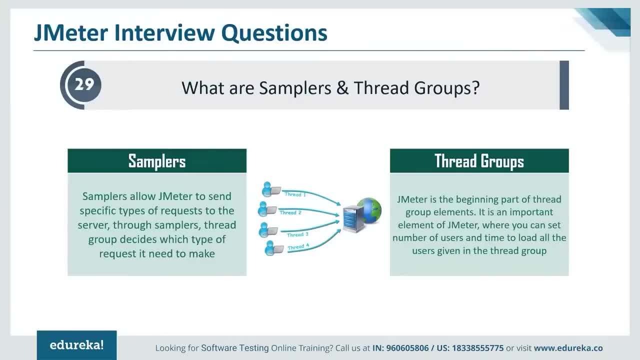 So, basically, using the samplers, We have our HTTP or HTTPS request that we want to send. So we have our HTTP request And, using the thread group, we specify the number of users that are present in the thread or the number of users that are performing the testing. 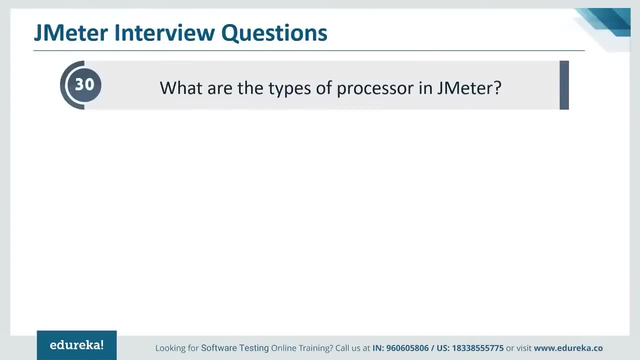 Now the next question is: what are the types of processor in Jmeter? Now, processor is basically used to modify the samplers in their scope. Now there are two types of processors in Jmeter. The first one is the pre processor and second one is the post processor. 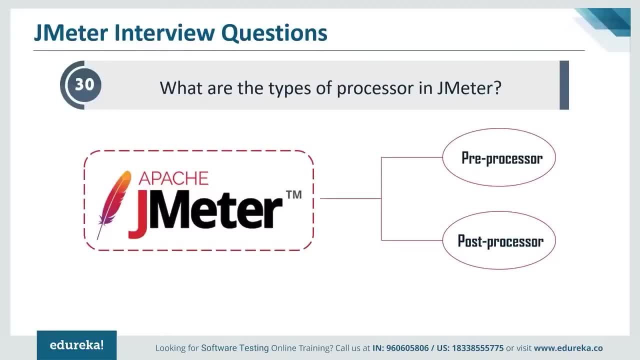 Now what is a pre processor? So the pre processor executes some action before making sampler request. So let's say you want a Jmeter to spider through the website under test parse link and return the HTML. So you would add some actions, such as the HTML link parser, to your controller. 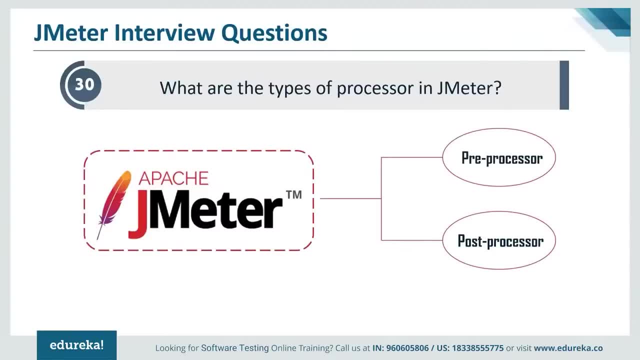 before creating an HTTP request. And what is a post processor? So the post processor executes some action after making a sampler request. So when Jmeter sends an HTTP request to the web server under test and get the response, you want Jmeter to stop the test. 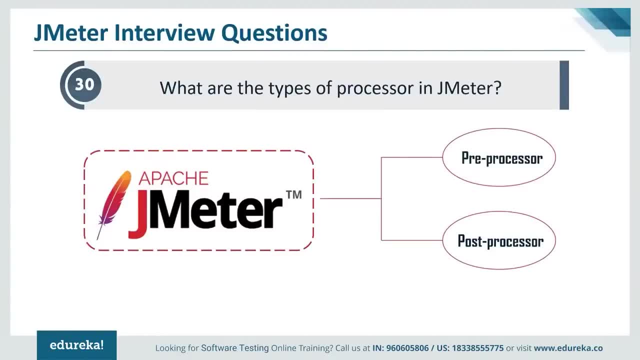 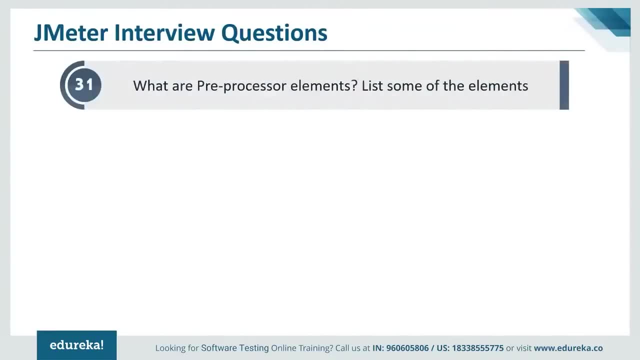 if the server response is an error Now you can use the post processor in order to do the task. Now moving on, the next question is: what are pre processor elements? List some of those elements. So a pre processor is something that will happen before the sampler executes. 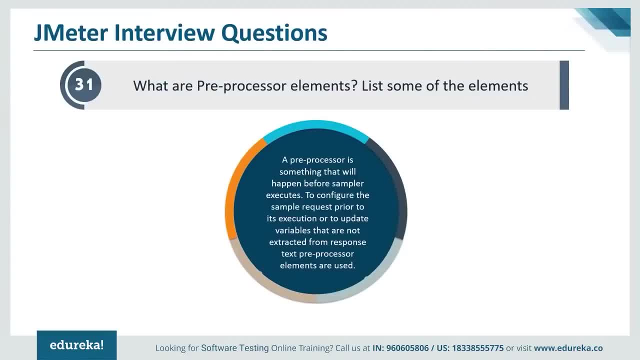 Now, in order to configure the sample request prior to its execution or to update variables that are not extracted from response text, pre processor elements are used Now. some of the elements include the HTTP URL rewriting modifier, the HTTP user parameter, the HTML link parser. 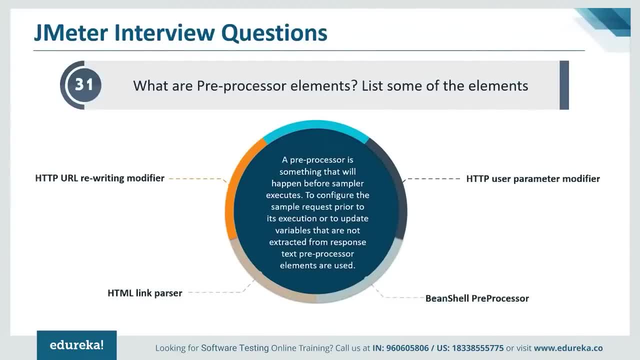 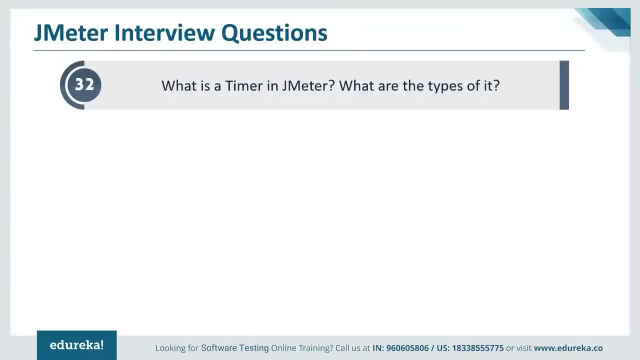 and also the bean shell pre processor. Moving on. the next question is: what is a timer in Jmeter? Also, what are the different types of it? Now, a Jmeter thread by default will send requests continuously without any pause. to get a pause between the request, timers are used. 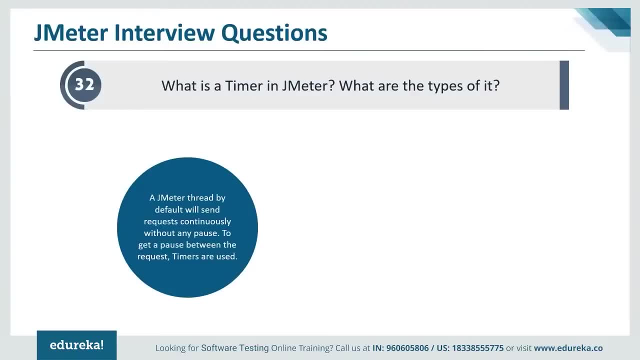 Now, if you perform load or stress testing on your server without any delay, it will be overloaded. Then it won't be able to give you realistic results and fail to simulate real-world user traffic experience. Now Jmeter timers are the solution to all these problems. 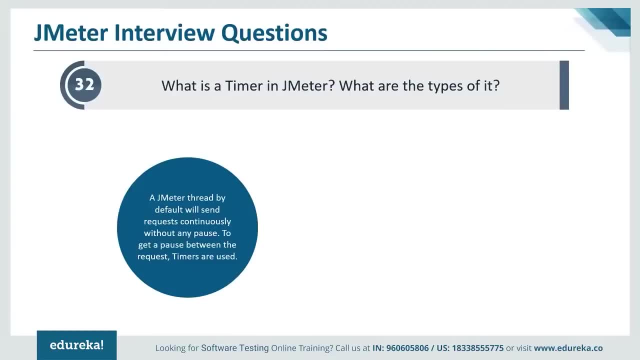 The timer element can be added in a test plan to apply weight between each sampler or request. Now let's have a look at some of the types of timer in Jmeter. So first we have the constant timer. Now the constant timer element delays each request. 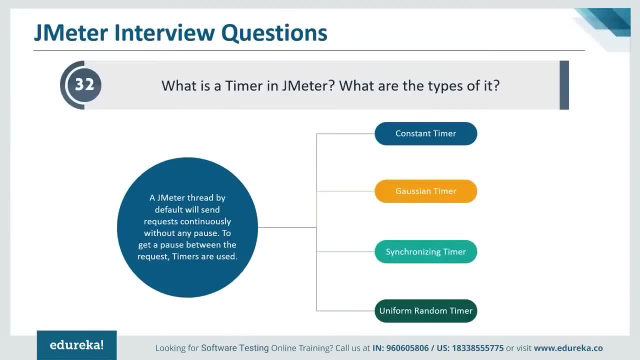 in a thread group for the same amount of time. Then we have the Gaussian random timer. Now the Gaussian random timer element is used to delay each user request for a random period of time. It has a random deviation around the constant delay offset based on Gaussian curve distribution. 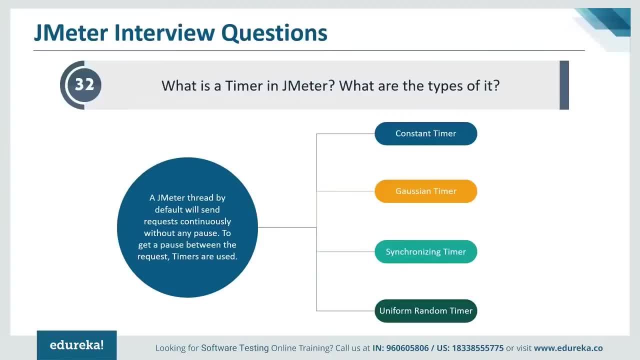 Then we have the synchronizing timer, which is used for synchronizing the wait period, And finally we have the uniform random timer. Now the uniform random timer element is used to delay each request for a random period of time. So your total amount of delay: 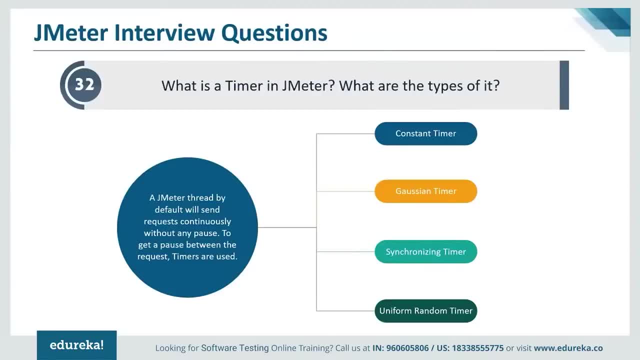 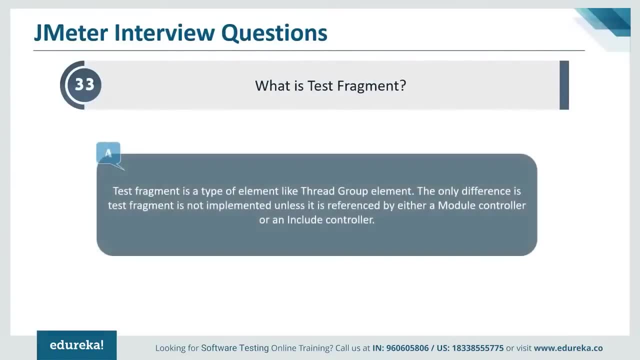 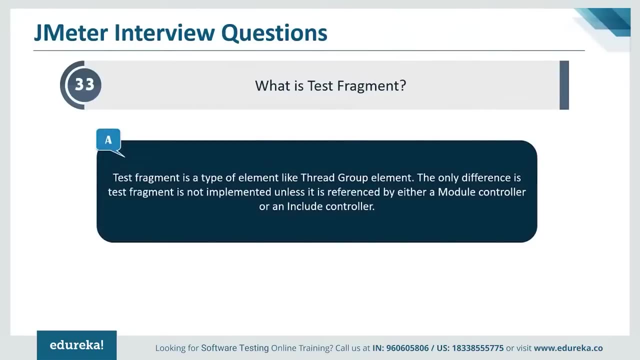 will be equal to random delay maximum plus your constant delay offset. The next question is: what is test fragment? Now? test fragment is basically a type of element like thread group element. Now, the only difference is test fragment is not implemented unless it is referenced by either a module controller. 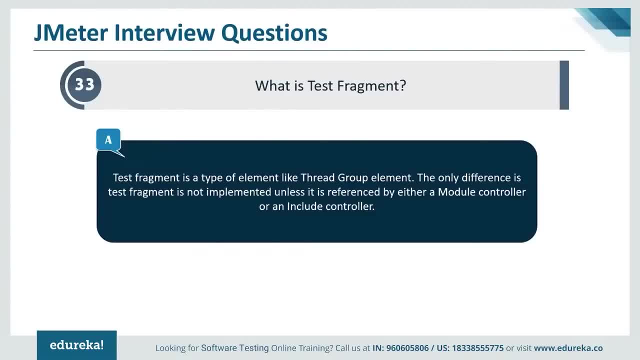 or an include controller. So basically it is an element that can be added directly under Jmeter test plan like the thread group, but it does nothing except holding other elements inside. It gets executed only when it is referenced by a module or include controller from other thread groups. 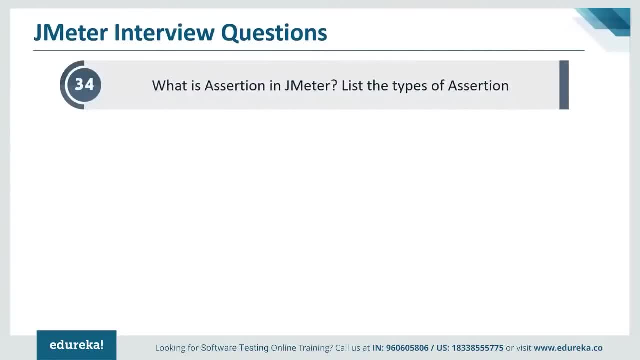 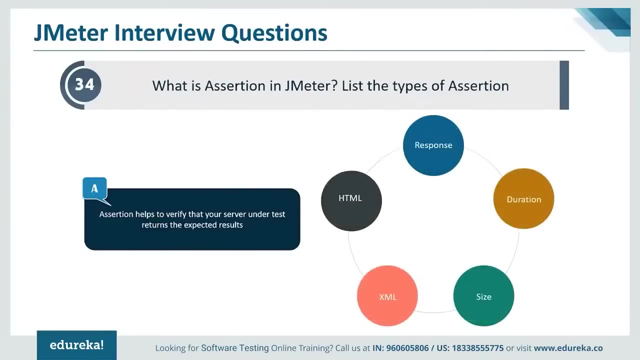 So the next question is: what is assertion in Jmeter and what are the different types of assertion? Now, assertion basically helps to verify that the server under test returns the expected results. Some commonly used assertion in Jmeter are the response: assertion duration, size. 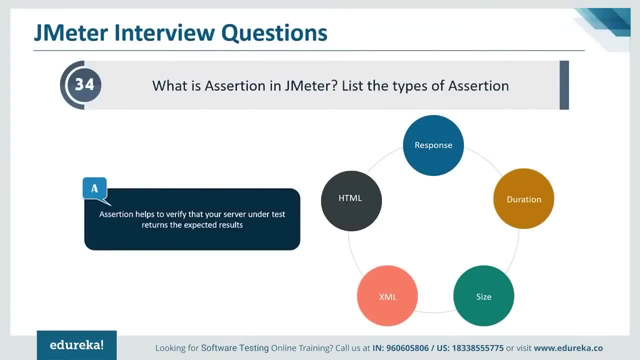 XML assertion and HTML assertion. So the response assertion facilitates the user by comparing the server response against a string pattern to check that the result is as expected, For example while waiting for a response from the server. the response assertion role is to verify that the server response has probable pattern, string or not. 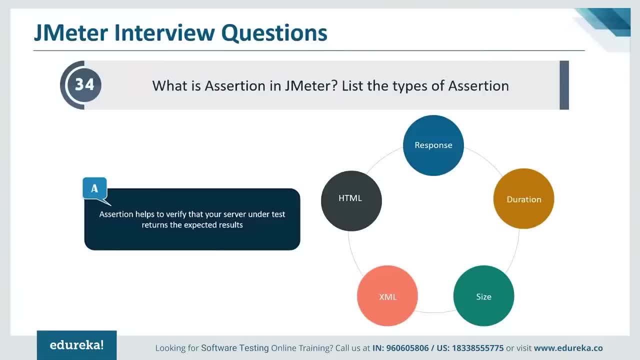 Now, in case of duration assertion, you may need to test the response from the server reaches in user defined time. If it takes longer than the defined time, server response fails, Then we have the size assertion. Now it is to test that each response coming from server. 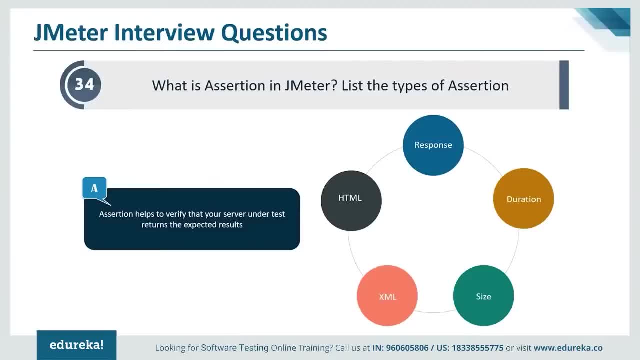 holds the expected number of bytes. It basically facilitates the user to specify the size that is equal to, greater than, less than or not equal to a given number of bytes. Now, for example, if the response packet from a server is less than expected- 5000 bytes in size, 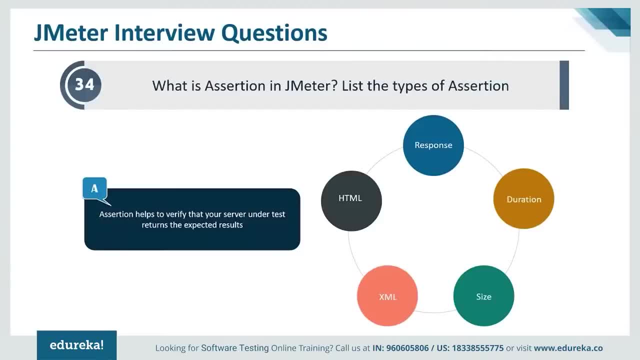 then a test case pass, else a test case will fail. Then we have the XML assertion which verifies that the response coming from the server holds the data in a correct XML format. and finally we have the HTML assertion. It is helpful for checking the syntax of the response data. 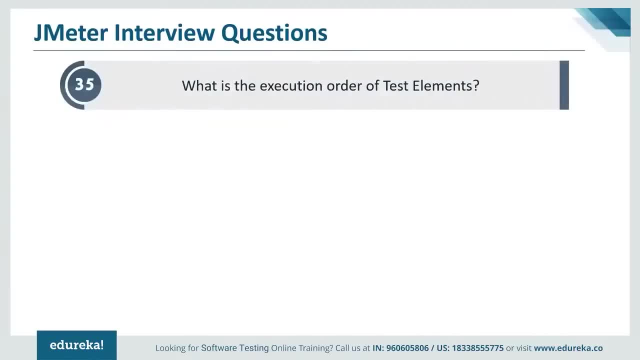 Now moving on. the next question is: what is the execution order of test elements? So first we have the configuration elements and then we have preprocessor, then timers, samplers, post processors, assertions and finally listeners. Now timers, assertions, pre and post processors. 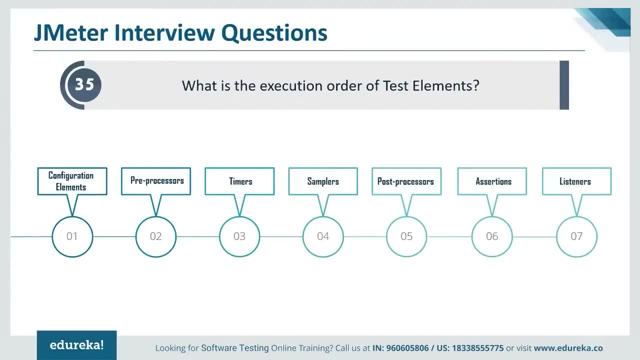 are only processed if there is a sampler to which they apply. The logic controllers and samplers are processed in the order in which they appear in the tree. Now other test elements are processed according to the scope in which they are found and the type of test element. 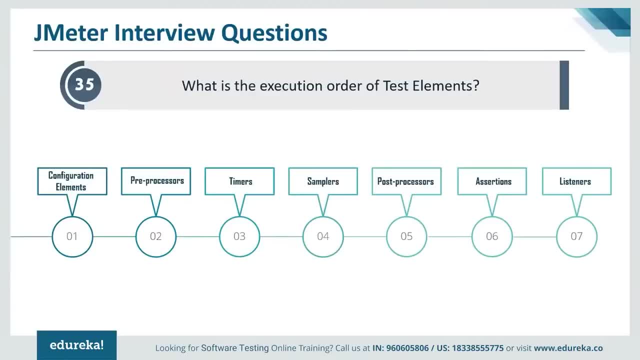 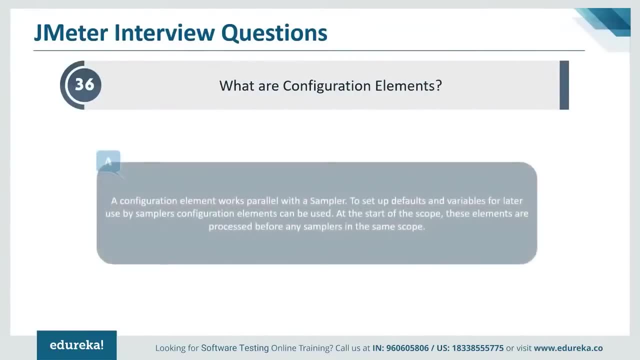 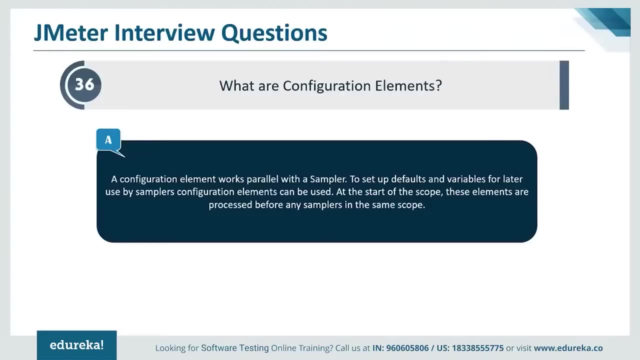 So this was the example of the configuration order for the test elements. Now moving on, the next question is: what are configuration elements? Now, a configuration element works parallel with a sampler to set up defaults and variables for later use by samplers. configuration elements can be used. 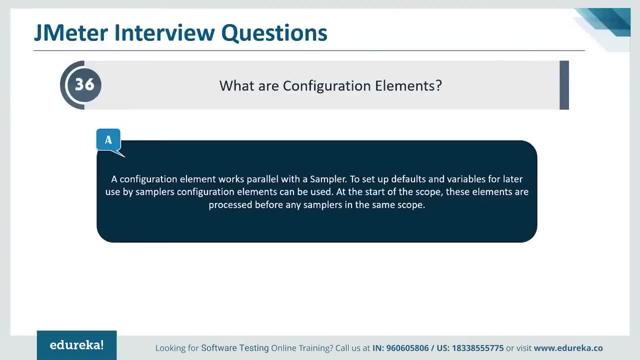 Now, at the start of the scope, these elements are processed before any samplers in the same scope. So the config elements in JMeter are used to configure or modify the sampler requests made to the server. These elements are added at the same or higher level of the samplers that we want to configure. 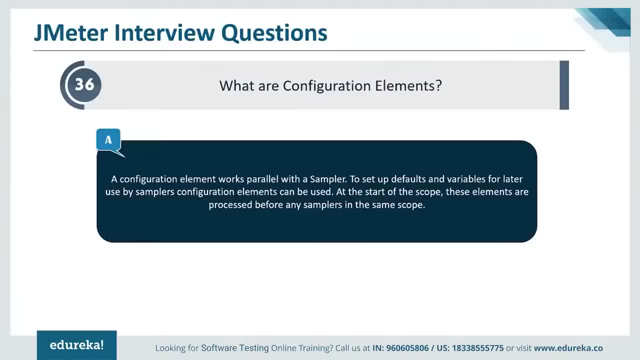 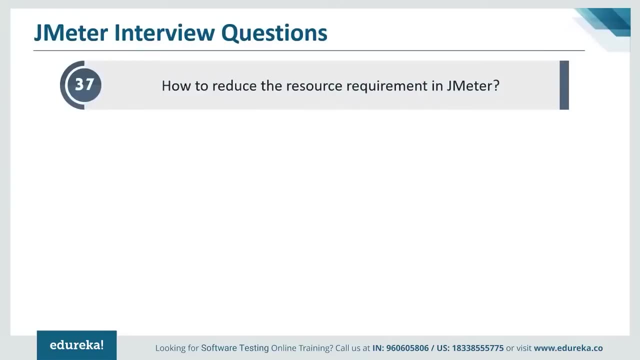 Some of the configuration elements in JMeter include the CSV data set config, the HTTP cache manager, HTTP cookie manager, user-defined variables, random variable and quite a few more. Now moving on. the next question is how to reduce the resource requirement in JMeter. 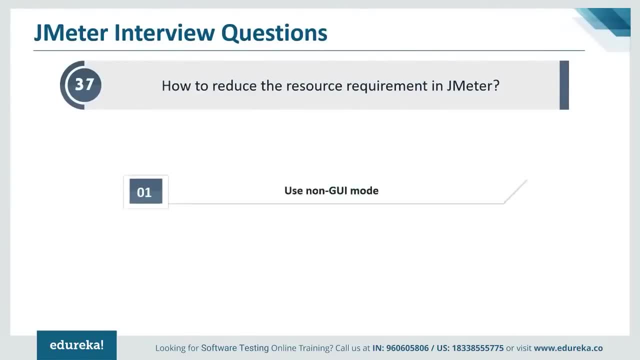 Now to reduce the resource requirements in JMeter we should use the non GUI mode. so for that we have the command as JMeter, hyphen n, hyphen T and then the location of the test script, then hyphen L and the location of a test results. 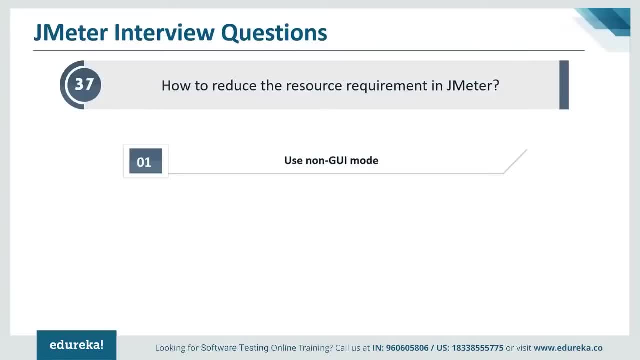 You can also check out the load test using JMeter tutorial in order to understand how to perform load testing in JMeter in the non GUI mode Next up during the load test. doesn't use the view results tree or view results in table listeners. It uses them only during the scripting phase. 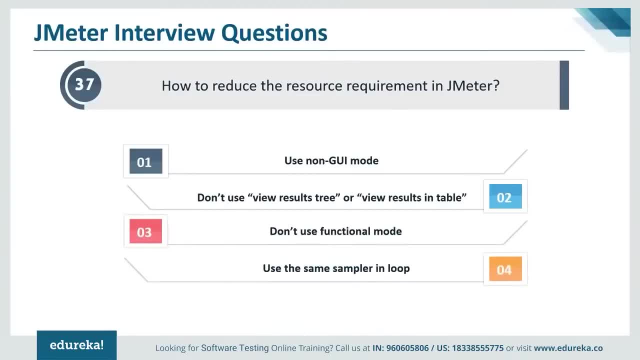 Also, we should not be using the functional mode. and finally, instead of using lots of similar samplers, we must use the same sampler in loop and use variable to vary the sample. So if we follow these steps, it will help us in reducing the resource requirement in JMeter. 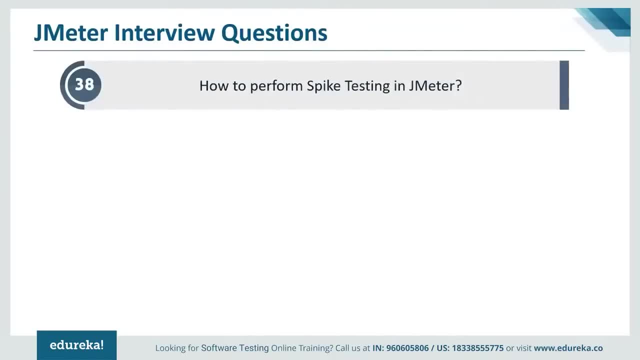 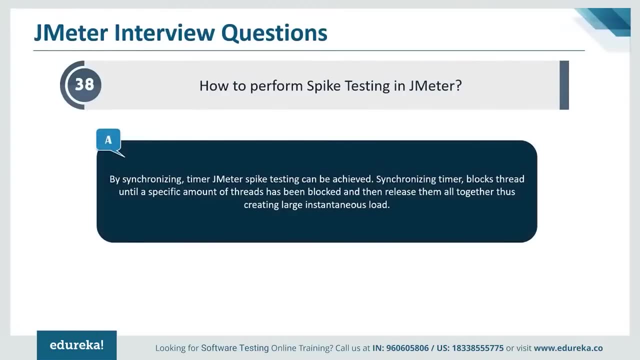 Now moving on how to perform spike testing in JMeter. Now, by synchronizing timer JMeter spike testing can be achieved. So synchronizing timer blocks the thread until a specific amount of threads has been blocked and then release them all together, Thus creating large instantaneous load. 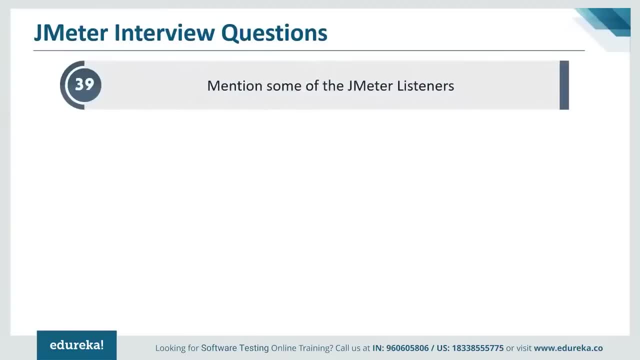 Now moving on. the next question is mentioned. some of the JMeter listeners Now listeners are the JMeter component that displays the test results. but there is more to them than just that. The variety of JMeter listeners enables performance engineers to monitor the request sent from JMeter. 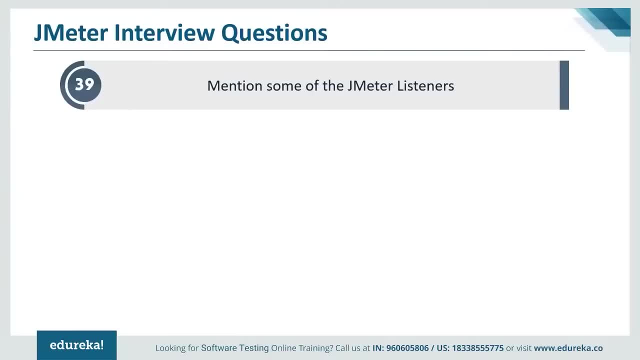 as well as to analyze the responses received from the system under test. So some of the JMeter listeners include the spline visualizer, the aggregate report, the view result tree, view results in table monitor, results distribution graph, bean shell listener and the summary report. 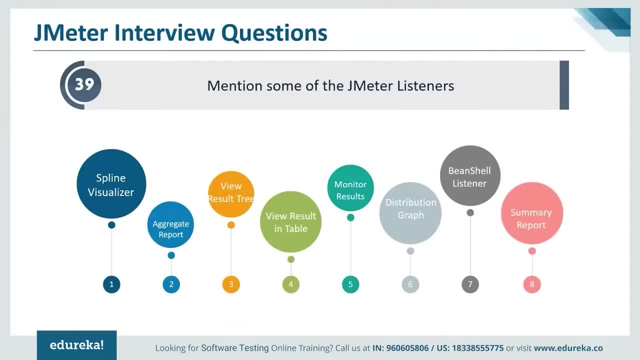 Now for each sample. the HTTP sampler produces the view results tree listener provides the request parameters, response parameters and the response data, and also one of the most useful elements of the view results tree listener is a tab that renders information transmitted in the sample body into the required format. 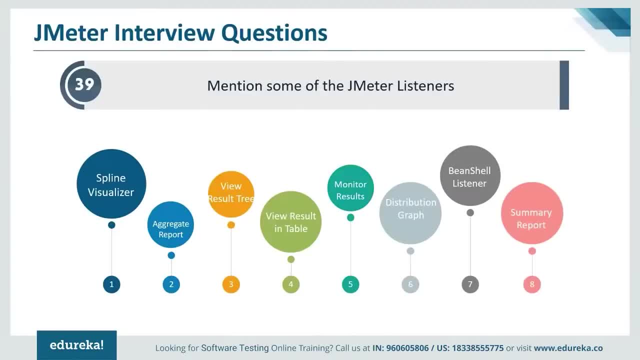 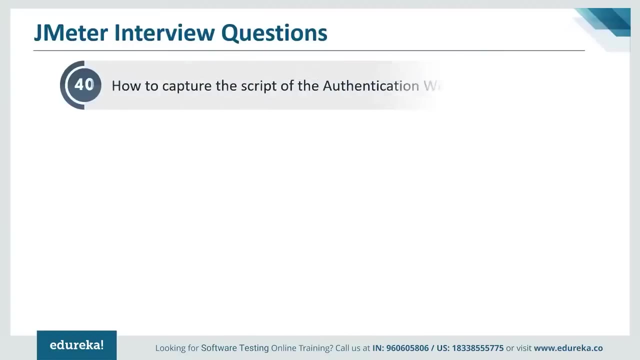 Also, the view result in table listener displays information about each sample in the form of a table. So the table shows time-related data for each sample: The payload data, the thread number and the sample execution results. Next question is how to capture the script. 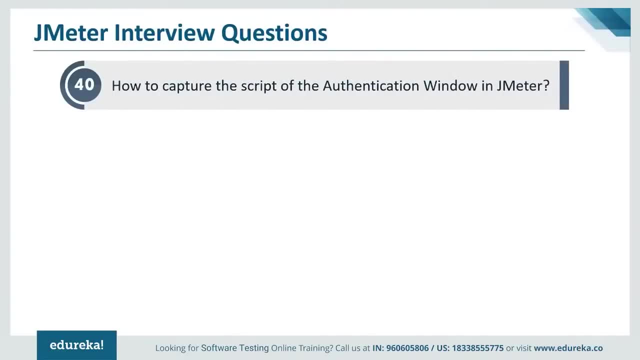 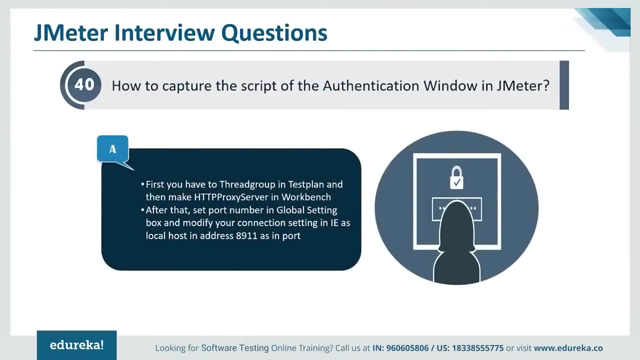 of the authentication window in JMeter. So normally you can capture the script by recording. So for that first you have to thread group in test plan and then make HTTP proxy server in workbench and after that you have to set the port number in global setting box. 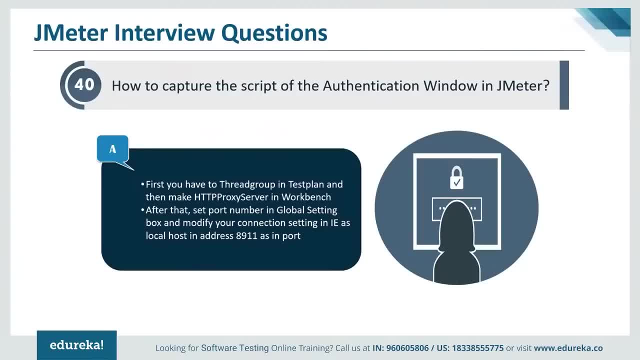 and modify your connection, setting in IE as localhost, in address 8911 as import. Then you can start your HTTP proxy server in JMeter and run your application for login. While you follow these steps, it will help you capture the script of your authentication window in JMeter itself. 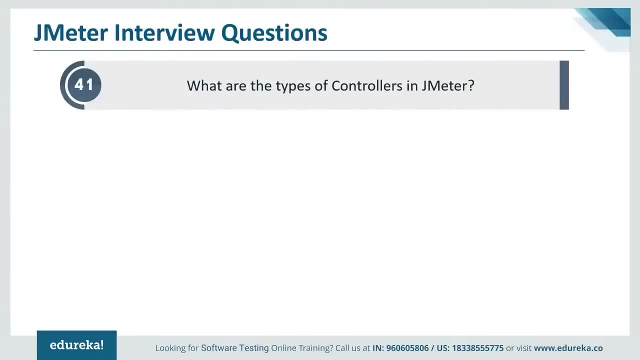 Moving on. the next question is: what are the types of controllers in JMeters? Now, normally we construct test plan which consists of small units of functionality like login at product or logout. Now the functionality can be stored inside controllers as modules. Now there are two main types of controllers in JMeter. 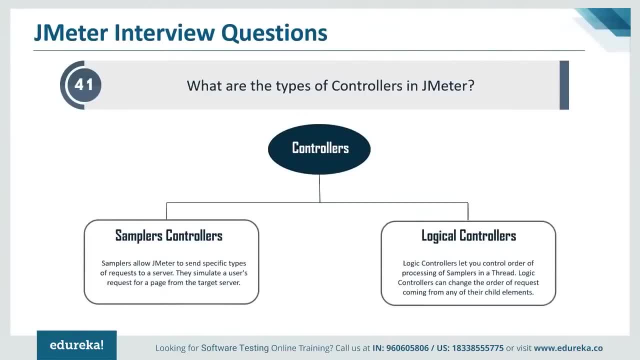 That is, the samplers controllers and the logical controllers. Now, samplers allow JMeter to send specific types of requests to a server. They basically simulate a user's request for a page from the target server. For example, you can add an HTTP request: 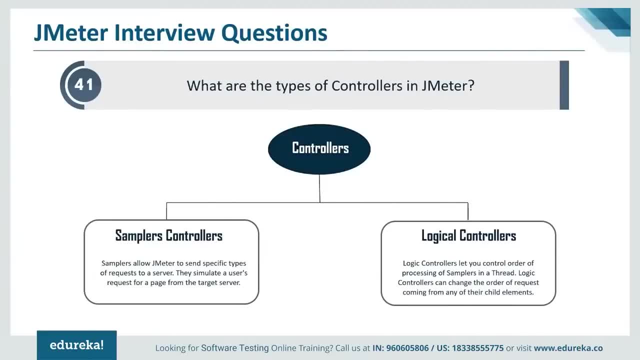 to your sampler. if you need to perform a post, get delete on a HTTP service. Next up is the logical controllers. So the logic controllers. let you control order of processing of samplers in a thread. So the logic controllers can change the order of requests coming from any of their child elements. 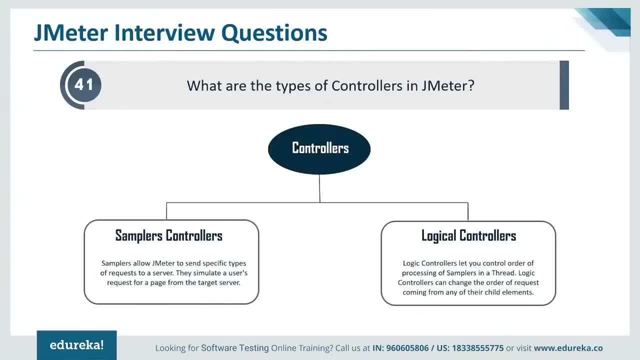 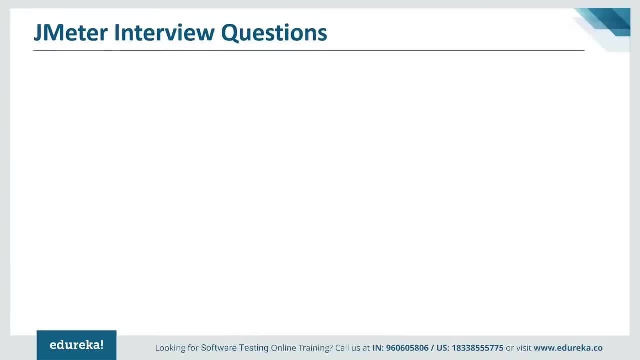 Some examples are the for each controller while controller, loop controller, if controller the runtime, interleave controller, throughput and run once controller. So these were two main types of controllers in JMeter. Now, moving on, the next question is: what are preprocessor and post processor elements? 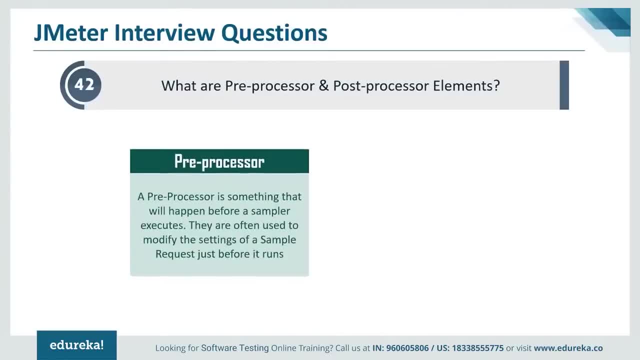 So what are preprocessor elements? So a preprocessor is something that will happen before a sampler executes, So they are often used to modify the settings of a sample request just before it runs. And next up, we have the post processor elements. So a post processor executes. 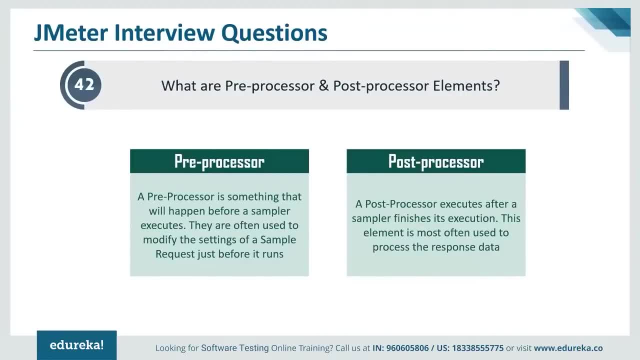 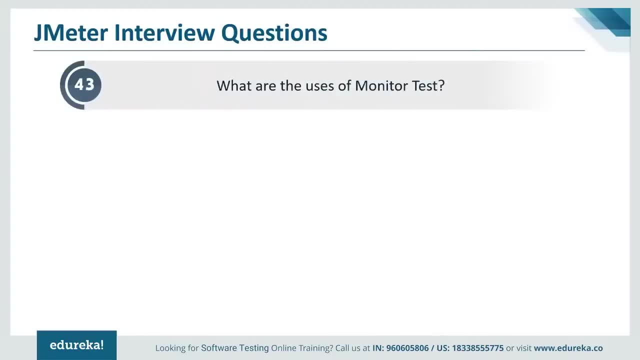 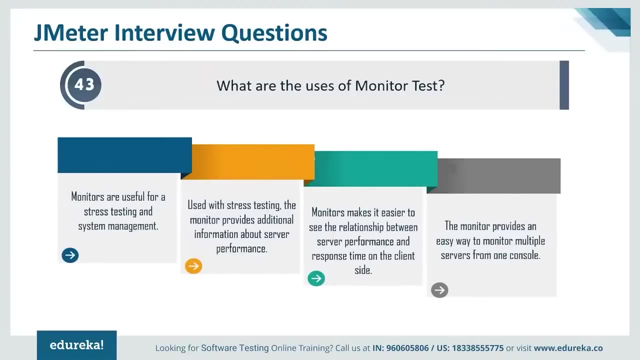 after a sampler finishes its execution. This element is most often used to process the response data. Now moving on, the next question is: what are the different uses of monitor test? Now, monitors are useful for a stress testing and system management. It is also used with stress testing. 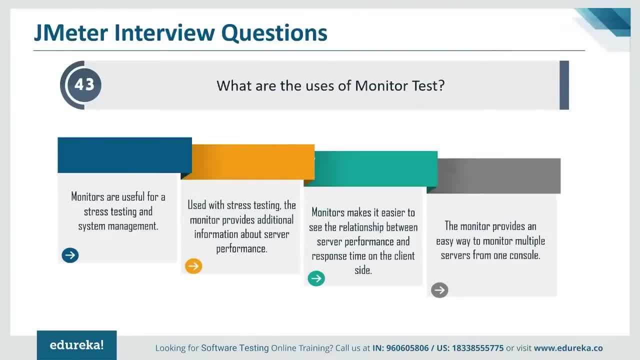 The monitor provides additional information about the server performance. Monitors also make it easier to see the relationship between server performance and response time on the client side. And finally, as an administration tool, the monitor provides an easy way to monitor multiple servers from one console. 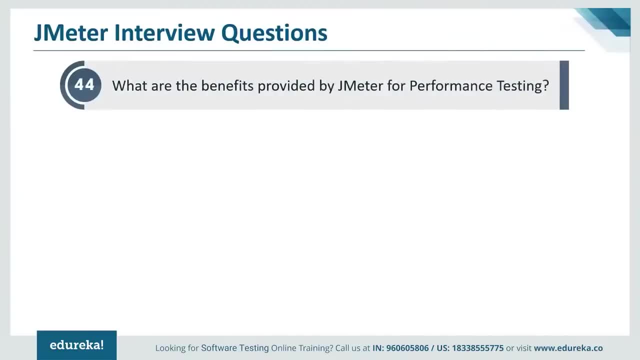 Now next question is: what are the benefits provided by JMeter for performance testing? Now, JMeter is one of the most preferred tools when it comes for performance testing, So let's have a look. what are the benefits that it provides, which makes it one of the most preferred tools? 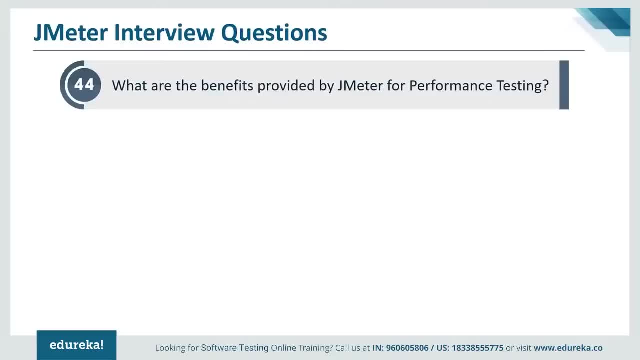 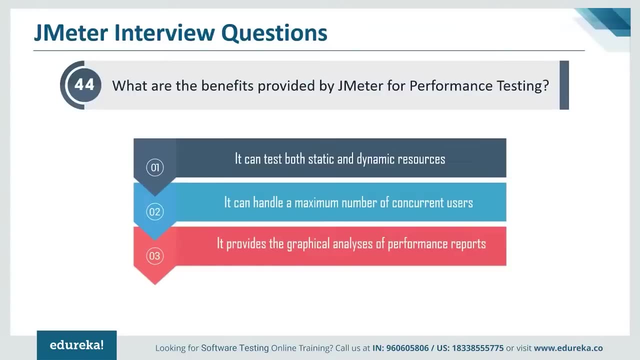 So some of the benefits on performance testing that JMeter offers are that it can be used to test performance for both static resources as well as dynamic resources. Not just that, it can also handle a maximum number of concurrent users then your websites can handle. and finally, it provides the graphical analysis. 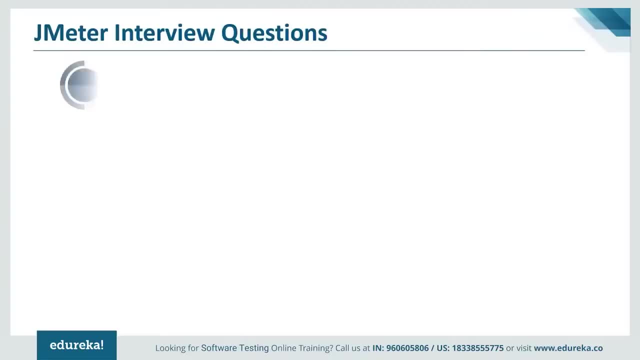 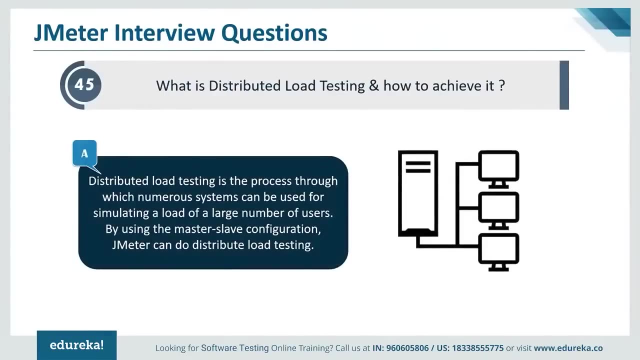 of performance reports. The next question is: what is distributed load testing and how to achieve it? Now, basically, distributed load testing is a process through which numerous systems can be used for simulating a load of a large number of users. Now by using the master slave configuration JMeter. 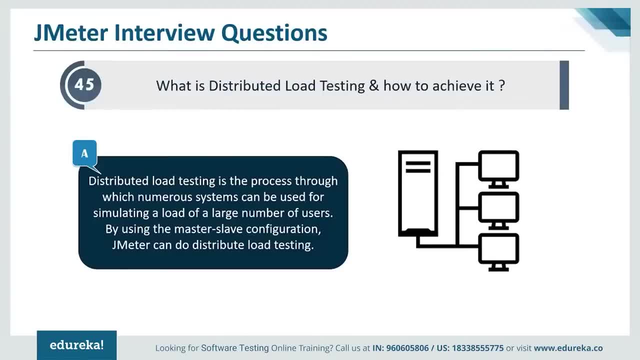 can do the distributed load testing. Now, as a single system cannot generate large number of threads, multiple systems are used for this testing. So, in this case, the system running JMeter GUI control each slave and the web server under test gets a request from these slaves. 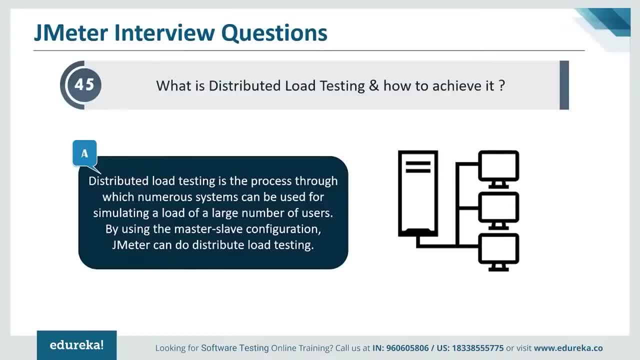 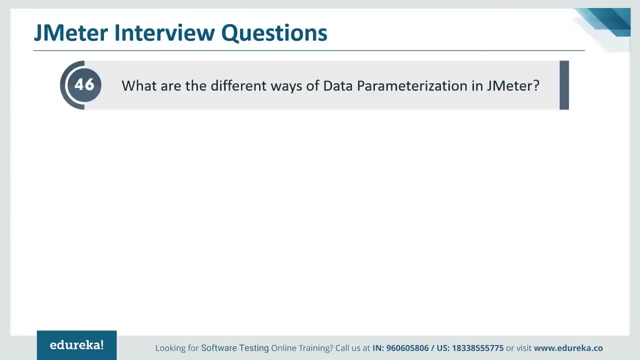 Whereas the system running JMeter server receives a command from the master, and this is how the master slave configuration works and helps the JMeter in performing the distributed load testing. Now, what are the different ways of data parameterization in JMeter? Now, instead of putting the hard-coded value, 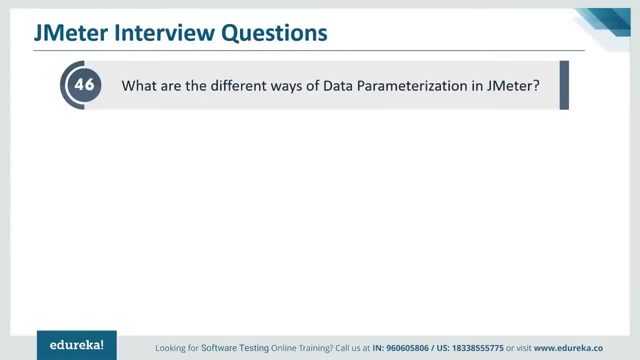 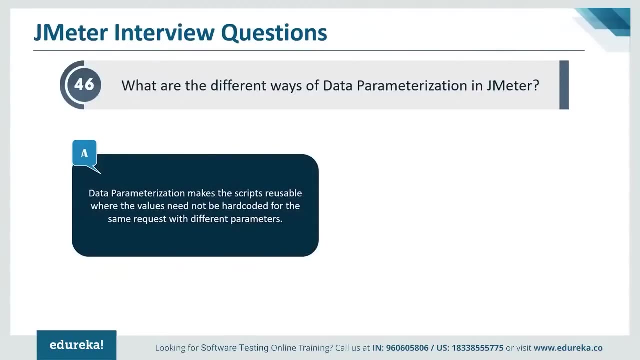 as input parameters for a functional or API testing. you might have thought about how we can use a file table, database objects for better test coverage. parameterization is the answer to it. So data parameterization makes the scripts reusable where the values need not be hard-coded. 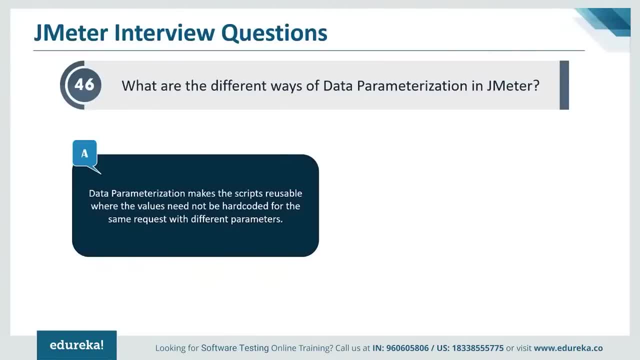 for the same request with different parameters. Now the different ways are the CSV data set configuration at the user-defined variables. Now we can easily parameterize that request by using an external CSV file and running the script across different users, and another method is by using the user-defined variables. 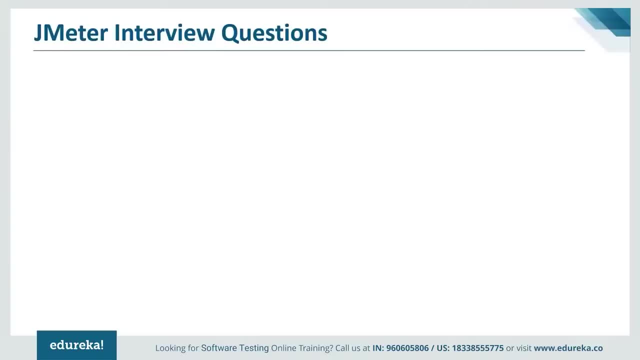 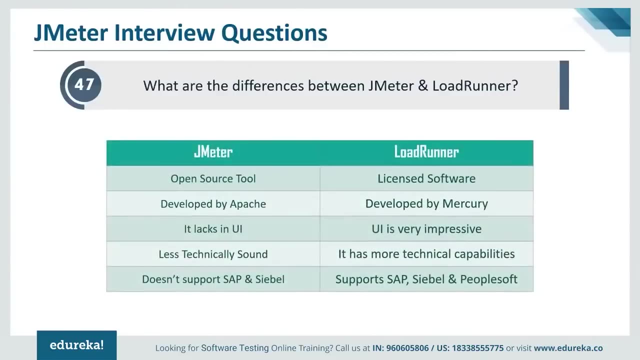 in case of data parameterization. Now moving on, the next question is: what are the differences between JMeter and load runner? So JMeter is basically an open source tool, whereas load runner is a licensed software. JMeter was also developed by Apache and load runner was developed by Mercury. 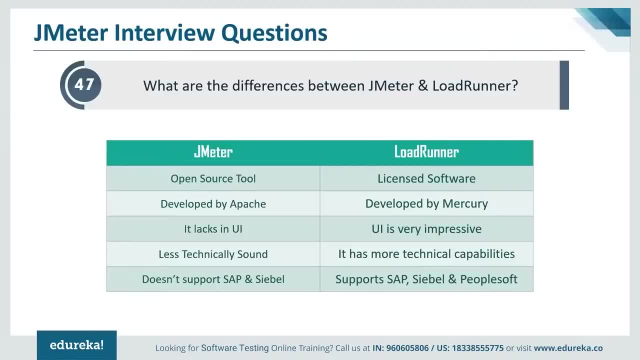 One problem in JMeter is that it lacks in the user interface, But in case of load runner, it has a very impressive user interface. JMeter is also considered to be less technically sound when compared to load runner, because load runner has more technical capabilities. 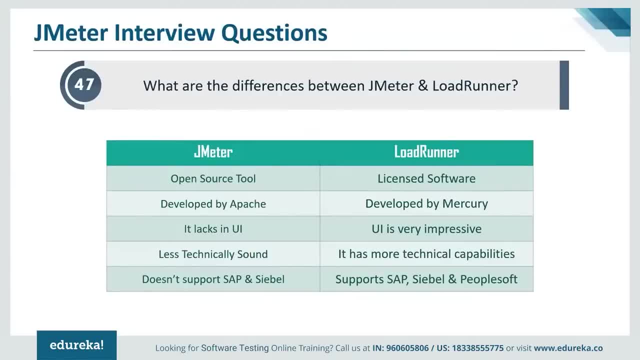 Also, JMeter doesn't support the SAP and Siebel, whereas load runner supports SAP, Siebel and also PeopleSoft. But because JMeter is an open source tool and readily available, it is still considered to be one of the most preferred tools when it comes to performance testing. 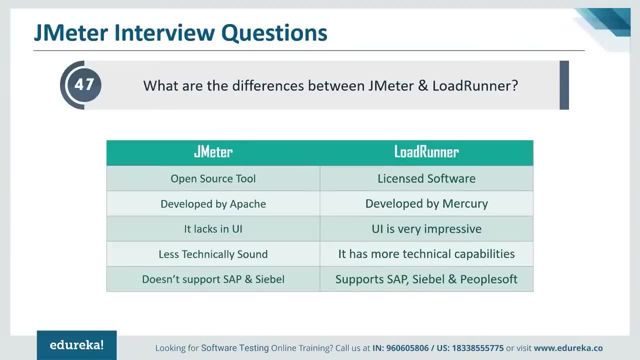 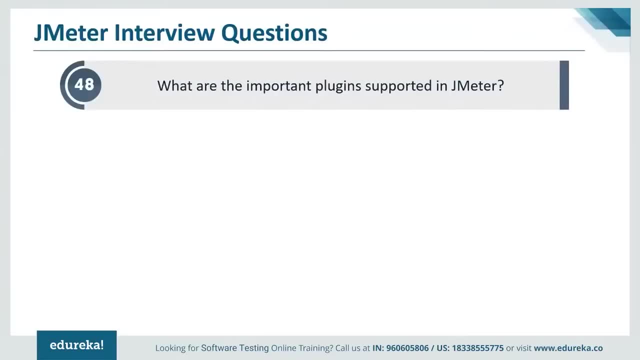 So these were some of the differences between JMeter and load runner. Now moving on. the next question is: what are the important plugins supported in JMeter? Now, JMeter supports different types of plugins which are helpful in generating high quality results. Some of the major plugins that are supported by JMeter: 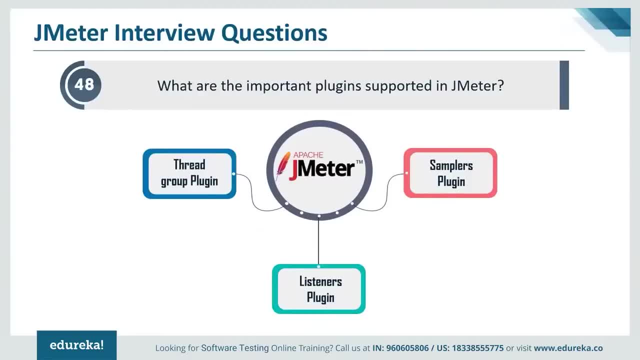 include the thread group plugin, the stepping thread group plugin, and next up is the samplers plugins like the WebDriver, and finally, we also have the listeners plugin. So these are some of the most important plugins that are required and also supported in JMeter. Now, moving on, the next question is mentioned. 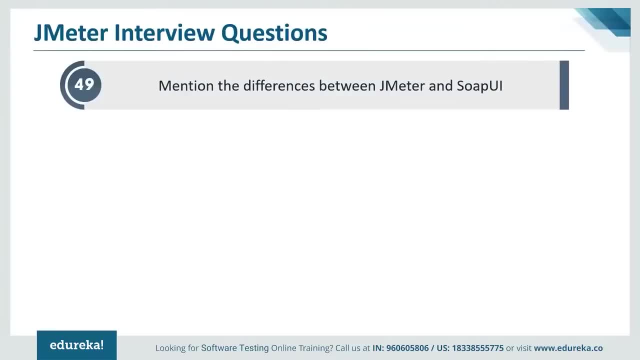 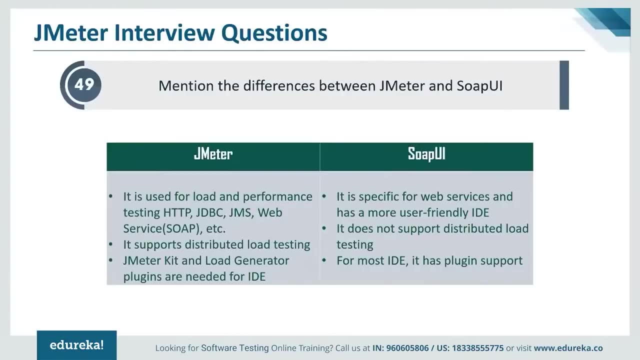 the differences between JMeter and SOAP UI. So JMeter is basically used for load and performance testing- HTTP, JDBC, JMS, web service and etc. Whereas the SOAP UI is specific for web services and has a more user-friendly IDE. JMeter also supports the distributed load testing. 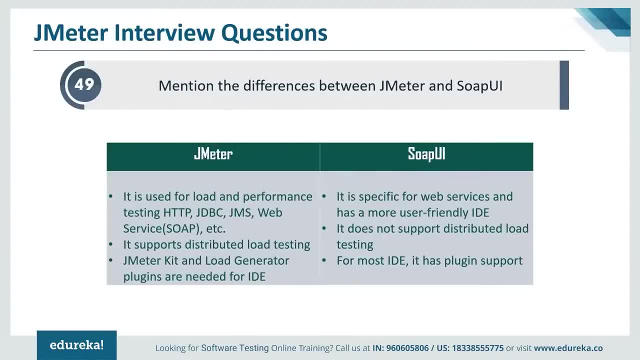 but SOAP UI does not support the distributed load testing, The JMeter kit and the load generator. plugins are needed for IDE, Whereas in case of SOAP UI, for most IDE it has the plugin support. So now let's move on to the final question of this section. 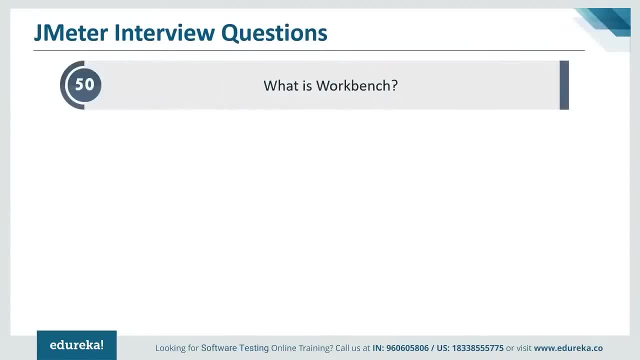 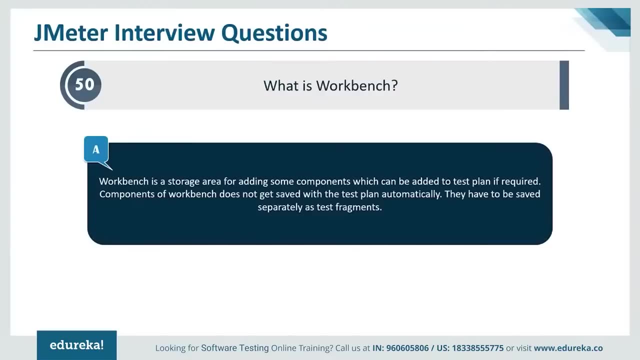 So the final question is: what is workbench Now? workbench is basically a storage area for adding some components which can be added to test plan if required. Components of workbench does not get saved with the test plan automatically. They have to be saved separately as test fragments. 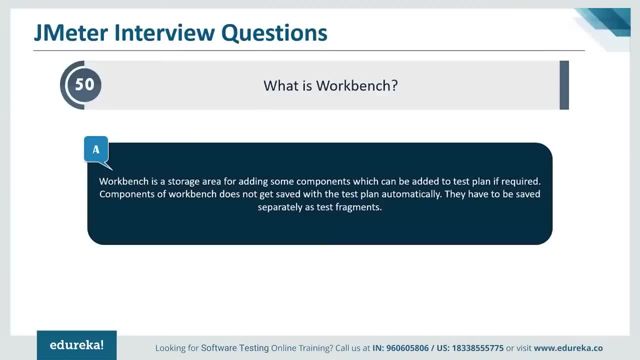 So these were the components where some of the most commonly asked questions on performance testing and JMeter. These interview questions will help you in clearing your interviews about testing. You can also go check out our software testing interview questions if you are preparing for any interview for a role in testing.